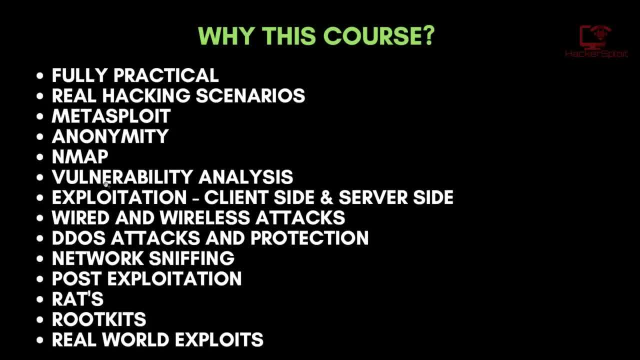 Stuff like that will then be taking a look at industry standard frameworks like Metasploit- how to use Metasploit for a for the full penetration testing experience will be then focusing on anonymity, And just not simple anonymity- will be looking at proxy chains. 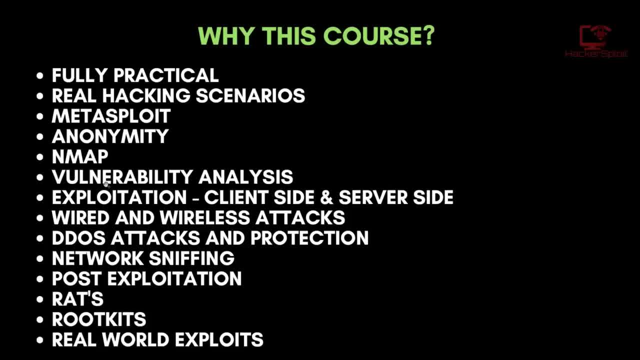 how to set up a VPN- how to set up a VPN in in regards to using proxy chains as well- will be then moving on to information gathering techniques. more specifically, the Nmap tool will be looking at how to use Nmap for advanced information gathering as well as basic information gathering. We'll then be moving on to vulnerability. 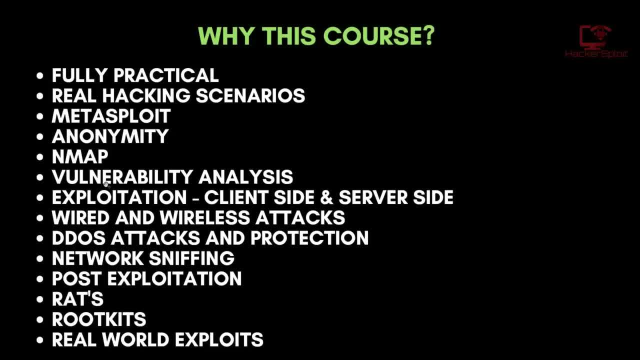 analysis, how to perform vulnerability analysis on web servers, etc. etc. We'll then be moving on to exploitation. Now, why is exploitation so important to me? Well, that's because I deal with exploitation. Hackersploit is a company that deals with penetration, testing and web. 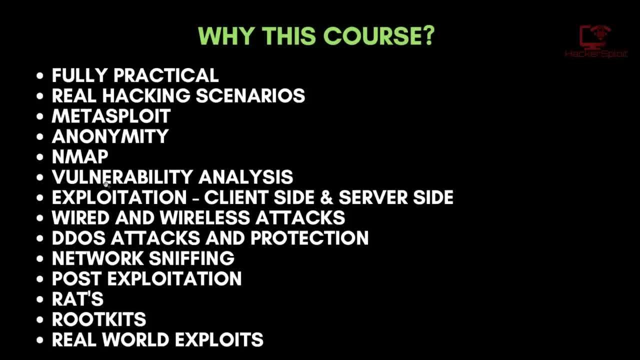 application penetration testing. So I know the both of the sides of it in terms of client side attacks and server side attacks. we'll be looking at all the frameworks. we'll be looking at Hydra, we'll be looking at the at the BEF framework as well. We'll then move on to something. 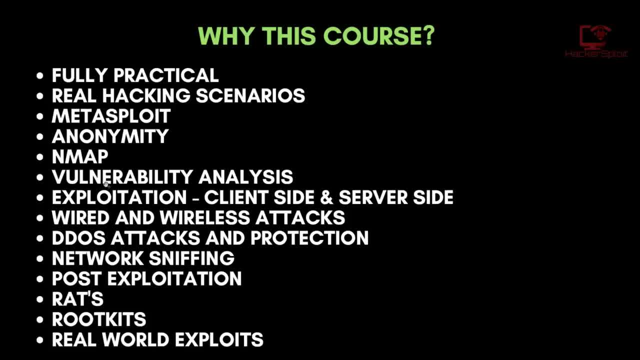 that is quite popular as well, And that is wired and wireless attacks, how to perform ARP spoofing, how to perform ARP poisoning And, finally, how to crack the WPA and the WPA2 encryption with different methods and methods that do work, using aircrack and airgeddon to perform the pixie dust. 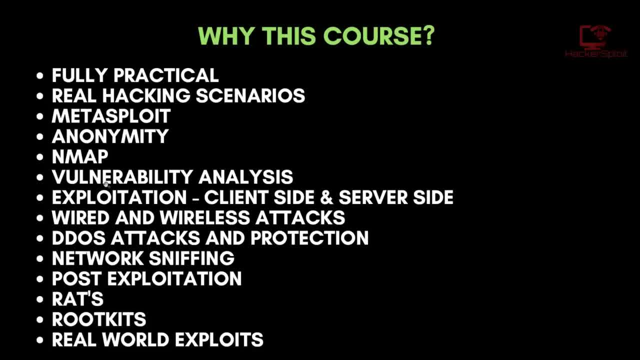 attacks. We'll be then looking at something that not only is it a very popular method, but it's also a very popular method to perform. not a lot of courses cover which are DDoS attacks, how to perform them and how to protect. 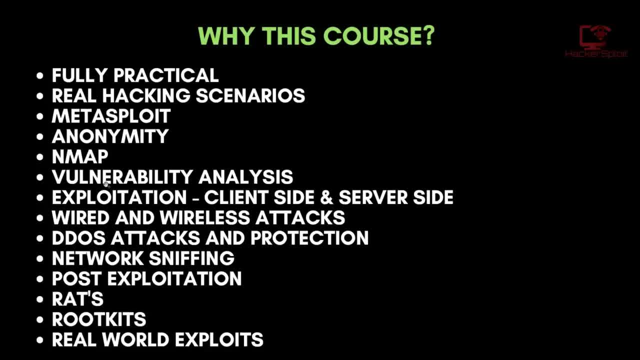 yourself against them. We'll be then moving on to network sniffing- how to use wireshark to capture packets on a network And, finally, looking at the last stage of ethical hacking, and my favorite, which is post exploitation. we'll be looking at creating backdoors, how to clear. 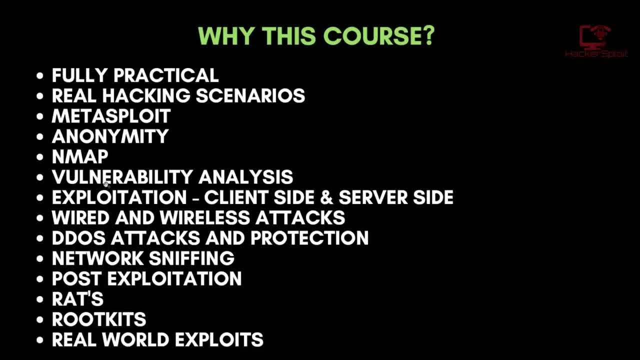 your tracks. we'll be looking at privilege escalation and how to maintain access within a system. We'll be then moving on to again one of my favorite, which is remote access tools. And if you do not know what a remote access tool, do not worry, we'll be covering what exactly it is in. 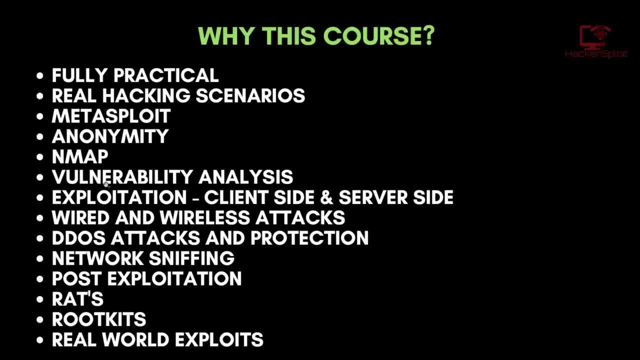 that section of the course. we'll be then looking at how to get rid of rootkits from Linux operating systems and Windows operating systems And finally, as I've mentioned, we'll be looking at real world exploits. we'll be focusing on real vulnerabilities, for example, the crack attacks. 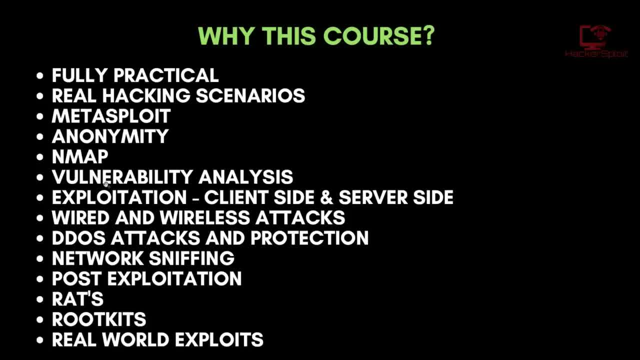 that allowed the WPA2 encryption to be broken. well, not broken, but exploited. we'll be then looking at the eternal blue exploits, and so much more. So what can I promise you With this course? Well, first of all, as I said, I'm going to be giving you a fully practical 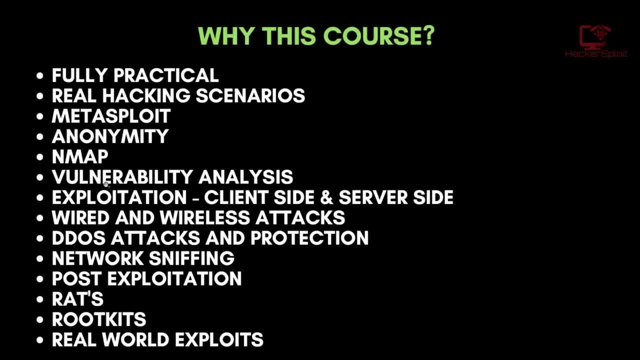 course And, secondly, this course is not about sales. I'm not going to be pushing you to buy this course. this course is going to be distributed free of charge one week for one week every month, And if you choose to buy this course, you're supporting us and the work that we do. this. 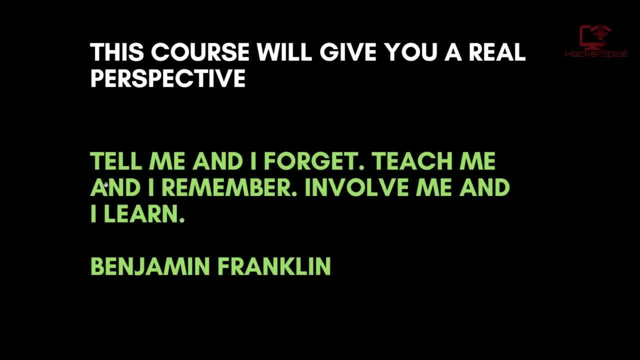 course is not going to be focused on sales, And if you do happen to buy the course and you're not satisfied with it, you can get a refund within 30 days. And if you do happen to buy the course, you can get a refund within 30 days as of you, as of when Udemy allows this to happen, If you purchase. 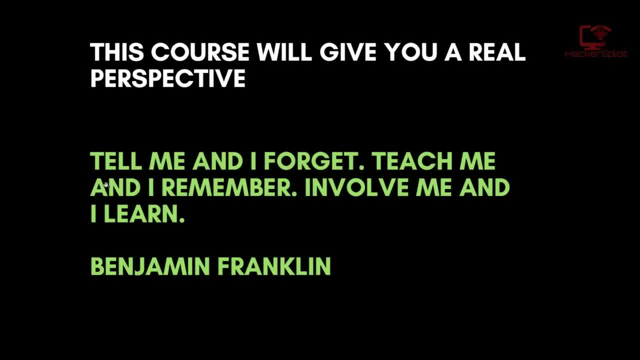 the course and you want to refund within 30 days. I'm pretty sure you know the terms that exist And I just want to end this introduction, or welcome to the course by, you know, quoting one of my favorite quotes by Benjamin Franklin, and that is: tell me, and I forget, teach me and I. 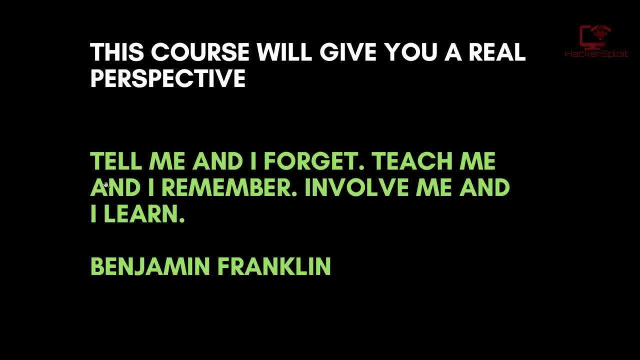 remember, involve me and I learn, And that's exactly what I want to do in this course. I want to involve you in hacking. I want to show you how it's really helpful, And I'm going to be talking to you in the next video. And if you do choose to take the course, welcome, and I'll be seeing you. 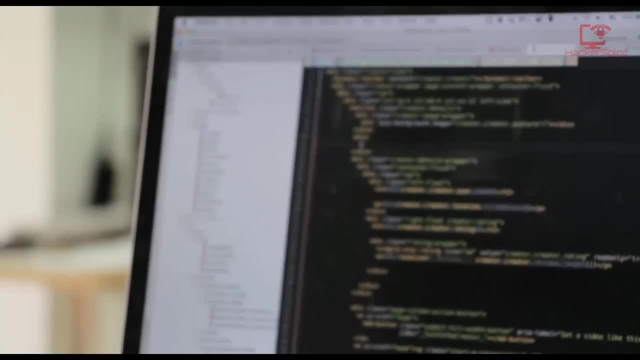 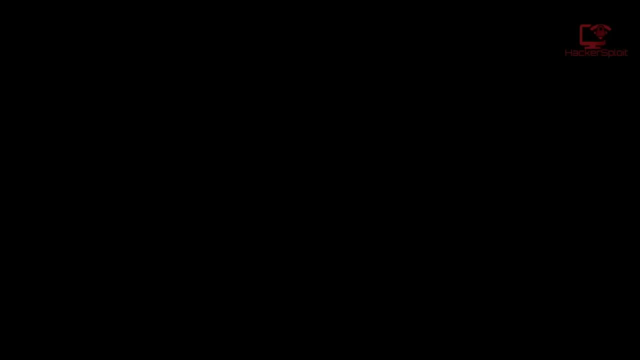 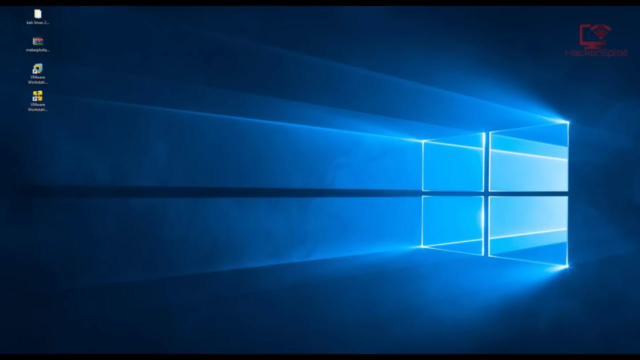 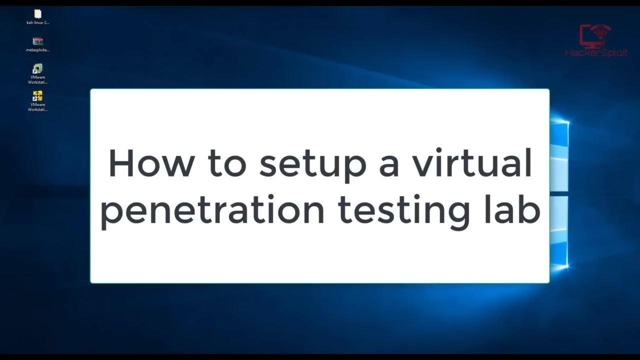 in the first video. Goodbye, Guys, Hack, Exploit here back again with another video, and welcome to the complete guide on how to set up your own virtual penetration testing lab where you can practice all your skills, and where you can practice all your skills and obviously improve as you move along. Now I just want to 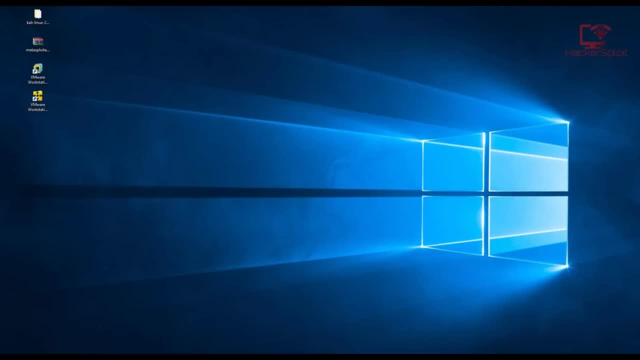 pass out a quick announcement that, regarding the SS7 exploitation video, I'm currently working with YouTube to get it accepted. Of course, I'm not going to be able to monetize it, but I'm still forcing it or trying to make sure that it gets published on YouTube. If that's not the case, I will have to host it on my 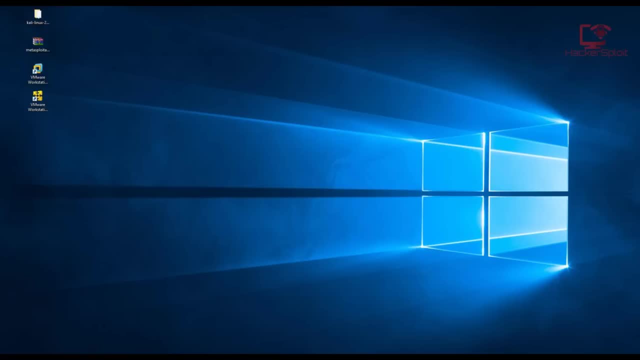 website, So then you can check it out over there. Reason being is that YouTube does not allow any demonstration of exploitation of a system that you do not own, And in the video I explain and show you how to exploit a GSM network And that type of thing. That being said, welcome to this video In. 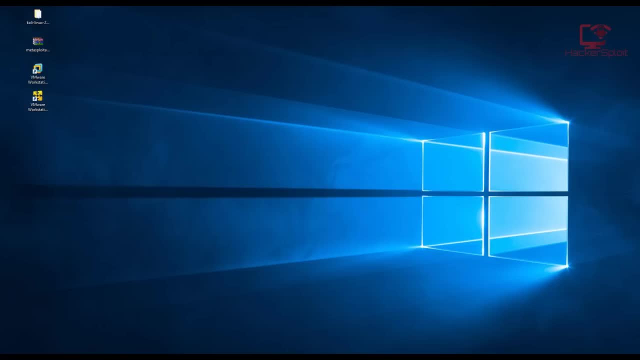 this video, I'm going to be showing you how to set up your own virtual penetration testing lab, So you can practice all your skills Now. before we get started, I just want to point out that if you're installing Kali Linux or Pareto s whatever penetration testing distribution that you decide, if you're installing it on a physical 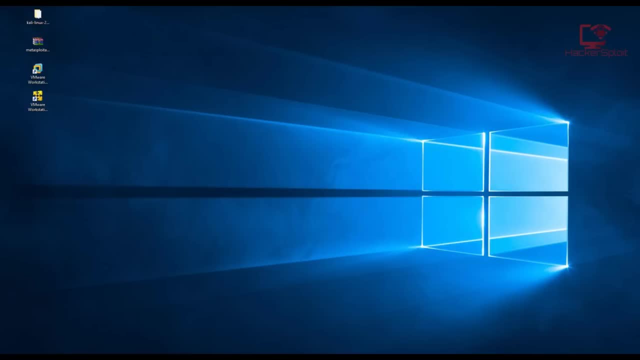 machine, then it will still be the same for you, as long as you have enough computers to run meta exploitable as a server, Or if you, if you then tend to go into virtualization, which is my recommended option, especially nowadays because computers are much faster and they're able to handle virtualization. 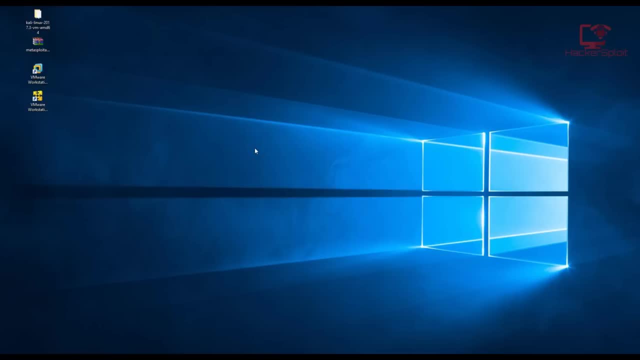 much, much better. All right, so let's get started, And what we're going to be doing is I'm going to be taking you through the different virtualization softwares. we're then going to move on to to actually selecting your penetration, testing, distribution, And then I'll show you how to get your 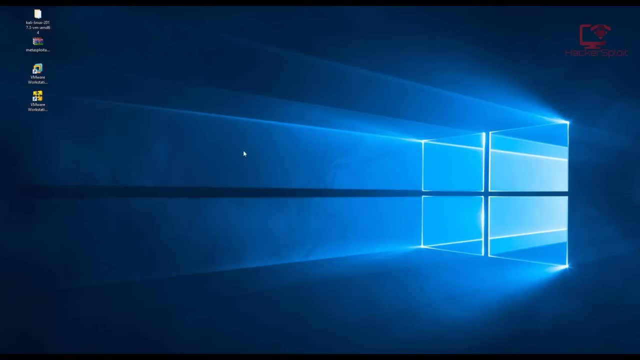 exploitable, or your, your, your vulnerable operating system or vulnerable server, which, in this case, is meta exploitable to All right, let's get started. So, as I said, the first thing that you want to make sure you have ready- or you want to make sure that you have hardware wise- is you have enough. 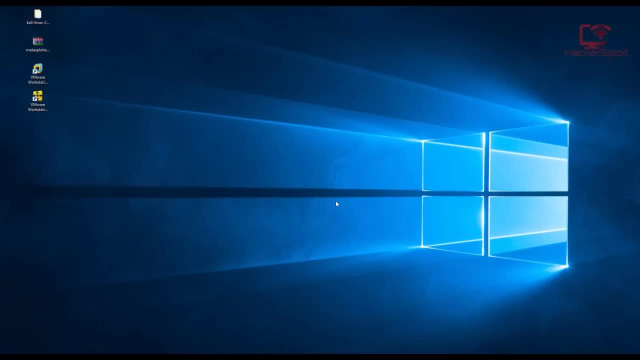 system resources. Now I'm just going to go ahead and say: the most important thing you need is virtualization. If your processor does not support virtualization, that means that you cannot or you are unable to use a virtualizing or a virtualization software. Okay, now, this is not very. 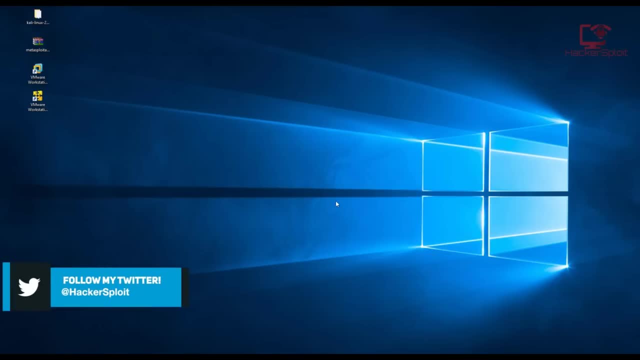 common because even the older, you know processes like the Pentium and the core two duos- they all support it- and some of the older AMD processes. it's a very, very common feature to have any processor have virtualization. Okay, now this will work on any operating system you could be. 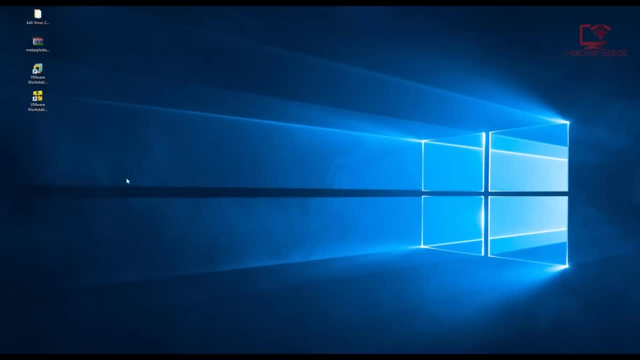 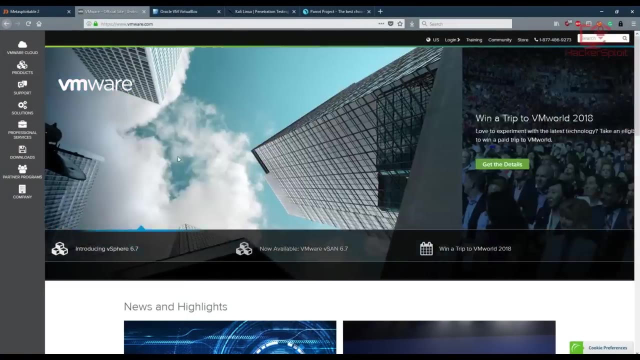 running macOS, you could be running Linux, and if you're running Windows, it'll be the same thing right here. Okay, so, as you can see, I've got these, these files, on my desktop and I'll be explaining them as we move along. Now let's get started with virtualization software. Now I'm going. 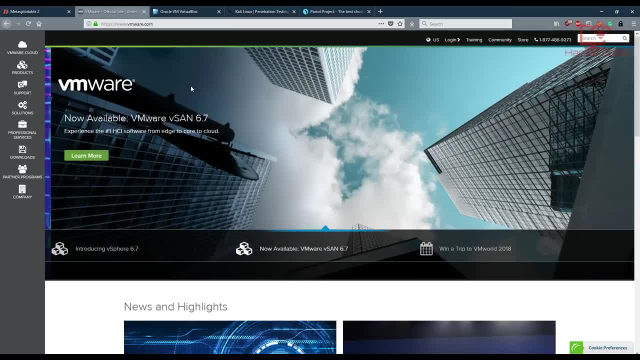 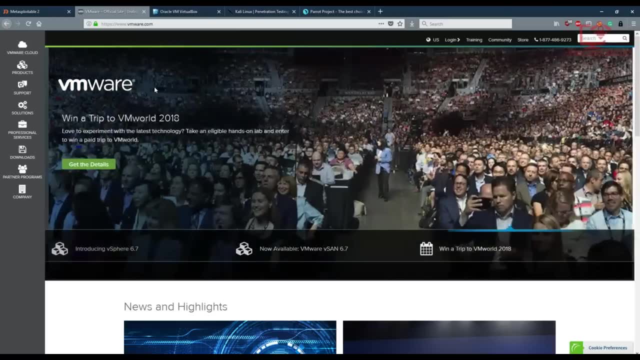 to start off with my favorite and what I recommend to you right now. All right, and that is VMware. Now you don't have to buy VMware. By the way, quick announcement: I'm going to be doing a giveaway. Probably when we hit 70 or 80,000 subscribers, I'm going to be giving away five. 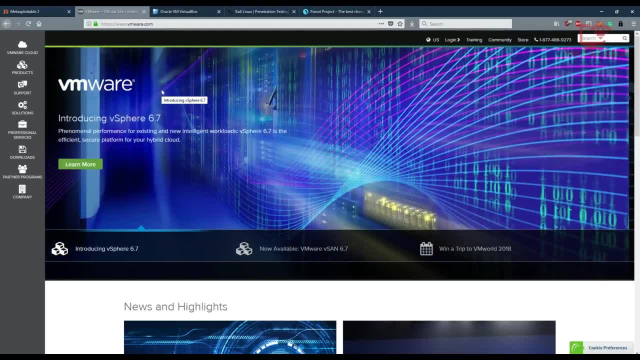 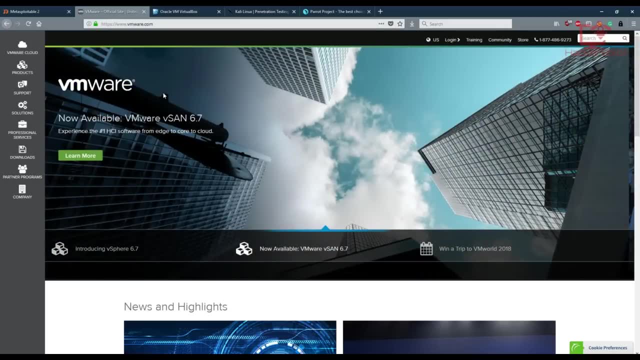 legitimate serial keys for VMware Pro so that you guys can also get started with it, because I've invested in it And it's absolutely fantastic, All right, But if you want to use the free one, I apologize for my phone notifications. Yeah, let me actually just turn that on silent. 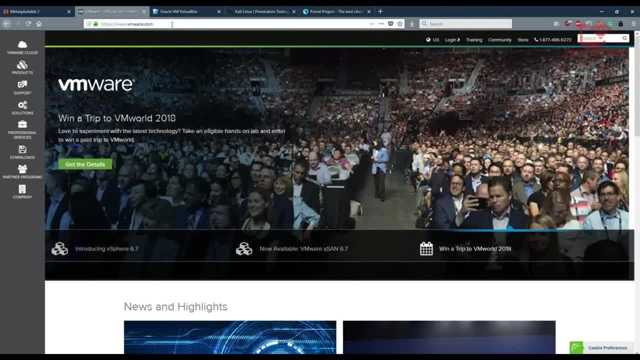 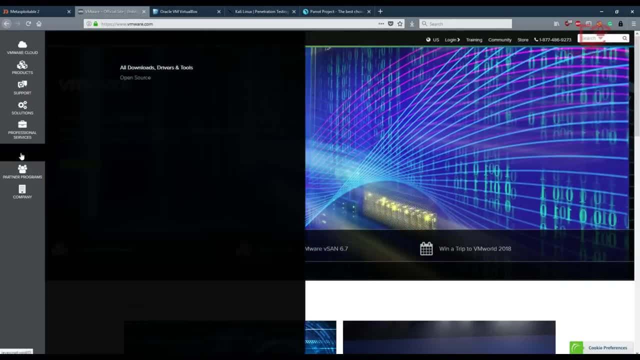 That being said, there is the free version and the website will be linked in the description so you can check it out for yourself. Okay, so let's get started with the download, So you can go to the left hand side here and click on downloads. All right, Now, if you look at product. 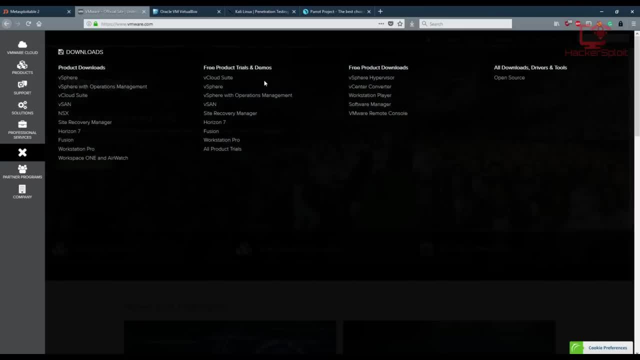 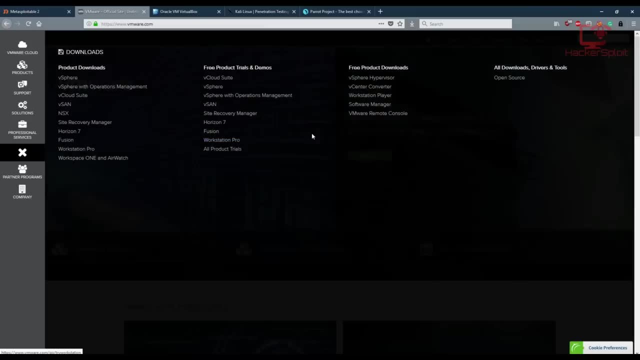 downloads. it'll show you all the products they have. you can then go to the free product trials and demos. Okay, you don't want to look for that. That all to do with demos. If you want to try VMware Workstation Pro, go ahead and try it. you can have a trial. you then want to go to your? 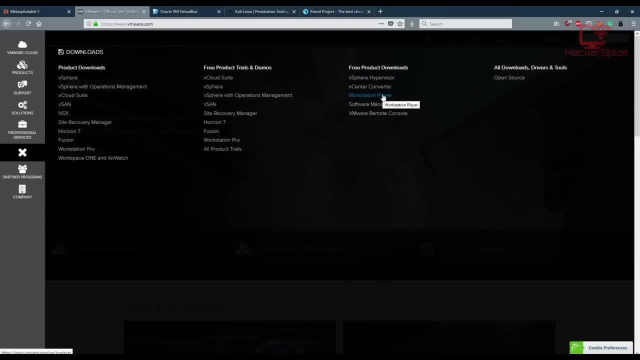 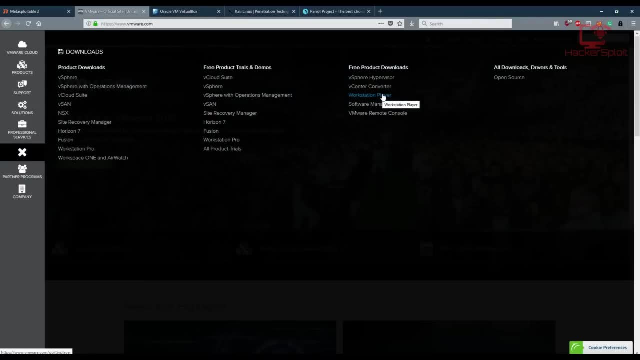 product downloads where you have workstation player. that is the free version and you can use it as much as you want. The difference between the free and pro version is that the pro version has more features in regards to do just making things easier when it comes down to virtualization. 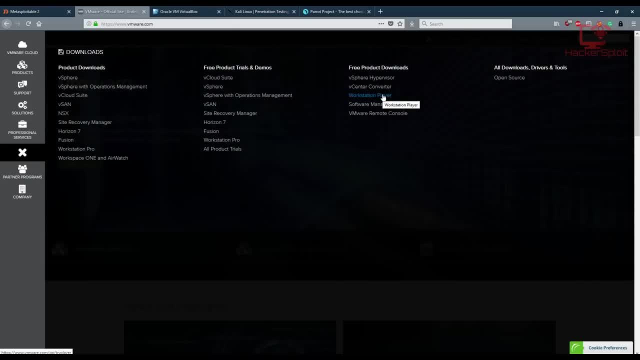 So you can. you can recover all that good stuff and probably make a video on the differences there, But if you're a beginner, you don't have to spend money on the professional version. Trust me, I use the free version and I've used it in many, many enterprise situations and it worked. 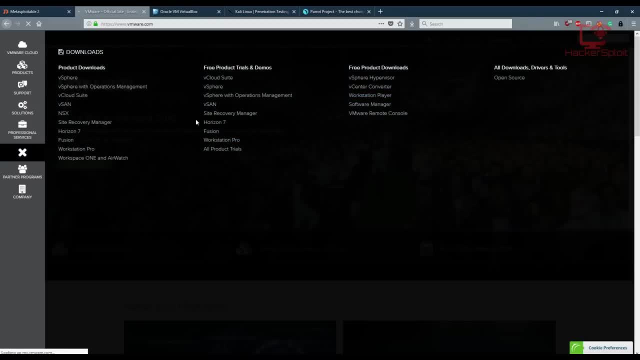 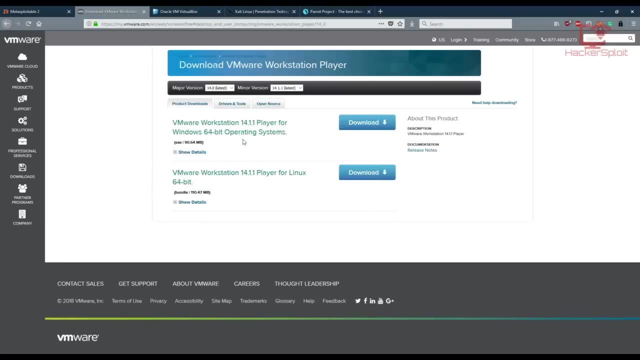 perfectly Okay. so you just want to click on one of the options here, So for example workstation player, and just let it load. apologize for my slow internet, if you know. for some reason it always is slow. So there you are. you can download it for Windows 64 bit operating systems and you. 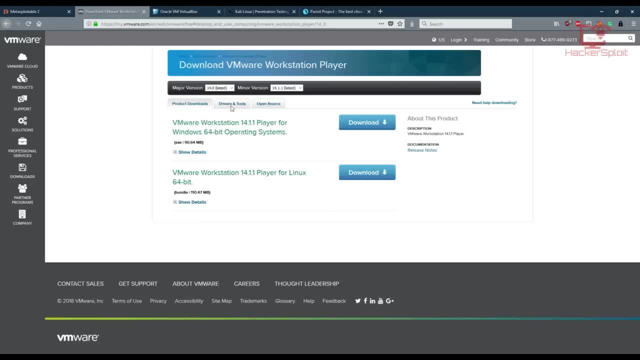 want, for you can select your option here for Linux. Now, if you're not interested or you don't like VMware, you can go for VirtualBox. VirtualBox is a virtual machine that allows you to download and install virtual machines. So if you're not interested or you don't like VMware, you can go for VirtualBox. 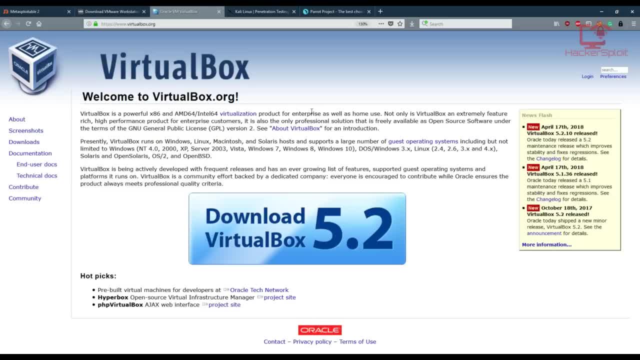 VirtualBox is a virtual machine that allows you to download and install virtual machines. VirtualBox was my favorite, but after a while it just has too many compatibility issues, especially with Kali Linux, And I'm going to be getting to do that in a second. 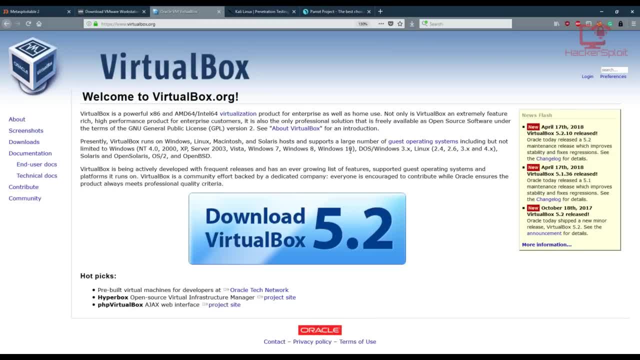 Alright. so VirtualBox is is essentially free and you can use it on Linux, you can use it on Windows. all that good stuff. Now, if you're running Mac OS, what I would recommend is that you use a software or a program called parallels. I'm sure you've. 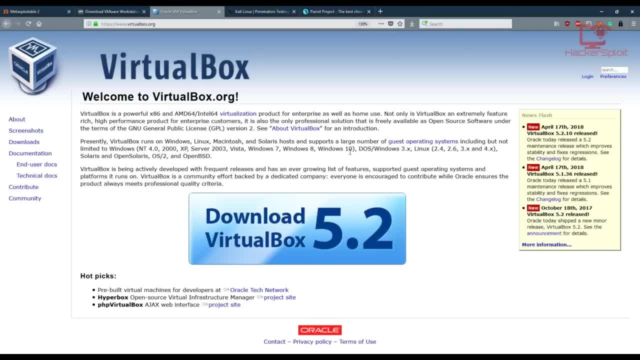 heard of it if you've been using a Mac, because that's that's essentially the only all the alternative to a virtualization software on the Mac OS platform. Okay, so don't worry if you're running a Mac. it's essentially the same process, just open up parallels. 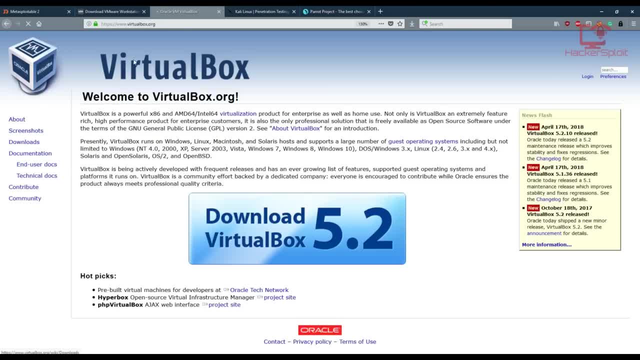 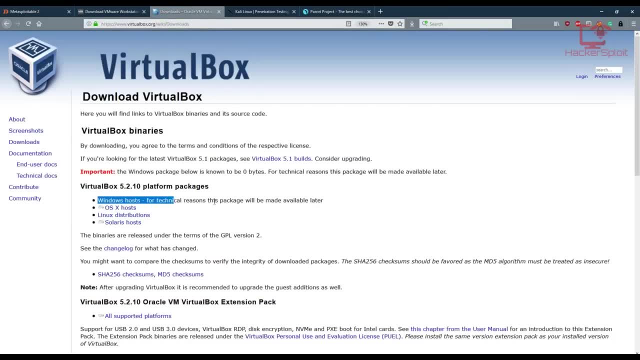 and you should be good. Okay, so with VirtualBox is it's completely free and you just can just go into downloads? don't worry, the link will be in the description And you want to look for the VirtualBox, the latest platform packages, And for some reason the Windows hosts is not. 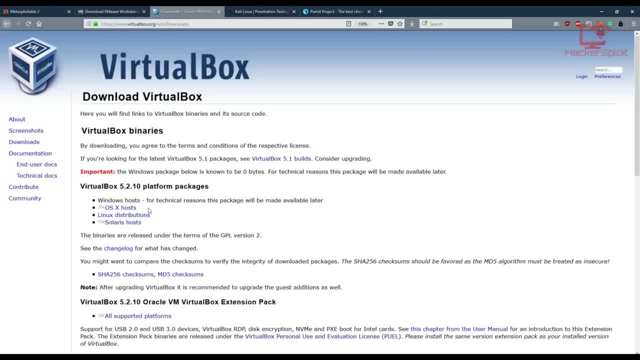 available right now So you can. Oh, by the way, they also added the USX. I believe they're going to be added, probably around the version five. Sorry about that. So you can also use VirtualBox On Mac OS. you can also use it on Linux and Solaris. So again, the. it's very simple. 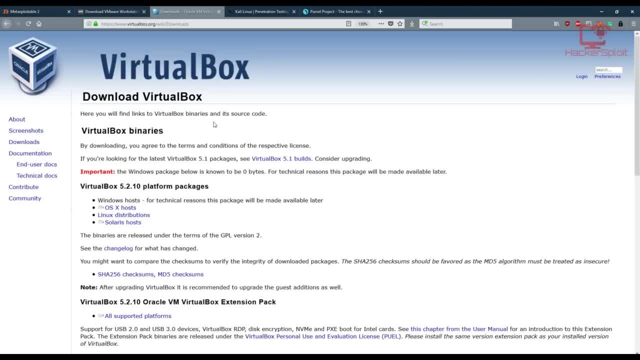 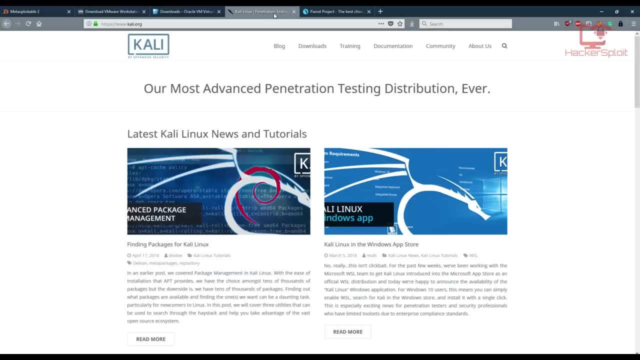 just download it and get it installed. Okay, so, once you've chosen your virtualization software, now it is one of the most taunting- is one of the most complicated. well, in my mind it's not really complicated, But for many beginners it's probably the most fidgety topic. 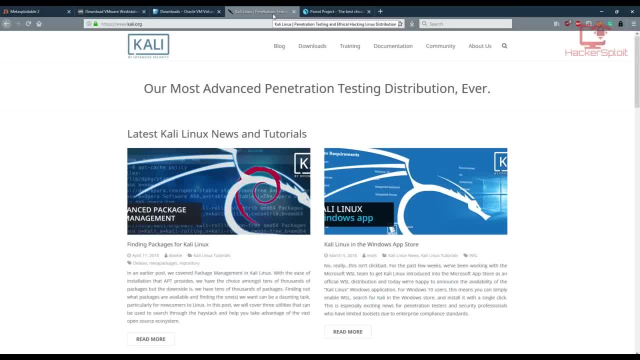 And that is selecting your penetration testing distribution. Now I'm going to recommend one of two, And that is Kali Linux. So you can use parrot, parrot OS or you can use Kali Linux. Now a lot of people ask me- or? 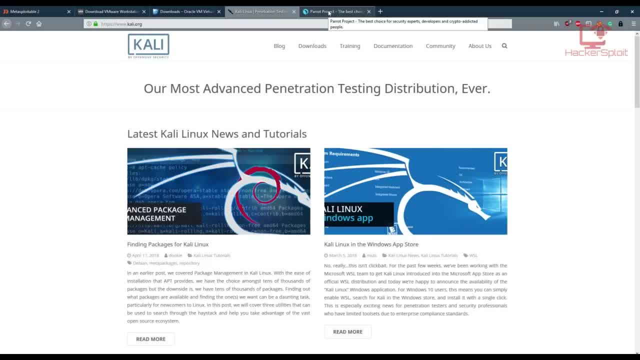 send me messages and, you know, post their comments in the description, in the comment section, saying which one is better, why it's better. And then there's always arguments, heated arguments, all of that, And here's what I say. okay, I was in the same dilemma, trust me. Well, mostly the time I 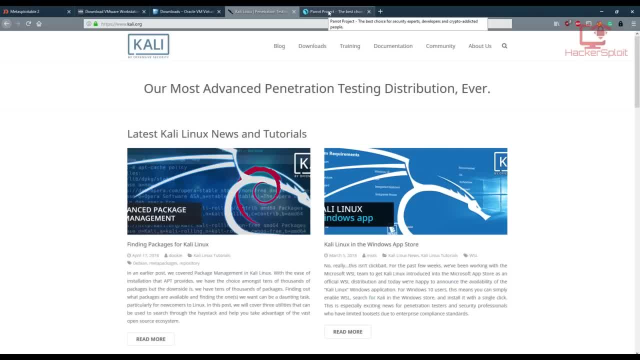 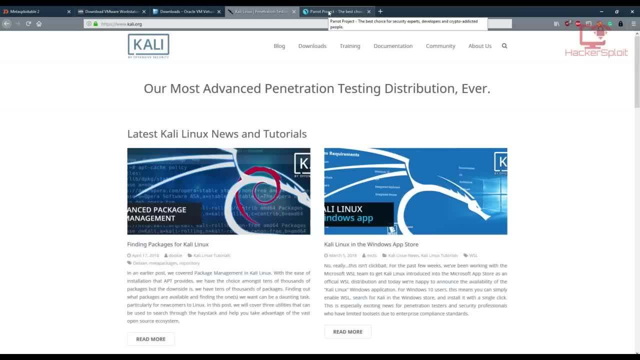 just choose one and stick with it. Now most people will say: start with Kali, master Kali, then you can use paradise. because it's essentially the same: functionality is transferred over, It's just that the difference is the operating system and the kernel and all of that. So it's. 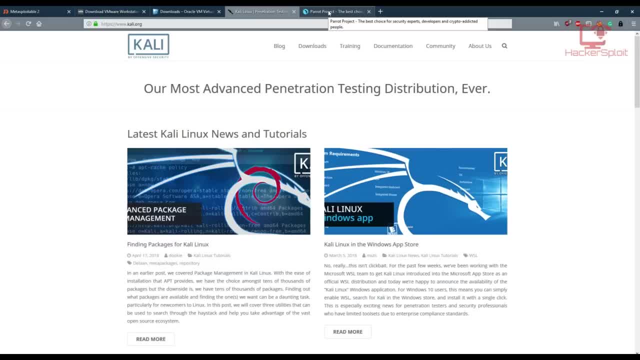 it's very little to do with the, the tools, because the tools are, you know, on all the platforms. So, again, it's all about what you like. So here's what I'm going to say: download each of them and then try which one you like. Okay, so maybe you can try Kali. 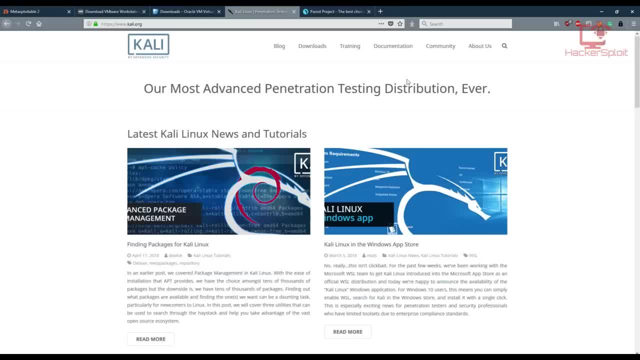 if you don't like it, try. parrot part is something that you may like, and do not be confused And do not be scared of making the decision. Once you've made the decision, stick with it And if you have any problems, then try and troubleshoot it. If you can't switch to the other one, All right, And in 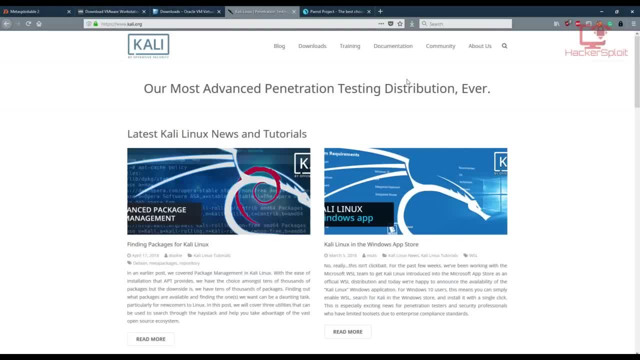 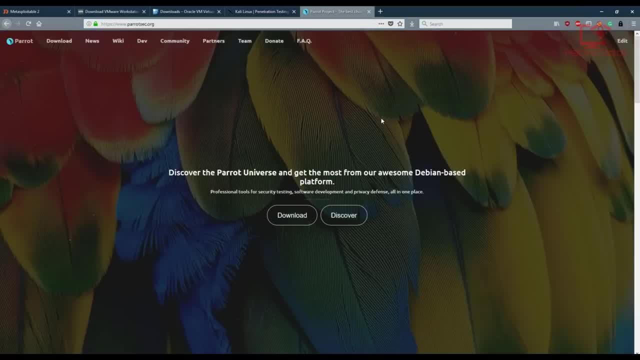 my opinion. I'll say this- that Kali Linux is an is an enterprise type of operating system, especially now. So it is what you I would call a industry standard. All right Now. parrot OS is fantastic. There's no doubt about that. I've used it for many, many projects. 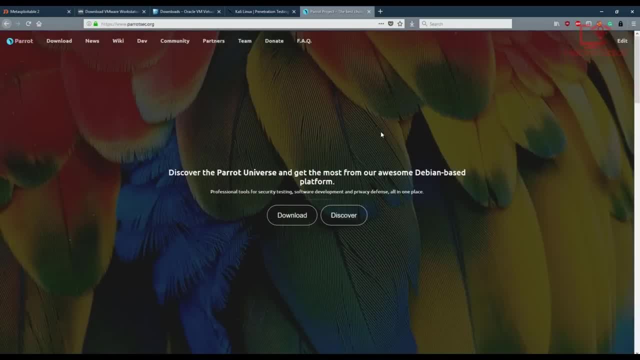 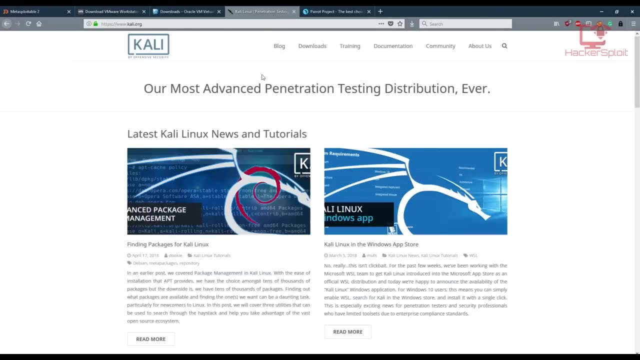 real life projects and I can tell you that it does work. But when you move on to a professional level, I would recommend Kali Linux because it is the benchmark And it is sort of required because the they're not going to allow you to just test systems, or employees are not going to allow you. 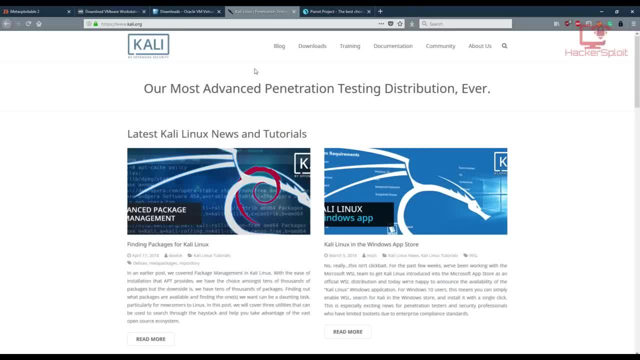 to test systems with tools that are not familiar. That's what I was also talking about. You know, installing all these weird scripts isn't really going to help, because you have to know how to use the industry standard, And that's what I was also talking about. you know, installing all these weird scripts isn't really going to help, because you have to know how to use the industry standard, And that's what I was also talking about. you know, installing all these weird scripts isn't really going to help, because you have to know how to use the industry standard tools. Okay, so you can. 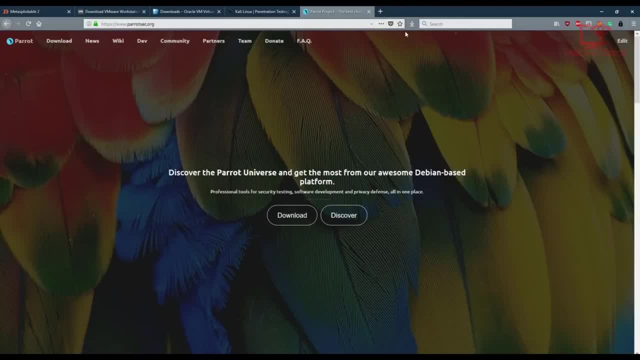 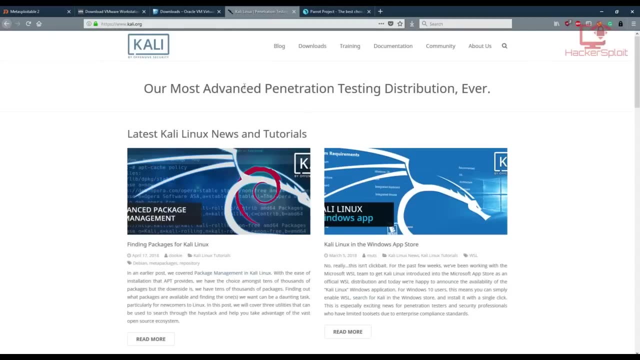 choose between Kali Linux and parrot OS. Now, when it comes to black arc and back box, all of that, all of those other distributions, I'm not really going to include them because that's again a matter of personal taste. Okay, So, getting back to Kali Linux, I just want to talk about something. 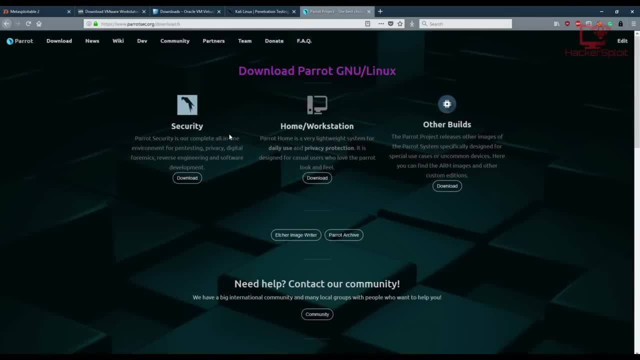 for parrot OS. the download is very simple. just go to download And you have three versions. okay, you have your security, which is the one you want to get. you then have workstation, which again is focused, is a lightweight system for. 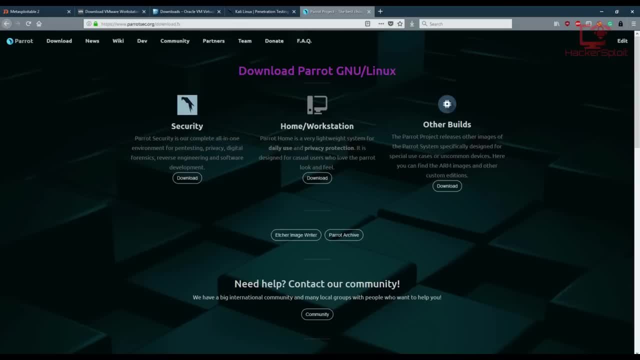 daily use and privacy protection. So it offers a solution for casual users, as you can see, who love the look and feel of part. you then have part security, which is a complete all in one environment for pen testing, privacy, digital forensics, reverse engineering and software. 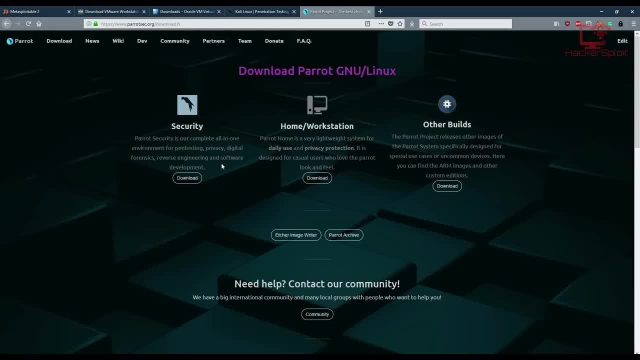 development. So again, it's focused on all of those facets And that's why I kind of like it And I've tried it out. But for me I'm not really doing, you know, digital forensics or reverse engineering. I have some of you might be doing it And if that's your field, then by all means. 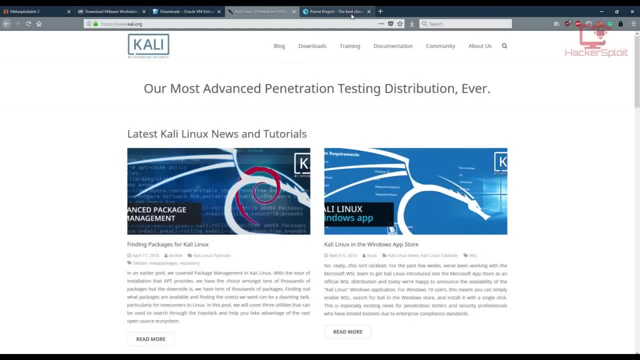 go ahead and download it. And if that's your field, then by all means go ahead and download it. And if that's your field, then by all means go ahead and download it. And if that's your field, then by all means go ahead and use para tours. Okay, now let's get back to. let's get back to. 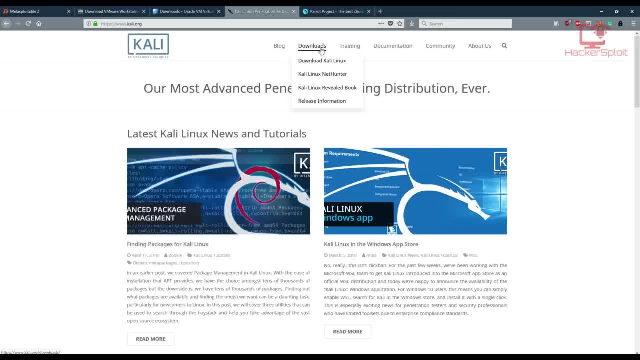 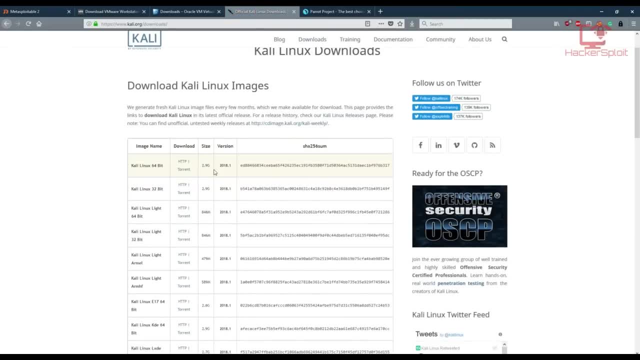 Kali Linux, And I just want to talk about the downloads. Now, if you're installing Kali Linux in a virtualized environment, I'm just going to show you a little tip here that will save you a lot of time: do not download the ISO file, All right. many people I've seen make this mistake. 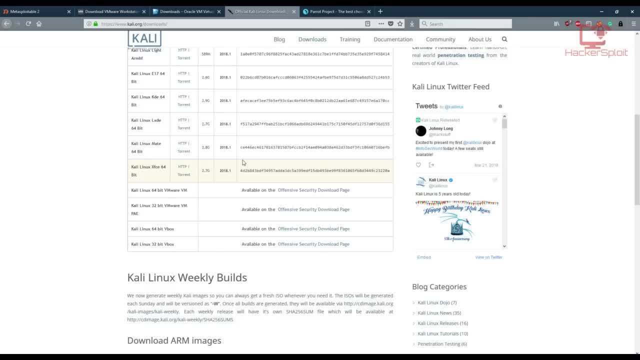 and I've made made any video, an installation video of Kali Linux, showing you how to install it using the ISO, even on a virtual machine, And you can see it's just really really heck tick. So why would you want to go through that? What I would recommend is just download the VM. 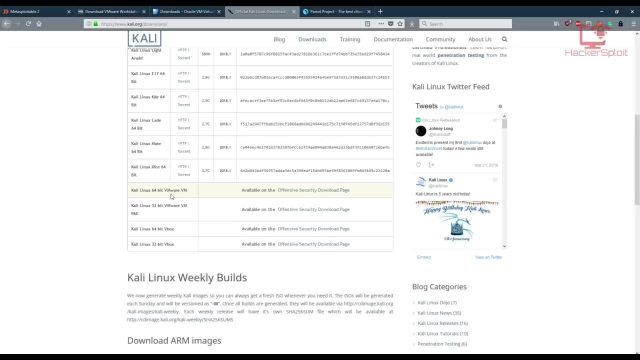 where virtual machine or the VirtualBox virtual machine. All right, as you can see, you have your VMware, your 64 bit and your 32 bit, and the same for VirtualBox. So for those of you are telling me it doesn't work on 64, on 32 bit, you can see here that indeed it is real and it is working. 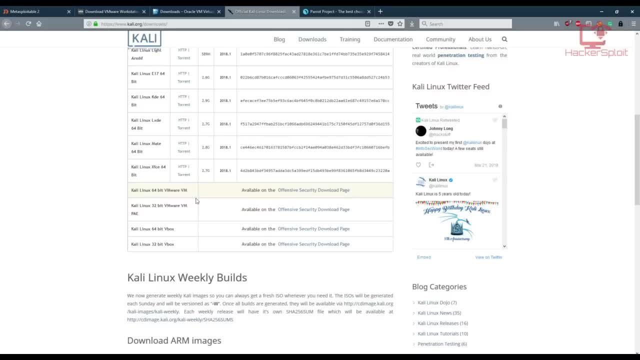 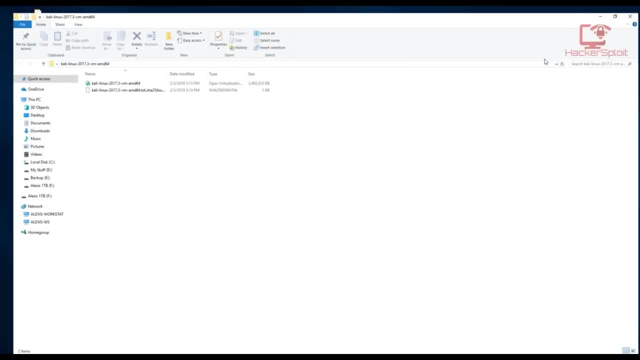 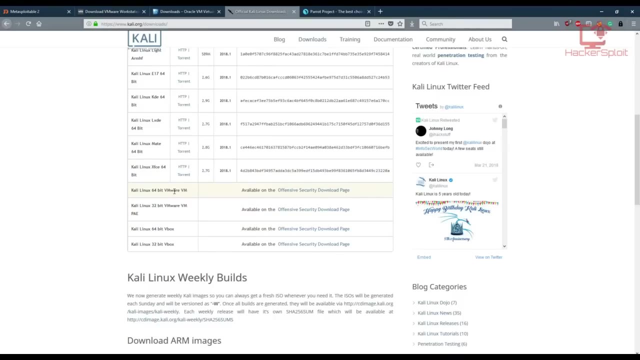 So once you download one of these dependent on the virtualization software you're using. so, for example, I've downloaded or I had the, the virtual, the VMware version. I'll show you know in a few seconds how easy it is to get it set up. So this virtual machine is already installed. 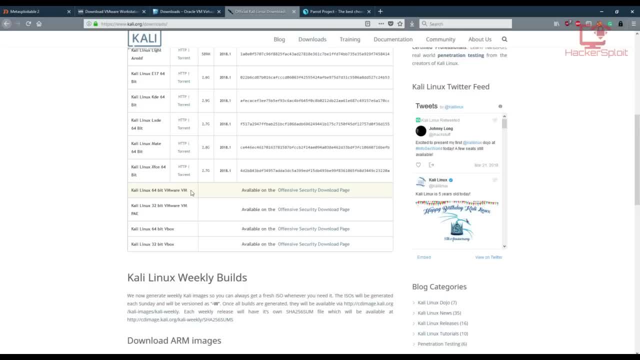 you don't need to go through the installation of Kali, it's already installed. you just need to import it into a virtual machine And that's it. And that's that. you get started immediately. Same for VirtualBox. Now for the rest of the video, I'll be continuing with VMware, And that's because. 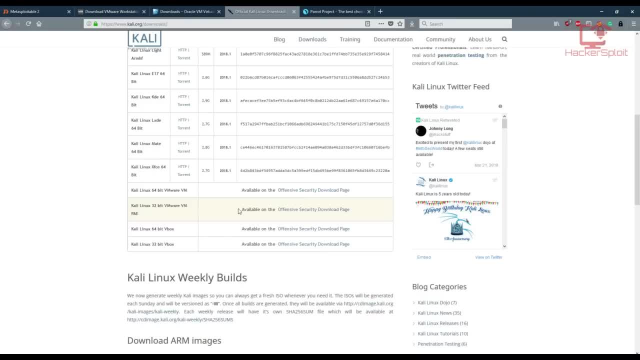 as I said, I've kind of lost control over the virtual machine. So I'm going to go ahead and lost the liking for VirtualBox And I have. that's no offense to VirtualBox, I just like VMware because it's never let me down And there aren't any compatibility issues with installing the. 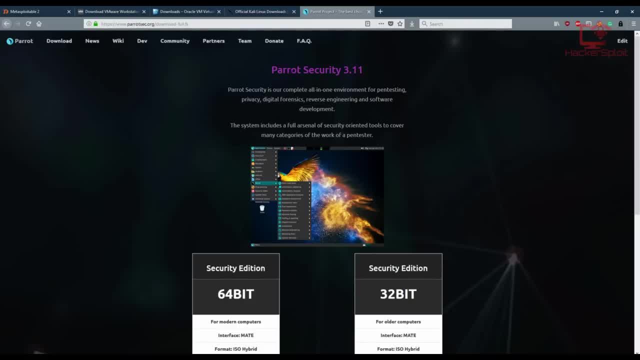 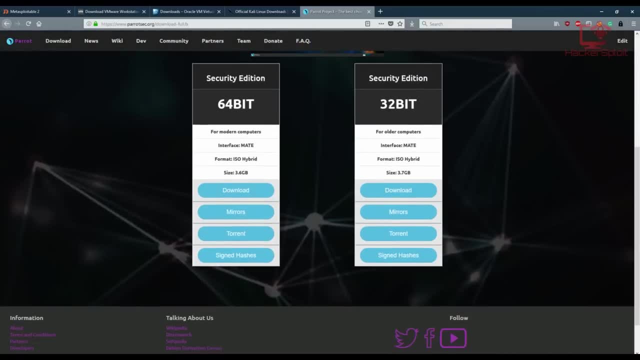 you know the libraries, or all of that you know. So, going back to parrot OS, you can see that the latest version as of recording this video is parrot OS 3.11.. Okay, and you have your 64 bit. 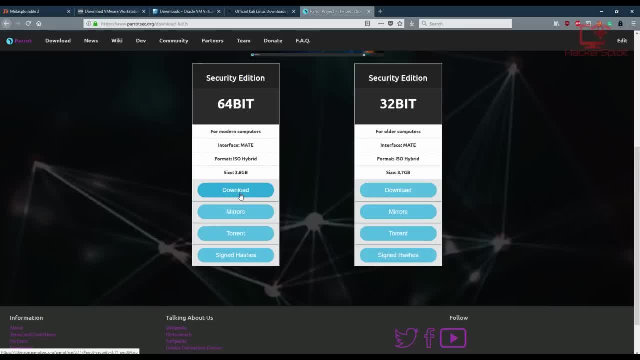 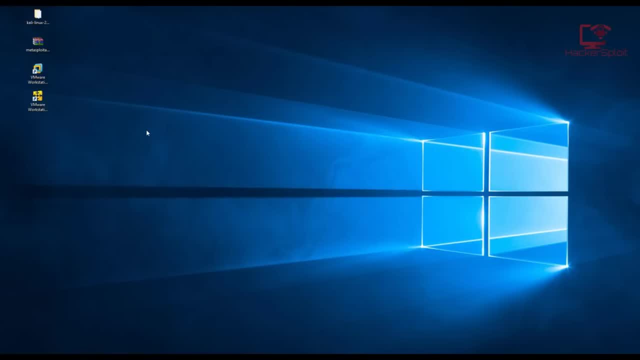 and your 32 bit And this is essentially the ISO. Alright, so the ISO for parrot is really very simple to install Or to create a virtual machine. all you need to do is open up your virtualization software. As I said, I'm going to be continuing with VMware Pro And, you can see, also have the VM or workstation. 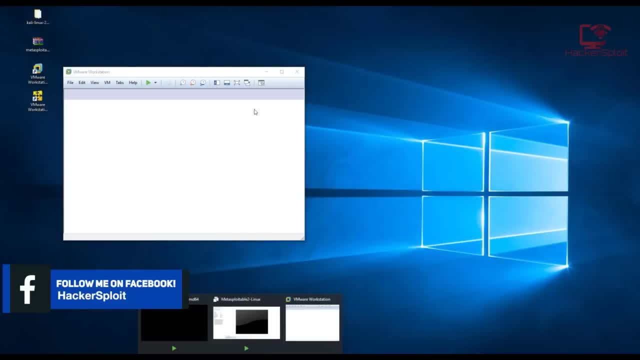 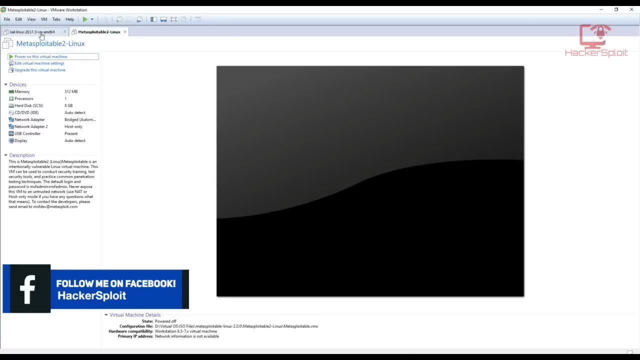 14 player. So if I just open up that or actually have it open, sorry about that. For some reason I opened it another instance there, So let me just show you something. I've already opened it up And you can see. these are the two virtual machines that I always have running. One of them is Kali. 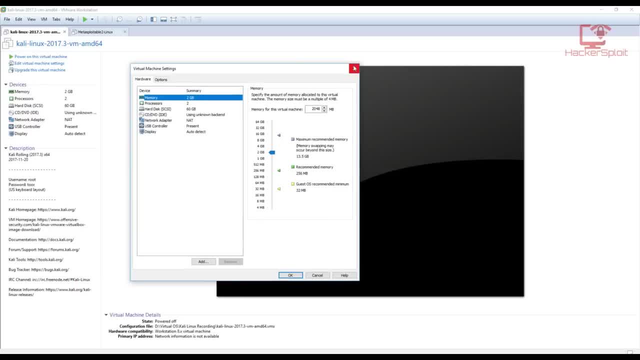 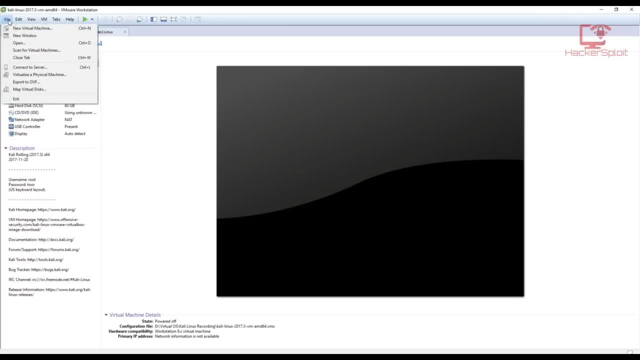 Linux. Don't worry about the title. I have updates So you can edit your virtual machine settings there And we'll get to that in a second. Alright, so I have Kali Linux and Metasploitable tool Now, don't worry about this. if you want to create a new, 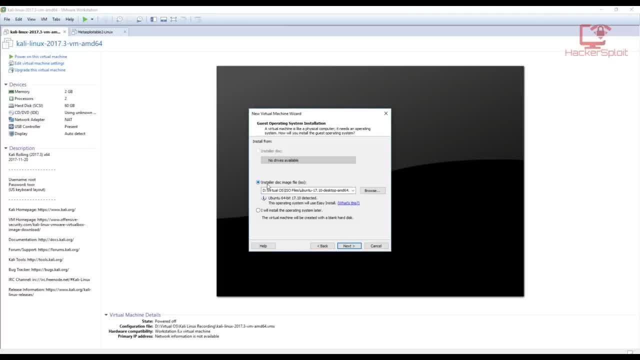 virtual machine. just going to file new virtual machine. go for typical, And next you want to then select your ISO image. as you can see, mine is for some reason selected in Ubuntu ISO, So just hit next. we'll use that as an example. So then it's going to prompt you, if you're running Ubuntu, to 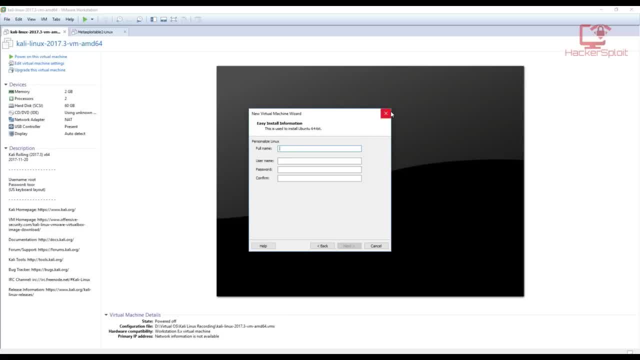 enter your full name, your username and password. If you're running para2s, it's not going to prompt you to do that, Okay. but, as I said, if you're running this on a virtualized piece of software, if you want to run this in terms of virtualization, 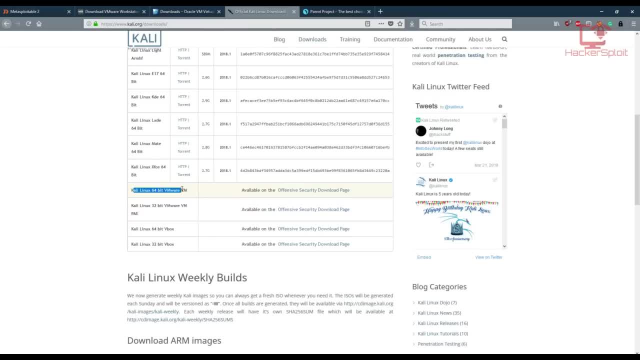 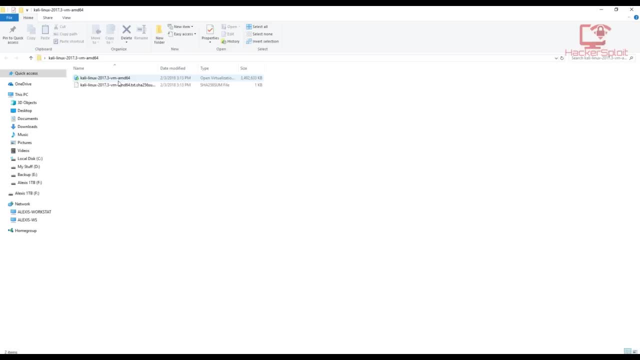 then download. do not download the ISO unless you're using para2s. download the virtual machine file here, because that automatically imports, And I'll show you that in a second. So let's say I've downloaded the VMware file here, I can just click on it right here. As you can see, once I click on 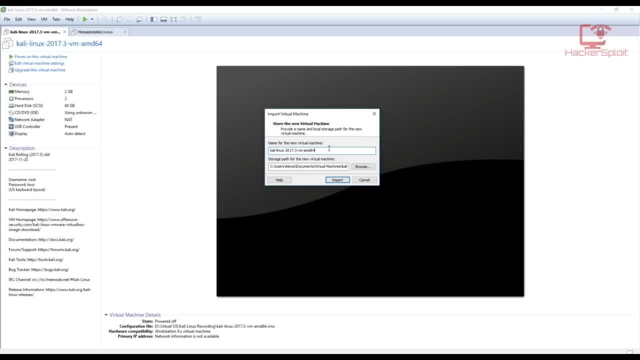 it. I already have it, So it's not going to prompt me, but it's going to prompt me again to to re import it And that's going to essentially wipe your current hard disk if you already have one installed. If you're new, just hit. 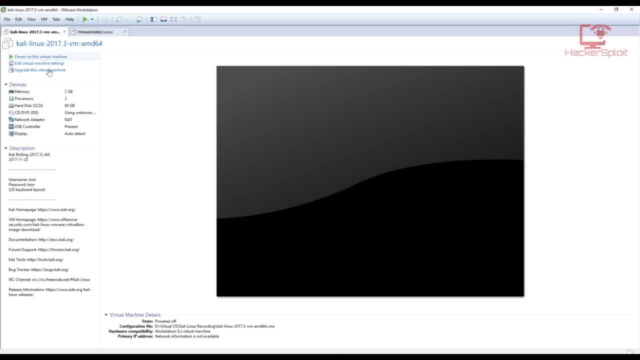 import and select the destination, And that's that you don't have to install it. Once it's imported, you're going to be given this beautiful menu here giving you the version again. you can edit it and change the name And it's going to give you this awesome description here saying this is the 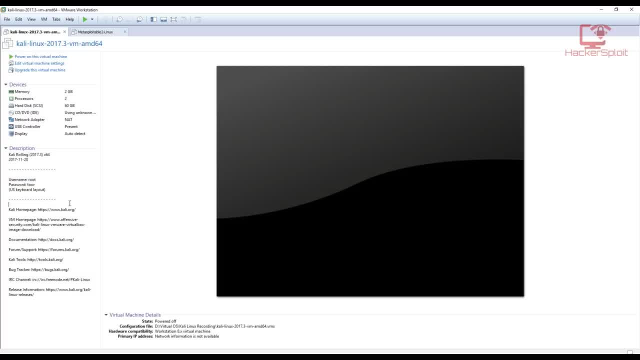 username is root, the password is Tor and the keyboard layout is us. Alright, so that's information that you can just check out and gives you the IRC channel, all that good stuff. Okay, so it's going to give you this little menu here. Excellent, So now you can edit. 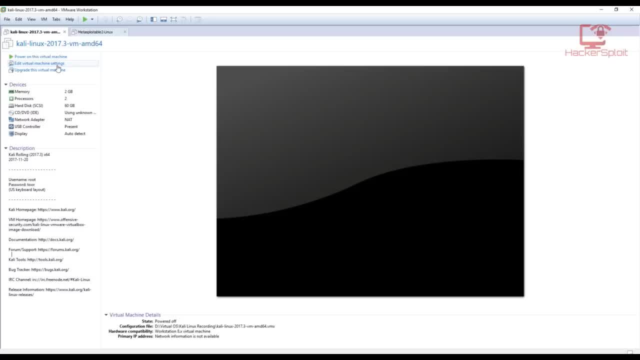 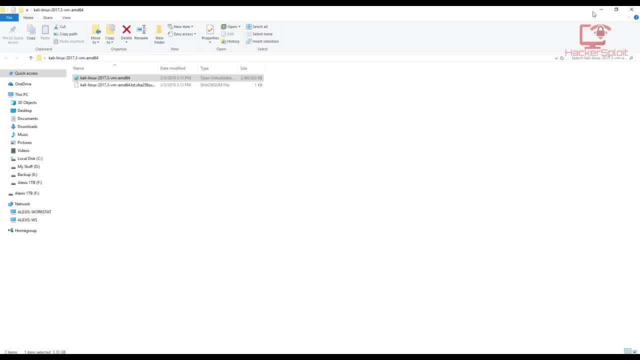 your virtual machine settings, which is what we're going to be talking about now. Okay, but before that, let me show you how to download your vulnerable operating system, which, in this case, is metasploitable to now. a lot of people have asked me to do the metasploitable three video And the 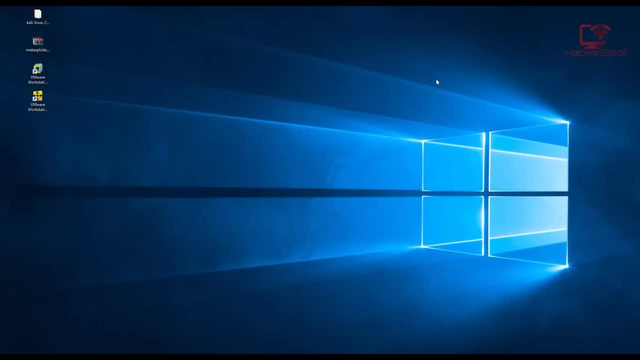 reason I haven't done it yet is because that thing has bugs, that I've tried it installing it on my computer and it worked after five hours of configuring it. I then tried it to try to do it on another computer same way. that gave me success. 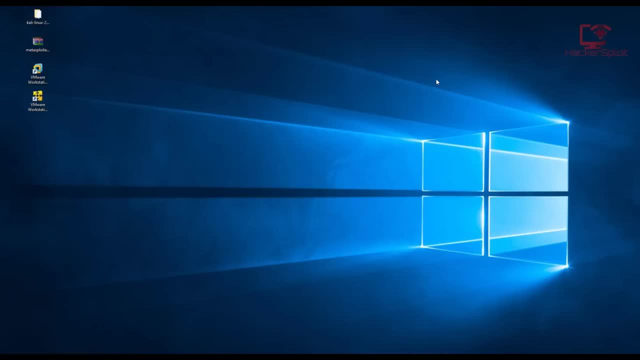 on one computer and it didn't work, So it it. it's come to my attention that you need to configure it individually for every computer, and a video, therefore, will not be a good, so I'll make a post on my website regarding how to select the appropriate settings. Okay, so again, it's very. 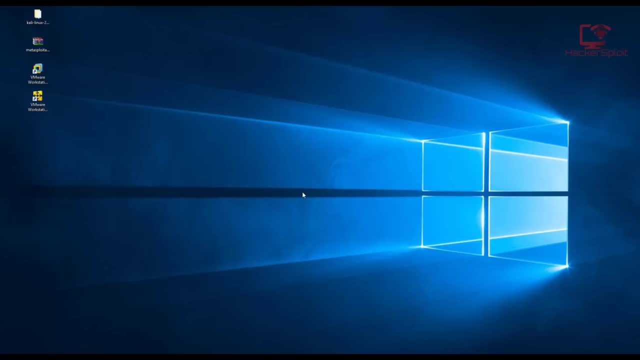 dependent on your hardware and you need to be really attentive when installing. it is just a pain in the neck. What I would recommend is just using metasploitable to and installing your own tools on it, or using CTFs. Alright, so you want to open the link in the description that takes you to the 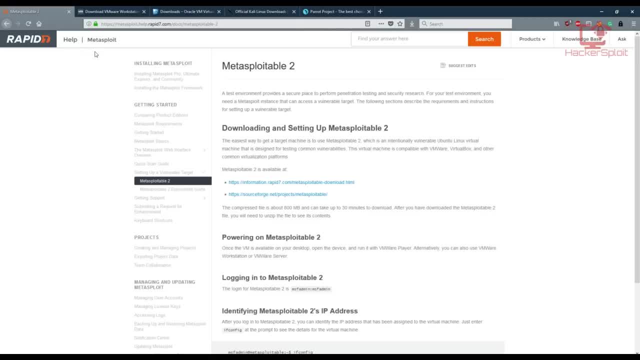 metasploitable to page. it's developed by rapid seven which, as you know, created metasploit. All right, and I'm sure you know about the metasploit framework And you can just go ahead and look at the download page. here you can go for the rapid seven download page. 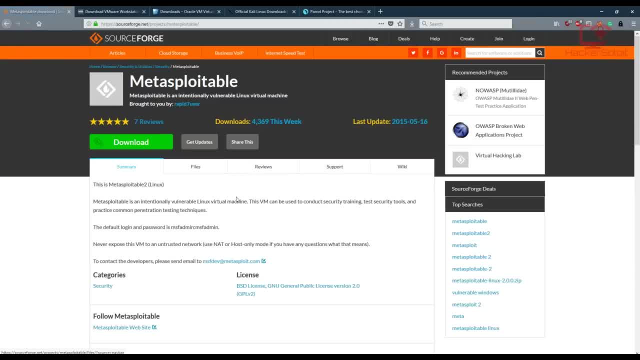 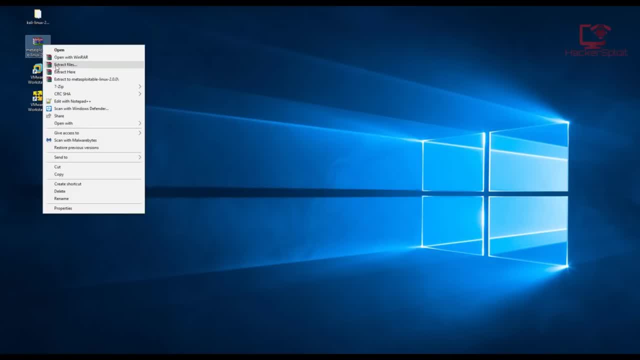 page or the source for the download page, and just click on it And it's gonna prompt you to download it, Alright. so once you have it downloaded, it's going to be a zip file on your desktop right here. So I'm just going to extract it, metasploitable to, just going to extract it to my desktop And as you. 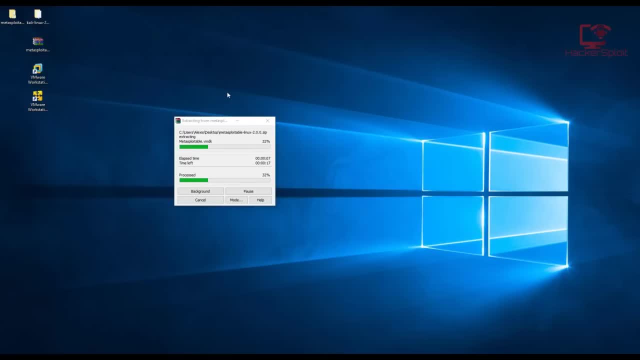 can see this runs exclusively, So let it just open up, because I really want to show you what I mean. All right, So let that just extract. I apologize for the speed, Although the file does take a while. even on all computers that have tried this on, It always is a quite a hefty. 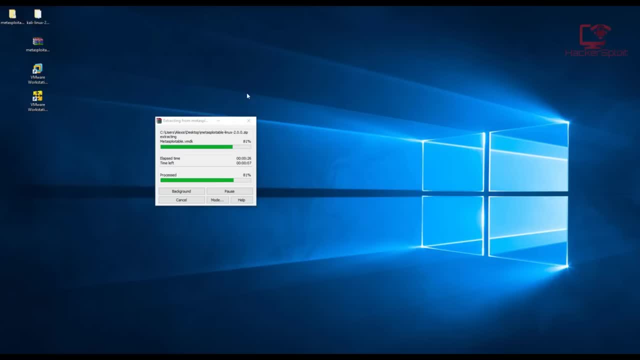 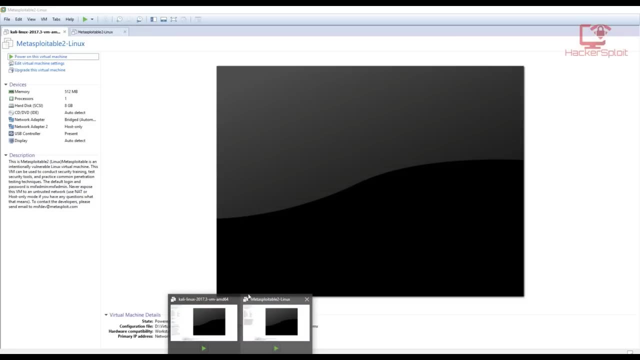 extraction process, probably because it was zipped very, very thoroughly. Okay, so let this complete and we can just move back into our virtual machines here. Alright, so I already have metasploitable imported. we'll be looking at the settings you need to set and then we'll be looking at the 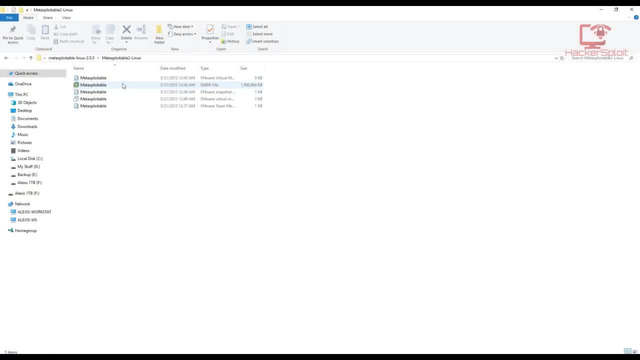 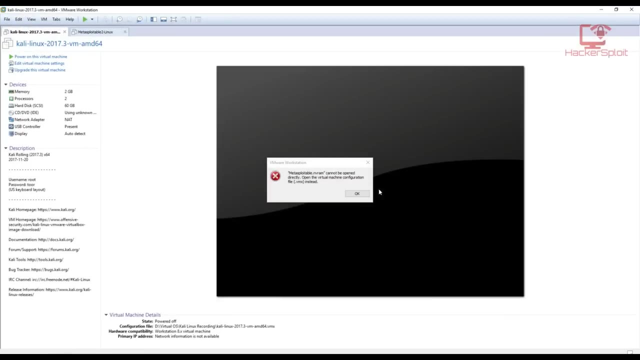 network configuration. Okay, so metasploitable two has successfully been extracted And, as you can see here, this is a virtual machine disk file, So you can just click on it and it will import it to the system the same way. So if I click on it you can see: whoops, sorry about that. If I just click my 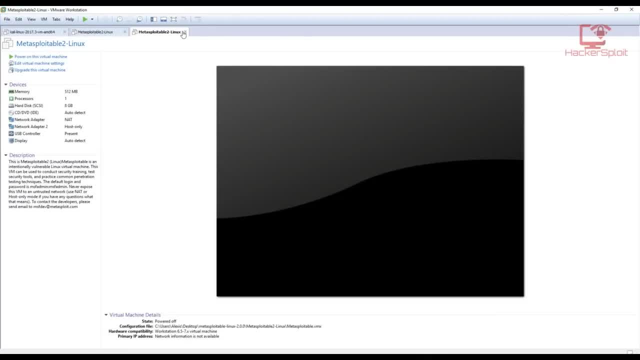 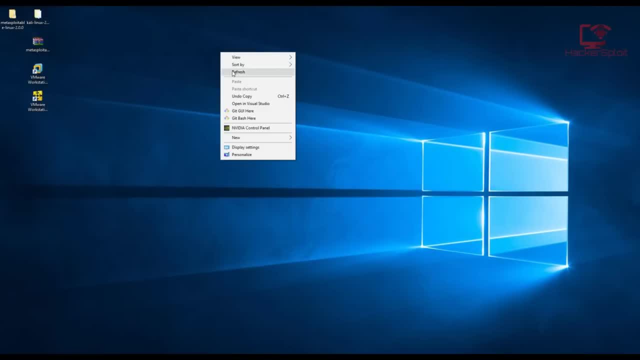 bad. sorry, you actually have to open the virtual machine file there And that will prompt it to open directly from there. Alright, so I already have one that has all my data saved there, So I'm not going to do that. Okay, so that once that's imported, let me just get rid of that, because I 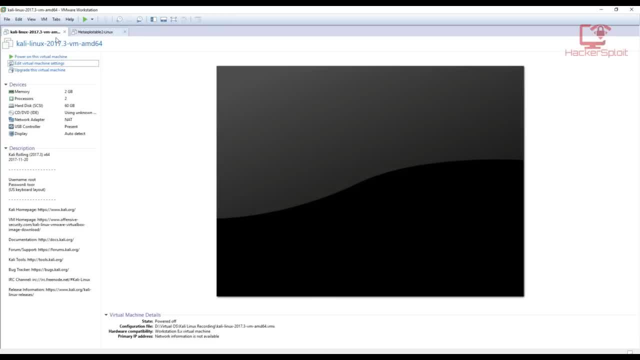 don't need it right now. Now we can get started with the virtual machine settings- Very important. So make sure you have Kali Linux opened in one tab or pirate OS, And you have metasploitable to open another tab. Now let's start. 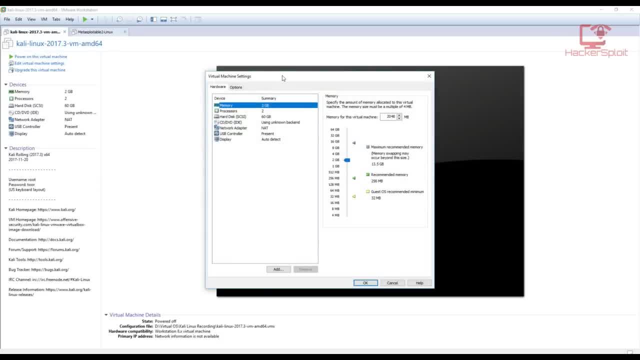 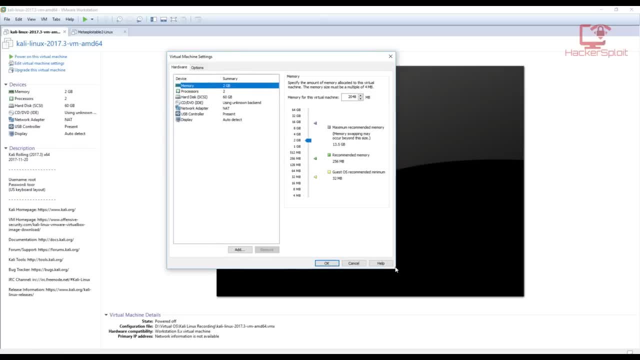 off with Kali Linux, the settings here, Alright, so you're going to go into edit virtual machine settings. Now, as I said, you must have, I would say, at least four gigabytes of RAM. Alright, And the reason being is: Kali Linux works great with two gigabytes. If you have more system, if you have 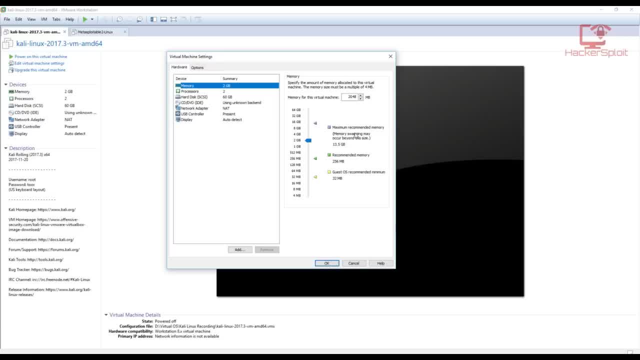 more RAM. you can then increase it What, Whatever you like. Now, if you're running a one gig- or I mean a two gig- computer that has two gigs of RAM, do not worry, you can reduce it to one gig as well, But it'll then be really, really. 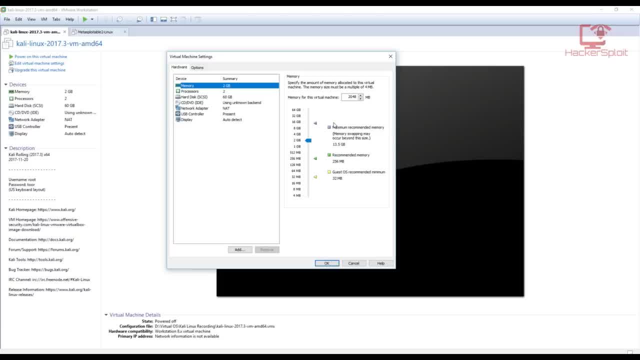 slow And you won't be able to open up programs. or, you know, Metasploit will take a huge amount of time to start up. All right. That being said, if you have a four gigabyte computer, just leave it at two. And if you have eight or 16, it doesn't matter, just leave it at two. it works really. 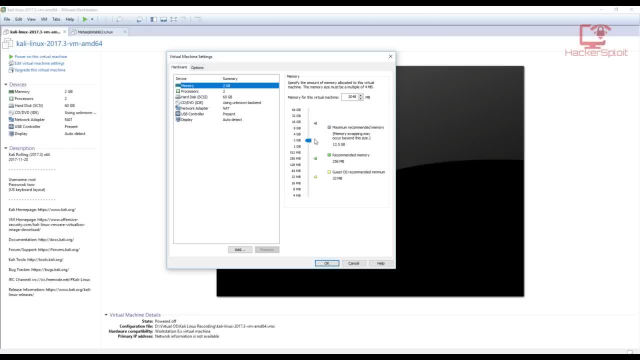 great there, Unless you start doing things like reverse engineering. you know things like that, things that are very resource hungry in the RAM department. Okay, so you then want to go into your processors. Now this is again very dependent on your hardware specifications and your processor. 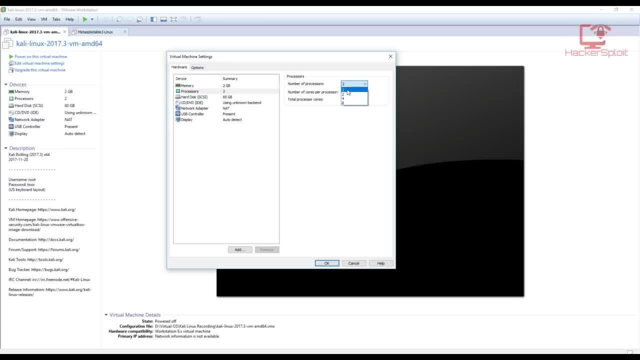 more specifically. So if you have a dual core processor, what I would recommend is just using one. Okay, Now you can select the number of cores per processor, And that essentially is hyper threading. Okay, So right now, as you can see, I've put two processes, and that theoretically. 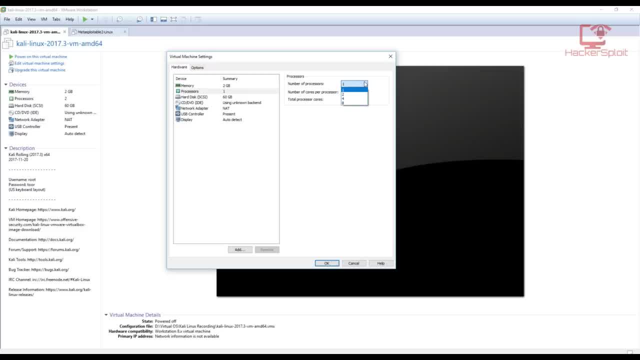 is wrong, because I only have one processor. Now, if you're running a four gig computer, you can run a server type of workstation that has two sockets on the motherboard. you can then select it from there, Alright. so I was just explaining that many people put this because they think they 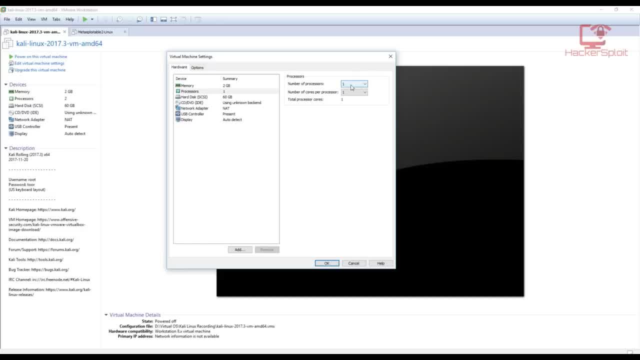 have a quad core. that that is for not really okay. so you want to make sure you select one processor- that I'm guessing that's what most of you have- And then you want to select the cause. All right, Now my processor has four cores, Alright, so I'm going to select two. that gives. 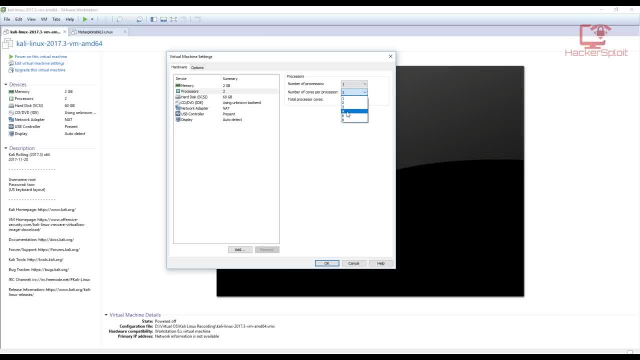 me an optimal performance. Now, if you want to give it all four, it will work great, But then you're all your host operating system. you're not going to be able to do that, So I'm going to select all four. Now, if you want to give it all four, it will work great, But then you're all your host operating. 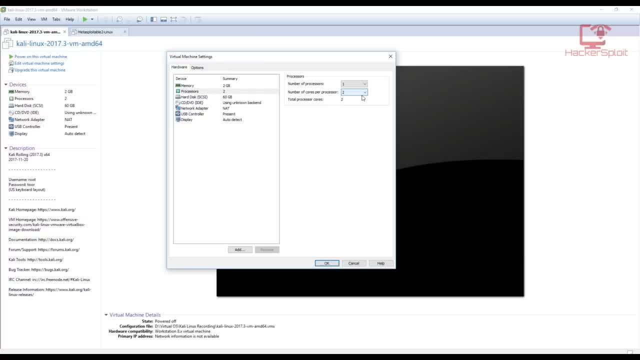 system will not work as efficiently as possible. So I would recommend two if you have a quad core, if you have a dual core, you can use one, one core, and that's perfectly fine, All right. or you can use two and you can just turn off what's running in the background. So that's how. 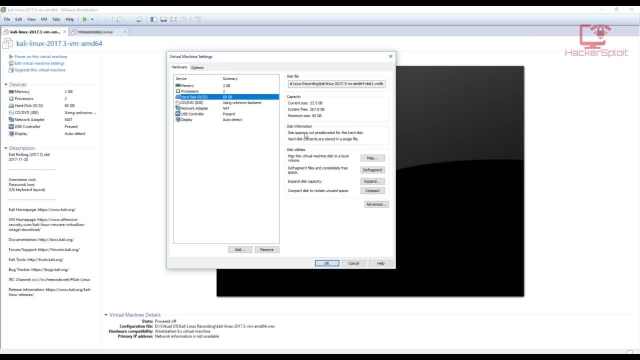 I like mine right there, Right. As for your hard disk, you can, you can. you can currently look at the size that it gives you: it's around 60 gigabytes. you can then also expand the disk capacity dependent on the, the type of files you're using. So, again, you can expand the disk capacity. 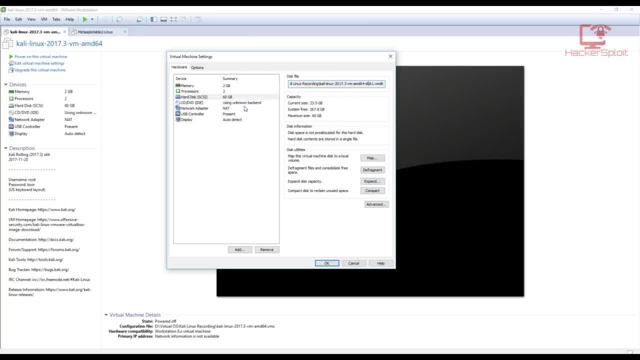 and expand it if you so choose to, And you also have your disk file location right there. All right, if you want to use a CD or DVD drive- which I'm guessing you don't- you don't need to touch anything there. And now for the network adapter settings. Now a lot of people get confused here. 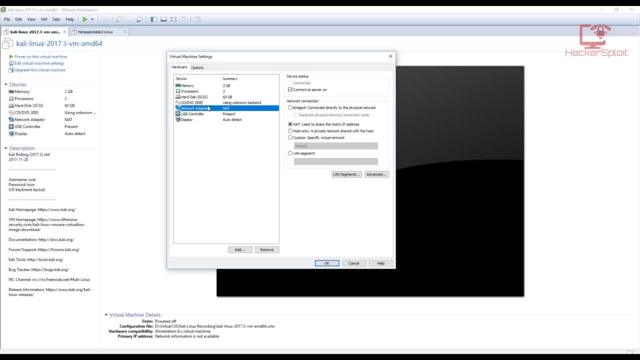 what we want to do is we want to make sure that that the virtual machines, both Kali Linux and metasploitable- or power to us, depending on what you're using- are connected to the physical network. That means they're using your adapter, your computer's host adapter. 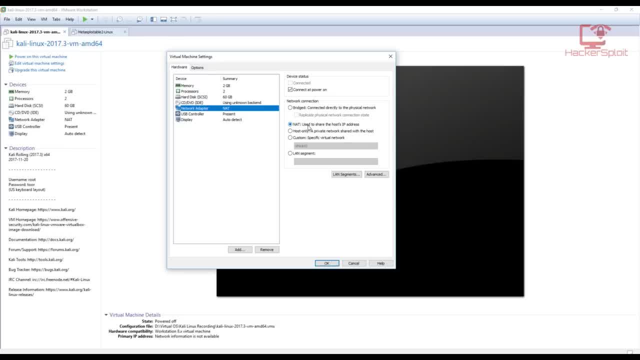 whether it's a Wi Fi adapter or it's an Ethernet adapter. Right now you can see I'm using that. So what this means: it's going to share the hosts IP address. Now what this means if I was to leave it. 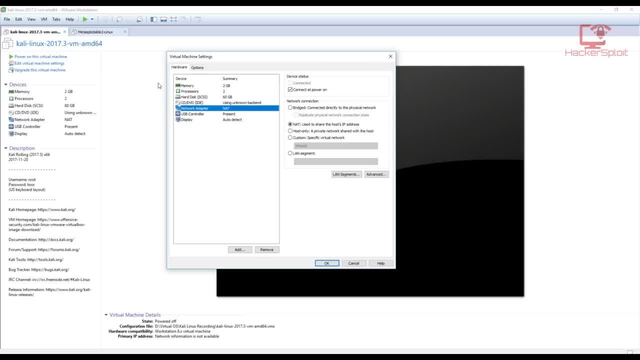 on that. that would mean that if I launched Kali Linux and I also launched metasploitable, they would have the same IP address as the host IP address, So it will have the same IP as Windows. Now most people think that that's okay. No, 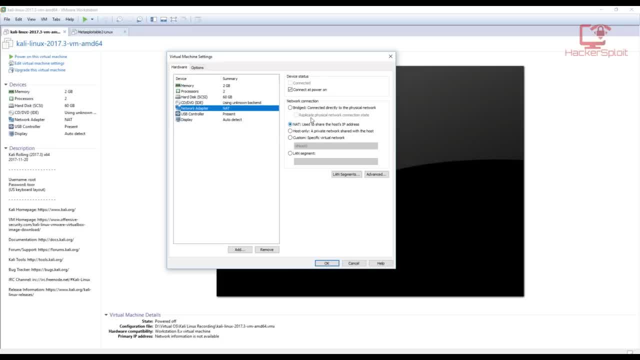 you do not Want that. you want each virtual machine to have its own IP address And you do that by going for a bridge connection and then replicate physical network connection state. that will make sure that it replicates the fact that it's on ethernet, it's on Wi Fi, it's going to also display it as Wi Fi. 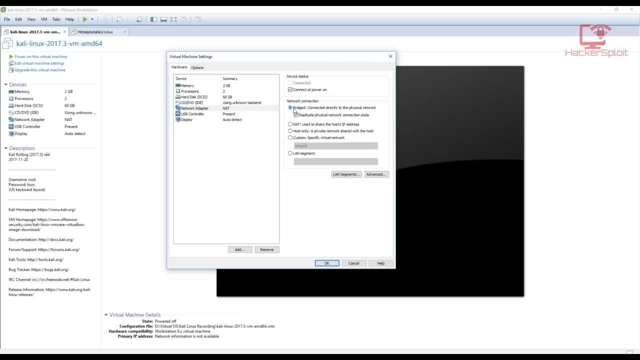 and they'll all have their own IP addresses, their own local IP addresses. Okay, so this very important make sure it's set to bridged. Alright, awesome. Once that's done, you can play around with your USB compatibility. If you have USB 3.0, you can connect to your USB 3.0,. 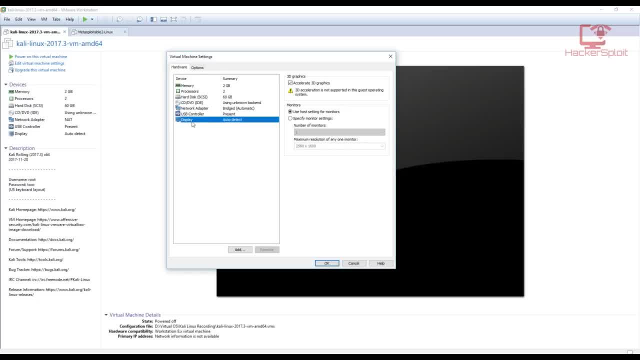 USB 3.0 drives that you want to be using. you can also do that as well, And you have your display settings. Now again, this is something that many people ask me: should I use accelerate 3d graphics? I would recommend that you do if you have a dedicated graphics card. However, if you 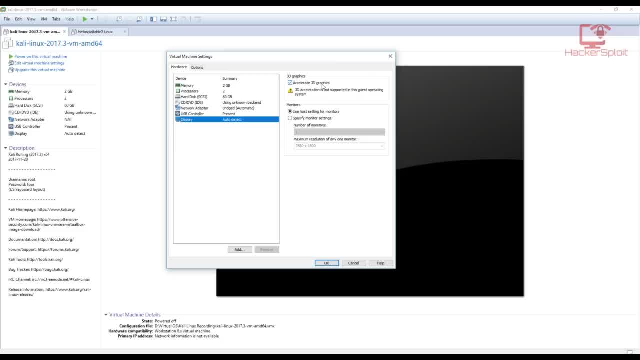 have an APU or integrated graphics card, then I would urge you to shy away from this. Now, many people also asked me: how do I use more than one monitor, because I have a triple monitor or a dual monitor setup And you can just specify the monitor settings depending on how many monitors. 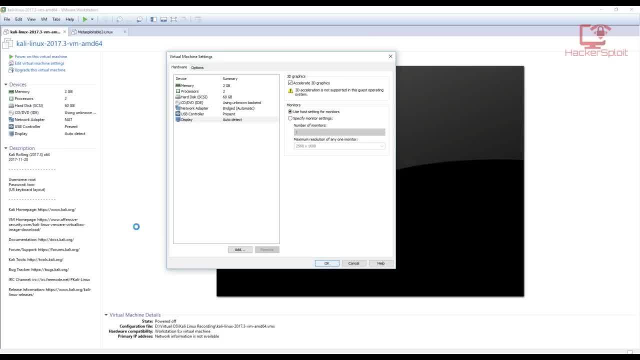 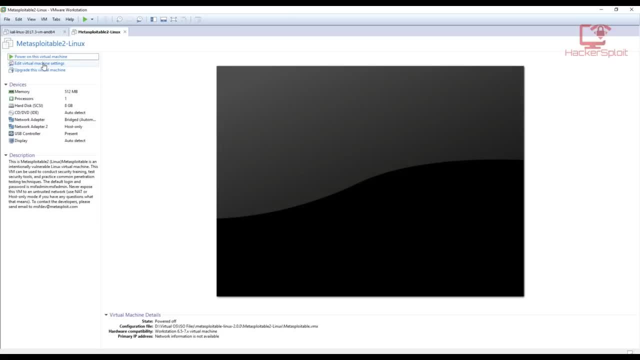 you have And you can select the resolution. So it's really that simple. Now, that's all the tough stuff, Let's hit OK, Those are the settings for Kali Linux. you know, want to go into Metasploitable 2, which again I want to just show you a few settings. go into Edit: virtual machine settings. 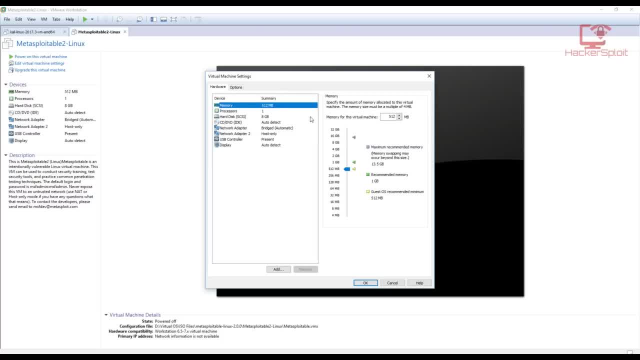 and you want to go into the memory Now? in my opinion, okay, you need. this is very important. If you're using Metasploitable 2 on your own, only one connecting to it, then you can change the RAM up to even 256 megabytes. But if you are, 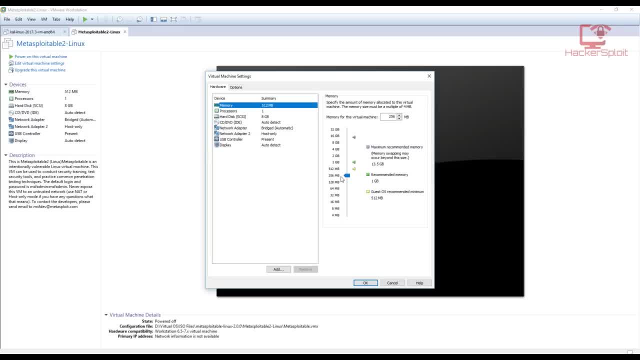 setting it up for your class. alright, and let's say you want your students or your friends to all try and use it at the same time. Remember, Metasploitable 2 here is acting as a server. Now servers, depending on the amount of requests and the amount of processes it is processing, will 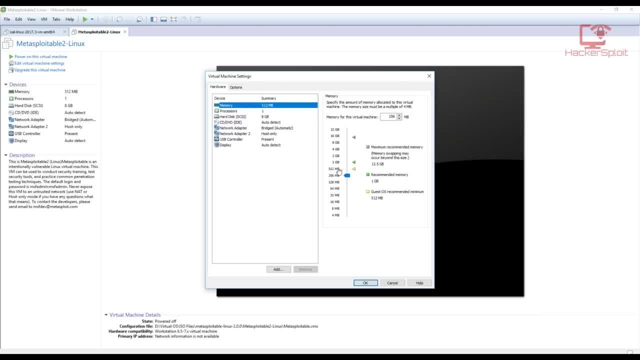 require more RAM. It's the it's like, for example- let me just use a stupid analogy- It's like Minecraft. Alright, Minecraft servers usually have about 8 to 16 gigabytes of RAM, And that's because they're processing or they're handling a lot of requests that are being sent by the players. Now, the more 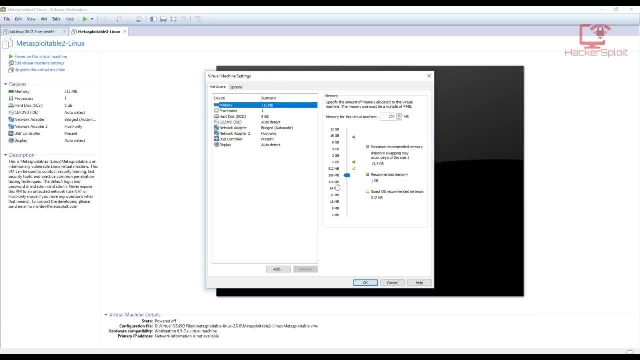 players you have, or the more users you have, the more RAM you'll need. So, again, feel free to change it to even 128 megabytes, Because, again, you're just going to. if you're the only one using it, you don't need a lot. And don't worry about the recommended settings Because, as you can see, 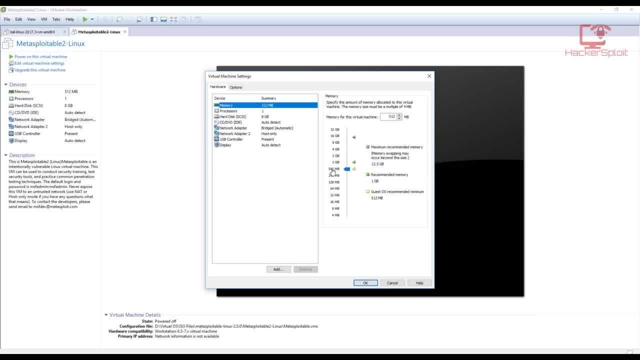 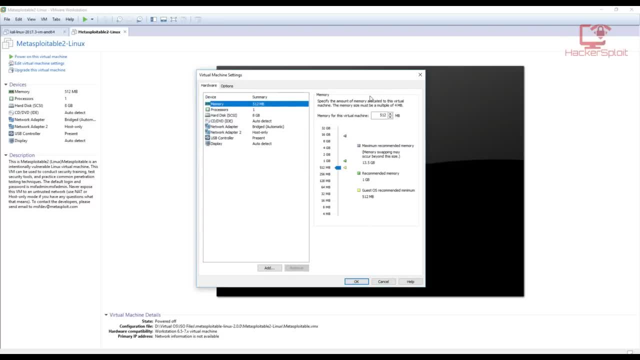 it's going to give you recommended suggestions dependent on your memory configuration. So I like leaving it at 512, because I'm usually testing it with a few other friends of mine And we're trying to do a few other settings with CTF. we're actually trying to create our own CTF website. 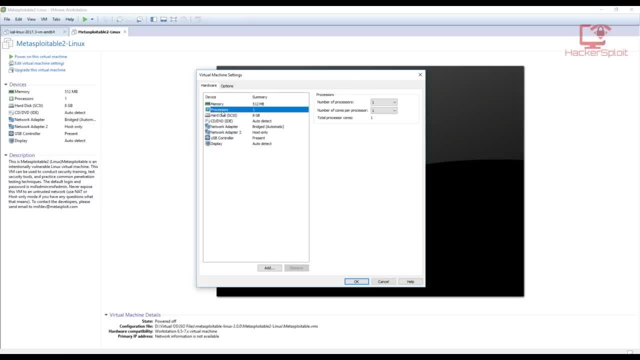 That's something I shouldn't have actually told you because I was keeping it in secret, But don't worry, that's coming out soon. As for the processor, I like keeping this to one: one processor and one core, so that it just uses one processor, Because, again, the process is very 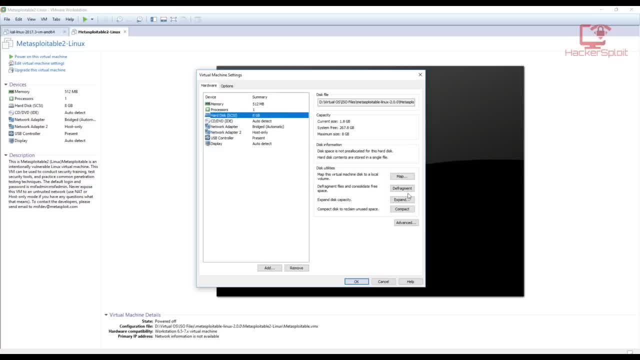 very minimal, Depending on what you're doing. The hard disk space is eight gigabytes. If you're installing your own files, you can expand them, And then you can do this in a few separate ways, So can expand it to what you want. now, as for the network adapter, make sure that it's bridged, and 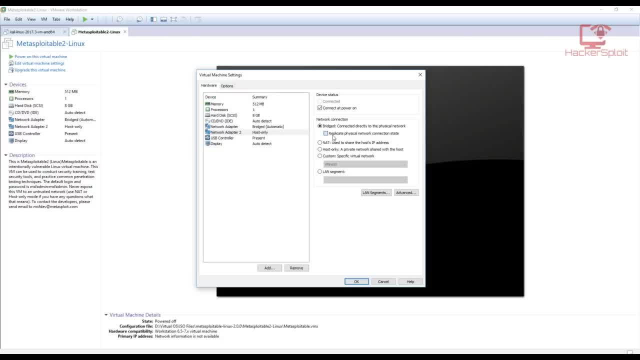 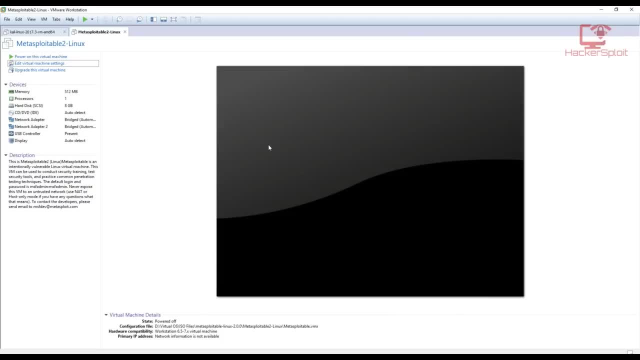 make sure that both options. if it prompts you for a dual network adapter configuration, make sure that they are both bridged right and once that's done you can just hit OK and you don't need to really use accelerated 3d graphics because metasploitable is a command line and lacks it. 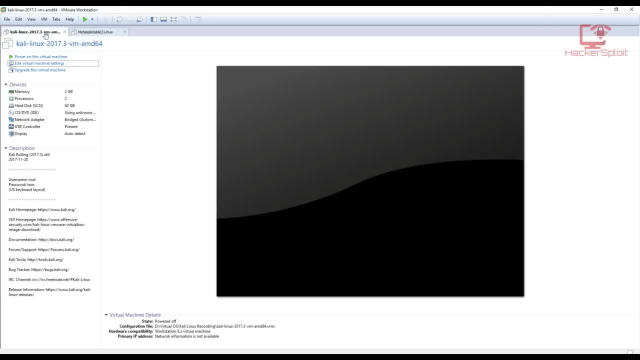 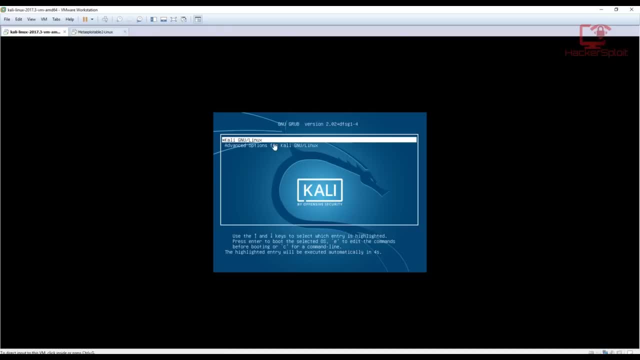 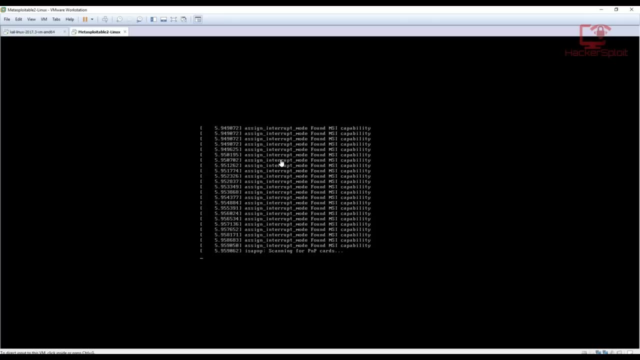 lacks a graphical user interface. okay, so, now that we have set up all our settings, now we can power on Kali Linux and we can also power on metasploitable too. okay, there we are, so it's prompted me to start up Kali Linux- excellent, and metasploitable is also starting. as I said, they do not have a. 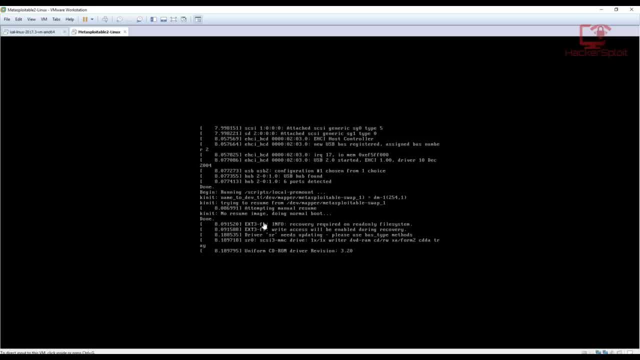 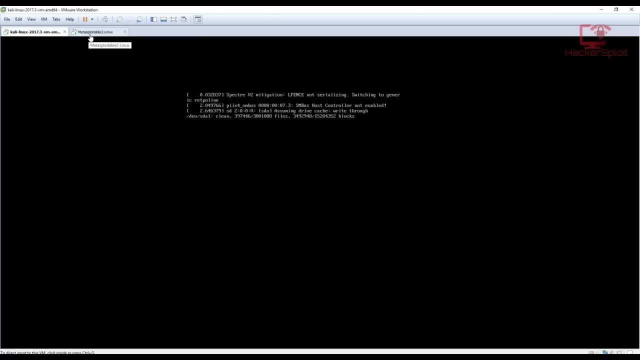 metasploitable 2 does not have a graphical user interface, so I'll show you how to log in and how to get your local adapter all right. so let calendar next start up there. it should be starting up anytime right now. there we are: metasploitable 2 has started up and it's starting the clock and the event managers that start up. 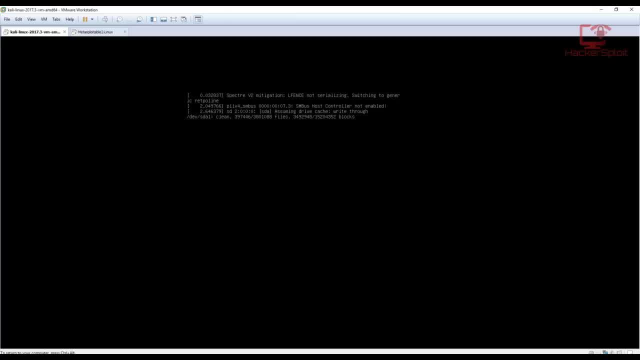 this is checking my disk. yeah, the storage device- yeah, storage device is clean and the blocks are also looking good, all right, so give it a few seconds to start up, and i think calil next should have started up by now. and there we are. let's just wait for them- both of them- to start up now. 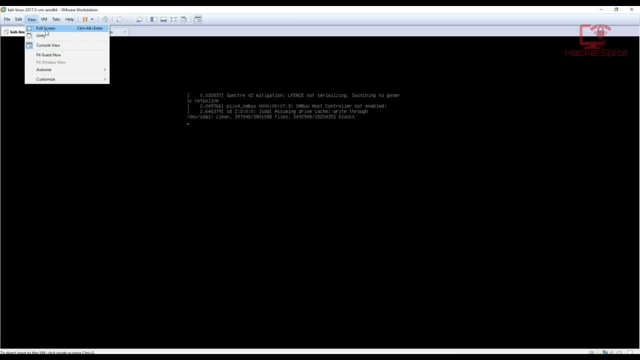 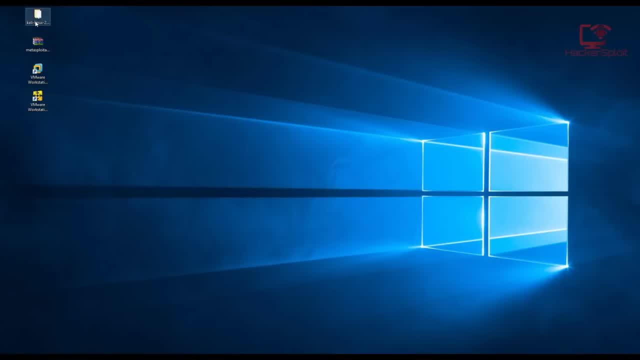 let me explain a few things. with virtual of vmware pro- uh, the great thing that i like is you can go into full screen mode immediately, and that's the also. another great thing is if you use the virtual machine file, the kali linux virtual machine file, it already has the vmware uh guest additions. 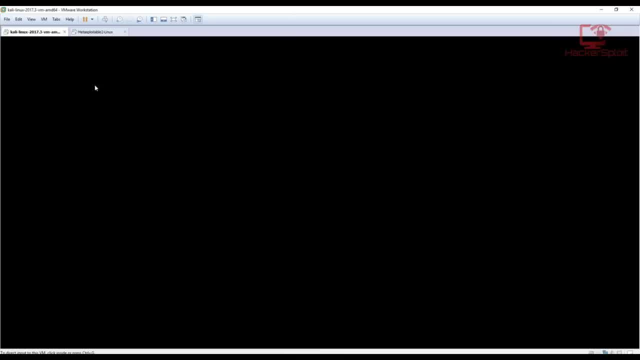 installed, so you don't have to install it. you're essentially, you're good to go and you can run it in full screen. and you can also do it in virtual machine mode and you can see that it's fully installed. so you don't have to install it. you're essentially, you're good to go and you can run it. 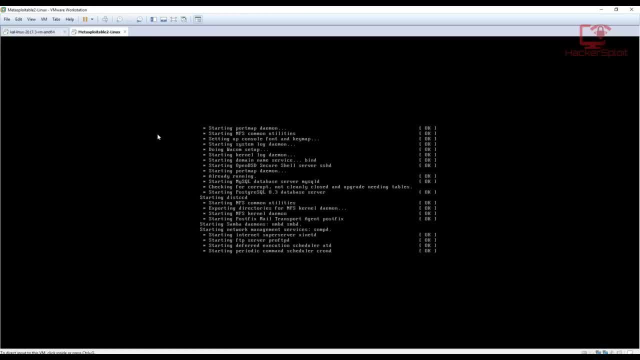 you know you can. it's well optimized. I am going to be making another video on how to configure VMware to work great with Kali Linux, because a lot of you guys have been telling me that it's slow, And I also had this problem And if and I sorted it out Okay. so I think Kali Linux should. 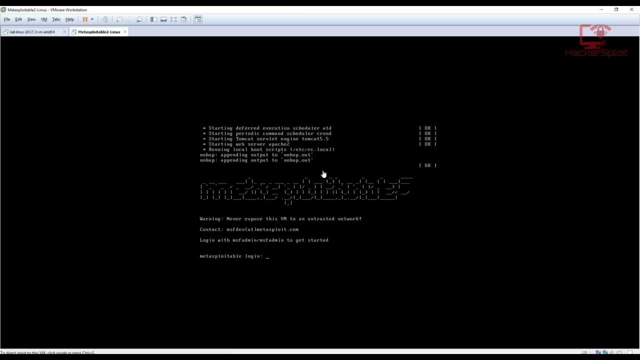 have started. you'll know that it started because you'll see the black mouse pointer there. Meta exploitable is started. So it's going to say here: never expose this virtual machine to an understated network. That's very, very true. Do not do that And you can log in with the MSF admin. 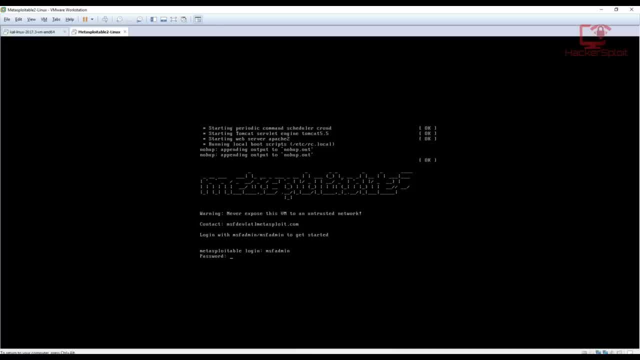 combo. Alright, so the username is MSF admin And the password is MSF admin. Whoops, sorry about that. There we are, And once we're logged in, it should tell you welcome. And there we are, As you. 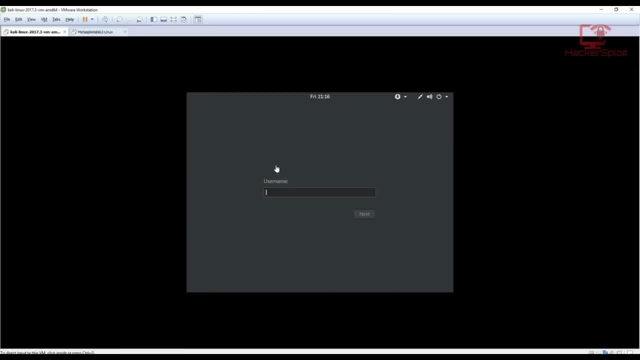 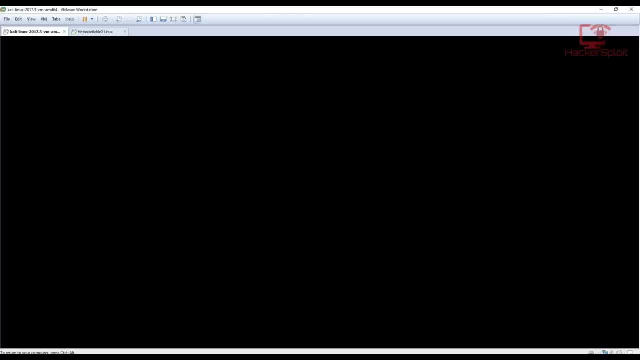 can see it is running on Ubuntu or Debian And let that just sit as it is. And there we are. we are in Kali Linux right now And the username is, as I said is, root And the password is Tor. Alright, now you can add your own username if. 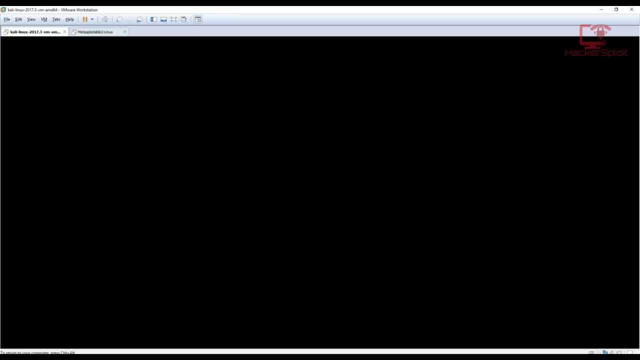 you want to, And essentially you have full control over the system. The default username and password is root and Tor. Alright, so give that a few seconds to start up And I'll go into full screen mode in a second. Let me just clear up metasploitable here. By the way, if, if you have, 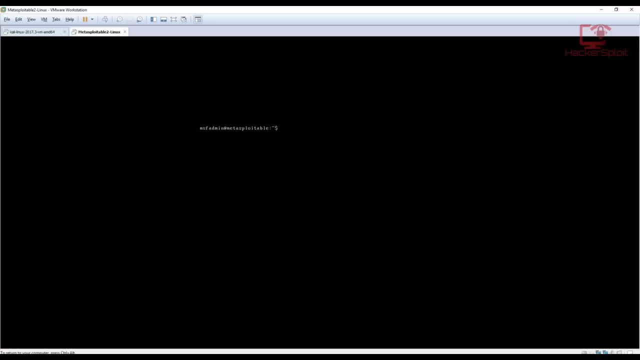 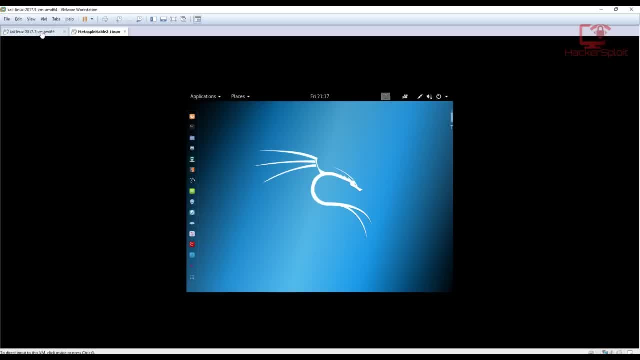 clicked in the virtual machine, you can see that my mouse point has disappeared. If you want to exit out of the virtual machine and go back to your host operating system, use the control plus Alt key and that will take you back there. Okay, so there we are. we have Kali Linux over here. 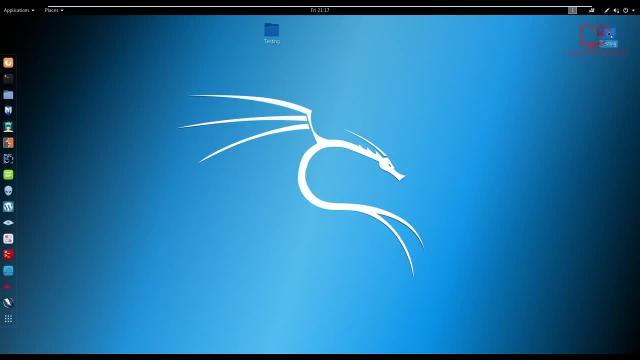 And now you can go into view and hit full screen and give it a few seconds to scale. Let me just move my folder back there And voila. Now again, if you're using Wi Fi, it should show up as wireless, a wireless. you should see a wireless adapter. it's going to be using the same bridged adapter. 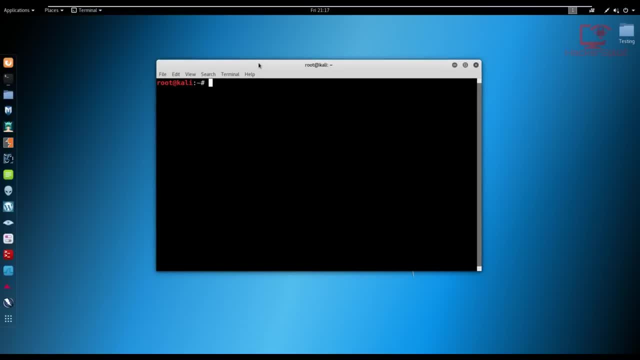 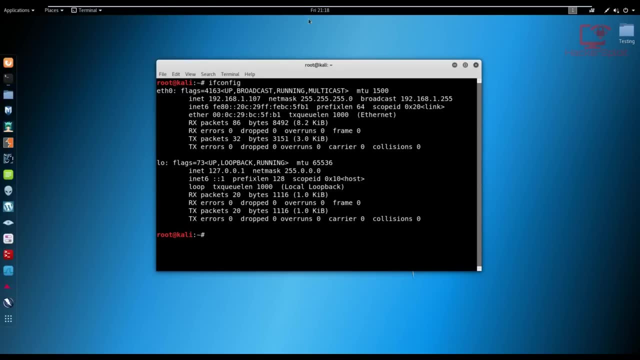 as your host operating system. So what we're going to do is I'm just going to hit if config here like so, And, as you can see, my local IP is 192.168.1.107.. Yours might be different. 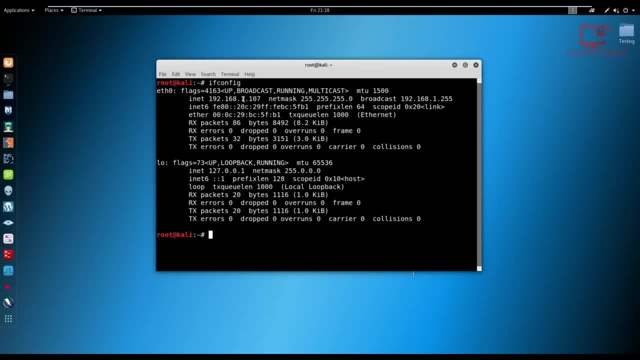 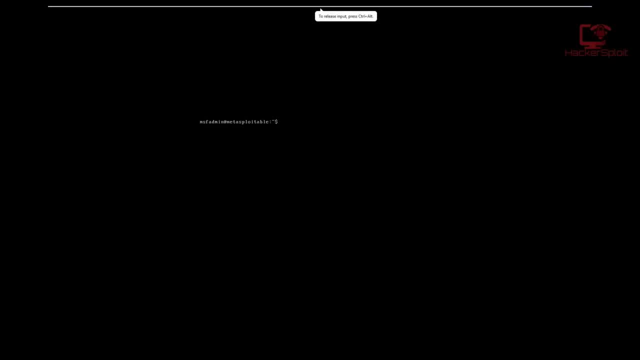 but you want to make sure that they are running under the same subnet. So the subnet will be 192.168.0, or one or two, depending on how many access points you have. Let's make sure they're on the same network. So I'm going to if config here, if config, And, as you can see, it's running. 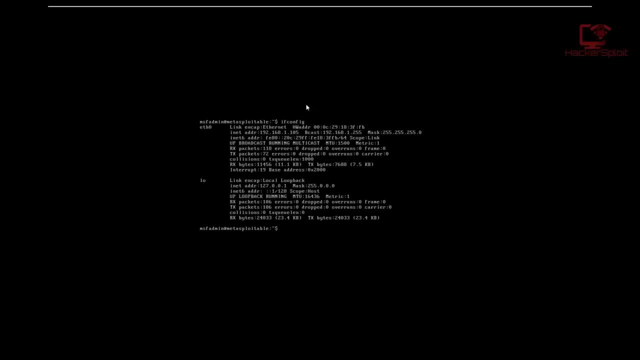 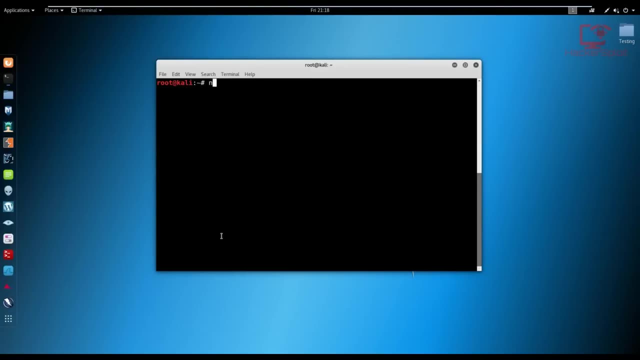 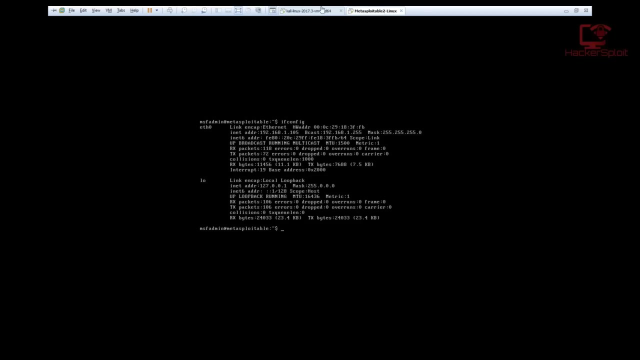 on the same network or the same subnet, which is 192.168.1.105.. You are, they can now communicate with each other. So, for example, if I said let me just run a simple whoops and map for 192.168.1 point, let me just check the IP here: 105.. Alright, so 105.. 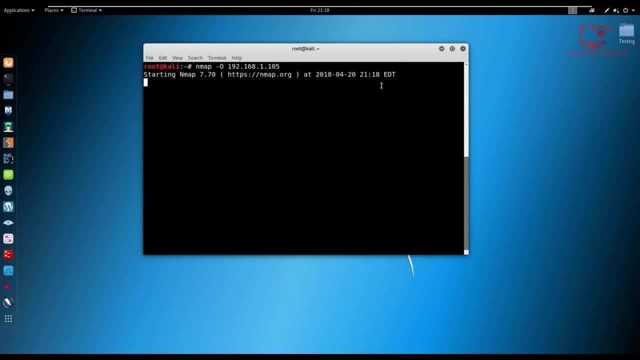 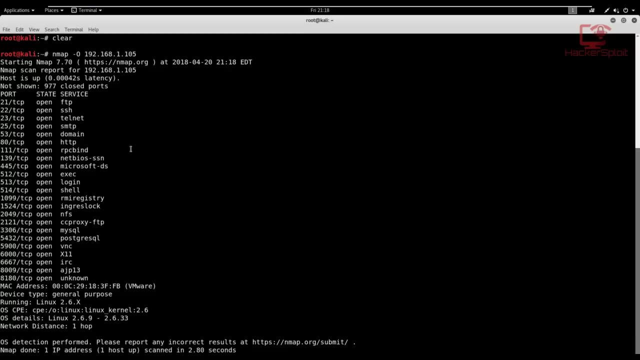 Oops, my bad 105. And I'm just gonna hit enter. Let's see what it is able to bring up. Let me expand that, as you can see, it's going to scan the Metis political to virtual machine And it's. 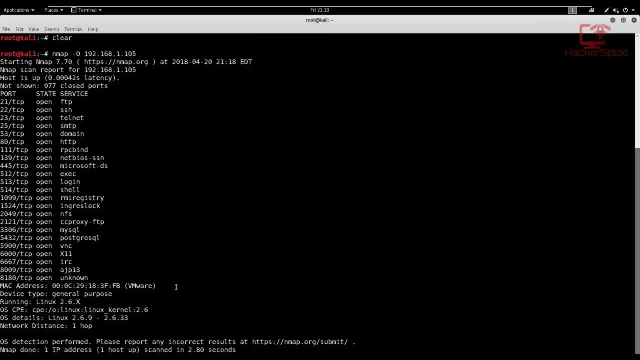 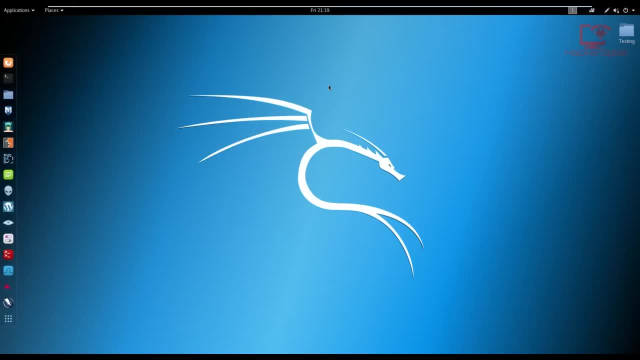 going to give me all this information. I essentially scanned for the operating system version. it's going to give you a MAC address, all that good stuff, And this is just a simple and map scan to show you that you can now work on your virtual machine. Alright, so that is. 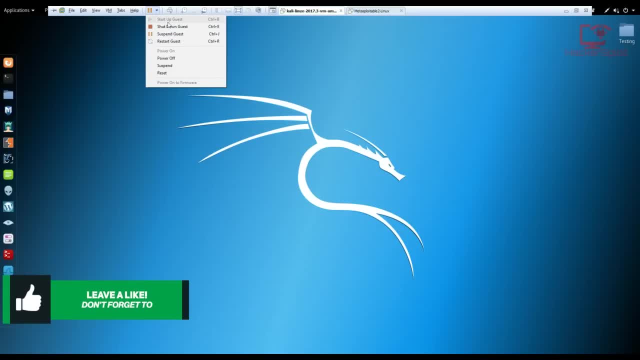 how to configure Kali Linux with Metis plateable two And again. the great features that I really like are that I can, you know, suspend the guest, I can take snapshots and you know, go back, go go forward if I have a mockup and you get the idea. Now. this video has been going on for a long. 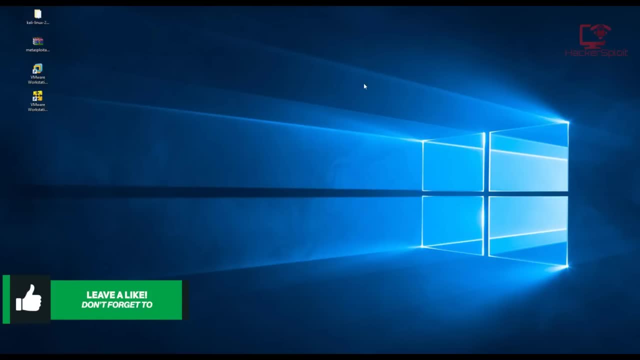 while now- And I'm going to end it right here by saying thank you, guys for all the support on the channel- A lot of you guys have been asking me for this video and how to show you how to configure your own virtual penetration testing lab. we're going. 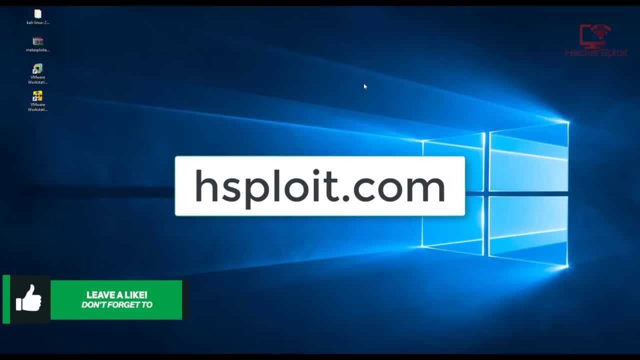 to be looking into CTFs in the future And I'm going to be continuing the web application penetration testing series. So that's going to be it for this video. I hope you enjoyed it or you found value in it. If you did, please leave a like down below. If you have any questions or suggestions, let me know. 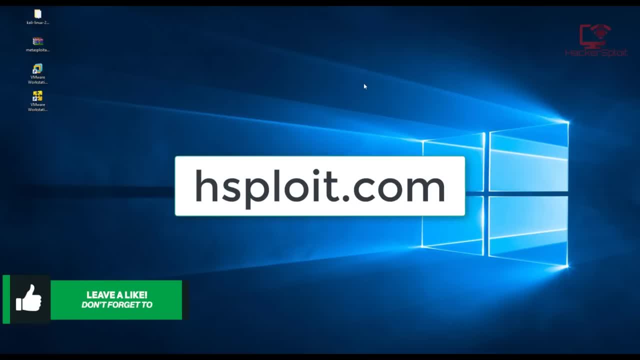 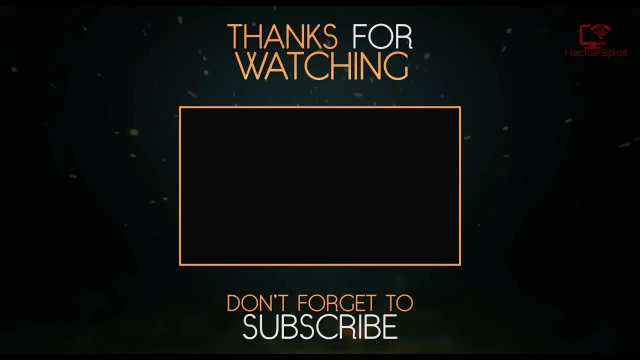 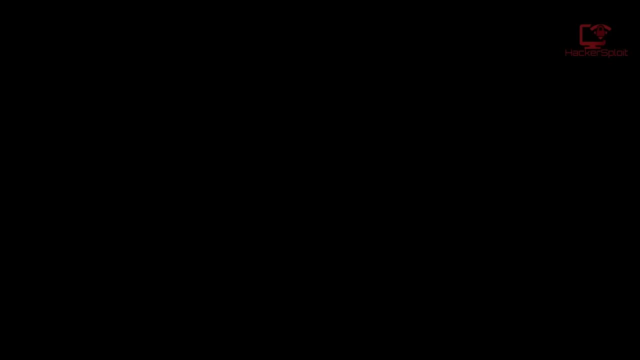 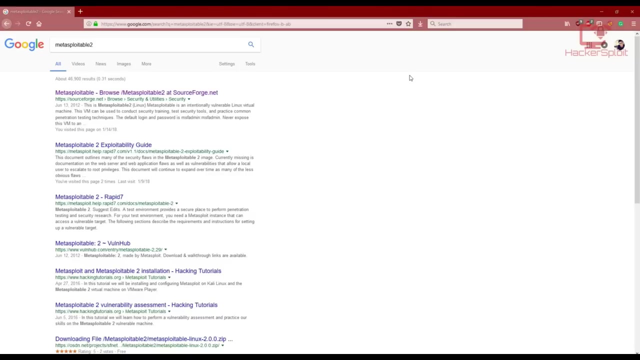 in the comment section or on my social networks, on my website, and I'll be seeing you in the next video. Hello everyone, and welcome to this lecture. In this lecture, we're going to be downloading and installing Metasploitable 2 on VMware- Alright, so let's get started Now. this is going to be very 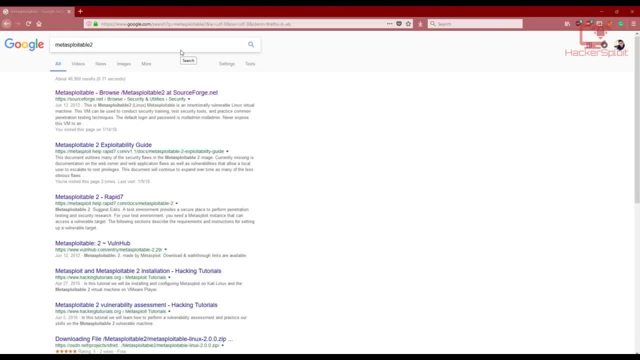 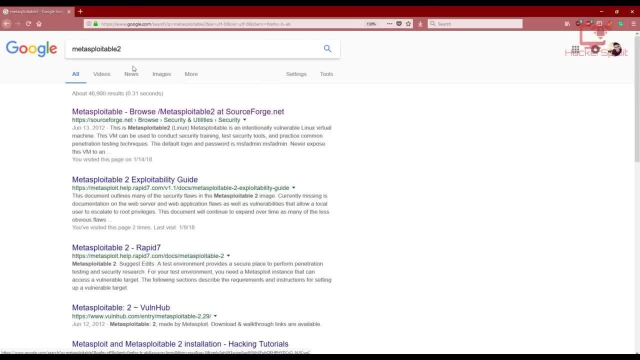 very important. So what I want you to do is just open up your browser and you can just do a quick Google search for Metasploitable 2.. Alright, so once you've Google searched that, as you can see, it's going to, it's going to give you some results. you want to make sure you. 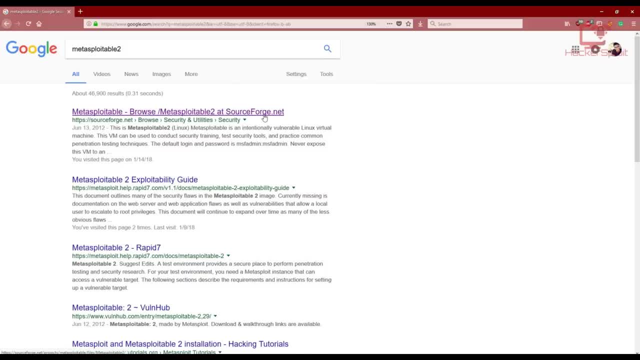 go to the sourceforgenet link. Alright, so it's going to be available at sourceforgenet. This is the best way to download it and get it on your computer. Alright, so click on the link And it's going to take you to sourceforgenet, And it's really very simple. What you want to do is just 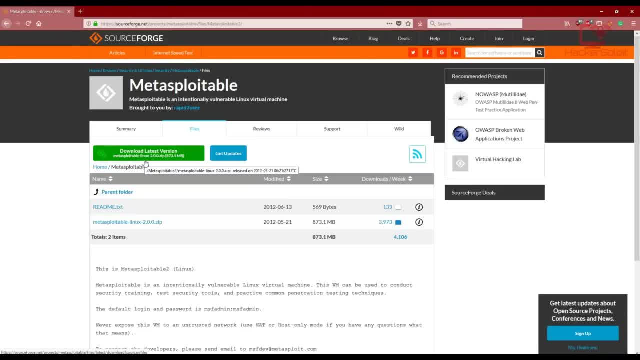 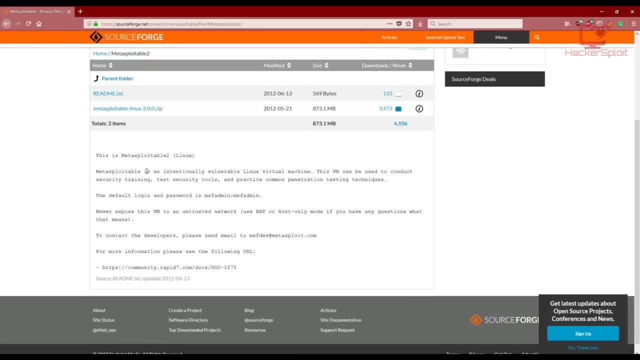 hit download the latest version, which is Metasploitable 2.. And you might be asking: well, what exactly is Metasploitable 2?? Well, what Metasploitable is? as you can see written right here, it is an intentionally 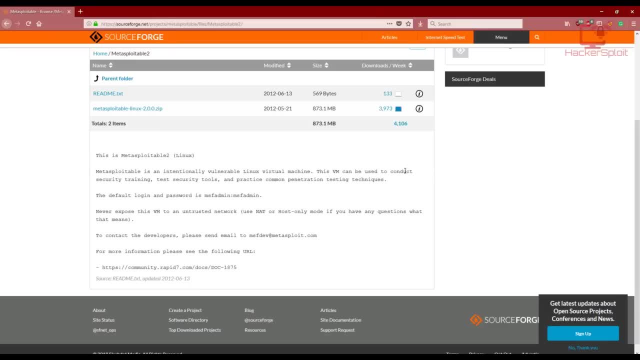 vulnerable Linux virtual machine. Alright, so this virtual machine can be used to conduct security training, test security tools and practice common penetration testing techniques- exactly what we're trying to do in this course. Alright, so why am I using Metasploitable 2?? Well, the reason I'm using 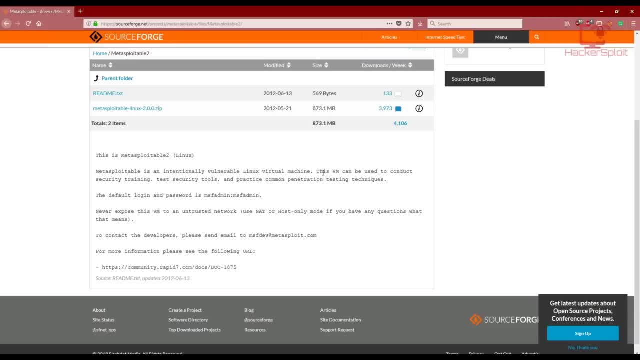 it is it best, emulates a target that is vulnerable And it will allow us to see the type of ports and the services that are running on these ports and how we can exploit them. But in this case, we're going to be looking at how we can, you know, scan a target for these ports and then, furthermore, 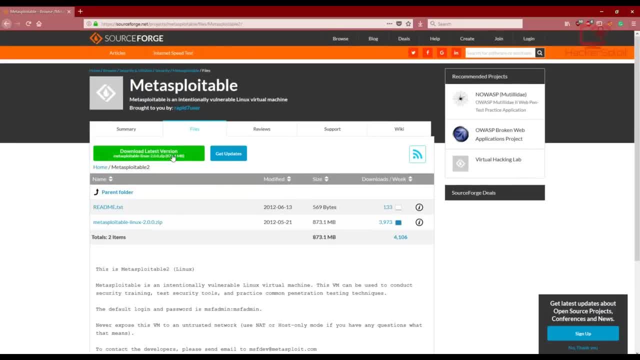 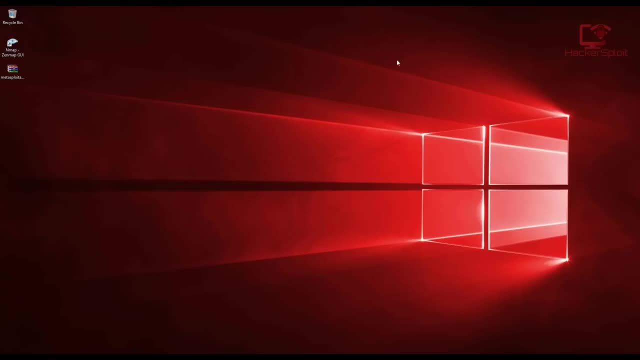 how you can exploit them. Alright. so what? it's really very simple. just hit download And it's about 873 megabytes. So it's a relatively large file, but just get it downloaded. It's a direct download And once you're done, I already have mine on my desktop And it's a zip file. 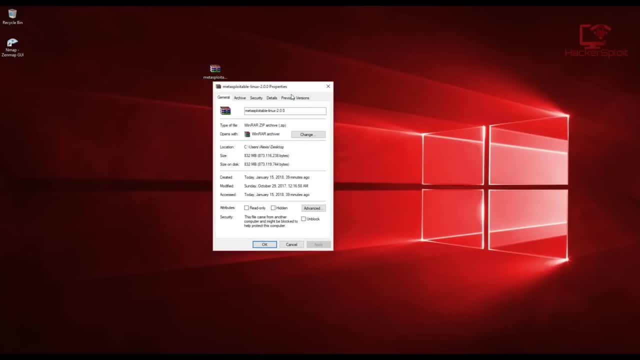 I believe- let me just check- the extension should be a zip file. Yes, it is a zip file. So the next step is to extract the zip file. Alright, so you can use your Windows extract tool Or, if you're on Linux, it's pretty much simple- just right click and extract it. 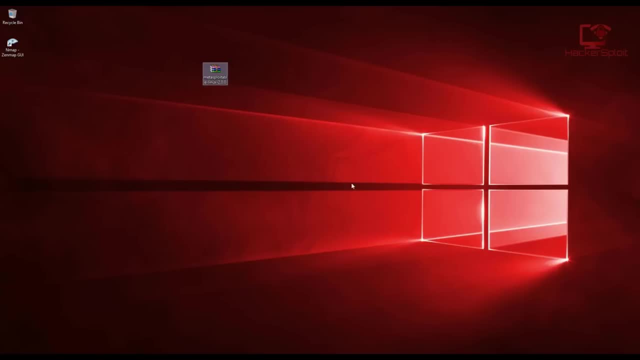 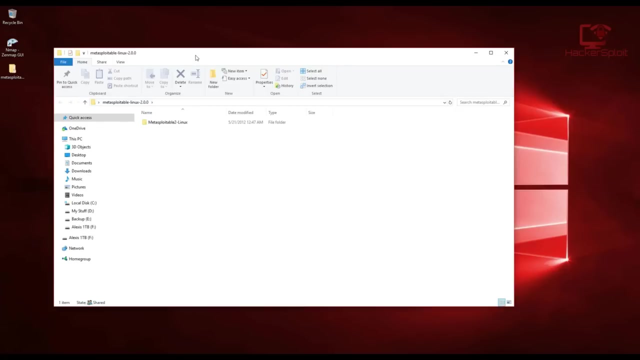 I'm on Windows. I'm going to be demonstrating this on Windows because I already have VMware installed. So there we are. it's going to start extracting it and just give it a few seconds, Alright, so once the file is extracted, it's going to give you this very cool looking folder. 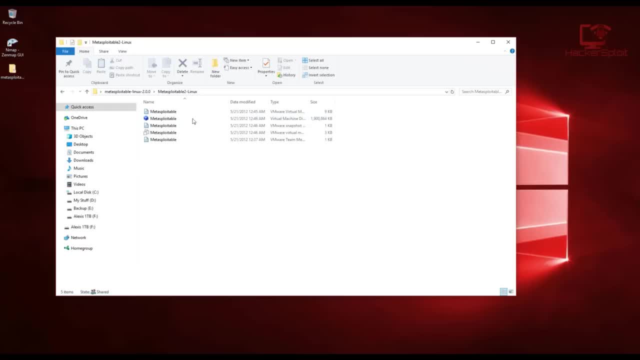 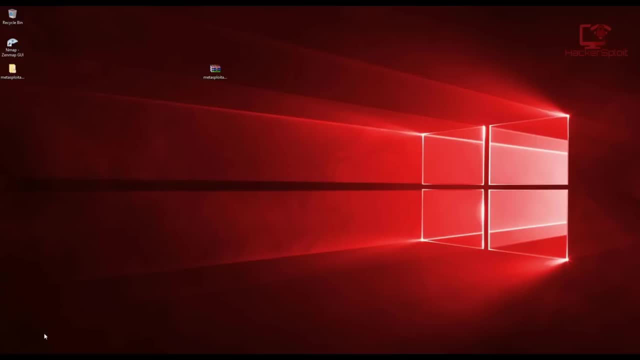 So once I open that up, it's going to give us another folder And inside there we have our VMware files. And, yeah, once you have all of these, we're ready to move to the next step. Alright, so now I want you to open up your VMware Player, which I already have here I do use. 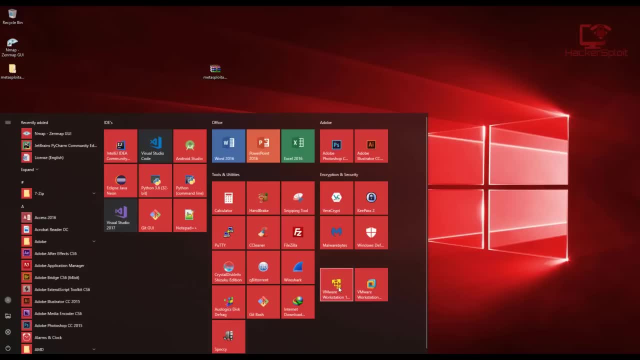 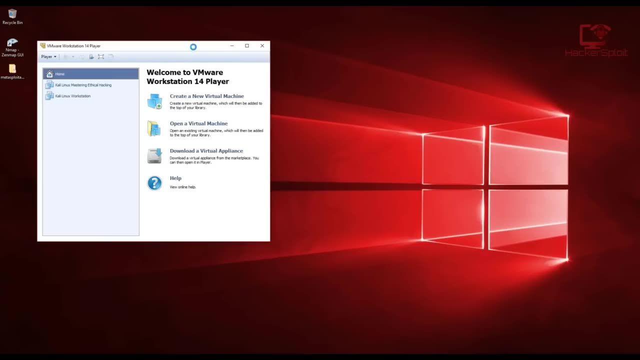 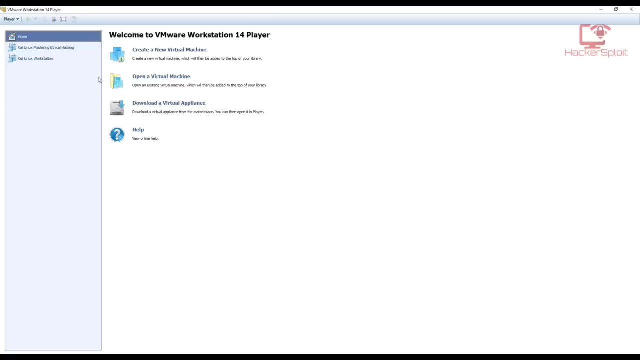 Workstation Pro, But for this demonstration we're going to stick with VMware Workstation Player, So just going to open it up. All right, give it a few seconds. There we are. Okay now, obviously you're not going to have any virtual machines like I do in here, So don't worry about that. 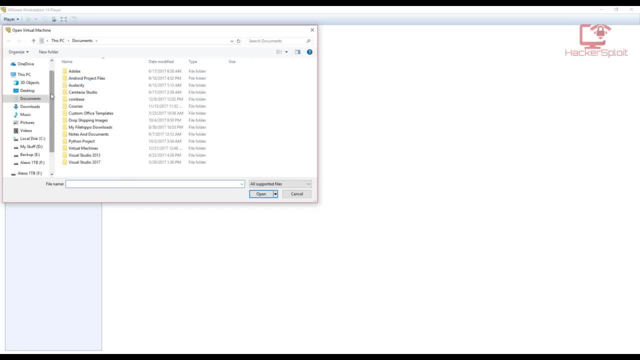 What you want to do is you want to go into open a virtual machine And it's going to prompt you to select your, your directory. So I'm using my desktop, that's where I have it saved. So I'm going to open up my Metasploitable 2 directory, the one we just extracted. 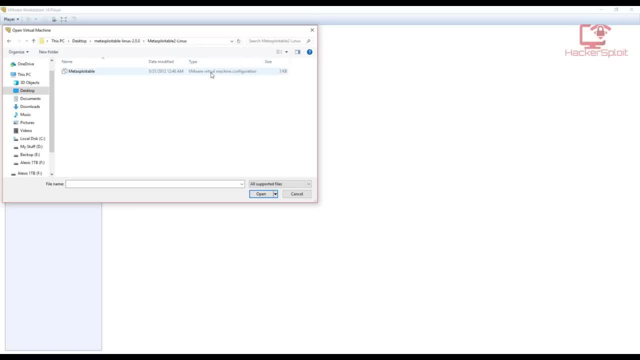 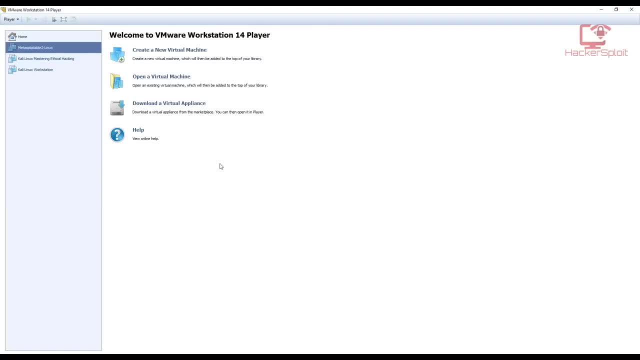 And I'm going to open that again. And you want to select the virtual, the virtual machine, VMware virtual machine configuration file? Alright, so it's going to only show this one. just open that up. Okay, give it a few seconds. There we are, And now we have a Metasploitable 2. 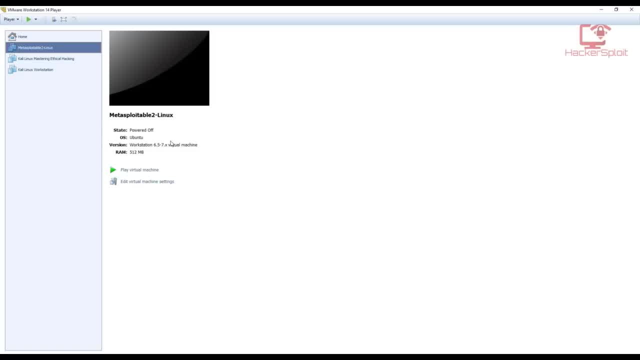 ready. But before we do that, we need to configure some of the physical resources that we're going to allocate to the virtual machine. Okay, so we want to edit the virtual machine settings. Right, And now here you can specify how much RAM or memory you want to, you want to provide to the virtual 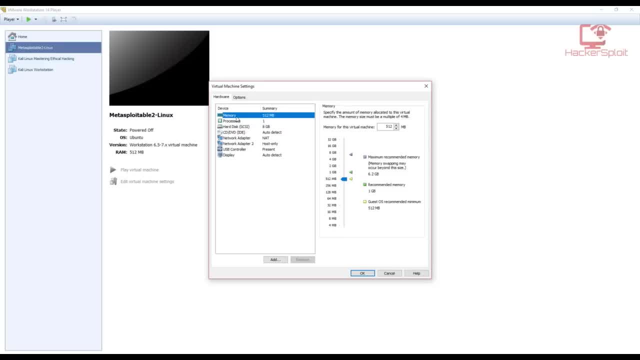 machine, how many processes you want the virtual machine to have. what I would recommend is just leaving in the at what, at what it comes set with. So it's going to use 512 megabytes of RAM, which is, you know, pretty reasonable Again if you have a system with lower, with lower resources. 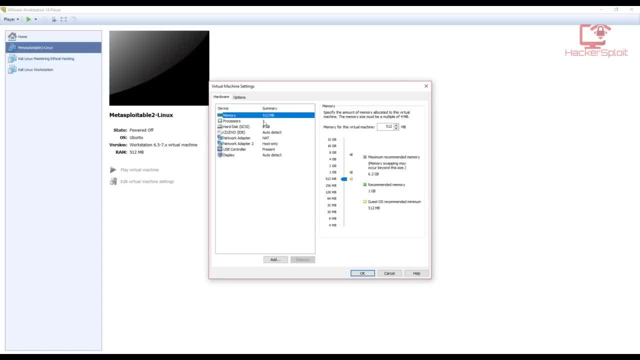 in terms of RAM, you can reduce that to meet your your current configuration. As for processes, you you can select the amount of processor calls you want to dedicate to the virtual machine. Since this is essentially a Linux server, I'll just leave it at what it recommends. And now you. 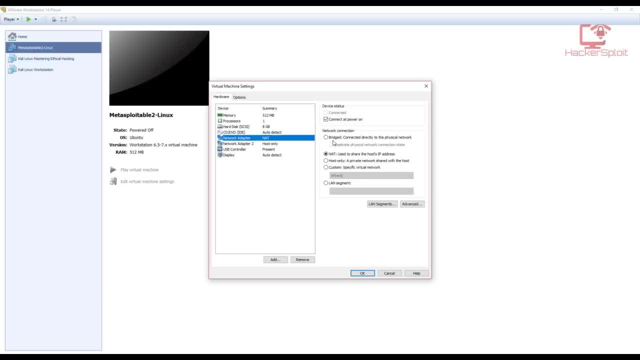 want to go to network adapter. Alright, so you want to. we want to bridge the, the connection, And that's because we want to connect it to our, to the current network that we're going to be using. So that means we want to make sure that we can all connect with each other and your virtual machine. 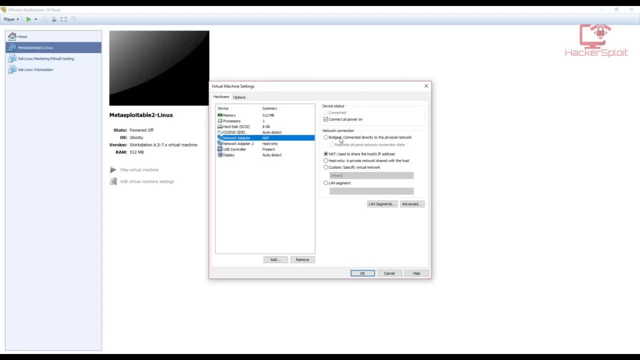 or your host or PC. So that means we want to make sure that we can all connect with each other and your virtual machine or your host or PC operating system can connect with your virtual machine, And we'll be seeing that in a few seconds. Okay, so I'm just gonna hit bridged And I want to say: replicate physical network connection. 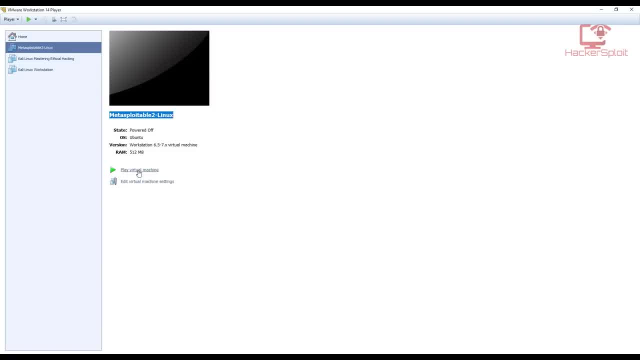 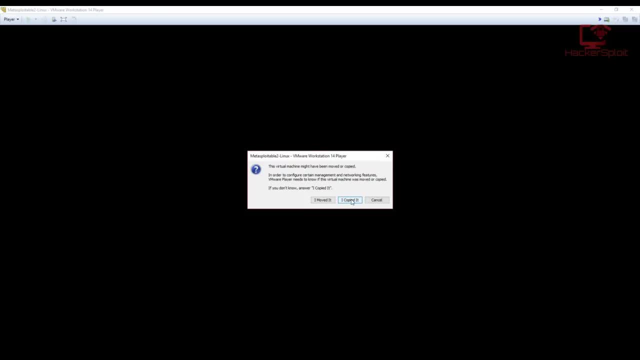 state and hit OK, Alright, now we are ready to launch. So I'm just going to hit play virtual machine And it's going to start up the virtual machine. If it gives you this prompt, just click on. I copied it. Okay, And it's going to start up the virtual machine. There, we are All right, it's. 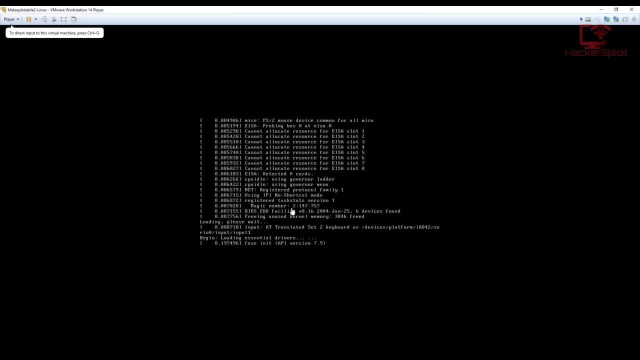 going to start up the grub bootloader. There we are: Fantastic, Everything's loading up as expected. All right, All right, we can now get started. So once Metasploitables 2 starts, it's going to give you this login screen and you might be a bit confused, but don't worry, the credentials are. 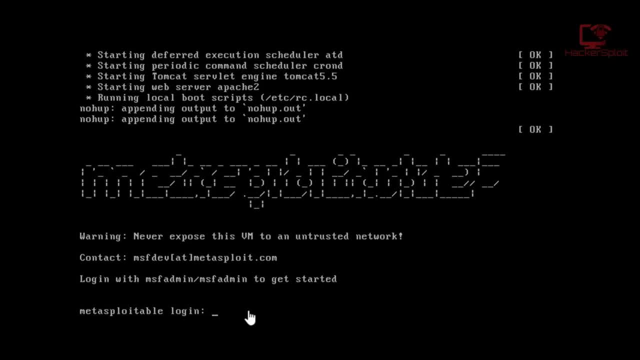 msfadmin for the login or the username, And so with the password, as you can see right here, it'll tell you that msfadmin admin for the username and msfadmin for the password. So let me just enter that in. 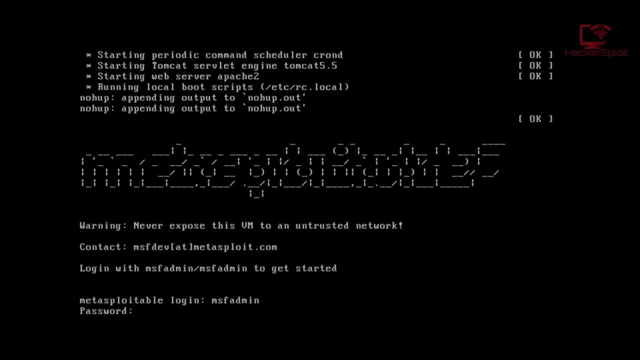 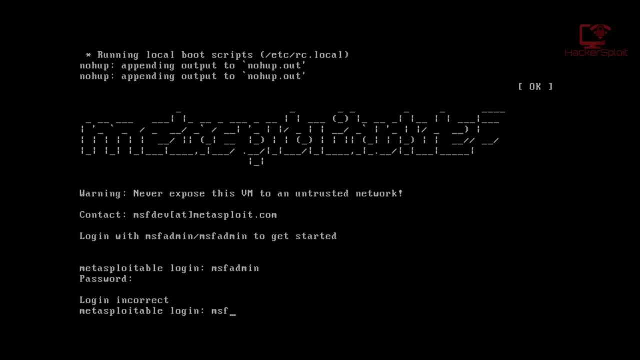 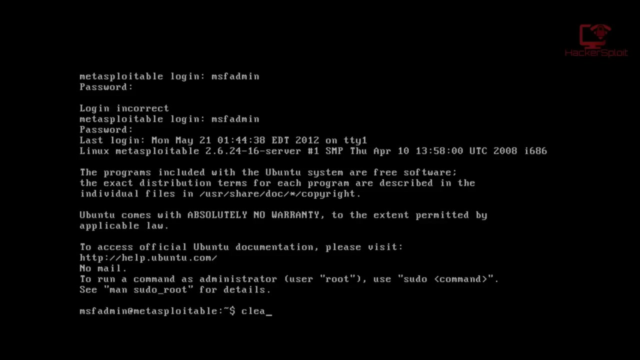 msfadmin. And for the password, the same thing. Whoops, I think, enter the password incorrectly. Let me just there, we are All right. So there, we are Fantastic, All right. So we've successfully logged into Metasploitable 2. And you can again. since it's a Linux server, you can. 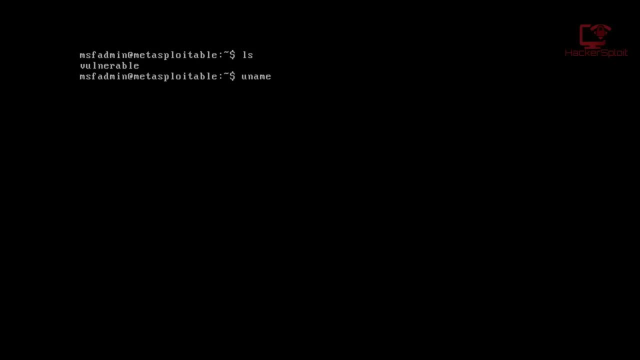 run some of the Linux, Linux commands. So let me just check, perform some commands here. So you name a whoops, There we are and, as you can see, Linux Metasploitable 2, it is the. it is. it is a Linux server. So again now to test that everything's working, what we can do. 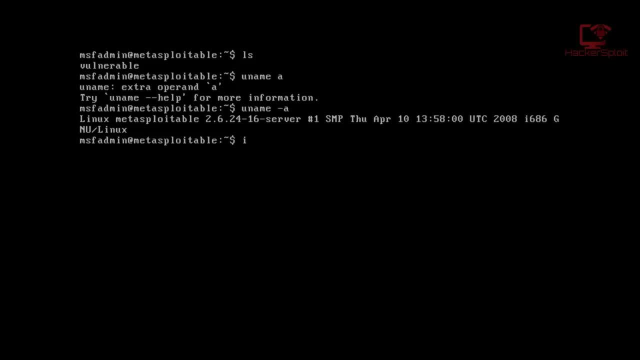 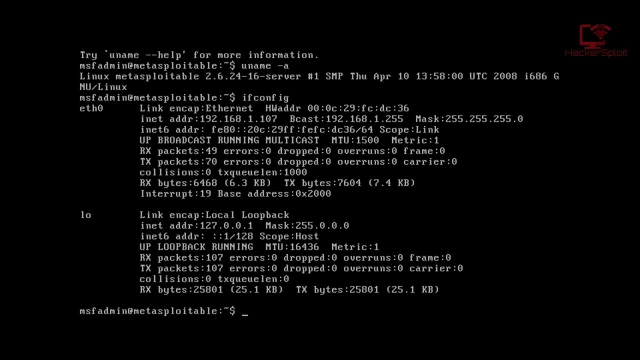 is, we can check the local IP address. All right, so let me just do that right now. We can check for the local IP address on the network for our Metasploitable 2 virtualまた machine. And there we are, we have actually got it. So I'm using Ethernet and the the address is: 192.168.1.107.. Yours will or might be different, depending on the router and your network range that you currently have. Okay so 192.168.1.107.. Very interesting. Now, how about we actually perform a test to see whether we can actually detect some of the ports running on this Linux? 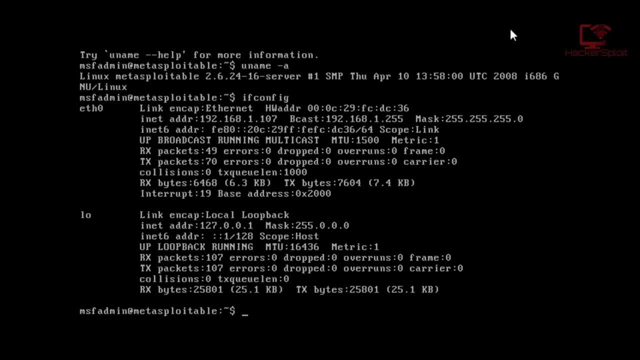 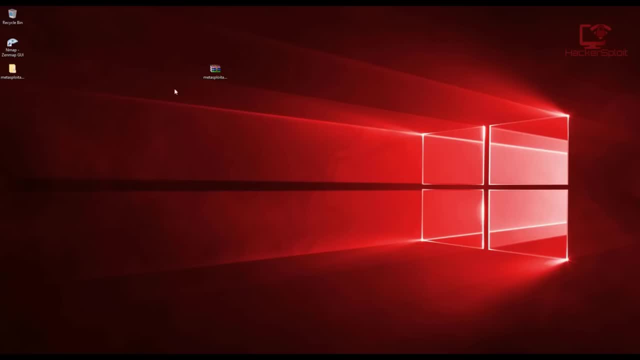 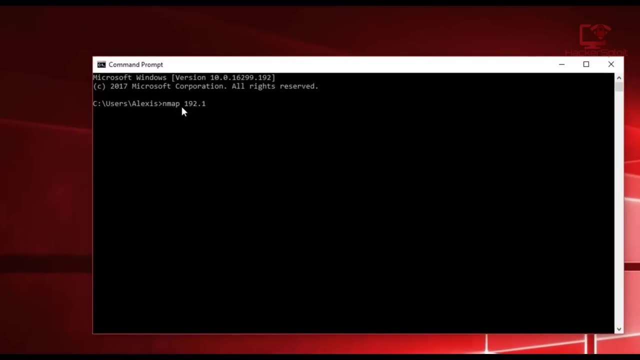 server or the Metasploitable tool using nmap. All right, let's try that. So what I'm going to do, I'm going to do this on Windows, So let me just minimize the virtual machine there. I'm going to open up my command prompt- really very simple- And I'm going to hit nmap 192.168. 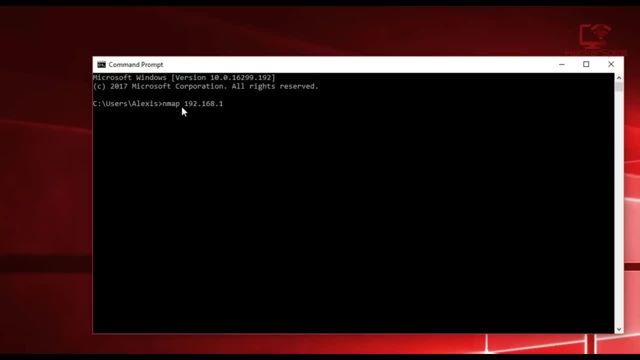 All right, I'm going to enter the IP address for the Metasploitable to virtual machine: 192.168.1.107.. And I'm going to hit enter And let's see what results we can get from the nmap scan. 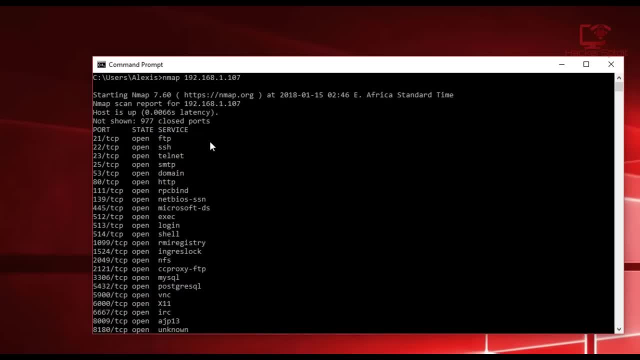 All right, fantastic, We're getting there. we are, we put, we successfully started the scan and we got a scan report. And this is why I was recommending that we use Metasploitable. two is because it contains all the useful ports And, since they're open, we can actually get an idea. 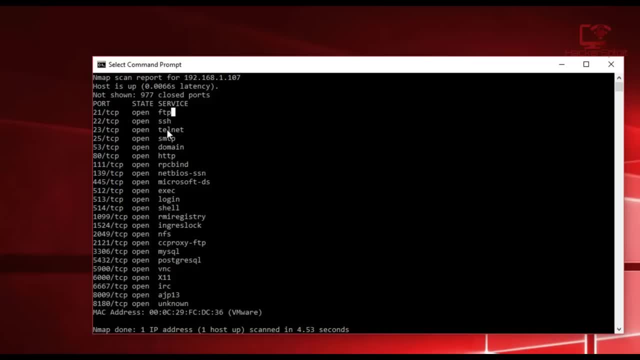 of what, the services that are running on them And, as you can see, it's detected all the posts that are currently running on them And, as you can see, it's detected all the ports that are currently running on them And, as you can see, it's detected all the ports that are currently. 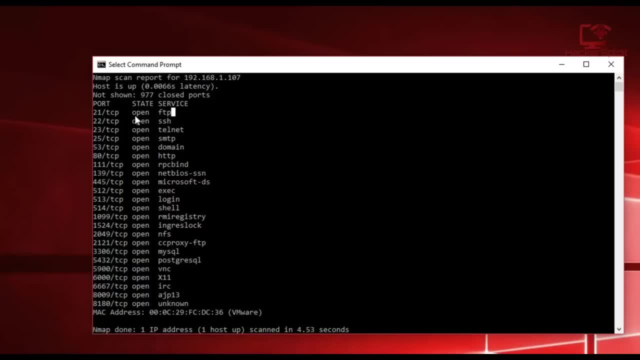 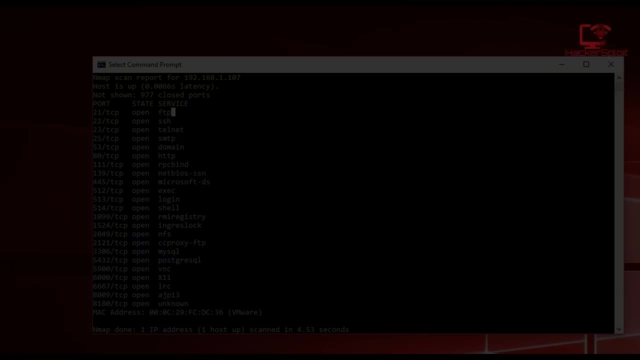 open and the services that are currently running on them. So we have our, we have our FTP port, our telnet port, we have our shell port, our MySQL database port, our PostgreSQL port, etc. etc. So that's going to be it for this lecture, All right, and I'll be seeing you in. 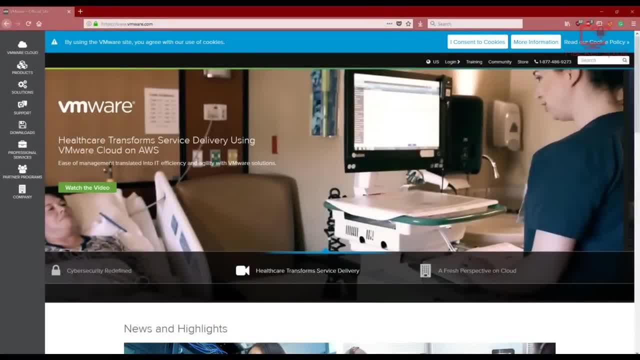 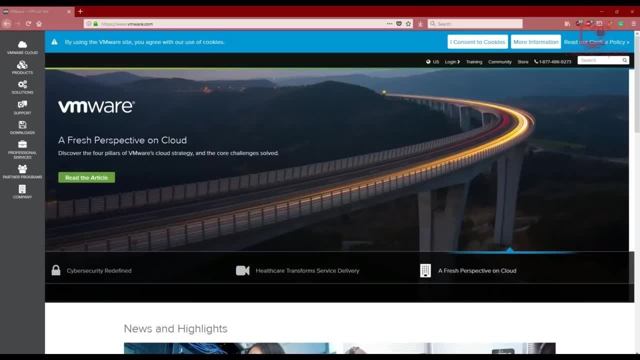 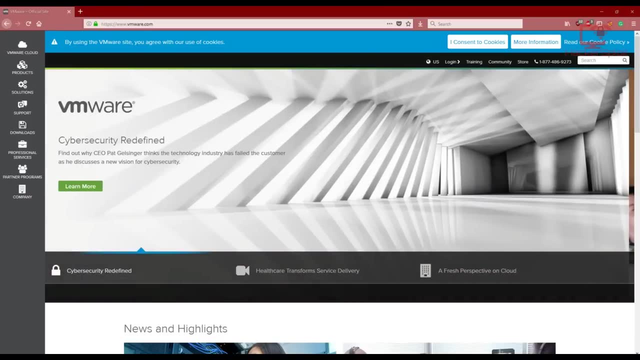 the next lecture. Hello everyone and welcome to this lecture. In this lecture we're going to be installing VMware, Alright, so that is going to be our virtualization software for the course, And that is depending on whether or not you're going to use Metasploitable two as your target. 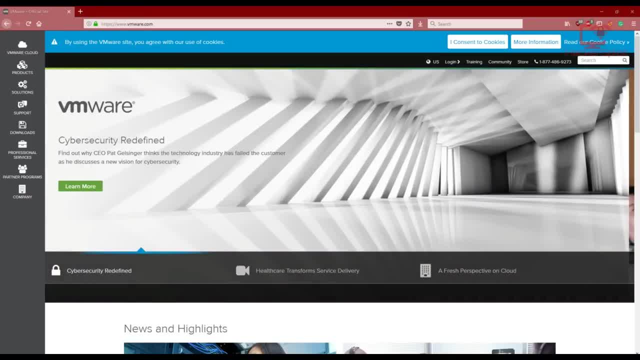 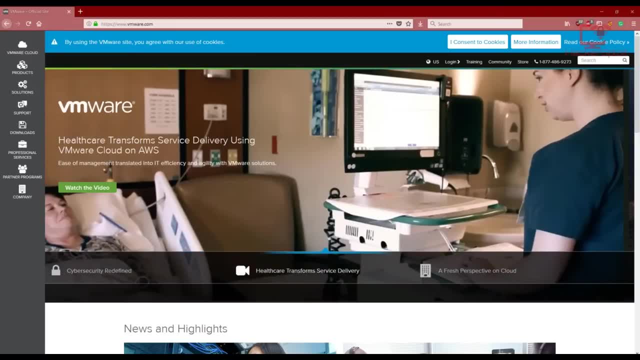 operating system for the purpose of the course. Now, if you do choose to go your own route and configure your own server for testing or your own network range for testing, by all means go ahead and do so. But if you're a beginner, I would really recommend that you go ahead and 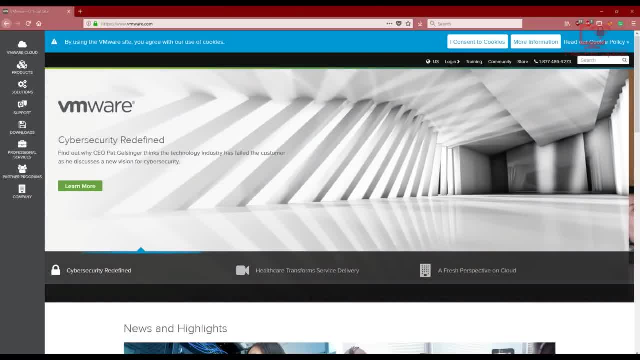 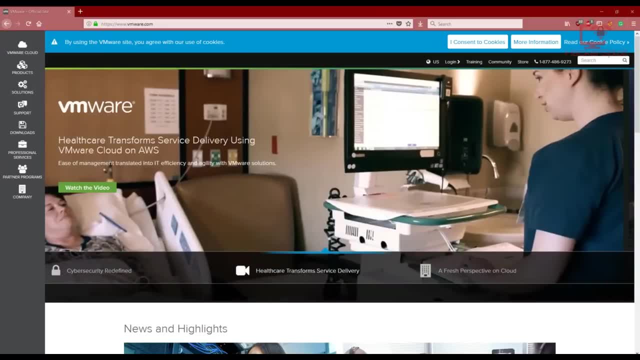 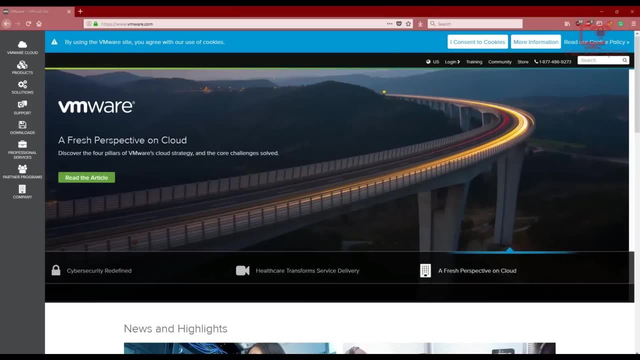 follow what I do and use a vulnerable operating system a of an operating system that is designed to be vulnerable, which is the Metasploitable two, And you can learn a lot about targets and how to scan for specific vulnerabilities or how to scan for ports, And there's a lot that we're going. 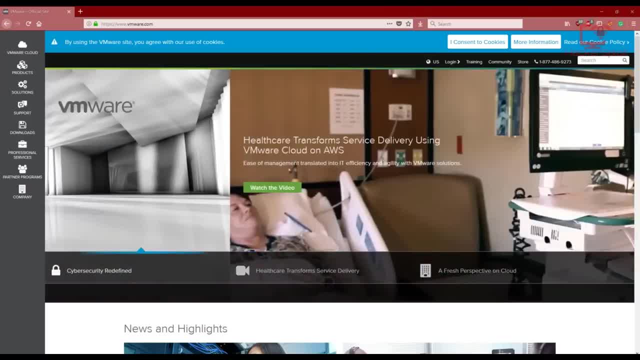 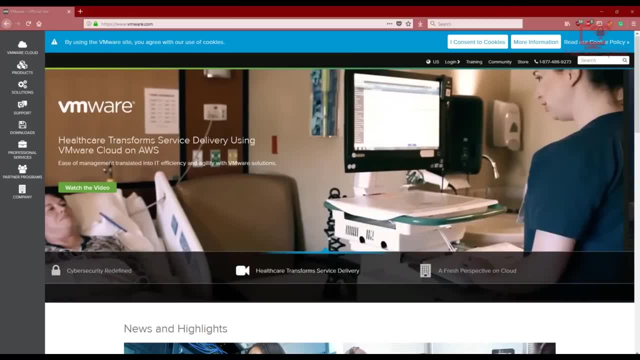 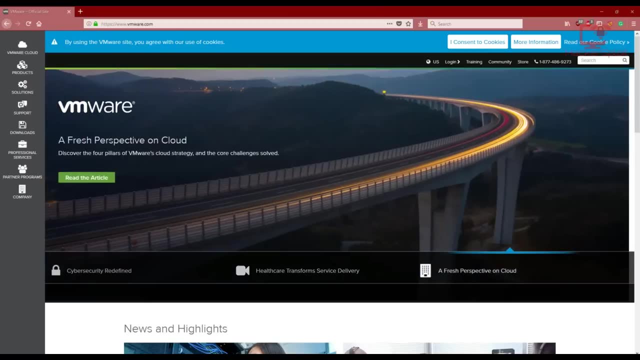 to be covering. Okay, so again, why am I saying: use VMware and not other virtualization softwares like VirtualBox? The reason is is because Metasploitable two works on VMware. All right, is, I'm going to go ahead and go ahead and do a little bit of a quick test. So if you're a beginner, 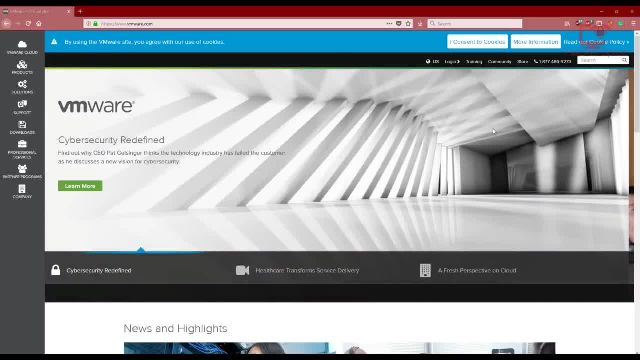 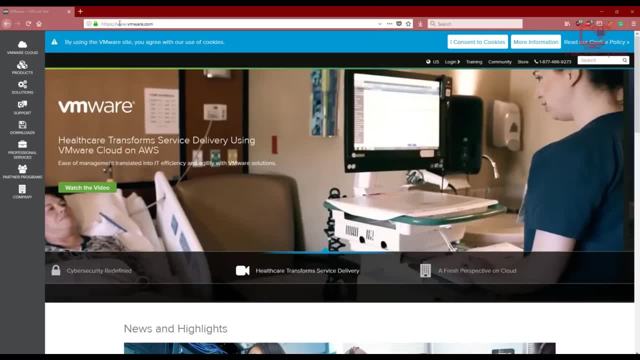 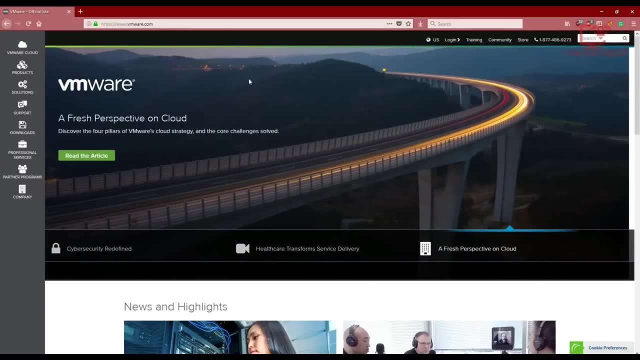 you're going to be using a virtual machine called Vmware And I'm going to be using the virtual machine called Vmware, And it's really much better to use VMware than VirtualBox. That is my personal opinion. Okay, So if you're using Windows or Linux, then then you can just go. 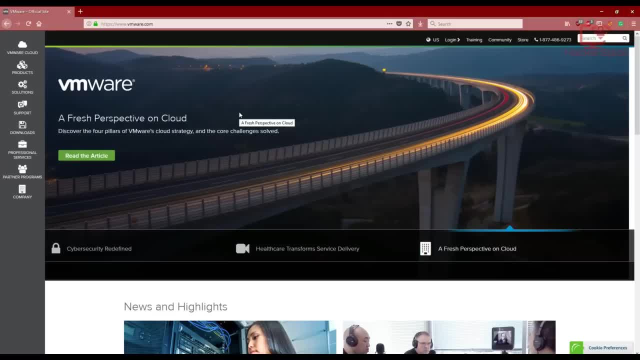 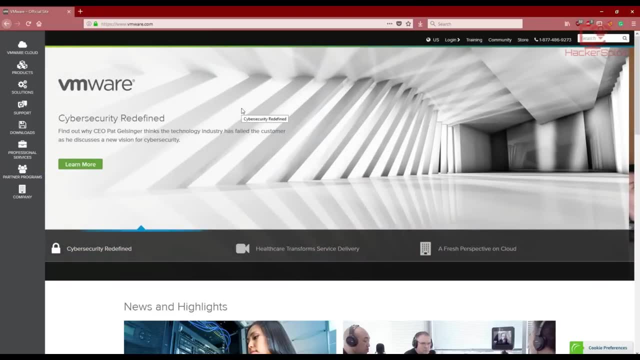 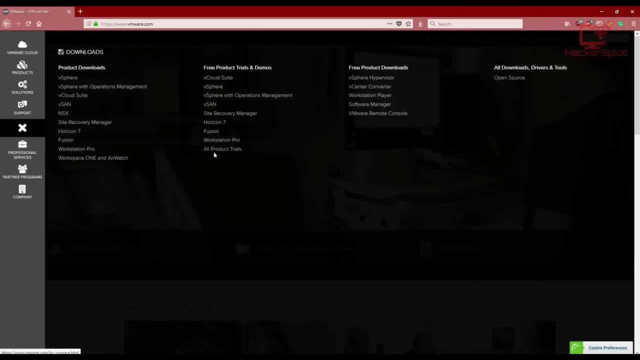 directly to the VMware pagecom, which is wwwvmwarecom. All right, and let me just consent to cookies there that we can get it installed. Okay, now, selecting the correct version is very, very important. Why do I say this? Well, there are two main reasons why I say this, And that's because a lot of people 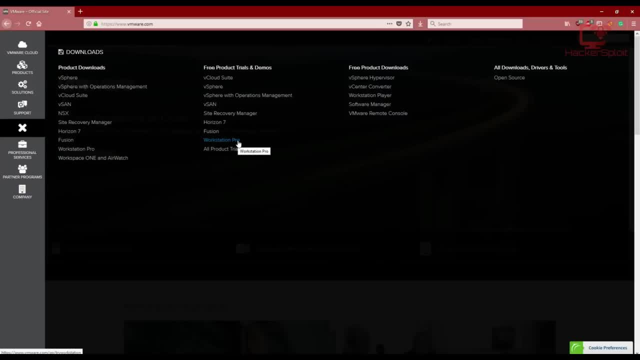 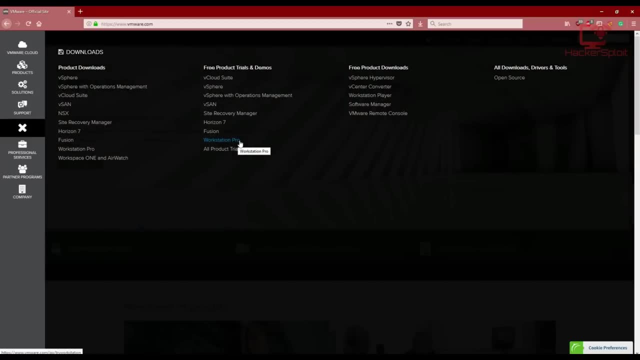 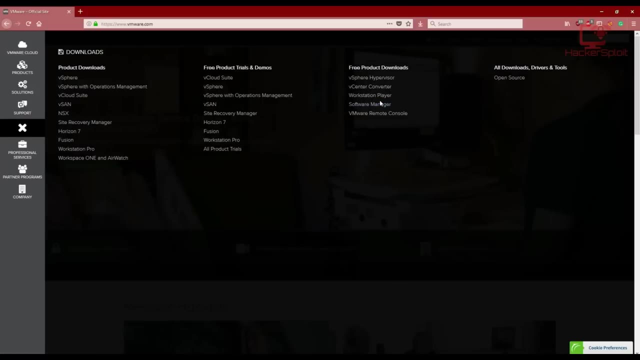 usually like to go with workstation pro right without noticing or realizing that it is a subscription or a license based software, which means that you have to pay for the license to use it. Okay, so VMware does offer the free version, which is workstation player, which I do recommend. 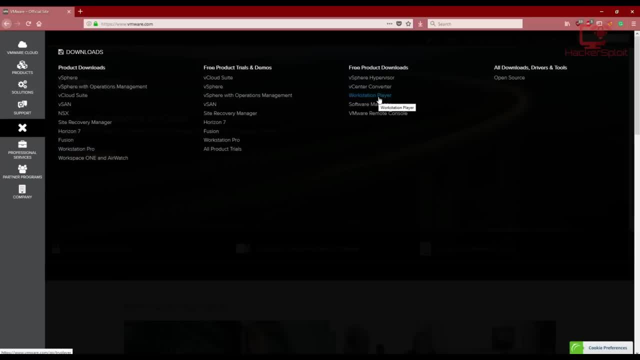 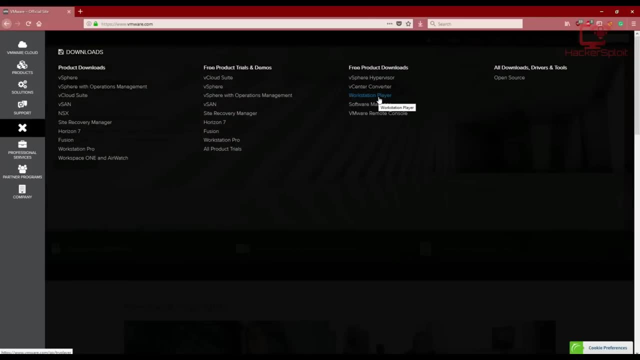 if you're just getting started with virtualization. Okay, you know, when you're learning about virtualization, it's very important to go with the basics and then move your way up. So again, workstation pro is probably directed at people who are using virtual machines a lot. 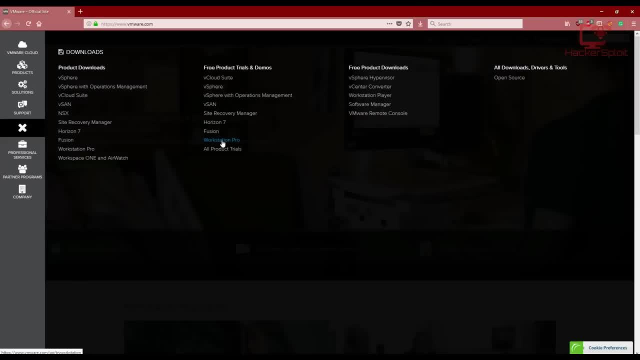 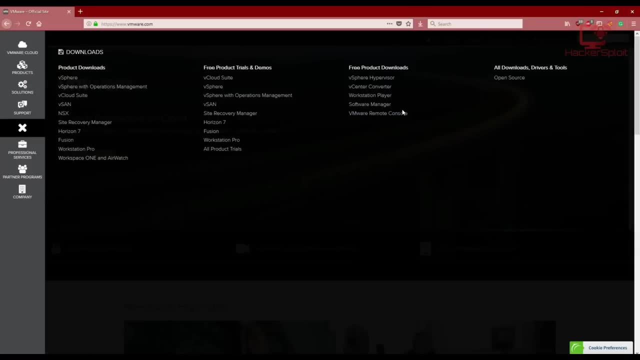 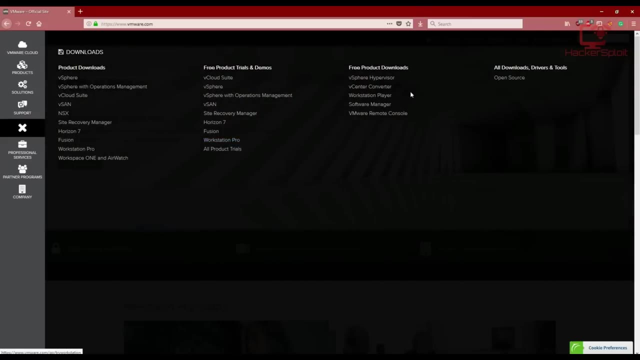 and probably you know using them more than I would say doing anything else. So, again, I would recommend going with workstation player, But if you're already experienced with virtualization and you want to try the workstation pro, by all means go ahead. So, going back to workstation player, just click. 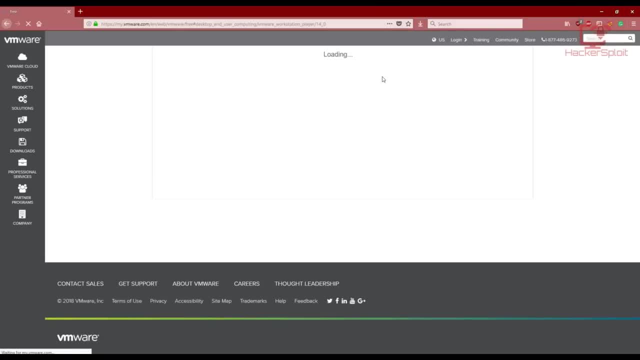 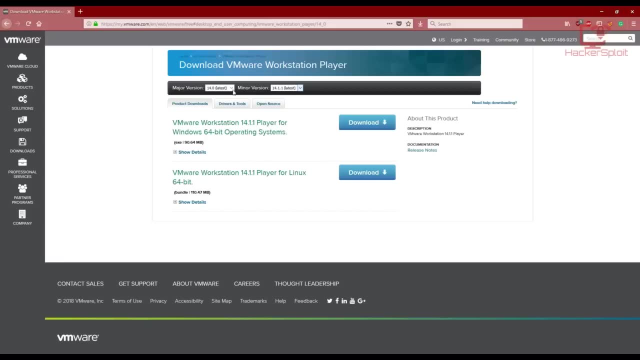 on it. as you can see, it's under free product downloads. you'll be able to use it as long as you want without any issues, Alright, so once we clicked on it and it'll take you to this download page, And the download page is going to offer you a few options, So you have your, your download for. 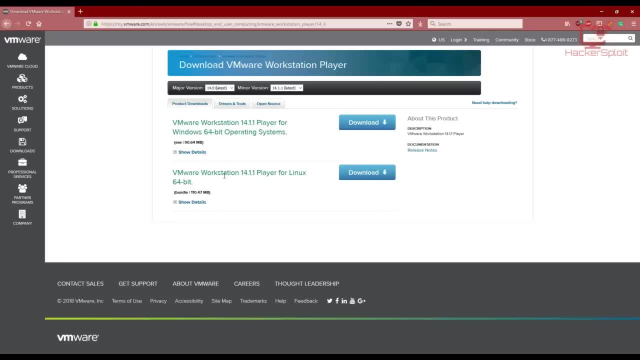 your Windows 64. bit operating systems and your you have your workstation we workstation player for Linux So you can go ahead and download that. links are here And it's about 90.6 megabytes and 104 Linux. So don't worry about that, just go ahead and hit download And it's a really simple setup. I'm not. 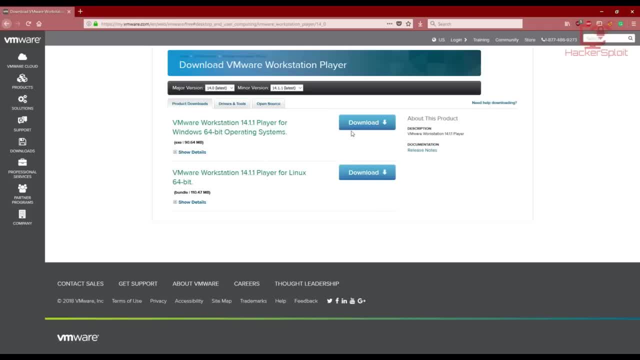 going to show you how to install it, because it's really very simple, And once you have it installed, we'll move on to the next lecture, where we'll be installing, downloading and installing metasploitable to which is the most important part. Alright, so I'll be seeing you in. 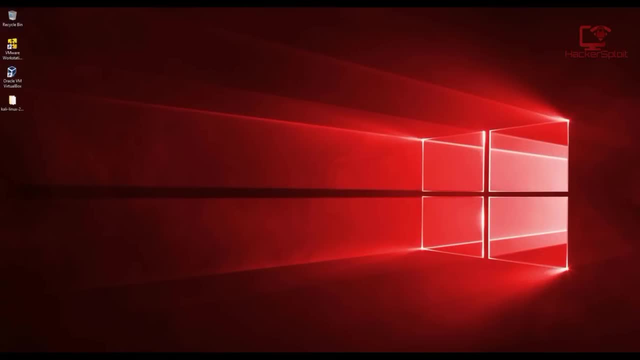 the next lecture. Hello everyone and welcome to this video. In this video, we're going to be installing Kali Linux on our virtualization software, more specifically, VMware. Alright now, depending on the version that you downloaded and installed, whether you chose to go with the free. 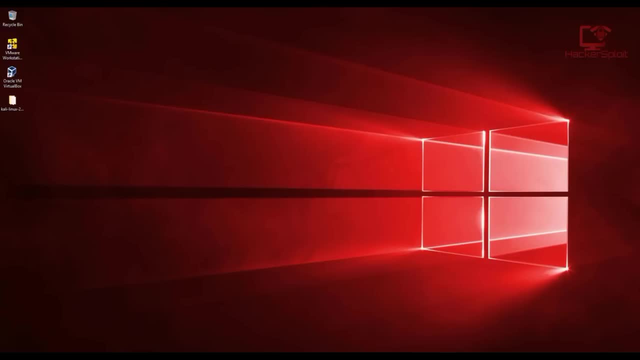 version or the paid version, it'll work exactly the same. And if you're using VirtualBox, the installation process is pretty much the same thing And we're going to be using VMware for the entire, the entirety of the course now, or, if you have, 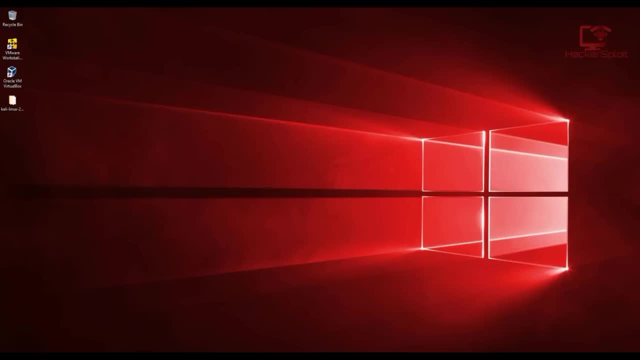 chosen to install Kali Linux on your, on your physical machine. that will work as well. Alright, so let's get started And I'll guide you through the installation steps with VMware. Alright, so I'm going to be using VMware Workstation Player, because that's what I would assume most of you. 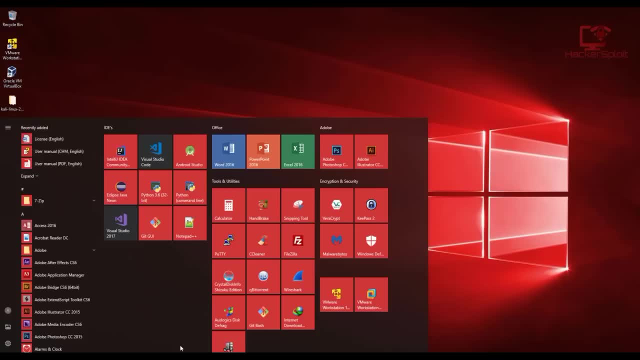 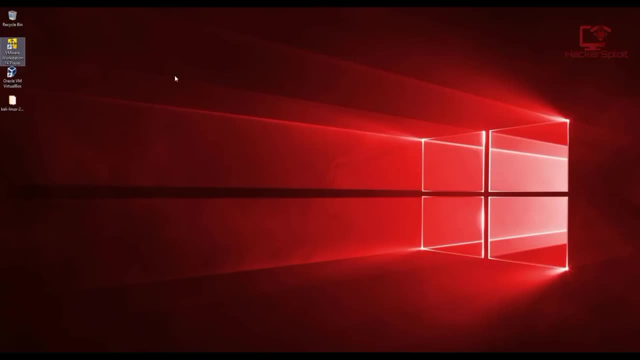 have chosen. If you're using the professional version, as I do, have installed right here, the installation process is pretty much the same, So let's get started. open up your Workstation Player, All right, and it'll take a few seconds. There we are, And I already have. 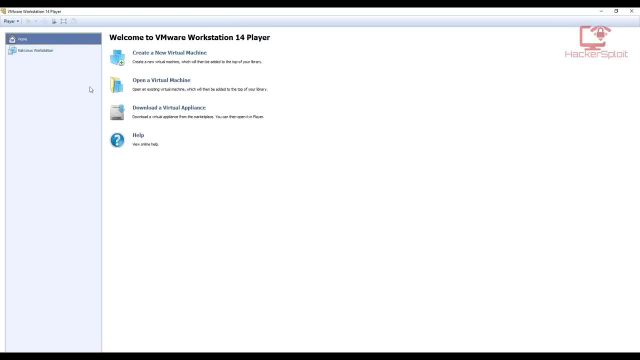 created a virtual machine, But don't worry about that. yours will be empty here, And all we have to do to create a new virtual machine is just click on Create a new virtual machine, Right. Really simple. There we are, And now it's going to ask you to select your in your installer disk image. 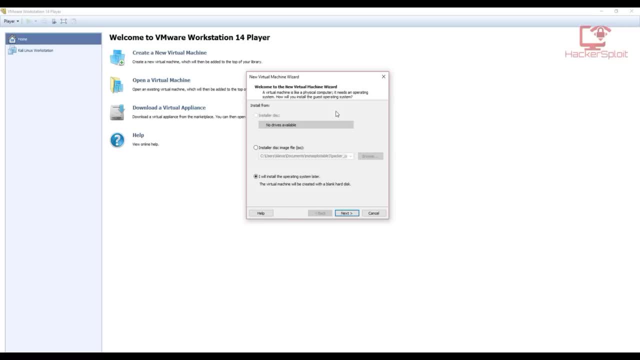 or your ISO file that we downloaded in the previous video where we were downloading Kali Linux. So I hope you guys have got the file. So just make sure you select install a disk image file And you want to specify where that file is saved. I saved mine on my desktop, So I'm just 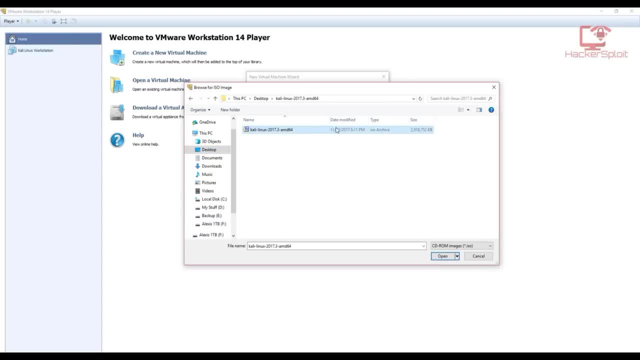 going to go to the folder and click on it. There we are, So make sure you select the ISO that you downloaded. that is appropriate, depending on the system or your computer's architecture. All right, so I'm going to hit open And it's going to give you this little error here saying: could not detect. 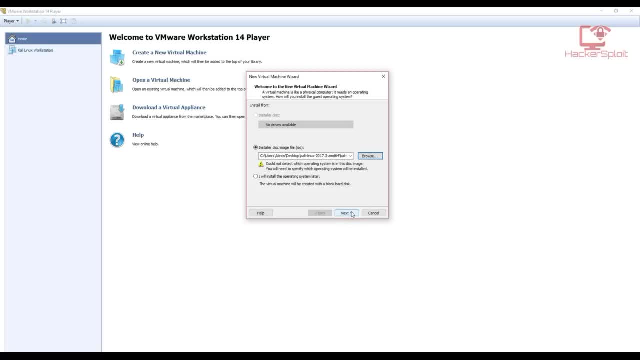 which operating system is in the disk image. don't worry about it. That hit on next is in the disk image. don't worry about that, Hit on next. And now you want to specify the guest operating system. Alright, so the guest operating system is simply what operating. 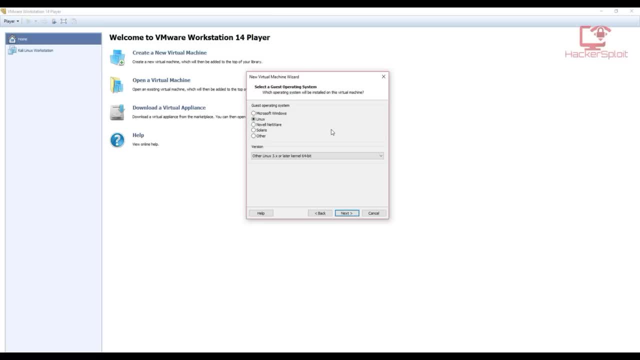 system this is and the kernel that it is running. Alright, so make sure you select Linux, because Kali Linux is based off Linux. And now for the version I want you to select your. you want to go ahead and select version three or later? Alright, so Linux version three or later if you're running. 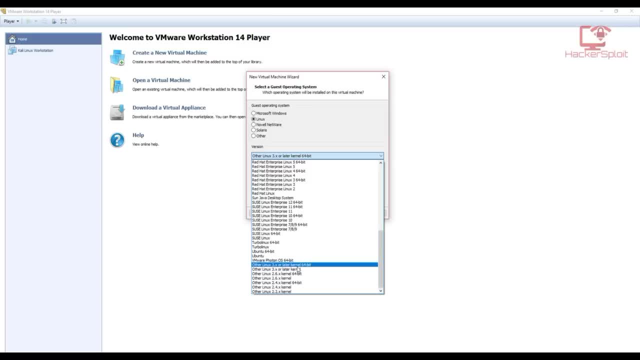 a 64 bit computer, make sure you select the one without 64 bit. If you're running a 64 bit computer, then you want to select the one that says 64 bit, And if you had 32 bit, make sure you select the one. 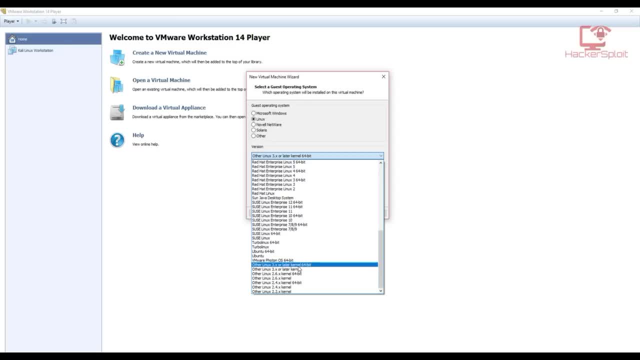 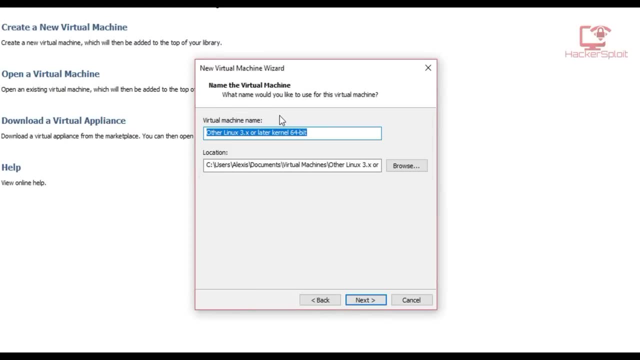 that is. that is simply plain, and that does not contain a 64 bit specification. Alright, so I have the 64 bit ISO and my computer is 64 bit, So I'm just going to click on that and hit next. And now it's going to ask you to give your virtual machine a name. 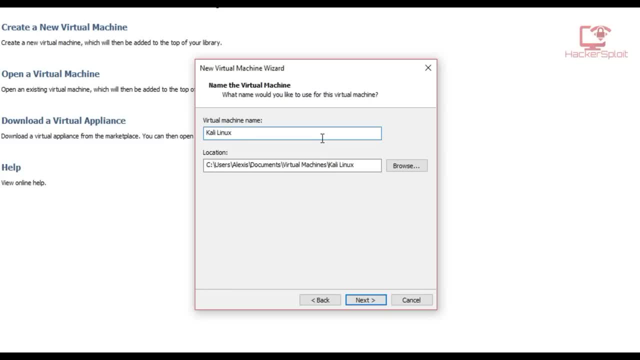 mine Kali Linux. I'm going to call it Kali Linux: Mastering ethical hacking. Alright, I'm just going to give it any name, given it a specific name, but you guys can call it whatever you want. And now it's going to ask you to specify your storage location for the virtual machine. So what I'm? 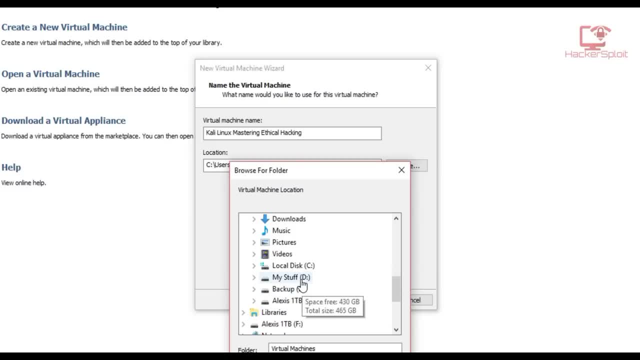 going to do is I'm just going to browse and you can store it wherever you feel is comfortable. I'm good, I have always folder Right here, So I'm just going to open it up And I'm going to create a new folder in there And I'm 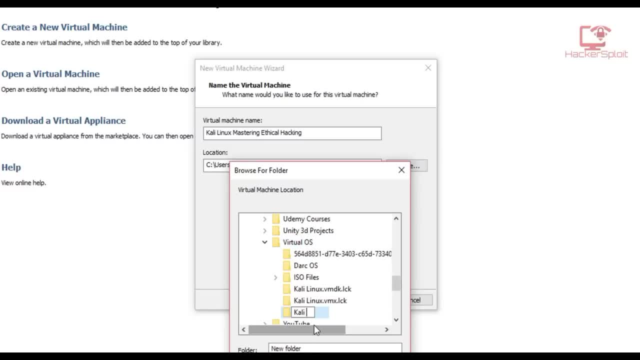 just going to call it Kali Linux VM where I'm just going to call it Kali Linux Hacking. All right, hacking Really really simple, And I'm going to save it in that folder. I'm going to hit OK And it's going to save my virtual machine in there. Again, you can specify whatever storage. 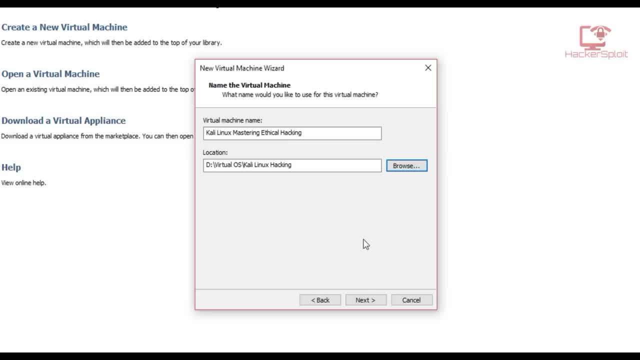 location you feel is comfortable. I'm going to hit next, And now it's going to ask me to specify the disk capacity that I want my virtual disk or my virtual hard drive to be in. I like selecting minus 20 gigabytes. If you're a beginner to this, I would recommend just using 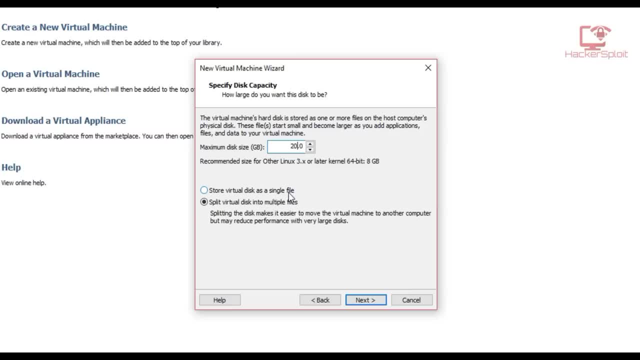 20 gigabytes. But if you have a little, if your computer does not have a lot of storage to spare, 10 gigabytes would work, Okay, but I would recommend 20 gigabytes because we're going to be installing a few files here and there And it may eat up quite a bit of space. All right, Now. 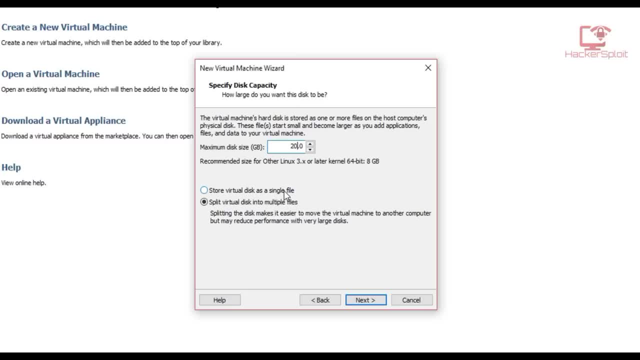 the option that is going to specify here as well is whether or not you want to store your virtual disk as a single file, or you want, whether you or not you want, to split it into multiple files. make sure you select: store it as a single disk, as a single, as a single disk file. And that's because 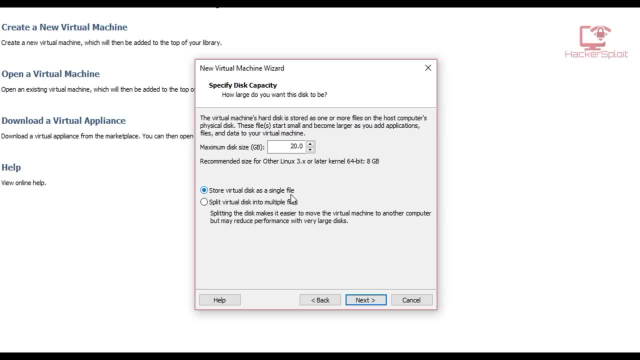 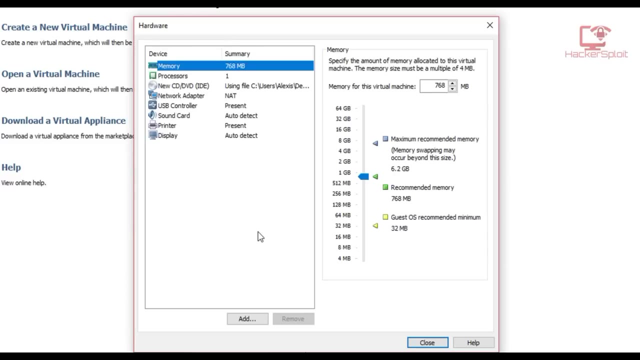 it'll make your virtual machine a whole lot faster and you won't run into any lags or slowdowns. All right, so I'm going to hit next now. And we can customize the hardware, And this is very, very easy. So you can customize it on what computer you're running and what you like to have your. 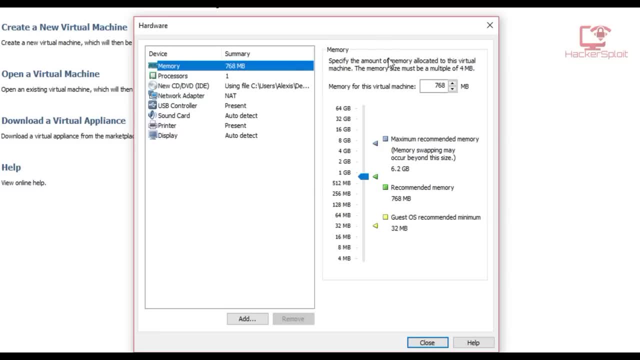 system and how you want it customized in terms of its hardware. Now for the memory. this is just simply: this is your RAM and how much RAM you want to specify to to your virtual machine. Now my. I have a gigabytes of RAM installed on my computer And what I would recommend for Kali Linux, for for: 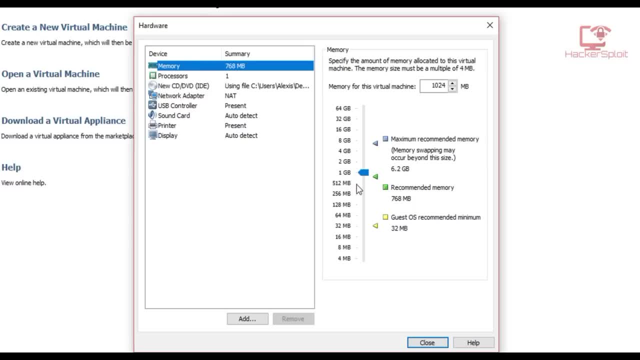 this course is one gigabyte- If you have more to spare, you can use it very, very liberally- and two or four gigabytes. If your computer is running two gigabytes of RAM, you can also use the recommended, which is 768, or take it down to 512. But if you do that, your system will be really. 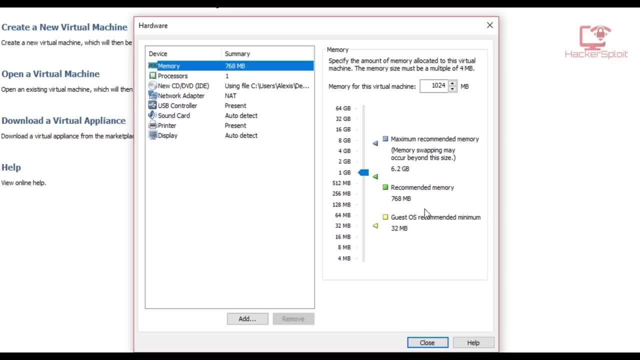 really slow, So I recommend about one gigabyte. That works great for me. Next, in terms of processes, again, this is highly dependent on what you have running on your in your system. For example, I have a quad core CPU, which means it has four processor cores, And that means I can specify up to four. or for this: 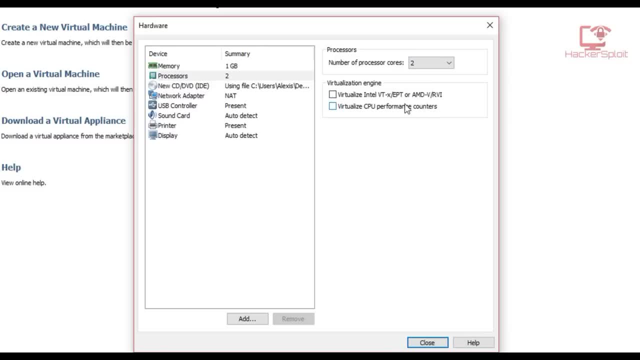 matter. I like to use about two. if you have a dual core CPU or a processor, make sure you select one, because it's always good to keep a balance between your host operating system and your guest and your guest operating system. All right, Now we want to move on to the network adapter, And this is very 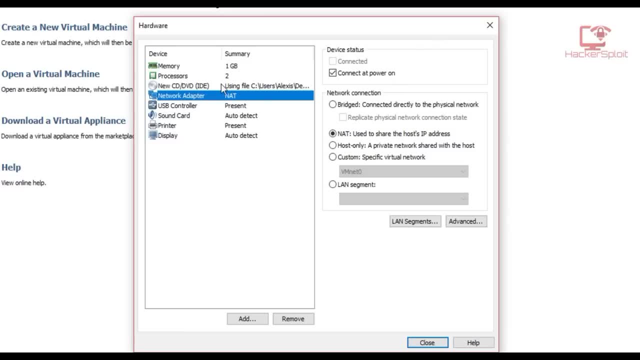 very important. I need to just show you this. we're going to be working with a few other virtual machines And what I'd recommend is to bridge your. I want you to bridge your connection directly to your physical adapter, your physical network adapter, whether you're running Wi Fi or 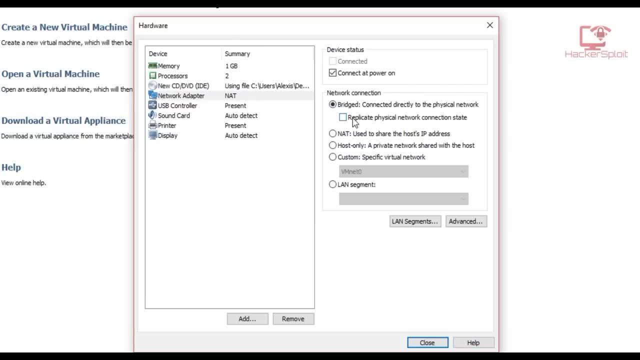 ethernet. So just click on bridge And I want you to click on replicate physical network connection. state Now what this means is that you will be able to communicate with other computers on your network And it will be based on your network as a as a valid computer, And they will be given an IP. 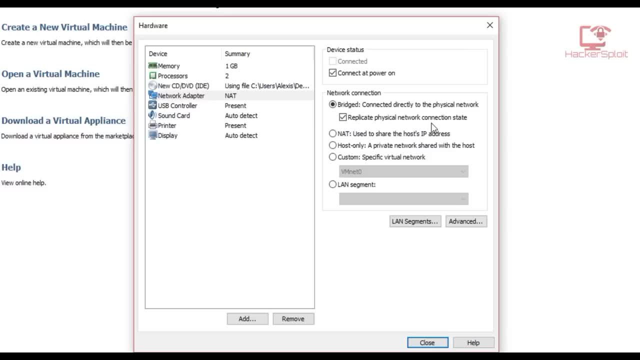 address Match. that All right. The next thing is your display, which is again very dependent on you. Now I have a dedicated graphics card, So I'm going to make sure I hit accelerate 3d graphics And again, if you do not. 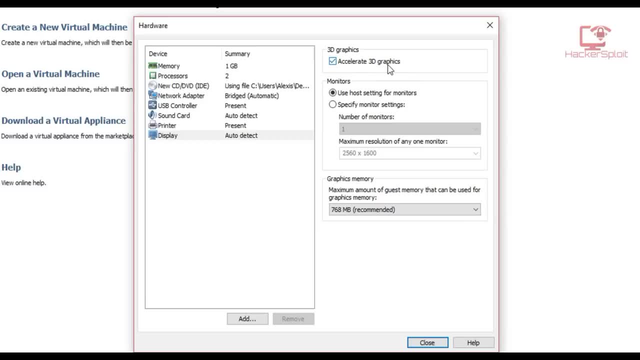 have a dedicated graphics card. you can leave that unchecked. I like having it because it makes Kali Linux a whole lot smoother in its interface. All right, Now as for the graphics memory, depending on how much memory you have dedicated to your system, 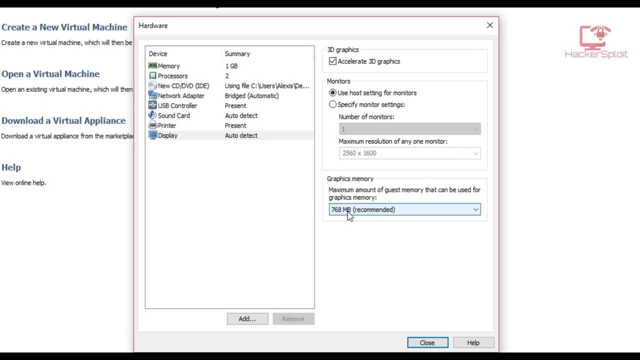 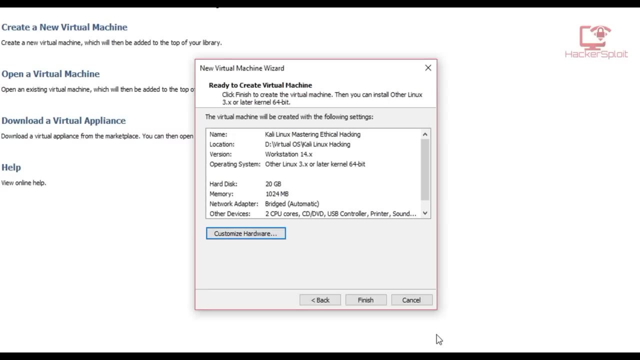 I have about two gigabytes. So it recommends about 768 megabytes And I'll leave it at that. you can specify what is comfortable for you, from 32 bit, from 32 megabytes to about two gigabytes. I'm just going to go with the recommended and I'm going to hit close. And there we are. we want to. 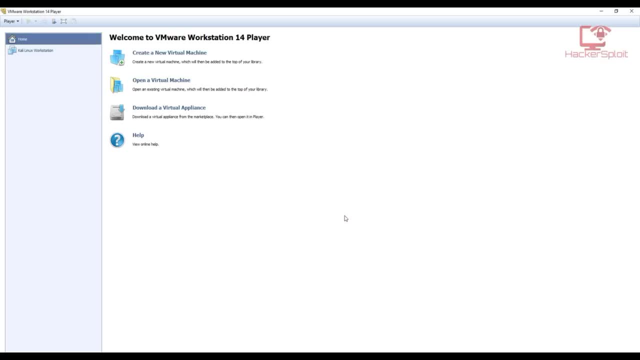 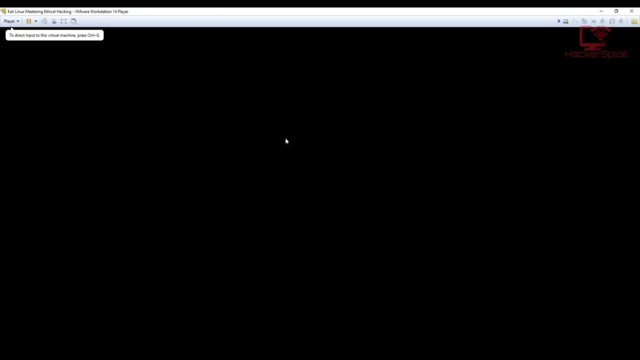 hit finish And we're ready to install Kali Linux. All right, so make sure you click on your virtual machine now And the one that we created, and just hit play virtual machine And it's going to start up. Give it a few seconds, shouldn't take too much time at all. There we are, the VMware BIOS has started up And it's going to lead you to this. 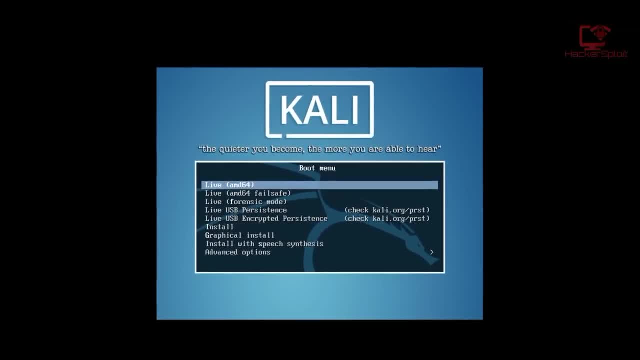 installation screen. All right, so it's going to ask you to select an option. Yes, what we're going to do is we're going to go for the graphical install. I'm going to click, hit on that And now it's going to start up the setup And it's going to start loading everything up. So 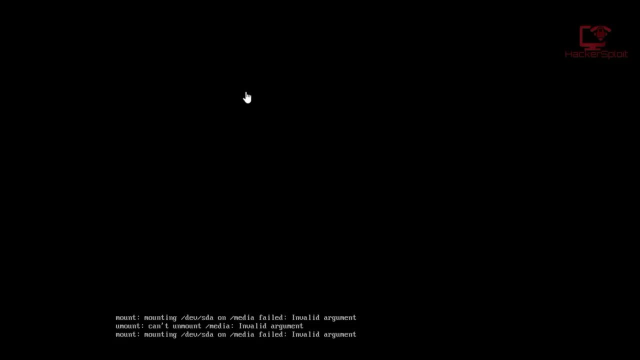 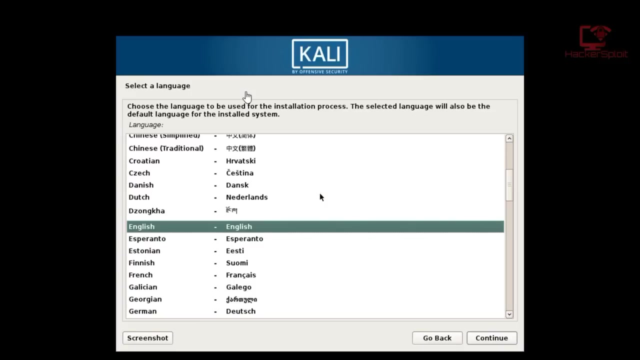 give this a few seconds, as you can see here. Don't worry, if it gives you a few errors here, It should start up anyway. All right, there we are, So now it's going to ask you to select your language. All right, so welcome to. 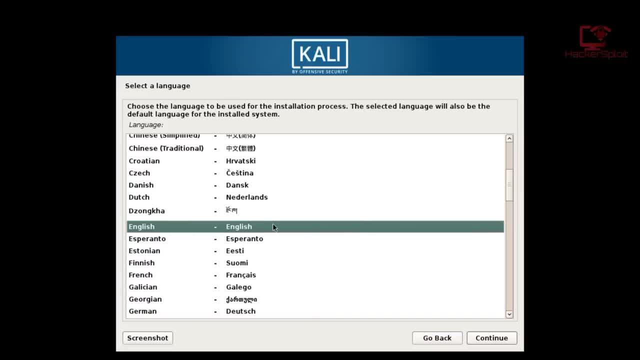 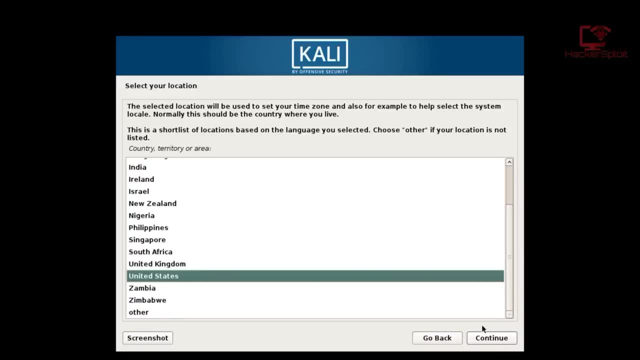 Kali Linux And you can go ahead and select the language that you wish to use. I'm going to be using English and I'm going to hit OK. And now you want to select your version of English And, again, depending on your location or your the country or territory in which you live, I'm 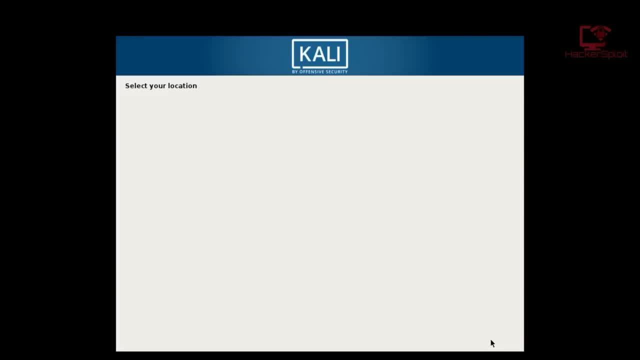 just going to hit United States, and it continue. Now you're to configure the keyboard. This is very, very important. A lot of people make mistakes here. make sure you select the keyboard layout that you are used to. So I'm used to the American English keyboard format, or. 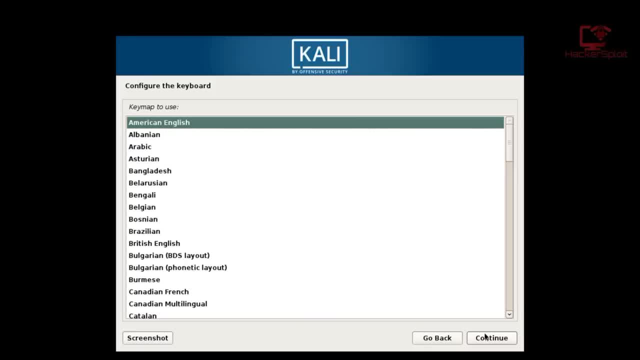 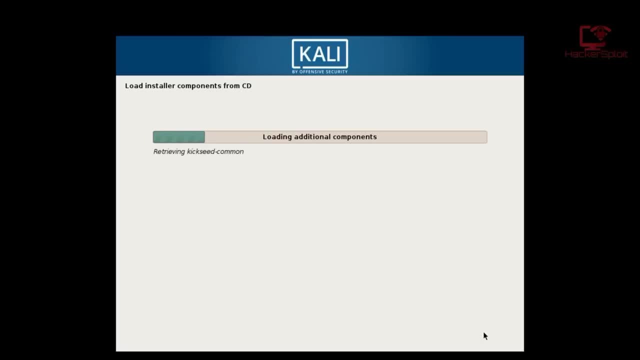 the layout, So I'm going to hit continue Now it's going to scan for all the files And it's going to load all the files onto your virtual disk image for installation. So give that a few seconds as well. Overall, the installation shouldn't take too much time at all. 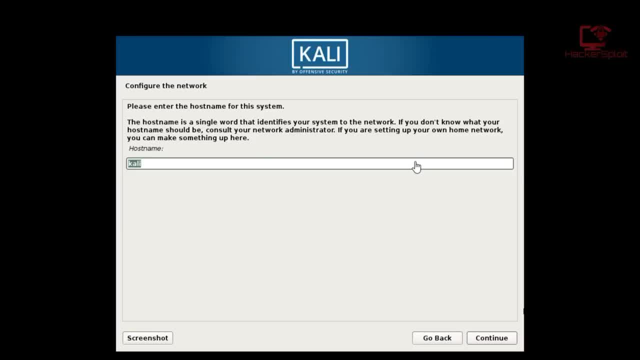 All right. so once it it has loaded all the files, it's going to ask you to configure your network And- this is very, very important- It's going to ask you for a host name. All right, this host name is essentially: this is going to be the name of your system or your computer, on your 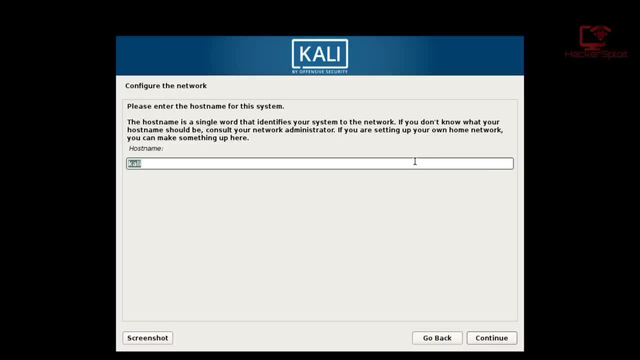 network, And this would be a very good way of identifying your computers. For example, if you had a network of computers, whether you're running this at home on your home network or you're running this in your office especially, this will be a unique identifier for you. 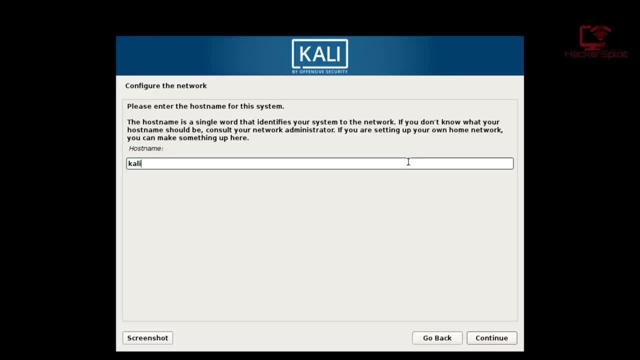 to uniquely identify your virtual machine. So I have two Kali workstations on my network, So I'm just going to call this Kali two, All right, and I'm going to hit continue. If you don't have any other computer running Kali Linux, you can just leave it as the default, which is: 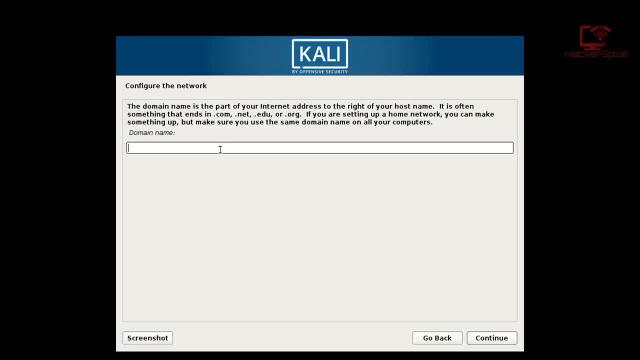 Kali, I'm going to hit. continue Now for the domain name. you can specify a domain name. if you're running this on your school network or your home or your- you know, your- company network, This is really, really dependent on you. But if you're running this on your, 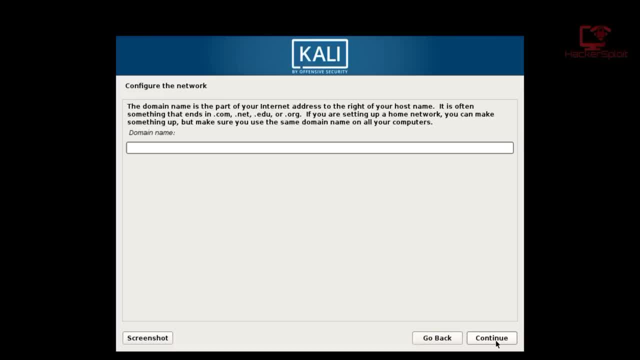 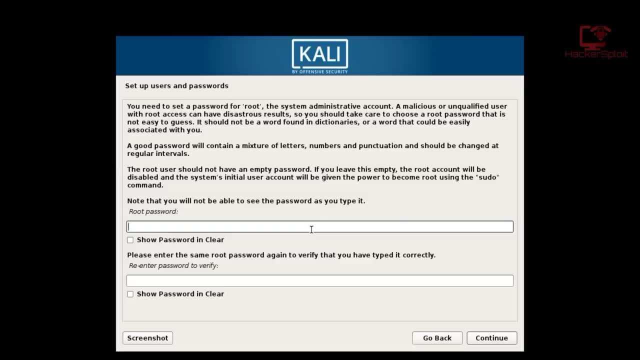 home network. you can just go ahead and hit continue. You don't need to do that. Alright, so it's going to ask you for your users and your passwords. Alright, so this is setting up your users and passwords. The first thing it's going to ask you is for your root password. This is 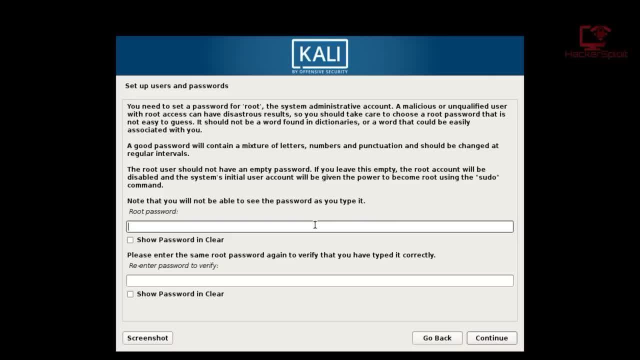 very, very important. Your root password is essentially going to give you, or will be used to grant you, administrative privileges or give you the super user mode in the Linux, in the Linux operating system. So it's very important that you remember this password. 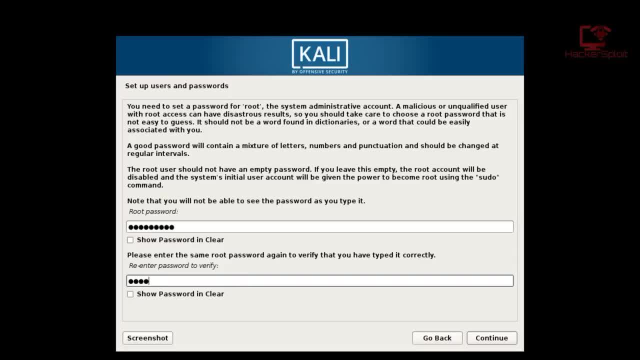 So I'm going to create the password here, Alright, and I'm going to repeat it again. You can. you can give it as anything that you feel is necessary. you can give a very secure system if, if that's what you require, Or you can just give it some very normal password, it really 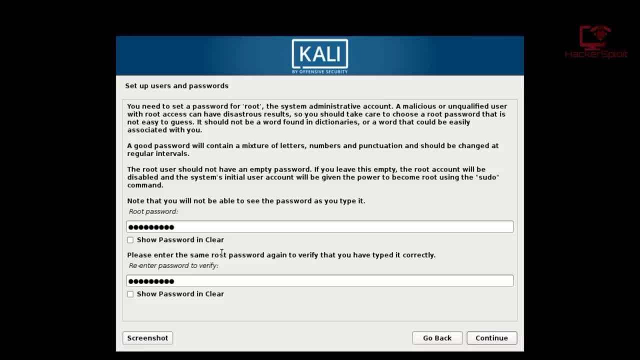 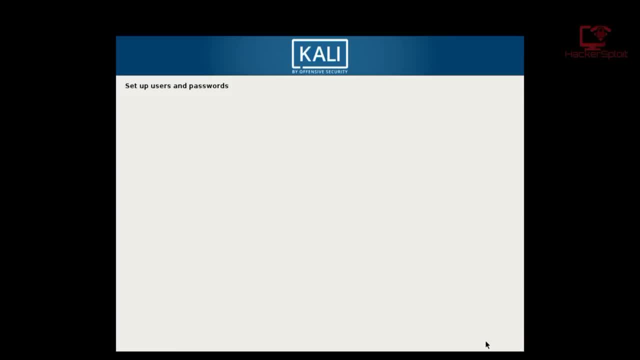 doesn't matter, because this is a virtual lab and there'll be not a lot of important stuff saved, But it's very important that you remember the password that you're using. Alright, I'm going to hit continue, And now it's going to ask you to configure your clock. All right, Now, this is very, very simple. 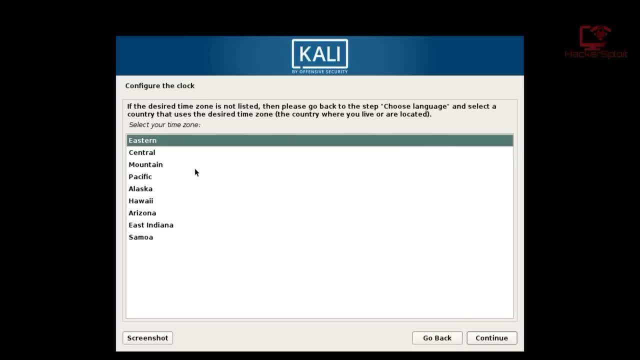 depending on the area that you live in. you want to just select your timezone, So I'm just going to select Eastern. you can go with whatever you want. really doesn't matter for me. we're going to Eastern, I'm going to continue. And now it's going to detect your disk and 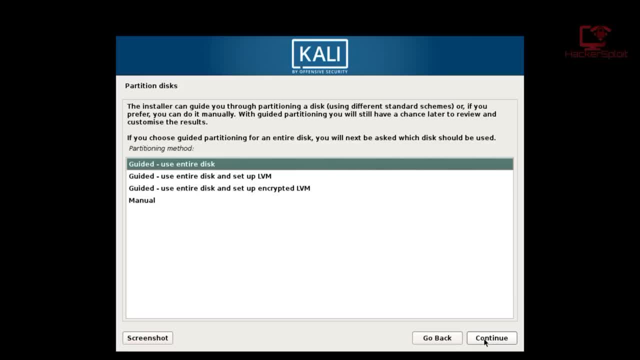 open the partitioner that comes inbuilt with Kali Linux. Alright, so this is very important now. So it's going to ask you now to select the disk in which you want to install Kali Linux, And so what? what I would recommend is just go for. 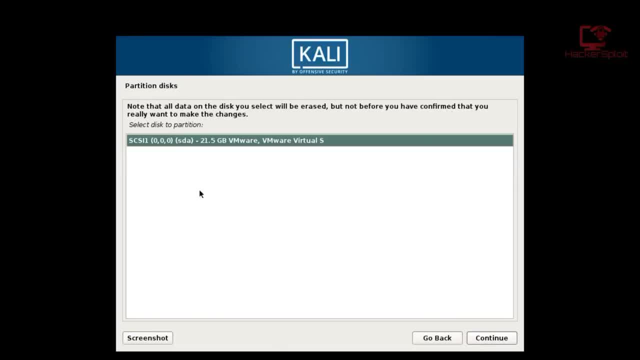 guided. use the entire disk. just hit continue And it's going to show you the virtual disk that we created. In my case it is the 21.5 gigabytes VMware virtual virtual disk. So I'm going to hit that and it's going to. it's going to start. it's going to prompt me to confirm how I want. 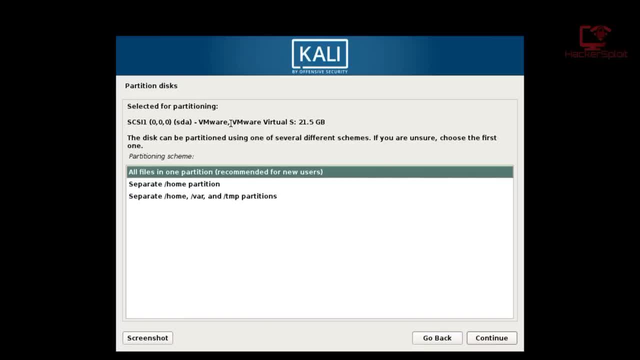 my, my disk partitioned Alright. so Linux, the Linux installation, has three partitions. it saves the system files in the home, var and temp partitions. So I would recommend as a beginner to save everything in one partition, alright, as it, as it says over here, recommended for new. 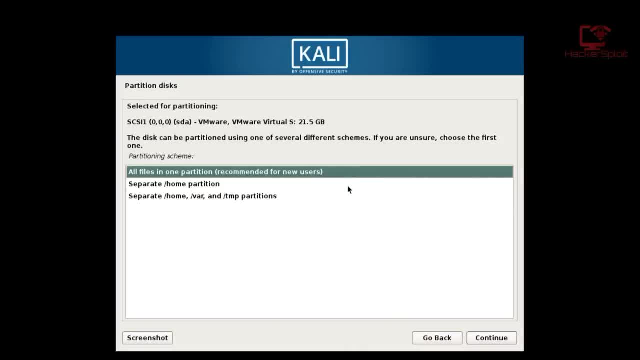 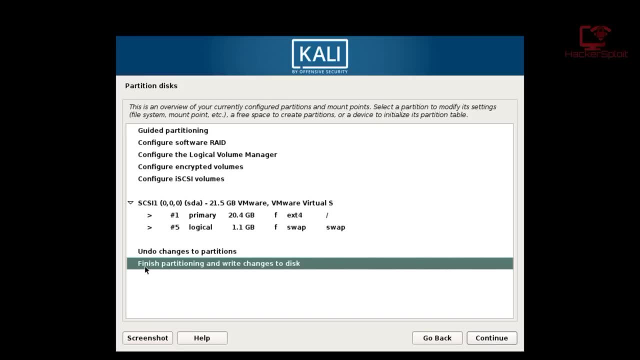 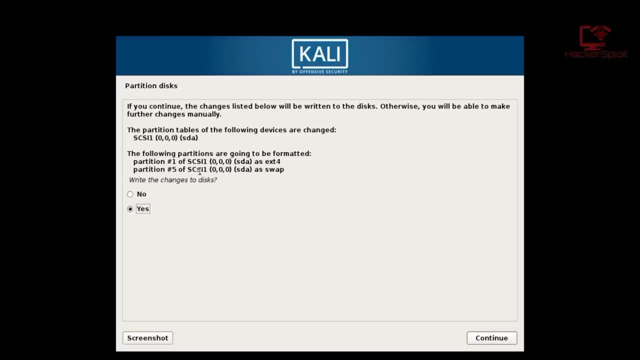 users And that's because you do not have to tinker around with the partitions and select specific swap space etc. etc. So just hit continue And you want to hit finish partitioning And write changes to disk? hit continue And it's going to ask you to confirm whether you want to write changes to the disk. Just hit Yes and 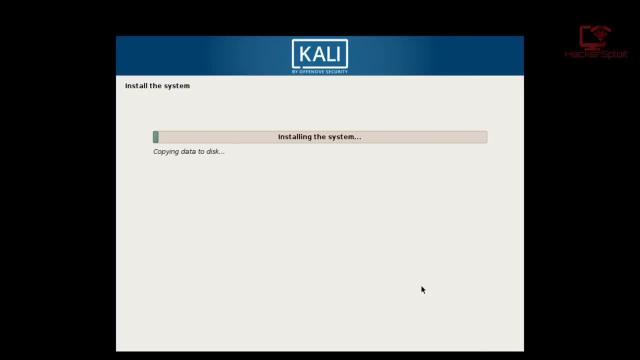 hit continue And it should start partitioning the disk And once it's done, it should start installing the system. Now this should it could take a while, depending on the on your hard drive on your computer, Or if you have an SSD running on your computer, it could go a whole lot. 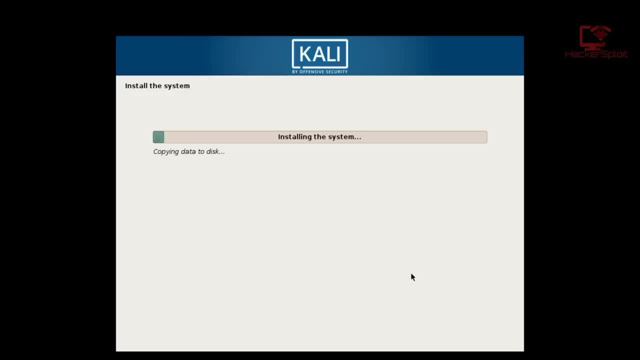 faster. So I'll get back to you when the installation is done. So I'll see you then, All right. so once the installation is complete, it's going to ask you to configure the package manager. All right, and it's going to ask you to. 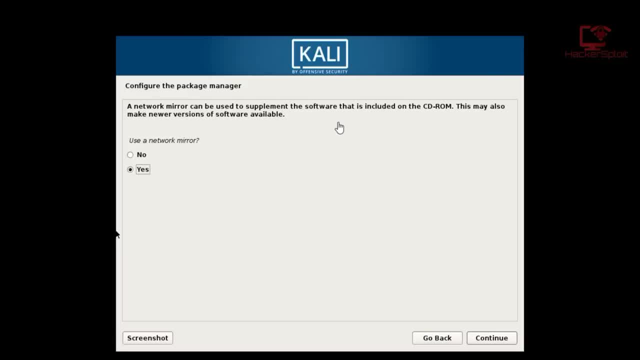 select a. whether or not you want to select a network mirror that can be used to download additional software and updates, All right, so I don't want to use a network mirror and I'm going to continue. All right, and it's going to get started to configure the package manager, So give it a few. 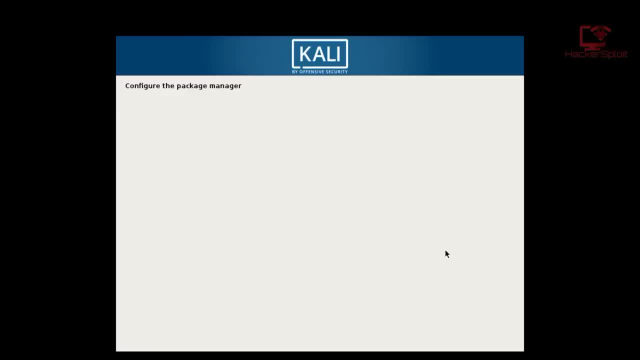 seconds as well. Shouldn't take too much time at all. All right, it's going to start installing the grub bootloader And essentially what this is. it's a bootloader that that is used to start up Cali Linux. All right, so that's just in case you're wondering what it is and how it affects the installation. Right now it's going to ask you whether or not you want to. 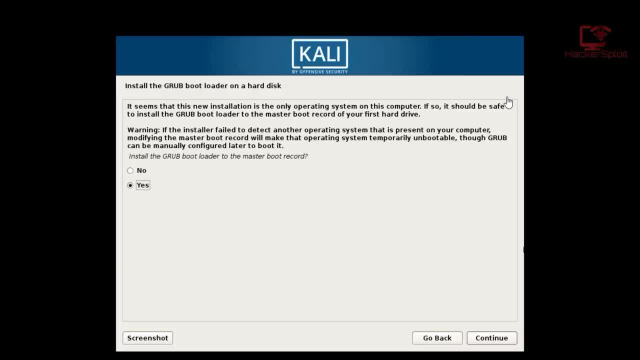 install the grub bootloader on your hard disk, And yes, we are do. The reason being is if you installed it on another hard drive, you had to specify that hard drive to get booted up first, And that really deals with installing it on a physical drive. But 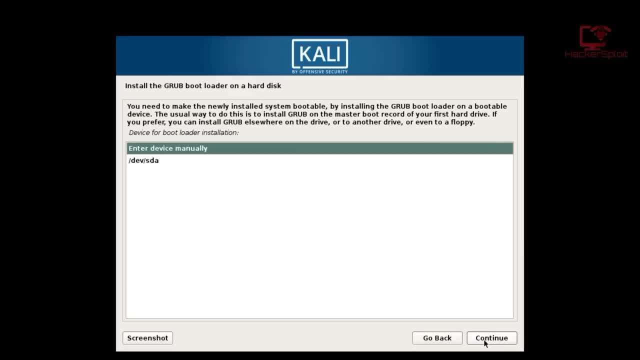 for the for the purpose of this video. just make sure you hit Yes and hit Continue And it's going to ask you to select the storage device. Now, we already- we only created one virtual disk, So we're going to select the device and the storage device a and hit Continue And it's going to install the. 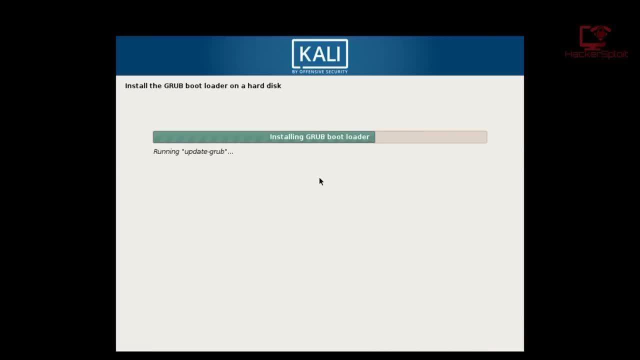 grab bootloader And again, just give it a few seconds. it shouldn't take too much time at all. There we are, And now it's going to finish the installation. It's going to set up the clock and just run any of the other update services that are required for the installation. So I'll 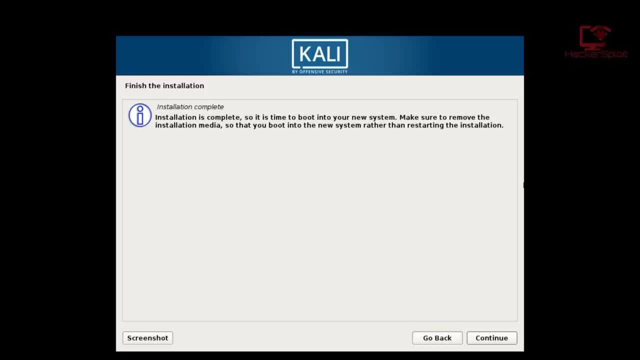 get back to you when it's done. Alright, so. alright, so once the installation is complete, it's gonna ask you to hit Continue to complete the installation. And now it's going to get rid of the packages- the installation packages that. 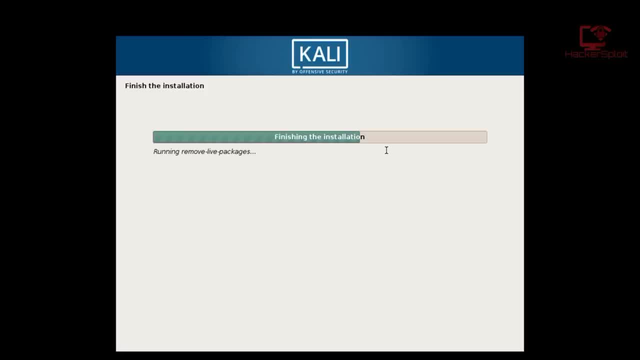 were left over during the installation. And just give it a few seconds. There we are, And once it's done, it's going to automatically reboot and it'll reboot you directly into Kali Linux. So just give it a few seconds. This whole process shouldn't take any more than 20. 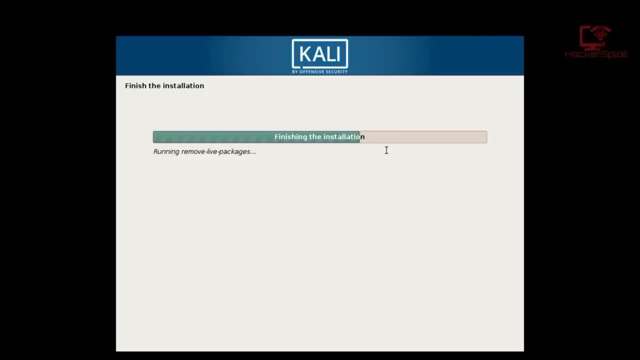 minutes, along with the installation of the files on your virtual disk image. Again, don't get too excited about it, Just solution. ego must be as easy in the beginning and should be based on either one of the ingenuuuu structures as it comes to Fi? educuies. but 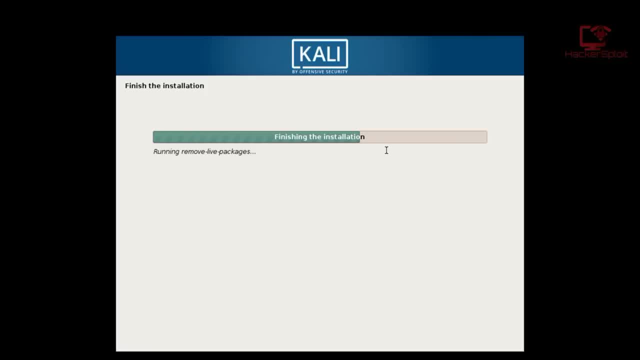 AWS backend? actually don't. So, whatever the type, function and therefore as far as the virtual drive are, as I said, it really depends on the on your computer and the system that you're trying to to do this on and whether or not your disk is a fast hard drive or using an SSD. so that is really. 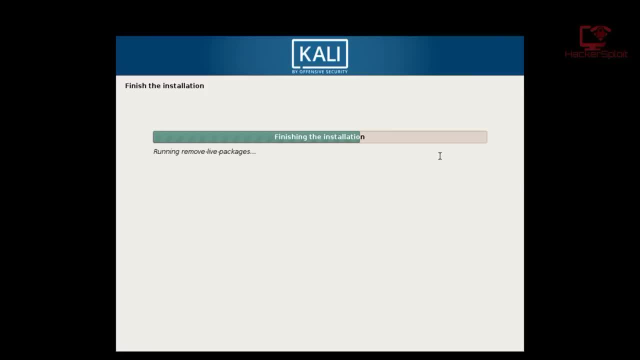 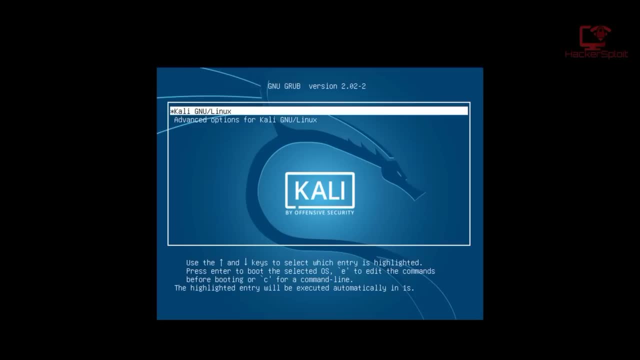 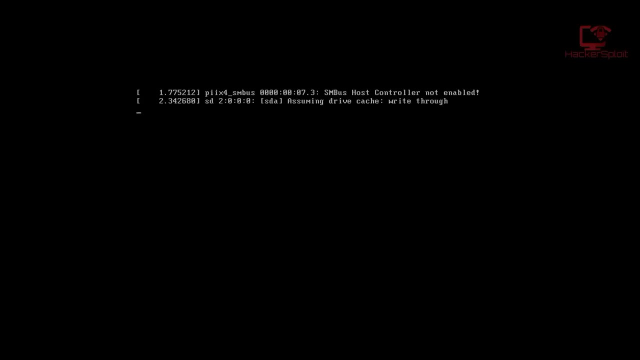 dependent on what system you're running. so just let it get rid of the live packages and I'll get back to you when it's ready. all right, so once it's done, it's gonna start up- and this is the start- the grub bootloader and it's gonna start Kali Linux up once it restarts. there we are, and 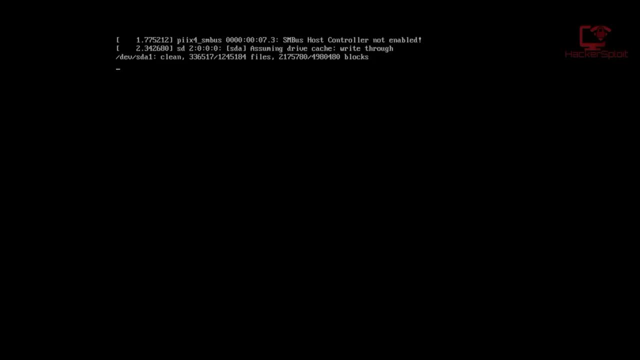 the system is starting up now, so just give it a few seconds to load everything up, and it should give us the login screen, where I'll give you the instructions as to what to use for the username and, obviously, the password that you set, which was the root password, which will be the default. 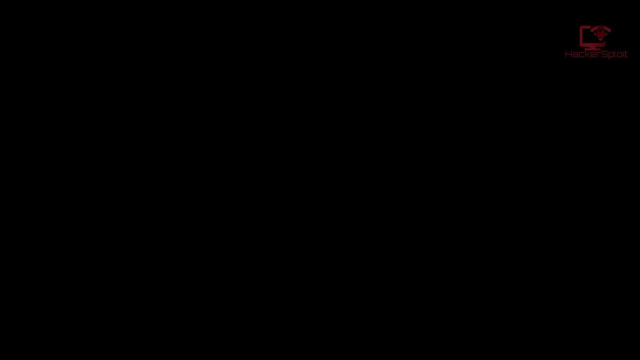 password, because we're going to be logging in using the root account. that's because we didn't create any user. all right, which I'll also be showing you how to do so. there we are: the system is started up and we can already see that we can use the Kali Linux. 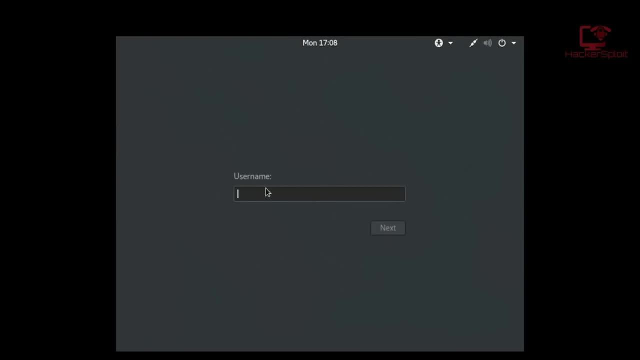 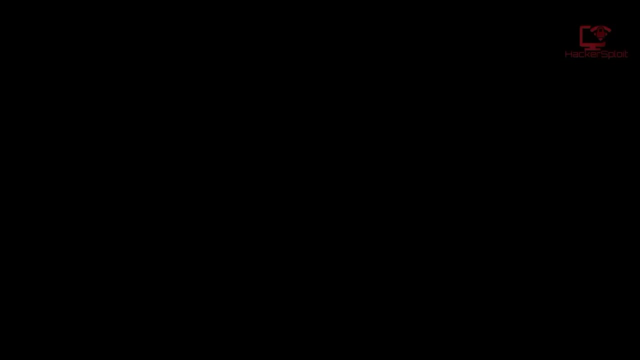 pointer. so again, just, it's just a matter of time before it starts up. there we are, and here we have Kali Linux, so let's, hopefully we can log in. so the username that you want to use is going to be root and the password is going to be the password that we set during the installation. so enter that and 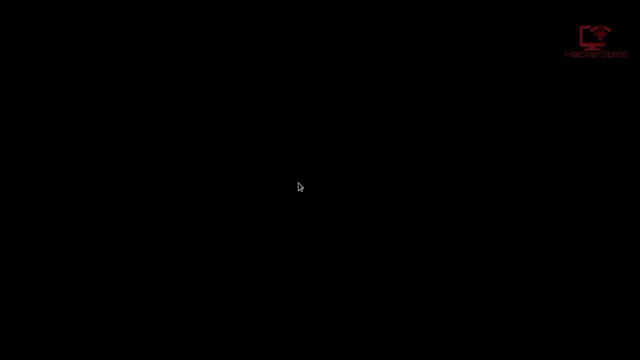 hit enter and there we are. it's going to start Kali Linux up. give it a few seconds to start up the desktop environment. it should be up anytime now and in the next videos we're going to be looking at how to customize Kali Linux. uh, you. 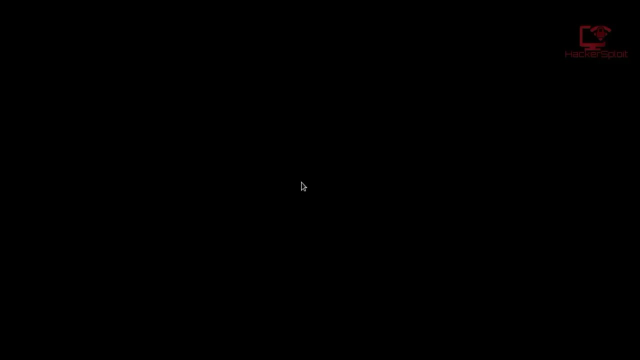 know, making, making sure it's working all right, and it works to your advantage rather than working against you. and I'm just going to show you how to get comfortable with Kali Linux, all right, so again, uh, the first startup. uh, shouldn't take too much time, and you know this is going to be, uh, this, this. 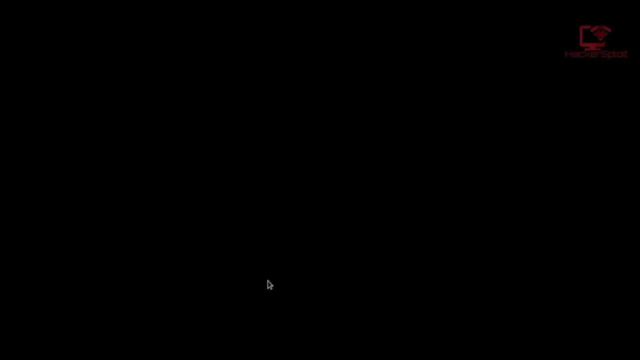 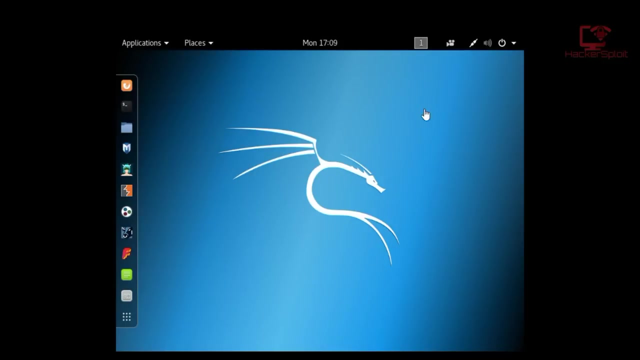 video procedure is going to happen only once, and that's because it's starting up for the first time. it's just configuring everything, so just have a bit of patience and it should start up all right. once you start up, welcome to Kali Linux. and, as you can see, uh, don't worry if the screen. 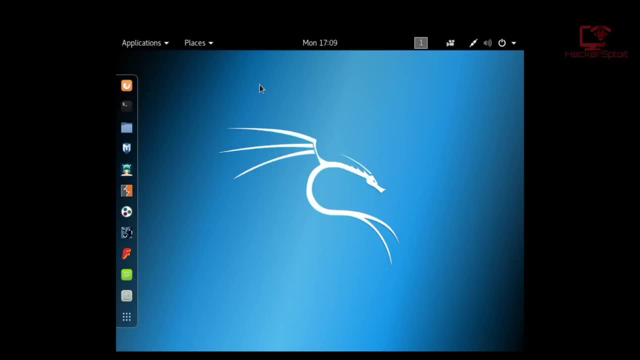 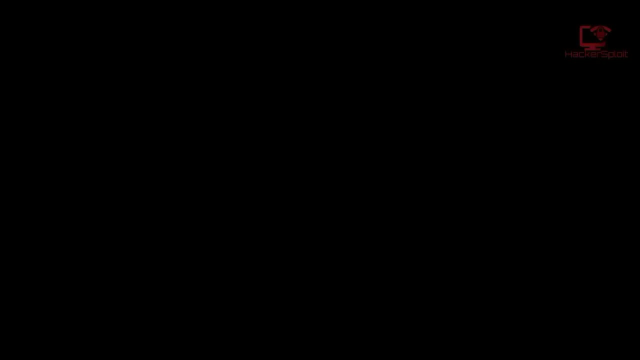 resolution is very, very slow. it's really simple to sort that out and that's what we'll be looking at in the next video. we'll be customizing Kali Linux and adding users, Etc, Etc. so I'll be seeing you in the next video. 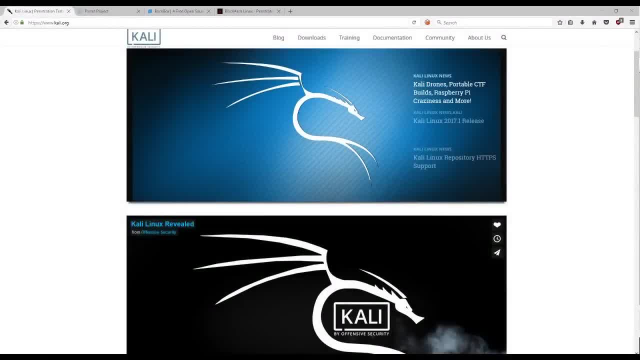 hey guys, hackersploit here back again with another video, and in this video I'm basically going to be showing you the top Linux distros for ethical hacking. and please do note that these are in my personal opinion and are not ranked, uh, in any order whatsoever. so basically, let's get started. 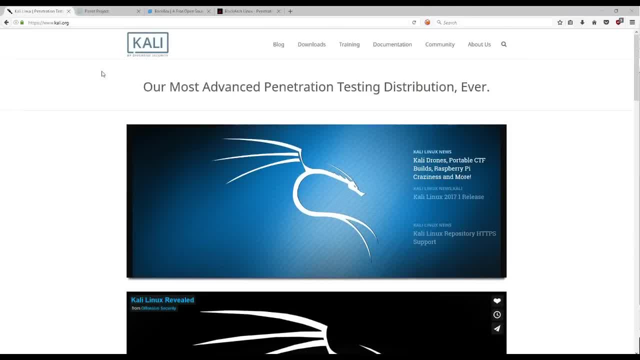 uh, the first one we're going to be looking at is Kali Linux. now, this will come as no to most of you because, again, Kali Linux is the benchmark in distributions, so it, Kali Linux, is based off, you can say the backtrack Linux. for those of you who, 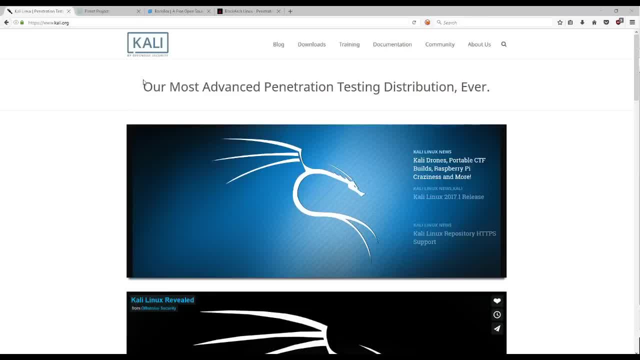 have actually been in penetration testing long enough to understand that. so basically it's a penetration. it's one of the most advanced penetration testing distributions, and the thing I like about Kali Linux is that it has rolling releases, which means that it's going to be updated frequently. it has the largest 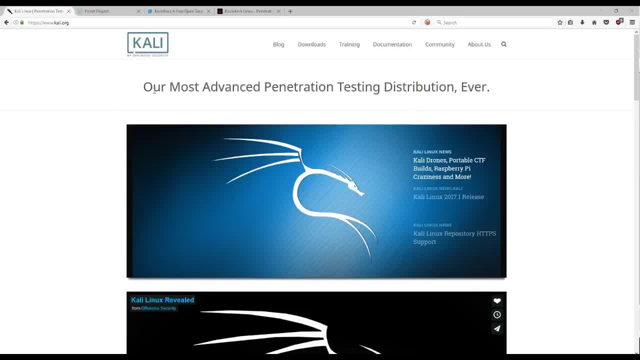 number of tools, and the tools are supported for Kali Linux. so that means if the tools are updated, they will get updated with Kali Linux when you update the distro itself. secondly, it's rock-stable. apart from a few issues with the desktop environment, I haven't had any issues in terms of system. 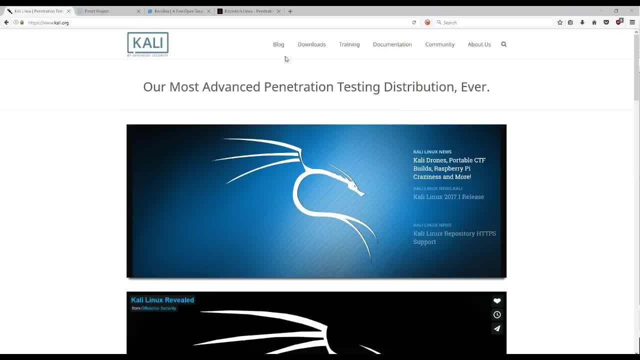 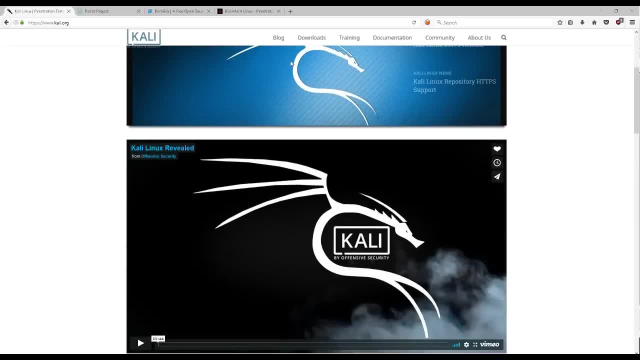 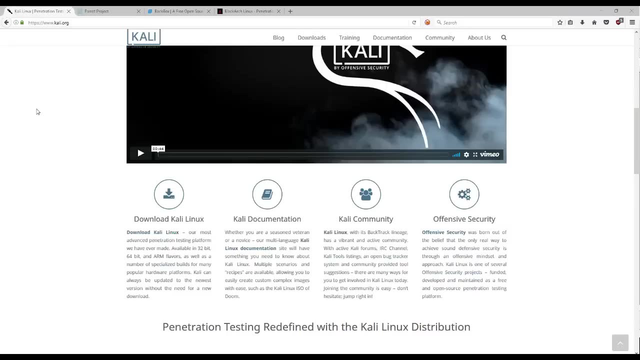 stability and stuff like that. again, it has fantastic documentation and training services that you can try out for yourself. you can also check out their blog. they have very, very cool videos and things that will help you around basically getting around the operating system. so again, one one of the reasons that I like it the most is it has a huge arsenal of 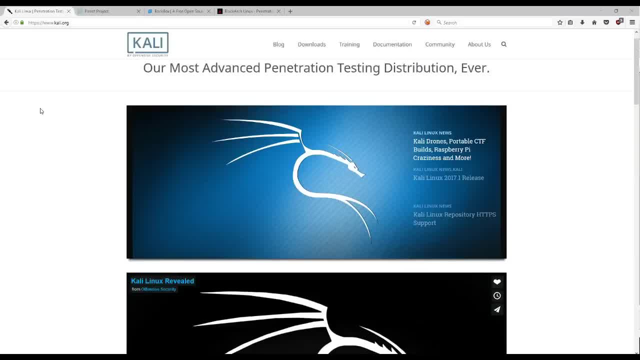 tools or scripts for that matter. that will just make your user experience a whole lot better, and you really don't need to start installing different stuff and, really honestly speaking, the industry stranded is Kali Linux. so this is basically, I think, one of my favorite ethical hacking or penetration. 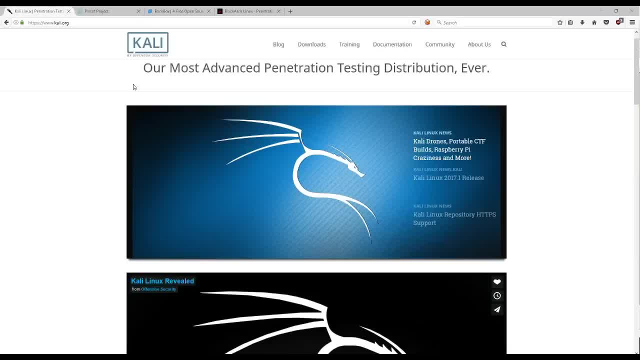 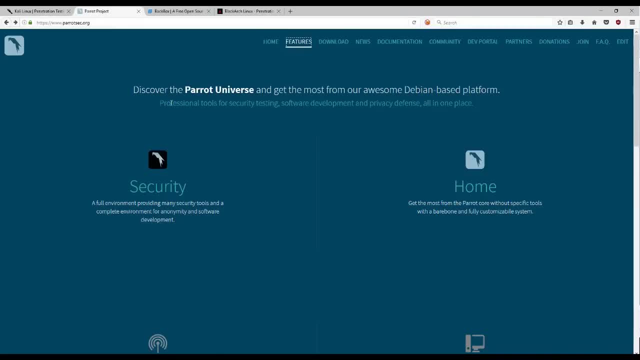 testing distributions. so let's move on to the second one. the second one, in my opinion, would be Parrot OS. now, some of you might not have heard of Parrot OS, but for those of you who have been on my channel, you know that I've made a few. 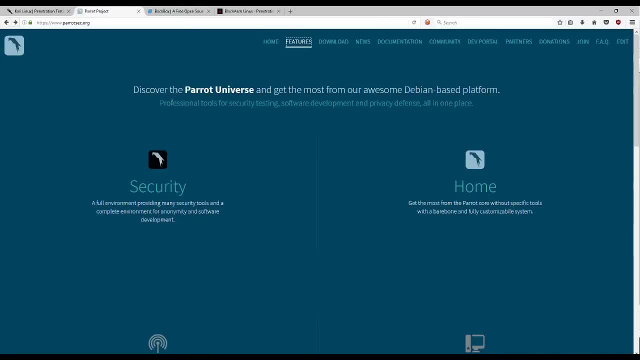 videos on Parrot OS and also a review. by the way, I will be leaving a. you can just check up this video. I will leave some cards taking you to the reviews of this next distributions, if you're interested in checking them out. so just the card should be right above right your screen right now, taking you to the review. so 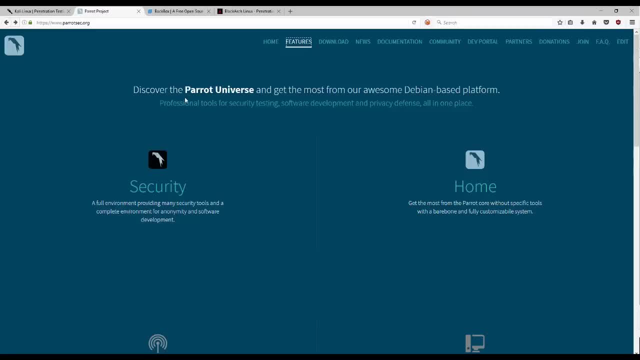 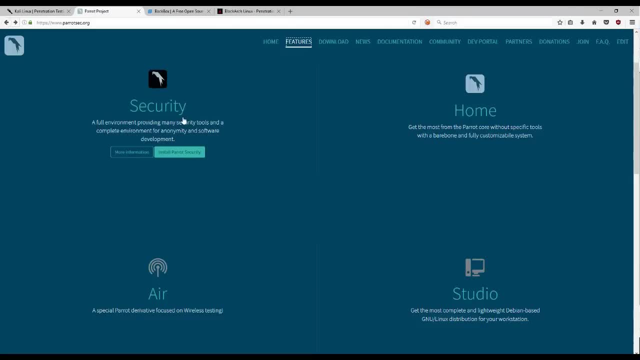 basically Parrot OS has. you have different versions of Parrot OS. by the way, the link to the website will be in the description section, just as a little pointer. so you have your security, you have your home version, you have your studio and you have your air. so, as you can see, 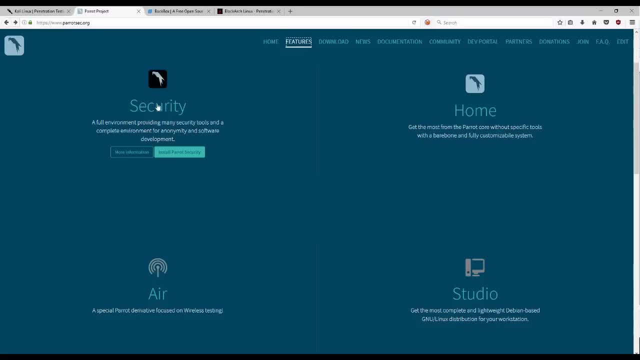 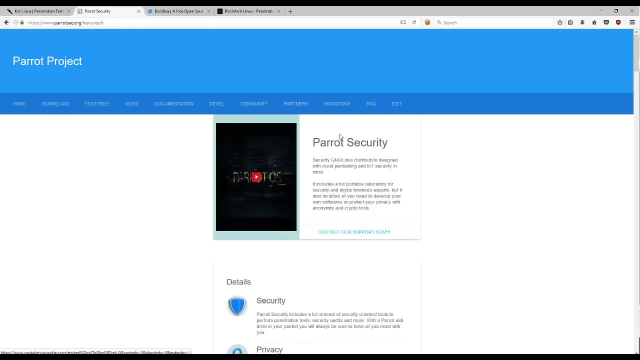 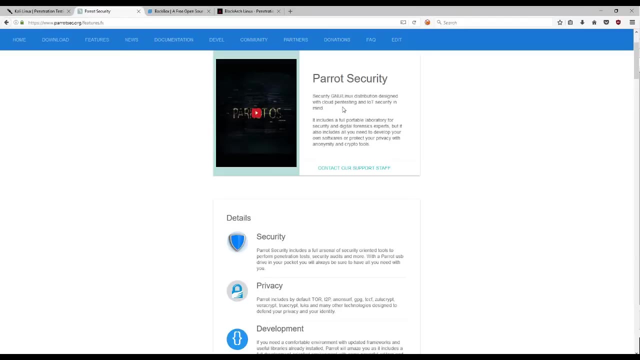 they'll give you a bit of information about it, but what we are focusing on is the security. so if we click on that, let's see what this is all about: more information, and it's going to tell you part. security is a Linux distribution designed with cloud pen testing and I Internet of Things security in mind. so 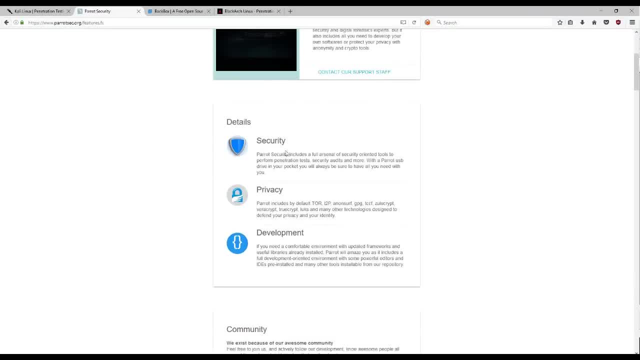 basically a part. the details here is that it's made for security, privacy and development. pretty awesome stuff, right? security includes a full arsenal of security oriented tools to perform penetration tests, security audits and more so. it basically provides you with an arsenal of penetration testing tools and scripts similar to Kali Linux. but this is where it really shines, it also. 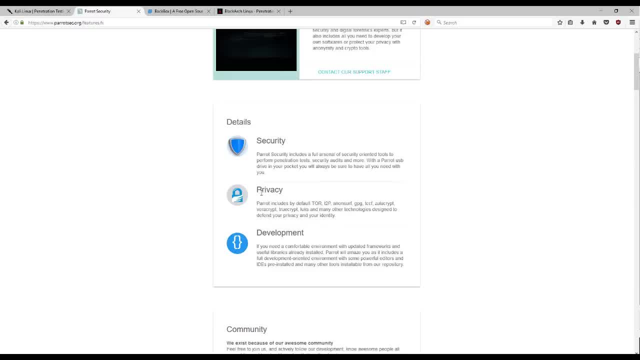 contains privacy, privacy tools, so you have a part was includes by default. it includes Tor I to P and on surf, GPG, TCCF, Zulu crypt, where crypt to crypt. so basically, encryption and cryptography services- pretty awesome. this is something that Kali Linux does not really shine as well as parrot OS does now in terms of. 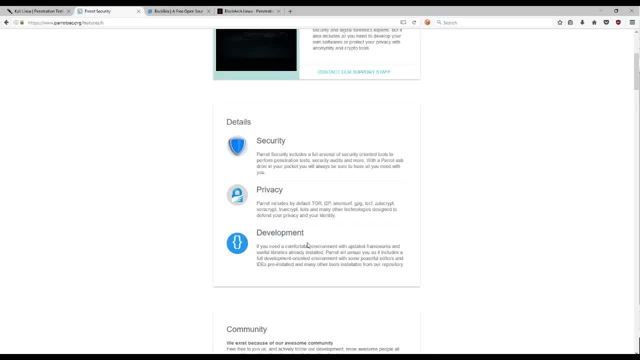 it also includes a very, very cool thing which I will highly recommend. if you guys are looking for a Linux distribution that really goes from penetration testing to development, this is perfect for you. so if you need a comfortable environment with updated frameworks and useful libraries already installed, parrot OS will amaze you, as it includes a full development oriented 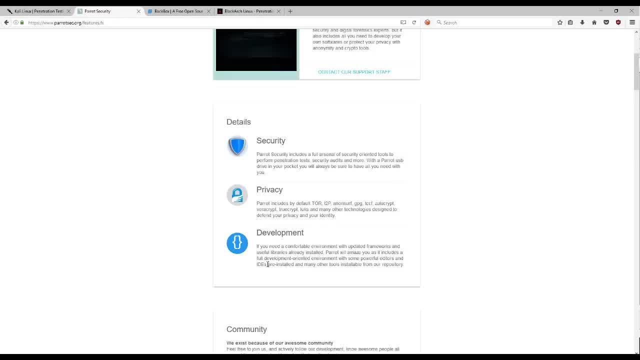 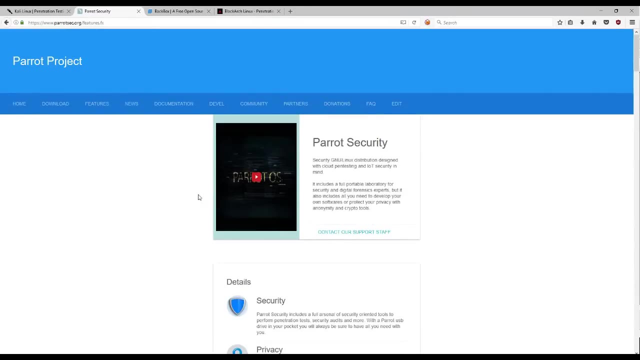 environment with some own editors and IDEs pre-installed and many other tools of installable from our repository. so it also basically has their own repository for tools that will also get updated. so if you guys are interested in a very, very balanced- well balanced- the distro for that basically moves from penetration testing to 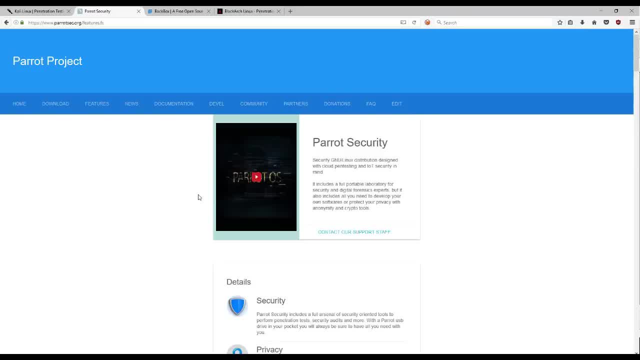 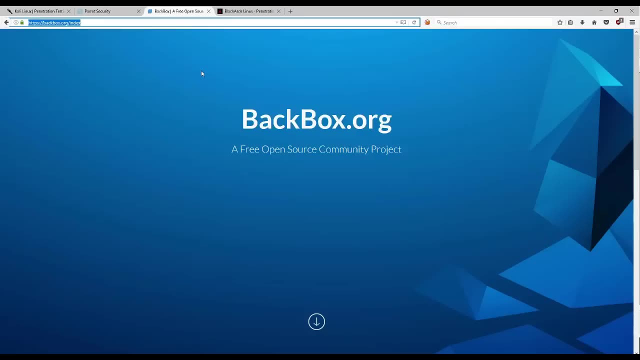 cryptography to development. go ahead and check parrot OS. in my opinion, it's one of the most balanced and well polished Linux distributions around the world. now the third one is going to be backbox Linux. now some of you may have heard of it, but it's a it's well. it's not really popular operating system. it's. 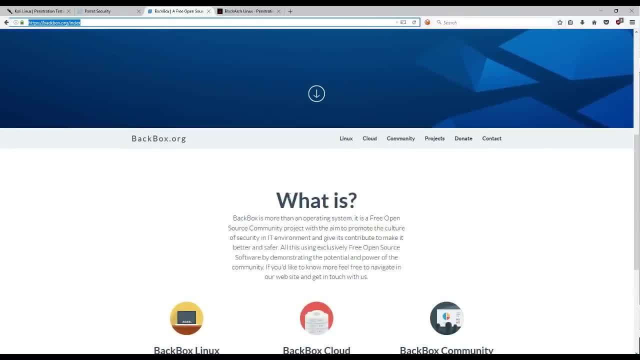 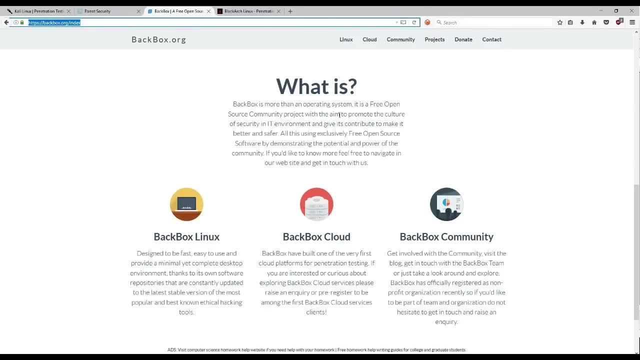 very popular with people who who do a lot of Wi-Fi penetration testing. so again it has. backbox is more than an operating system. it's a free, open source community project with the aim to promote the culture of security in IT environment and give its contribution to make it better and safe. I'm not sure whether that was typed incorrectly, but 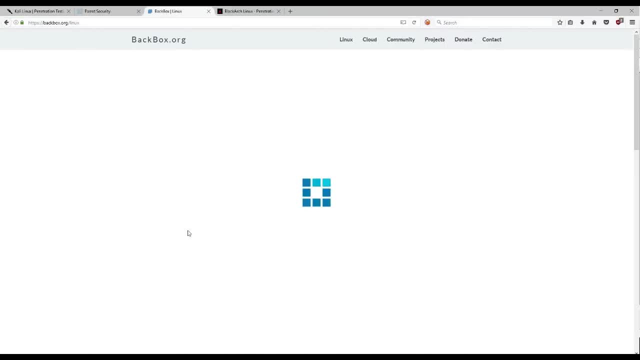 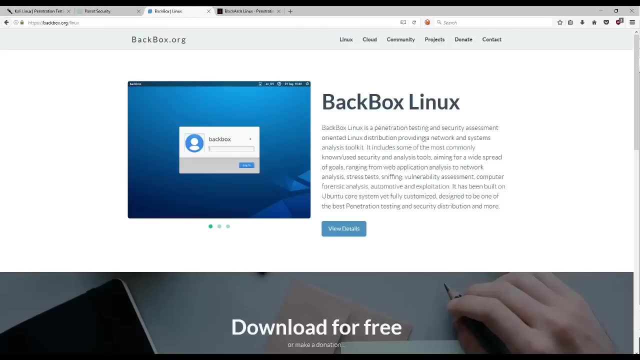 backbox Linux, because that's the one that we want to look at. so backbox Linux is a penetration testing and security assessment oriented Linux distribution providing network and systems analysis toolkit. it includes some of the most commonly known and used security and analysis tools aiming for widespread, for a widespread range of goals, from web application analysis. 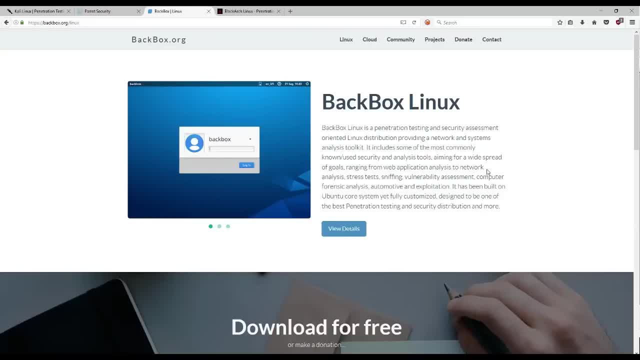 to networks analysis, stress testing, sniffing, vulnerability assessment, Etc. Etc. so, basically it is. it's built on Ubuntu core, so for those of you who are already familiar with Ubuntu, this will be perfect for you. um, it's fully customizable and designed to be one of the best penetration. 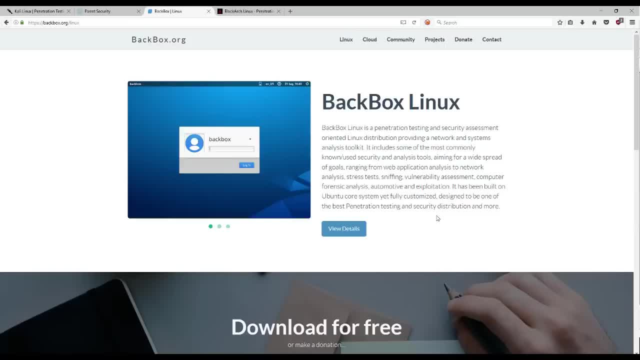 testing and security distributions available now. again. the review to this uh distro will just pop up right above your screen on the top right, so make sure, if you want to check it out, go ahead. I made a video on it. now, to be honest, uh, this is I. I would like to call this uh. 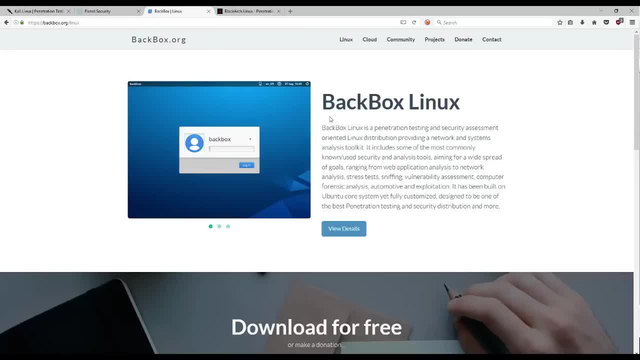 Ubuntu with the tools that you'll be most likely be using on other Linux distros, like, for example, burp suite, SQL map, Etc, Etc. so it has the most popular tools but doesn't have everything. so, again, this will provide a bit of a balance between Ubuntu, which is a fantastic desktop, and laptop. 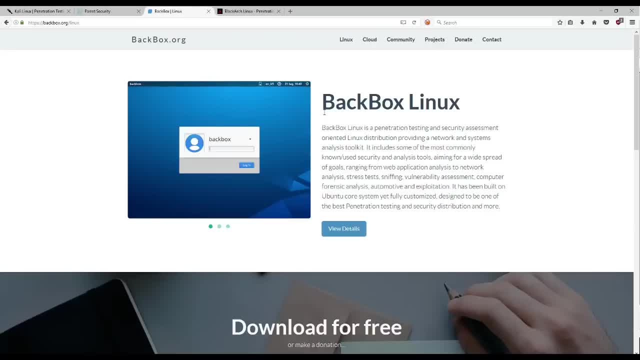 operating system on its own. it's really really well polished. so, yeah, it has Ubuntu, and that means you'll be getting updates. in addition to that, you have the penetration testing tools, so, in my opinion, would I recommend this. I would recommend this for people who want just a bit of 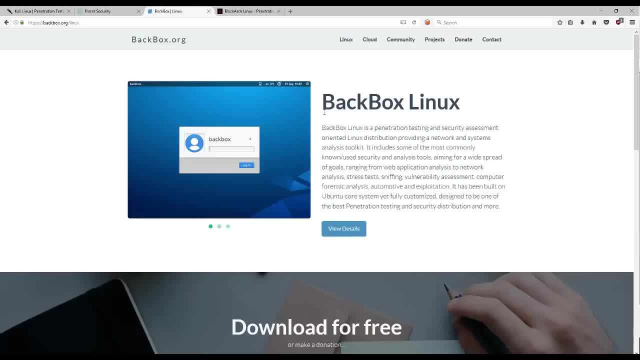 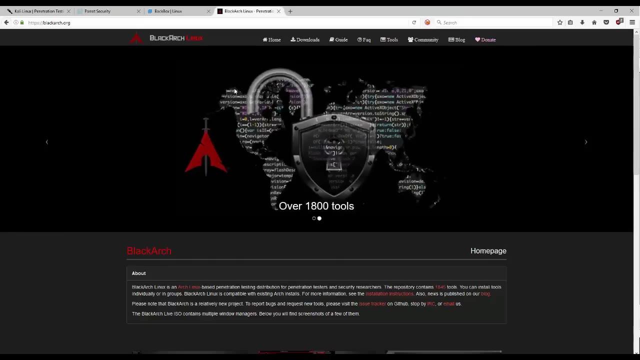 of both worlds really, who want maybe more of Ubuntu and less of the penetration testing side of things, but who appreciate the having the tools. so definitely go ahead and check this out. also very, very viable and good option. now the fourth one and the last one in my opinion, is black arc. 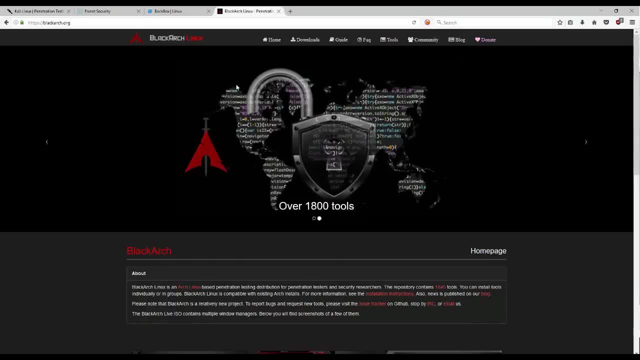 Linux now, for some reason, a lot of people. well, it's a. it's mainly a divided uh topic when it comes to black arc Linux, because people will- many people- will say that black arc Linux is the best compared to Kali Linux and others will say black arc is basically just. 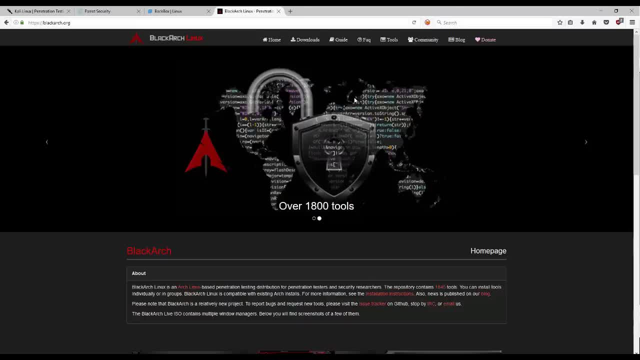 uh, it's just another penetration testing Distro. I have reviewed it again. the review will be in the top right. um, in my opinion, it basically it is a fantastic penetration testing distribution, to be honest, but it is based on our clinics. all right. now, this is where the- where I usually 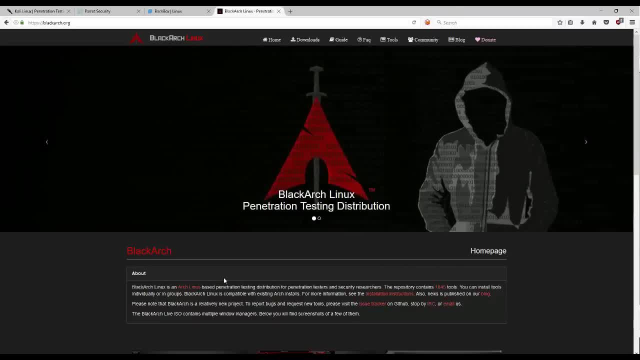 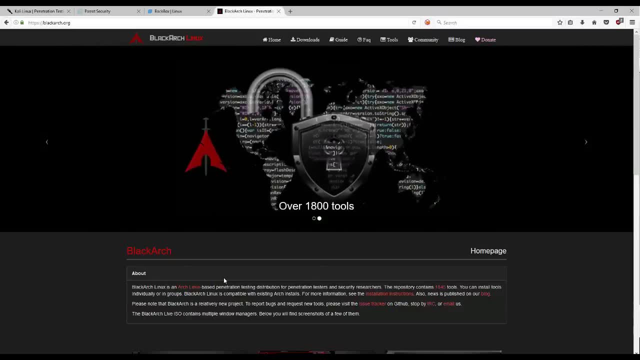 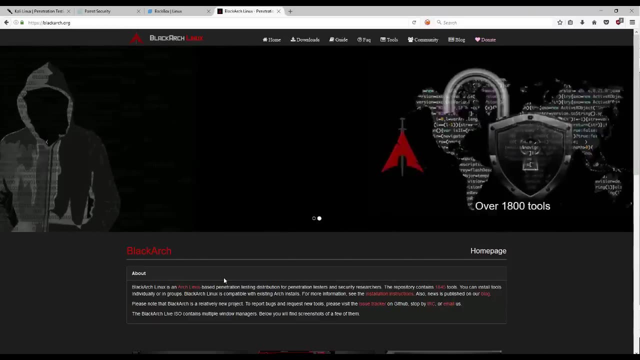 tell people to to understand what they're dealing with. now, the reason black arc was created is basically, if you've ever experienced a Linux distribution, you know that the the uh. basically, if you switch from Debian to Fedora and arc, it's kind of different in terms of navigating yourself. 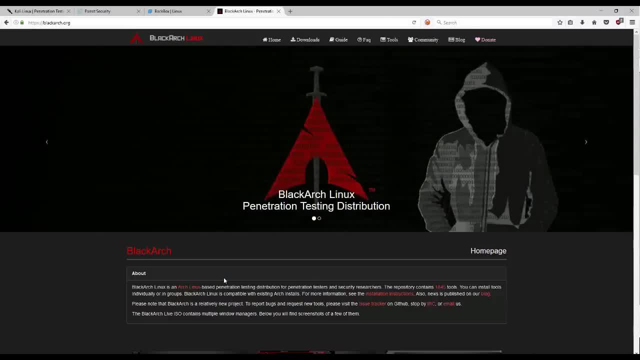 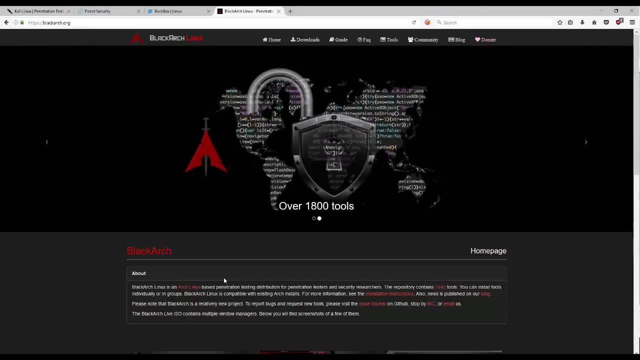 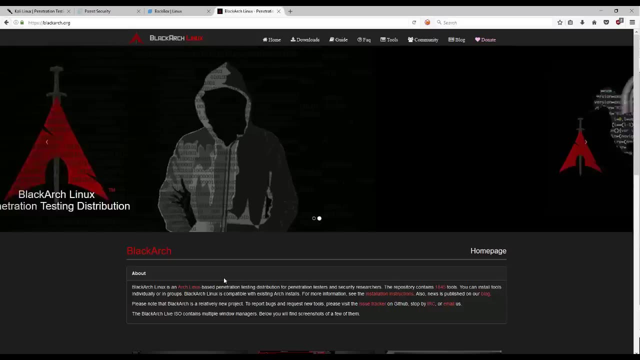 or moving around, uh, or just basically using the operating system. the, uh, the terminal commands are slightly different, and that's where I tell people: black arc Linux is good for people already accustomed to arc Linux. that's what it was created for. it was created to give people who are already familiar with using arc an option. 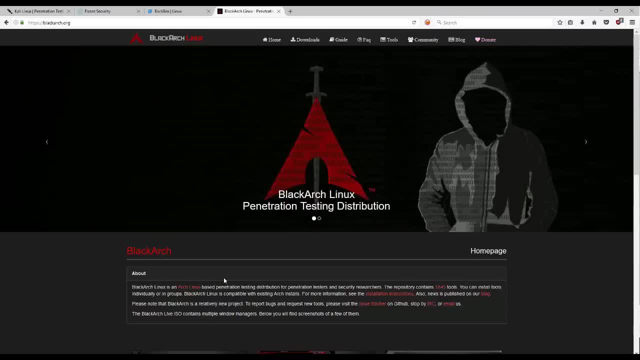 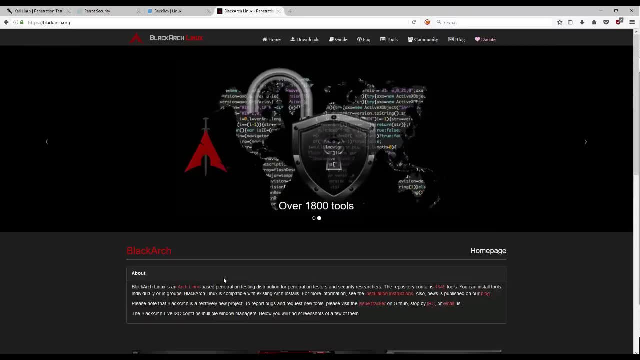 or an alternative to Kali Linux, because they found it also quite weird moving from arc to a uh to Fedora or Debian based operating system. so in essence, as you can see, black arc Linux is an arc Linux based penetration testing distribution for pen pen testers and security researchers. 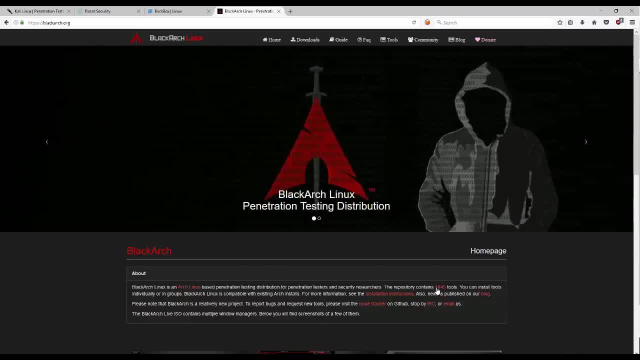 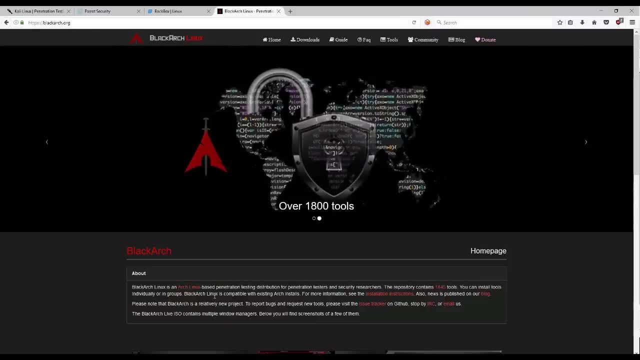 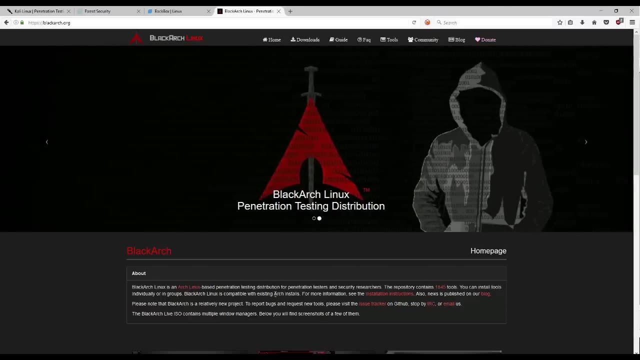 the repository contains 1845 tools. you can install the tools individually or by groups. um, basically, black arc Linux is compatible with the existing arc installs. let me just stop you right there. so that's basically what I was trying to point out. you can already, you can install it on. 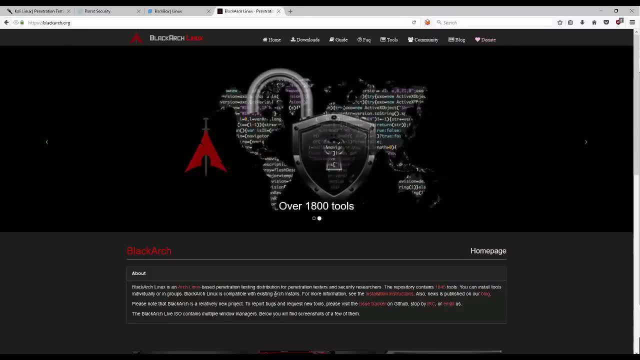 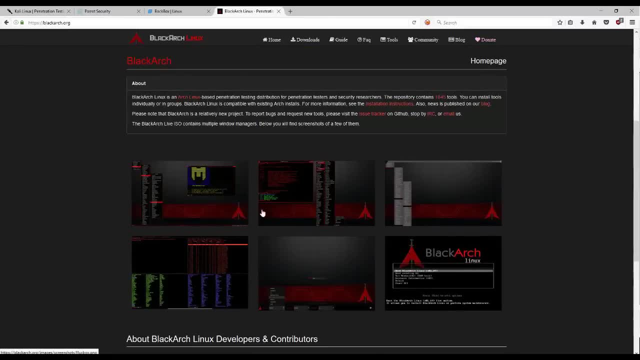 top of your arc installation and will work perfectly. now, uh, if you go ahead and see the screenshots, it doesn't come with much of uh of a desktop environment. so I, in my opinion, I would not recommend this for beginners. I would recommend this to people who are already accustomed with. 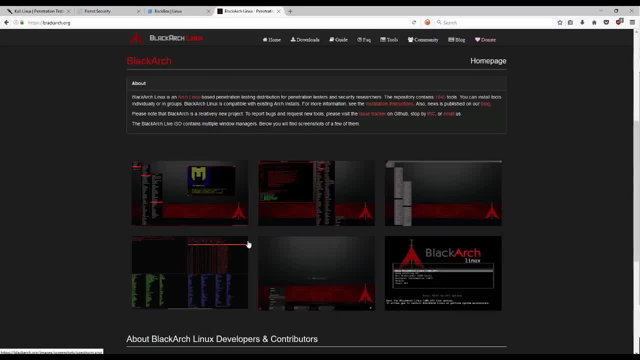 arc Linux firstly. secondly, a person who is used to using uh, who is used to installing and customizing a Linux distribution. so if you're good with Linux and you're you've been using Linux for a while now and you know how to install the dist, the different desktop environments, uh, this would would be an 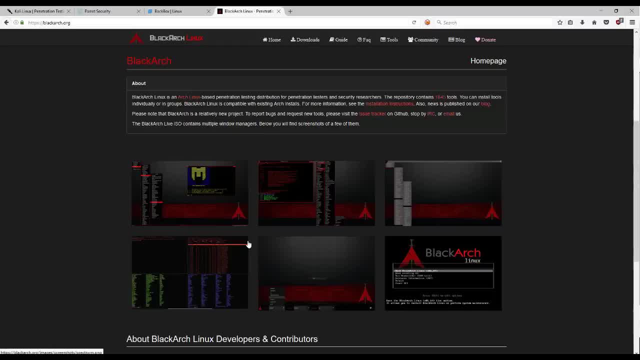 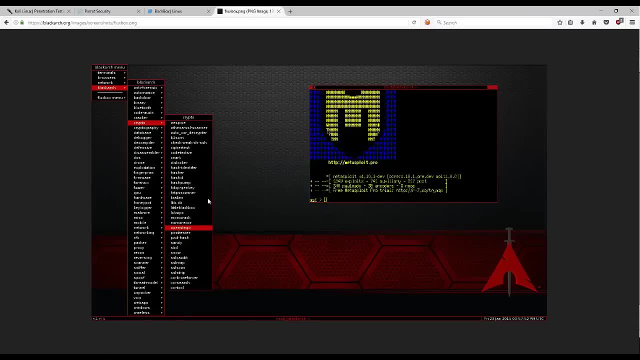 option that you might want to check out. um again, you. the review will be on the top right of the screen. I have made a video on it and, as you can see from the screenshots, it has all the tools you have: metasploit, as you can see, you have your cryptography. uh, it has a lot of stuff and the 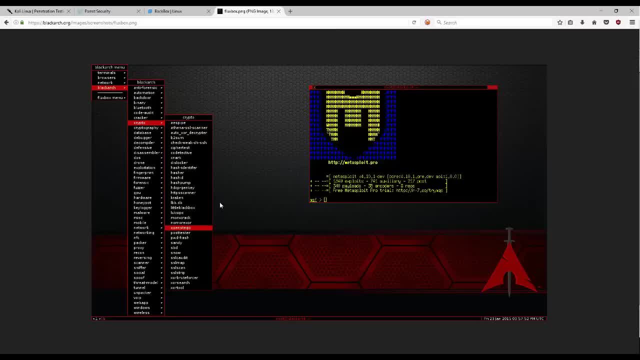 thing I like about black arc Linux is that it's categorized really well: the tools. it's a singular operating system, meaning that it's mainly going to be focused on penetration testing. it wouldn't work really well as a daily driver, so to speak, for web browsing. it would work, but it wouldn't. it wouldn't. 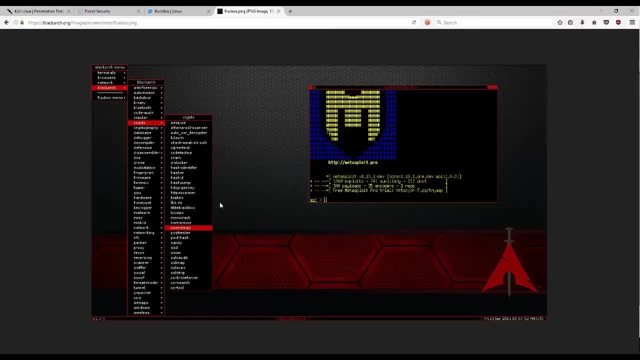 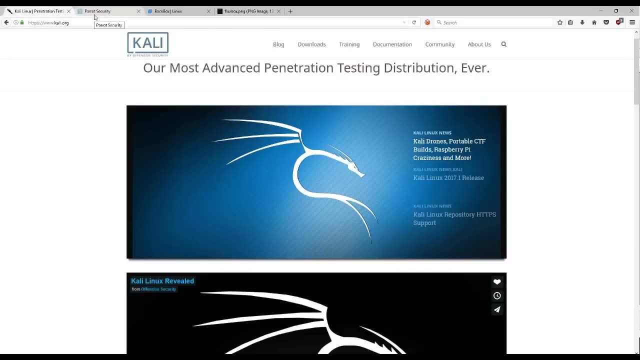 work well. so that's where I would uh just throw out a bit of caution right there. if you're expecting a more polished operating system, you might want to check out uh, possibly uh pirate OS. so that's basically it, guys. uh, you can go ahead and check these uh the websites in. they will be linked in the description section. again the reviews. 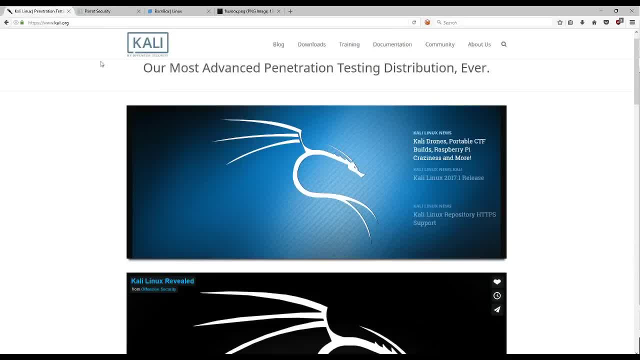 will also be uh linked throughout this video so you can go and check them out and make your decision. so thank you so much for watching this video. guys, if you found this video helpful, please leave a like down below. if you have any questions or suggestions, let me know in the comment section. you can also hit me up on my 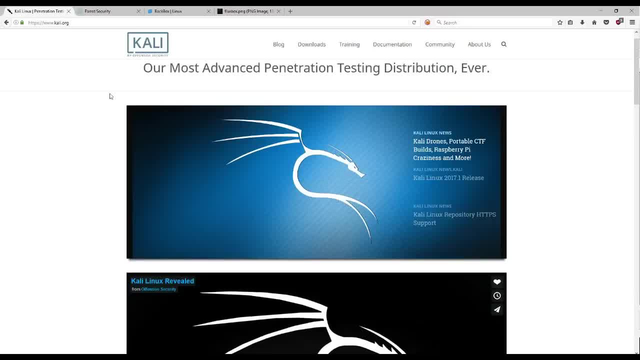 social networks. if you want to ask me personal type of questions, uh, you can hit me up on kick uh. in addition, I've also set up a Discord server. the link will be in the description section for those of you interested in joining, go ahead and join and we can discuss all uh, whatever we've 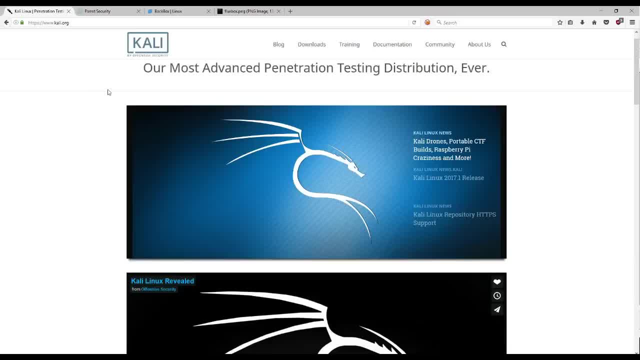 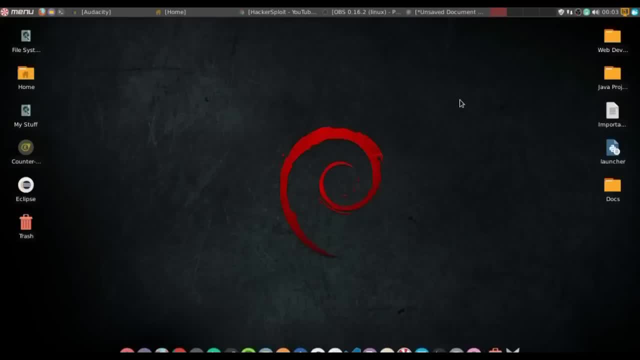 been doing really. so thank you for watching this video, guys, and have a fantastic day, peace. hey guys, hack exploit here back again with another video and just a quick, a little tutorial video before we move on to the next tutorial, um, of the next video in this series. uh, a lot of people have 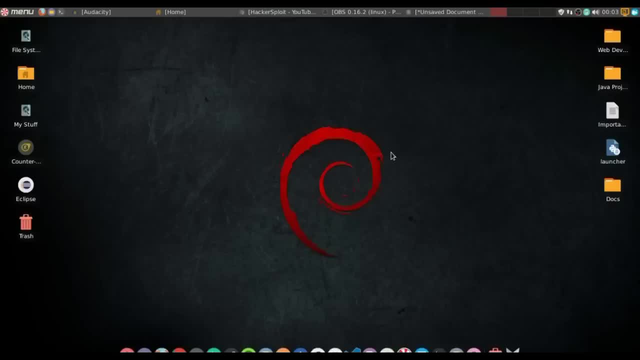 been asking me, uh, which distro I would recommend for beginners. now, look, I have no specific distro. I use a lot of Linux distros every day. as you can see, right now I'm using a peppermint OS as my desktop distro. I use this as my daily driver on my main computer. 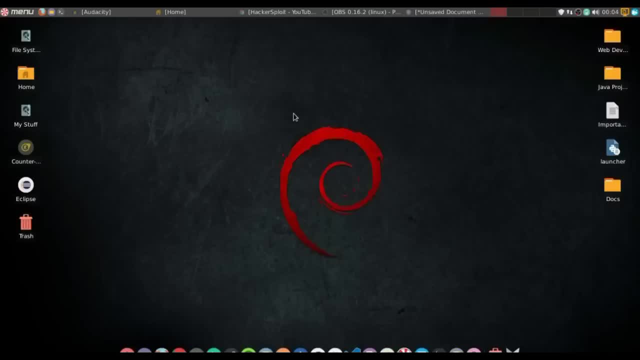 and uh, the people have asked me: well, for ethical hacking, what Linux distro do I recommend? well, as you know, there are- well- actually you may not know that there are actually 12 to, I think, 16- penetration testing distros out there, and it can be really intimidating selecting the correct one. 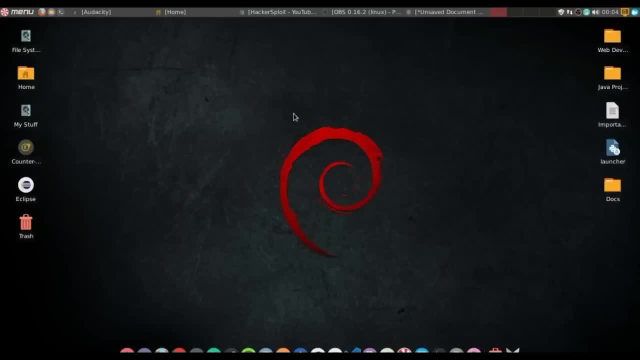 for you, and the truth is there isn't a correct one and the what I'm. the reason I'm saying this is because I can install all those penetration testing tools on version or any linux distro, and i'm going to show you that right now i'm going to install all those. 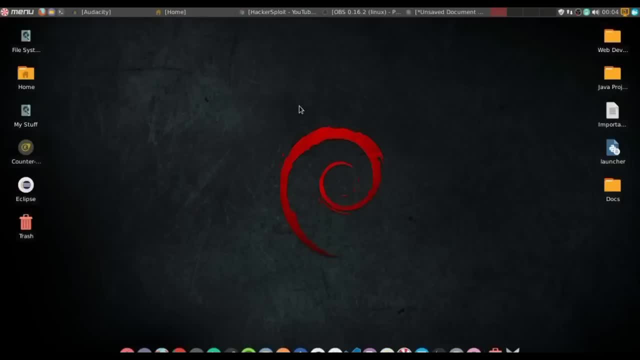 kali or parrot os tools on peppermint os or any version or or any linux distro for that reason or for that matter. uh, for example, you can do it on ubuntu, linux mint and you can actually use them as penetration testing distros. uh, so, uh, really it you. it all comes down to what you're. 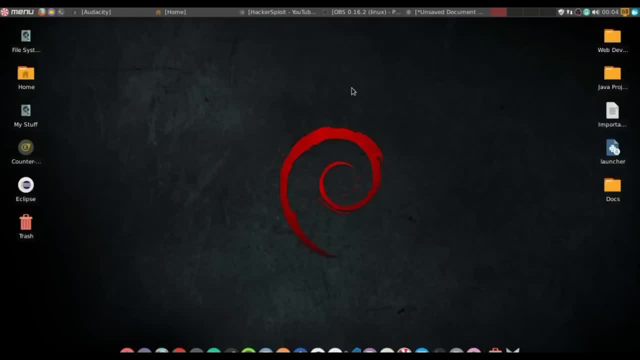 comfortable with. so if you want to install these packages on any linux, just all you want to do is um. by the way, i'm going to be showing this just for the debian uh distros, for arc videos, or maybe i'll make another one, but this is just for debian uh distros, because that's what both. 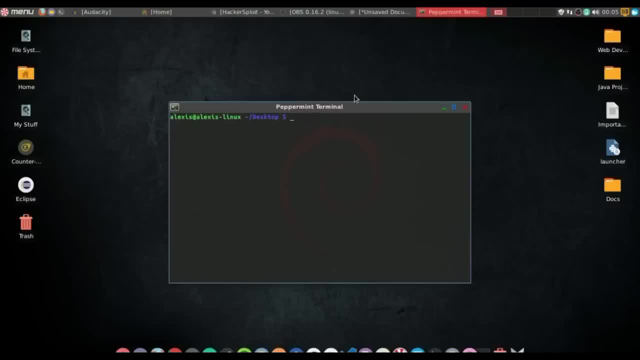 kali and apparatus are based off. so i'm just going to open a terminal here and i'm going to enter my root. so i'm actually on my route right now and i have a couple of commands. i've put them in a text document. they will be in the description section, so you can just 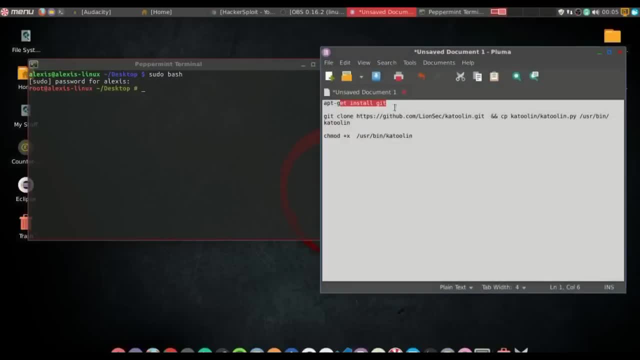 go ahead and type them in and they will be in the description section, so you can just go ahead and copy it from there if you don't want to type them out. uh, so first thing you want to do is you want to basically install git. all right, so the only make sure you install git so you can access the github. 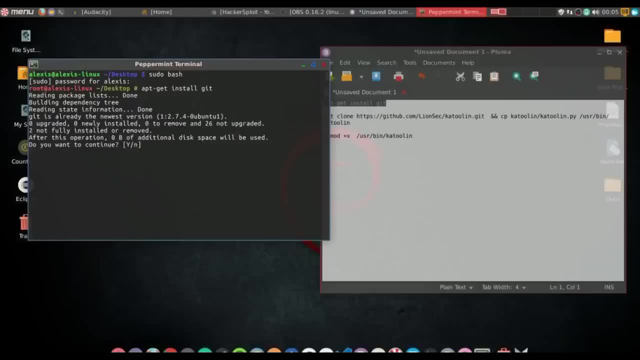 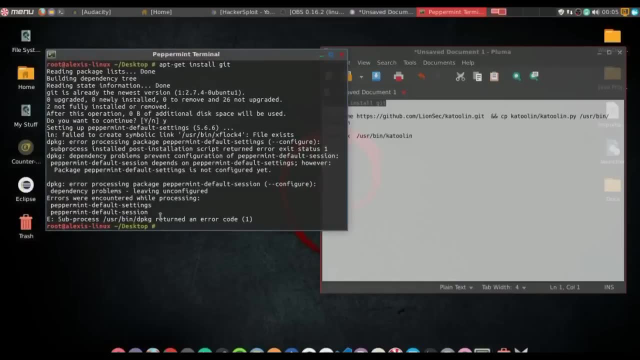 repositories. uh, so it's going to read the package. i already have git installed, so it's going to ask you to install it and you'll pretty much get install it. uh, don't worry about this error code. this is a personal uh, basically just something that happens in peppermint os. next thing you want: 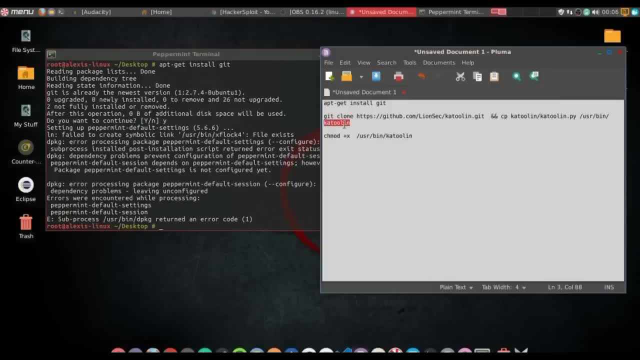 to add is the: uh, you want to add the github repository, so you want to add the github repository. is the katulin. this is basically the, the repository on github that basically gives you access to these tools. so you want to add that repository, so just add it. i already have it. so 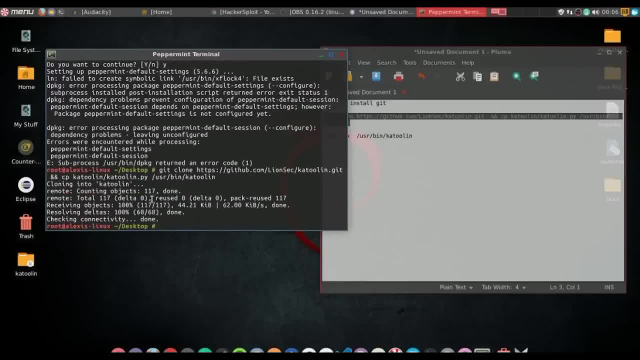 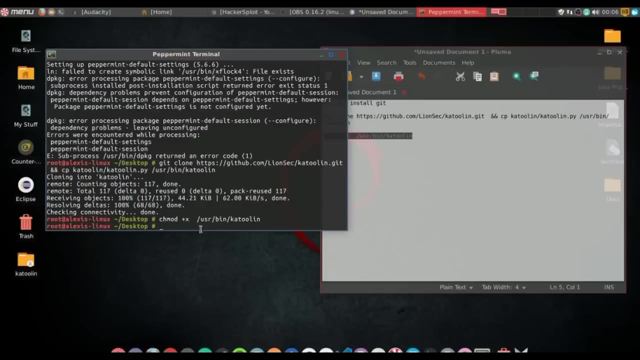 i really do not need it. as you can see, just cloned it um. next thing you want to do is you want to turn the katulin into a, an executable, so you're going to use the chmod um command. we're just going to paste that there and we're going to run it, and it's because it's not going to give you any. 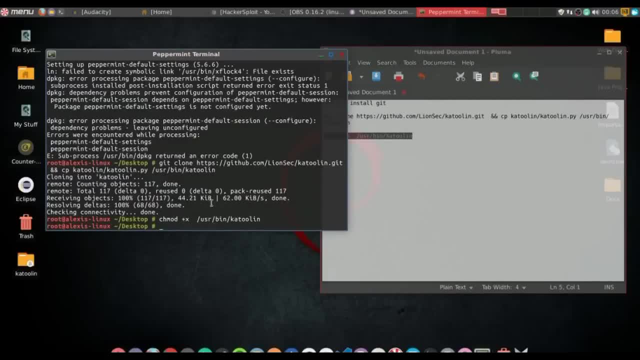 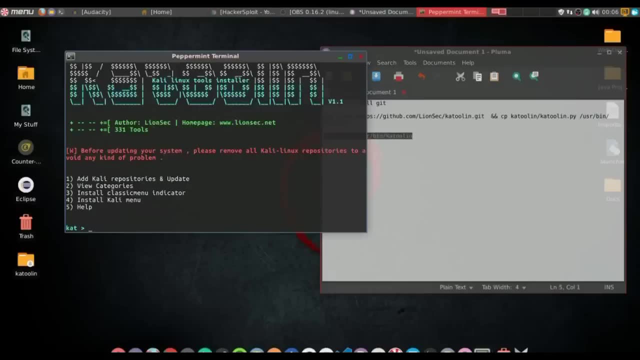 uh, any uh result or any message? uh, so, pretty much after that. uh, you should be good. now all you have to do is just launch katulin. um, just launch it and there you are, katulin. so basically, these are all the kali linux repositories. uh, so, as you can see, you can actually add them and update them. 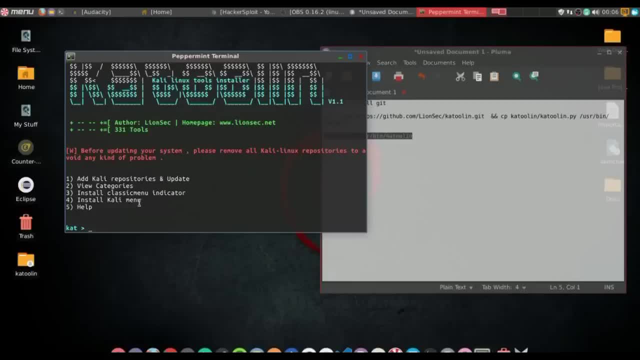 you can view, you can install the classic menu indicator and the install the kali menu. so really, as i said, uh, you, it's not up, it's not really about the linux distro, it's just about what suits you best. so, as you can see, we have- if i just view the categories of what 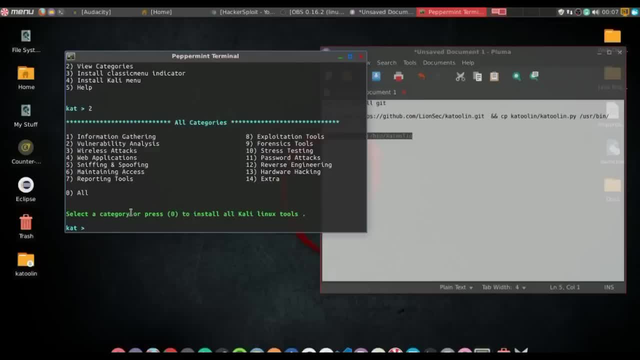 i can install. you have all the actual um, the actual sections in the in both kali, linux, black arc, um actually on almost all penetration penetration testing distros. excuse me, uh, so you have information gathering and there you can really find uh tools like nmap, hping 3. 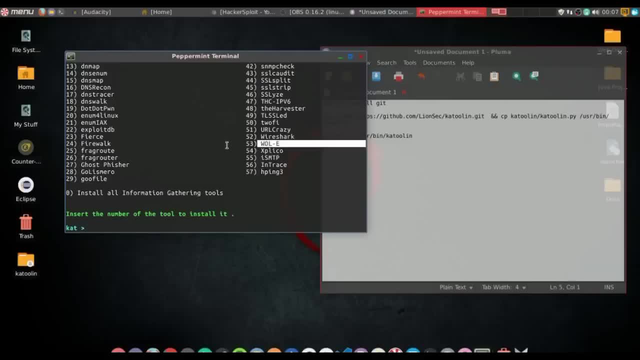 explico wireshark. so really you can install anything you need and specifically what you need. so if you guys are really not keen on moving to kali, linux or parrot os, don't worry, you can actually install all the packages from here and still run your distro, the. 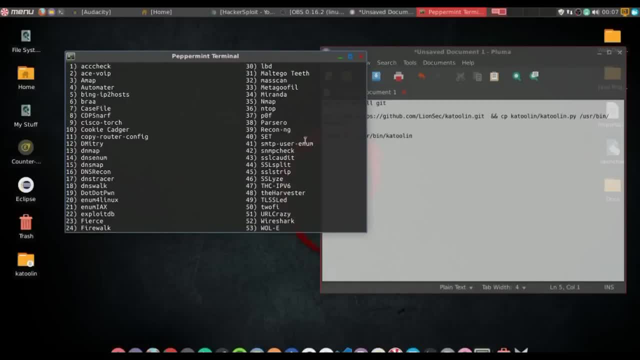 way it is. so you can actually run ubuntu with these tools, and that's actually an advantage, because ubuntu is much stable than kali linux, uh. but i really have seen that parrot os is quite, quite stable. i i have installed quite a bit of packages and it's run in pretty, pretty cool. 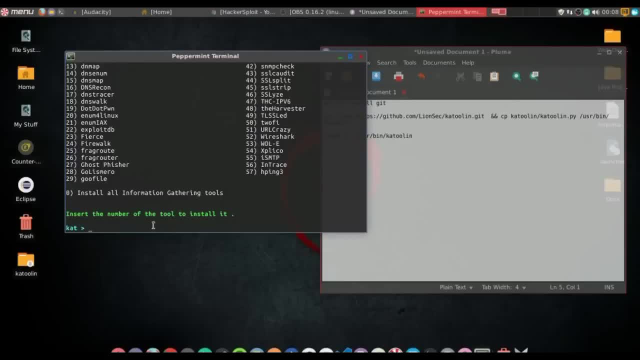 anyway, enough of that. this was just a quick little tutorial before we proceed, and just to clear up the the the air on people who are still on the fence as to what uh distro they want us they want to use. anyway, guys, that's basically it for this tutorial. uh, quick reminder, i'm going to 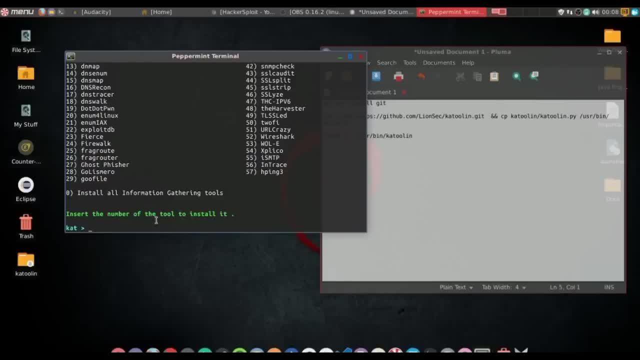 be continuing the ethical hiking series. uh, the video will be right after this one. uh, just a quick uh reminder that tomorrow we're actually going to do the deep web video, so that'll probably come any the afternoon to the evening. i just wanted to let you guys know that's every saturday and i also was. 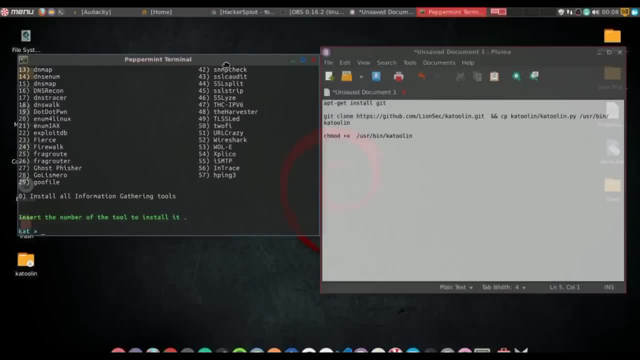 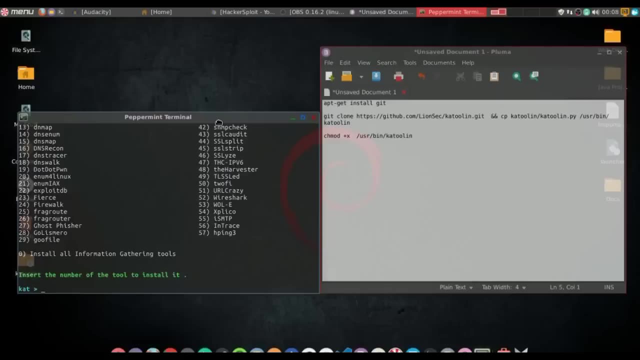 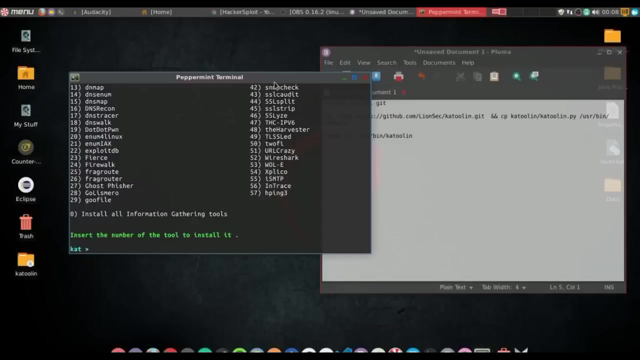 thinking of starting a new series, maybe on sunday or even possibly on saturday. uh, basically an ask me, a video where you can basically ask all your questions. maybe we can run it live and i can answer them live. so, yeah, that's up to you guys. let me know in the comment section below, otherwise, guys, 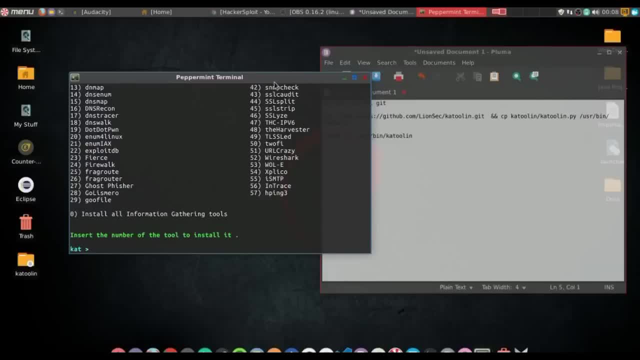 thank you for watching the video. if it helped you, leave a like. if you didn't uh dislike the video and if you have any questions, hit me up in the comment section or in on any of my social networks. i will reply to your question. um, if this video again, if this video did help you, please share the video. 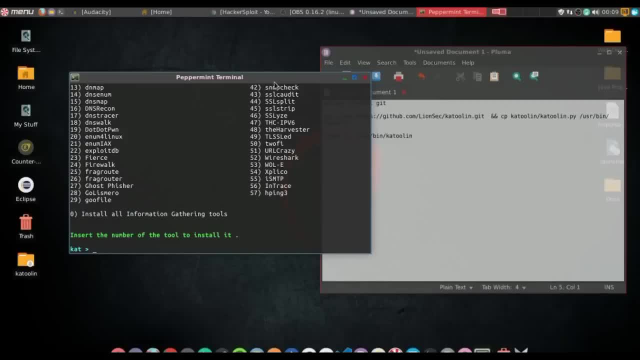 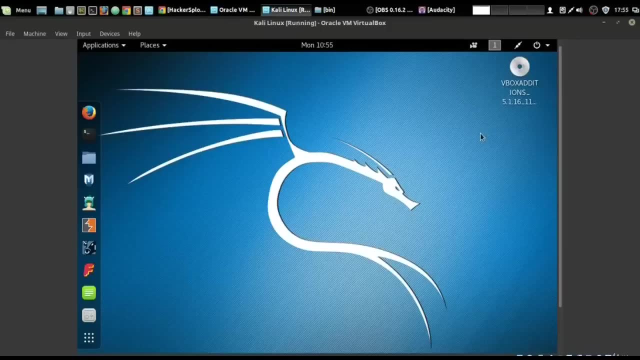 it really helps a lot of people and it will help me, uh. so, yeah, guys, uh, thank you for watching and have a fantastic day. peace, hey guys. hackersploit here, back again with another video and welcome to back to the ethical hacking course. now, in today's video, we're going to be talking 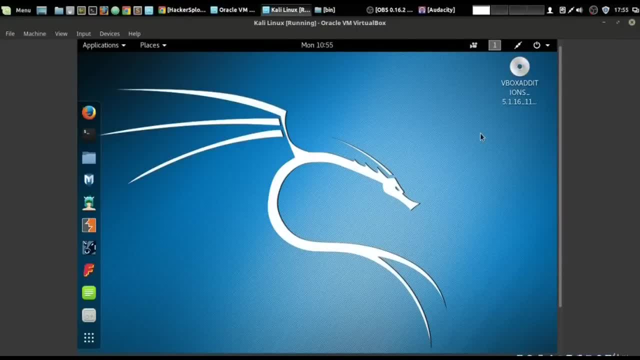 about proxy chains. so you might be asking yourself: what are proxy chains? well, proxy chains are a series of proxies that will basically give you anonymity or or will anonymize anything that you're doing, whether it be it being- uh, you're performing an nmap scan or you're performing a brute force. 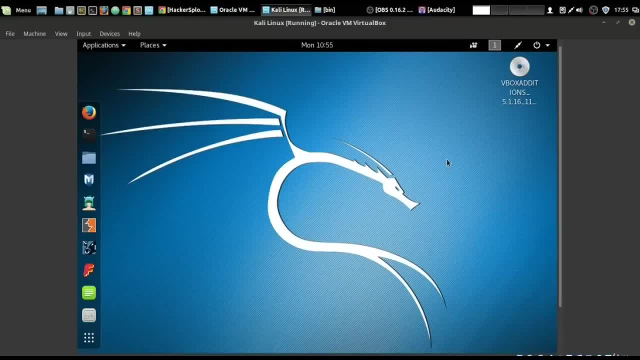 attack, or you're performing sql injection or you're just browsing the web. this will basically anonymize anything that you're doing. now you might be asking what's the difference between a proxy? well, proxies are usually found in browsers and they basically anonymize http connections or web connections or things that you're doing on on the internet, whereas proxy chains will. 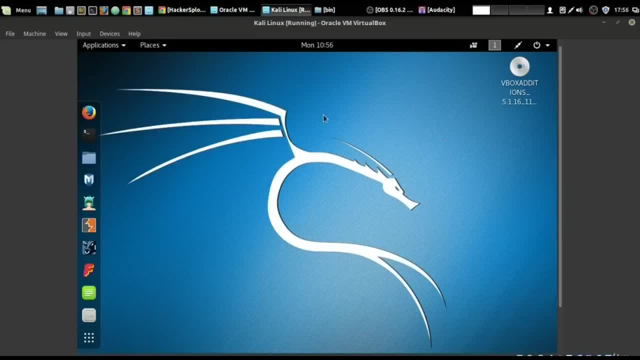 basically anonymize all the activities that you're doing now, when, when, using the penetration testing distros, proxy chains are already installed. so i would recommend, if you're ever going to configure them, just use a penetration testing distro, as it will be much easier. so in this video, you can. 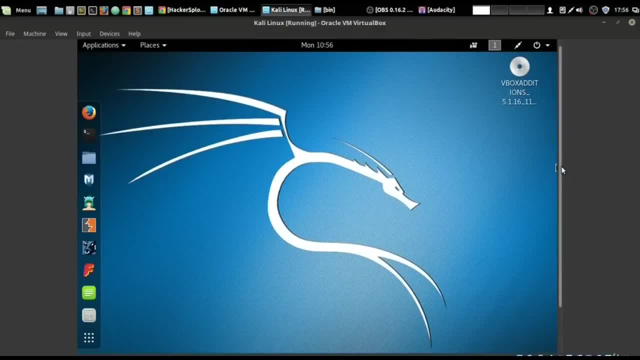 use using kali linux. uh, that's because i just want it to be a bit diverse. i don't want to select one distro and go with that. i'm going to use the different distros because i know a lot of you have different uh distros and you. you might feel that i'm ignoring those distros, but i'm not. so anyway, 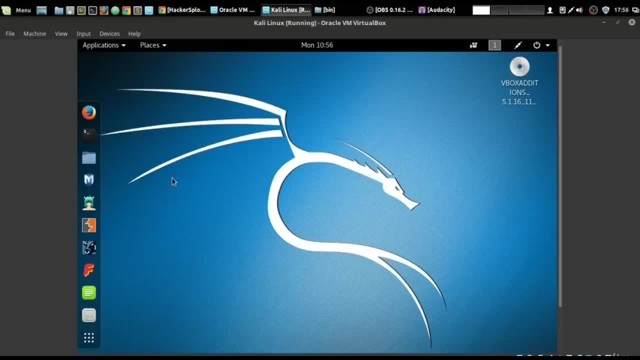 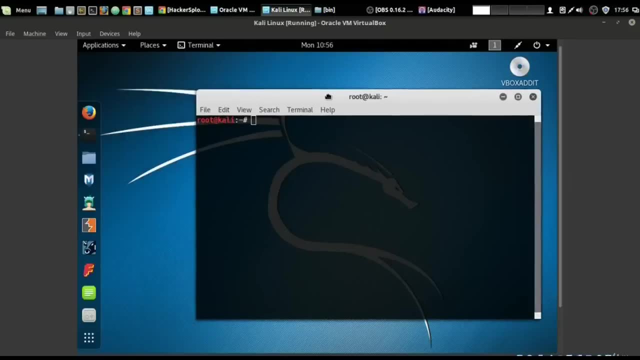 this is basically. proxy chains are installed on paratois, on kali, linux or even on blackhawk. so since they're already installed, all you have to do is open the terminal, like you always should and, uh, have to actually to configure the um, the proxy chains, we have to. 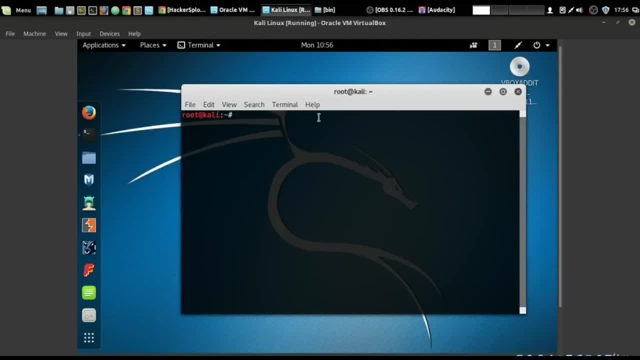 use the proxychainsconfiguration file, which can be found in the following directory. so the first thing we're going to use the nano editor and we're going to say etc or etc. that's the directory we're going to go into, because kali linux is already in the root directory. we then 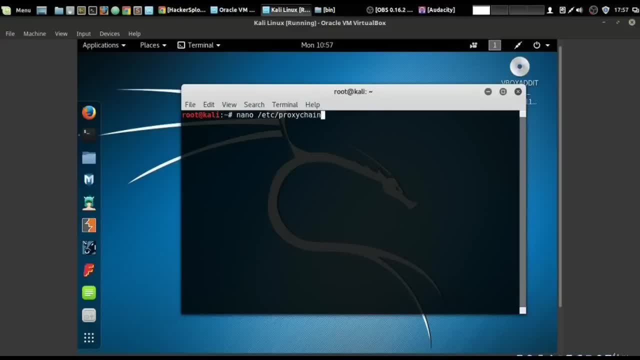 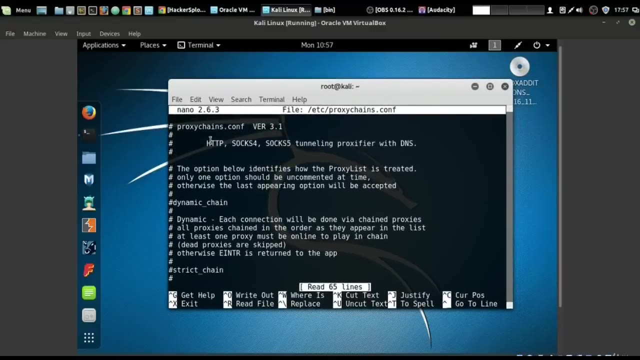 want to select the proxy planes. proxychainsconfiguration, configurationc- onf for it. that's the dot configuration extension, all right, so uh, enter there. we are very cool. so it's using the nano editor and it's going to open the file. so we're using proxychainsconfiguration. 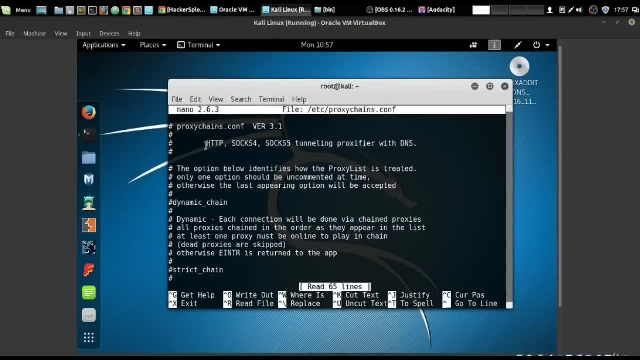 version 3.1 that comes in the latest distros. now let's start with. the first thing that might appear uh new to you guys is these hashes here, or these hashtags as they are called. well, basically, the hashes are just comments in the configuration file. what i mean is, if you ever have done programming, you know that when you comment it's just for. 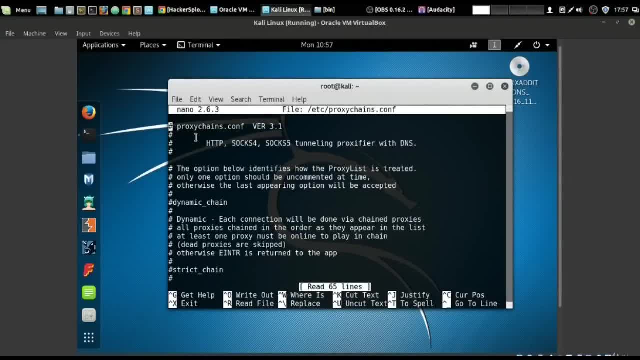 documentation. well, these actual commands, but they've been commented to turn them off, so i'll get to turning them off in a second, so don't worry about the hashes now. another important thing is this line here now: http: socks 4, socks 5, tunneling, proxy fire with dns. these are basically the formats. 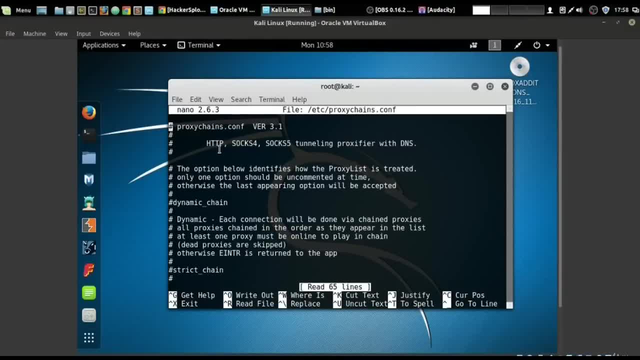 of proxies. http proxies are. you're very familiar with them. they're being used in the top browser. sox4 are really not popular anymore, but they anonymize pretty well, and sox5 is what we're gonna, what, what i would recommend and what we're gonna use in this video, and they'll basically um, they'll. 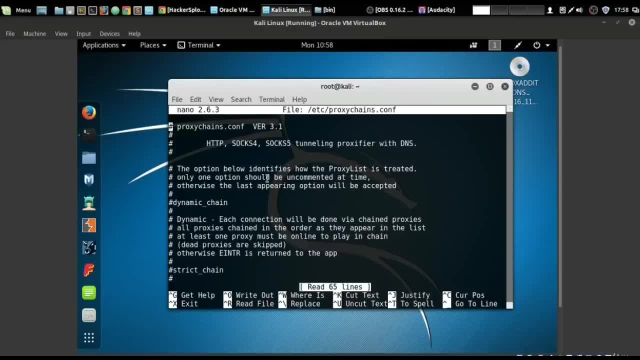 anonymize everything that you're doing on your system. um, all right, so we have explained what that is. now let's go down here into a dynamic chain. now, this is the most important thing here: dynamic chains are the most stable and the fastest proxies that you can use and basically, the 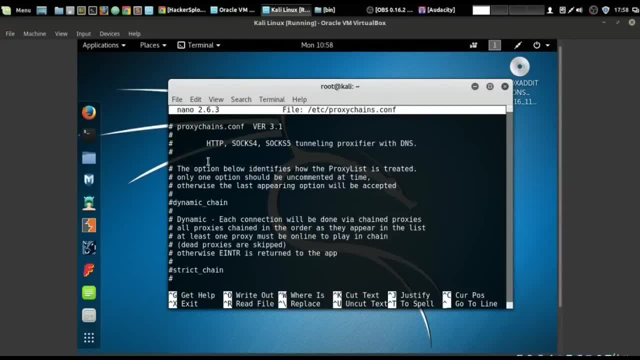 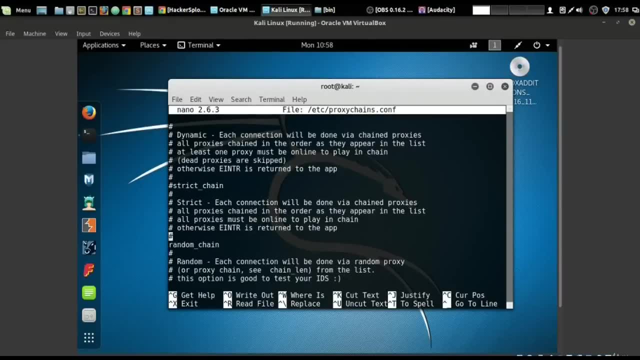 most common way to use them is by using a random chain. by the way, if you want to scroll down the configuration file, use your mouse wheel or use the arrows. i find the arrows much better because i can specify with a button or a key. so, as you can see, one of the lines is uncommented. we have the random. 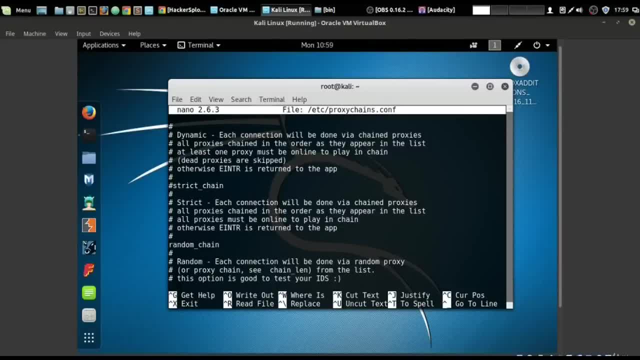 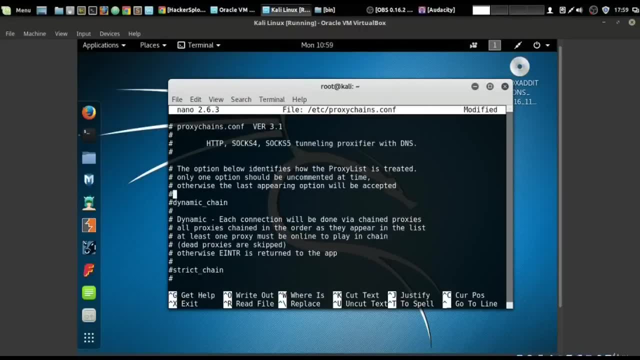 chain. now, don't worry about that. let's actually just comment that for this, um, for this video, what that means is that it's just going to use your ip address, so the proxies are really not active. if you activate a proxy, we'll- uh, we'll- remove this. hash and dynamic chains have been activated so that. 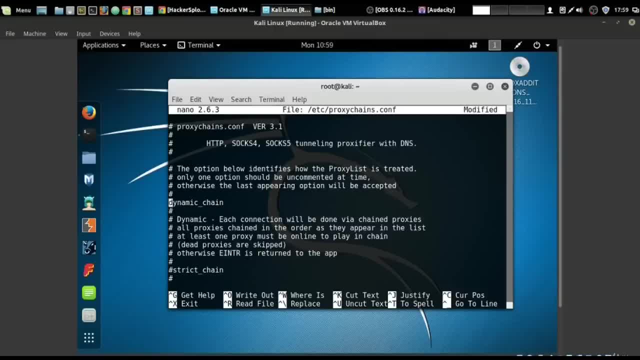 means you're actually using a proxy right now. uh, i'll get to configuring uh the proxy in detail just in in a second. now, dynamic proxies: each connection will be done by chain proxies, right? so basically this will will go through a series of ip addresses or proxies in different countries. 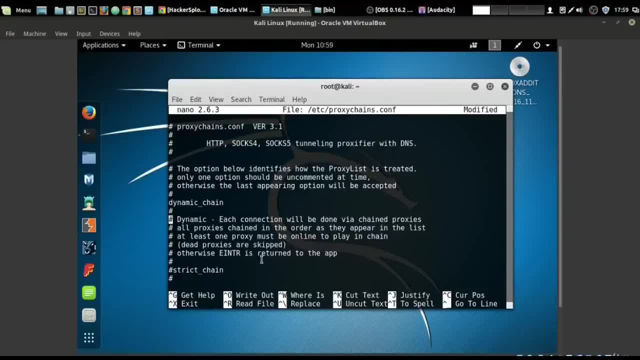 as we will specify down below in the configuration section. so the reason why this is the fastest is because, uh, basically it's, it's going through, uh, what i would, i would say uh is a very good system for proxies. as you can see, it's going to say here: all proxies chained in the order as they appear in the list. at least one proxy must. 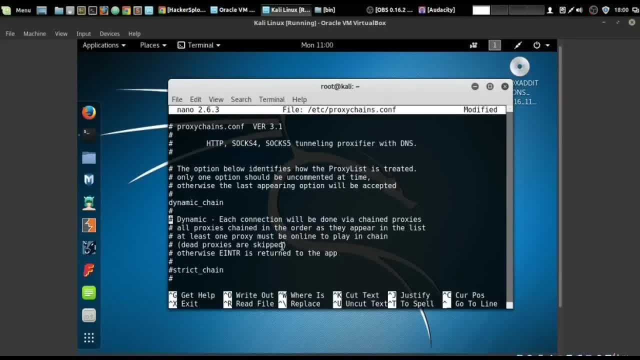 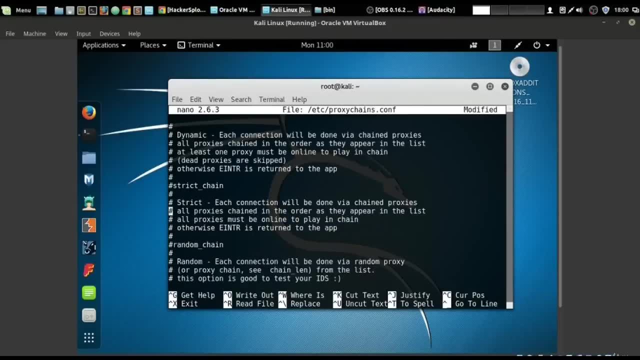 be online. we already know that dead proxies are skipped, so it will not go through a dead proxy and then prompt you that the connection is not working. uh, just ignore strict chains. for now that's a bit. strict chain will just stick to the ips that you've given it or the proxies that you've given it. 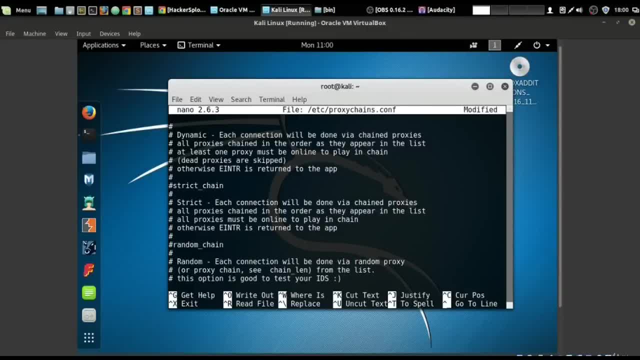 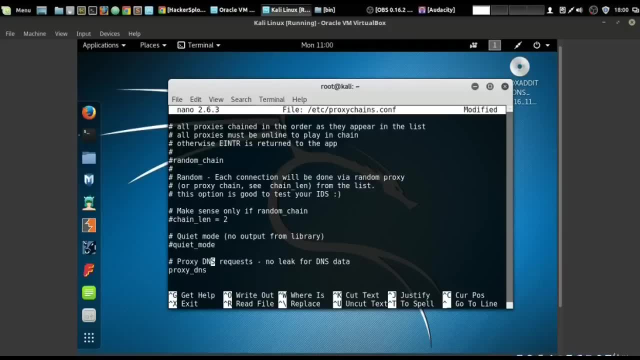 and it will stay to most. in most cases it will only use one of the proxies. random chain is just a normal connection. now in proxy dns requests in this section here i just want to explain something. this is usually where the beginners make mistakes. what this means: no leak for dns data. what this means is: um, usually, when, when, basically anonymizing your system. 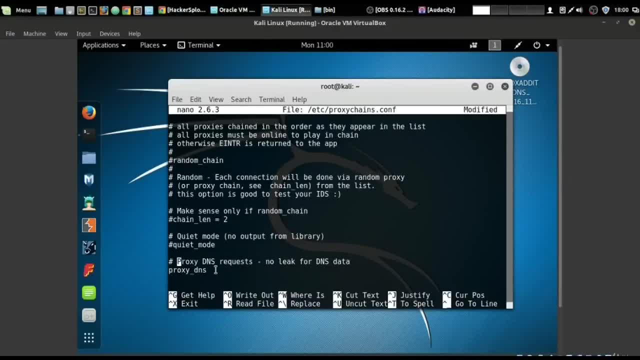 when you're performing anything. really, you can use a proxy, but you have to also change your dns. all right, let me explain why. most of the beginners will use a proxy, and it will change their location every five to ten minutes, or even faster than that. so it's bouncing all around the world. you're using 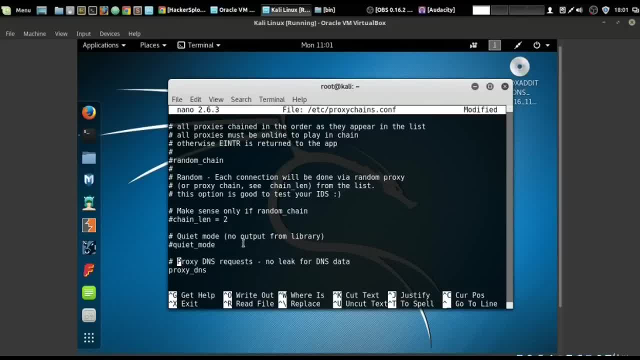 different locations, but your dns is in your in the country you're in. so when a website like youtube accesses, or when you access youtube, for example, it's going to log your ip. the ip will belong to, let's say, france, and, and you've not changed your dns, so your dns will show. 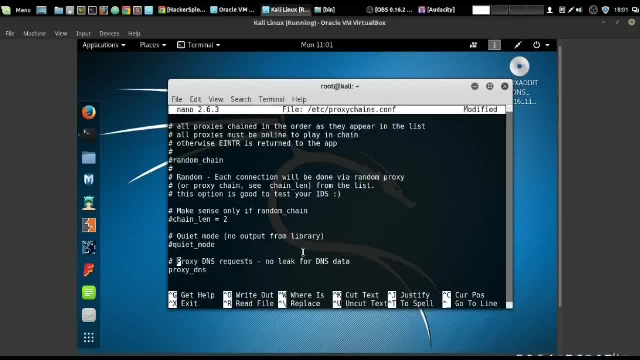 your host country. let's say, your host country is germany and you're accessing using a proxy. youtube will already know that you're using a proxy because they can see that you're using different ips and but your dns is in is one is in one country and from there they can track you and 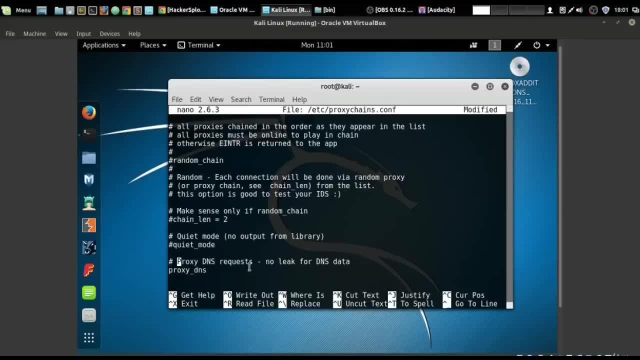 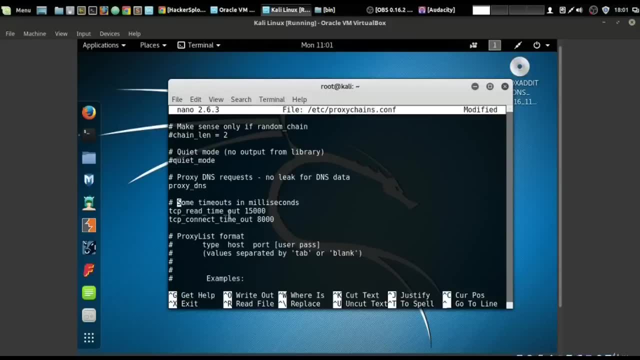 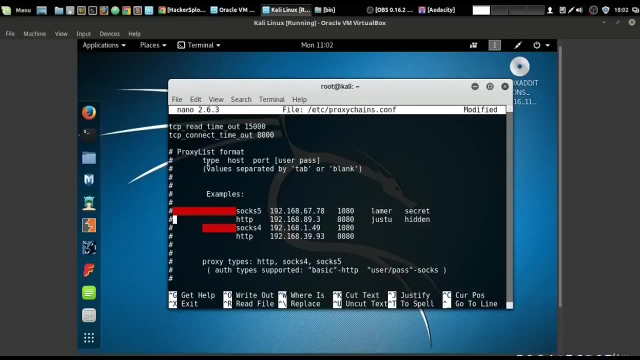 you. you get the idea. so always change your dns wills, uh, using proxies. it just increases your anonymity and just it makes you look, uh, a bit professional, not like a a non professional would go about it. so, um, let's go down to the proxy list format. all right, now, this is again. they'll give you like examples of how they would appear, so i 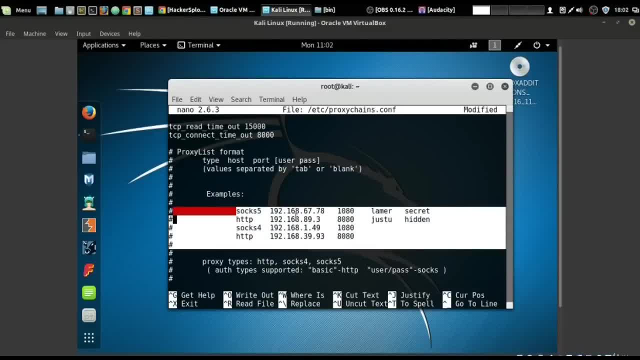 want you guys to pay attention to these formats here. just go over these formats and just look at, just understand the format. we'll get into configuring uh, holding the 5成背景, and then i'll just complete this page first and then we'll continue. 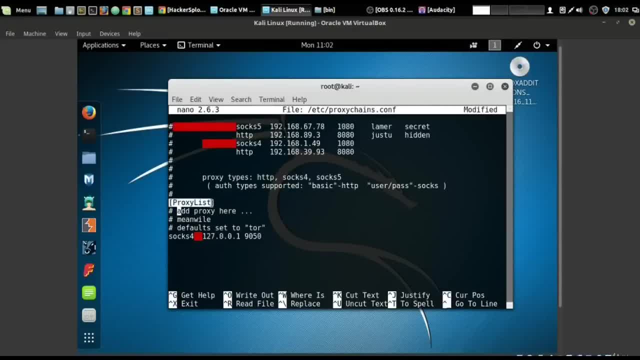 kind on the image is, but i always focus highly. right now you hit ok. so if you want, you can make and, and the proxy down below here. so, as you can see, this is the proxy list down below and uh. basically it's using a socks for uh 127.0.0.1950, which is the tor. 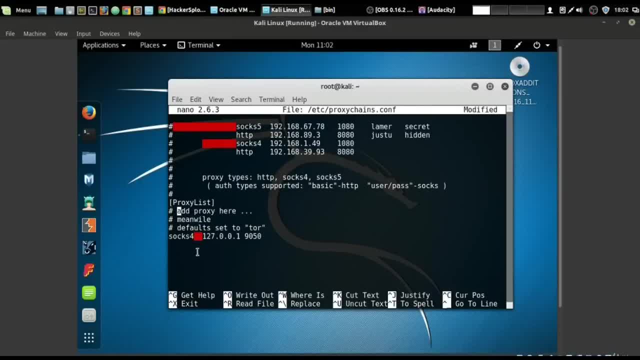 it's using the tor proxy, which it's saying socks for i know it's basically for http, so i'm gonna get in the to in the next video using your own proxies. so otherwise, guys, i hope this video helped you. if you did, leave a like. if you enjoyed the video, leave a like. if it didn't help you, let. 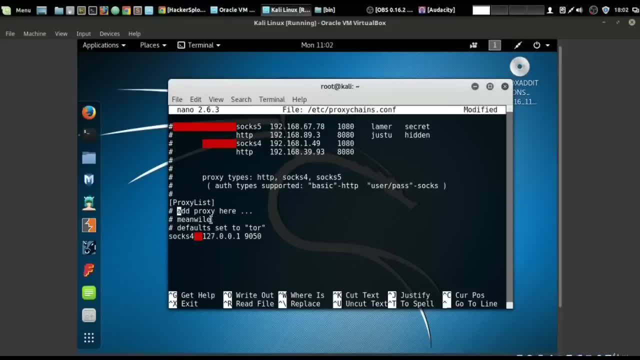 me know in the comment section. if you have any questions again, hit me up on kick my social media. by the way, don't forget to follow me on my social video on my social media. excuse me, have a fantastic day. the next video is coming soon. in fact, it's coming in a few minutes. peace. 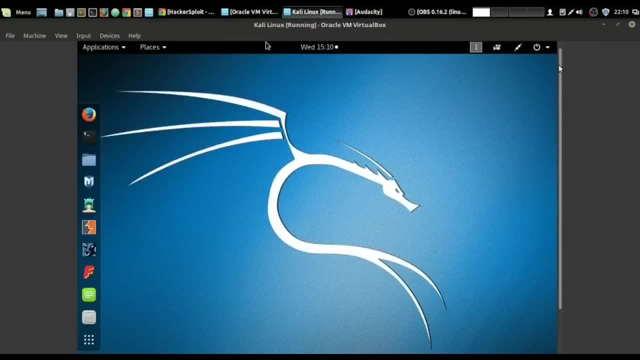 hey guys, hackersploit here back again with another video and welcome back to the ethical hacking course. today we're going to be talking about proxy chains. so this is actually going to be the second proxy chain tutorial in the video. i'm going to be talking about the proxy. 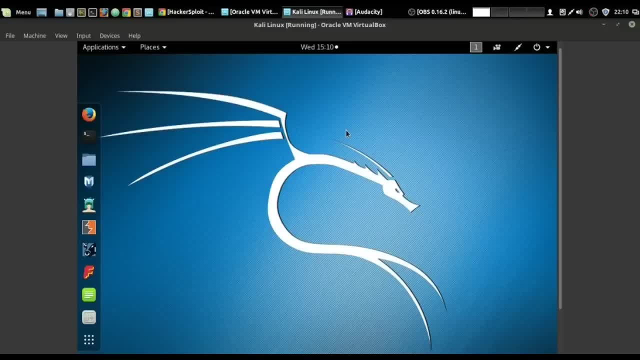 previous video I talked about proxy chains, what they are, how they work, and I introduced you guys to the proxychainsconfiguration file. so in this video, I'm going to go into some really advanced stuff when it comes to proxy chains. I'm going to show you how to set it up. I'm going to show you that it 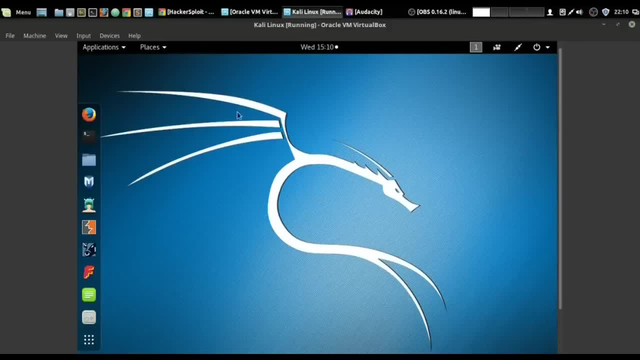 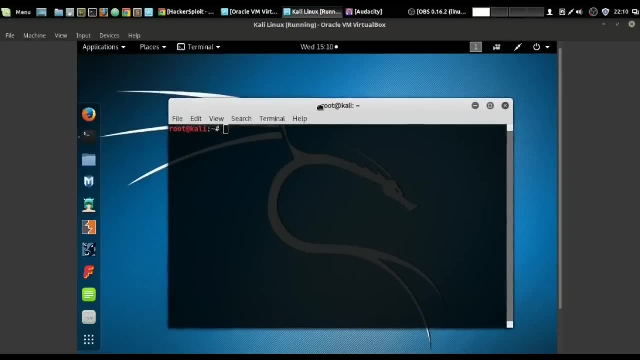 actually works live. so I hope you guys are ready. so let's get to it. so, like any other ethical hacking videos, it all begins in the humble shell of the terminal. so open up your terminal and let's get started. so in the previous video, I was using the nano editor, and I'm gonna keep on using the nano editor. 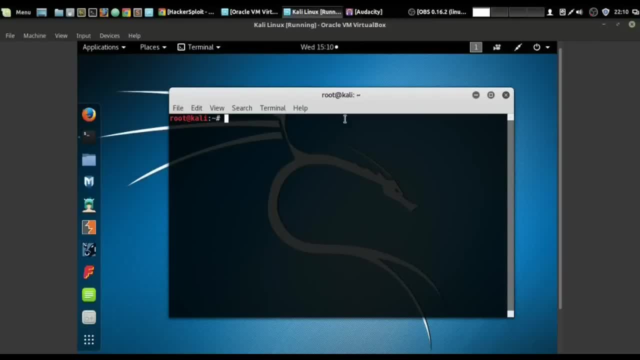 now let me explain why you guys might be asking yourself. well, there's the vim editor and there's so many others. why aren't I using any of those? well, I'm trying to keep these tutorials as beginner friendly as possible so that almost everyone can understand them and it's very easy for them to grasp the 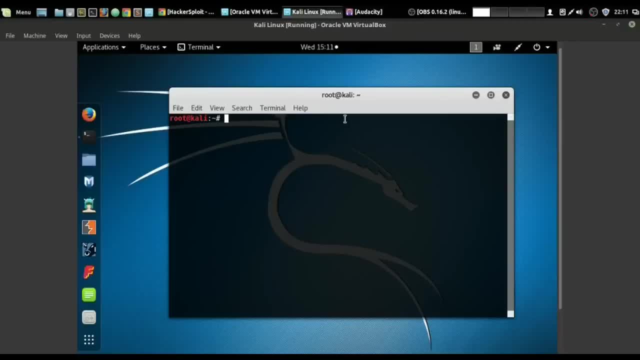 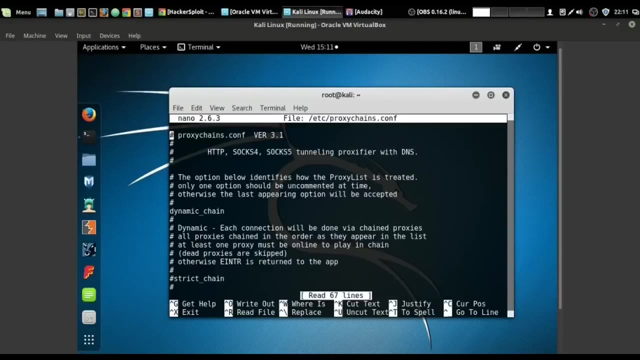 concept of editing a configuration file in the terminal. so let's get started nano, and we're going to access the proxychainsconfiguration file. we're going to go to the etc or etc and proxychainsconfiguration and let's open that up now. in the previous video I explained why we need to. 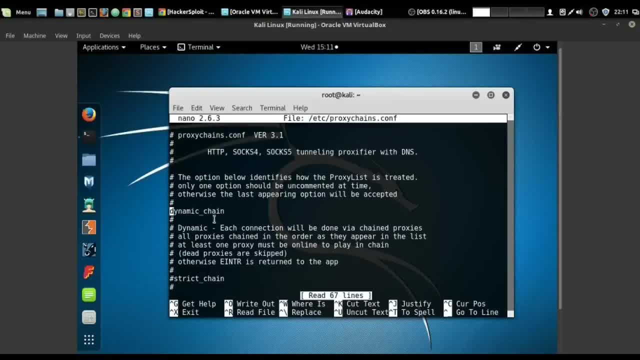 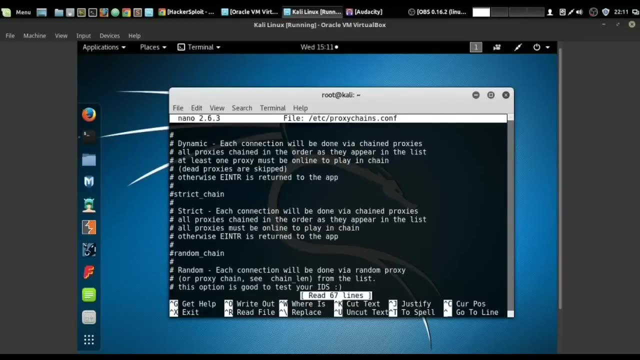 uncomment the dynamic chain. that's basically activating the dynamic chain. now, the dynamic chain will basically allow the IP IP addresses to change in a very dynamic, in a very dynamic way. so let's get started. so let's go ahead and update theatin. well, ok, this is actually important to say that. you know, these braces don't look like. 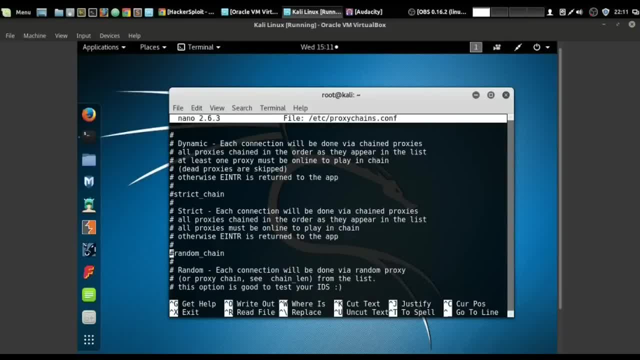 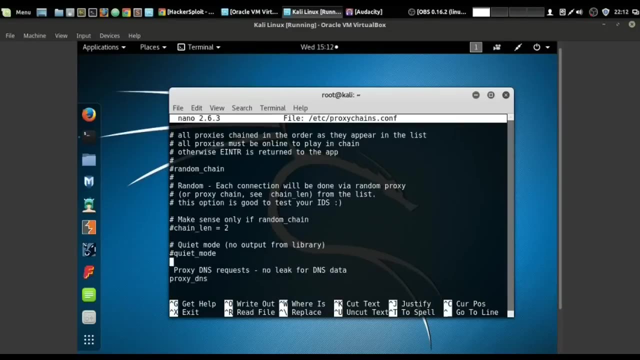 inka tong very smart braces? to be honest, its not�� so. usually when you don't have network, you just use a bootable keyboard and your proxy. it doesn't work. you're basically stumped and you have to restart the process all over again. so let's go all the way down. now I also. 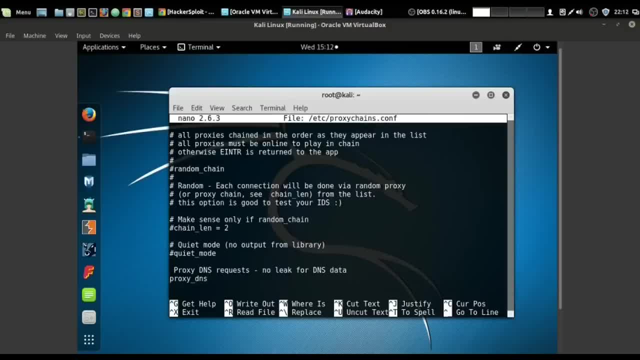 told you to uncomment the proxy DNS requests. no leak for DNS data. this is basically will will prevent leaking of DNS data. so your, even if you have not using a custom DNS that's in not in your country, it'll actually. it'll actually just follow the IPs DNS to whichever country that's in. so this is very. 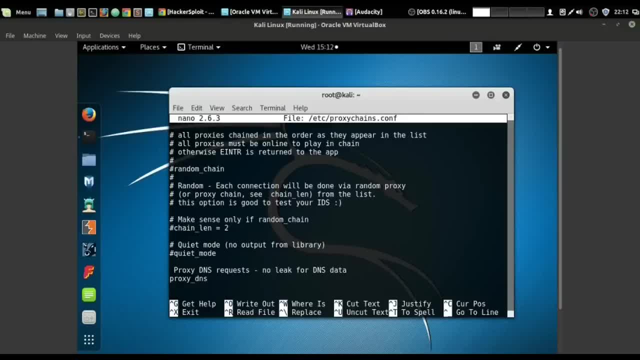 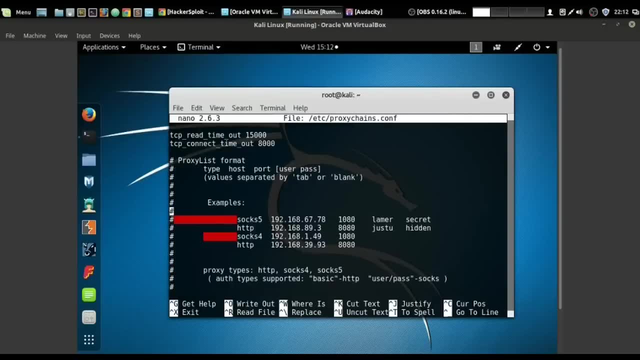 important. make sure that that active, and you can do that by uncommenting, as I did with the, the dynamic chain up there. so let's go down all the way to the example section now. in the example section I told you guys to take a look at the format of the, of basically how a proxy chain or a proxy fire DNS works. 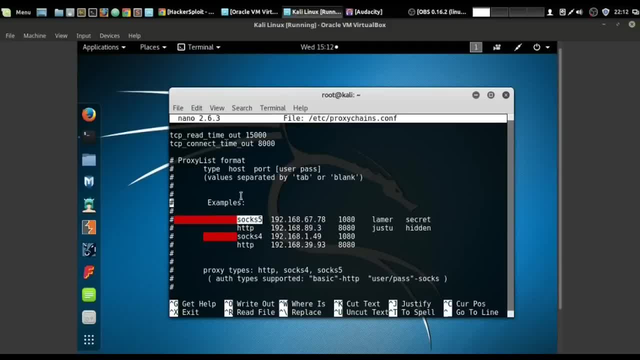 now, this is the proxy fire DNS. there is socks five. that's what you're going to be using because it's the safest and it's the fastest, really, and this is the first and it's the fastest, and this is the second and it's the fastest. 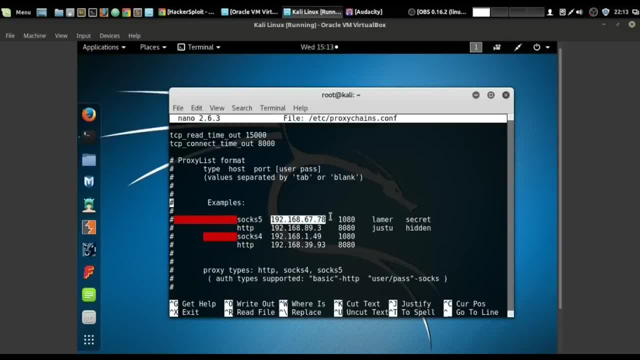 is the address of the proxy. not nothing really to say there. that's basically just the address. you then have the port. you guys know what ports are, and right here a lot of people have been asking me what this is. well, basically, this is the username and password examples. so if you actually 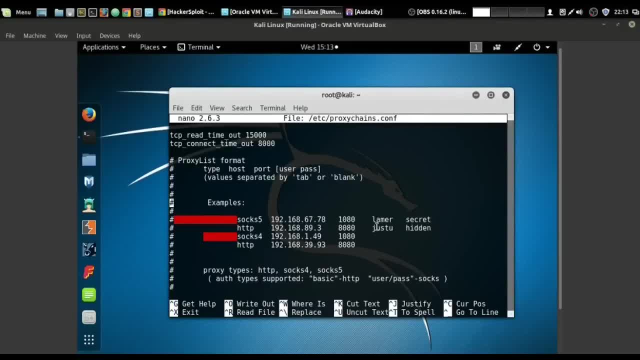 buy a proxy or a proxy fire or a proxy chain. in most cases they'll usually give you a username and password and this is where you get to enter them. so we're going to use tor and the proxy chains in in in interlation together, so they're actually going to work together. so let me explain. 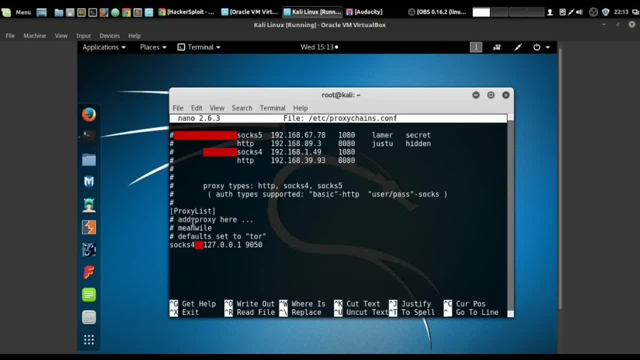 how we're going to do that. so in the proxy list section here, this is actually where we configure the proxies. as you can see, the defaults have been set to tor, but it's been used in the socks 4, but we don't want that. but instead of removing that, we're just going to use this one. so 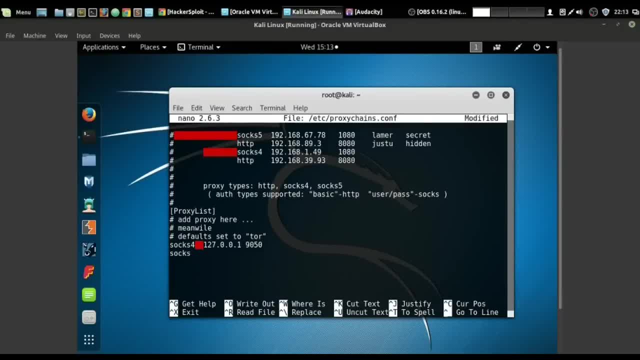 go to the line just below socks 4 and we're going to add socks 5 and you want to hit the tab button on your keyboard. that's basically. you're going to follow the format of the command above it, so it's going to form follow the format just above, which is a very good format: 127.0.0.1 and 90: 50.. all right now why are 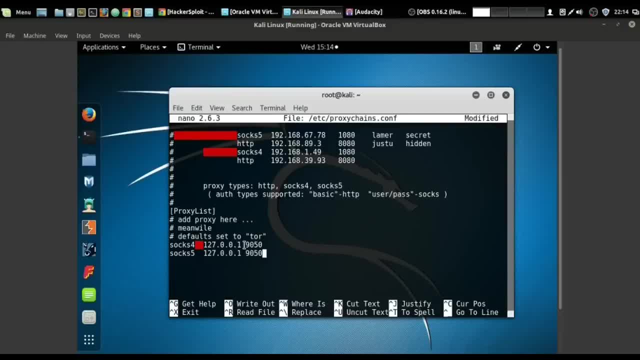 we using 127.0.01. firstly, that's the basic tor proxy configuration. that that's where the ip is and this is basically your ipn. this is how you can actually test by running this to test if the proxy chains are working. so, socks, we've actually configured and, to be honest, we're actually done here. now i'm going to show you the. 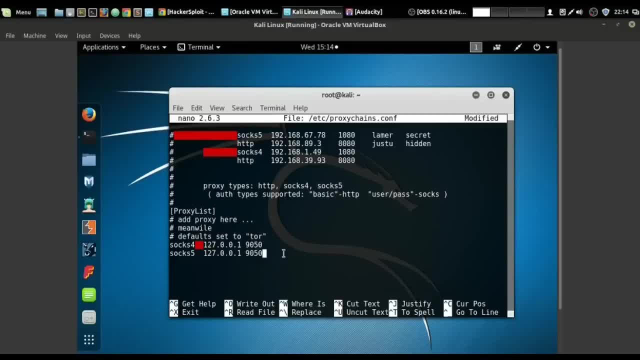 proxy chains. working with an example, or actually i'm just going to run it live. so we're going to save this file and to save the file you want to hit control o and it's going to ask you to write to to write the changes and i'm going to hit enter and it's written and to exit the nano editor hit. 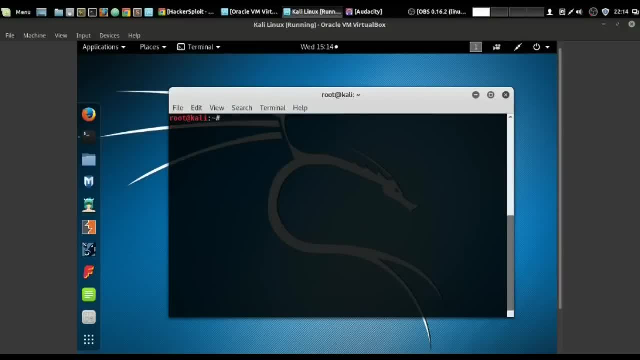 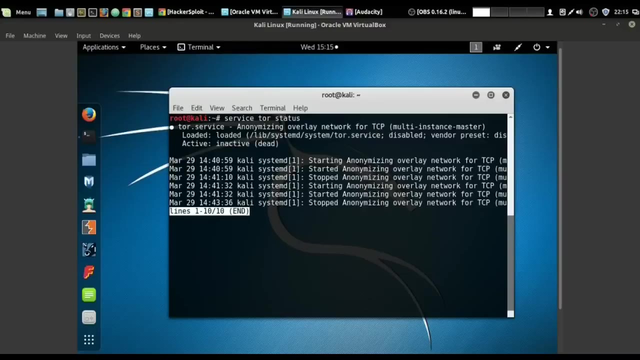 control x, all right, and we're going to clear the console and finally we can begin checking it. so the first thing we're going to do is we're going to check if the tor service is running. most likely it's not running, uh, so let's check. uh, tor service. actually it is running, um. 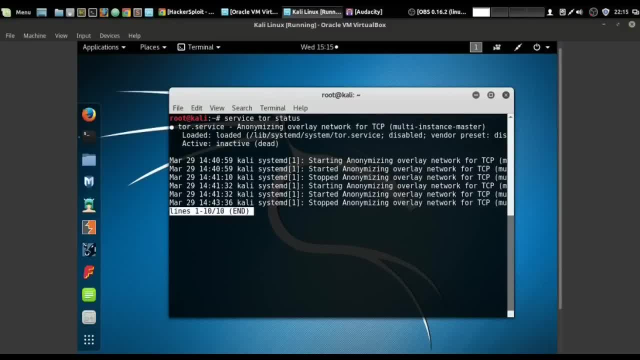 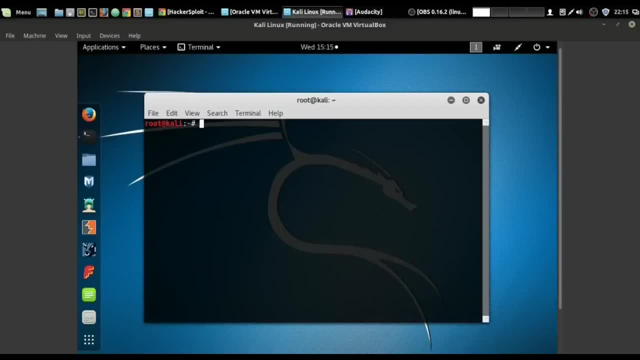 well, hold on, all right, uh. so what i'm gonna do is, um, what i'm gonna do is is i'm gonna close this terminal and i'm gonna open another one and i'm gonna stop it. stop, uh. actually, hold on it's service, all right, and I've stopped it. if yours is not open, don't worry, just skip this. 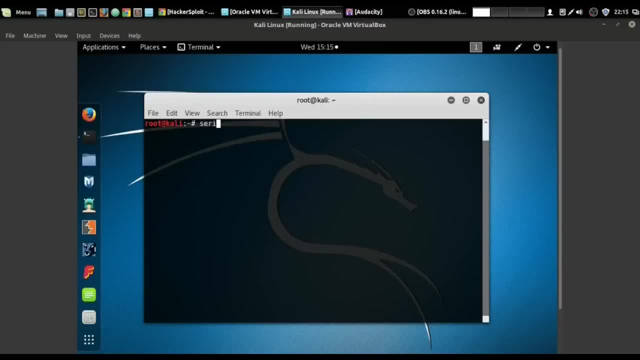 step and we're gonna start it again. service door start, all right, and I'm gonna hit service service store start and it's, it's gonna start the tour service. now we can actually begin with the proxy chains. as I explained, we're going to using, we're going to be using the tour proxies with basically going to 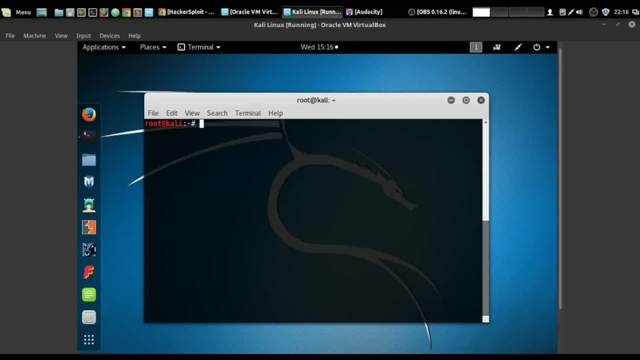 using the tour proxies with the proxy chains configuration file, at least for this video. so the way to test this is: we're going to type proxy chains, proxy chains. we're going to use a browser. I'm going to use Firefox. that's basically whoops. my typing today is pretty bad. Firefox: you can use ice weasel and 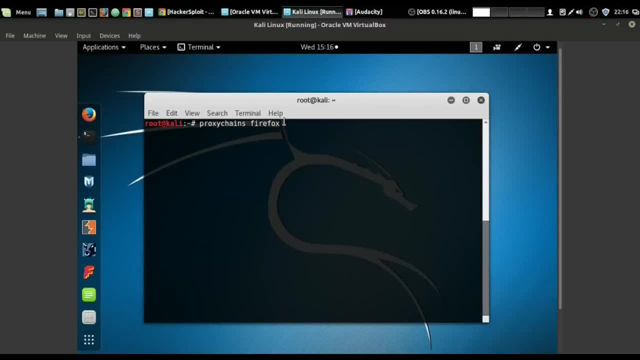 basically, ice weasel is just Firefox, so we're going to use Firefox anyway and we're going to enter a test website to test whether the proxies are working. I'm going to use wwwduckduckgocom, and the reason I'm using this is not anything particular. I 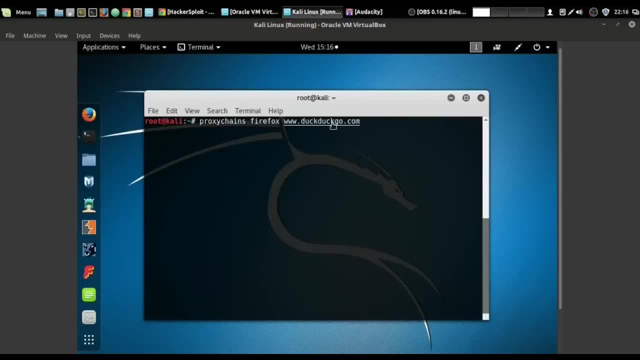 just want to also recommend this search engine to you guys. I know you guys are very fond of Google, but duckduckgo is one of the sites or search engines that does not keep your IP addresses and track you, so it's in terms of anonymity and when you're performing like who is scans on targets I would recommend. 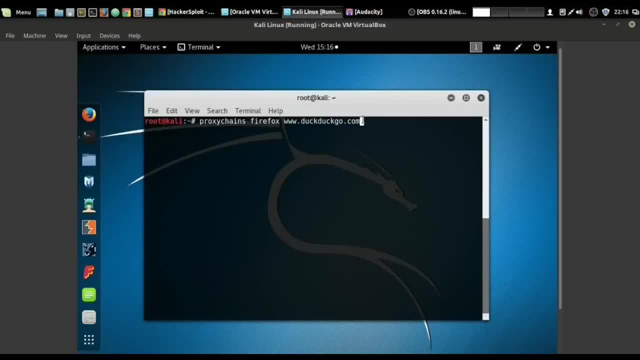 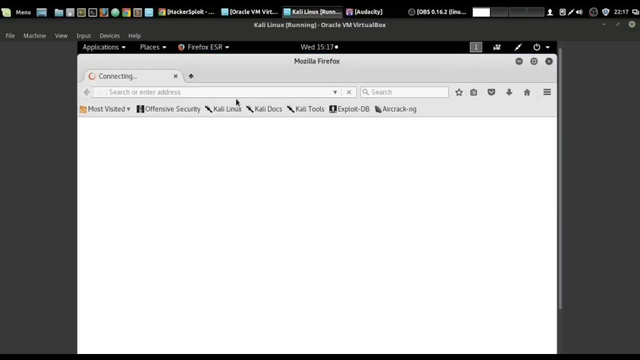 duckduckgo. it just keeps you safer. but anyway, we're using proxy chains, so all you need to do is hit enter and it's going to start proxy chains and it's going to open Firefox and it's going to open wwwduckduckgocom. obviously it's. 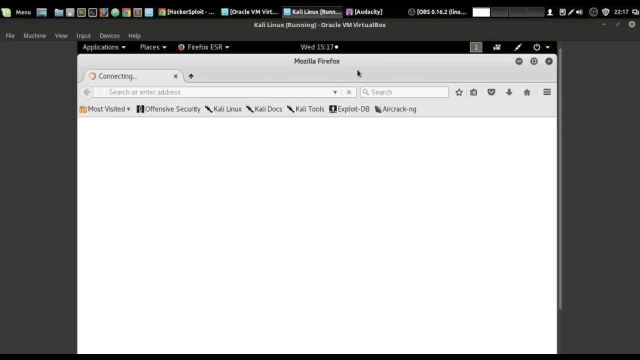 going to take a while because it's running through the proxy chains, and just give it its time and it should start. it should open up duckduckgo. and there you have it. it's opened up duckduckgo. but you might be asking: how do I know? I'm 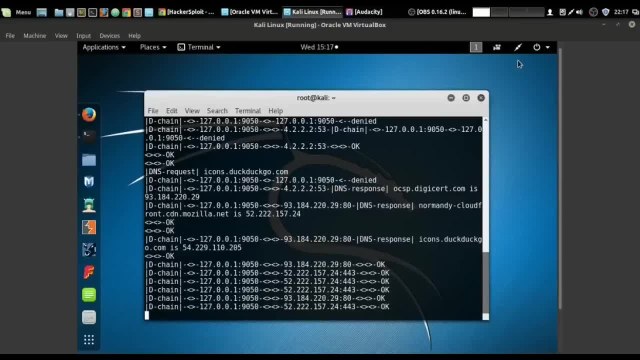 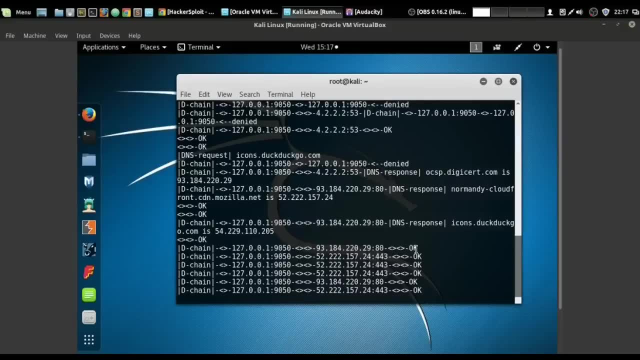 anonymous, or how do I know I'm safe? well, firstly, let's look at the terminal so, as you can see, you're going to see that it's basically accepted these IPs and you don't have to worry about what it outputs here. so, to test it, I'm going to 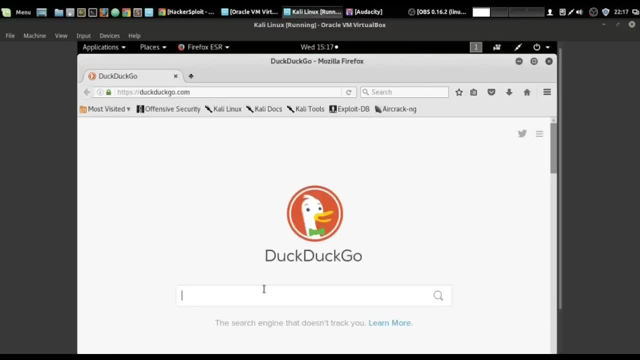 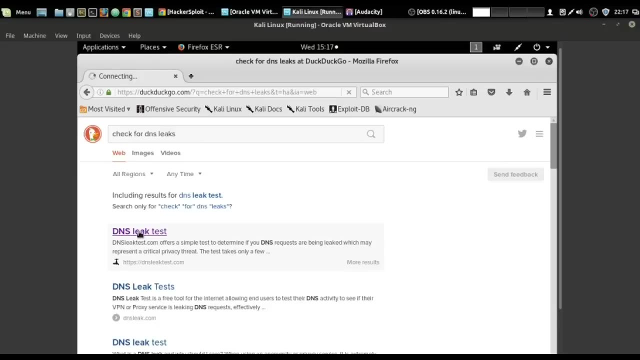 check for DNS leaks. now, how do we check for DNS leaks? we're basically just going to do a duckduckgo search check for DNS leaks, all right, and it's going to hopefully return some results. that was very quick and we're going to test the DNS leak test, all right, so let's open that up, all right. so, as you can see, the 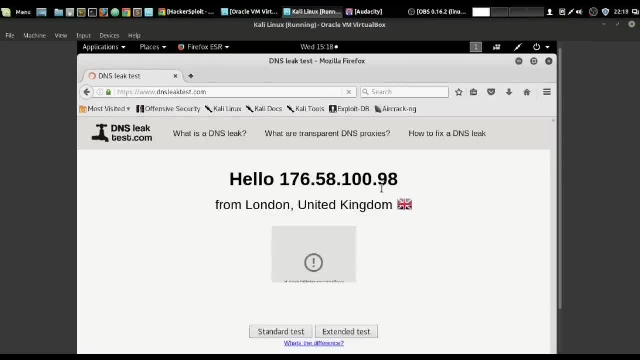 can see it said. my address is 176 58 198 from London, United Kingdom. I can tell you for a fact that I'm not in London in United Kingdom. I'm well, I'm really, really, I'm really far from here. so, as you can see, it's actually working and if 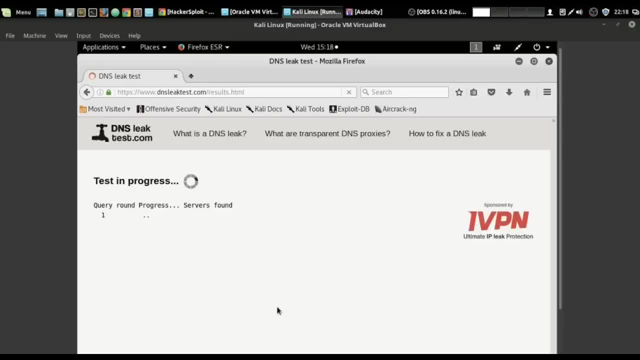 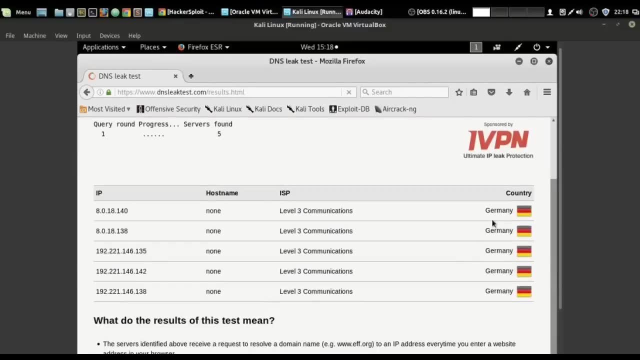 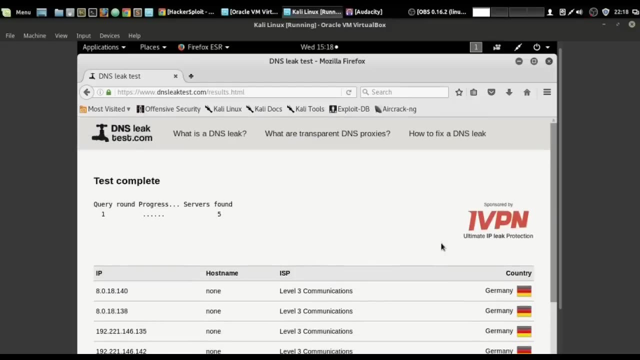 we start the standard test to test whether any DNS information was leaked regarding my real location, we'll see that it's probably gonna give us a UK DNS or is actually given as a German DNS. so that's actually even better. it just makes you more anonymous. now you guys might also be asking: how do we know? 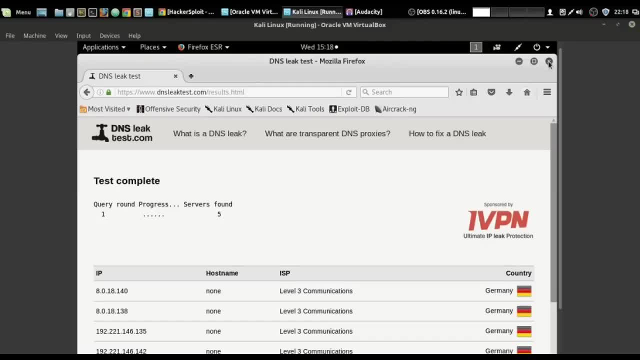 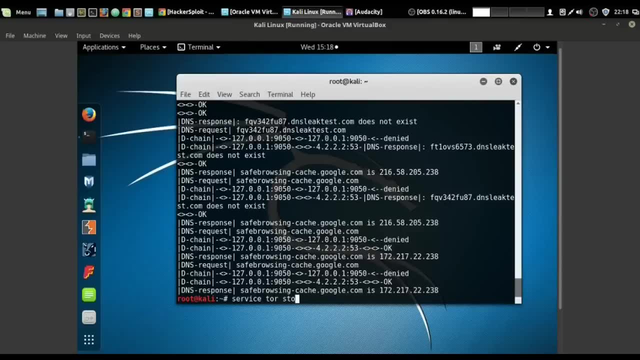 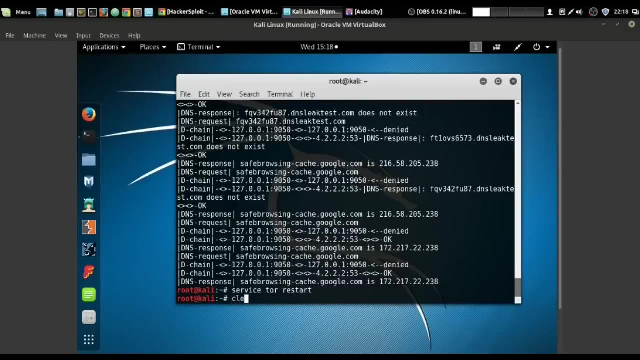 this is working and my IP will be changing. well, to do that, I'm just gonna close this browser and I'm gonna say: service store, stop. or I could say: service store. we start to save the time. all right, and once that's done, I'm gonna clear this and I'm going to save it, and I'm going to save it and I'm going to. 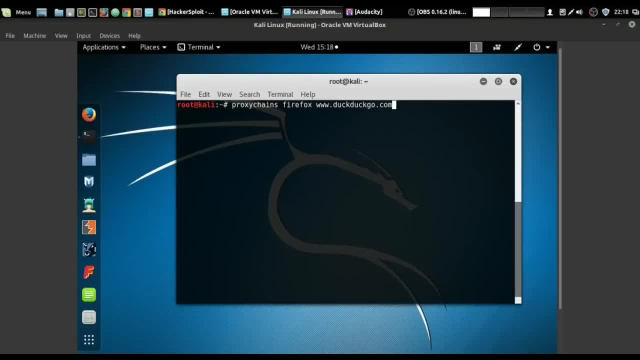 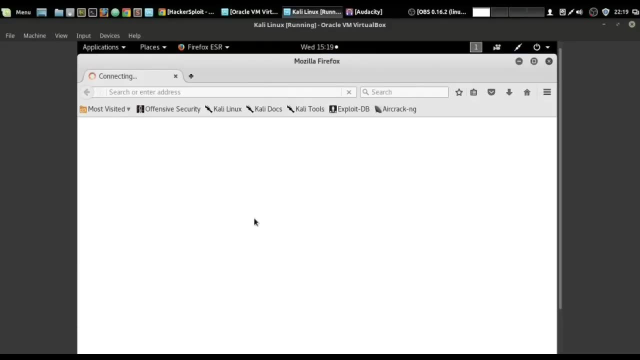 say, I'm gonna run the previous command, the proxy change Firefox doctor gocom, just to test that, and let it start up again. and there you are, it should start up again. depending on which proxy it's using, it'll either be faster or slower. if it doesn't work, don't worry, just give it a few seconds and it should. it should. 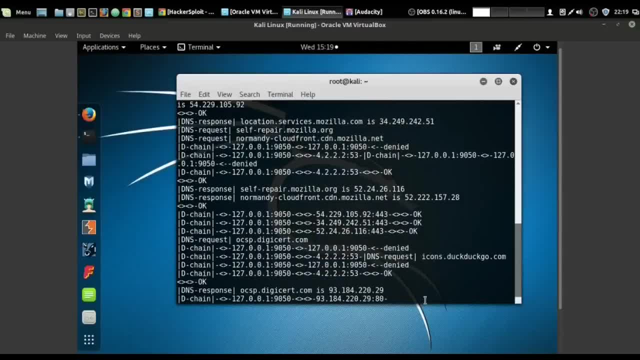 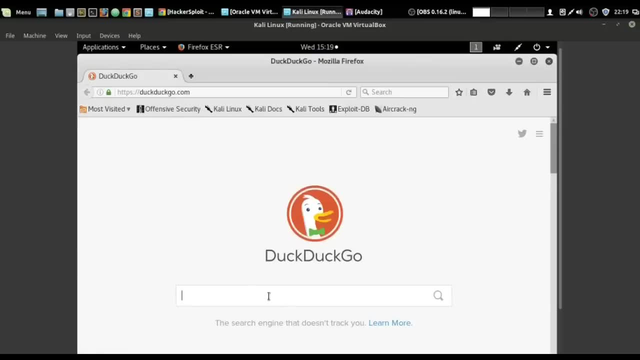 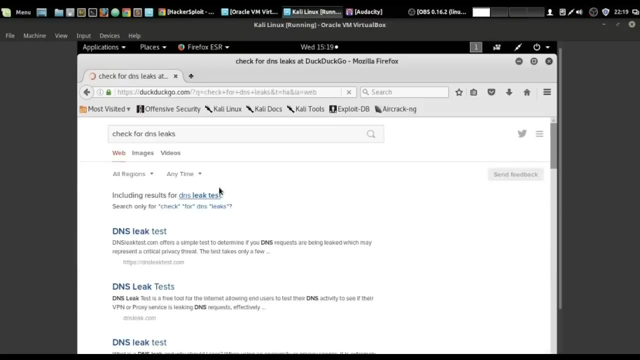 work because it will go through this, the series of proxy changes you can see here, and some will be denied and some will work anyway. it's returned, doctor go, so we can actually form the DNS search again. so check for DNS, DNS leaks. all right, again, very fast, let's check for DNS. 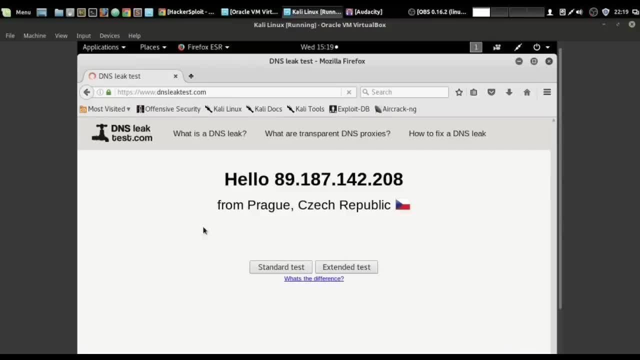 leaks and we should hopefully have a different IP. and there you are, guys, it's actually giving us an IP from Prague, the Czech Czech Republic. so if I butchered that, let's check what a DNS it's giving us. let's see what DNS it's giving us very 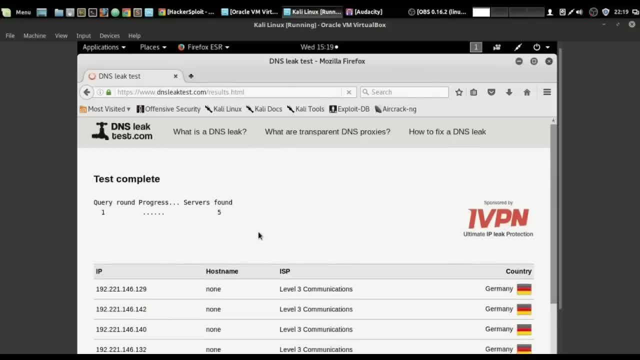 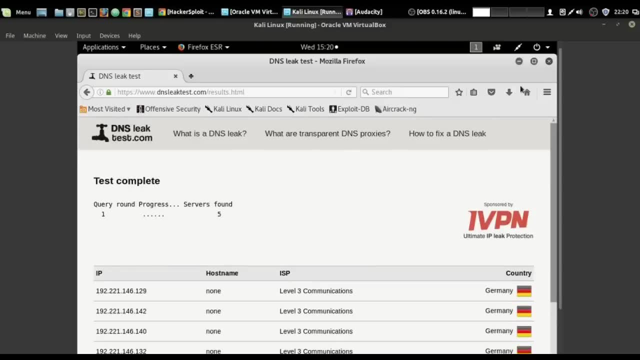 nice. it's running the test a bit slow, but it's worth it, whether you're performing scans or SQL injection. and there we are- Germany. so this is actually pretty cool, and I've actually shown you guys that it really does work. if you use this method, you're going to be anonymous, and that's all I can really say. knock. 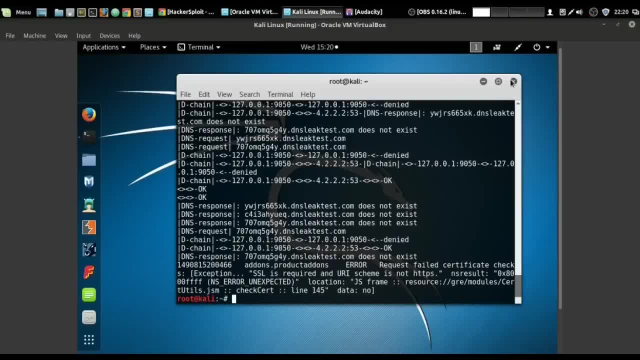 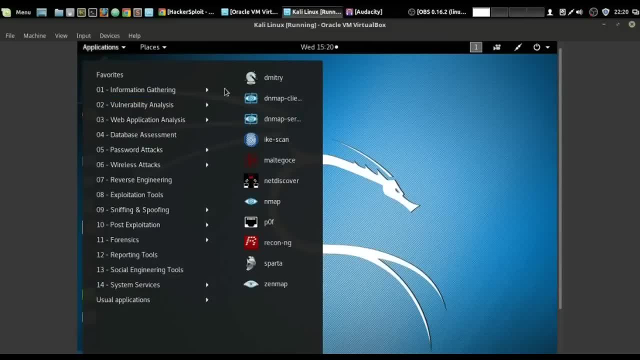 yourselves out, go ahead and do anything you want. this is really useful for for those, for people who are complaining about scanning the nmap dot- scan me dot. nmap dot org. now you can actually just change your IP and keep on using their domain- for educational purposes, obviously, anyway. 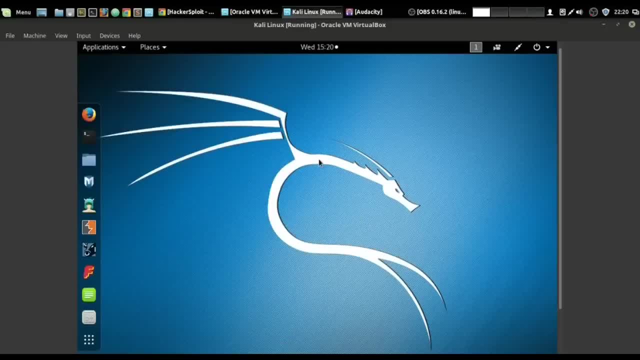 guys, you can see that it's working. I'm anonymous right now. I hope you guys enjoyed this video, or I hope this video helped you. if it did leave a like, please share it, because a lot of other people need this information and if they can get it that'll be just great. if you have any questions, the comment section you. 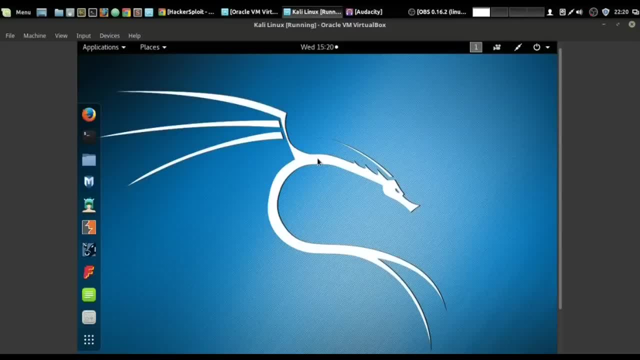 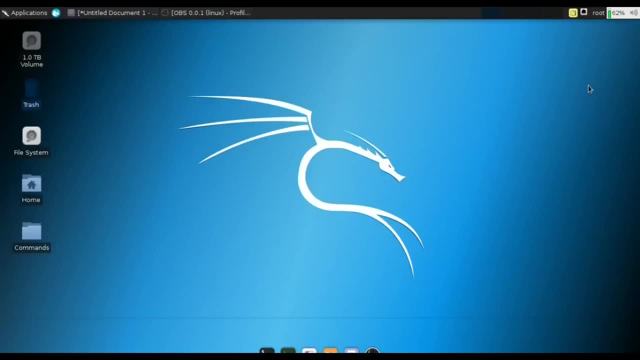 can contact me on, on my kick or on any of my social media, on my social networks anyway, guys. thank you guys for watching and I'll see you guys in the next video. guys, so much for watching the video, peace, hey guys. hackersploit here back again with another video and welcome back to the ethical hacking course, and I 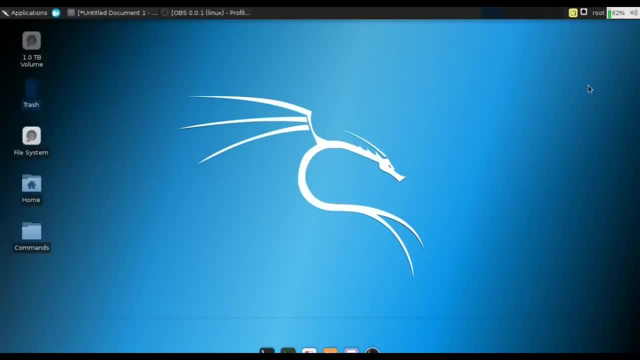 just want to show you guys a little quick tip here. so quite a few of you guys have actually told me in the comment section in my previous video regarding using proxy chains that it gets really, really complicated and that you have to install the door service and what not. so I'm actually gonna show you. 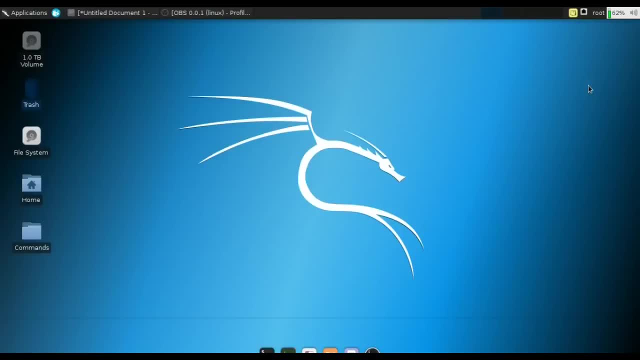 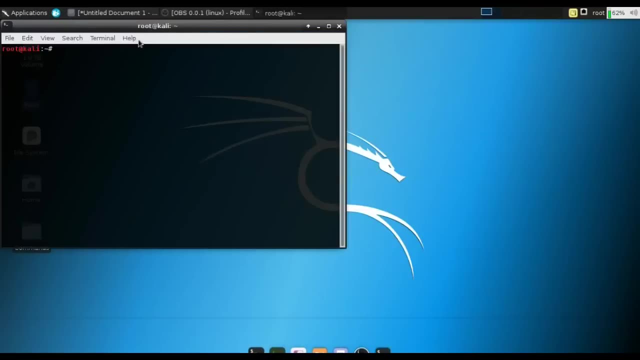 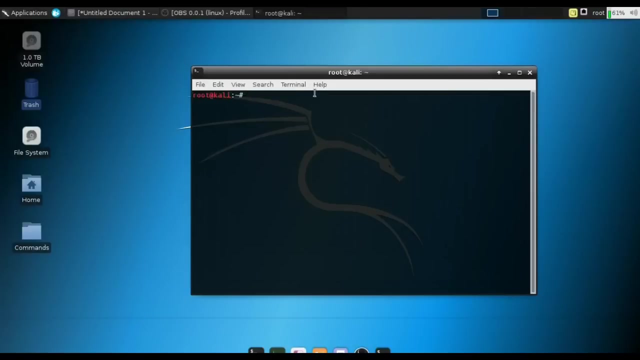 how to do that and how to anonymize your entire system using proxies, more specifically the Tor proxies. so for this you're basically just gonna need the terminal, as I mentioned below, and you're gonna have to install a program, actually a repository, called anon surf or anonymous surf. so I have the repos right. 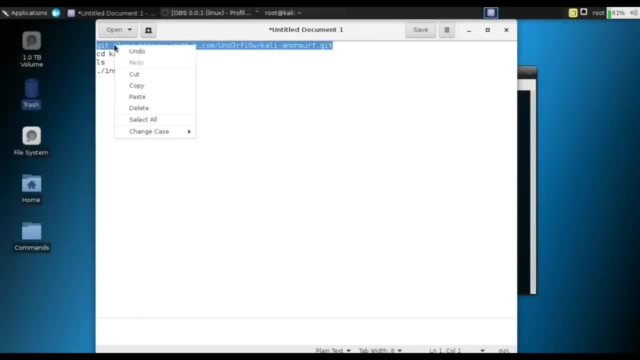 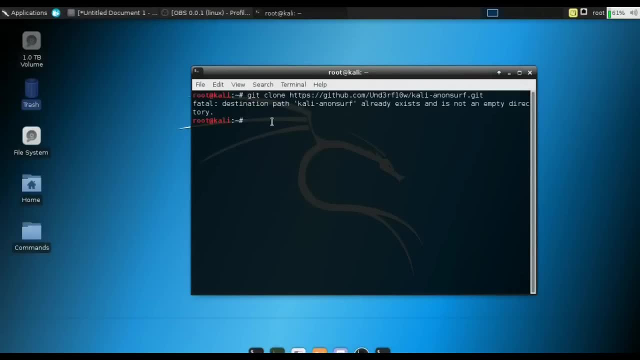 here. I will put them in the description section. so the first thing you have to do is you have to add the repository, which is the anon surf dot git from git hub. let's add that I already have it, so it's really pointless from my point of. 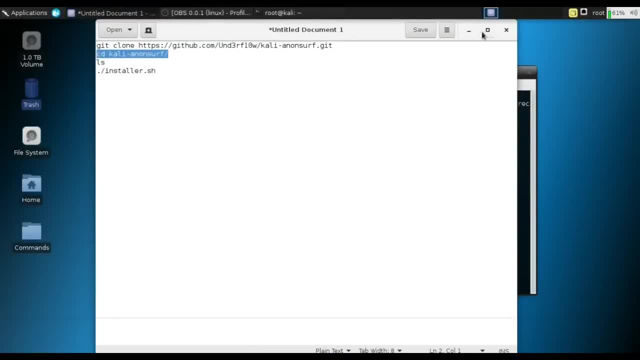 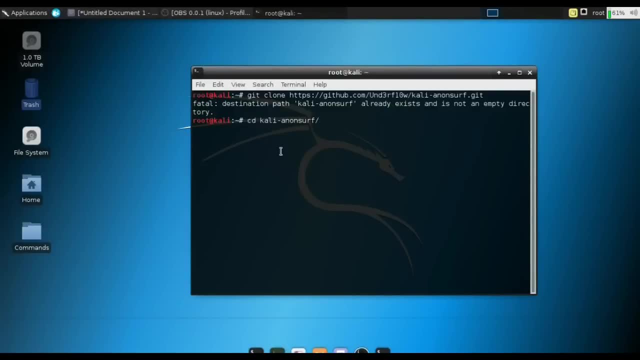 view. so the next step, once it's installed by, as I've said, it's already installed on mine, so I just have to browse to the anon surf directory, which you should do after you've installed it. so, once it's installed, enter the following command: cd Kali, hyphen, anon surf, and it's gonna take you into the 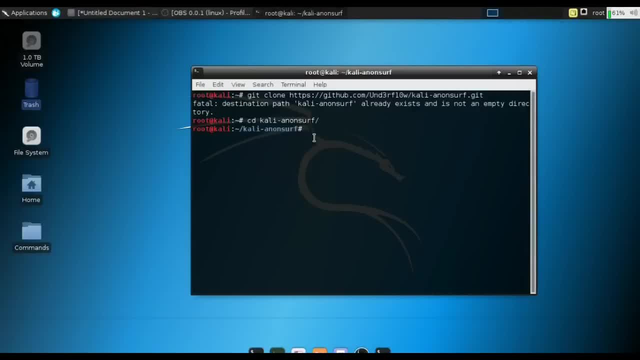 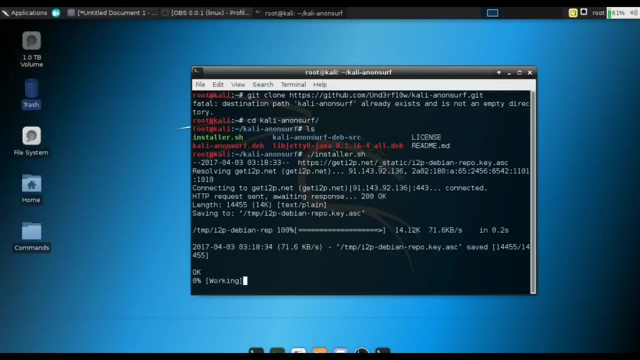 directory and just list, and I really don't need that right now. LS, and we want to run the installer dot sh or installer dot shell file. so after you've run that, just run this and it's gonna install it. I'm just gonna reinstall it on mine and just let. 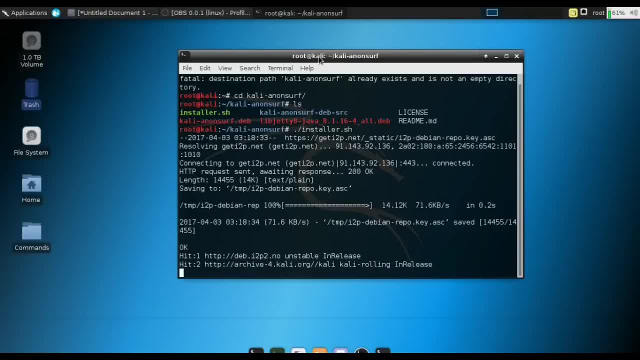 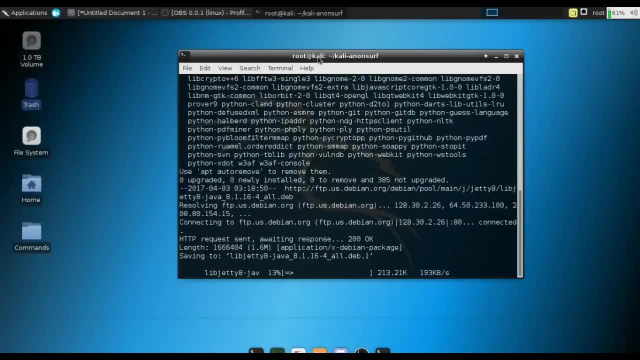 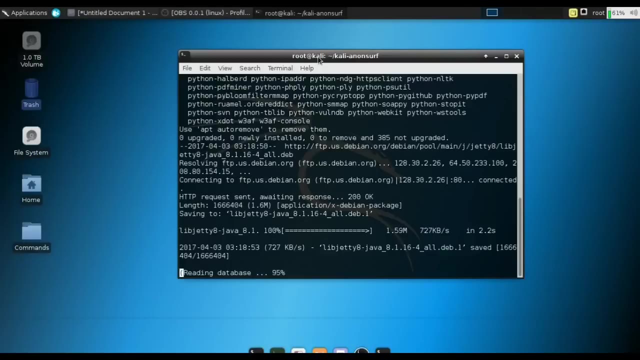 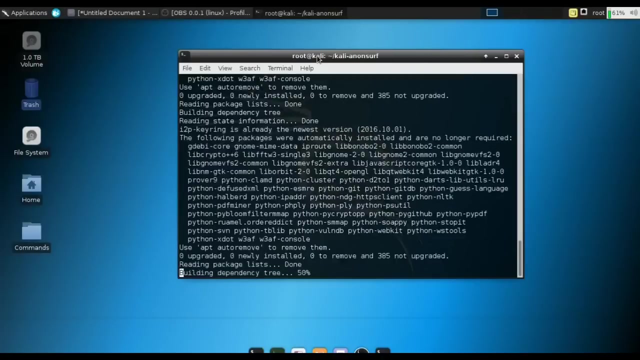 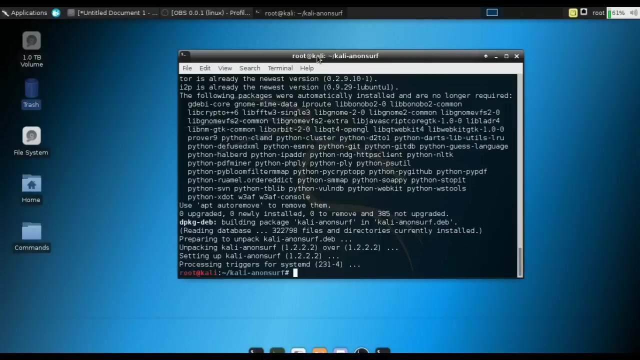 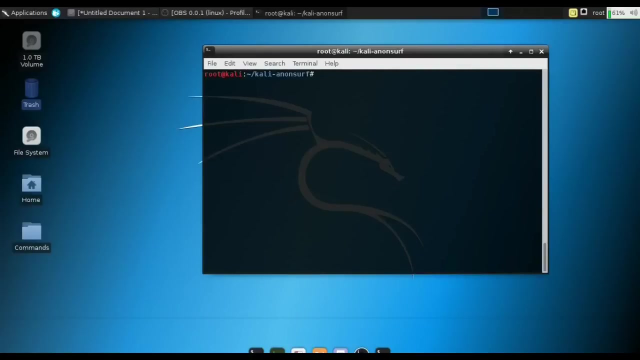 it complete, and it should actually just take a few seconds and you're good. so let's actually just wait for this to complete, alrighty. so once it's actually finished installing- which I had to do on mine- I'm gonna clear the terminal and what you want to do is just run the installer dot. 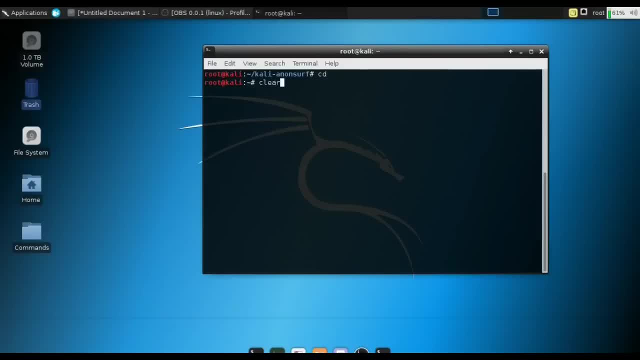 shell file and take my PerspectiveVisual settings correctly, then just run a test run. that I finished. I'm sure it'd work. but I think it's pretty easy and I'm gonna do it like�� containers as well. just to start here enough. I am just gonna go back into my 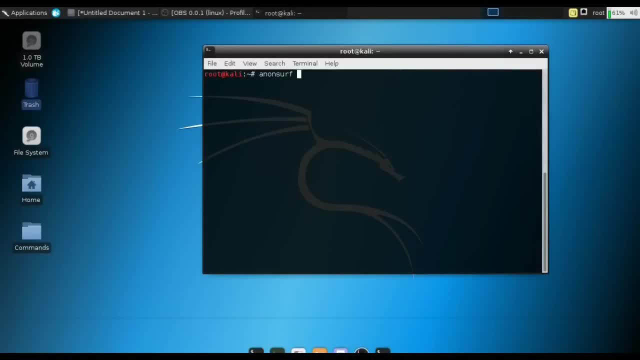 home directory. I'm gonna clear that again. you really don't need to do that. so basically file to consoleusrpxanon surf. so basically we have installed the repositories and we're basically ready to use it. so, anon and i'm just going get Hao command, just do basically show you guys how is simple it is, so basically to start it. you have these steps. I need help command just to basically show you guys how it is, so basically to start it. you have these steps. 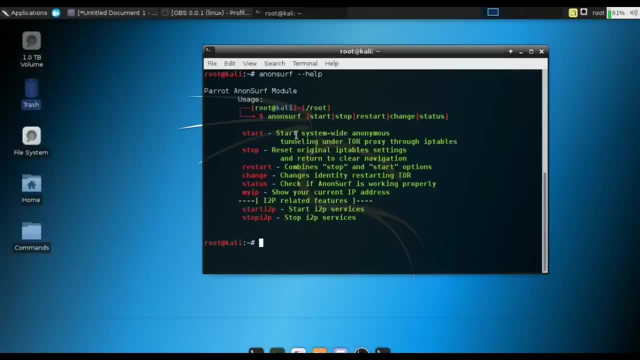 start, stop, restart, change and the status whether it's running. so we have the start. so this start system-wide anonymous tunneling under the top proxy. so basically, it's very similar to proxy chains, as i demonstrated in the proxy chains video, which will be linked in the description. 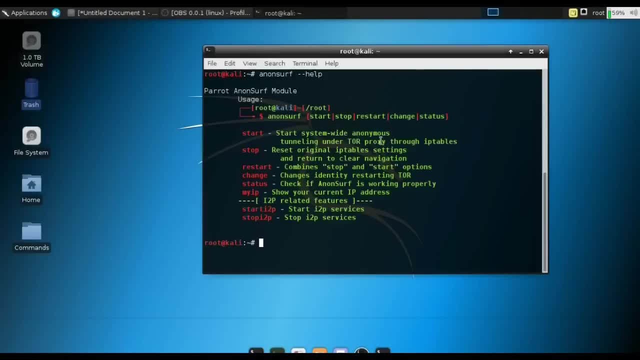 and at the end of this video. so basically what this means is going to anonymize your entire system with the top proxies and by restarting it, you just basically get a new identity, as you guys are pretty much, i think. uh, you, you understand that with tor, every time you, you can basically change your identities and what that means. it will change the ip and therefore change your identities. as for dns leaks, i'm not quite sure whether this really does work. i haven't really really tested that, but uh, it should work using the top proxies. so you have the start: stop, restart, change you can. 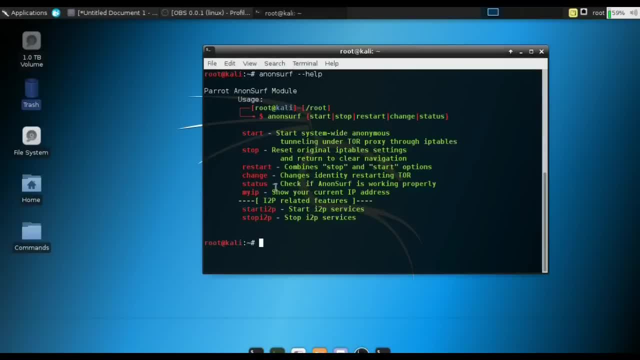 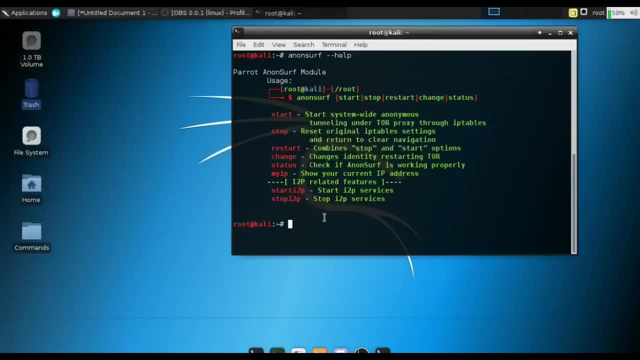 change the identity, restarting tor, as i mentioned, and this: uh, you can check the status and it'll show you the status. and you can change the identity, restarting tor, as i mentioned, and this: you can check the status and it'll show you, uh, your country ip. so let's actually run this pretty awesome stuff. so what i'm going to do is say: 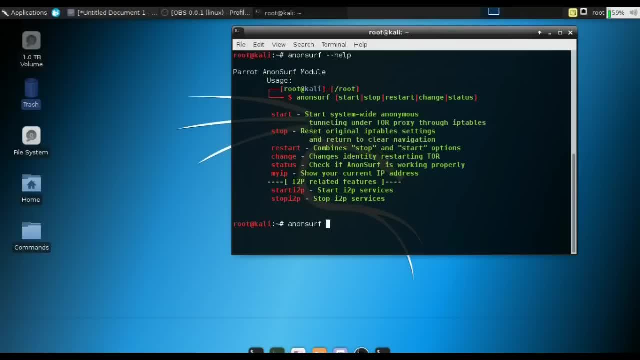 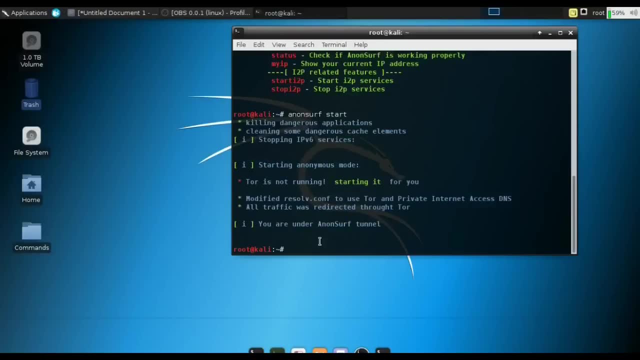 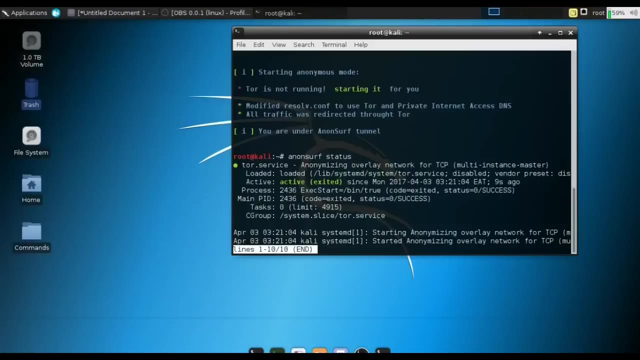 and non surf, uh, swoops and on surf, and we're going to say start, and it's going to start, all right, um, once it's started, what we're going to do is we're going to say um and non surf status, all right, and it's actually running. so 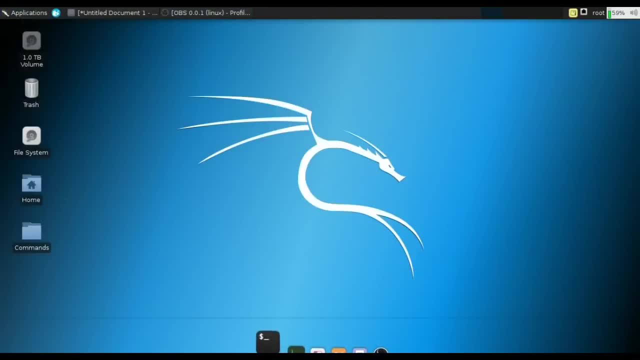 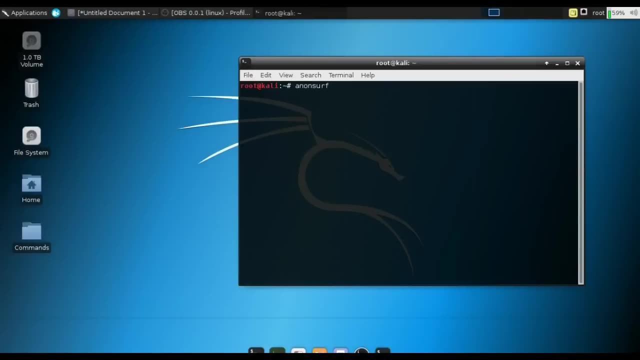 so let's close this terminal because that's started a process and we're going to just check, uh, the stuff right now and on and on surf help, and let's check what our current ip address is. so my ip. it's taking a few seconds to load it. so there we are, it's giving. 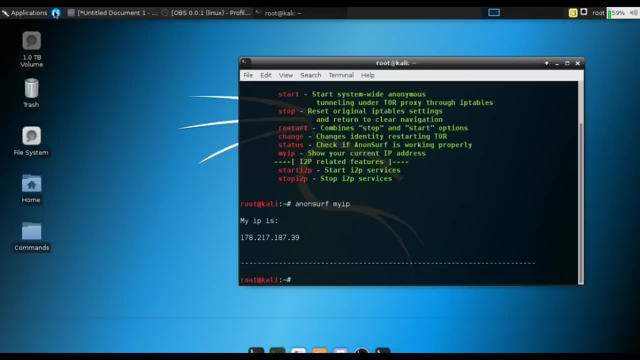 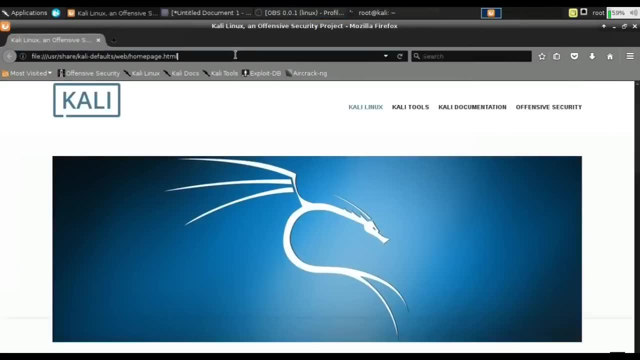 us an ip. we- we can't really actually tell what ip, uh or what country this belongs to, but we can check that right now. so in the same process, i'm going to also check for the dns leaks. so let's, let me just check for for dns leaks and i'm going to use, uh, duckduckgo, uh, let's see how fast it'll. 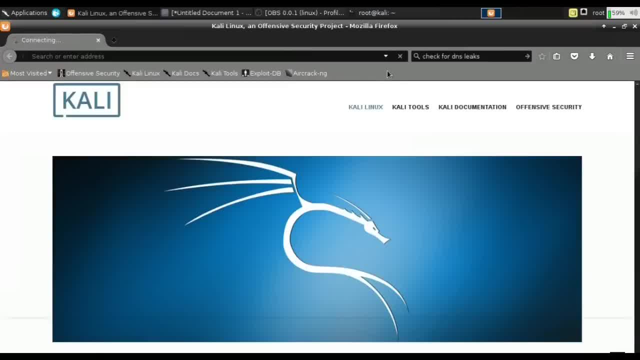 actually load it. uh, as i mentioned, sometimes the proxies- the top proxies will- will be kind of slow, as you guys are already used to it. so i'm going to just check it out and i'm going to go ahead and see how fast it's going to load. so let's see how fast it's going to load. so i'm going to go ahead and 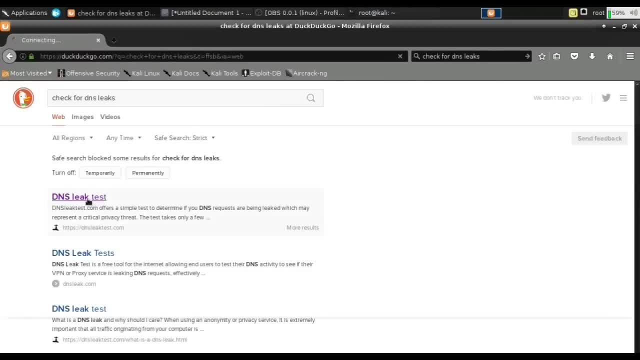 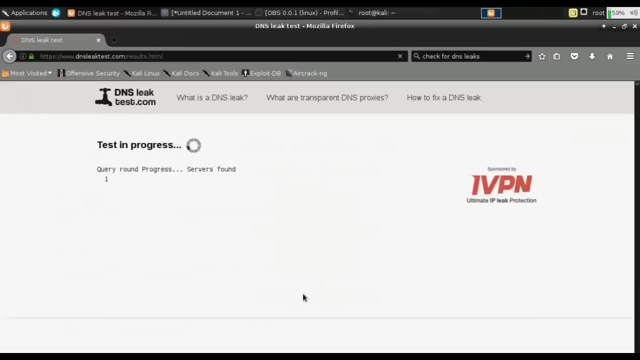 using the deep web. but here we are: uh, check for dns leaks, let's open that up. and there we are. so it's saying: uh, from oslo, norway, that's the ip address. uh, we then have: um, let's check for some actual dns leaks and let's see if that actually worked. 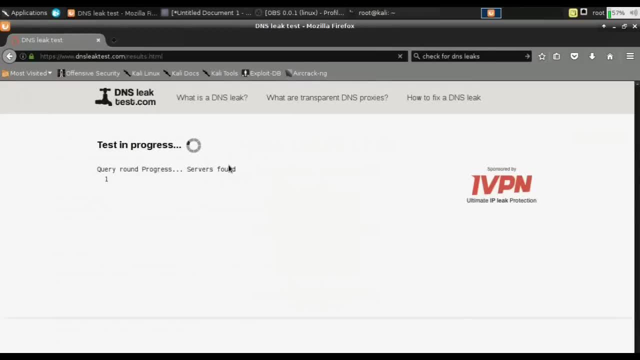 uh, to differentiate the ip from the dns, to change that. so this is basically going to provide us almost 100 percent anonymity as long as you stick to um, as long as you just keep on restarting the service. so let's see how long this takes. it should, shouldn't take all that long. 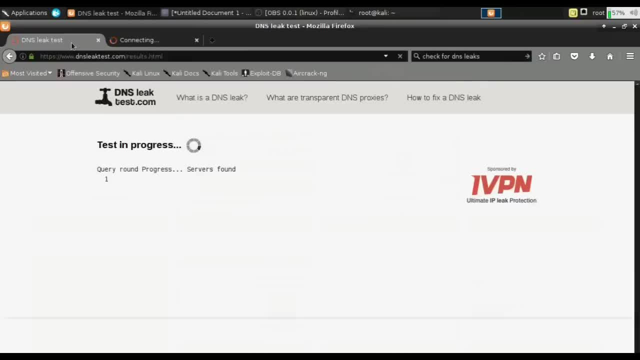 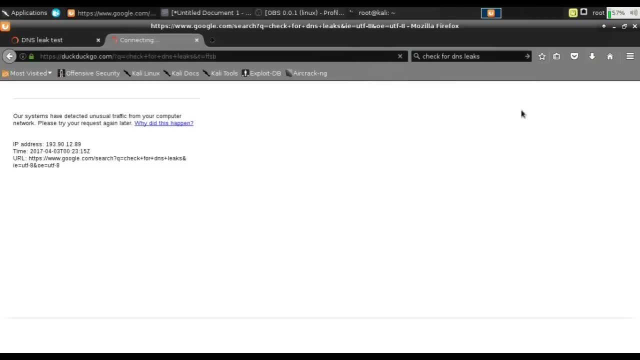 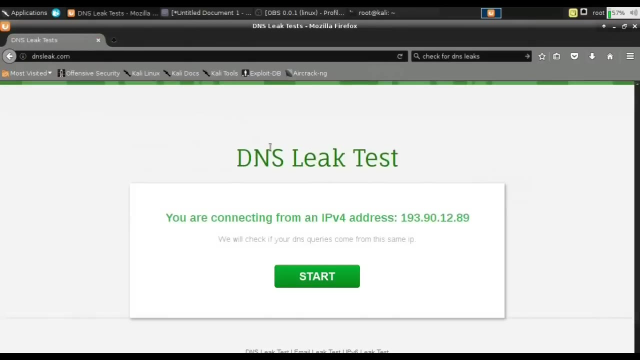 all right, so i'm just going to check for another one right here, because that one is taking a whole lot of time. oops, i should have actually known that google would have refused that, so let's actually just check from here. that's actually taking too long. 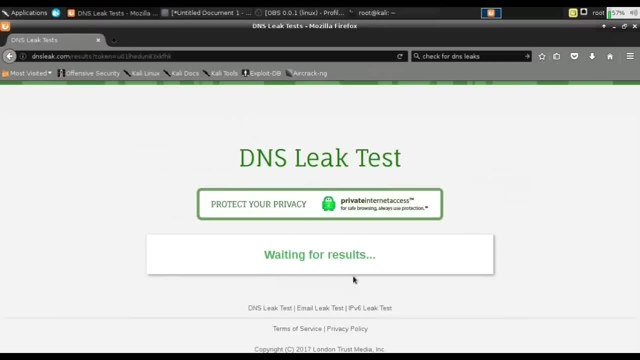 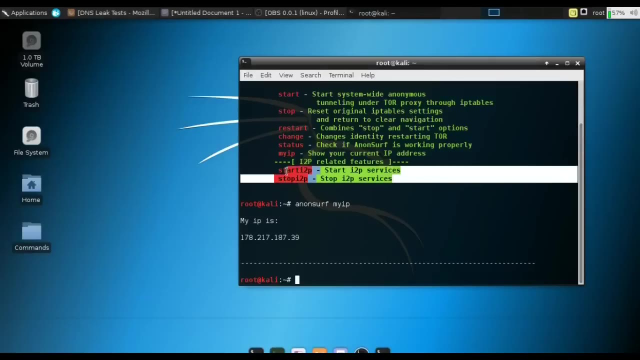 um, so let's start. let's see how fast this site actually takes to calculate the results. so the ip belongs to norway, oslo, norway, in particular, and basically that's how you can actually do it. for the other services, you have i2p, which is really not. 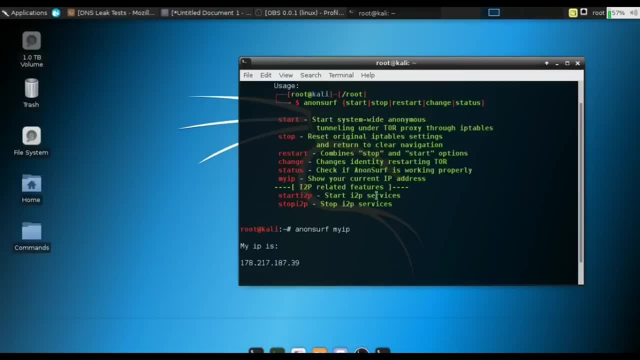 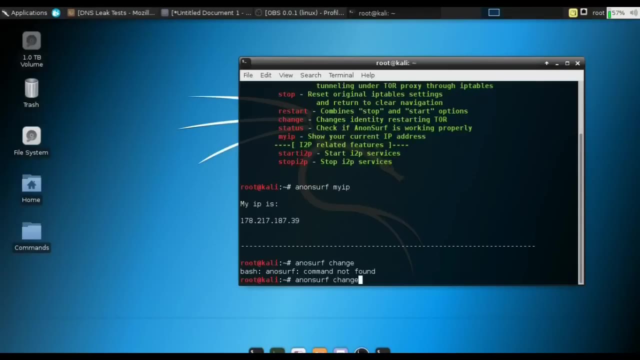 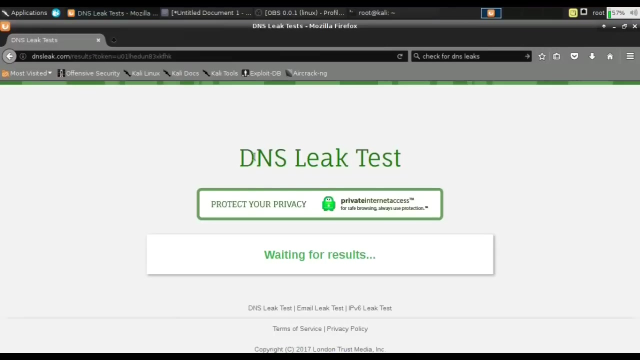 important right now. it's quite an ice up, outdated method, but basically we can actually just change the identity. so, and on surf change, which will basically, oops, change, and it's going to change, and it's forced to change to the nodes, so we can actually just check for DNS leaks one more time through the duck, duck go. 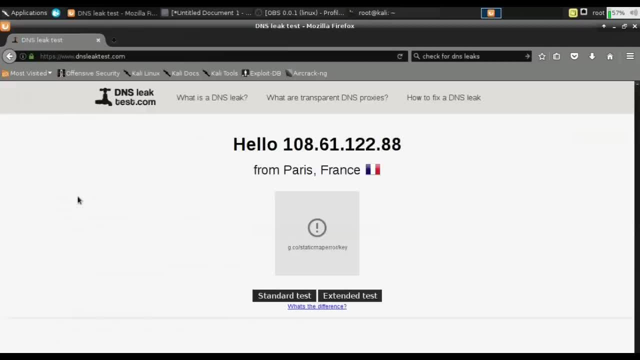 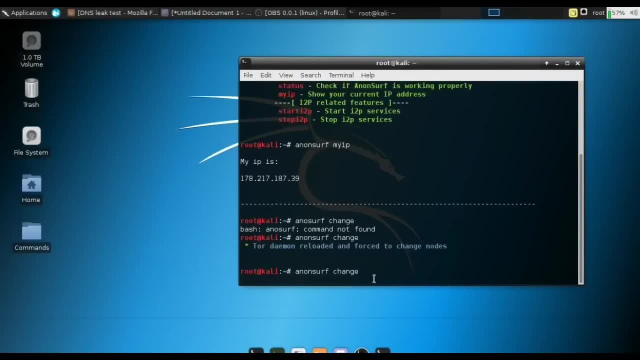 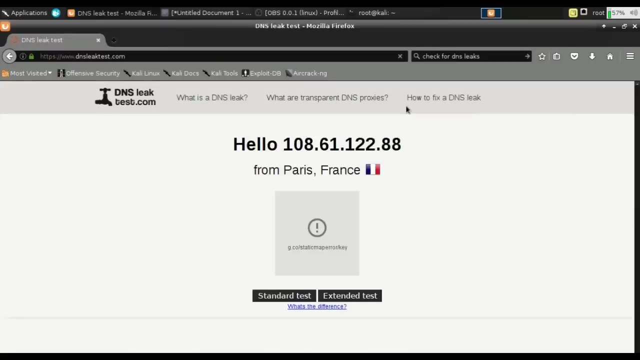 search engine, because I don't want to go through a bunch of captures and stuff like that. so again Paris, France, and let's actually just test this as many times as we can. and on surf change, so it said France, and let's refresh this page, let's see what we get. again, the proxies might slow it down quite a bit. 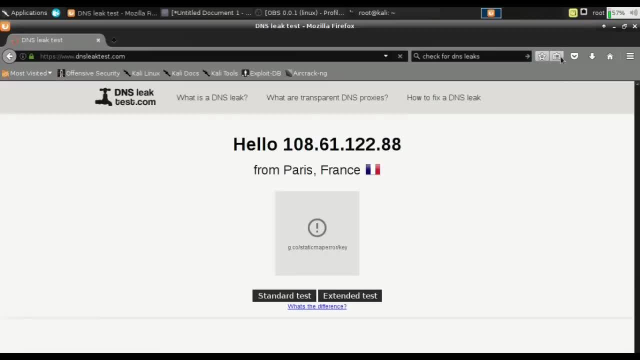 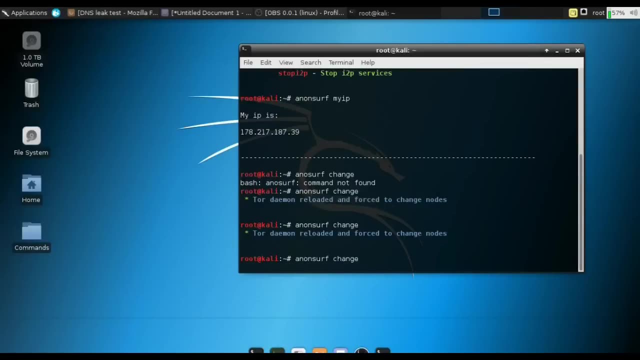 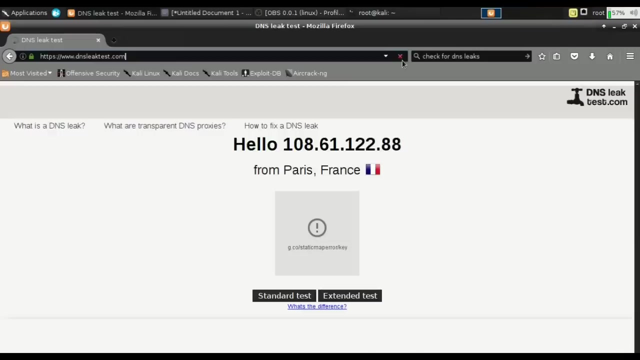 but anyway, let's just see what we get. taking quite a bit of time on this one, let's just restart the process. and on surf change, let's get an another one. let's see what we get: another identity. let's restart the site again. actually, let's just restart it from the, from the search engine, because it's. 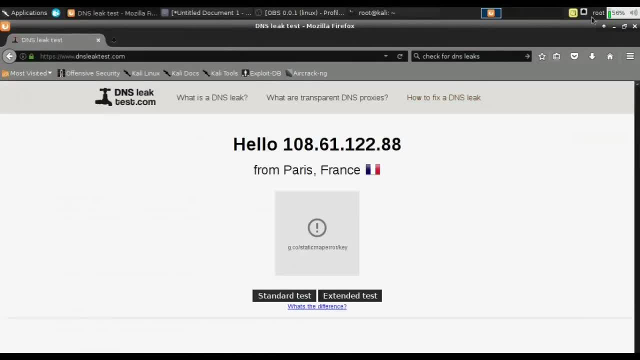 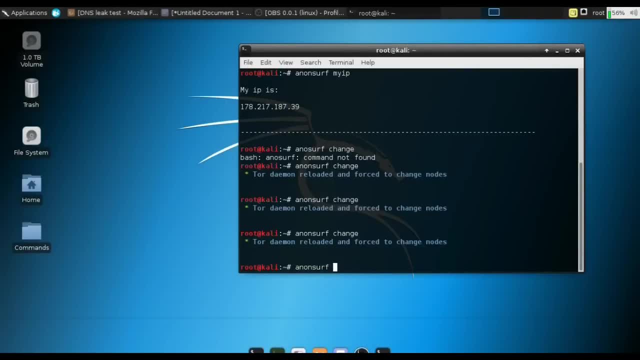 probably using the current cookies that it's loaded, so it's actually giving us the same one. that's pretty weird. so what I think you should do is an unserved restart. let's restart it and it is going to restart, and let us actually try that again. 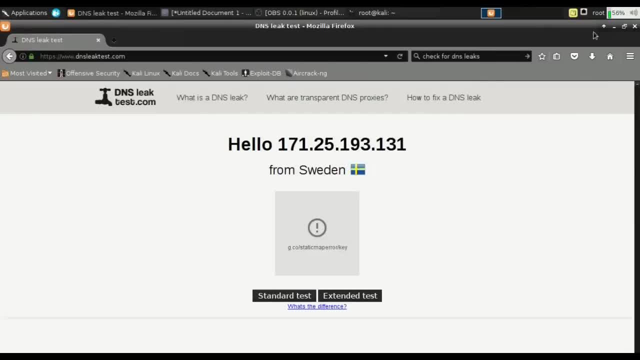 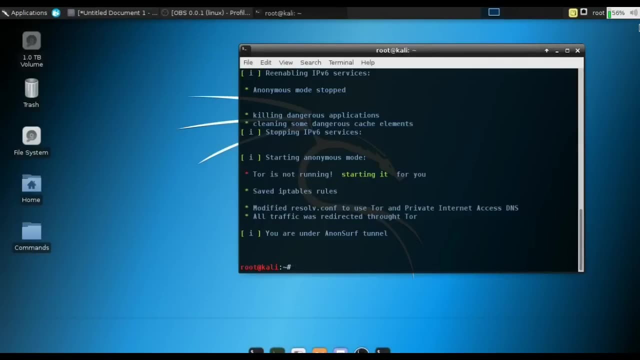 that's it there we are. so, basically, restarting is more important or more effective than changing the identity, as i had mentioned earlier in the video. so this is pretty much it, guys. uh, that's. this is basically an alternative to proxy chains, just making it a whole lot simpler in instead of 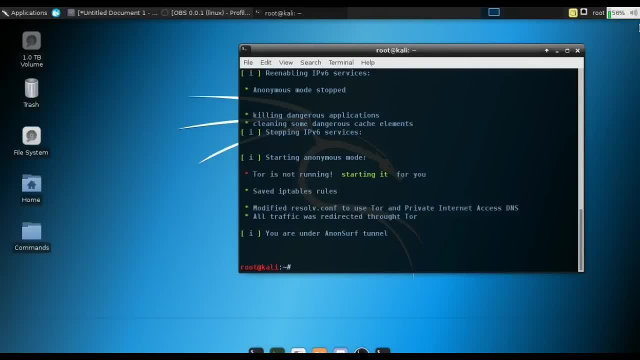 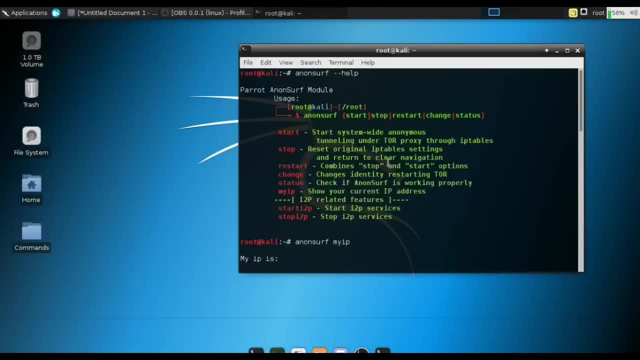 going inside the proxychainsconfiguration file and starting the tor service. so this basically, in fact, i wouldn't- uh, i wouldn't mind using this when i'm when i'm performing scans or stuff like that, because it just makes it a whole lot simpler and easier and it's actually working, as you can. 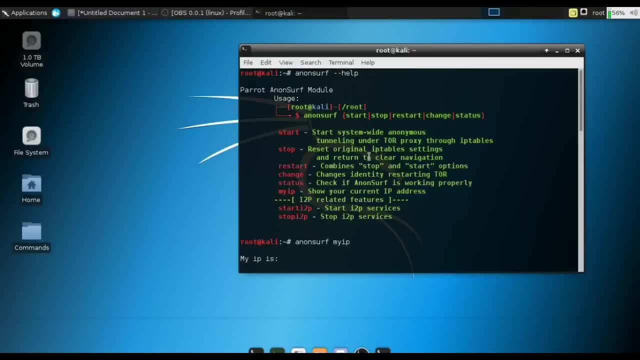 see. so that's it for this video, guys. hope this video helped you guys. um, if you have any questions, let me know in the comment section. hit me up on kick. hit me up on my social media. i'm always there to answer questions. uh, please make sure you share this video, in case a few people who need 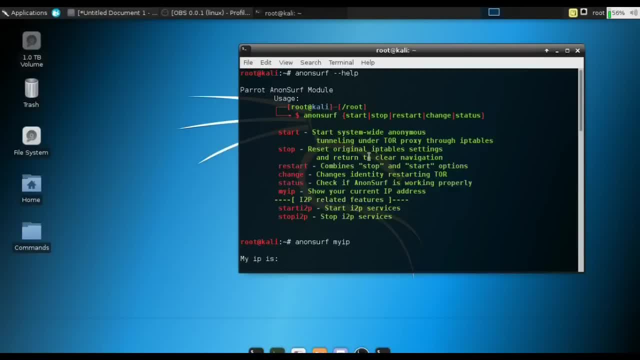 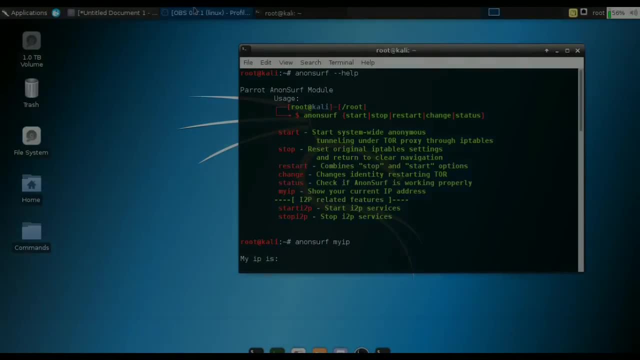 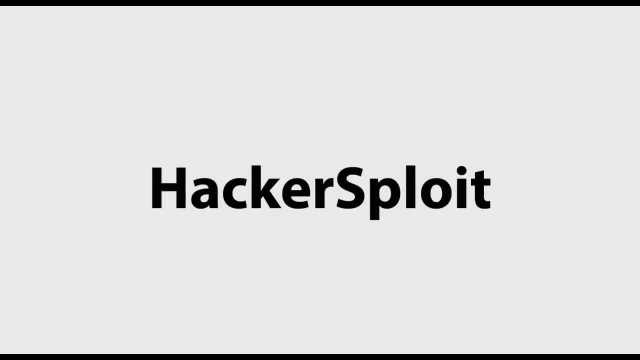 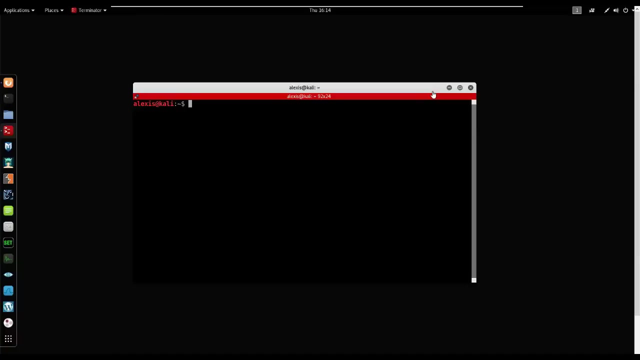 this information can actually get it again. guys, thank you so much for the support on the channel. thank you for watching my videos and have a fantastic day- peace. hey guys, hackersploit here back again with another video, and in this video video, and in this video i'm going to be showing you how to set up vpn. 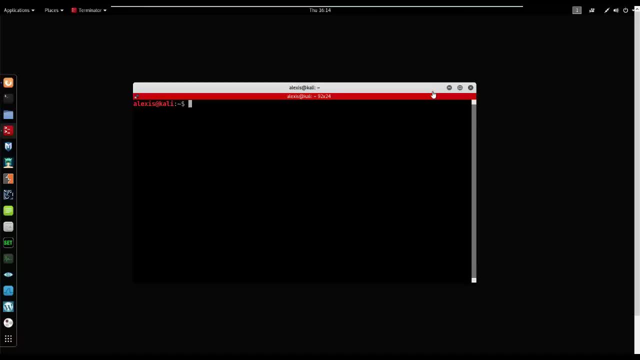 for free in kali linux. more specifically, you can use this on any other linux distro that you want. it will work perfectly, and the reason i'm making this video is a lot of you guys have requested it, and that's because the proxy chains configuration videos that i made are a little bit complicated. 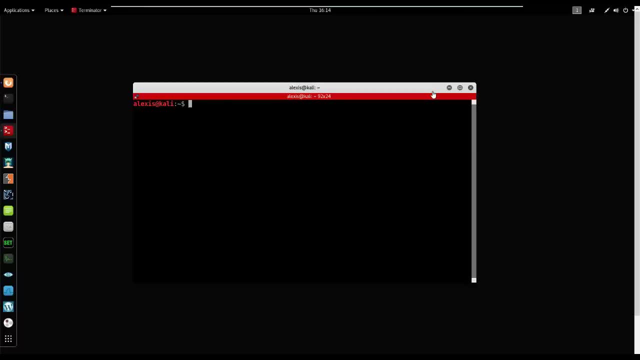 and are bringing a lot of problems. i will be making a follow-up video to those proxy chains, videos to sort everything out and to clarify a few things, and uh that that video will help you uh troubleshoot your own the problems that you have with your proxy chains. 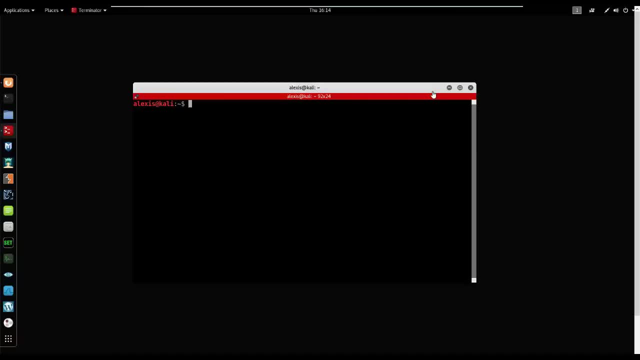 but again, the reason i'm making this video is a lot of you guys have been requesting it to. i've been requesting me to make a vpn uh on linux b稿 video on how to set it up and how to get it running and basically explaining how to do it. 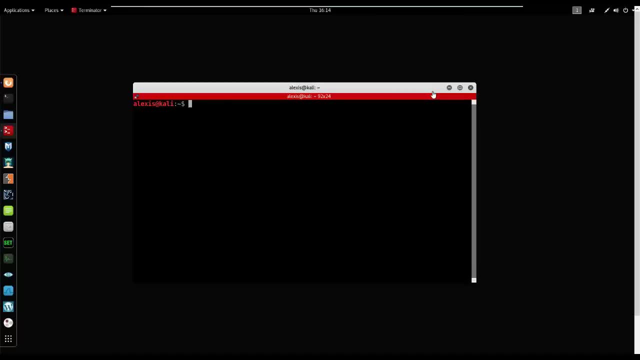 now, before we get started, i just want to point out something: vpn is not my preferred option when it comes down to anonymity. it doesn't matter whether you're browsing a. vpn just won't cut it in terms of giving you, i would say, 90 of anonymity, and the reason is this. okay, firstly, you have two. 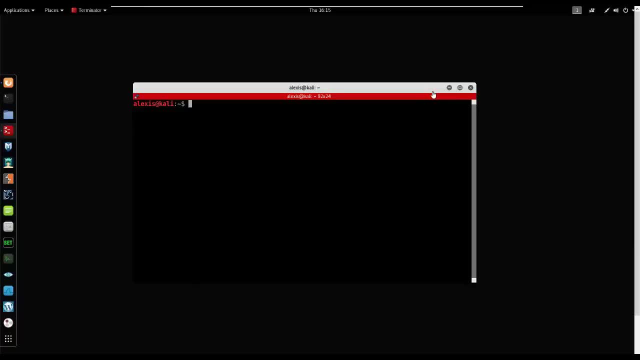 you have your free vpn services or servers and your paid vpn services, which obviously it's obviously it's obvious to tell that the paid versions are going to provide you with a much better speed, are not going to log your information, or some of them may be doing it, i'm not sure. but 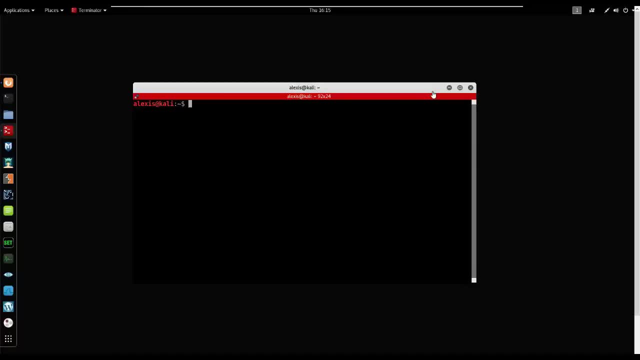 they're. so you know, some of them log your traffic in case they get questioned by authorities if you did anything illegal. they will be, they will, you know. provide them with your browser and they will provide you with your vpn, and they will provide you with your vpn. and. 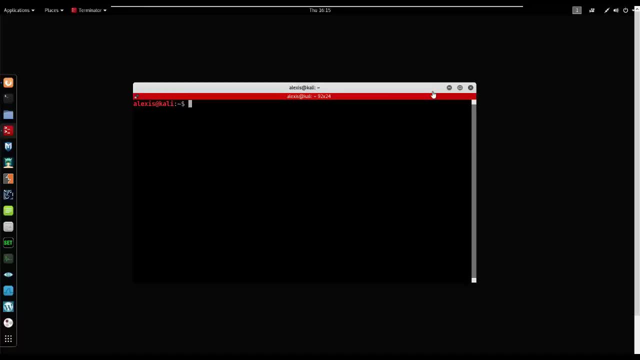 information and your DNS information, which is what I'm getting to very, very closely. what I'm trying to say is they're going to be plenty of free ones out there, and that's what I'm going to throw out a bit of a caution: that please be sure of the VPN server or service you're choosing, because if that VPN 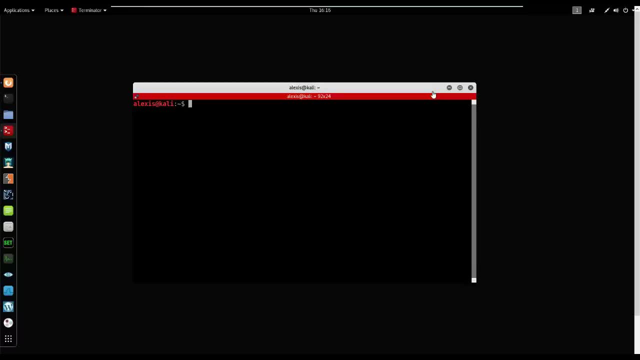 server is set up for it illegitimate purposes, meaning the owner of that VPN server is, in all essence, logging your traffic or your, the sites you're visiting. well, that just defeats the purpose of even having a VPN in the first place. so you know, in this video I'm going to be showing you one of the 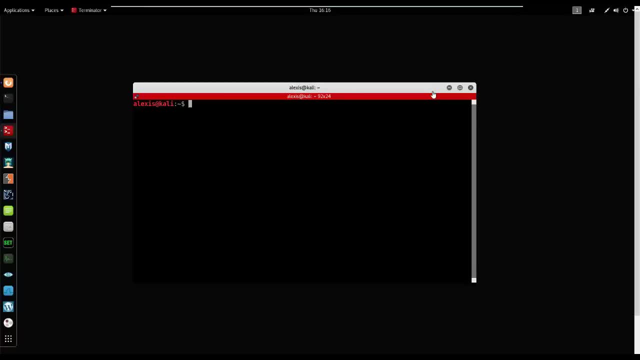 best free options available and I would recommend that you stick to it unless you find another one that's better and is proven to be legitimate. okay, so that's just a little disclaimer that I wanted to point out now, again, when it comes down to DNS information being leaked. 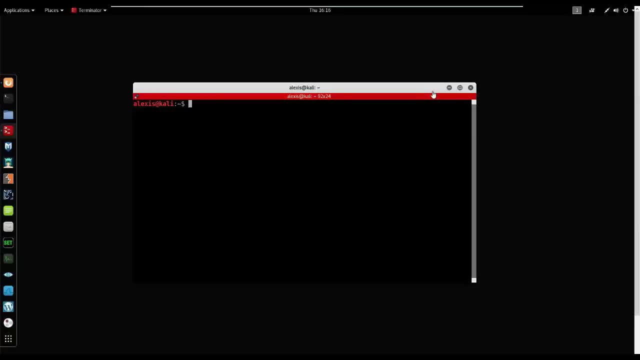 I can't say that it's a good thing or not. it's a good thing, but it's a good thing. I can tell you for a fact that a VPN is not is probably gonna leak your information. I would say a VPN provides you at least with 60 percent of. 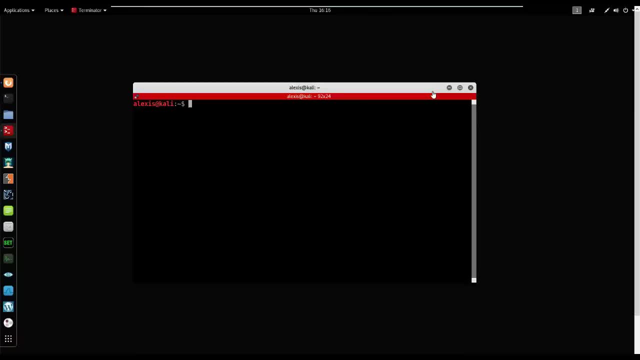 anonymity. I'm not going to say that a lot of people are going to look at your DNS information, but if you're changing your IP address with a VPN, you're really forgetting that your DNS information can provide authorities or anyone who pokes into it with information about your DNS. 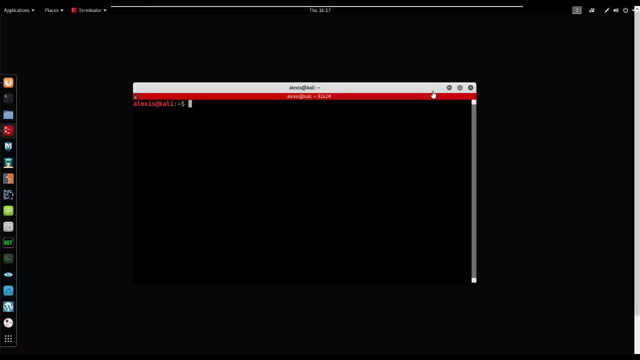 and from there can deduce your location. so it really doesn't matter if you've changed your IP address. if your DNS information points to a geographical location, that's it. they've got your location and from there they can just pinpoint your activities. but let's get started. so I'm going to open you just. 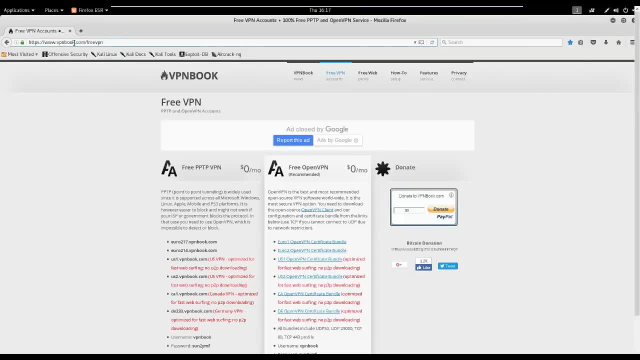 want to open up your browser, and this is the service that we're going to be using. we're going to be using VPN bookcom, or a VPN book. comm provides free VPN services. as you can see here, it costs zero dollars a month, which is awesome. if you want to donate to them, I 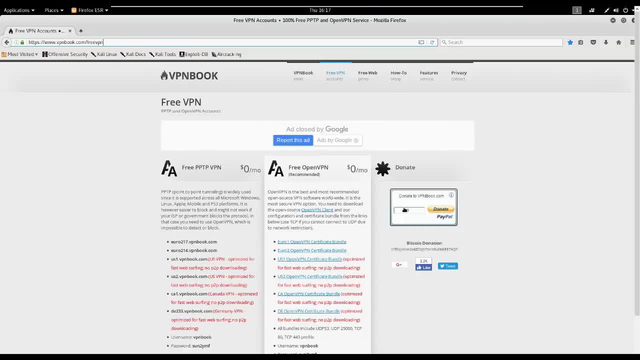 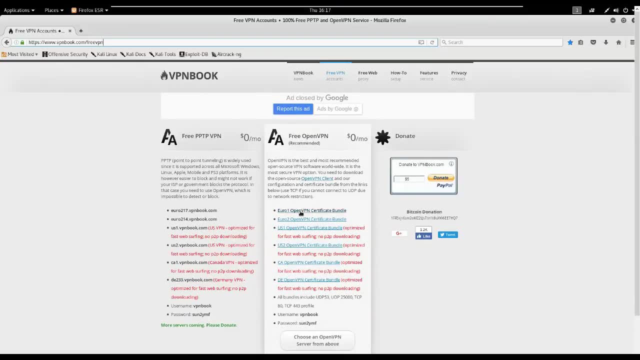 would recommend it because the service they are providing is fast, it's reliable and it's secure. so we're going to be using free, open VPN, okay, which is recommended, obviously- and they provide you a different certificate bundles depending on your location, so you can select. you have your euro. 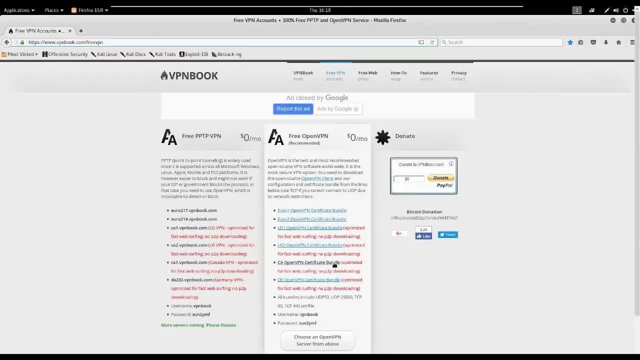 one euro, two us one. us two, CA one- I'm guessing that's California, probably, I'm not sure, don't hit me on the head with that- and, as you can see, it's going to tell you, optimized for fast web surfing, so no p2p downloading, so it's going to allow you to browse the web, you know, with great 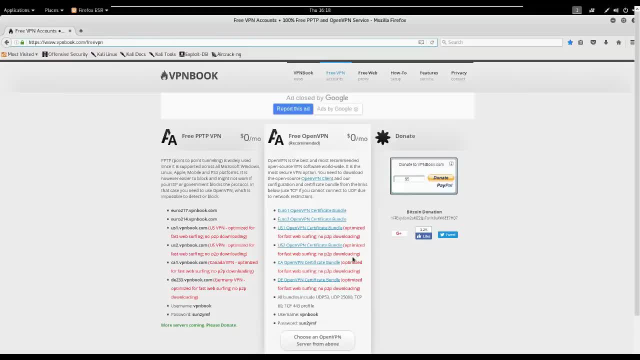 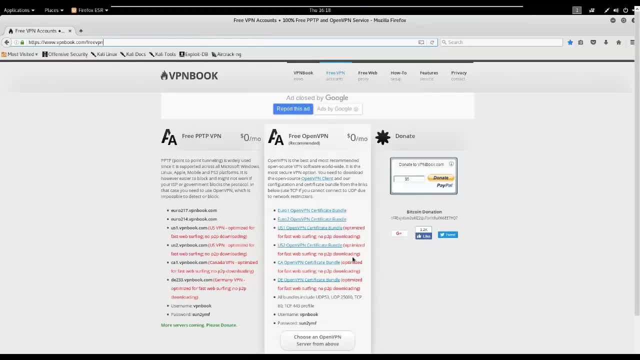 you want to go into a, a paid VPN, okay, so let's get started now with setting this up. so, as I said, you can choose your certificate bundle, which are all which include udp53, udp25000, tcp80, tcp443. so that means, if you have a network or your network is has blocked UDP connections, you can use the. 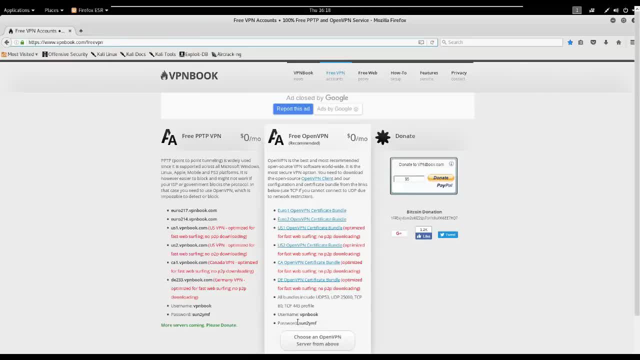 TCP certificates. they also provide you with the username and password, which are going to be very useful in a short while. so just download any certificate bundle that you like. I'm just going to try Euro 2, for example. it's going to be a very small file, so that shouldn't be an issue. it's about 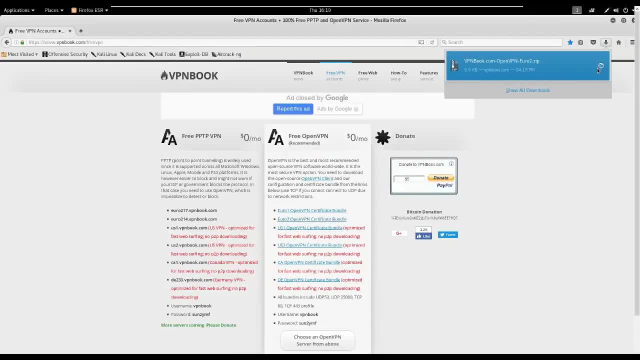 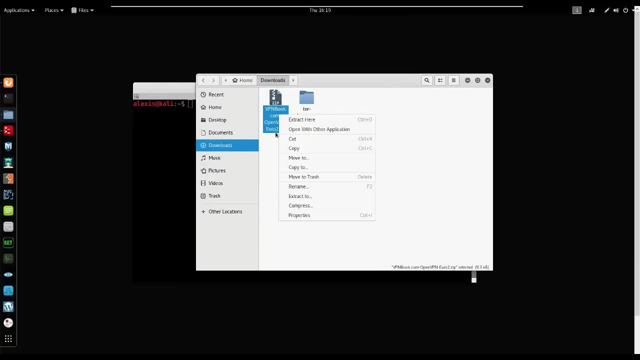 nine kilobytes. so I'm going to save it and it's going to download instantly and I'm going to open the folder. as you can see, I have it in my downloads folder and now I'm going to extract it, because it's a zip file. so make sure you extract it in that folder. in this case, I'm in my downloads folder. 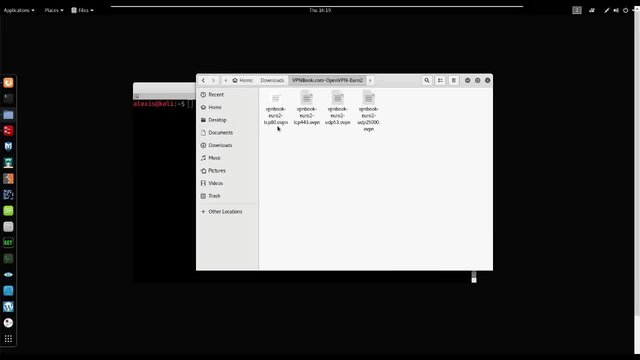 I'm going to enter that folder and, as you can see, we have the certificate files, the dot open VPN certificate files. so you have your tcp80, tcp443, udp53, etc. etc. the one I'm going to be using, and I'm guessing you're going to be using, is udp25000, again, if your network has restrictions. 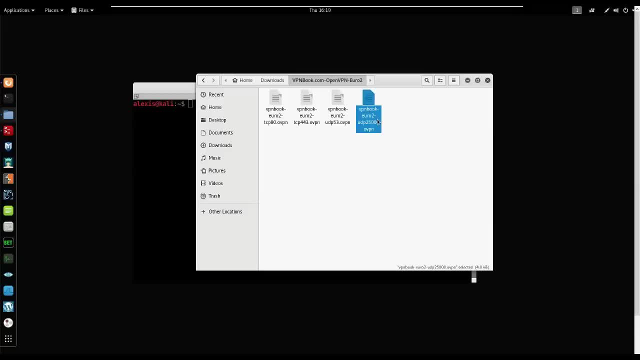 you can choose any of the other three certificates, but I'm guessing this is the one you're going to be using, so I'm just going to copy the entire file name with the open VPN extension, just because I want to save time and I don't want to have to go through the process of typing it. I'm 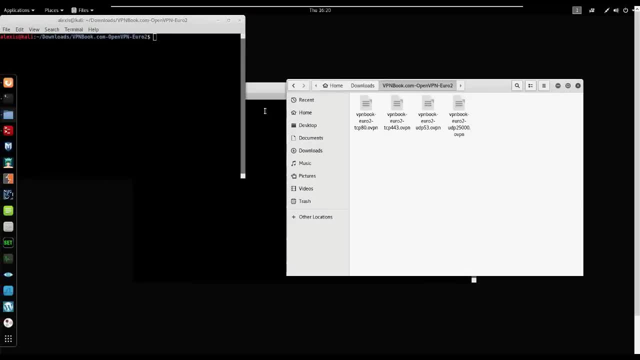 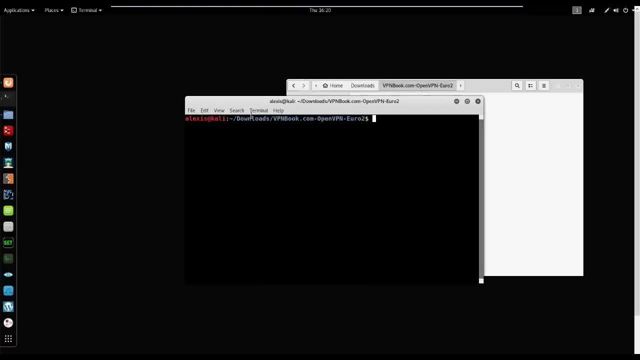 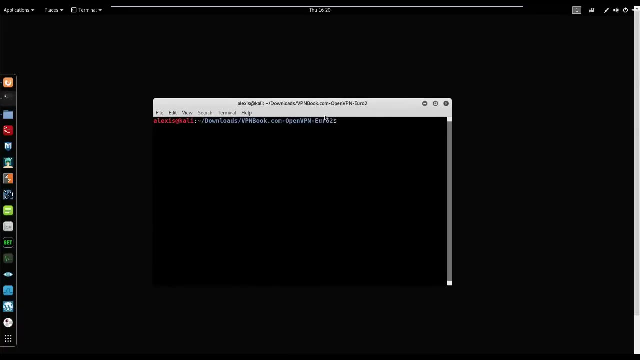 then going to open a terminal in this folder like so. let me just get rid of that like so, and what I'm going to do is I'm just going to zoom in so we can see everything that we're working on right now and we can get started now with setting it up. now it's very important that we use we enter into root. 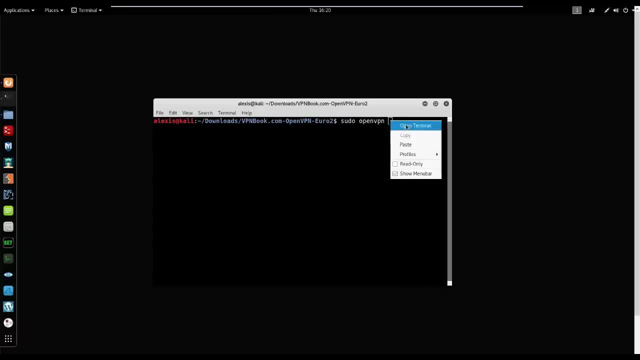 open VPN. all right, so we're specifying that we're using open VPN and now you want to give the certificate file, which I've pasted the name there and it already knows that I'm in my downloads and in the vpnbookcom, the VPN folder that contains the VPN certificates. so I'm going to hit enter. 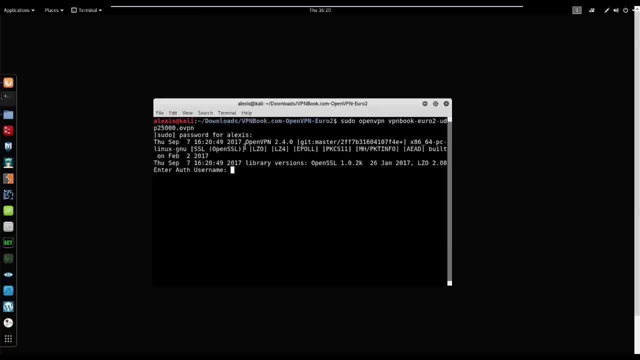 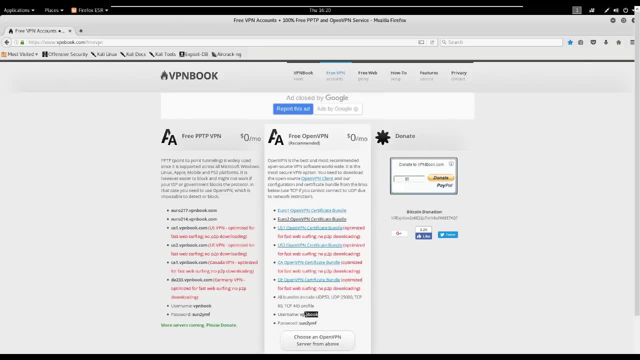 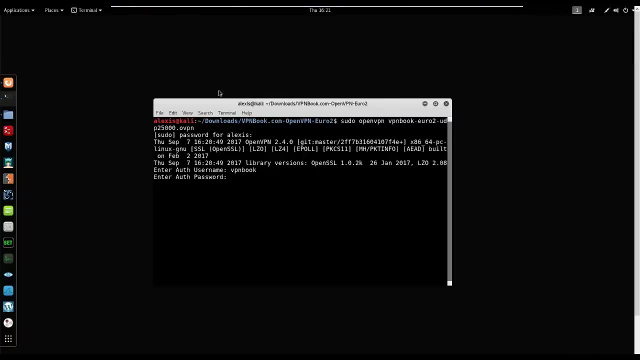 and it's going to ask me for my password- remember, this is my root password and I've given it there- and then it's going to ask for the authoritator username, which, in this case, they have provided. okay, so we can just copy that, or, in fact, let me just type it: VPN book and I'm going to hit enter. 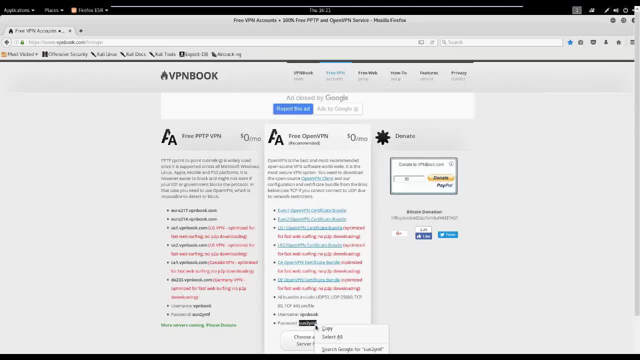 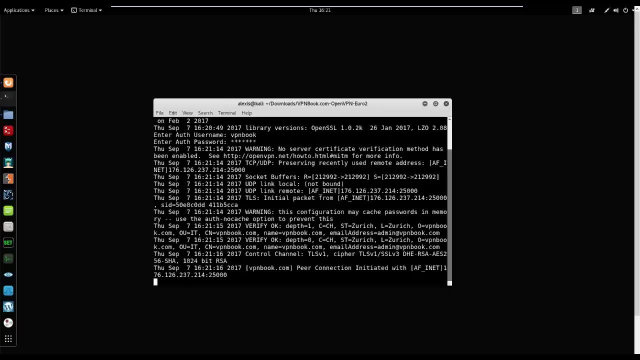 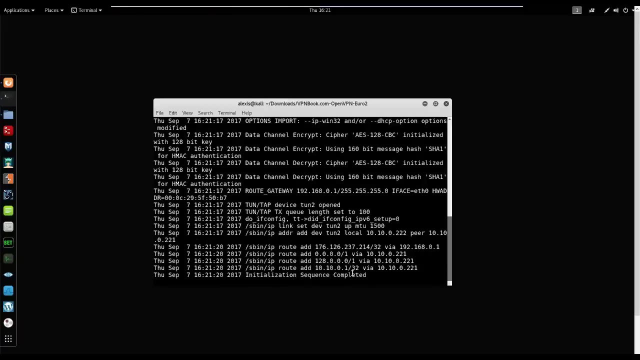 it's going to ask for the password, which is son to IMF. I'm just going to copy that- I don't want to make any mistakes like so- and I'm going to hit enter. so it's going to start the whole VPN service and just give it a few seconds and once it tells you, initialization sequence completed. from then, 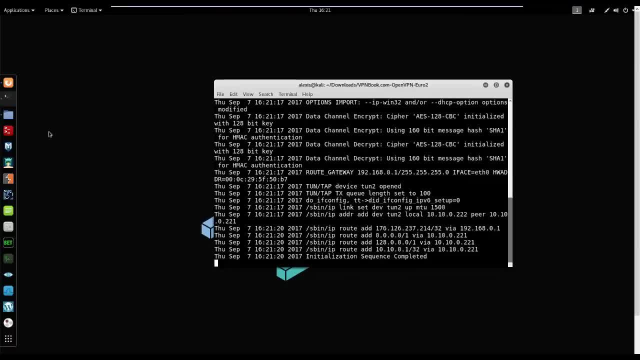 onwards, you're connected to the VPN. now again, the speed may not be the best speed, but it's good speed. I can. I can vote for that, so I'm just going to close it. I'm just going to close this up and we're going to try and open up a site. 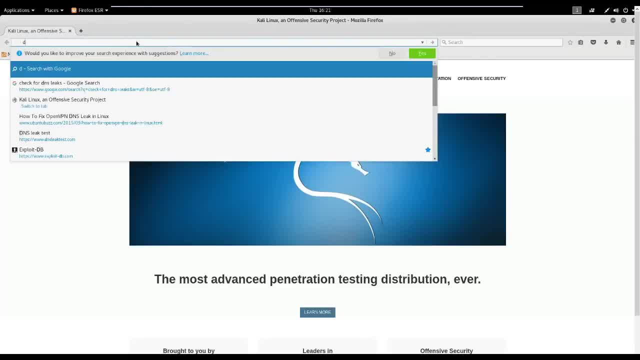 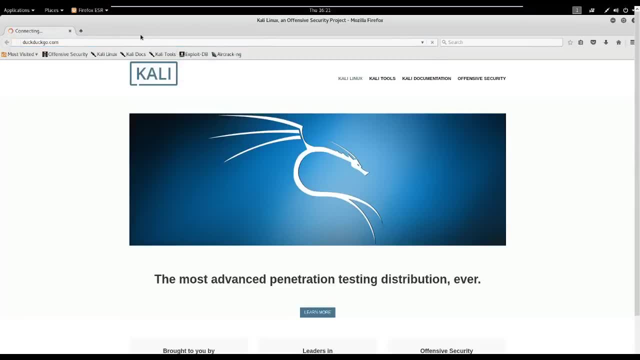 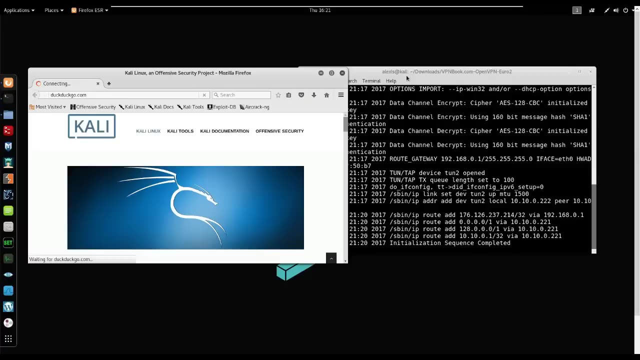 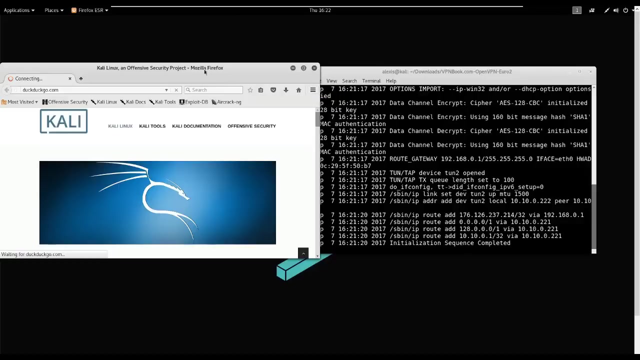 here. so let me just try and open up duck gocom like so, and let's see if it allows us to access. that means we essentially have connected to the VPN service, or service for that matter. don't worry if it's a little bit slow at the beginning, that is. 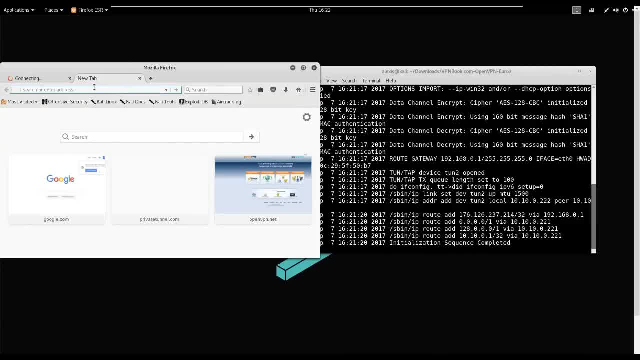 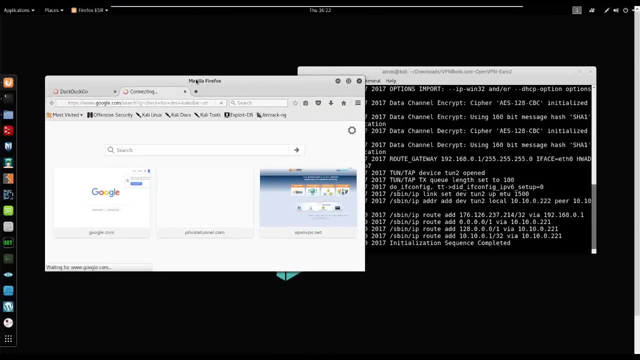 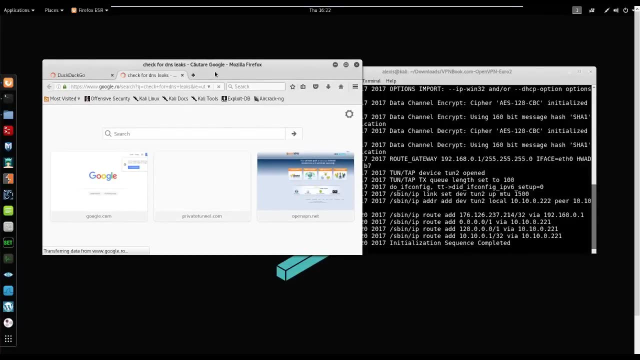 usually what happens, but, as I said, don't don't worry if that's that's the case. so I'm going to check for DNS leaks as well, because I just want to show you that it indeed changes the IP but will leak some of my DNS information unless I change it. but for this- VPN certificates, I'm really 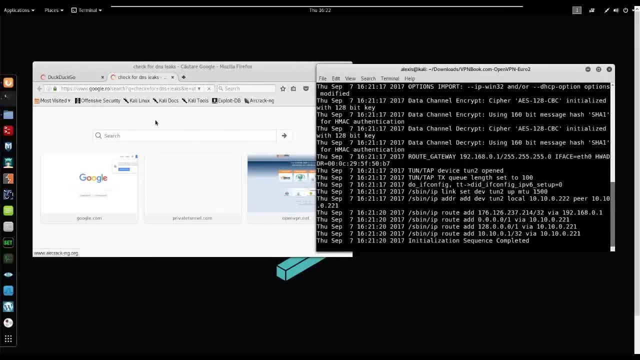 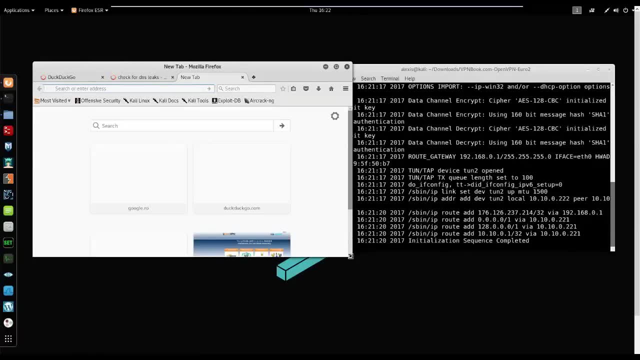 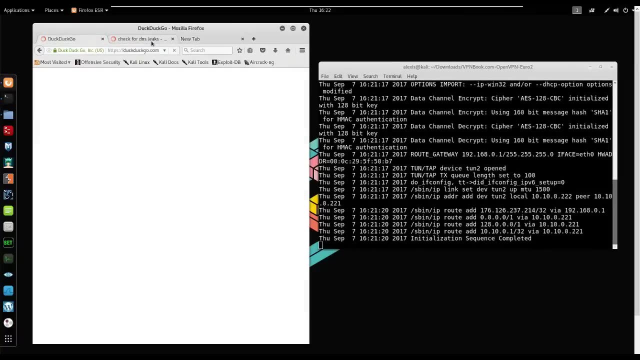 working on a way to stop the DNS information from leaking, but I'll get to that probably in another video. now, as you can see, it's quite slow. nothing really is opening. let me just enlarge this slightly here so we can have a split menu and we can see what's going on. so, yeah, it's loading up, but quite slowly. Oh, dr Koo is opened. 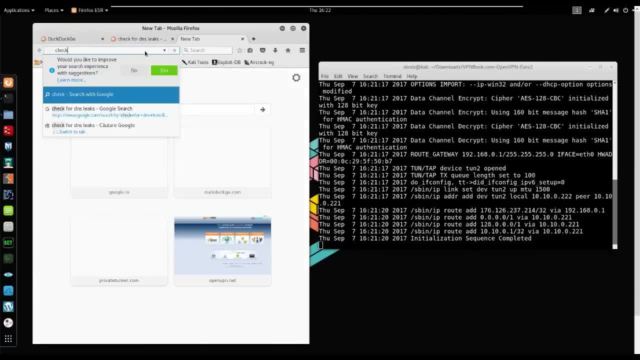 up and for some reason it's taking quite a while. let me just open up another check for DNS tab. I can already tell that it's changed my IP because it's giving me googlero. I'm not sure what. what country that is? probably Romania, probably I'm not sure, but 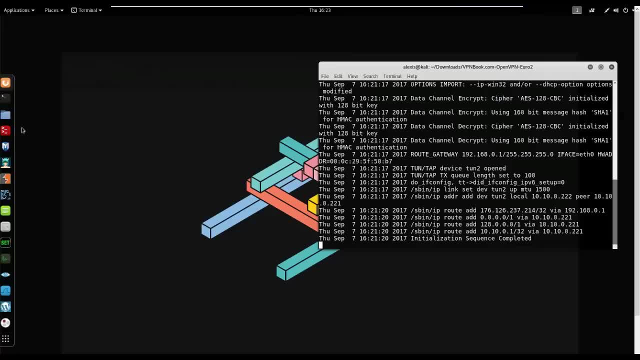 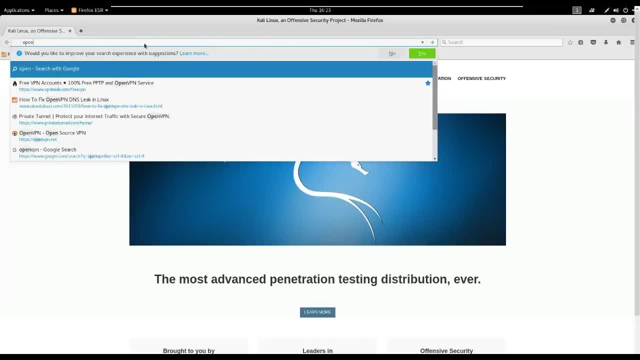 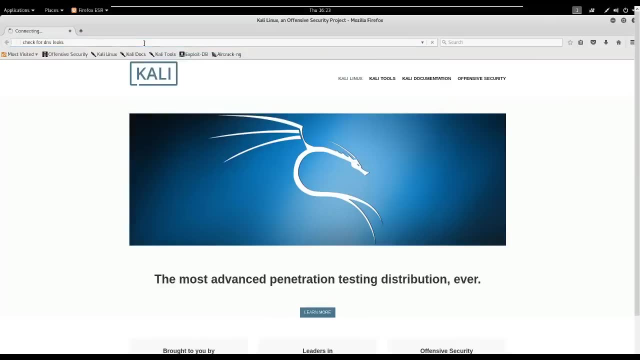 if it opens up, that would be fantastic. or let me just close these three tabs. this is usually the problem with VPNs: they're really really slow if you use the free versions, but it shouldn't be that. I'm really curious as to see why that's. this is the case. so for DNS leaks, okay, and if I just try and 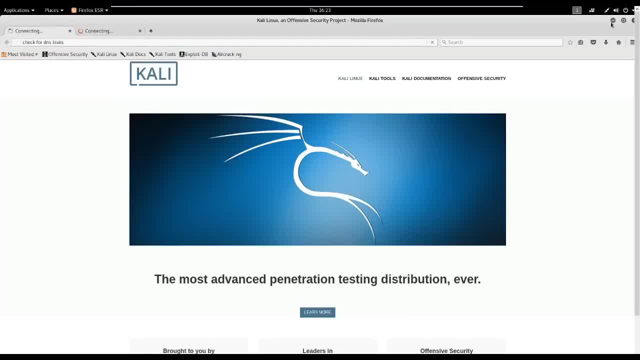 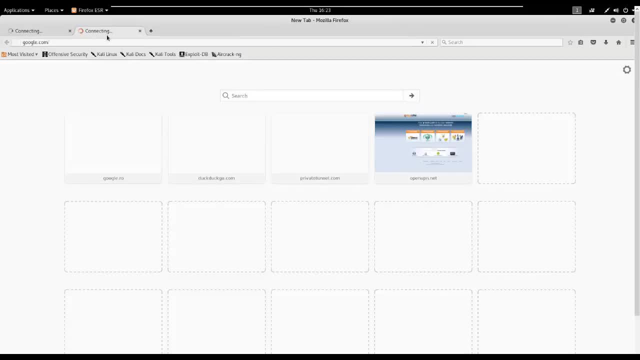 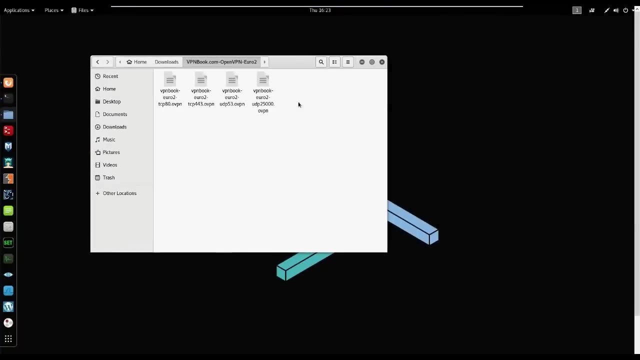 open up a search engine like Google, it should open up quickly. I'm not sure why it's giving us. it's really really slow right now. that is pretty weird, but it should load very quickly now. if I was to examine the files which I'm going to show you right now, we're using the 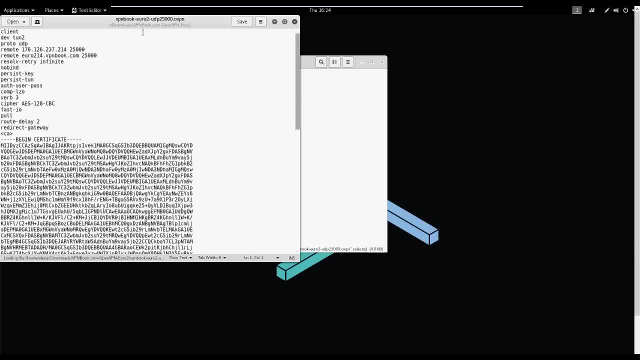 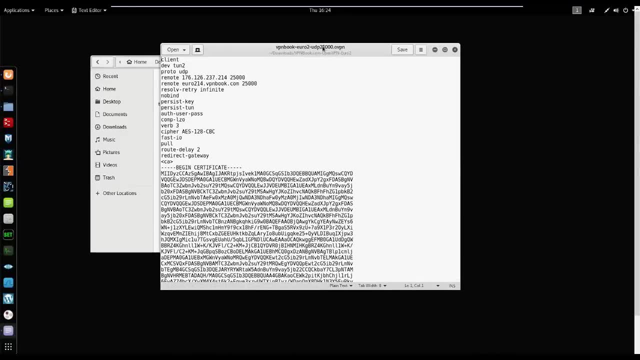 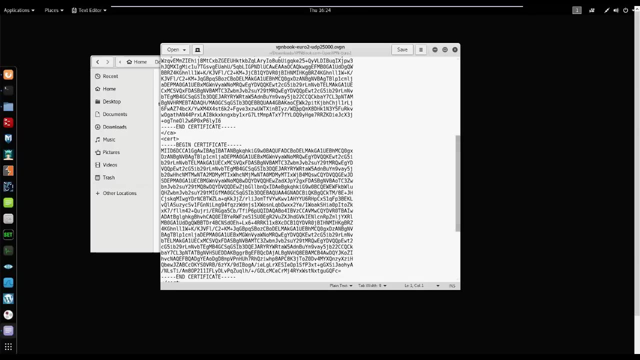 UDP 25,000 dot open VPN file. if we open that up right now, you can see there's some parameters here that we can change, and this is what I'm guess, guessing. you can set some security information that will change the DNS leak information. as you can see, you have your private keys, your certificates. 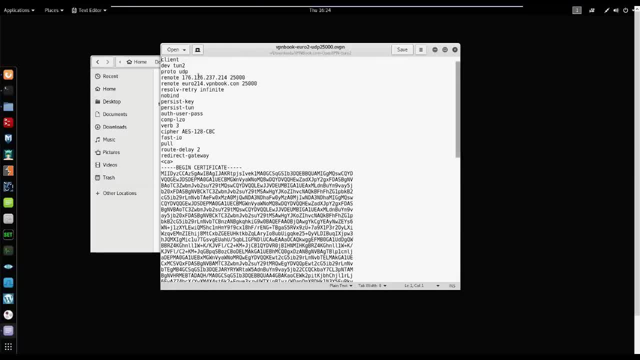 and stuff like that. so, as you can see if I can just explain a few things, it's: this is the remote draw, as you can see: euro 214.vpnbookcom with the port number: uh, no binding persist. the key of the user password combination which you have entered is then going to use the encryption AES 128 bit. I'm. 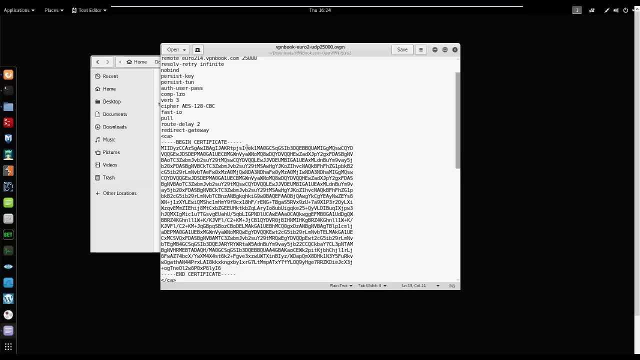 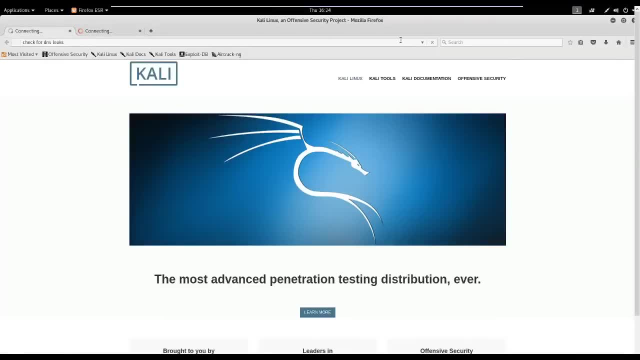 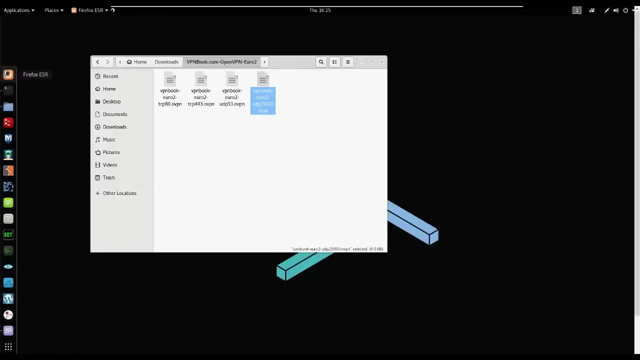 guessing fastio it's then gonna pull and redirect to the Gateway. so I would recommend, if you know, this is pretty interesting stuff, just to see how it all goes through. and we're still loading here. this is really really slow guys. I'm actually quite shocked at the moment, but it's always good to test. 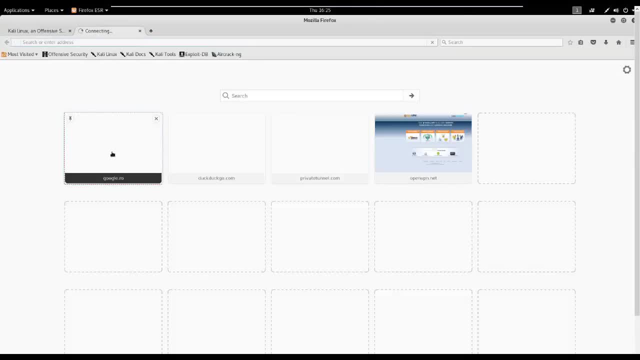 things on the fly, and it's also good for me to do that. it would be a shame of if I cut the video and I pretended that it was working when it wasn't right. so let me just try and open up Google here again and hopefully it works. or if it doesn't work, uh, what we'll have to do is, as we'll have to use, 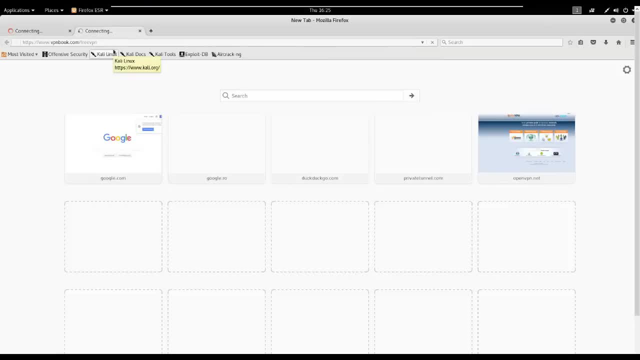 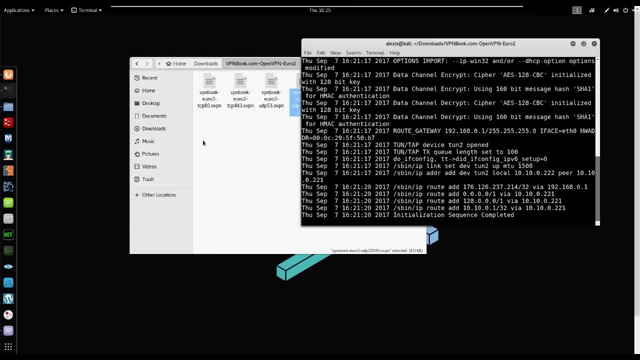 another. we'll have to use another VPN uh certificate bundle from probably another location, probably the US location, because this is looking really really slow, as I said. um, it could be due to the fact that there are many users on it right now, but again, I can be sure. uh, so what I'm going to do is I'm just going to close. 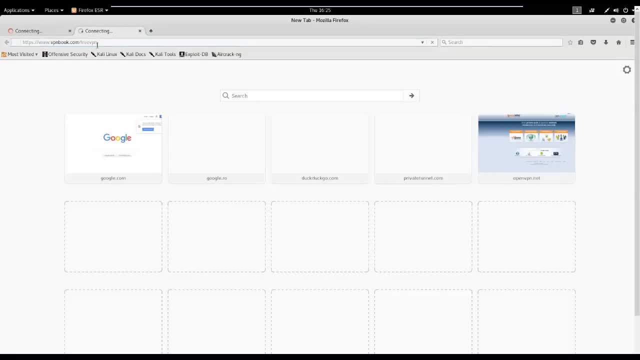 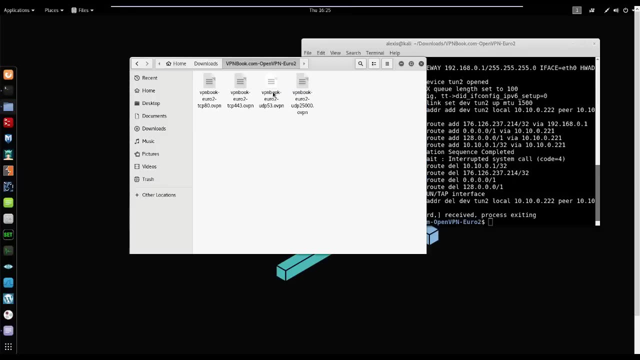 this one up right now and hopefully that will allow us to access something here. uh, when I go back to my normal internet connection, what I'm going to do is I'm going to use the UDP um UDP 53, so rename. I'm guessing. uh, quite few people, oops. uh, excuse me, um rename. 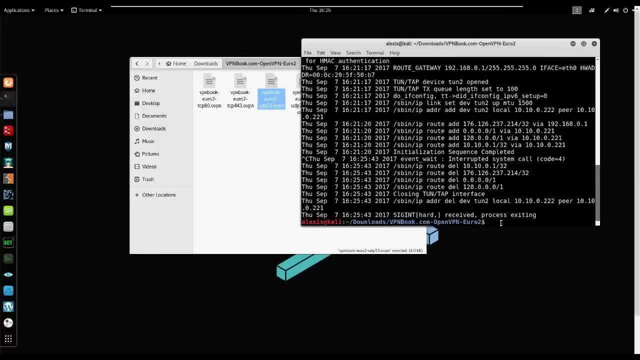 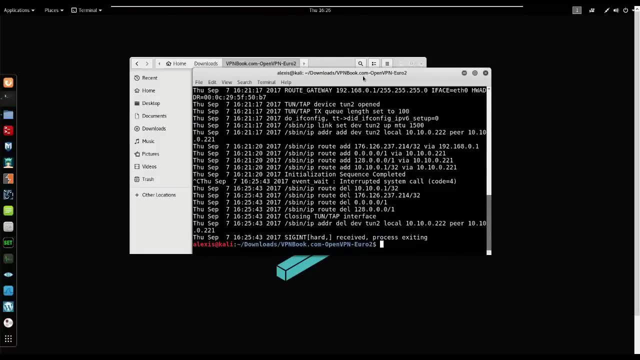 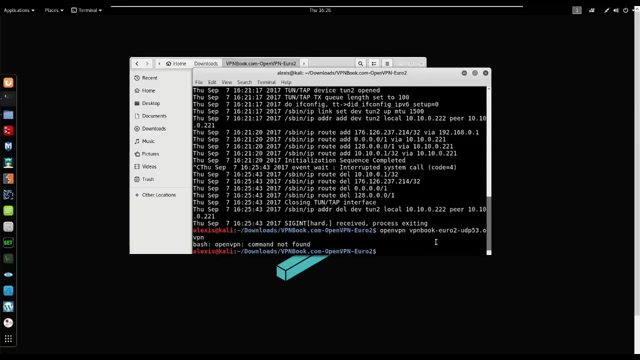 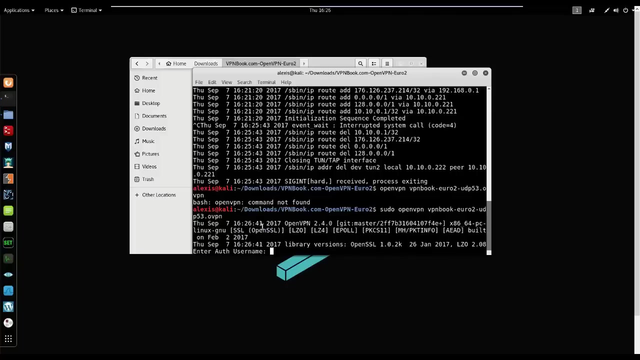 oh, my God man, my fingers are letting me down today. all right, so let me just use that service again this time. uh, we're already in route. uh, open VPN, like, so I'm going to put that in, hmm, for some reason. oh, yes, sudo, open VPN. excuse me for making some really amateur mistakes here. 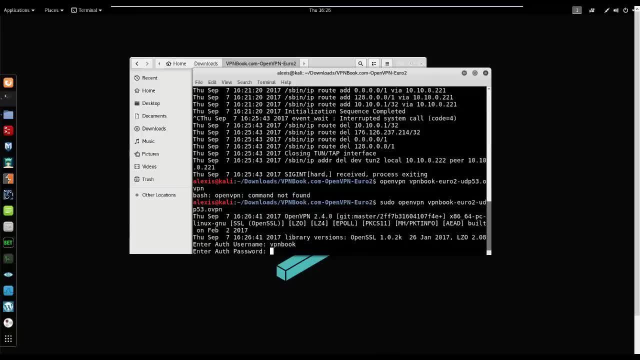 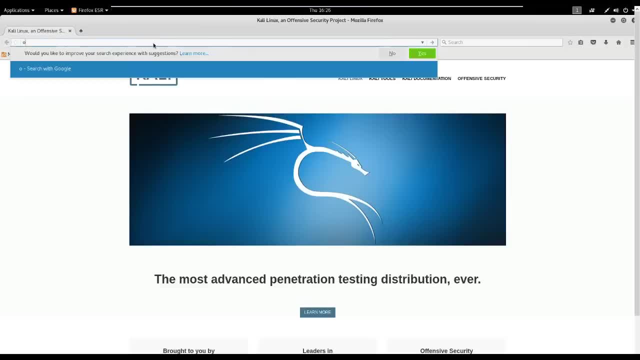 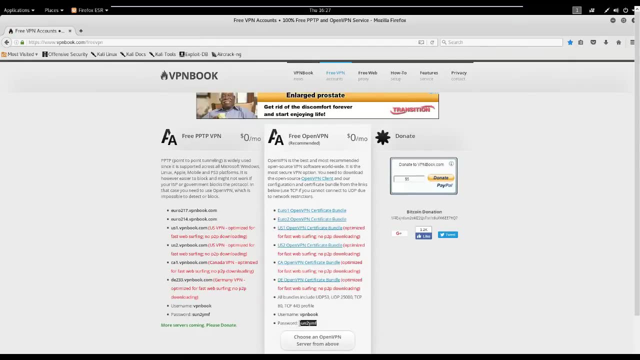 um, VPN book. I'm guessing that's the username, if I remember. VPN book. what's the password? oops, we need to look that up. how could I have forgotten to do that? so let's look for that like so. hopefully my internet connection works without the VPN service, so, as you can see, my 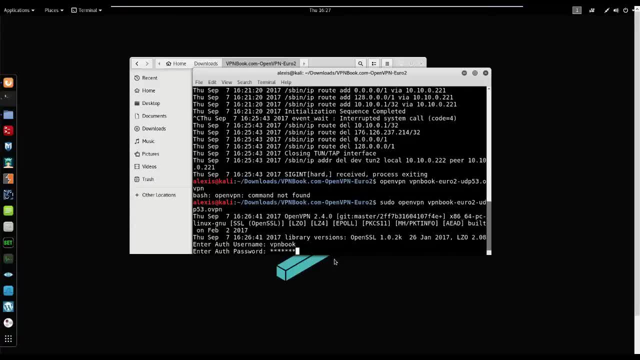 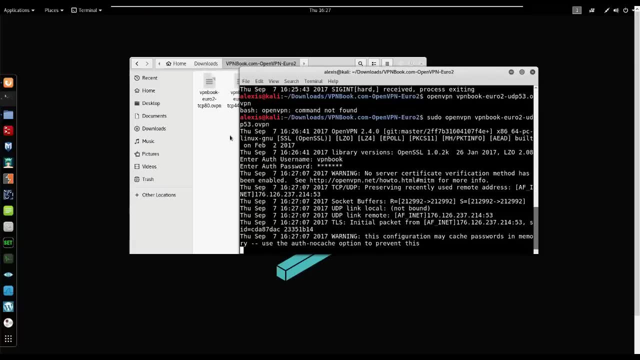 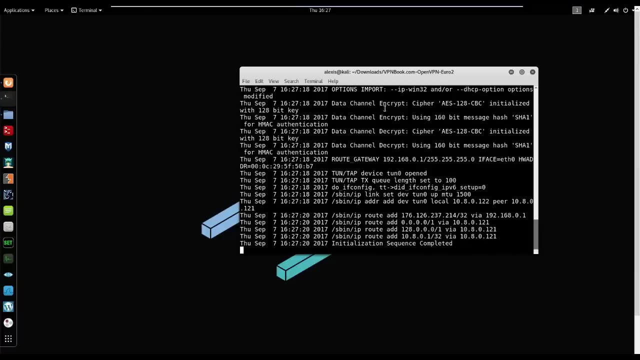 internet works perfectly. uh, when I turn to the VPN, I really get a slow connection, so let me try and use this right now. uh, the UDP 53 certificate file. um, yeah, it looks like it's working. yeah, all right, so initializing sequence is complete. let's see if that works at all. 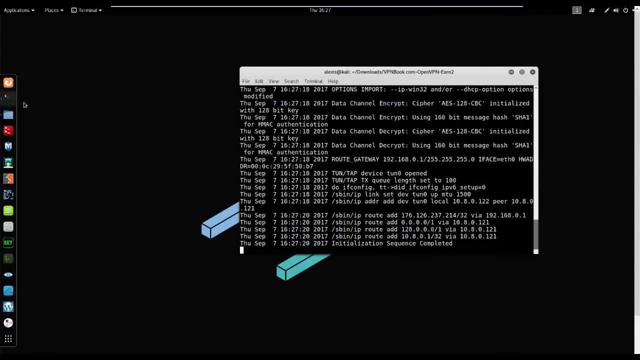 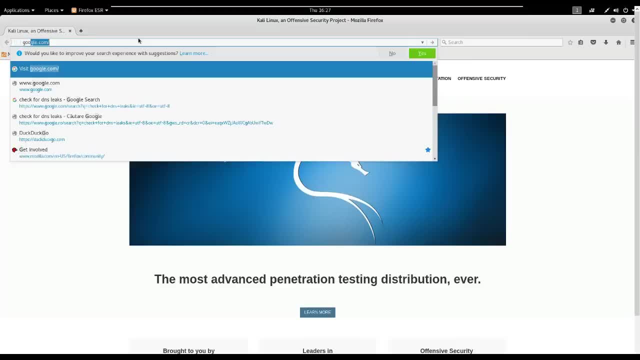 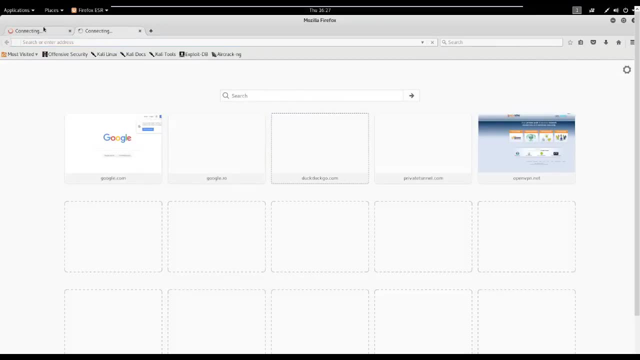 so I'm going to close that out up. it's always good to restart the browser just so everything loads up correctly with the correct uh VPN settings that you have set. so, um, again, I'm just going to try googlecom and let's see what we get, if we get anything at all. um, drgocom, let's try and open that up as well. 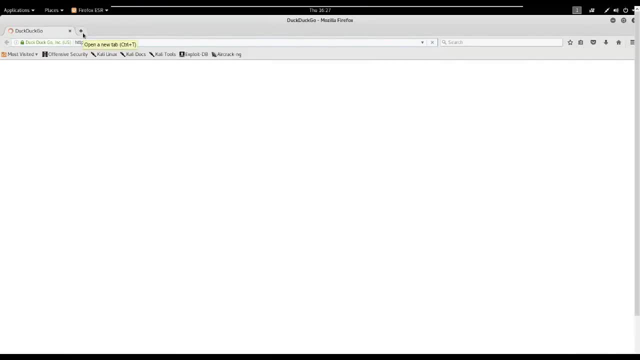 and there we go. okay, doctor go. seems to have opened. I don't know if this site will open up. that's the error that we keep on getting. all right. there we are. so, as you can see, now works if we use the UDP 53 certificate file. again, it's very, very. 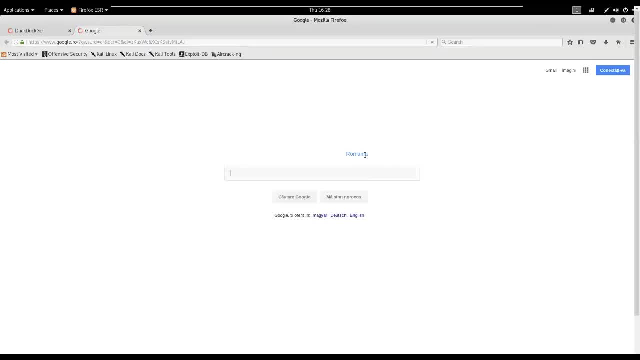 slow, but I can tell you that we're in Romania and the fact is I don't live in Romania, so that just tells you that, indeed, the IP has changed and I can use the VPN. I really I'm really shocked as to how slow it is, but I said it's. probably under heavy load right now. the servers are currently being used a lot since they are free, but I'll be finding different other different free options available that you can try out, especially for Linux. but this is again where what I was trying to point out- proxy chains are just so much better at. 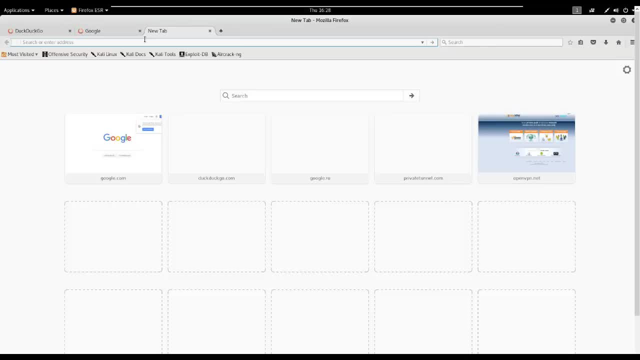 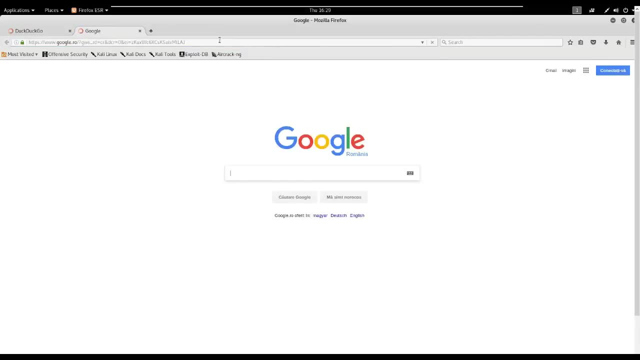 everything. they are faster, even though they are slightly slower than your normal internet connection. they're just much faster, you know, you know. so it just really is a slow, slow process. but anyway, you guys can try this out and let me know what you think. you can try all the different, the certificate. 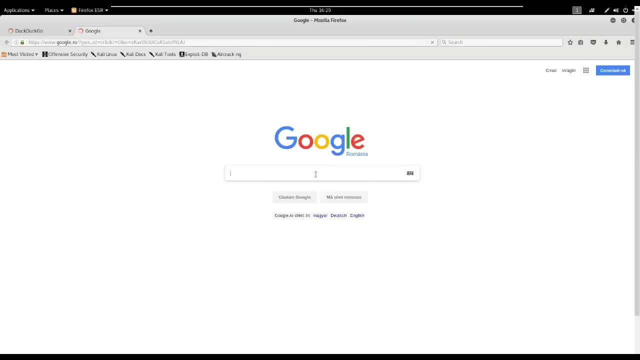 packages from different locations and let me know which ones are the fastest. and yeah, I hope you guys found value in this video. if you did, please leave a like down below. it means a lot. if you found this video helpful again, you might want to share it so that other people can get access to this video as well. if 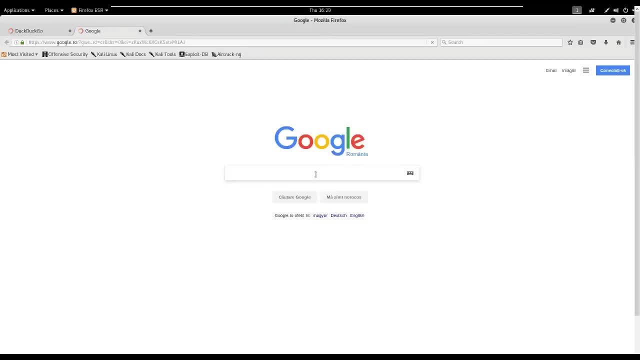 you guys have any questions or suggestions, let me know in the comment section down below, or you can hit me up on my social networks. I'm mostly on Twitter. that's my social network. I'm mostly on Twitter. that's my social. that's my number one social network networking site. you can again hit me up. 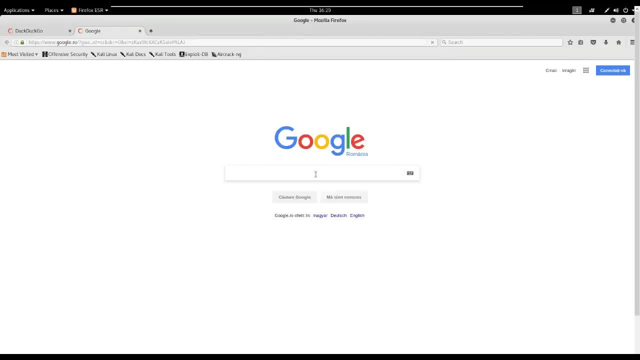 on Facebook or on my kick for personal questions. in addition, I've opened up a discord server for discussions. so if you guys want to have discussions on discord, you can hop on over there. the links will be in the description to all of my networks and you can just connect and we can just have a nice discussion. 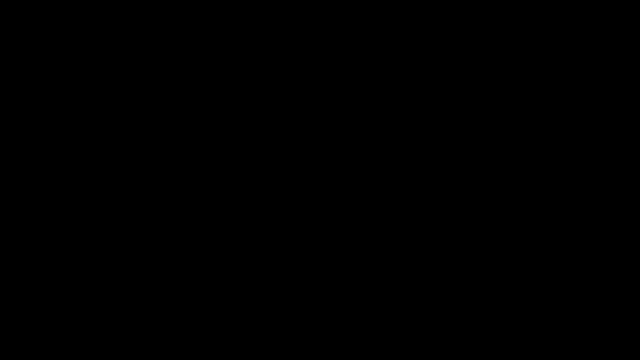 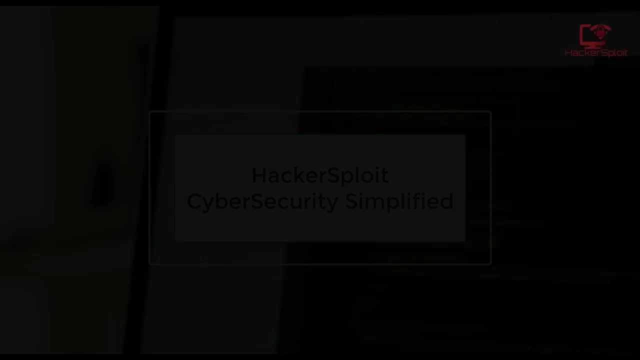 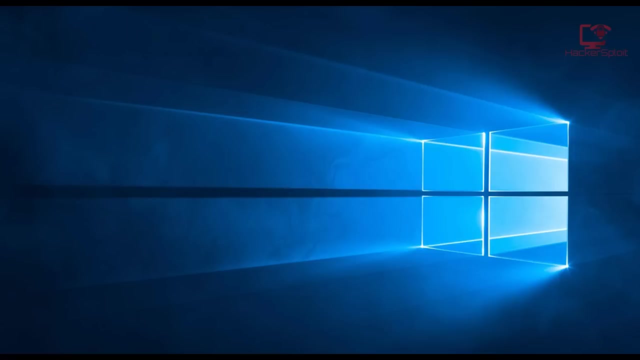 anyway, guys, thank you so much for watching and I'll be seeing you in the next video. hey guys, hack exploit. here back again with another video, and in this video I'm gonna be showing you how to set up your VPN with proxy chain so that it works. 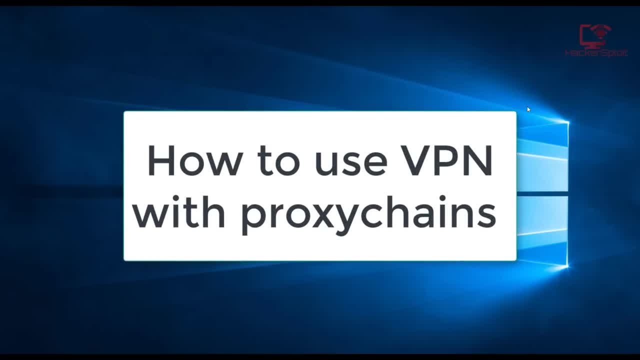 together with Kali Linux or parrot OS in a virtualized environment. okay, so I'm going to assume that you already have selected your VPN at your VPN provider. if you haven't, I would recommend not VPN. you can check them out with the link in the description. that being said, I'm not gonna promote anything else. 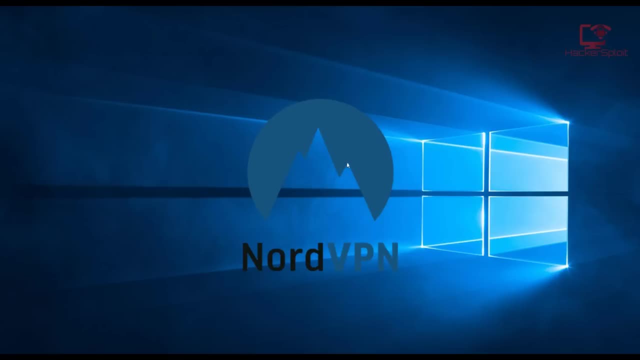 a lot of you guys have been asking me for this and whether or not it increases your security, and I'm gonna answer that in a second. but before I actually do that, I just want to say that I am making the videos dependent and in regards to the chronological order in which you guys posted them. so, for example, we have 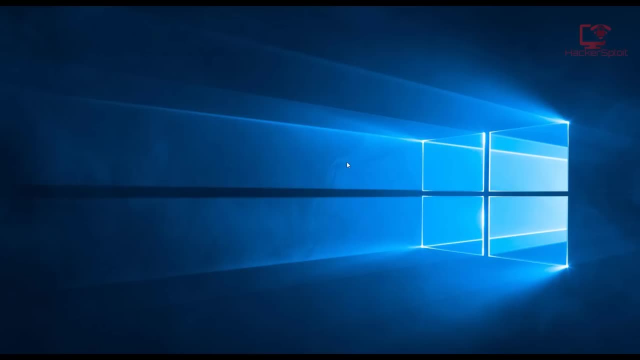 the two other guides coming out. we have the complete anonymity guide and the complete system hardening guide that was requested by mr GF- why? I'm just gonna call you that. so if you are watching this video and you're not subscribed to my channel yet, I will be posting the full video on the website as soon as I can. 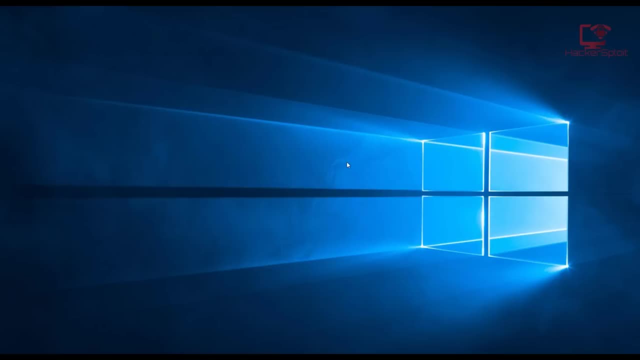 that video is also coming out. the SS 7 video was rejected by YouTube, so I'll have to upload it to the site. what else let me see quickly before we move on. the web application penetration testing series is still ongoing. that being said, let's get started with the video. okay, so I already have not VPN opened and I'm 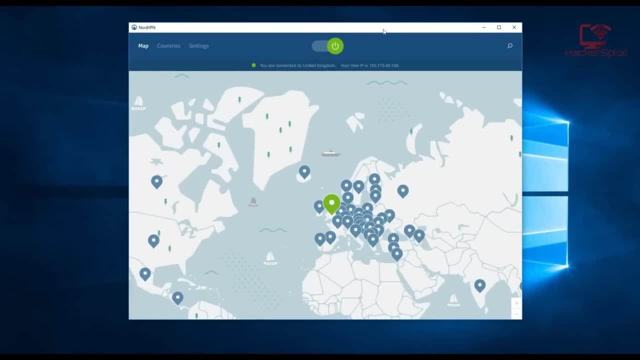 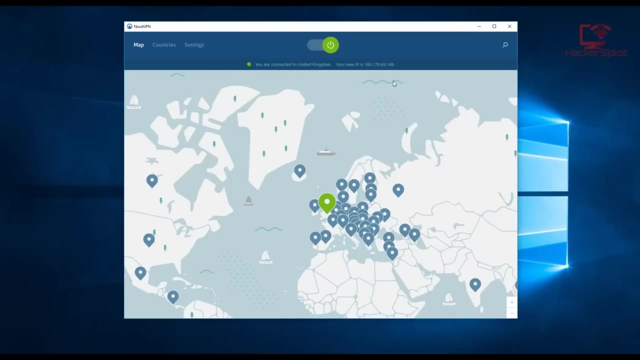 connected to a server in the United Kingdom. all right now. many people were asking: can I use my VPN in conjunction with Kali Linux, and then can I also use proxy chains, And will it increase security? The answer is yes, it will increase security, But at 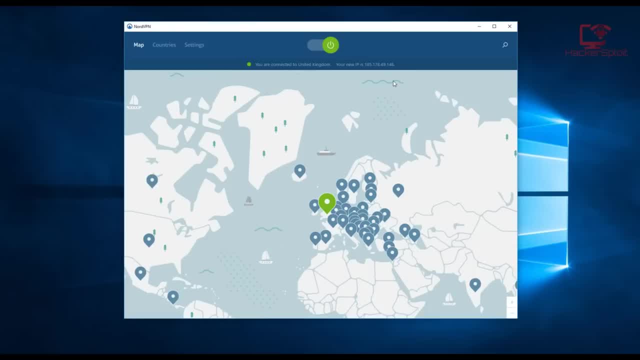 what expense or at what cost, you might be asking. Well, what you're sacrificing is speed. Okay, now again. for most of you this might not be an issue, But depending on the speed of your eyes, of your VPN service or your ISP, you know you have to take that all into into consideration. So again, 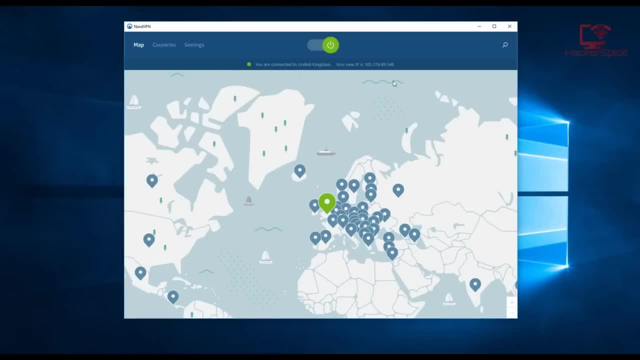 what I'm saying is your VPN might slow down your speed to a certain extent, And there's no question is asked there. And then, as we know, proxy chains is also very slow because it is going through a series of proxies And under the door network, that's if you're using the door relay. Okay. 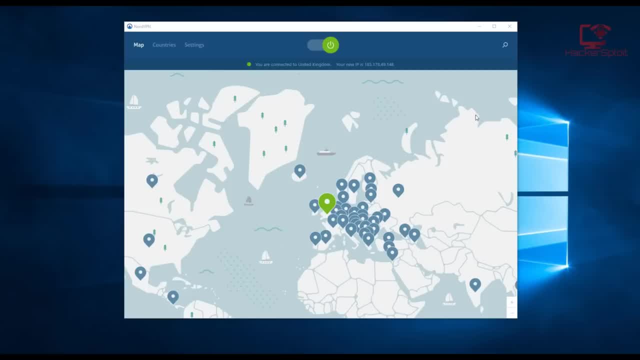 so the first thing I would recommend that you do is, on your host operating system, which I'm guessing is going to be Windows, but it could be Linux- you must change your domain name server All right Now. usually with most of the good VPNs like NordVPN, they will automatically use. 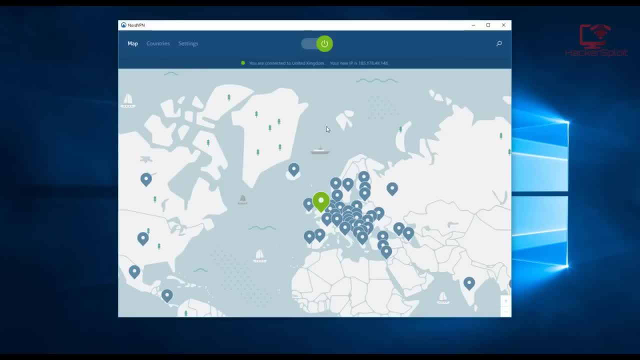 the domain name server in the well, essentially in the location Of that server. So, for example, if you're not United Kingdom, it's going to use a DNS from the United Kingdom, And now again, I do recommend that you use a safer one, probably like Cloud. 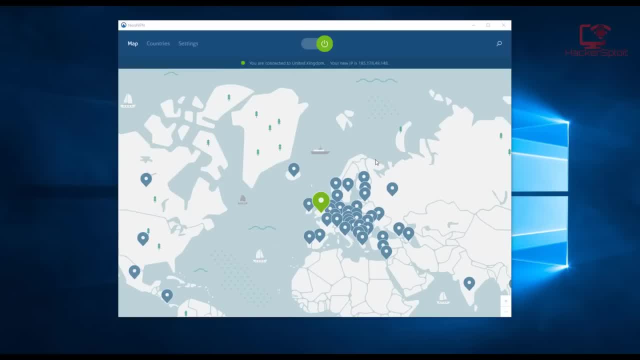 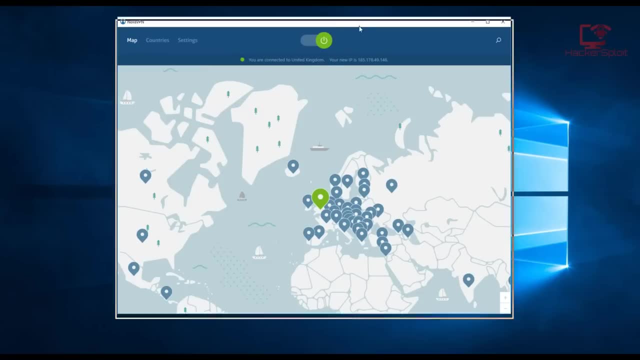 Flares or whatever you choose to use. that's all up to you. So make sure you have your domain name- a server- changed, or you can choose to use the one that your VPN is providing you with. whatever you choose, it's up to you. Now I have Kali Linux open here And the settings that you 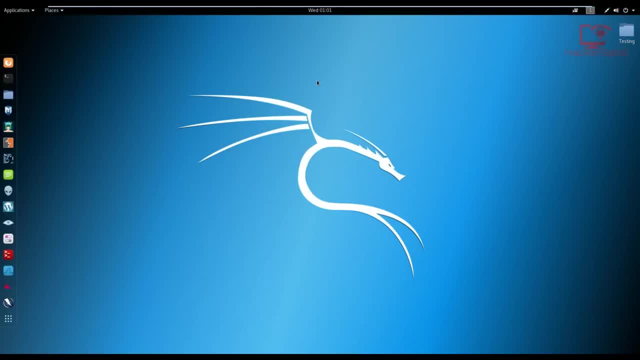 guys were asking me is how to configure it with my virtual machine. Now you're also asking me whether I should- you should- install two instances of your VPN: one on your host operating system and one on your virtual machine. And the truth is: 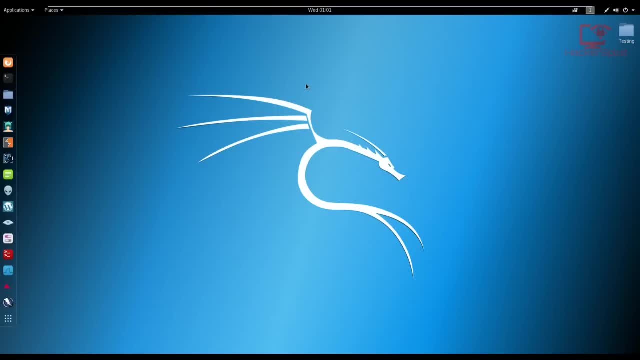 you don't need to do that. What you should do is you should use your host operating systems IP address on your virtual machine. if that's what you're looking for Now, you might be asking: well, why should I do this? Why can't I just run it on your virtual machine? the truth is: 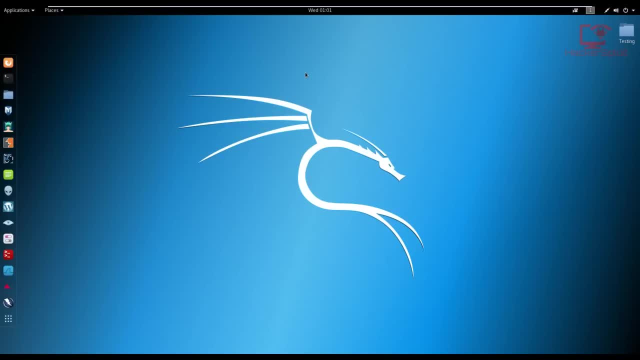 you can run it on your virtual machine, But, again, we're focused on minimizing the resources that are required by the virtual machine. So it's it's. I would recommend that you run everything on your host operating system in regards to connections and VPNs, And then you can use your penetration testing operating system. for what? 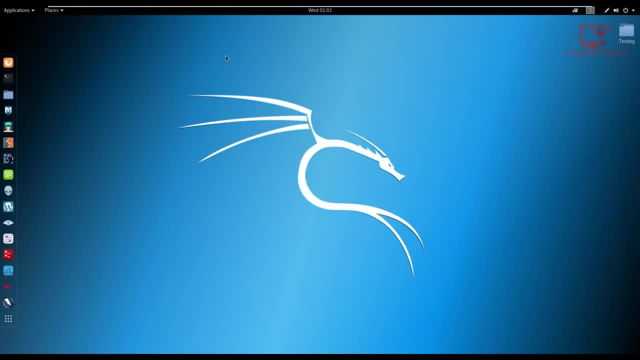 it's used for, which is penetration testing. Okay, so what I'm going to do now is I'm just going to show you how to configure that with your VM. So you're going to your VM settings. I'm going to be using VMware. the settings should be the same for VirtualBox, Although, as I mentioned, I'm really 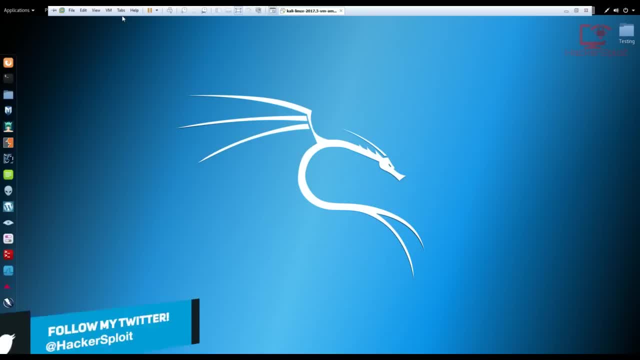 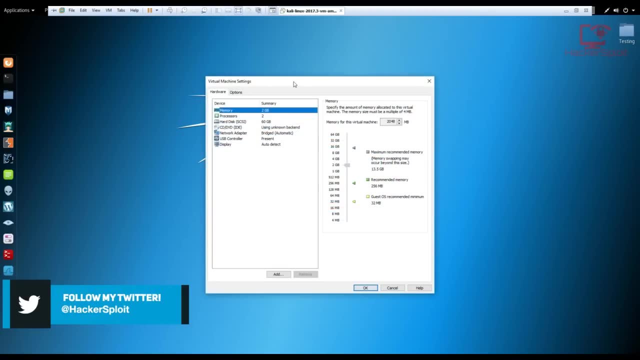 getting out of, out of touch or well, VirtualBox is not my favorite at the moment. So, VM and you want to go into your settings, All right. and you want to go into your network adapter, And instead of bridged, you can go for. 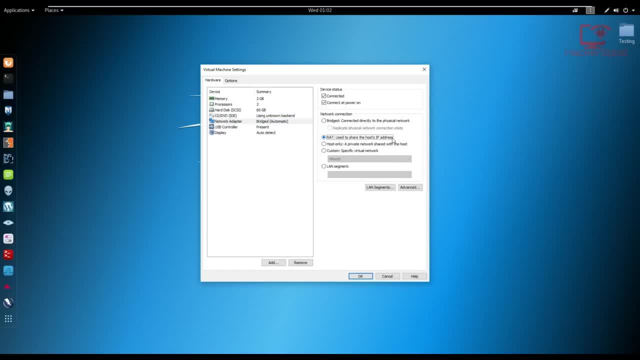 NAT. All right, Now, what this means is it's going to use- it's going to use- your host operating, your host operating systems IP address. So that means it's going to use Windows IP address, which, in this case, is the VPN IP address that is provided to us. So now Kali Linux will also be connected to 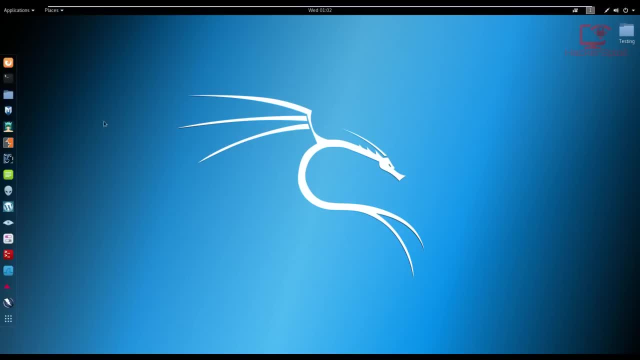 the VPN. All right. so once you do that, just hit OK. And for safe precaution, you can also change your your DNS settings here And you can also restart your network manager, just in case. but it should do it for you. As you can see, there we are. it is. 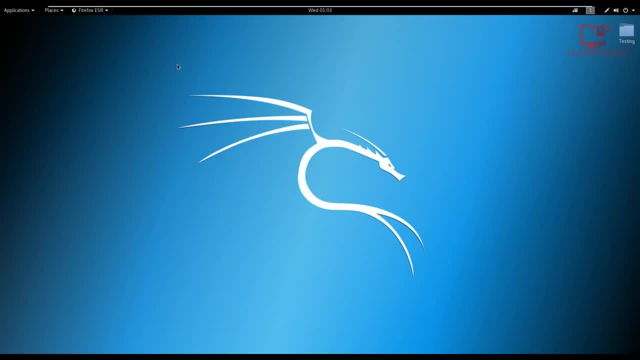 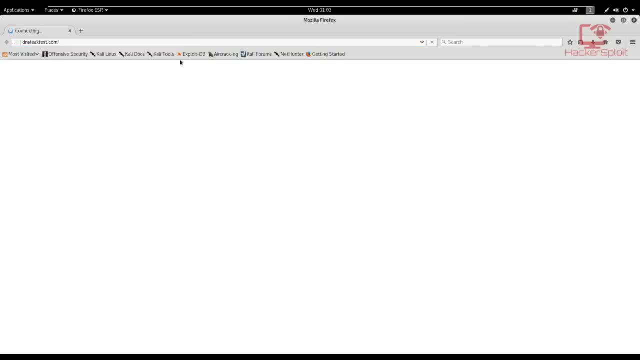 connected And what we can do now is run a DNS leak test just to show you. Alright. so let me just open the DNS leak test here. It turns out I was using the DNS leak test, Alright. so there we are. 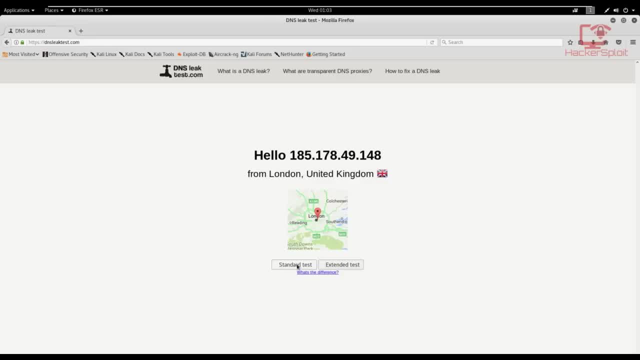 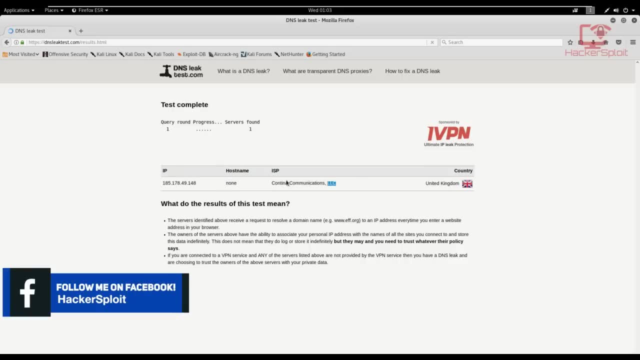 let's open that up And, as you can see, it's using United Kingdom. I'm going to perform a standard test to show you that it does use the domain name server in the country that the server lies. So you can see, it's United Kingdom. 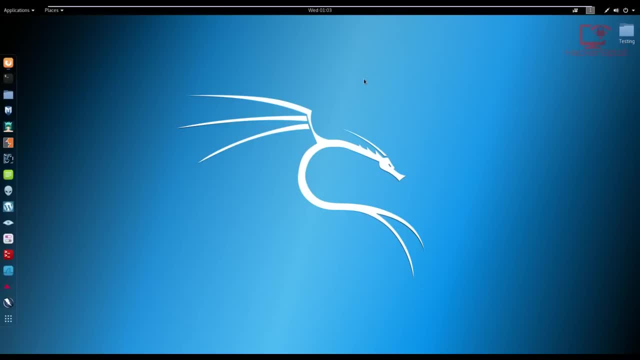 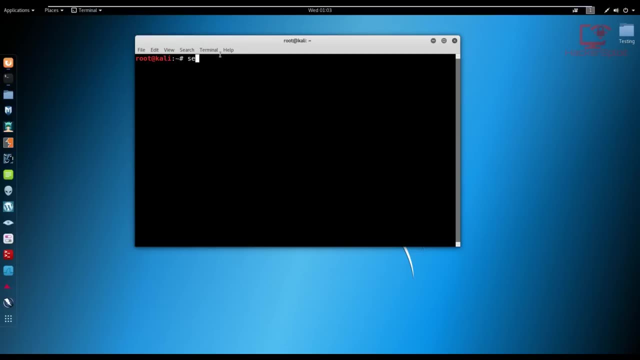 Now you're asking me if I can use proxy chains in conjunction with my VPN, And the truth is, yes, you can, but you're going to sacrifice a lot of speed, Alright. so the first thing again, since we're using the Tor relay or the Tor proxy, is make sure you have Tor started. I'm going to 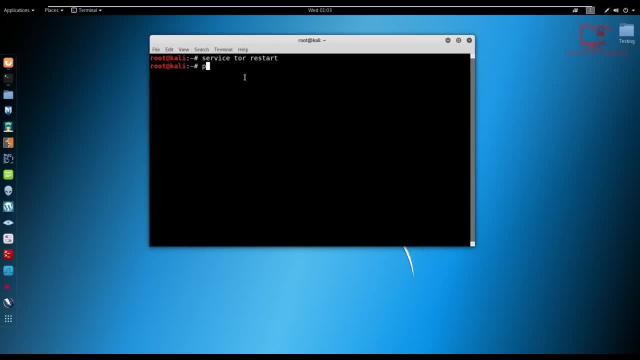 restart my service, Tor restart, and then you can use your proxy chains. You can use proxy chains in an instance with any program. So proxy chains. This time we're going to use Firefox because we are testing the IP here. Firefox and DNS leak test. Sorry about that DNS. 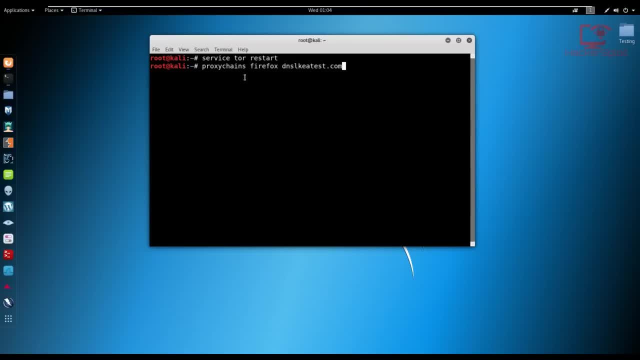 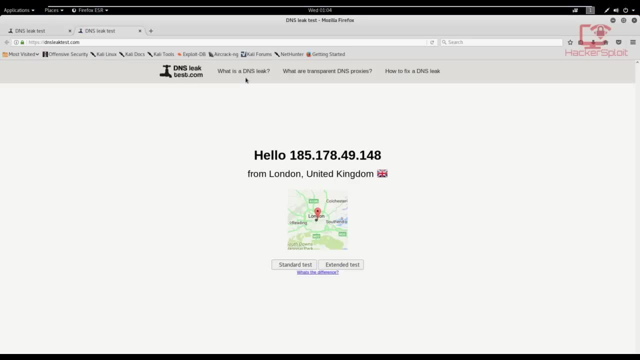 leak testcom. You know, my keyboard is quite far away from me. DNS And that's the wrong spelling there. leak, leak test. There we are And let me hit enter And for some reason it's still showing United Kingdom, And I think I know why is because we did not close down Mozilla. So make sure you're. 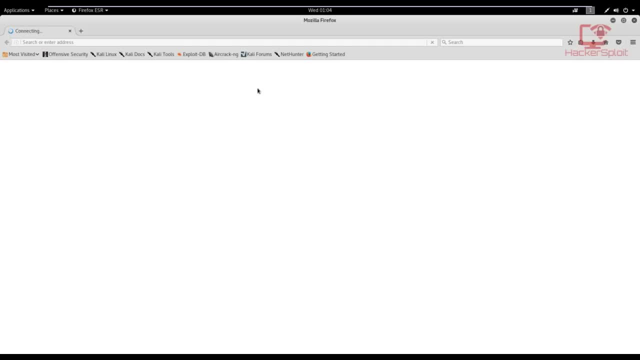 going to start a completely new instance. So let me start that again And, as you can see, random chain is working, So give that a few seconds to load up And you'll see that it is going to take significantly longer than with your VPN. As you can see from United Kingdom, we're now bouncing. 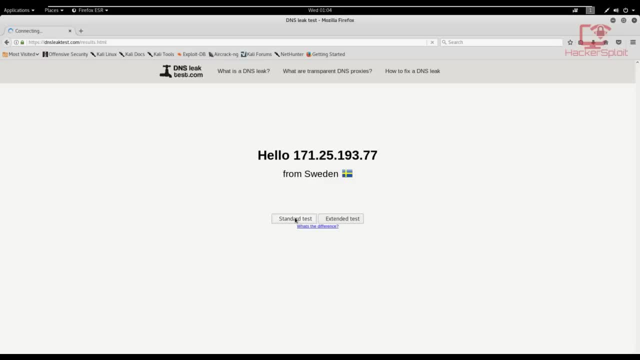 off to Sweden, which, as you can see, is quite different. So I'm going to perform a standard test and let's see what DNS that we are given here. They should not load up. that's because we're using the Tor proxy, And this is where essentially well looks like we are using. 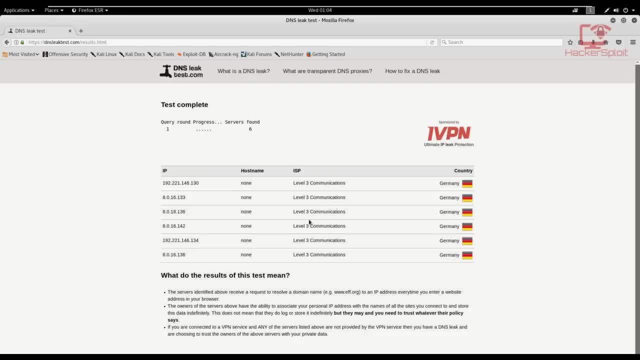 we're using a German one which is being provided to us by the proxy, But again, make sure that your, your first DNS, or the the first DNS server that your traffic is going to be flowing through, is a secure one, because this one won't matter, even if you know your first one was going through your 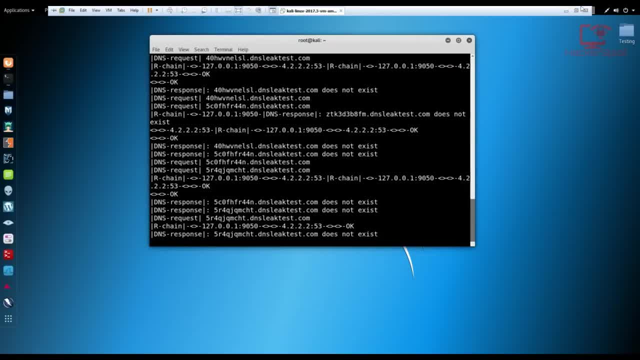 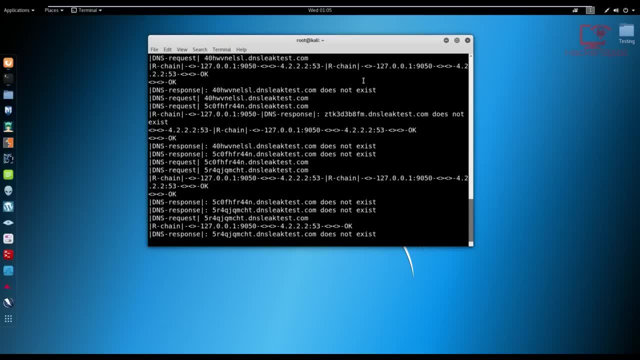 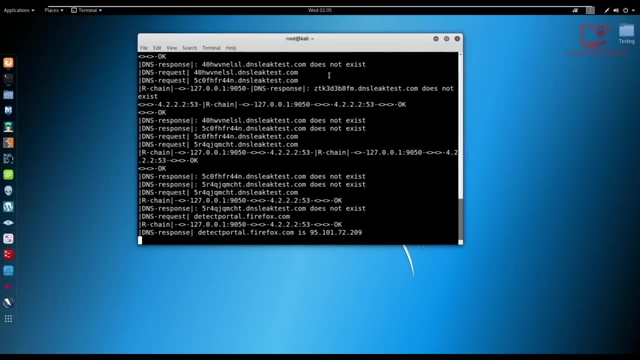 ISP. So again, make sure your host operating system has a trustworthy DNS And then make sure that your Kali Linux is also running a trustworthy DNS, And then after that you pretty much should be absolutely anonymous. And, as you can see, proxy change is working really, really well with. 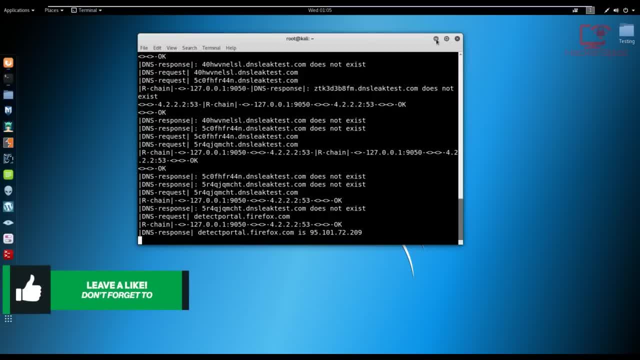 your VPN. That being said, that's going to be it for this video. If you found value in this video, if you enjoyed it, please leave a like down below. If you have any questions or suggestions, let me know in the comment section or on my social networks, Or you can also post your. 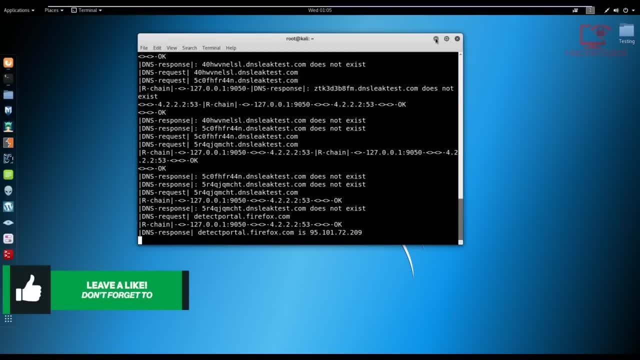 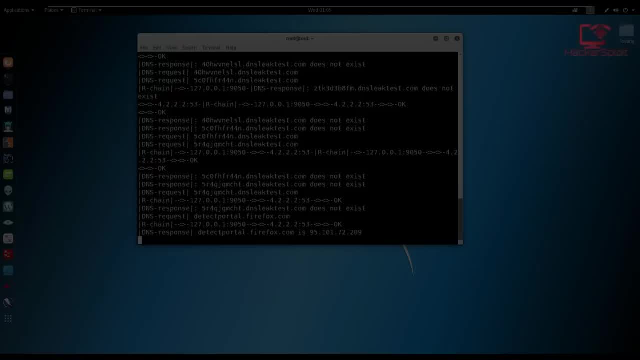 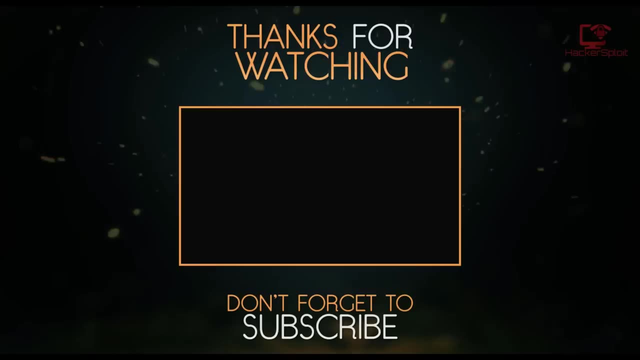 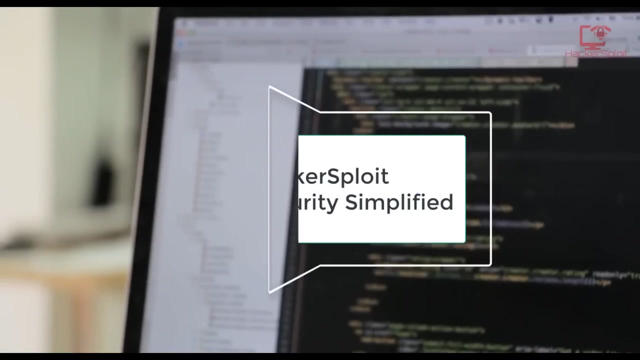 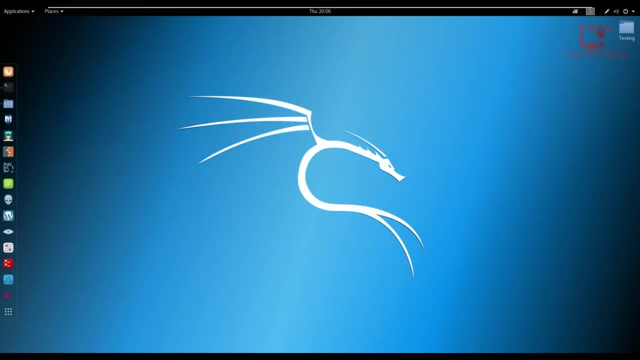 questions on my website. For the latest hacking news and resources, you can check out my website, hsploitcom. And that's going to be it for this video and I'll be seeing you in the next video. Peace, Hey guys. Hackers plight here back again with another video And in this video, 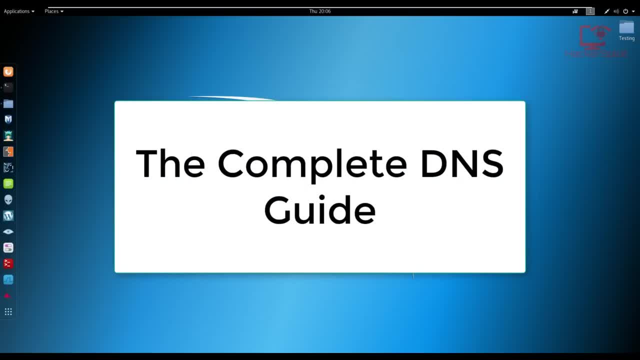 we're going to be looking at DNS y, DNS is important and how to change your DNS. And finally, we're going to be taking look at cloud fares, new DNS service- Alright, so again, you might be looking. you might look at this. 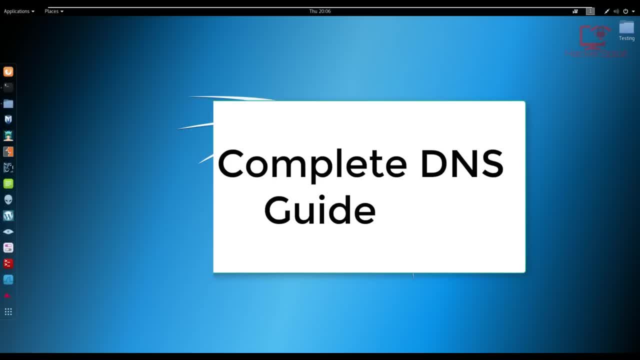 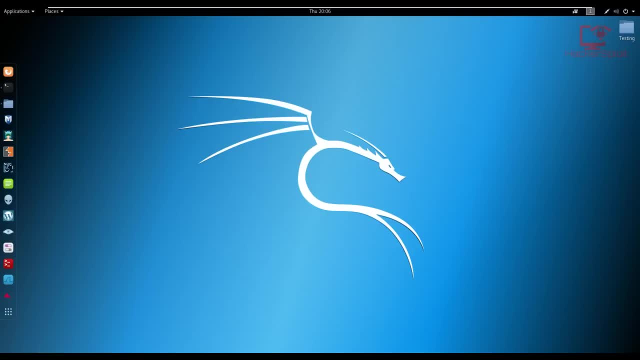 as your complete guide to a DNS, And that's what I intend this video to be. Alright, so why am I making this video? Let's start off with that simple question. Well, the reason I'm making this video is because I made a DNS video previously with the proxy chains videos. it followed up. 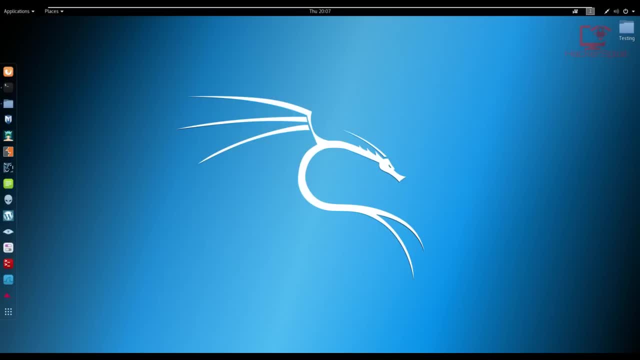 promptly after that, And I was explaining why it is important to mask your DNS or to change your DNS- Well, in order to give you a higher sense of anonymity, and I'm going to be explaining everything now. So, even if you know DNS, I would still recommend that you watch this video, because 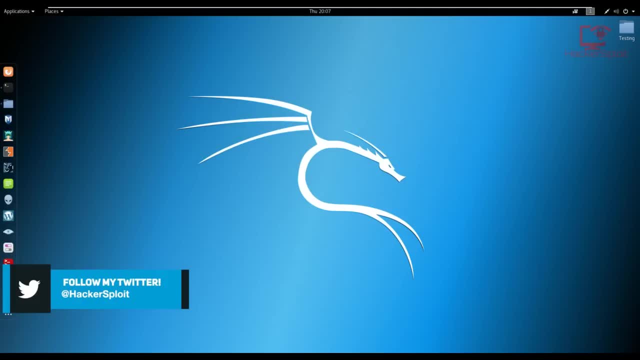 I'll be explaining a lot of small tips that you might have missed out. Alright, so don't worry if you're a beginner, just take it in, sit down, relax and let's get started. So the first thing you might be asking yourself if you've never heard of it is: what is a DNS? What is DNS? Well, 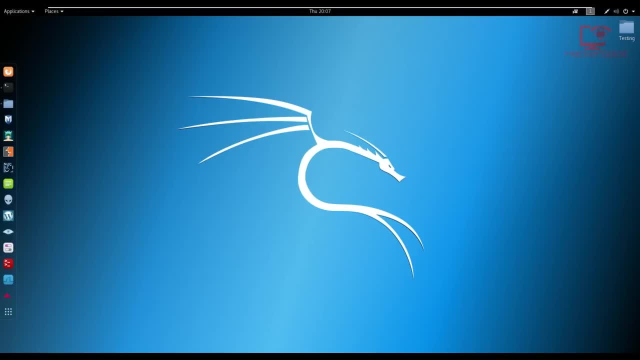 DNS essentially means domain name server. So what is the purpose of a domain name server? Well, it's its purpose. its simple purpose is to resolve a domain to an IP address. So let's say you go to your browser and you type in googlecom. Well, your what happens is your browser connects. 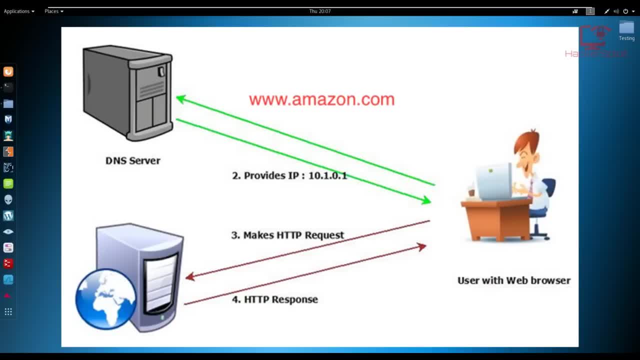 to the ISP. Alright, your ISP then connects to a domain name server And that domain name server checks: Alright, so this guy entered googlecom. Can we find any IP address related to googlecom? If it finds one, it gets that IP, it sends a request to that IP. 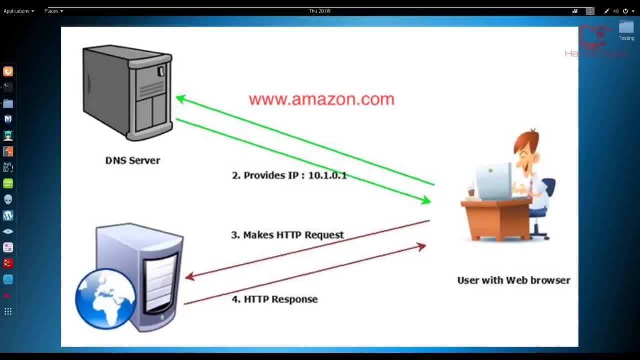 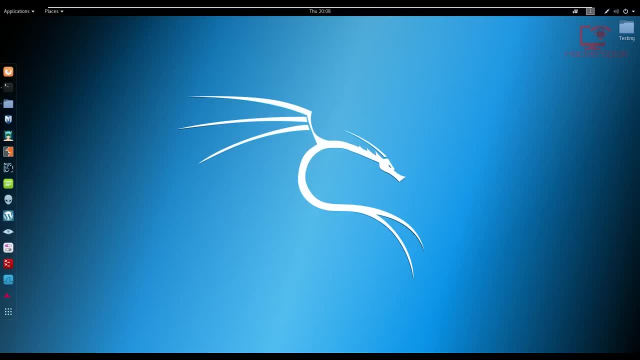 which is obviously Google Server. that server then sends data back, which is then processed by a browser. a browser and the web page is displayed. Alright, so a domain name server resolves a domain to an IP address or a server address, whatever you want to call it. 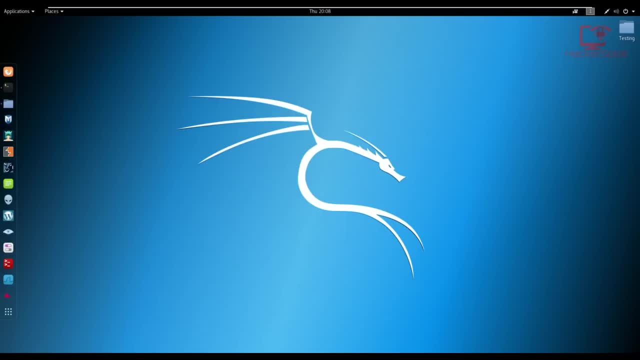 Okay, Now why is it so important in terms of anonymity and privacy? Well, the reason, as we were looking at with proxy chains and using it with a VPN- is: let's say, use proxy chains and you're trying to change your IP. Well, that's fine, But what happens if someone snoops into your? 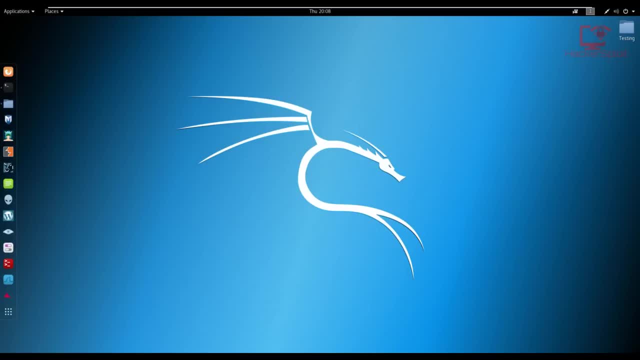 DNS information. Well, your DNS information will leak your ISP information, which of course reveals what country you're in. And if they know the ISP, they can easily get your IP address. And you know, there was no point in using proxy chains at all. All right, now we have looked at some of 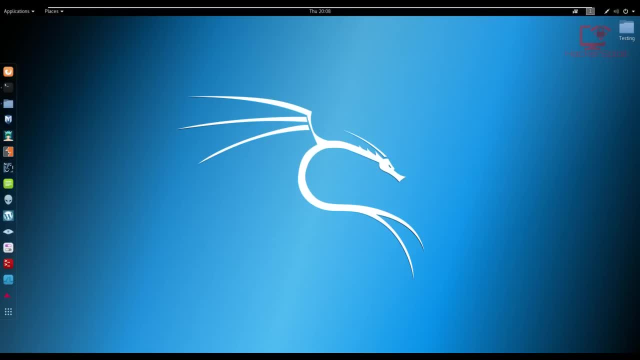 the, the most common DNS servers. in that video We looked at, we looked at open DNS, which is great, But nowadays become really, really slow. But the great thing about open DNS is they actually they actually keep your, your browsing activity private. So again, it cannot be so. again, it cannot be it. 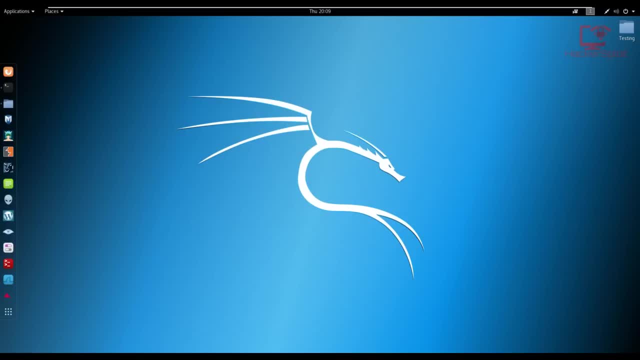 cannot be tracked, which is awesome. Now, the problem with the Google domain name server, which most of you are using- and I've really recommended that you don't use it- is because it only improves your, your page loading speed of the speed, for so, for example, Facebook, for example Google, 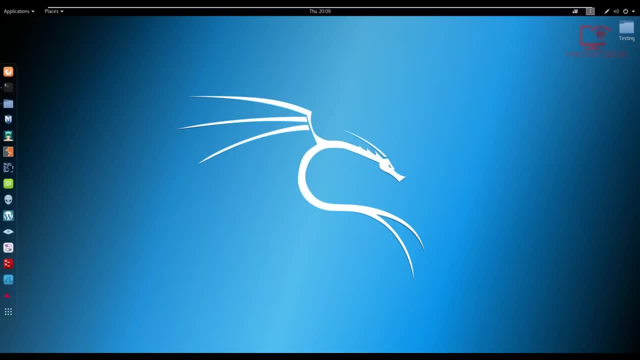 YouTube, so it only load sites faster, that it wants you to load faster, or you know sites that have essential services. hope you're getting the idea. So the DNS server for Google was 8.8.8.8.. Now that one I know. 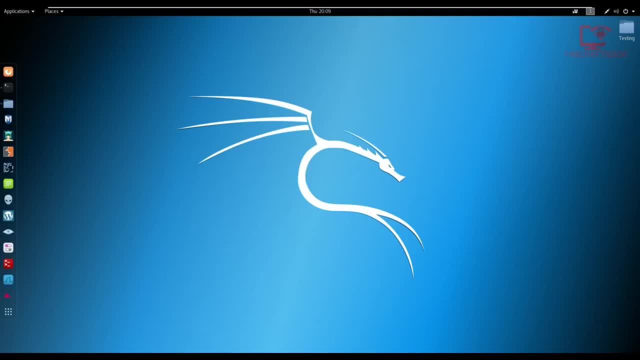 most of you have heard. many of your it teachers or professors have told you to use that. But please, for the love of God, do not use that. that is gonna get you in a lot of trouble, especially, especially- if you're planning to keep yourself anonymous, Even if you're using a VPN. you need to change. 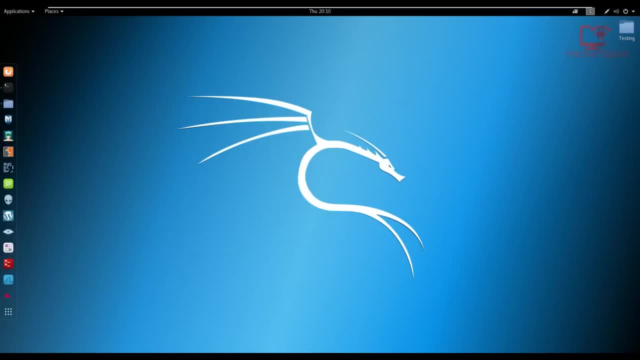 your domain name server, which is why I'm using the Google domain name server, which is one of the what we're going to be focusing on now. So I'm going to show you how to change your domain name server on Kali Linux and on Windows. Alright, so it's really very simple Now, as I said, 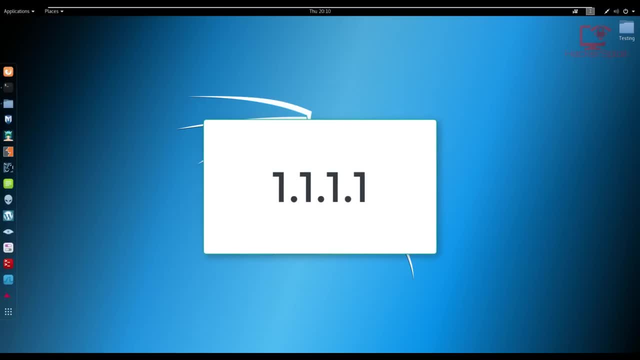 we were talking about, about CloudFares new DNS service, and their DNS service is simply 1.1.1.1.. Simple as that And it's awesome. And again, you might be asking yourself: well, why are we using? 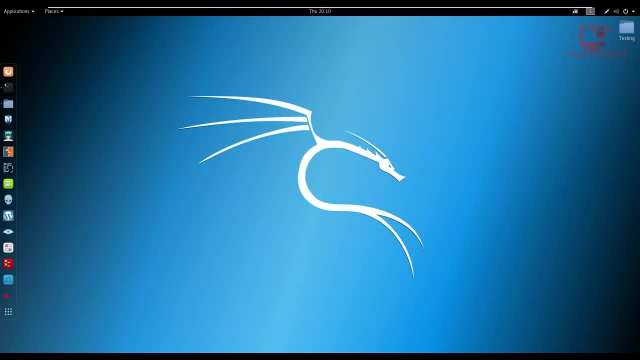 CloudFares new DNS DNS service. Well, number one. it's going to prove your browsing or page loading speed by 25%, And this is actually true. I've tried loading, you know, sites like the Washington Post, even on my mobile device. It was fun, It was unbelievable. 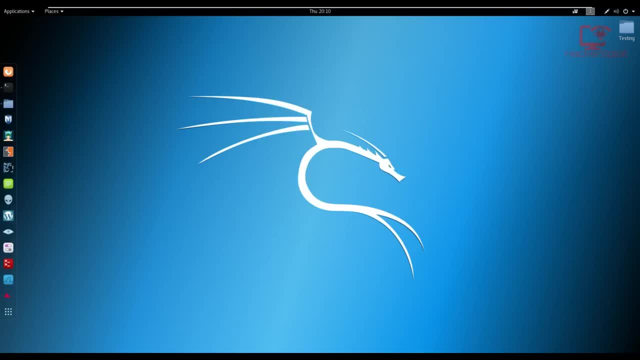 how fast it's loading the site. So the DNS servers are really really quick. And secondly, this was set up especially, especially and specifically for privacy and to prevent your ISP from tracking your browsing activity, Because, remember, if you're new and you, let's just take. 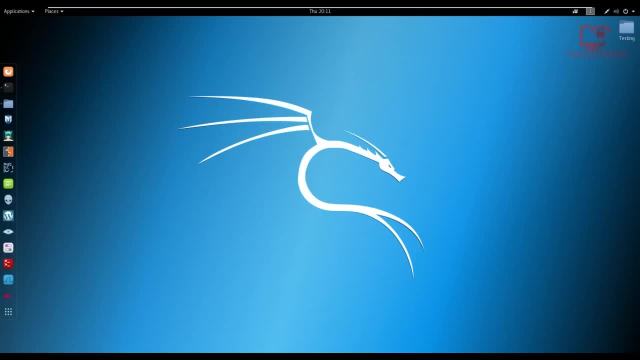 a simple example. Let's say you're a new user and you're using a browser and you're using a laptop. let's say you have your ISP installer router for you and they have provided you with an internet connection. Alright. so you, you know, you whip out your laptop and you connect to the. 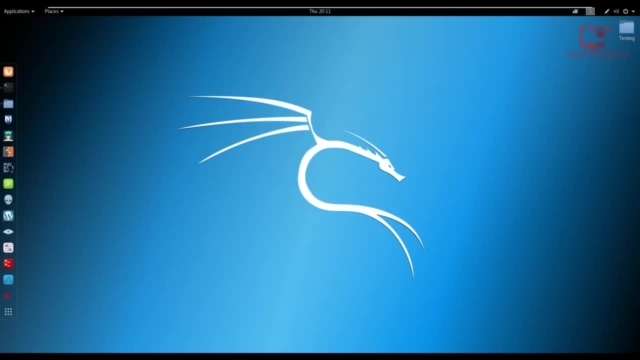 Wi Fi network And you think, wow, this is fantastic. Let's see, let me just whip out a VPN. Let's say you have a VPN and you're not changing your domain name server. Well, your IP is going to change. But guess what's not going to change? 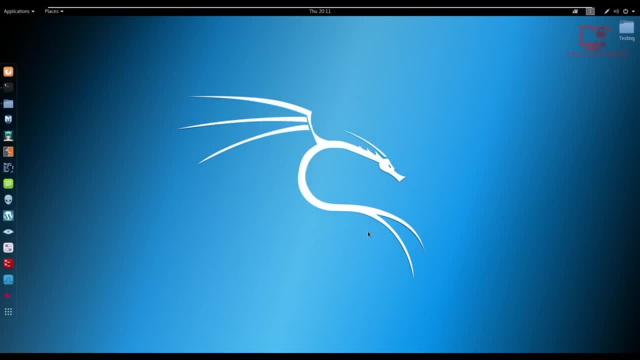 your DNS is not going to change And in most cases they have set the DNS to their IP or your IP, which is obviously theirs, And they're just going through your browsing history or activity if they want to, Alright. so again, if you're looking for privacy and you really, really want- 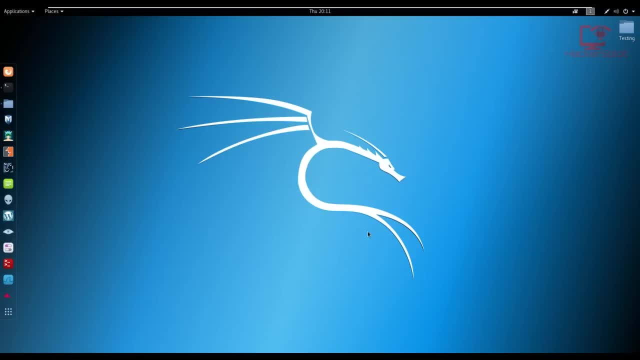 to or you're focused on fighting, on fighting net neutrality, phone or against whatever. I don't, it doesn't really matter. whatever your stance is, you know I'm with you, But again, I'm focused on freedom and anonymity and privacy of data. That's why I'm making this video, So let's 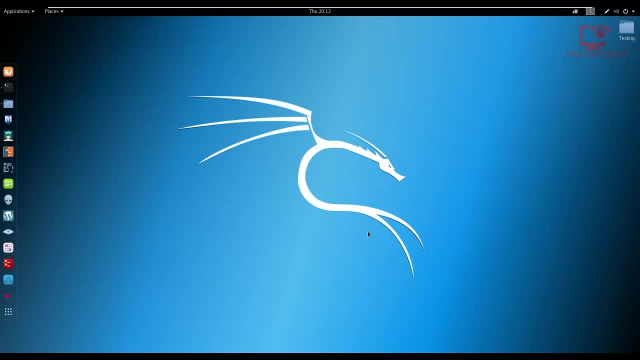 get started with how to change your domain name server. Firstly, on Kali Linux: Alright, so I'll be linking the blog post for CloudFares. I'll be linking CloudFares blog post in the description So you can check that out for yourself. Alright, so to change it on Kali Linux. it's really very. 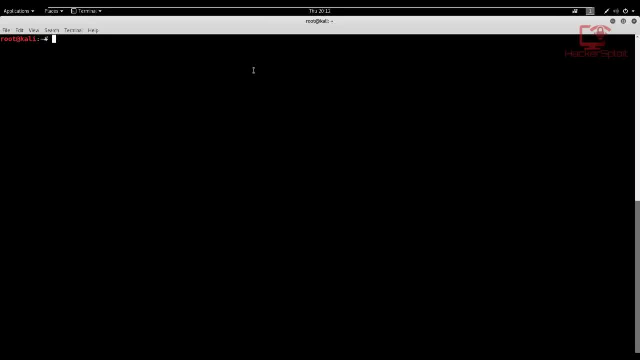 simple It is. it is essentially. the setting lies in a file called the resolve configuration file, which you can edit using any editor. whether you're using you can do this on any Linux distribution, doesn't really matter. All right, so I'm going to use the nano editor. you can use the G edit leaf pad whatever you feel is. 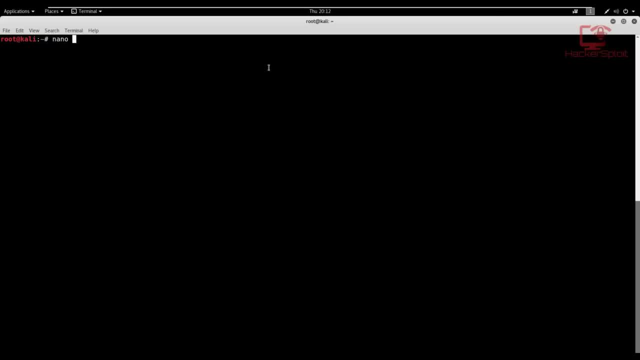 comfortable for you. I'm not going to force you to use anything. Alright. so, nano, it lies in the etc folder, or etc folder. Again, you can browse using the file explorer, if that's what you like, And resolvecom, Alright, resolvecom. That's. that's the configuration file. And if I enter, 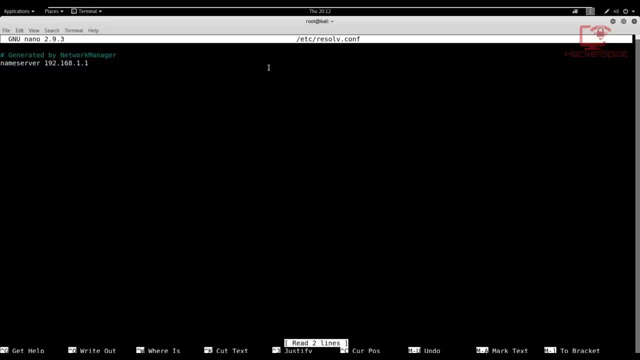 Oh, what's this? What's happening here? generated by network manager, as you can see, my current name server, or domain name server, is set to my routers IP address, which means again my ISP is going to be tracking the browsing history from this computer. Now I changed it back, just to show you. 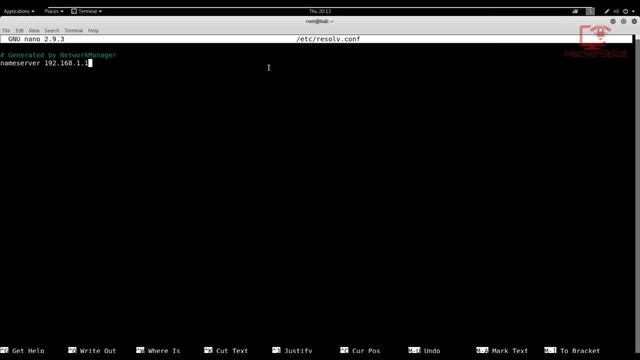 how dangerous and how insanely vulnerable you can become with with something like this. Alright, so simply, just just just get rid of your the- whether it's set to the router or your access point IP, and set it to 1.1 point 1.1.. Now, if you don't want to use CloudFares, 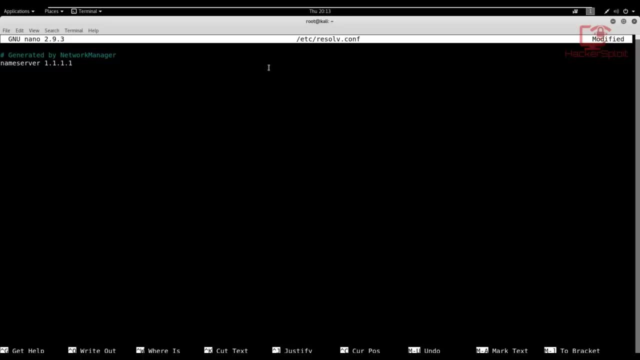 the domain name server. you can use open DNS, you can use Komodo DNS, you can use Google if you want to. But again, I'm going to be your friend here And I'm going to tell you: please, please, please. 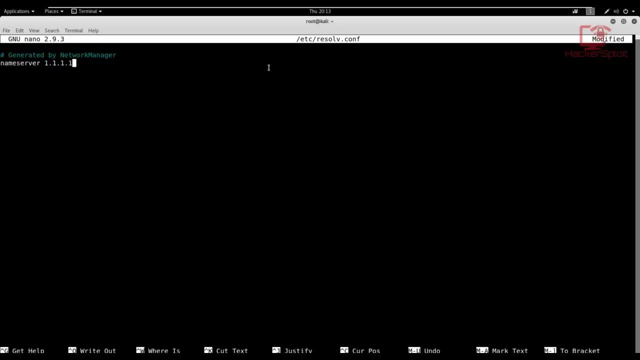 just use something that's secure. I'm begging you guys because I'm when. you know, when shit hits the fan And when your data is starting to be looked at and it's going to be sold, you're going to be in a lot of shit. So I'm just telling you that right now, as a friend I don't mean to be, you know. 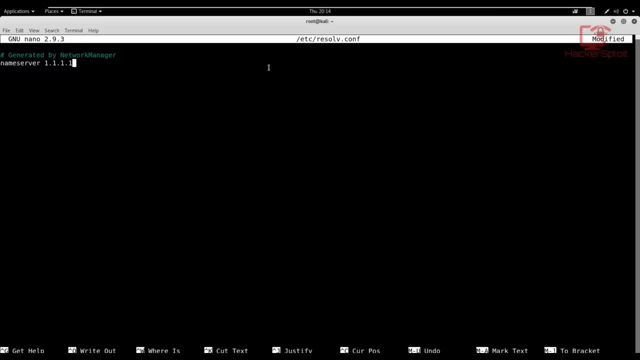 to be wild or extreme, But just listen, what I'm telling you guys, is the reason I've made this video. Alright, so to save it with nano, just hit Ctrl O and it's going to ask you whether you want to write to the file. 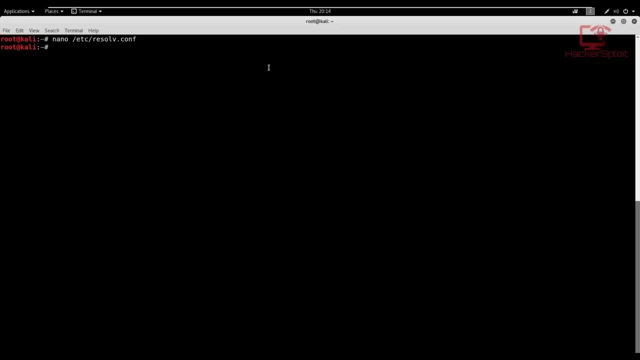 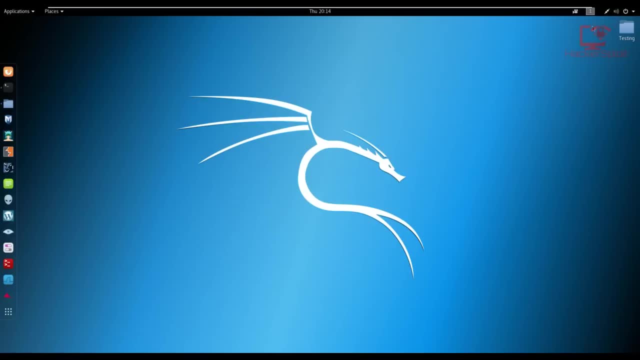 just hit Enter And now just hit Ctrl X to exit the nano editor. Once that's done, I'm going to open up my browser. Now again, I'm not using any VPN or proxy chains. I'm just showing you that this is. this is what's going to happen. If you're not using any VPN, my IP address will be leaked. 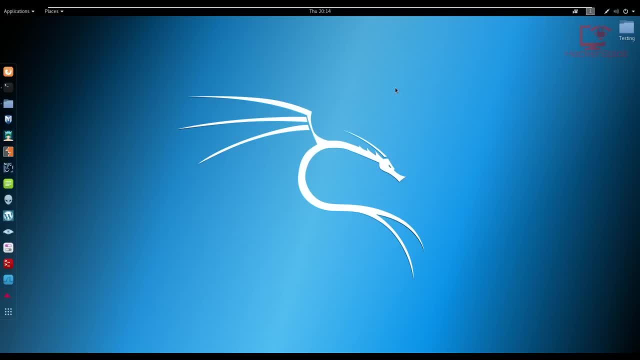 No problem about that. You can use VPN or proxy chains. By the way, if you're interested in a VPN service, check out the link in the description. you can check out the VPN links that I have in the description. they will give you a huge discount off your off of your order. It's really important. 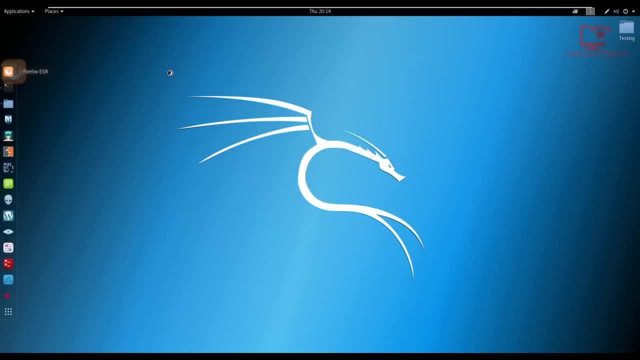 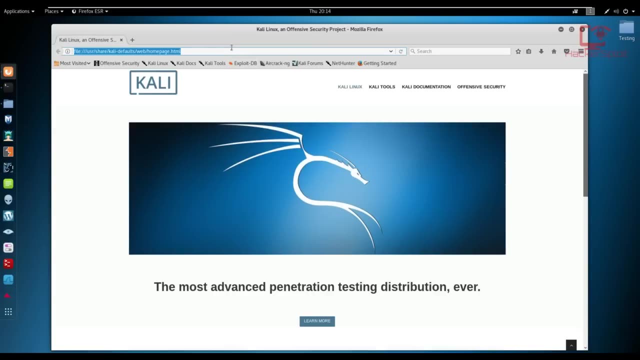 that you have a VPN, Alright. getting back to testing for any DNS leaks: of course we're gonna have a DNS leaks, but they're not going to be from ISP, Alright. so DNS leak testcom- I'm going to be hiding my real IP because I said as I said, I'm not using any pro, anything like. 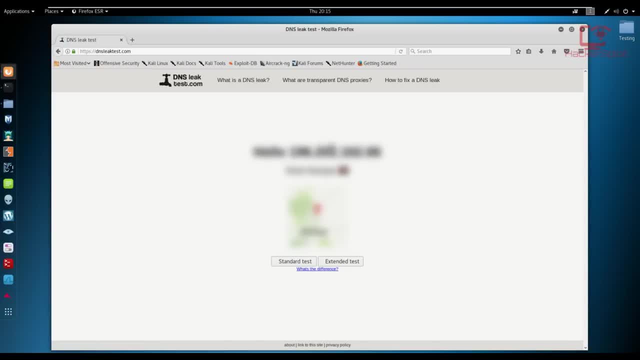 proxy chains or VPN. I'm just showing you that, indeed, your DNS will not be leaked, your DNS information, Alright. so I'm going to hit standard. this should be bled. I'm going to hit standard test And what will happen here is: it should tell you that you're using Cloudflare, Alright. 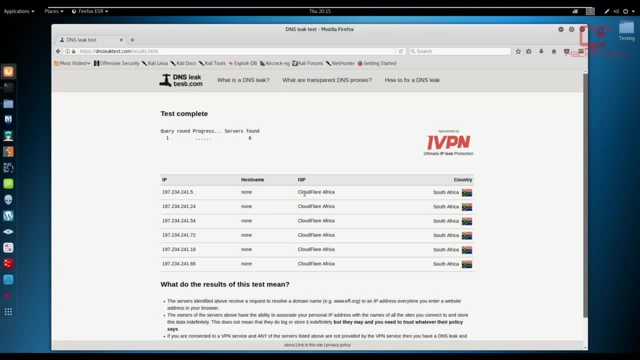 if it tells you using Cloudflare as your ISP, you're good. Now that means again, your ISP is going to show up as Cloudflare and Cloudflare is not releasing any of your browsing activity And you're pretty much going to be using Cloudflare as your ISP. So you're going to have to do a lot of. 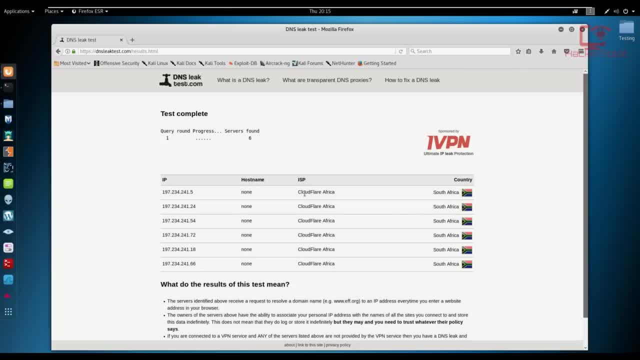 good there And you're going through Cloudflare. So again, if you're looking for an awesome domain name server, this is for you And it's as simple as that. That's how easy it is to change it And you're good. Now for those of you on Windows and you're not really interested on how to do it with: 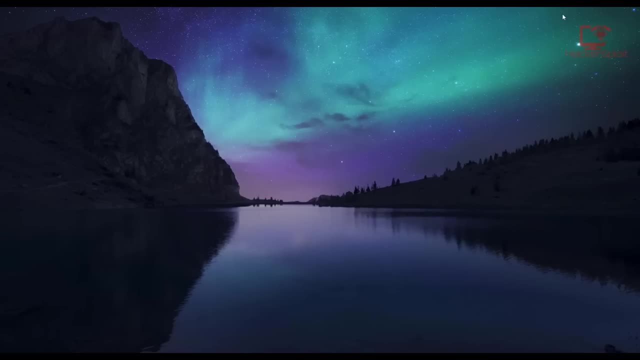 Linux. it's very, very simple. Let me just go back into my Windows operating system here. And you want to right click on your network manager and you want to go into the open network and internet settings, Or you can go into your control panel. for us hardcore Windows users, network and internet. 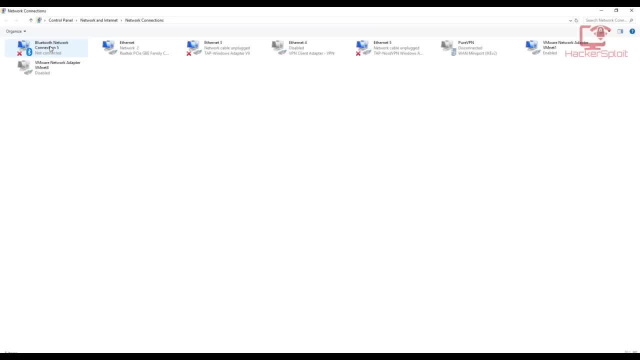 network and sharing center. you're gonna go to change adapter settings. you're gonna right click on the adapter using, whether it's Wi Fi or Ethernet. I'm using Ethernet, So I'm going to right click and hit properties And it's going to open up my Ethernet properties. Now you want to go. 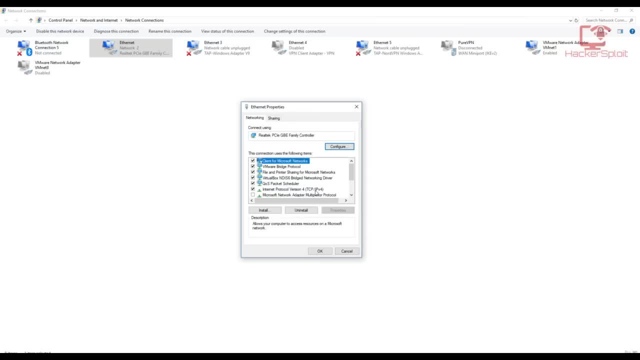 into your internet protocol version for your TCP IP v4 version. If you're using IPv6,, make sure you change that as well, But I doubt that you're using it. click on properties And you'll go. you see, right now it's saying: obtain DNS server or address automatically. Again, I reverted it. 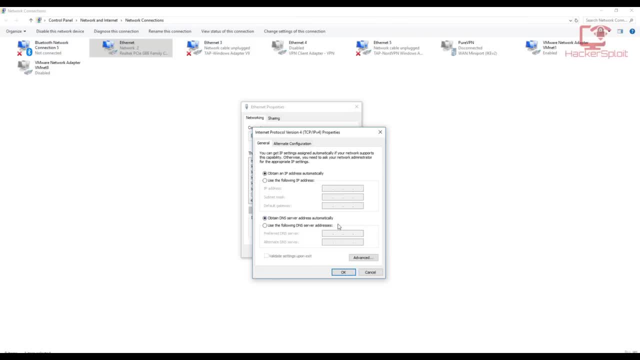 to show you that, in this case, is going to use your ISP domain name server, which again DNS leaks. So yeah, so you want to hit: use the following DNS server addresses. So just hit 1.1, sorry, 1.1, point 1.1.. And you can enter an alternate DNS server if this one doesn't work. 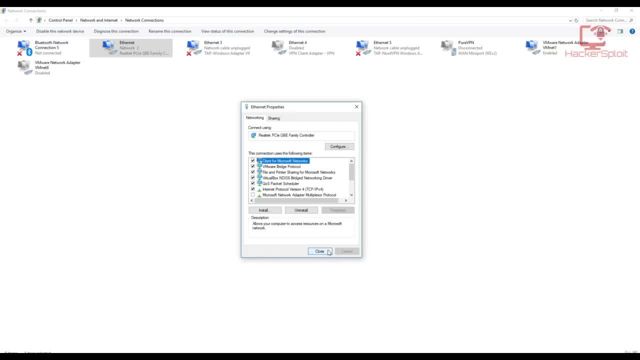 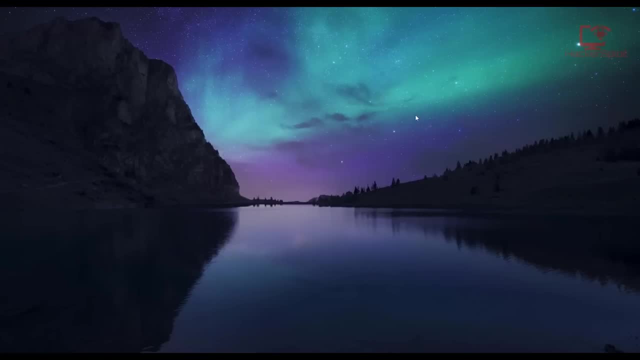 And you can just hit validate settings upon exit and just hit OK and close and you should be done. And that is how to successfully change your DNS server. Sorry, I don't know why. that was launching the Windows diagnostics And, as you saw, I was able. 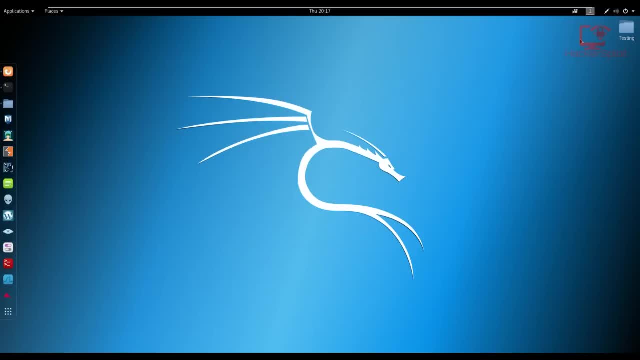 to successfully change my domain name server. So, yeah, that is what a DNS is, what DNS is, why it's important and how to change it, And we've looked at one of the best options right now, which is Cloudflare. Alright, so this is a very important video that I just thought I'd push out so you can. 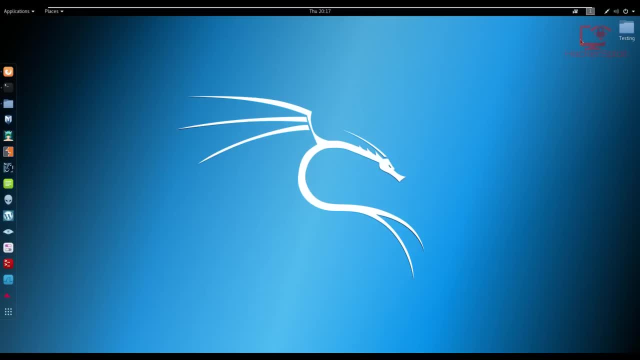 consider it as the complete guide to DNS. Now, again, I really encourage you guys to share this with friends or family or people, Or people you'd think will benefit from this. This is you really, really huge guys, because they're going to be a lot of changes in the future regarding internet and privacy. So, again, 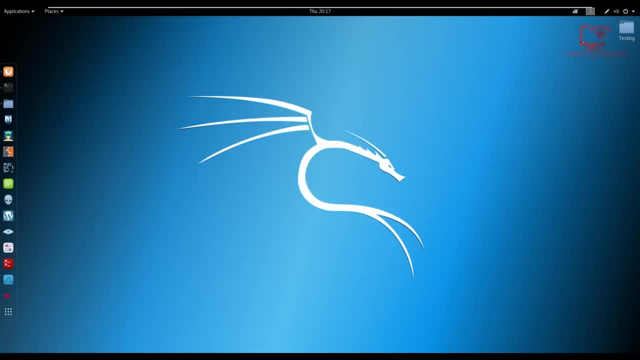 you've seen with the Facebook data breach, that your data is not being taken seriously at all. So, again, I'm really really making this video just, you know, to keep you guys safe, And again, as I said, I'm your friend. That's all I want for you guys. I just want the best. 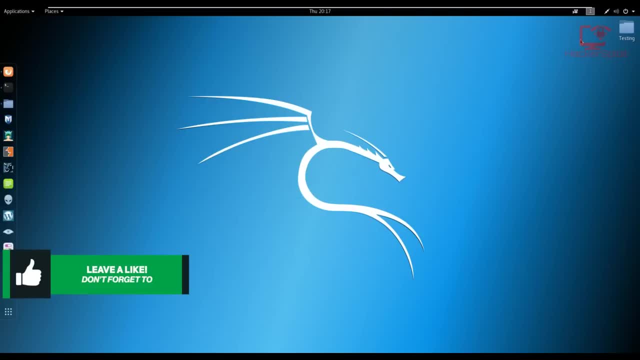 for you and your families and for your friends, you know just the best. So again, thank you so much for watching this video. If you enjoyed it or found value in it, please leave a like down below. If you have any questions or suggestions, let me know in the comment section on my social. 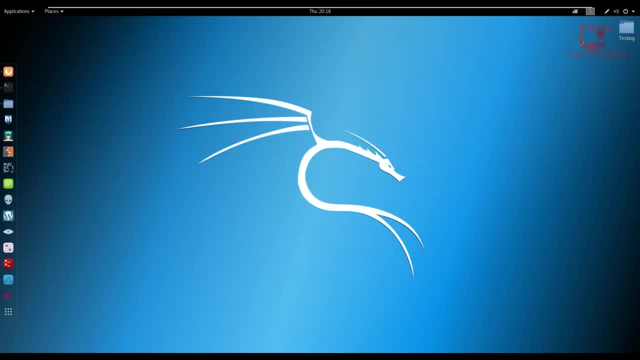 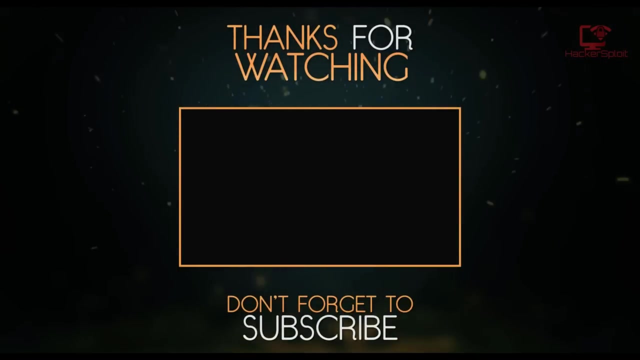 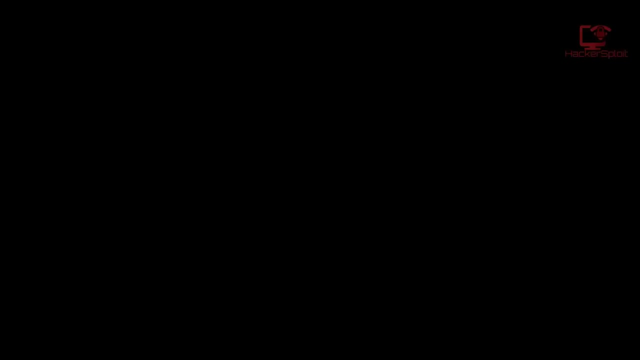 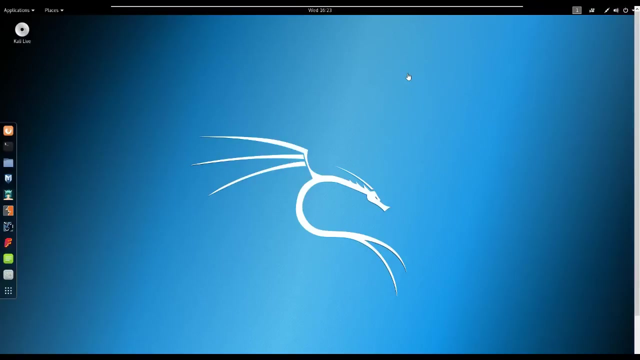 networks or you can post your questions on my website. The link will be in the description. Thank you so much for watching and I'll be seeing you in the next video. Peace, Hey guys. hackersploit here back again with another video and I humbly apologize. 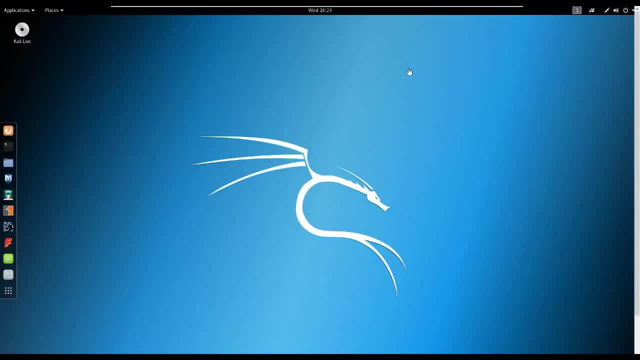 for the lack of videos over the last one or two weeks, The reason being, as I've said previously in other videos, I'm planning to do this as a full time job or my occupation, or content creation on hacking Linux programs, And I've just been sorting out a few other things and I've managed to sort them out. 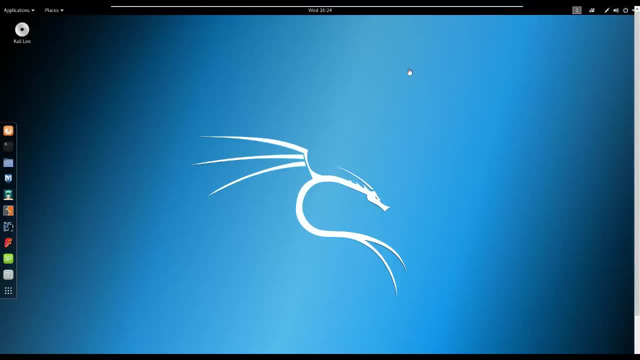 So this is because of you who love sending suggestions. I really, really appreciate them. just send any video ideas you have And I'll make them. you know, just send them in and I'll make them in accordance to how you've sent them, in the order that you've sent them. 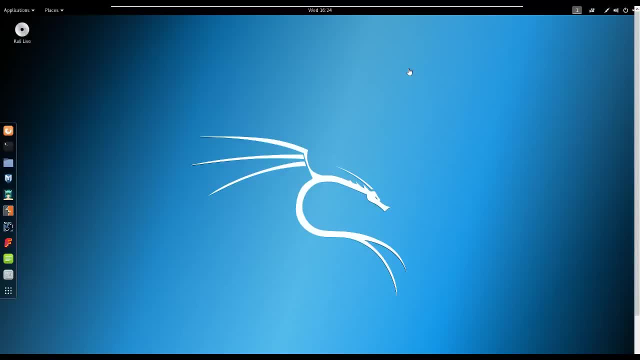 Anyway, enough of the chit chat in this video I'm going to be. in this set of videos I'm going to be taking you through the Linux terminal and how to use it and how to navigate around the Linux system with the terminal- The reason I'm making this series of videos. 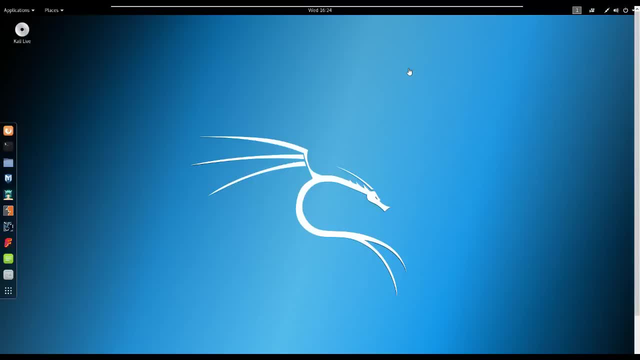 is because a lot of you guys are beginners to Linux and also to the Linux distro world And you know the Linux terminal is very, very important when you're using Linux, because essentially the GUI that comes with Linux is pretty much it's. it's not the best you know. 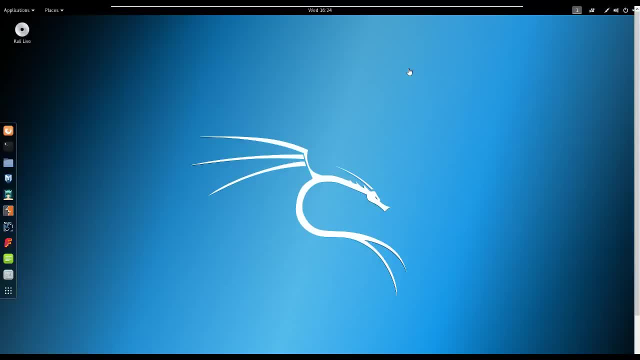 it's not something you can rely on, Especially when you're trying to connect to remote servers. you usually do it through SSH or secure shell, And so you're going to be using a terminal that can be used by those of you who like using it by its real name, not its abbreviation, and you're going to be faced with the terminal. 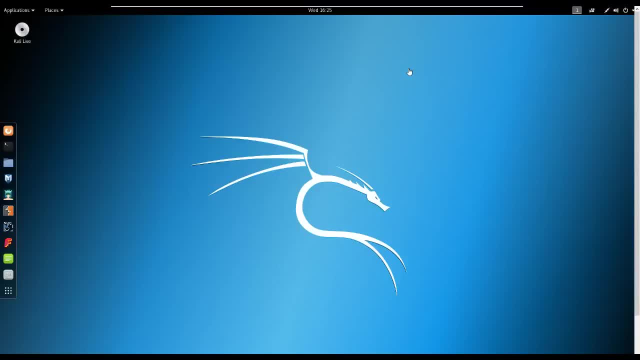 And if it intimidates you, you know it can really be something not to muck around with, because you can be intimidated of the terminal and then make mistakes. For example, you know you connecting to a server and then you know not knowing your way around and then making a mistake. 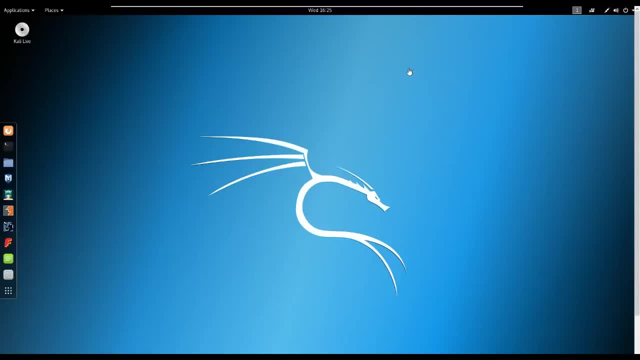 deleting files that probably have very, very high integrity. scary, and you should be getting used to the terminal. it's not a intimidating at all once you get used to it, so let's just begin. in this video, I'm just gonna show you how to customize the terminal to your liking, because that's one of the 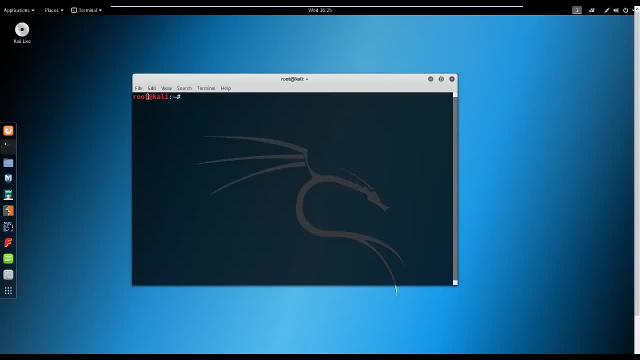 ways of making it less dreadful, so just open up the terminal. I'm using Kali Linux, so let's just begin. it's gonna be pretty much similar for any Linux distro that you're currently using. you can basically create a customized profile for yourself, if that's what you're looking for, or you can just edit the. 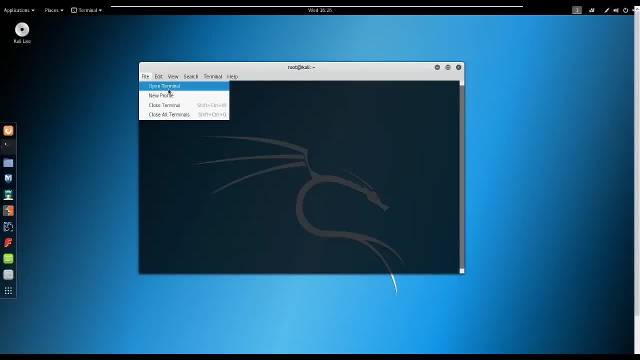 custom profile that comes with the terminal, or the default profile, which I'm gonna be showing you how to do. so. if you want to edit your profile and you want to change, for example, the font, the font color, the background of the terminal, the transparency, you get the idea. so how would we do that really go? 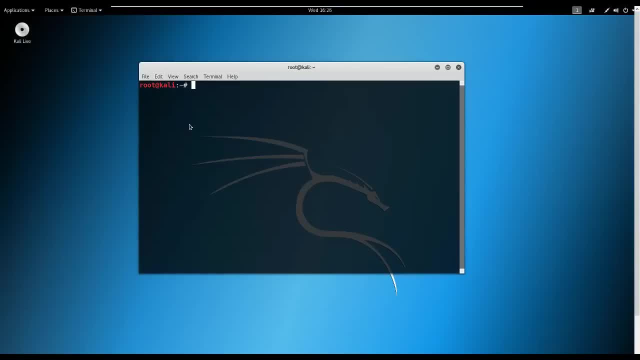 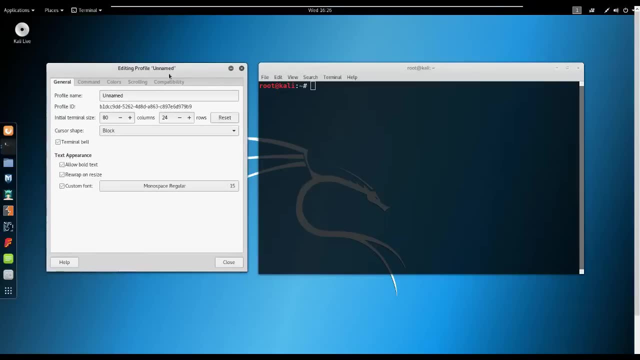 into edit and profile preferences. all right, so you want to click on that and it's gonna open this little menu. let me just bring them side to side so you can see the changes being made alive. in general, you can give the. you can give the profile a name, so let's call this: 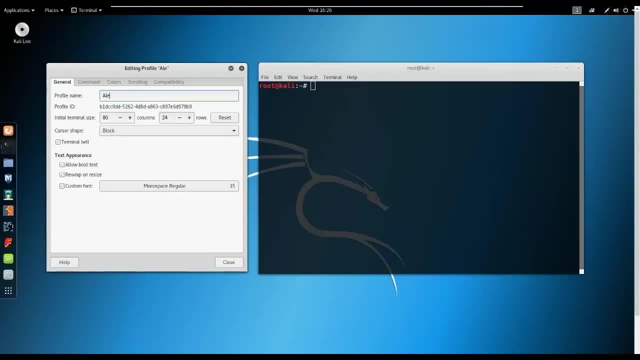 profile. you can just give it your name, so let's call it Alexis. I'm gonna give it my name. I'm gonna call it default. all right, now, that's gonna be the profile name. don't worry about the initial terminal size, or you call it the default size. that's gonna be the profile name. don't worry about the initial terminal size, or you could. 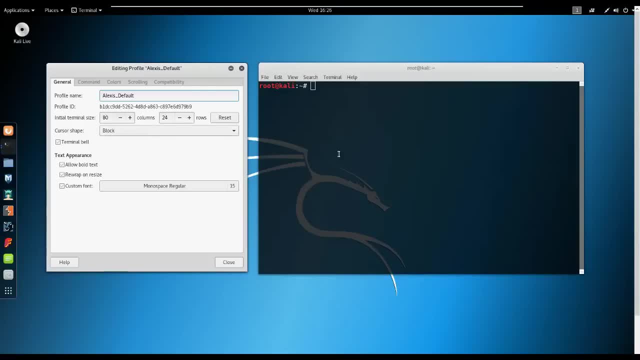 worry about that. if you you don't like the starting size of the terminal and you keep on adjusting its size, you can increase that maybe to whatever you want. I'm fine with 80. that's pretty much what I like. additionally, you could reset it if you make changes and you don't remember the 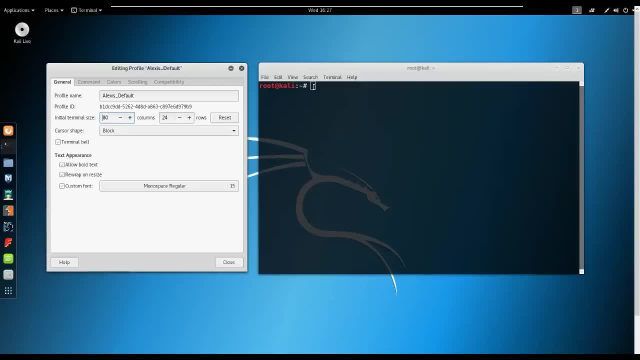 original values. when it comes to cursor shape, this is your little cursor right here. some people don't like the block cursor and usually prefer the I beam, which is very simple and minimalistic. oops, excuse me, I was actually typing over there, so, as you can see, that's some people like that, but for me, 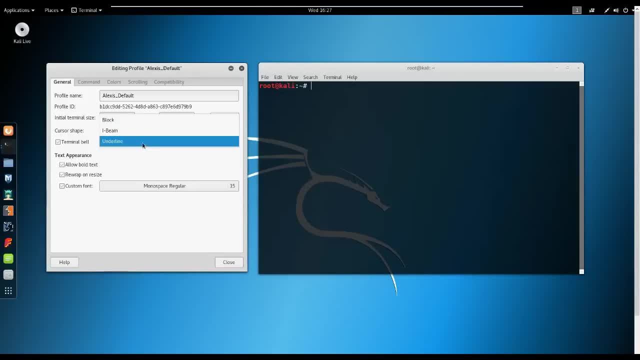 personally, I like the block. for those of you as well who like the underline, which is also quite nice. I like that a lot, but it's just not a universal for me. I like the block type. I've gotten used to that. in addition, you can increase your text. 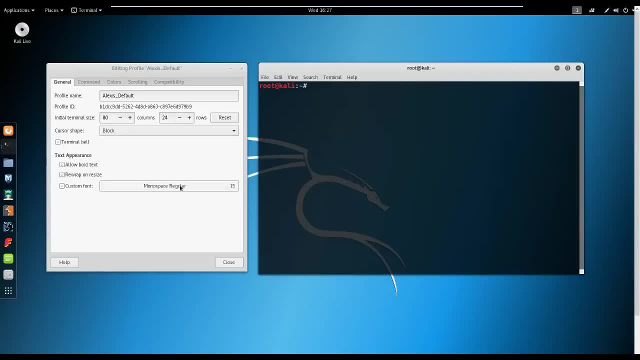 you can increase your text size. you can also change your your font. I like using the monospace font that comes with pretty much all Linux distros. you can also rewrap the content. you can also allow bold text if you want, which is very, very important. I highly encourage that you keep that. 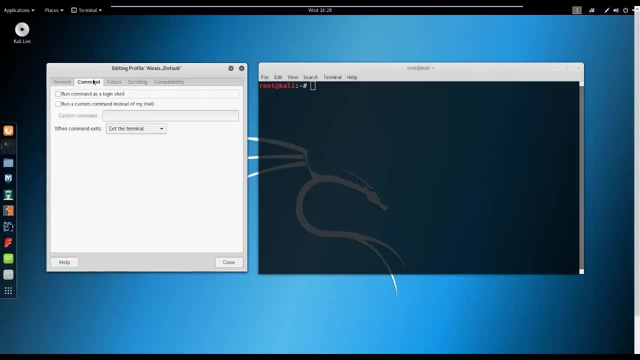 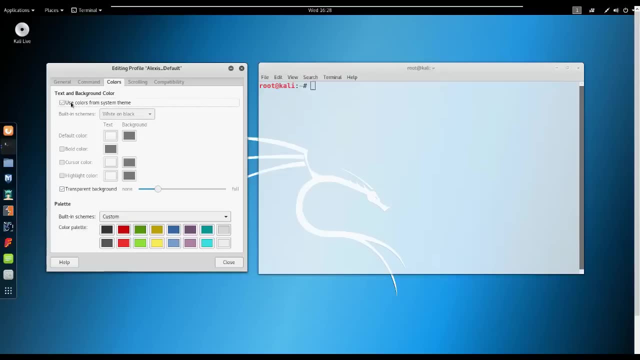 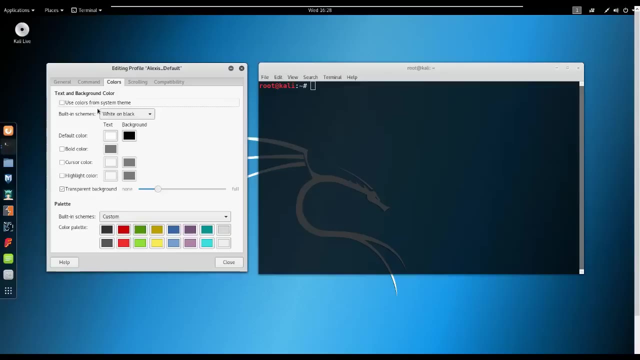 checked. when it comes to commands, don't really touch any of this, is just custom stuff. when it comes to colors, you can choose to use colors from your system scheme, which I'll show you in us in a few, in a second. when you look at the built-in schemes, white on black is text and then the 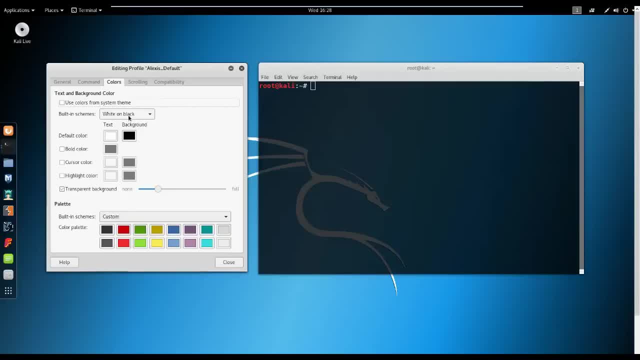 background color of the terminal, which so the text is white and the background color is going to be black, which you can edit over here. you can edit the text color. for example, some people like going with green and, as you can see, it gives you a nice little color up there. and if I just let me just try and run command: 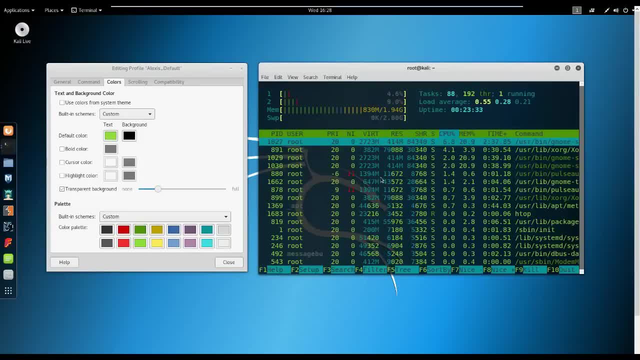 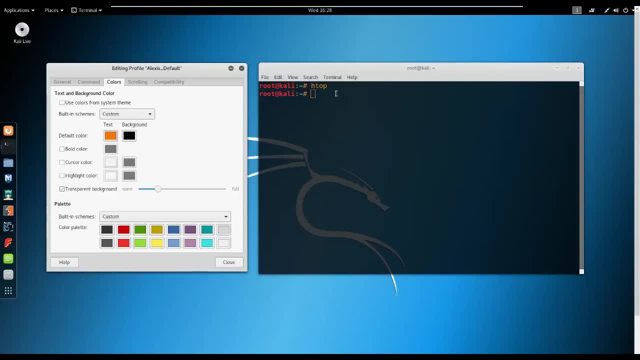 right there, all right. so let's look at that. as you can see, the text color is going to be green if I switch that to something like orange. I've also seen orange being quite popular right now- edge top. excuse me, let me just move back to the terminal. as you can see, it's going to highlight in: 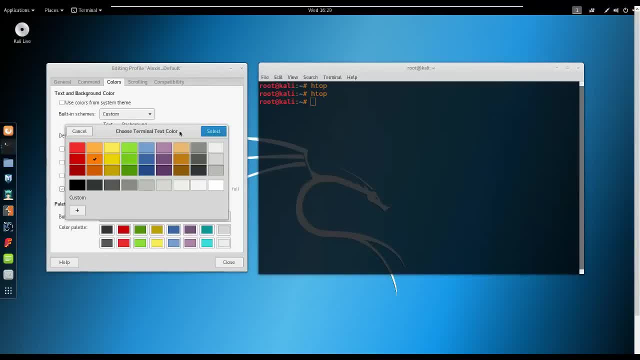 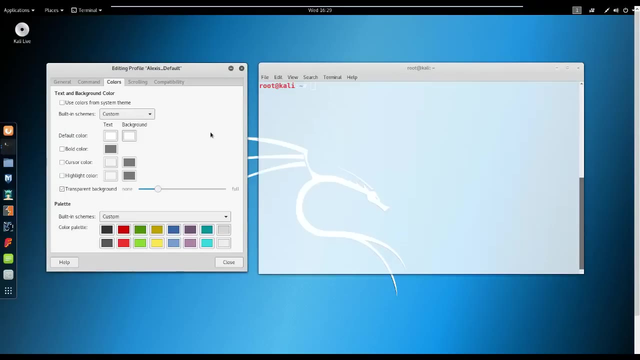 orange the main text. I like keeping it white and I like keeping the background black. another cool color scheme that I've seen is quite popular and is also quite neat as well is when you do the background white. when you use the white background and the text, you can probably have that as green or red, and 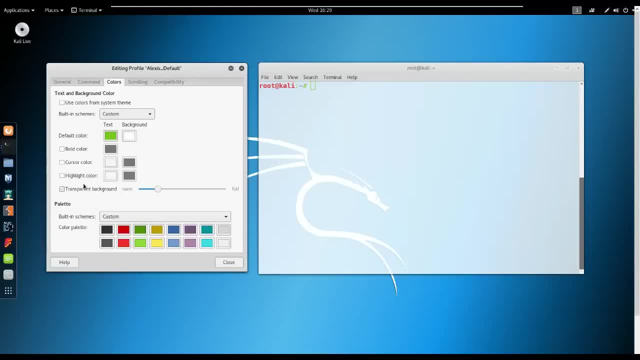 let me just show you what that looks like if I just disable transparency, or let me just keep that on and reduce it slightly. a lot of people really really like this type of terminal where the background is white and it looks quite cool. actually, I'm not gonna lie, let me use the edge top command, as you can see. 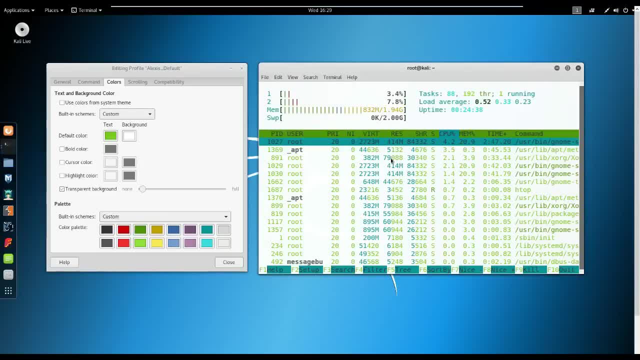 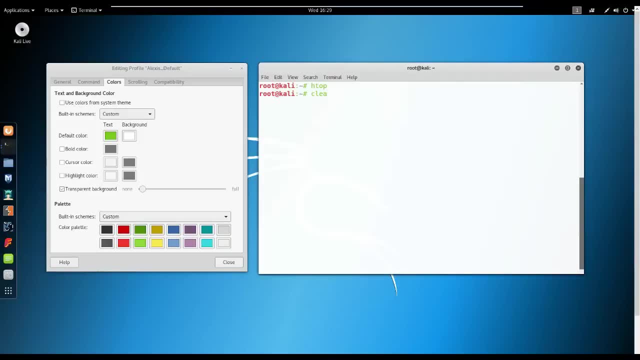 it has a very, very nice contrast with the other colors, but for me personally I think it's a very nice contrast with the other colors, but for me personally it's just too much. it's too bright and you know I wear glasses, so yeah, it's really taxing on my eyes, especially at night when I'm working. so 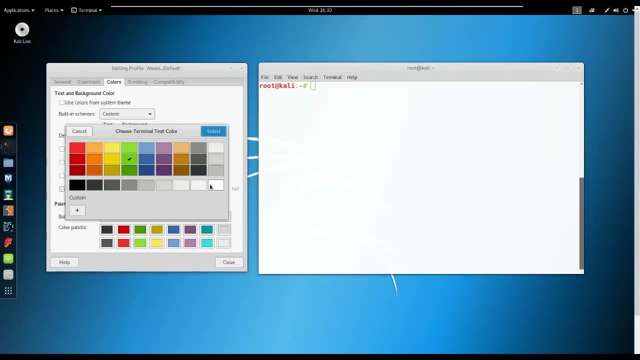 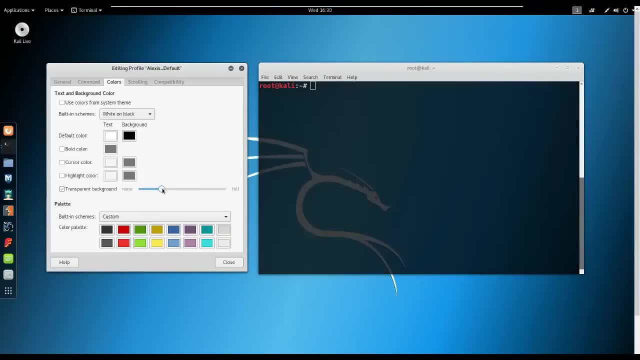 I'm just gonna change that to. I'm gonna change the text to white and the background color to black, with a bit of transparency. you can also edit the transparency if you want some, which is also pretty cool. I like that, and you can go ahead and make changes to the color scheme right here. this is all about you. 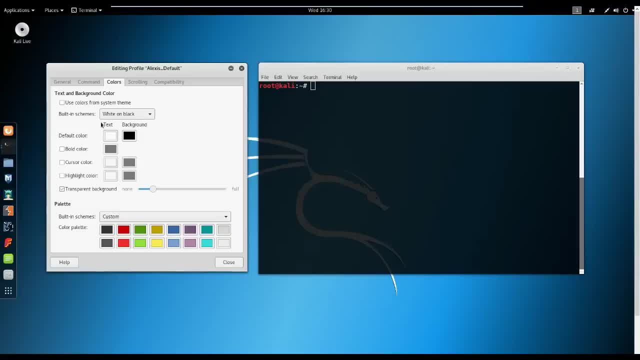 just customize it to what you feel comfortable with and immediately you'll see it will not be scary for you anymore. looking at scrolling: make sure you have scroll bar. that's very important when going through, like, for example, documents, or when you cat files. compatibility don't touch anything right here, yeah. 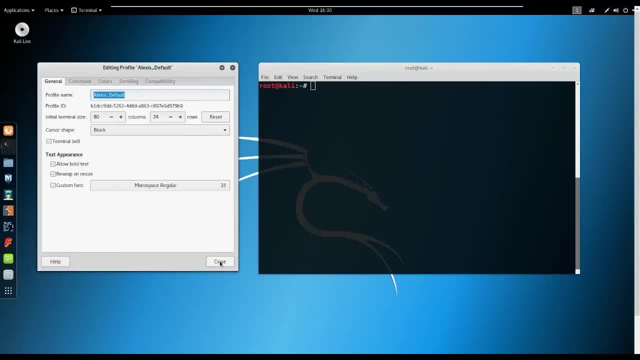 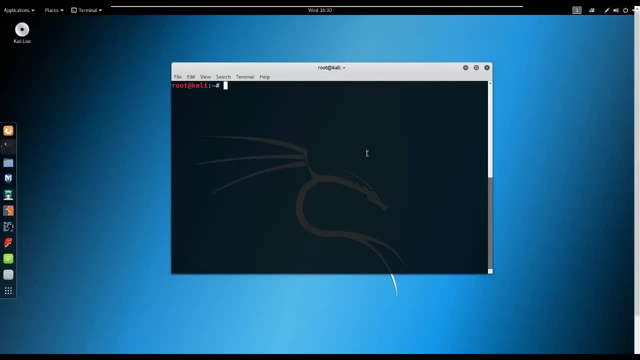 that's pretty much it. when it comes to customizing the terminal to your liking, I like keeping it the default way, primarily because I learned how to use it that way, but I also have a lot of experience with customizing the terminal. I've learned how to customize it, and you know when I'm running this on my main. 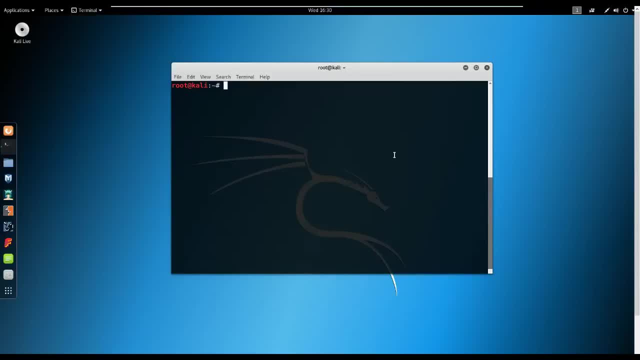 systems. I customize it, you know, just to make it look how I like it. I usually go for the white on black type of thing or white on green, not the that type of stuff. anyway, that's basically it for this first video. in the next video we're. 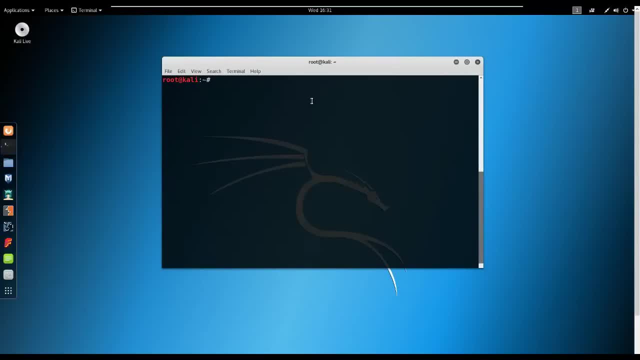 going to be going through some terminal commands that will hopefully make make you a pretty, pretty good pro in navigating a Linux with the terminal. so I hope you guys found value in this video. if you did, please leave a like. if you guys didn't like this video, let me know why in the comment section in. 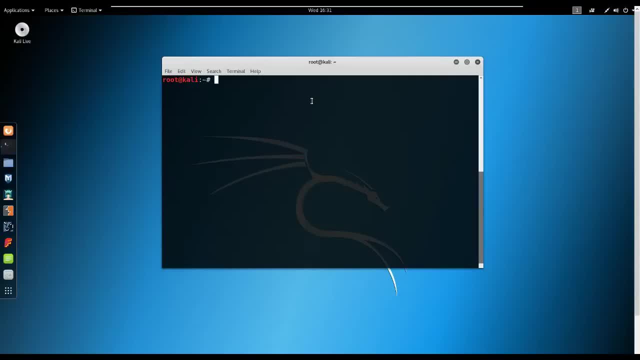 addition, if you have any questions or suggestions or any video suggestions, leave them in the comment section. if you want to contact me, you can hit me up on my social networks. on my kick, you can also check out my blog. I make a lot of posts over there. what else do I need to tell you? by the way, guys, I would really 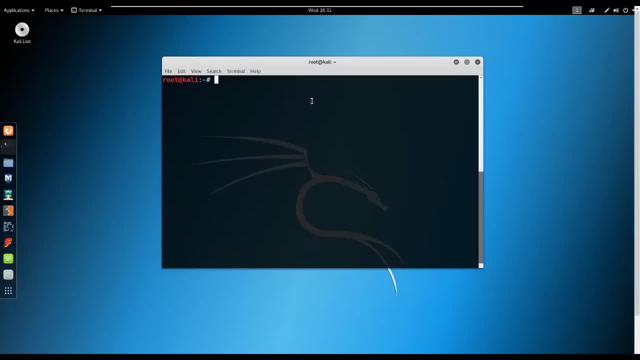 really recommend if you could share these videos with the people who need it. you know a lot of people need these videos but really can't find them, so that will do me and you guys a lot of a lot of good. that's basically it for these guys. I know this was kind of a kind of a random type of video, but you guys wanted. 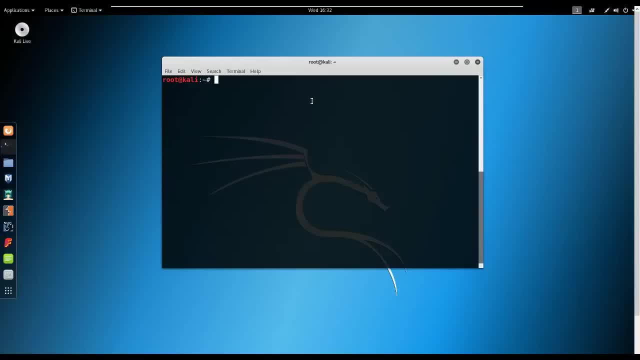 hacking videos and I'm making them and I hope that that are making them. well, let me know what you guys think. I really, really appreciate your feedback and I appreciate your support. I mean, this channel has grown so much over over the last couple of years and I'm so so gunned down over 3 years. I always get. 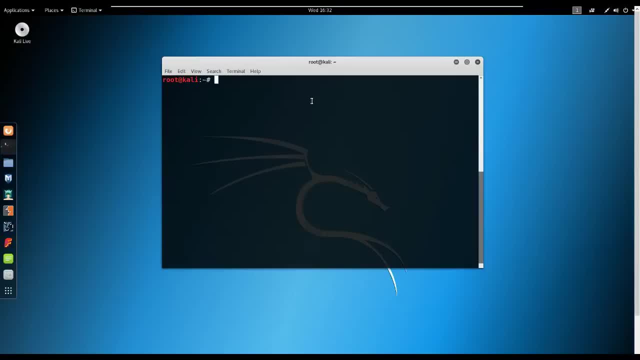 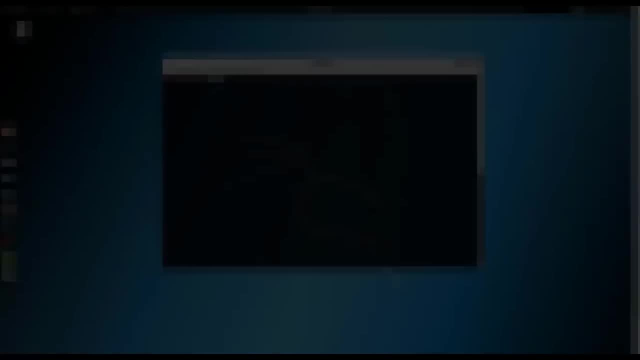 surprised every time I'm providing content. so it's been, I won't. it's incredible. so like also like you, take this chance to say thank you. thank you so much for the support, guys. it's unbelievable and I am committed to providing you guys with content now on a daily basis. thank you so much, guys, and 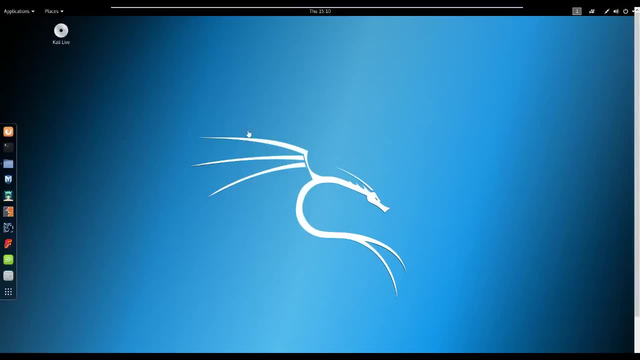 have a fantastic day. hey guys, Hackers Bloyed here back again with another video and we're gonna be picking off where we left off- from going to be looking at some linux commands- and hopefully they'll make you a much better linux user. there are quite some good commands that i found that are quite useful and what i found to. 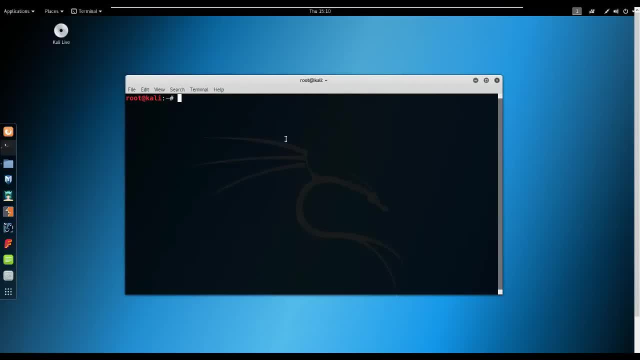 be the best that you should be knowing. so open up your terminal and let's get started. so in the previous video, we talked about how to customize the terminal to your liking in terms of visuality and aesthetics, but now we're going to get started with the nitty gritty. so the first thing, i think 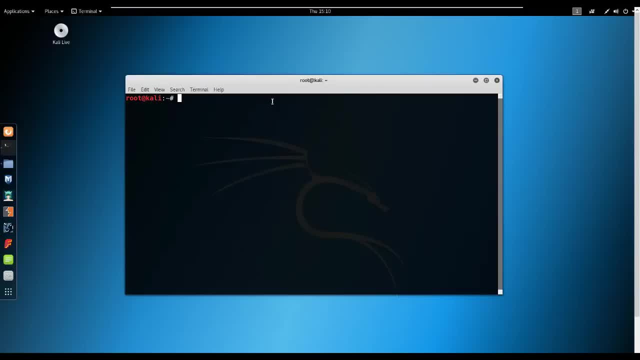 that you should know is how to enter root mode or the root or administrator. it's basically like having an administrator privileges if you're used to windows, so by default i'm actually in the root user right now. i've not actually created a profile, as you can see, i have not created a personal. 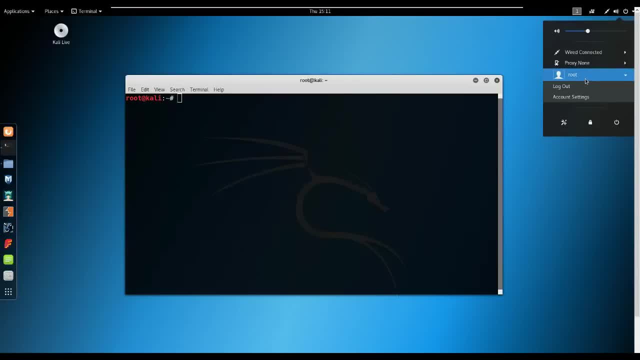 profile with my name or anything like that, like that. if you did, however it would, if you opened a terminal, you would not be in the root directory. so in order for you to do that, there are two ways. you can go about it: by using the su, which is sue or super user. if you hit enter, it's going. 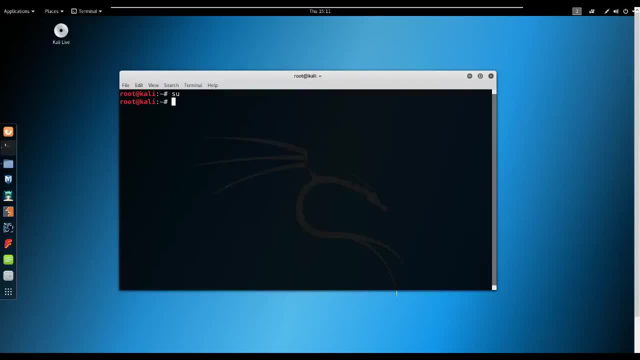 to take you into root. if you have a root password, it's going to ask you for your root password and once you enter that, it's going to take you into root mode. the other way of doing it is sudo bash- all right, and if you hit that again it's going to ask you for a password if you had a root password. 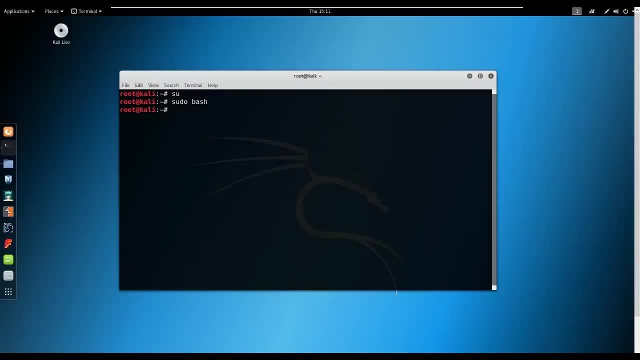 with, which i recommend you do, and then it's going to take you into root. now one more command. if you have a root password and you want to start- uh, you want to start over- just use the clear command. pretty simple, right, and that clears everything for you all. right now let's get started. so i'm 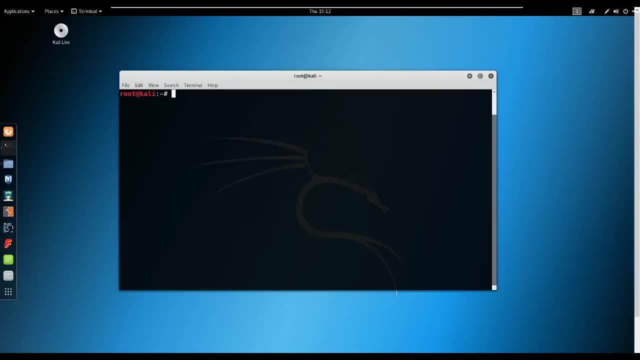 currently in the root directory. but what if i didn't know that, like for many of you, for example, if you're going to be connecting to a linux server, the only thing that you're going to have at your disposal is the terminal, and it's very essential that you know how to. 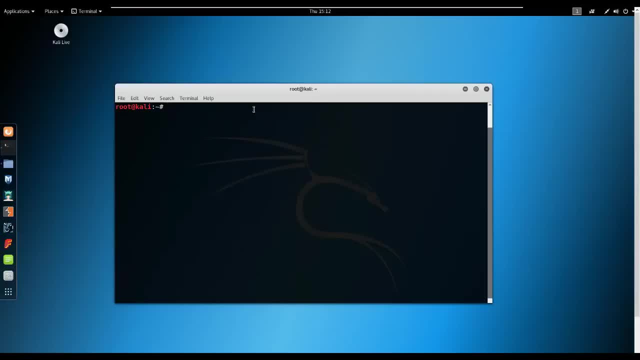 navigate the, uh, the file system, the, the linux file systems, and know how to check where you are exactly. so how would we do that? so right now, let's say i wanted to check what my current working directory was, and how would they do that? we use the pwd, which means print working directory. 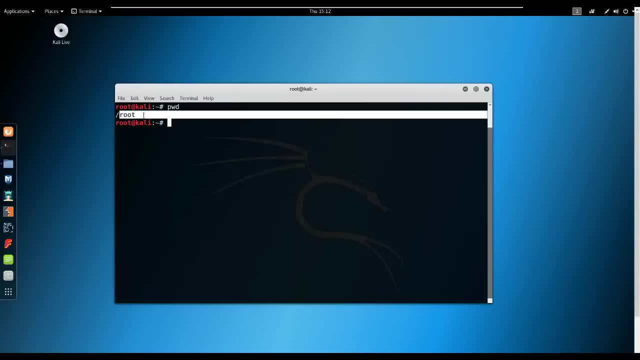 pretty simple, and if i hit enter, it's going to tell me i'm in root. all right, so at least i know i'm in root now. now, let's say i want to change. let's say, instead of root, i want to move on to my desktop. right, so what would i do? hmm, let's see if i list all files in root. all right, before we. 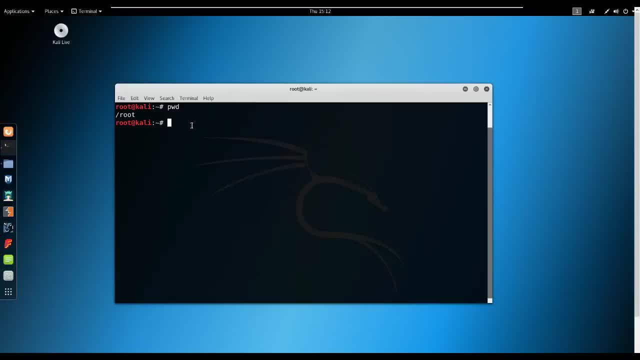 move further. let's say i wanted to move um into my desktop. how would i do that? so the command for that is cd, which literally translates to change directory. all right, pretty simple linux. the terminal commands are really very simple and, as i said, it gets really intuitive, user intuitive. 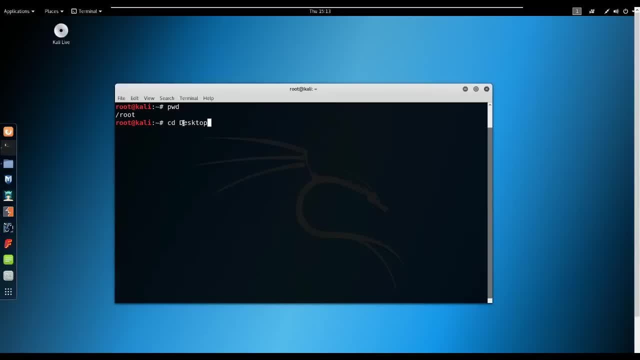 and desktop. this is case sensitive, of course. the desktop is a very um. i like to say that linux takes their their file structure very seriously. so cd desktop and it's going to take me to my desktop, so i'm currently now working on the desktop. what if i wanted to see the files listed on my desktop? 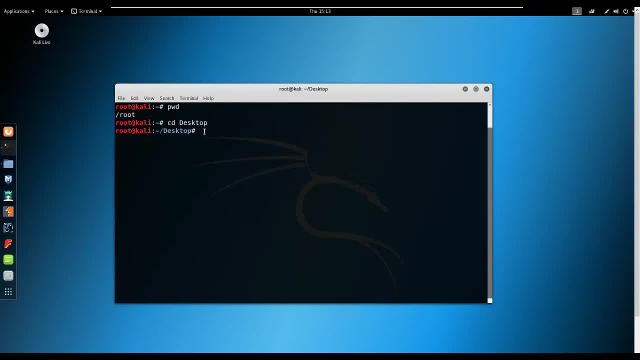 right now. i currently have no files or folders, so we really won't get anything out of that. all right, so let's say we want to create a folder or a directory on the desktop. how do we go about doing that? well, we would. we would use the mkdir, which translates to make directory. 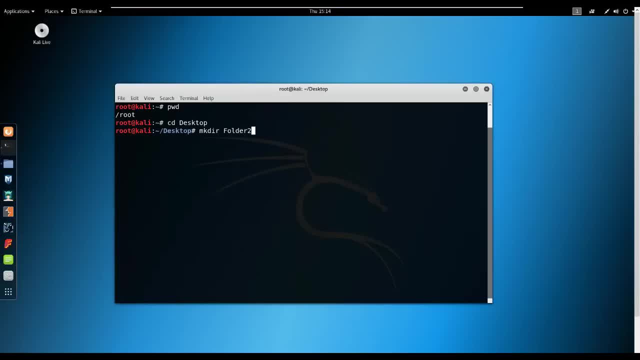 and we give the directory a name, so let's call it folder two or folder one- and, as you can see, it's going to create a folder on your desktop called folder one. what if i wanted to get rid of this folder? what would i do? well, for that, i would use the rm dir and i would give the folder. 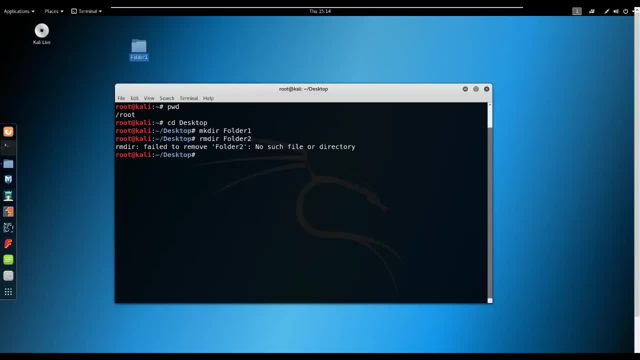 one to remove folder two. all right, but remember, oops, excuse me. uh, it's actually folder one, rmdir, folder one. but, as i said, remember. let me just clear the terminal. we are creating all of these directories and let's say, we created a directory like a week ago and we don't remember what. 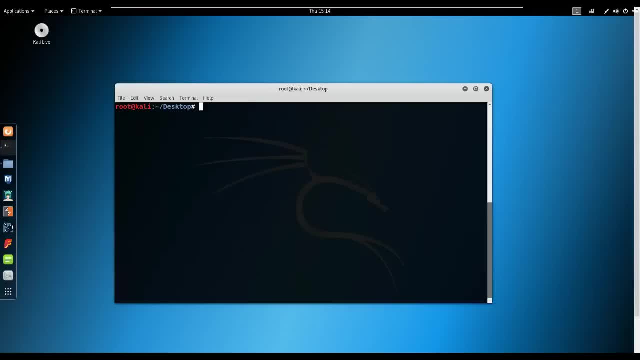 directories exist on the desktop. how do we display what directories exist? so let's say, i create another folder and i call it folder one. all right, let's create folder one and let's create another folder called folder three, um folders uh, 60, 55, for example. so we have this bunch of folders on the desktop. 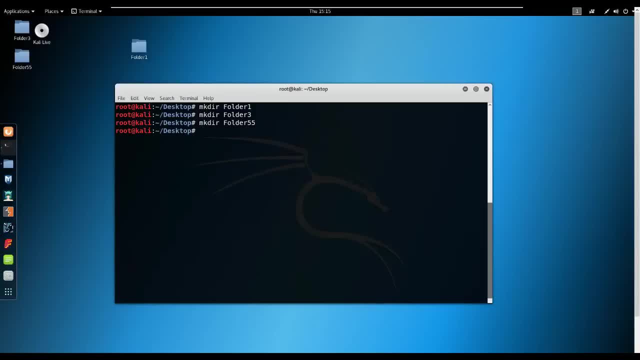 how would we list whatever we have on the desktop? because remember this, very, very, in most situations you're not going to get a graphical user interface to your adv, you know, at your advantage, or at your finger, at your fingertips. so the command we use is the ls command. 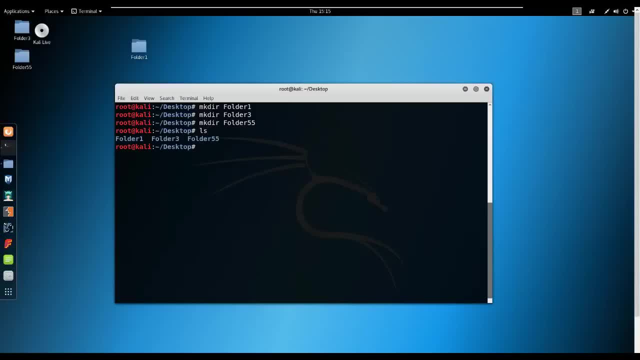 which translates to list: all right, so if we hit that, it's going to tell you it's going to display both folders and files you have on your desktop. uh, in addition, the ls command also has some parameters that can fine-tune your display results. so let's say we wanted some more. 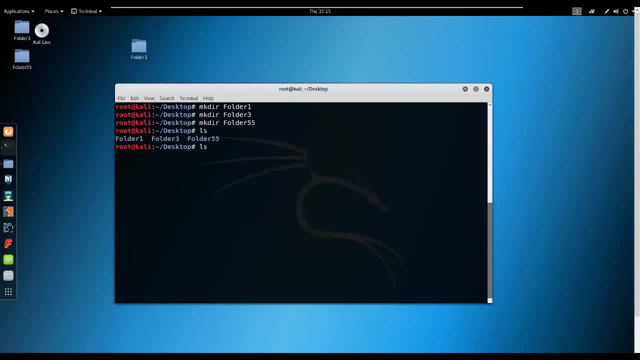 information about the folders, like we wanted to know the, what user created the folder, at what time it was created, information like that. so to add a parameter, we use the hyphen and l. all right, l is the the parameter, but to add a parameter, we use the hyphen, uh, the parameter we are going to. 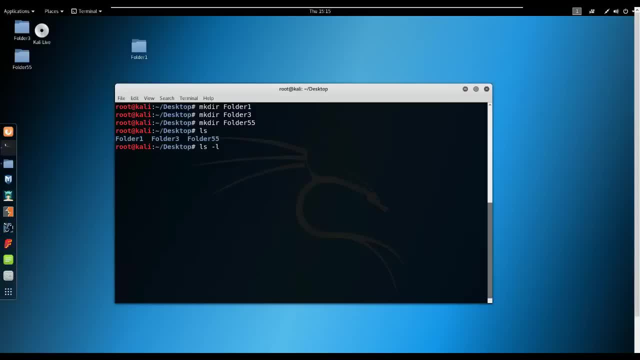 be using now is l, which is going to show additional information about the folders and files. so let's hit enter and, as you can see, it's going to tell you that we have. these are the permissions, all right. so whether uh users able to read, write or edit, modify or delete uh the files or folders. 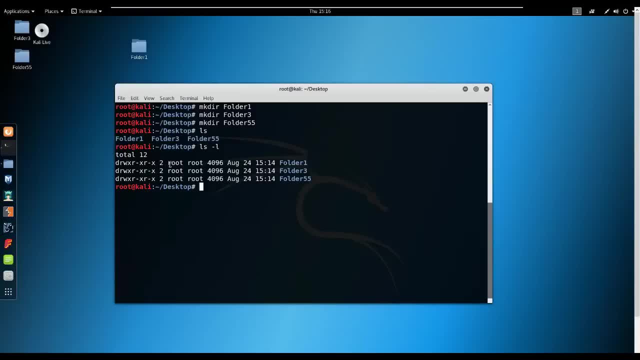 i'm pretty sure you guys are familiar with permission file permissions. you then have the person who created them. i'm pretty sure you guys are familiar with permission file permissions. you then have the person who created them. uh, in in this case, we know it's root. you have the time of creation and the name. 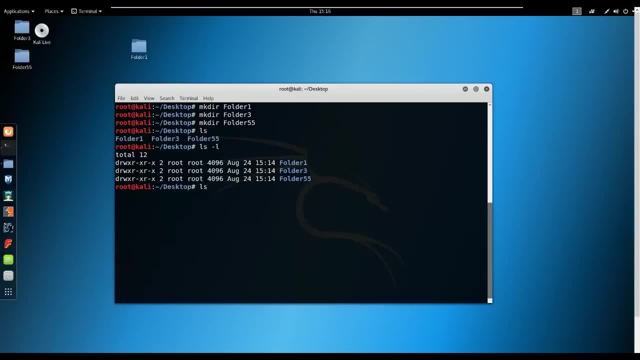 all right, so we also have another ls um, another ls command that will- uh will, allow us to fine-tune our results again, but this time this command is going to allow us to view all the files on the desktop, whether or not they're hidden, literally everything, that's. 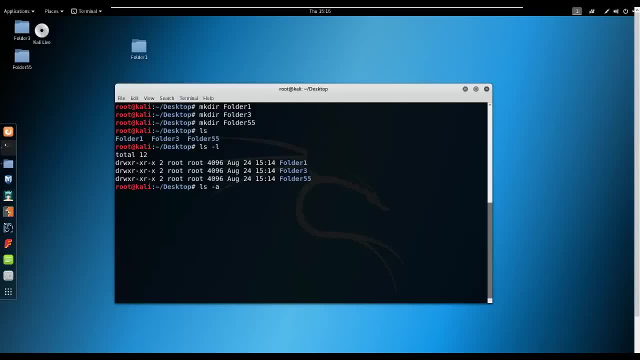 on the desktop and that is the lsa command. all right, the lsa command will display everything that you have on the desktop or in the directory that you're currently in. so i'm going to hit enter and, as you can see, it's going to display everything. we have nothing else really. so, yeah, yeah, it's. 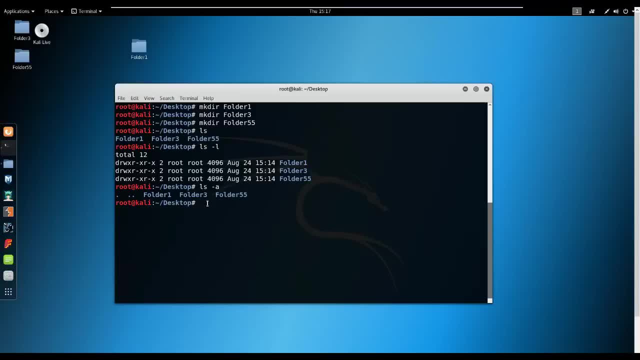 not going to display it, all right, so we've. we've actually talked about quite a lot now. now one really important thing that we have to look at. firstly, let me just get rid of some folders um, folder, folder three and folder 55. oh, excuse me, uh, folder 55 not found. all right, let me just 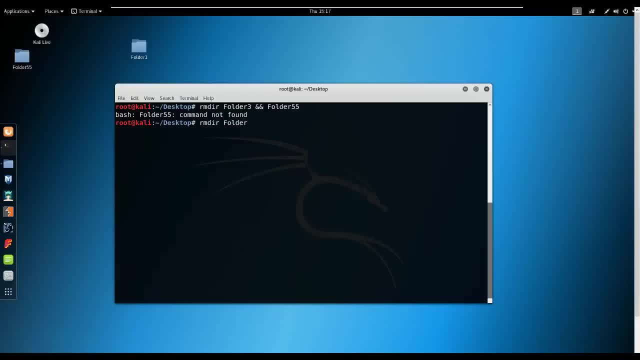 remove that manually. remove directory folder 55. there we are all right, we can clear that up. so we've talked about navigating with the change directory, but we have not talked about moving backwards, because we said we can use the cd to navigate into a directory and you know. so, so on and so. 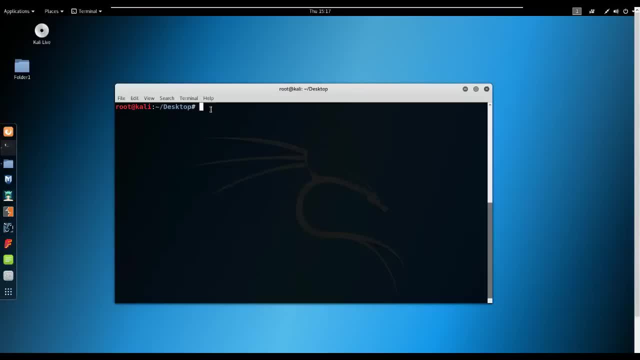 forth. but what if we wanted to go backwards? right now we are on the desktop. what if we wanted to go backwards? well, we use the cd, but we space user space and use two full stops. all right, that will take you backwards. and that takes me back to my root. as you can see, 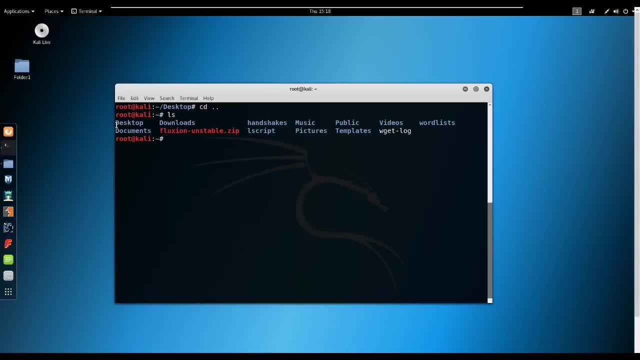 and if we list all files in root, as you can see, it's going to tell you the files that exist on um, on your, on your root, for in inside your root directory. so again, from here you can browse into any other directory that you want. but let's go back into cd desktop, into desktop, excuse me. 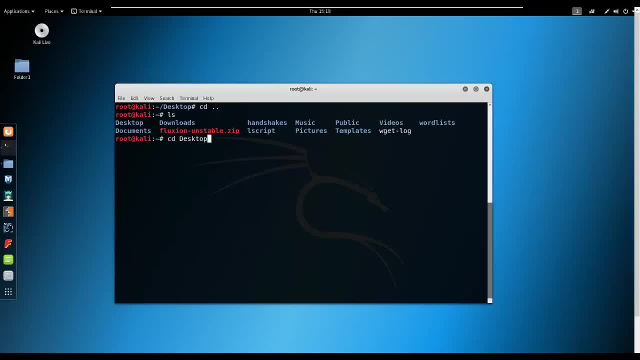 that was actually quite weird. cd desktop- that doesn't make any sense at all. so cd desktop, all right. so we've talked about going back. um, we've talked about changing directory listing files, uh, printing the working directory. what else do we need to do? we're going to go back to cd. 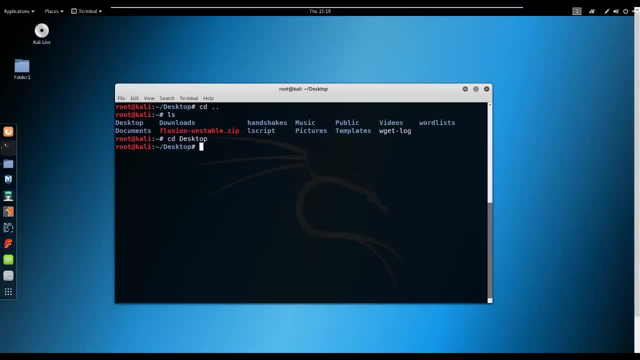 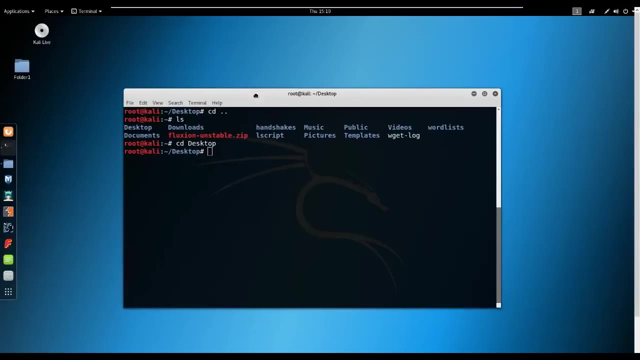 do we need to look at. we've talked about clear, all right. one more thing i want to talk about: uh, very, very important, um, as i said there, um, they're going to be some in terminal editors, text editors that you you're gonna you have to learn how to use them because, as i said, the 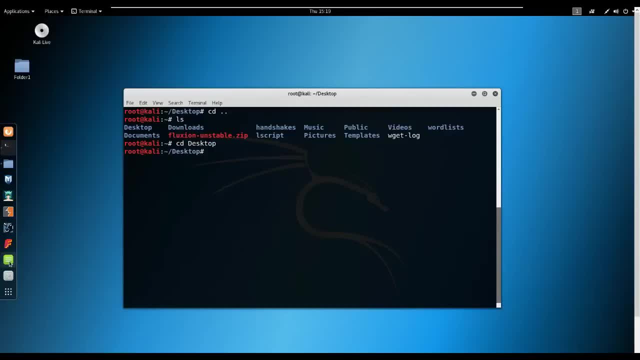 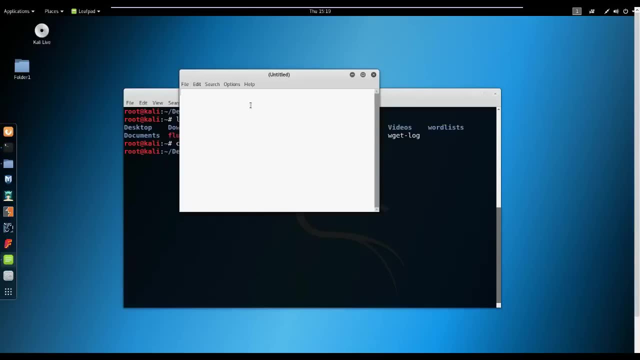 terminal is pretty much the only thing you're going to have at your disposal. so let me just create a, a small little document. i'm going to save it on the desktop, all right, or i can save it in folder one, so let's just. let's just type some random stuff, let's say: hello, this is, this is an encrypted. 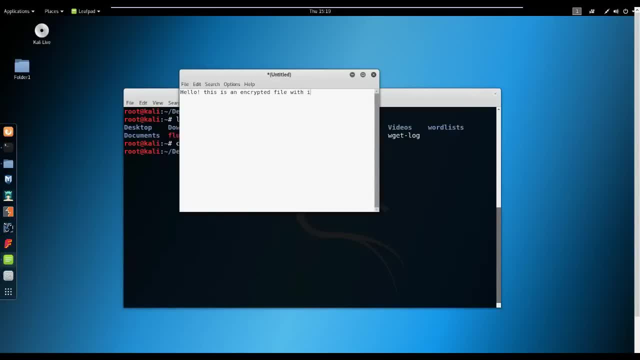 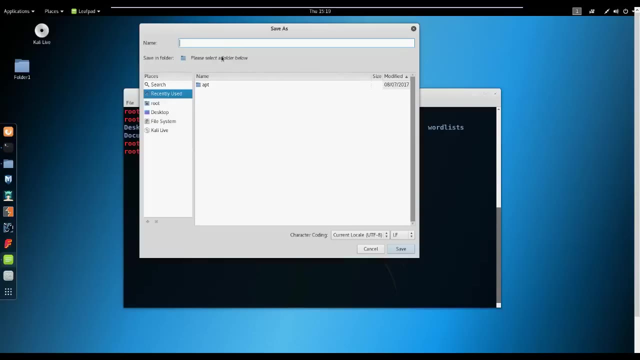 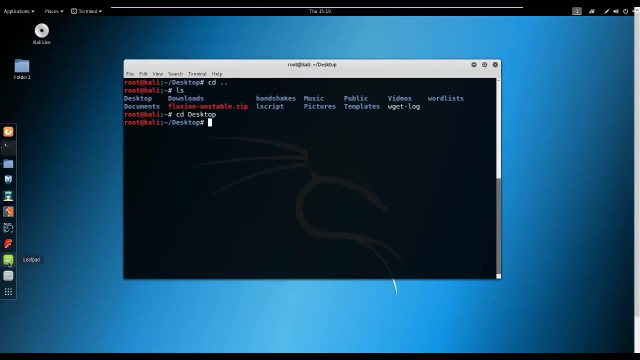 encrypted file file with info with what my typing is uh about, with information about uh, ufos, all right, so i'm gonna save this uh as a document on my desktop in folder one. i'm gonna call this um secrets, all right, just a stupid little name, and i'm gonna save it now. remember, as i said, a leaf pad, which is what i use to create the 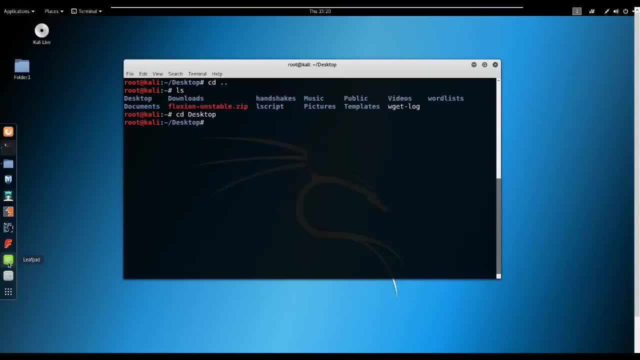 document is not going to work, um, you know if you're connecting to a remote server or through ssh, so it's very important to use, to know how to use the inbuilt um, the inbuilt text editors. all right, i'm not going to be covering that in this video, but i'm going to be covering that in this. 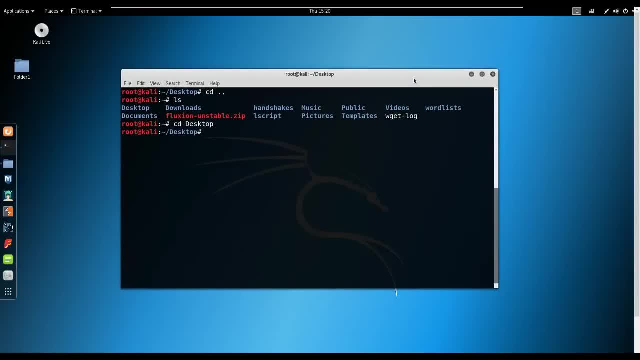 lecture. we'll look at the, the editors, like nano, in the next lecture, uh, in the next couple of lectures. and we have vim, which is very, very useful. but let's look at how we can just display the contents of a file, uh, just on the terminal, without any formatting or any stuff like that. so let's. 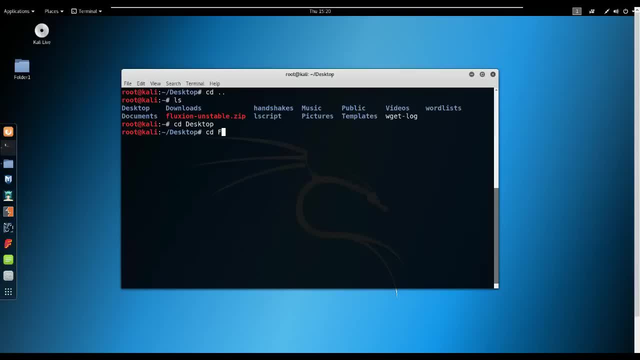 browse into the folder that we saved that, in which is folder one where we save the document. and if we clear the terminal now and let's have a look what's inside, so we have secret, all right, pretty cool. so the command we use to display everything or to display the contents? 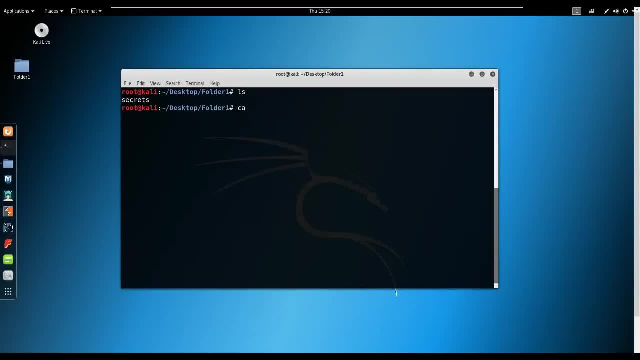 of the file, not really formatted in a way that is respective to the nature of the file. we use the cat command right the cat command and secrets. we use the tab button. it will auto complete it for us, so cat secrets, and, as you can see, it displays whatever you typed in that document. 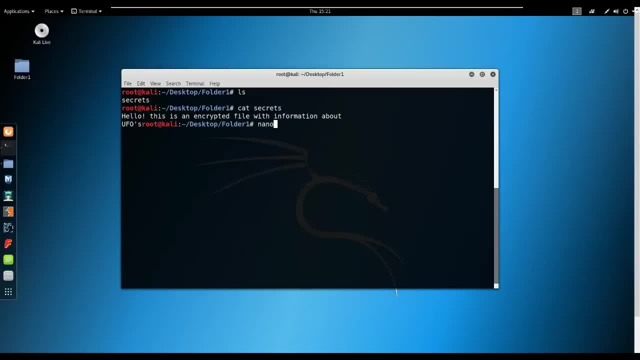 as i said, um, you have other editors, like nano, all right, which you can open up and you can type whatever you want. let's say: uh, this is also an in my typing today, encrypted, an encrypted document, all right, and to save it out, to print it, to basically output. 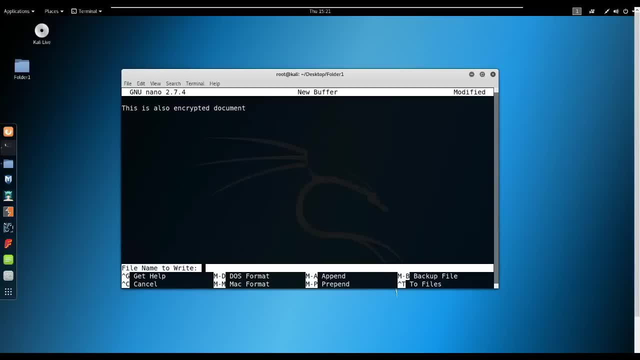 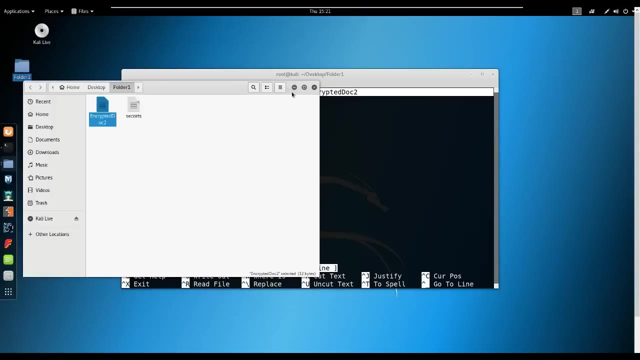 the file we use o and we uh, let's give it a name, let's call it encrypted doc 2, and i'm gonna hit enter and it's uh, i wonder where it saved it. actually, that's quite interesting. oh yes, it did save it in folder 2.. as you can see, encrypted doc 2.. uh, now, if you want to exit, nano. 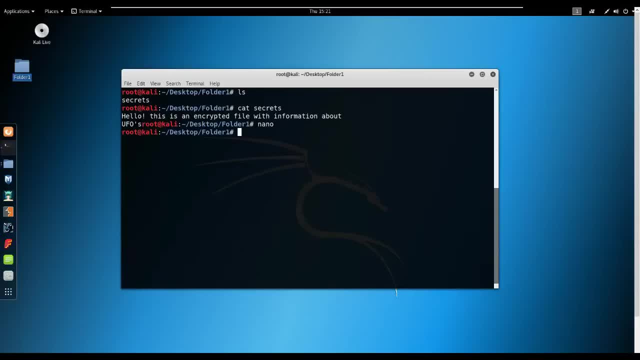 don't worry about whatever i'm doing in nano right now. this will get to using nano in a few other lectures. so let's clear that. and if we list all the files in the folder one right now, you can see that we have the encrypted doc 2 which i created with nano and the secrets which i created with. 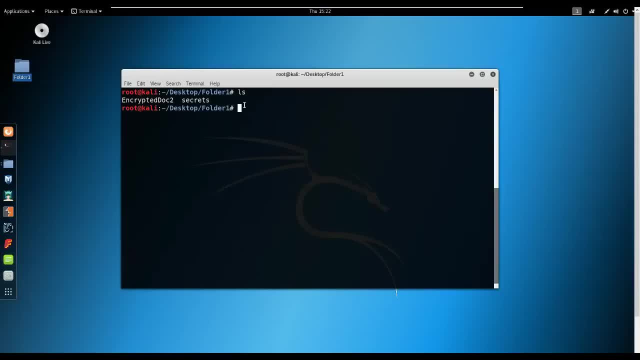 leaf pad, which is a GUI text editor. So if I wanted to display a document with nano, what would I do? I use nano, which is a text editor, and I use the secrets. let's say we wanted to use secrets And, as you can see, it's going to display it out pretty well as well. So it works quite well. So. 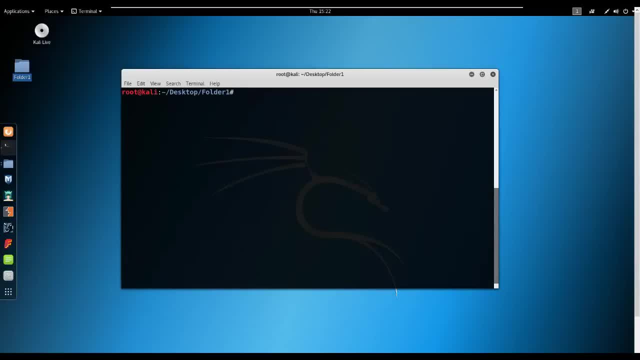 I'm going to exit that And let's see what else we need to look into. I know the video is getting quite long now Let me just move back to my desktop. So what do we need to look into right now? Here we are. So one of the most important resources that you'll have ever in Linux is the. 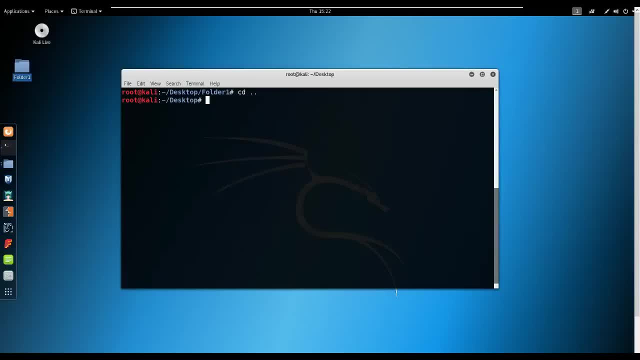 manual. Linux does come with a manual, believe it or not. for those of you who are quite skeptical about the documentation surrounding Linux, Linux comes with a full on manual. they might be asking: well, how do I access this manual? The great thing is, you can access it. 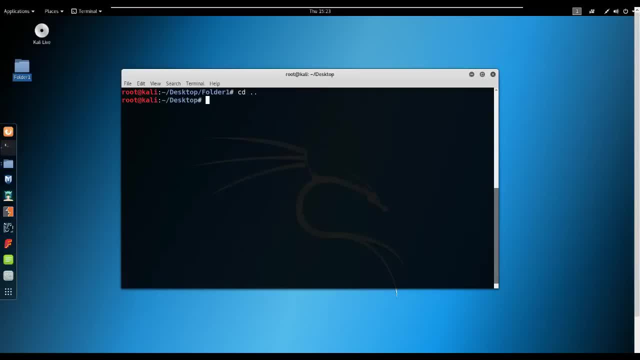 you can access it with in your terminal. So let's say you wanted some, you wanted to know about the copy or the change directory command, Alright. so, man, and let's say you use the copy command- Oops, excuse me, man- and CP. Alright, let me just start that over. Man means manual right, So you're. 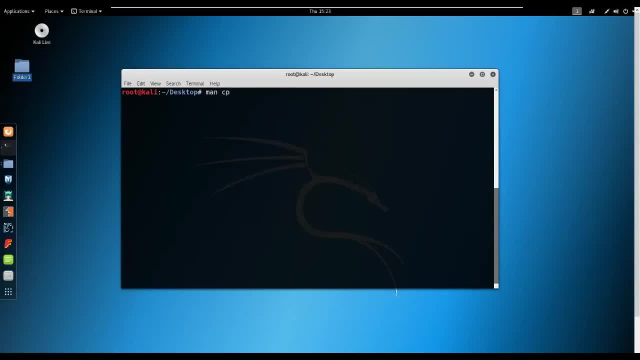 telling the terminal open. the manual and the command I want you to look into is CP. As you can see, it's the same as the, the copy command. So it's going to give you the full information about the copy command. And it's going to give you the full information about the copy command. 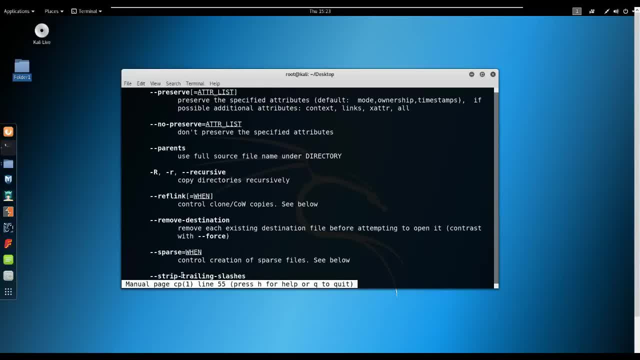 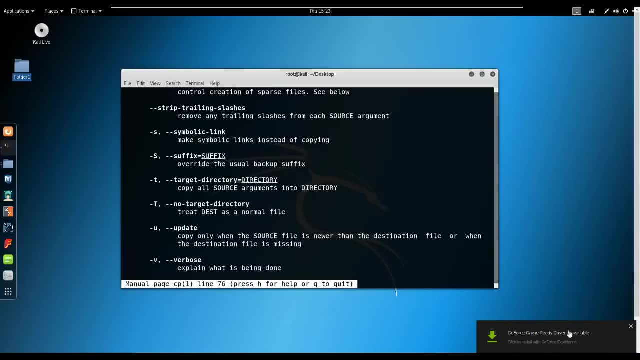 And you can go through it and look. you know, this is how I learned Linux: just going through the manual, looking at the different attributes you can use And, I'm guessing, get the idea And it's quite simple. you can, you can navigate the manual very, very simply. We've got a. 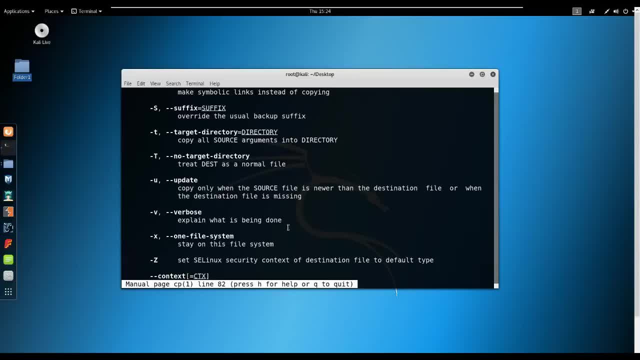 NVIDIA graphics driver available. Well, I'm not going to look into that for a while. quit, so I'm gonna quit. the manual is one thing at your advantage. the other thing that you have at your advantage is the help command. so let's say we can use. 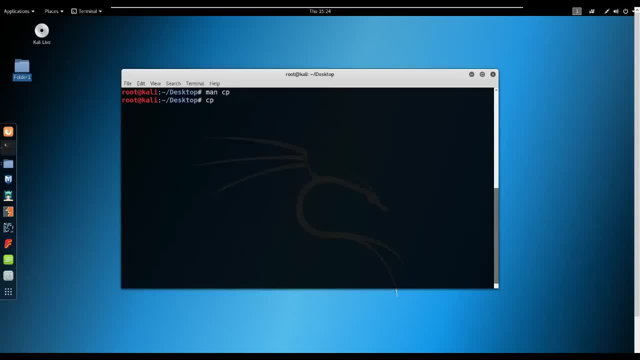 let's use CP, which is copy. I'll. I'll be talking to you guys about how to use the copy and the move commands in the next lecture, because that requires quite a lot of explaining and you have to get the directories right and blah, blah, blah. so CP, and the next command is help, which is a universal command that will 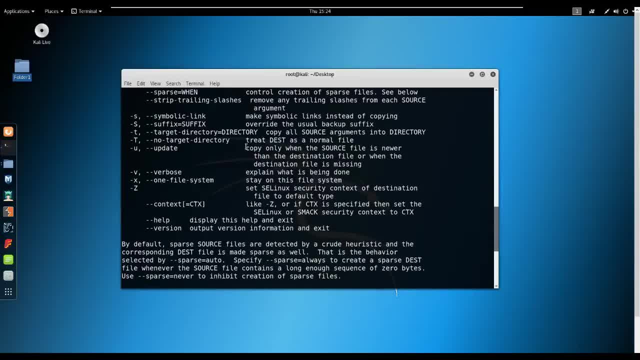 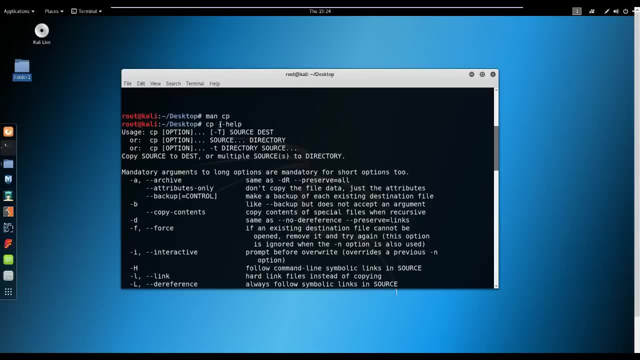 give you help with any command that you have. as you can see, it's given us everything and I know I've used this before in previous videos, but I really didn't explain that the help command is very, very, very useful. I mean it's, it's awesome. so, as you can see, it's gonna tell you it's gonna give you a lot of. 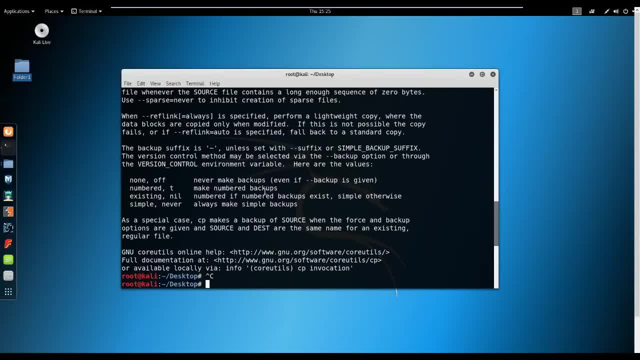 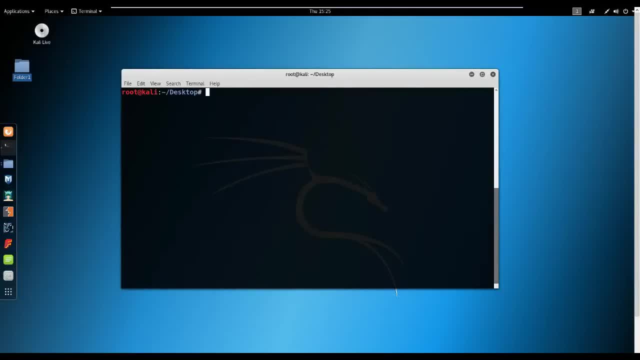 the commands and what they do and you get the idea it's a help command. so let's clear that up. and yeah, we've actually talked about a lot of commands in this video and there's still a lot that we'll get into, like, as I said, copying, you know. 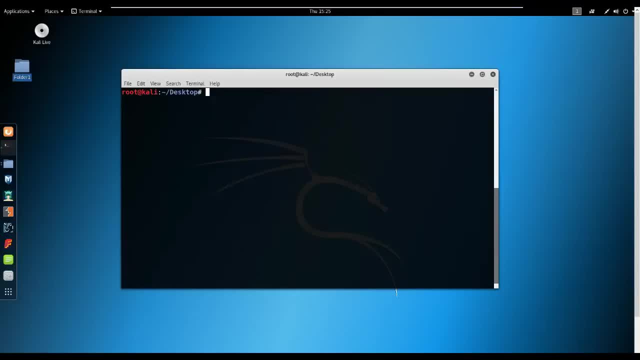 compressing files. the works really. so that's basically it for this video. guys, I hope you found value in this video. if you enjoyed the video or you liked it, please leave a like down below. it really does help. if you didn't like the video, please let me know why you didn't in the comment section below your feedback is. 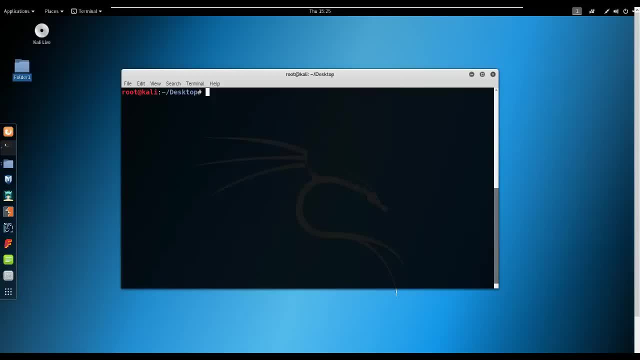 always appreciated. if you have any questions, let me know in the comment section on my social networks or on kick. I'm always available on kick almost 24- 7, apart from when I obviously have to get some shut-eye. but I try and respond as quickly as possible. 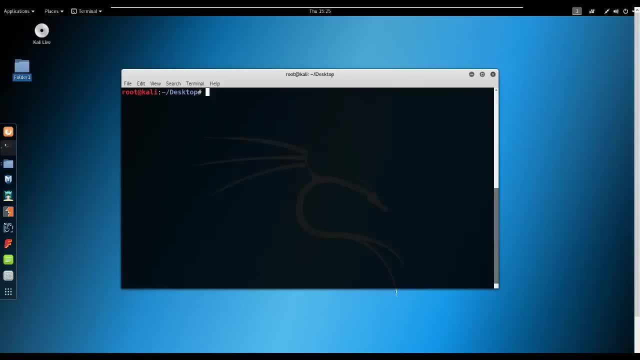 one more thing, guys. I've just hit 8,000 subscribers. I mean it's, it's mind-blowing how far I've come, and I mean I couldn't have believed that I would have reached this far. and I just want to say thank you, you know, thank you. 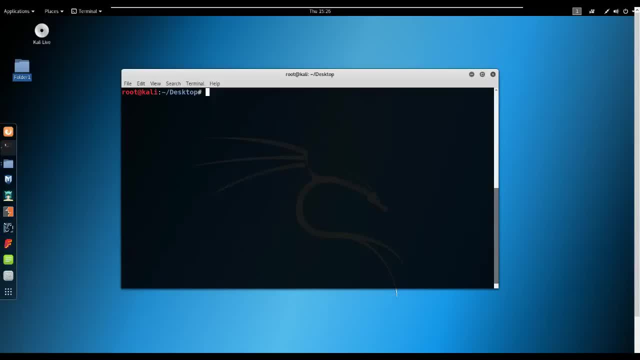 thank you. thank you so so very much for the support. you guys are amazing and it's probably, I think, the best community on YouTube right now in terms of support. so thank you so very much and, as always, I'm committed to providing you guys with content on a daily basis. otherwise, thank. 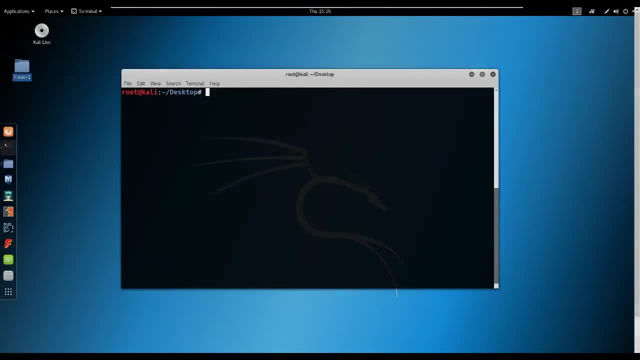 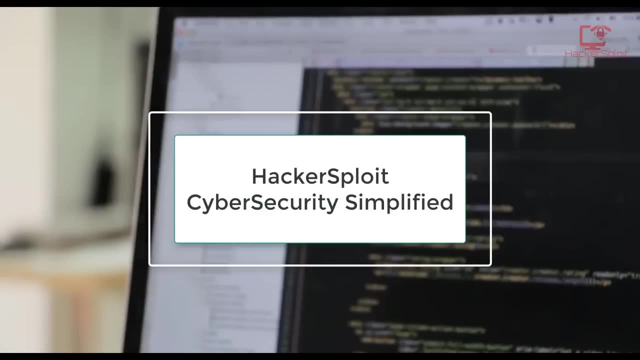 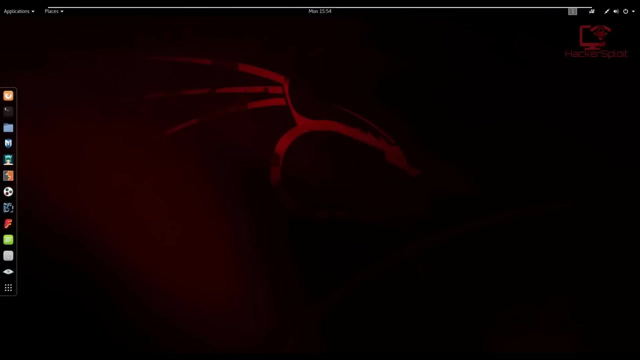 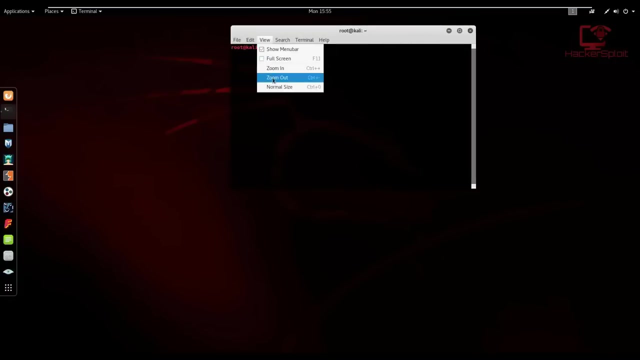 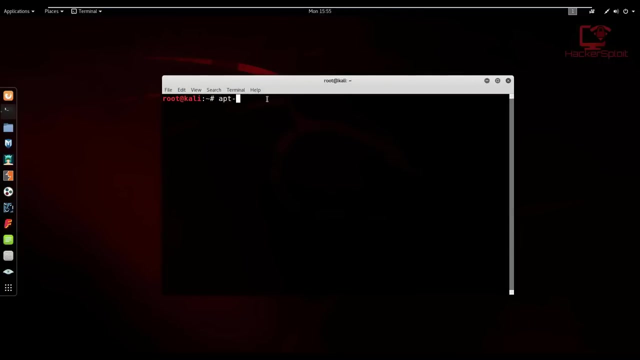 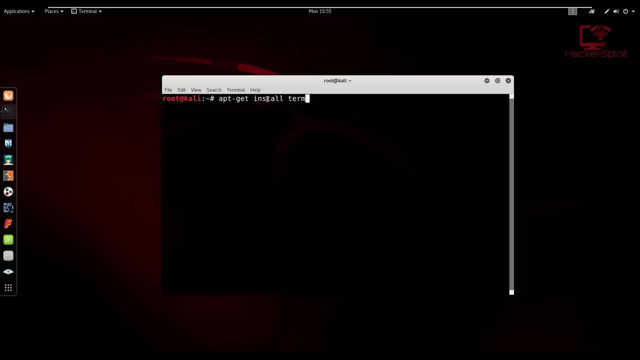 software that you're using. like I said, you can do everything you're doing right now with stand alone. you're not going to do it all at once, I'm just going to show you how to do it, and it actually allows you to be a bit more robust with your. 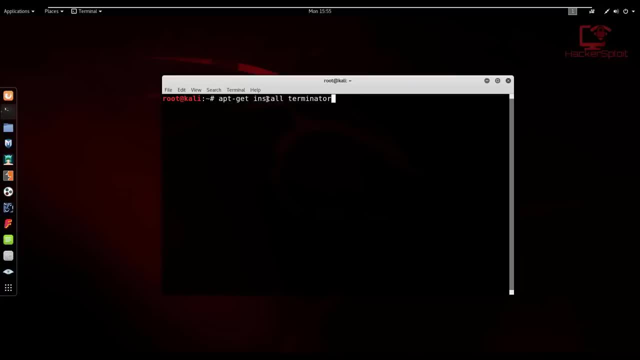 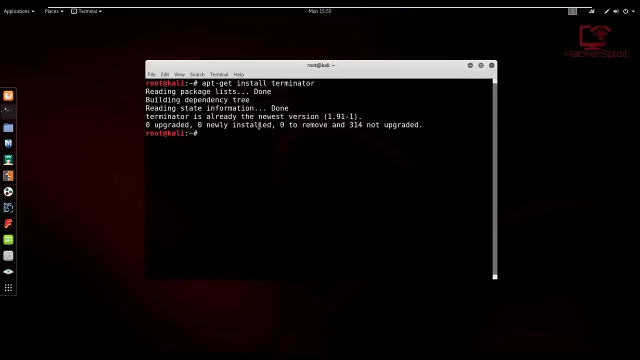 make sure you use the sudo or super user. i'm already in route so i don't need to enter. so get installed terminator and once i hit enter, it should download it and install it. i already have it installed because, as i said, i use it a lot and this is what i prefer. 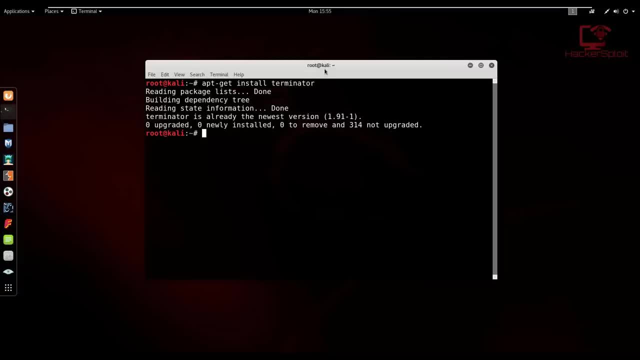 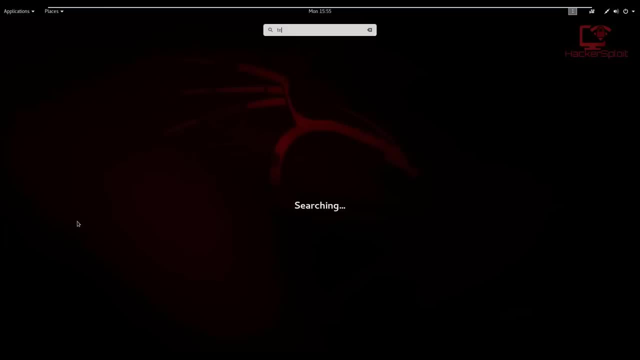 when i'm doing my uh, you know, when i'm doing my work, projects and stuff like that, and i'm going to show you why in a second. all right, so that's done. once yours is installed, um, you can basically search for it. uh, so, terminator, and it's gonna be the red one, all right, so i'm gonna add this: 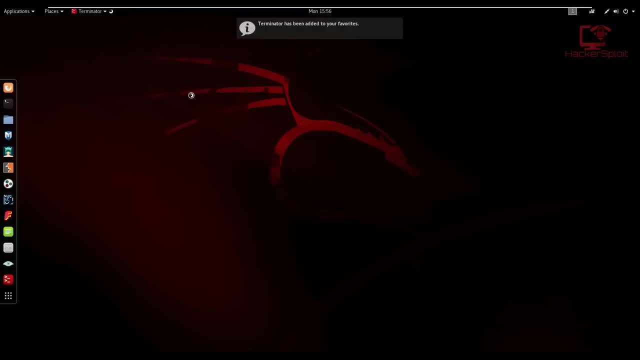 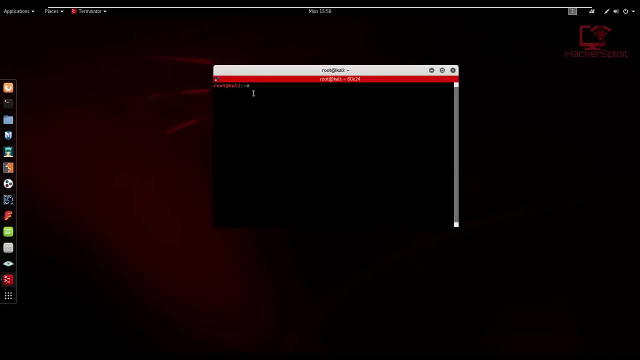 to my favorites right now. and once i launch it, uh, it's going to open up the terminal. let's give it a few seconds. there we are and you might be asking yourself: well, uh, what's this? uh, you know, it just works like a normal. uh, it just works like a normal terminal, and you're right it. 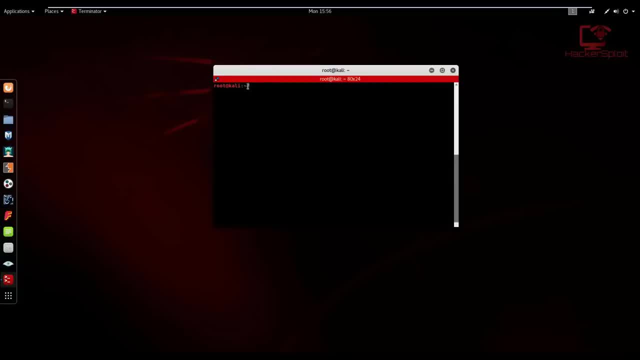 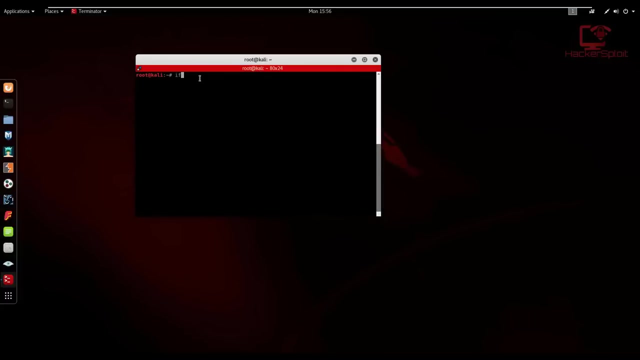 is a normal terminal. the reason i use it is it allows me to uh, to have multiple terminals opened up in this same instance. so let me show you what i mean. all right, so if i wanted to, if i was working on a different project, for example, let's say i wanted to start scanning, uh, for let's say i wanted, 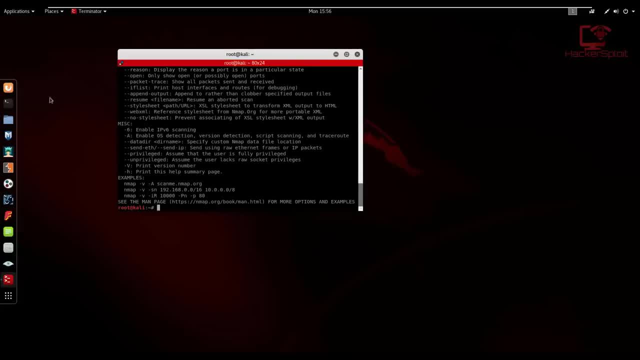 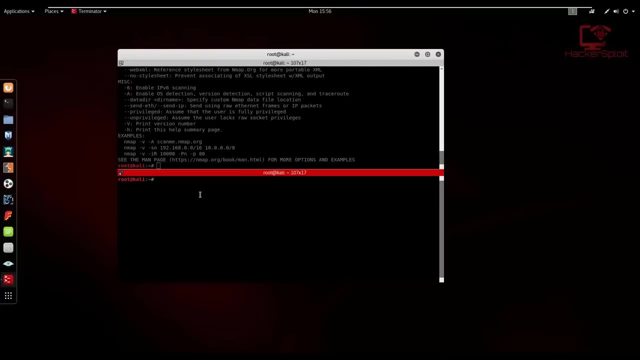 to open up nmap here, whatever, and i wanted to open another terminal instead of opening another instance. what i would do is i would split it vertically and it would open another one for me, all right. and then i could uh, let's say, open, uh something like nikto, all right, and open that up. 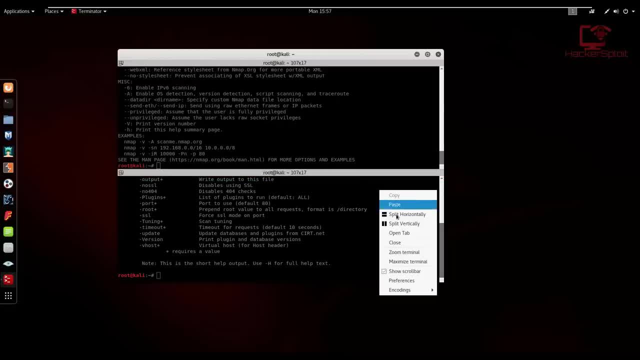 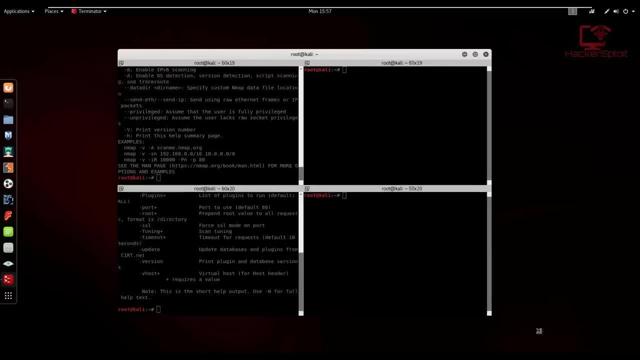 like so. and what if i wanted to open a little bit more? i could split it vertically and open one more, there and again split it vertically and open another one, and i guess you guys can see why this is so cool and awesome. it allows you to view all your running processes in one, which 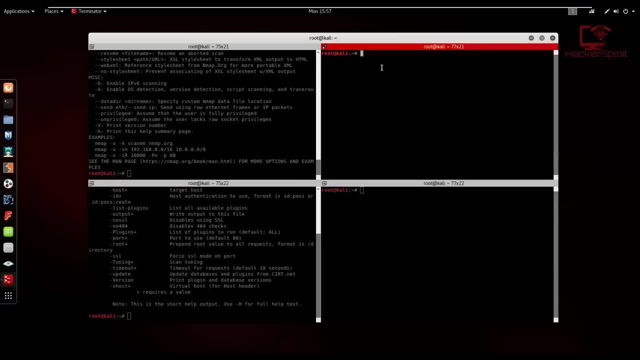 is awesome, instead of switching from one terminal to another. so i could go for proxy chains here, uh, chains um, and i could say um, proxy chains, firefox, oops, and like, um, like something like duck, duck, gocom, something like so, and it will start up there and that's good, we're working and open. 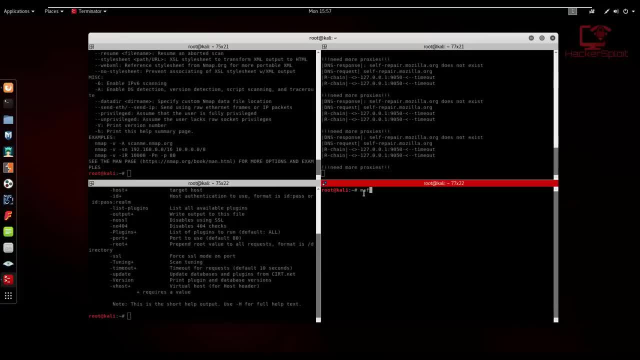 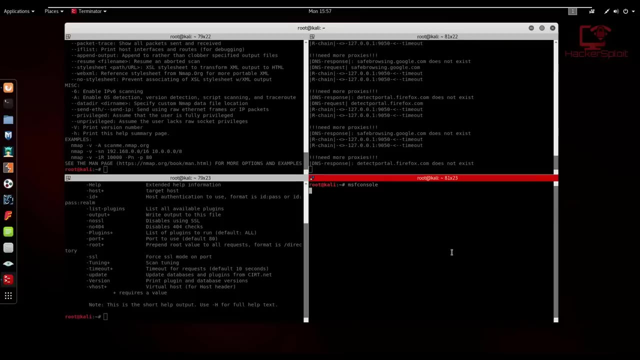 up there and in the fourth one we can- oops, msf console, we can open up, uh, oops, we can open up metasploit there and it should start up as well, and i guess you guys can see how awesome this is. so it allows you to view your terminal in more of a robust view and in a split window and you can see. 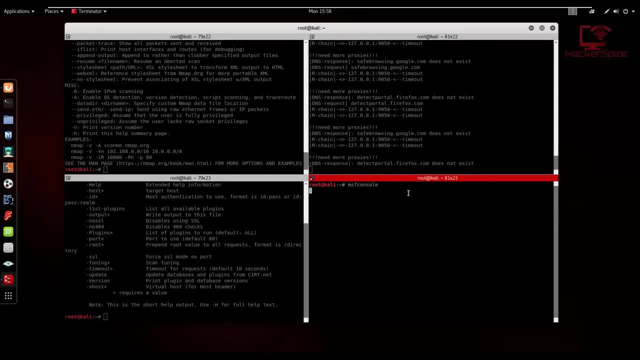 how it's running in one, and it's pretty, pretty awesome. so this is a little quick tip that i wanted to show you guys and it hopefully it will improve your productivity and your workflow in cali linux, which is very, very important, especially as you move on to larger and larger projects. 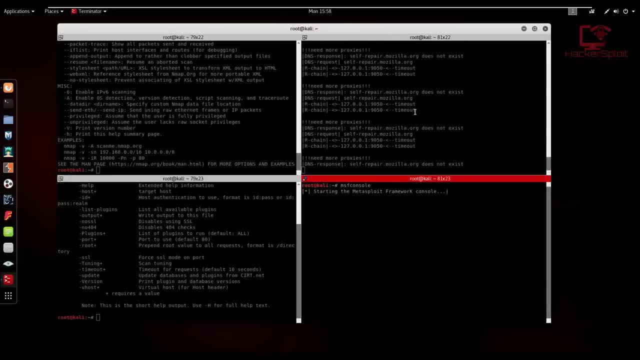 you need to- uh, you know- speed up the process and be very, very efficient at what you do, so i hope you guys found value in this video. if you did, please leave a like down below. again. suggestions or questions are welcome. leave them in the comment section or if you have any personalized questions. 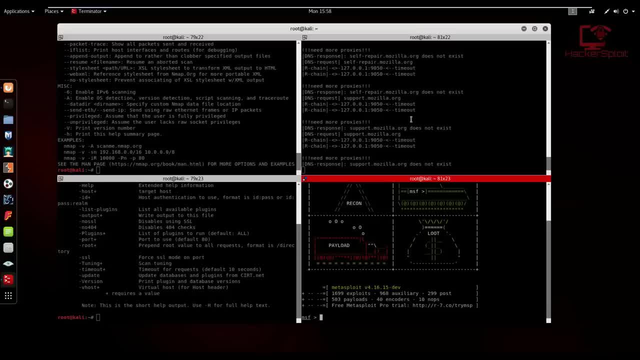 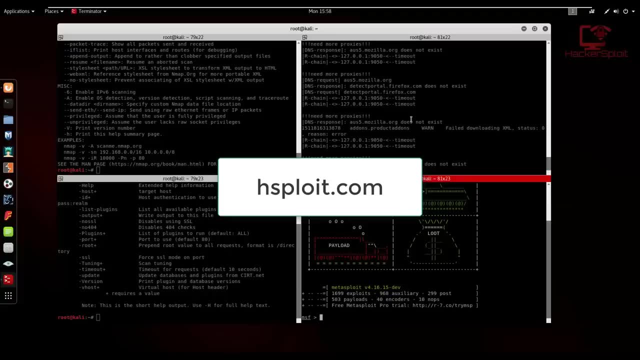 you can hit me up on my social networks or on kick for the latest hacking news and resources. check out my website, hackersploitcom or hssploitcom- the link will be in the description and i'm adding tons of new news and guides to the website, so make sure to check it out for a lot of cool resources. 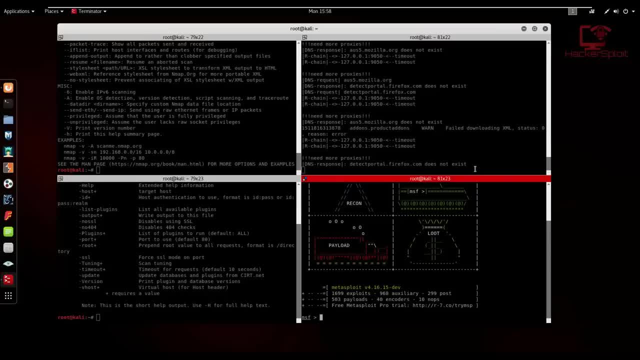 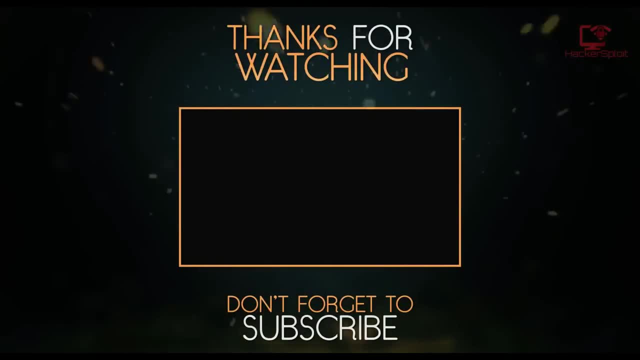 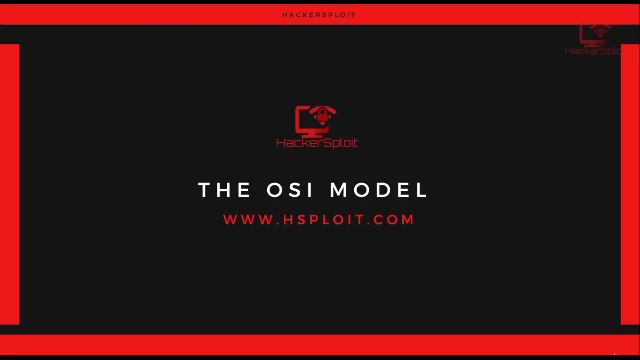 and, yeah, i hope this video helped you guys and i'll be seeing you in the next video. peace out, hello everyone and welcome to this video. in this video, we're going to be going over the osi model, all right. so you might be asking yourself: why exactly do we need to go through the networking? 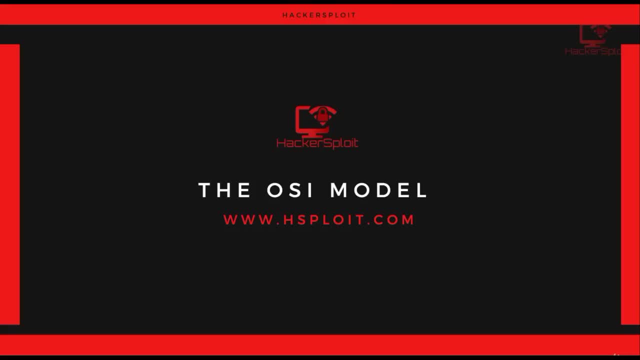 fundamentals. well, if you look out there and you see most of the courses on nmap or network scanning, they really just focus on the actual scanning. but the truth is many of the people who are actually going to take the course are really beginners to the whole process of network scanning and therefore, 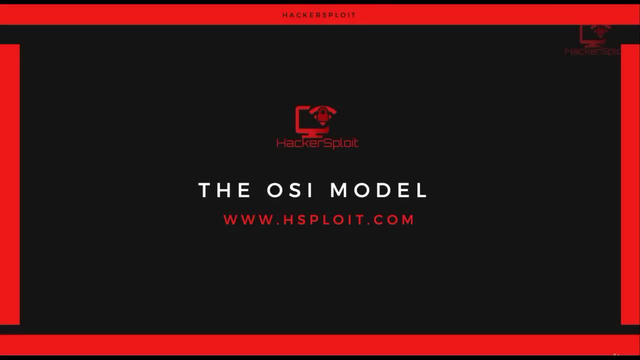 it is essential to understand, first and foremost, the osi model and how nmap works with the uh- the osi model- for you to understand some of the scans that we're going to be performing, therefore giving you a much better understanding of how the network scanning process is and how to perform your own. 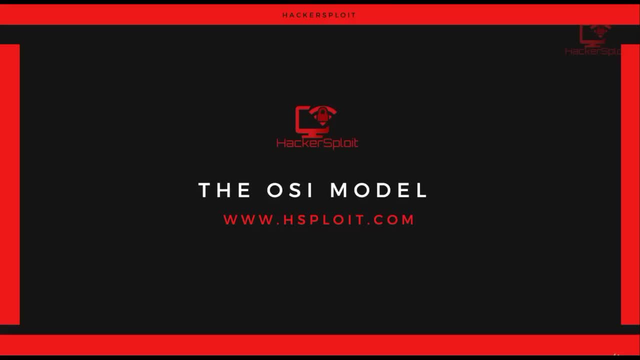 custom scans, all right. so it's very, very important that you understand the basics, or the at least the fundamentals of networking. and to get this started, we're going to be looking at the osi model, we're only going to be looking at it, basically, and that is to. 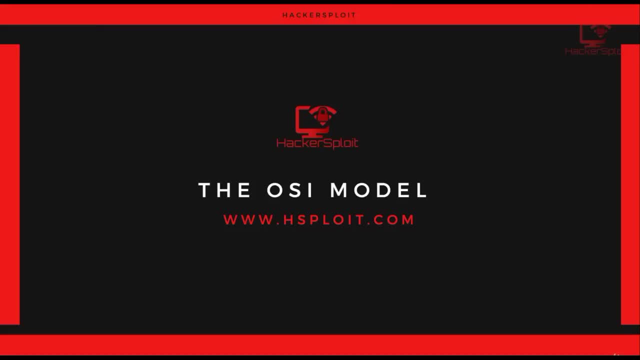 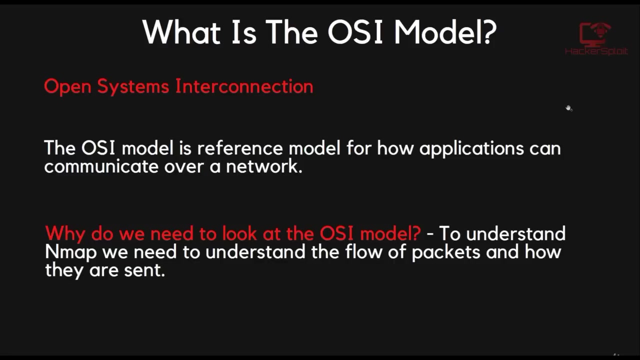 furthermore, explain the layers that nmap uses. uh, you know of the osi model- and then, furthermore, understanding the protocols that are used in those layers. all right, so let's get started with the osi model now. by definition, the osi model is uh or stands for the open systems interconnection, all. 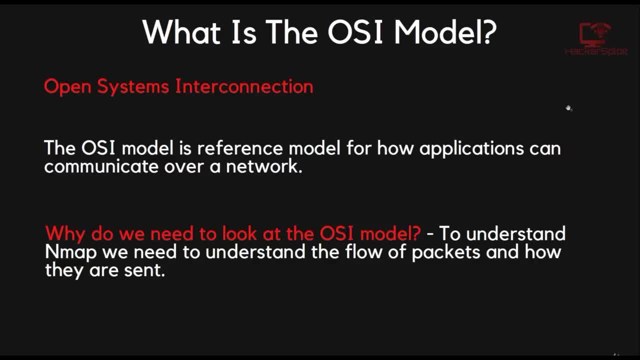 right, so it acts as a model or a reference point for how applications can communicate over a network. all right, so it's a reference point for network engineers or systems administrators to look at the osi model and how they can communicate over a network. all right, so it's a reference point. 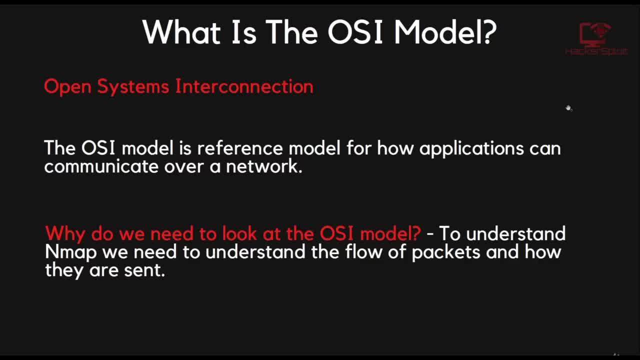 and understand how applications communicate over a network. so why do we need to look at the osi model? all right, we need to look at it to understand uh, nmap and how the flow of packets uh is on the network and uh, how packets are sent on the network. all right, so we need to understand how packets are. 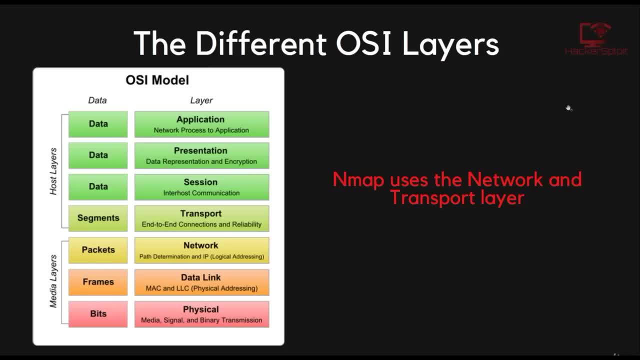 sent and how they flow on a network. all right, so if we just look at the, the different osi layers, that would obviously that the osi model is built upon. you have the seven layers, and the most important ones that we're going to be looking at are the osi model and the network. so we're going 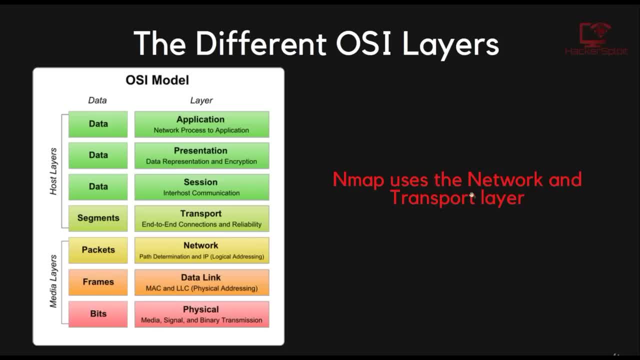 to be looking at or focusing on are the network layers and the transport layers. all right, so as you can see here, we have the network and the transport layers. now i will be looking at this in the next videos, and that's because they do require their own- uh, their own video for you to. 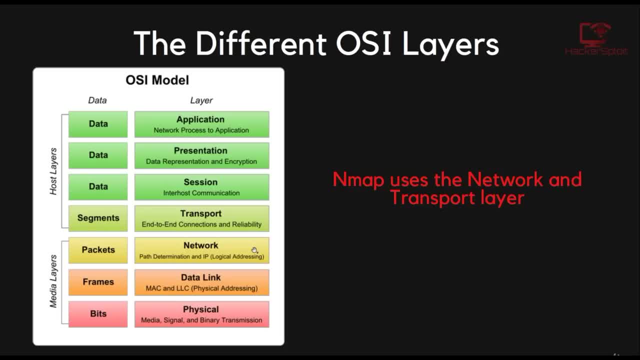 understand how they work and the protocols that exist within them, right. so i would recommend that you go through the osi model and understand how each of these layers communicate with each other and why they're so important. but when it comes down to nmap, nmap uses the network and the transport. 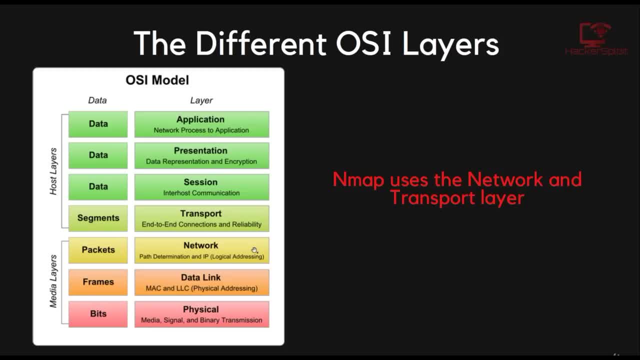 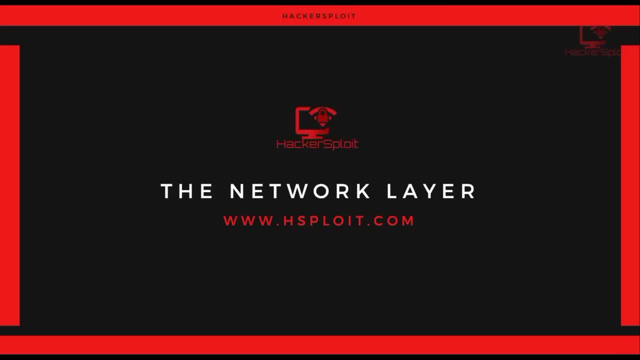 layer and that's what we're going to be paying attention to. all right, so i'll be seeing you in the next video. hello everyone and welcome to this video. in this video, we're going to get started with our network fundamentals, more specifically, with what the network layer is and how it relates. 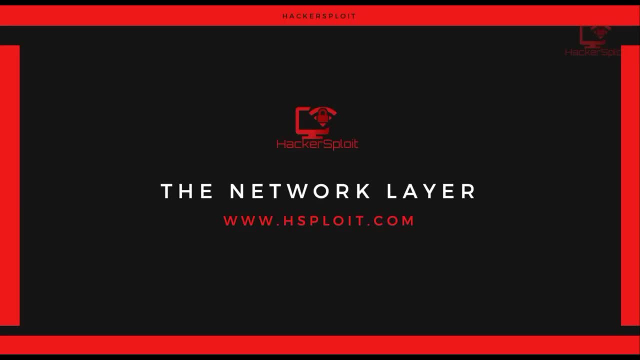 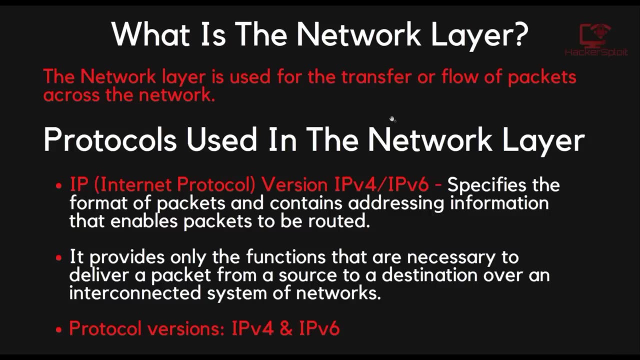 to the osi model and, furthermore, how it will allow us to understand how nmap works much, much better. all right, so let's get started. and uh, to get started, the first thing we need to ask ourselves is: what exactly is the network layer? so, the network layer is used for the transfer or the flow of packets across the network, right so? 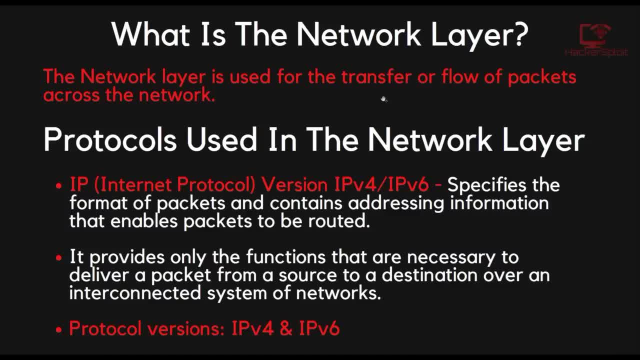 this layer is used for how packets are going to be transferred across the network. now, the protocols that are used in this layer may sound familiar to you. you might have already understood, or you might already know, the protocols that i'll be showing you right now. now, the most important protocol is the internet protocol. that is sub-denoted into the versions. 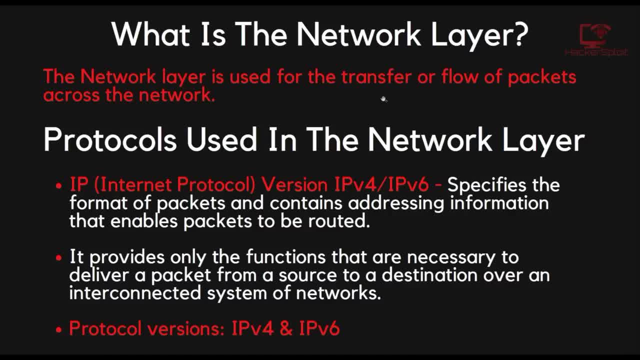 we have the older version, which is ipv4, and the newer version, which is ipv6. all right, so ip version 4 and ip version 6.. all right, so the ip protocol, or the internet protocol, sorry, specifies the format of the packets and contains addressing information that enables the 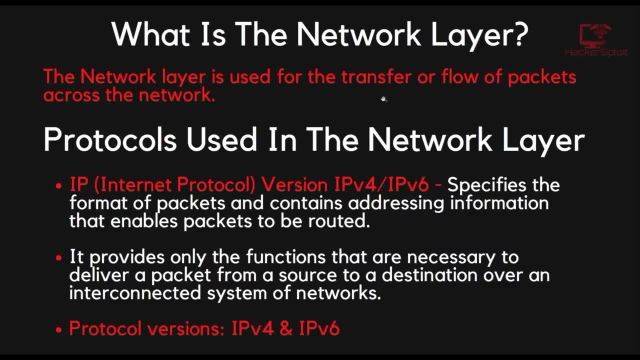 packets to be routed, all right. so, essentially, the internet protocol will specify the format of the packets and will contain the addressing information. uh, in the sense that it it contains information like the mac address, etc. etc. that allows the packets to be routed across a network. all right, 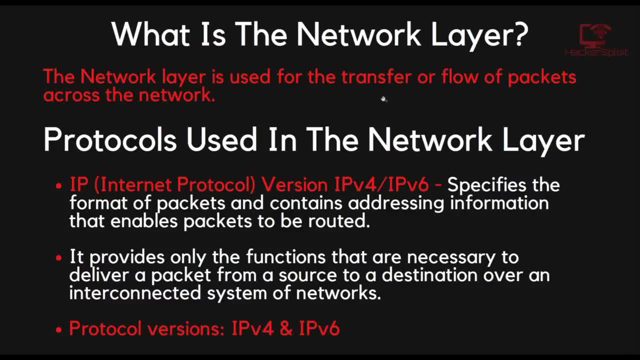 so it provides only the functions that are necessary to deliver a packet from a source to a destination over an inter interconnected system of networks. all right, so its purpose is to make sure that a packet is sent to its destination from its source and to make sure it gets sent there uh correctly and obviously, uh efficiently. now, as i said, the protocol versions: 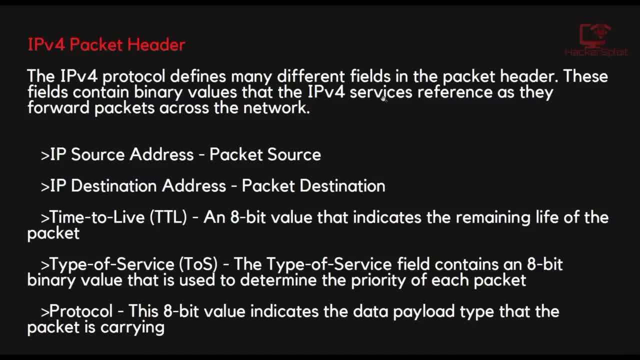 that we have are ipv4 and ipv6. now, when we look at the ipv4 packet header- all right, the packet header is very, very important to understand. uh, the information that is contained within the header. all right, so the ipv4 protocol defines many different fields in the packet header right. 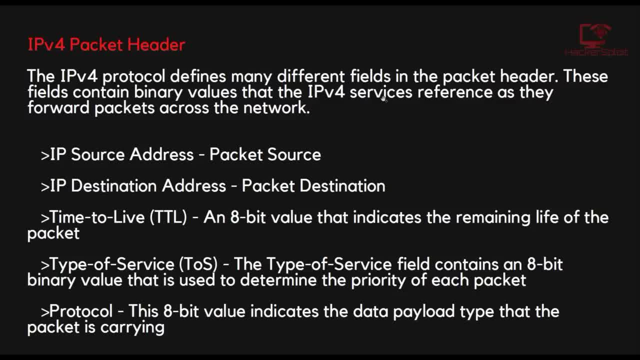 so these fields contain binary values that the ip for the ipv4 services reference as they forward packets across the network. all right, so essentially the information in the ipv4 packet header is essentially information about, as you can see, firstly the ip source address, the packet source. so where is this packet coming from? you then have your ip destination address. where is this packet? 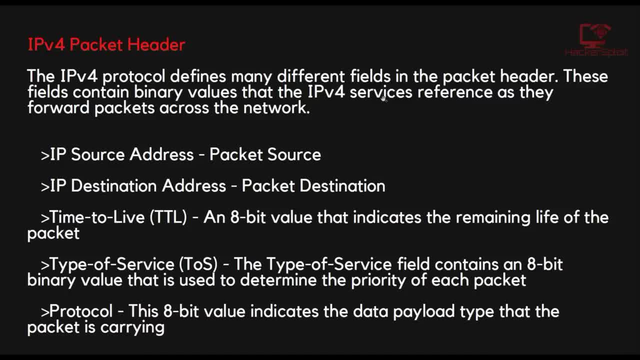 going to what ip address? is this packet destined for? all right, you then have your time to live, which is essentially an 8-bit value that indicates the remaining life of the packet and how long the the packet can be transferred. okay, you then have your type of service, which again contains uh. essentially they. 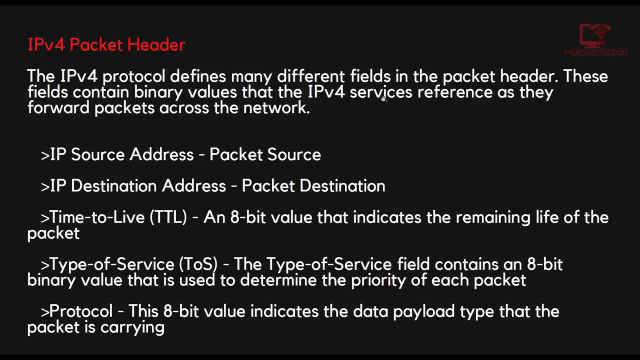 all contain an 8-bit binary value that is, in this case, used to determine the priority of each packet. all right, so the type of service is used to prioritize, uh, the packets depending on their priority, obviously. and finally, you have the protocol, which is again an 8-bit value that indicates the data payload that the packet is. 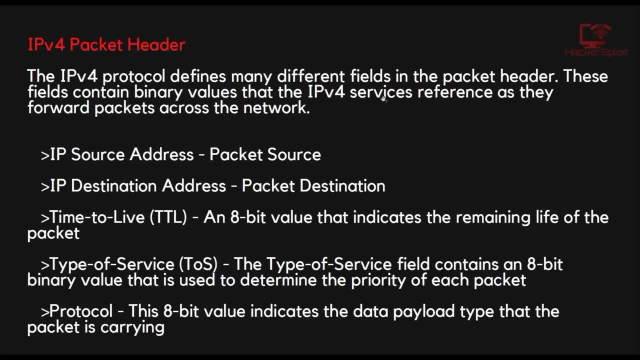 carrying all right. so the uh, the ipv4 packet header is essentially? it contains information, as i said, uh, that will help the packet to be routed. that is what the uh, the internet protocol, is used for in this case. uh, very, very simply, to understand what's happening here, it contains uh. 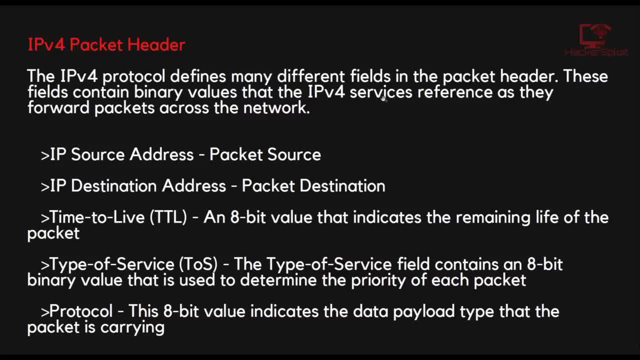 you know the ip source address. so, essentially, what that means is: where is this ip coming from? all right, where is this packet coming from? it then has the destination address, where it's obviously going to contain the address to which this packet is supposed to be delivered, and then, furthermore, we have the three other packet headers that are not really important. 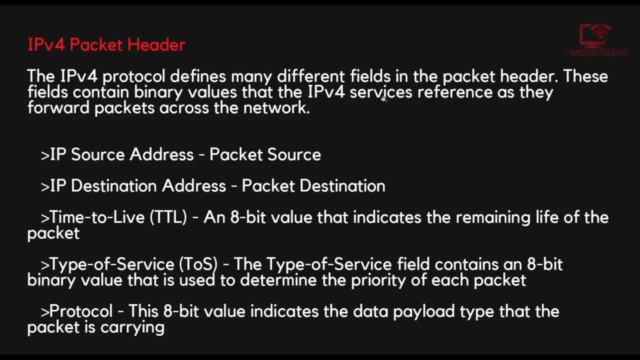 but are equally as important, depending on the types of packets you're sending. you have your time to live, you have your type of service, your type of service and your protocol all right. so that is going to be it for this video. now, that was a very, very good or basic introduction to 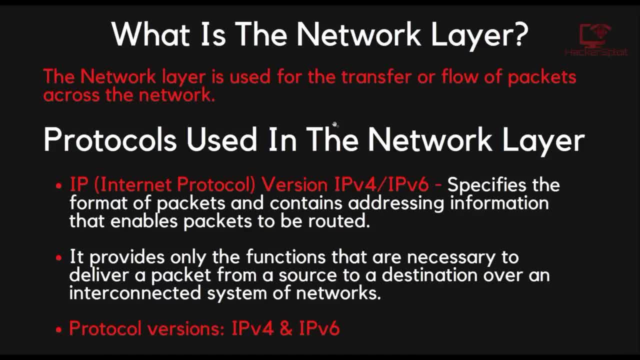 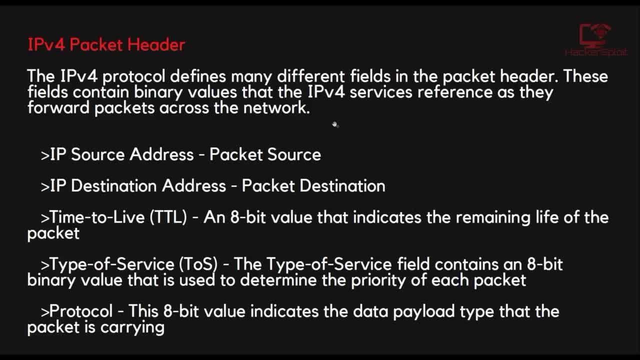 what the network layer is and what it is going to be. uh, it is all going to be about now. the reason cover this is because, when we'll be performing the scans, i will be referencing a lot of these, uh, a lot of these packet header information so that you can understand the type of scans we 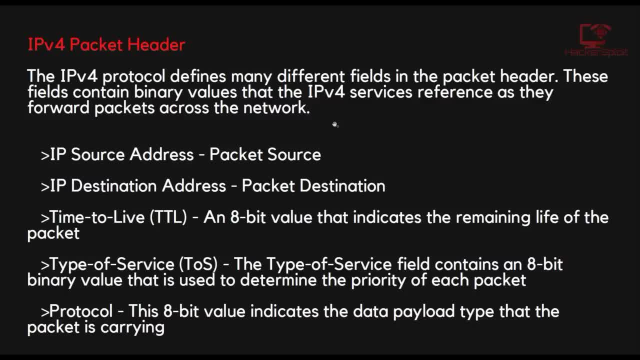 are carrying out and why they're important. all right, so again, this is just the network fundamentals regarding the osi layer, more specifically in this video, the network layer. so it's very, very important to understand- uh, you know- important information like what the network layer is used. 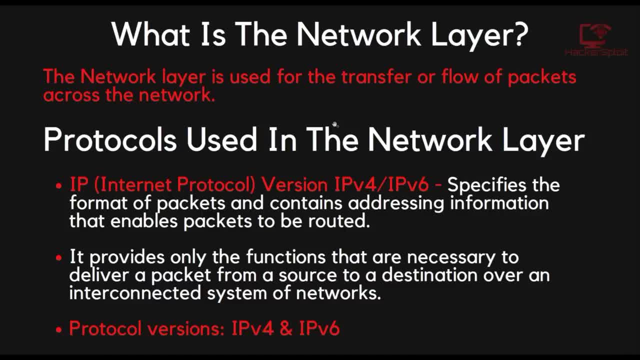 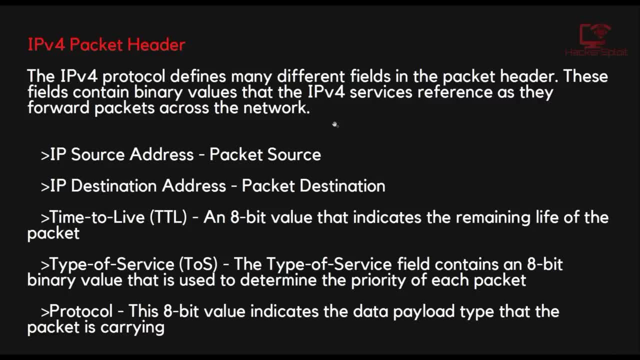 for the protocols that exist within the network layer, the protocol versions, what exists in the, the packet headers and, finally, after you understand that, you'll have a great idea of how packets are sent across the network. all right, so in the next, in the next video, we'll 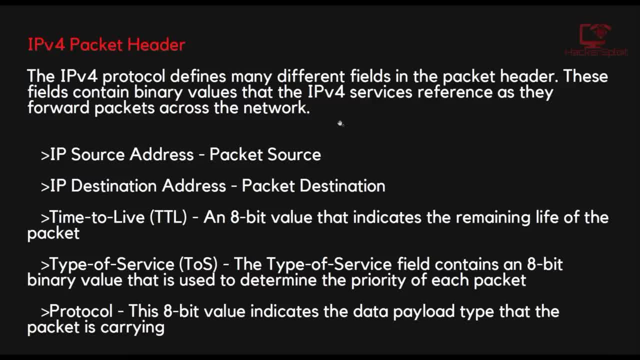 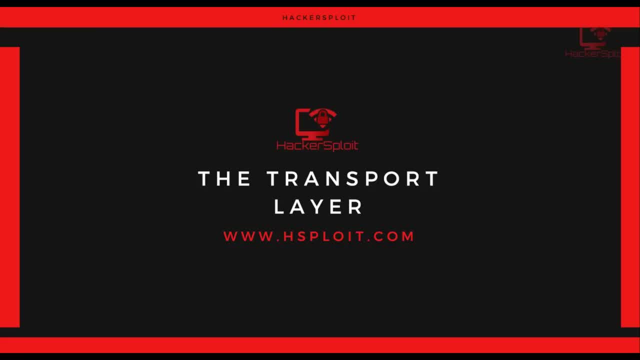 actually be looking at the transfer layer, so i'll be seeing you in that the next video. hello and welcome to this video. in this video we're going to get started with the transport layer, all right. so in the previous video we looked at the network layer, and now it's time to get started. 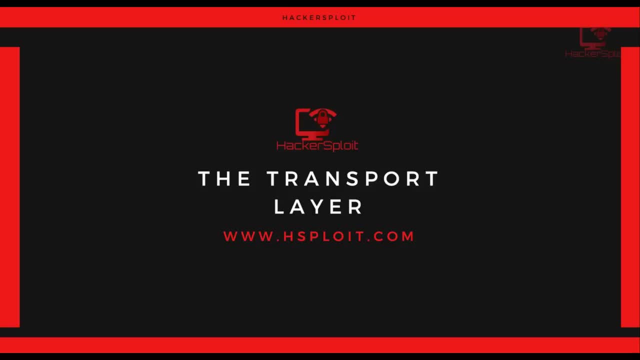 with one of the most important layers- uh, you know, on the usi model- and one of them that nmap utilizes really, really strongly, and that is the transport layer. all right, so let us uh look at what the transport layer is. well, the transport layer is essentially used for the 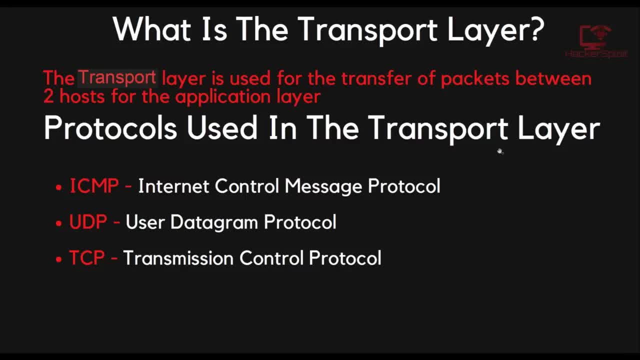 transfer of packets between two hosts for the application layer. right, so it is used uh for the transfer of packets between two hosts, uh for the purpose of the application layer. now, we'll look more into this as we move along. all right, now let's get started with the protocols that are used. 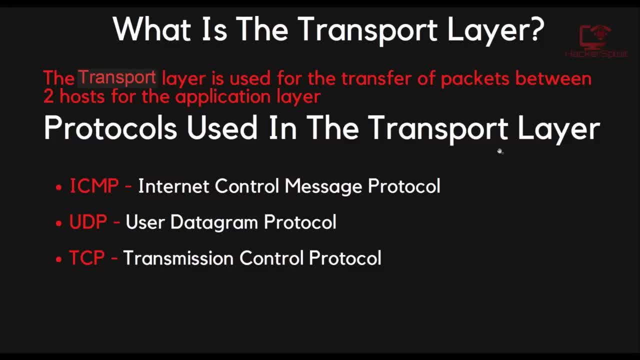 in the transport layer now getting started. we have the icmp protocol, all right, which is the internet control message protocol. we'll look at what it does in a few seconds. we then have your udp protocol, which is your user datagram protocol, and finally, uh, one that you may be familiar with, or you should be familiar with, that is the tcp or. 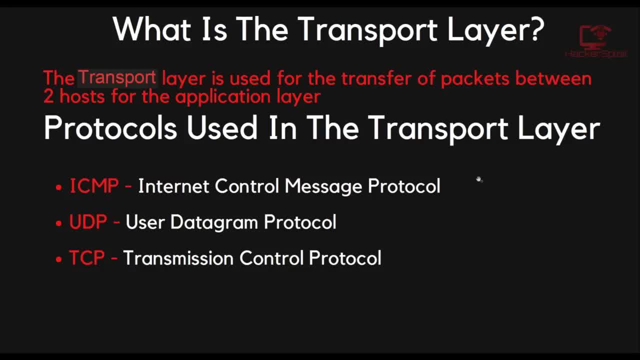 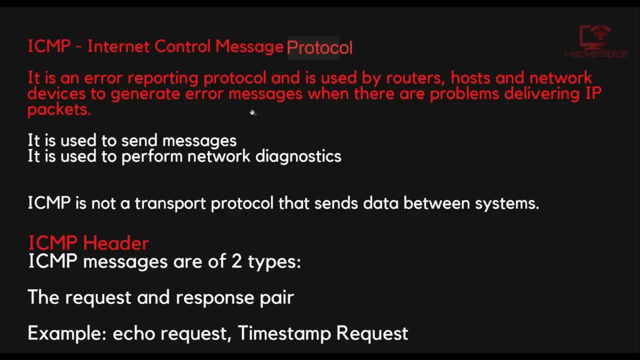 your transmission control protocol, right so? so let's look at how each of these works. all right, so if we go into the icmp, which is the internet control message protocol, you can see that it is an error give error reporting protocol that is used for the transfer of packets between two hosts. 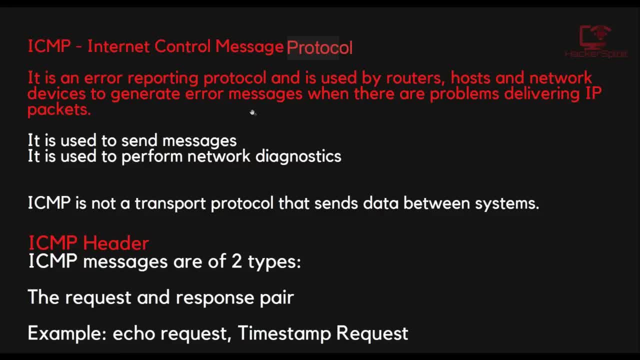 is used by routers, hosts and network devices to generate error messages when there are problems delivering ip packets or internet protocol packets. all right, so the primary function for the icmp part, or the the internet control message protocol, is: it is used to send messages and it is used to 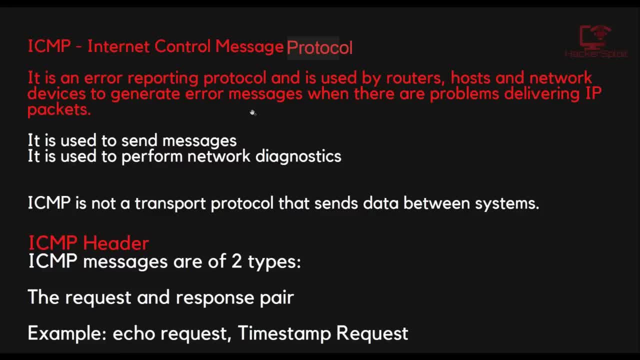 perform network diagnostics. we'll be looking at this a lot with nmap and i'm sure you'll be really, really excited to see how this works. all right, so the most important thing to understand is that it is used to send messages or probes, and it is used to perform network diagnostics. uh, the one thing. 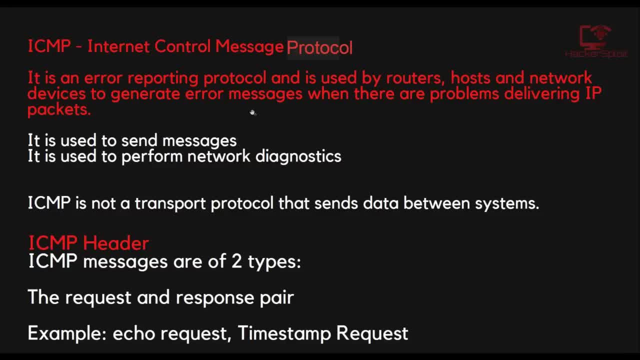 you need to understand is that icmp is not a transport protocol that sends data between system systems, so it does not deal with the sending of data. now, when it comes down to the icmp header, we have two types of uh. we have two types of flags or messages that are in in the icmp header. all right, 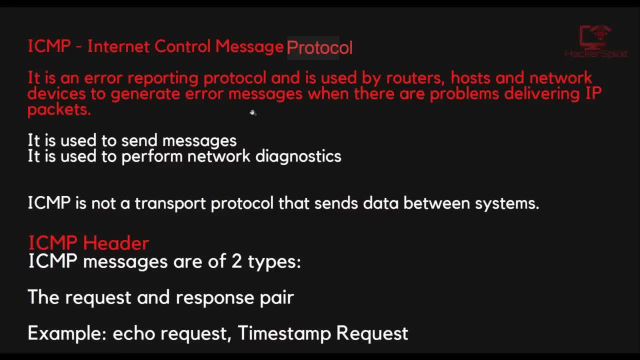 so you have the request and the response pair. all right. so now this- i'm pretty sure you you have heard of it, but it uh you might know- the first of all about this is that the iq request uh and the echo response. so we'll be looking at all of these uh icmp requests and response pairs again. these are quite advanced. 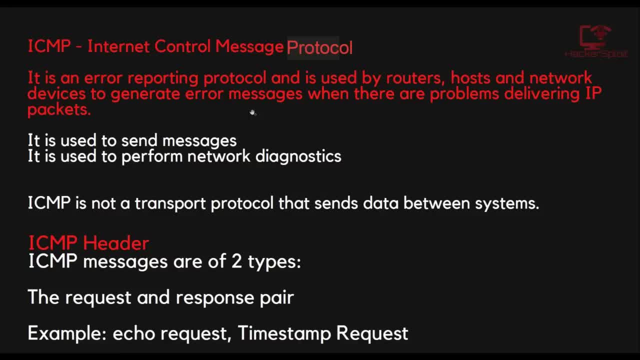 but when performing the scans, i'll be explaining them. the only thing you need to understand is that you have your echo requests, you have your timestamp request, etc. etc. and, since they're in pairs, you have your echo request and your echo response. all right, moving along to the udp, which 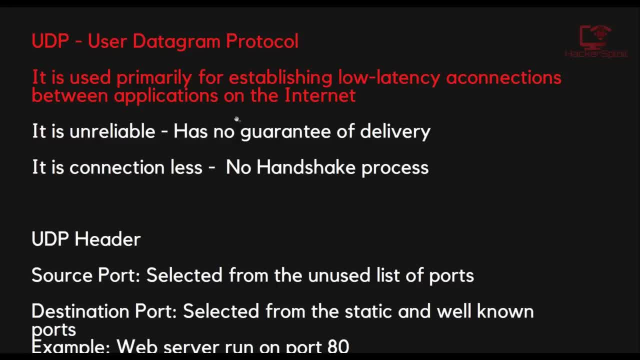 is the user datagram protocol, uh. the udp is used primarily for establishing latency connections between applications on the internet. all right now. the two common features about UDP is that number one. it is a very, very unreliable, in the sense that the packets are not. there is no guarantee that the packets will be delivered to their destination, and the great 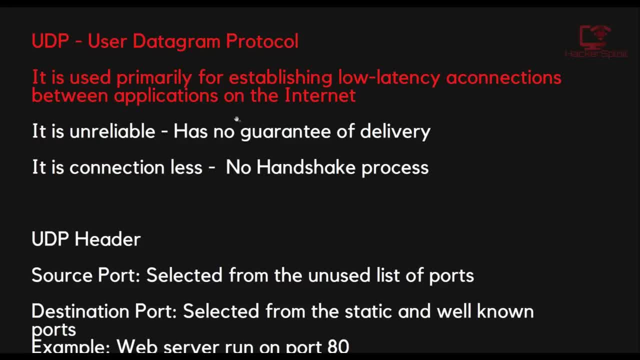 thing about it is it is connection less in the sense that there is no handshake process required. we'll be looking at the three-way handshake when we start talking about the TCP or the transmission control protocol, but for now, just understand that UDP is used for it's essentially used for. 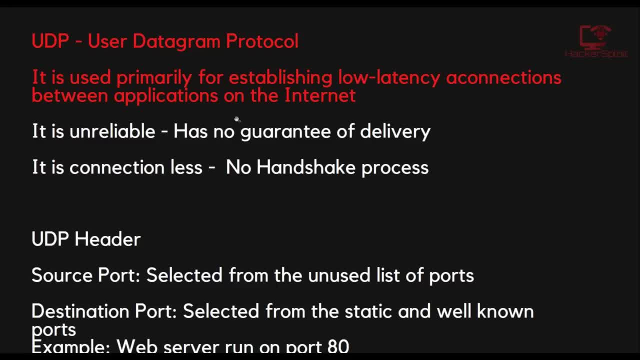 establishing low latency connections between applications on the internet. now, the great thing about it, as I said, it is, firstly, connection less, in the sense that there is no handshake process, and secondly, it is extremely fast. all right now, when it comes down to its disadvantage, it is very 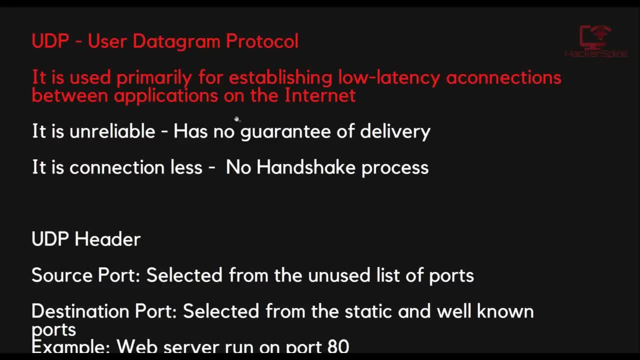 very unreliable in the sense that the you have no guarantee whether or not the packets will be delivered to be a destination. now, looking at the UDP header, we have our source port and our destination port, all right. so the UDP protocol essentially, as I said, is used for low latency connections. so the source port, that it. 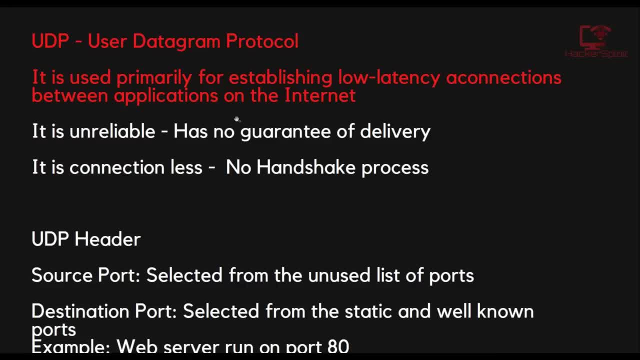 will be leaving. in terms of the ports that it will be used for communication will, essentially it will use a range of ports that is not very, very commonly used, so you know, you can talk about ports like port 4000, etc. etc. and finally, the destination port is going to be selected from a static and well-. 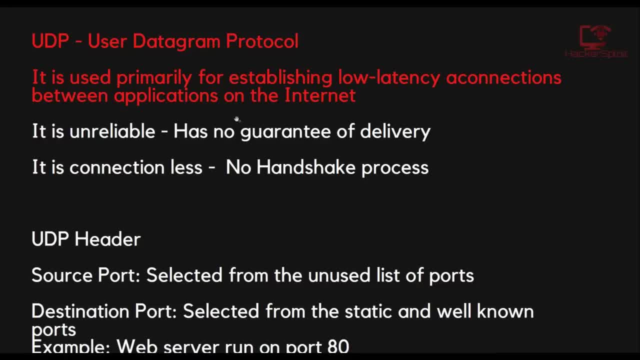 known list of ports. for example, it will target the port 80 where you have your. you know your different protocols that are running. you have your web server that's running on port 8080. sorry, that is not supposed to be on port 80 but on port 8080. all right, so that is the UDP or the use datagram. 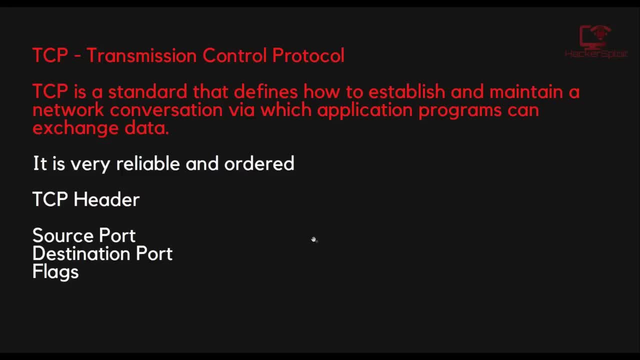 protocol when it comes down to the TCP or the transmission control protocol. TCP is essentially a standard that defines how to establish and maintain a network conversation via which app occasion programs can exchange data alright. so it's a protocol that governs how two devices, or two or more devices can establish a connection between themselves and, obviously, how they can. 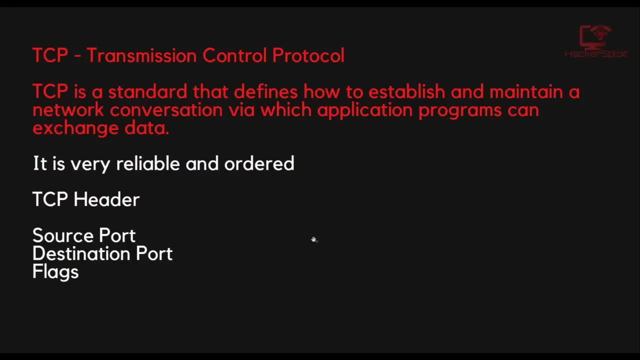 exchange data between each other. alright, now, the great thing about TCP is that it's very, very reliable and it is ordered okay. now, looking at the TCP header: the very this is very, very important to understand. in terms of the information stored in the TCP header, you have your source port and your 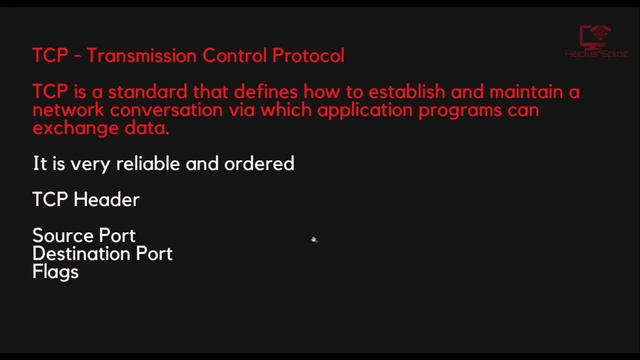 destination port, again all from a list of: firstly, your source port, leaving a port that is not very, very commonly used, And the destination port, you know going to post it a very, very common, like port 8080.. Your port 80. 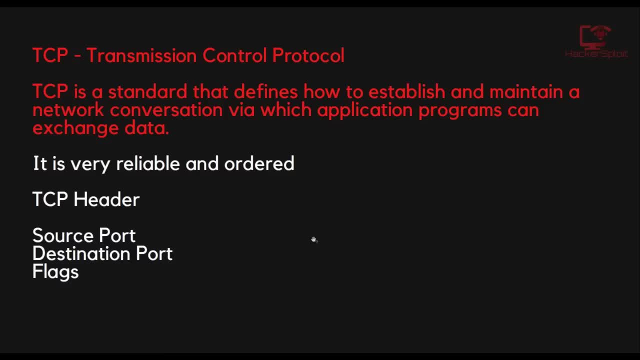 itself, and we know, for example, SSH connections going through port 22.. And finally, the last piece of information that is very important, that is carried in the TCP header, are the flags. Now we'll be looking at what flags we're talking about here And, more specifically, we'll be looking at this in 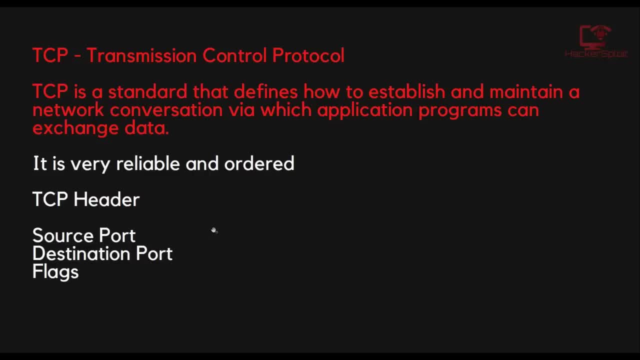 the next video when we'll be talking about the three way handshake and why it is important to understand how it works. Alright, so I'll be seeing you in the next video and we'll get started on the the three way handshake and how a connection is established. Alright, so I'll be seeing you in the. 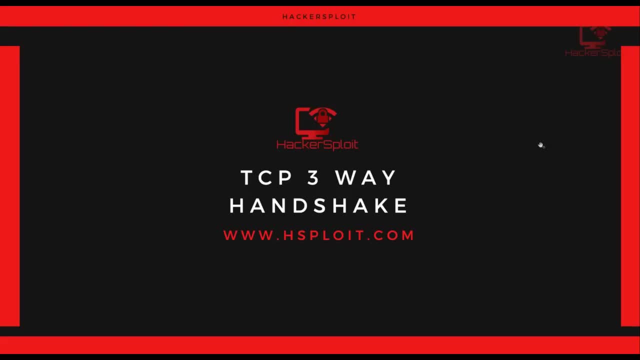 next video. Hello everyone and welcome to this video. In this video we're going to be looking at the TCP three way handshake Right now. this is very, very important to understand how the connection process or how a connection is established. 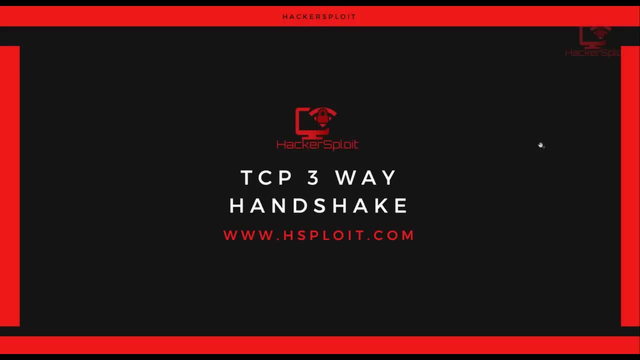 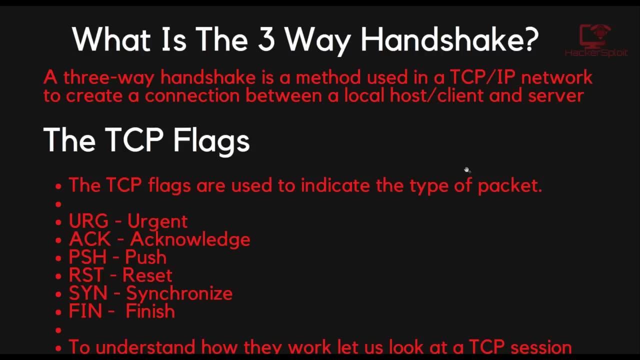 Using the TCP or the transmission control protocol. Alright, so let's get started, And I hope you're ready, because it's really exciting, Alright. so the first thing you might be asking yourself is: what exactly is a three way handshake? Well, a three way handshake is a method that is used in 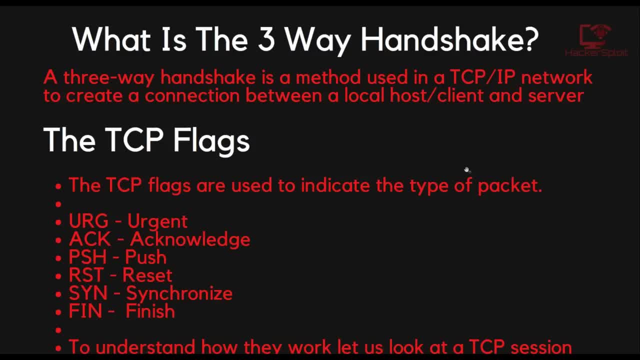 the TCP, slash IP or the transmission control protocol, slash internet protocol network to create a connection between a local host and a, or a client and a server. Alright, now your server could be your target, depending on whether or not you're using the TCP or the transmission control. 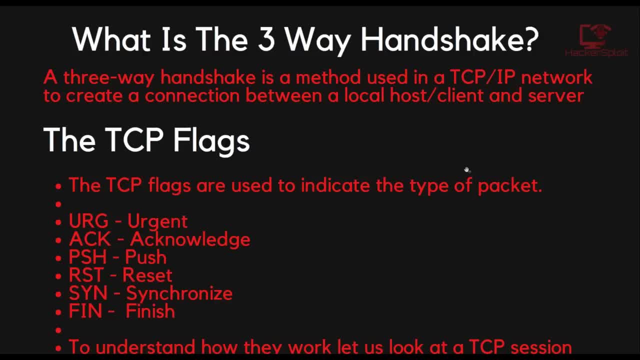 or not you're performing a scan, but we'll be getting into that Now. as I said, one of the most important things- that that is included in the TCP header are the TCP flags. Alright, so the TCP flags are used to indicate the type of packet that is being sent. Now let's look at the TCP flags. This: 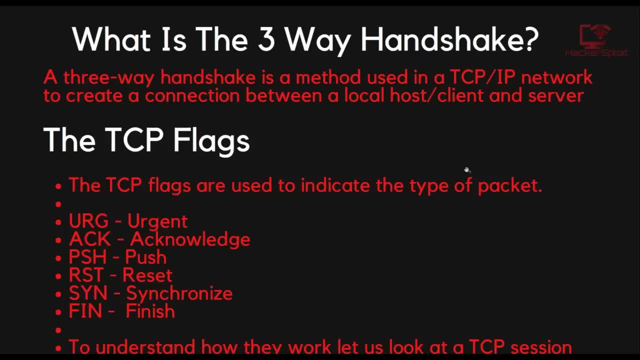 is very, very important because we'll be looking at this a lot when it comes down to nmap Alright. so the first TCP flag we have is the urge or the urgent Alright. and you then have your ACK, which is for acknowledge. you have your push, which is denoted by psh. you have your RST, which is reset. 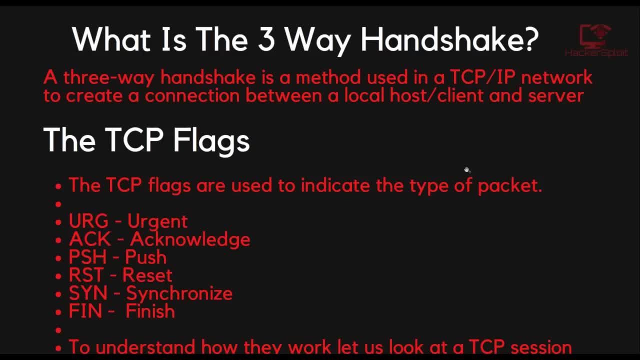 s y n, which is synchronized, and you have your fin, which is finished. they are all used to indicate the type of packet that is being sent Right, and you will understand this one will when we'll be looking at the and at how the TCP session is created. and now the connection is established. 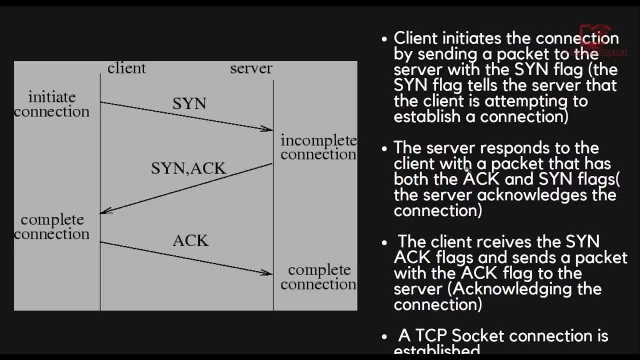 using the three way handshake. Alright, so let's look at that right now. Alright, so here I have a diagram that is simply explaining the connection between a client server. all right, so essentially what's happening is the client initiates the connection by sending. 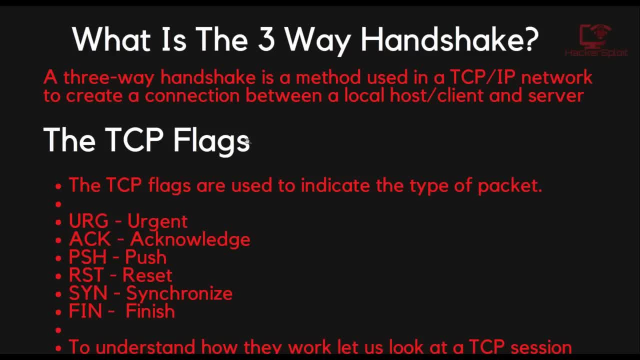 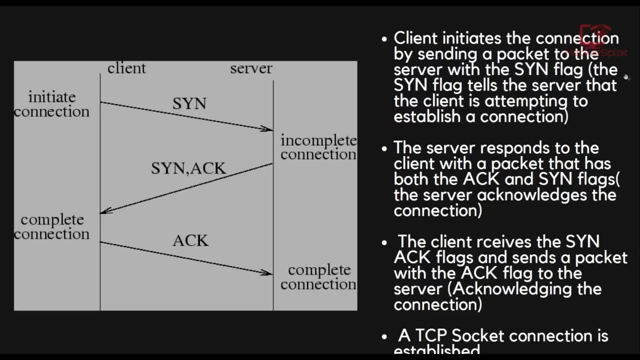 a packet to the server with the sin. all right, the sin is the synchronized packet. all right, so it's sending a sin flag. so it's gonna. it's gonna send a packet to the server with the sin flag. all right, so the sin flag is going to tell the server that the client is attempting to establish a connection. 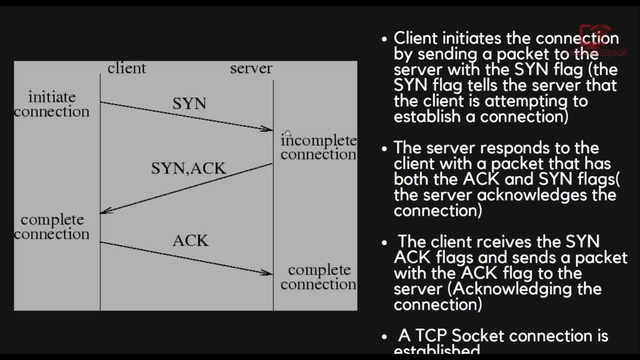 so, essentially, what's happening? what's happening is the client is going to send a packet to the server with the sin flag, all right, so it's saying it's a send. the purpose of this is it's telling the server that, hey, I want to establish a connection with you. all right, so the server 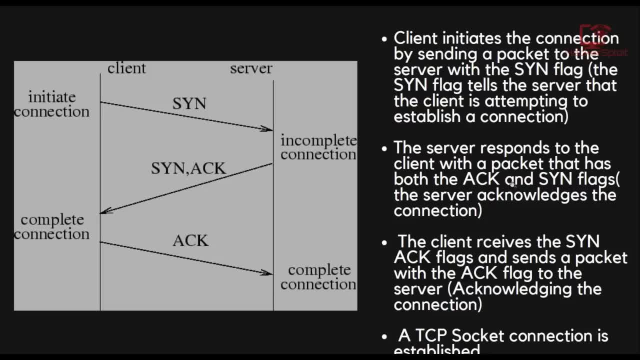 will then respond to the client with a packet that has the, both the acknowledge and the synchronized flags. all right, so aCK is is short for acknowledge. so essentially, the server will respond to the client with a packet that has the that has both the aCK or the acknowledge and the sin flags. 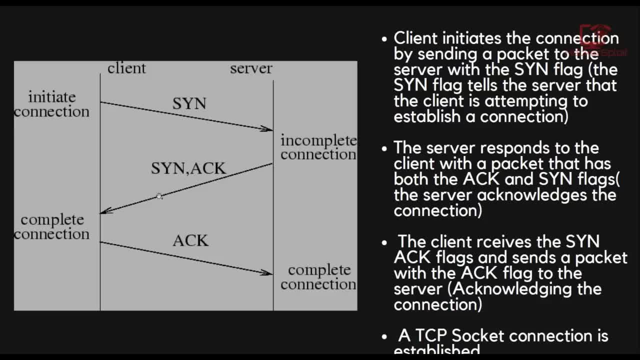 you Alright. so essentially, what's happening here is the server is going to send these, this packet with the two flags, the synchronize and the acknowledge flags, And what this means is that the server has is is acknowledging the connection. Alright. so then the client then receives the synonac flags. 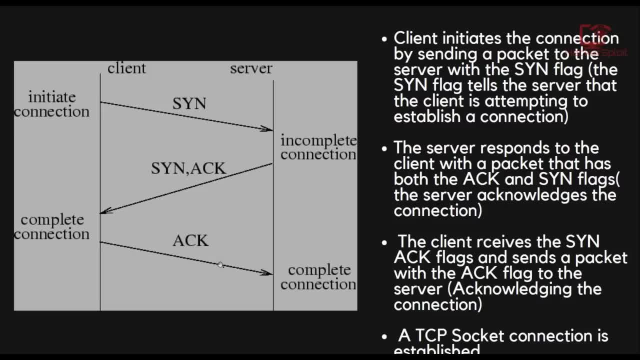 and sends a packet back to the server with the acknowledge flag essentially acknowledging the connection, And once that is complete, a TCP socket connection is established. Alright, so let me explain that really, really simply. Alright, so let's say you wanted to connect. 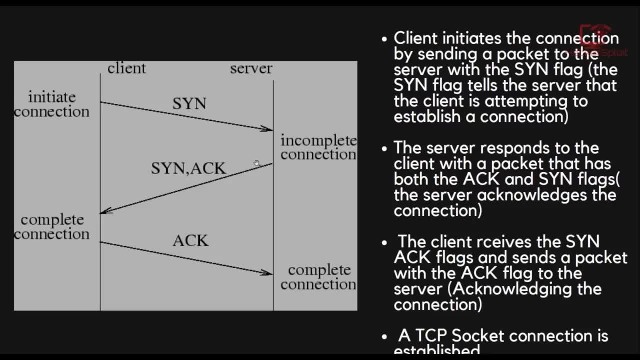 to a server. Alright, now the first thing you would do is you'd send them a packet with the sin flag. So you essentially what you're telling them is: hey, I want to connect to you, Alright, so you're sending them a synchronized flag. the server will then respond to you with the: 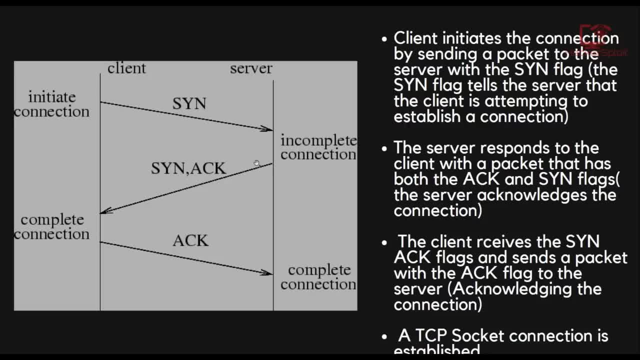 acknowledge and the synchronized flag with a packet with the acknowledge and the synchronize, the synonac synchronize flag saying Okay, we can connect to each other, Alright. you then receive the synchronize and the acknowledge packet. that you receive the packet that contains the synchronize. 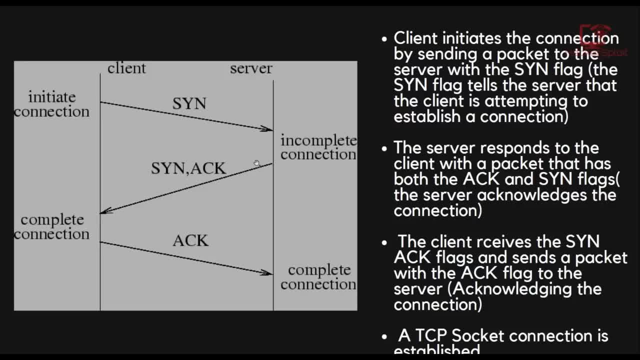 and the acknowledge flags And you send back to the server and acknowledge a packet that contains the acknowledgement flag, essentially acknowledging the connection, and a connection is created or completed. Alright, so moving on to the, to a simple diagram that I have here. I'm not sure you can. 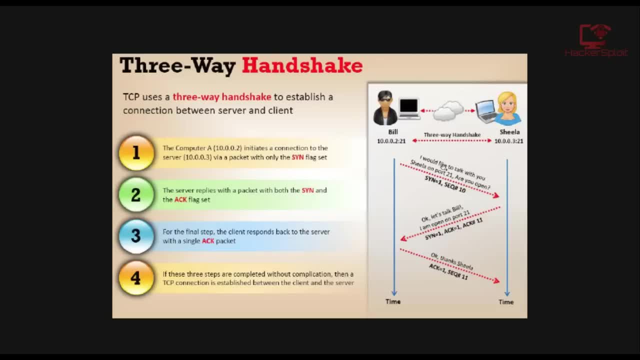 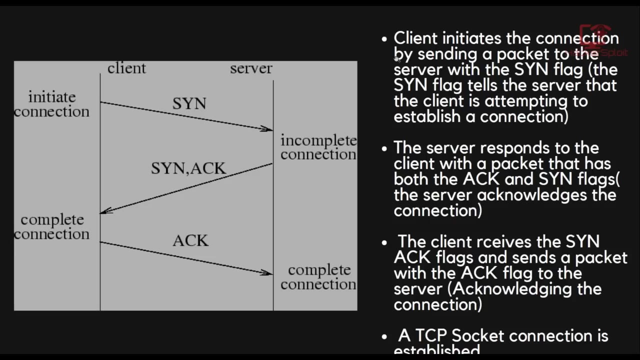 read it. If you can just look at how the connection goes through here, This is also a very, very good way of understanding how the the three way and check works when it comes down to TCP. you know, showing you how a connection is established between a connection and a server. Alright, so I hope you. 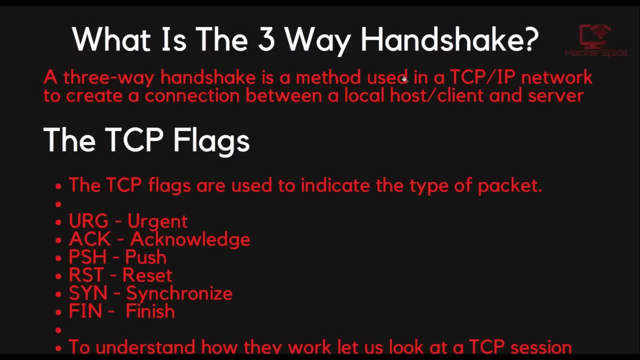 this was a very, very simple way of me essentially explaining to you, and you've understood, how the three way and check works, because it is very, very important, especially given the TCP flags, because we will be looking at, At actually using them when we'll be working with nmap. Alright, so that was how the three 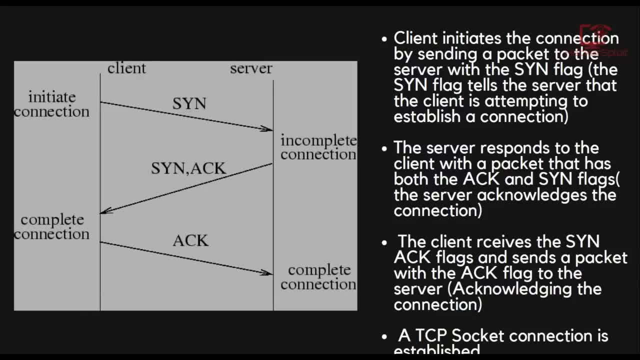 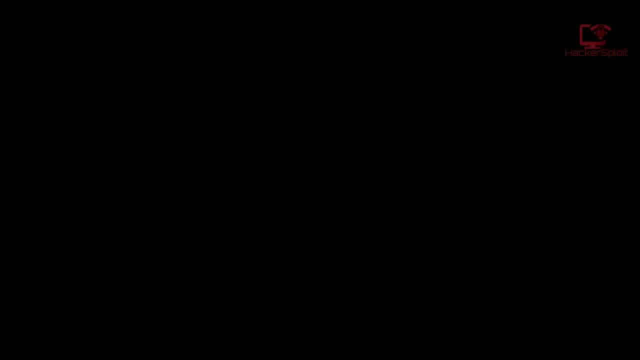 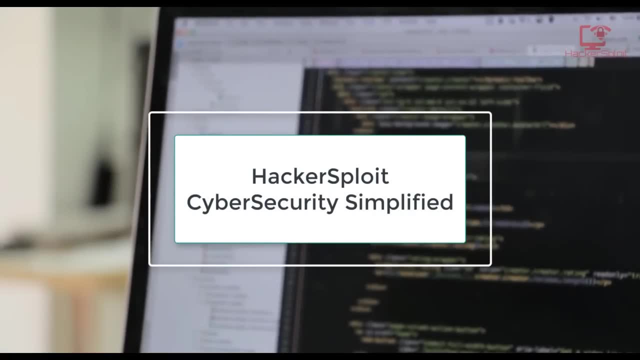 way handshake works and how a connection is established using the TCP slash IP. Alright, so that's going to be it for this lecture And I'll be seeing you in the next video. Hey guys, hack exploit here back again with another video, And in this video we're going to 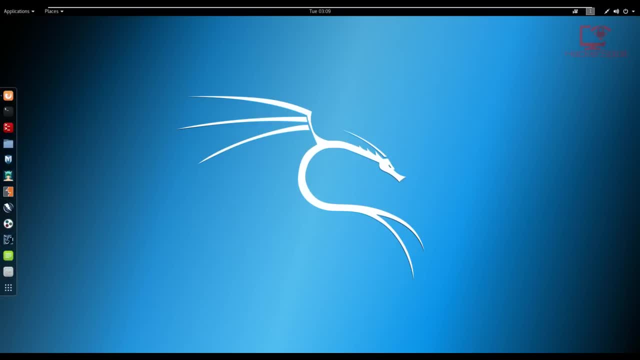 be looking at Information gathering with online tools Now, as I mentioned before, information gathering is the most essential step of a penetration test And it's really, really important to have a good idea of what your target is, how they're set up, what network they're running And if you're targeting a 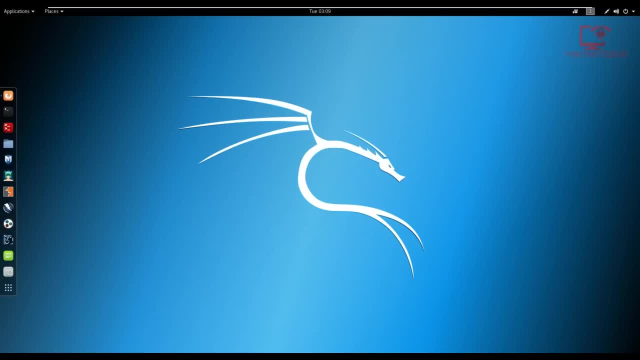 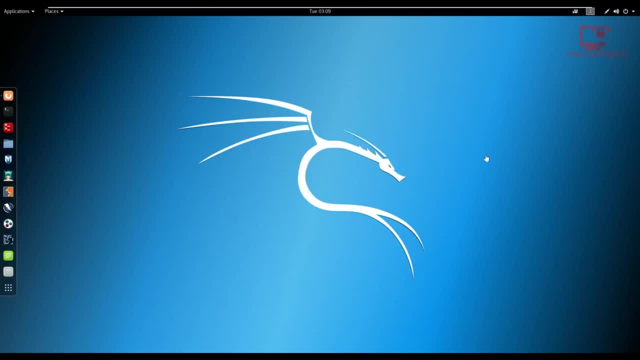 there a content management system running, etc. etc. Alright, so I'm currently on Kali Linux right now, And I'm going to be showing you online tools in this video, So you probably already know them, But if you do not, do not worry, they will be linked in the resources section of this lecture. 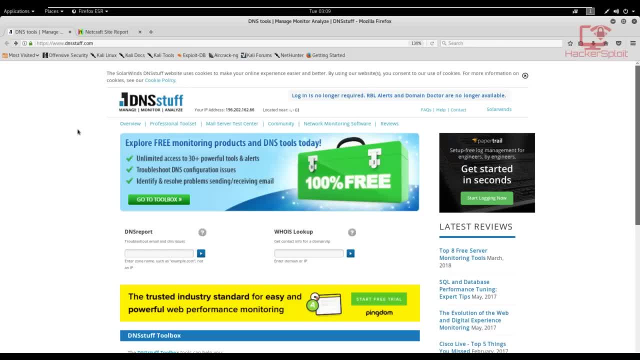 The first website that I'm going to be showing you, and that is my favorite, is dnsstuffcom. Alright, so dnsstuff allows you. dnsstuffcom allows you to enumerate or to gather information in regards to DNS, DNS reconnaissance, and obviously allows you to perform a who is lookup on your domain or IP. 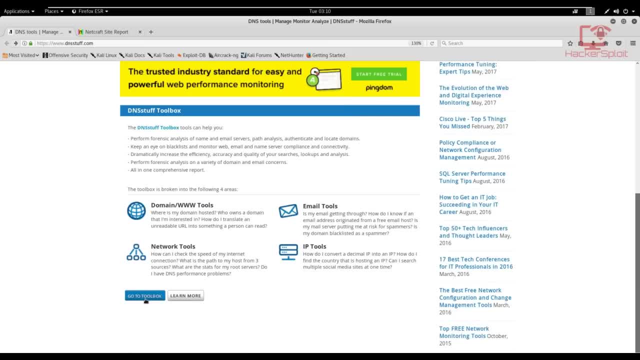 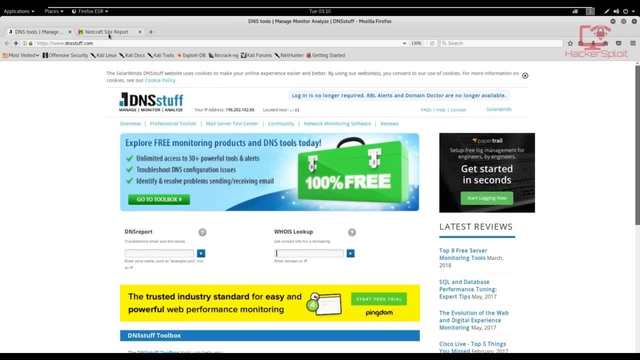 address: Alright. so the other great thing is thing is it offers a toolbox, which we'll be getting to very, very shortly. But before we get into into doing anything with the toolbox, let me show you the other website, which is net craft. Alright, so net craft, as you know, is a site. 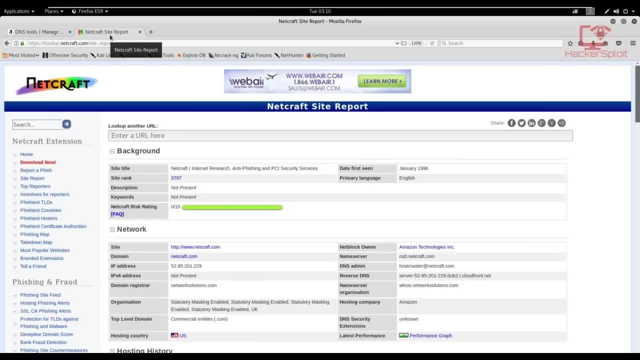 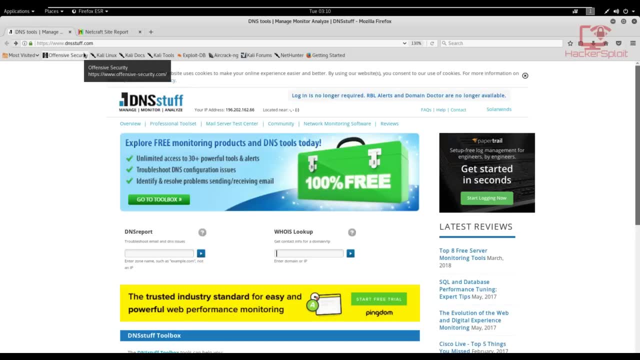 that's been there for a while now and gives you a comprehensive overview of what exactly is running on on the website, and we'll be looking at it shortly. Alright, so let's get started with DNS stuff Now. I'm not going to be going through everything because, again, it's pretty self. 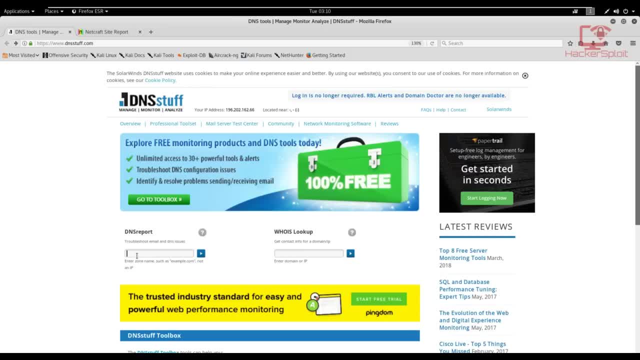 explanatory as to what each of these dialog boxes allows you to do. And when we talk about DNS reports, if I just type in my website right here, hsploitcom, it is going to generate some DNS information in regards to my website. Alright, so as you can see DNS report information, so give it. 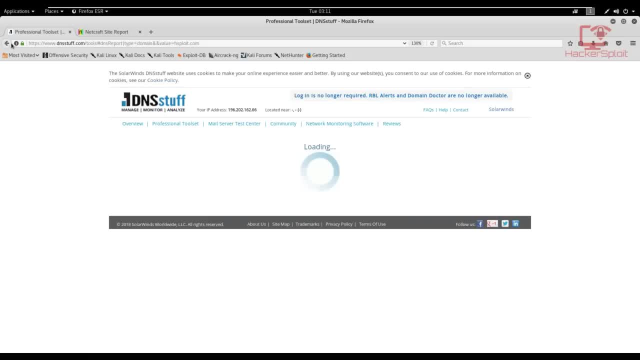 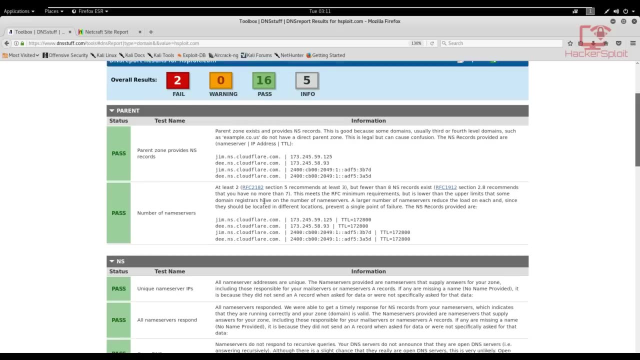 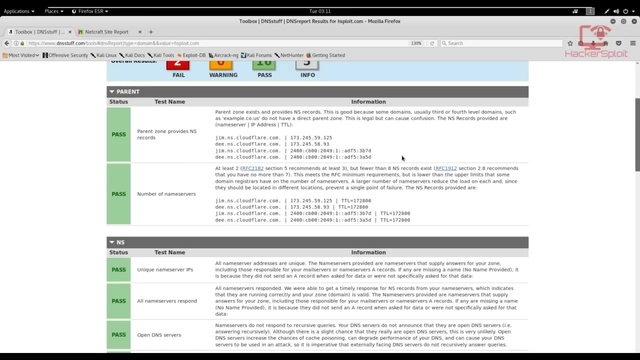 a few seconds to load, and just give it a few seconds to load here. it shouldn't take too much time. There we are Alright. so it's going to start giving us information about our parent zone DNS service which, as you can see, for my website, our Cloudflare, which protect my website. so 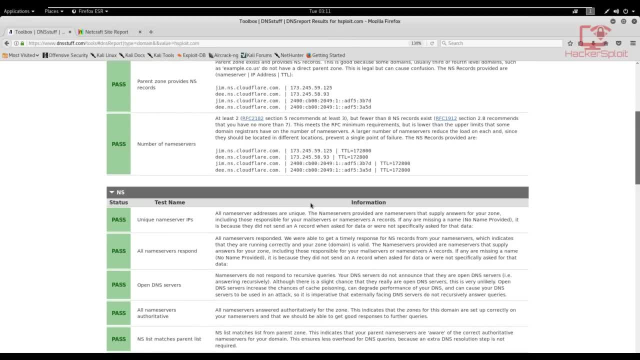 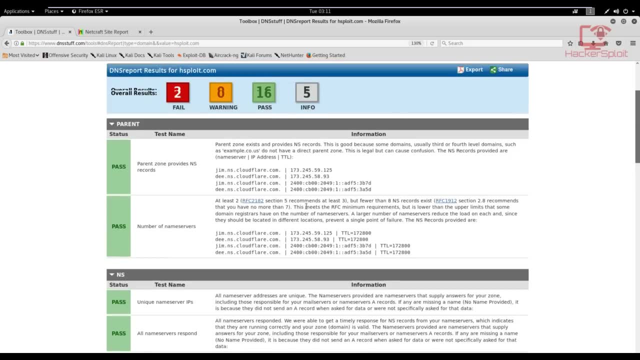 all my name servers go through Cloudflare And you have other information in regards to the open DNS servers being used, etc. etc. Alright, so that will give you information in regards to DNS So you can check that out for yourself. Now going 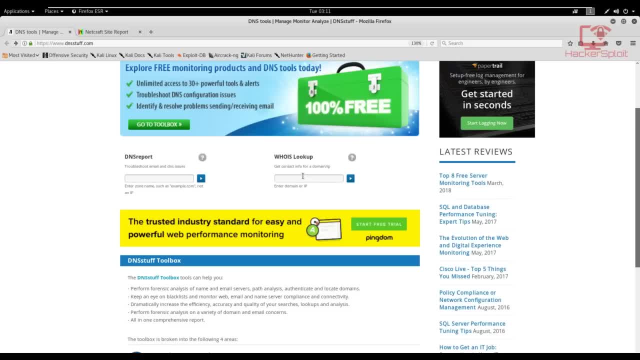 back here. if we look at the other scan that we can perform, which is the who is lookup, so we can perform a who is lookup for my website. So, as you know, who is lookup will generate all and any information in regards to a domain. Alright, so let me just click on that and it will generate. 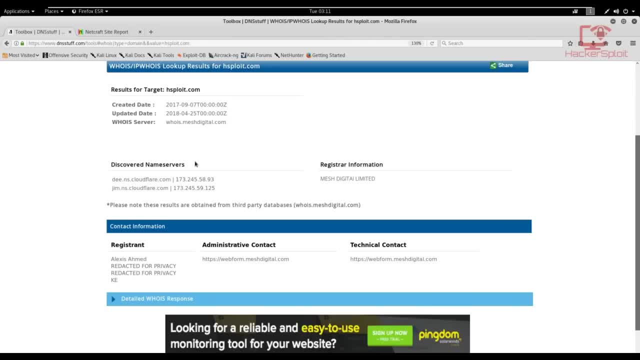 that information for us. So there we are. as you can see, the domain was created when it was updated, the who is server, from which the information was gathered, the name servers, which we've looked at before, which is Cloudflare, and the contact. 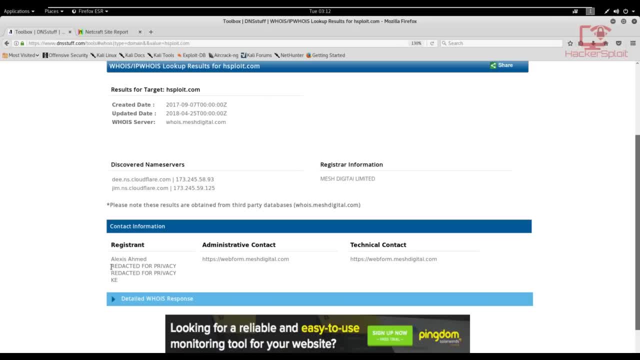 information. Now, as you can see, for myself, it'll give my name right here, But all the other information is redicated for privacy, And that's because I chose to have that with my domain. And this is also another important test. For example, if you're performing a penetration test on a 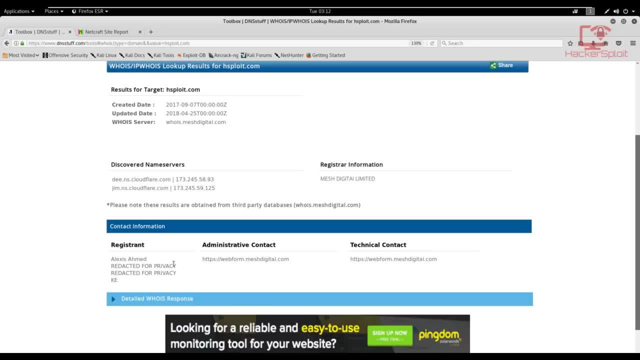 website and you've started with information gathering. usually, if the, if the person who registered the domain did not sign up for domain privacy, information like their contact details and address will be available. here will be open source and available to anyone who performs this scan, So you can see how valuable that type of information is. So once let me just 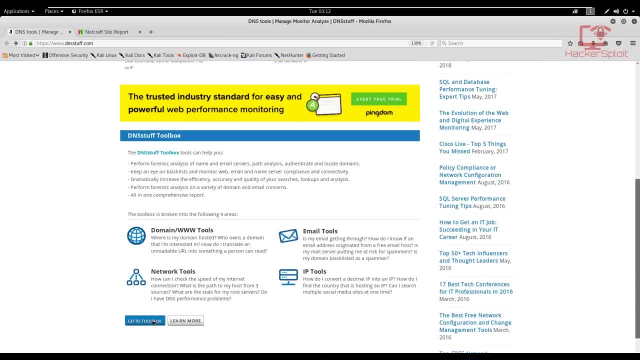 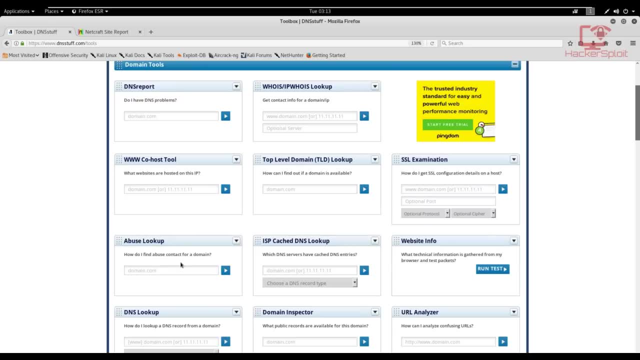 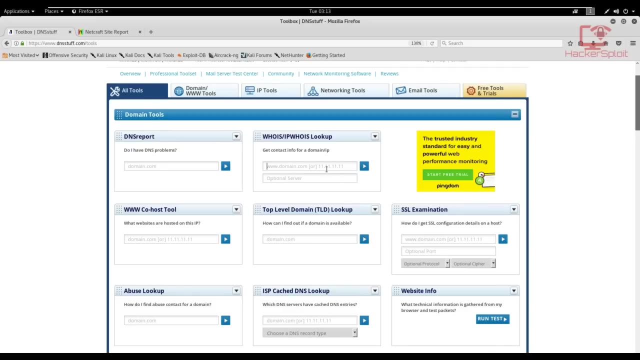 go back here And if I go to the toolbox, which is right here, the toolbox has a wide variety of tools that I'm sure you'll find really, really helpful. So if we take a look at them here so you can see, you can perform. you can check for DNS, for DNS report. you can perform. who is lookup on? 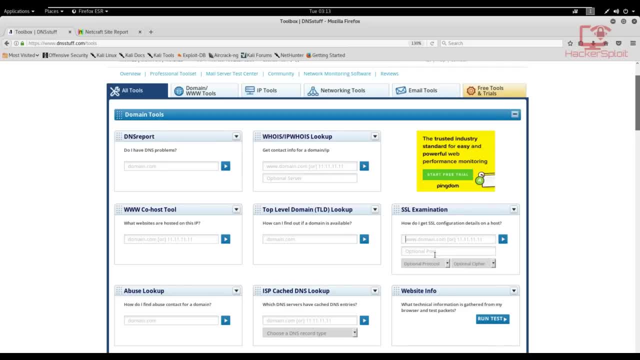 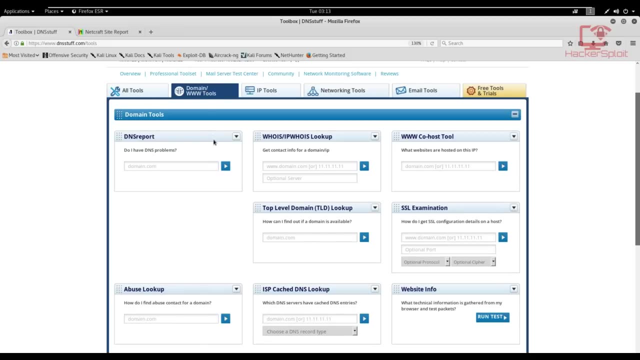 IP, who is lookup. you can look at SSL examination. you know, adding the port just to test whether the site has SSL And what certificate it's using. you can then look at the domain, the domain tools which will again will generate a DNS report if you wanted to. SSL examination- TDA, TLD- sorry you. 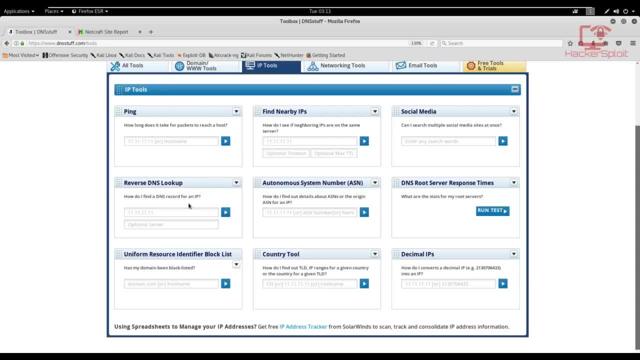 IP tools which are right here, which allows you to perform a ping, reverse DNS lookup. you have your country tool which will allow you to generate IP ranges for a specific country, etc. etc. So overall, dnsstuffcom is pretty much my go to place for all of the tools, essentially. 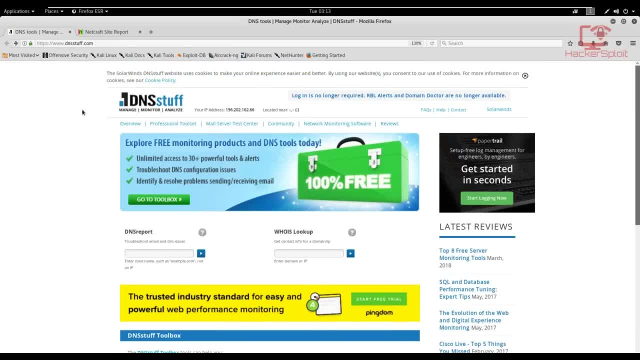 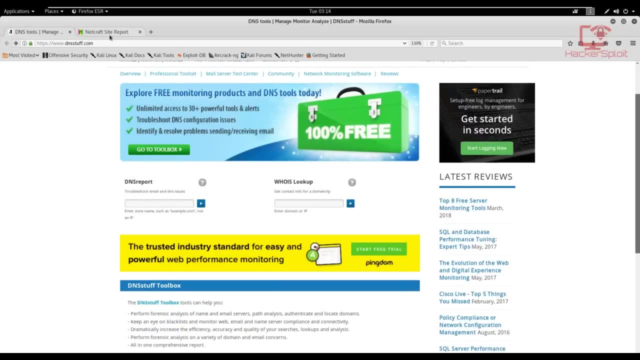 when I want to make, when I want it to be running autonomously or automatically. this is where I go, because it generates all the information that I need really, really quickly. Alright, now it comes down to websites. specifically, I use net craft. this essentially allows me to understand. 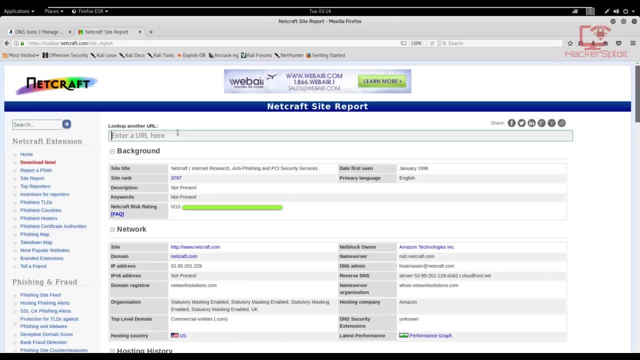 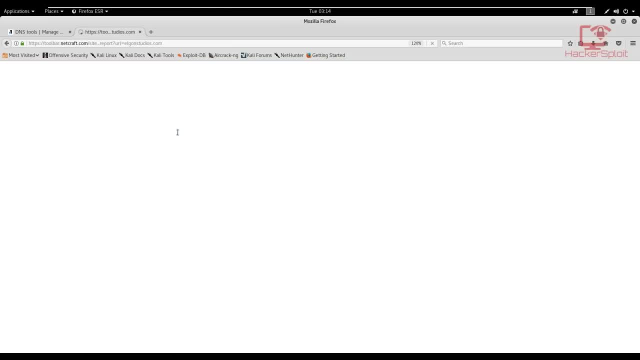 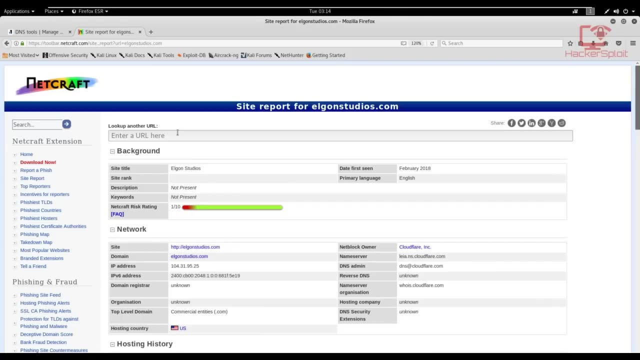 what is running behind a website. So, for example, if I was to run a simple site here like l gone studioscom, that is a domain that I own And again it's, it's. it's not I don't use it very often, But it's a site that I just happen to have. And again, all my websites. 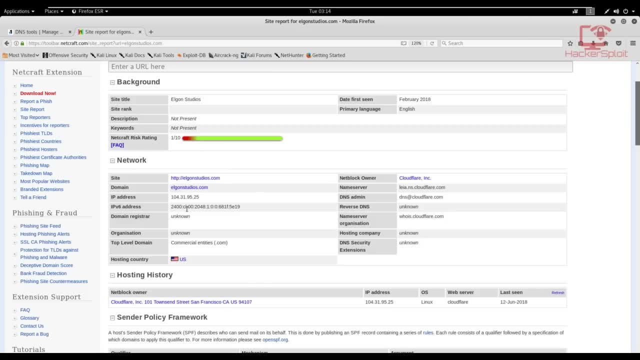 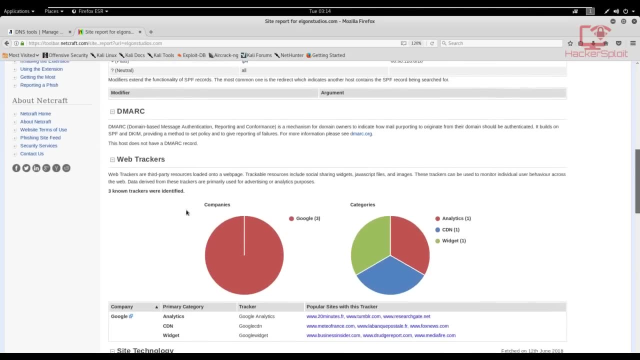 are protected- protected by Cloudflare. So it's going to tell me what IP address the website's server is being hosted on. All right, it's gonna tell me if we just go back down here into the web trackers. is going to tell me what web trackers have been identified. So for 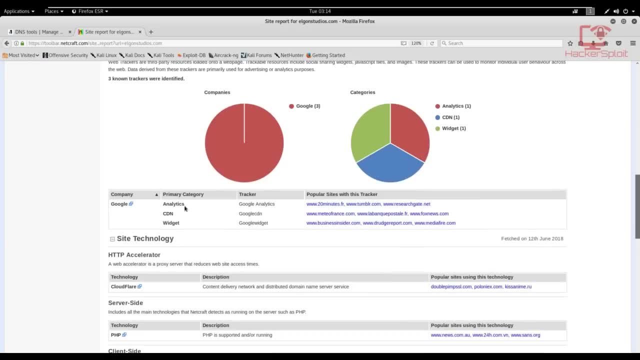 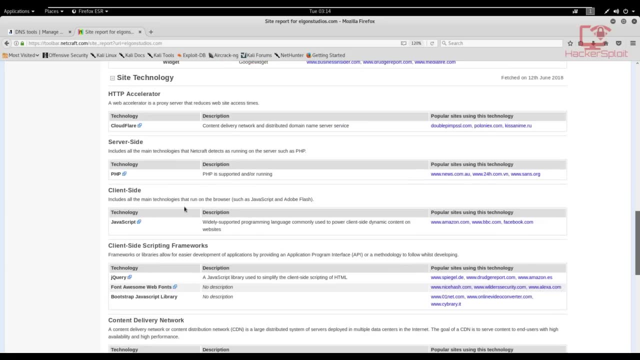 right now. you can see I have a CDN- Google CDN, Google Analytics- all important information. As for my HTTP accelerator, you can see I'm using Cloudflare. PHP is running on the website, So that will give you a good idea of what is running in terms of. 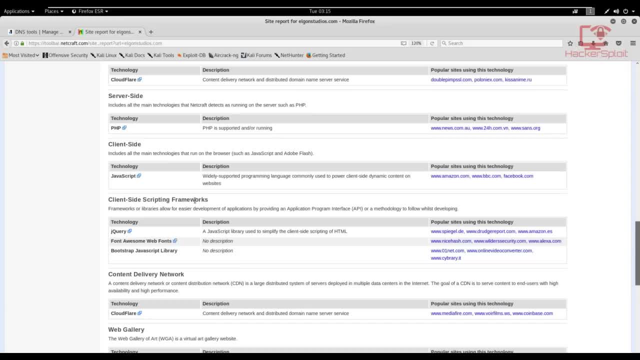 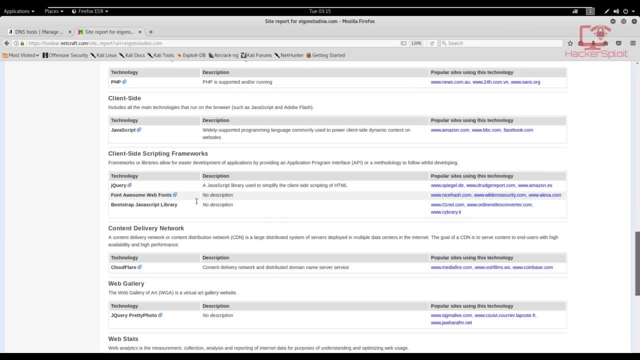 the server side technologies. you have JavaScript, you have your client side script in frameworks. you have bootstrap running, you have jQuery, So again, it's letting you know what frameworks are running on the website. So really, really awesome, whether you have a content. 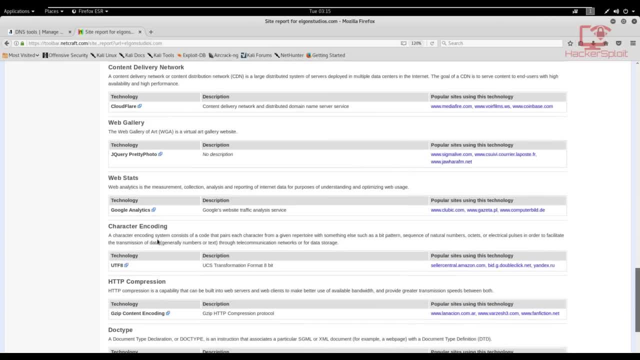 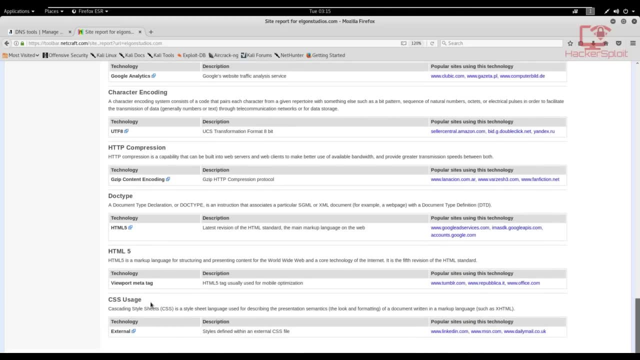 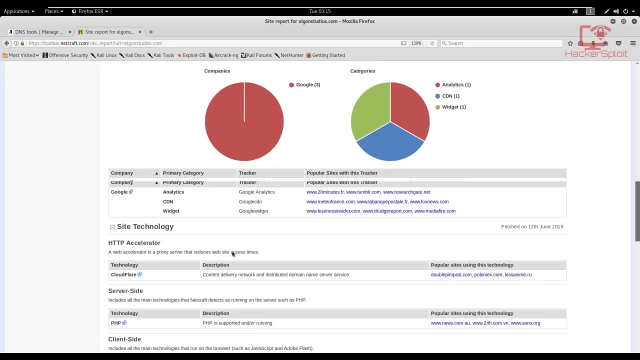 delivery network and you have web gallery, web stats, character encoding. let's see what. some more important information: HTML5, very, very important, and the CSS usage. no content management system like like Joomla or WordPress. So again, that's something that. 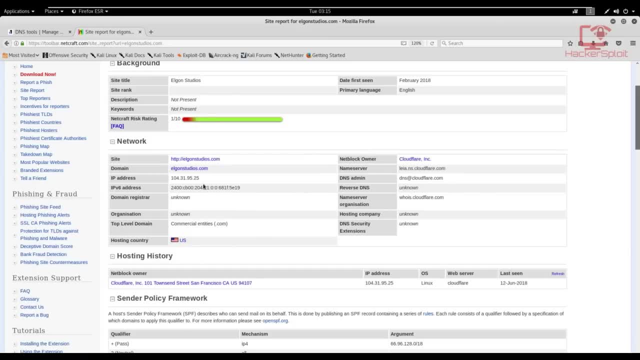 you might find really, really important. As for the IP address, I'll give you that right here, the domain registrar which, as I said, mine, all my websites are protected from, and you have your reverse DNS information, the DNS administrator. 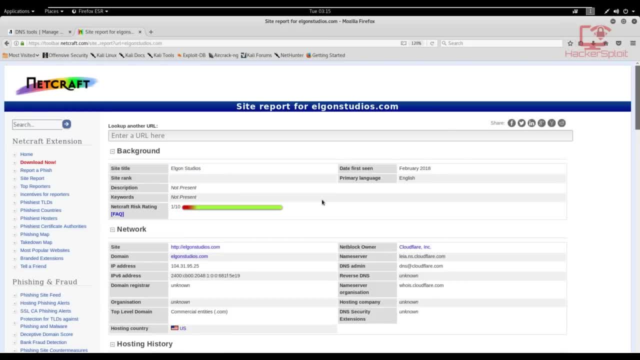 email, all that good stuff. So again, this is a fantastic website that allows you to check or to perform information gathering on your target, whether it be an IP address or a domain. All right, so that's going to be it for this video. In the next video, we're going to be looking at how to 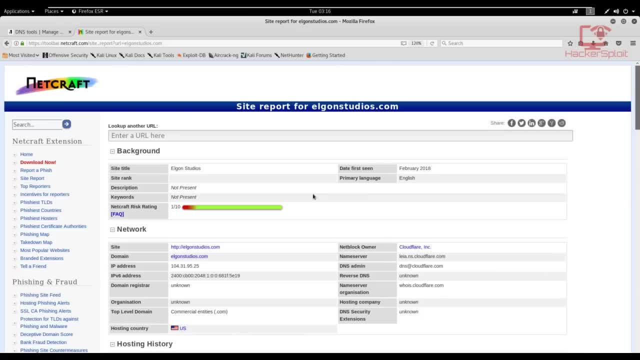 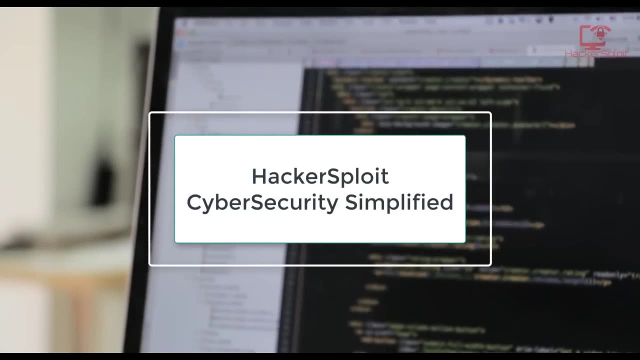 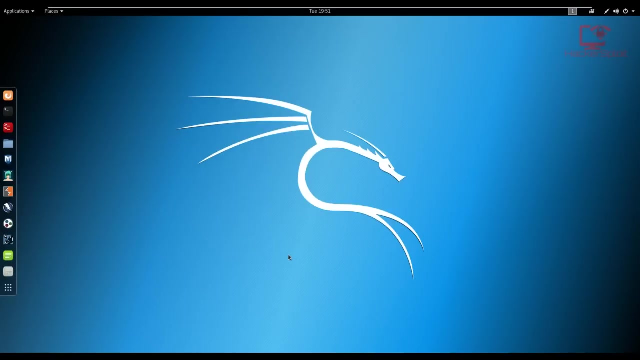 emails will with the harvester and how to essentially grab emails that belong to a specific domain. alright, so that's going to be it for this video and I'll be seeing you in the next video. hey guys, hack exploit. here back again with another video. in this video, we're going to be look at the emails using the. 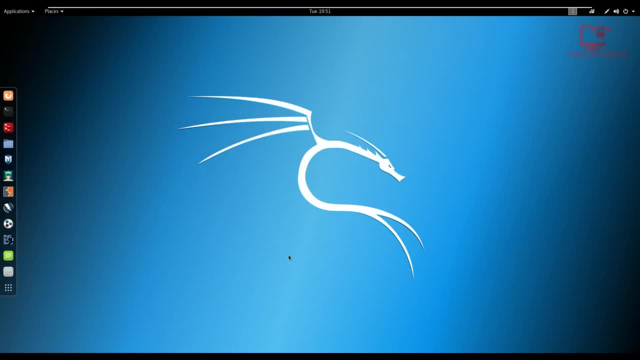 harvester, alright. so, as I mentioned in the previous video, gathering information about your target is very important, and one of the facets of this section includes and involves the gathering of email addresses that belong to a specific website, domain or company. alright, and again, this can be very 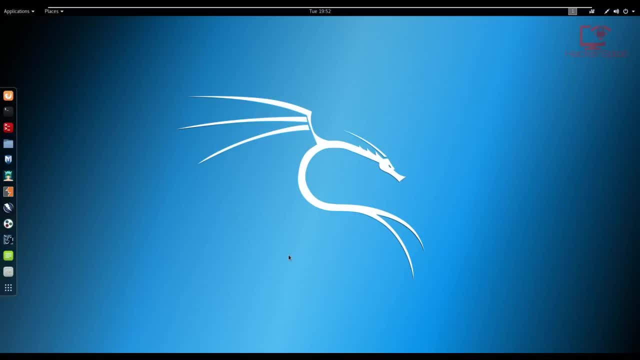 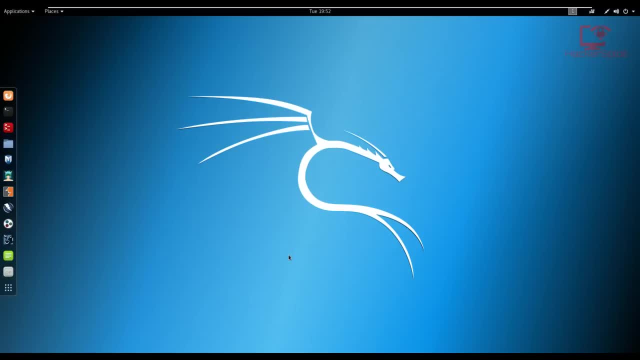 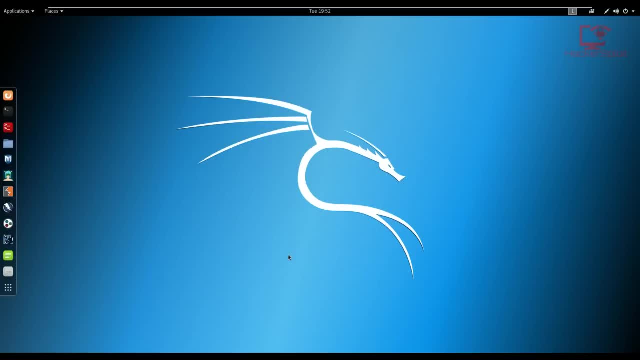 malicious software which, when executed on their computer, can give us, you know, access to that computer, etc, etc. of course I've made it really very simple, but you get the idea. having the emails of the of the employees of the company- employees working at the company- can be very, very useful because that they can 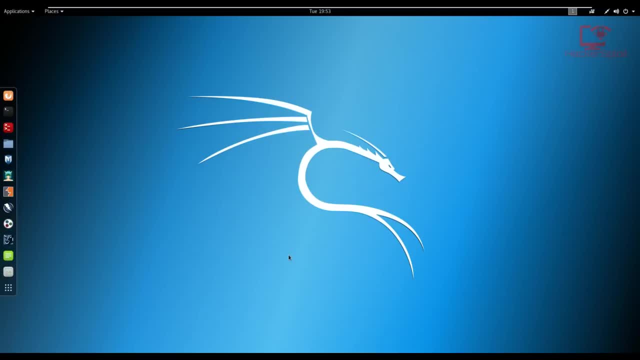 give us direct access to people who actually in contact with hardware there and software, alright, so let's get started. and by default at the harvester is pre-installed in Cali next, and any other in any other penetration testing distribution, so don't worry about that. so just open up your terminal and if you 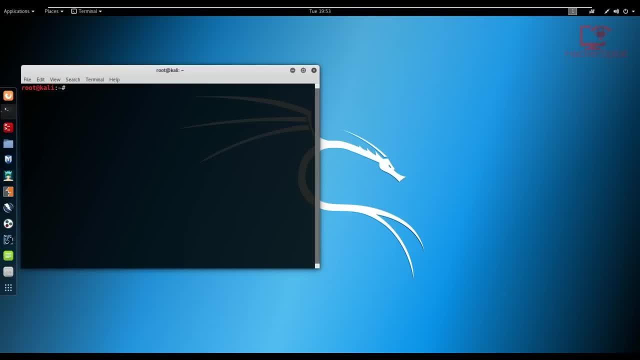 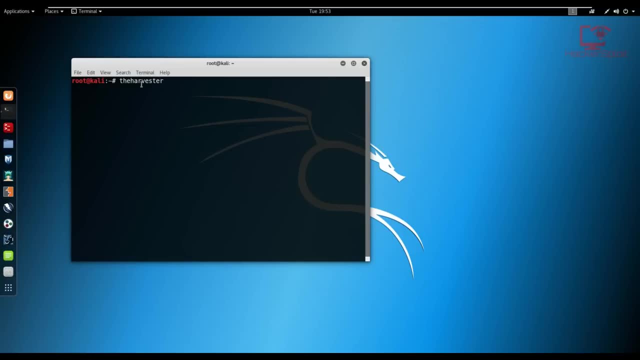 if you just look at the current status right now, you can see that if we, if we were to go it in the in the harvester- all right, so the harvester, like so and just type that in, you can see we're gonna have some options. that is gonna give us now the 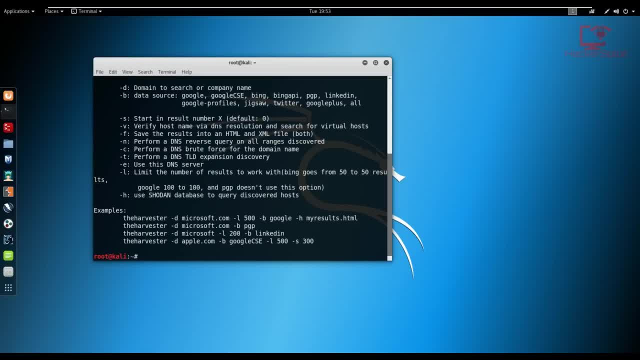 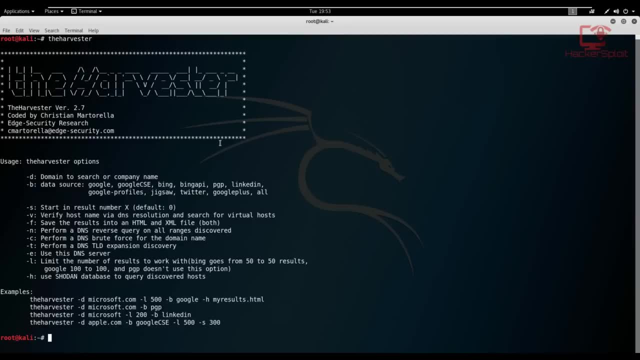 most important option that you need to understand here is this. all right, now I'm going to be going through all the options that it does provide. let me just expand this so you can see what's going on. all right, so the D- the D argument or option- is the most important one, because it allows us to specify a domain name or 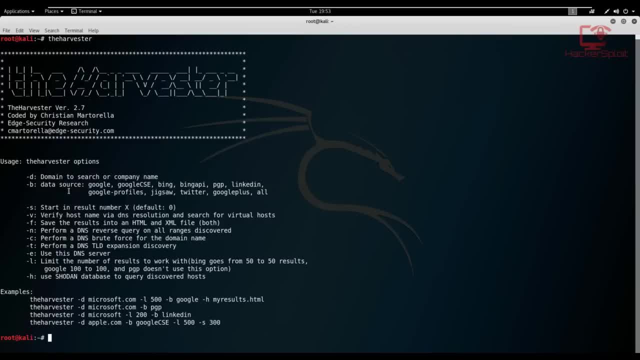 to search, to search for a company name. you then have your data sources, which allow you to search from different data sources. you have Google, you have Bing, PGP, LinkedIn, Google profiles, Twitter, Google plus, just being amongst the favorites. my favorites are Google and LinkedIn, and I'll explain. 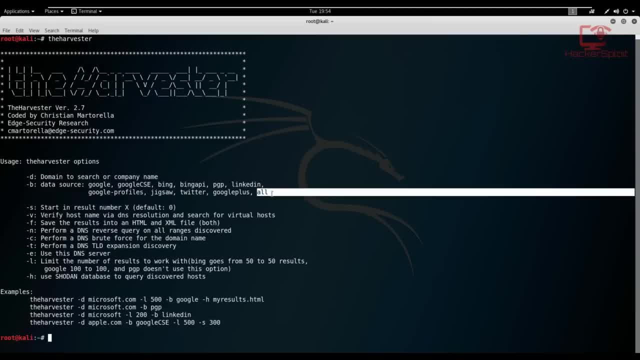 what that means in a second. and of course, you can also use all the data sources. all right, you can then use the other commands or options which are not go through right now, because these are more of an advanced option and have nothing to do with the actual searching. 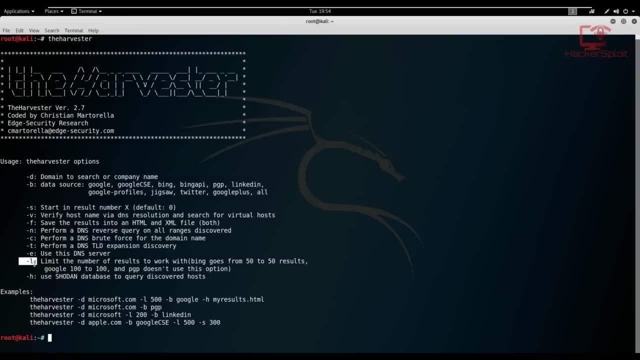 then have the limit Alright. so the L command or option allows you to limit the number of results to work with. So, for example, if I was to say 100, that means it would return 100 emails or 100 results of whatever it has been able to gather. Okay, so if we look at the examples here, 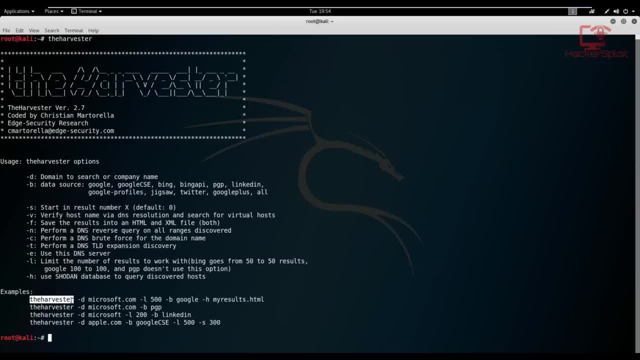 that is given us. you can see that we start up the harvester by typing in the harvester And we use the D command, And the microsoftcom website is then listed, which will use it as an example, and I'll also. I'll also show you another website. we then have the L command, which is the- the amount. 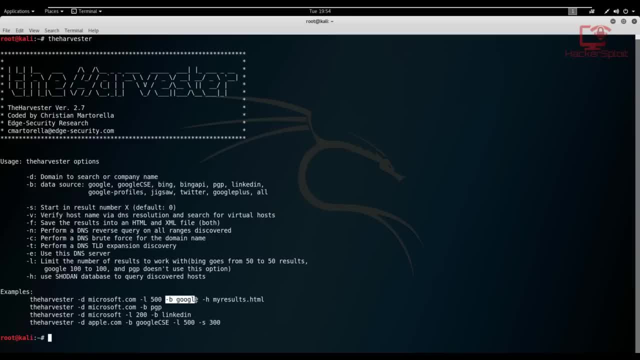 of results you want to be displayed, and then B for the data source And you can use the H command which, as you can see over here, allows you to use the Shodan database. So if you don't know what a Shodan database is, is Shodan is essentially a search engine that allows you to search for. 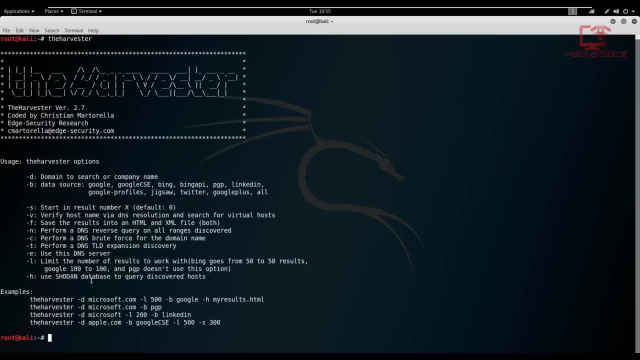 Internet of Things and essentially, a very advanced search engine, something that I've taken a look at later on in this course. Alright, but for now we'll keep it really, really simple. So what we're going to do is we're just going to start up the 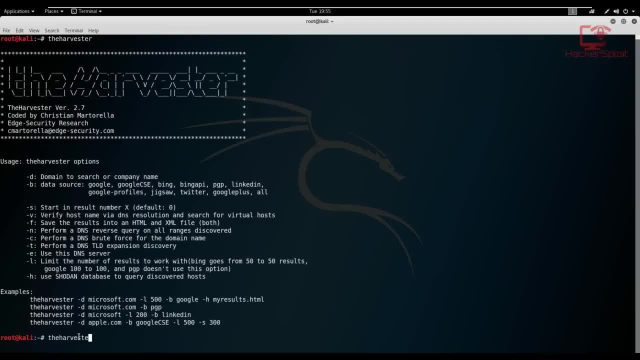 harvester, So the the harvester, and we're going to use D, and now we specify the domain or the company website. So, for example, we'll try bbccom, Alright, and we'll specify results of up to 100.. All right, just keeping it really simple. Again, you can change this to whatever you want And the 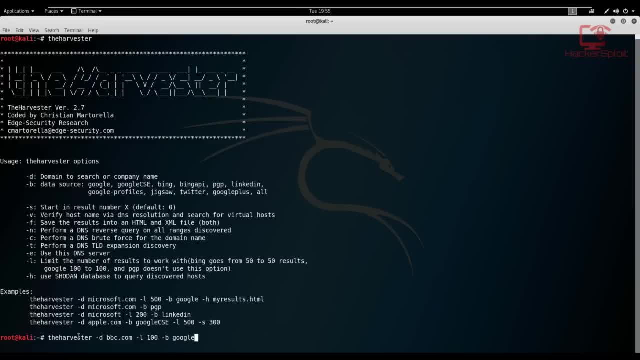 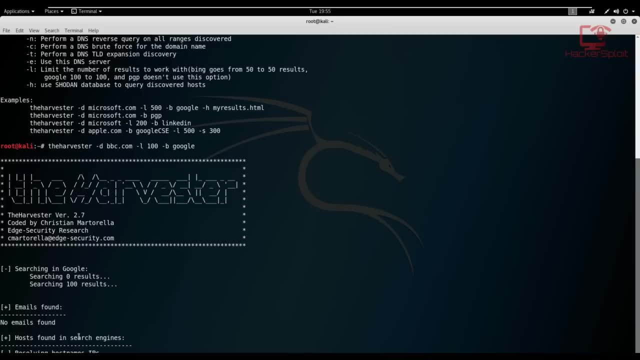 data source being Google, Alright, so we're not going to specify anything. So let's hit enter And let's see what results were the harvester is able to get. Give us okay, so you can. just going to start resolving hostnames And there we are. we were not. 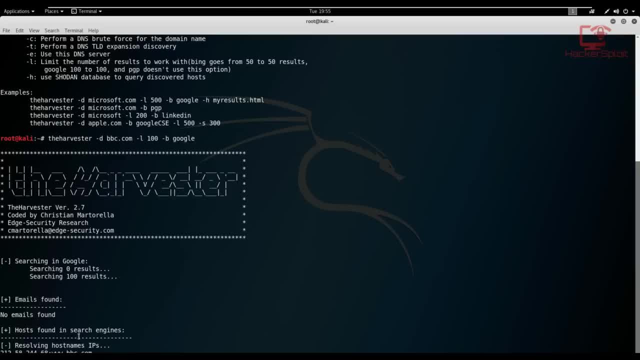 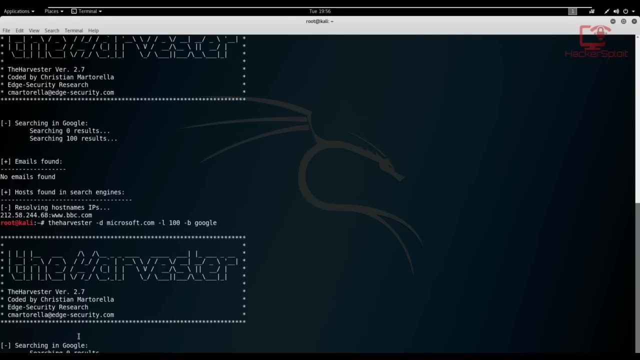 able to find have to find any emails. but that's fine. We'll try it again with another domain. Let's try. Let's try in Microsoftcom And let's see if we're able to gather any types of emails here that we can. that can be helpful to us. Alright, so we were able to get one email here. 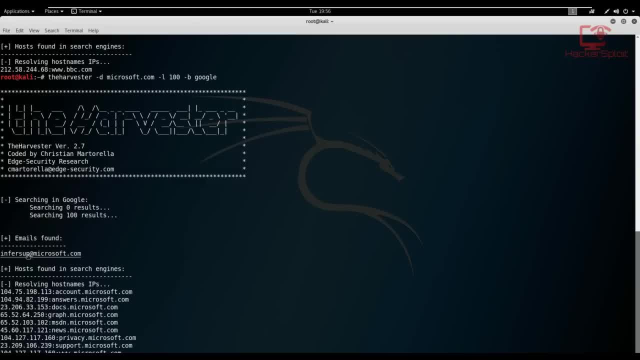 And, as you can see, we have. we have the info sub at Microsoftcom. That's pretty much a contact email that allows outsiders to contact Microsoft. nothing important there. you then have the hosts that it was able to find, So you can see. 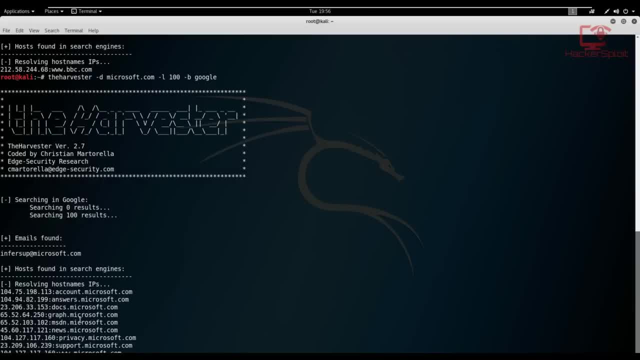 that we have the sub domains. here you have your newsmicrosoftcom with the different IP addresses, which again is extremely helpful when we're talking about information gathering. Okay, so let's try one more website, just to see if we can get some more emails. Alright, let me just 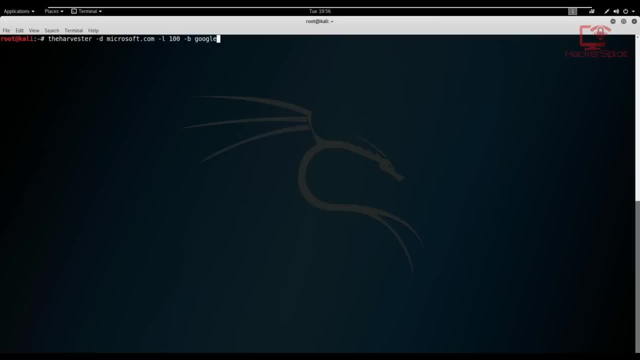 think of one. Let's try redditcom. All right, So the harvester and we'll try redditcom. Like so and let's hit enter. Let's see if we're able to get any emails from readycom. All right, there we are. So we can see that we have press at readycom, am a at readycom and licensing. 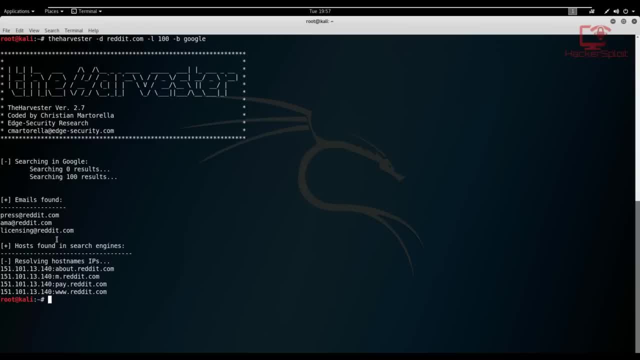 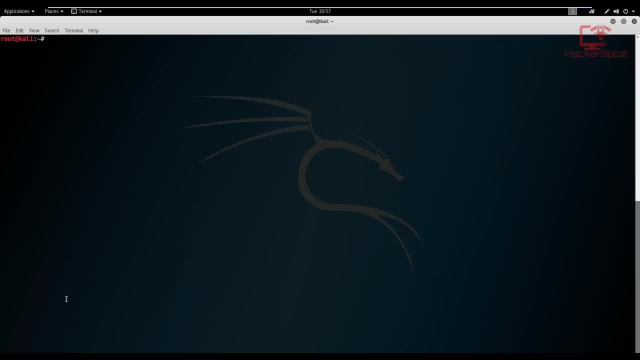 at radiocom. Again, not very, not very special, nothing special we're able to find over here. So let's try another one. Alright, just one more, just to see if we can get one result with a lot of emails. 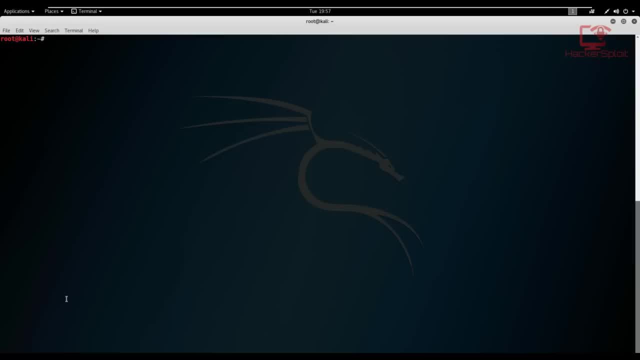 Of course, with your. if you're performing a penetration test, then any other client website you will. obviously, if you're able to find emails, then again that is something that you can report as well to your employer. Alright, so if we run this command again and let me 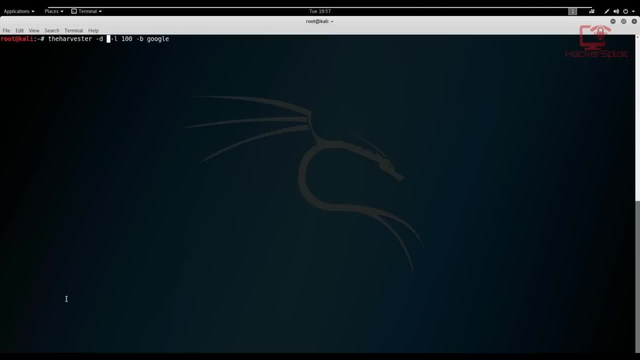 try one of my websites. Alright, let me just try my website here. My website should show no email address gathered because I have actually protected myself from it. So, as you can see, I only have one domain, which is HS ploycom. 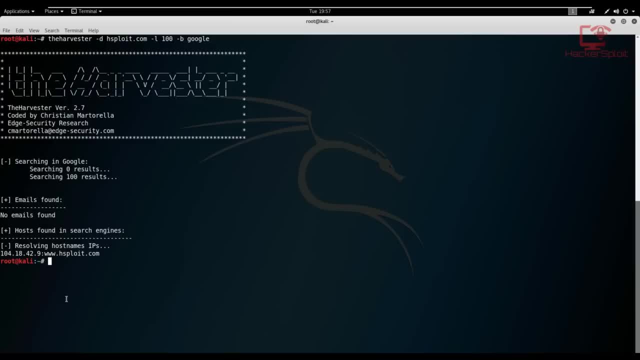 And no emails were able to be found. Let me just try and see if I can find a website here that we can actually use. that should have something that we could use. Let me just think here We can try one more. Let me try. 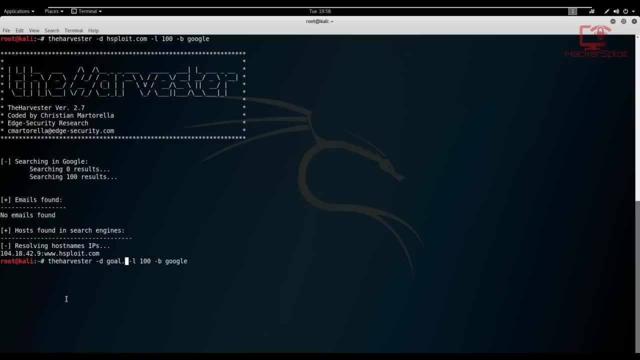 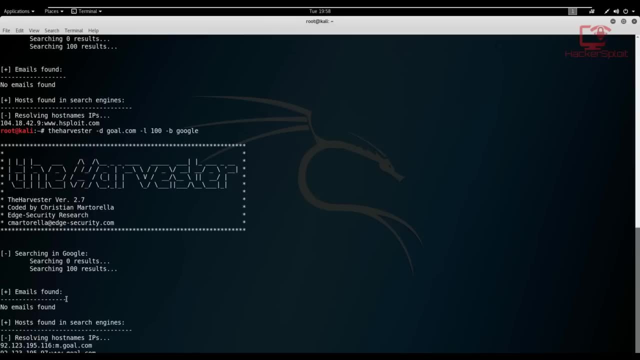 goalcom. All right, goalcom is a very decide that I visit often. It's a football website, So let's see what emails we're able to gather here. nothing at all, But anyway, you get the idea Performing this on your, on on your. 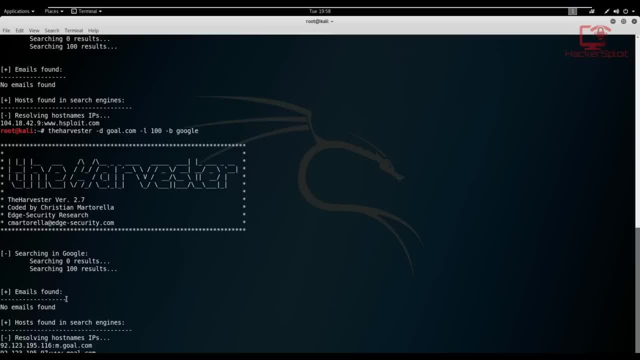 website, or your employer's website, can be really helpful, And it'll give you insight as to what attackers can actually access when it comes down to email addresses for customers or employees, in you know, for employees working for that company. That being said, that's going to be it for this video, and I'll be seeing you in the 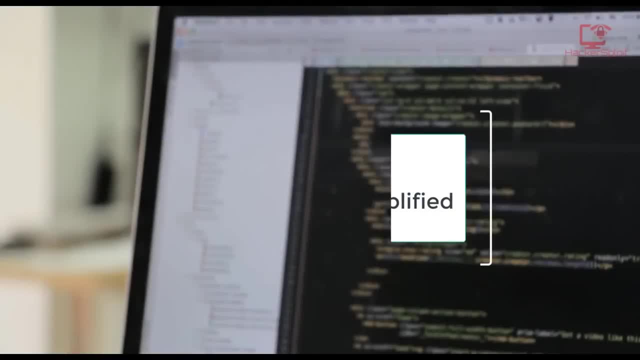 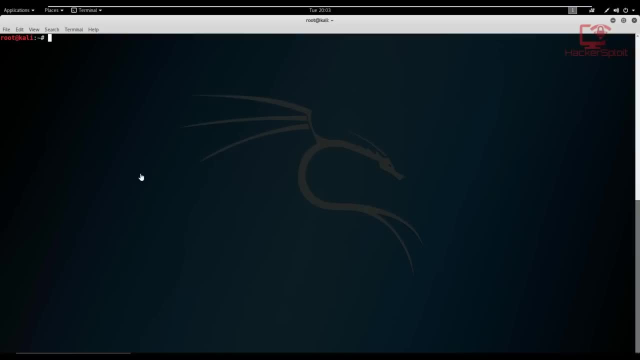 next video. Hey guys, Hackers ploy here back again, And with another video, and in this video I'm going to be showing you how to perform a Whois lookup on Kali Linux. All right, So when it comes down to, 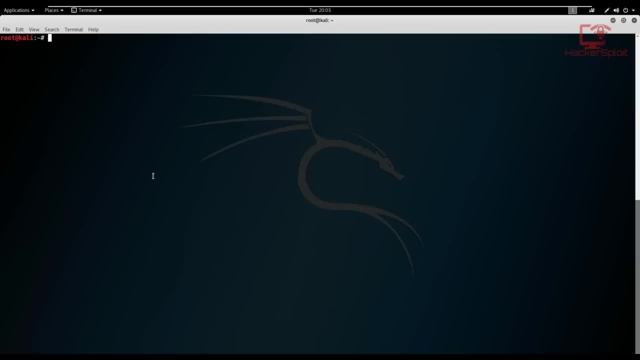 gathering Whois information. as I mentioned in the previous video, we looked at how to gather Whois information using online tools like dnsstuffcom and the netcraft toolbar. Now, again, those are very, very good tools, But again, it is also very important to understand how to perform this information scanning. 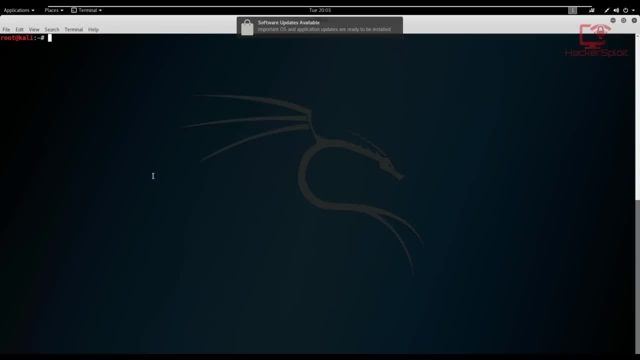 techniques on Kali Linux or on your pen tests operating system or distribution. Alright, so it calsea next. it's really very simple, And if you're not understanding right now what Whois lookup really is or what it deals with, It's really very simple. Whois lookup? essentially you asking, you asking the internet or you asking the. 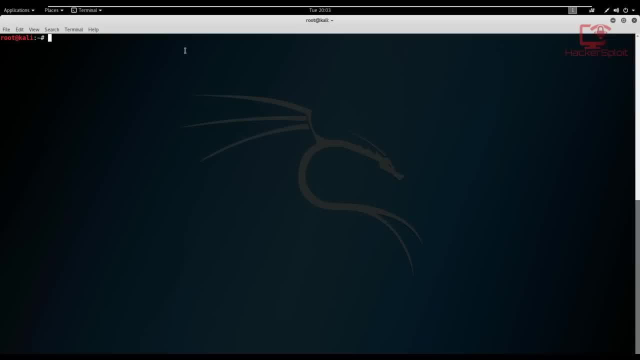 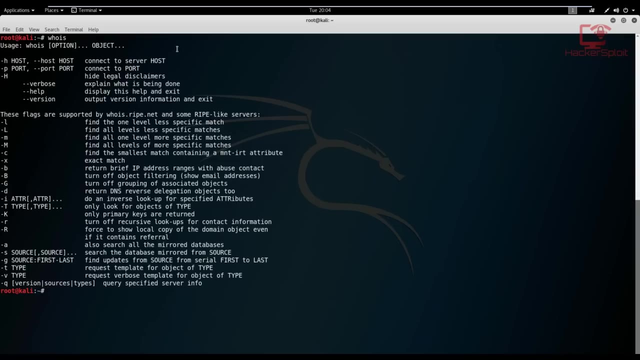 online database or any database you're essentially looking up, right? So you're saying who? who is this domain? Who is this domain registered to? can you tell me some more information about this domain? All right, So to get started, all you have to do is just type in the who is information. Alright now. 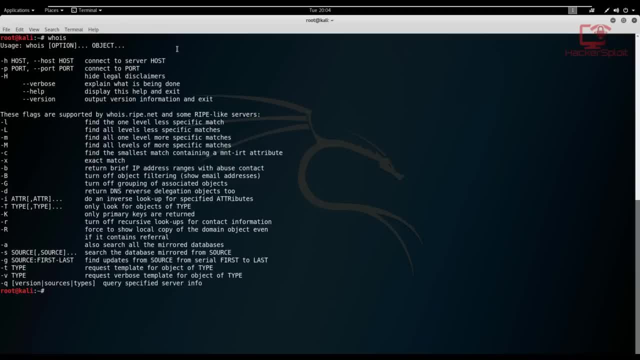 this is a very, very advanced tool, And the reason I'm saying that is because I'm not going to go through how to use it completely. I'm just going to show you how to get the information that you're looking at, or the information that your most, that is, the most interesting and information that is. 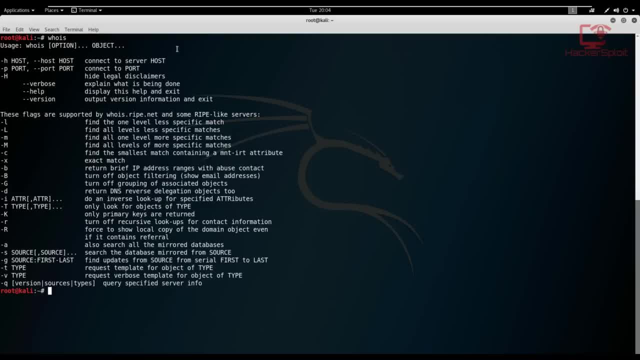 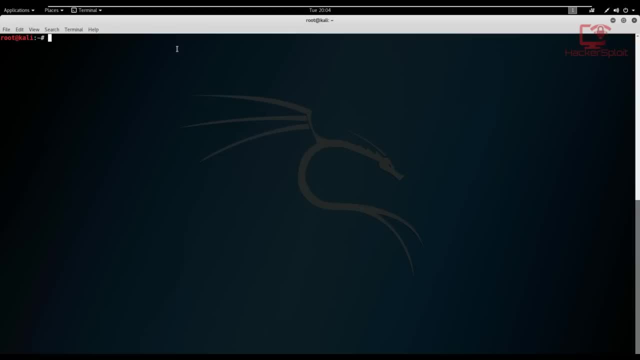 going to help you in your penetration test. Alright, so let's say you have a domain that you want to perform a who's lookup on and you want to get an understanding of what exactly this website. what's going on with this website? you want to know what, what hosting company it's? 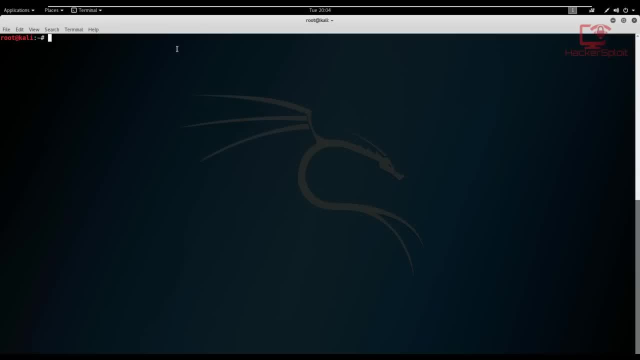 registered to. you want to get some information about who registered the domain, etc. etc. Alright, so to do this, we just type in who is and I'm going to be using my website. alright, so hsploitcom. Now I already have security features in place, which is again something. 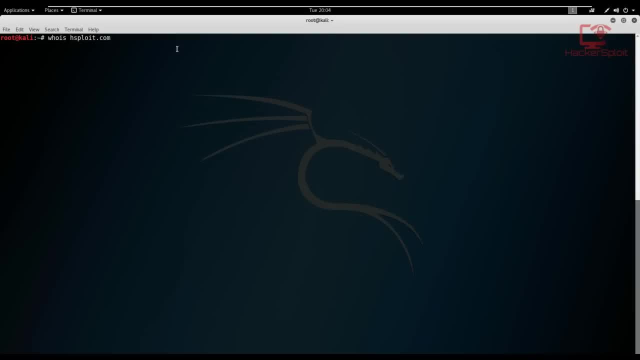 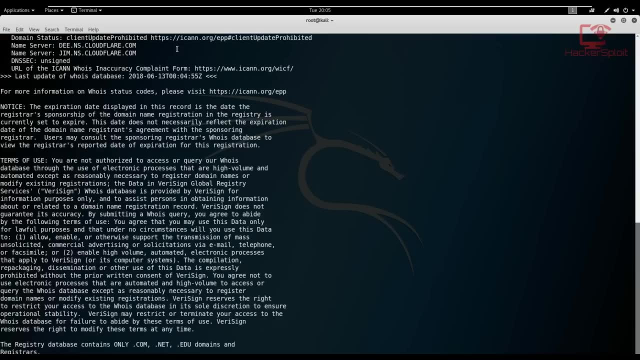 that you should be taking away from this is that again, you can protect yourself from E in information gathering scans like this, And I'll show you that in a few seconds. So if I type in who is and my website, you can see the scan is going to complete, And if we just scroll all the 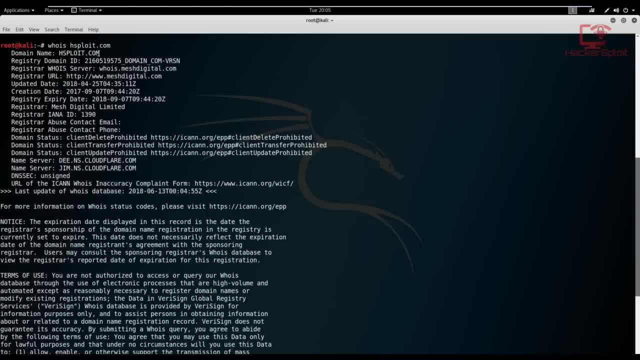 way to the top. we have the results here. Alright, so it's going to tell you your domain name, which is hs, hsploitcom, the registry domain, the registrar, who is server, that's really not important- The update date, the credit creation date and the registry expiry date of the domain. 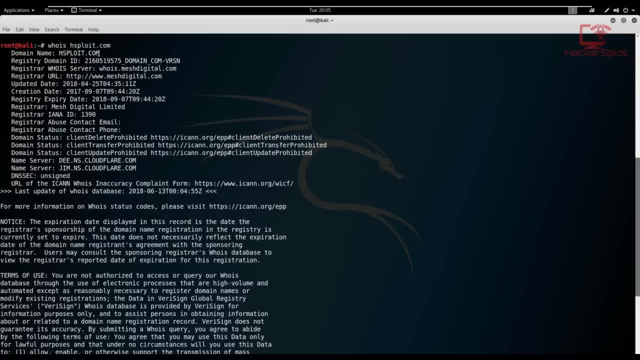 is very important, So you can see when this domain was was bought, when it was active, when it was updated and when the expiration date is all right. you then have the registrar abuse contact email and phone, which is again I have blocked, just to. 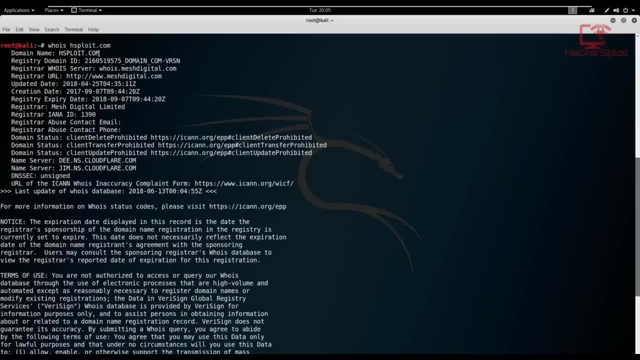 give my website privacy and then it's going to give you additional information, like the name servers, which will give you a better understanding of what type of what type of system is running behind the website and is is, if any, is there any protection system in front of the website Or is? 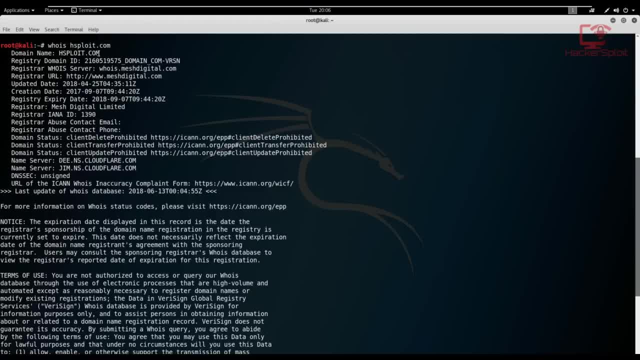 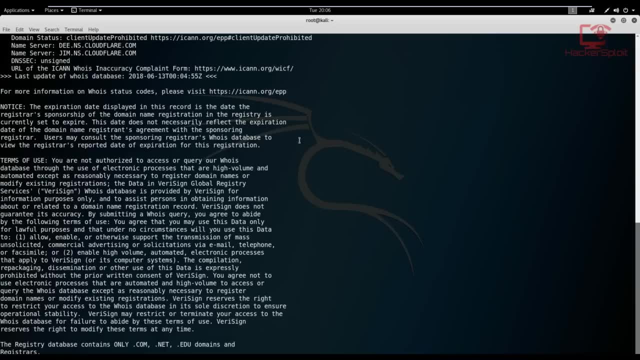 is there any firewall that is blocking or is protecting the website? That being said, that is how to perform a simple who is lookup with Cadillac. It's a very, very important skill to know because it gives you an idea of what the domain, what's going on with the domain. If I just 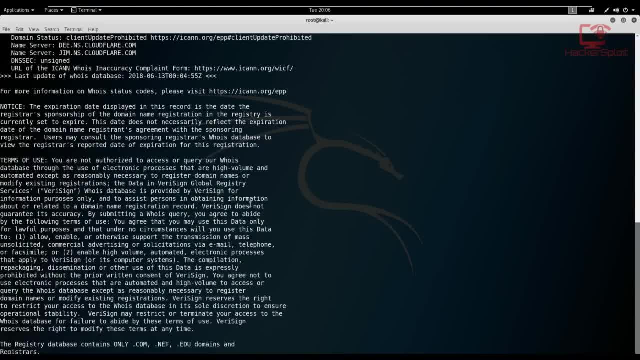 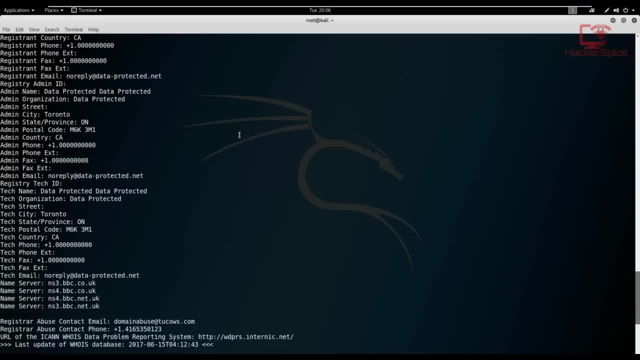 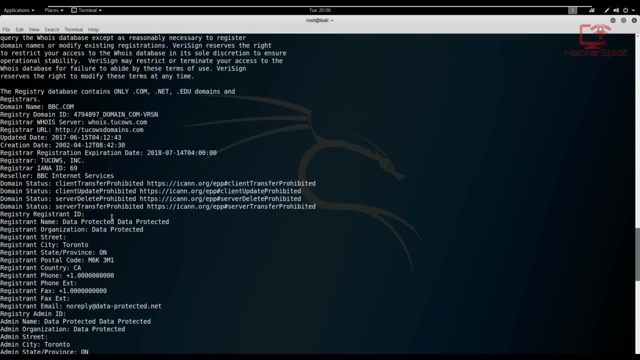 type in again who iscom here and I use bbccom. it'll give us information in regards to the bbccom domain And, as you can see, we have much more information now And this is because it is a fully legal. you can see that we have the domain name, you have the registrant name, the registrant. 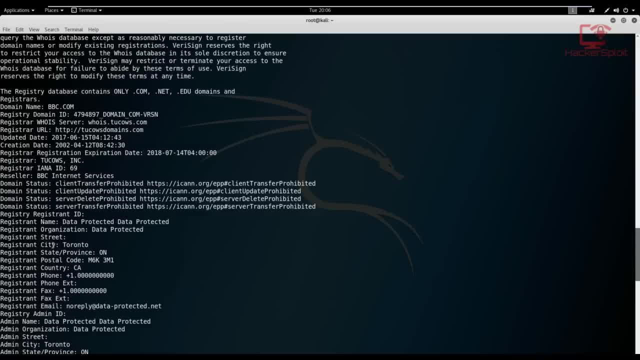 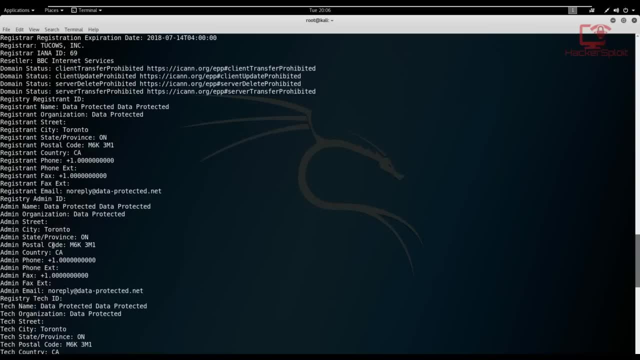 city. so we can, we have an idea of what's going on here. So you can see that that this was registered to a hosting company in Canada. Alright, so we've got that idea. we then have the admin phone, you have the admin email. right here you have the province, all of that good stuff and the 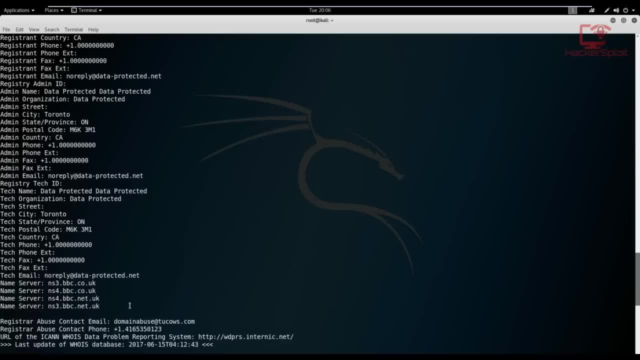 name servers, which are very, very important. Alright, so that is how to perform a simple who is look up And, as you can see, it's really very simple And you can switch from domain to domain, just gathering in enough information about your domain before you actually perform any type of. 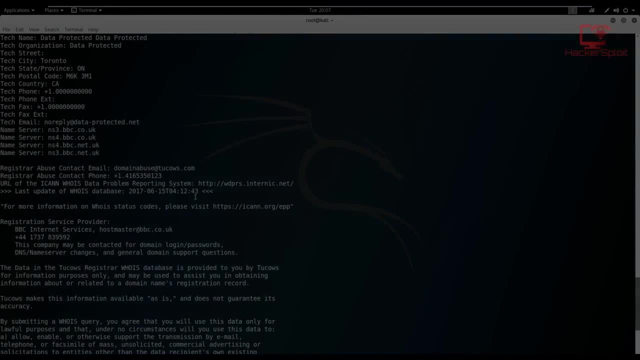 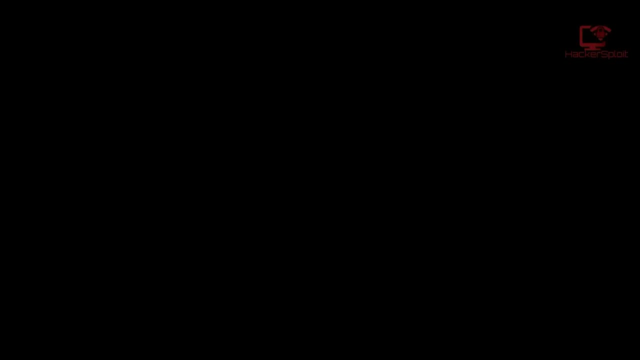 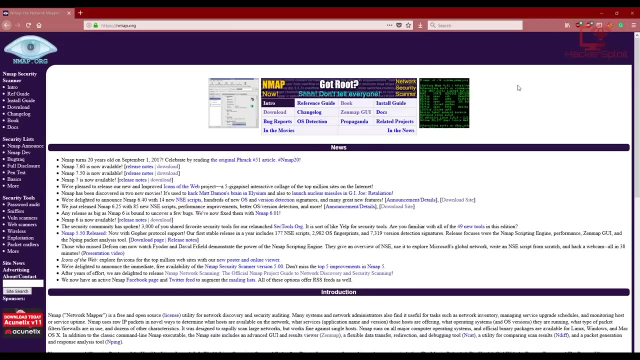 attack on your target. That being said, that's going to be it for this video, And I'm going to be seeing you in the next video. Hello, Evan, and welcome to this lecture. In this lecture, we're going to be downloading and installing and map on Windows. Alright, so before we get started, 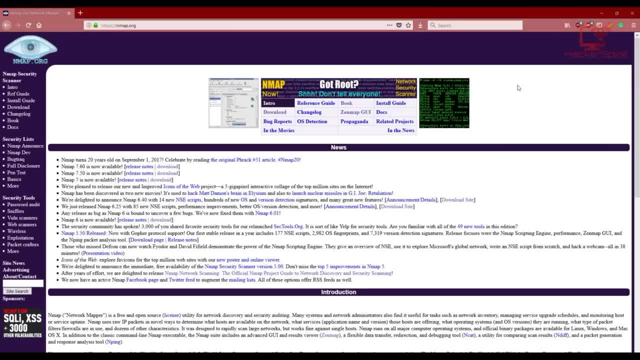 I just want to point something out Now. n map from the beginning was mainly developed for Linux or with Linux in mind. Now, over the years, n map has actually focused down on Windows and I'm updated the n map version or binaries for Windows. 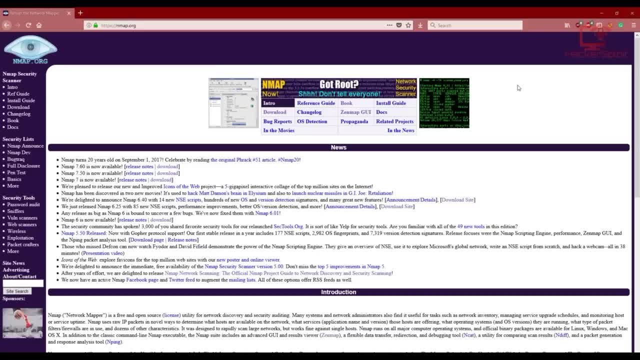 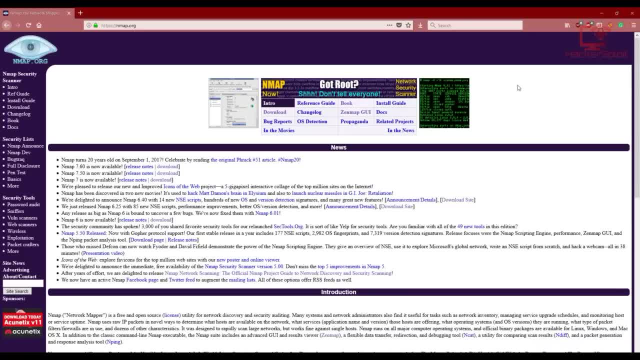 exactly the same way. Alright, so let's get started. So the first thing you want to do is, obviously, we need to get the file downloaded, or the setup file downloaded, And in order to do that, you just want to open up your browser and head over to n maporg. Alright, so it's really very 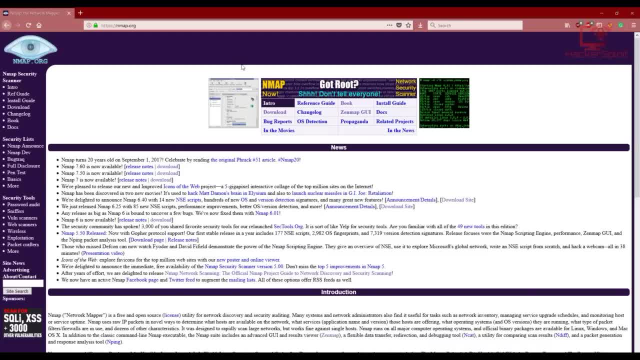 simple, So n maporg. that's the website And it's a very fairly really simple website And in order to download it, just go ahead to this to the. you can choose to go through the download page directly Or you can just go to the n map release notes right here. 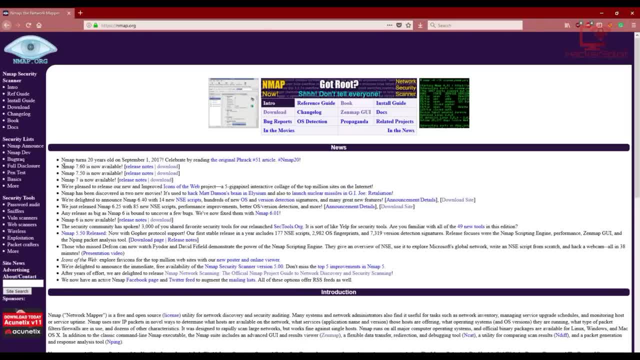 or the release, the release log that states that the latest version 7.60.. As of this recording, but any changes made will also be made to the course, in case there are any important updates. Alright, so you can choose to download it directly from here Or you can go to the download section. 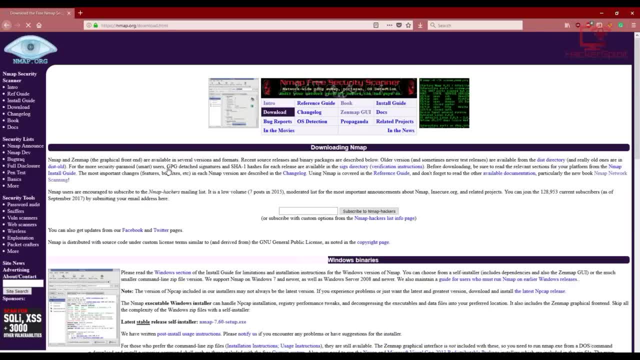 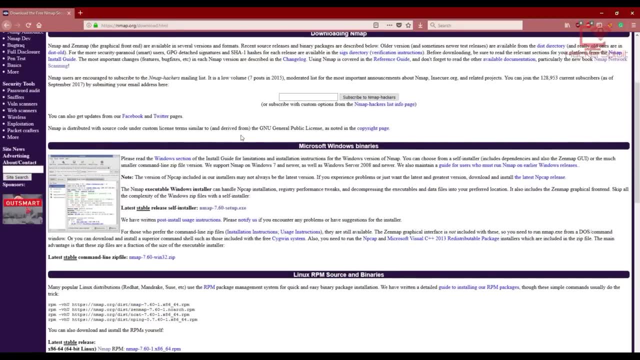 right there. We're just going to click here, All right, and it's going to take us to the download page And we're going to go to the download page. And we're going to go to the download page And it's a fairly simple but a fairly clogged website And you might get a bit confused, But don't worry. 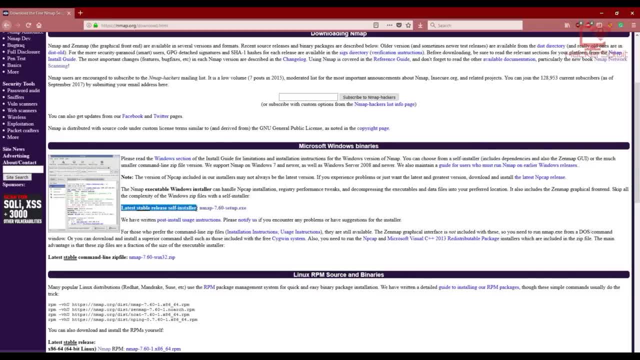 you want to go to this bold sentence right here? Whoops, let me just go back there And it's going to tell you the latest stable release self installer. So this is an executable file, All right, And it's very important that you understand that. if you're running Windows, I would recommend. 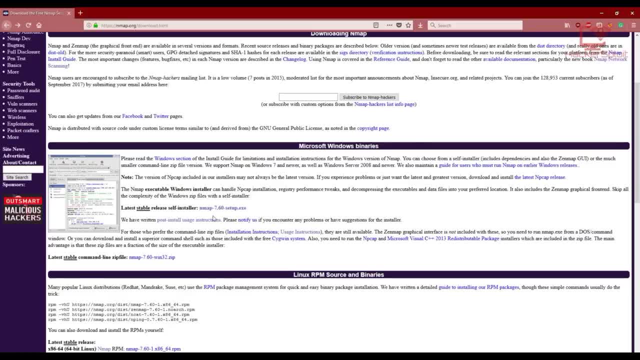 that you use the executable file because it will allow you to use the n map, the n map framework or the n map tools in the command line. Alright, so just click on this right here And it's going to prompt you to download the file. So it's about 26 megabytes, really, really small. I have mine. 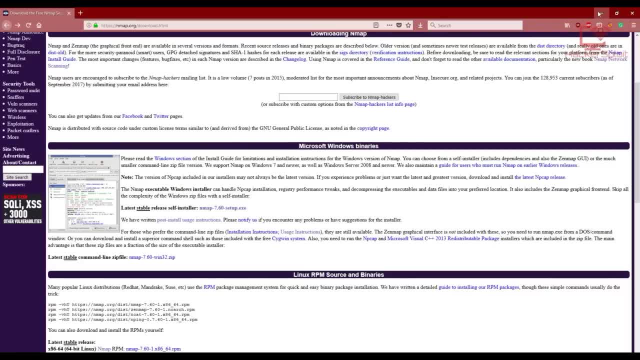 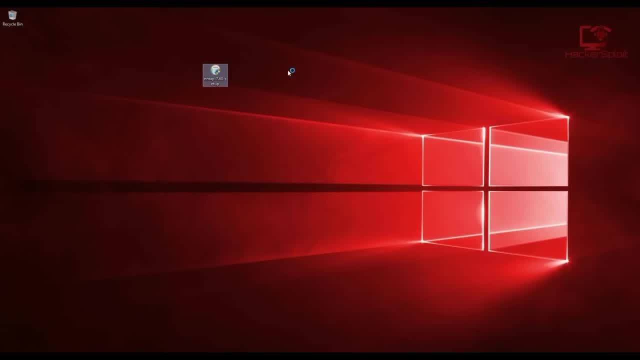 downloaded. So we're going to go to the installation process. So I'm going to minimize my browser and I have my file saved on my desktop right here. So I'm just going to run it And let's go through the installation. So it's going to ask you for an administrator privileges. grant it And 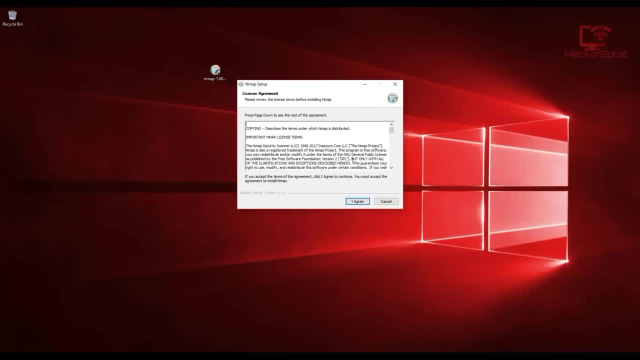 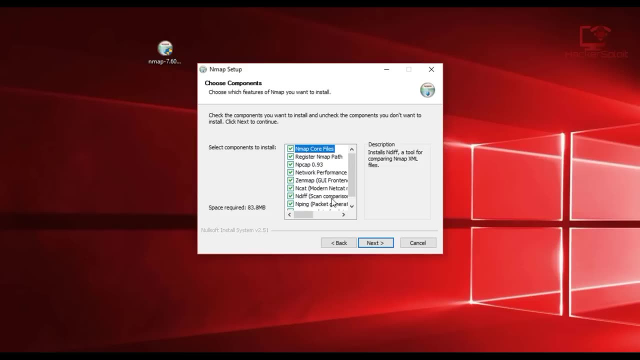 now we can go through the setup wizard, which is very, very simple, So I'm going to agree to the terms. Now, very important, it's going to give you an option to select the components that you want to install. It's very, very important that you select everything. All right Now. as you can see, 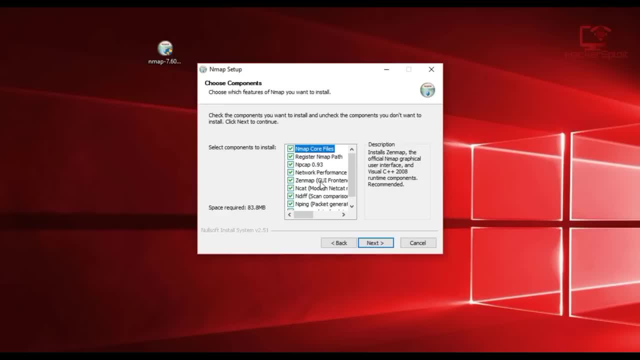 it gives you the option to install ZenMap. we're going to be going through ZenMap in this course, So I recommend that you take that and make sure that everything is ticked here, especially n PCAP. All right, so, as you can see when you hover over it, it tells you that n PCAP is required for most n map scans. 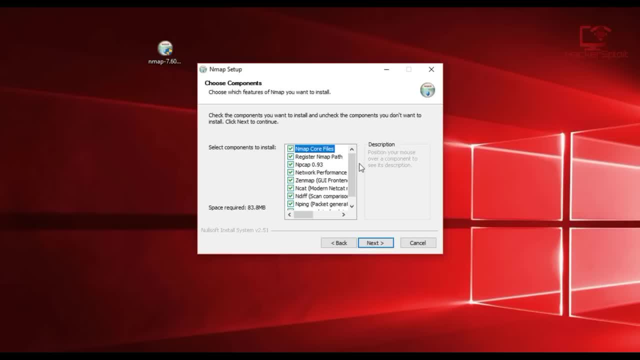 unless it's already installed. So it's very, very important that you check everything, And I would recommend that you leave it that way. Alright, so just hit next And it's going to prompt you to select your destination folder. That's fine with me. I'm going to hit install And the installation. 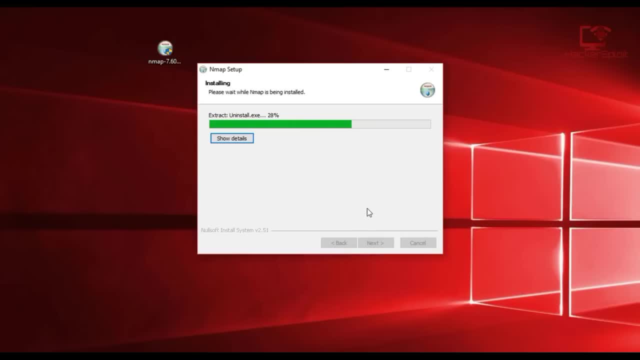 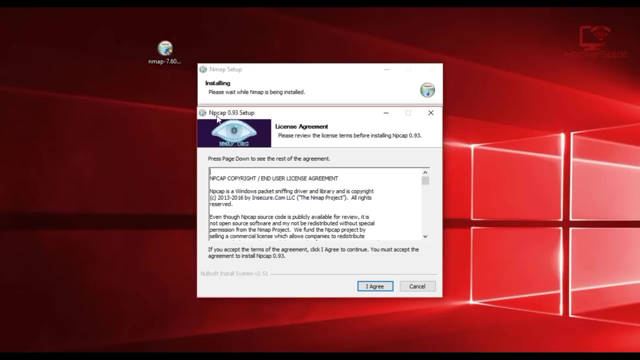 process should be fairly simple and really really quick. Alright, so we're almost done here. Just give it its time. shouldn't take too much time, All right. so now it's going to ask me to. it's going to prompt me to go through the n PCAP setup. 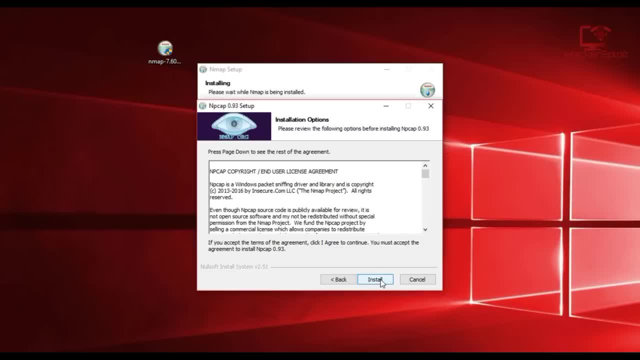 So again, this is very, very important, So I'm going to hit agree And it's going to ask me for the installation options here. So automatically start n PCAP at driver boot time. Yes, I would recommend that you leave that on so you don't have to start it whenever you want to use whenever you. 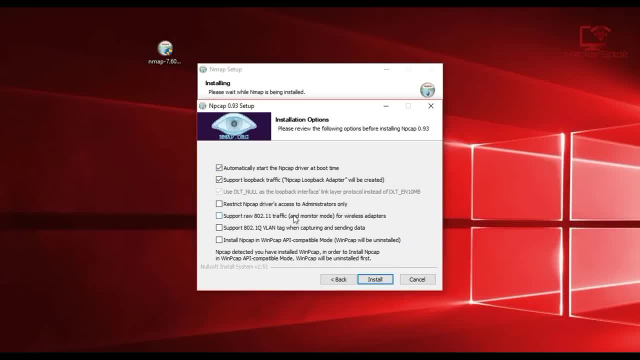 want to use n PCAP n map. Alright, so you can restrict n PCAP driver for the administrator accounts only. but I would not recommend that you click on that. Alright, so you can support raw 802, point 11.. So that is a. 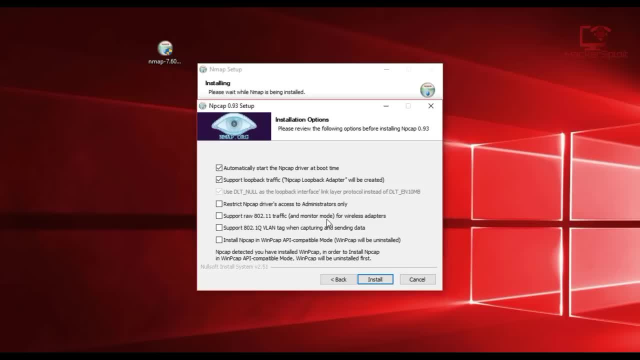 wireless standard and monitor mode. So this is, if you have a specific network adapter, more specifically, an adapter that allows you to perform packet sniffing and a network card that allows the monitor mode to be turned on, Alright. so what I would recommend is that you just leave this. 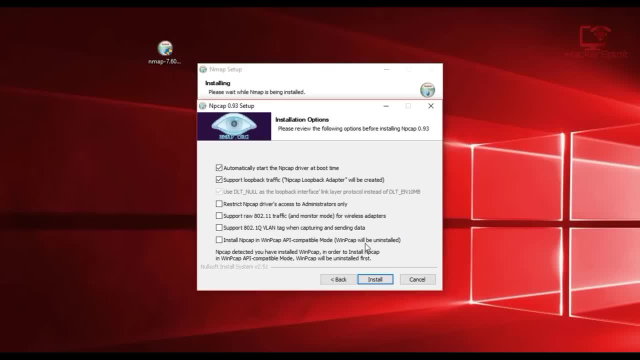 unchecked, because these are very special settings for very special circumstances. So just hit install And it's going to take you through the install of the n PCAP driver. All right, again, this shouldn't take too much time at all, But this is the most important step. Otherwise, n map. 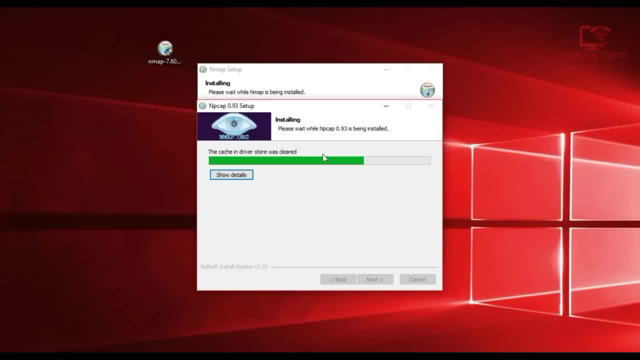 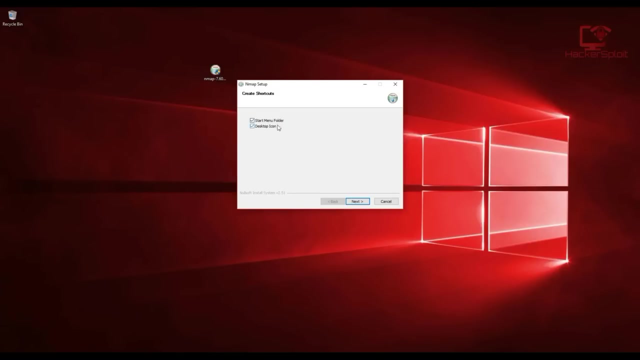 wouldn't work at all. All right, So I'm going to hit next, And it's going to prompt you to do is going to prompt you asking you if you want a shortcut on your desktop or if you want one on your Start menu. I'm going to like both, So 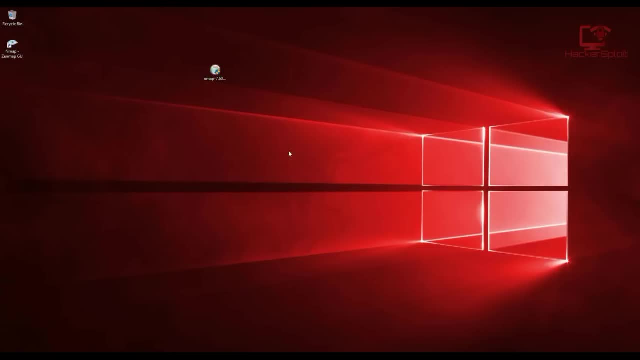 I'm going to hit next and finish. Excellent. So, as you can see, it's given me a shortcut on my desktop for ZenMap, So we're going to be looking at that in future videos, But for now, we want to actually go through the command line interface, which is the most important, because we're 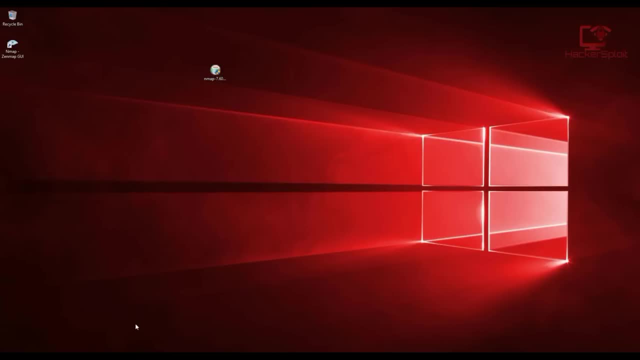 going to be looking at all the commands that we can use Right, So open up your command prompt. or, if you don't have it already on your taskbar- which I'm guessing you do not- what you want to do is you just want to go onto your Start menu, or you want to use your keyboard shortcut, your Windows button. 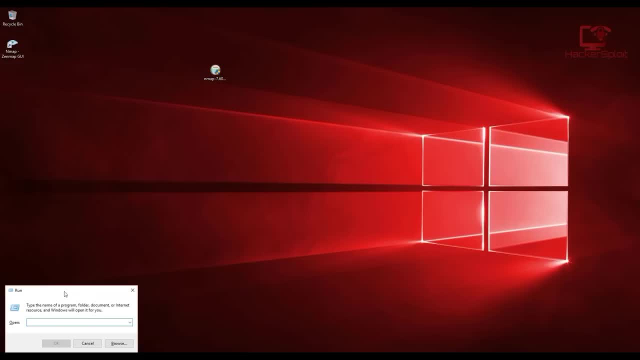 or your Windows key plus R and it's going to prompt up your run service box right here. And you just want to hit CMD? All right, and just hit OK And it's going to open up your command prompt. Excellent, All right, so now we can get. 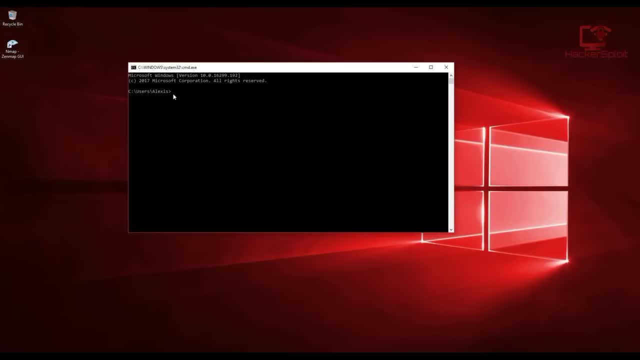 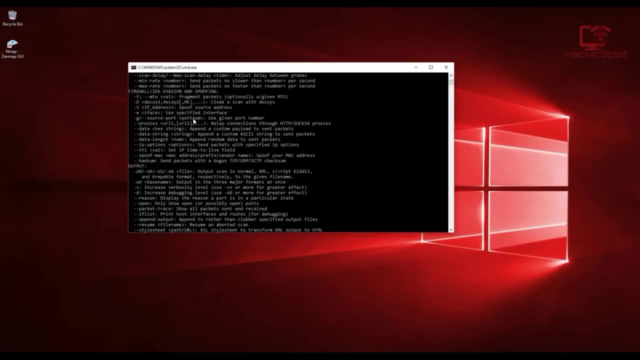 started. So, in order to perform a quick test to make sure that everything's installed, all we have to do is just hit Nmap And it's going to print out some some text here, which is essentially the manual or a command line. 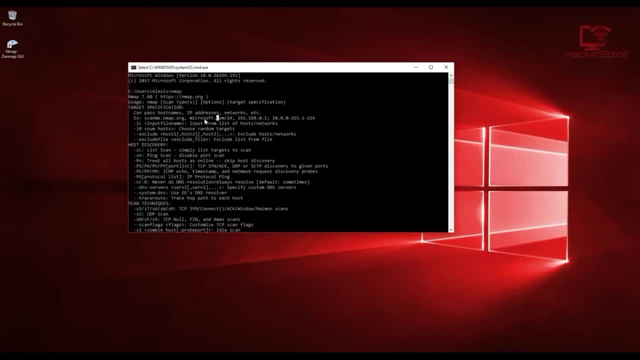 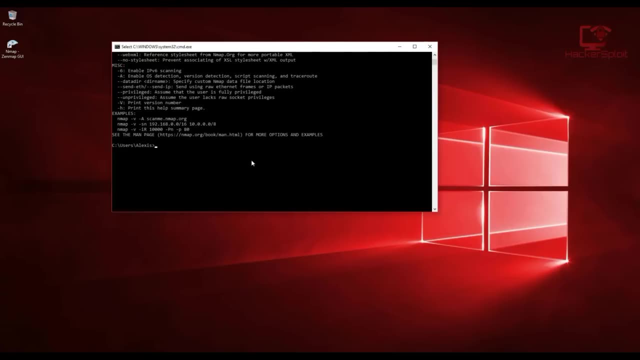 manual that it comes with, And essentially this is all the options that you can use, So do not be overwhelmed at all. we'll be going through all of this. So Nmap is successfully installed And you can actually run one more command to check the version that you have installed. So Nmap hyphen. 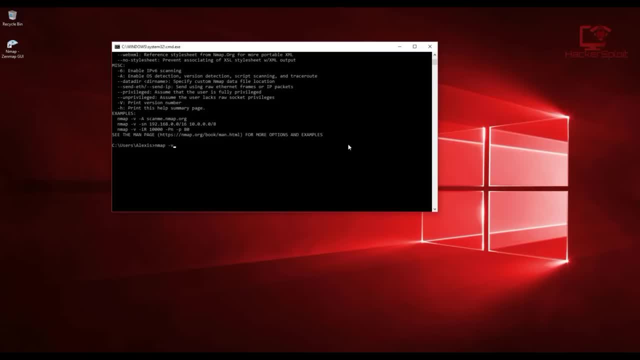 v or dash v, which is Nmap for version, and it's going to print out the version of Nmap that you have currently installed. I'm just going to hit that And, as you can see, we have Nmap 70.60.. 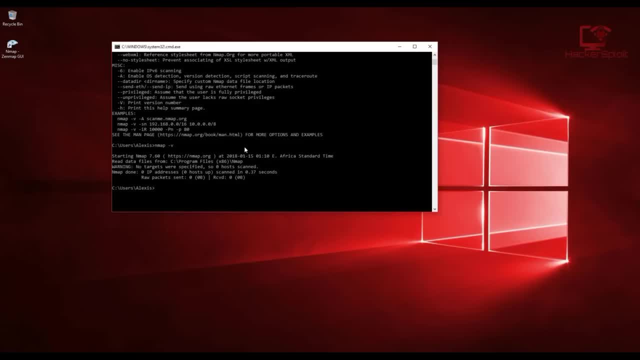 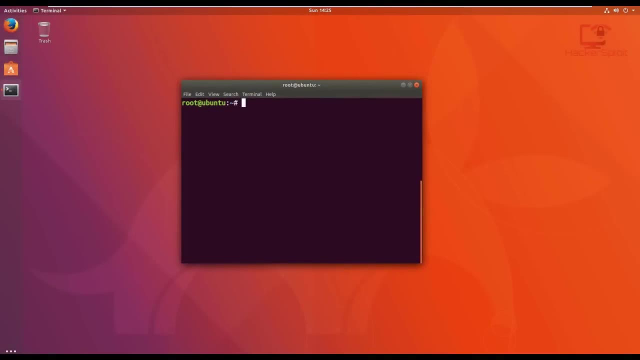 Excellent. So we have Nmap installed on Windows, And in the next lecture we're going to be looking at how to install it on Linux. I'll be so. I'll be seeing you in the next lecture. Hello everyone and welcome to this lecture. In this lecture, we're going to be installing Nmap on Linux. 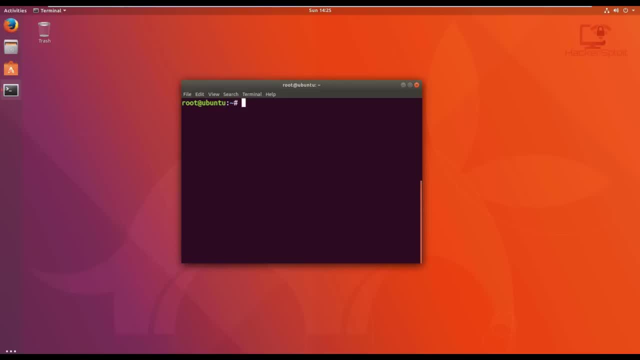 Right now, before we get started, I just want to throw out a disclaimer. this will work on any Linux distribution that you have running and installed. Alright, so I'm currently running Ubuntu, which is a base distribution. you could be running Fedora, And I'm going to be showing you how to install it on. 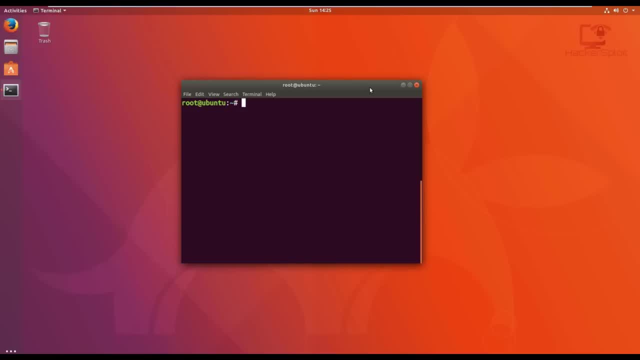 Fedora as well. Alright, so it's really very simple. You know we can install everything using the package managers that come with our distributions, So everything happens in the terminal. Now I've already got root access, So again it I really just like working in root when I'm installing. 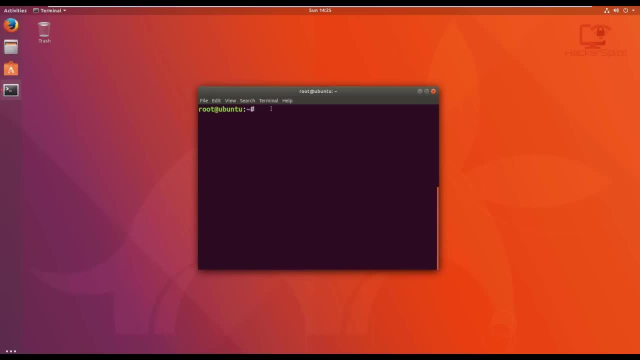 software, So you can use your package manager or that you have installed on your Linux distribution, or you can just use the normal command line method. Alright, so, or the terminal method, as it were. So let's get started. So with Debian, which is what I have running here. let me just drag that there. 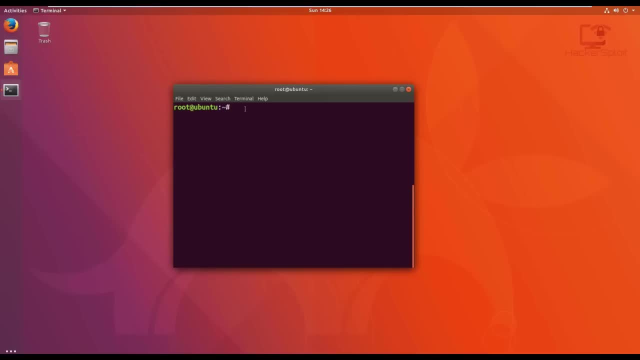 There we are. Alright. so what we're going to be using is we're going to be using the aptitude package manager. So if you're familiar with Linux, you probably already know what I'm talking about. But if you're not familiar with Linux, don't worry. it's essentially a package manager that allows you to install. 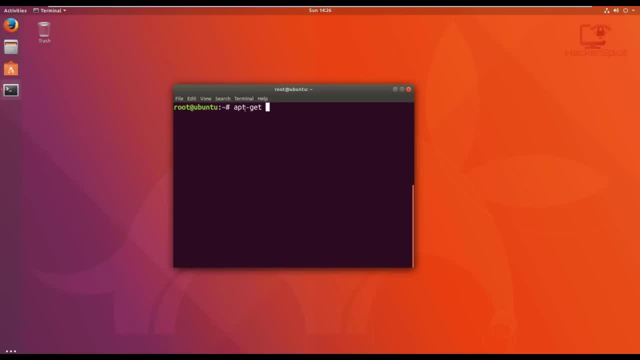 software Alright. so apt Get install and map Alright. that's the command that we're going to be using to get an map installed. Now, if you're running Fedora or a Fedora based distribution, what you can do is you can use: 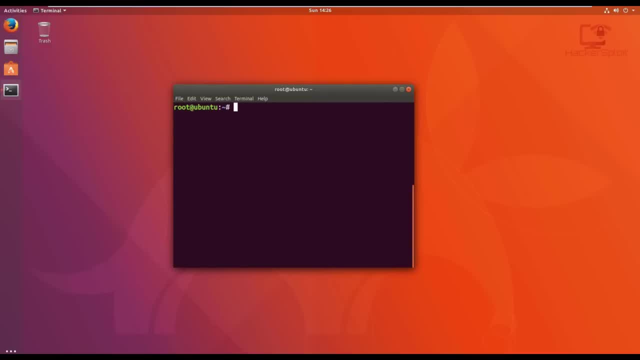 the command yum. Alright, so that's the package manager. So yum, install and map. Alright, so that's how you go about installing and map on a Fedora based distribution. So let's go back to using our aptitude package manager, which is what I'm guessing. 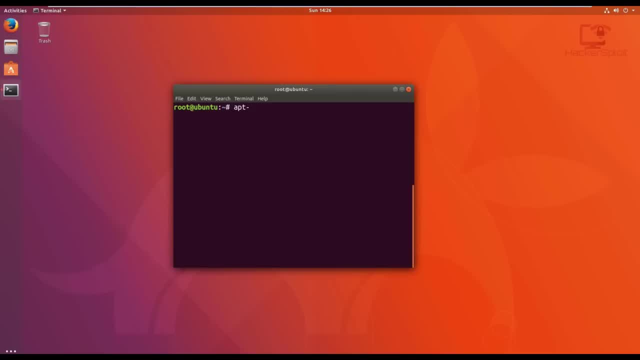 Most of you are going to be using, because I would guess that most of you are running a Debian based operating system or a Debian based distribution of Linux. Alright, so apt, get install, oops and map. Alright, and just hit Enter And it'll automatically be installed. you don't need to add anything to your. 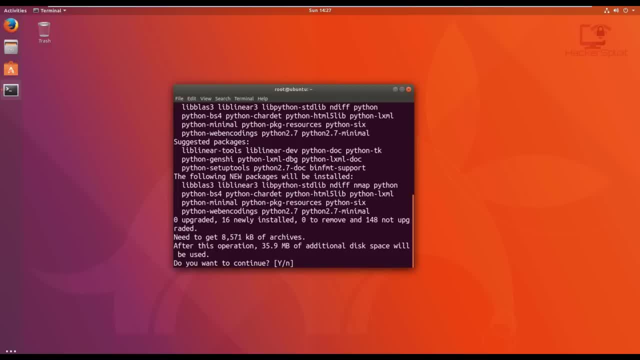 repositories, because nmap is already. it already exists in the Debian and the Fedora repositories, So it's going to prompt you to download files. So just hit yes or Y and hit enter and it's going to start the download process. Now, depending onto. 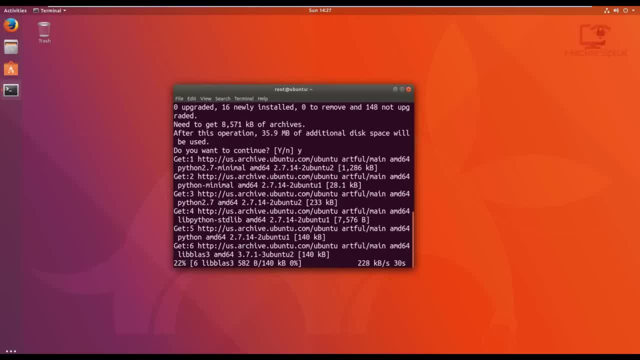 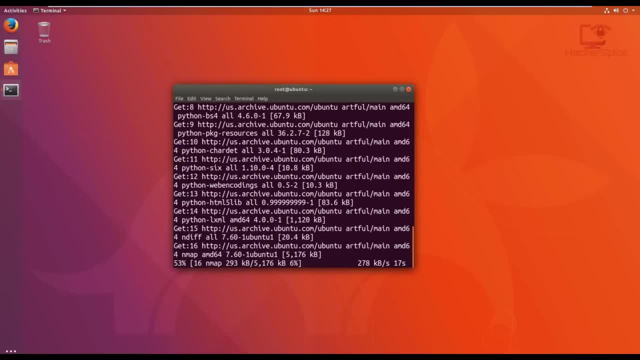 the speed of internet connection. it'll take as much time as it needs. So let it download and let it install for you, And once it's installed, we can actually get started with testing it. Alright, so give it a few seconds, shouldn't? 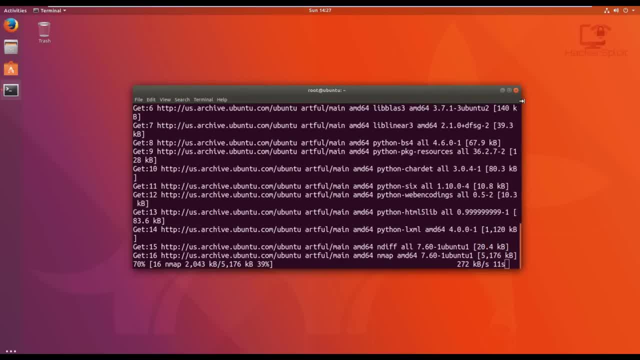 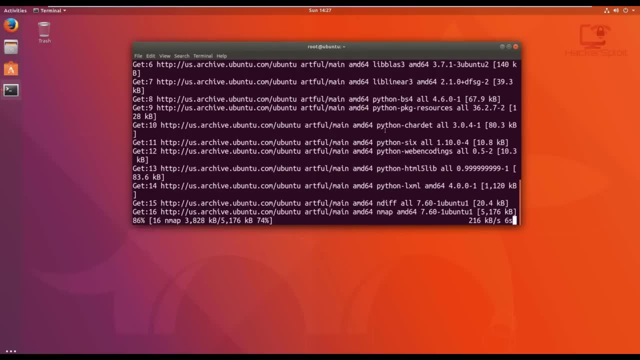 take too much time at all. Let me just expand this So we have a better picture of what's going on. All right, So again, give it a few seconds. Let's get started. seconds, it shouldn't take too much time at all. it's about 30 megabytes of data that needs to. 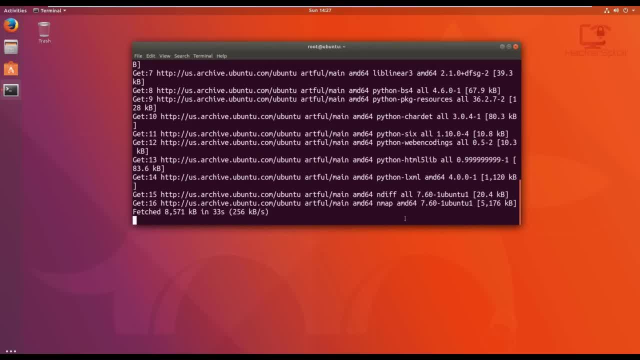 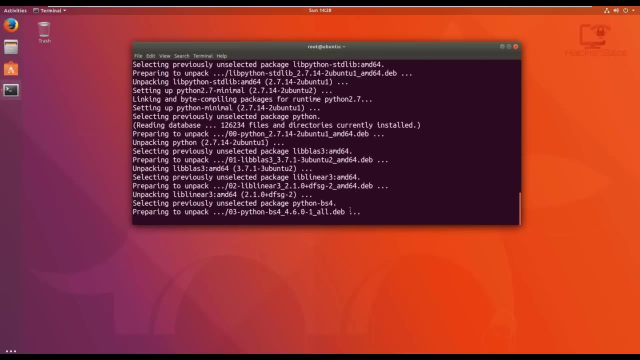 be downloaded. please do pardon my internet connection speed. it may be affecting the download here. all right, there we are. looks like it's downloaded and give it a few seconds. all right, there we are. it's going to start unpacking, uh, the the libraries, or essentially what it's doing is it's installing it. okay, all right. 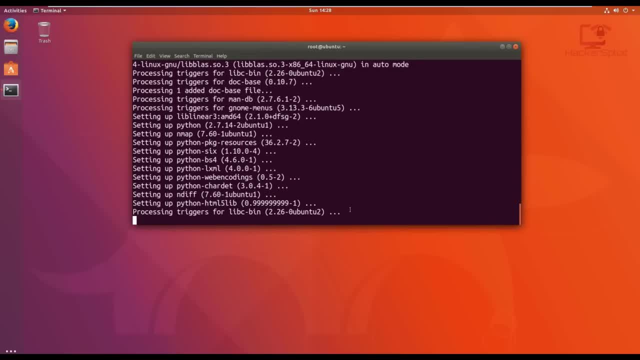 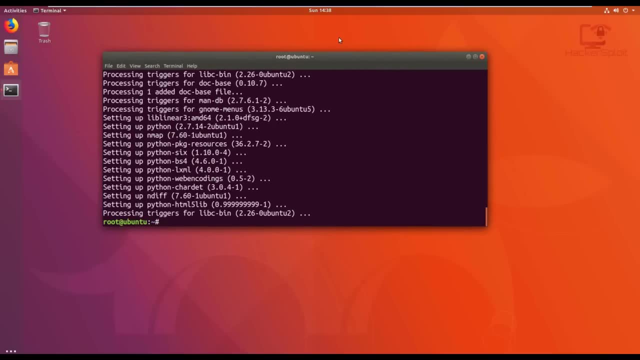 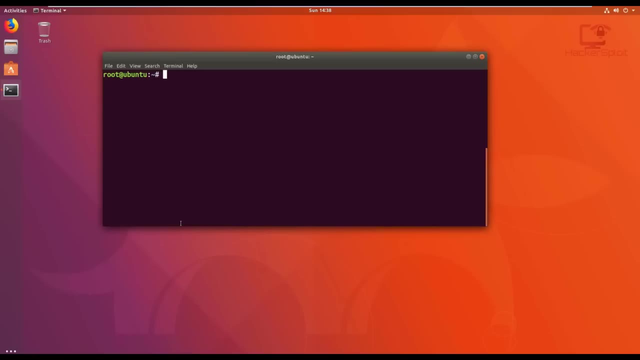 all right. so once it's installed, uh, what we can do is we can just test to see everything's working all right. so it's really very simple. let me just clear up my terminal and, uh, how i'm going to test it is. i'm just going to use nmap and if i hit enter, it should display something. there we are. 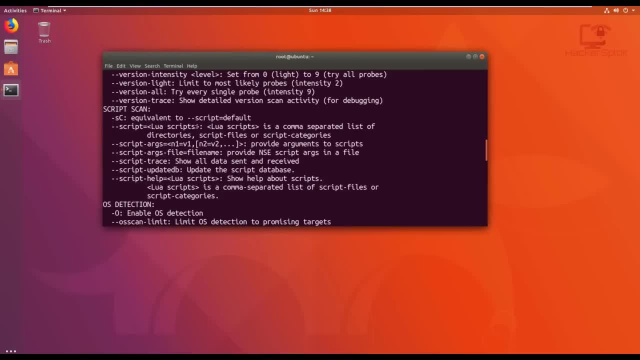 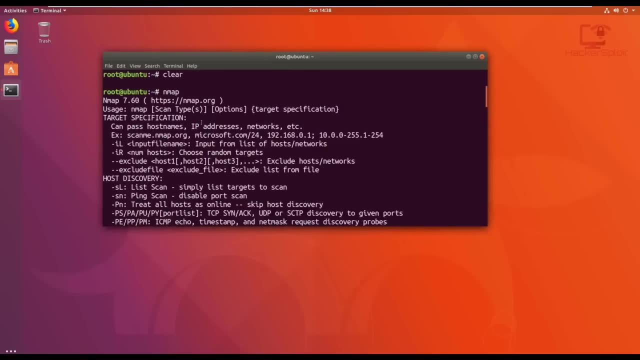 it's going to display the options, or rather the help menu that contains all the options that you can use in terms of the commands uh, for the different types of scans that you can perform. all right, so the other way you can test whether it's installed is to check the version that is. 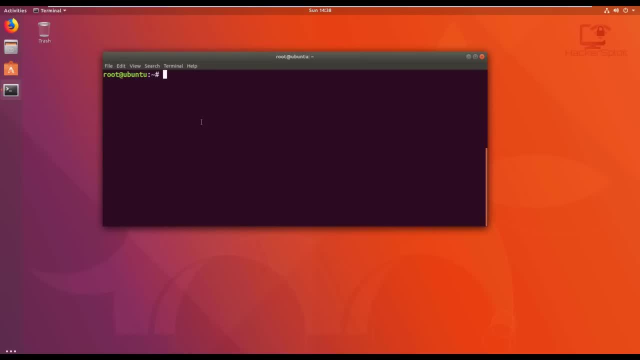 installed and we can do that using the standard syntax. you should get pretty used to this. uh, to perform any nmap scan, everything has to start with nmap. all right, so nmap, and we use our first command. that's the first command we're learning and the command is how to check the. 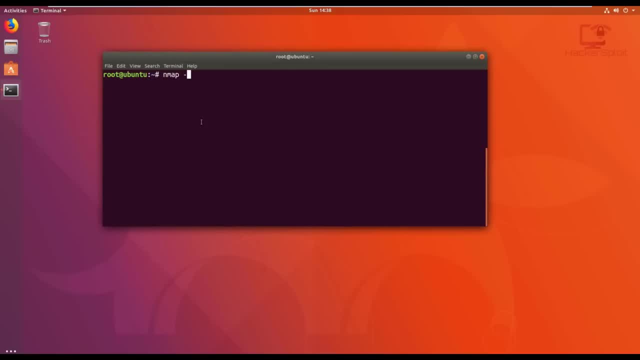 version of nmap that is installed. so we're going to check the version of nmap that is installed. so nmap dash v, all right, and once i hit enter, it's going to display the nmap version that is currently installed there. we are fantastic, all right. so that's going to be it for this lecture. 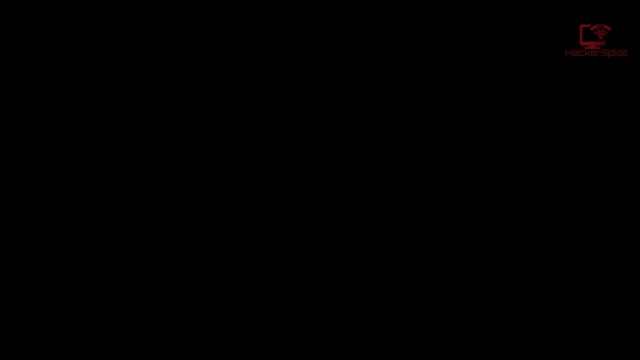 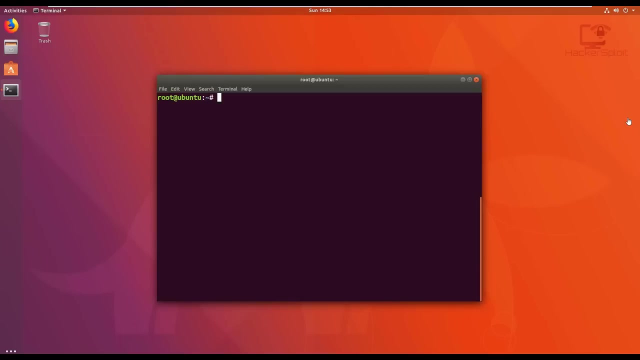 i'll be seeing you in the next lecture. hello everyone, and welcome to this lecture. in this lecture, we're going to be looking at how to install zenmap on linux. all right, so, as you already know, zenmap comes pre-packaged with nmap on windows, but on linux you have to actually 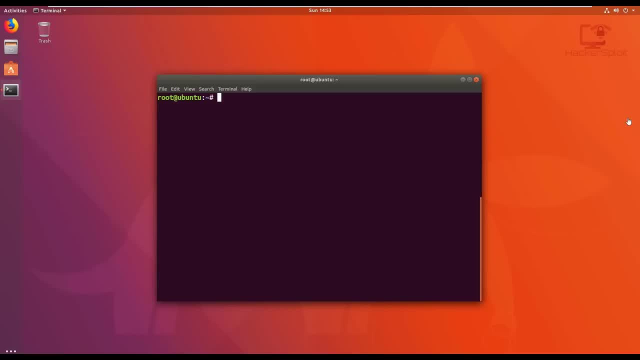 download it separately, all right. so if you don't know what zenmap is, uh, it is, simply put, a gui based version of nmap, all right. so it gives you gui functionality, which makes things a whole lot easier. but, as i said, it is very, very important to important to learn the fundamentals of nmap. 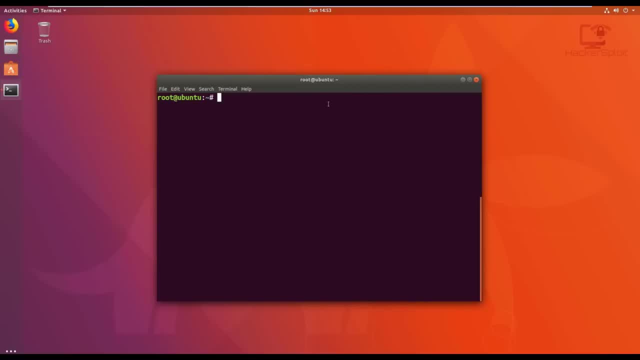 but having uh said that, uh, let me show you how to install it. so again, it'll work on any distribution, whether you're using debian, fedora or even an arch based uh distribution of linux. so you use your package manager. in this case, i'm using the aptitude package manager. apt- get install. 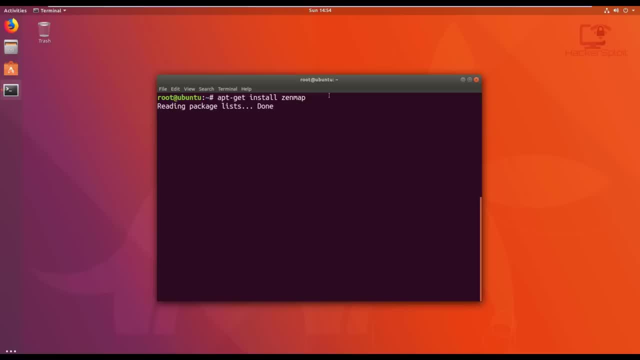 and zenmap. all right, very, very easy. and once that's done, again, it's automatically added to the repositories of any debian distribution or any any of the linux distributions. all right, so it's again. it's a very, very popular and very powerful network scanning tool. so it's going to ask you to download the files that are required, so i'm going to hit yes. 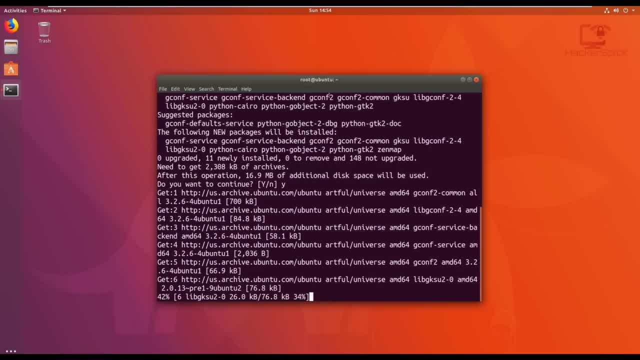 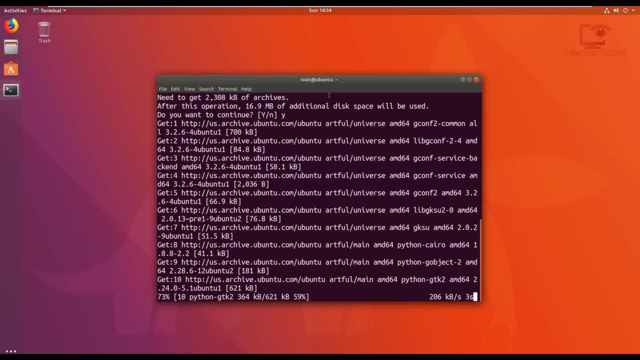 and it's going to connect and start downloading the files again. depending on the speed of your internet connection, it can take, uh you know, a few seconds up to a few minutes. hopefully you don't have a as bad as a connection as i do at the moment. 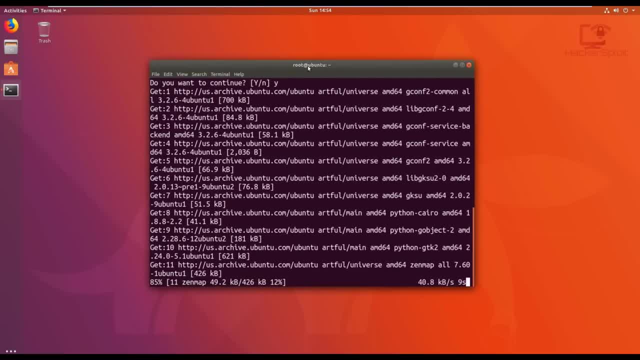 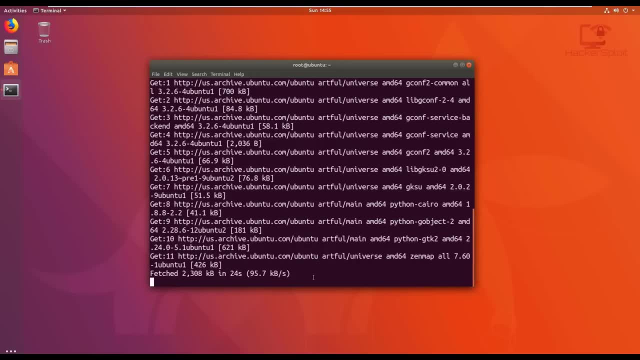 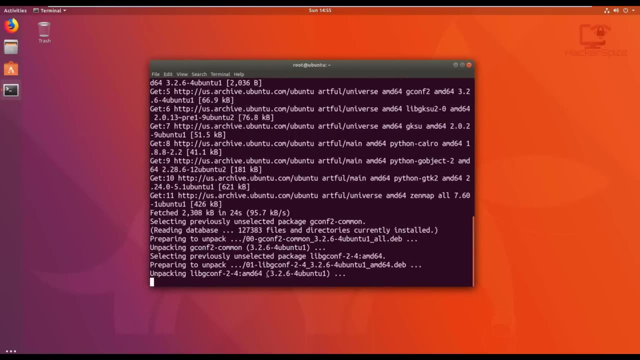 but again, it is a relatively quick process and shouldn't take too much time at all. all right, so we're almost done here, just getting the files downloaded, all right. there we are 24 seconds and 95.7 seconds, uh kilobytes per second. uh. so yeah, that's not the best speed there. all right, so now it's going. 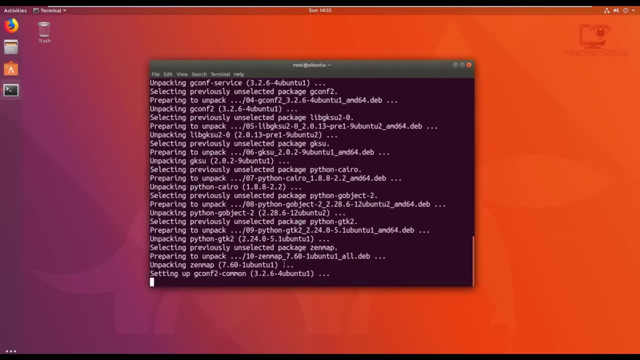 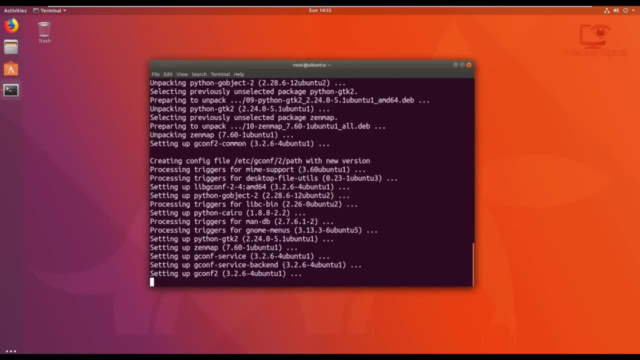 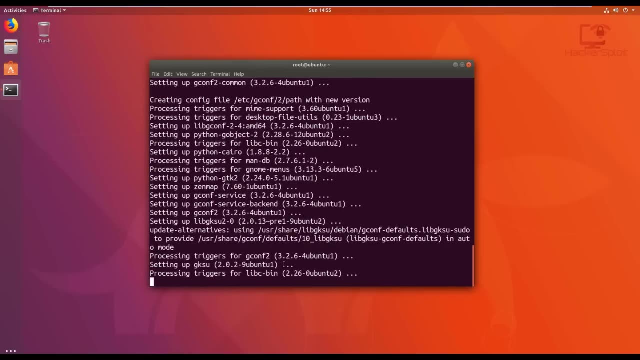 to unpack the files. all right, there, we are almost done. so again, installing it separately with linux is quite nice because it gives you the ability to modularize how you want these services installed again on linux. you don't have to install any special driver. as i said, nmap was designed. 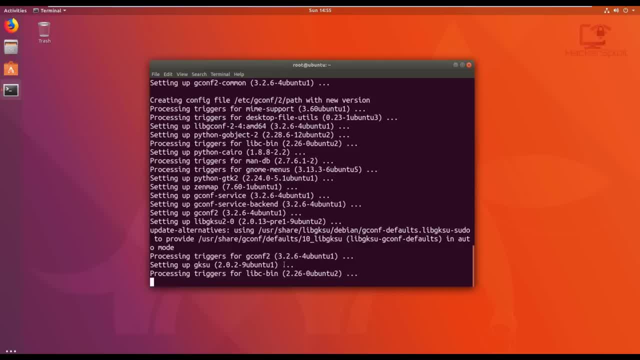 to be a continuous uh network app builder to be able to configure, stated, and it's basically that the nmap framework or the nmap tool was designed, uh, with onlinux for linux and again, it works really, really great with linux. all right, so the download and installation is. 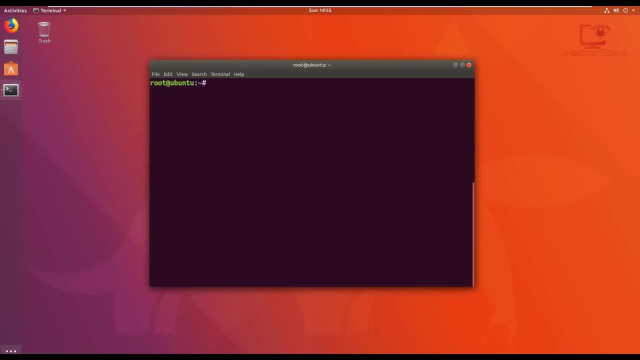 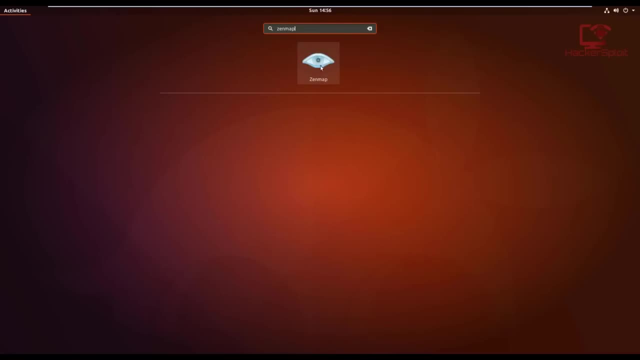 complete. what we can do to launch it is: you can launch it from your terminal or you can go ahead and launch it from your application launcher if your distribution or your desktop environment has one, so you can search for it right here. so zenmap, uh, i'm on ubuntu and there we are, it is. 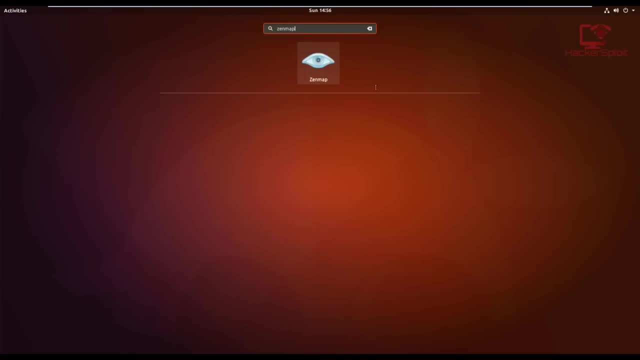 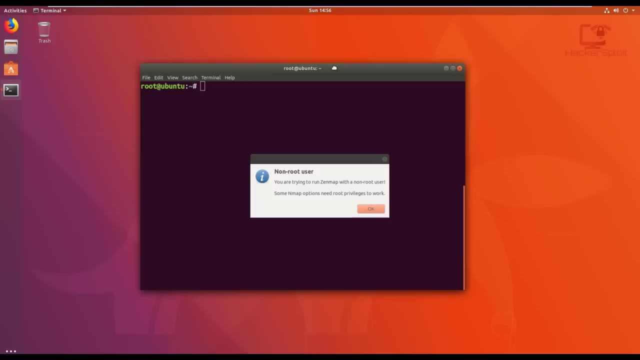 So if I click on it, just give it a few seconds. I do beg you a pardon, And that is because my I'm running this distribution on a virtual machine And it could be quite slow Alright, so if it gives you this, it's very important. This is also something that you need to take into account, So 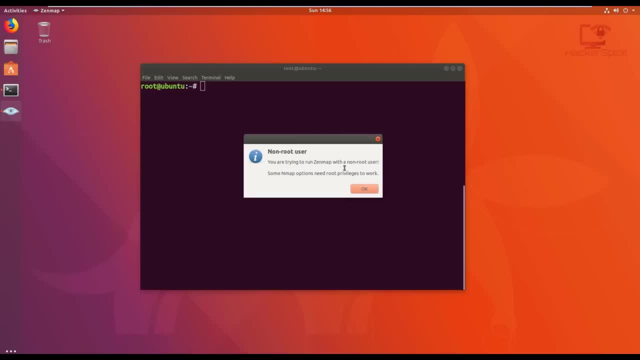 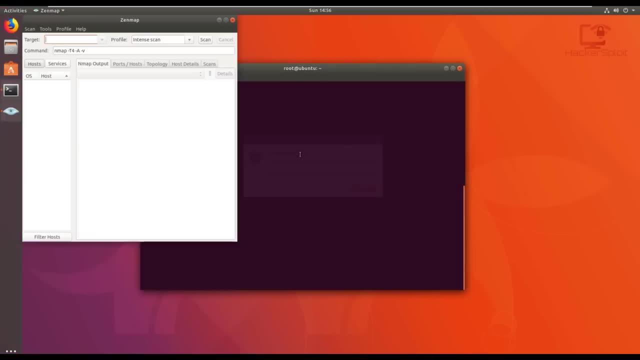 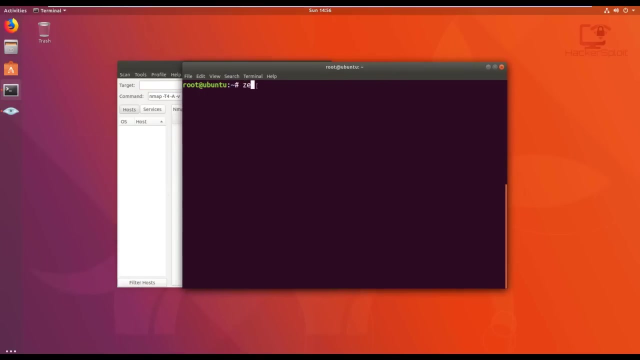 it's going to say a non root user. you're trying to run Zen map with a non root user. some and map options need root privileges, Alright, so don't worry about that. What this essentially means is that if you want to use the full functionality, you should launch it from root- Alright, so what? 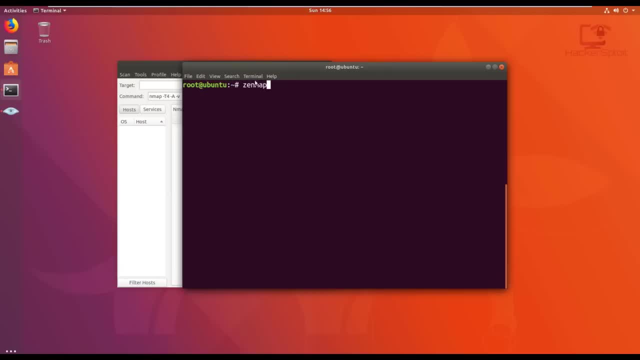 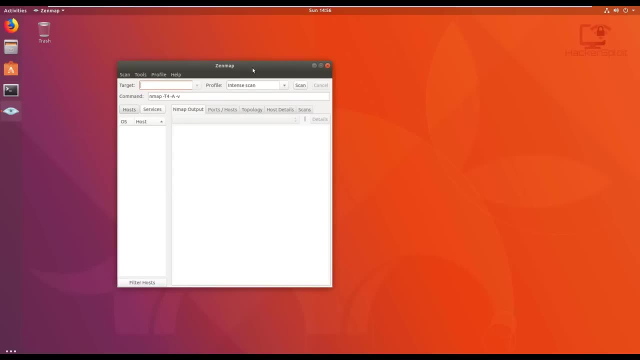 you would do is just go and hit Zen map, And from root, obviously, and it will give you the ability to use everything. Alright, so here is Zen map. Let me just close the terminal And there we are, a fantastic GUI tool, And we'll be going through this. I've dedicated an entire section in the course. 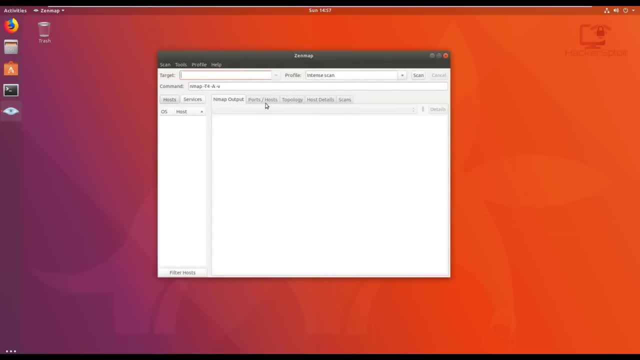 to how to use Zen map, because, again, it does really really help with efficiency and performance productivity. Alright, so that's going to be it for this lecture. I'll be seeing you in the next lecture. Hello everyone, and welcome to this lecture. And in this lecture we're going to get. 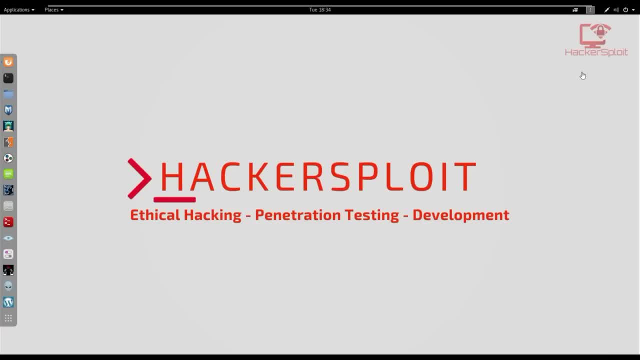 started with scanning. More specifically, we're going to be looking at how to perform a single scan, or we're going to be looking at how to how to perform a scan on a single target. Alright, so let's get started Now. hopefully you've set up your environment and your your penetration testing. 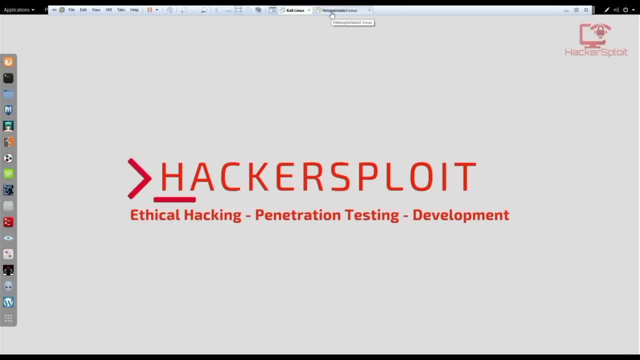 lab And hopefully, you have a target. In this case, I'm going to be using meta exploitable tool And it is what I recommend for the course. Right, So let's get started Now. you can. you can do this on Windows or Linux. I'm going to. 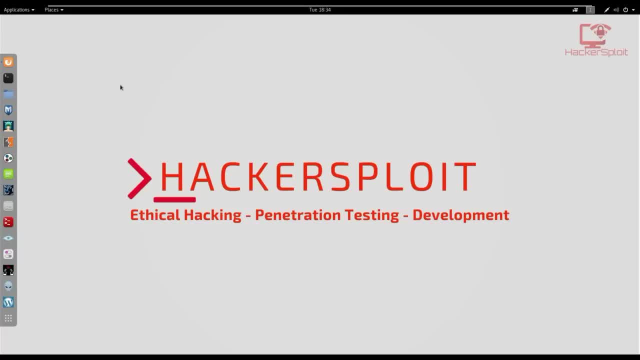 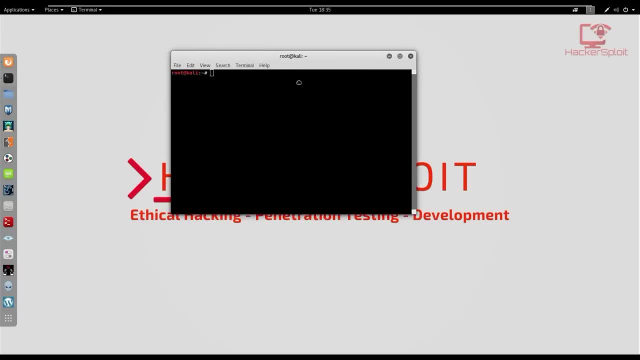 be doing this through Kali Linux, because it's more in tune with penetration testing. Alright, so I want you to open up a terminal. Okay, let me just open that up, And what I'm going to do is I'm just going to increase the font size. Alright, so we're scanning for a single target Now in this. 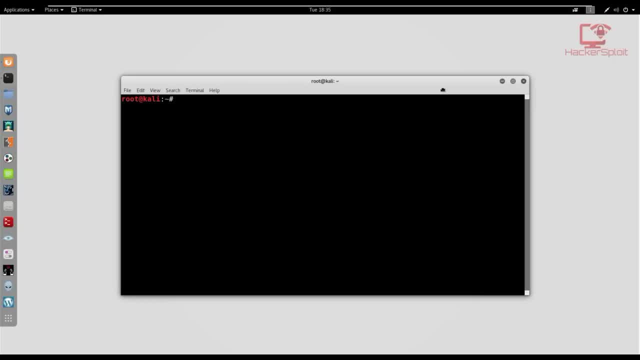 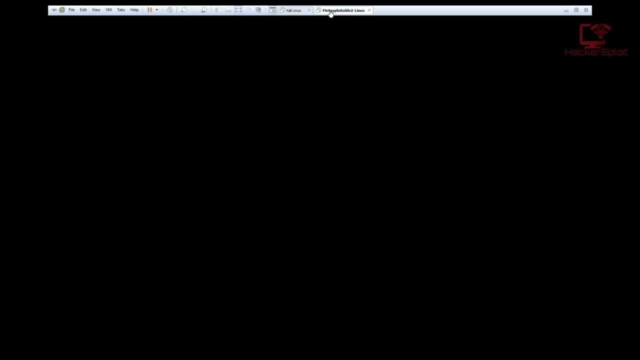 case, I'm going to be scanning meta exploitable tool, So let's go ahead and run the meta exploitable tool virtual machine that is running on my local network. Okay, so if I go to my meta exploitable tool virtual machine and let me just start it up, 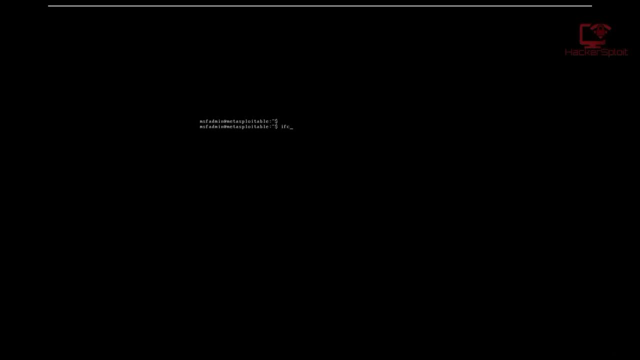 like so. Alright, so I'm going to run the if config command to find the local IP address for the virtual machine so that we can scan it. Okay, so I'm going to hit enter And there we are. if we look at the INET address, which is the local address on the on my local area network, it's: 192.168.1.107.. Now, this could be, or should be, different for you, depending on what type of router you're using and what IP ranges you have set up. Alright, so I already have got the IP. now. 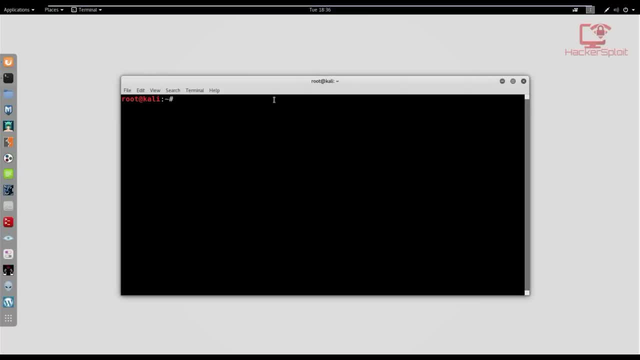 and we're going to scan it with nmap. Alright, so, as we've said before, nmap is really easy to start up. we all we need to do is use the nmap command And now we can enter our target right. So entering 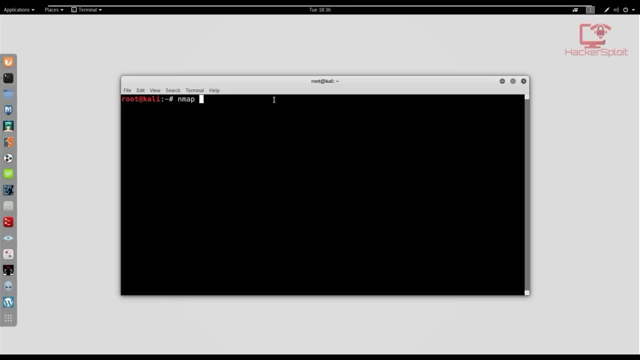 our target, with no options or with no commands, really will perform a basic scan on the target. Alright, so let me show you what I mean. So if I enter the IP address for the meta exploitable to virtual machine, which is 192.168.1.107,, it'll perform a basic scan. remember, we're not using 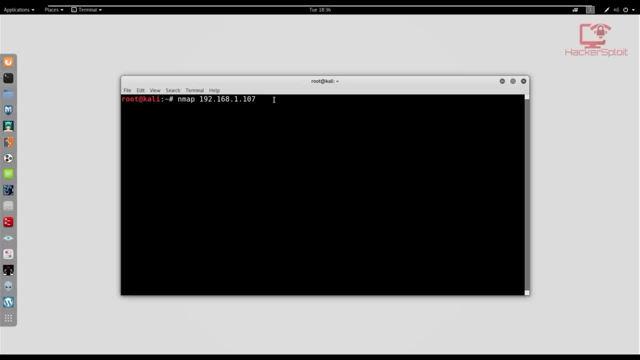 any commands or any options here. Okay, so if I just hit enter, it's going to start a scan and immediately return the results, And this is why I was really encouraging you to use meta exploitable too, because it gives you a very good idea of what a scan is, how it is comprised and how we can you. 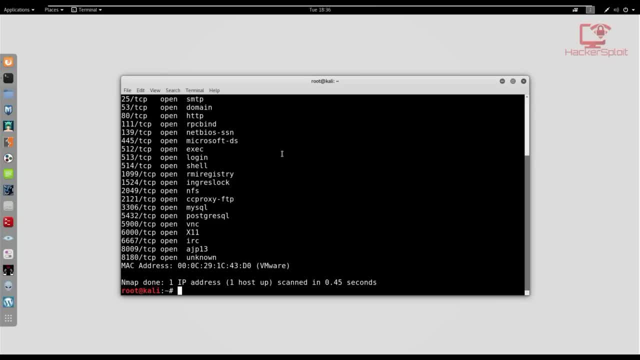 know, get along with all of this. Alright. so that is how to perform a scan on a single target, Right. So the syntax is very simple, right? We have n, the nmap command, which starts the nmap, the, which starts nmap, and then we, which is then followed by our. 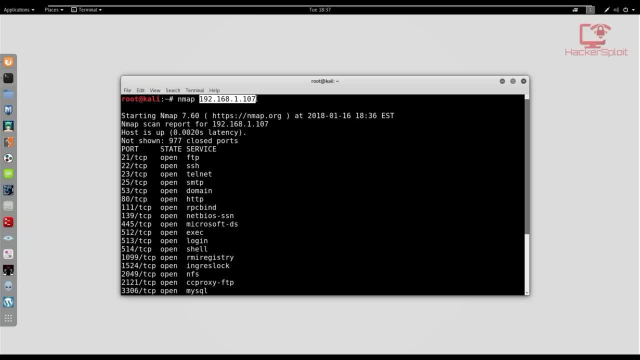 our target right now. our target could be an IP address. it could be a website, for example, And again, if you do not use any commands or options, it will perform a basic scan. Now let's look at something very, very interesting. Once we've started the scan, it's going to give us some 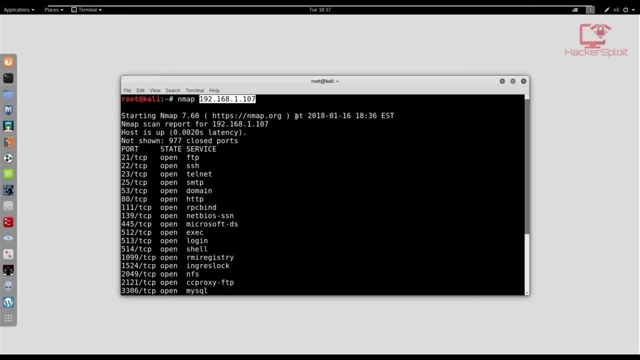 information. So it's going to say it gives us information about the nmap version And it's going to give us a timestamp here, So 2018, the 16th of January 2018, and the time all right now. 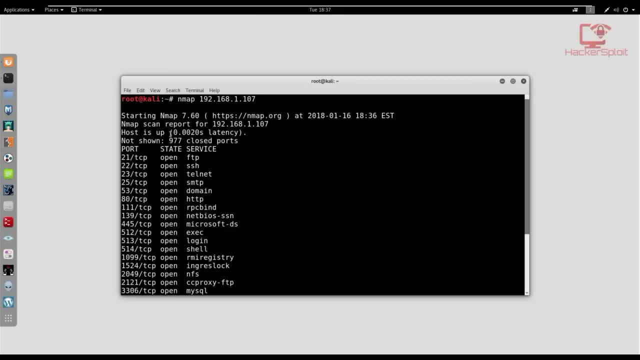 looking at the scan report. it's going to give you the scan report And it's going to start up with whether or not the host is up, whether or not the IP address is currently up and the latency connection to the IP address which, as you can see, is very, very small, which means the 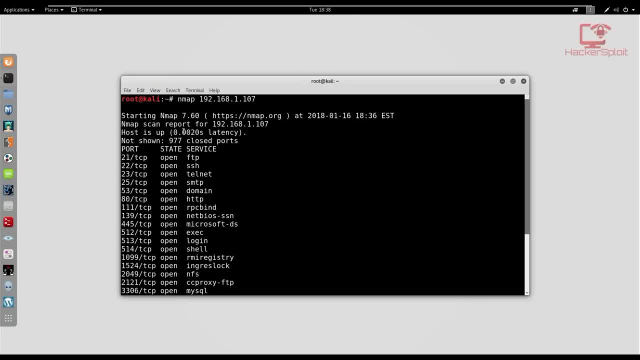 connection is very, very good. Now, by default, nmap will scan for 1000 ports. okay, 1000 of the of the most common ports. as you can see, it has scanned 977, it is scanned 1000.. 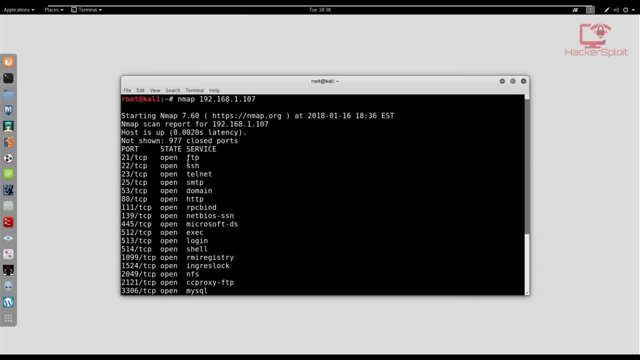 And it says it as well, it has returned more than you can see over there. So, in terms of the results it has, it has returned information And the way it's sorted is firstly from the port right and then the state of the port, which can be open, filtered or closed- right and the service. 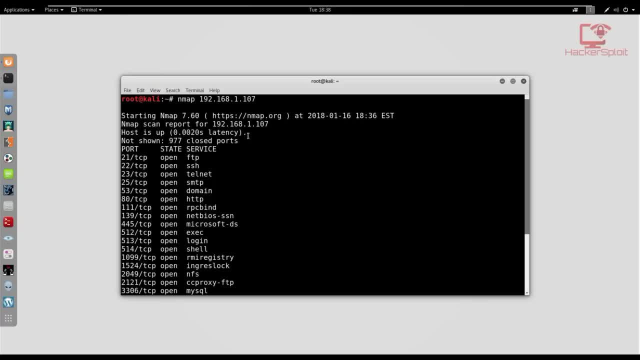 running on that port. Now, it's very important to understand the different ports in networking and the services that run on these ports. For example, we know that port 21 is the FTP port, we know that port 22 is SSH, and so on and so forth. Right, So it's very. 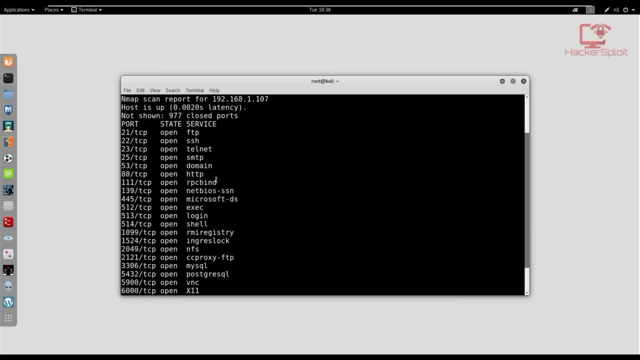 very important to know how the information will be sorted and displayed to you. Alright, so the port is simply the port number or the protocol, the state of the port, which is again the status of the port, and the service, which is the type of service that is running on the port. 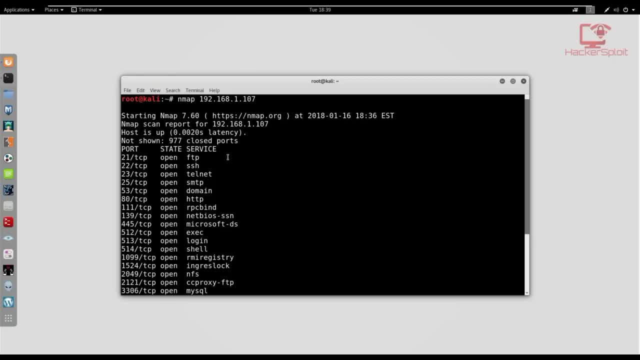 Alright, so, as I've said, a default and map scan will check for 1000 TCP IP ports, right, and then, depending on the what the host, depending on the results got from the host, the ports can be open, closed or filtered, or unfiltered. Okay, so that is how to perform a. 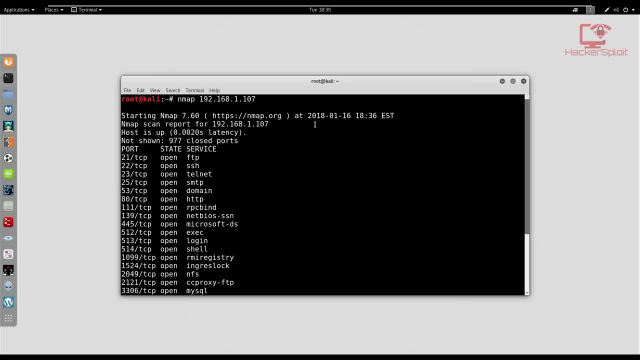 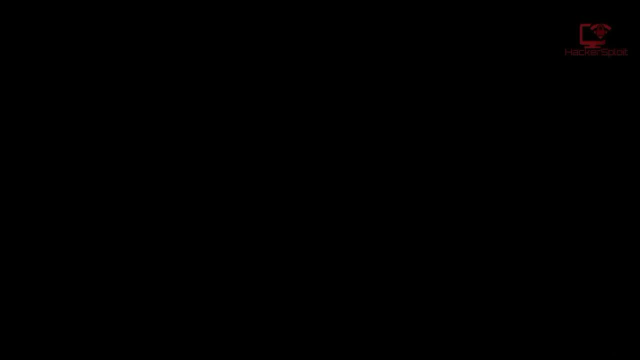 single scan on a single target, And in the next lecture we'll be looking at how to perform scans on multiple targets. Alright, so I'll see you in the next lecture. Hello everyone, and welcome to this lecture. In this lecture, we're going to be looking at 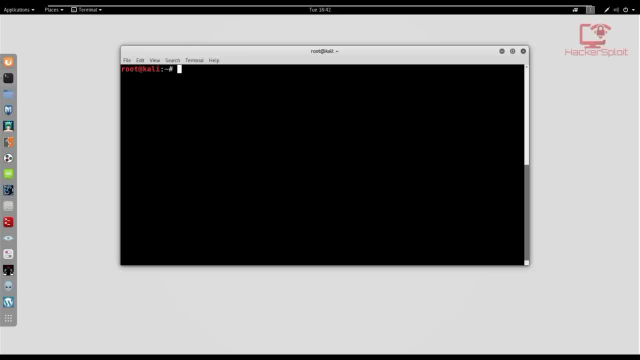 scanning multiple targets: Alright, so in the previous lecture we looked at how to scan a single target. Now we are going to look at how to scan multiple targets. Now it is possible in nmap to to scan more than one target or hosts at the same time. Alright, so let's see how we can do that. Firstly, 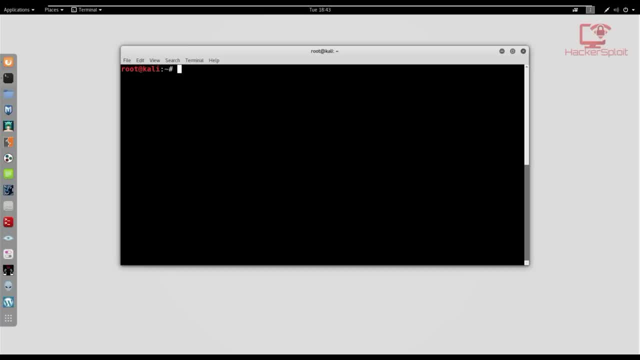 firstly with the syntax. Now, please note that we're not using any commands right now. I'm just showing you how one would go about scanning. you know, two targets at the same time, And if you want to scan multiple targets, you can do that. So you can scan multiple targets at the 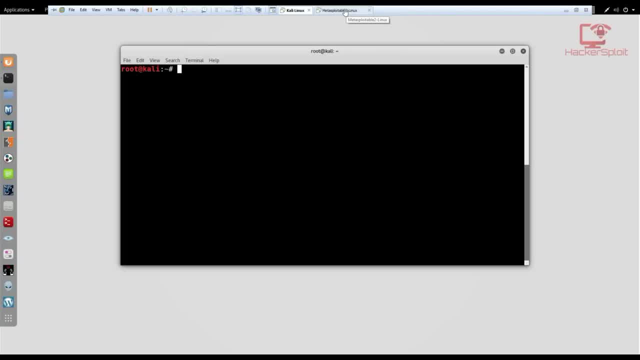 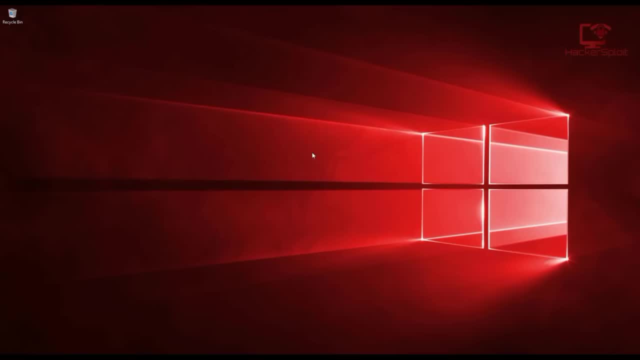 same time, or multiple targets at the same time. Alright, so let's get started Now. as I said, I already have my Metasploitable two virtual machine running. Now what I'm going to do is I'm running Windows as my host, as my host operating system, So I'm just going to find out the IP. 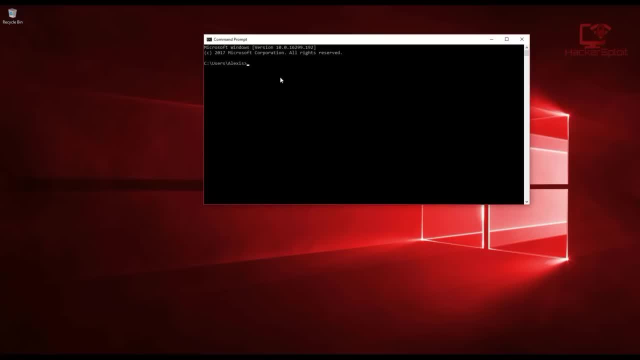 address and I'm going to scan for my Windows machine And I'm also going to perform a scan on my Metasploit machine. Alright, because I want to tie together two IP addresses or two hosts. So I'm going to run a command line for Windows And that will return IPv4 address, my local IPv4. 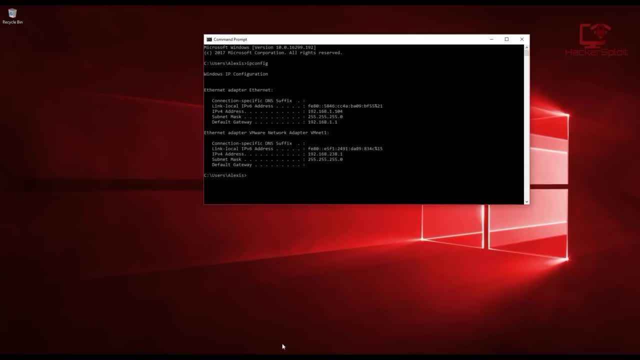 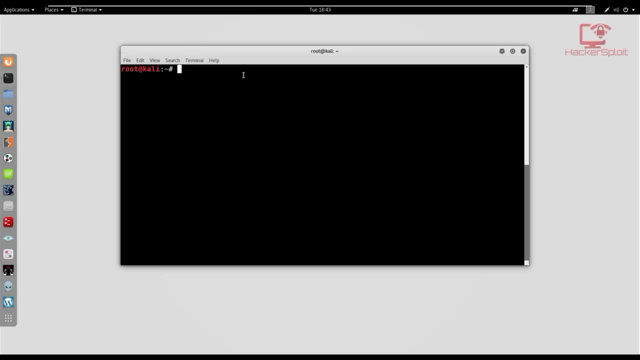 address, which is 192.168.1.104.. Alright, excellent. Let's move into Kali Linux again, And the syntax is really very simple, as we already know it is. So we start off with nmap, And the syntax then is very simple. You have your two targets. In this case, we are starting off. 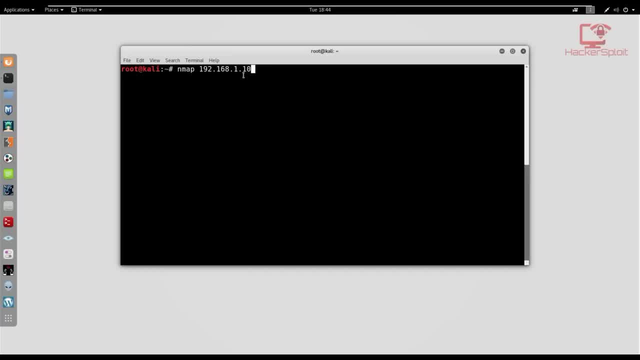 with the Windows, with my host operating system, which is 1.104.. And I'm going to give a space, Alright, so you just have to give a space between your targets, So which is then followed by the Metasploitable virtual machine IP address 0.1.107.. Alright, 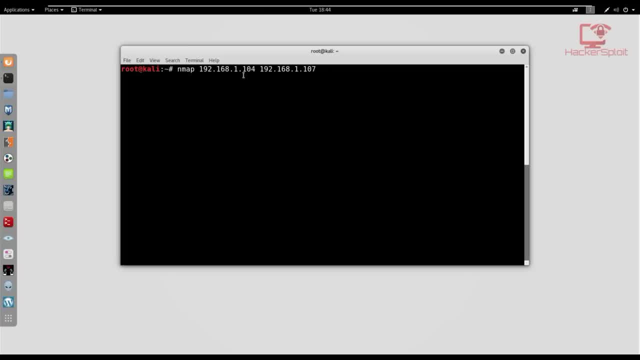 which is the IP address there, And that is how to scan for multiple targets. Now you can increase the amount of targets that you want to scan by just using a space And once you're ready, just hit enter And it's going to start the scan, Of course, depending on the type of operating system. 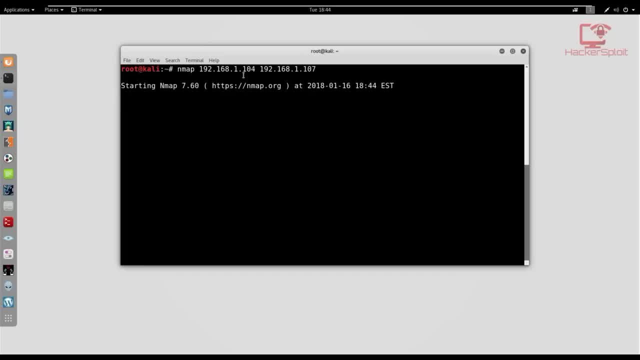 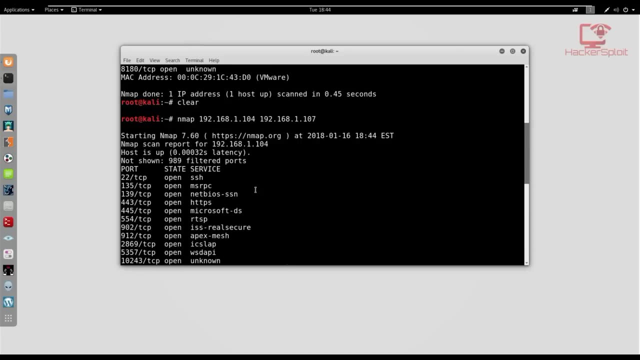 that your target or your host is running. it could take a bit of time, depending on depending on how the latency is and a lot of factors, But regardless of that, it's going to return the results, as you can see, And we can just move upwards. And now that the great thing is that. 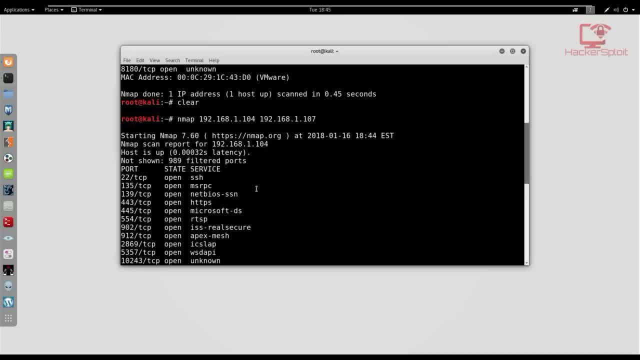 it sorts. it sorts the information or the output, or the results for us. Okay, so, firstly, as you can see, it gives you the information, the basic information that we looked at, And it has started the scan with the first one, as in the order that we initiated the scan. So the Windows operating. 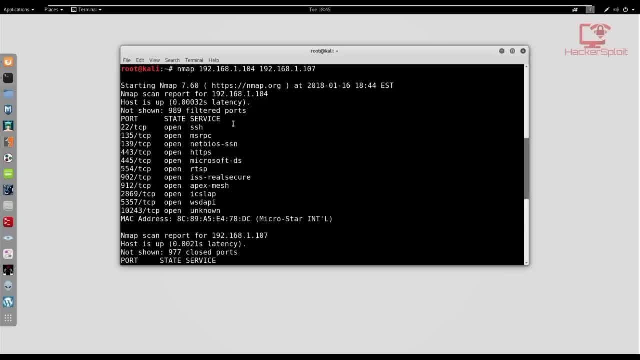 system first, and, as you can see, it has returned these ports with, with you know, the according services that are running on on the ports. Alright, so we have the SSH port, the HTTPS and the other ports that come with a Windows operating system. So, realistically speaking, 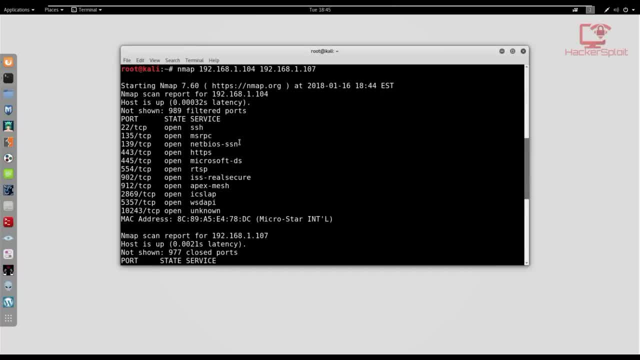 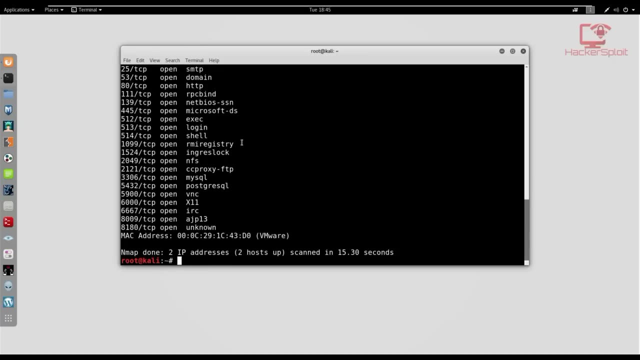 the Windows operating system is quite safe. Just by looking at the ports right Now, looking at the, the scan results from the, the meta exploitable to virtual machine, as you can see, which we already got previously, we can see that this does indeed. 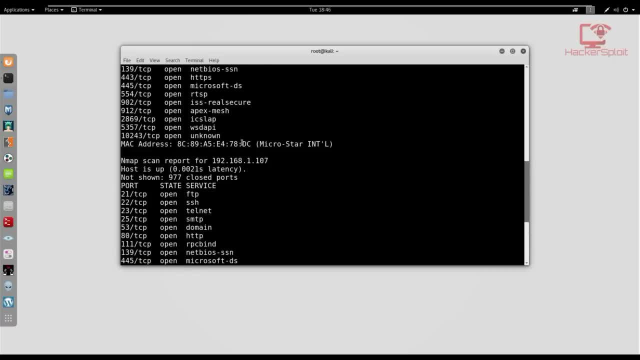 return the results that we got previously, And that is how one would go about scanning for multiple targets. Alright, so again, since all the targets are on the same subnet, if you have added them on the same side subnet, you can use a comma to separate them and you can add different types of results. Now, 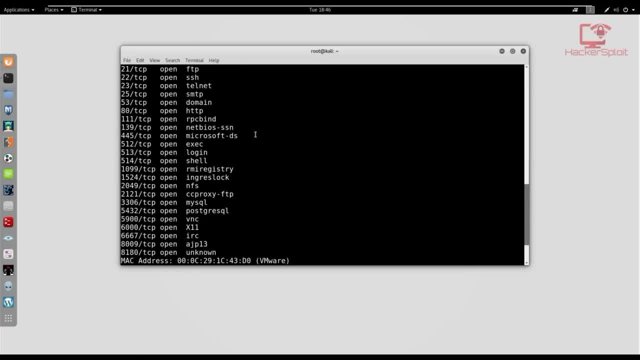 what I mean is, instead of scanning the way we did, using the syntax that we did, if the if you are two computers on the same subnet, what you can do is you can launch an Nmap scan and use the network range right. So, 192.1, 68,, whoops, 168.1, point 104.. Alright, so I want to scan 104. And 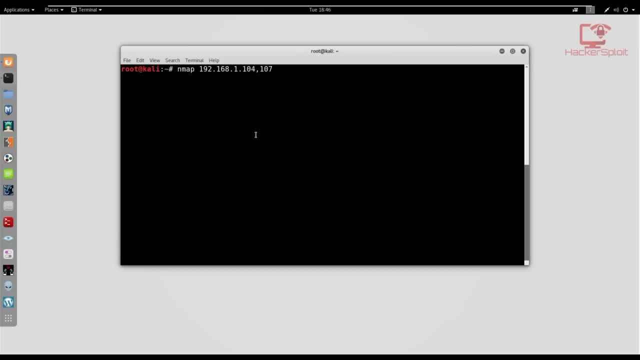 I want to scan 107. So I use a comma and 107.. Alright, so it understands that they're on the same subnet and it's going to scan the next IP address that obviously is identified with 107. So if I hit enter, it's going to return the same results that we had. obviously it's going to scan. 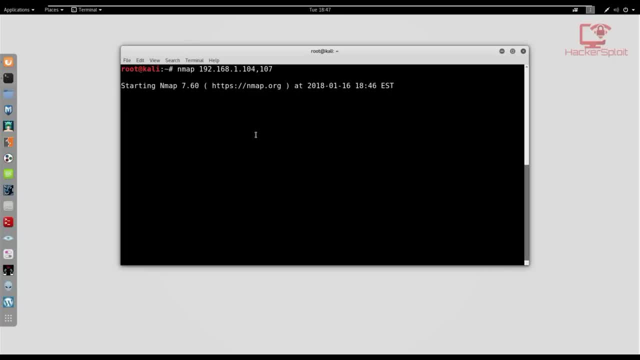 for the Windows machine first, and then it's going to move on to the, to the meta exploitable, to virtual machine. Alright, so again, I'd probably take about 15 seconds, similar to the previous one. There we are. this time it took 16 seconds And indeed it has returned the results as we. 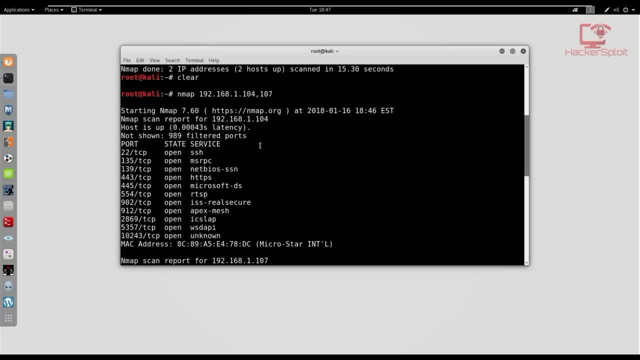 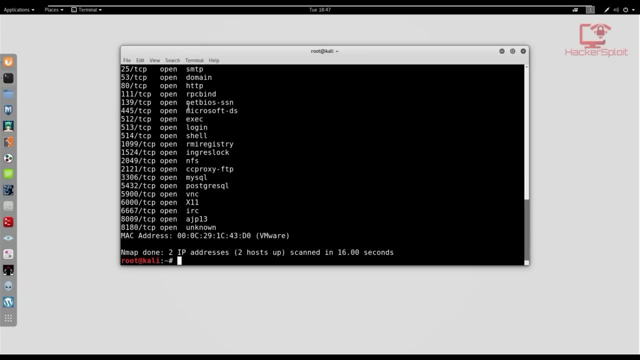 wanted them or as we needed them. Okay, so, as you can see, it's returned the results there And it has also returned the results for the. it has returned the results for the meta exploitable to machine there. So that is how to scan for multiple targets with the different types of syntax. 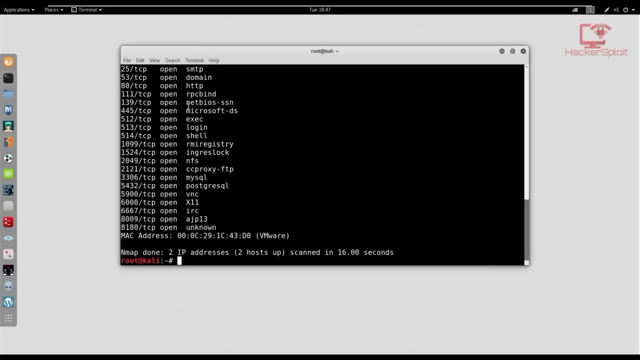 depending on whether or not the devices or the computers on the same subnet. But if they're not, you can go about scanning the two different hosts In that way, in where you use the space instead of the comma. Alright, so that's going to be it for 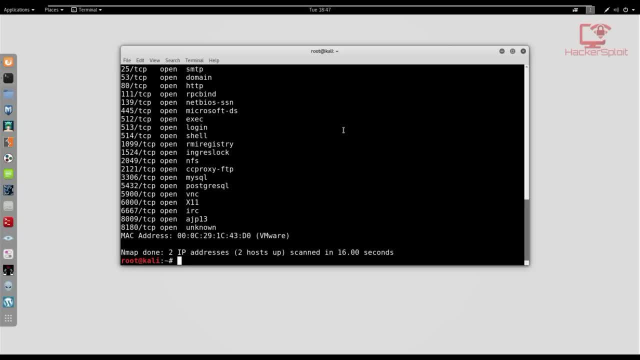 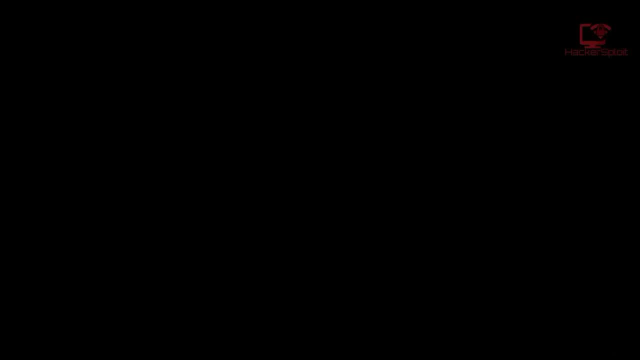 this lecture. Next lecture, we're going to be looking at how to scan a range of addresses or a range of hosts or targets. Alright, so I'll see you in the next lecture. Hello, everyone, welcome to this lecture. In this lecture, we're going to be looking at how to scan a range of IP. 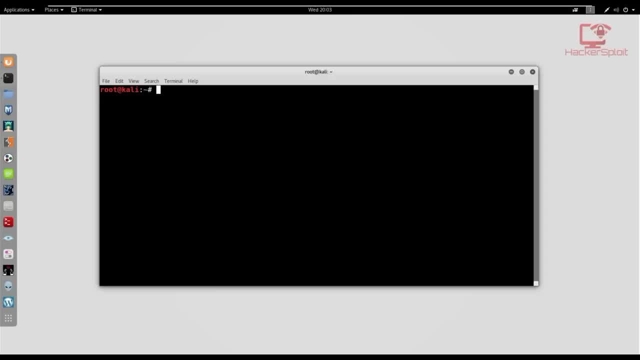 addresses, Alright. so why is this important? Well, the reason this is important is because IP scanning a range of IP addresses is good for target specification. Now, what do I mean? It simply can be used to scan, to specify. let's say you wanted to scan your entire network And obviously you specify it with a range. 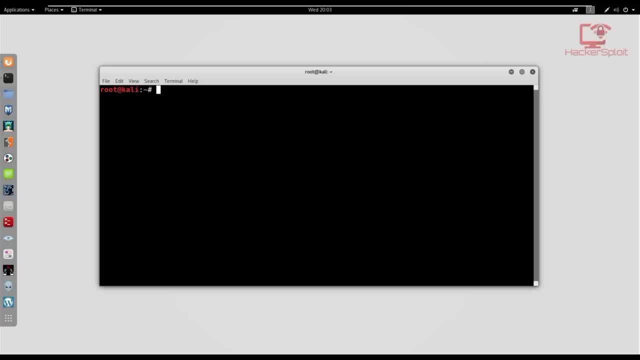 that you, that you want to specify. obviously, again, as you can see, this is where it really gets good with target specification. So let's say I only wanted to scan a specific a range of IP addresses. let's add: configured a subnet And I, you know a subnet that runs under certain. 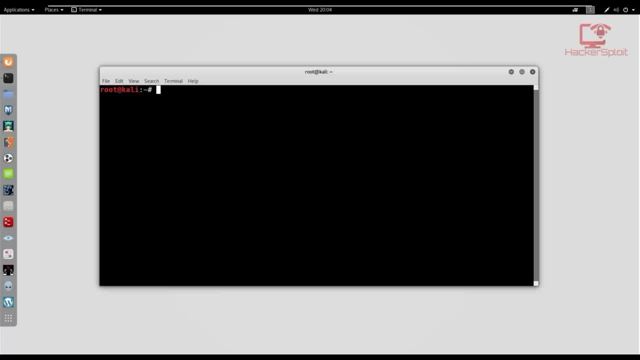 circumstances and I wanted to scan a range of IP addresses. All right, let's see how I could do that, And if you'll take this, stop, this will speed it up. This will speed it up your software, so you'll of IPs that belong to that subnet. So this is where this would come really, really handy Now. 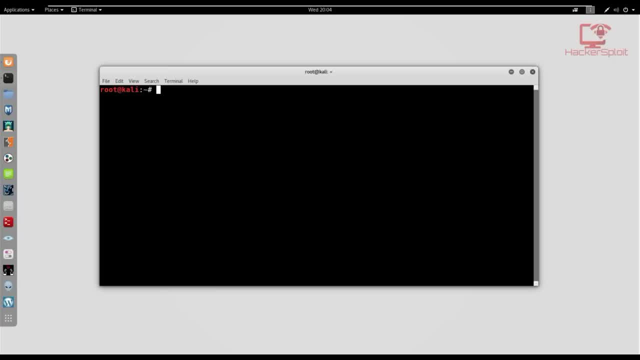 before we get started, I just want to show you guys a quick little command that will help you a lot as you try and master nmap. Okay, so this command is really very simple. It is the nmap help command. Alright, so you simply open it up with nmap And you use the help, which is. 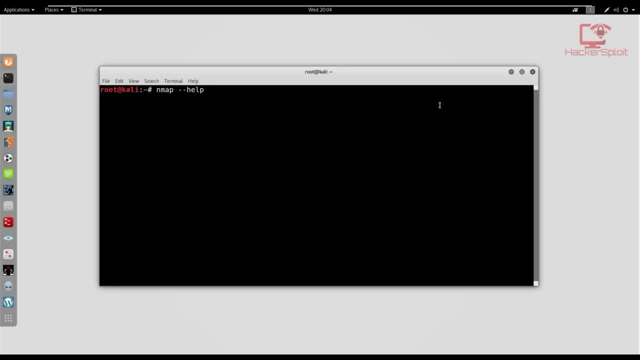 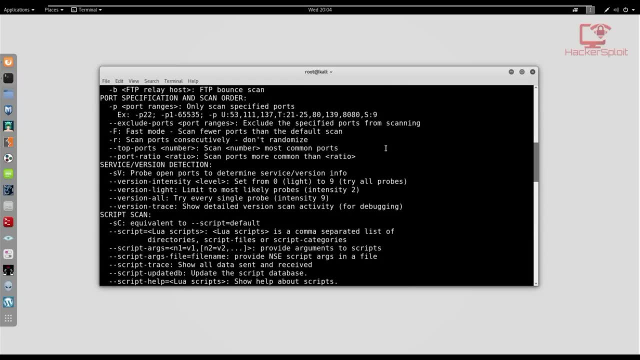 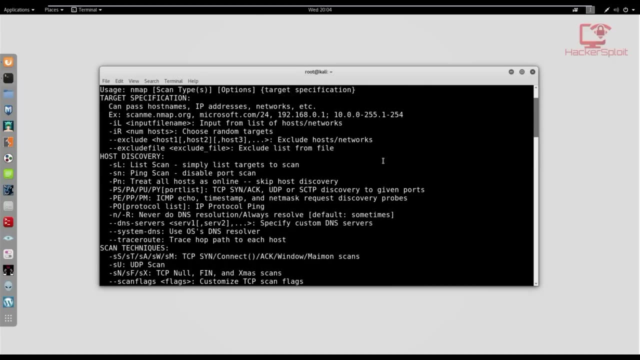 obviously beginning with the two dashes, Alright, and if I hit Enter, essentially it's going to return this long list of information. Now, this may seem really really confusing And you may be asking yourself, well, wow, this is a lot to take in. Well, the truth is, you just have to look at: 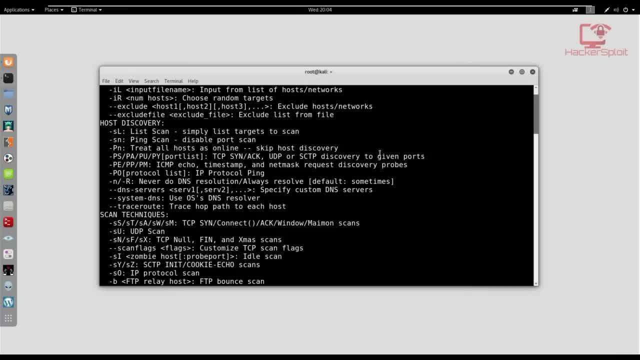 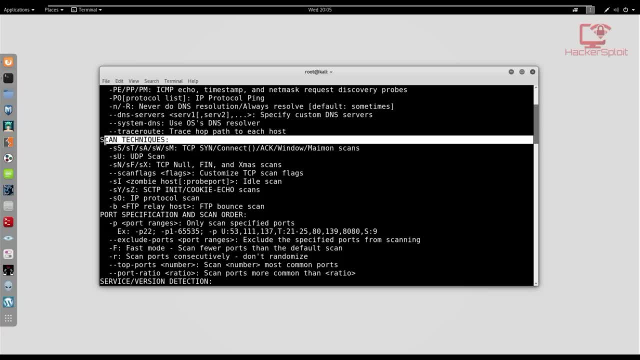 it And you shouldn't really focus on learning what each of these, each of these commands does. As you can see, it is specifying the different types of commands you can use And it is categorized under, you know, categories like scan techniques, port specification and scan order. 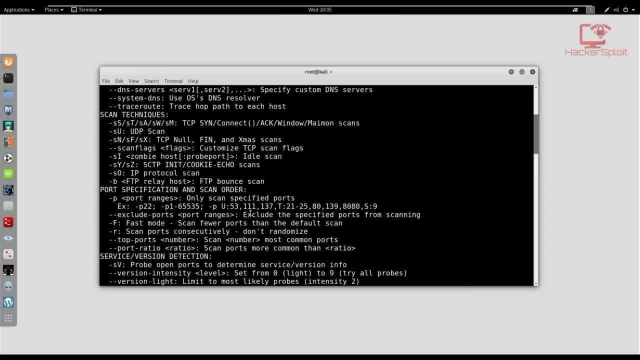 we'll be looking at all of this, But it is very important after you've gone through the course, if you look back here, you'll start seeing that you understand what each of these commands is doing, Alright, so I would really encourage you to go through this and understand it as well, Because it will really, really help. 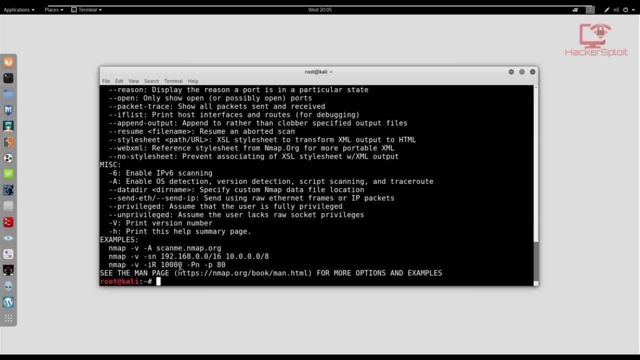 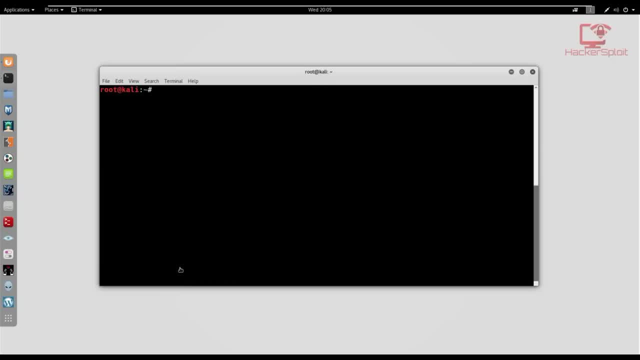 you especially moving forward as you look to master nmap, Alright. so let's get started now with scanning a range of IP addresses. Now I have, I have a local area network, alright, And on my local area network you can say: I have, you know, I have mobile devices, I have tablets, I have computers And 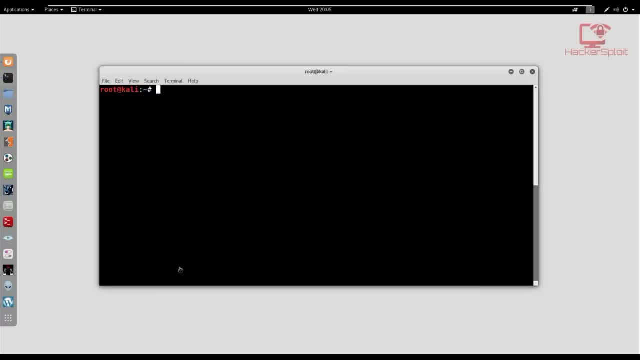 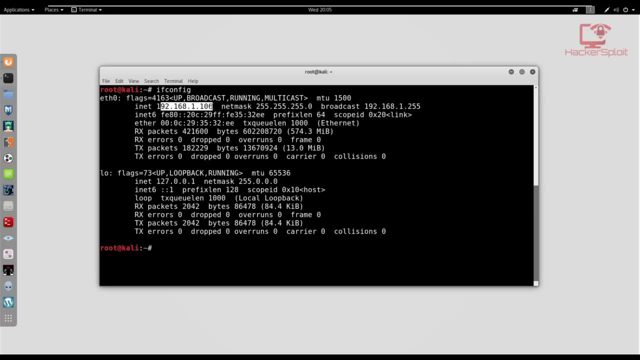 of course, the computer that I'm currently working on. Now, if I opened up the if config command, alright, this would display what my IP address is. Alright, so we do really don't care what this IP address is, because we are not scanning this. we want to scan a range of IP addresses, Okay. 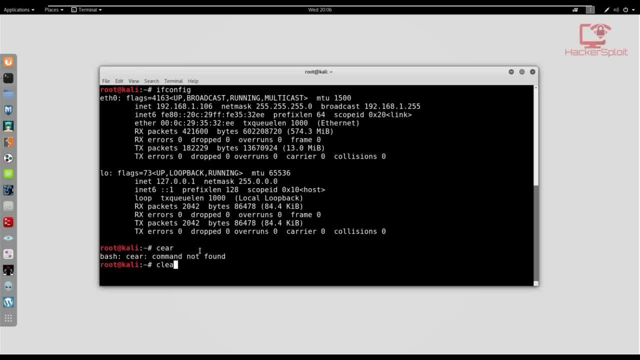 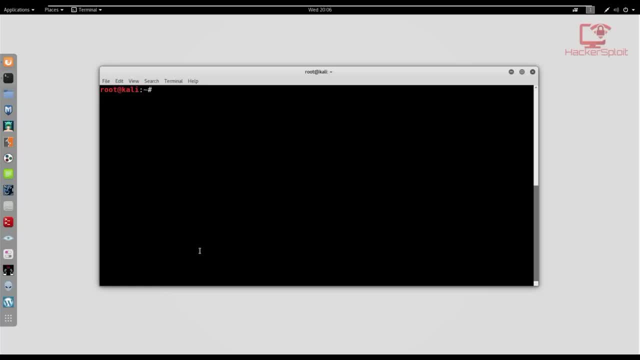 so let's say on our whoops. and let me just clear that up on our local area network, on your network, you want to scan a specific range of IP addresses. how would you go about doing this? Alright, so on my network I have actually created a subnet where all my I have two routers. Alright, 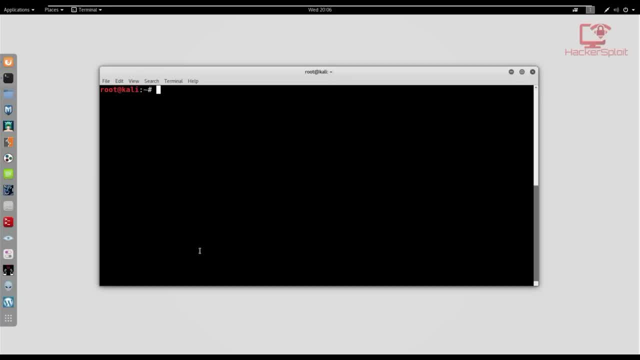 so, on my first router that I use for my Wi Fi connection, on my second connection, I created a subnet that runs under different, a different IP range, And I'll explain that right now. Alright, so let's get started. So, in order to obviously use the command, we have to start it off with nmap And 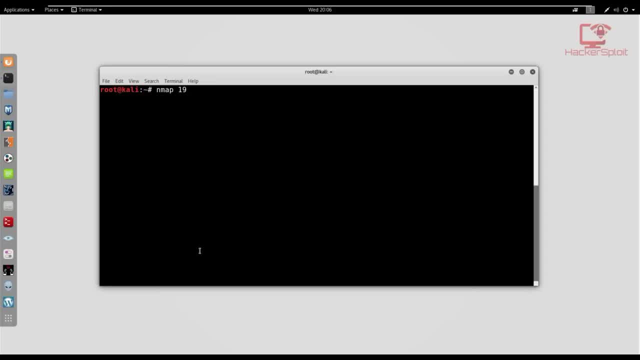 specify the range. now. Probably you already know what your default gateway is. your default gateway is is the- again is the IP address structure, and it's going to be pretty much similar here. So 192.168, Alright, and point one. Now, this is where I specified my own, my own subnet, Alright, usually. 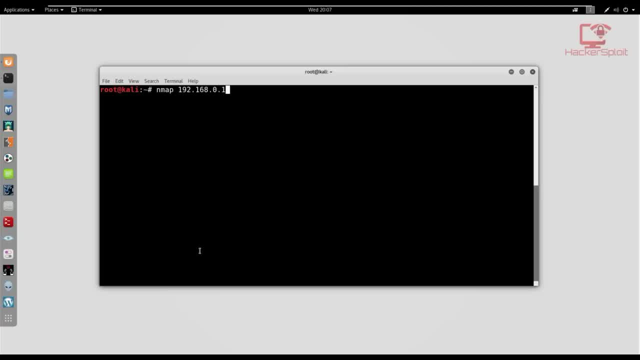 without, as they go about zero and one, okay for, and then you specify the range. But with mine I'm using a 1.1.. And then here is where you specify the range. Alright, so let's say you had about. you know you can, depending on the size of. 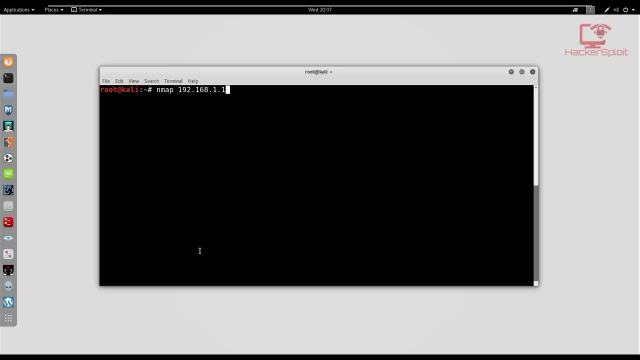 your network. I would recommend that you scan for a range of 100.. That will probably make sure that you discover all the devices on your network. Now my, as I've stated before, on my network I use DHCP, which means that my IP addresses are randomly. all the devices are randomly given different types. 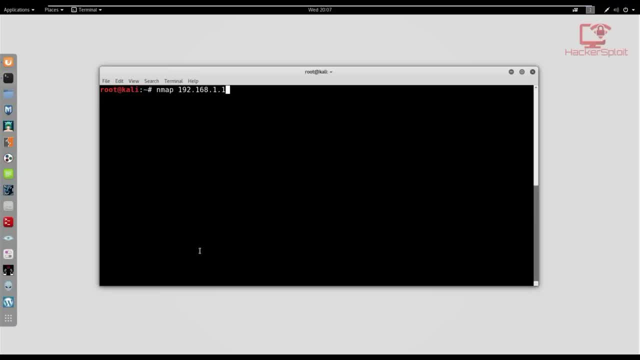 of IP addresses and that is to help with security. So I'll go larger range, like 200.. All right, And, as you can see, we're not specifying any commands, which means it's just going to perform a normal scan, the most basic of scans. So once I hit Enter, this will scan all the IP. 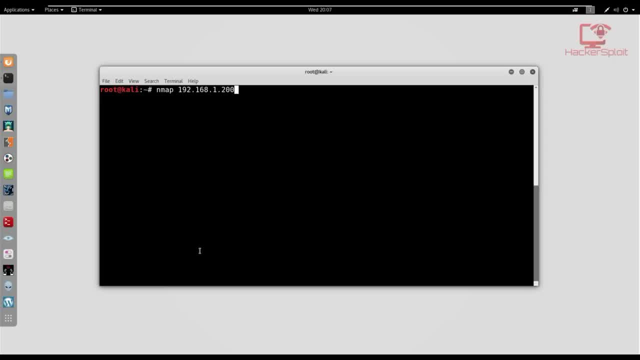 addresses on my network range And we'll obviously, if it discovers a computer is going to scan it and it's going to return the results. So let's hit Enter And whoops, for some reason I'm not getting a result. 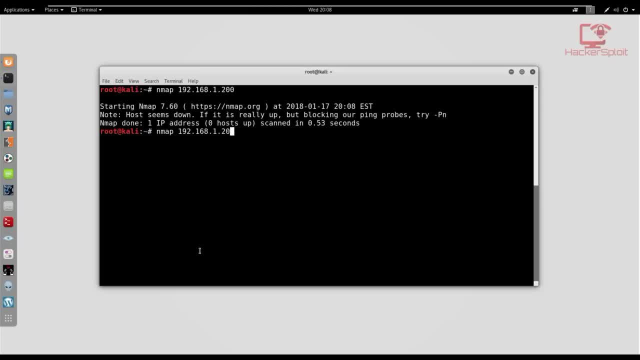 Alright, so I can actually show you my mistake here. Again, it's very, very important to get syntax right, So my mistake was not specifying the range properly. So one to 200.. All right, that's how you, properly, you know, assign a range that you want to scan. So I'm going to 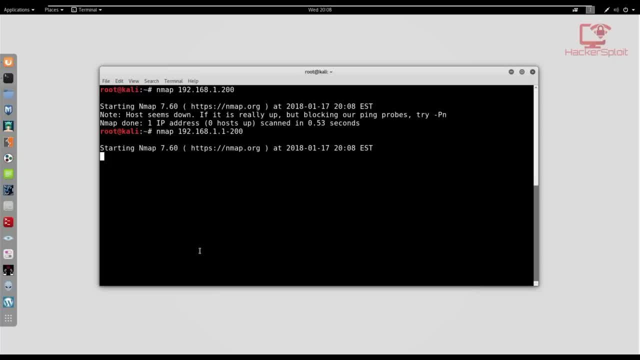 hit Enter again And it's probably going to take a long time, because there are 200 IPs that it has to scan through And out of all of those IPs it's probably only going to discover about like six or eight, because those are the 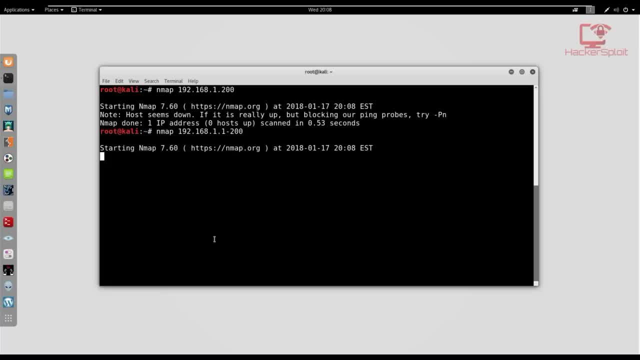 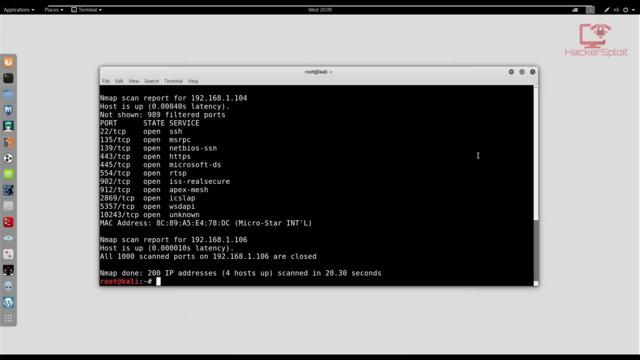 amount of devices on my network, So I'll get back to you when the is complete. all right, so the scan is complete and it has returned. as you can see the results here, I will give you a summary of the of these scan results. so and map done: 200 IP addresses. 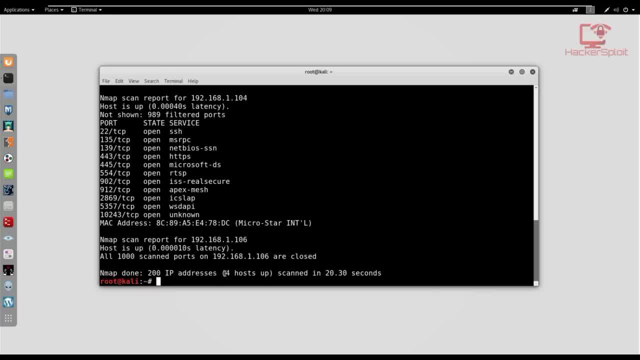 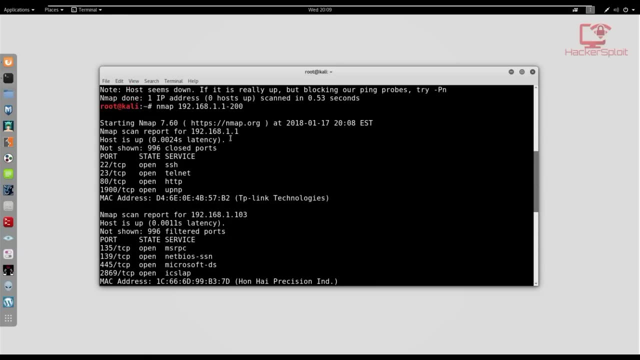 is scanned for 200 IP addresses, because we specify the range and it'll give us information about the amount of hosts that were up. so, essentially, I only have four devices that are currently online, and that is true. okay, so let's see what devices it returned. so this is where the scan began and the 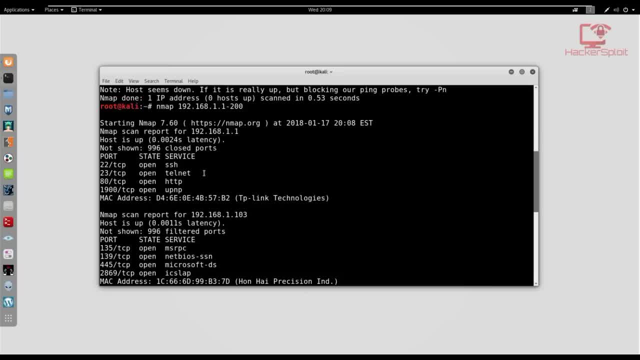 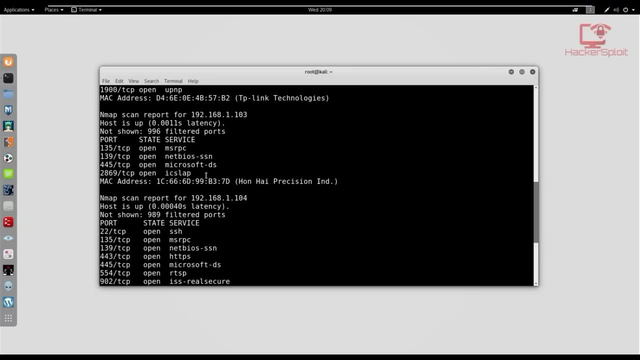 first scan was it actually detected my router. so, as you can see here, these services that are running on the different port. so we have our SSH port, our telnet port, which is always good to see you in a router, and that is something again that you really want to look at. closing all right now. 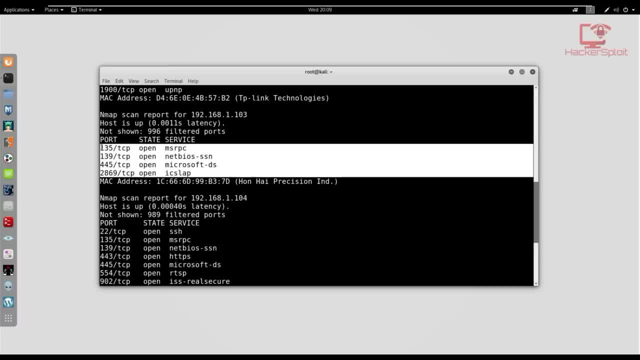 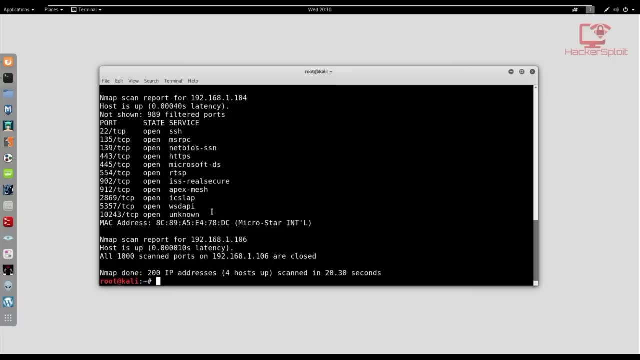 looking at the other computers, this is my other workstation and, as you can see, this is probably a Windows operating system because it has a lot of Microsoft services running on the different ports specified. okay, and finally we have this computer right here, which is, again, it's also running Windows, but I'm running Kali Linux on a virtual. 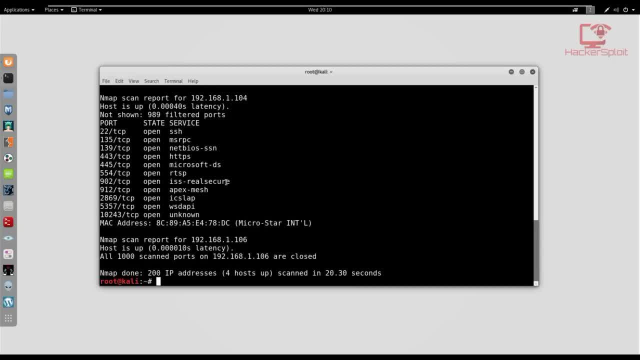 machine. I don't have metasploitable 2 currently running, so again, it's not going to detect that. so again, that is how to scan for a range of IP addresses and you can experiment with the different ranges that you want to scan for. and you can experiment with the different ranges that. 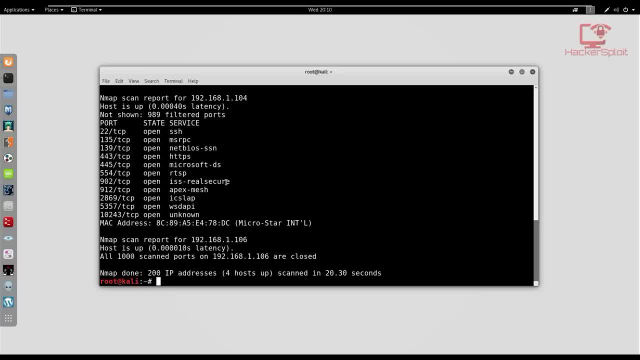 you want to scan for and you can experiment with the different ranges that you want to scan for you have on your network. and this will really come in handy for specialized networks where you have a different type of ranges. for example, if you know, in a, an enterprise environment where 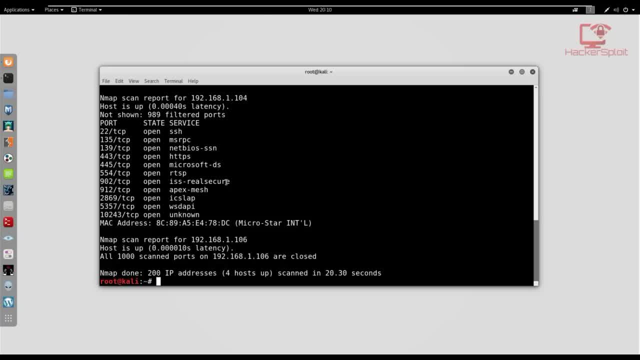 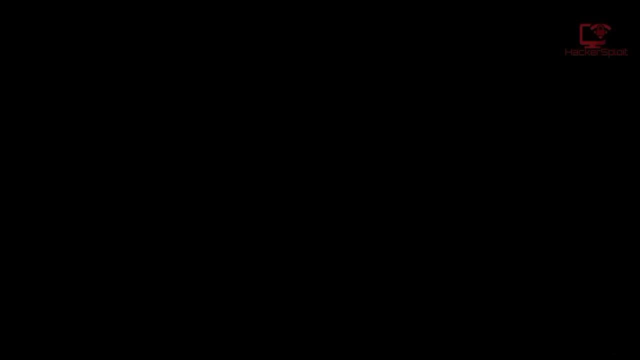 you would have different IP ranges for administrative computers, different for employee computers, etc. etc. all right, so that's going to be it for this lecture. in the next lecture we're going to be looking at how to scan entire subnets. all right, so I'll be seeing you in the next lecture. hello. 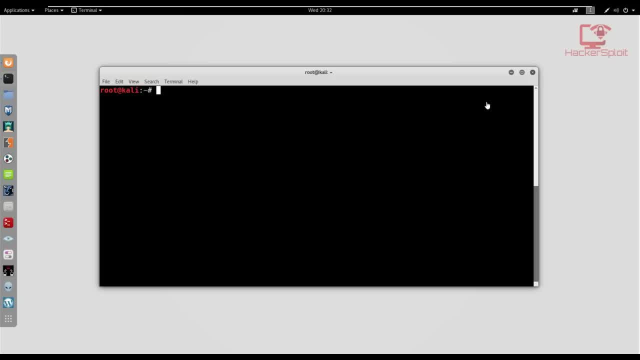 everyone. welcome back to my YouTube channel and welcome back to my YouTube channel and welcome everyone. welcome back to my YouTube channel and welcome to this lecture. in this lecture, we're going to be looking at how to scan an entire subnet, all right, so let's get started now. as we mentioned, or? 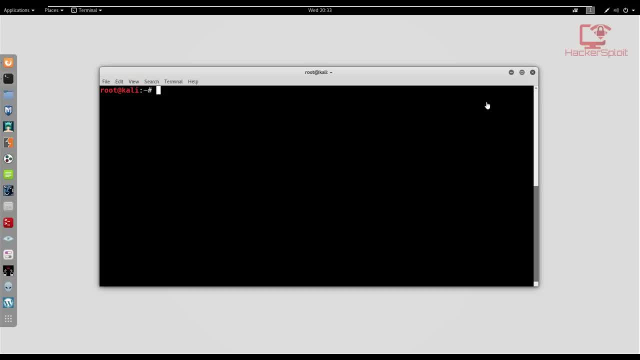 as I mentioned previously, in the previous video we looked at IP ranges. now the thing with subnet is obviously: a subnet is a subdivision of a network. all right. now I have two subnets on my network and they're very, very simple to understand. I'm pretty sure you already understand this. my first subnet is: 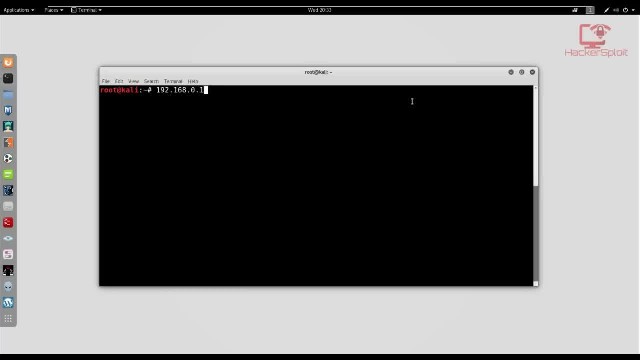 one, 82, point 168, point zero, point one, all right, and my second one is one eighty two point one. sixty eight point one, point again point one, and which is what we looked at previously. this is my, this is what. this is the subnet that I use for all my computers and for my office, right the other. 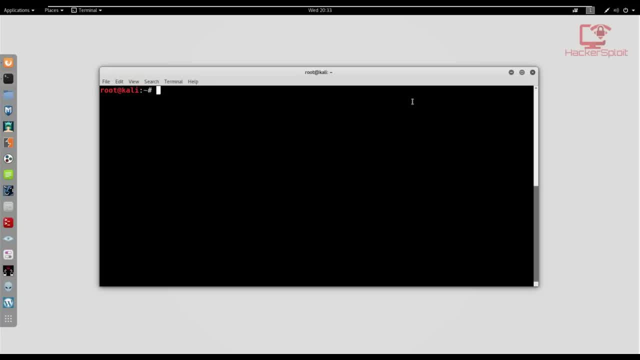 subnet is for my Wi-Fi network and is- again I really like to keep it- for wireless connectivity. all right. so if I wanted to scan an entire subnet, what this would mean is I would have to use this, the inter domain routing- Alright, so essentially, we can do this really simply, So I'm going to try. 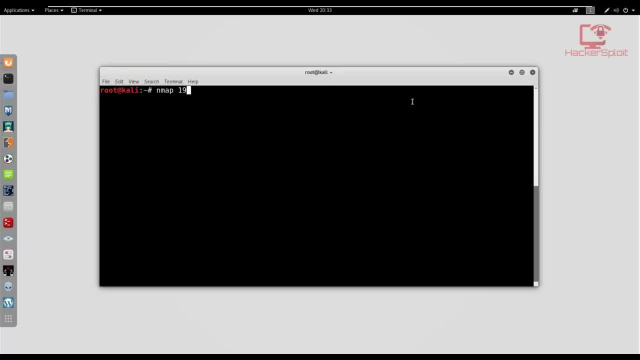 and scan my Wi Fi network. So nmap, Alright, 192, 1.168.. But in this state I'm going to, I'm going to use point zero, that is the other subnet, And then I would specify, I would specify point one. 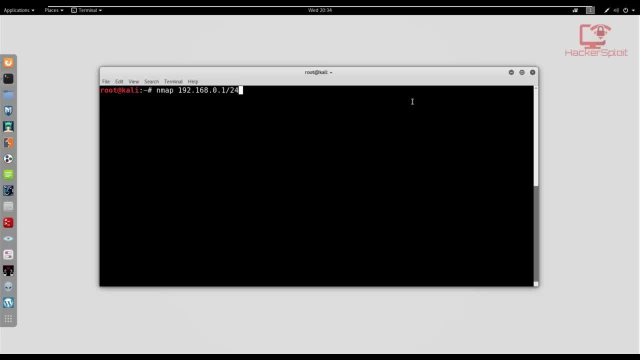 and then I specify the subnet, which is the subnet mask is 255.255.255.0,, which is also denoted by the slash 24.. And essentially, this will scan all 20 256 IP addresses under the subnet and will return which which hosts are currently up and the ports that are opened, filtered, closed. 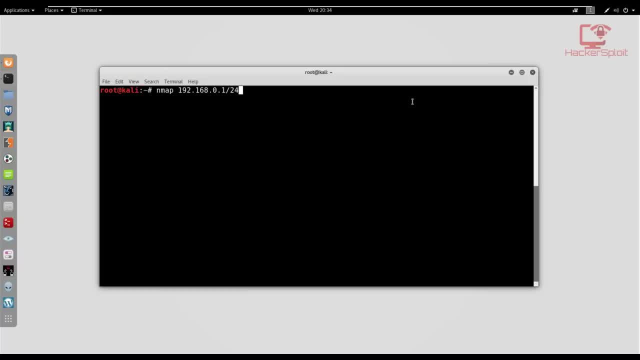 and the service is running on them And, again, since we're not using any commands, it's going to assume or nmap is going to perform a very basic scan. So once I hit enter, it's obviously going to start up the scan. And you know the scan is going to take quite a while because it's going to scan. 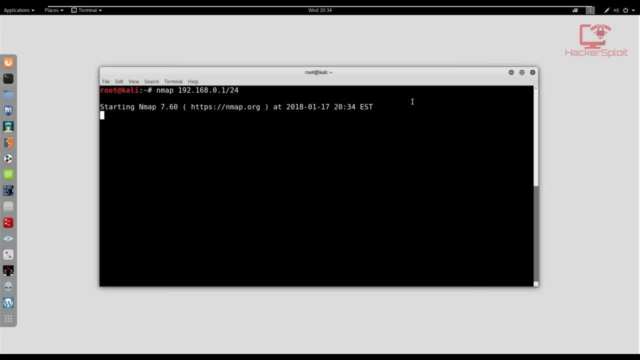 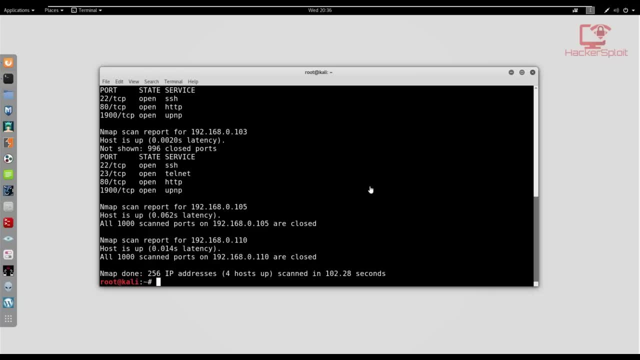 through all the 256 IP addresses. So again, I'll get back to you when the scan is complete. All right, so the scan is complete and it has. it has returned results. So let's take a look at what it returned. So it scanned the subnet And, as you can see, it scanned the entire subnet. 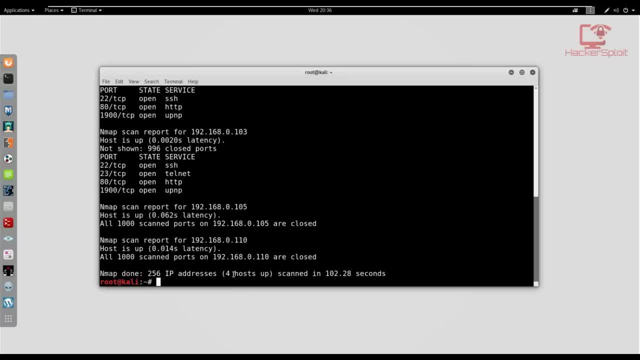 which was 256 IP addresses, And it detected that only four hosts were up in the time of 102 seconds. Alright, so not too long there And there we are. So now we're going to go ahead and run the scan And, as you can see, we're going to run the scan. So now we're going to run the scan And, as you can see, we're going to run the scan And, as you can see, we're going to run the scan And, as you can see, we're going to run the scan. So it has returned. 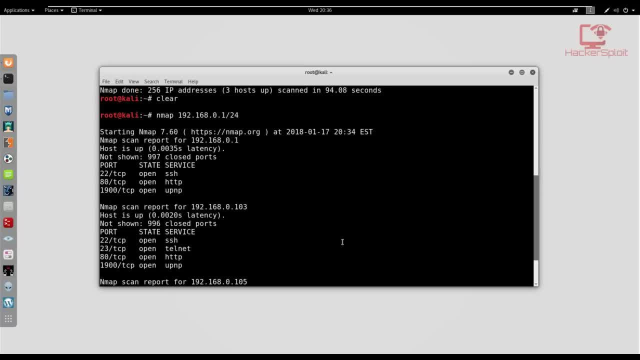 results for the devices that are currently on my Wi Fi network And, as you can see, there we are. these are the ports and the services, the respective services that are running over there And, as you can see, this is perfect. It has scanned every device under the subnet that I 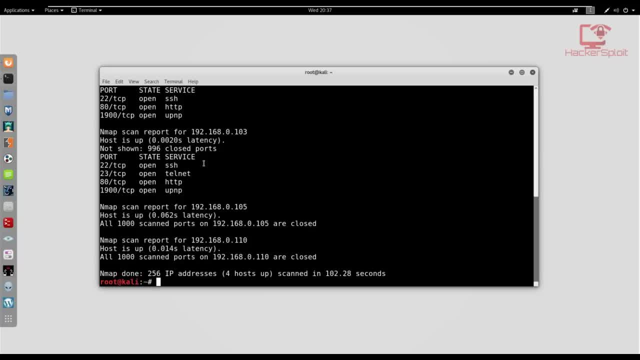 specified it to. And again I can specify the different subnet. For example, if I wanted to specify my older or the subnet that I use for my, for my office, I can do that and return all the IP addresses under that subnet. Alright, so that's how to scan an entire subnet. Of course this is. 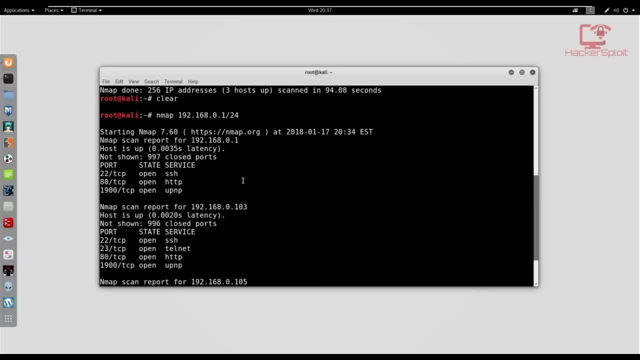 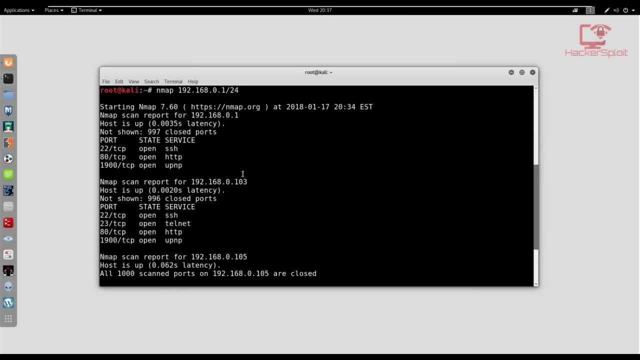 quite simple to do And, as you can see, I'm- I hope you're- learning a lot out of this- and how to differentiate subnets from an IP range, And really it comes down to how your network is structured, or how the organization network is structured, And once you have a good idea of how that all 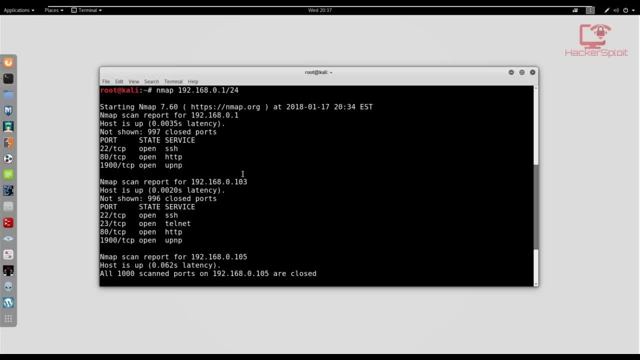 works. performing scans or specialized scans is going to be really, really awesome, And we'll be looking at how to incorporate that into your network And once you have a good idea of how that all works, you can incorporate commands with them to perform very, very specialized scans on. 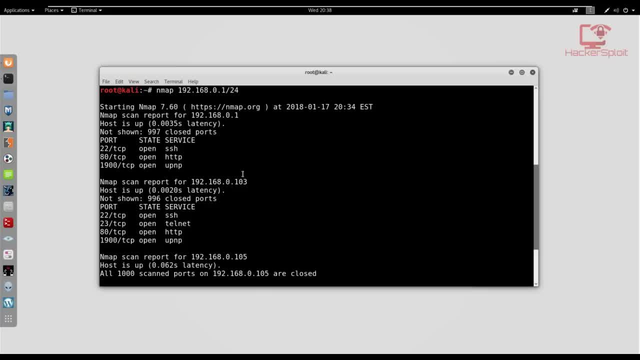 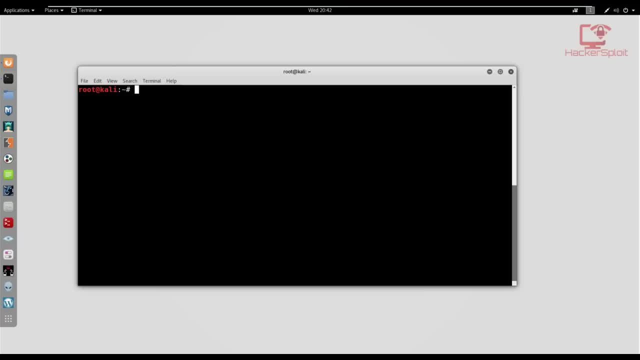 targets, hosts, subnets or IP ranges. Alright, so I'll see you in the next lecture. Hello everyone, and welcome to this lecture. In this lecture, we're going to be looking at how to scan a list of targets. Now we might be sitting there asking yourself: what exactly do you mean? 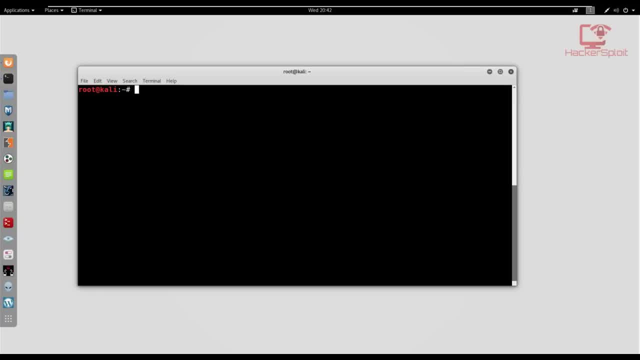 Well, let's take an example. Alright, let's say you have a large number of systems or IP addresses that you want to scan. Alright, so you can enter all of these IP addresses you know in a list, in a txt file. 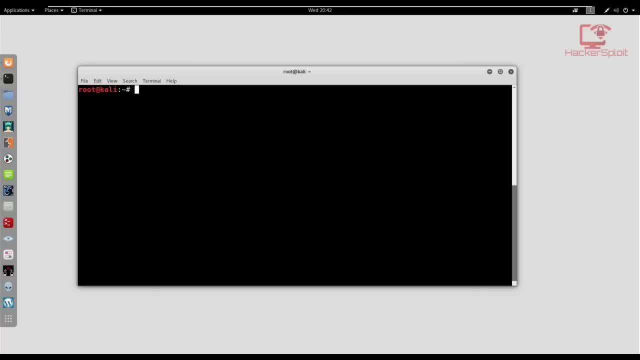 and then you can input that into N map and perform the scan from there. So again, you might be asking yourself: why is this important? Well, take in, for instance, you have a certain amount, a certain ip addresses that, let's say, for example, are running the or are actually servers, and you want to be. 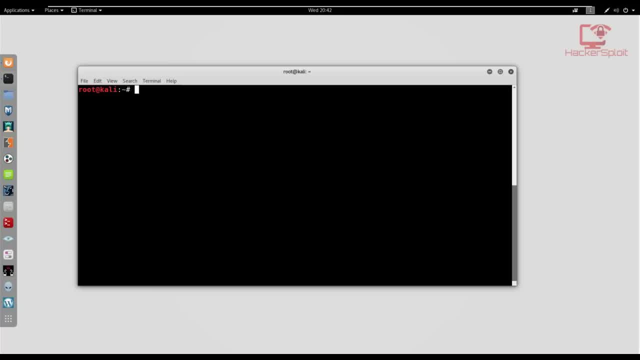 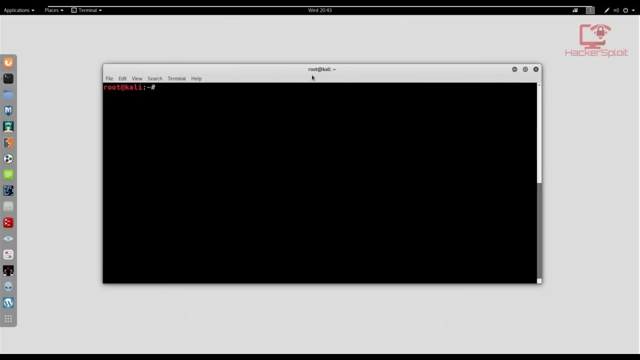 performing regular scans on them to make sure that everything is, you know, in order, making sure that the ports are correctly configured, etc. etc. Alright, so what I'm going to do is I'm actually going to do this right now. So, as you can see, I'm I'm in my terminal. Now you can do this in. 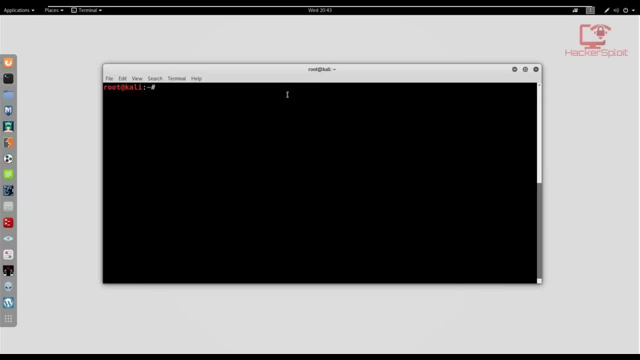 any operating system that you choose to run. All I encourage you to do is to create the list, or in your working directory. In my case, I'm going to do that in my desktop. So I'm going to change my directory to the desktop And what I'm going to do is I'm just going to create a new file here. 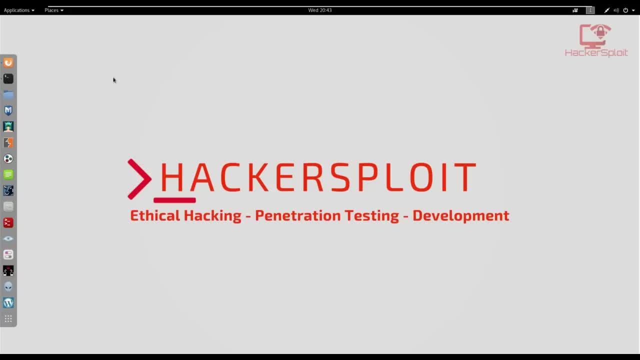 Alright, so I'm just going to minimize that And, again, you can use any text editor that you want. So I'm going to use leaf pad, which I have here, And well, in here I can specify the IP addresses. 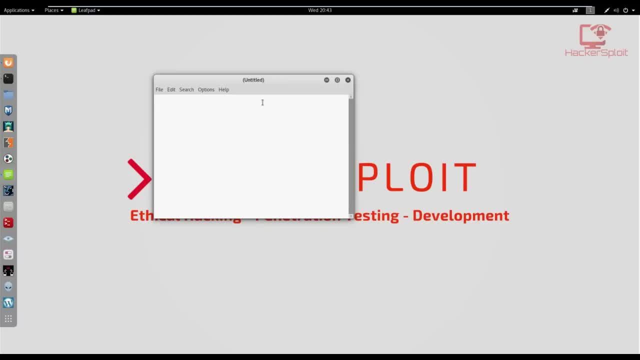 So it's really very simple to specify them. So let's say I specified 192.1, 68.1 point 104,. right, whoops, point 104.. All right, 192.1, 68.1 point 103,, which is all. 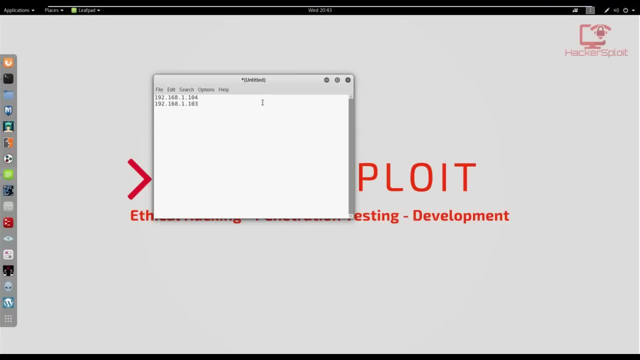 these are devices that are currently on my, on my network. So, let's say, I only wanted to scan those two IP addresses. So let me, I'm going to save this on my desktop. Alright, so desktop, as I can just call it, targets dot txt, right, dot txt. That's very, very important And I'm going to save it. 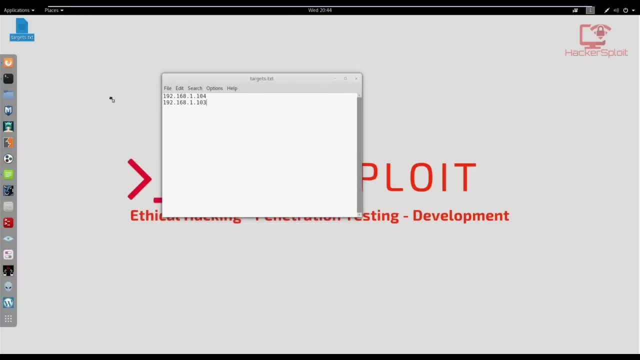 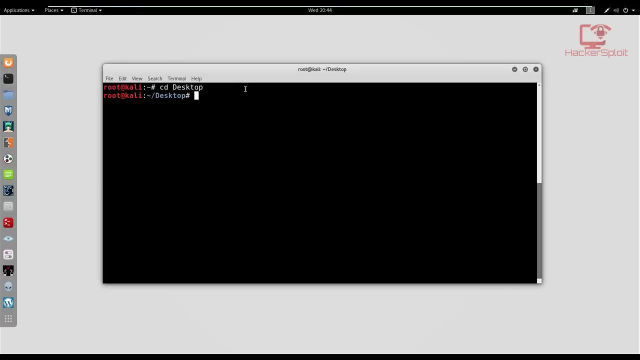 there And just give it a few seconds. There we are. So there's the file, So we have actually created it. And then let me close the leaf pad text editor. And then now you might be asking: Well, what do we do now? Well, the first thing I'm going to do is I'm 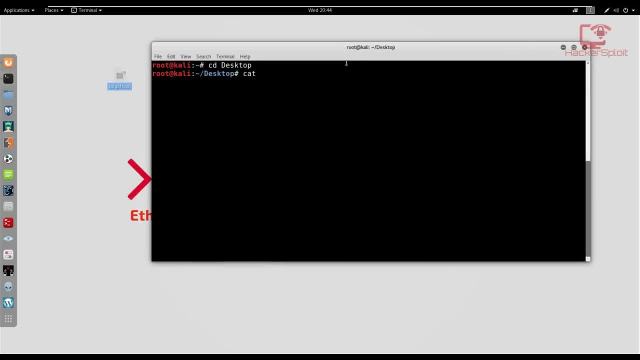 just going to try and see if I can get the results to print out on the terminal. So targets dot txt. And there we are. we can see the. we can see that the IP addresses there. So what I'm going to do is let me just clear the terminal and we can get started with our scan. So the syntax is really. 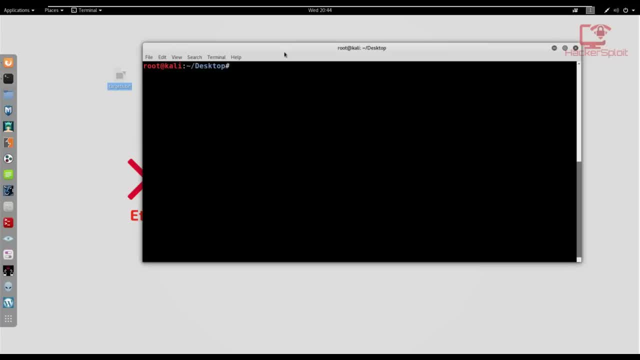 very simple. All right, Now the list has to contain IP addresses. So let's say, I want to say you know that should be scanned. And again I give you an example: If you had special, you know computers that you're giving high priority to, this is a great way of doing it, Alright, So 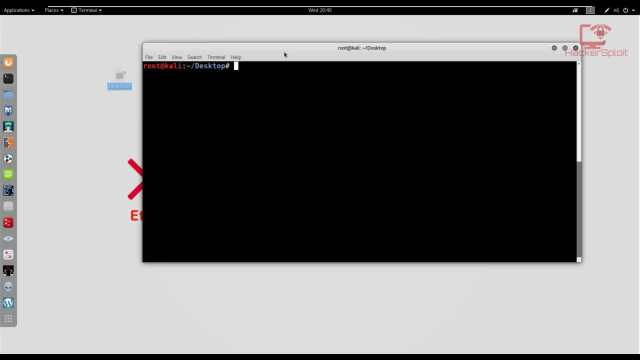 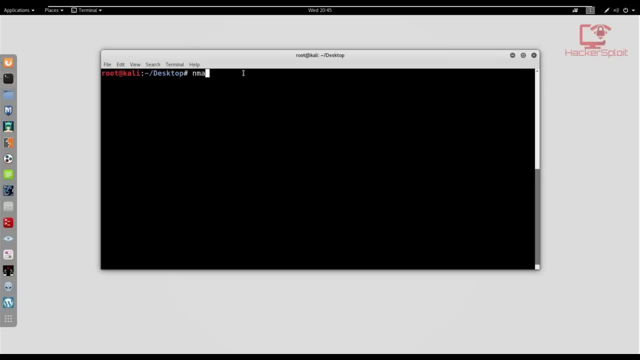 in this case, we're going to get started with our first command or parameter Alright, and the parameter is the IL parameter. Alright, so let me, let me show you how this works. So we started off with n map Alright, and now we use the parameter or the command IL. So is the dash, now all commands. 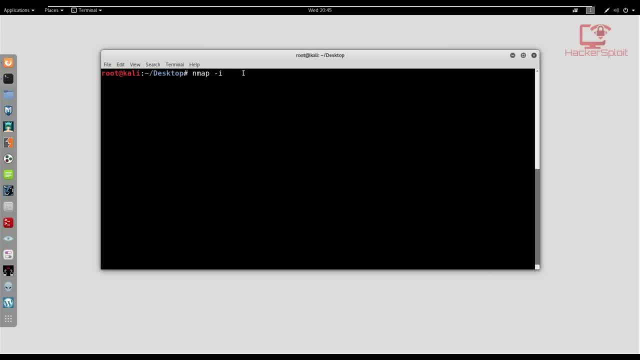 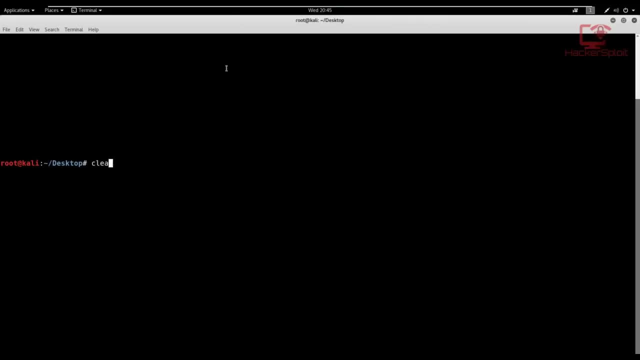 are going to follow this syntax And then we use a lowercase, a lowercase l I, sorry, a lowercase i, followed by a large l, All right, So let me just enlarge this, Let me clear and let's do that again. So, n map I and L All. 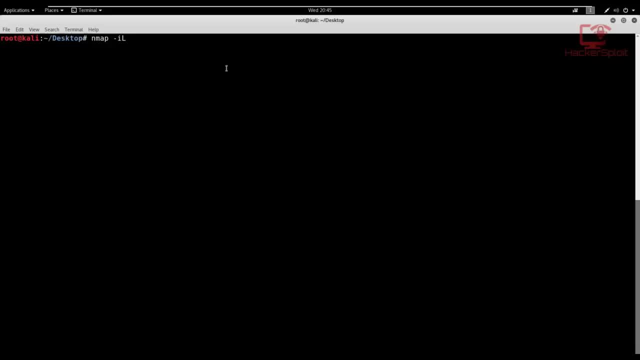 right, so the IL parameter, and then we specify the name of the list, which in this case we know it as targets right, targets dot txt, and we give the extension and hit enter All right, and it's going to start and map, as you can see. 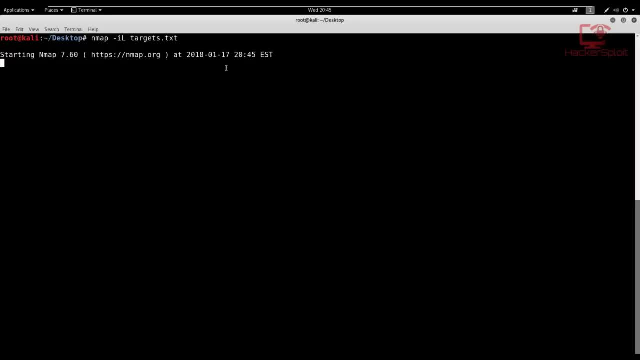 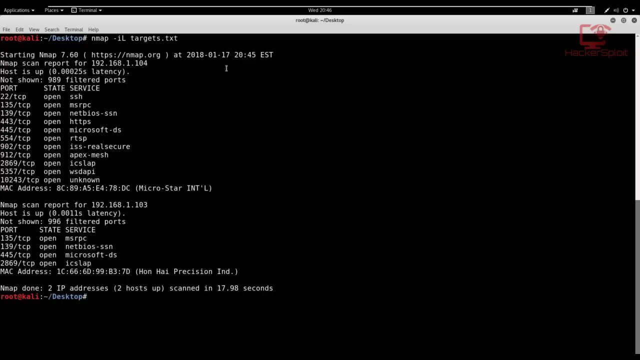 so it already knows what we're telling it to do And, given the parameter, the IL parameter, is used to its Well. it essentially tells n map to extract the targets from the list that we have specified. So it really is telling n map. hey, look here. I want you to take these results in this, in this txt. 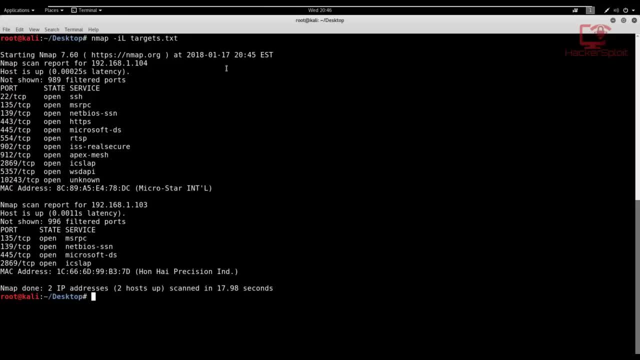 file And I want you to scan them with any other parameters that you have specified, which in this case, we know we haven't specified any. All right, so let's go ahead and do that. So, let's go ahead and do that. So let's go ahead and do that. 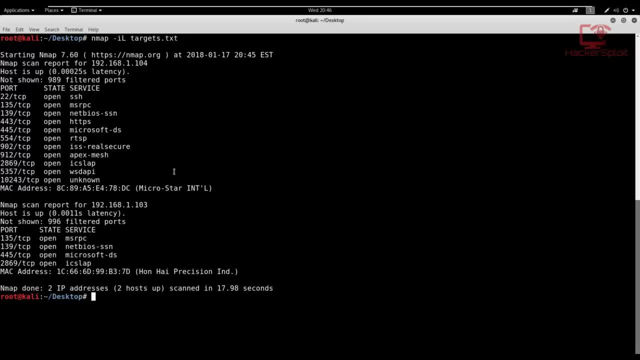 And, as you can see, it has returned And these are the two Windows computers running on my network And it has completed the scan. As you can see, note, two IP addresses scan and two hosts were up, scanned in 17.98 seconds And you can go ahead and analyze the results, But for now the results are. 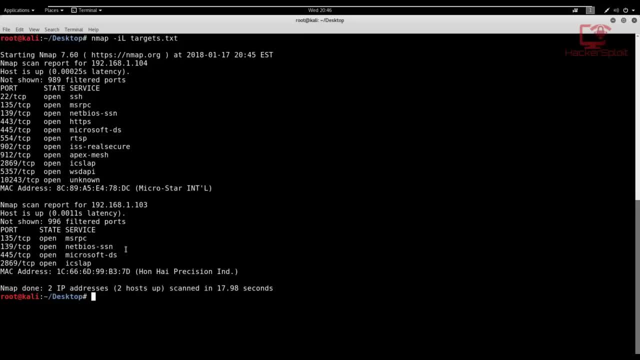 not that important because we're not really looking at that. we're just getting acquainted with n map, Right? So that is how to perform, or how to scan a list of targets. All right, And that was pretty simple. I hope you guys get the gist. So the IL command essentially allows you, or is allows you, to specify. 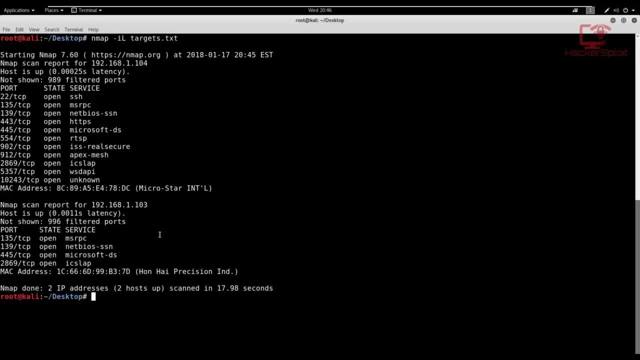 to n map to get the to get targets or IP addresses from a list that you have created, and you can also specify the location. All right, so that's going to be it for this lecture. I'll be seeing you in the next lecture. 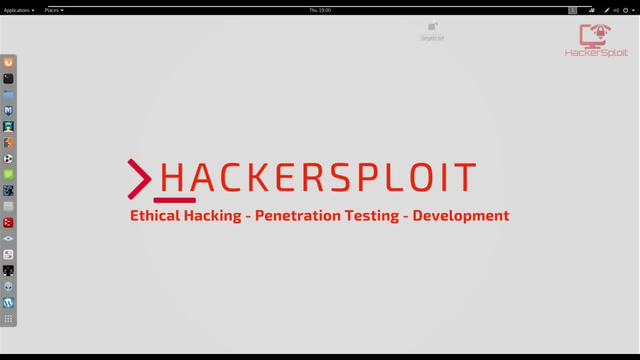 Hello everyone and welcome to this lecture. In this lecture, we're going to be looking at how to exclude targets or IP addresses from a scan, All right, So simply put, we're going to be looking at how to exclude a certain IP addresses or a specific IP. 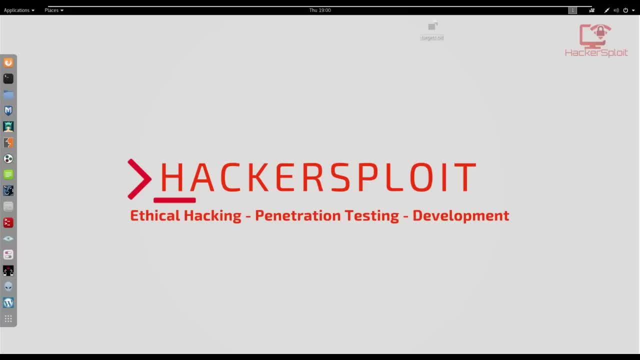 address from a scan. So let's say you wanted to scan a subnet but you wanted to exclude some IP addresses for the, you know, for the sake of saving time. or you just want to, especially, you want to specialize your scan onto a certain number of computers and obviously excluding one. All right, 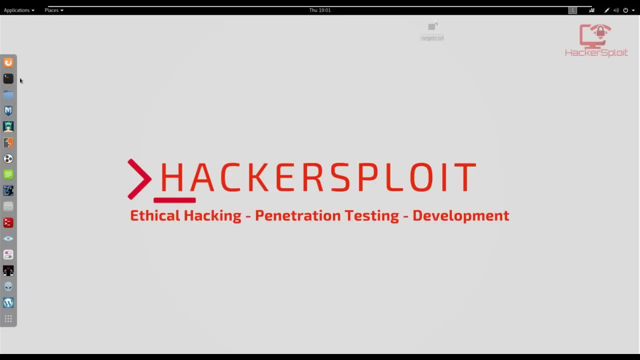 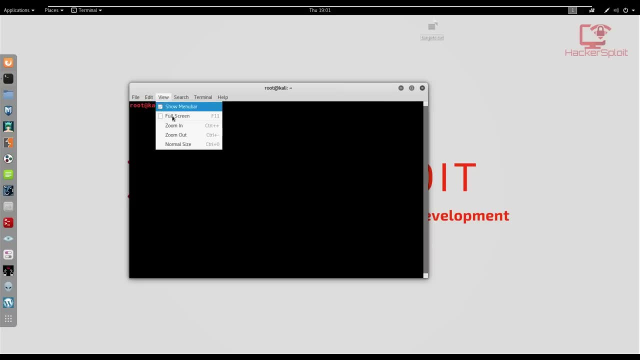 so let's get started Now. what we are going to be doing in this lecture is I'm going to perform a scan on my subnet, which is my local area network. All right, so let me just zoom this in So we have a- you know, a good picture of what's. 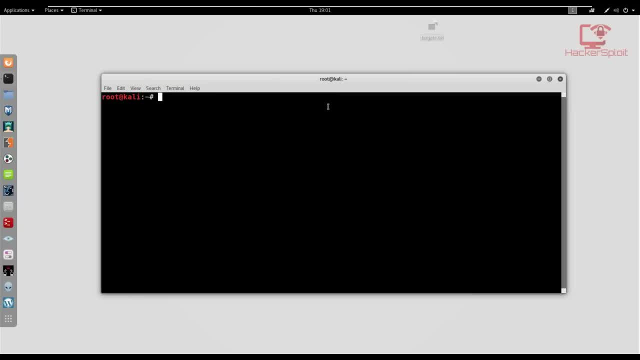 going on All right. So essentially, what I'm going to do is I'm going to scan my subnet And I'm going to exclude my Windows operating system or my- my current host operating system in which I'm running this virtual machine on All right. so I'm not going to exclude my Kali Linux, of course it's not. 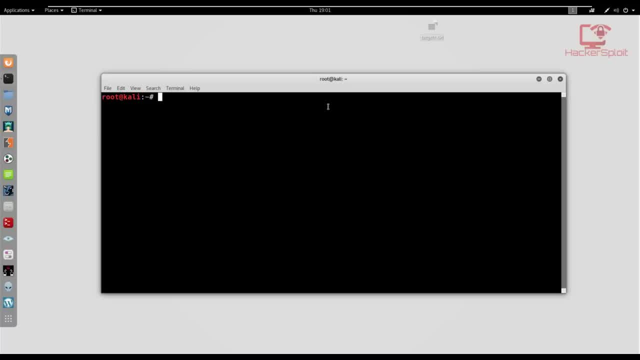 going to scan the own computer, But nonetheless I'll be excluding my Windows so that you can see that it does work All right. so, simply put, we're going to be using the nmap command, And let me just enlarge this so we have a better idea of what's going on. So I'm going to 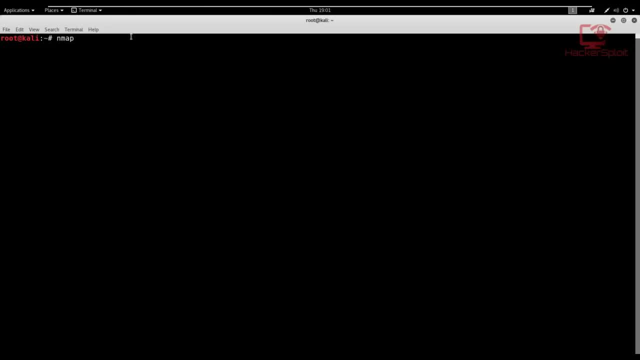 enlarge this nmap And now we specify the target And then we use the, we use the parameter exclude And then with that is also followed by the target that we want to exclude. All right, So in this case we are scanning a subnet. 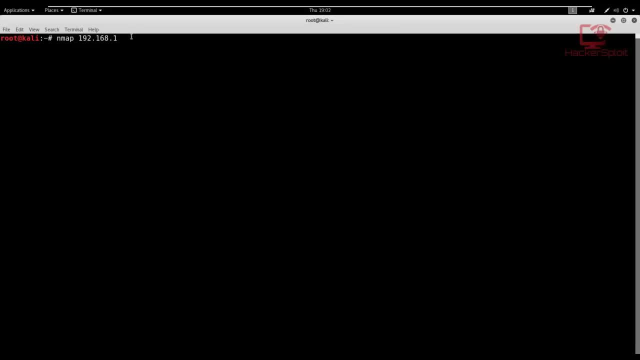 192.168.1. All right, 0.1 and 25.1. four right, you're scanning the entire subnet, But again we're excluding the Windows operating system or the Windows computer on my network. So to do that we use the double, double, dash and hit. 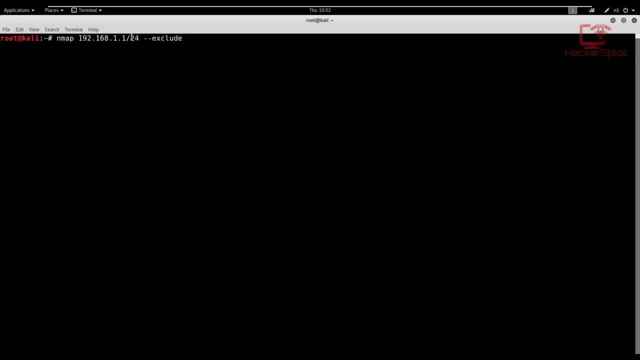 exclude, Very, very simple exclude. And after that we give the targets or the target that we want to exclude. So we could say 192.168.1.104.. That is the IP address of my Windows computer. that is on my. 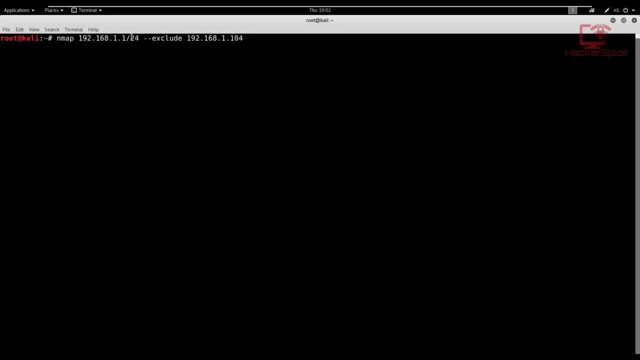 network. All right, so once I hit enter, it's going to perform the scan and it's going to exclude that operating system. So let's hit enter And let's see what results we get. All right, so the scan is started and I'll get back to you when the scan is complete. 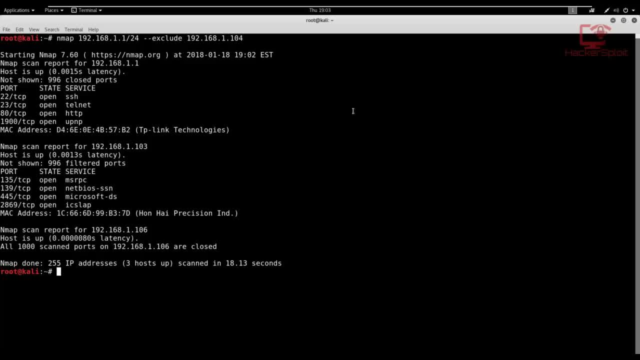 All right, so the scan is complete And, as you can see, to return the results. and it's only the only devices that it managed to get on my network And I, specifically, I did that purposely, I only left my other Windows workstation. 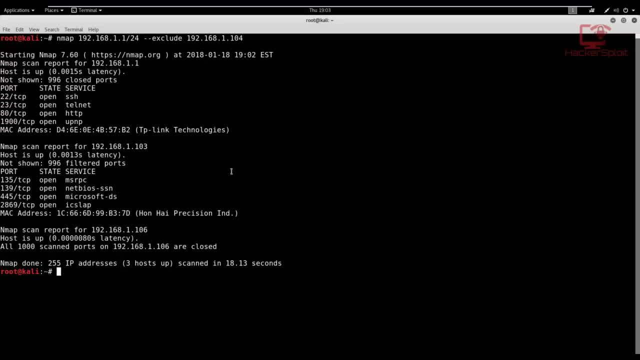 Currently online and the router obviously. So, as you can see, it did work. And just to prove that it did work, I'm just going to get rid of the exclude Right And I'm going to try and, being my, I'm going to try and scan the windows, the 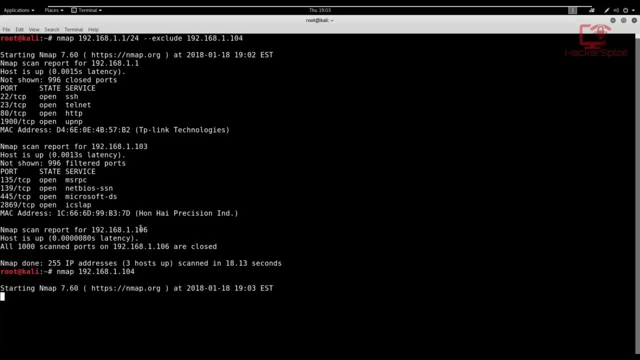 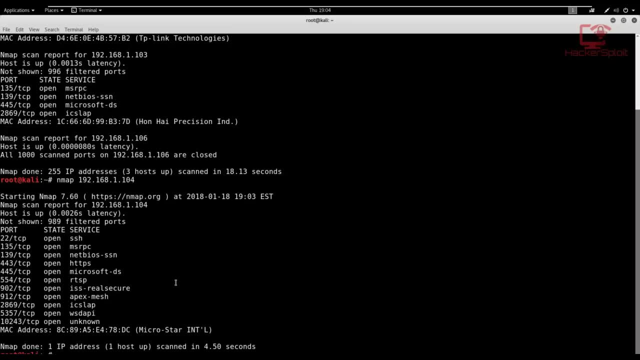 windows machine that I did exclude from the scan. So I'm just gonna hit enter And you'll probably see that it will get the results. it will scan and they, as you can see, it has got it there Fantastic. So we know that the exclude 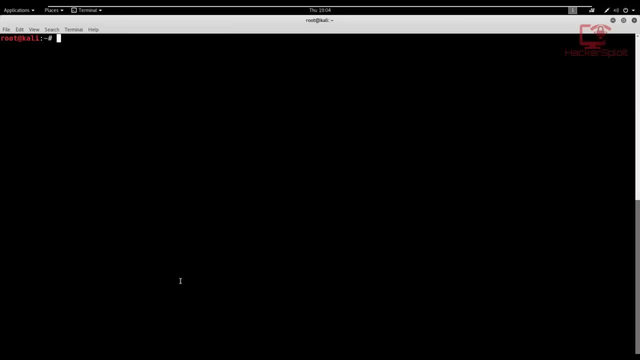 does work and how it works. now looking at at some other options that you can use with the exclude command, as I said, you can specify more than one target, all right. so the exclude option is very useful if you want to exclude specific hosts, let's say when scanning a large number of addresses, all. 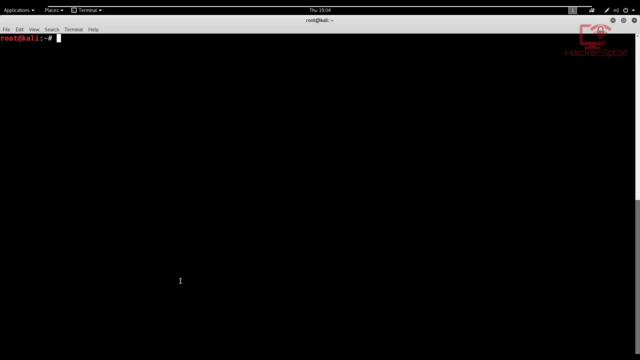 right. so let's, let's look at an example here in which we can use this. all right, so what we're going to do now is we're going to just scan an entire subnet, so nmap again, 192.168.1.1, the subnet 24, and we're going to exclude- right now, we are going to exclude a range, all right, so. 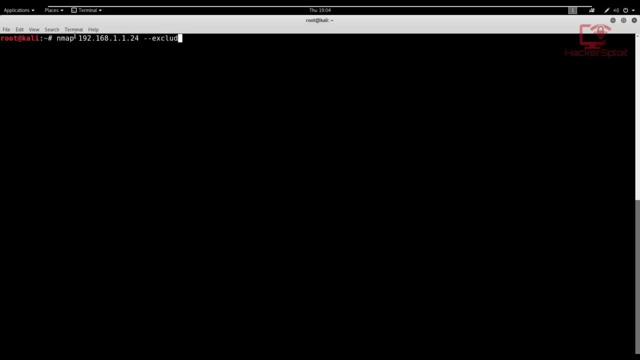 we've looked at the, we've looked at ranges, at IP ranges and how to incorporate them into your nmap scans. so let's say we wanted to exclude a range, let's say range of one or three to 104. so essentially we're getting rid. we're getting rid of the two windows workstations. 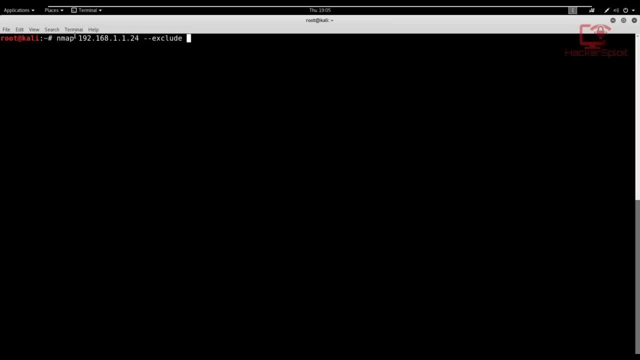 because I know that the IPs are 104 and 103 respectively. all right, so I'm going to exclude 192.168.1. all right, 0.100. so I'm going to say 103 to 104, right? so that's the range of IPs that I'm. 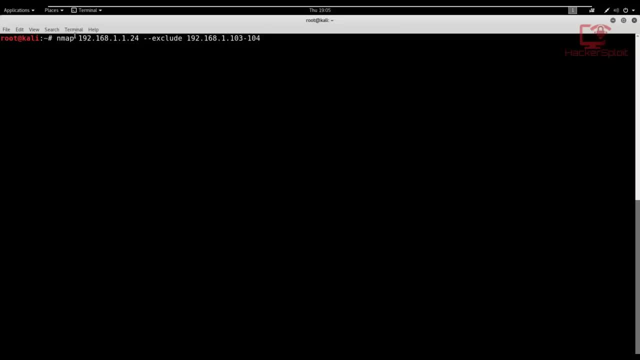 going to exclude from the scan on the entire subnet. so once I hit enter- whoops, my mistake. I actually forgot to use the correct syntax there, so I have to use a forward slash there and I'm going to hit enter and it's going to start the scan and the results will be a very, very obvious. 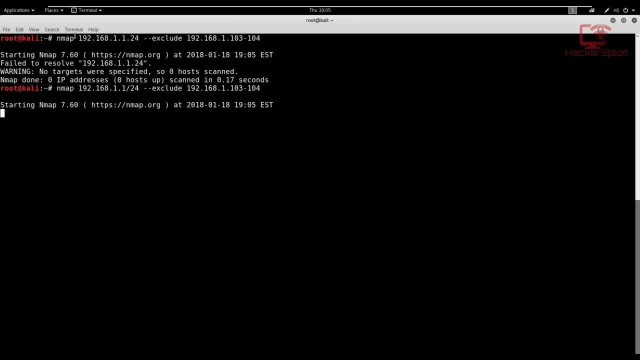 essentially what's going to happen is it's going to scan the entire subnet and but it's going to exclude the IP range of 103 to 104, which is essentially two IP addresses. but on my network the account for the computers, that are, the computers, the two windows computers that are 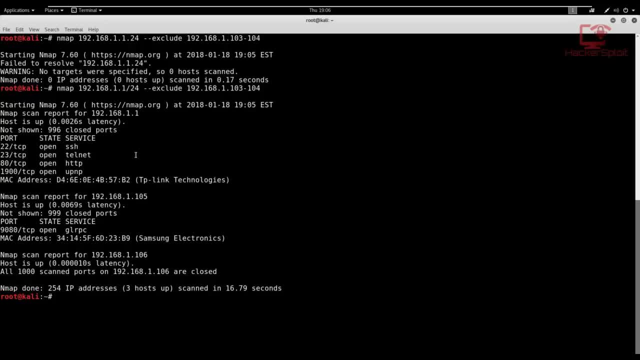 running on my network, all right. so, as you can see, it has returned my router and one of my mobile devices that is currently on my network right here. and, yeah, that's essentially how you how to exclude a certain range of IP addresses. so that's going to be, that's going to be it for this lecture and I'll 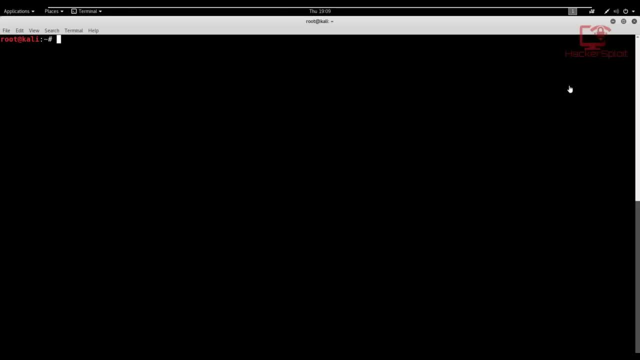 be seeing you in the next lecture. hello, Irvin, and welcome to this lecture. in this lecture, we're going to be looking at how to exclude targets using a list. now, we've actually looked at how to use a list to exclude targets using a list. now we've actually looked at how to use a list. 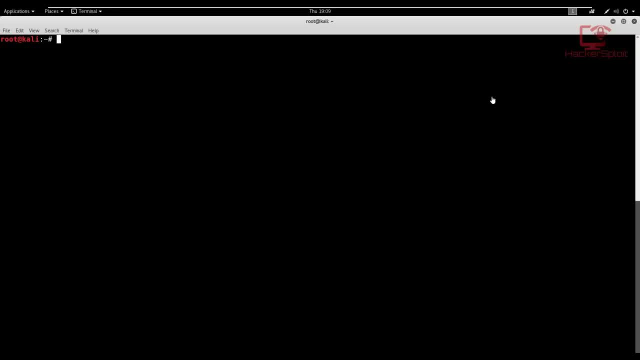 for certain, you know, for certain specifications using nmap. all right, so in this lecture we're going to be looking at how to use the exclude function, but in this case we're going to be using it, to you know, to exclude targets using a list that we've created. so the list will contain a. 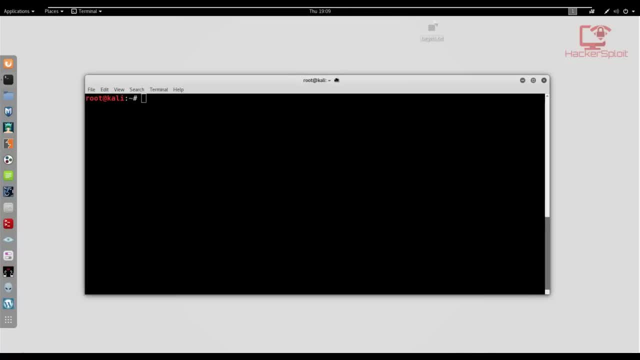 list of IP addresses that you want to exclude from a certain scan that you want to perform, all right. so I'm pretty sure you're familiar with what we're gonna do. we're gonna create a list that is going that we're not currently, that we do not want to scan, all right, so let's get started. so I'm just 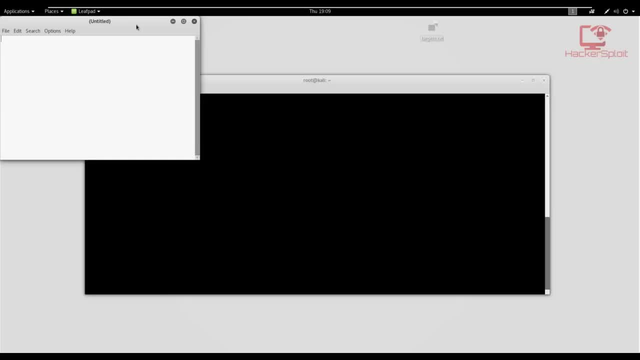 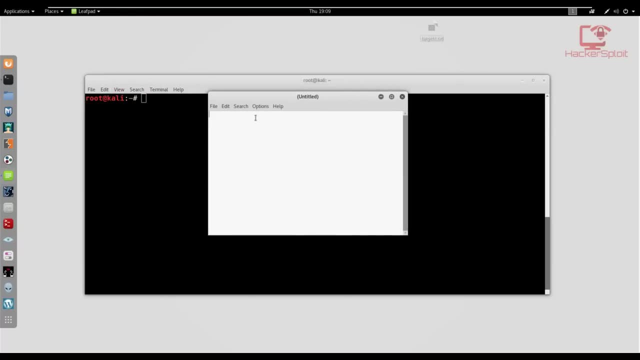 going to open up my text editor, so I'm just going to be using leafpad. you can open up whatever one you want, and I'm just going to give a list of the IP addresses that I want to exclude from the scan. all right, so I'm going to exclude the current host operating system, which is Windows or the current. 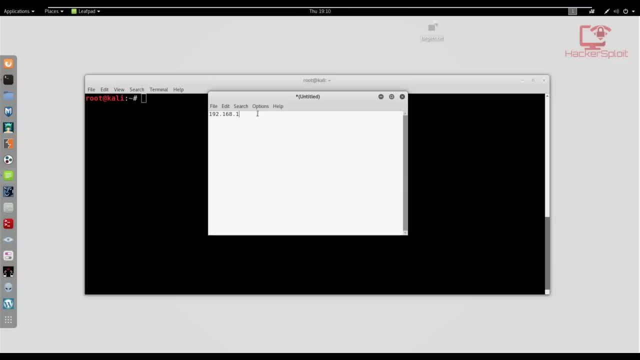 host computer which is Windows, which is running Windows, that is 1.104, and I'm going to also cut out my other Windows computer, which is 1.103, similar to the previous one, and we can also get rid of. you know that that's pretty much it. we can also get rid of the router, right? so 192 point, 168 point. 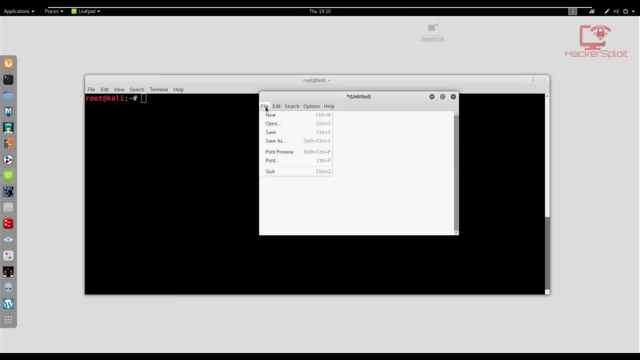 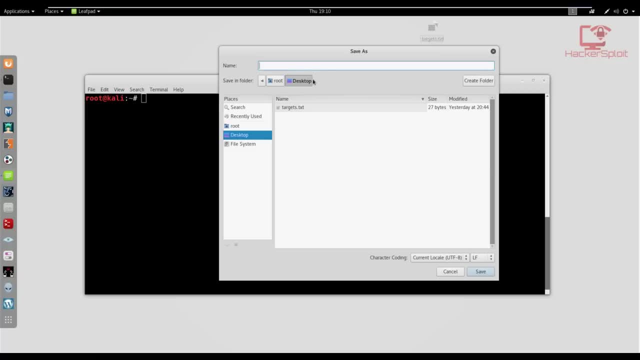 one point one, all right, so I'm gonna save this. I'm gonna save it on my desktop or in my working directory, so I'll have to actually switch, so I'm just gonna call it. I'm just gonna call it exclude and dot TX T. alright, that extension is very, very important and I'm gonna hit save. all right, fantastic now. 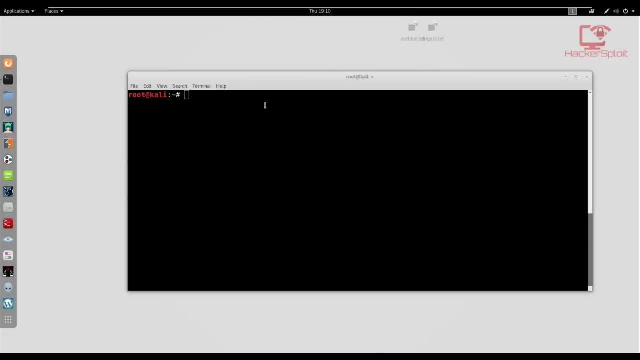 let me just close that up and, as you can see, the TXT file exists here and what I'm gonna do is I'm going to change my directory to desktop. awesome, all, right, now we can get started. so, essentially, if I just display the contents here- so exclude whoops, exclude dot TXT- you can see that it indeed 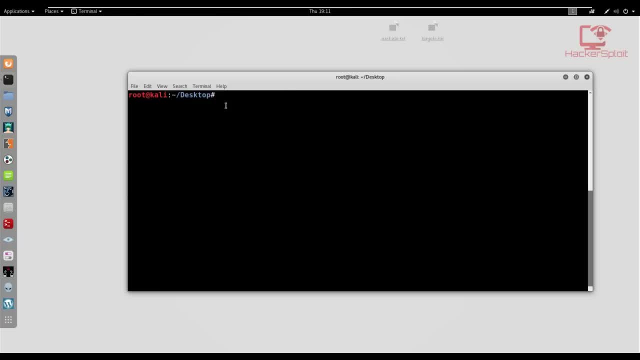 it does display the IP addresses that we have set to exclude. now, looking at the syntax that we're going to be using, we're going to be using the nmap, obviously followed by the targets, and then the exclude file parameter, followed by the name of the file and the 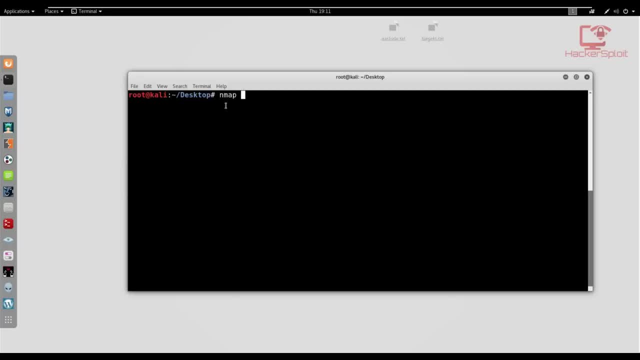 extension. all right, so let's get started. so I'm going to be scanning my assume I'm going to be scanning my subnet. so 192 nmap, 192 point 168, point one, point one, and the in the subnet of 24, which is obviously, we know is a. 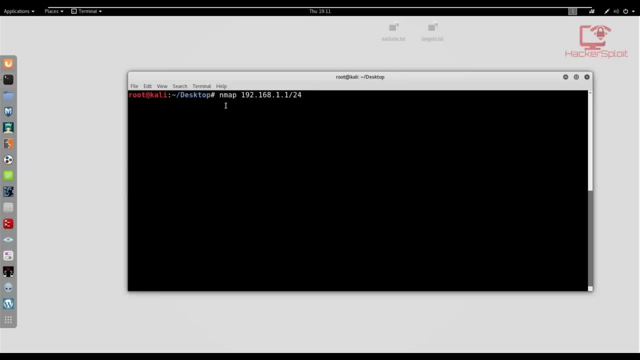 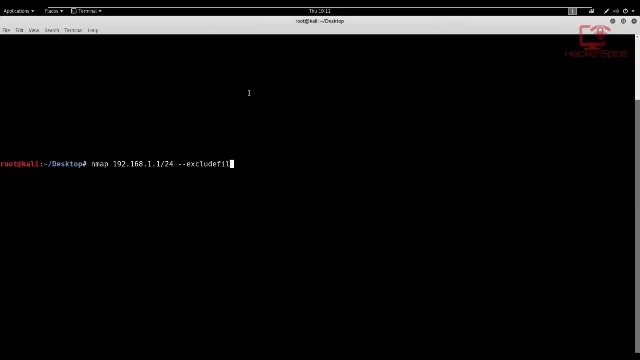 is in a version. all right, so we're then going to use the exclude file. so instead of exclude, we're going to be using the exclude file parameter. so that is the exclude file. all right, let me just enlarge, let me just maximize this window. whoops, let's do that again. let me just clear it out. so 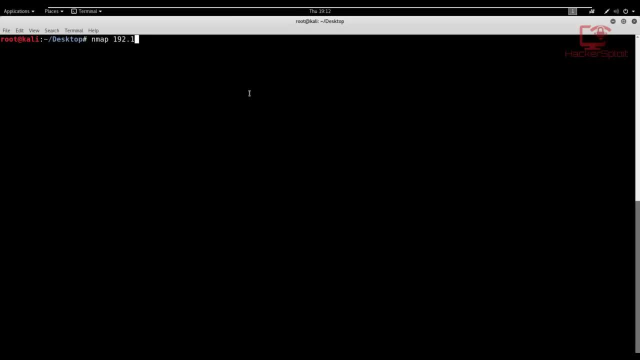 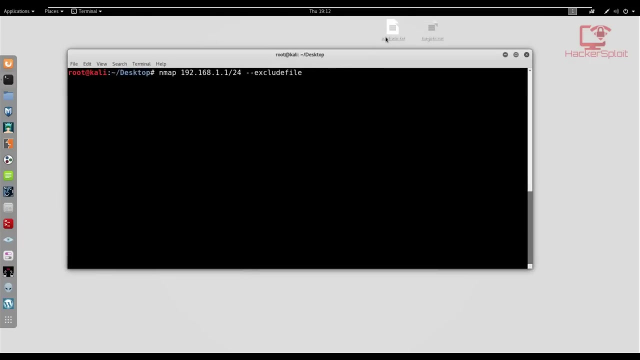 nmap and we're scanning uh, the subnet, so 182.168.1, uh, point one twenty four, and followed by the parameter exclude file. so exclude file, all right, and then that is followed by the, uh, the list uh, of, or the name of the of the of the document in which you have stored the list of IP addresses. 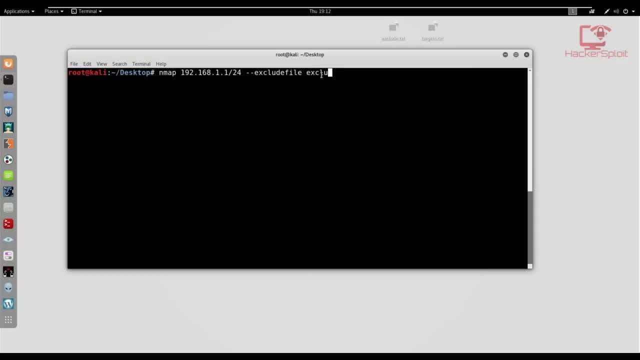 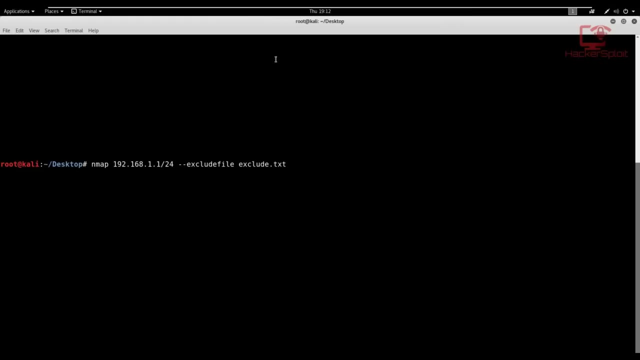 that you want to exclude, in this case the, the exclude dot txt. whoops, there we are: exclude dot txt, which is on the desktop. all right, so fantastic. now we can actually just hit enter and this should essentially scan, uh the entire subnet, uh, and exclude the IP addresses that we. 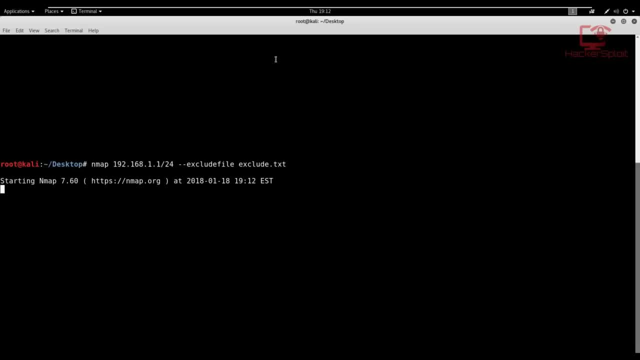 have provided in the excludetxt file. so I'm going to hit enter and it's going to start the scan, all right, and obviously it's going to take a few seconds, and this time because it's going through the entire subnet and, uh, it's excluded, probably. I have two Windows uh computers on my network and I 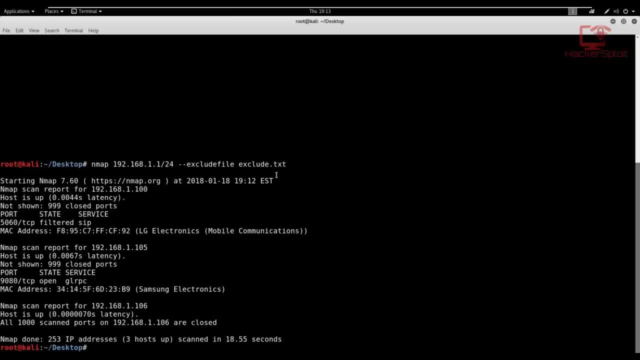 have two Linux computers so, uh, probably one of them is up. and no, actually it's only my Samsung device and my Nexus 5X that is currently online, as you can see. so, indeed, it did exclude the router IP address. so we actually- you know, this is fantastic- we're getting to learn how we can, you know, specialize our, our scans and to you, 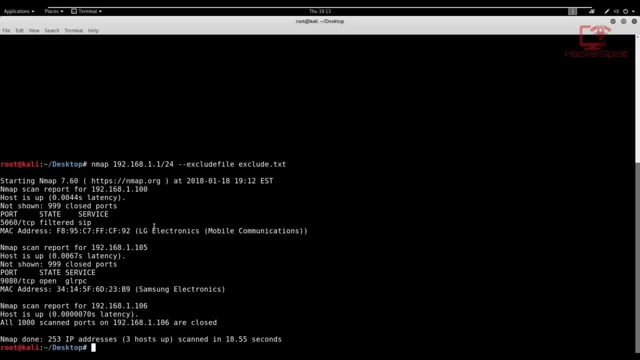 know, just scan what we want to scan, all right, so, as you can see, it's uh discovered my Nexus 5X device and one of my Samsung mobile devices, and there you are fantastic. so that is simply how to exclude targets or IP addresses from a scan using a list. all right, so. 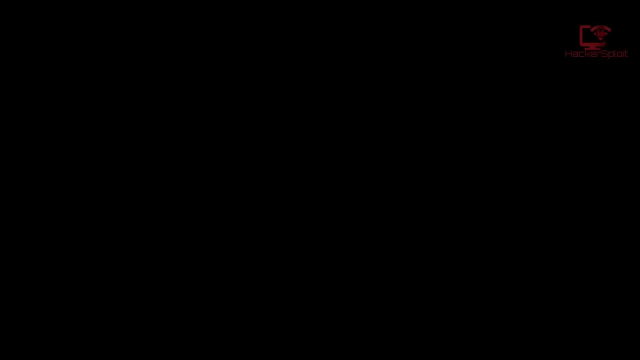 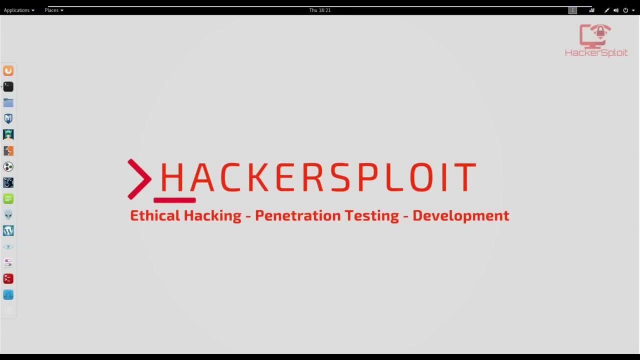 yeah, thank you so much for watching this lecture and I'll be seeing you in the next lecture. hello everyone, welcome to this video. in this video, we're going to be looking at how to perform an advanced scan on our target. more specifically, our target is going to be the Metasploitable 2 virtual. 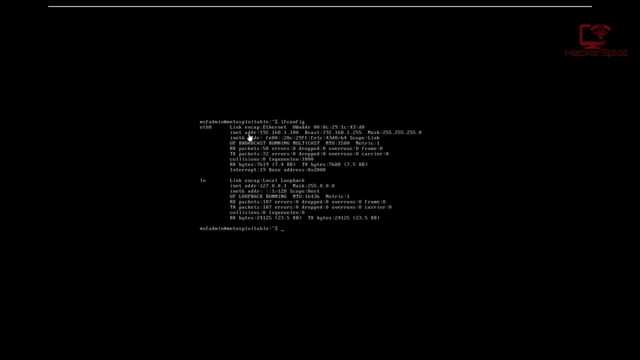 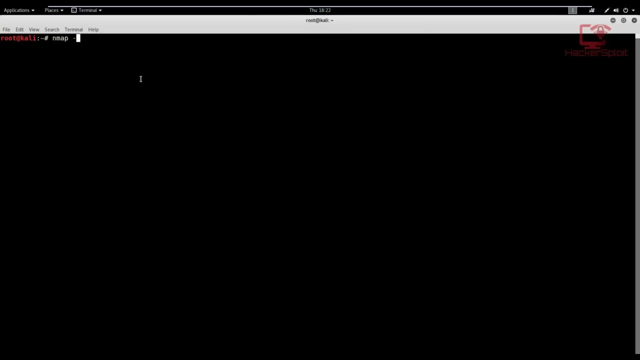 machine. so again, make sure you have that up and running and you know the local IP address after the connection. in my case the local IP address is 192.168.1.100. all right, so let us just open up our terminal and we can just open up the nmap help command. all right, so the nmap help command as. 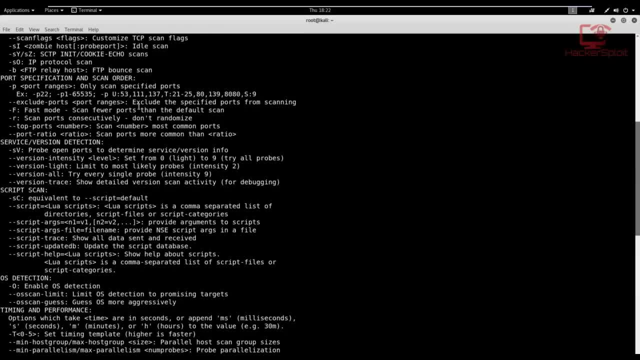 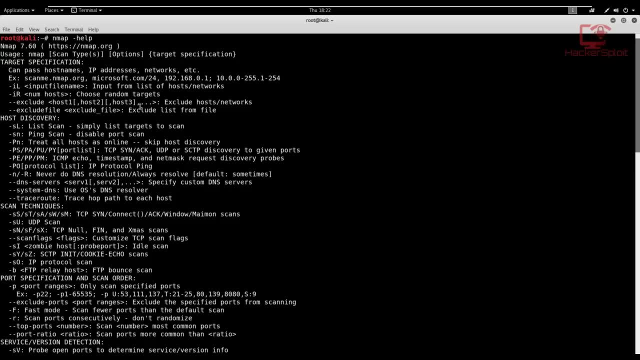 simple as that and just give it a few seconds. there we are all right, fantastic. so, as I said, in this video, we're going to be looking at how to perform an advanced scan, or an aggressive scan, for that matter, or matter all right. so in order to perform an aggressive scan, we're going to be using 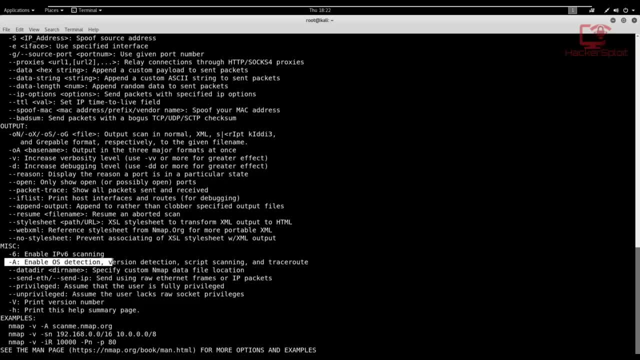 the command or the a parameter. all right. so, as you can see, the a parameter here, which is again for aggressive scanning, has several options that it gives you or results that it will scan, for it enables OS detection, so it will detect the operating system that is running on our target. 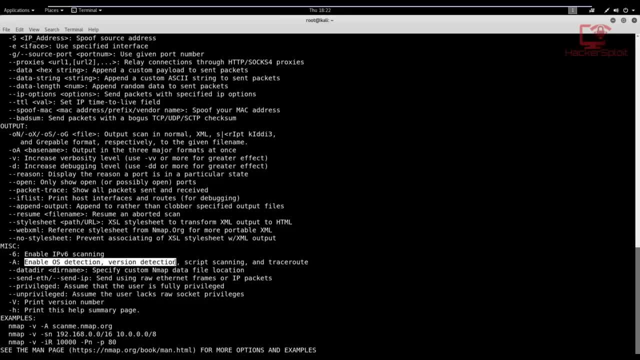 that we are scanning the version of the software that is running. so again, if your, if your target has an FTP port that's open, it's going to detect what version of the software or the service that is running on the FTP port. it'll scan for scripts, perform a trace route and, more specifically, some of the 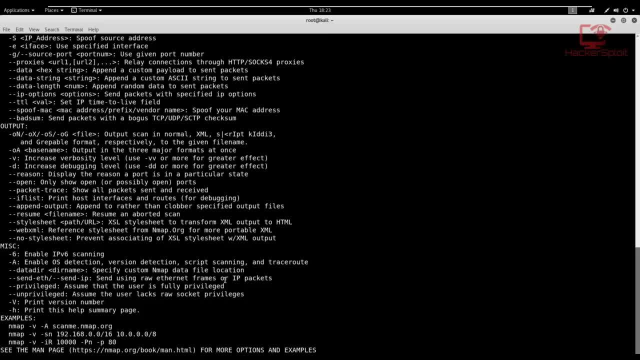 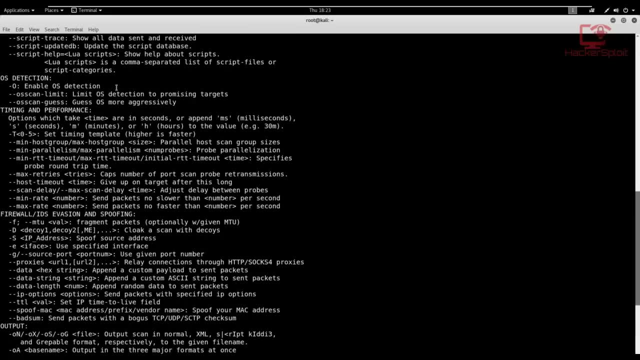 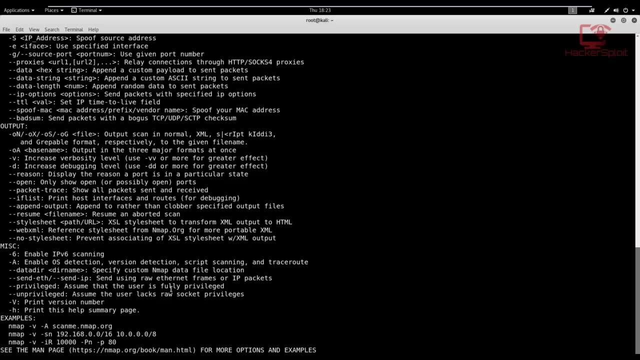 other uh, fantastic uh, options that it does give you is the ability to use the O command. so it actually includes the O command right here. so, if I can just find the O parameter again, it enables OS detection. so it it is a combination of a multiple, uh, multiple types of commands, so in 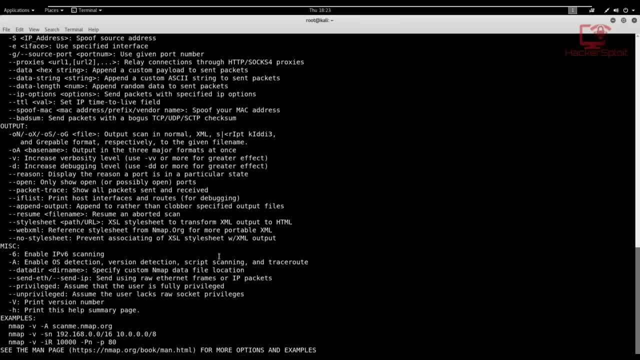 this case it's a combination of the O command, it is a combination of the trace route command, et cetera, et cetera. all right, so in order to use it, it is really very simple. all we have to do is we just- firstly- let me just clear that up- we just start off with the nmap command and we use our 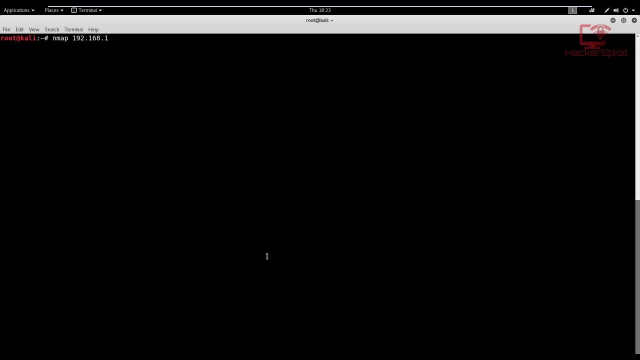 target IP address. now, your target IP address could be local or it could be a public IP address if you're targeting- uh, if you're trying to target a computer that is outside of your network. so in my case, the IP address for the meta exploitable 2 virtual machine is 192.168.1.100. 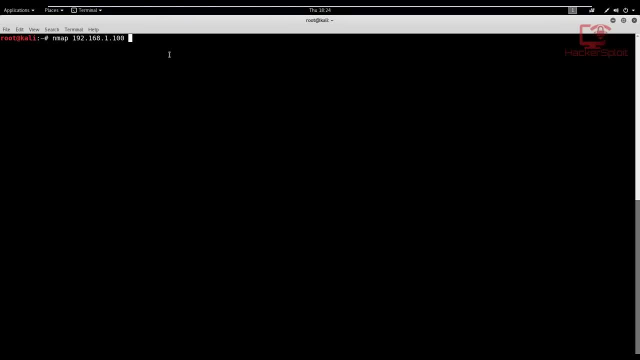 fantastic. so we're going to enter that in. uh, really, simply like so. and now you might be asking: well, what's happening here? well, I aren't we supposed to specify the parameter? well, yes, we specify the parameter before the target. so the parameter is the a command, as you can see. and 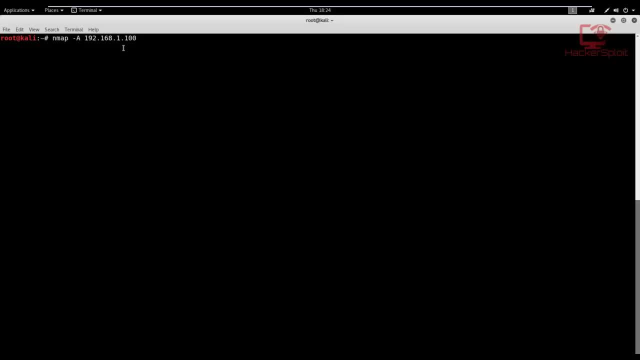 there you are. so it's nmap a 192.168.1.100, and you just hit enter. now, by default, you can also run this on a network range or a subnet if you. if you feel that you need to scan it on a network again, you can choose an IP range if you feel, uh, the need to as well. so let us just hit. 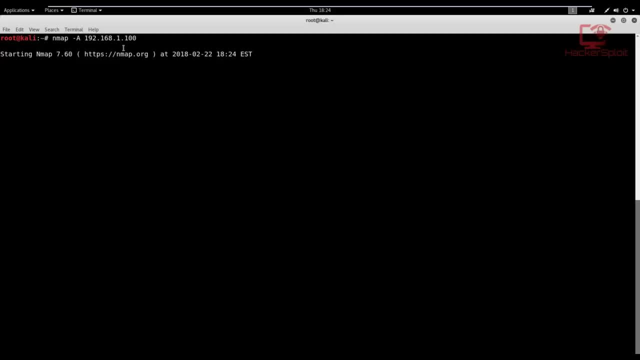 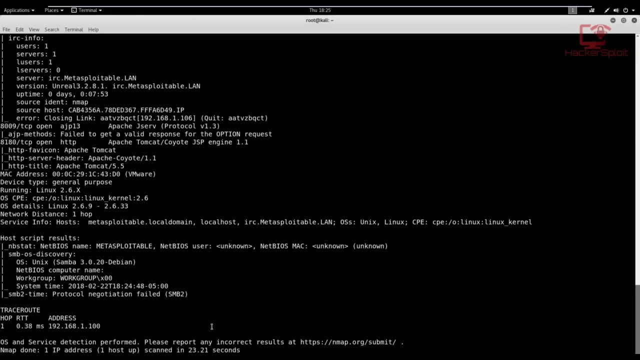 enter and let's see, uh, what results we get. all right, so I've started the scan, as you can see, and then we're just going to give it a few seconds and I'll get back to you once the scan is complete. all right, so the scan is complete and here we have the results. so what I'm going to do is I'm 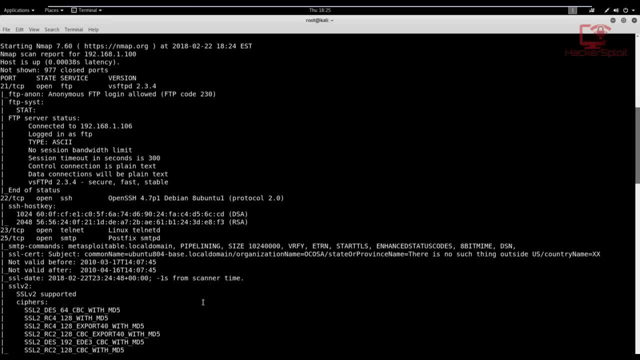 just going to go all the way to the top here and we're just going to analyze the results that we got all right. so, as for the timestamp, we can see that it gives us a nice timestamp there and it obviously tells us that the host is up and it goes through the the ports that it's supposed to scan through, and 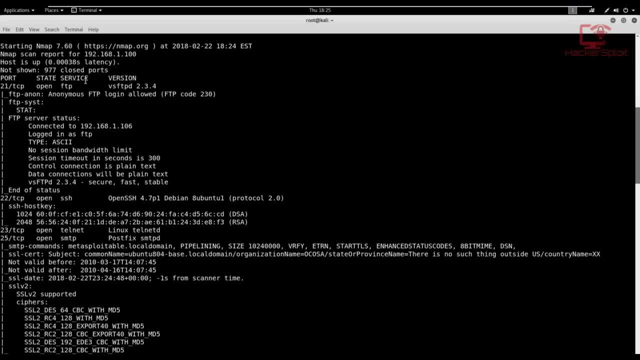 as you can see, 977 ports were closed. as for the other ports that were open, you can see it is sorted in terms of the port, the state, the service and the version. again, very, very important that we can see the version that is allowed or that is currently installed. so in this case, where the vsftpd 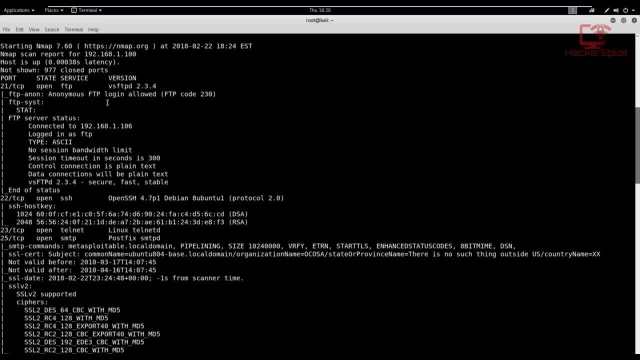 2.3.4, which is vulnerable by default on uh, on the virtual, on the metasploitable to virtual machine. so, as you can see, you now have versions of the softwares that are currently running, all the services that are running on the ports. so, by default, you can see that we get some uh, some. 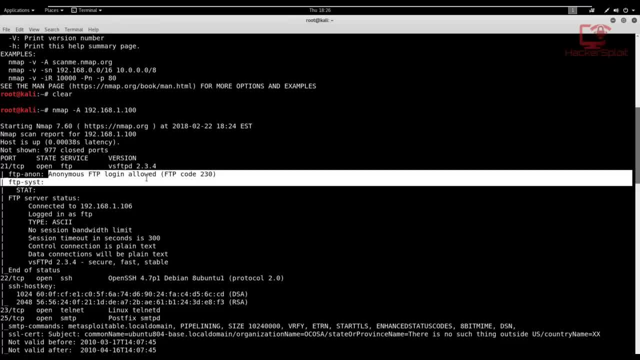 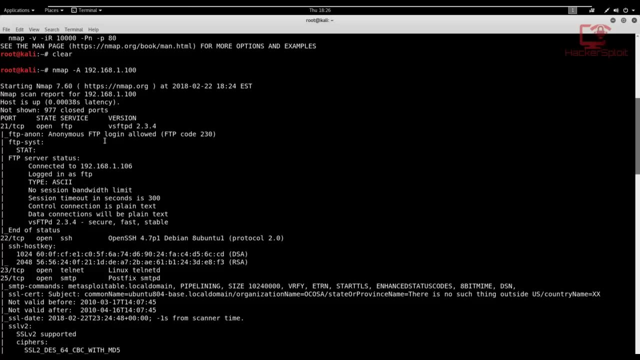 more information about the ftp port. so it's going to tell you that the, the anonymous ftp login, is allowed. now that is, again, that is a huge security flaw that, uh, by default, should be disabled and anonymous ftp logins should not be allowed anyway. so, again, this is a fantastic way of finding what services are currently running and any 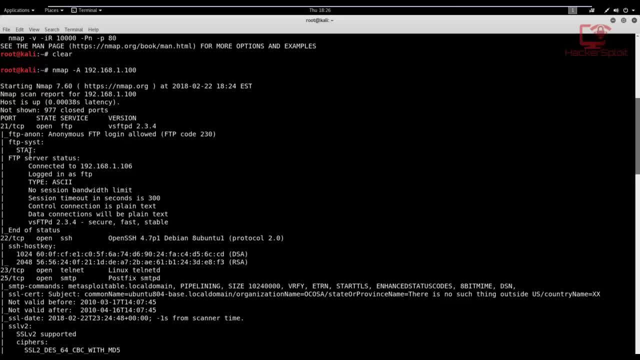 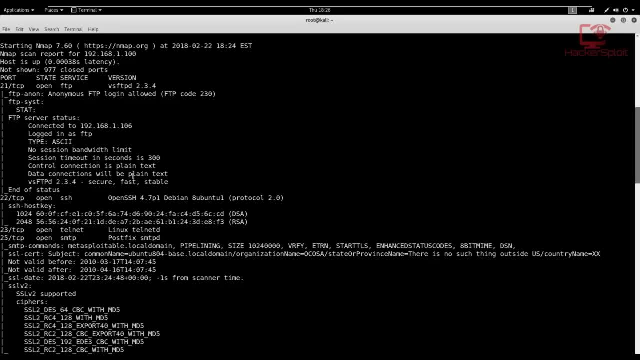 vulnerabilities that could be, um, that could be existing. all right. so as for the ftp service date, as you can see, it gives you information about the ftp software, the version and, uh, again, any information regarding whether or not anonymous ftp logins are allowed. all right, as for the other ports. 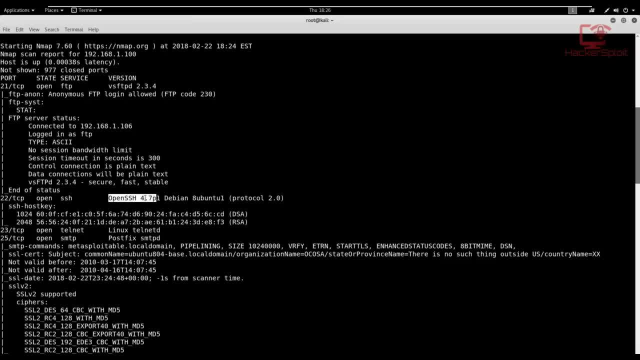 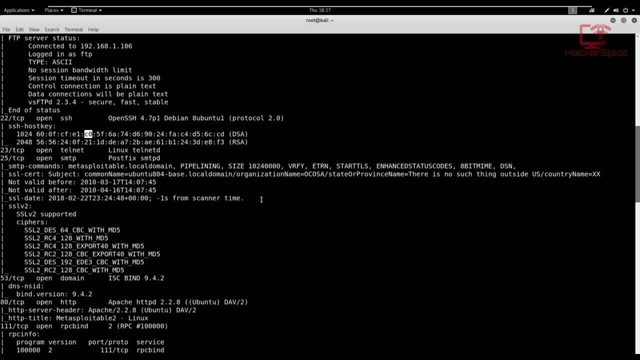 you can see, for example, the ssh- uh, the ssh port. you have your open ssh that is running on the m2 uh, and something really, really interesting is it was able to get the ssh host keys, which are right here. fantastic as well, information that was leaked there. you have your telnet- uh, yes, mtp port. 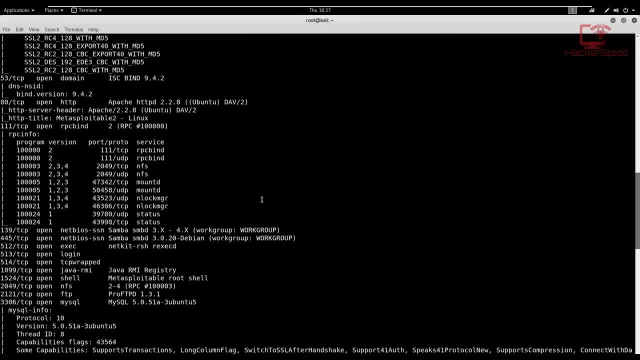 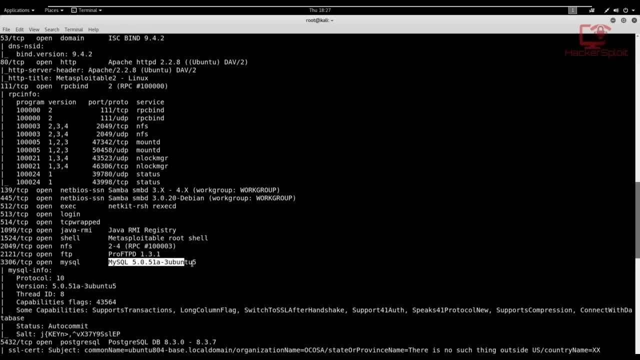 that is currently open, and if we just scroll all the way to the bottom here, we can see we have the, the tcp port, which is by default always there. you have your mysql, so again it tells you what version of mysql is currently running, which, again by default. if you do your research and vulnerability, 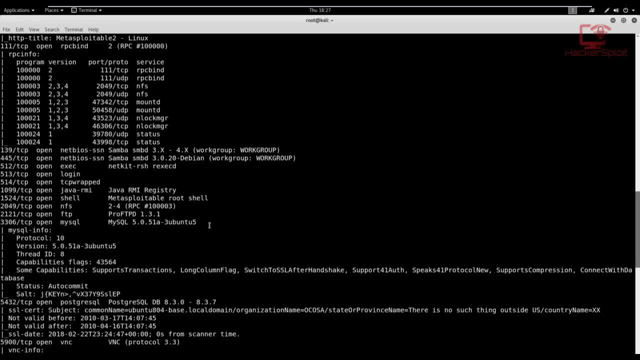 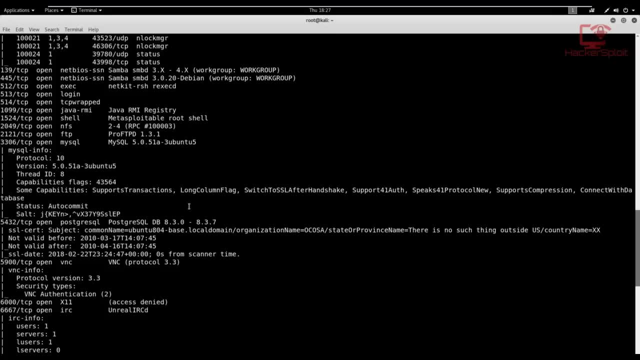 you'll find that this is also vulnerable to an sql brute force login. so it's always always interesting to run the aggressive or the advanced scan on your target to get information, to get more information about your target regarding the the versions of the software that is running all right. 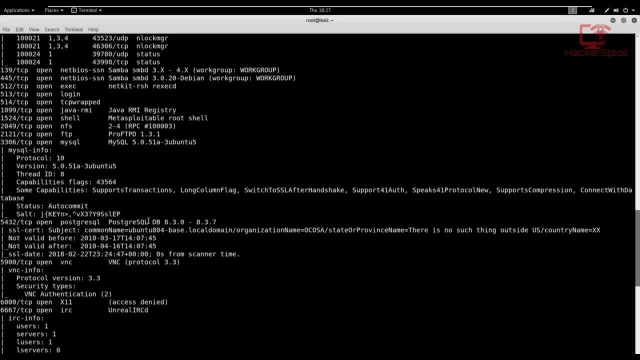 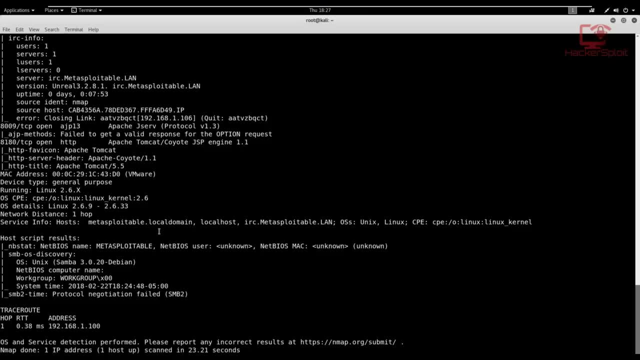 really, really important. okay, as for your postgresql database, you can also see that the port is open, um, and if we just scroll all the way to the bottom here, looking at the other results that we were able to gather, you can see that we were able to get the the net bios name, which is metasploitable. 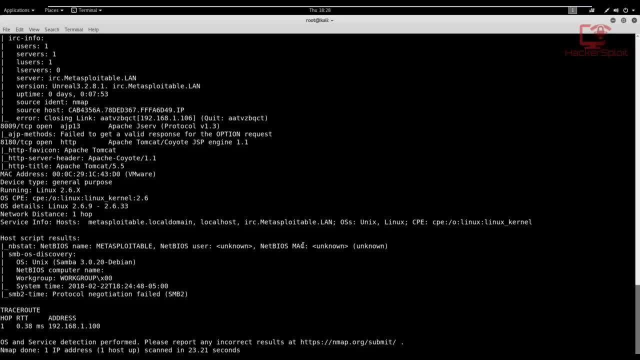 really, really important information you can gather here. you can gather the username, the Mac address, and as for the operating system, it was able to detect it as unix, which is running samba, the samba server, and it gives you the work group information. so this is regarding the web, uh, the 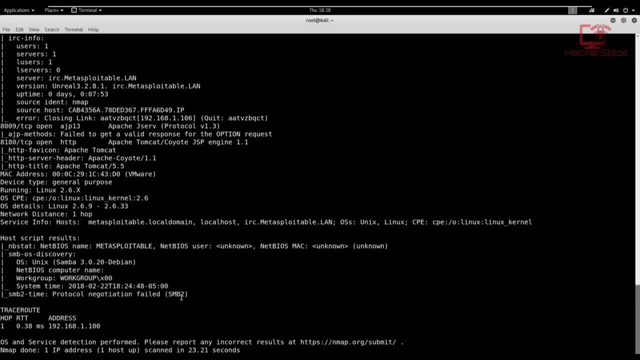 the file, the local server that is running on the uh, on the virtual machine, all right. so, as you can see, then also, we performed a trace route here with information regarding the trace route, which you can also analyze for yourself. again, depending on what Target you're scanning, the results will vary. 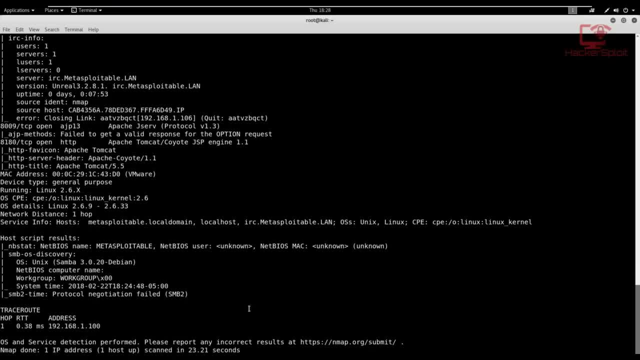 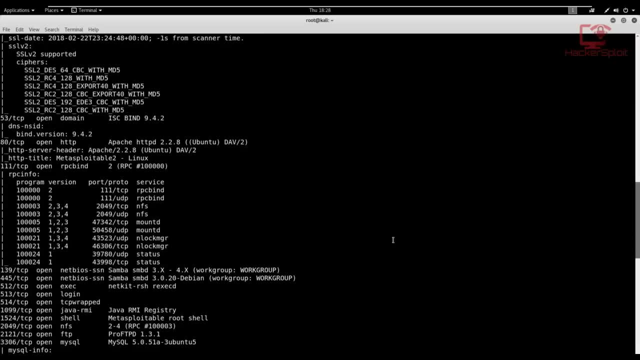 all right, so that was how to perform the aggressive scan on a target, and, uh, that's going to be it for this video. in the next video, we'll be looking at some output options and how to output your results to files. all right, so I'll be seeing you in the next video. 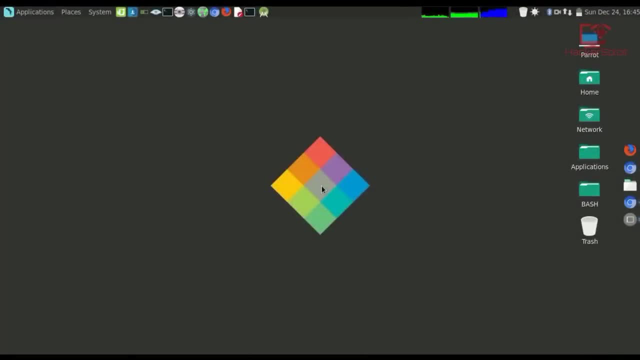 foreign to be looking at metasploit all right now. this is going to be the complete metasploit course and this is going to take you from guys an advanced user of the metasploit framework all right now. as I said, this is going to be an advanced course and it's going to take you beginner to Advanced. 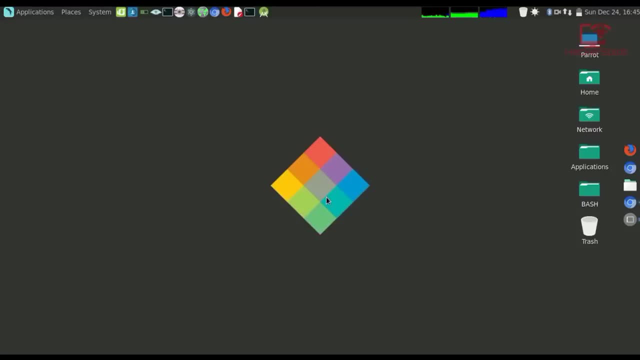 so that is the goal of the course and I'm going to try and cover it within one week. so I'm gonna, you know, make the videos and I'm going to upload them, and hopefully you guys like the format in which I'll be uploading them, So I'm not going to waste time. 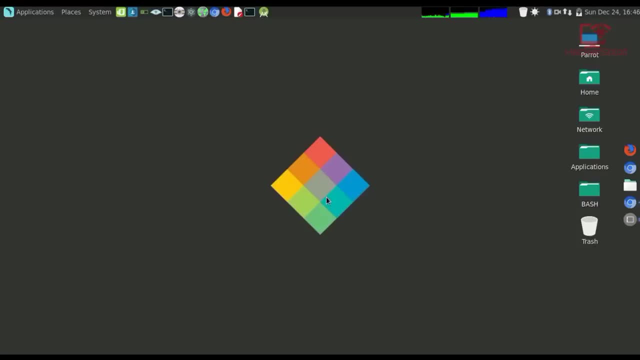 on one series. I'm going to complete it and then we'll move on to the next one, Right? So I've made a lot of videos about Metasploit, but I realized that I really didn't cover the basics and how to navigate around this. And you know, for most of the beginners, you really don't understand. 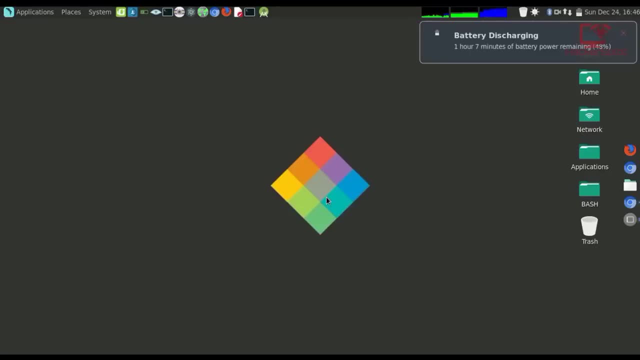 Some of you guys did not understand the format and the way Metasploit works. All right, So let's get started. So this is going to be part one and we're going to be looking at all the basics to get started with Right. OK. So for those of you already asking what operating system I'm using, 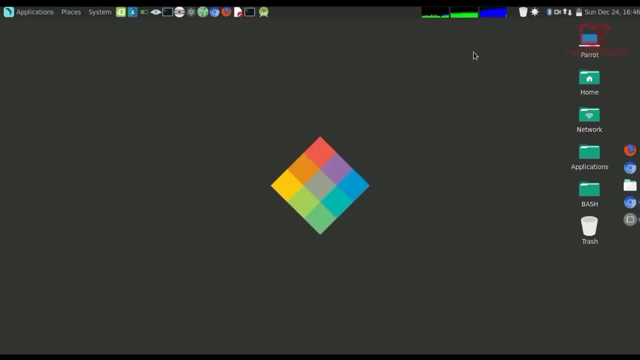 I'm using ParatOS for this demonstration. I just seem to really, really enjoy the latest update, and I've been using it as my daily driver on my laptop. As you can see, I'm recording this on my laptop. So yeah, let's get started. So what is Metasploit? All right, So Metasploit. 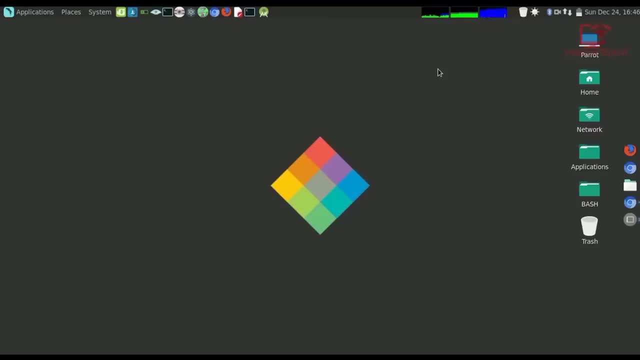 essentially is the. you know it's the leading exploitation framework. All right, So it is used by nearly every penetration tester or ethical hacker- or hacker for that matter- And it is really really important that you master it, for you to, you know, to to enter this field Right. 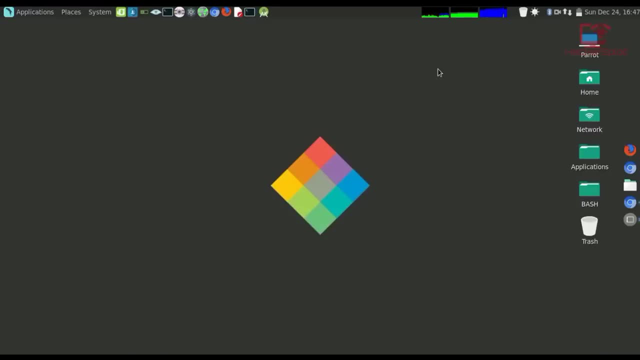 Or, to you know, to prosper in this field. Now it was developed by Rapid7.. All right, So Rapid7 is a company that owns the different. it owns these different vulnerability scanners like Nexpose, And it again, as I've said, it owns Metasploit. All right, Now looking at the 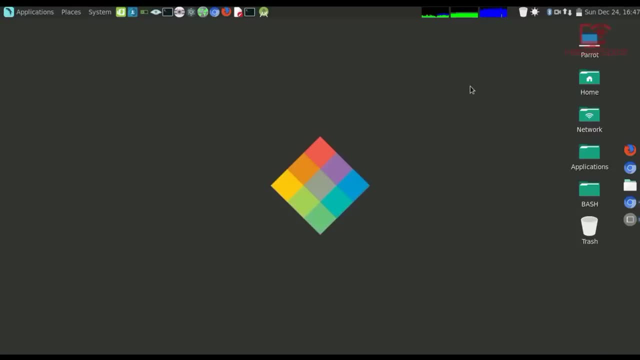 Metasploit interfaces. we have already looked at some throughout. you know the channel, And one of them is the MSF console. All right, So these are the multiple Metasploit interfaces. So we have MSF console. We have Armitage. All right, So Armitage is. 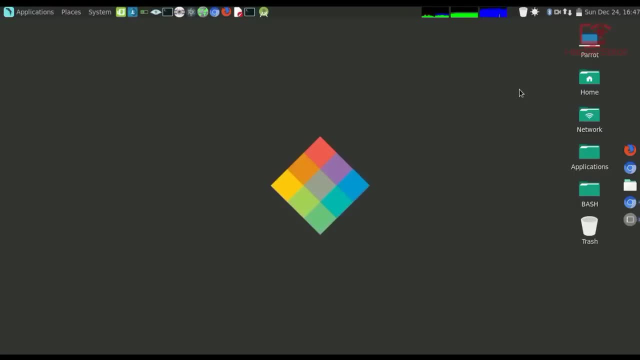 is simply put, a GUI framework that allows you to to use the Metasploit framework, The MSF console is. it gives you an interactive command line like interface that allows you to also use the the framework, which is what we're going to be looking at, because it's the most, it's the easiest to set. 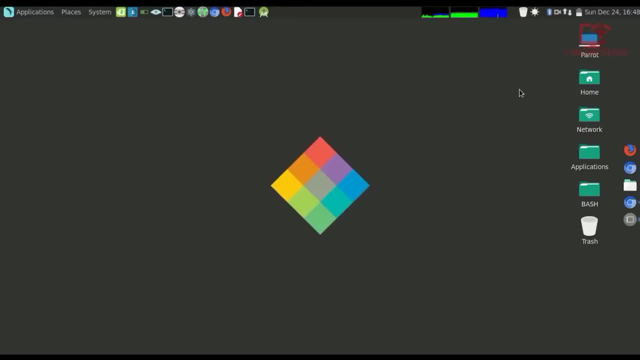 up. You then have the MSF CLI, which is which is going to be a very literal, literal Linux command that also allows you to use, or the Metasploit framework. you then have, finally, the MSF web, which is the browser based interface, which is what we looked at, where we set up the community. 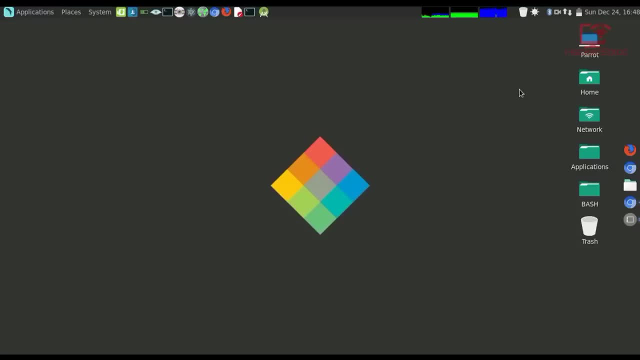 version and we were able to scan for our targets and find the vulnerabilities right. So, as I said, we're going to be focusing on MSF console Now you know. the first thing to understand is that Metasploit, as we have looked at pre in previous videos, I really didn't show you how to set it up. 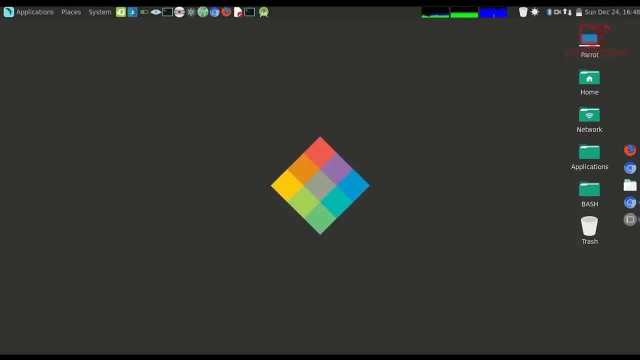 correctly and how to make it faster, because most of you realized it And a lot of you guys raised that question: do I need to start any services? Yes, you do need to start the services, All right now. you need to start the PostgreSQL database service, which does come with the major penetration. 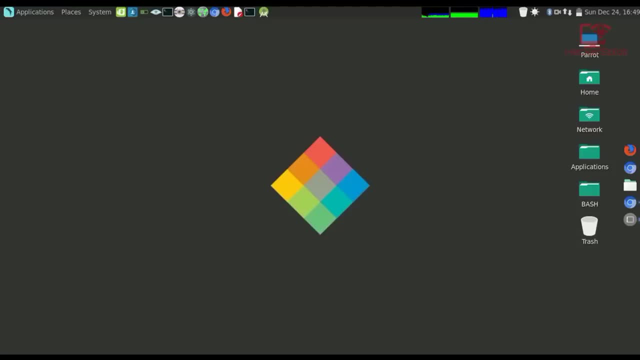 testing distributions. So if you, if you're running this on a normal Linux distribution, you know, I recommend that you switch to a penetration testing distribution because these tools will be already pre installed Right, So you don't need to run this on your main computer, like I am, you can. 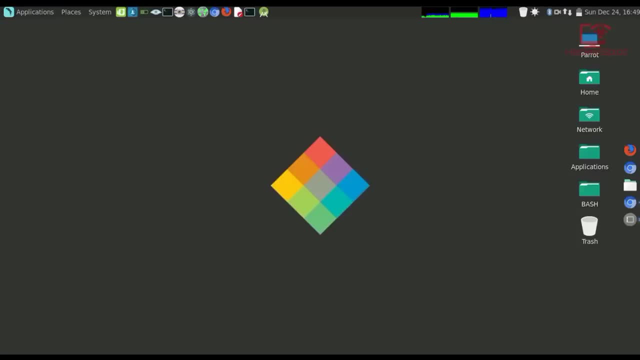 also run it in a virtualized environment moving along. So we have to start the PostgreSQL database, Alright. so what this will do is it will allow Metasploit to run faster searches And that will allow Metasploit to store the information while you are performing the scanning and or exploitation. 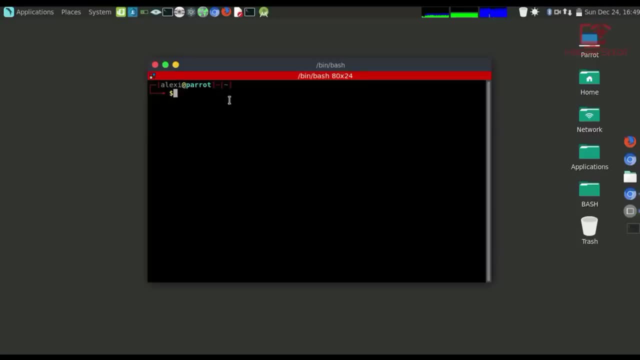 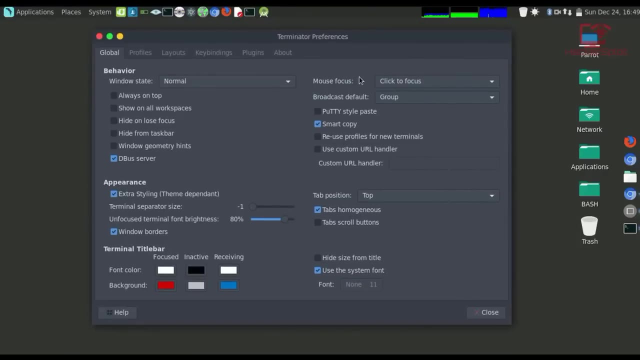 Alright, so I'm going to open up my terminal here And what I'm going to do is let me just try and zoom this in. So I should have done that before I started the video. But you know what? I'm just going to run this through the para terminal because I don't want to confuse you. 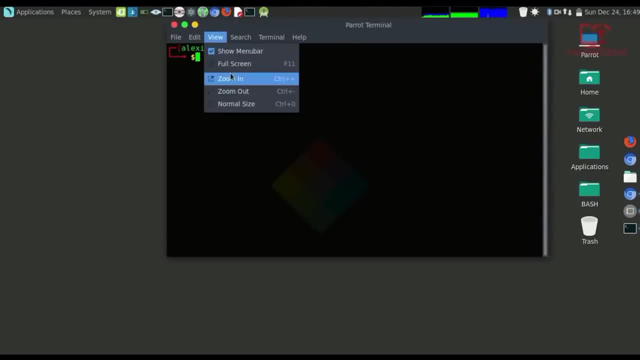 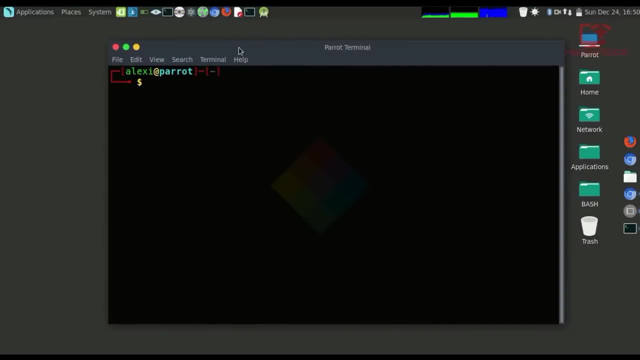 guys, Right. So let me just zoom that in So we can have a good view of what's going on. Alright, so it's very, very simple to start your PostgreSQL service, as you know, with Linux, So it's service post, very, very simple post. 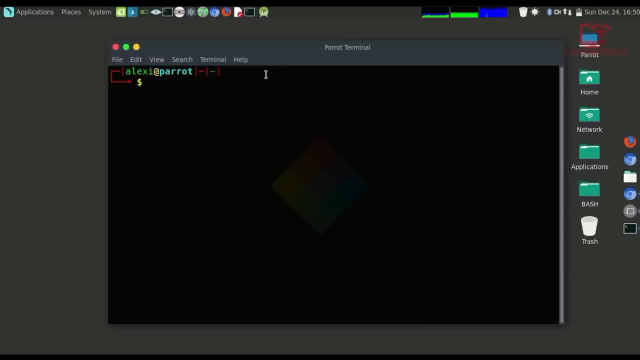 Gress. whoops, my bad, Sorry about that. Oops, there we are Alright. so service Boost: Please forgive my typing. I'm on a laptop right now. Boost rescue: Alright, and we can start. Whoops, my bad again. 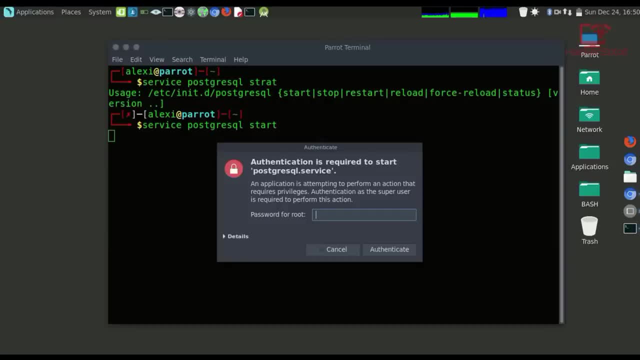 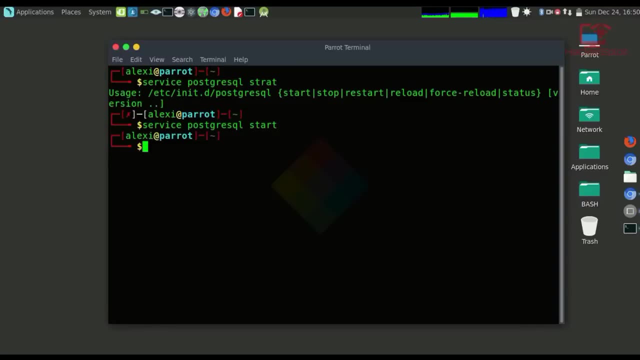 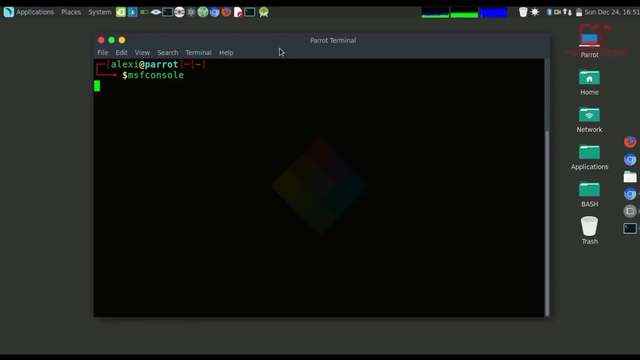 Alright, and you want to start the service now, And it's going to ask you for your root password, So make sure you enter that. And once the service is started, we can then move on to use the service. So, for the first time, I'm going to go to the MSF console, Alright, which is the command line interface. So, again, start it up, So, MSF console, and you'll see that it reloads much, much faster than when you, if you, didn't, start up the PostgreSQL database, Alright. so just give it, give the first run, a bit of time, because again, it's building the database and it should load up immediately, right? So, as you can see, it's starting the Metasploit framework console, And give that a few seconds, as always. Now I'm going to go back to my Mac to use the software and update my Proxmox. Now I'm going to go to my Mac to use my Proxmox And I'm going to go back to my Mac to use my Proxmox And I'm going to go back to my Mac to use my Proxmox And I'm going to go back to my Mac to use my Proxmox And I'm. 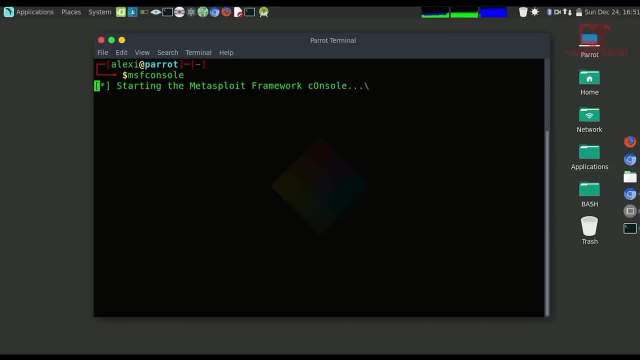 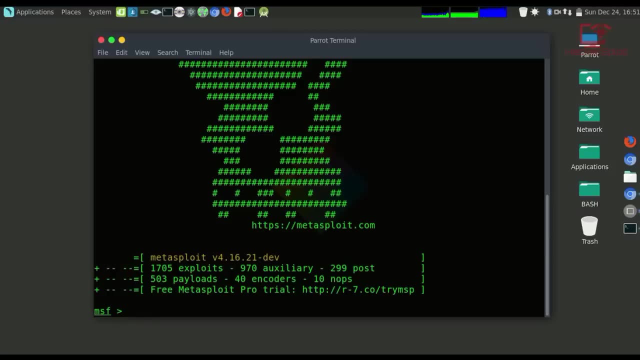 one thing i want to just tell you, and a lot of you guys have been asking me, is: what are the system requirements? you know, if, if you want to become a penetration tester, the truth is, uh, the thing that you'll need the most is going to be ram. now, the minimum i would recommend, 2gb works fine, but if 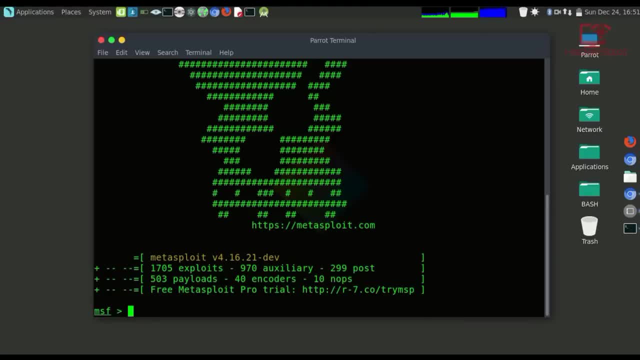 you're going to be running a lot of penetration tests. i would recommend that you get a minimum of four gigabytes of ram and then you can, uh, possibly upgrade to eight, and the ideal what would be eight to twelve, all right. so again, you also want to make sure that your processor 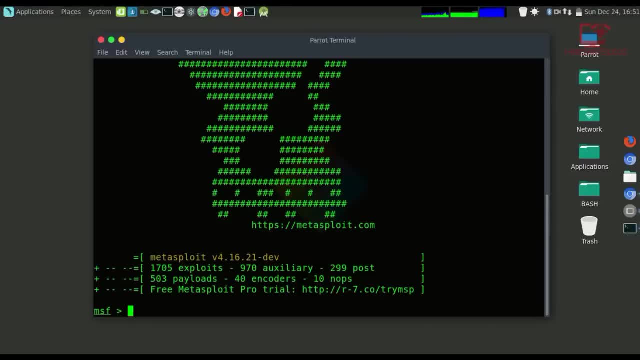 can match that. so i would recommend you know an i5 or an i3 processor, a good one, quadco hopefully. uh, depending on you know, on what you can afford, it really really doesn't matter. but if you want some great efficiency, i recommend you get a computer with, uh, some good ram, all right. so 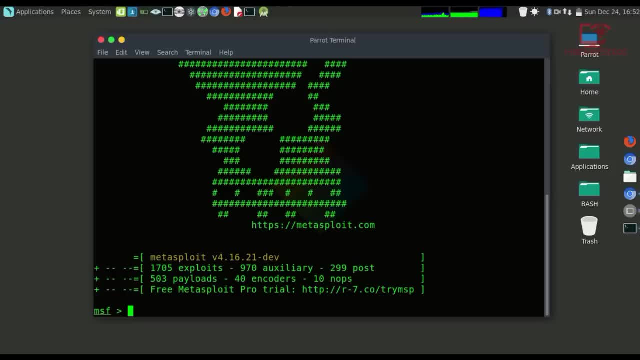 yeah, once it starts up, it's really really very simple, and i've gone through this before now. uh, you're wondering what are the other ways of launching it. what you can do is go to your uh. you know, in cali linux it's simply your, it's your menu. uh, in paratois, uh, it lies, they lie in the. 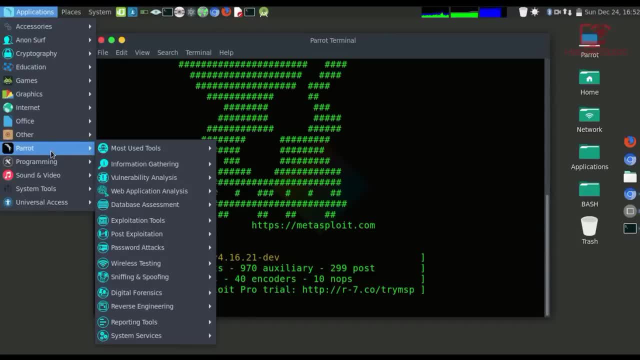 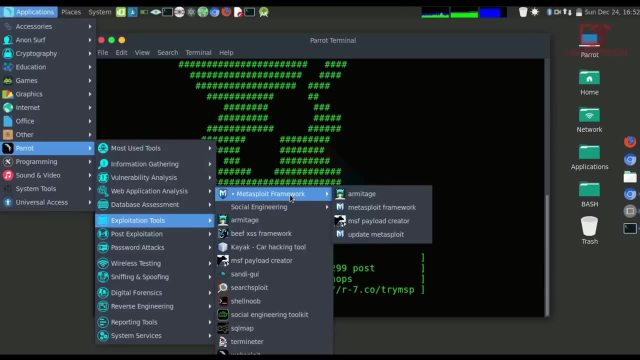 same um, in the same category. they lie in exploitation tools. all right, so when, once you open exploitation tools, you can see that the metasploit framework exists and it gives you the various options that you can use, you have armitage, uh, the metasploit framework, and you 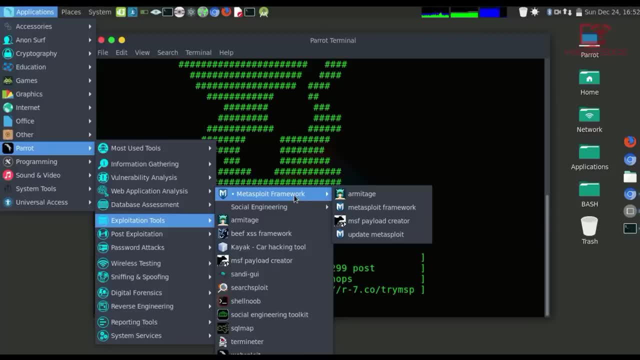 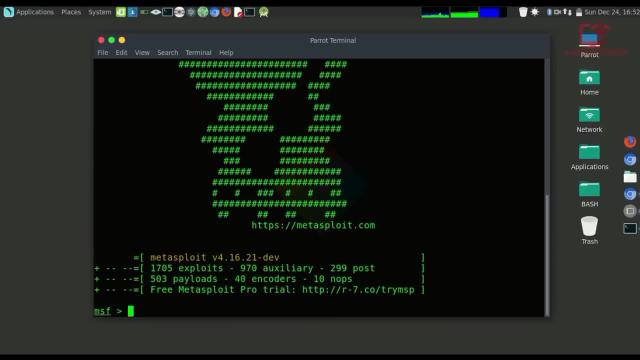 can update it, and this is a another way of accessing it if you don't want to go through it through the terminal. all right, now let's look at the metasploit keywords that are very, very important. now, this is something that i did not fully cover, so i'm going to do it right now. 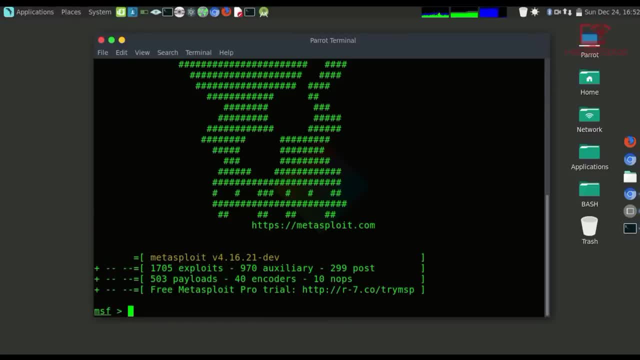 now, metasploit has six types of modules. we use mostly four of them, the most all right, but i'm going to explain them to you. so the first thing we have is exploits. all right, it has exploits, it has payloads, it has the auxiliary, it has knobs, it has post and it has encoders. all right, 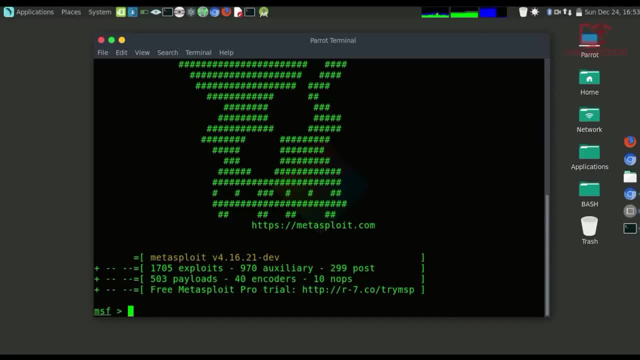 now let me explain what they are very, very simply and very quickly now. an exploit is a model, is a module that will take advantage of a system. all right, so it'll take advantage of our system's vulnerability. all right, so it's not gonna, you know, just take advantage of a system that is patched. 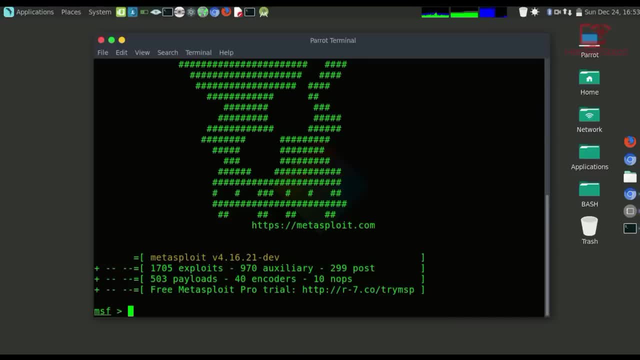 or does not have any vulnerability. it needs to have a vulnerability, all right, and then it will. it will install a payload on the system, all right. now. the payload can either be a reverse shell or a metapretor, all right, so it'll give you access to that computer in form of the payload now. 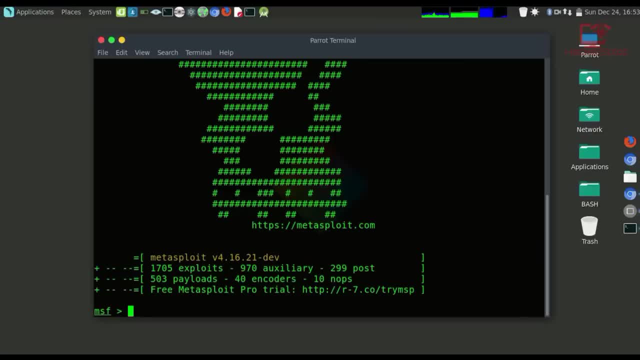 you know, usually with other systems or in other environments, you would usually call these payloads things like rootkits and stuff like that. but for now just understand that the payload is what the exploit will try and plant on the system. all right, so that will give you that access. 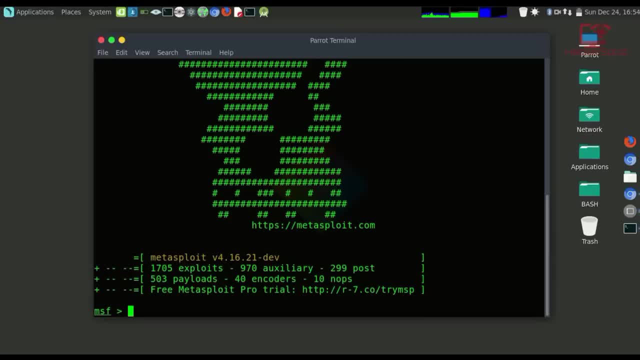 to that computer and then you can exploit, uh, uh through a vulnerability that is then exploited. all right. so that's simple. now. once i've explained that, now let's look at some of the basic commands. now, one of the best commands that you know you can use is the help command, and if i open up that, 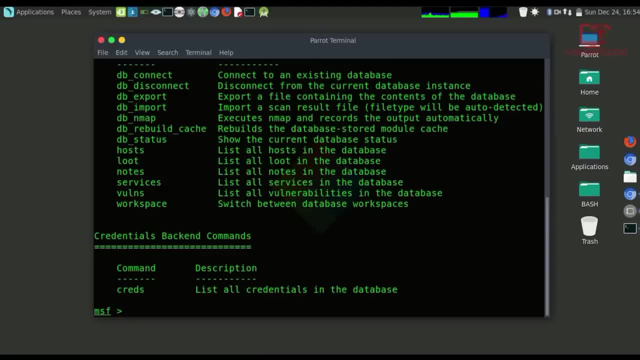 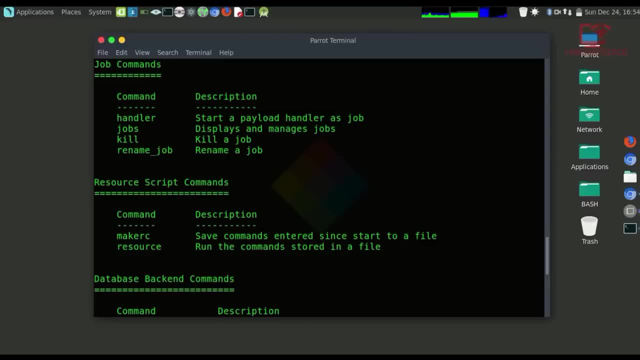 up right now. you can see that. um, all right, whoops, let me. there we are. if you open this up, it will give you all the help commands, all the commands that are very, very important for you, and, again, this is very, very useful. it will give you the ability to, at any time you know, refer to this documentation so if you're lost, 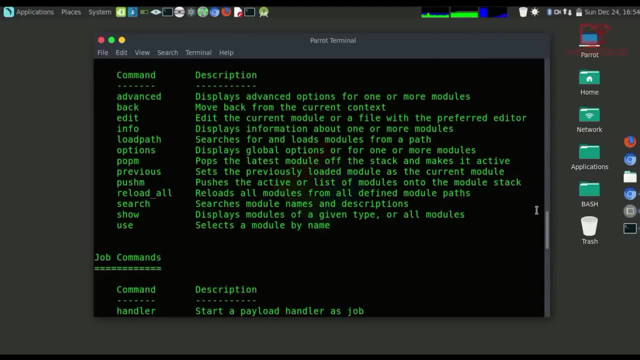 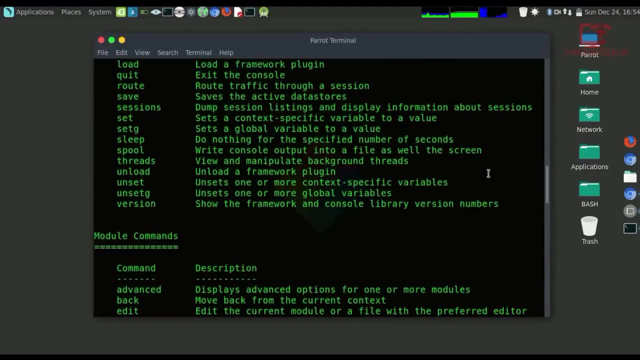 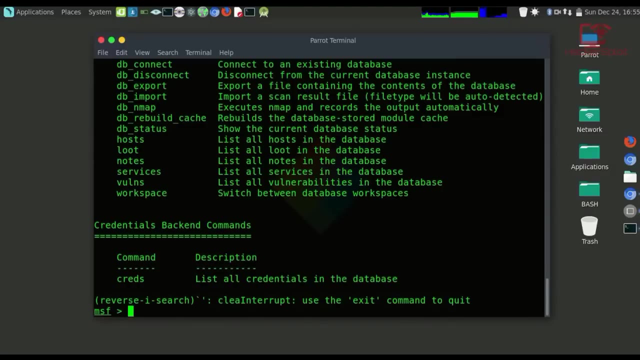 this can be a very, very good way of um, of using uh, or of getting guidance using this framework, so you can go through this if you're feeling a bit lost, all right. so that's the help command, very, very important, and you'll find yourself, uh, using this quite a lot, right? all right? 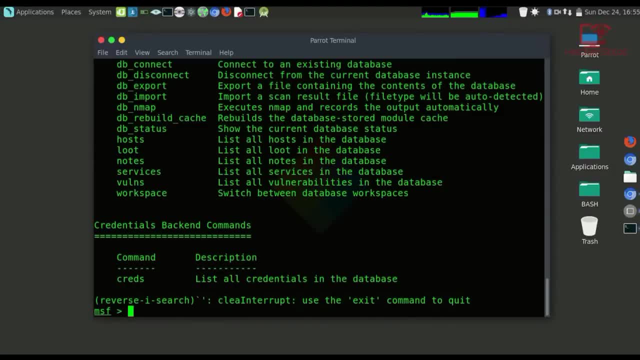 now let's look at the other commands. now, one of the most useful ones is the use command, because the use command will allow you to load a module, all right. so, for example, we can load many, many modules here and one of the most, you know, the most common ones that you can start. 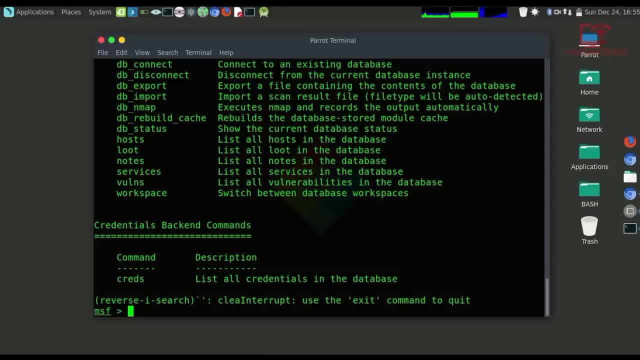 to load is the um. let's see one that comes straight off my head, uh, of the back of my head. it is the x. yeah, i think i remember this one. this was quite an old uh exploit and allows us to exploit the um, the adobe flash. uh, i think it's the plugin. 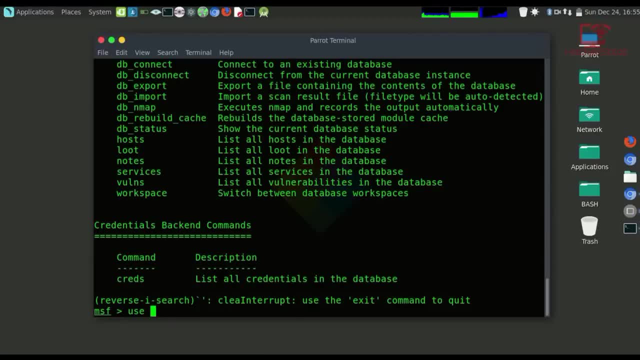 yeah, the adobe flash plugin, all right. so let me try see if i remember. so use exploit. so you use the use command allows you to use a module. so then you give the module name. all right, so use exploit. and then it was windows. all right, so it is a windows and then browser, right? 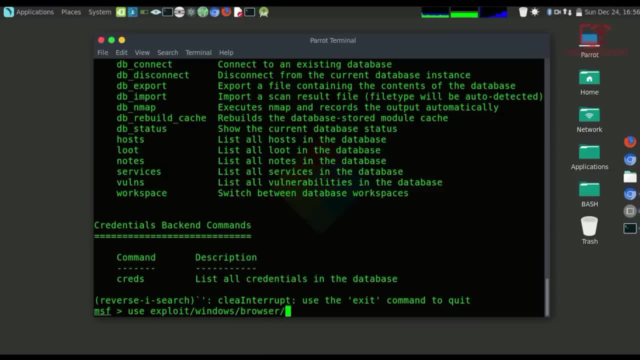 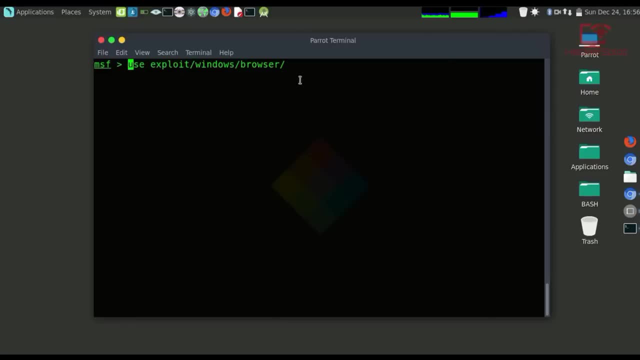 and uh, was it flash? oops, uh, let me just bring that in into context here. like so, uh, i think i already clicked on it. i'm really, really sorry about that. um so, let me just close that up. there we are, uh so use. sorry about that, i launched it by mistake. 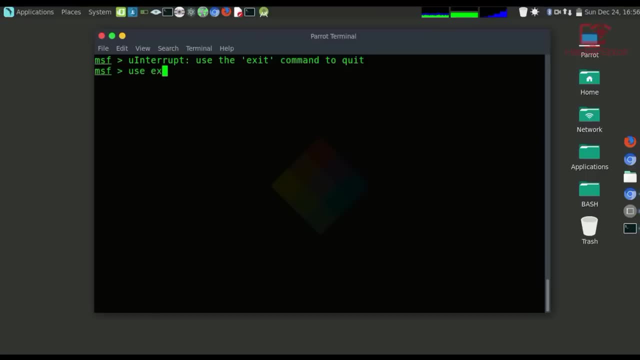 so let me remember to use exploit um windows, right, um windows. uh, was it windows browser? i'm not sure if it is the correct one. use windows browser, all right. so here you can see. it's the exploit: adobe avm, uh, app sci الك bill, i believe it. 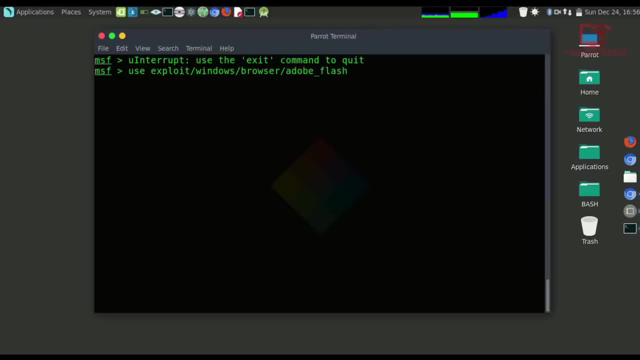 is, and it is the adobe, whoops, adobe flash. uh, avm 2, i believe was the vulnerability. oops, underscore my bad avm 2. all right, use exploit. uh, adobe, avm 2. let's see if that's the correct one. there we are. 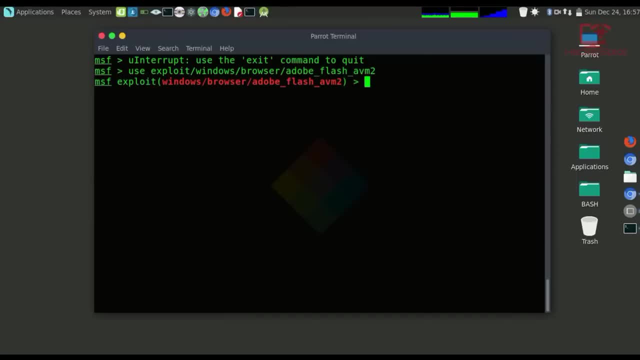 all right. so that is the exploit. i'm glad i remember it right. so that is also a very, very men's ploy. it has successfully loaded the module. now one thing to understand is: if it loads the module correctly, it will display the module name in red all. 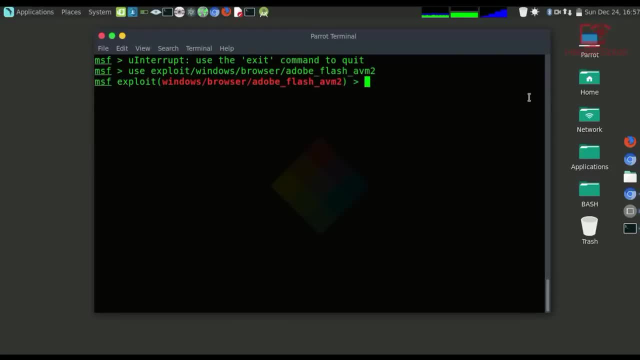 right. so that's something you know you can take home. now, since it's become red, we know that we can use it now. the best command to use now in this case is the show command, and the show command will allow you to. it'll basically give you. 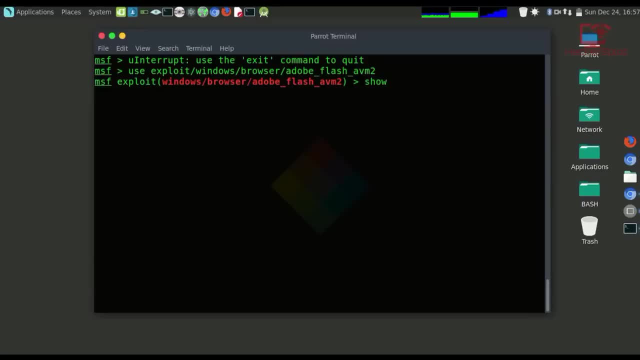 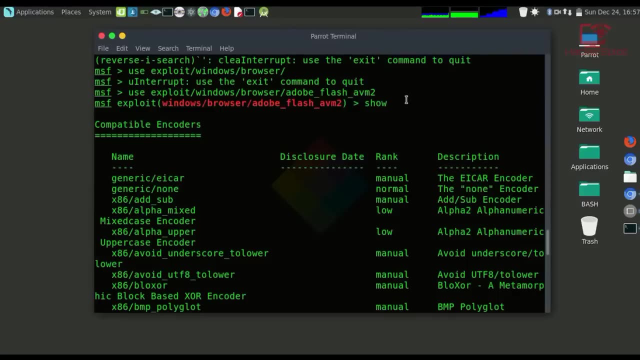 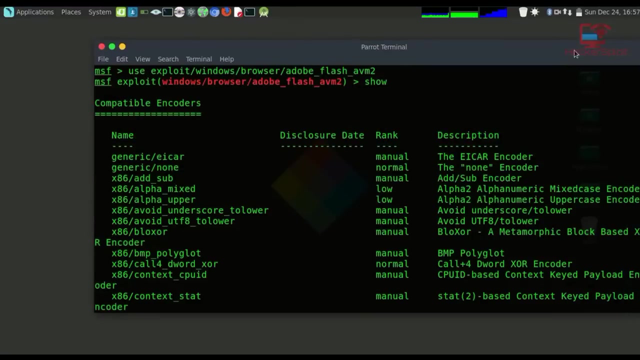 information on the module. all right. so if I say, show, there we are, it's going to give us some information. now it may seem overwhelming, but really don't worry. so it's gonna give you some information and you really don't need to worry about what it's telling me because I'm using a, I'm using the flash player exploit and 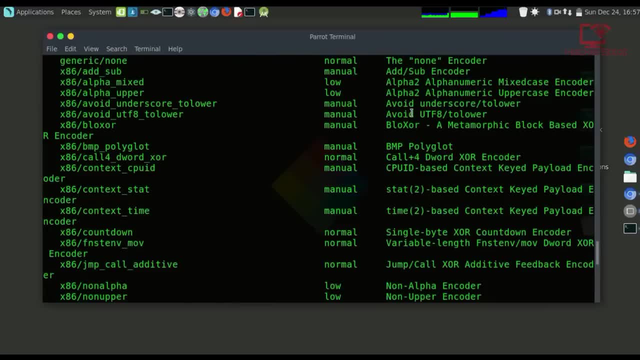 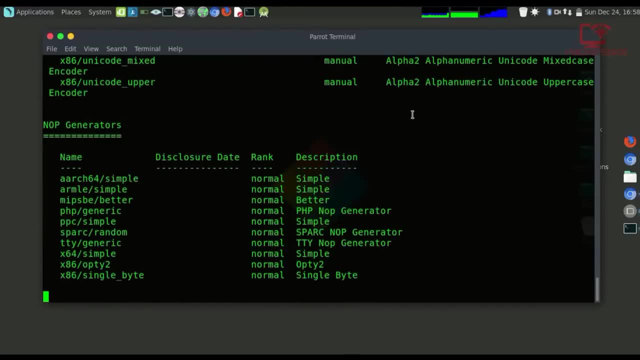 all of this may seem like nonsense to you, but we'll get to how to use the correct modules. all right, so, as you can see, it's given me some options and very, very nicely there, you, you know these are the. it's given us information about the. 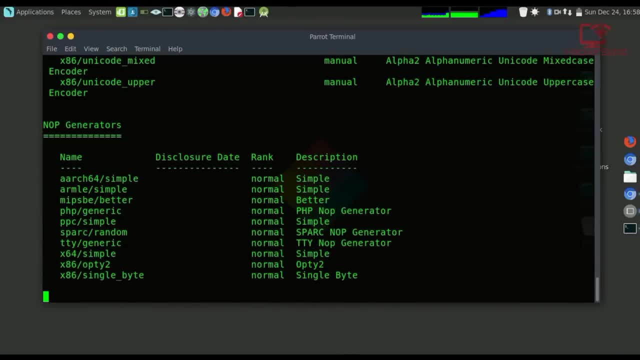 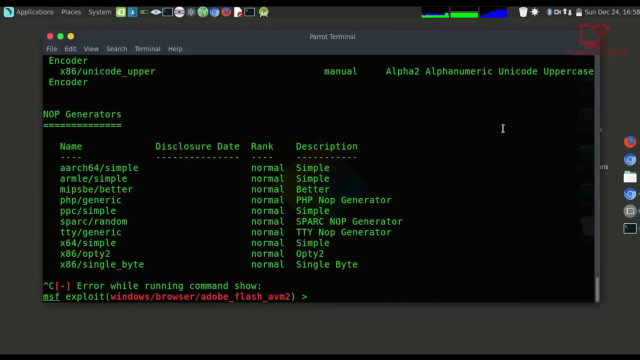 the exploit or the module. right, so now what we can do is we've already show, we have already shown what exists, the information that exists. now we can show options. all right, so the options will show us the options that we can change about the module. all right, so it will give us, you know, the, it will give us options that we can change. 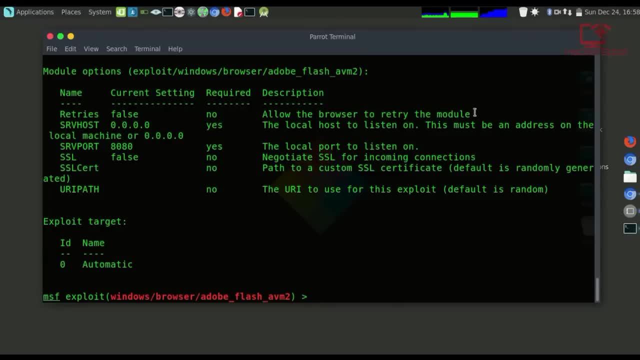 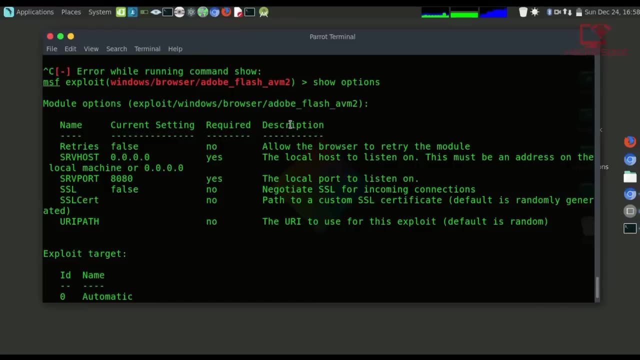 so if I say, show options, there we are, it's going to say what now these are. you can customize depending on how, you, how and the method of exploitation. all right, so you have the server host, you have the local machine, the server port, whether it has SSL, the SSL certificate, you. 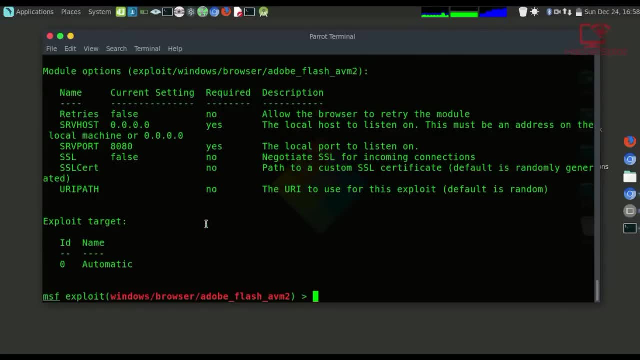 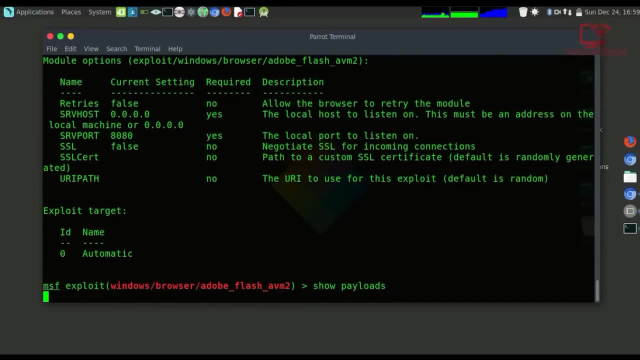 can change all of these options. all right now. the other options that we have is the payloads- show payloads. all right, once we show the payloads, just give it a few seconds. it's gonna take a few seconds, obviously, right. so give it a few seconds and it should load up really anytime now again. 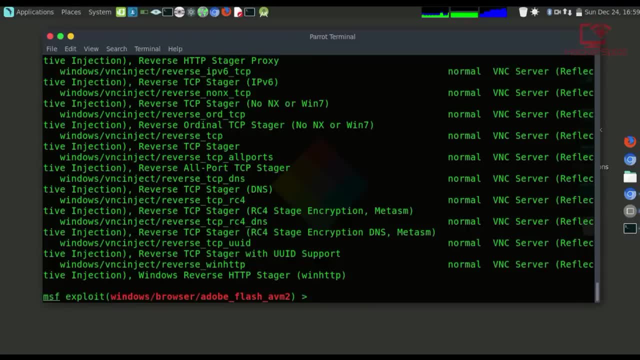 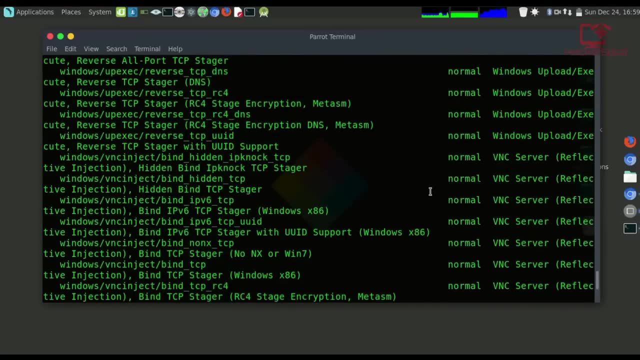 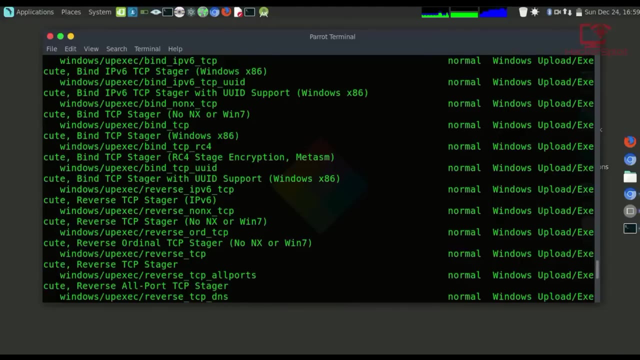 please bear with me, guys, my I'm running this on a laptop. there, we are all right. so these are all the payloads that you can load now. these, as we have looked at, you know, in previous videos with Metasploit, give us different, different ways of approaching an attack. all right, so it will give. 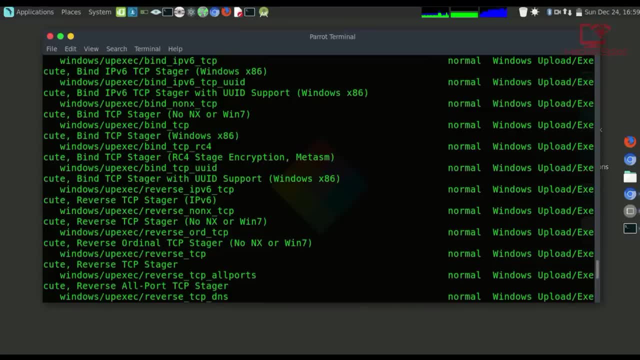 you or you, it will give you all the payloads that you need to be able to use in order to get the payloads that are compatible with this exploit all right now, if we look at the other options, so you, we will be looking at all of this. if you look at the other options, we have the show targets, all. 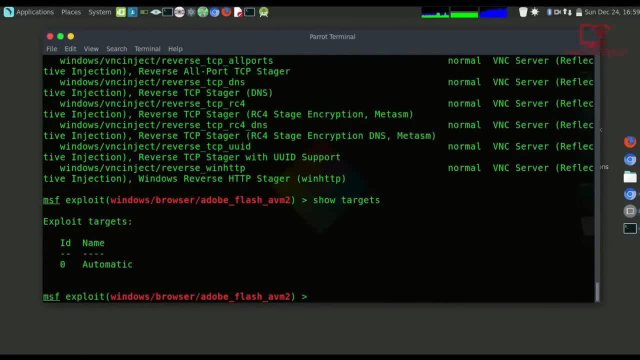 right, so show targets- will show you the targets that you can change, which, in this case, is just: we have not set anything. all right, now the targets, um, we can. it's going to display the targets that you're trying to target, um, and you know the thing is, with a different exploits you can have. 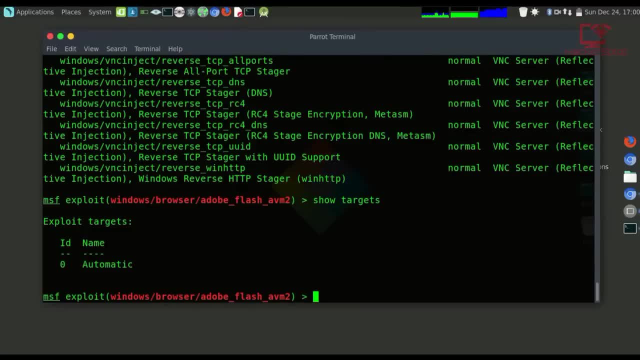 a lot of different targets. you can specify many, many targets, all right, and it's really important that you get this right now. some other commands, uh that we can use, you know that can describe, uh that can give us information about the module or the exploit that we're using. is the show info. 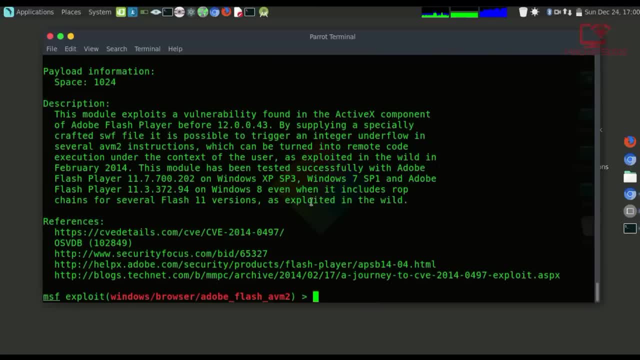 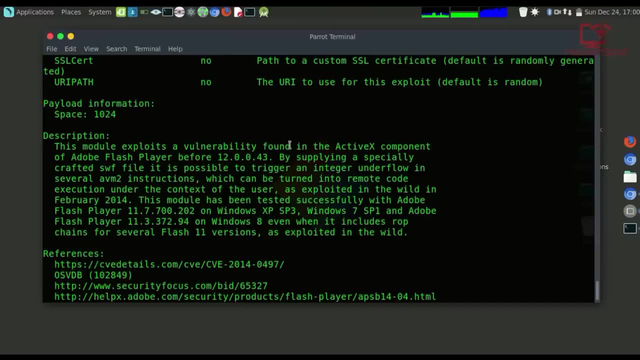 all right, the show info will give you information about. uh, it will give you information about the exploit, all right. so, as you can see here, this module exploits of vulnerability found in the activex component of the Adobe Flash player before 12.0.0.43. all right, so again, it's for a specific version and will not work on. 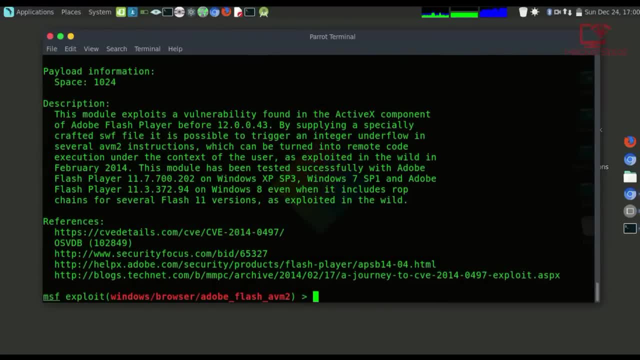 the latest one. we already knew that. right, that's the trick. now, uh, there's a lot of other comments that you can look at, and one of them is the msf search. all right, so you can use the search command, and the search command will give you the ability, uh, to search and find the module that you need. 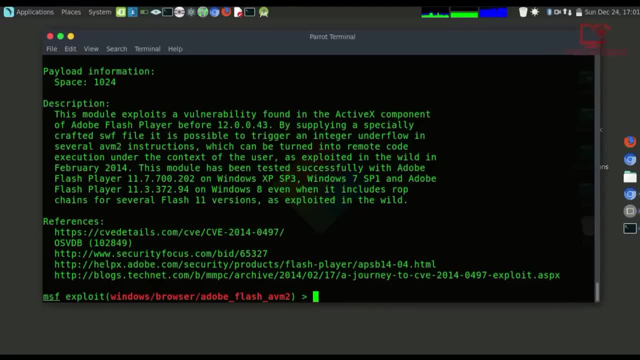 all right now. you know, Metasploit has a lot of modules and finding one, finding the right one, is probably the- uh, you know, the most important thing, and it can also can be the most time consuming, so you need to learn how to use the, the search. 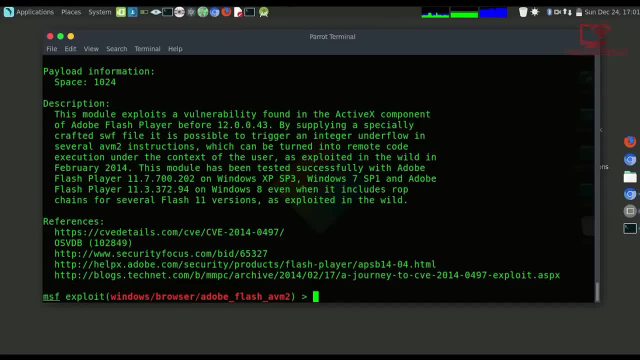 command. all right. now, with the search command, it comes with um, with some very, very important keywords. the search command comes with the keywords like the platform, all right, so this is to Target or to search for the platform specifically. you then have the type, all right. so, as we already discussed, you then have the name and this is if you're searching for a specific name. 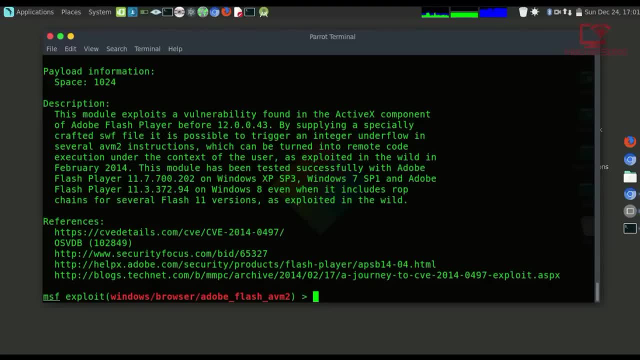 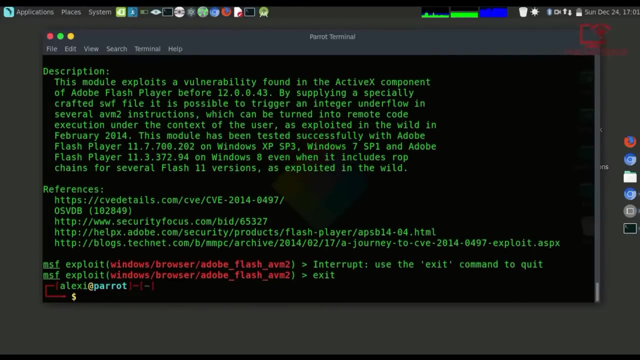 right, so we can do this very, very nicely right now. all right, so what I'm going to do is, uh, I'm just gonna, I'm just gonna control C- whoops, let me just uh exit this. all right, so I'm going to start the msf console again, just to show you how this would work. all right, so I'm going to start. 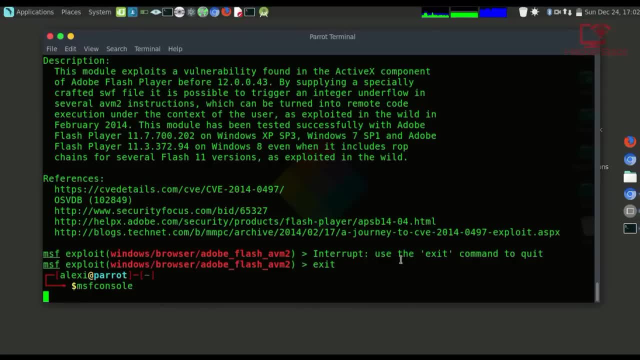 again and, uh, let's just give it a few seconds and I'm going to show you how to do this, all right? so, as I said, uh, using the search command allows you to search for exploits, so that's great, and then we'll be looking at the other ones, right? so let it start up. I'm really, really sorry about the. 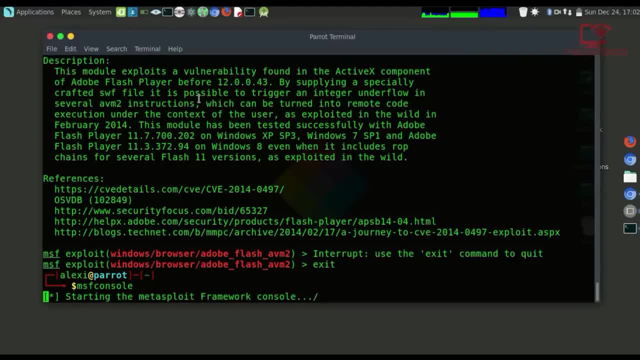 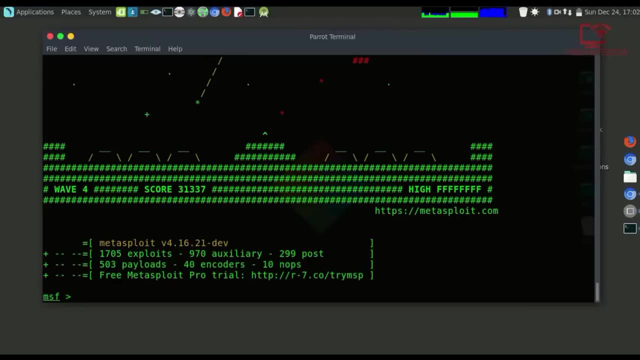 slow startup times again, um, you know just, uh, bear with me, should start up there, we are all right. so, as I was saying, uh, the most important one is the search, all right? so, if we search, it's very simple. so search type, all right, so that's the keyword type. 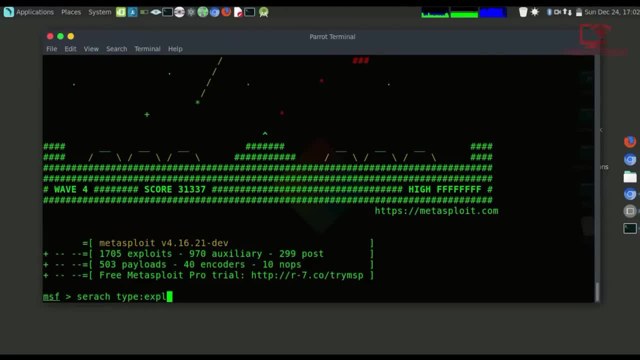 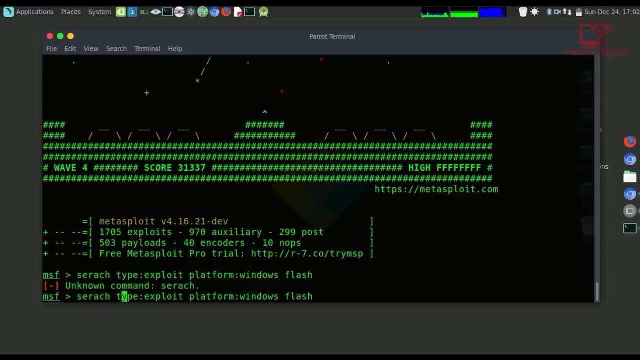 the type is going to be an exploit, we're going to search for the same one. so, type exploit, it is an exploit. the platform was Windows. the platform was Windows and flash, all right. so if we search for that, whoops, my bad, pardon me, guys, my typing today is: 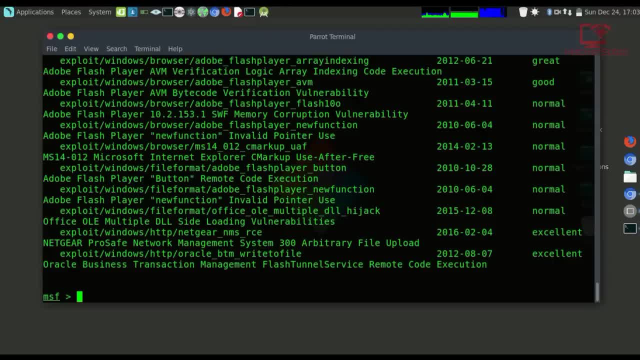 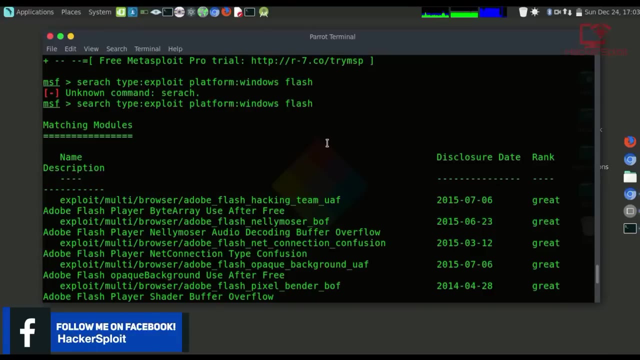 um, there, we are all right and it's going to give us all of these options. now, uh, the correct one that we want, uh is the. uh is probably the first one. it's going to lie up here and there's a lot of them that you can use or that we can use, uh. you know some of them are. they're sorted with the. 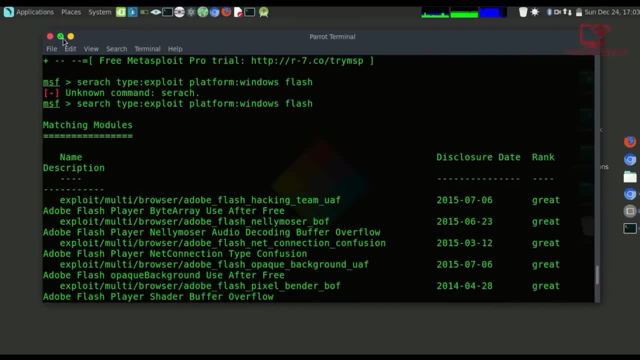 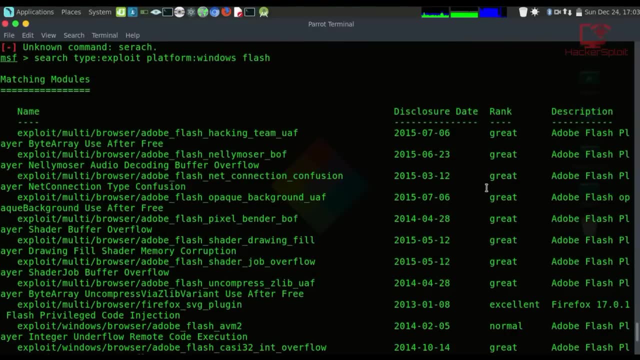 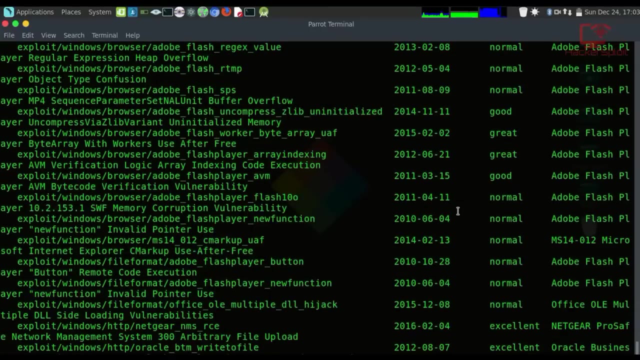 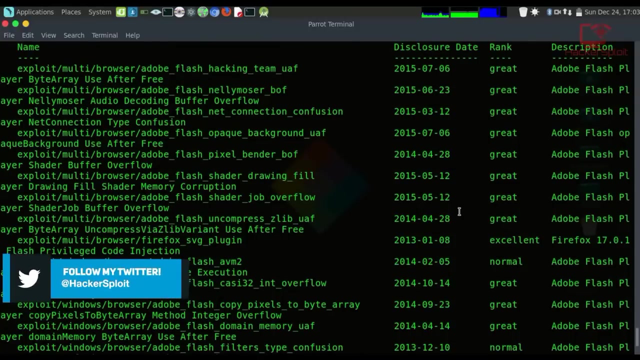 their date, their date, and this allows you to you know, specify or to get a one that works okay. so what we do now is we need to set all right. uh, now, when I'm saying set you, that allows you to set a specific um, it allows you to set the specific payload or the exploit that you're trying to use. 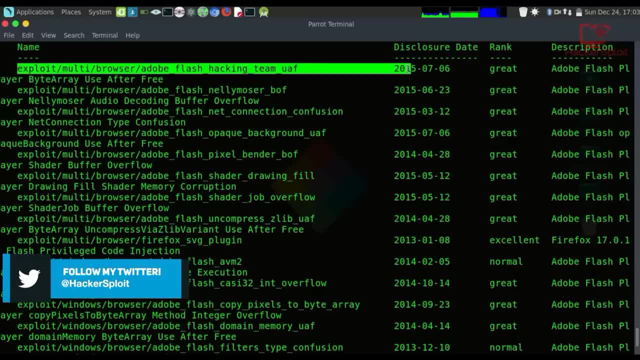 in this case, we can. you know, you can just use the first one, because I don't want to go through all of these ones. there's a lot that you can use over here and, as you can see, uh, this is the one that we were using previously. the exploit, uh, the avm2, it's very, very. 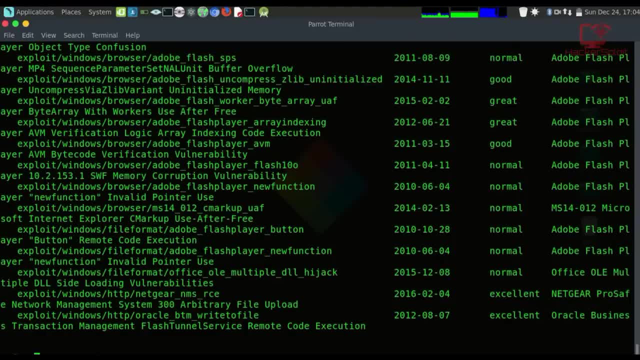 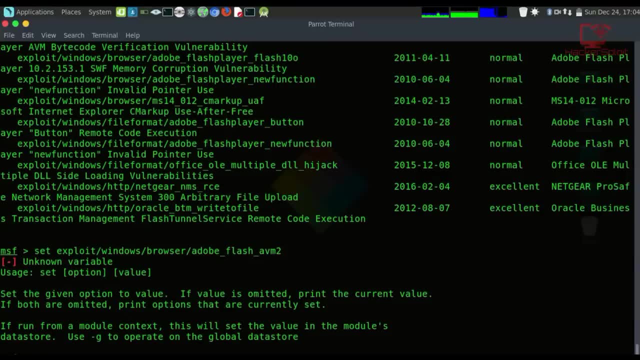 popular one at some given time. so we're going to say set all right, and I'm just going to paste that in there. there we are, and uh, whoops, uh, set option. oh, sorry about that, guys. uh, apologies, apologies, apologies, all right, so we have to use the use and uh, whoops, and I'm going to paste that. 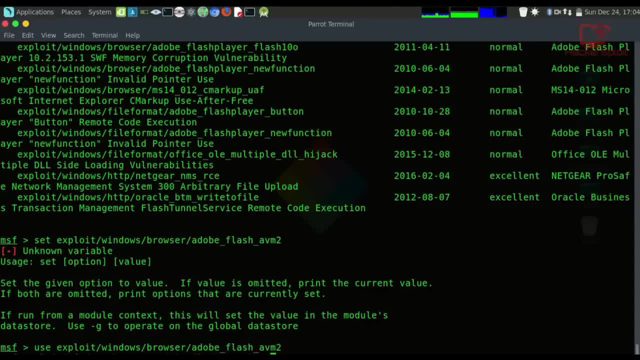 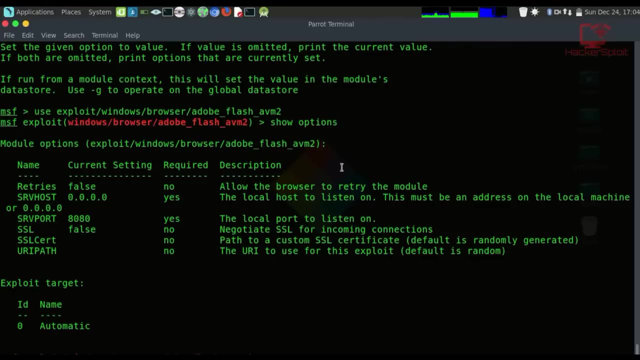 in there, use, there we are, um, so that's the module that we were using. and then we use the set to set options. so we can say, show options like so, and we have the options here and then to set the specific options. what you just do is you use things like, let's say, if you wanted to set the server port, so 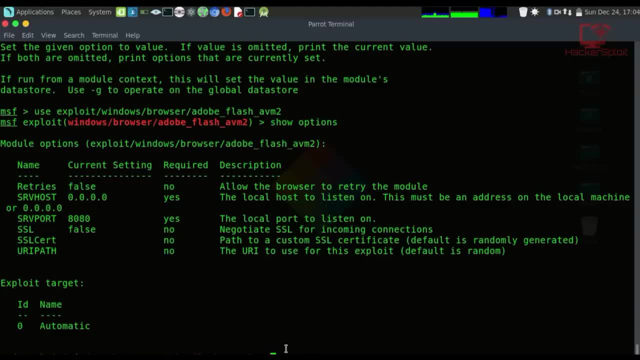 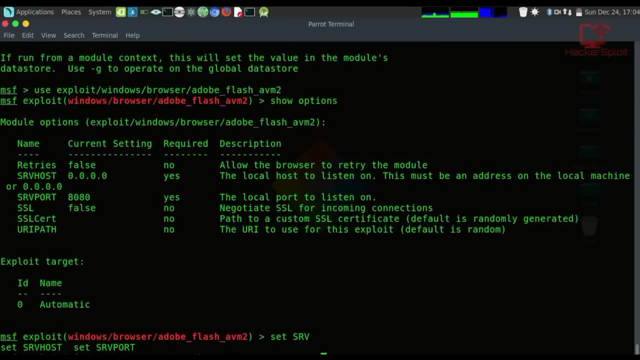 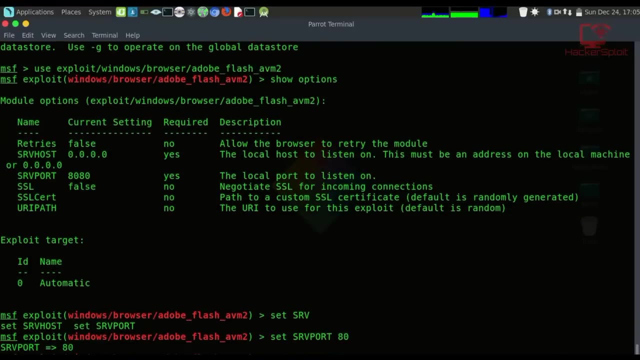 usually this would be: uh, set uh SRV server, whoops server port right, and we'll set that to 80. right, and that will set it to 80.. we can then uh say, um, uh, we can set other things, like we can set a lot of other stuff, and once you're all set, so let's say: 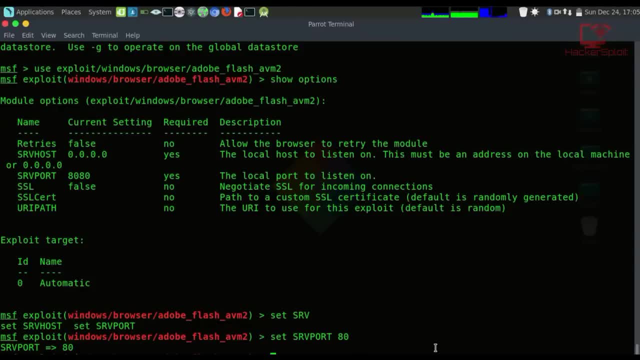 we could say, uh, set the server host to something like: um, set the server host, then that's going to be the host IP. so SRV host, all right, to something like 192, 168.0.1. of course this doesn't make any sense because I'm not really targeting a system, and you will also. 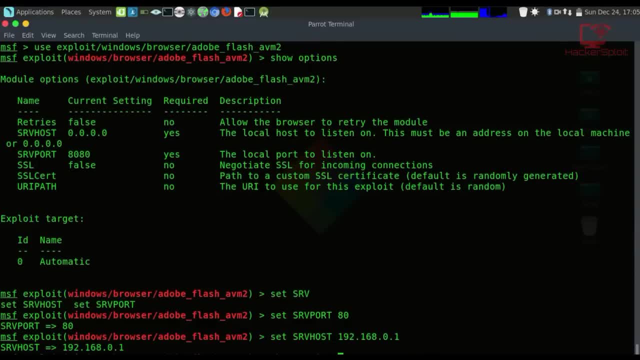 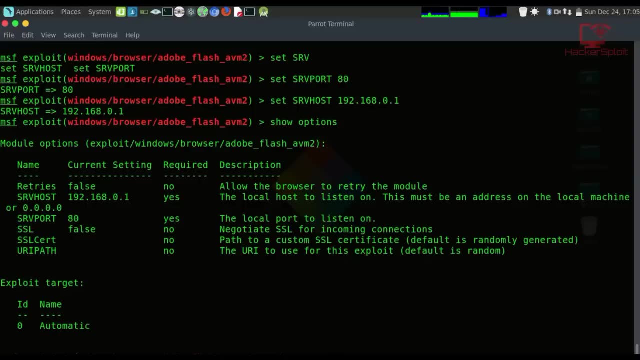 set. and then, if you say, show options again, as you can see, it's going to show you the options that you did set, which we set were the server host and the server port. and once you're ready to exploit, once you've set all the options, all you have to do is just hit exploit and it will exploit it. uh. 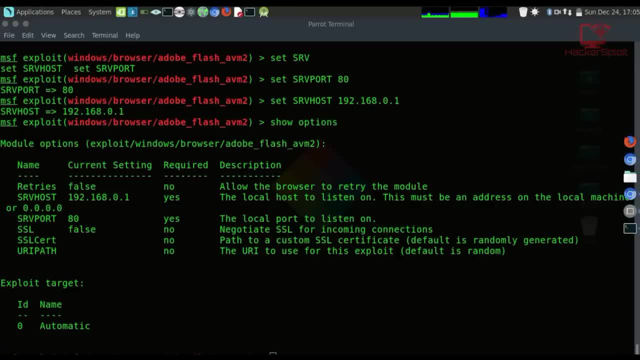 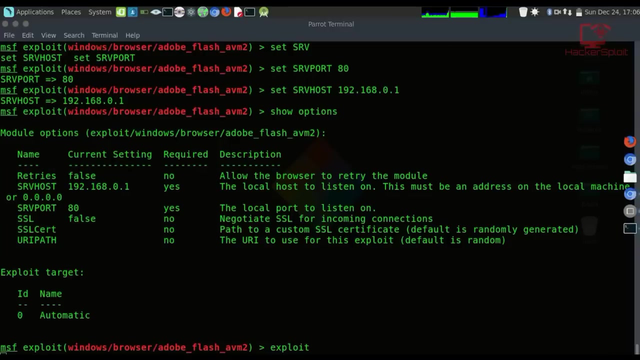 perfectly, right. so let let's try that right now, uh, and of course it's not going to give us anything, right, because we've, um, we've not done anything. so if I hit exploit, it's going to hit exploit and it's not done anything important here, right? so, uh, just give it a few seconds, right, um, again, as you can. 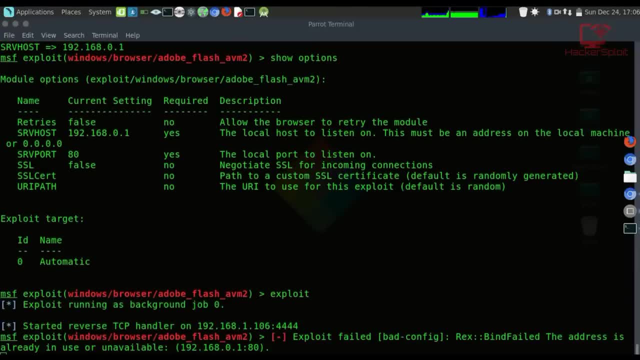 see it's not displaying anything because there we are, all right. so it did start a reverse TCP handler, uh, on a specific on this IP using the port. uh, you know, four, four, four, four, four, all right, but we're not going to get anything out of that really right now. I'm pretty, pretty sure of that, right all. 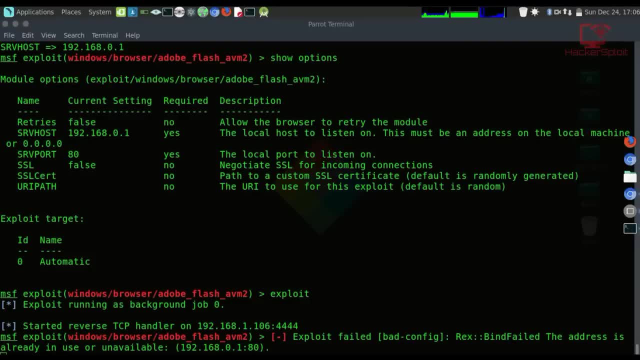 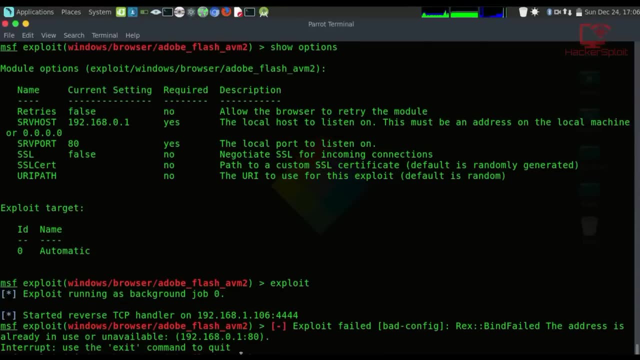 right. so once that's done, uh, once you're done exploiting- or in this case, as you can see, we have not really exploited anything- uh, we can just let me just close this. uh, there we are and we're done. now, the last commands that I want to show you are the exit or the back command, which takes you a. 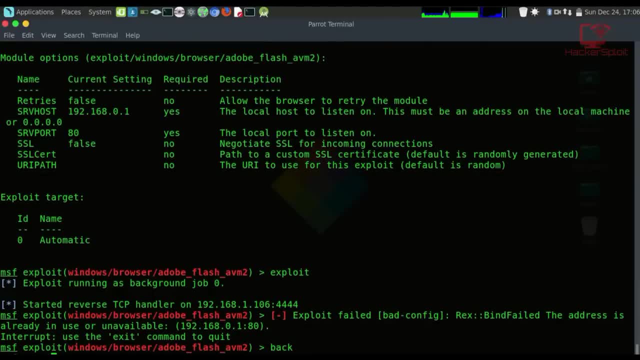 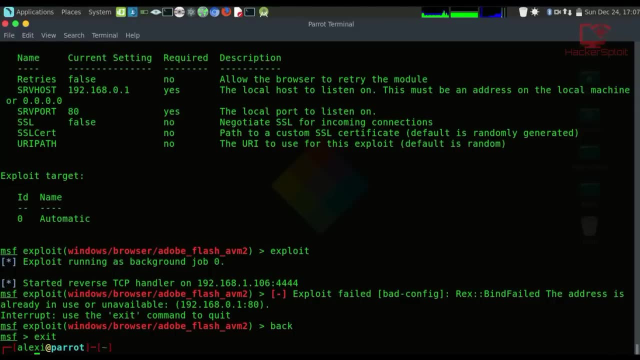 step back and you can use the exit command to exit, uh, the Metasploit or the MSF console, uh framework. all right, and these are, or that is all, the basics that I needed to cover in the first video. now, in this video, we're going to be looking at some really, really advanced stuff, so we're going to 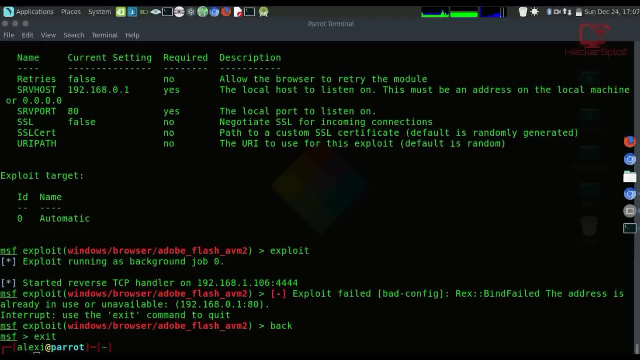 be looking at the module types uh, we'll be looking at performing reconnaissance, the armitage doi, and we'll be looking at exploiting some Windows systems and then, finally, we'll be building our own custom payloads with the MSF venom uh framework or interface. all right, so thank you so much for. 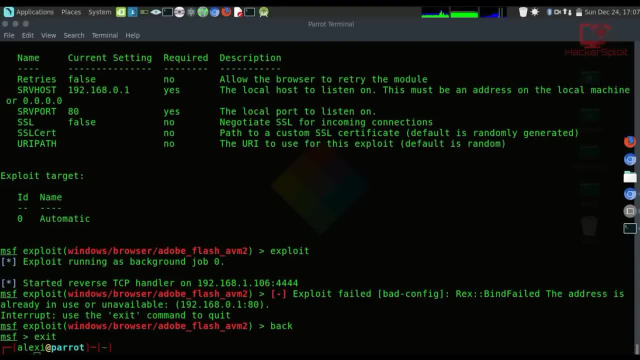 watching this video. guys, if you found value in this video, please leave a like down below and you know. if you have any questions or suggestions, let me know in the comment section down below or you can hit me up on my social networks. for the documented article or the, uh, the documented. 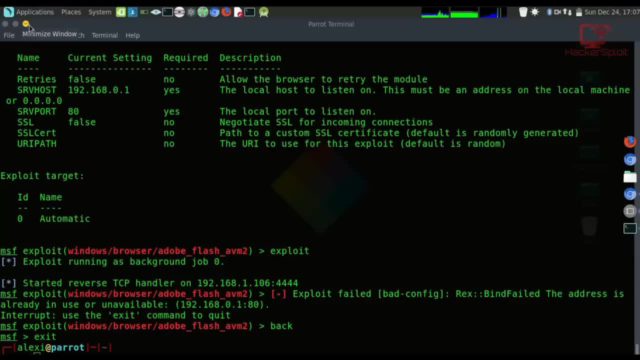 version of this video, check out my website hsploitcom. link will be in the description and you can also get this on my application. so I guess again, guys, thank you so much for watching Merry Christmas and I'll be seeing you in the next video. peace. 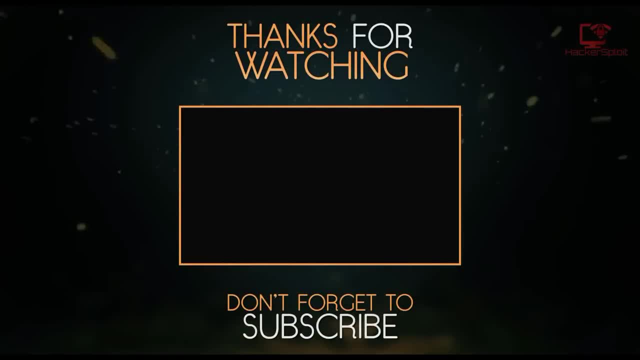 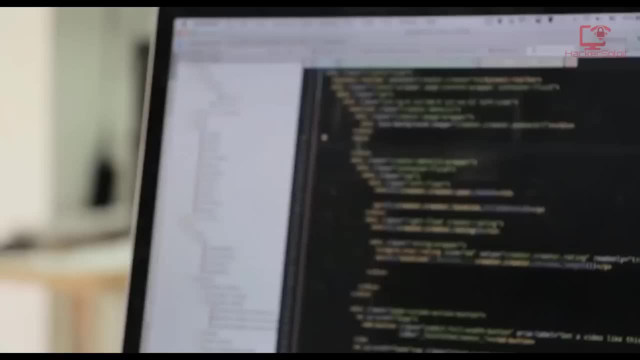 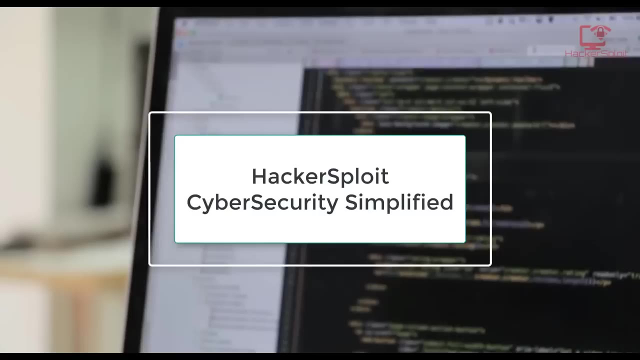 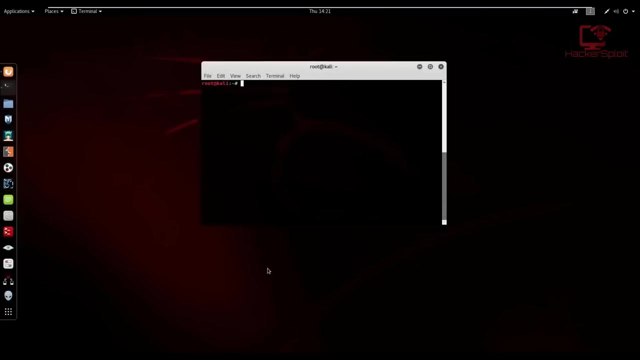 out Peach. hey guys, hacker exploit. here back again with another video, and in this video we're going to be looking at modules in metasploit. so this is part two of the Metasploit uh series, or the Metasploit course, and in this video we're going to be looking at modules. so, as we touched upon, 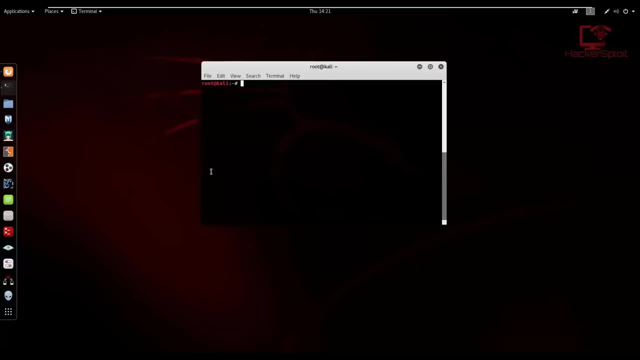 in the previous video we looked at what modules are very basically, and the purpose of that video was to take you through the interface and get you comfortable with using Metasploit. right, but now it's time to understand what each of the components are again. that will give you a better 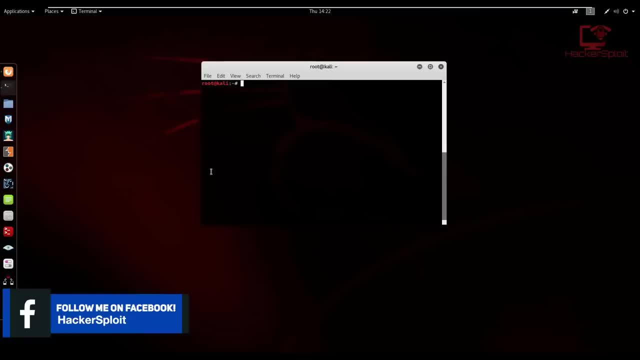 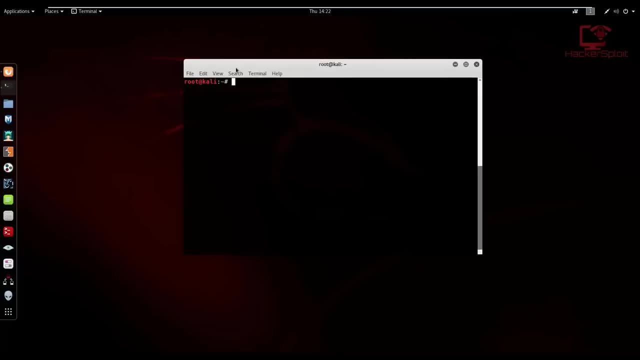 understanding of how they all work and, as we already know, if you understand something, you can get to use it much, much better than if you just, you know, zoomed over some of the concepts and some of the the you know the real core functionality of Metasploit, right? so what I'm? 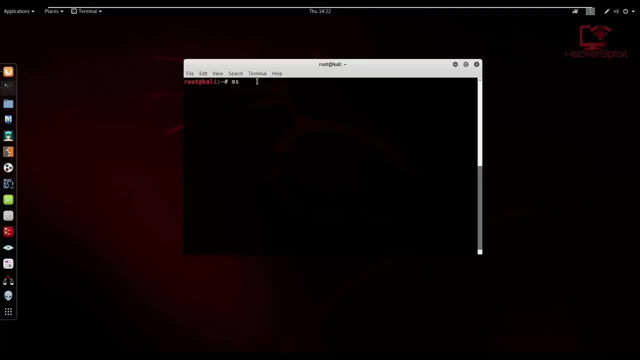 going to do is I'm just going to start up. I'm back on Kali, by the way, so some of you guys thought that I was actually sticking with Parrot. I like to keep things a little bit different here and there. so msf console, oops. I'm going to just start off with that and let that the the framework load. 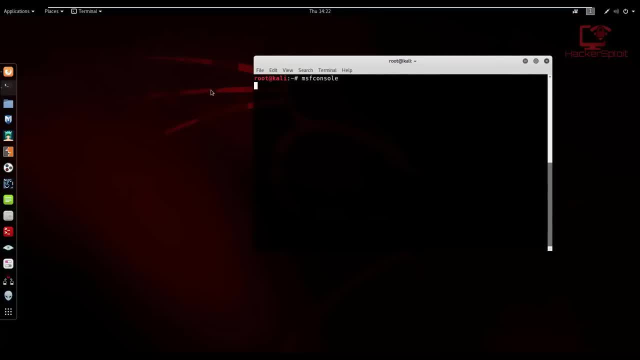 again, I'm running this on a virtual machine, so you know resources are not going to be the best right now. but while while that's starting up, I'd want to explain a few things. now, as I mentioned, all right you, when I when the Metasploit console opens, it gives you some options, right, and it'll show you the types of 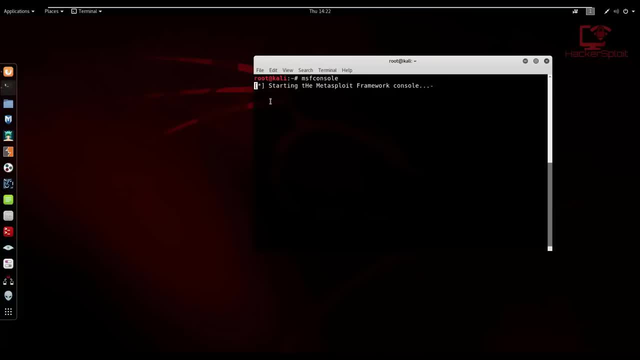 modules. now, the types of modules are like the auxilary, the payloads, the exploits, the encoders, the knobs, all right, so there are six of them and one of them is the post. all right, so in total you have your exploits, your payloads, your auxilary, your encoders, and your post and your knobs. 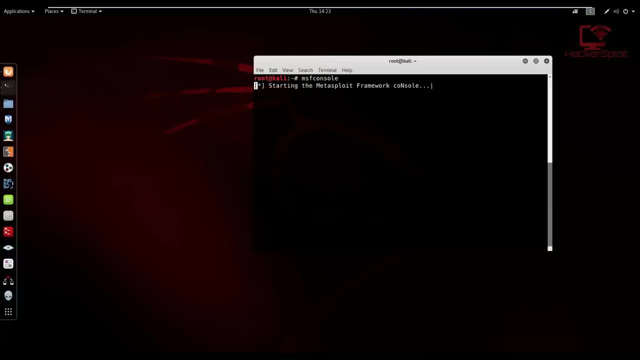 all. right now, looking at the architecture, you know Metasploit. again, it's very, very, very important that you understand this. looking at the architecture, the, the. the basic structure is that modules are categorized into six, which I've already mentioned: the exploits, payloads, auxilary encoders, post and 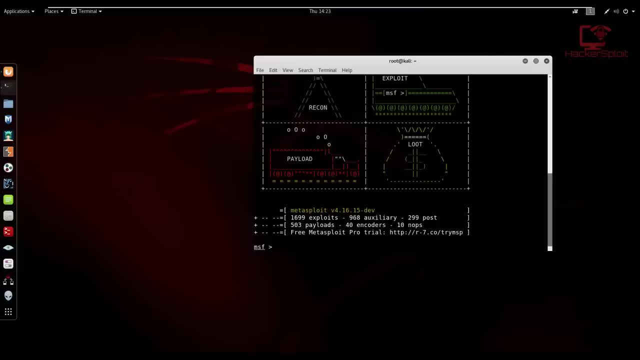 knobs, and then it the. that is then a superseded by the, the MSF console or the Metasploit console or framework, and then it is it. it is superseded then by the core and then finally, by the Rex in terms of the libraries. so to put this, 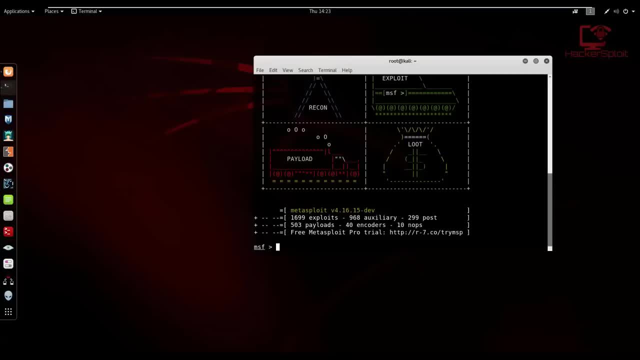 into the interface in. to put it into sense, when it comes down to interfaces, you have your GUI and Armitage, you then have your command line interface and then, finally, your console. so I hope you get that in terms of the architecture, all right. now something very, very important to understand is to understand where the modules are stored. all right. 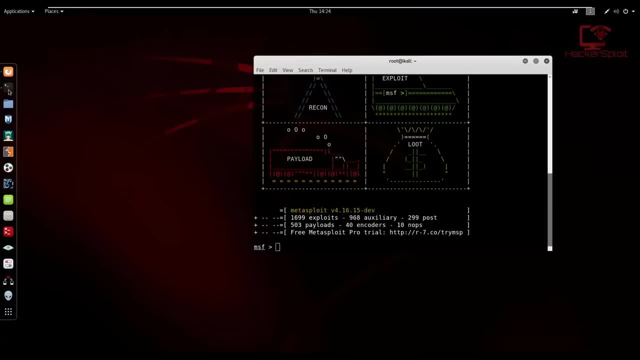 so we can just go, you know, open a new terminal here. hopefully that lets me open it up right now. all right, so new window again. bear with me, the speed could be a bit of an issue, but don't worry about it, I'll sort that out in probably the next videos. it won't be this slow. for some reason it's. 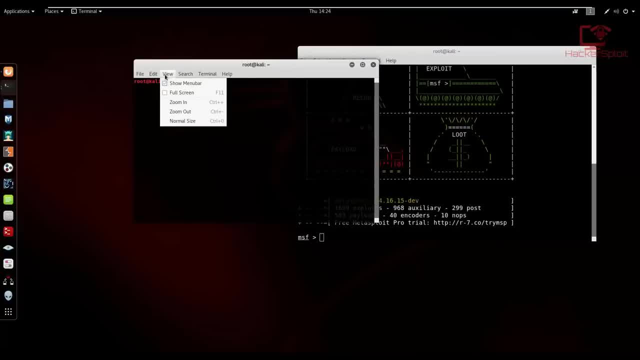 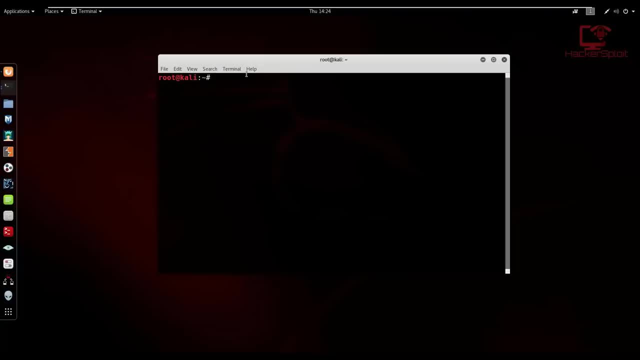 really, really lagging out right now. all right, so what I'm gonna do now is: let me just zoom in so a a better picture of what's going on here. all right, so now, most of the time- or all of the time, should I say- the Metasploit modules are stored in the user and the share folder. all right, or? 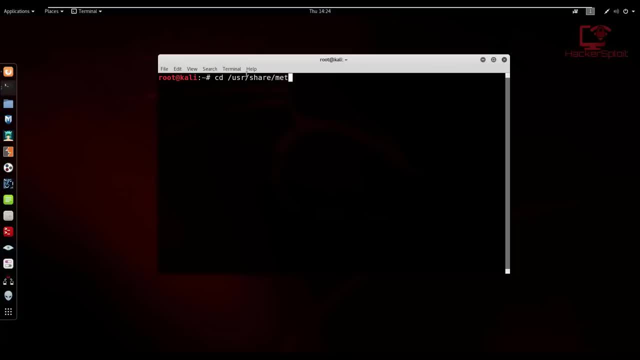 the shared folder. share and again Metasploit framework. whoops, let me just complete that Metasploit framework framework. all right. now, again, that's a directory. now you might be wondering what is in here. well, the modules line here, all right. so if I list all the files in here, as you can see, 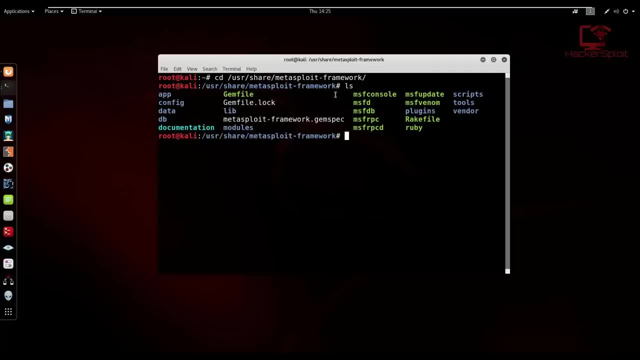 we have an interesting bunch of files. we what the one we're targeting is going to be the modules folder, right here. right, because that's another way of accessing the currently installed modules or the used modules, right? so see, uh, let's go into them into that folder. if we list the files in 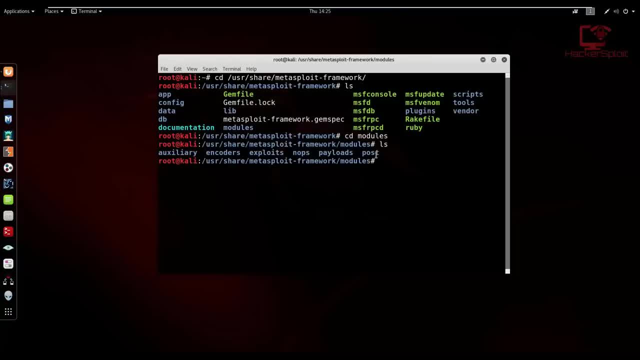 here. as you can see, it's further divided into the six categories that I mentioned earlier. we have our auxiliary encoders, exploits, synops, payloads and post right very, very interesting. you might be asking: what do we do now? now, the point here is: I was trying to explain the directory, the file directory structure, and 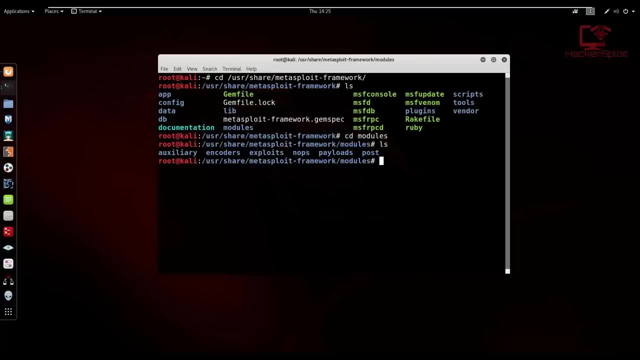 how it's really sorted out. okay, now the modules. uh, the directory contains the six sub directories, all right, which then contain a different type of module. uh, sorted into into what you see. all right, now let's start off with the exploits. right? the exploits usually are used for 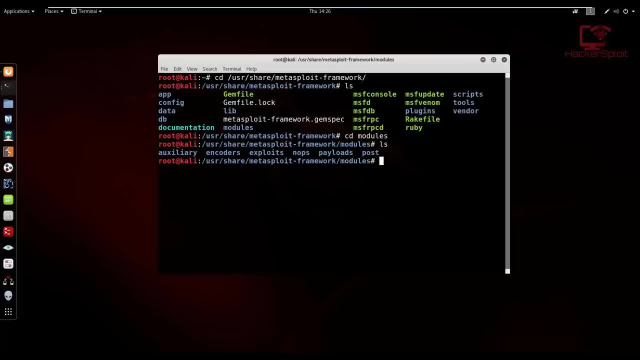 exploitation. you know very, very, that's very easy to understand. uh, these are modules that are well allow, that were created for, for you to take advantage of an exploit or a vulnerability in a system. okay, so let's see what we have in exploits. so I'm just going to go into exploits. 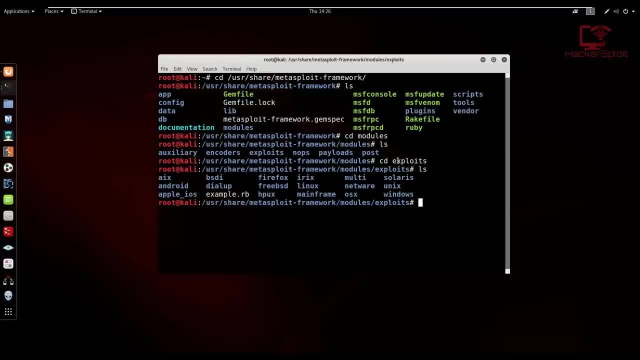 right now. see the exploits, if I list that, as you can see, these are the current exploits that you have sorted out in terms of the operating system or the target operating system in which there is a vulnerability. so you know, for example, you have Apple, iOS, Android, Firefox, free BSD, Linux, you have your Solaris, Unix. 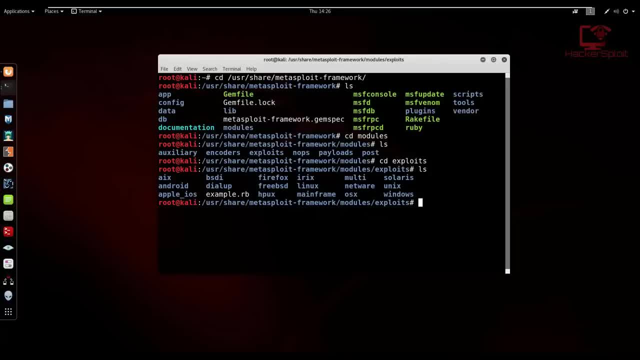 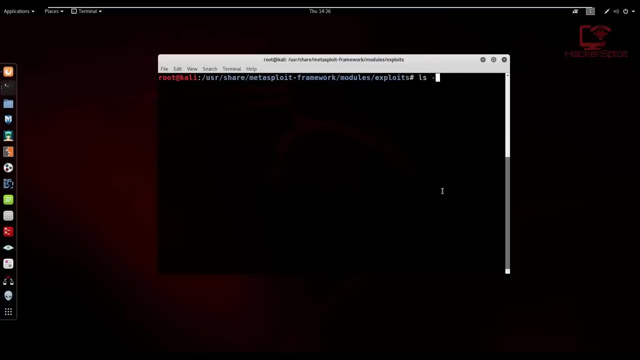 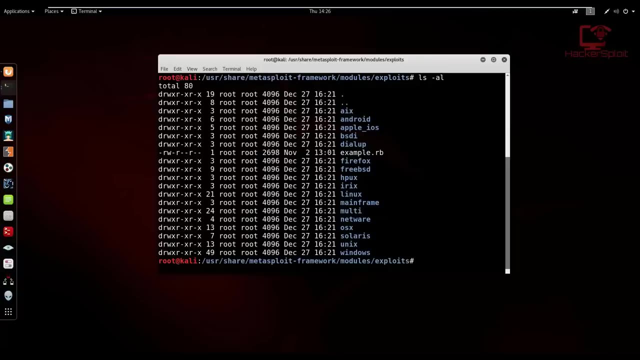 Windows and obviously a Mac OS X, all right. so, as you can see, this lists everything really really well. uh, let me just list that correctly. I wanted to list everything there. we are all right. so, as you can see, they're listed into further sub directories, which are sorted in terms of the. 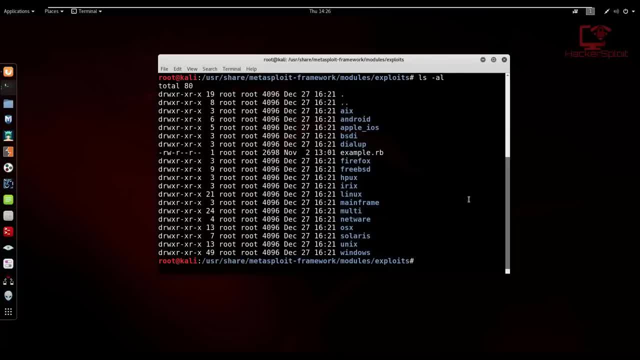 operating systems. now we'll be looking, uh, again, these are just meant, or you know, specific to the operating system you're trying to target. so if I was to try to try to target Windows, and I list what's in here, as you can see, you're going to have a lot of other files and the again. 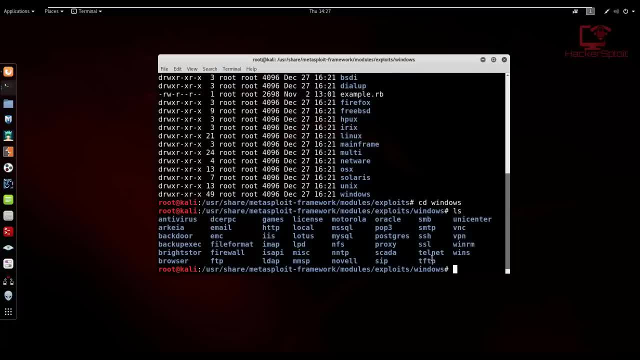 further sub directed into their different forms of vulnerabilities. like you could exploit the, the Oracle, PostgreSQL, proxies, um, the firewall, Etc, Etc. you get the idea. so exploits are used to, to take advantage or to exploit a vulnerability in a system. right, that's one type of um, of a. 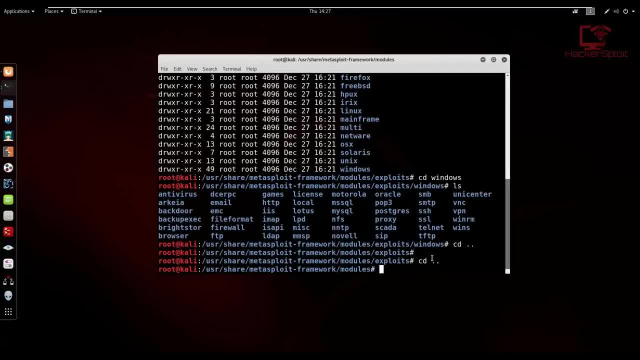 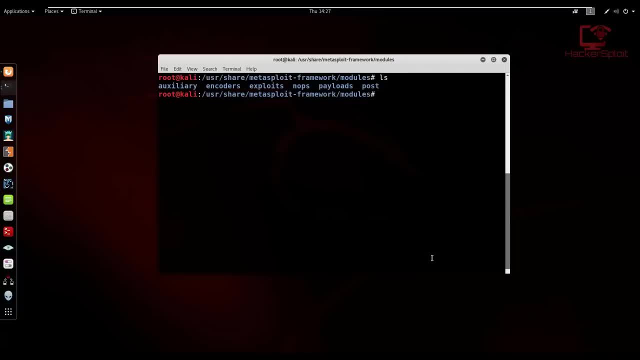 module now. uh, I'm going to back out and I'm just going to clear that, and let's look at what other modules that we have. the other modules that we have are the payloads. all right, or you can go into the encoders, but let's look at payloads first. all right, so payloads- uh, these are files that are left. 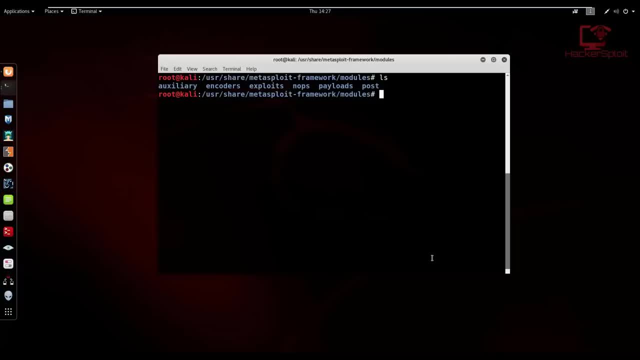 on the exploited system. all right and, basically speaking, what they allow you to do is they give the attacker access or control over the system right now. um, these are usually called root kits, uh, or well, most of the time they're really separated from each other, so not so basically not all payloads are root kits and you simply put payloads allow. 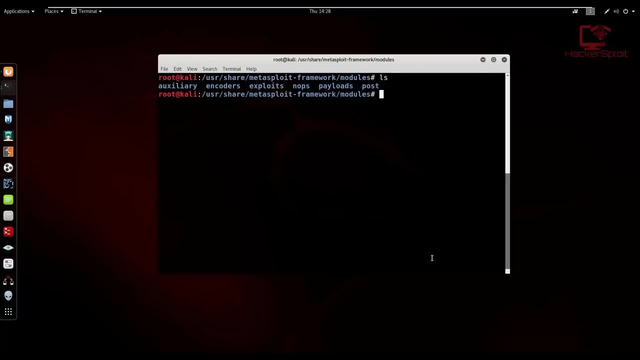 the attacker to own the system all right in which they are left in. so let's see what we have in the payloads folder- right CD payloads- and if we list all the files there, as you can see, you have your single stages and these stages. so let's see what we have inside each of these directory. 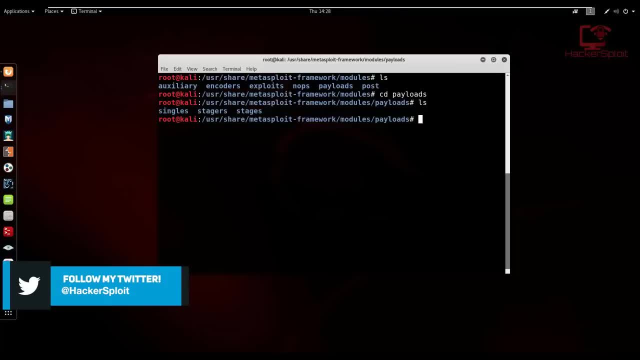 now the. as I've said, they've been divided further into three directories: uh, singles. are these? these are small? um well, I don't know how to explain it to you. these are like these small. uh, these are small pieces of code, or, or, I don't want to say exploits. they're usually designed, uh, they're. 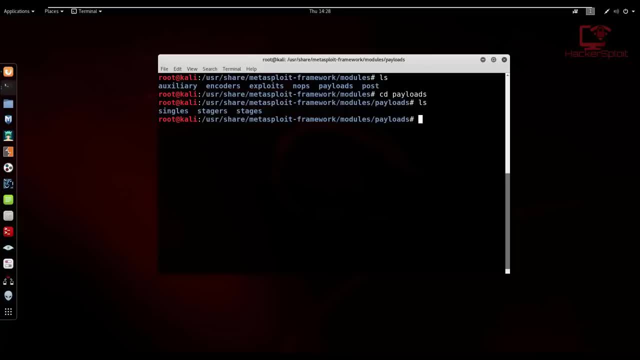 designed to to take like one single action. all right, now stages are used for performing or, you know, creating a communication between the attacker and the um and the target, and this can be then further used to deliver another payload. all right, and stages, stages are very, very large payloads that 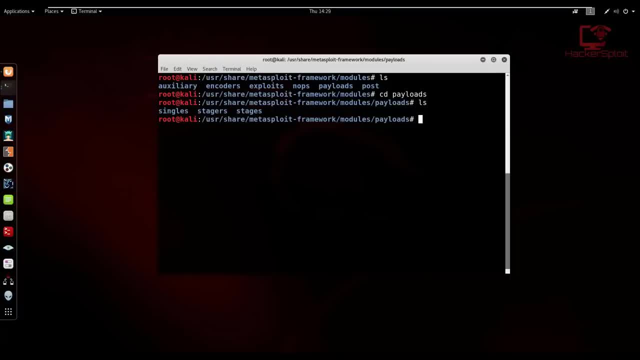 can give the, that can give the attacker like a very, very, very good control over the target. uh, so you, for example, this can allow you to have meterpreter instances, you can have VNC and stuff like that, right, uh, and that's what, um, what payloads offer in terms of single stages and stages. so singles are very, very small. they're. 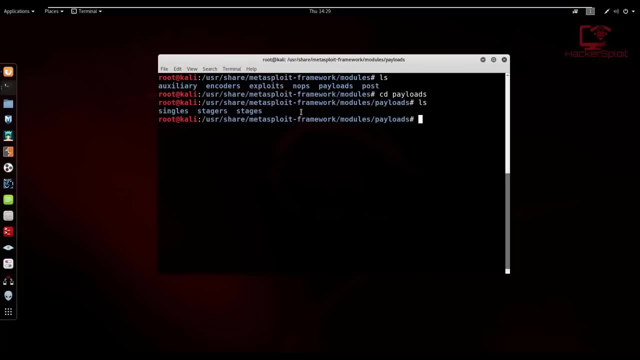 used for performing one specific attack. like you know, key logging, for example- that's a very, very vague example- stages allow you to perform or to um, to create a communication, an instance of a communication between the attacker and the target that can then be used to send another payload to. 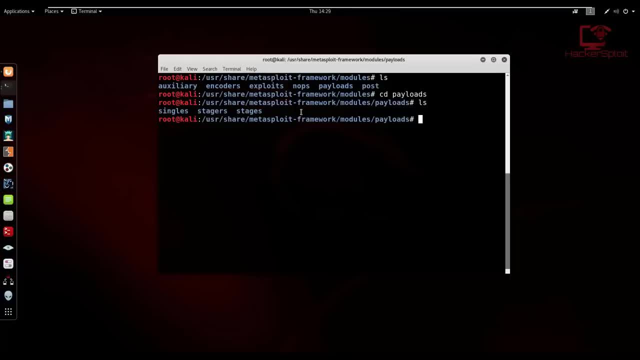 the system, the, the target system, right stages are very large payloads that allow you to perform large or, you know, potentially more dangerous uh types of attacks, uh, the likes of you know, VNC connections or meterpreter shells or even reverse shells, to be very, very basic. right now let's go back here. 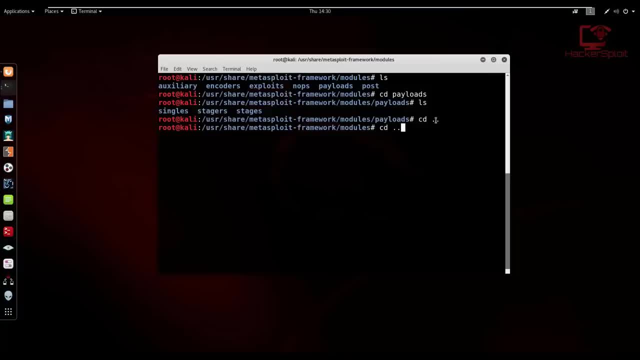 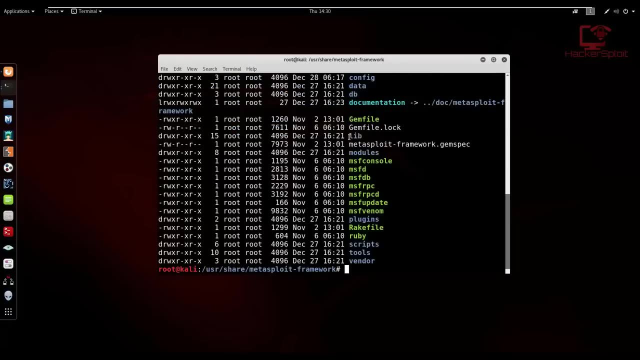 okay, and I'm just going to go back and again, we're looking at the other types of the other types of modules here. the next one that we're going to look at is the auxiliary. uh, and the the auxiliary. oops, let me just go back into modules. I seem to have gone further. 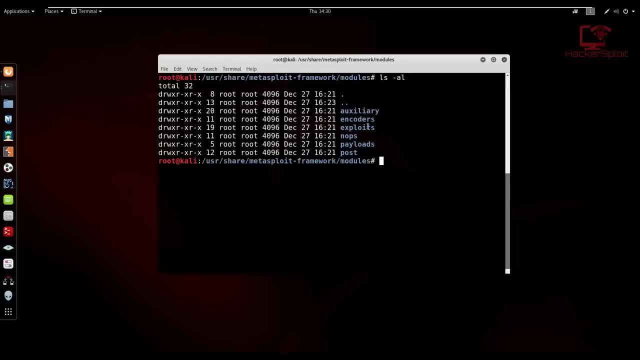 out all right. so, uh, looking at the. we have looked at the exploits and the payloads. now let's look at the auxiliary. all right, the auxiliary is something very, very interesting. all right, the auxiliary, uh, will give you a very, very, very um, unique types of attacks in, in the sense they give you things. 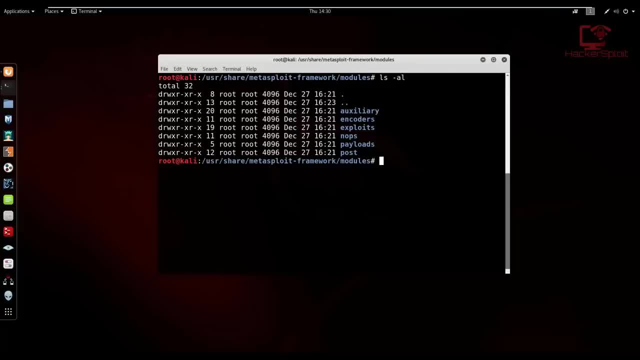 like: uh, DOS, uh, they give from DOS functionality, they give you further functionality, they give you scanners and uh, Again, this is becoming really, really popular because again, they're giving you things that that you cannot find in other- any of the other categories, whether it be payloads and exploits. 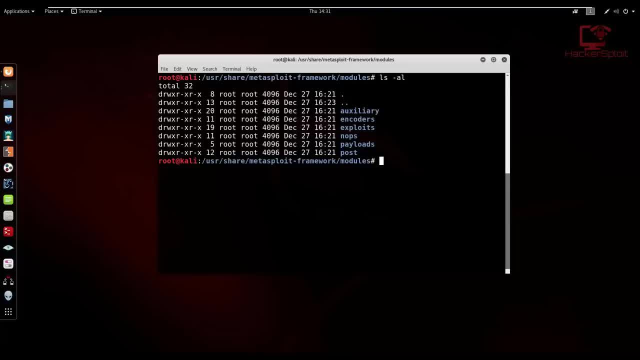 All right. So the auxiliary is giving you very, very robust tools, things like, you know, DOS functionality, as I've said, scanners, So you know vulnerability scanners and stuff like that, So things that can really really come in handy. 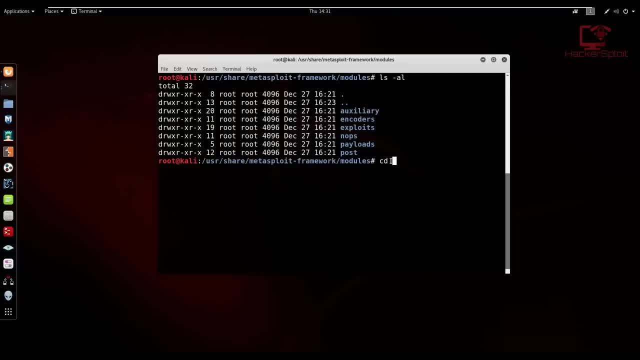 So let's explore this further, Right? So CD, a change directory into auxiliary, All right, And we'll list that in there And, as you can see, it's sorted into something very, very interesting. So you have your crawlers, you have your sniffers, parsers, your scanners, your spoofers and you can check them out. 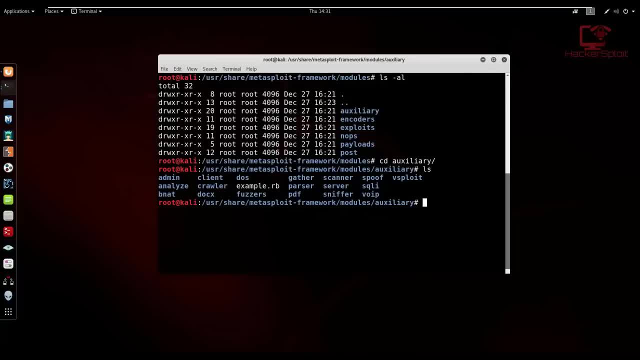 There's some. you know they're divided further into these awesome directories. Right Now, again they're they're going to be categorized into. you know directories that you will find familiar if you've been hacking for a while. You know things like sniffers, fuzzers, et cetera, et cetera. 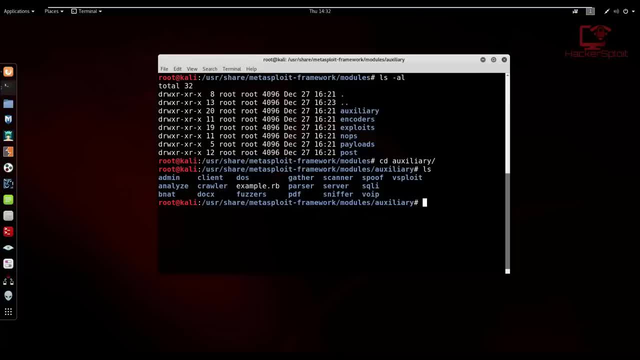 And they're the primary use of. an of the auxiliary is to is to scan the target system. All right, So they allow you to scan for vulnerabilities and to perform probably most likely denial of service attacks. OK, so that's. that's basically what the auxiliary is, simply put. 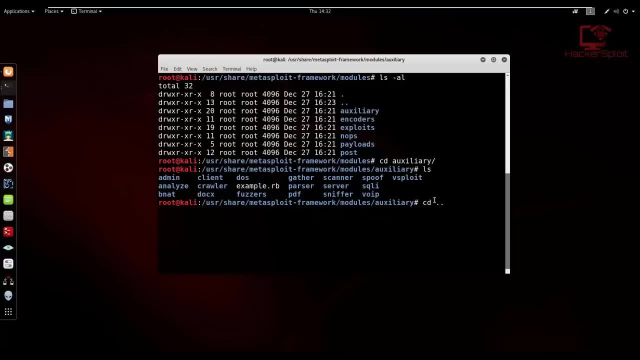 All right, Now let's look at the other modules. Right, All right. So I'm just going to go back and I'm going to list everything again. And now we have the encoders. All right, The encoders are very, very interesting. 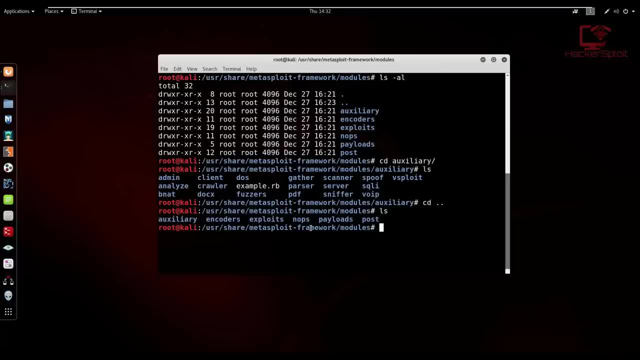 All right, These are simply do what they, they sound or what they say. The. the encoders are used to reencode payloads and exploits, All right, So they're used to- and a lot of people have been asking me this- Well, they're used to get past security systems such as antivirus. 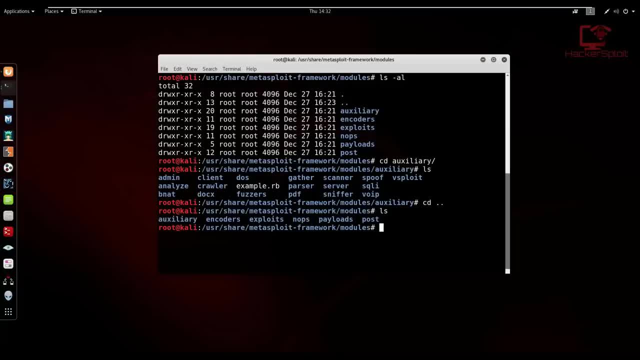 All right. So this is where you really, you really want to be looking. if you're looking for encoders or if you're looking for Evasion techniques, Right. So let's look at what we can find inside. It's a CD encoders. 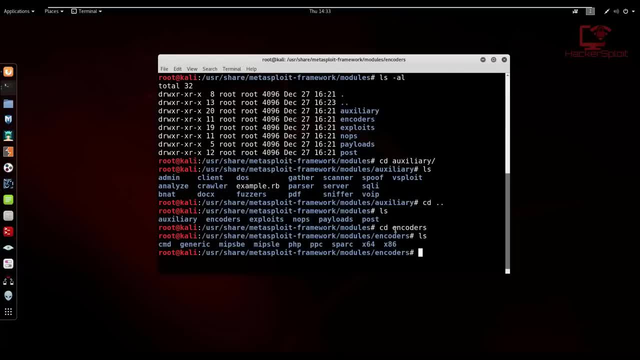 Right, And let's list what we have inside. So, as you can see, we have different types here And this may be confusing. Let's browse further into these, the subcategories, which, one of them being the PHP list list, And in here you might not understand what's going on. 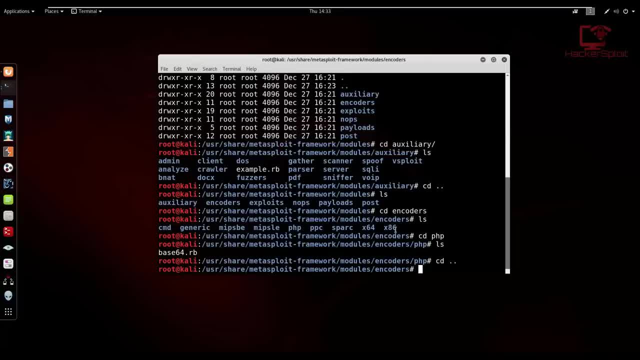 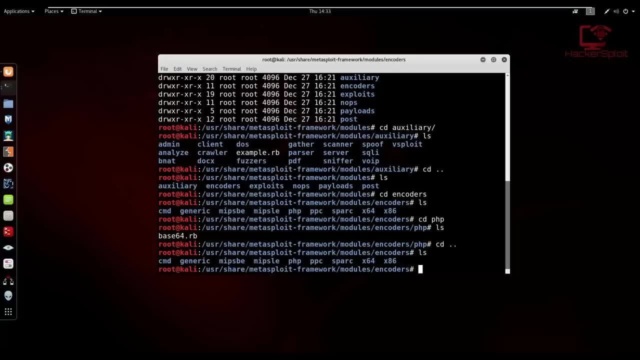 And we'll trust me, we'll be looking at all of this because it's very, very vital to understand this. Now, listing all the sub directories, you can see That they are divided into somewhat understandable categories, Right, So they are divided into, you know, for example, CPU architectures like 64 bit, 32 bit, 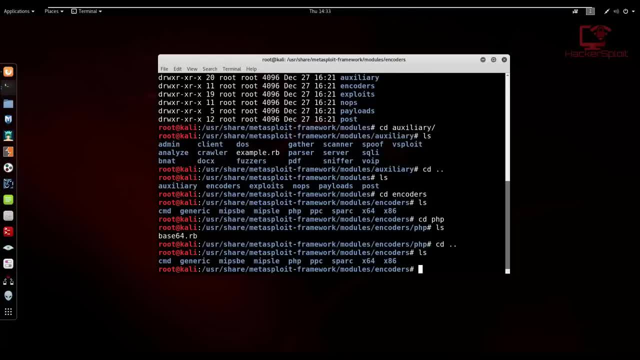 You have your, your command prompts, you have your PHP, All right. So these are, they are used, or give you the option to create an encoder or to use a specific encoder based upon the target system. So if your system is 64 bit, 32 bit, you want to go through PHP. 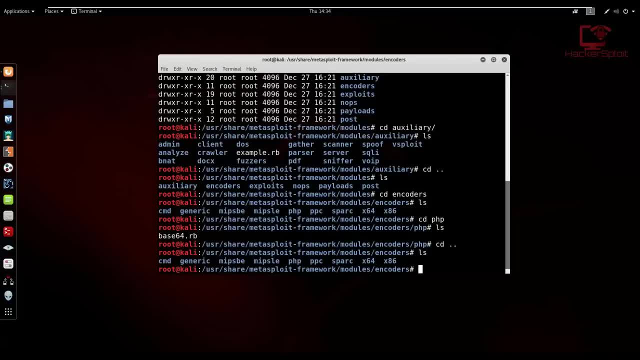 You want to use the command prompt. So again, I hope you guys are getting the idea. But it's very, very important to understand how these are divided, because once you understand that you know, it just becomes a whole lot easier. 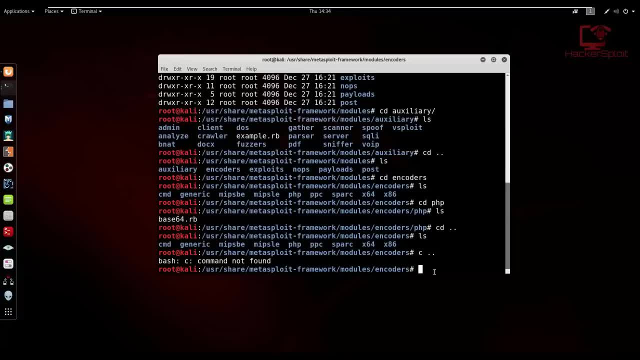 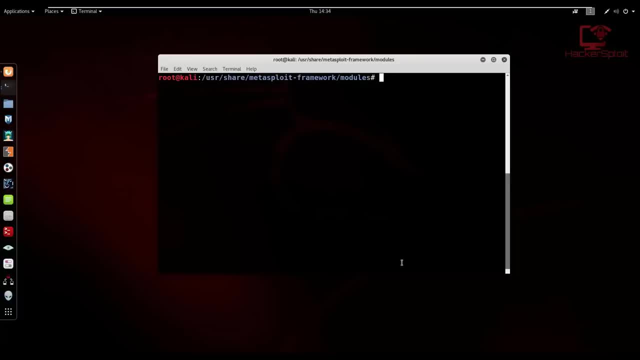 So let's go back here. Oops, My mouse pointer was there. Oops, All right. Now let's look at knobs. Right, Knops are something very, very interesting and something that not a lot of people take seriously. But essentially what? 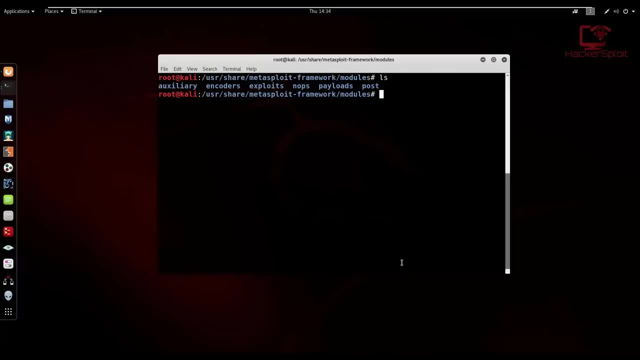 They are OK. for those of you who have done programing or you've done computer science, I'm sure you've taken a class on machine programing or machine languages. All right, Now a knob is is usually, or mostly, most commonly known as a no operation. 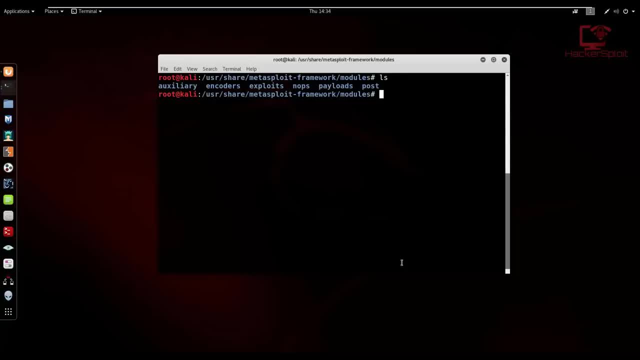 All right Now. this, what this allows you to do, is what, or what this means is, are not causes the systems Processor or the CPU to do nothing for an entire clock cycle. All right Now, this is very important to understand, Right? You might be asking: well, what the hell is this or what? 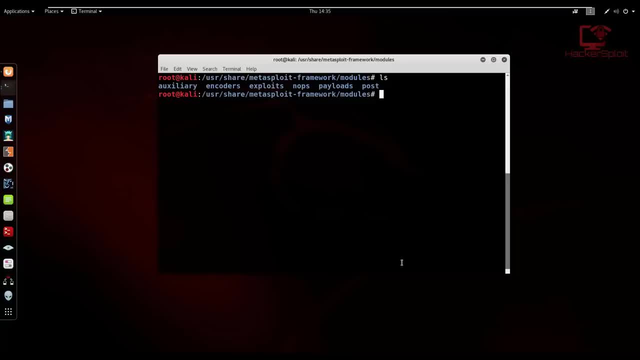 How is this going to help us? Well, knobs are very, very good for allowing you to get a system to to, to perform or to run a specific specific file, or code for that matter. Um, after you've exploited the buffer overflow. Now this may sound like gibberish if you've never done anything to do with, you know very low level language or machine language programing. 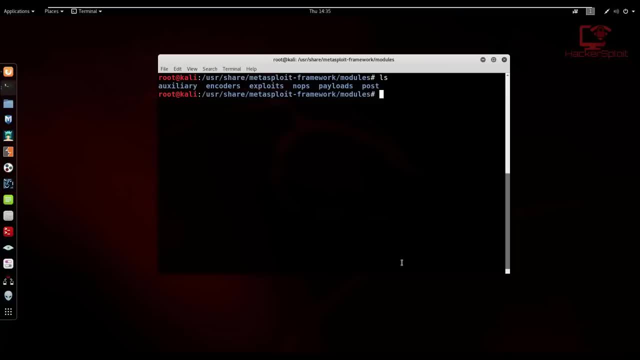 But you really don't have to worry about this. They are used to exploit the buffer overflow. OK, And essentially you really just need to know is that they're used to allow you, or they allow you, to run or to execute code or remote execute code on the target machine. 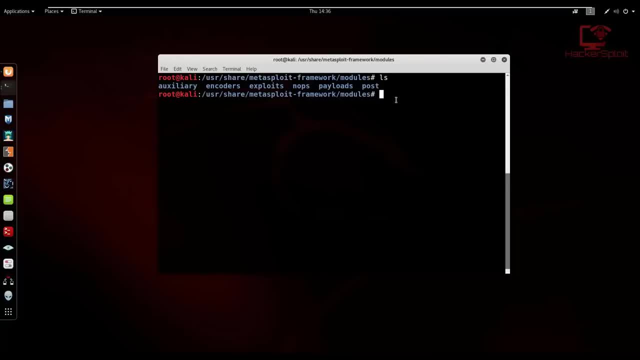 OK, All right. So again we can just browse into knobs and we can list and again sorted, simp, quite similarly to what you would have on your encoders. You have your architectures, you have your, your different languages in which you can pass it. 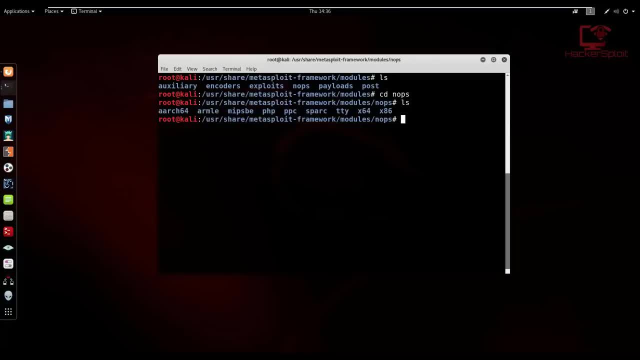 You have your again. your architectures are there, All right, So they are subdivided into multiple architectures and stuff like that. All right, Now Going back? All right, Let me just go back. So you just know that this is used to exploit the buffer overflow. 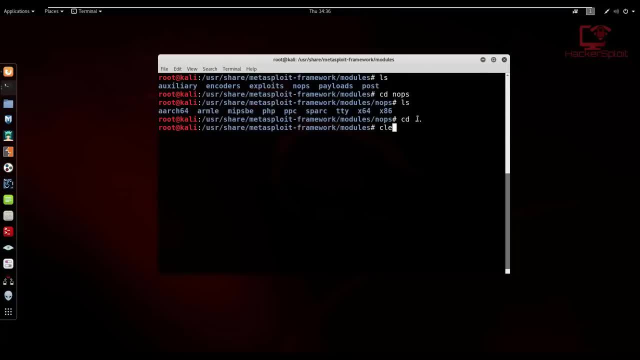 There's nothing really interesting there, but we'll be using it also because they do come in very handy when you're talking about much more complex and you very, very, very tightly secured systems. Now, again, we have looked at most, we've looked at these module categories and again they all provide you with a different way of 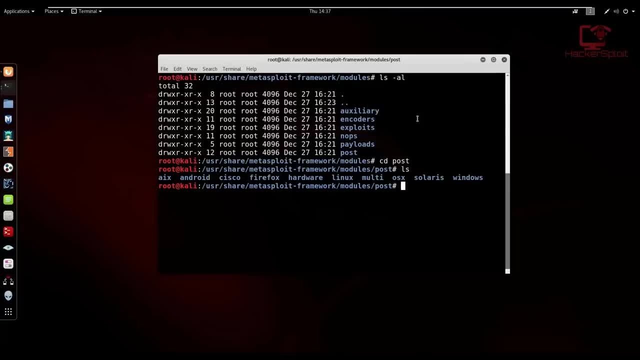 Of Getting in into a system and also you know they give you a lot of functionality, and understanding how these are subdivided- For example, the auxiliaries, the encoders, the exploits, the knobs, the payloads and the post- are very, very important for you to understand. 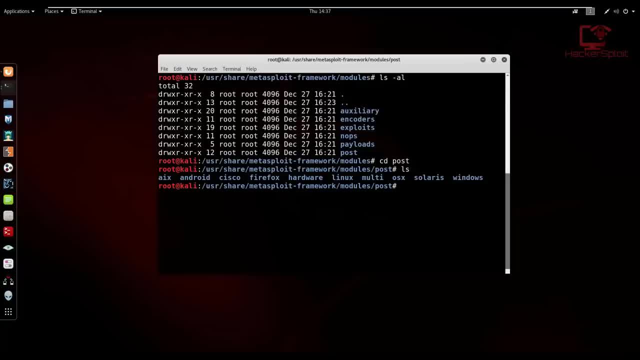 And I hope you guys have have understood what they all do. now, talking about posts, which is the last one here, Posts are simply what it means is post exploitation. I'm sure most of you knew that And these are you know they're going to be used after the, after the system has been exploited. 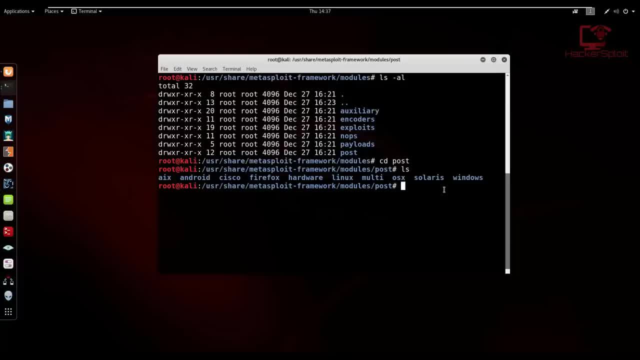 So you get it there. You know they allow you to perform extra, extra pieces of functionality, or they give you extra pieces of functionality once you've exploited the system. All right, So in in in hackers, or in penetration testing terms. it allows you to, they allow you to to perform, you know, further attacks. 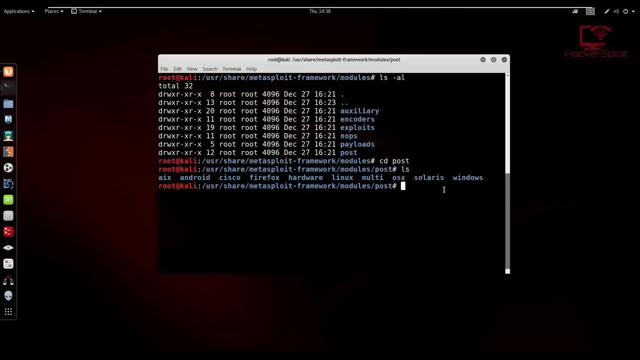 On the system after the system has been owned, All right. So these can include, as we have done previously, you know, things like key loggers, spying on the webcam or the microphone, et cetera, et cetera, And again it's subdivided into the operating systems of choice. 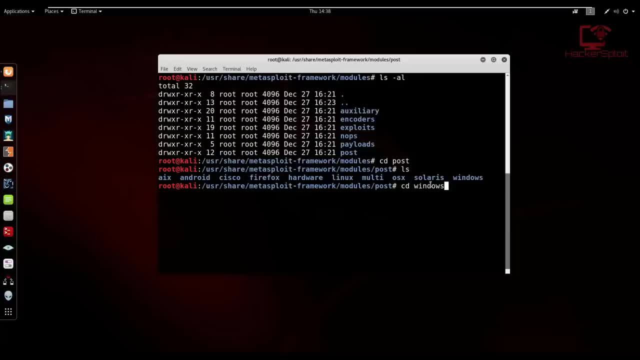 We can check out, for example, Windows, which is probably the most vulnerable operating system ever created on this planet. But that's for another day, Right, All right, Sorry about that. So, as you can see, You have your different categories and then I've told you I already knew this was going to be there. 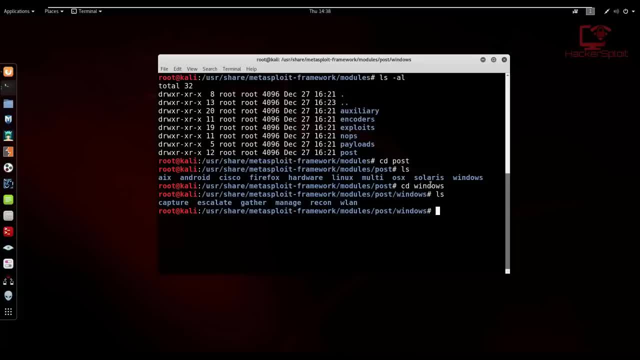 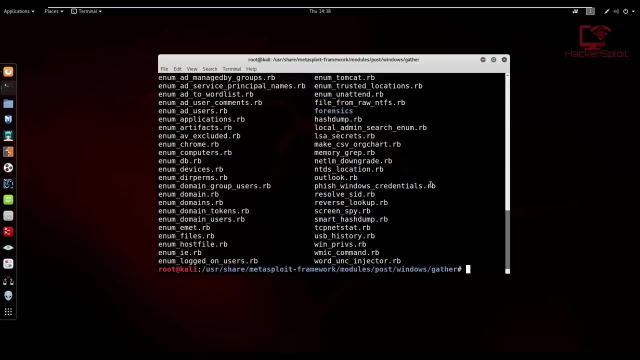 You have your captures. you have your privilege escalation. you have your gathering. you have your managed gathering being where you would find your key loggers. So if I just open that up and I list the files in there, you're going to see that there's a lot of stuff in here. 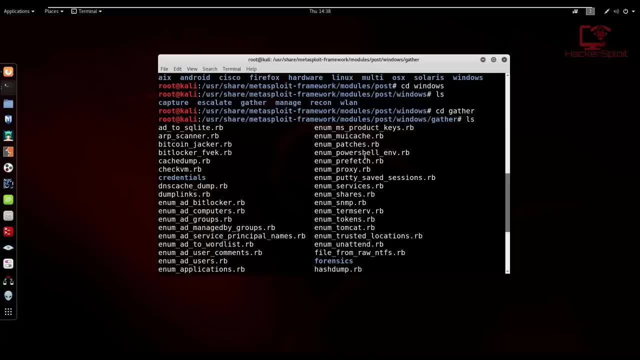 Right, And one of my favorite ones- I actually remember doing this back when I was in school- was using the one of these, these exploits right here, or these modules, If I may say so. it was to enumerate the product keys and you know, you can actually just delete the Windows activation protocol on the Windows computer and they would basically be be stuck with with Windows without any sense of activation. 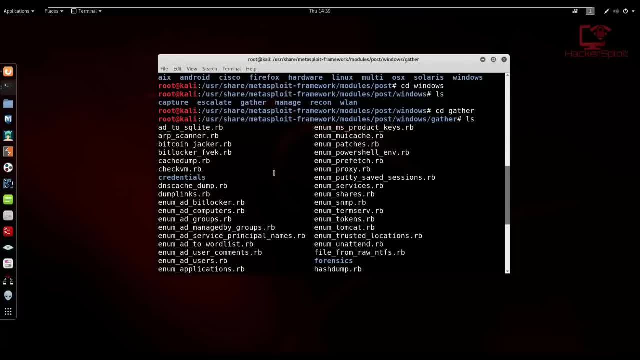 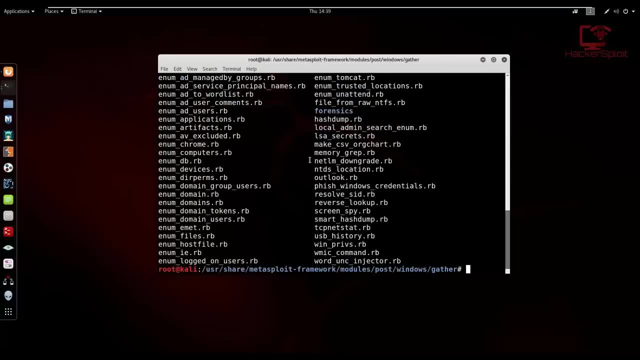 And the operating system would be really, really burnt to the ground. Some of the interesting ones, as you can see: a Bitcoin jacker- Hmm, That's pretty interesting, But I'm just going to skip over that because That's for another day. 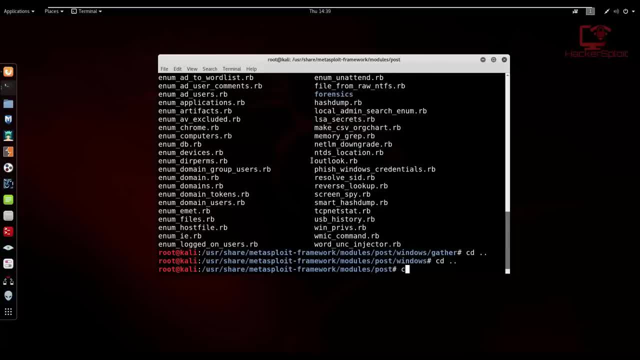 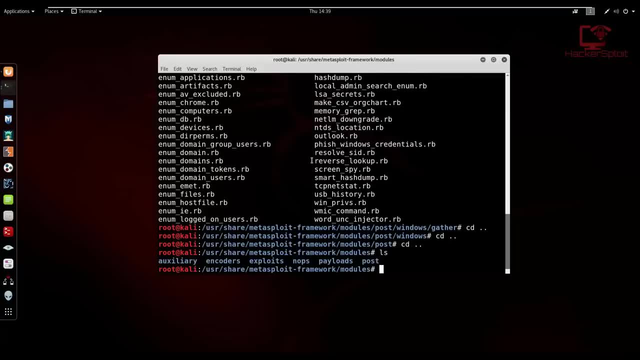 Right, All right. So, looking back at the categories that you have in here and the, the modules you have, your auxiliary encoders, exploits, knobs, payloads and posts, And I hope, in this video of understood what they all have have in, you know, in terms of Metasploit. 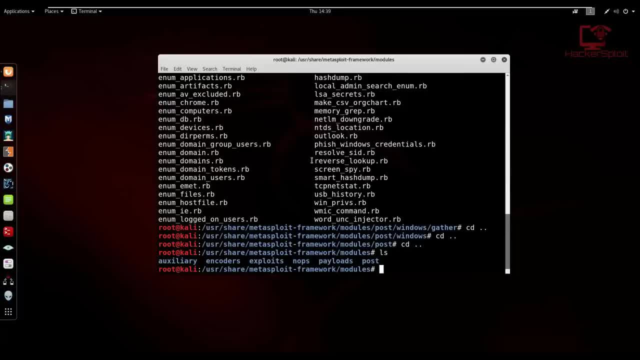 And I'm sure, once you've understood these, using Metasploit will be a complete breeze. You know there'll be no struggle at all understanding how everything works. So yeah, guys, that's going to be it for this video. I hope you found value in this video. 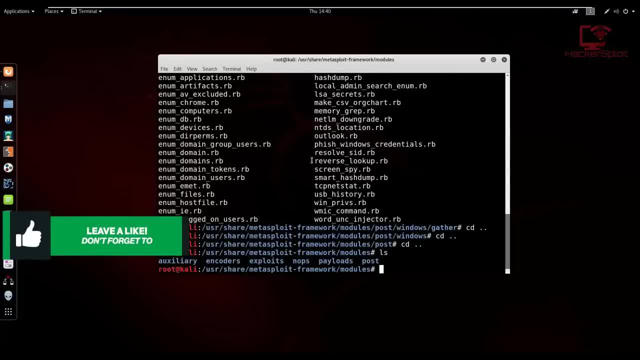 If you did, please leave a like down below and hopefully you can share it with someone who also needs these types of videos. And yeah, thank you so much for the support. If you have any questions or suggestions, let me know in the comments section down below or you can hit me up on my social networks. 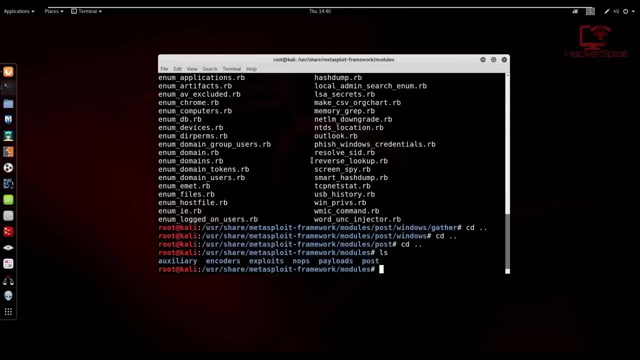 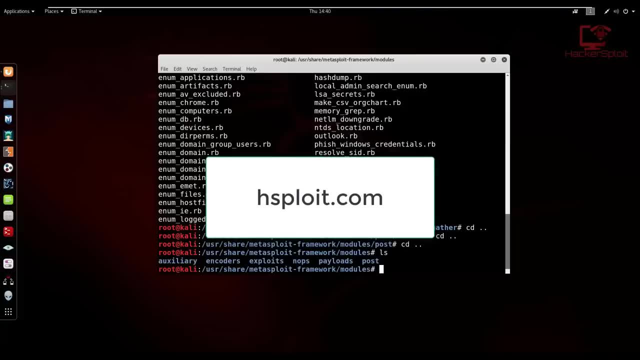 You can contact me on Kik or if you have any further questions, you can ask them on my website. There's a forum section as well, So you can also ask me there, and you can communicate with other subscribers on the channel. So there's lots of ways to communicate with me and with other subscribers. 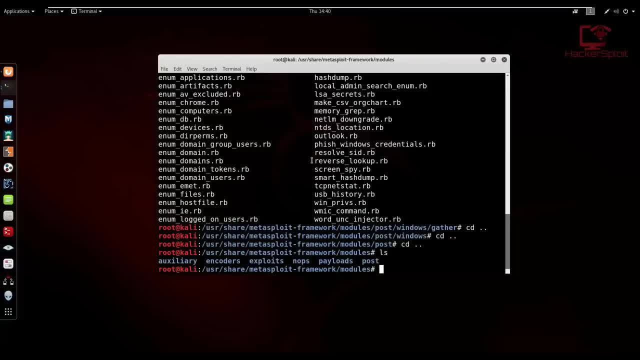 Of the channel. So again, for the latest hacking news and resources, please check out my website. The link will be in the description: Hsploitcom. And yeah, thank you so much for watching and I'll be seeing you in the next video piece. 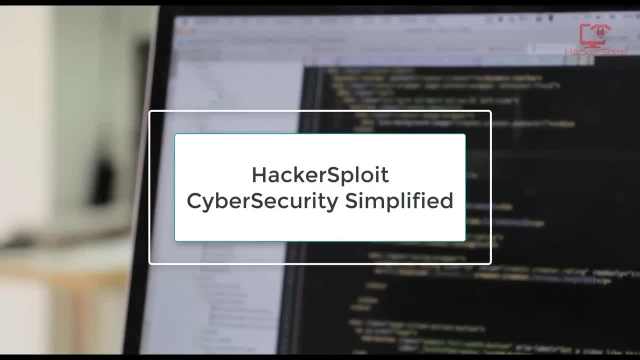 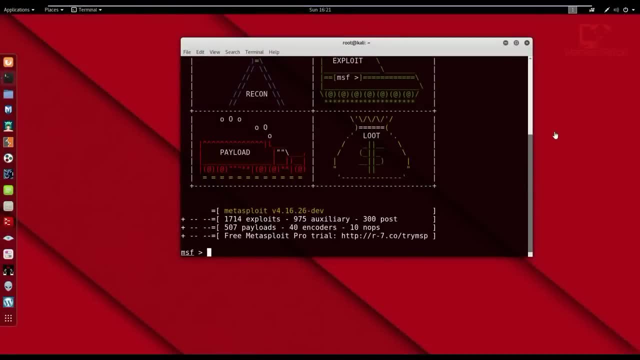 Hey guys, Hackersploit here back again with another video and welcome back to the Metasploit course Now. in this video we're going to be looking at information gathering with the Metasploit framework, more specifically, the Metasploit console. 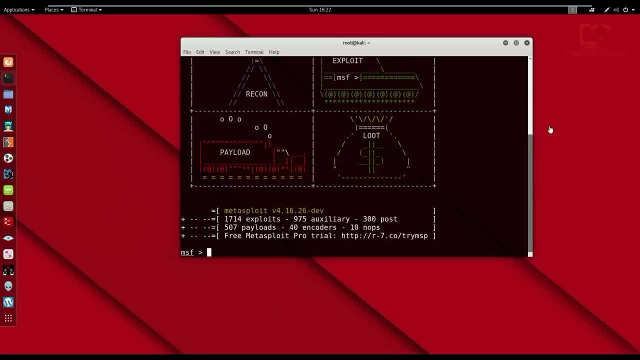 All right. So let's get started Now. just prerequisite: I have a virtual machine. I have the Metasploit 2 virtual machine running And I'm just going to show you how to do that. I'm just going to be using it as a kind of a target system for illustration purposes. 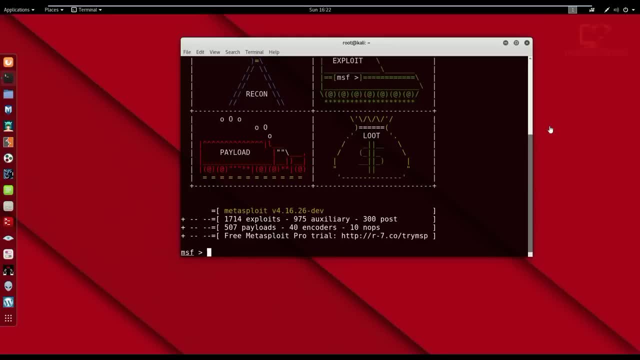 You know, I like to create a lab and that's what keeps my videos, you know, stay within the range of legality. So, again, I'm just demonstrating how this all works. All right. So information gathering more specifically, for example, we can look at using the Nmap. 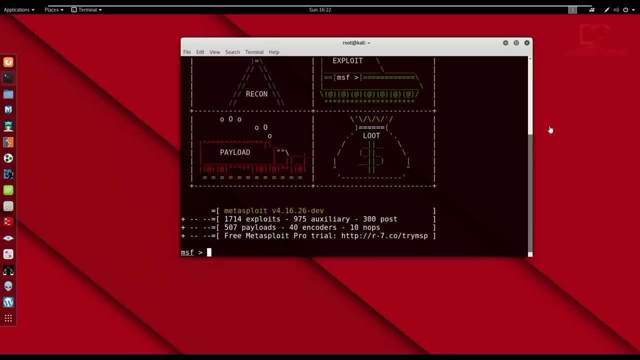 We can look at using how to use Nmap to perform port scanning. We can look at how to scan for SSH services. So we look at all of that. So you might be confused and you might be asking yourself: well, how is this even possible? 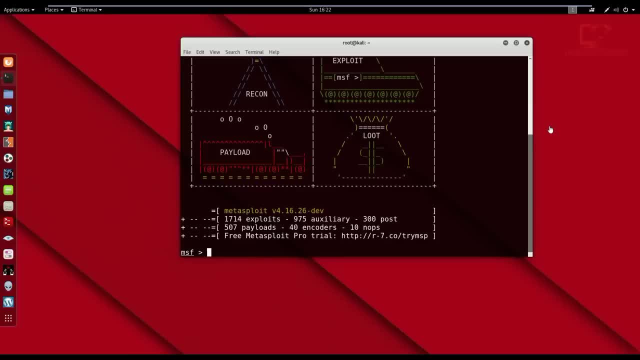 Right now again using a framework like Metasploit to perform in information gathering kinds. it tends to keep things in a more in a modular, modularized fashion. All right, Now what I mean is is, let's say, you're dealing with a target directly. 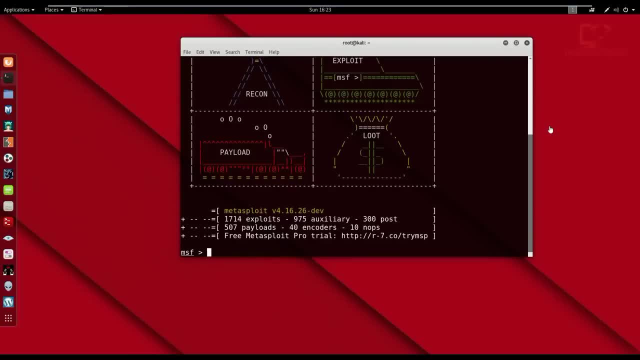 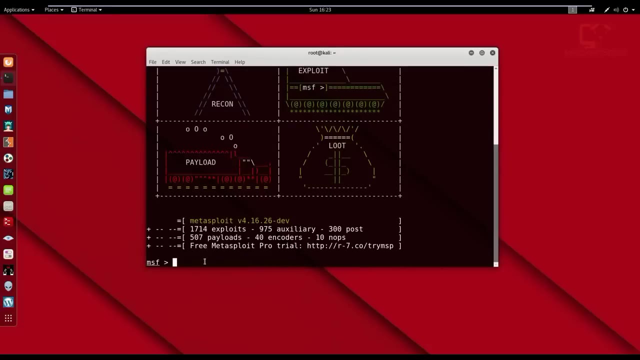 All right. So this is a fantastic way of using for frameworks like Nmap, for example, To perform sports scanning, in this case, which will, which is what we're going to do. All right, So I already have my Metasploit, the MSF console, open here, and it's really very simple. 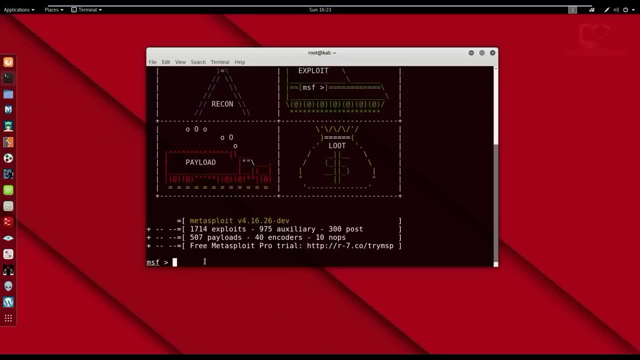 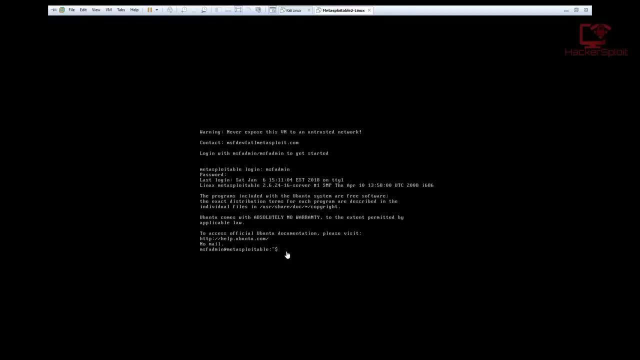 Right, Like if I wanted to perform an Nmap scan. let's say we had, we already have a target Right, And again I'm going to use the Metasploit to IP address here, So let me just get that up again. 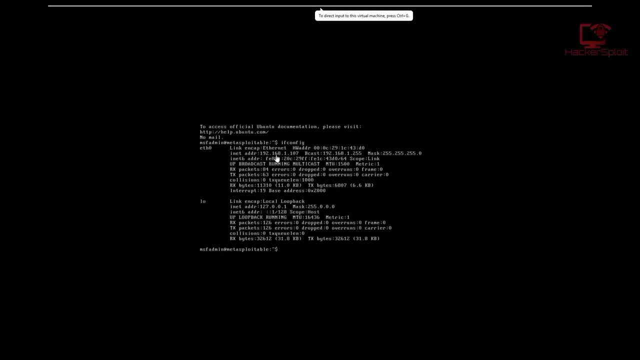 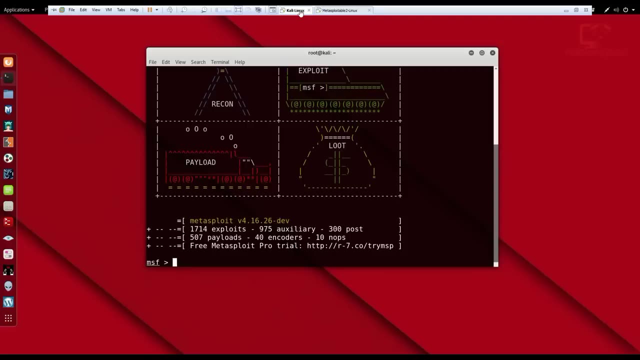 It is bridged to my adapters. So there we are, 192.168.1.. Point one, seven. OK, so that is going to be the bridged: its bridge to my, its bridge to my network. That means they're all going to be on the same network. 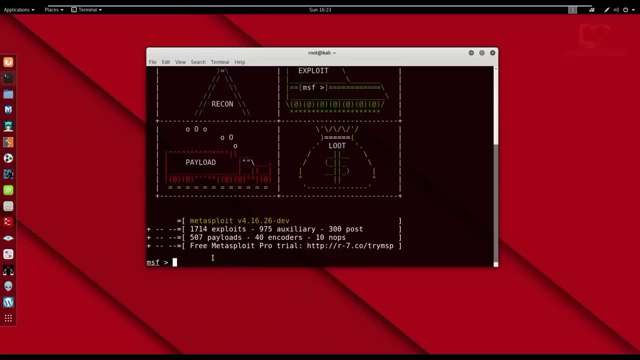 All right. So for those of you having trouble with that, that's how to fix that issue- where you can detect it on the same network. All right, So I could perform a simple port scan on Nmap. So I would say Nmap, just as you would. 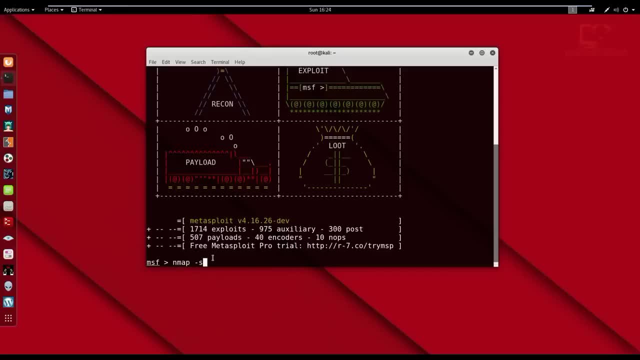 All right, Nmap. And then I would use the commands S and capital T. What these commands do? I'm pretty sure you already know them. It it initiates the three way handshake and will essentially just detect the open ports on the target machine. 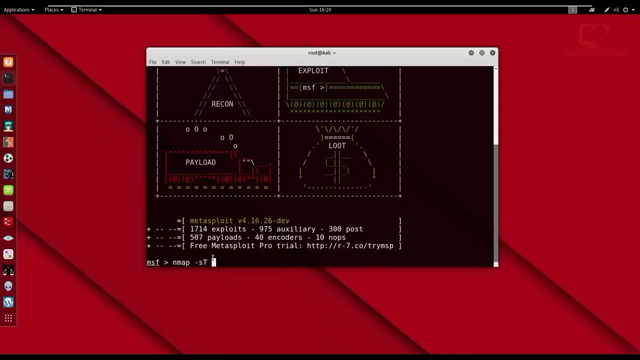 Now, the target machine being Metasploitable2, it'll have a lot of open ports, All right. So 192.168.1.107.. OK, And we're going to start that, and it'll just open up the Nmap framework. 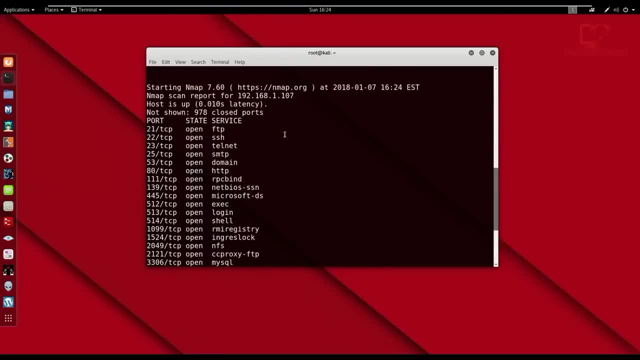 And there we are. Those are the results, So you can see all the ports that open, Probably all of them. We have your FTP, SSH, Telnet, you have your, you know your login, your MySQL, et cetera, et cetera. 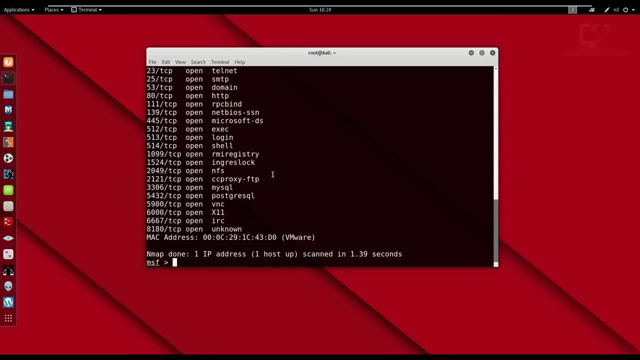 Right now. that's pretty cool. you know that we can actually use the Nmap, the Nmap framework, in information gathering, Right. So I'm pretty sure you guys already know how to how to use Nmap. But I'm going to show you one more command, because a lot of people ask me this. 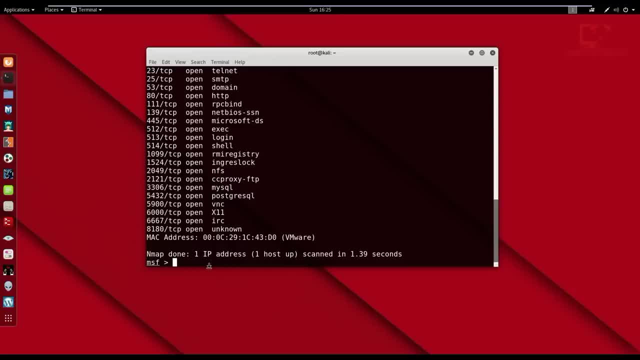 And this is when a site has probably a firewall and you want to perform a stealth Can. All right, So a stealth scan essentially allows you. what it'll do is really, it will give you a connection between the target and the scanner. All right, So it will give you, you know, the ability to to perform it in a more promiscuous manner, while still maintaining maintaining. 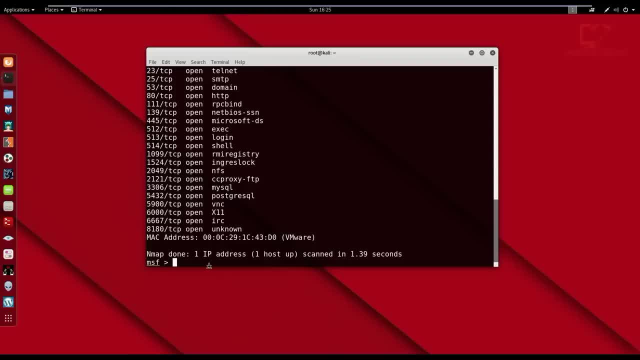 I don't know how to explain this. It'll not do it in a in more of a direct way, So probably the target will not recognize it so much As a scan. All right, So in order to do this, we're going to obviously use the Nmap and it's we use the commands, the SS. 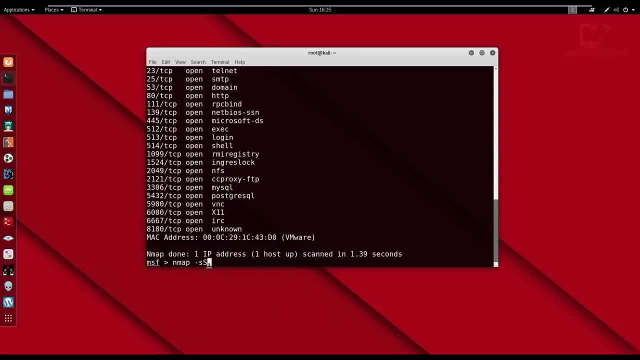 All right. So a small S and a large S. I'm pretty sure you're familiar with the syntax, You know what this means And again we'll just target the system- And again exploitable- to not being, you know, very, very secured. 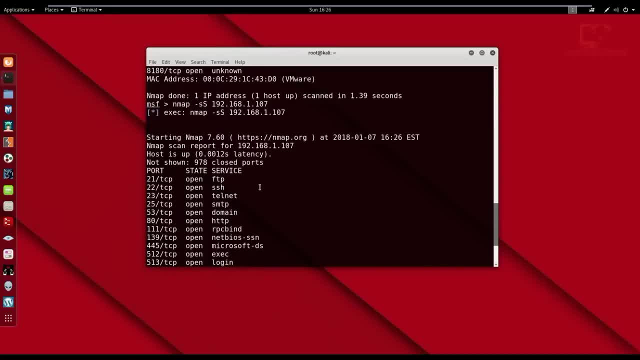 It should return us There. we are Really really quickly. All right, So that's, if you want to perform a stealth scan, All right. So that's very, very interesting. Now, looking at the other type of information gathering that we can, you know, carry out, we can actually use auxiliaries. 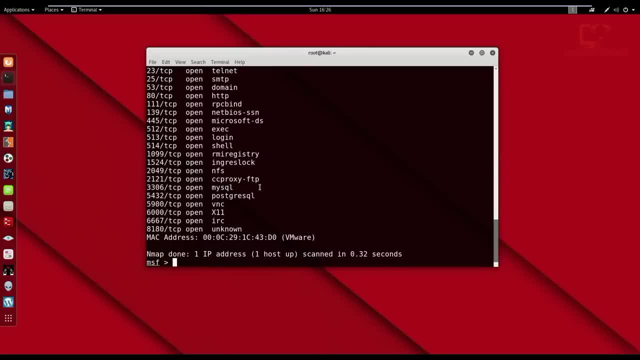 We can use the auxiliary modules or the scanner modules that come with Metasploit. All right. So you might be asking yourself: well, you know what. what do you mean exactly? Well, what I mean is: we can actually use the inbuilt modules that come with Metasploit or, you know, in the form of auxiliaries, where you have your scanners. 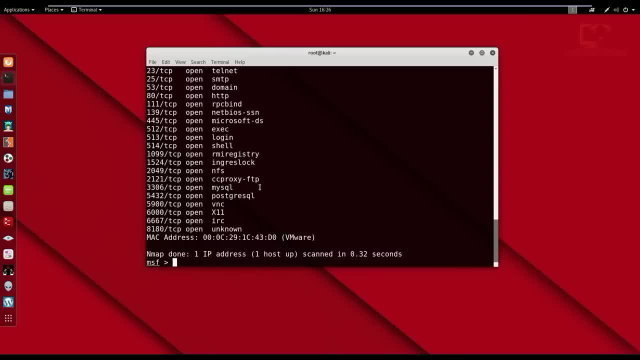 As I explained The previous video, they allow you to use the inbuilt scanners, which are considered to be information gathering tools. Now, probably not a lot of you guys have actually used this, and that's fine. You know, it's really really very simple to do. 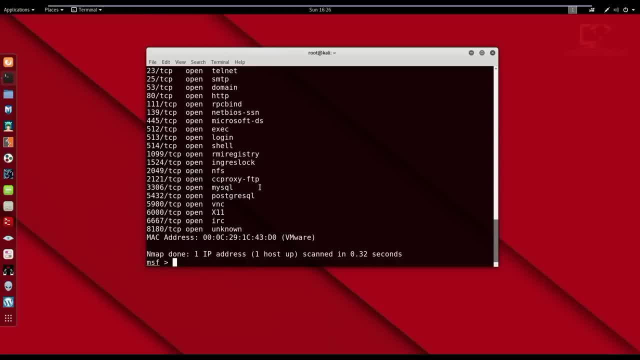 And that's what we're going to do now. All right, So what we're going to do is- I'm going to demonstrate this. Let me just clear the console. I'm going to demonstrate this very, very simply using the SSH scanner. 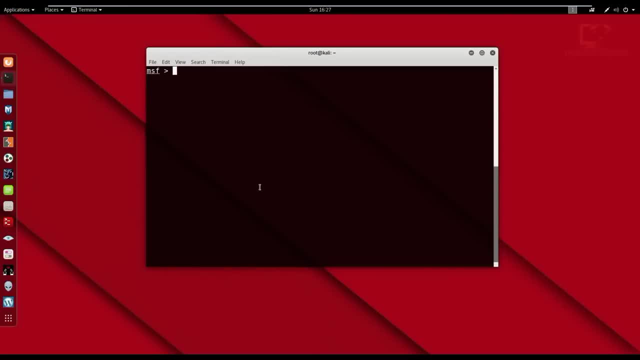 All right. So this is an inbuilt scanner that comes with Metasploit. I'm pretty sure probably most of you have gone through it. It's a very- it's not, you know- very, very early on using the Metasploit, the Metasploit framework. 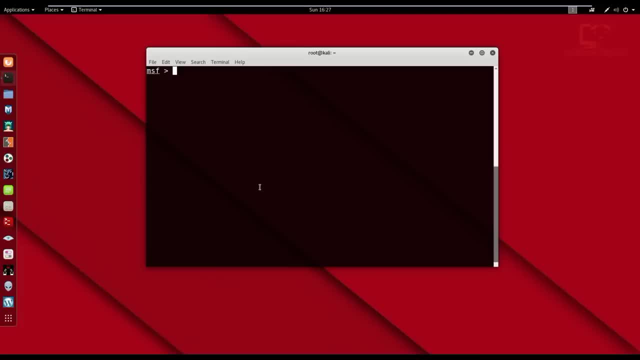 All right. So essentially what it'll do, it'll allow you to detect the SSH versions that are running on a target. OK, so if you don't know what SSH means, it's SSH is secure shell, All right. It is essentially uses users cryptography and authentication, you know, to connect between 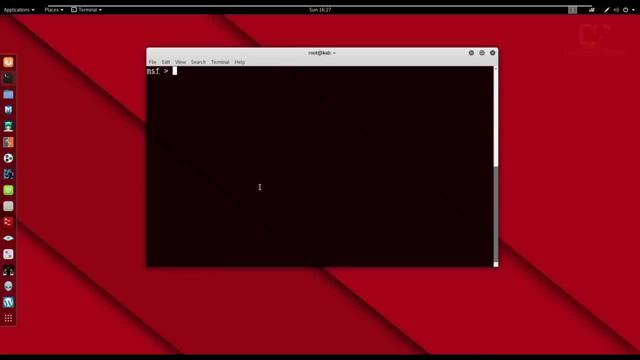 Two computers as a connection between two computers. Right, So let's get started Now. we're going to be using the auxiliary called SSH version, All right, So I'll show you how to do this in a few seconds. So what we're going to do is we're going to utilize the search command. 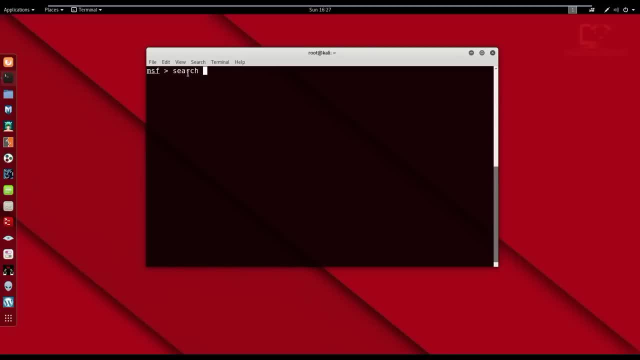 The search command allows us to search for modules. In this case, we're using the auxiliary and, furthermore, the scanner. All right, So what we're going to do is we're going to say search SSH version. All right, Search SSH version. 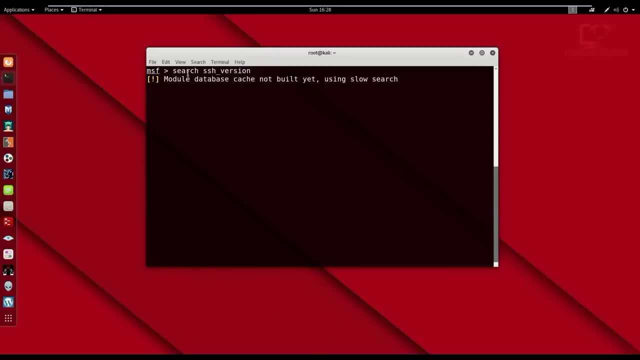 And again, you can start up the database, if you want to, or the PostgreSQL database if you want to, Or if not. you can just, you know, you can just let it perform the normal search, which is again it is, it's a slow search. 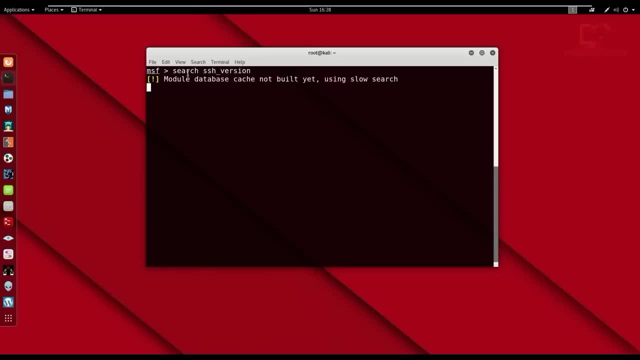 But nonetheless it'll return the results that we want. All right, So just give it a few seconds. It shouldn't take too much time at all. Again, you'd be much better off if you started up the database and you had it properly configured. 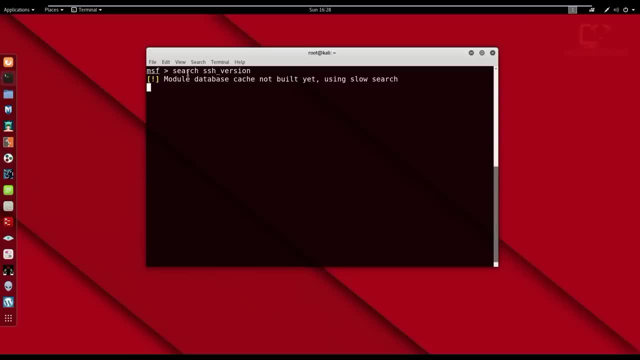 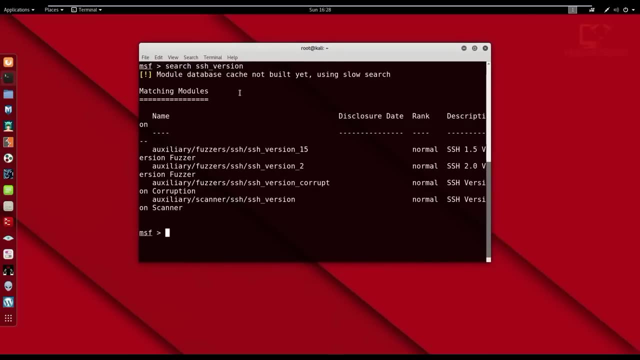 All right, But I didn't, So I'm sorry about that. Again, it shouldn't take too much time. In fact, it's probably taking quite a while now, But the search results are pretty much standardized. There we are, So we have the search results. 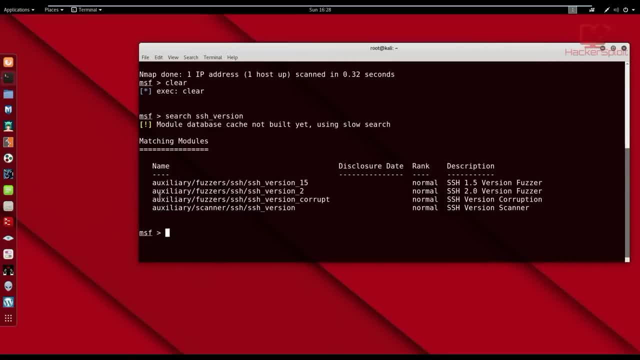 Now, what we're going to be using is the auxiliary scanner, because we don't want fuzzers- We already discussed what those ones were. We want these auxiliary scanner, All right. So I hope you guys remember the, the syntax. So we're going to say so: this is the one we're going to be using. 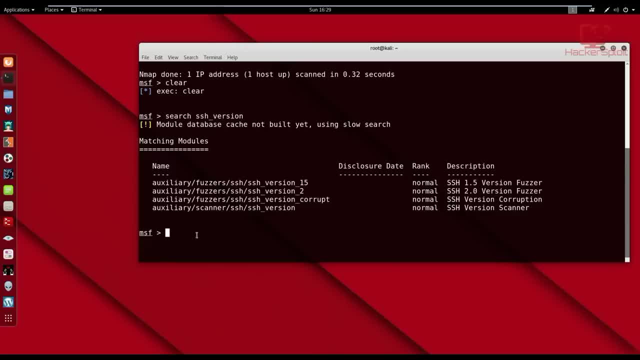 The auxiliary scanner SSH version. So what we're going to do is we're going to use the, we're going to use the use, We're going to use the use command to select that one. All right, So to use auxiliary- auxiliary. oops, I should have actually just copied it. 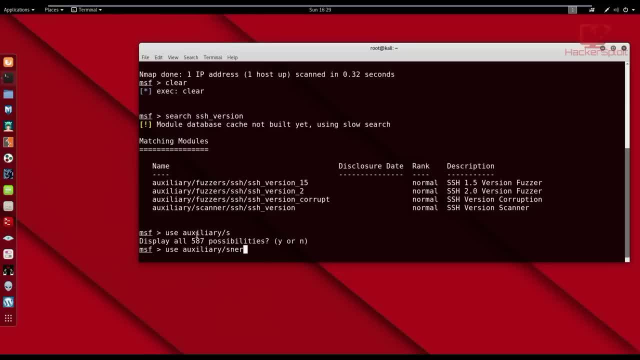 And oops, oh my, Sorry about that, guys, Let me just copy it So just to keep things really really simple, Because even if it was a scanner, it shouldn't. it should have actually detected that itself. So let me just paste that in there again. 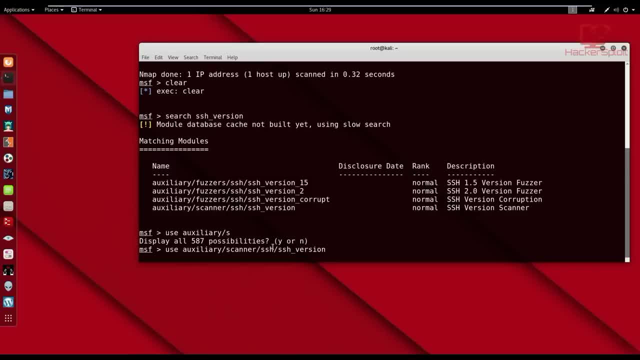 A lot of people ask why I do that with the mouse pointer, And that's just to reinforce the idea of me actually copying and pasting something, Because if I did it with my keyboard strokes some people would ask me what I did. And there's really not. it's not important that we go through that. 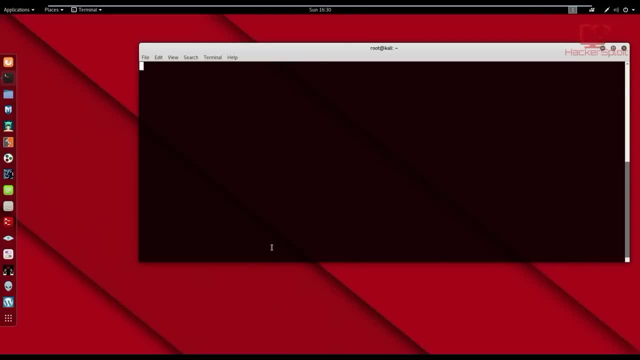 So I'm going to hit enter And there we are. So let me just clear that out. And it's using the scanner SSH, SSH version. So essentially it's just getting information about. it's getting information about the target in terms of what SSH version it's running on the SSH port. 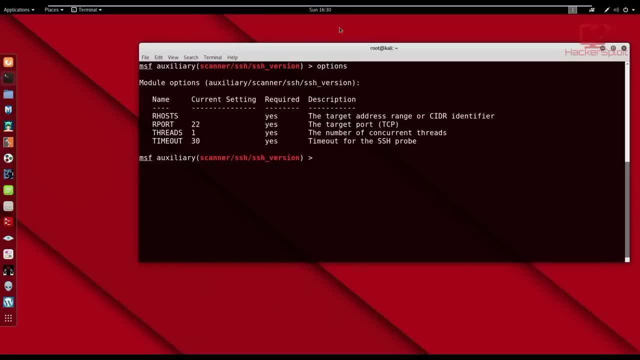 All right, so we can look at the options that we have here And, as you can see, the port is set to 22,, which is the default TCP port. you have the threads, which is what we'll be looking at, and the timeout. 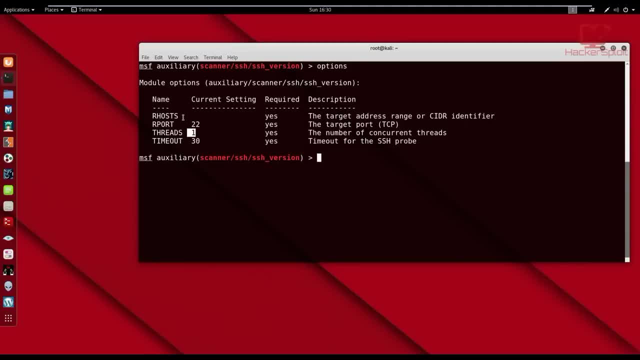 So usually the timeout is pretty much okay, but we need to change the threads and the our host. All right, The our host is the target address And it's also a range, so we can actually use a range. Okay, but in this case we're not going to use a range because, again, I only have the. 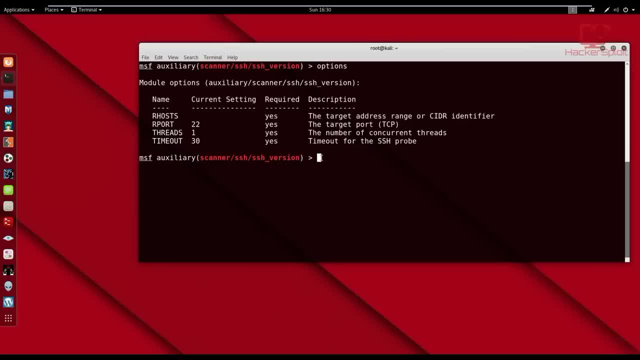 about three computers running on my network right now. So you know it's probably going to get only like one of them, because my SSH ports are all closed on the other computers. So let's set the R hosts like so And I'm just going to use the Metasploitable2 target machine .107.. 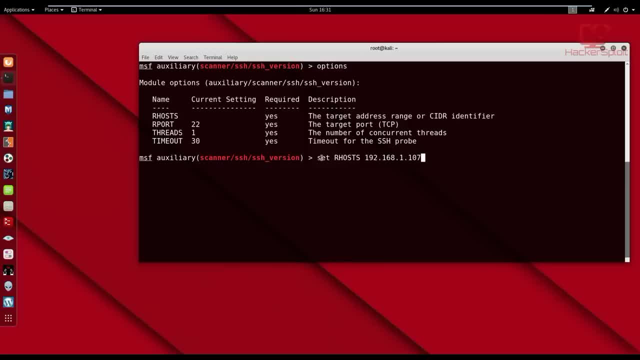 Right, And once that's done, we want to set the threads. So let's go to my network. So I'm going to get my network And I'm going to call my network to something quite high, like, something like a hundred. yeah, that sounds about right there we. 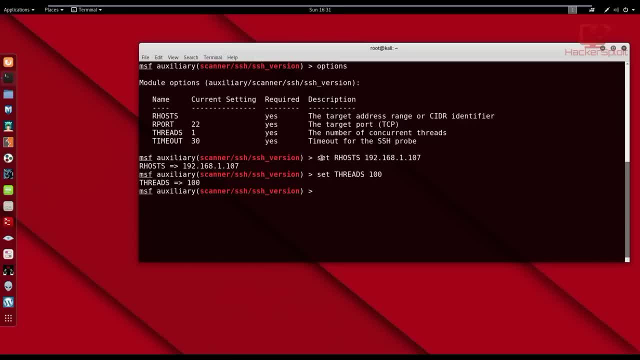 are. and finally, once we're ready, all we have to do is hit run, not exploit, because we're not exploiting anything. that's also a mistake that many, many people make is they actually go directly, for, you know, for the exploit command. so just hit run and there we are, immediately it's going to. 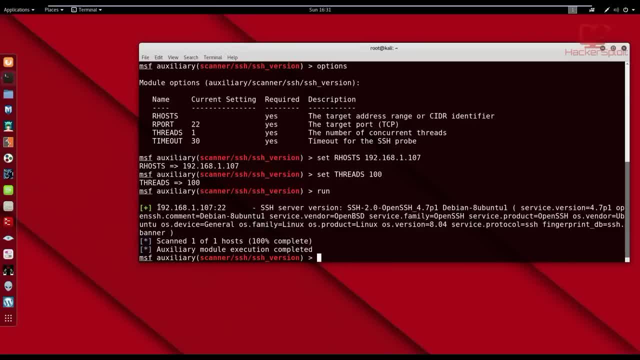 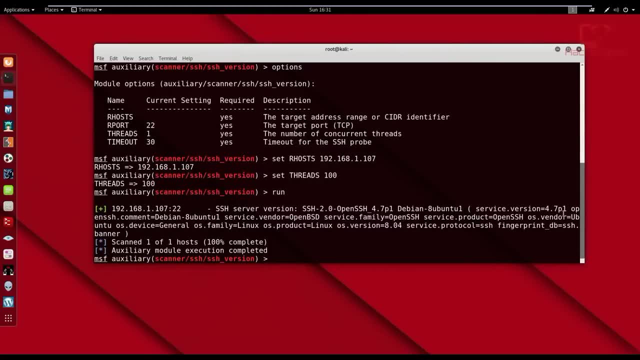 return the results. so on that on the meta exploitable to machine, we have the SSH version running, SSH version 2.0, open SSH. it's running Ubuntu and the version number is written there and again this is can be valuable information. you know you could find exploits related to the. 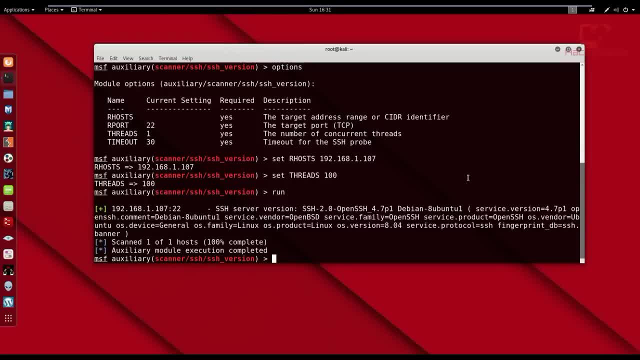 version of SSH running and that's for the exploitation stage which will be getting to. but it's important to know how to use the meta exploit, how to use the meta split framework in any way, whether it's the meta exploit console or you're using the other frameworks, the GUI frameworks. 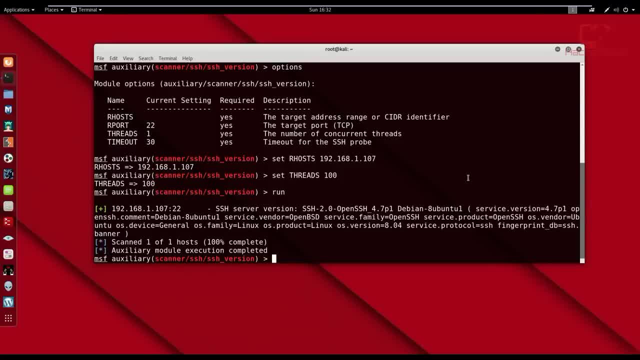 right. so there's a lot of other things that you can do with in terms of information gathering. you can also use, you can also search for the FTP version and you can look at other things like sweeping and banner grabbing. but really that I'm sure if you've done it before, you know, you know. 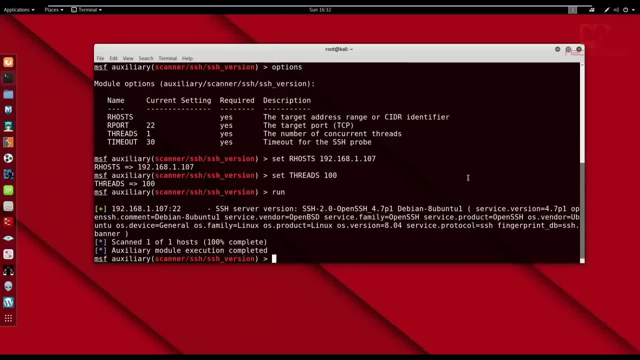 with hacking, you learn information gathering first and you learn about all the frameworks for gathering information. so I just wanted to show you how to utilize the auxiliary module where you can use scanners- or fuzzes, for that matter- to gather information about your target. it's really really very interesting. so 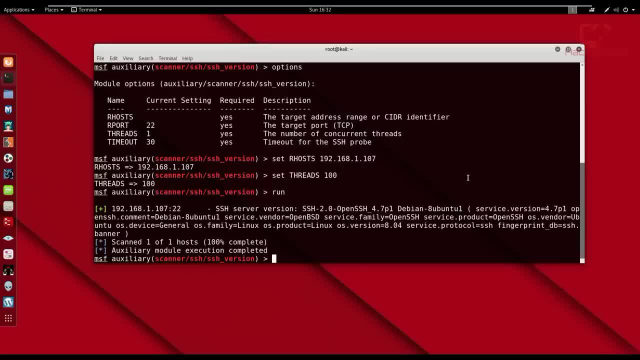 that's gonna be it for this video. I told I give you a bit of an introduction and you know, just move you around how to use all of these in a modularized way to perform individual tasks, right? so I hope you guys found value in this video. if you did, please leave a like down below if you have. 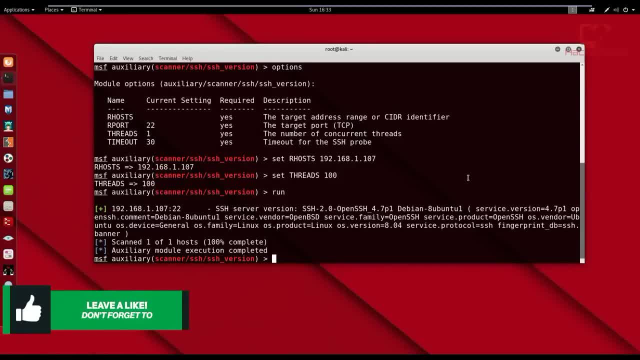 any questions or suggestions, please do let me know in the comments below and I'll see you in the next video. suggestions: just let me know in the comment section or you can hit me up on my social networks and you know, for the latest version, for the documented version of this, of this video, you can check out my website. hey, Jess ploy. 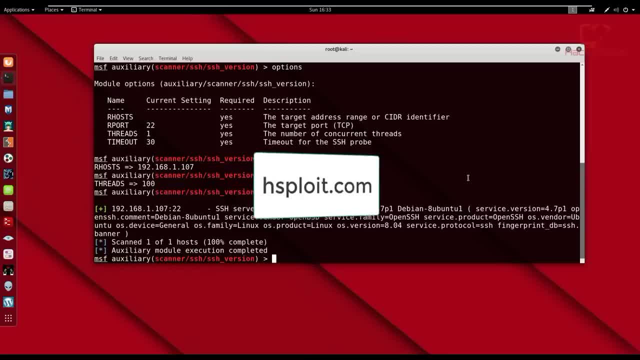 comm is the latest hacking news there and you can also get tutorials. you know, different PDFs, guides just guiding you on your way as you learn hacking. and yeah, thank you so much, guys, for watching this video. thank you so much for the support. I appreciate it and in the next video we'll be looking at how to. 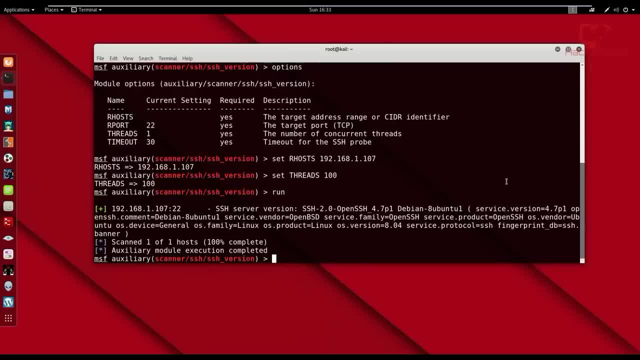 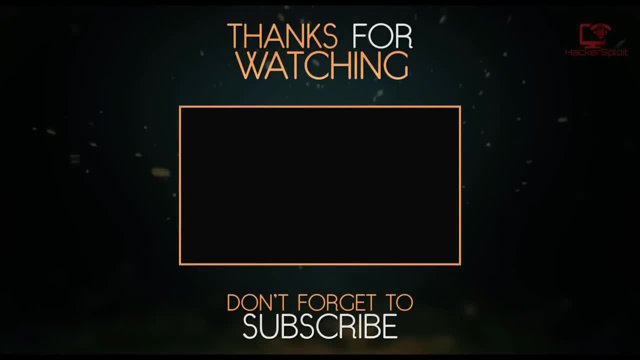 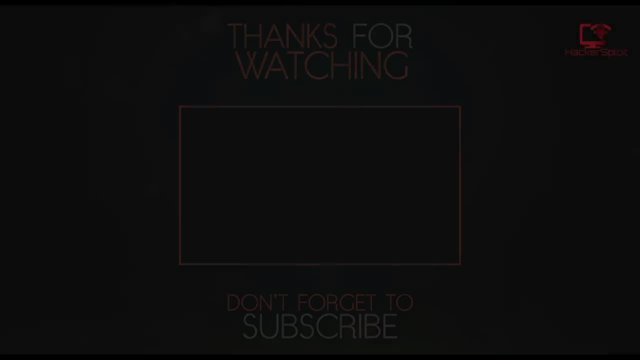 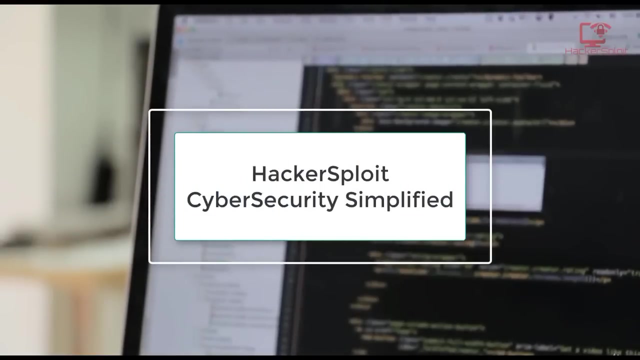 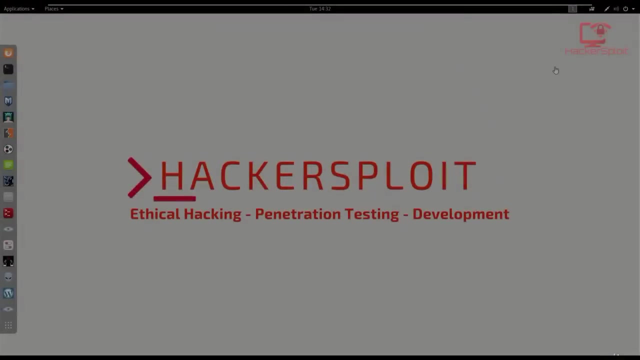 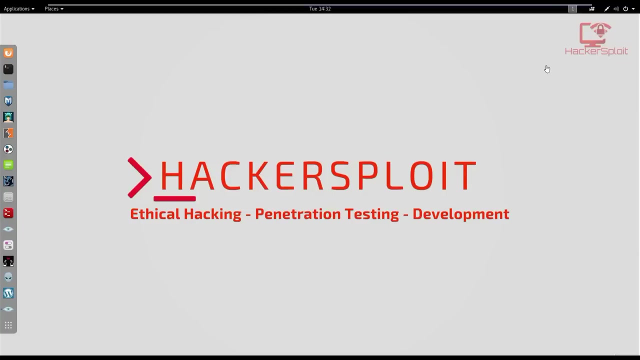 nieces alright. so thanks so much for watching and I'll be seeing you in the next video. peace, hey guys. Hackersploit here back again with another video, and thank you so much, guys, for all the support. just want to throw that out immediately. I will finally hit 30,000 subscribers, that is. 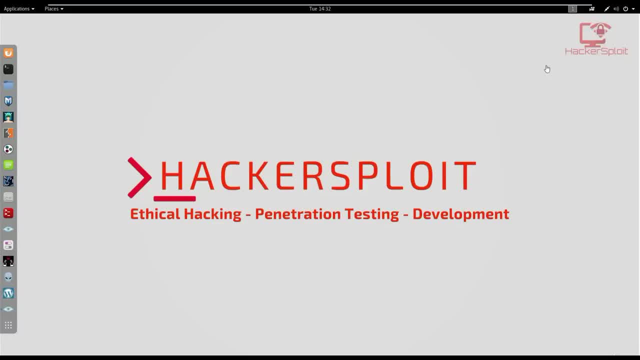 incredible and you know I just can't thank you guys enough, and I promise to make even more informative and obviously more videos on the channel. all right, that being said, let's get started with today's video. so in today's video, we're gonna be continuing with our Metasploit. 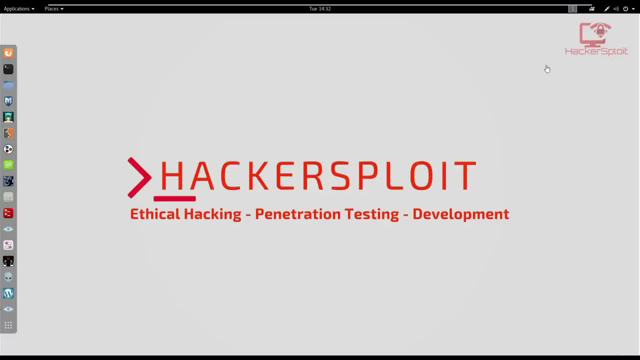 video, and I promise to make even more informative and obviously more videos on the channel. alright, that being said, let's get started with today's video. so in today's video we're gonna be continuing with our Metasploit, and today we'll be looking at some basic exploitation. alright, so again. 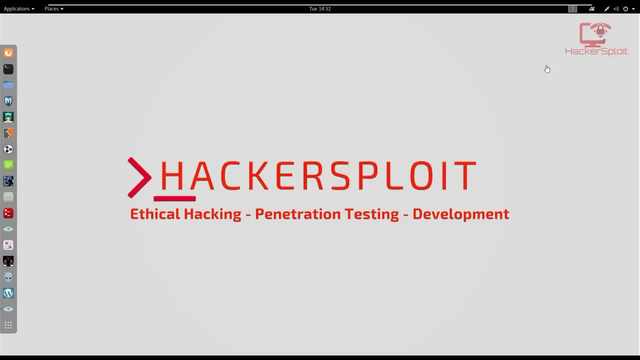 following up from the information gathering section, where we learned how to gather information, we're still going to be touching up on information gathering using, you know, web vulnerability scanners or like, for example, open vs, and we'll be looking at all of that right, but for now, let's 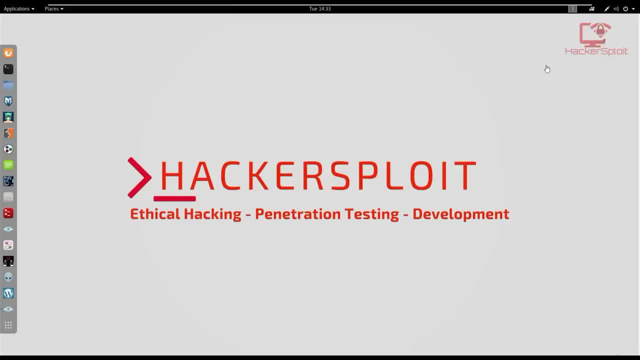 focus on some basic exploitation now before we start, I just want to let you guys know that I'm using Metasploitable 2 and I would recommend that you use it as well, all right now. reason being is because it goes hand-in-hand with Metasploit and it's a fantastic way of learning or practicing your 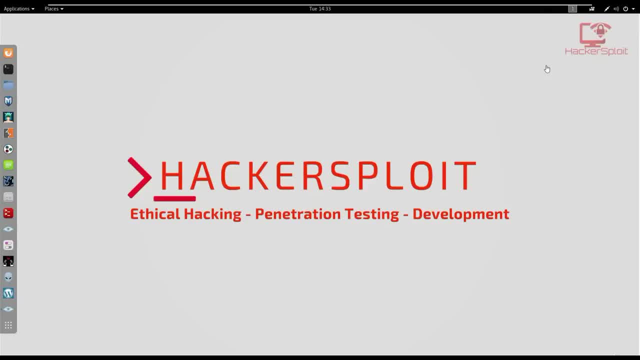 exploitation. you know you can, you can configure it to match your, your, your skills and you can increase the security, etc. etc. by the way, we'll also be looking at the web applications that come with Metasploitable 2, for example, the damn vulnerable web application Matilda day, etc. etc. but 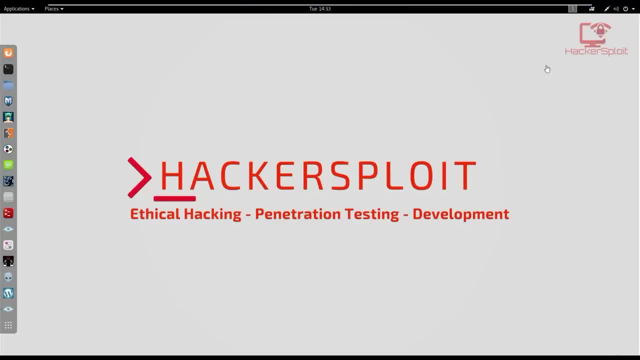 but for today let's look at some basic exploitation. alright, so I already have Metasploitable 2 running as a virtual machine and I already know the IP address. so what I'm going to do is I'm just gonna perform an nmap scan with. 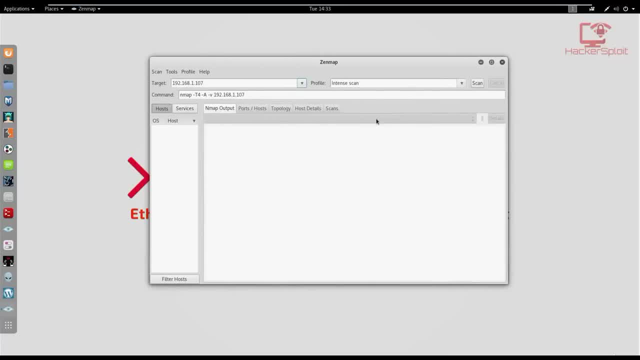 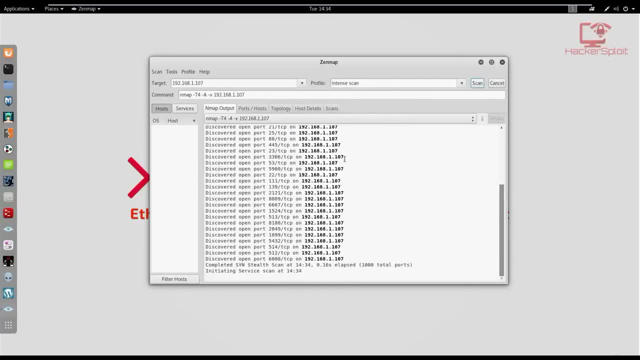 ZenMap here, so we have a visual representation of what's going on. okay, so I'm just gonna perform a scan and while it's scanning, as you can see, it's already discovered the open ports. so we know that's good. so let me just open up. 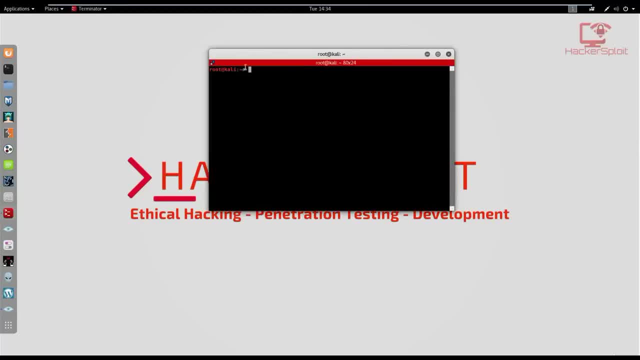 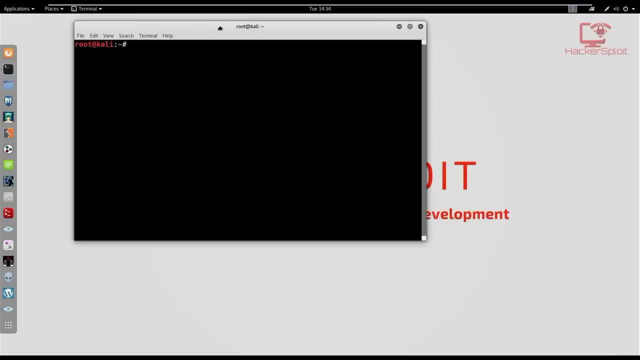 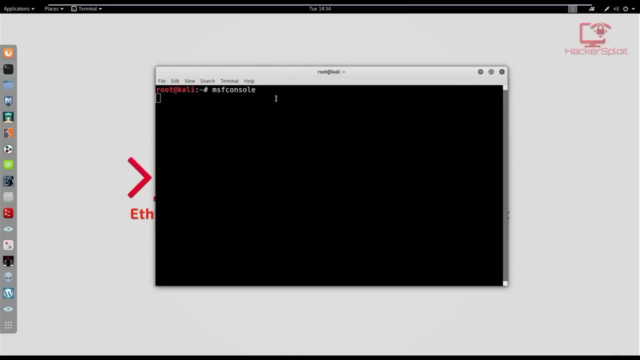 my terminal here and we can start up the Metasploit console. but let me just use the normal terminal here, so we have a good idea or we can see what's going on in the terminal. so I'm gonna start off the MSF console, alright, or the Metasploit console as it. 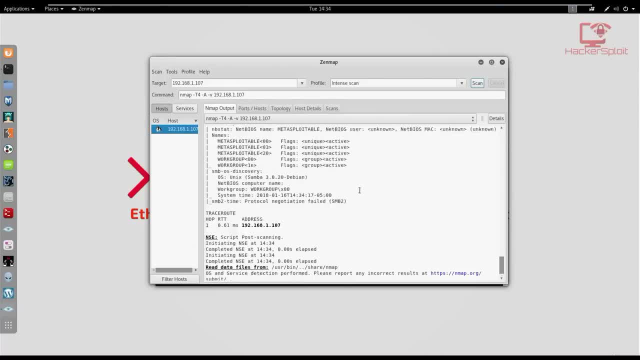 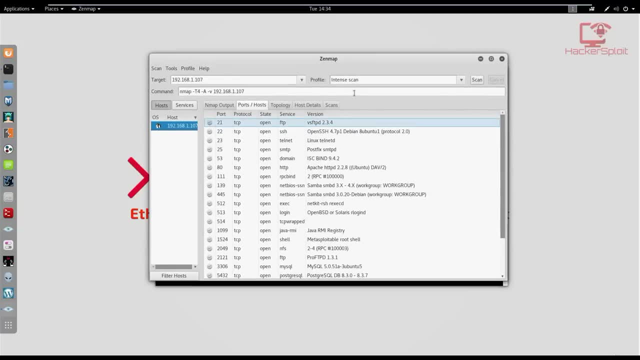 is. so, while they're starting, let's check what information nmap, or in this case, ZenMap, has gathered. alright, so we've got the ports, and today we're going to be exploiting the first one. all right, the first service, which is the FTP port. so it's running vs FTP vs FTP D, all right. so 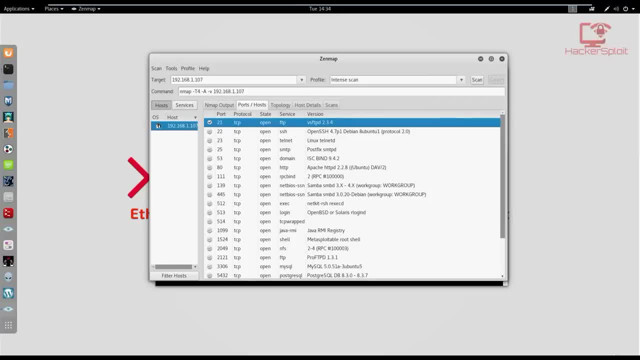 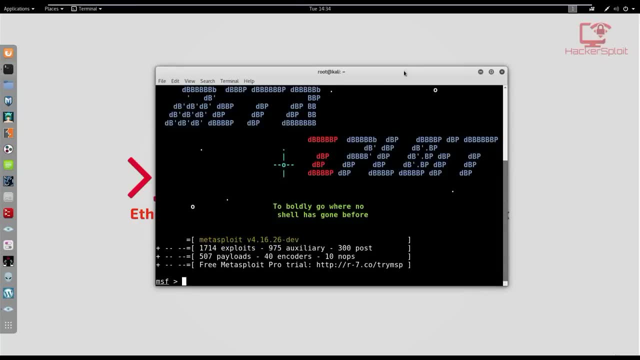 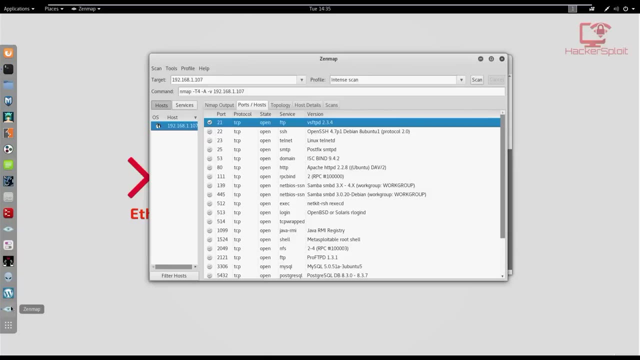 that's very important that we understand that it's running that service, because that's what we're going to be exploiting today. okay, so let's check if met, the Metasploit console, has started up there. we are fantastic, all right. so what do we need to do first? all right. so, as I said, the first thing that we need to know is: 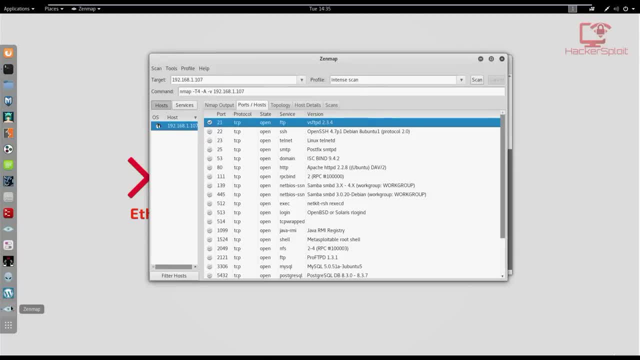 what service are we trying to? are we trying to attack? in this case, we are trying to attack the port 21, the FTP port, and the software version or the service version is vs FTP D, 2.3 point for now. this is a very old software, or a. 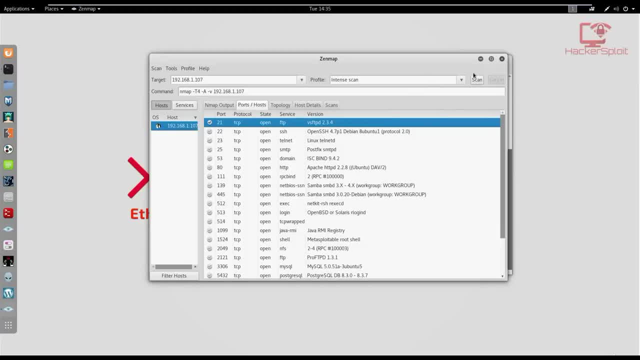 service version that is running and it is extremely vulnerable. and, again, because it is Metasploit abal, we know that this is designed to be vulnerable. so, whoops, let me just go back here. so let's actually use some of the exploits that come with Metasploit abal. 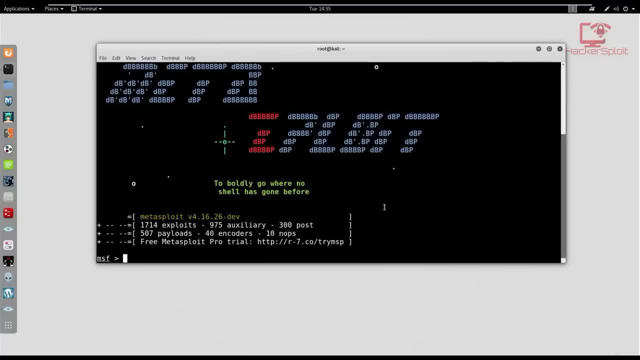 right, so let me just expand my console there, and what we need to do now is, if you remember, with the basic commands that we went through, is we're going to be using an exploit, all right. so again, obviously from the title of the video you already guessed that, that we're going to be using an exploit. so from 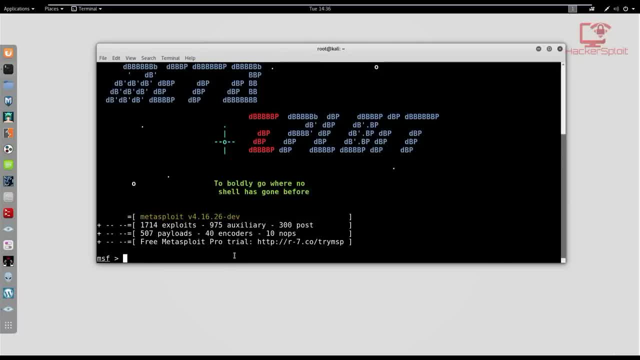 this stage onwards. I'm guessing that you're familiar with the syntax that we're going to be using, so the first thing we need to do is we need to search. we need to search for an exploit, all right. so it's really very simple. all we do is hit search. 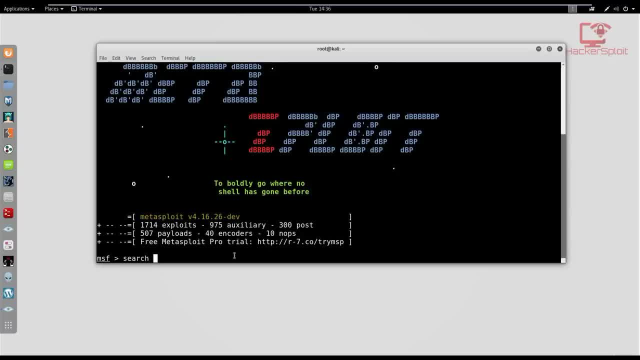 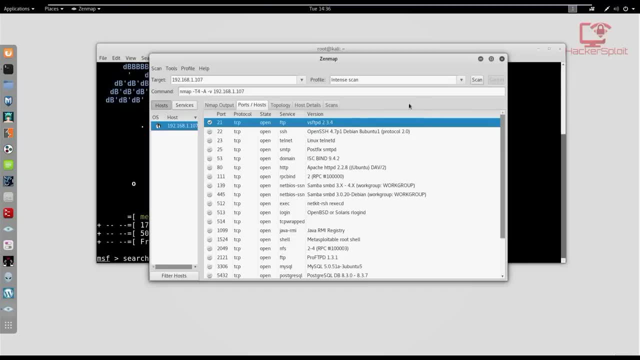 and now we go with the information that we have. all right, let's say we did not know at all what we're doing here. what we would do is would go from the version that we have, which is vs FTP D, all right, so we would search for vulnerabilities. 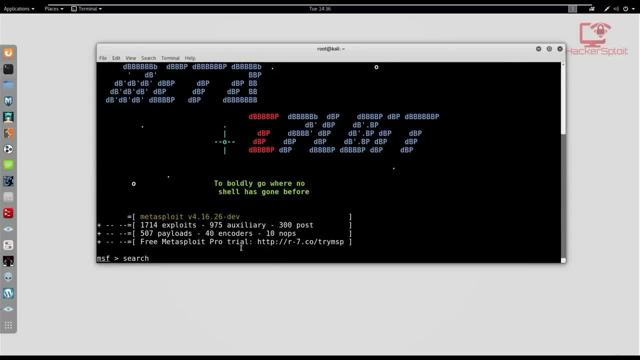 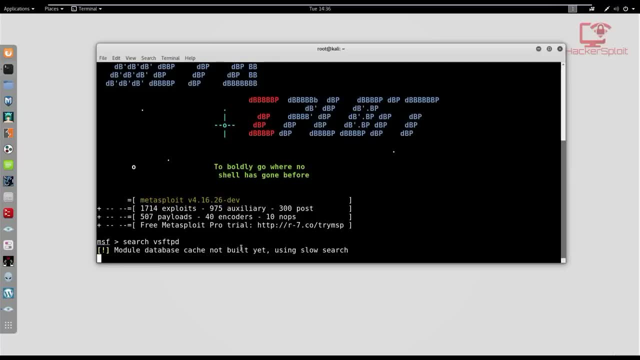 that involve the vs FTP D service. all right, so service. so search vs FTP D. right, and I'm just gonna search now. again, I've not started the database or built the database, so it's gonna take a few seconds. no need to worry there and just let it go on and it's gonna. it's gonna respond or it's gonna display or 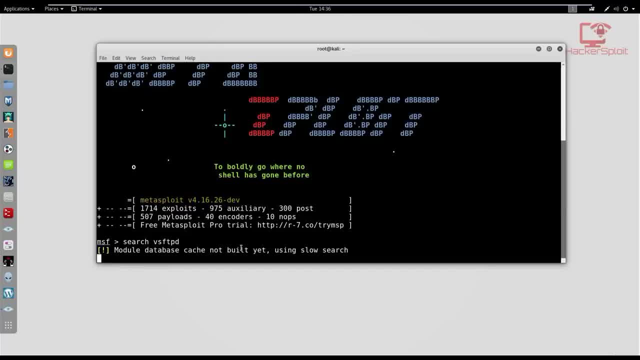 it's gonna output some results for exploits that we can use, depending on the service. okay, so just give it a few seconds and let's see what we get, what exploits we can actually use to exploit the meta exploitable to vulnerabilities on the FTP port. all right now, going back to the ports here, as you can see, we can. 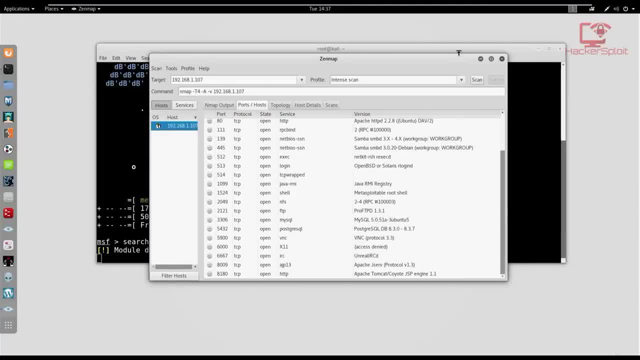 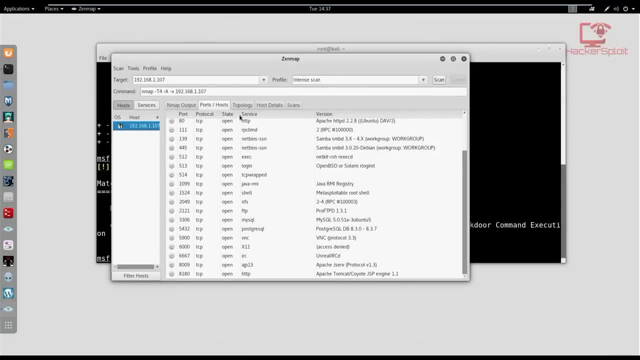 see that the state of the port is opens, which is pretty obvious. that's a great. that's how we'll be able to get the attack. But when we'll be moving on to more advanced states, when you know when we have port, states can be open or filtered, we'll be looking at how to. 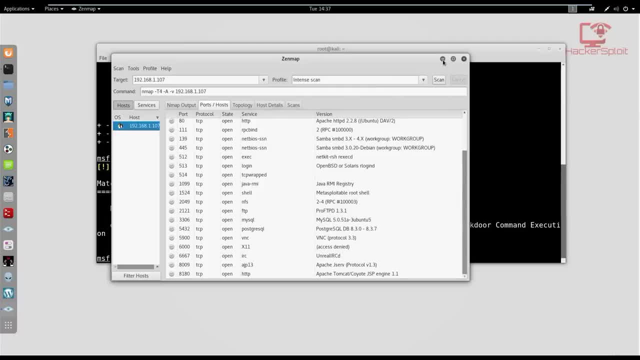 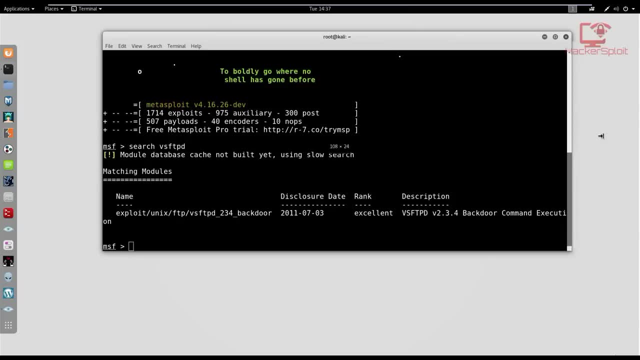 determine whether or not we can perform an attack on it. Alright, so it looks like we've responded. there we are. that's the exploit that we are going to be using. Alright, so let me just enlarge that so you can see: Alright, so matching modules. alright, so it's found one. Now it's going to ask: 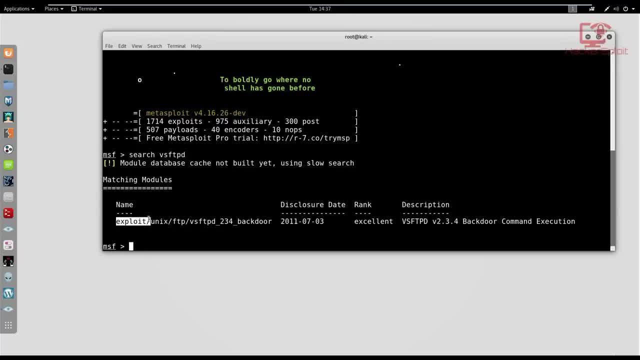 us and, of course, this is an exploit. So it's an exploit for Unix- Alright, fantastic. It's an exploit for FTP- All right, that is great. It's an exploit for vs ftpd 2.3.4.. Fantastic, So we've. 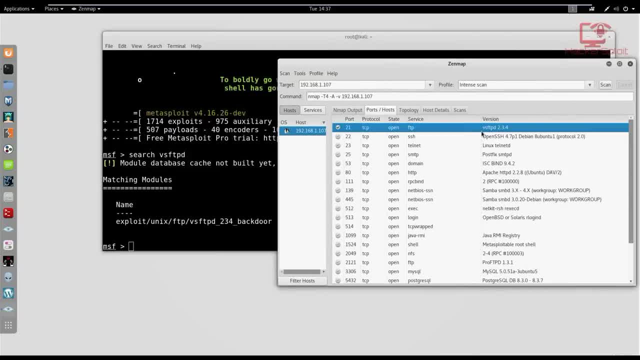 actually found an exploit that matches what we're looking for. So again, it's an FTP port And it's running vs ftpd 2.3.4.. So excellent, we've found what we needed. Now let's look at the additional. 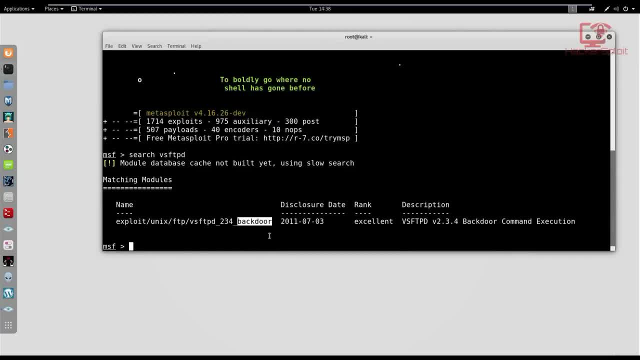 information. It is back door right, Very important. Let's look at the disclosure date. So that was when it was disclosed. Obviously it's a very, very old vulnerability. Again, you know, for the purpose of learning, the rank is excellent, which means it has been used and has been confirmed to work. 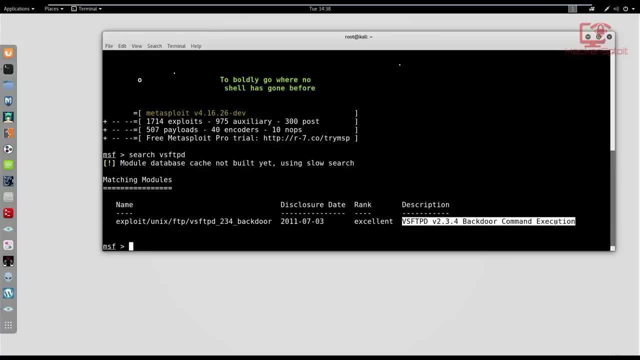 The description simply describes what it's all about. We have the vs ftpd, which is the software version and the version number, followed by the function or the exploit that this gives you right? So it's a backdoor command execution. Fantastic, Now let's use this exploit. 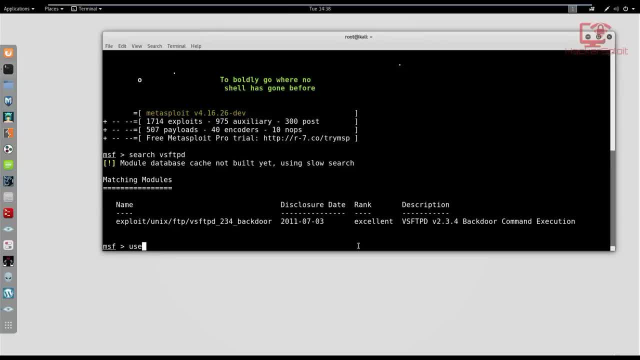 How do we go about doing that? Well, simply put, we just use, and we can just copy this right Again. the reason I highlight this is to just show you how it's done. Alright, so we can paste that with Ctrl, Shift, V, or you can right click and paste it as well. Alright, so we're going to be using that. 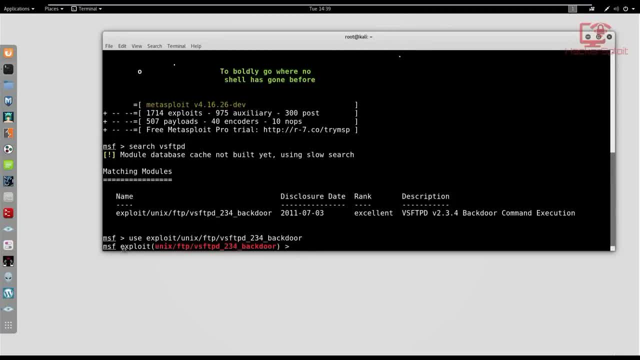 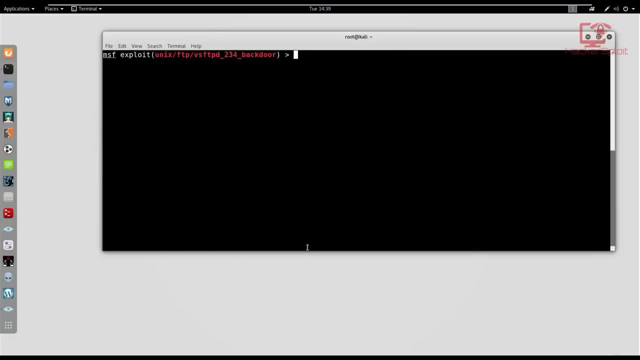 and we just hit enter And if it's successful, it should say exploit and give the name of the exploit: Awesome. Now, as I said, if you know the syntax, they are the most efficient thing to do now, or the most the best thing to do now is to show the options, Alright. so, show options, Alright. so 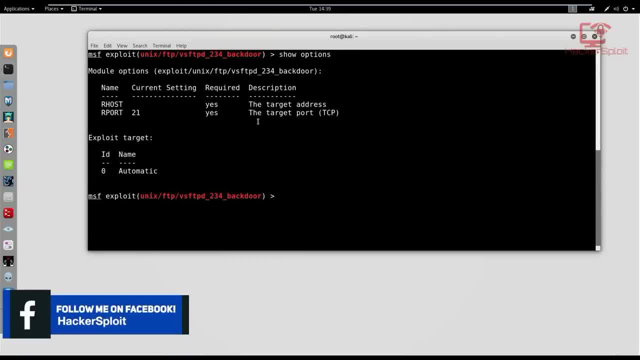 there we are. these are the options that are available with the exploit. So we already know that the let's go through this stage by stage. Alright, so when it shows you the options, usually with different exploits or different modules, you'll have different options. that 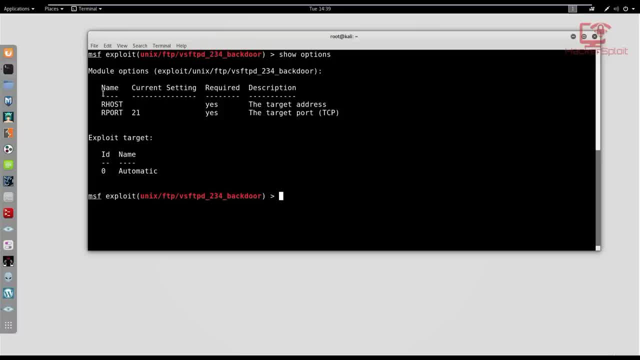 you can customize depending on the, on the attack vector, Alright, so, for example, here we have the name, all right, the name of the option which, in this case, we can change, the our host, which is the IP address, or the, the target IP that you have to set in order for you to perform the exploit, right? 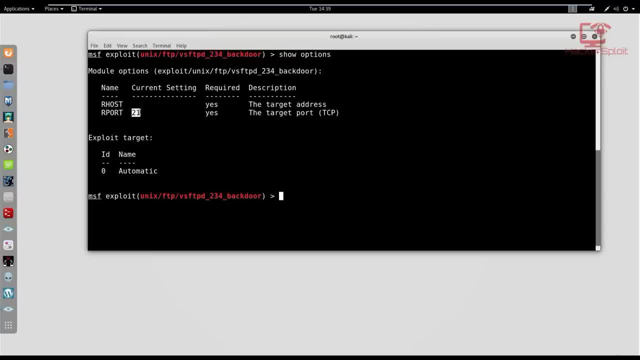 And then for the output, since it already knows it's running on. the FTP port is running on port 21.. It'll already set that for you. But if a port is missed, correctly configured- which I've seen- it is running on port 21.. But if a port is miscorrectly configured, which I've seen, it is. 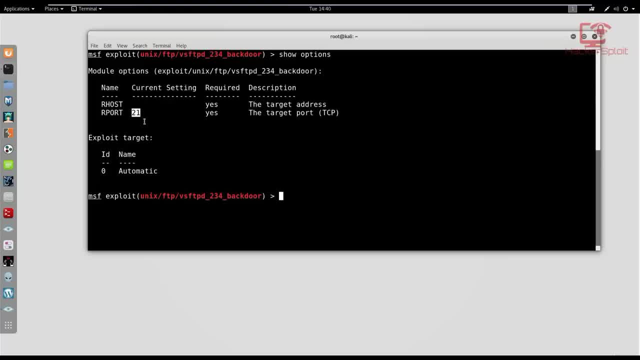 incorrectly configured, which I've seen many times before, trust me, on many, many top servers. I've actually seen this with you- know myself that where this is, the systems administrator actually configures the FTP port onto another port number. Now, when this happens, it's very 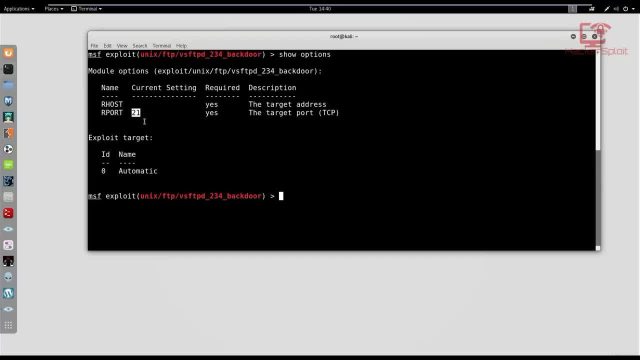 important that you get to know this, And that's why I said information gathering is critical. Alright, so now we need to actually set the our host, which we we've looked at before. So it's simply put: set our host, All right. 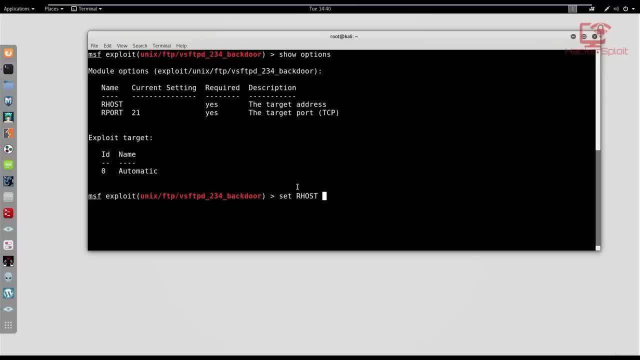 So set our host. And finally, you have to know the IP address. In this case, I've set up a virtual lab and I'm running this on my local network, So the IP address is going to be a local IP address or a private IP address, So 192.168.1.107.. Right, that's my metasploitable to IP address yours. 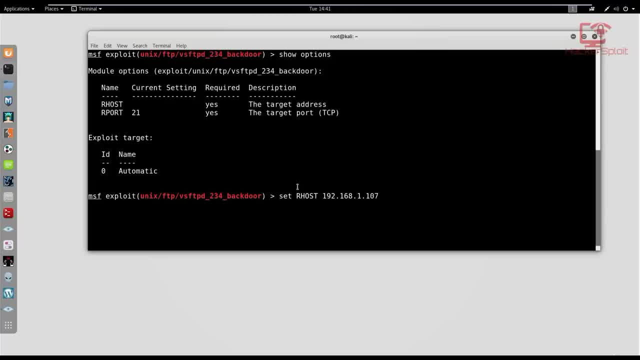 might be different. it should be different Again. you know your network is not going to be identical to mine. Alright, moving along. So we're setting the our host to that And that is the syntax that we're using, And we're going to hit Enter And it's going to give you the, the option that our host is set to. 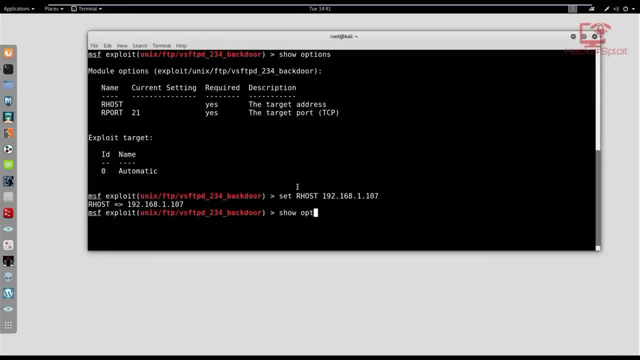 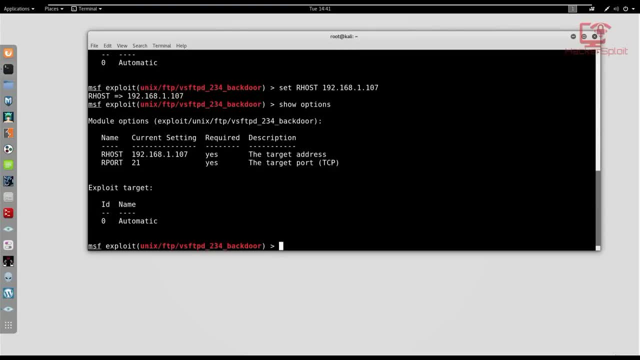 that current IP address. we can now show the options again to confirm that indeed, it did set And, as you can see, yes, it did. Now all we have to do, or what is left, is we just need to hit exploit and it will open up a backdoor. Hopefully, all right. everything went as planned, So exploit. 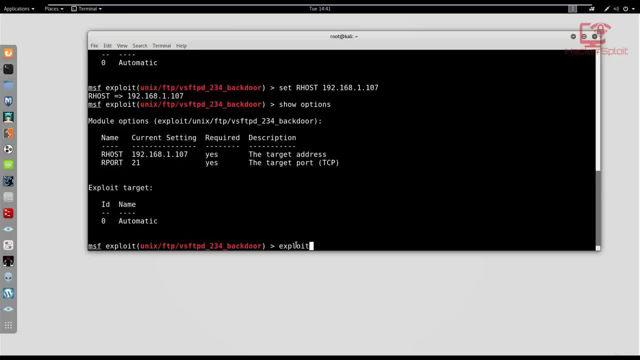 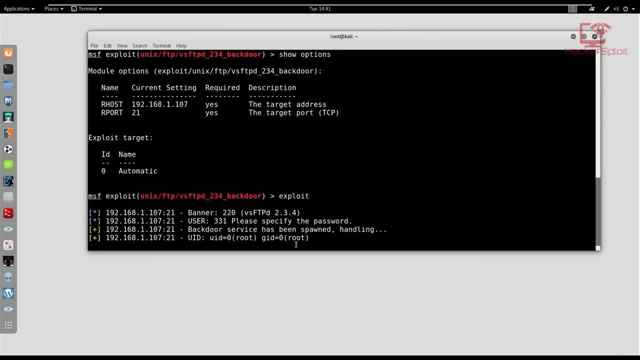 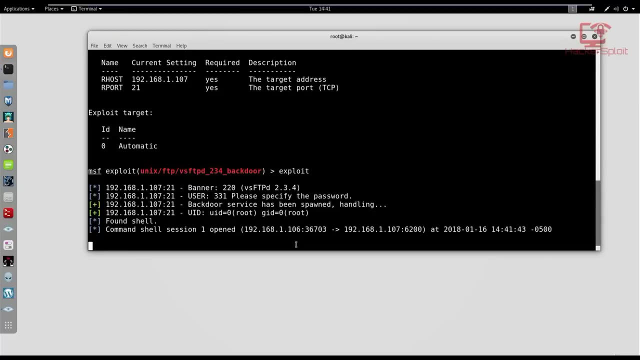 oops, exploit, And we hit Enter. And if everything went as planned and everything should have as I've gone as planned, we should get a backdoor. There we are fantastic. It has worked. it has created a reverse shell and a command shell actually. So there we are. 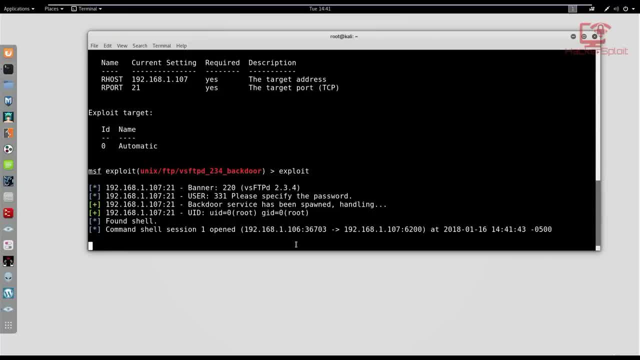 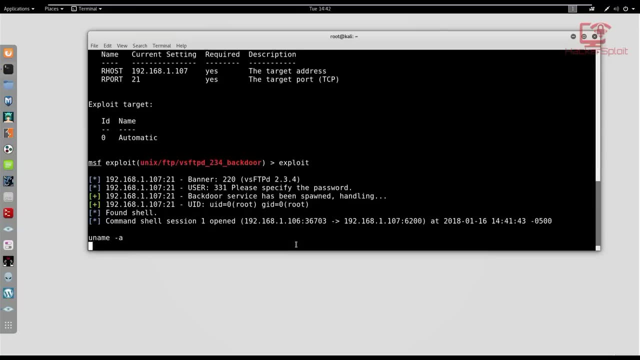 we can see the port that is outgoing and the port that is incoming and the date at which the this was open. Alright, so you might be asking: well, what are we doing here? Well, we actually have a reverse shell. So if I you name a, all right. if I just check some Linux commands, there we are. 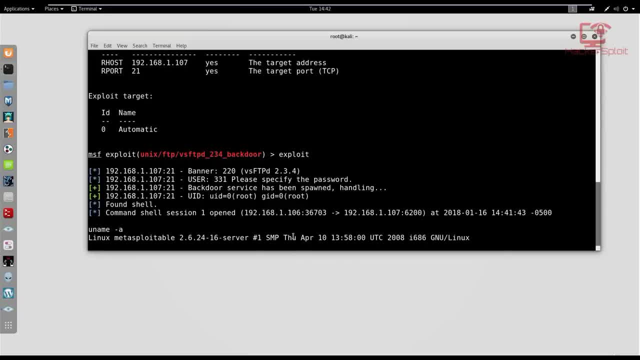 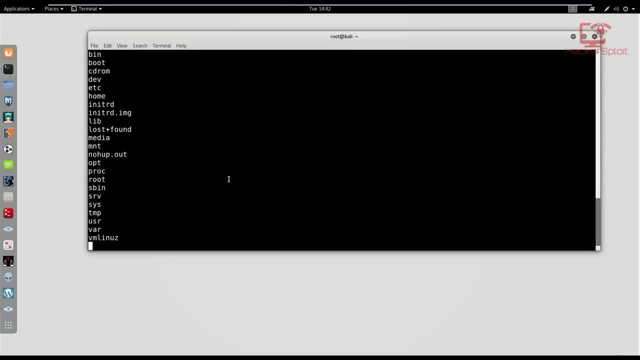 Linux metasploitable to server, blah, blah blah with the date that exists there, etc. etc. So we actually have, we have access to the server. Fantastic. So if we list the files, as you can see, we have this. Now, this is what I'm talking about. the damage that can be done here is is: 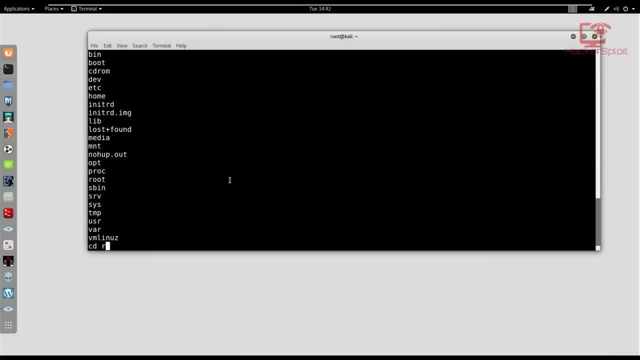 quite, quite a lot. So you know you can actually enter the root directory. Let's list what we have in there. We have the desktop. let's see what we have on the desktop. of course there's not going to be anything because I haven't put anything on the desktop And that's because I don't have a 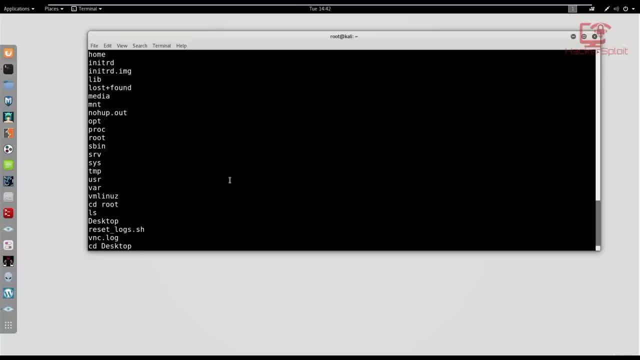 desktop or a a desktop environment installed on the metasploitable to. So if I list what's in there, as you can see, there's going to be nothing. but I'm guessing you guessed the idea, That is, some basic exploitation of the services that are currently running on metasploitable to. now we'll 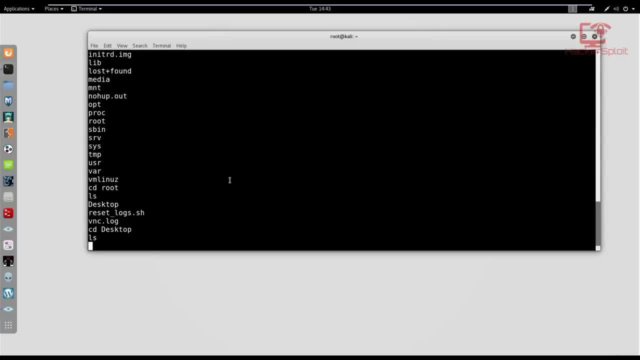 be moving along into more advanced ones and said we'll be looking at web web penetration testing. we'll be looking at the web apps that currently come with metasploitable To like the damn vulnerable web application or PHP, my admin, etc. etc. So that's going to be for. 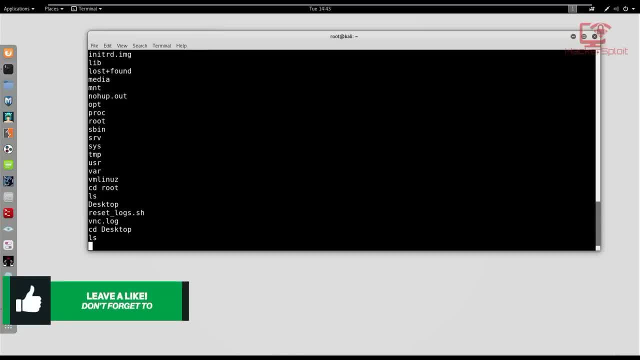 this video. guys, I hope you found value in this video. If you did, please leave a like down below. If you have any questions at all, let me know in the in the comment section, And you can hit me up on my social networks or on kick For the documented version of this tutorial or of this. 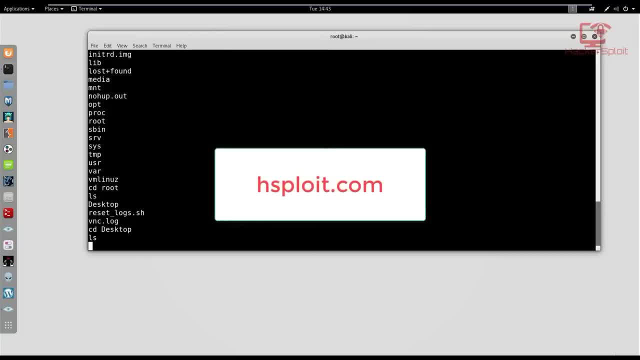 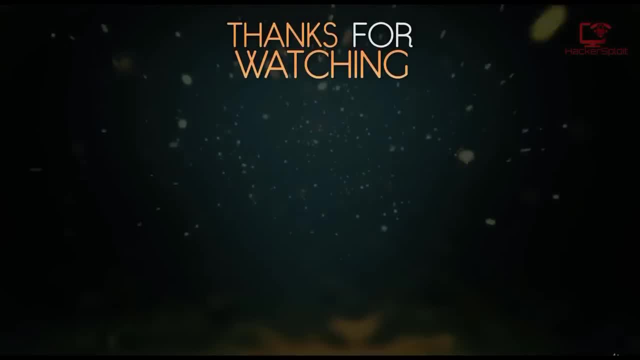 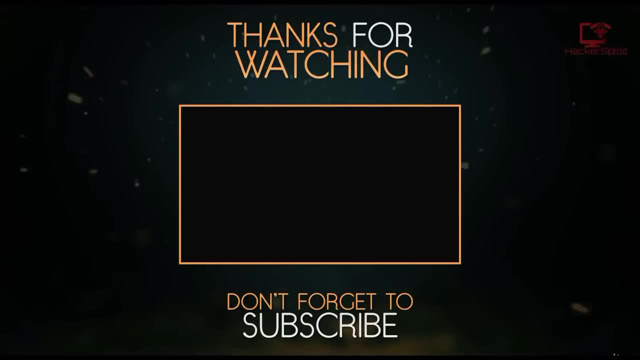 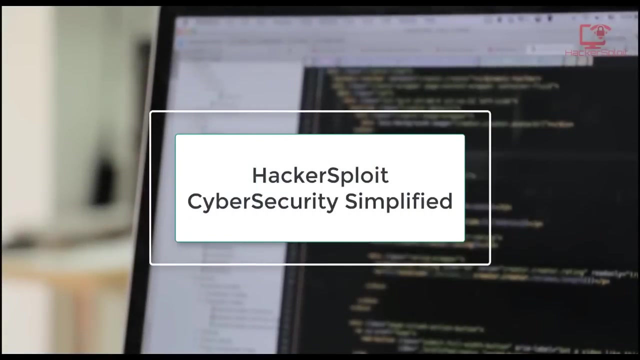 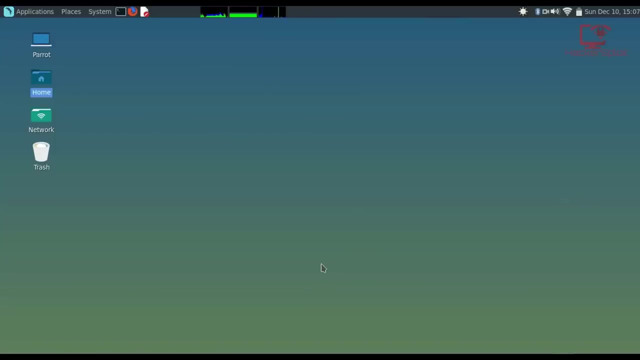 video. you can check out my website, hsploitcom. The link will be in the description, as always, and I'll be seeing you in the next video: Peace, peace, Any on which one you want to get installed, And you might be asking yourself for what exactly is. 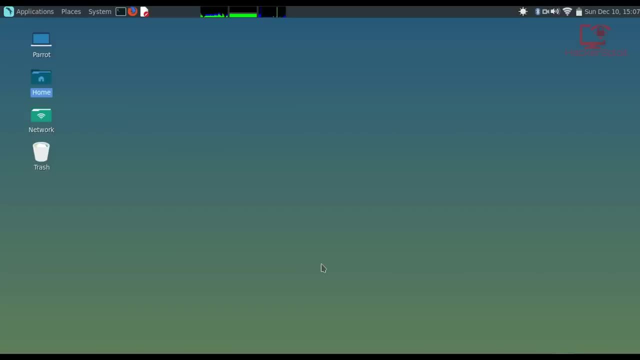 metasploit. I thought we already knew what metasploit is. Well, that's true, But what you're looking at or to use on Kali Linux or on pirate OS is the metasploit console. Alright, so that is essentially metasploit for the command line. Now, what I'm talking about is the metasploit framework. 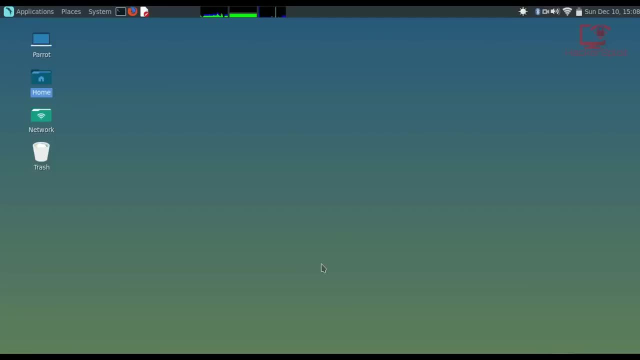 that is, a GUI framework that will discover, that will allow you to discover open ports on a network, and then it will send out the installed services on the target or the server or website that you're trying to scan on. Alright, so again, you might be asking yourself: well, what's the? what's different, What's the? 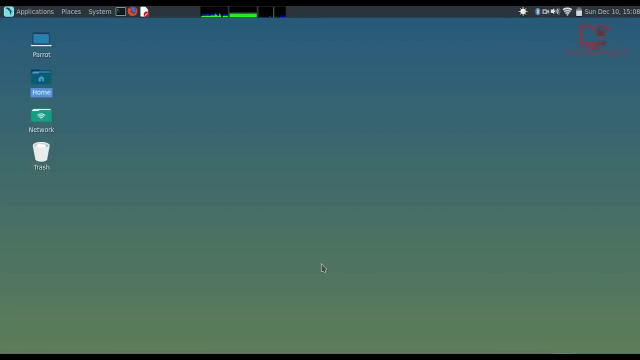 advantage. Why do I need to use this? Well, the main or the best part is that it maps the services that will be installed on those ports to the metasploit modules or exploits, and will allow you to execute the exploits on the the port. 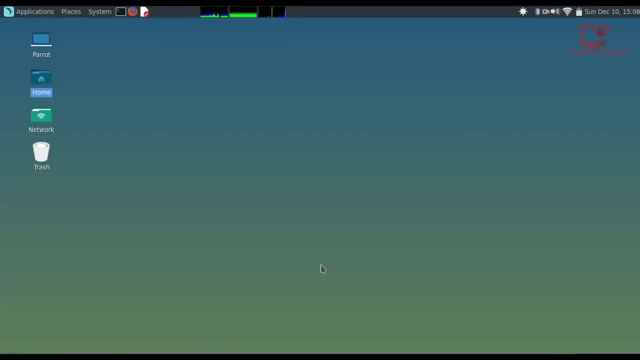 you choose. So, to put it really really simply, it will allow you to scan your network. Okay, so once you've scanned your network, what will happen is it will show you the ports and the services running on these ports. So let's say you had a port running an FTP, So you have your FTP port, and it was. 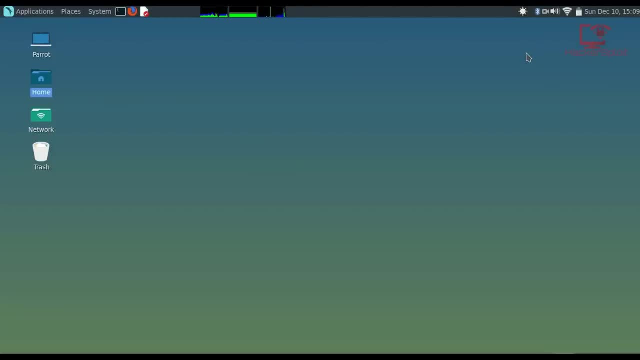 running a specific service. what it will do is it will get all the exploits that are compatible with the service that is installed on that port, And then we'll show you the exploits that you can use to perform your attacks, And it's very, very similar to what you'd find on the metasploit console. 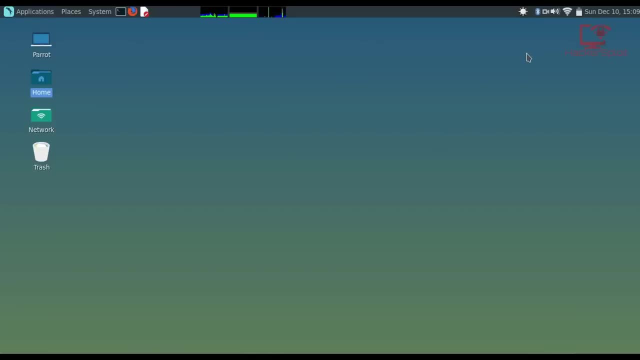 But in this case it will show you the best options, Alright. so it's really, really awesome And it's more of a professional based tool, right? So what you want to do is it's completely free. the community version is completely free. There is the pro version, but that's if you're really 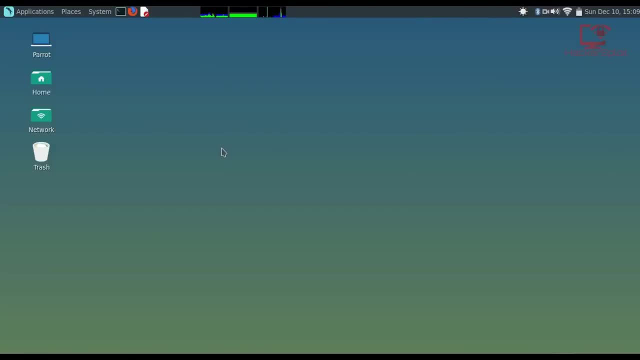 into into this in on a more professional level, I have used the professional version And if you're moving into network penetration testing, it is a really really good option, Alright. so let's get started. It's really really very simple, Alright, so I'm just going to be putting the links in the description to make it. 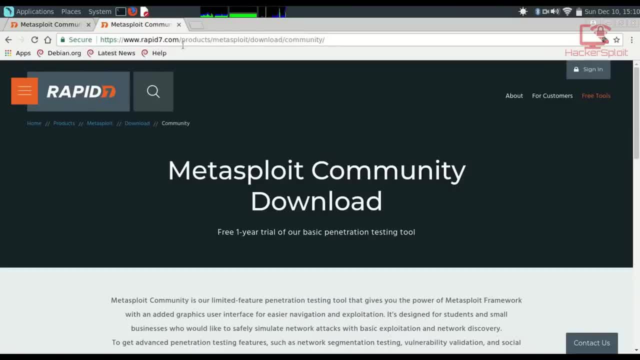 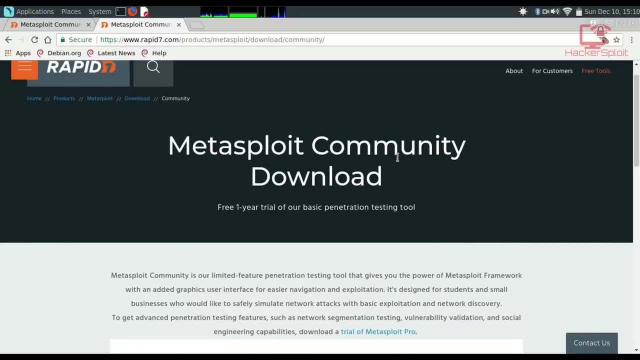 easier for you. You want to go to rapid sevencom Again. they developed metasploit, So this is their product products: metasploit download and community Alright. so, as you can see, metasploit community download and it'll give you a free one year trial, So it'll actually give you a serial key. 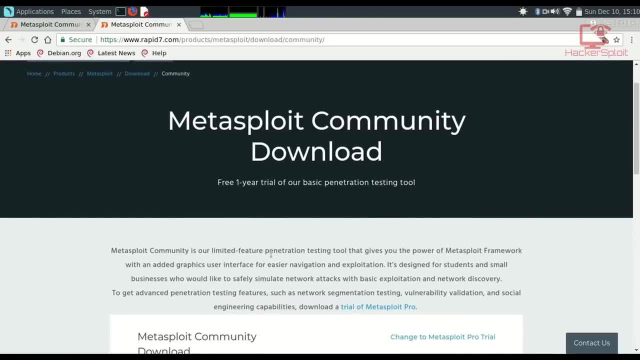 for you to use and to test. So the metasploit community is our limited feature penetration testing tool that gives you power of the metasploit framework with an added graphics user, graphical user interface for easy navigation and exploitation. right So it's designed for students and small businesses who would like to 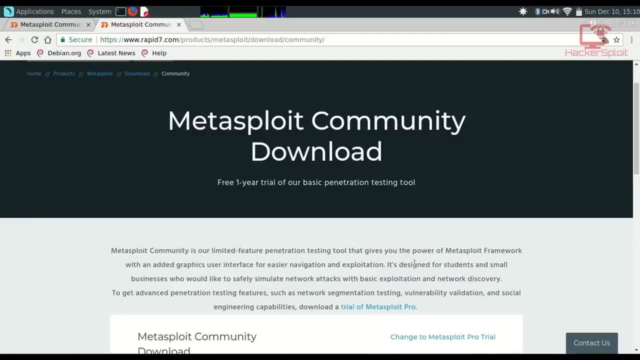 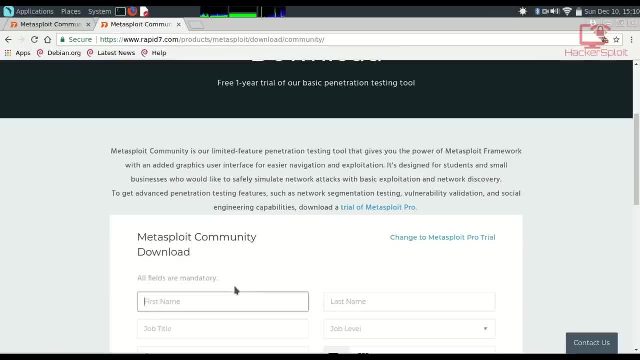 safely simulate network attacks with basic exploitation and network discovery. Alright, so what you need to do is you just need to enter your details here: your name, your email. it's very important that you enter your valid email, a working email, where they'll be. they'll. 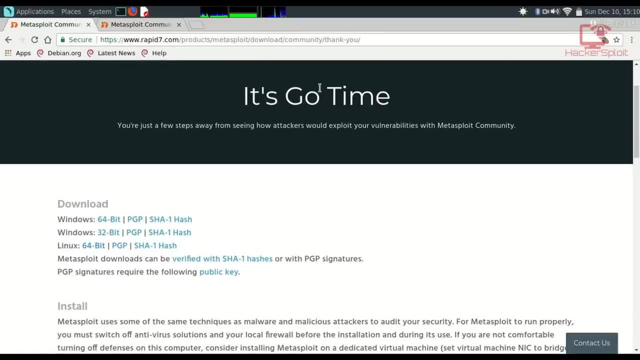 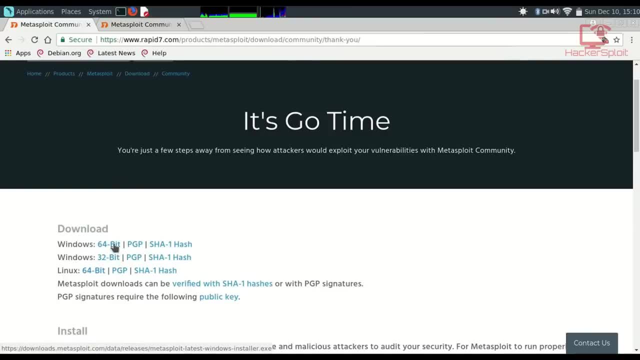 send you your serial key. So once that's done, it's gonna take you to this page And, as you can see, it's good time, And it's going to show you the downloads. So it does work on Windows, because it's a web based graphical user interface. So you have your windows and you have your Linux In my. 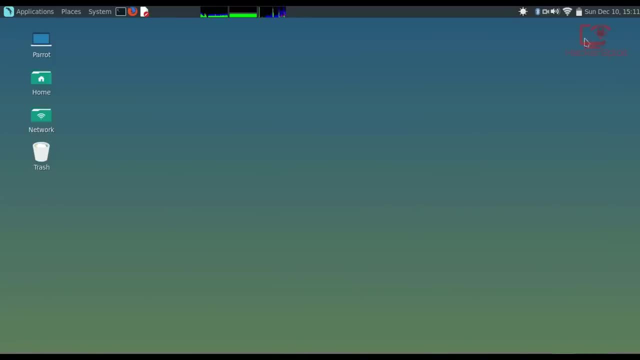 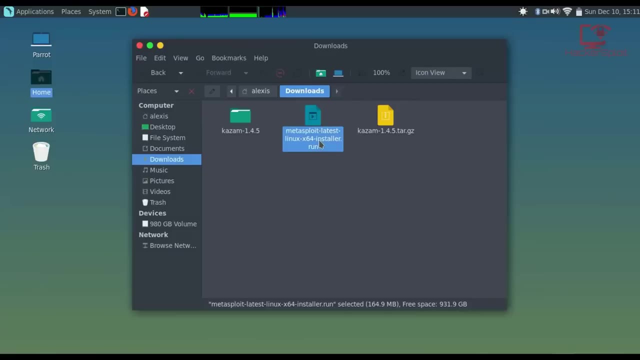 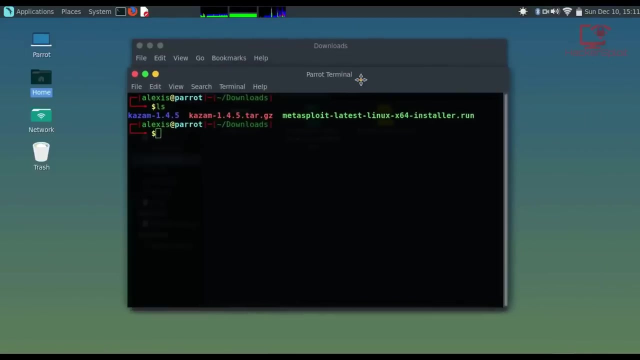 case, I'm running like 64 bit, So just click on it and it'll download the file for you. Alright, so once you've downloaded the file, what you want to do is you want to go into the installer. This is, it's going to be a very, very simple installer, and what you want to do is, obviously, if you look at, 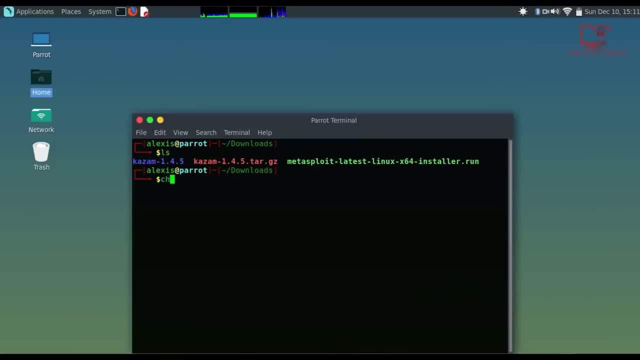 the permissions. you will not be able to run it immediately, so just change the permissions. with chmod plus x, whoops plus x, and you want to just select the metasploit framework. there we are the installer. so make sure you change the permissions to allow execution and once that's done, just run. 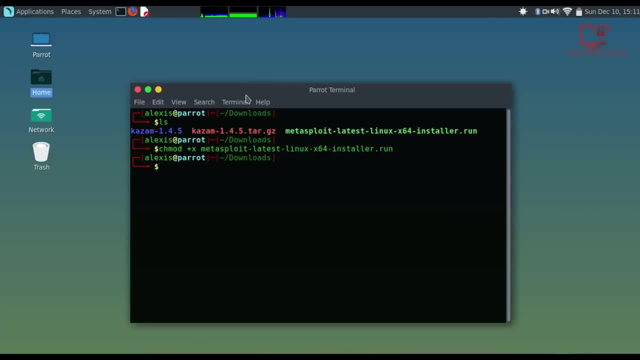 it and it's a very, very simple installation. it'll probably take a few minutes to get installed. the installation process is really, sim, uh, very, very simple, so i really don't need to take you through it and it'll take quite a bit of time, so just give it enough time to install. in addition, 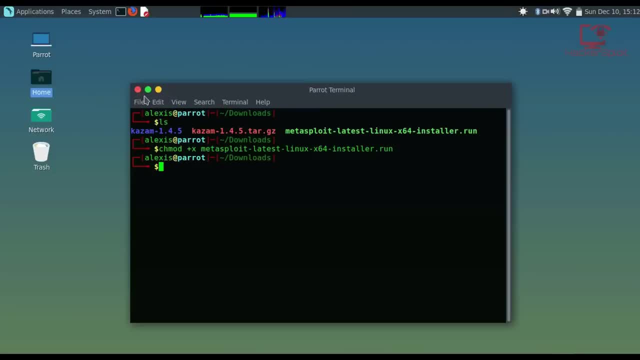 to that. uh, i've already installed it so we don't need to go through the installation process. so once it's installed, um, it'll probably prompt you to open the, the user interface, and, as i said, it does open in the browser. if it doesn't open for whatever reason, it's really really very simple to. 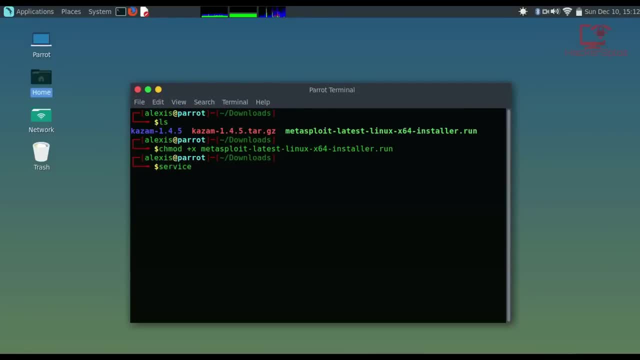 start and the first thing you do is you go to the browser and you go to the browser and you go to the user interface and you go to the rotationIDE glue. um, i believe you're gonna go to go to the original backupноеxpress, right, and it should do this. an let's first to tell you, it's just a. 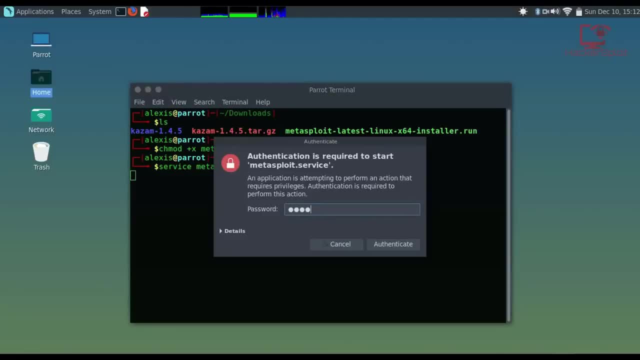 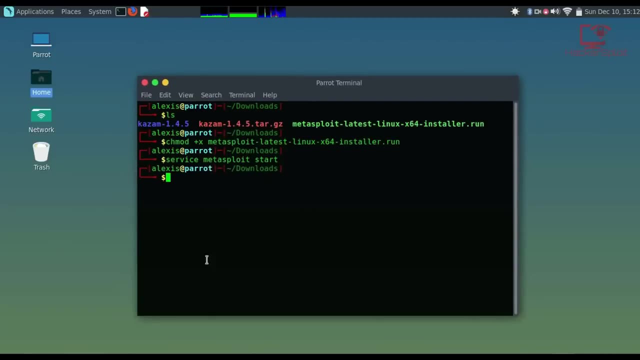 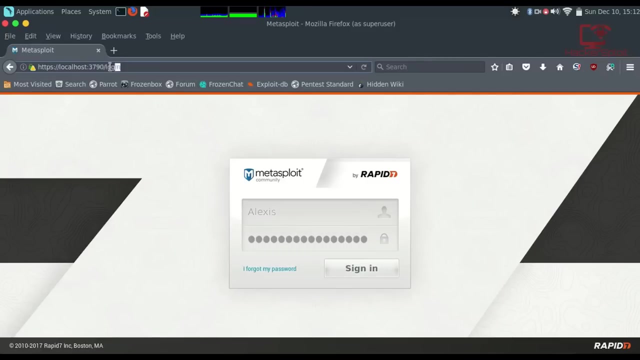 simple guide to how to start the service, all right. so the first thing i want to tell you is you need to start the service. if you installed it as a service, all right. so service metasploit, uh, whoops, metasploit. start, all right, and once you hit that, it should be good to go, and it's going to be. 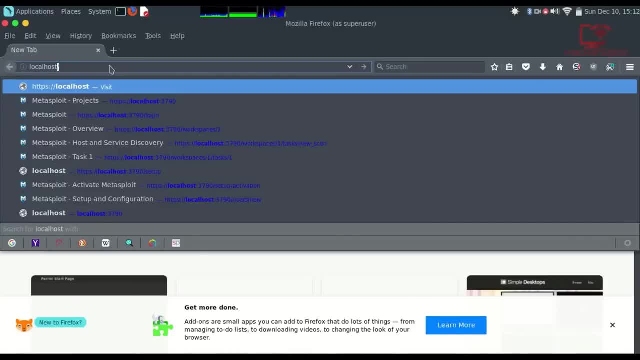 bonus if for your administrator password. all right. so let me just enter that right now. there we are and it's going to start the service, and what you want to do now is just open up your browser. uh cần jede localhost. localhost like so and localhost with the port 3790. all right, that's the port you want. 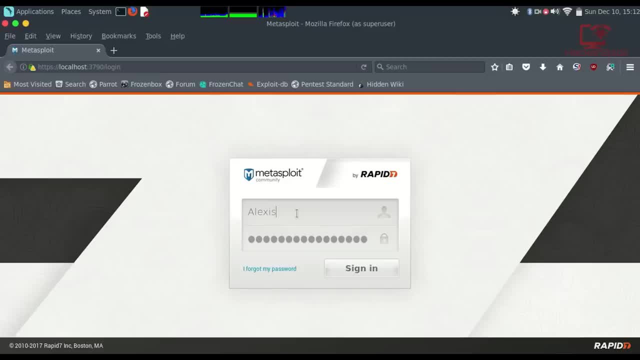 to visit. there we are and again is going to prompt you to create an account, and by this time they should have sent you a serial key. once you've created your account, this is going to be your user account. you can just sign in, all right. and once you have signed in, this is the Metasploit. 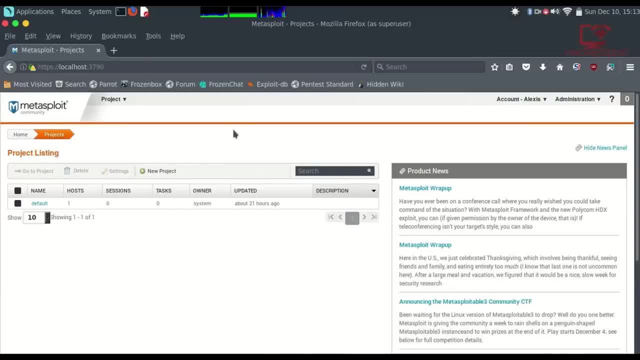 community framework and, as you can see, it's really really well designed, and let me just breeze you through the user interface so you have a good idea of what's going on here. all right, so, starting at the top, you have your project section where you can create different projects based on. 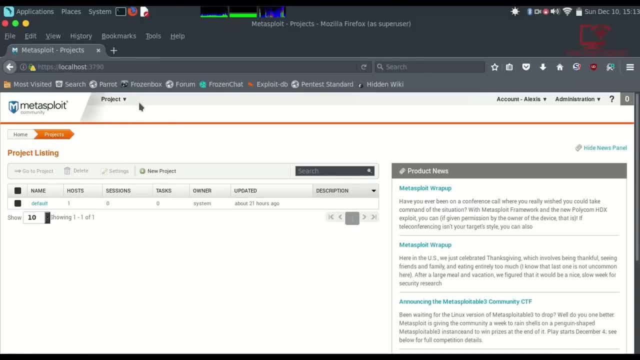 different IP addresses or targets that you want to scan or perform attacks on. so very, very good, it allows you to sort all your stuff out. you then have your account settings where you can, you know, change your settings or log out. you can then check out your administration. 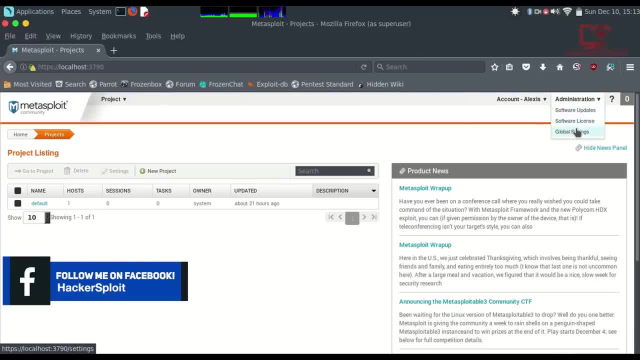 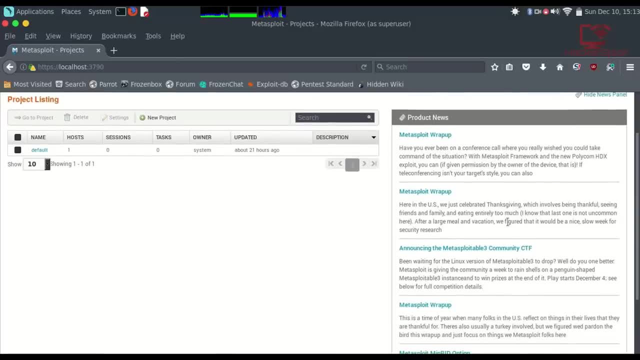 you can then check out your administration. you can then check out your administration tab here. that allows you to check for software updates, to check your software license and the global settings. all right, so that's just to do with personalization and customization. you then have your news panel. as you can see here, that is based on the rapid seven website. so this is. 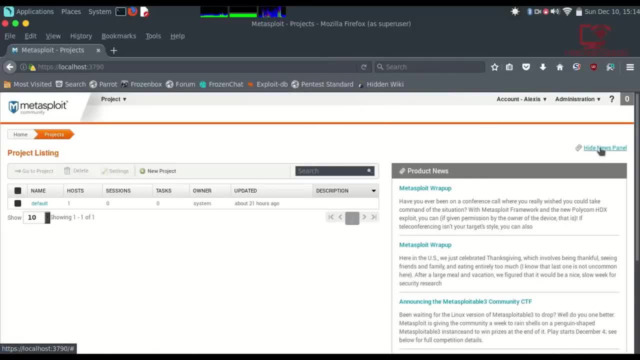 the latest news that they have here. let me just zoom back in and you can choose to hide the news panel. nothing really important there. now let's get to the main, which is the projects. all right, so you have your project listing and we'll give you a default one. so what I'm going? 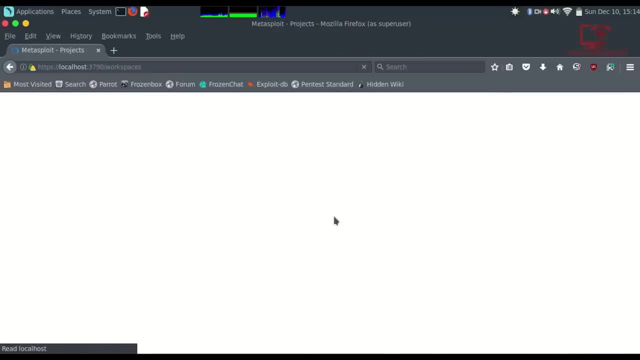 to do is I'm going to go to the main page and I'm going to go to the main page and I'm going to do is: I'm just going to delete that right and after I delete it, what we're going to do is we're. 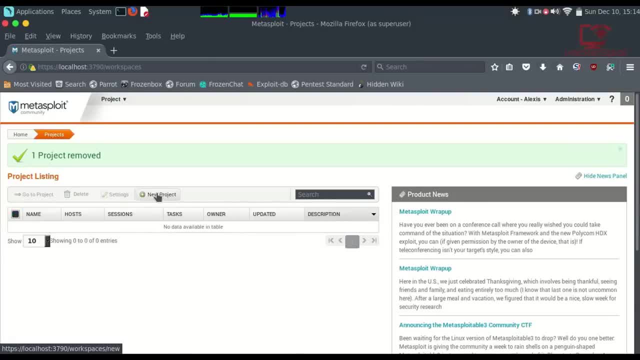 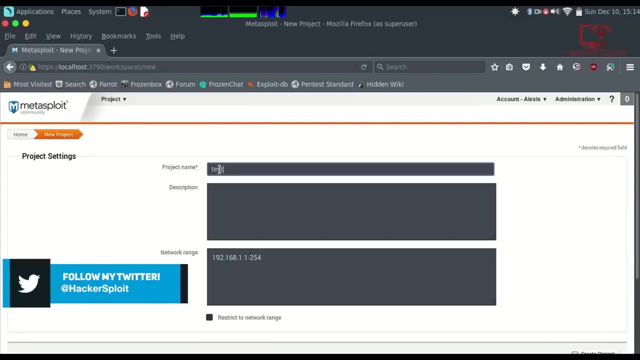 going to create a new project, right? so it's really really very simple. we're going to go into here new project like so, and it's going to ask you for a project name, so I can just call it test, like so, test. and just call it test home network, right? so this is going to be performed on our own home. 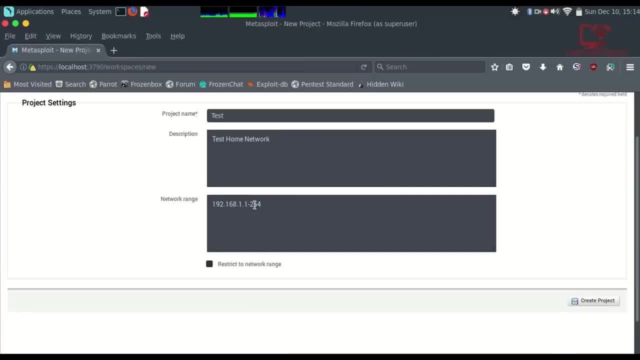 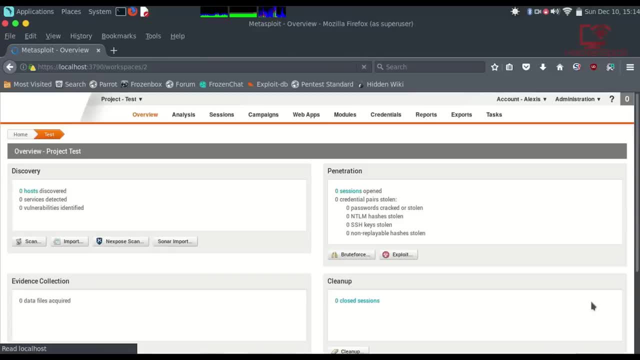 network. so, yeah, it's already given us a network range and, yes, I do want to follow that range. so 192, this is my local IP or my private IP address. so I'm just going to create the project and there we are. so it's really really very simple to understand what's going on here now. so you have your discovery, this: 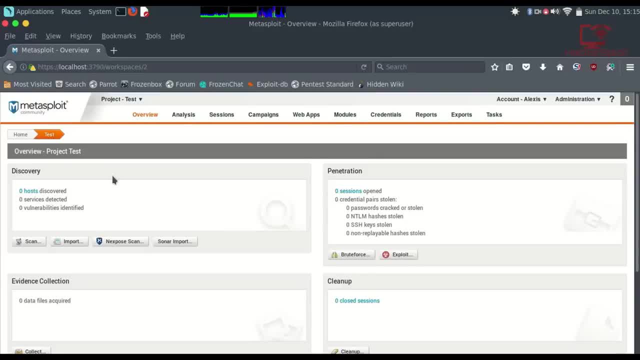 is where it's going to be all about: what ports were discovered, what services and vulnerabilities were discovered in penetration and the penetration section. this is where you're going to be doing your brute force and your exploiting. all right, we'll be looking at this in the in the future videos regarding this topic, but 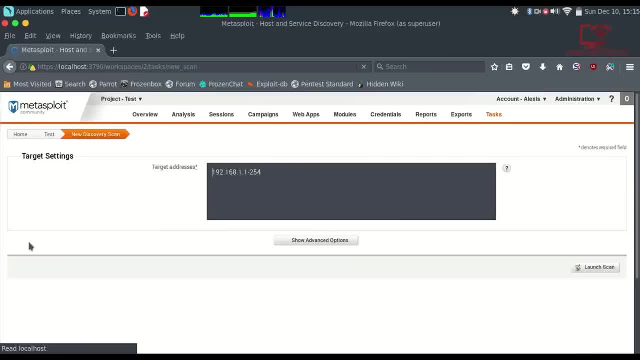 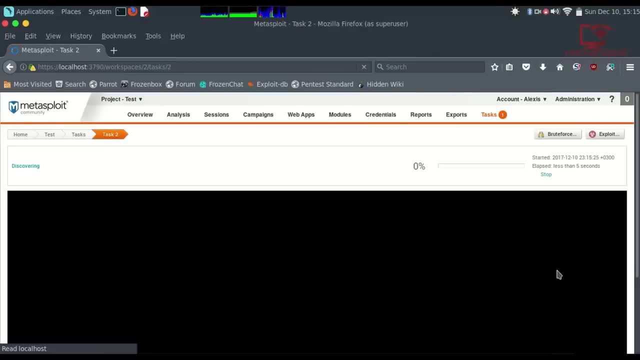 to start off, we can just try and perform a scan, all right, and when I hit scan, you're going to enter your target addresses or your target range, so I'm just gonna launch the scan, right, and I'll take a few seconds. that's something that I needed to tell you, and what it's going to do is obviously. 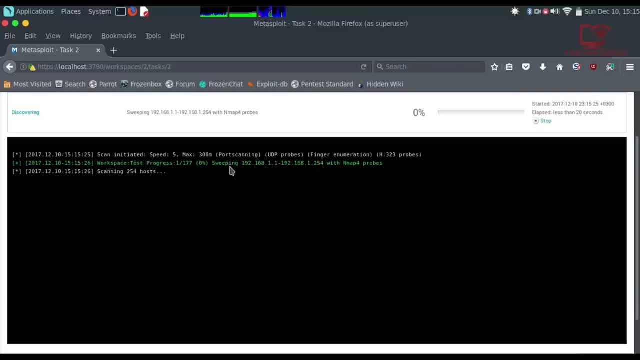 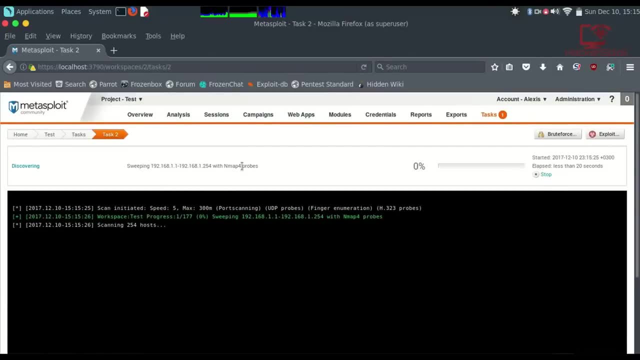 it's going to perform an nmap scan on the network range that you're provided, obviously, and it's going to start scanning the hosts. I probably should have reduced the range of networks. obviously it's going to take a bit of time. it usually does take quite a bit of time, a bit slower than nmap, but it does work alright. so once you've 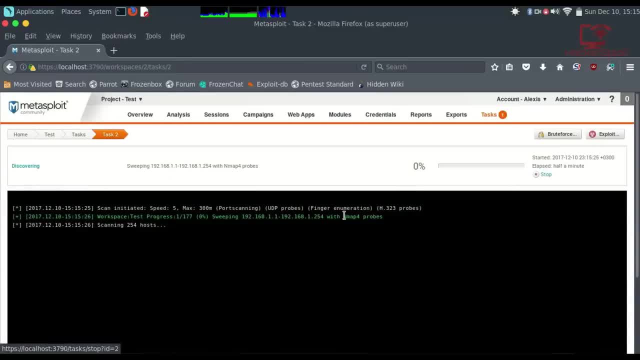 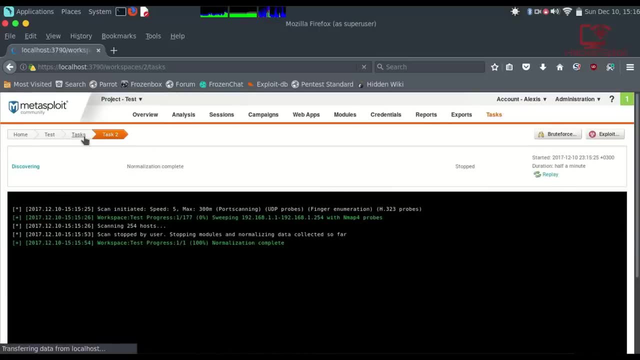 scanned. it will then give you the vulnerabilities that you can access. alright, so I'm just gonna stop this because, again, it's not very important for us right now. let me just stop that, for some read that they're. we already stopped. let's look at tasks again. all right, and test. let's move to this project. 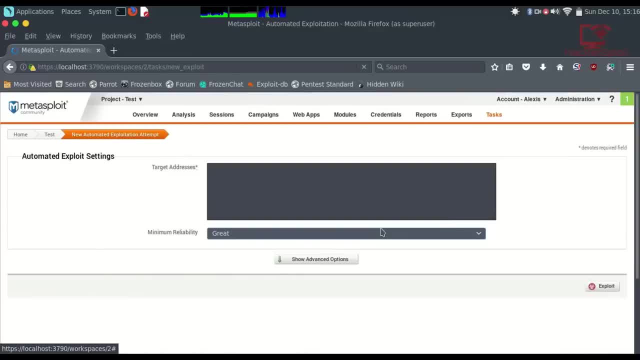 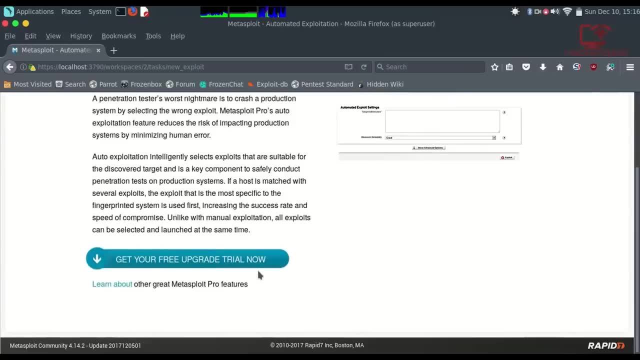 again and moving on to the exploit section, I hit exploit, it will show us there we are. so get a free upgrade to try smart exploitation again, that's if you want to move to your Metasploit Pro. but I'll be showing you how to perform the exploits directly without using the Metasploit. 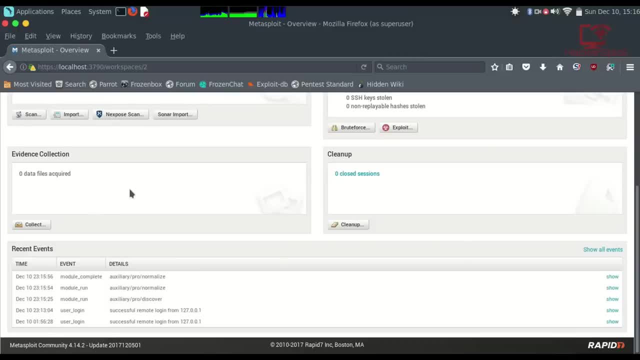 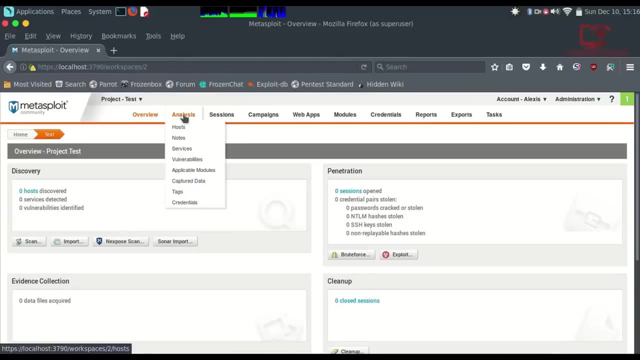 Pro. all right. you then can collect evidence and this is more to do with the web and cookies stuff like that. you then have your analysis section. this is where you can look at the- you know, different information that was captured. you have your sessions, campaigns, web apps modules. so web apps is to deal with if you 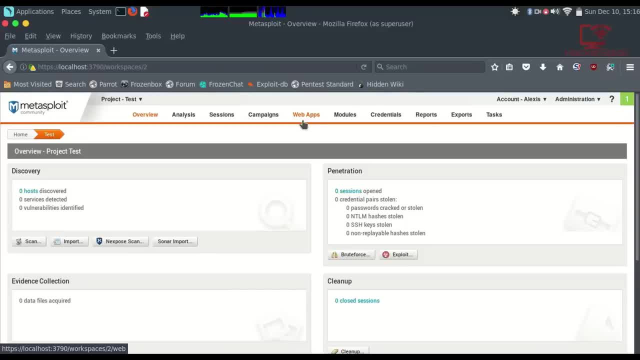 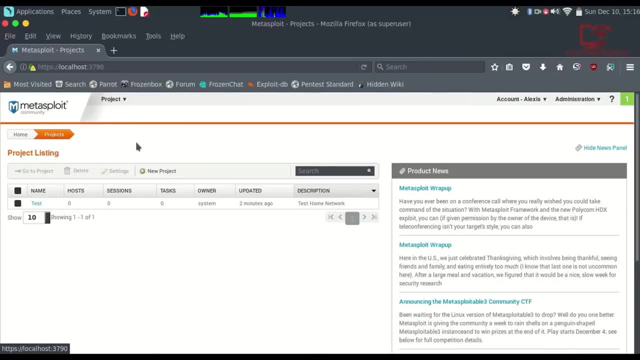 performed a scan on a web server and it had web apps and that you would like to scan and exploit. that's what it will deal with. but that's a basic overview of how to use Metasploit and, more specifically, Metasploit community. so it's a very, very powerful tool. as I said, it's oriented more on the professional. 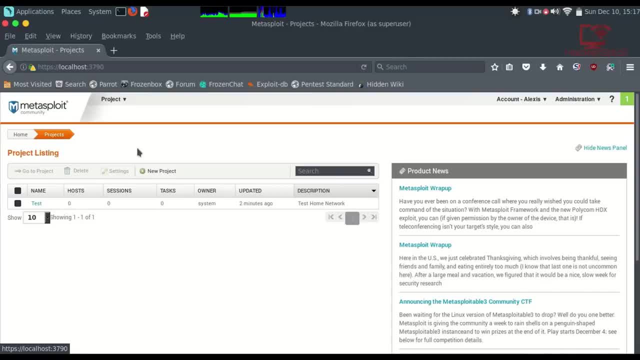 or enterprise level, depending on what state you are in your penetration testing career. granted, that is a very, very important thing to learn, so i hope you guys found value in this video. if you did, please leave a like down below. if you have any questions or suggestions, leave them in the comment. 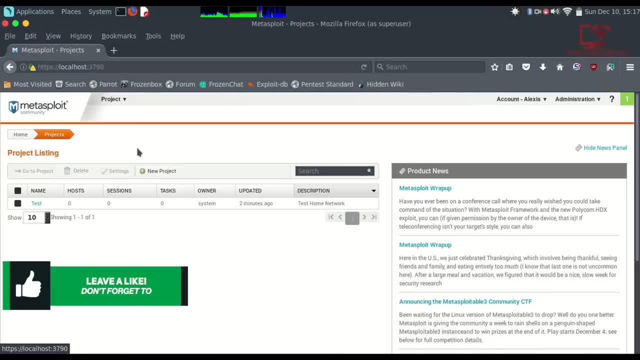 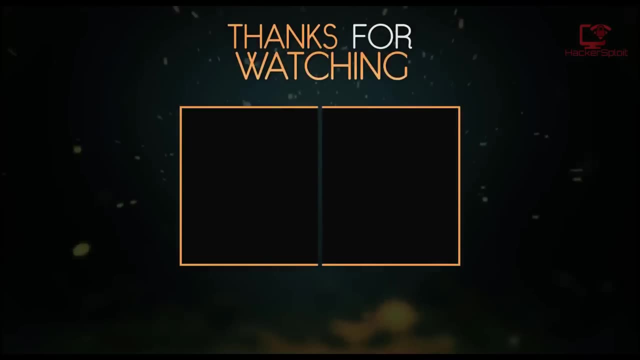 section, or you can hit me up on my social networks or on kick for the latest hacking news and resources. check out my website. you can also ask me questions there. the link is 었어요com and yeah, thank you so much for watching this video, guys. peace. 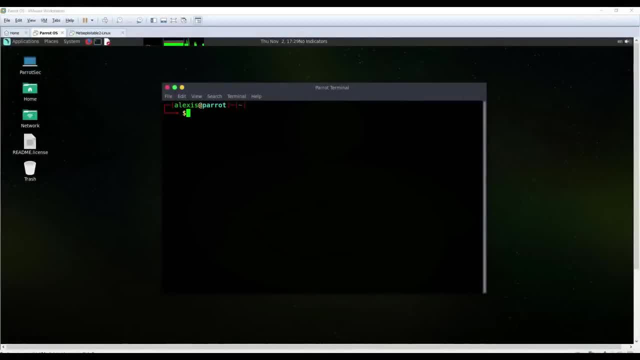 hey guys, Hackersploit here back again with another video, and in this video we're going to be looking at hacking web servers, or basically gaining access to web servers. so let's get started. so this video is going to be be about gaining access to web servers. so essentially, these are going to be: 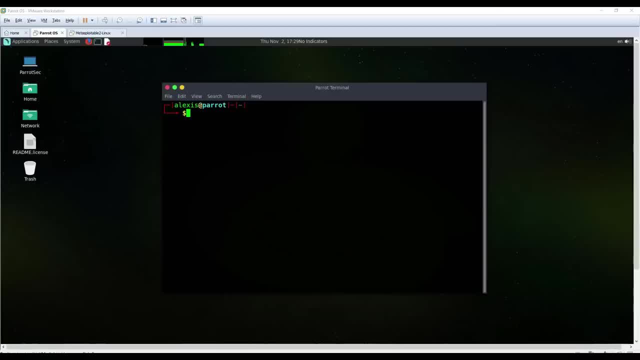 server-side attacks. now, this essentially means that the, the, or the real thing that you need here is the target or the server's IP address, which, we are lucky, in most cases, is usually going to be static or will not change very much. so, for example, if you had a domain like facebookcom- and I'm just saying you- 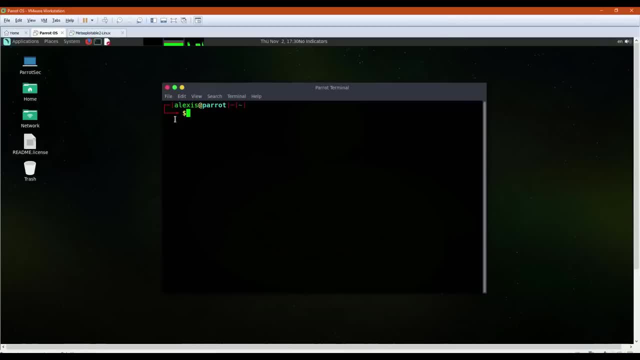 wanted to attack facebookcom, the first thing you would do. I'm running parrot OS as my operating system of choice for this video. again, I just wanted to have some a bit of mixing here with Kali Linux and parrot OS, etc, etc. so, as I was saying, you know, to get the server IP address you essentially need 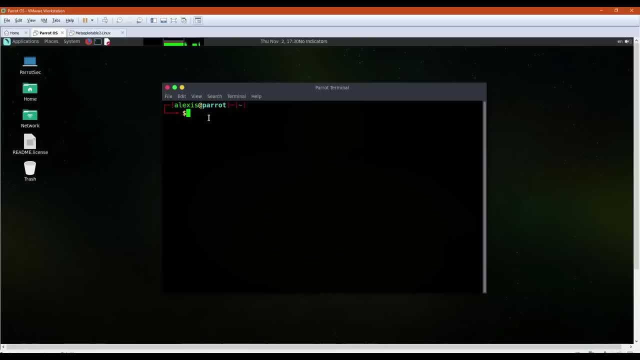 to check if it's running, and the one way you could do this is by pinging it. so we can try and ping something like facebookcom and if let's see if we get a response. yeah, we do get a response. so we know that facebookcom is up and running and we have the IP address and this IP address. 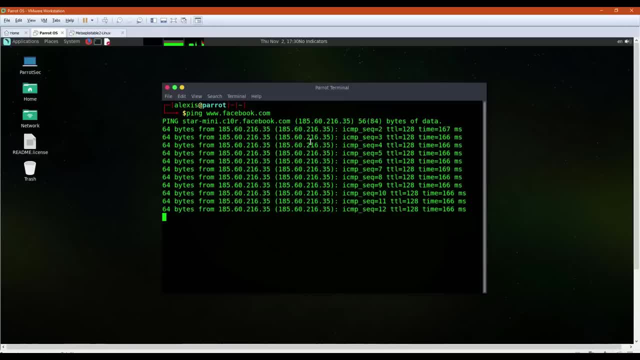 may be changing here and there, but for the most part it will stay the way it is, so that's a very good thing. now, the difference between server-side and client-side is that the client-side requires a bit of user interaction. so, for example, if we wanted to exploit a person's computer, it would require the 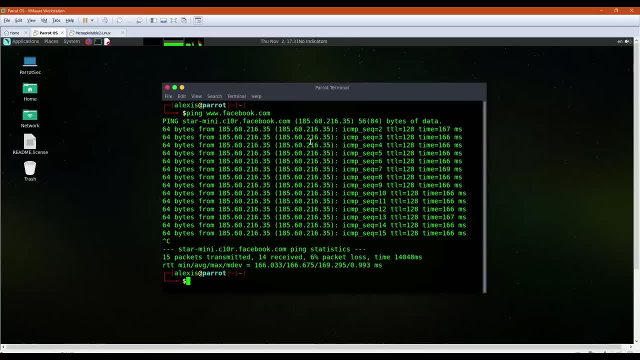 user to perform a bit of interaction, like running a program or running a file that contains malware or an exploit. you know something like reverse TCP, shell, something like that, etc. etc. I hope you guys are getting the idea now. as I said, when we're talking about servers, 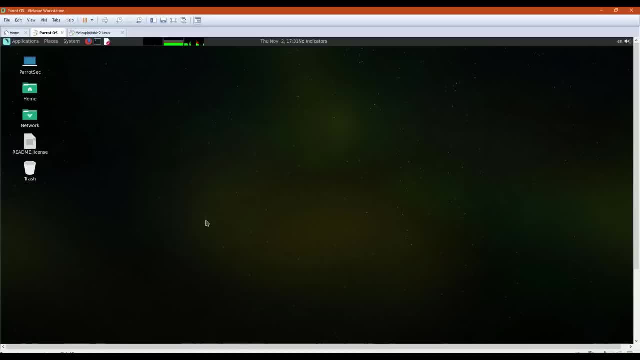 one of the best ways to practice this is by using metaploitable. alright, more specifically, metaploitable2.. now, metasploitable is an operating system, a Linux operating system, that is essentially made to be vulnerable and is there to allow you to work with кей. акушь м. nächste Party claimed medication Ums清да. 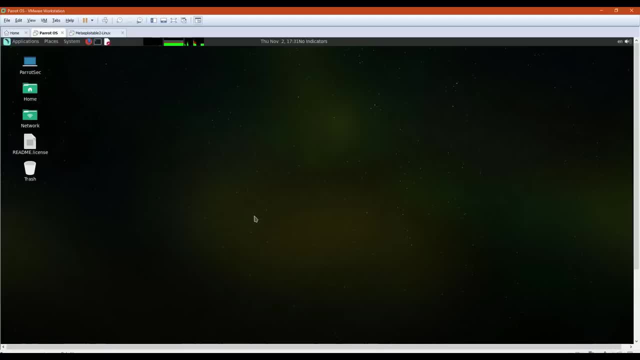 customize your lab so it works as a virtual lab that allows you to learn and to practice your pen testing skills against server based systems. so it comes pre-installed with a whole lot of services that are vulnerable and the operating system, as I said, is designed to be vulnerable. so that's what we're. 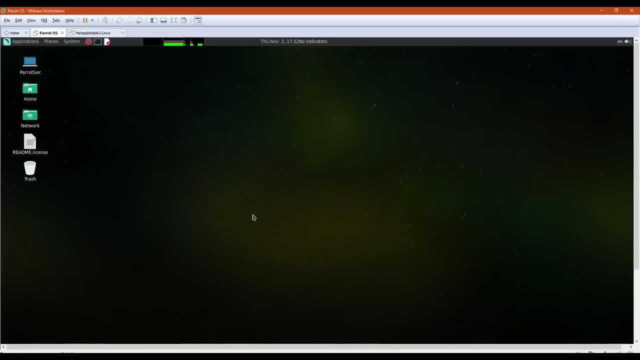 going to be using to be testing out our attacks. now I'm going to be linking the the download in the download link in the description for Metasploit, so go ahead and download it. it's a virtual machine file, so you can only open it through a virtual machine and it really does not need a system resources, as you. 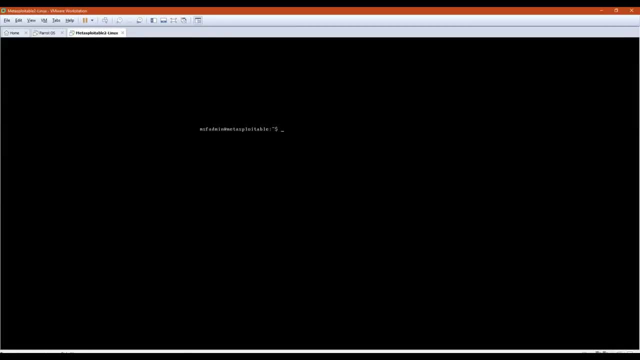 can see. I have it opened here and I'm just using the default login credentials. I haven't created a user and it's as vanilla as can be. so the most essential thing, as I said, is getting the IP. so I'm on my local network again. you can use. 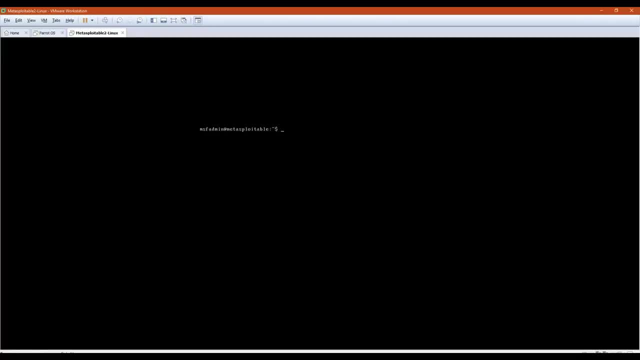 your public IPs to target machines, which is one of the ways we'll be using for client-side attacks and also for server-side attacks. but I'm going to be working on my network, because the virtual machines are on my network, obviously, but the the principle stays the same. now, make sure that your virtual 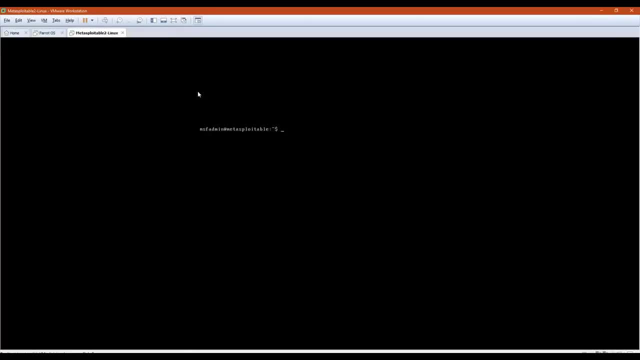 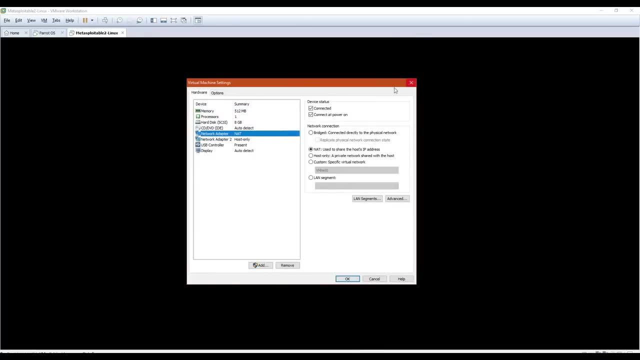 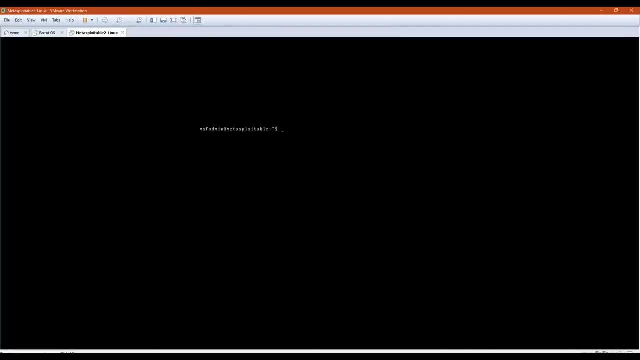 machine is make sure that your virtual machine is running in the NAT mode on your network, essentially meaning that you've created a domain for it. alright, so it's gonna share the host IP address. now let's find out what the local IP address is for the Metasploitable virtual machine. So I'm just going to hit ifconfig. It does not have a. 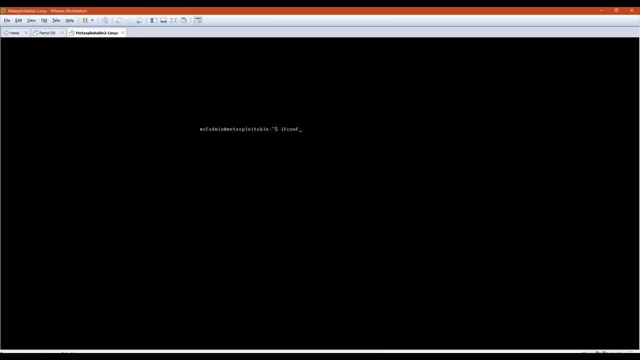 graphical user interface or a desktop environment, but you can install that and you can use it like that. But I'm just going to keep it as vanilla as possible. So, ifconfig, all right to get the local IP And, as you can see, the local IP is 192.168.2.129.. All right, so that's what we're. 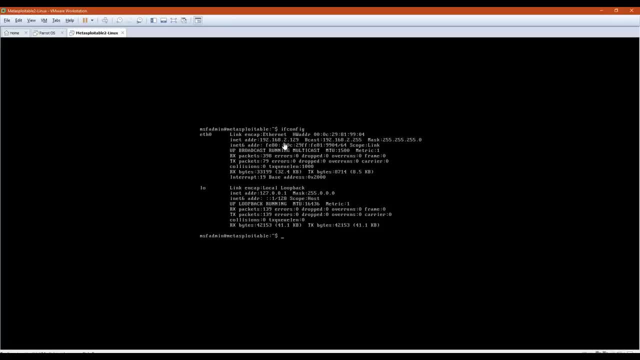 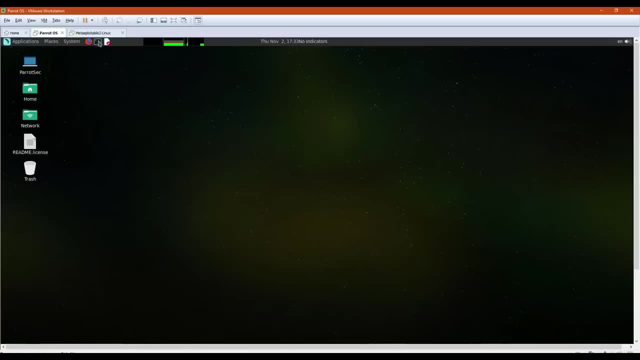 going to be trying to connect to Now, as I said, this is a web server. All right, Metasploitable is going to act as a web server or a server. So if we go back to Parrot OS and I open up a browser, 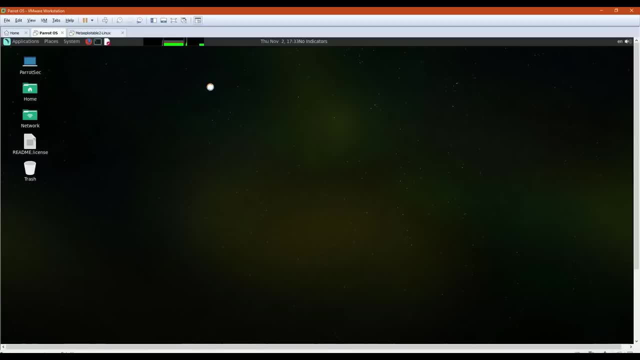 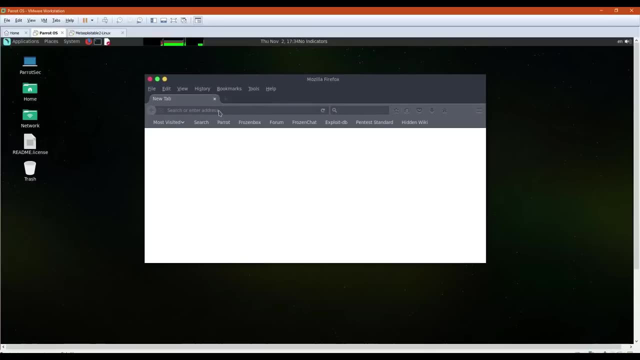 and let this open up Firefox really, really quickly. I don't know why it's taking so much time. This is all right. there we go. So now what I'm going to do is I'm going to enter the IP address of the Metasploitable machine. 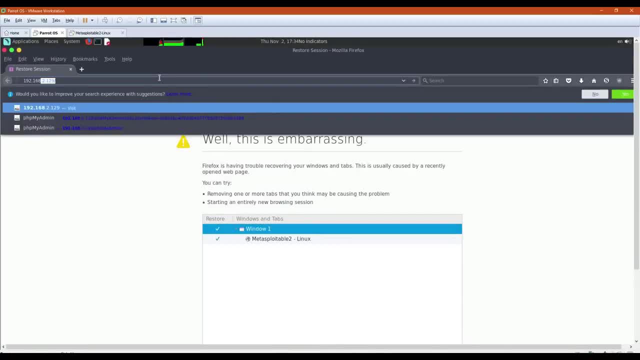 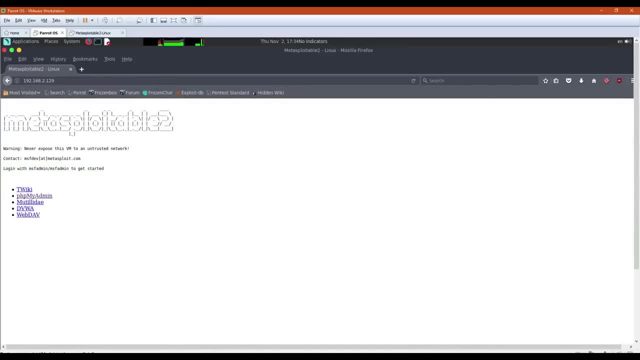 All right, so I'm just going to hit 192.168.2.129.. I already have it in my search bar And, as you can see, if I enter the IP address of the Metasploitable machine, it's going to give me the web server. So I 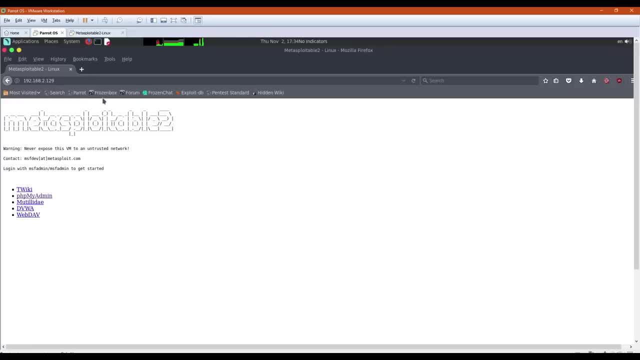 entered the the IP address of the Metasploitable machine and we can access it as a server. So that means it's working And the first thing you'll realize is that there there's no security. So can essentially log into this server, which is why metasploitable is encouraged to be run. 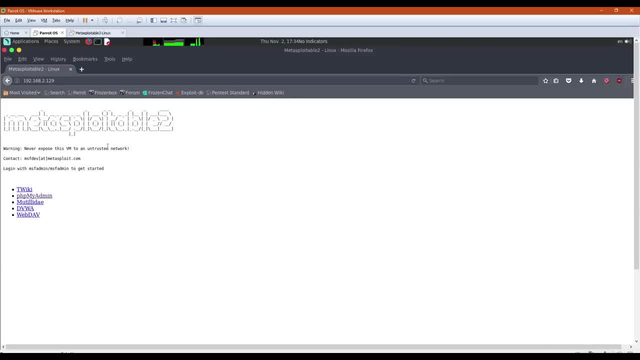 in a virtualized environment so metasploitable as you can see- warning: never expose this vm to an untrusted network. and you can contact it then. so it basically comes with all of these cool things like php. my admin for php. you have matilda, which is awesome for testing your php. 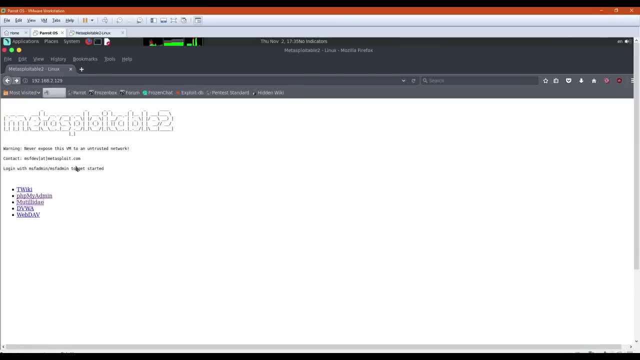 scripts and vulnerabilities, which we'll be looking at. no, no, no doubt about that. we then have the damn vulnerable web application, which, again, is one of the things you'll be trying to crack. and here we are. we have a notification from youtube and we have one of these. 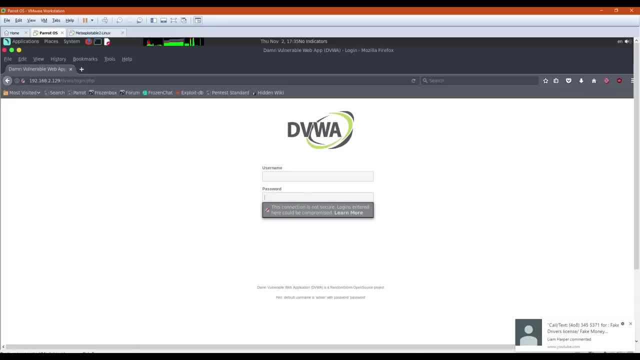 fake comments saying for fake driver's license. i'm gonna deal with him later. anyway, that's beside the point. so this is essentially the server. now, when trying to attack a server, what are you doing? you're trying to attack a server. you're trying to attack a server. you're trying to attack. 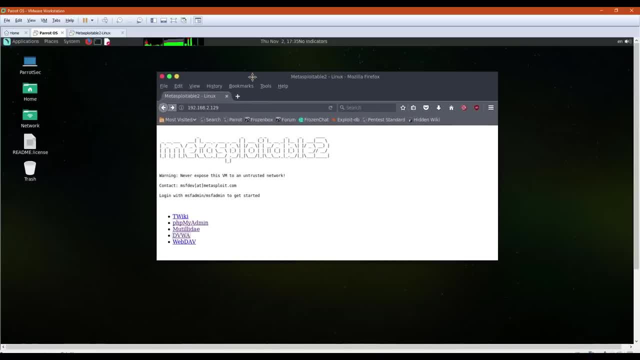 the server. you're trying to attack a server. you're trying to attack a server you're trying to attack looking for. well, one of the things you're looking for is because right now, we are still in the information gathering phase. we need to gather information about the server. so, one of the tools 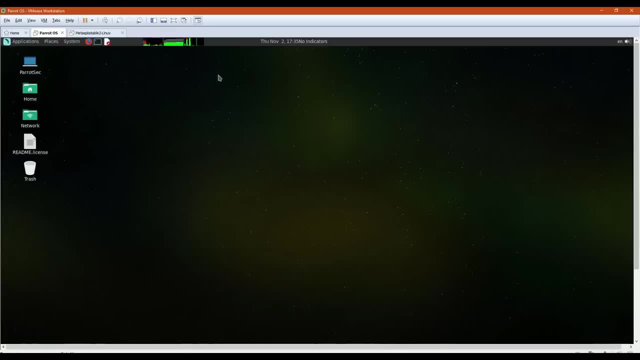 we can use is nmap or zenmap. i would encourage you to use zenmap if you're a beginner, to have a good understanding of how things are displayed. i've always recommended that. so let's move. uh, let's just go to applications, and in pirate os it's in information gathering and zenmap. all right, 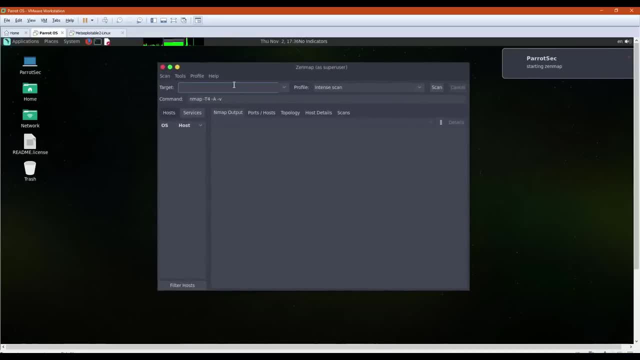 so it's starting up zenmap and all you have to do is just enter the ip in the target again. it can be a local uh ip address or a public ip address and we can just go ahead and use the intense scan. and here are the commands. if you want to use it in nmap, you're pretty much scanning. 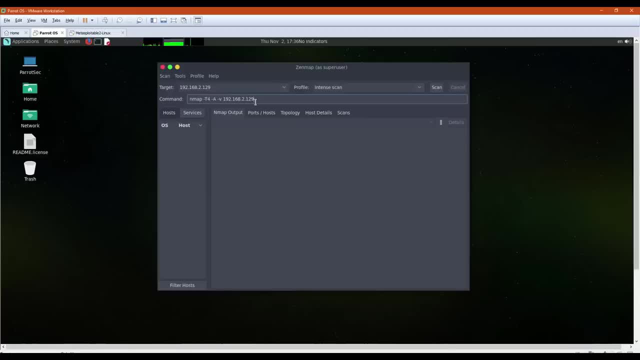 if you're boosting the information, you're getting all the services, uh and the ipv4 information. so if we scan for this, uh, it's going to essentially show us all the what ports are open, what services are running, so you can then move on from there. so let's give it a scan and uh, it'll essentially 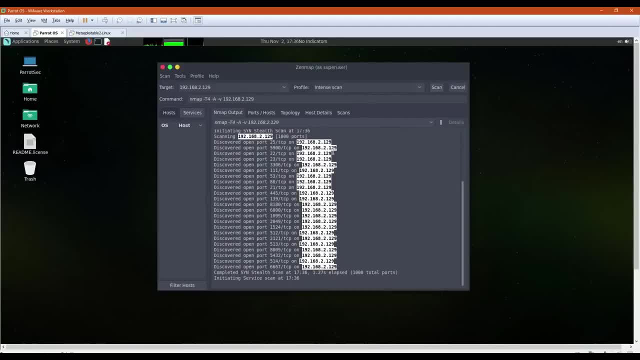 show us what's running on this uh server so, as you can see right off the bat, you have a plethora of awesome ports open here, like if you saw this on a server- of course not a server built for vulnerability. this would be like the, you know, the gold mine for a pen test or an ethical hacker. 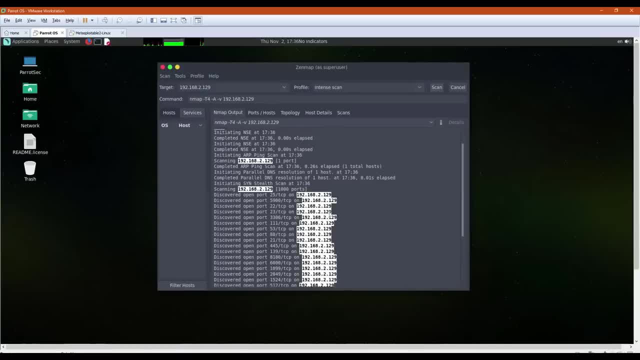 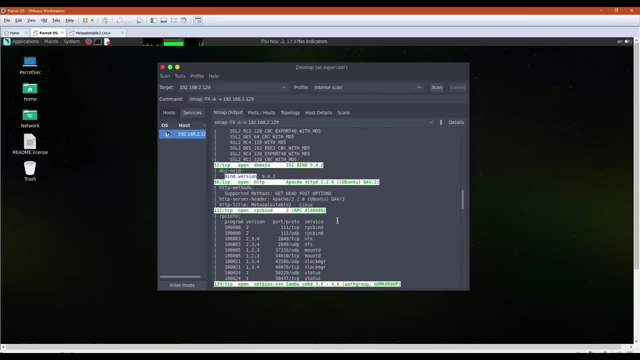 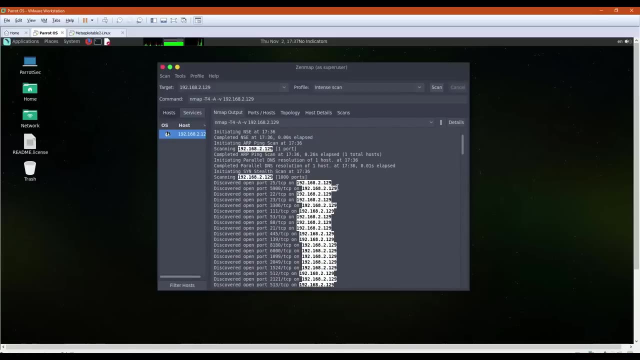 or a hacker for that matter. so, as you can see, you have all your tcp, you have your ftp ports open, which is super to say the least. um, so, as you can see, i believe the scan is done. let's uh see, is it done? yeah, there we go, so you really can just scroll uh. 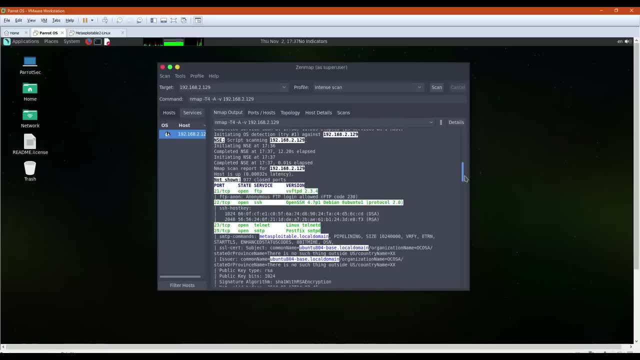 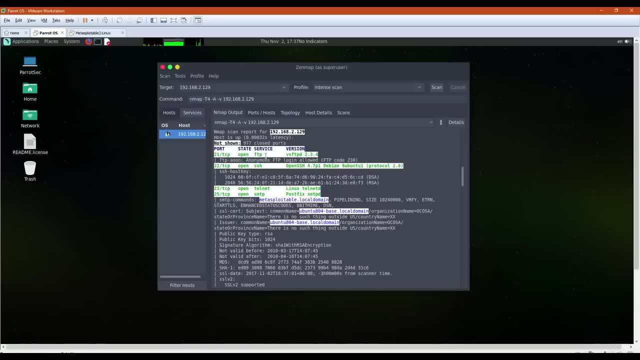 through the, the results that it gives you. and, uh, if you go down here to the port, uh, so there, there we go. so we have, um, it has, port 21 is open, which is, uh, the ftp. i believe it was configured wrongly. that's the way it's designed to be. so with ftp, it means 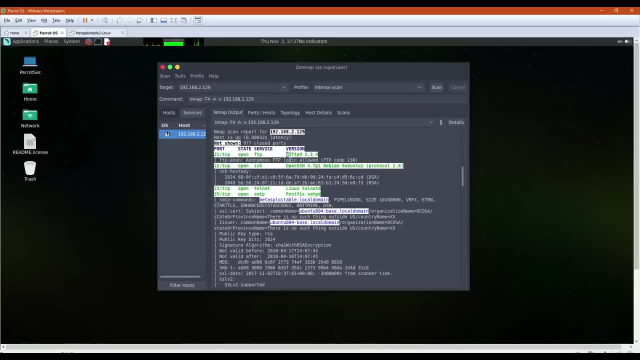 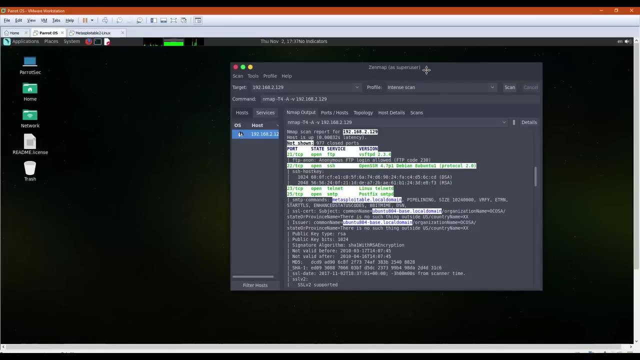 you can basically upload and download files from the server using this software right here, which i'll get to in a second. you then have ssh- awesome, awesome, awesome stuff there. so ssh is essentially secure shell, which means you can connect to the server. all right, granted, you have the username and the password to go along with it. so we can actually try that out right. 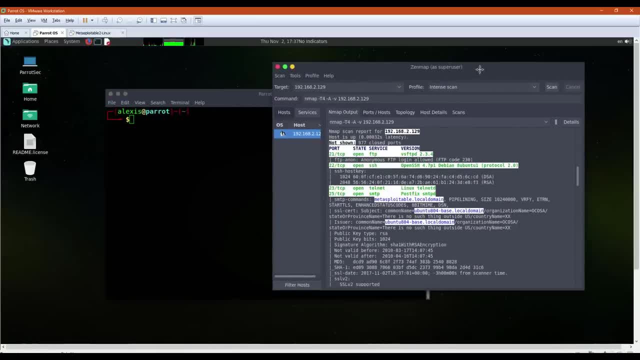 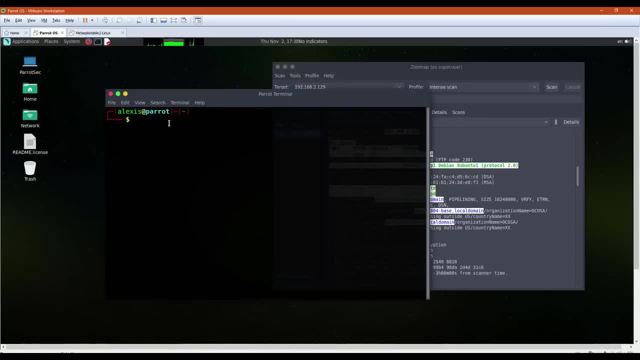 now from my parrotos. so let's say, uh, we wanted to, we, we can see that the ssh port is open and we have the username and password. uh, so what we can do, or if there was an exploit we could use, that would be even better. so i'm going to just use ssh, all right, and the username for the metasploit. 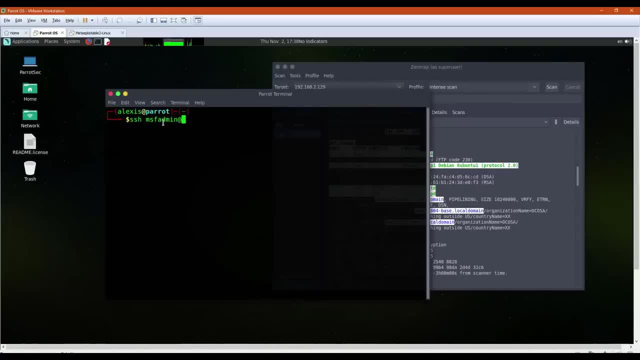 virtual machine is msf admin. all right, at the ip address, which is 192, oops 168.2.129, and that should give us- uh, we don't have to specify the port- the port is always going to be port 22, and if we hit, 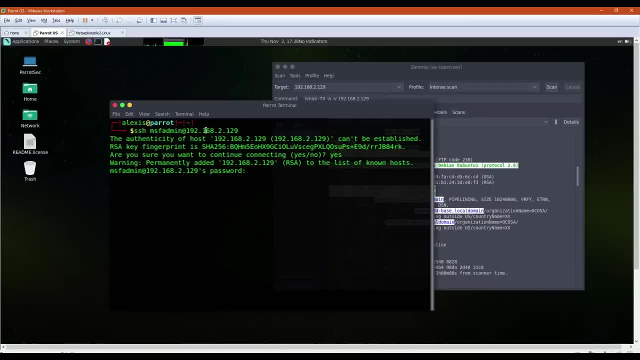 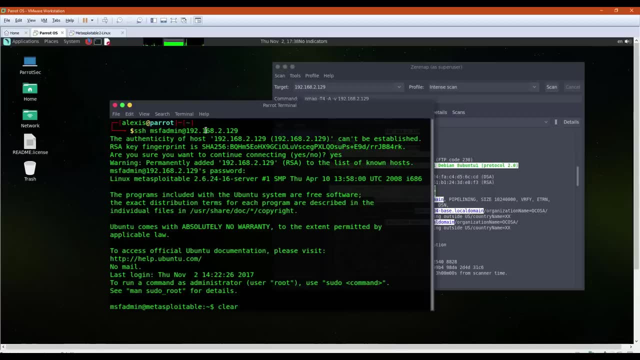 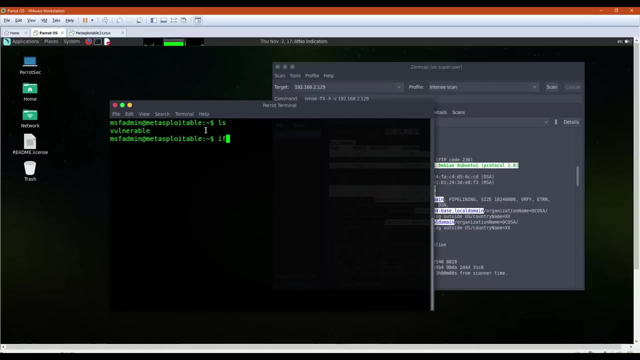 enter. yes, it's going to ask us for the rsa key, and there we are. so the password is msf admin by default. and there we are. we are in the metasploitable machine and we can list the files, and those are the current files, in there. we can also, you know, view the ip address if we wanted. 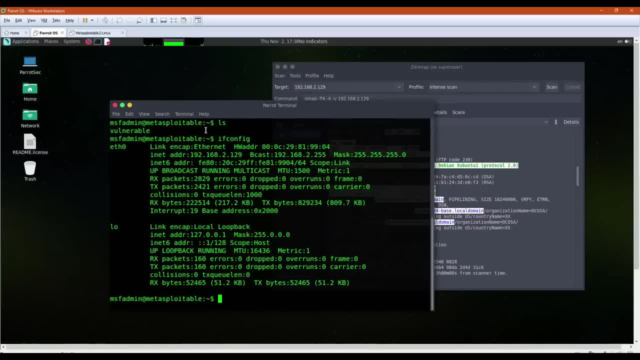 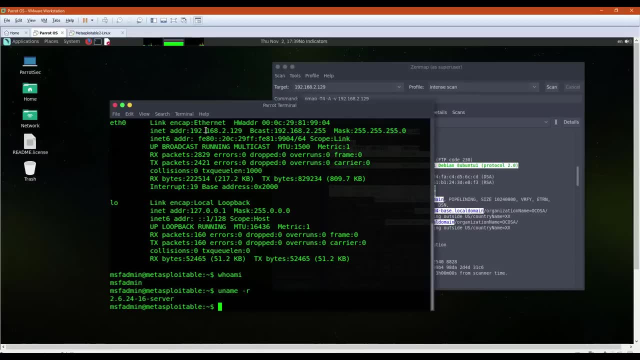 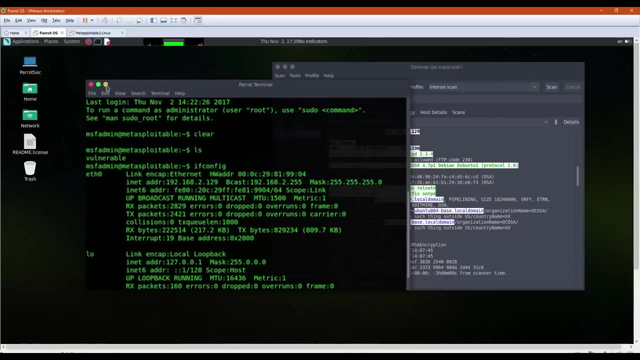 to like. so ethernet. uh, there we are. that's the ip address. uh, you name uh r and there we are. that's the server. so awesome. so that means we can actually- uh, you know, go through ssh. but, uh, again, some of you may be saying, yes, it is vulnerable, uh, and i 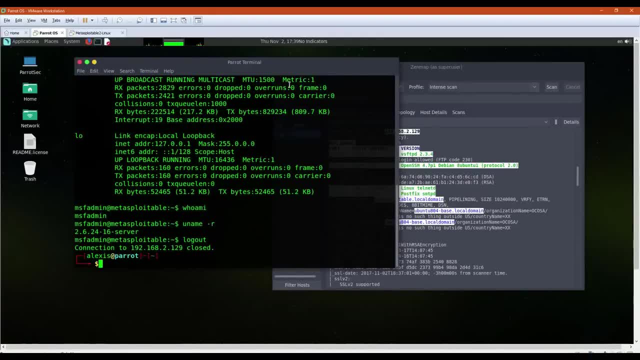 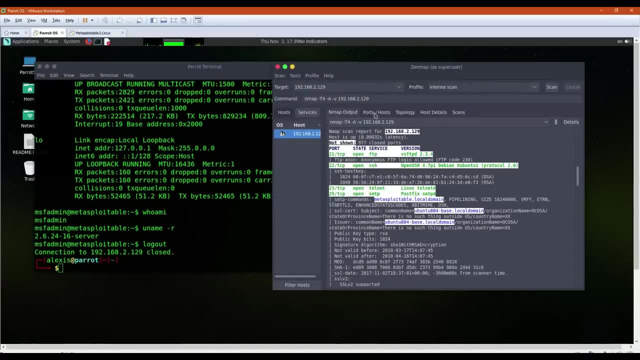 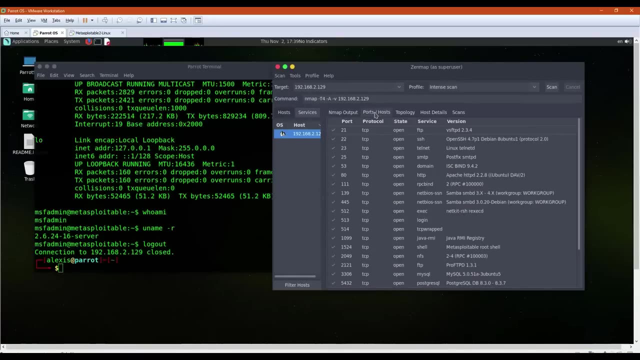 understand that. i'm just showing you how one would approach it. so let me just log out of the m, the metasploitable machine there, and if we go back here again, you can just move on to the ports and hosts tab right here and it's going to show you all the ports with the services that they're running. so uh, for the ssh. 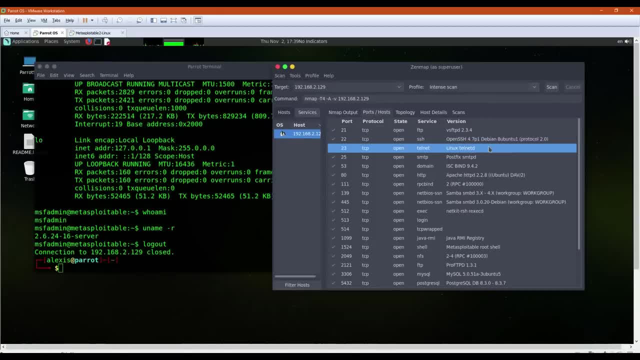 port. you have debian. it's based off debian. you have your telnet, which is just, uh, a shame at this point, you know, because that is, it can easily be cracked. you have your samba web servers- uh, what else do? you have metasploitable root shell. we're going to be looking at that. so we have mysql. 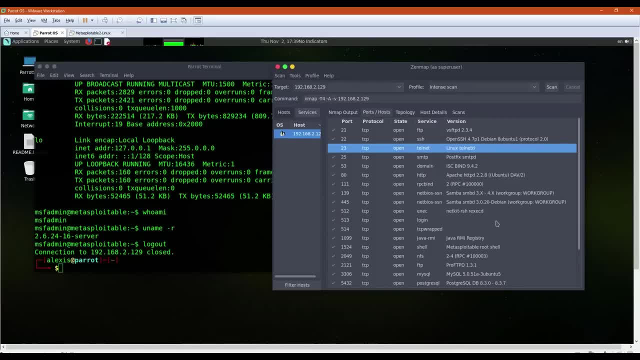 databases. so this is really, uh, metasploitable, is really an operating system designed to be, uh, based off of the ssh port, and you can customize how vulnerable it is to test your skills. now, the, the. the essence here, uh, or what i was getting at, is, as you can see, with the information that we have, 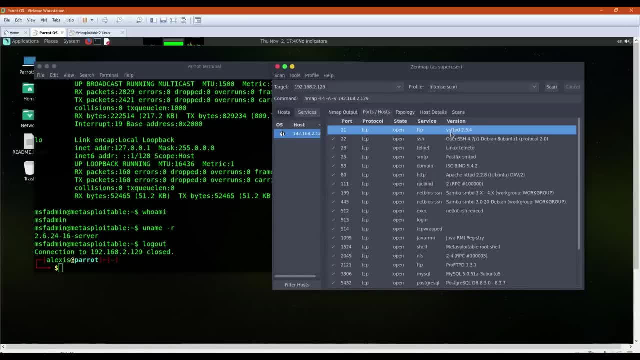 gathered already, we can perform a plethora of attacks. now we have this: if ftp server here and uh, what a hacker would do in this case is he would look for an exploit for this software or for the service that it's running. in this case, it's using vs ftpd. all right, which is version 2.3.4, so we can. 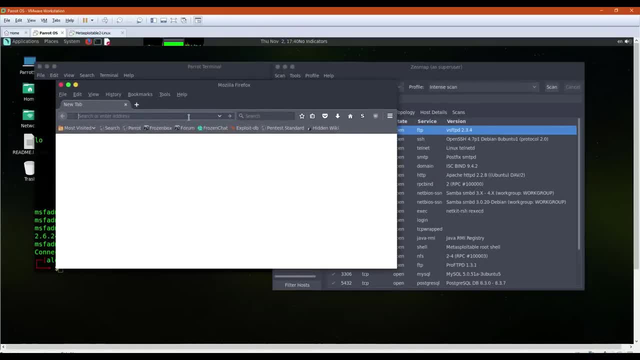 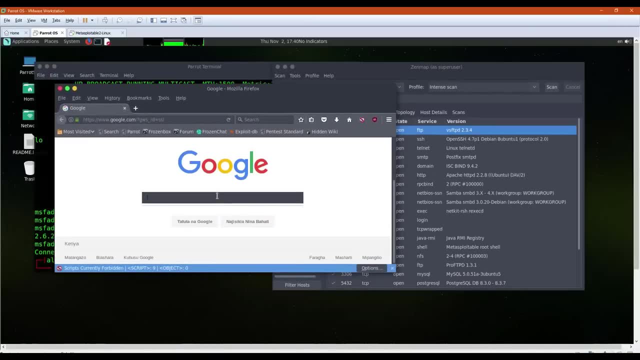 actually just google it. it's as simple as that, you know. so we can just google. uh, we can just google it. i know i don't encourage you to use google, but you know, yeah, we're not doing anything really dangerous right now. so vf, uh, vsf, vsf, t, p, d, 2.3.4. uh, let me just change that back to there we are. 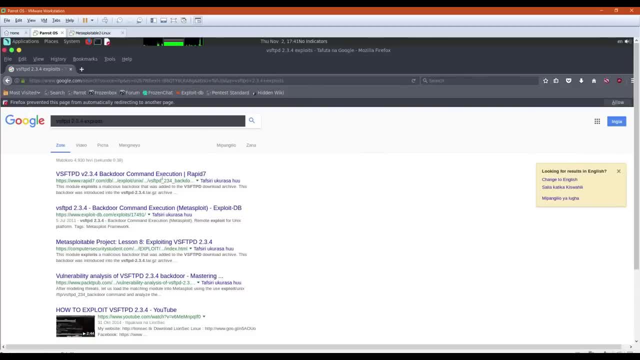 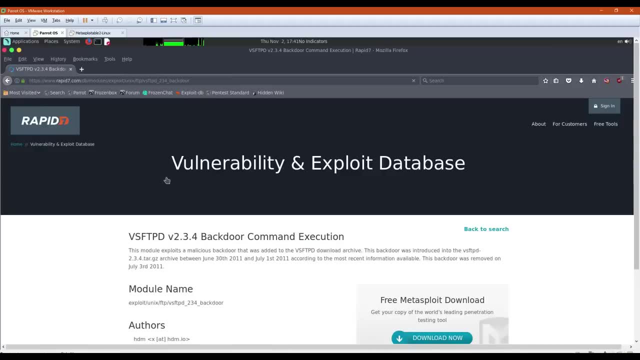 right here. so we have, uh, the vf2.7, uh. this means that, uh, we're using vf2.7, uh, but we're not using vf2.7, uh. and uh, how do should i? how should i set it back up, vf2.7? i mean, vf2.7 is actually. 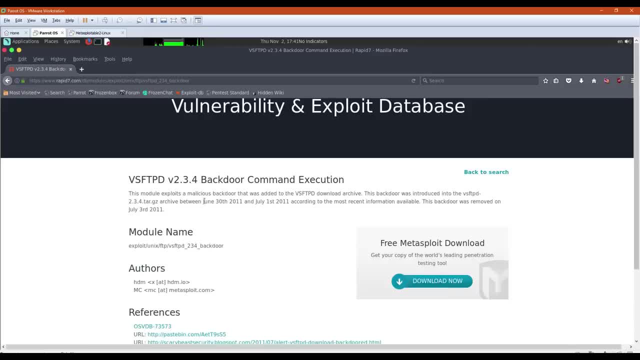 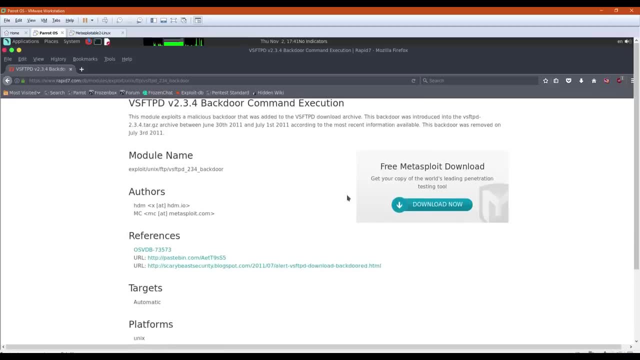 a game which is a kind of a common model in popular companies, uh. so we can just say: uh, vf2.7 was uh, one of the uh, one of the main uh, uh, uh systems that vf2.7 is needed for in to use. as you can see here, vf2.7 is a type of vf2.7, which means that when you are заявing: 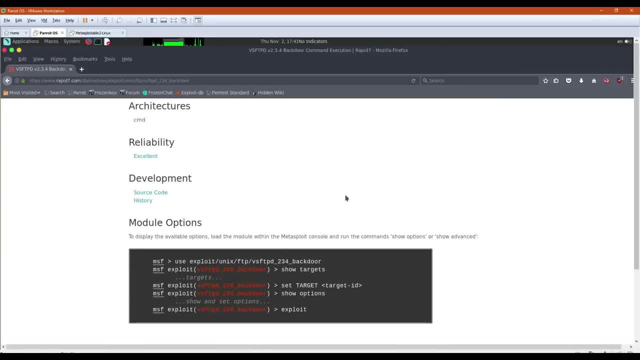 the vf2.7 in your machine. you will be out of the game when you are saying that we are not going to use vf2.7. awesome, now again, this is going to be using the. you're obviously going to be using Metasploit, right, so you can go ahead and start using Metasploit for. 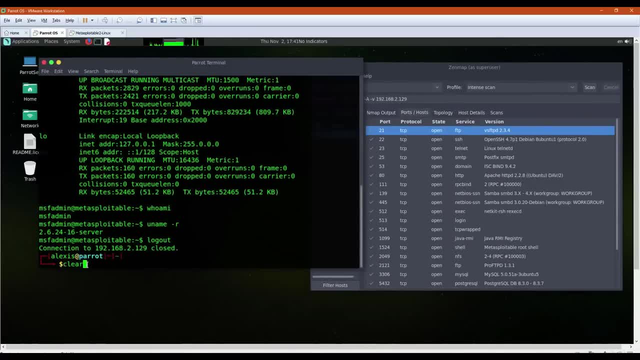 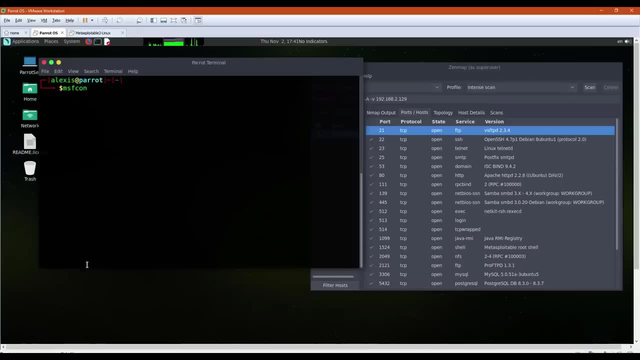 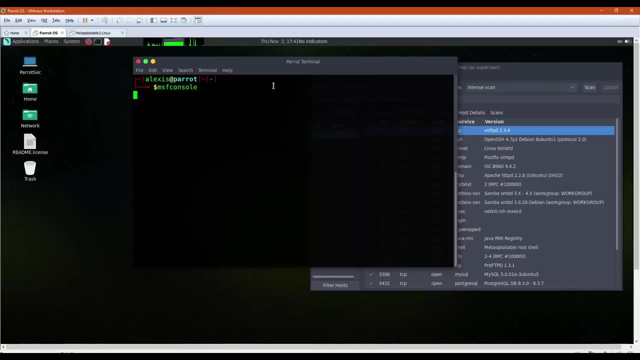 that, but I want to keep that for a later video, because Metasploit really deserves its own video for exploiting AV server. or you can actually just try it right now, msfconsole, and it really gives you all the information you need in terms of the exploit. so just let it start up again. this is one of the things. 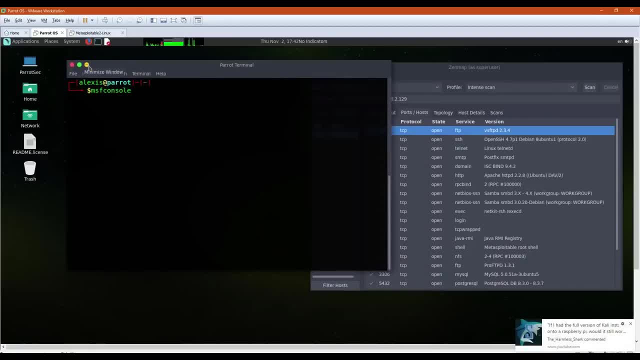 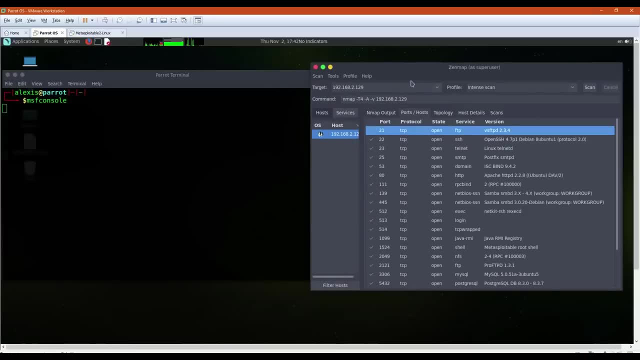 I was trying to avoid the startup on. this is always a long time and we got another notification there. let me just clear that out. but essentially what I'm trying to put across is here is: it's really, really important that you have good information gathering skills. again, you have your HTTP server port open and 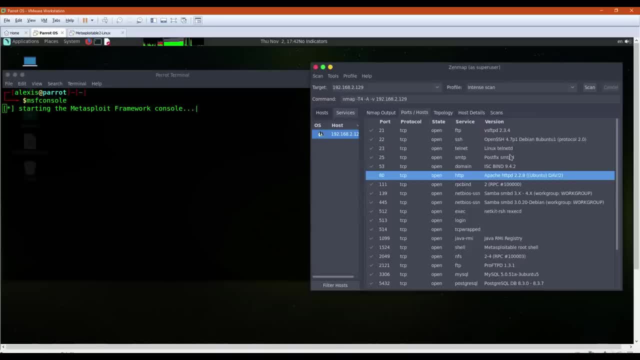 that's running Apache. so again, Apache exploits. go ahead and search for that. even if you don't know how to do that, just go ahead and search for that and find one. you can use Metasploit, which is what most people would use, or they will try and connect through SSH, but many people want to install a backdoor for. 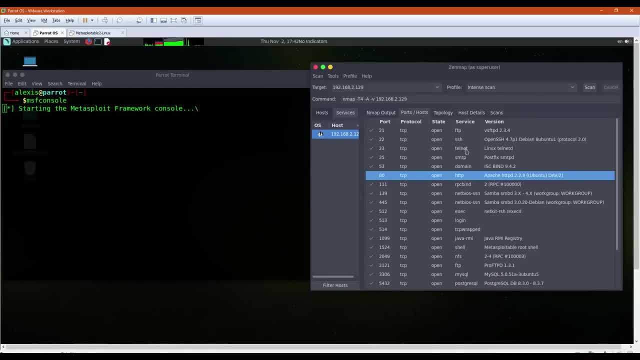 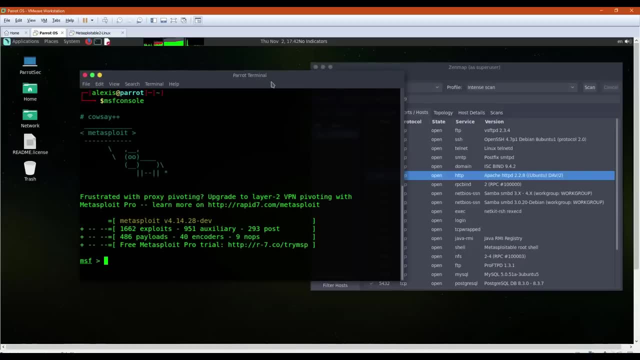 example, or find remote code execution, or reverse shell, etc. etc. things like that. but that's a basic way of gaining access to a server. now I know it's not the most advanced way, but we'll be moving on to using things like Metasploit and stuff. 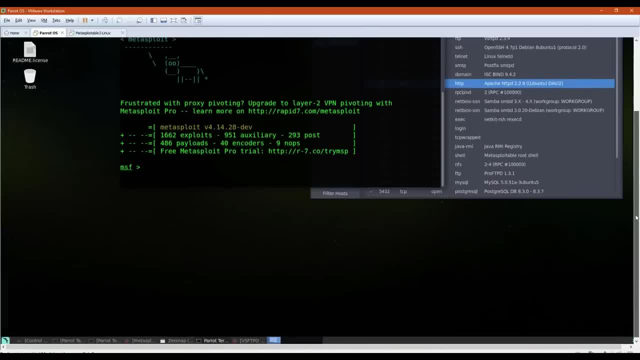 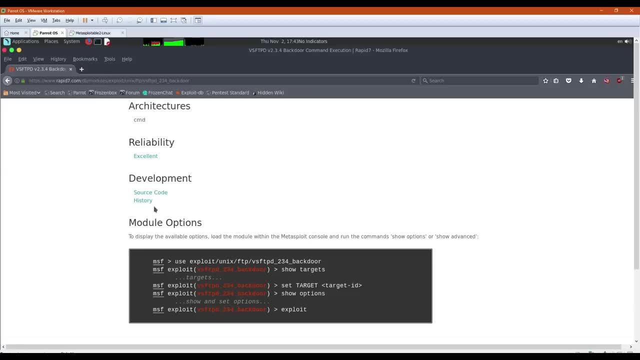 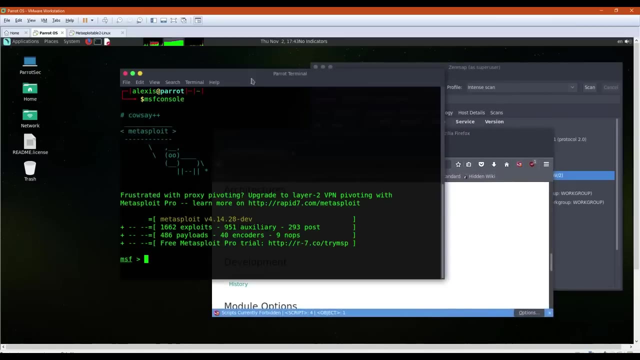 like that. but in the meantime we can actually just try and use this. let me just go back to my browser here. so use exploit. I don't want to type this right now. that judge it will just be wasting time for you guys as well. so I'm just going to use the exploit that it's saying here. so Metasploit knows. 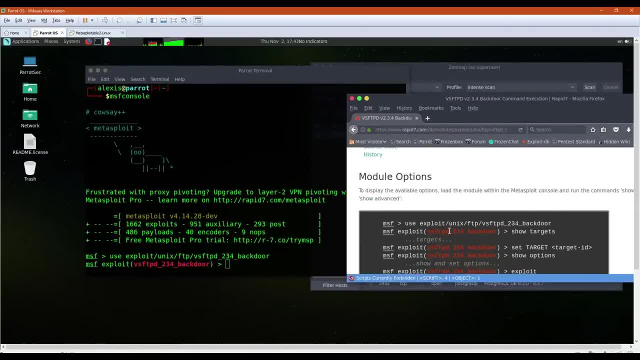 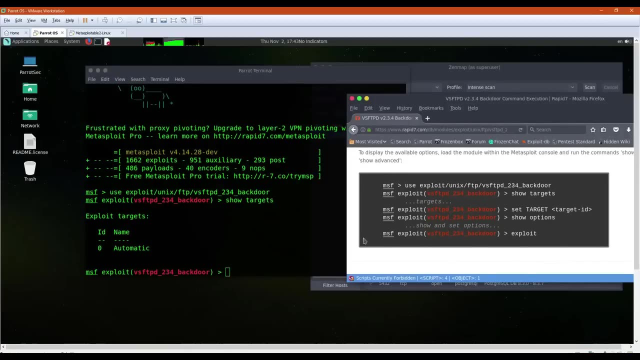 what exploit we want to use. so there we are, it's recognized it. so now we want to show the targets. show targets ID name- nothing there right now and you can show options or, but first obviously you have to set your target ID. so let's first show the options for some. 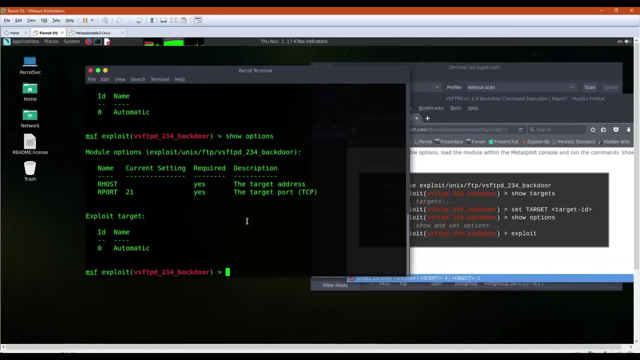 of you who know how to use. so let's set target, set target whoops, set target, this the target address, and we put it in there. so two point one sixty eight point two point one twenty nine, I believe that's it the target, and we can then 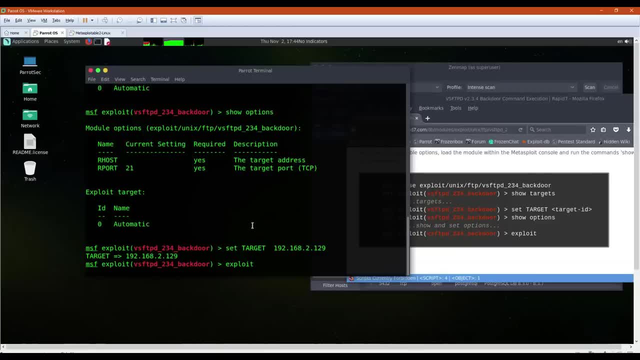 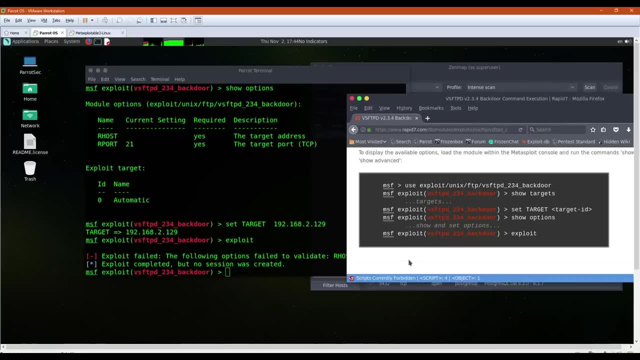 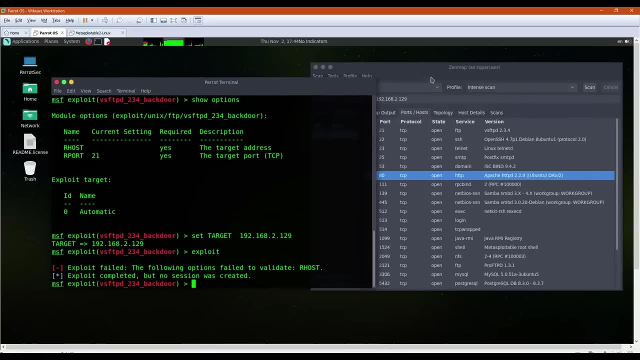 finally exploit it. so let's run it and let's see if we get anything in return. there we are: exploit completed, but session. but no session was created. I'll have to look into that, but anyway, you guys get the idea. I really didn't want to put emphasis on Metasploit right now. there's a lot of other much better. 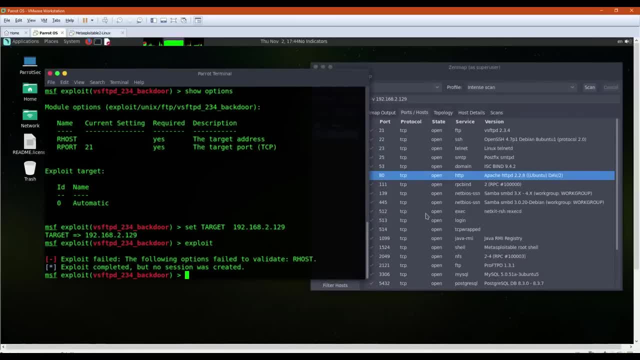 exploits that you can be using, especially when looking at web service. we'll be configuring the Metasploitable machine to be a bit more secure so we can actually test our skills more effectively. anyway, guys, that's going to be it for this video. this is just going to be one video in the series of gaining. 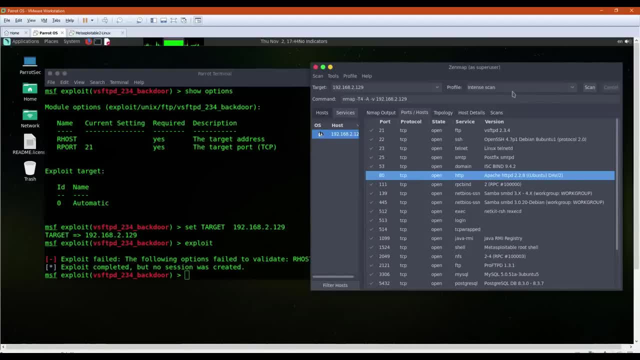 access, whether it be server side or client side attacks. I hope you guys found value in this video. if you did, please leave a like down below. if you have any questions, let me know in the comment section or you can hit me up on my social networks. if you have any personal questions, you can hit me up on kick. 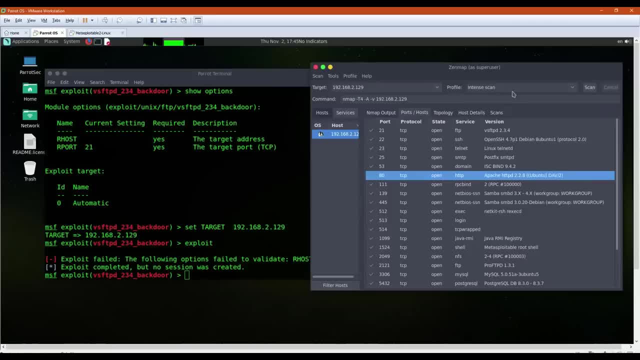 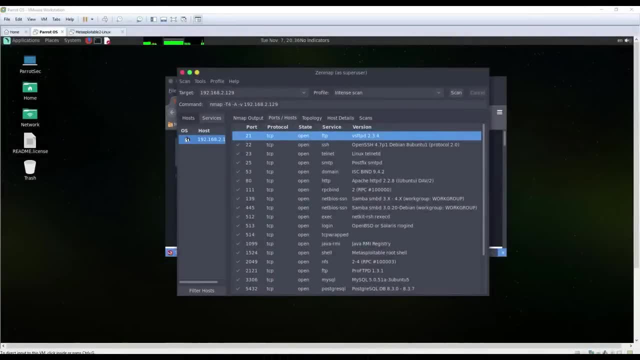 for the latest hacking news and resources, check out my website link will be in the description, and I hope you have a fantastic day. peace, hey guys. Hackersploit. here back again with another video, and in this video we're going to be continuing where we left off, where I'm going to be showing you how to 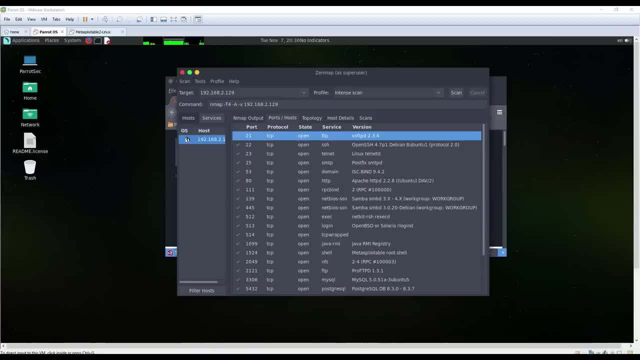 use Metasploit to run an exploit on a service. in this case, we're going to be using Metasploitable and we're going to be exploiting the FTP port so that we can upload and download files to and from the web server. so let's get started. so in the previous video I actually I showed 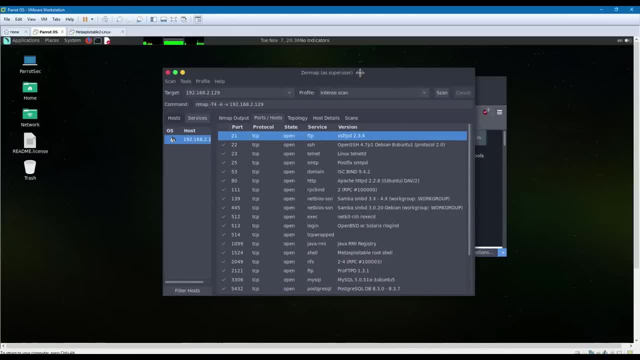 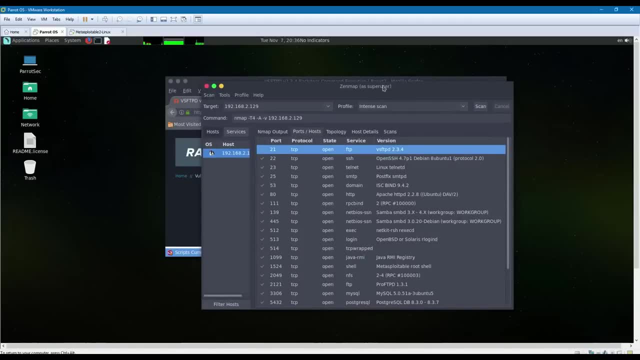 you guys how to set up or how to use Metasploitable to basically exercise or test your skills in exploiting. so essentially what we did is we scanned the IP address, the local IP address- for Metasploitable, and we essentially gave it an nmap scan to find out what services were running and the ports that 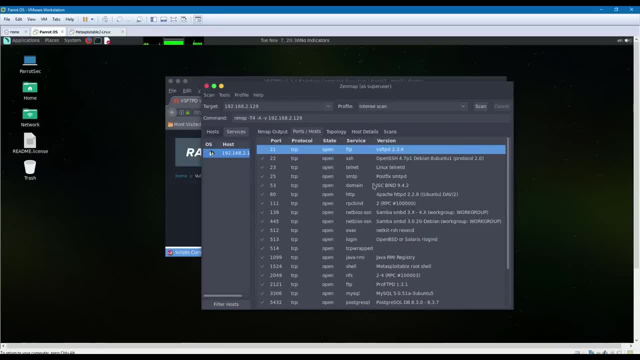 we found that were open were obviously going to be all the ports, and that's because Metasploitable is configured to be that way. so the main thing that we're going to be doing now is I'm going to show you how to run an exploit on one of 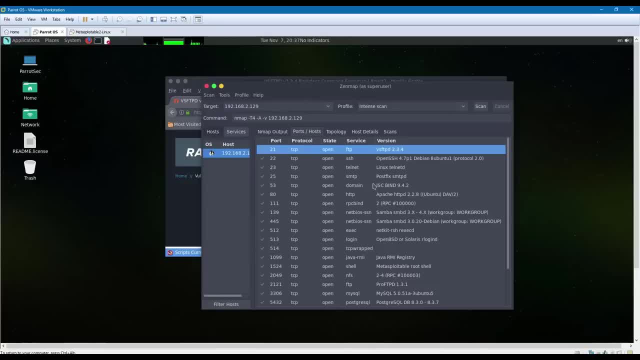 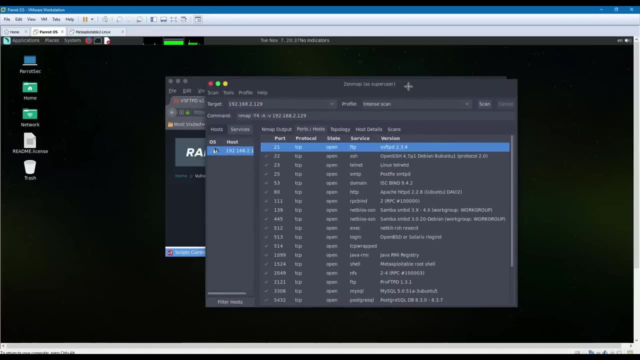 these services, more specifically the FTP service, because a lot of you guys thought that I didn't know how to use Metasploit. I just breezed over it because I wanted to do that in this video. so we're actually going to be using Metasploit in this video and I'll show you how to use it. so let's get. 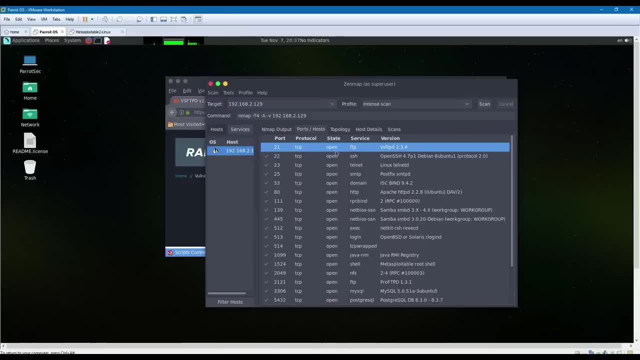 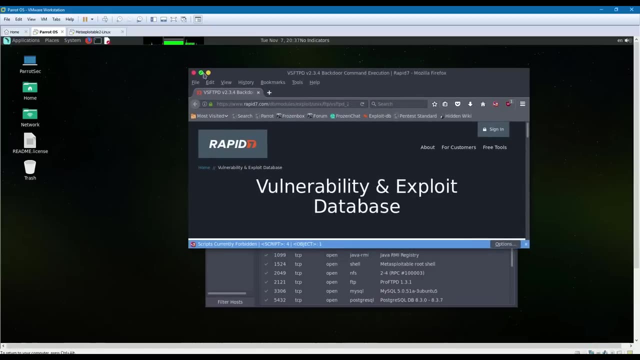 started. so we know that the port that we're setting is the FTP port, which is port 21, so we know that it's configured correctly. now the service that it's running, or the service version that it's running, is vsftpd 2.3.4. so what we did is we googled this service to find. 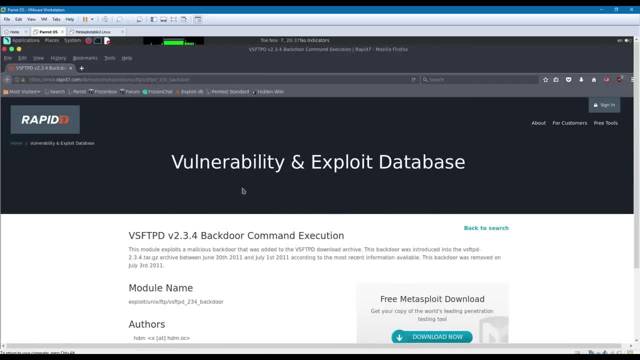 exploits. for it again. you can use any other website to search for exploits, any search engine. many people like to search on exploit DB or exploit database, because that's where you'd find most of the exploits. so I found the exploit on rapid7.com. now, rapid7 is the company that 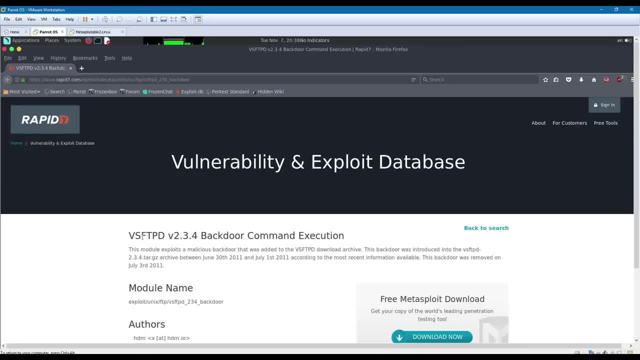 develops Metasploit and they essentially have an exploit for this service, which is vsftpd, which is the FTP service for the specific version 2.3.4, which the exploit is a backdoor command execution which allows you know commands to be executed a bit like what you would have in a reverse shell, and 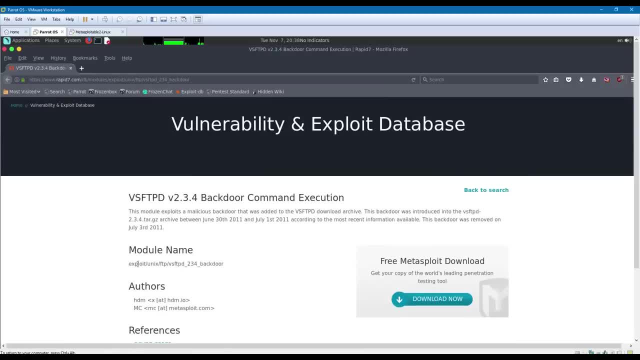 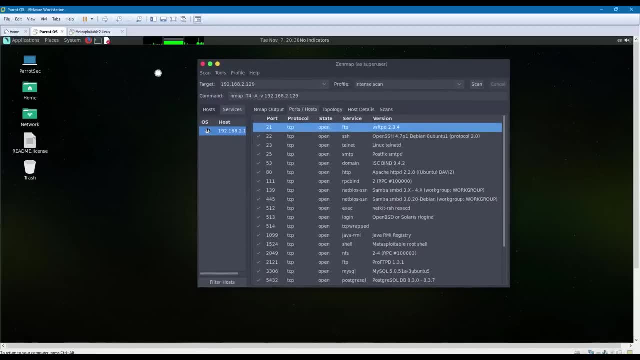 so what we're going to do is we already have the exploit here, the module here. so when talking about Metasploit, which is what we're gonna be using, not Metasploitable now, let us just start it up. so, to start up, Metasploit you. 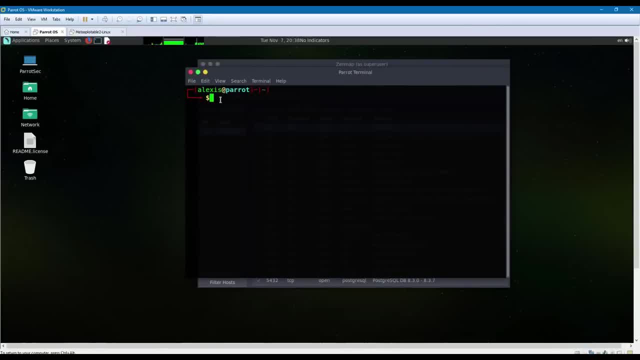 just open up your terminal again. I'm running Parrot OS. it really doesn't matter what pen testing OS are using, so MSF console. alright, MSF console, and just give it a few seconds to start up, and that's it. uh, it shouldn't take too much time and we should be good to go so while that's starting up. uh, let. 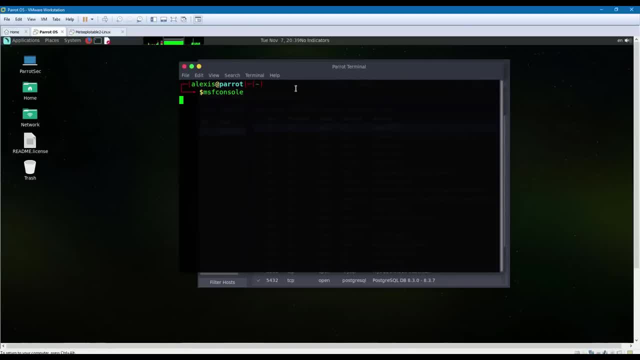 me explain what metasploit is. all right, metasploit is a large database of exploits, all right, and it essentially allows you to use these exploits to your advantage and to exploit systems. now, whatever you systems you try and exploit, that's up to you. but the cool thing about metasploit is it allows 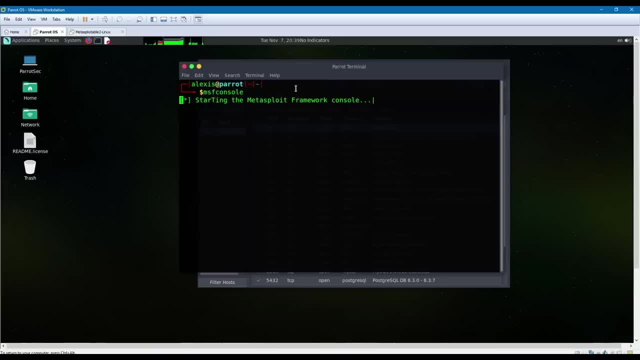 you to create your own, your own exploits, which is awesome. so if you're an advanced user and you actually- uh, you are working with websites or services most of the time and you find vulnerabilities, you can create an exploit, uh, for the purpose of security and patching. so that's up. 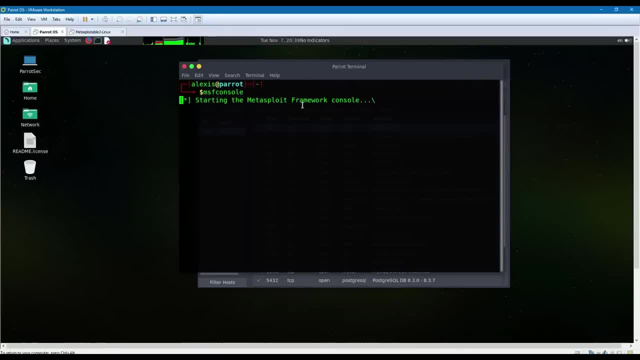 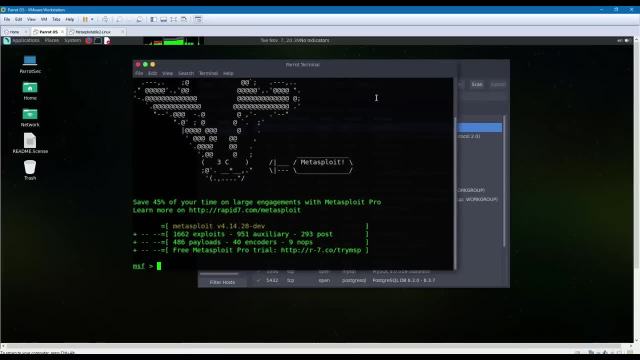 to you. so, as you can see here, it's going to take a while. it's going to start the metasploit framework console and we should begin there we are. so, as you can see, metasploit is pretty pretty, uh simple to navigate. you have your information, um, so it's it's telling you to check out metasploit. 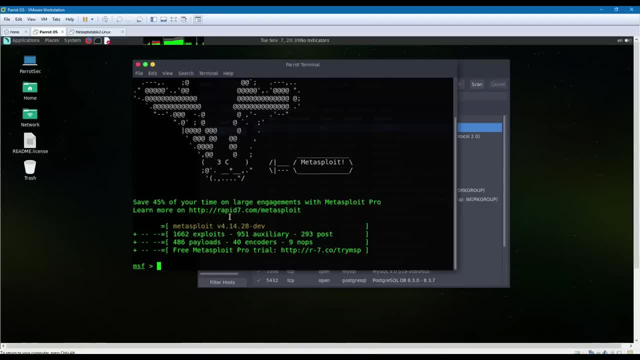 pro, which is a very good option if you're going to use this tool a lot. uh, in terms of the other information, we have 1662 exploits, which is pretty awesome, and yeah, let's get started now. uh, pretty much, there are a bunch of commands that you have to be familiar with with metasploit, and one of 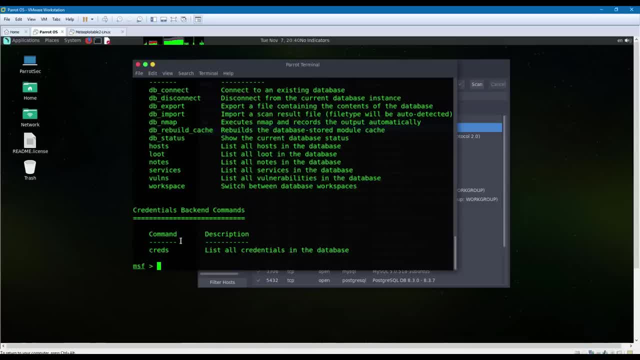 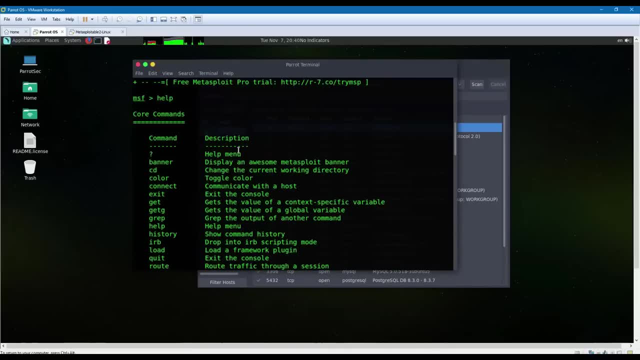 them is obviously the help command. so if we type in help, it's going to give us information or help, really. so this is essentially the user's manual. now i'm just going to tell you a little bit about it and then i'm going to show you the most important commands that will really, really help. 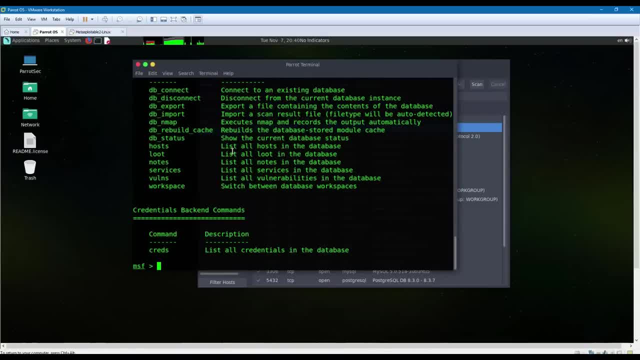 you right now. so the most important commands right now are the- uh, obviously the msf console command, which will start metasploit for you. you then have the use command- right, so that's as simple as that- which allows you to use an exploit, right. you then have the show command, the show. 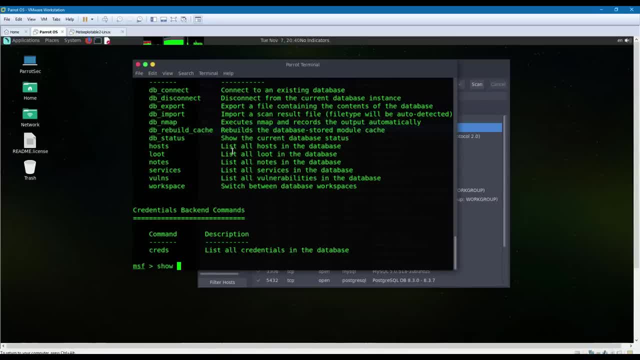 command allows you to show the exploits or the options available for the exploit. all right, you have your set command. your set command allows you to configure an, an exploit or an option, and you have, finally, your exploit option, which essentially makes you run the exploit that you're currently. 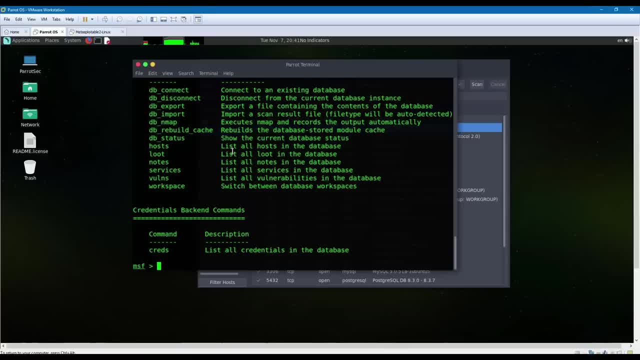 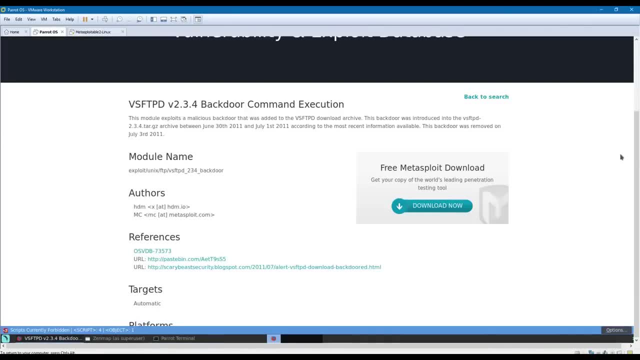 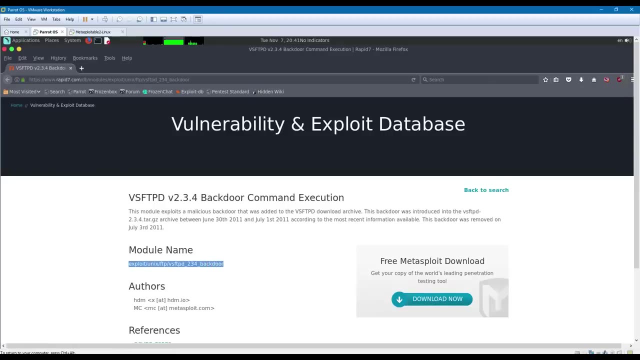 that you currently want to run. so it's really very simple. now what we need to do is we need the- uh, we need the name of the, of the exploit. in this case, the module name is right here and it'll just give you in the form that you need it. so just copy this, because this is the name of the module. 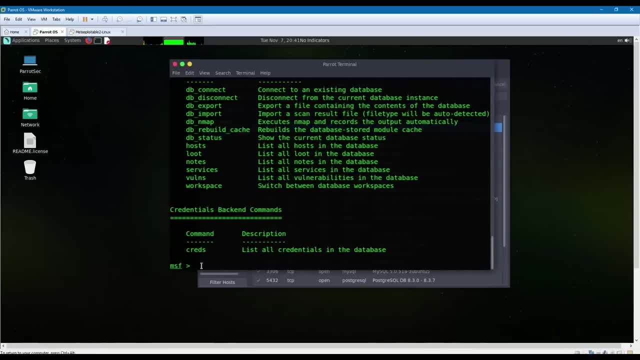 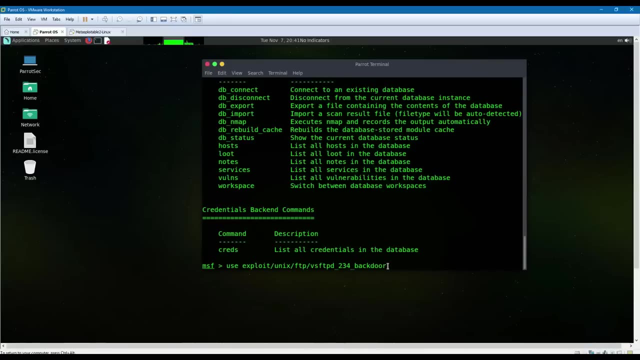 or the exploit for this matter. and in metasploit, uh, what you want to do is just type in use, because that's the exploit that we want to use, and just paste in the name. all right now. uh, let me just minimize this, that could be a distraction, all right. so once we have hit that, uh, well, just hit. 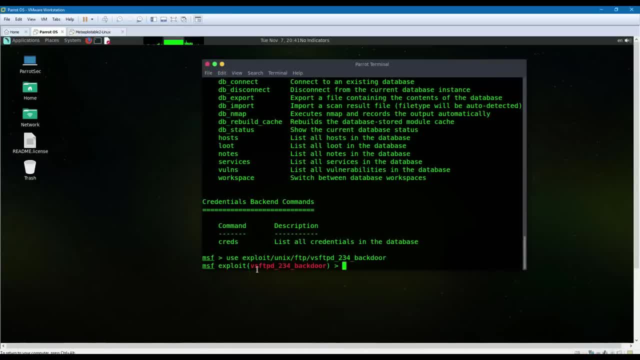 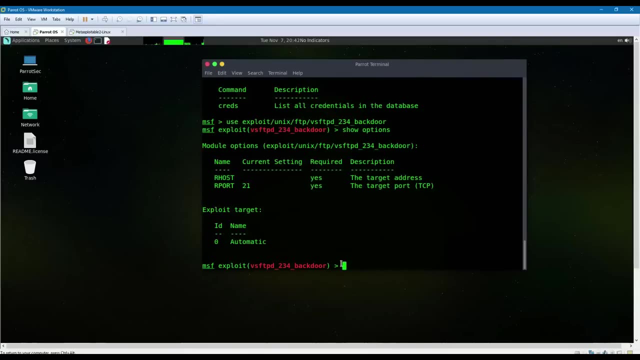 enter and, as you can see, it's going to automatically detect that, uh, you know that this exploit is, and it is, a valid exploit. uh, now, what you can do is you can show the options. all right, so show options and, essentially, this will show you the options that you can change and configure. 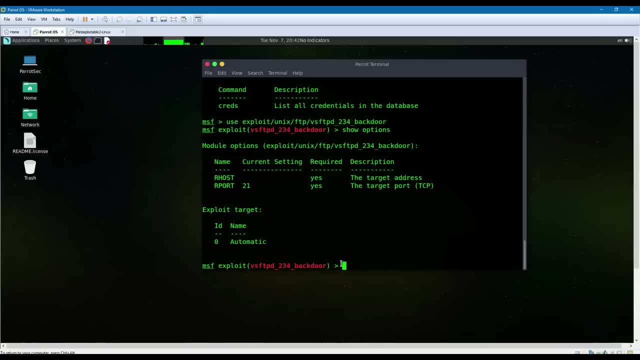 according to what or how you want the exploit to run. now, in the previous video I touched upon this very lightly and you guys thought that I changed, uh, the things incorrectly and the reason being is I did it really really quickly and my job was not to actually show you the exploit. but let's do it. 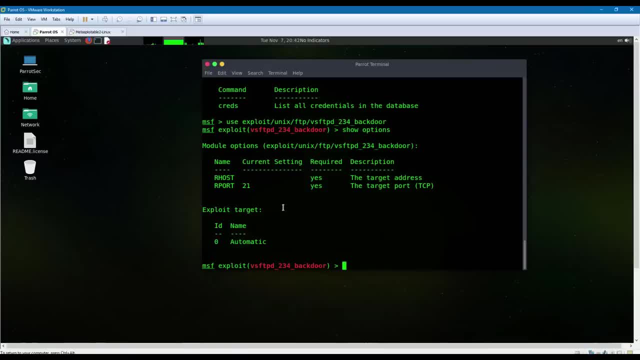 now, uh, what we need to do is we need to understand a few things. first, the R host is your, is the target address, all right, and the R port, which is already configured to 21, is correct because we know the port is configured correctly. if it was configured to something like port 22 by mistake, that could 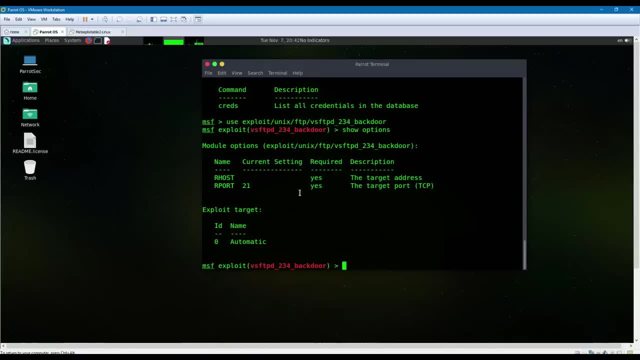 also be, uh, something that you need to change now, to change the R host to what we want, which is the IP of the metasploitable machine, the machine that we want to exploit. in this case, we need to, uh, essentially say, set our host, all right, so set our host and we use the IP, so 192.168.2.129. 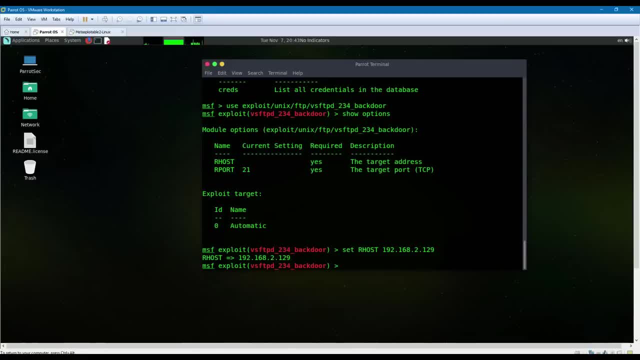 all right. and if we set that it's going to say our host is equal to, and now we can essentially just check, we can say show options to make sure that everything is configured correctly before and our port is configured correctly because, as I said, uh, the port that we're trying to target here, 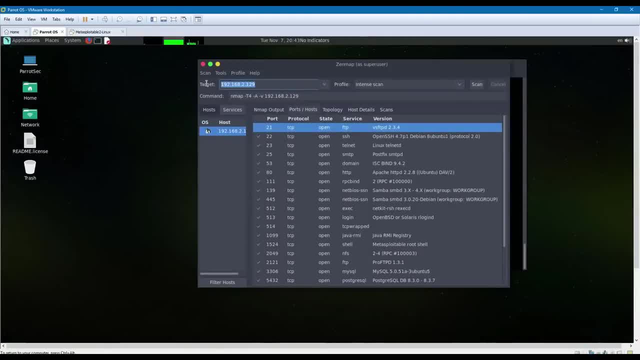 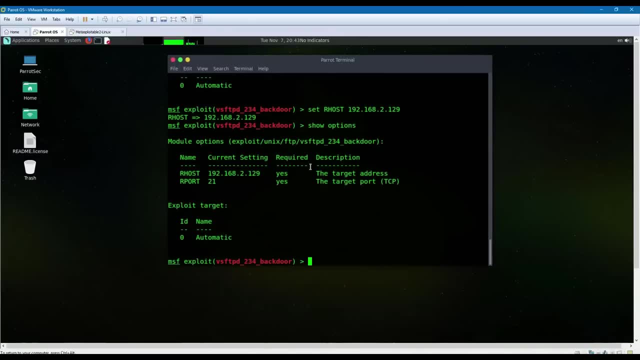 is, is going to be port 21 and the IP address is right there: 192.168.2.129. and again, you can ping yours to test it if it's still running. and yeah now, uh, what we can do now is all we have to do. 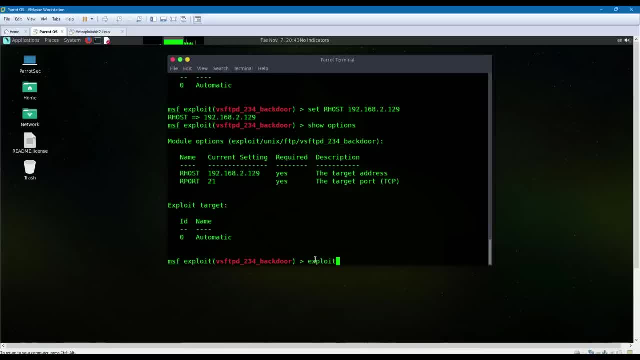 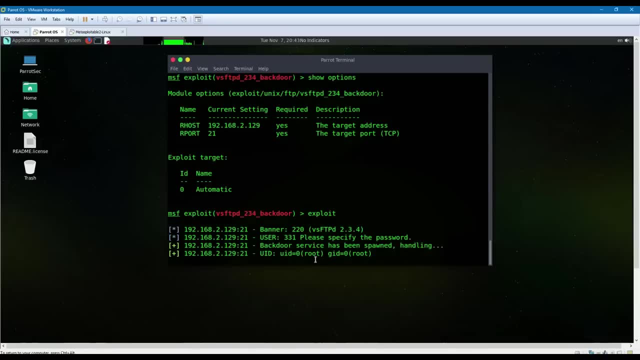 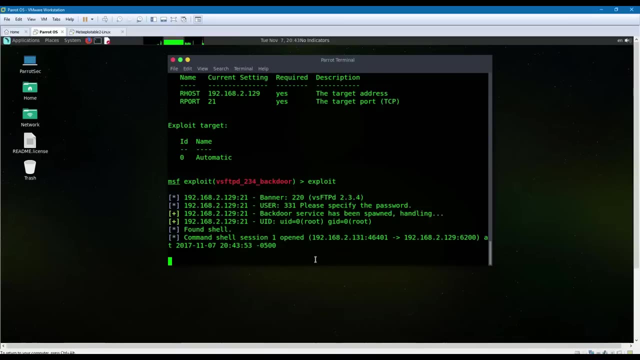 is say exploit: right, as simple as that. and we hit enter and let's see what we get, all right, and there we are. so it's uh, going to start the banner capture and it's going to say: command, shell session one open. so it's opened a shell session, which means this system is Linux. 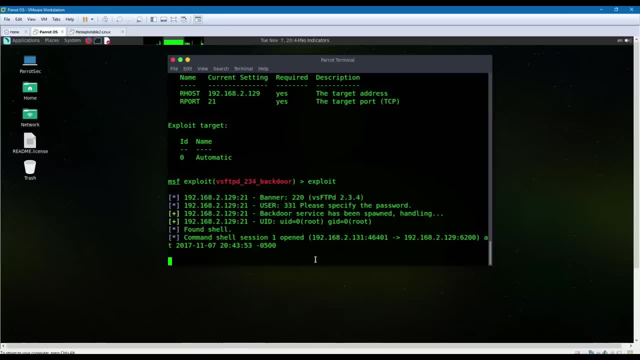 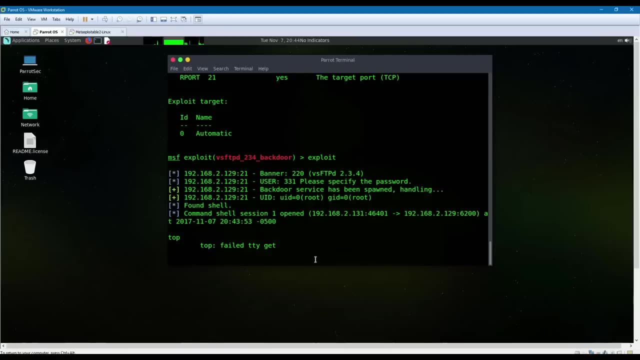 obviously, and we can run our Linux commands. so pretty, pretty awesome. and, as you can see, we can send commands back and forth. so let's try a few commands, let's see if we can run a task manager. uh, whoops, we did not. I don't think that's installed on the metasploitable. 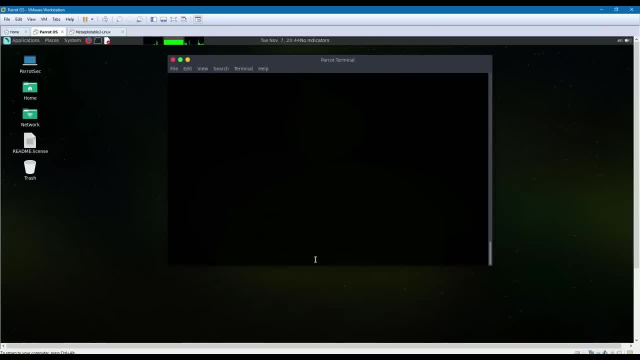 machine. um, let's see if we can run the clear command there we are awesome. so now we have a clear uh, bash or shell, sorry about that- and we can try something like you name are, uh, whoops, you name are, and uh, there it's going to tell us the server version. you have, your, you name a, and there we are. 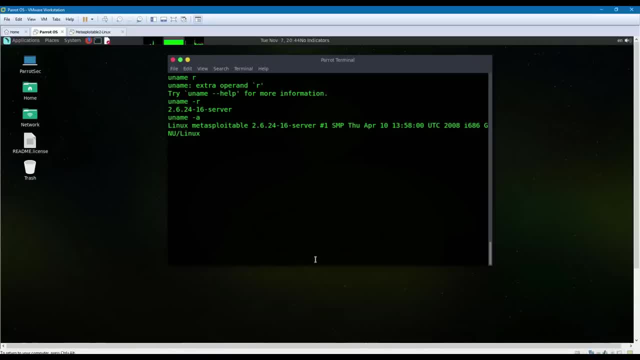 Linux metasploitable, blah, blah, blah we. then we can also list all the files available and uh whoa, there's a lot of files in there and I guess you guys can see the power of this. if you have a server that has this vulnerability, depending on the service that it's running, you get the idea. it's very, very powerful. 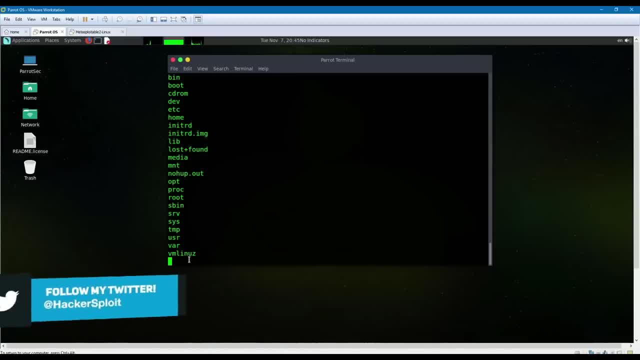 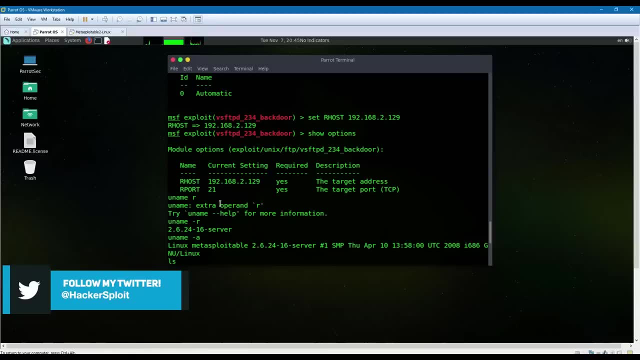 and you can run a plethora of commands, you know. so it's. it's pretty, pretty awesome. uh, that's going to be it for this video, guys. a little bit of a short video, but this is a very uh important introduction to metasploit. it's. what's not important is the fact that we're using a simple 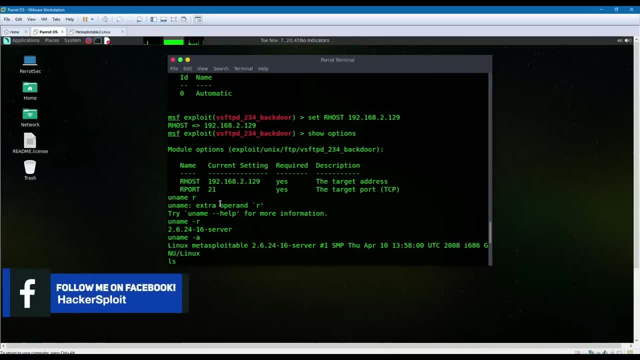 exploit. it's very important that I'm showing you guys how to use it and how to get comfortable with it, so I hope you guys found value in that video. if you did, please leave a like down below. if you have any questions or suggestions, uh, let me know in. 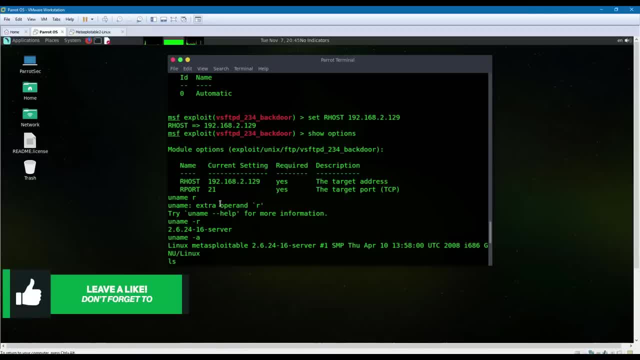 the comment section down below or you can hit me up on my social networks, um, the links will also be in the description. if you have any personal questions, uh, you know, hit me up on kick for the latest hacking news and resources. check out my website link will be in the description and have. 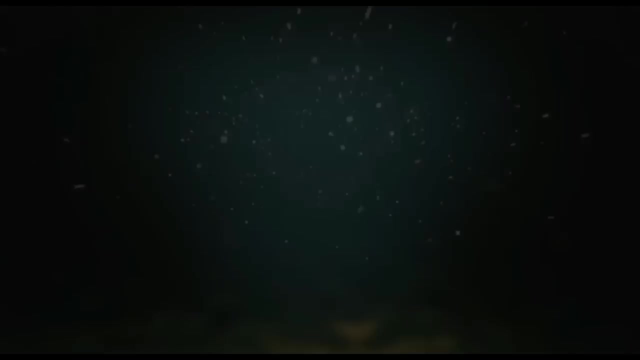 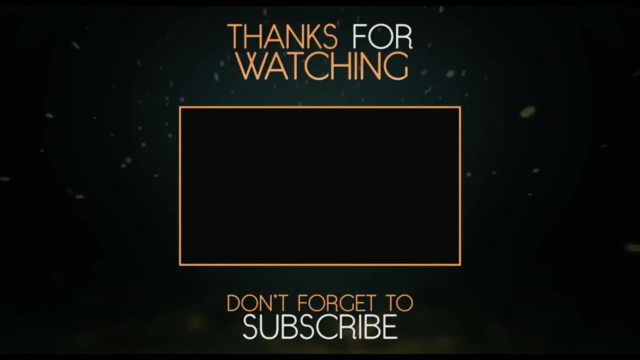 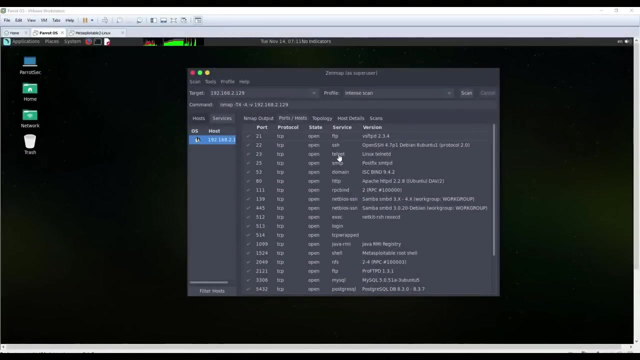 a fantastic day. peace continue. hey guys, hackersploit here back again with another video, and in this video we're going to be looking at a web server hacking. so we're going to be continuing where we left off and this time we're going to be trying to exploit the port 139, which is the Samba. it's running the Samba. 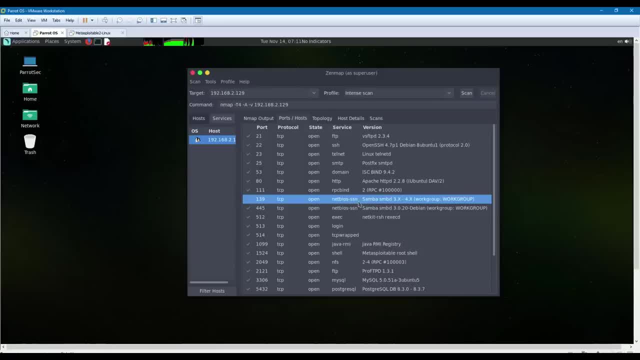 server right here. so again, we're going to be scanning our metasploitable machine, so go ahead and do that, if you have not already, and once the scan is complete, we have some open ports. now, of course, in the previous videos I've made, many of you have said that this is- uh, you know. 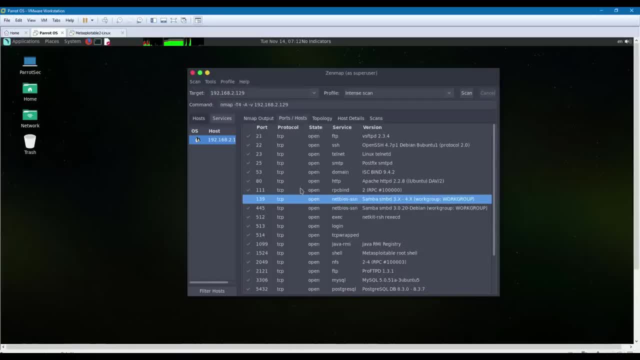 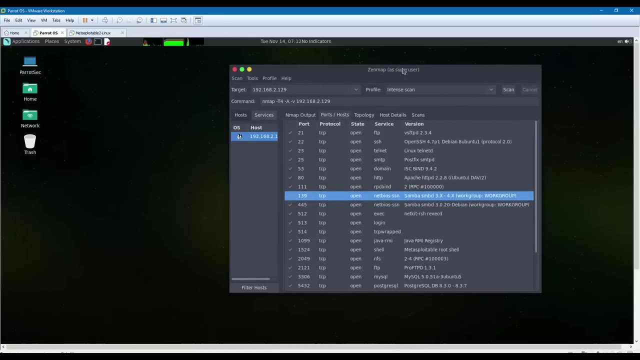 that, uh, this is basic stuff. well, the the reason I'm using this. I'm showing you the different ways of using metasploit in in different ways whenever you have uh, for example, a very unique uh exploit that you want to use, and one of the most unique ones is the Samba server. all right now, rapid 7. 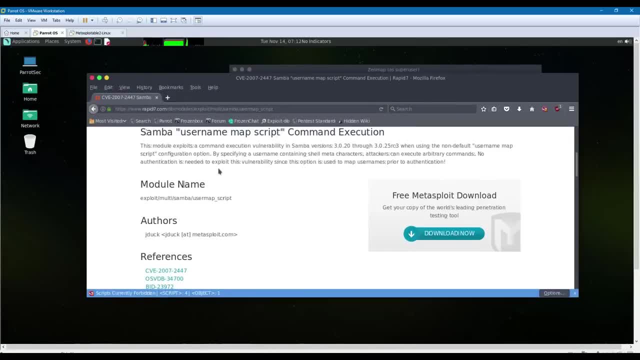 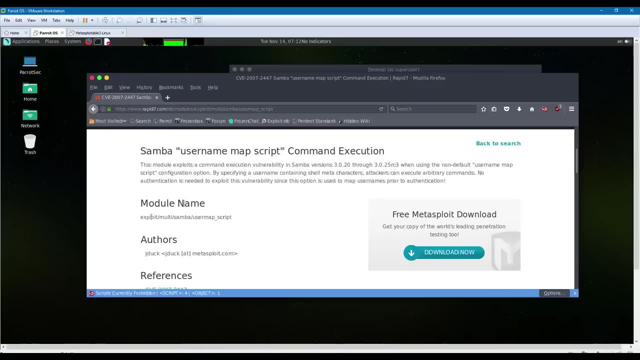 exploit has this vulnerability with the Samba. it allows a command execution without authentication, which is awesome. so what I'm going to do is I'm just going to be using metasploit and I'm going to show you something really unique about this. now, this exploit, or this server, the Samba server- 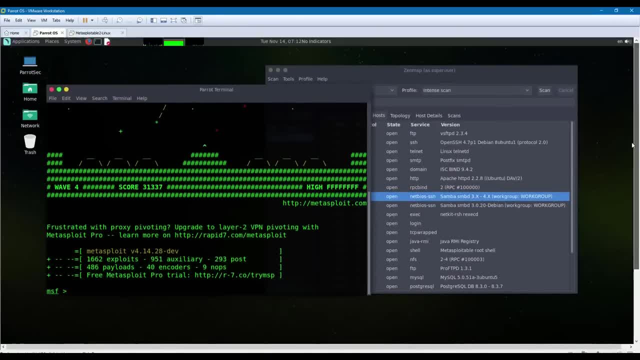 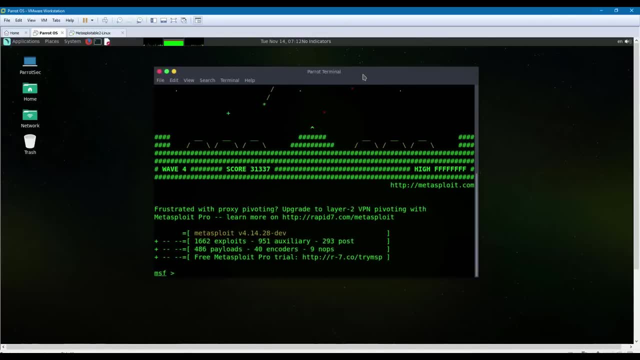 does not run, it does not have a backdoor installed already now that means it's it's pure vanilla, and that means that to exploit anything here we would need to use a payload, because it does have a buffer overflow, and the only way we can make use of a buffer overflow is by using a payload. so let me. 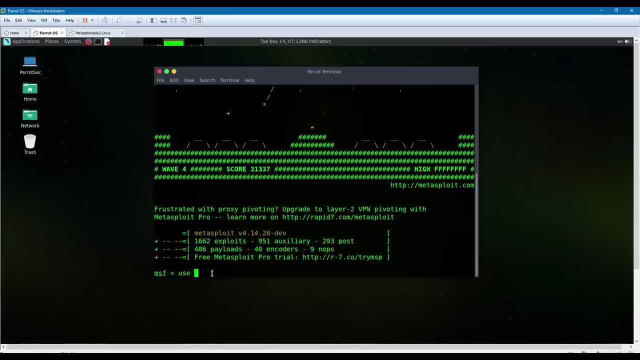 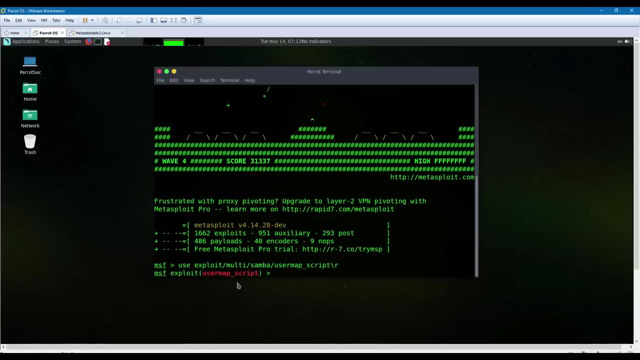 just show you what I mean. so I've got the exploit, so I'm gonna paste the exploit here, right? so I'm going to say: use exploit multi Samba user user map script. and there we are. so let's look at the options available. all right, and right now it's telling me that the options available are the: 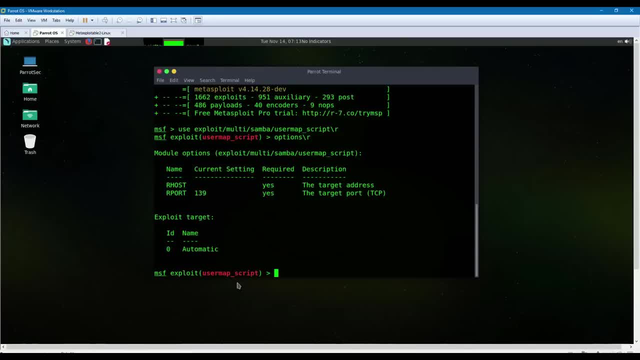 our host, which is the target IP address and the port. the port is fine because it's configured correctly as port 139.. Awesome, all right. so let's set the our host to the IP. all right, so the the IP is for me, is going to be again. you can check this by going to your metasploitable machine and just running the if. 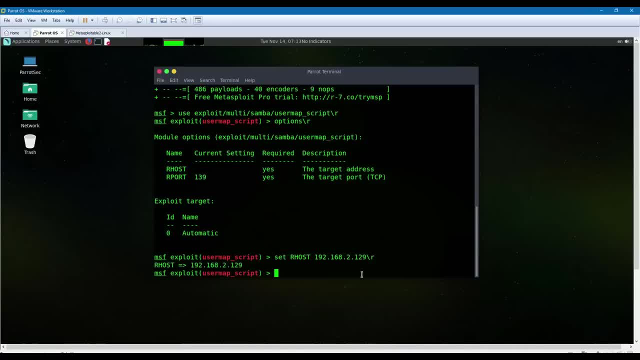 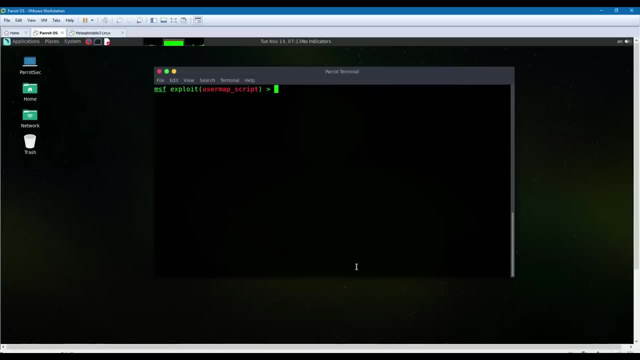 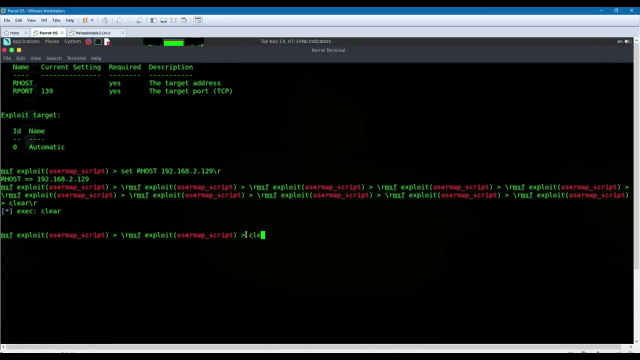 config option. so, once you have said that, now, if we try and exploit this, nothing will happen because, as I've said, we need to run, basically we need to. you need to exploit the buffer overflow and we can do that by by using a payload. so, to see, to view the payloads available in metasploit, what you do is: 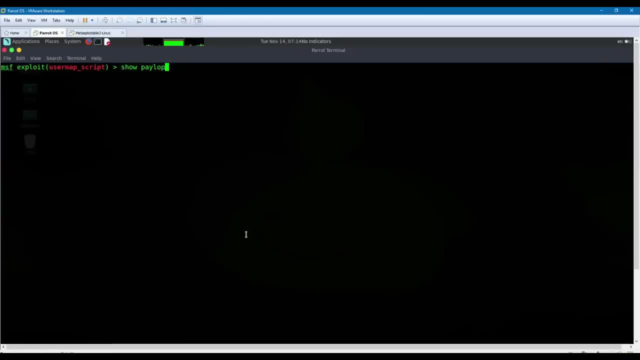 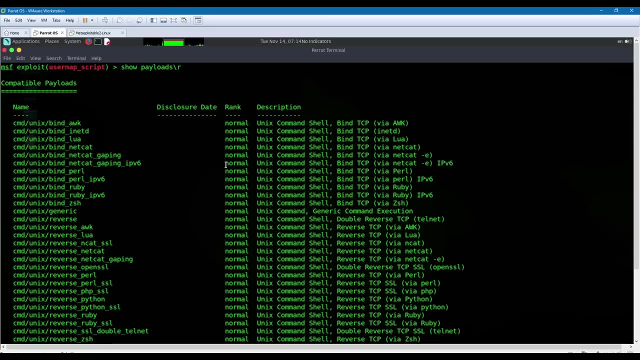 you say: show, all right, payloads. oops, show payloads, and it will show you the payloads available for this exploit, all right. so just give it a few seconds and there we are. so we have. so we know that is using the unix command and we have the, the name and the description. so, as you can see, 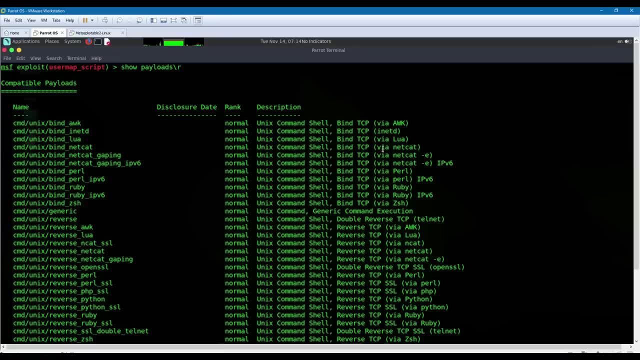 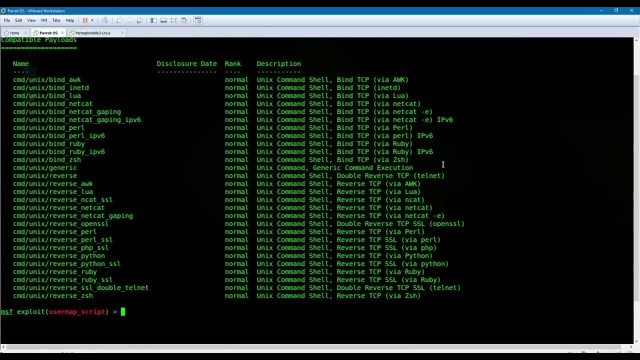 there are very many options that you can use you, as I said, this is a good reason to learn netcat because it gives you the the option to use netcat as a payload. there'll be a lot here which will be all looking through. as you can see they've been. 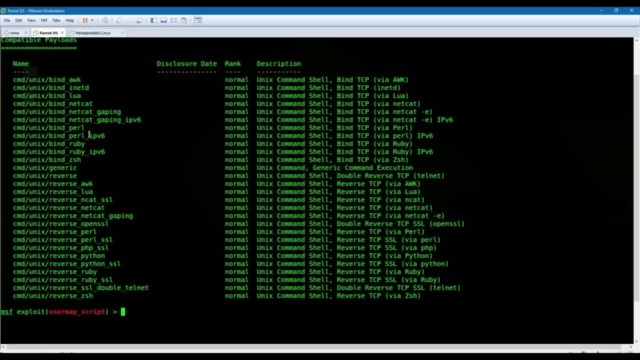 programmed in different languages so you can run the payloads in different languages, and so on and so forth. now, the one I'm going to be using is: I'm going to be looking for the reverse shell, because I want to create a reverse shell where what's happening is, instead of me connecting to the to, to. 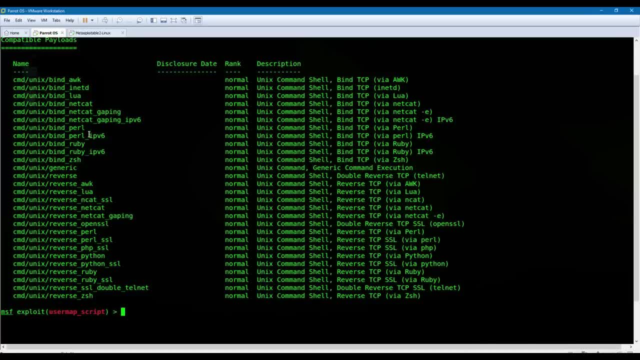 the target computer, in this case our metasploitable machine- and in case it has a firewall, which in most cases a web server would likely have, it's going to refuse a connection, right? so, uh, now, the reason we use reverse TCP is it's awesome because it allows the, the web server, to communicate back. 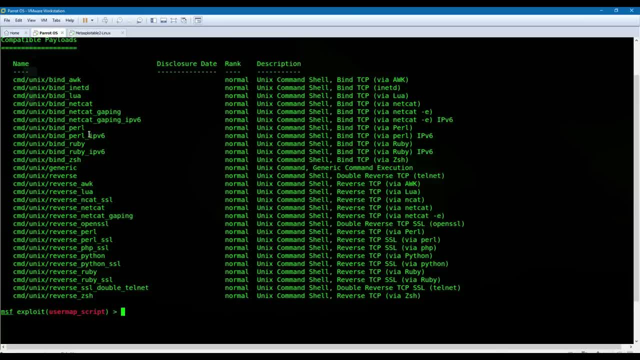 to us on a port that we specify. now that's going to be something that the firewall can't stop, so it's awesome. it's very, very cool to use uh, something like um, uh, to use something like reverse, uh, reverse shell or something of that, uh, something of that. 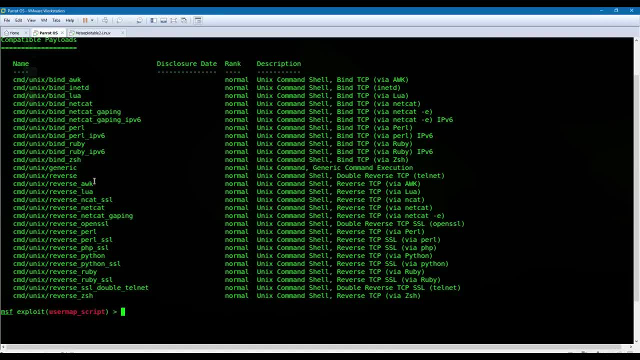 equivalent. all right, so we can use here the um, we can use the. we can use any of these reverse shell uh payloads. obviously the most popular one is going to be the netcat one because again, it's going to use netcat as a means of communication. so I'm just going to copy the exploit and then. 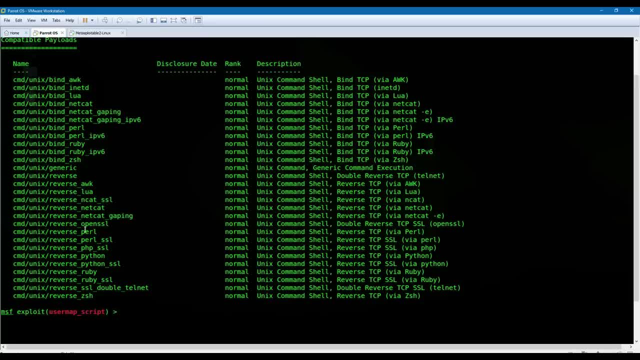 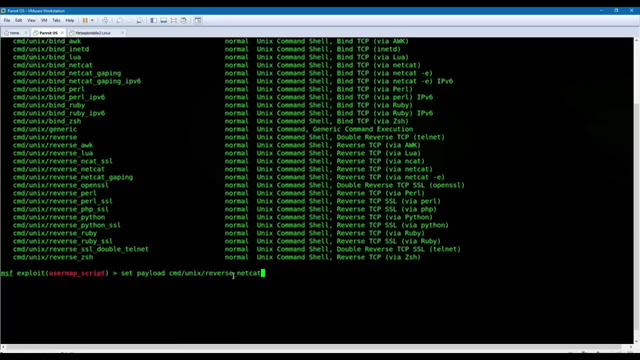 in here you want to set the- uh sorry, you want to copy the payload and in here I want to just set the payload. so, set pay payload and I'm just going to paste the name in of the payload. uh, let me just do that. um, oops, let me just do this right now. all right, so 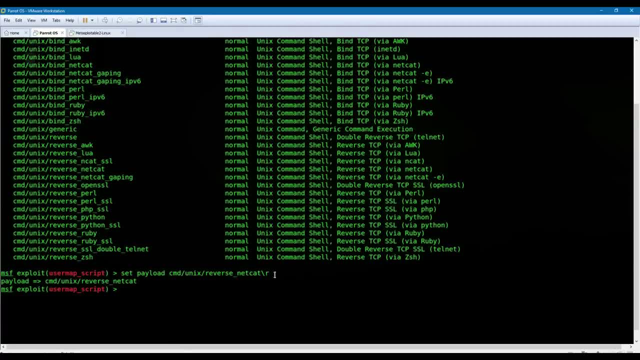 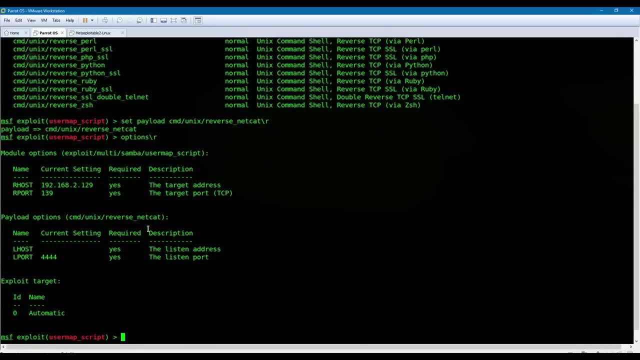 that's the payload we want to use. now. something interesting will happen if we check for the options now. we have different options. now we have the listening address, which is going to be my IP address or the machine that you're using, and then you have the listening port, which, again, you can. 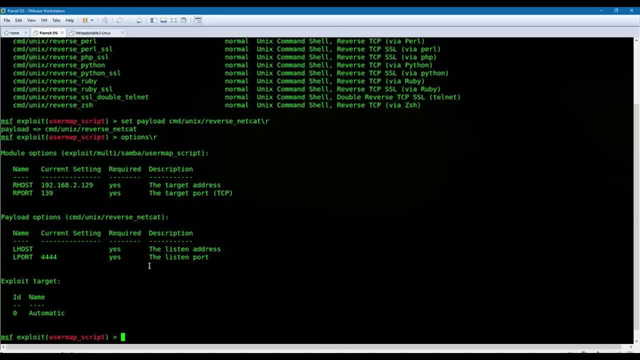 try to make it more promiscuous. for example, you could say that the listening port could be 80. you know the you can use 80 as a port because that web server, when communicating to you, will realize: okay, this is normal browsing, because it's going through port 80. that's where all the traffic usually goes. 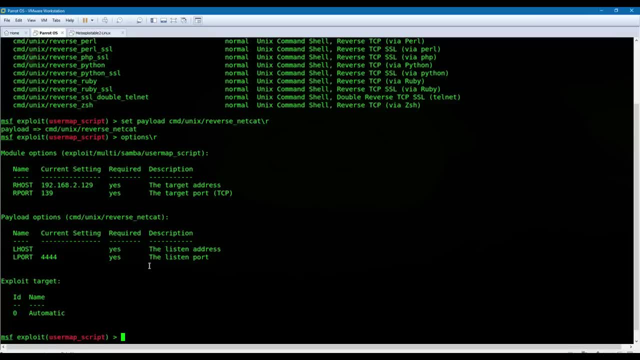 through and it will connect without an issue. uh, as I said, with some firewalls, if you use any other ports, it might detect that. you know, hey, this is a weird port that it's using and this could be dangerous. so block that connection- outgoing connection. but in this case we know that metasploitable is not going to stop that, so you 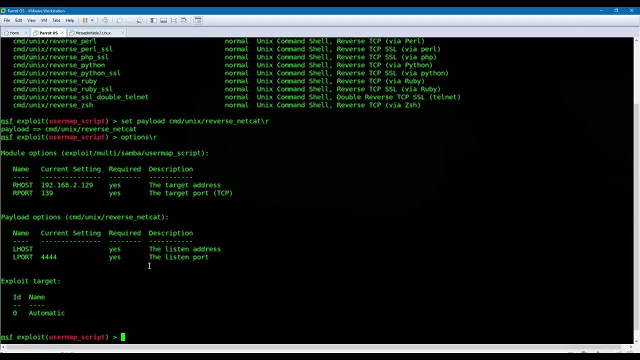 can use any port that you want, but please do remember that if you're going to use a port like 80 or ports that are configured, make sure you have no service running on it or it will conflict all right. so that's also very, very important to understand. so let's configure the L host, which 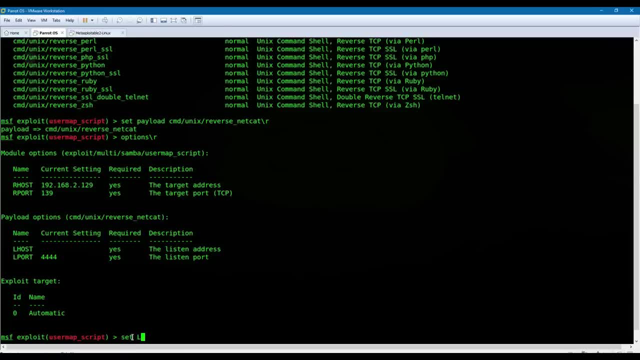 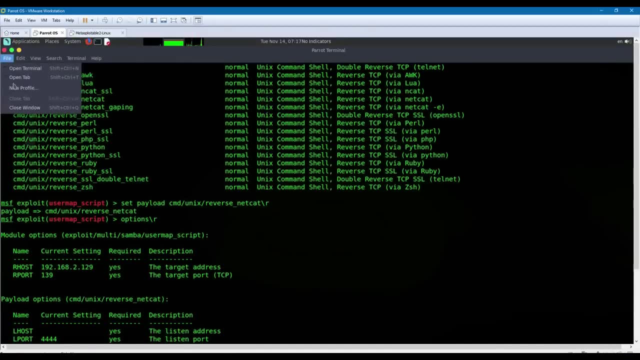 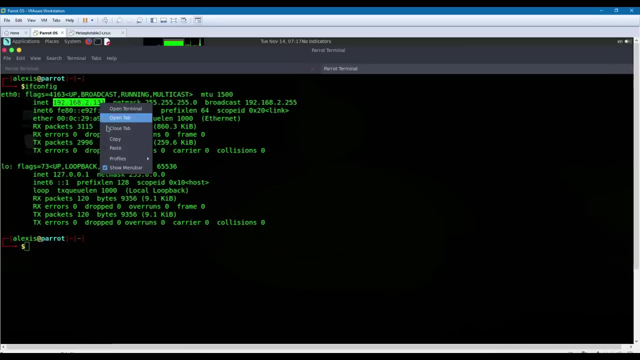 is your IP address. so set L host and I need to get my IP address. I should have actually thought that through. uh, so let me just create a new tab here, and I'm just going to check for mine here, like so, and there it is 192.168.2. let me just copy that here. 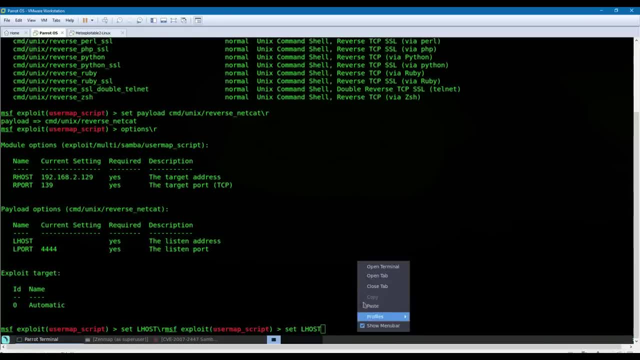 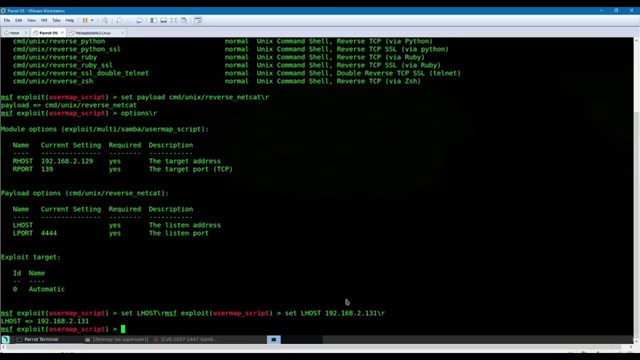 and we can paste that in here, paste it like: so oops, let me just uh, in fact, let me just do that again. so set L host and paste that back, and there we go, we have set our L host, as I can, as I've said, uh, you do, you don't need to change your L port. but again, it depends on. 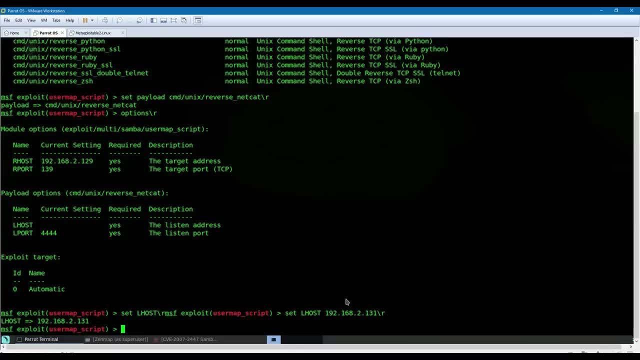 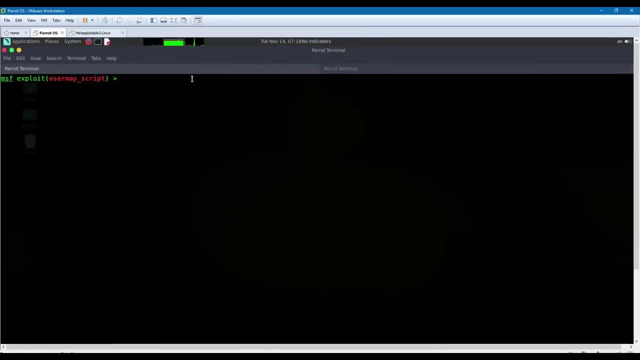 the server that you're trying to attack and run this exploit on. in most cases it will detect it, but uh, if it's coming from a port that is not very common, for example, the port 444. so if you look at the options now, we can see that we've set our R host and the R port, which are correct, the 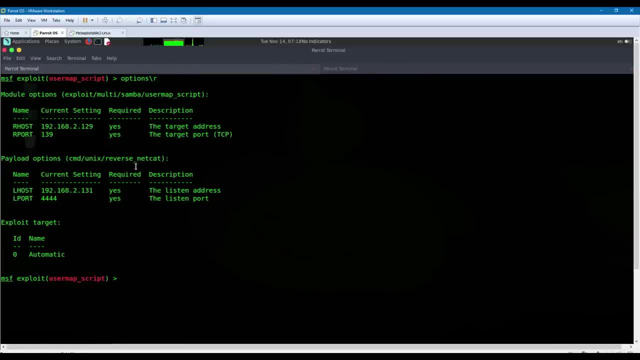 port that we're trying to attack is 139, which is running December server. we then have the L host, which is our IP here, our local IP, and we then have our L port, which is the port is going to listen to uh. that's the port the server is going to connect to, uh with outgoing traffic. so this all looks good. 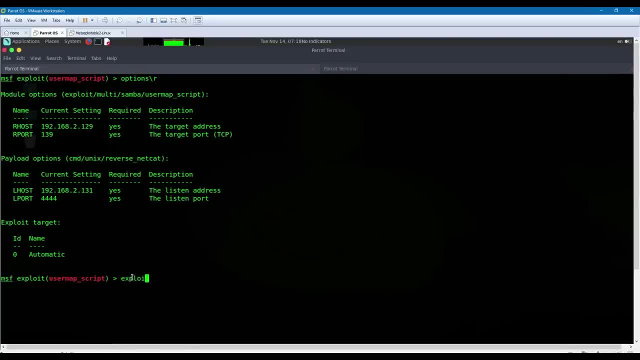 let's see if we can actually run it. so I'm going to hit exploit right and there we are. uh, reverse shell opened and we can go ahead and run some commands. so we are in. so let me just clear the console. all right, so what I can do now is say something like: you name a whoops, you name a there. 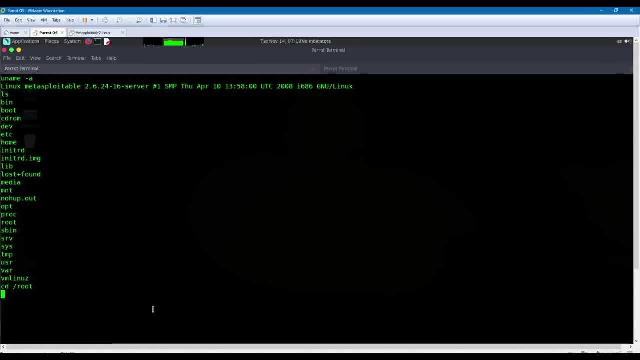 is: uh, let's go to the root. uh, um, let's see what's in root. uh, there we are, desktop. we have files on the desktop. um, let's look at the uh, which, what we have in here? we have nothing in the desktop. let's go back and let me just clear this again and let's see what files exist. whoops, I cannot see what I'm. 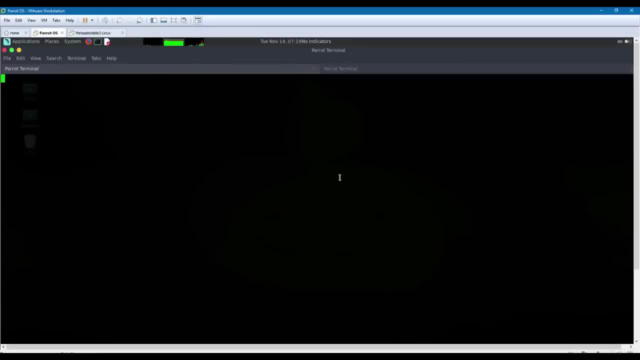 typing in like so, and I believe those are some VNC files. so, uh, cat VNC. uh, whoops, let me just give you the files that were existing inside here. uh, so we have vnclog. so cat vnclog. uh, all right, awesome, we can see that we have the, uh, the log files here for all the VNC servers. 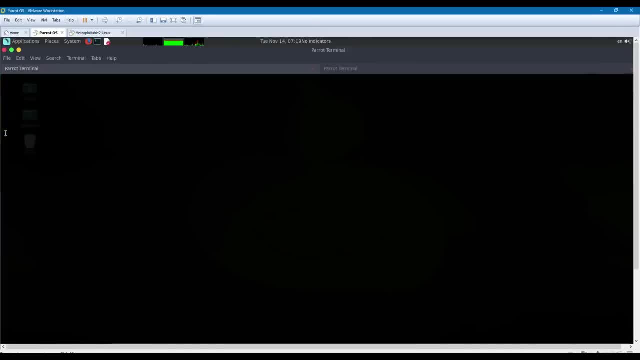 awesome. so, as you can see, we have initiated our reverse shell, and that was a good way of explaining how to use payloads because, in most, in most cases, uh, the exploits that you will be running don't have backdoors in the services that you're trying to attack. and one of the good 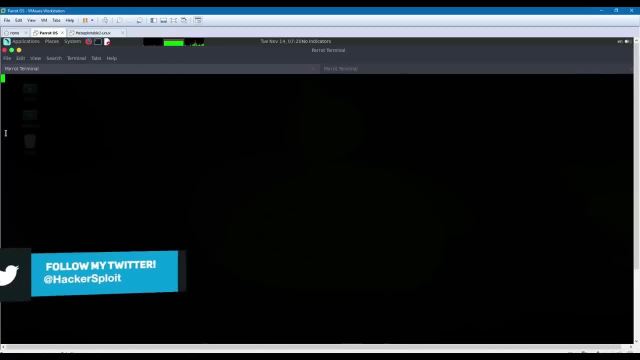 examples was using Samba. Samba has no backdoor, but it allows- uh, it allows- command execution without authentication, so it's awesome. so remember that you can use any type of payload that you wanted. that comes with the exploit and from that you can change the your, your approach of, of attacking the. 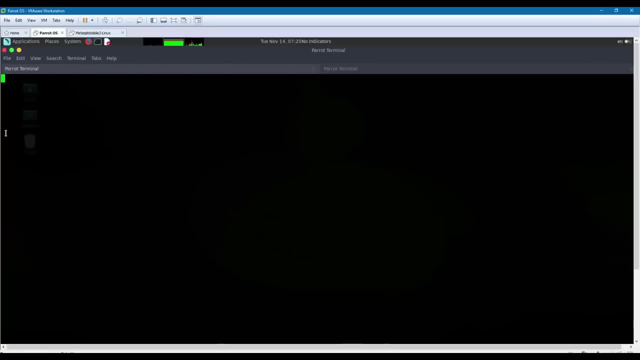 web server. so that's going to be it for this video, guys. I hope you guys found value in this video. if you did, please leave a like down below and if you have any questions or suggestions, let me know in the comment section. you can hit me up on my social networks. if you have any personalized questions, you can hit me. 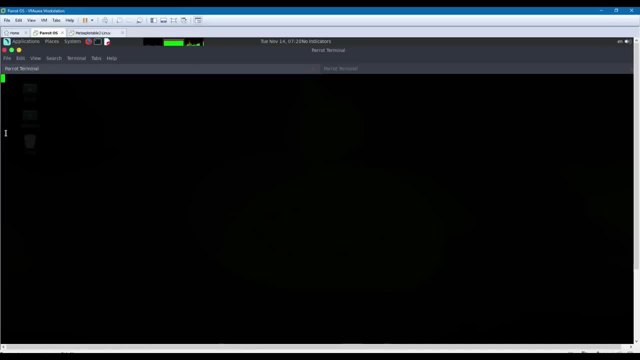 up on kick. and, by the way, guys, something very, very important is I've added a forum section to my website so you can go and sign up and you can post the video suggestions for the new videos you want to see on the channel, and I'll be picking random ones and I'm going to have a Q a series. 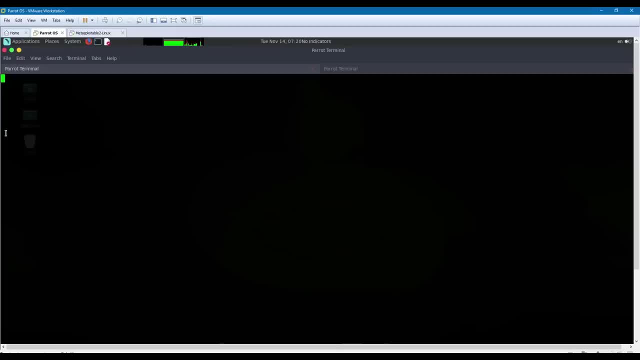 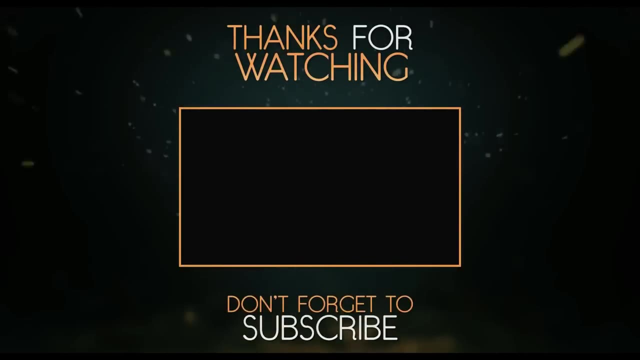 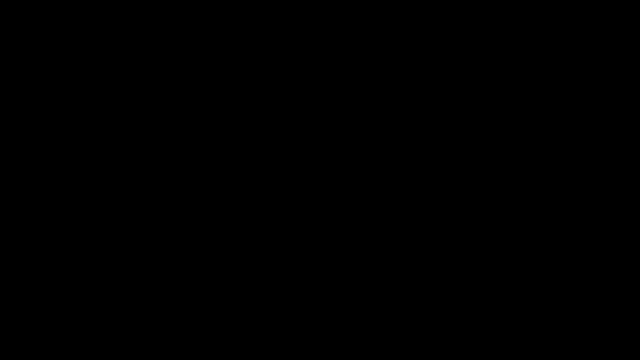 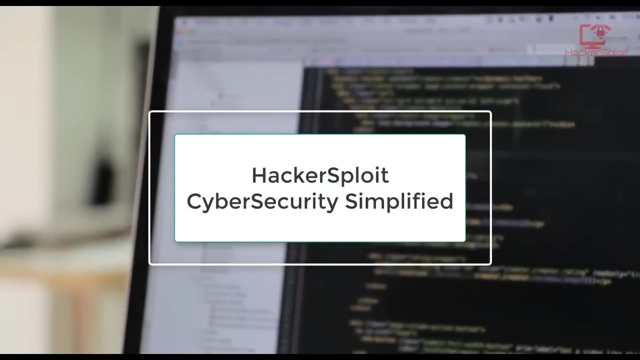 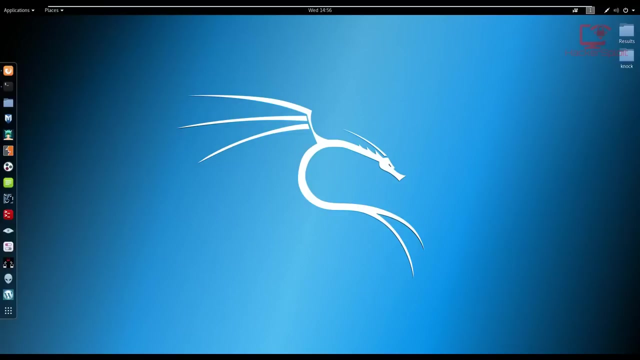 where, every week, I'm going to be trying to answer all your questions, so you can also post your questions there. anyway, guys, thank you so much for watching and have a fantastic day. peace, hey guys. hack exploit here back again with another video and welcome to the web server. 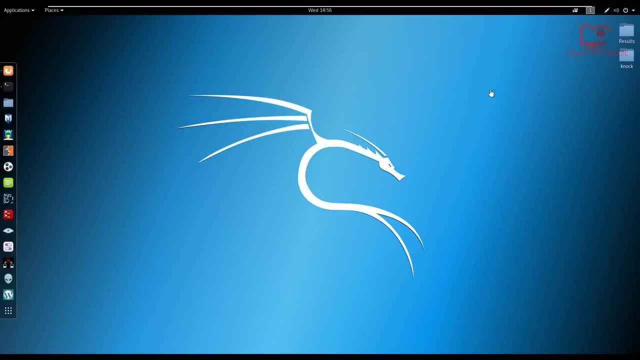 penetration testing series where we're going to be getting started with our first video. I know I've touched upon WordPress scan and stuff like that, but this is now, you know, taking you through the basics and moving your way up. all right. so for those of you asking about Hydra and the word list, 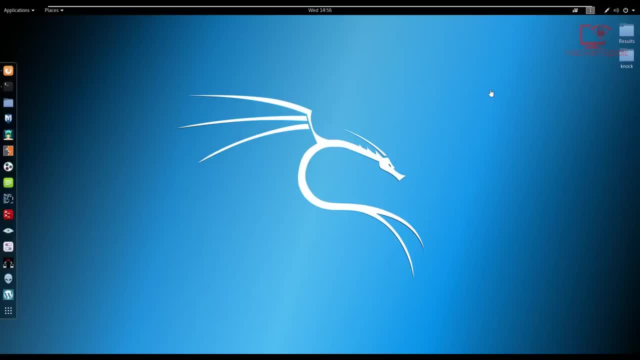 I will be uploading the word list to my website after upload this video. as for Hydra, Hydra belongs to the cracking- uh, the cracking, the cracking section, which we'll be getting to, but you know we're going to be talking about web penetration testing, all right, so in this video we're going 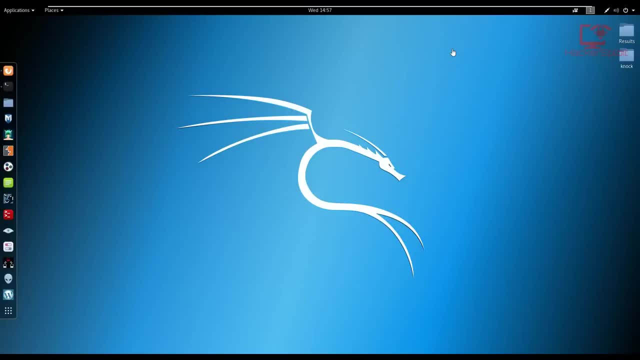 to be looking at nicto, which is a web vulnerability scanner, or a website. it's a website web server security scanner and it is, you know it's- fantastic for detecting vulnerabilities on the server. all right, uh, now the thing I like about nicto- and I use it a lot in the professional, uh you know- for 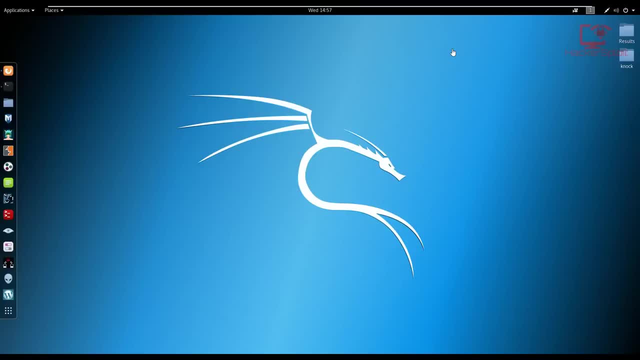 professional projects. it really detects server misconfiguration. now, what do I mean? you know, most of the time, uh, you know system administrators, or you know the people who actually set up the website hosting. they really don't know what they're doing. uh, well, and this comes, you know, in in forms of uh, leaving subdomains wide open for people to. you know, just find and. 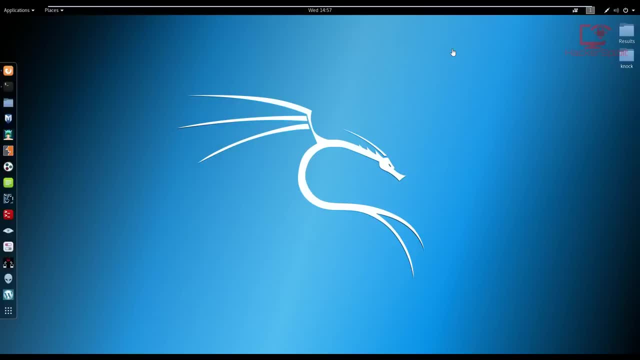 furthermore, exploit, uh, but you know, just finding random server misconfiguration, like misconfiguring ports, uh, you know. uh, let's see something like the, the get and post commands, all of that great stuff which you know might sound a bit confusing to you if you're a. 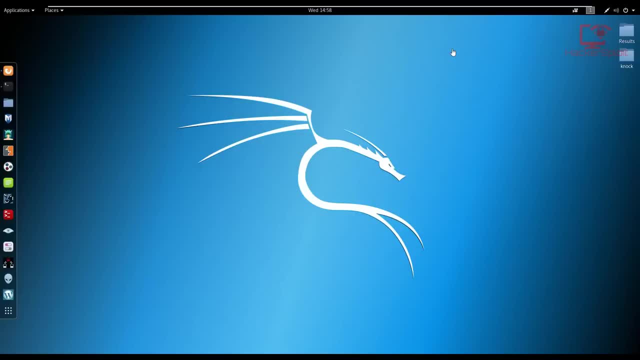 beginner now, but when we'll be moving along, you know, using tools like burp suite, we'll get all it will get into this really, really, uh, in in depth, right, uh, so let's get started. now. I'm going to be using the web, uh, the WordPress, uh virtual machine, or the WordPress server that we actually configured. 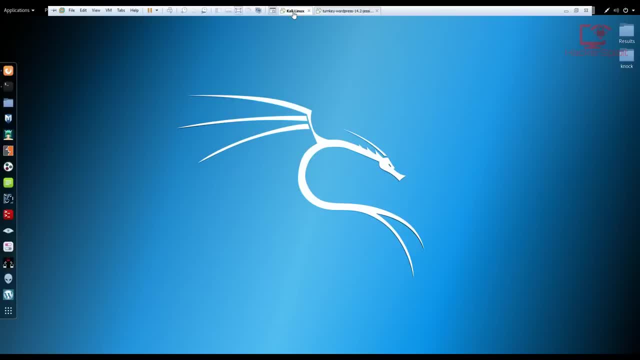 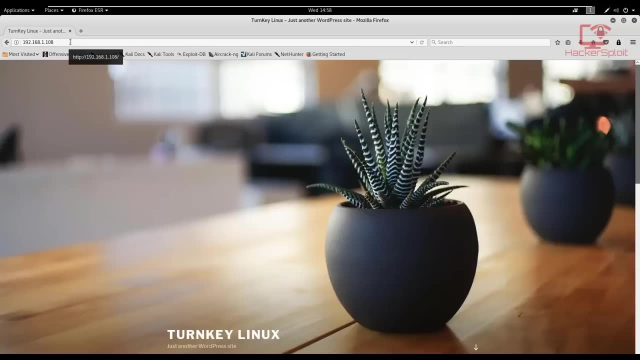 so I've reset it again and it is using new credentials that I I'm unaware of, but the IP address is still the same and I've opened it up, uh on my, uh on on Mozilla Firefox. there we are. that's the IP address, 192.168.1.108, and it is uh. 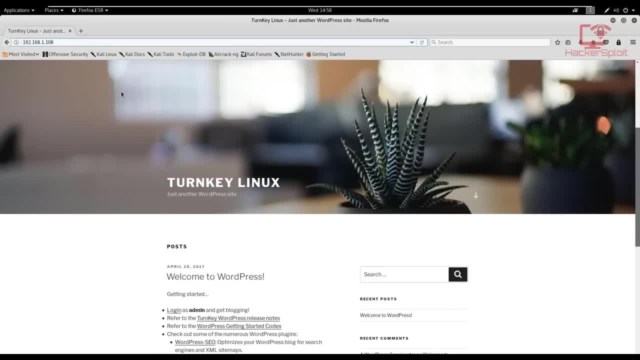 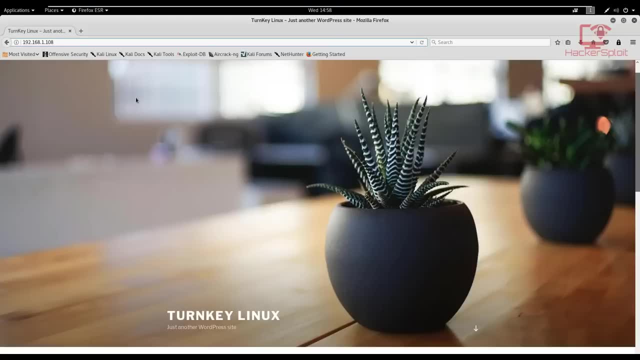 indeed, the WordPress site that is being hosted on the debian server. now what I'm going to do is, as we move along, I'm going to actually log in to the WordPress site and I'm going to update the WordPress version and the plugins to make it more secure. that way it becomes a little bit more. 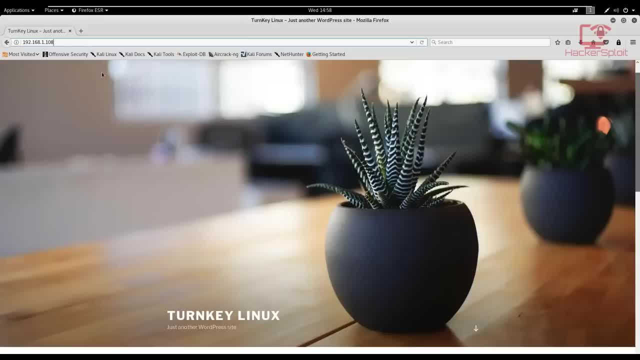 challenging. all right, but for now we're going to be using, we're going to be looking at it, at how to use nicto, all right, to scan for any vulnerabilities that we might find on the site. so, as you can see, I already have it locked to my favorites here on my dock because I use it quite. 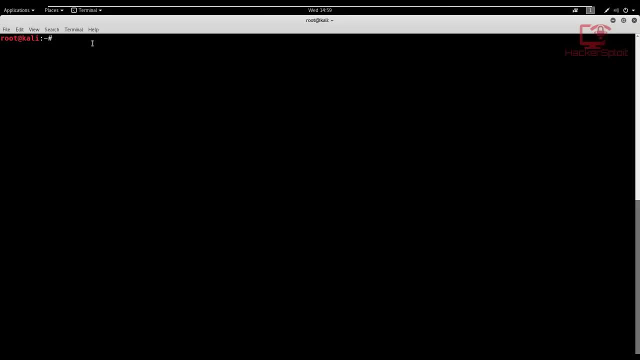 a lot, but to launch it it's really very simple. just open up your terminal and just hit in nicto. all right, now what I'm going to do is I'm just going to open up the help menu, because it is very, very important here, uh, so that I can explain what each of the commands are are and what they. 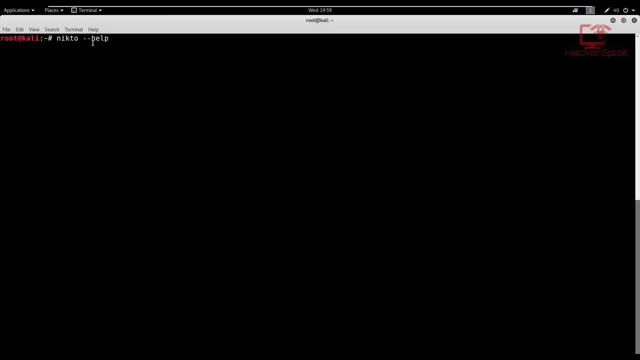 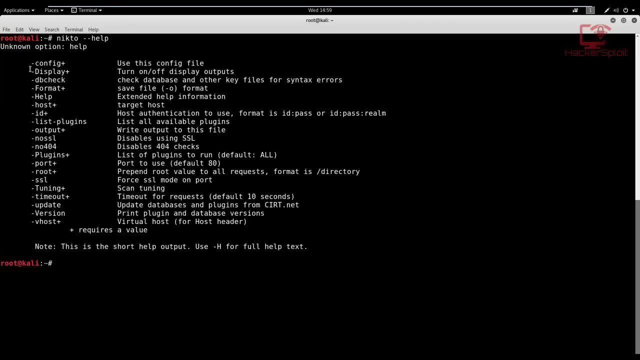 do and, more specifically, the commands that we're going to be looking at are going to be looking at in this video. all right, so let me just open that up and, as you can see, uh, we've got um from the right, from the beginning. we can see that it's sorted really, really well, and this is why I 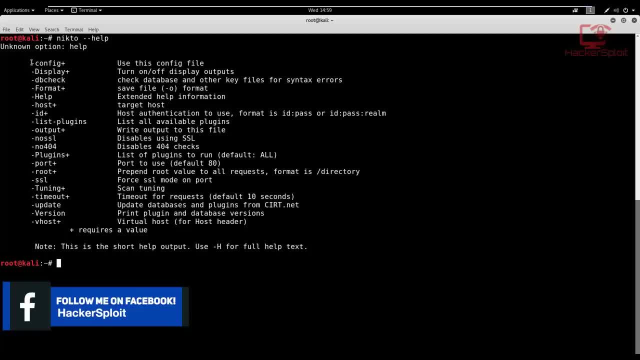 really like: uh, nicto? now some of you might be asking, or you might have this question in your mind. well, you showed us about WordPress scan. doesn't this just do the exact same thing? well, WordPress scan is only designed to sniff out vulnerabilities on a WordPress website. the good thing about nicto is it works on any web web server or website for that. 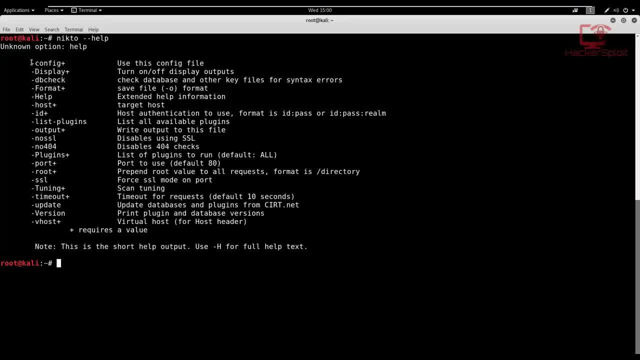 matter and you know, once you know that it's really really fun. fantastic, because it works on any site or any web server, as we have already seen. uh, so let's look at what these commands do now. some of the most important commands are: the DB check, which it checks for databases, uh, the format which allows. 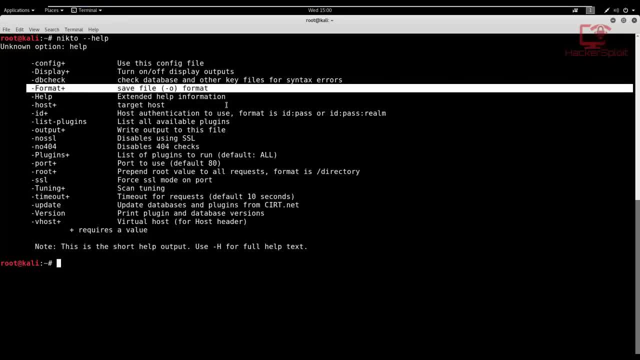 us to change the, the output format. more specifically, the help, the help menu which is specified here, which is again is great because it gives you help. we then have the host- very, very important- allows you to select the host, which, without this command, you would not be able to use nicto pretty much. 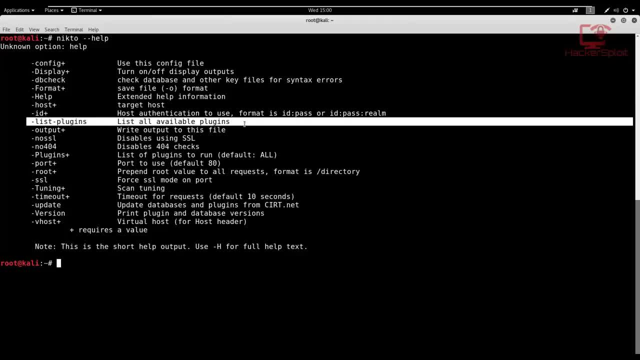 all right. you then have uh plugins to list all the plugins. you then have the output which allows you to output uh your results into a file. are very, very important if you're a penetration tester to always have documentation of all the scans you're performing. you have no SSL which disables using SSL. 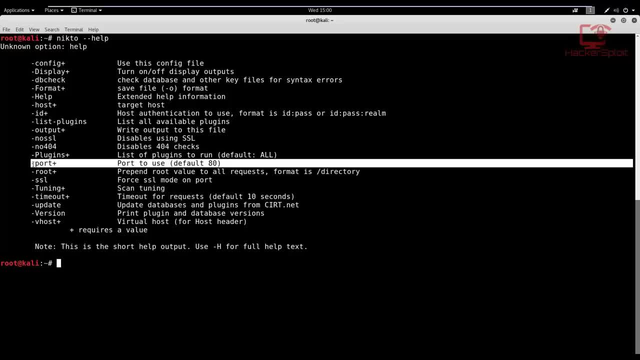 uh, the port which you are going to be using in this video, we're going to be specifying to use the default port, which is port 80, which I'll show you how to specify. you can also change the port if you want, to which you know would make a lot of sense. uh, unless you're performing some serious. 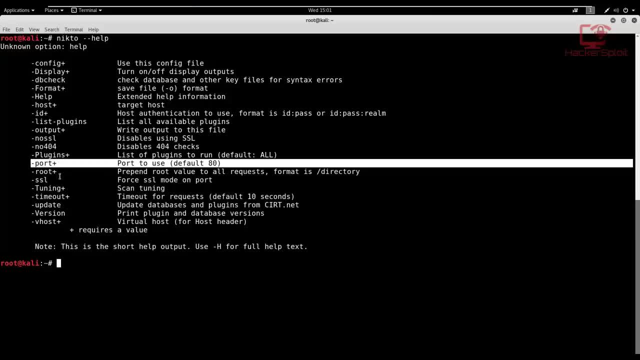 scan. that is more specialized. uh, you then have your force SSL mode on the port, which is not that important- you don't come across that a lot- and you can update it and you can print the plugin and, if you want to, all right. so let's get started with the commands that we're going to be using. so I'm 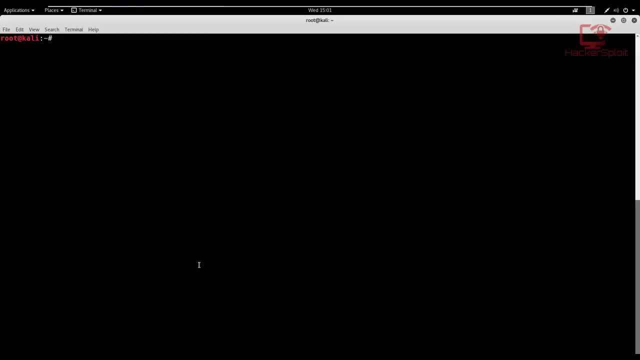 just going to clear this out and we're going to get started now. so, if we remember correctly, we're going to use nicto and to specify the host we use the H command and after this I would use the. I'll select the web, the website address, or the domain for that matter, or the IP addresses I'm going to 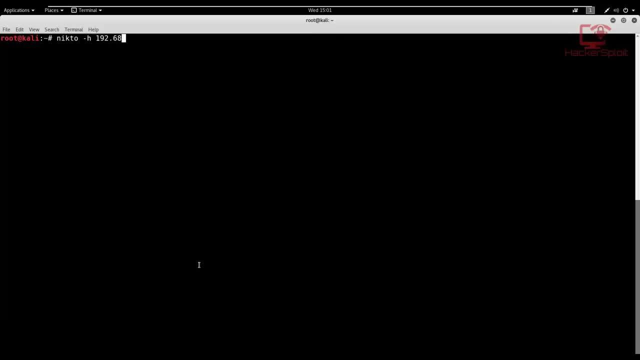 be doing now. so 192.168, whoops, 0.1, 0.108, uh, and I've selected, uh, that I've used the command, the H command, which means I'm using that's the host. I now want to specify the port, which is the only other command that I'm going to be using. 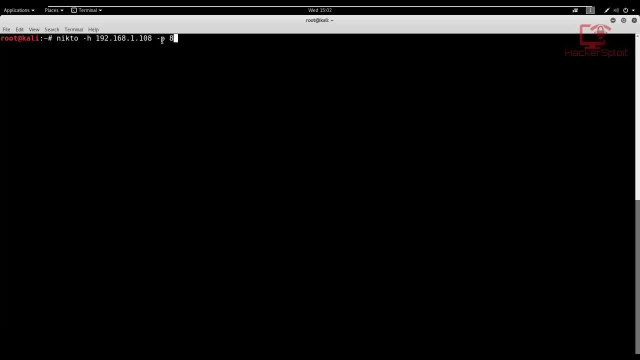 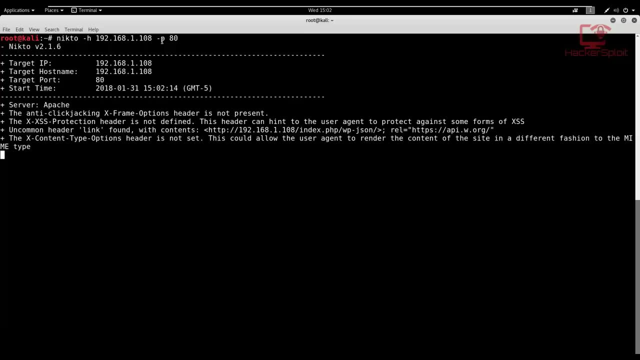 so we use the P and the, we're specifying the port, which is port 80, and let's hit enter and let's see what vulnerabilities we can find here. all right, so I'm going to hit enter and it's going to detect the server, which is Apache, which we already know, as we have looked at this previously. 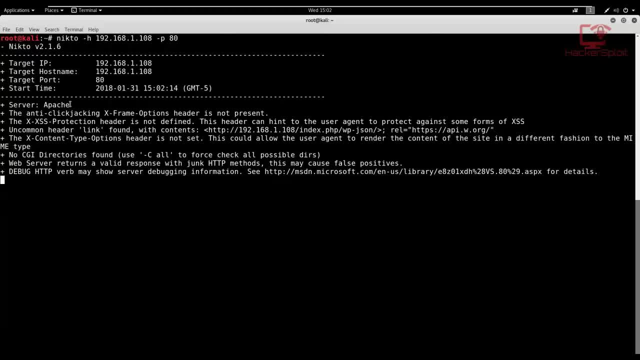 and uh, there we are. it's already got the cross. uh. the cross-site scripting protection header is not defined. that's a very, very huge vulnerability. we'll be looking at how to exploit all of these, uh the you know vulnerabilities like cross site scripting, uh using tools like burp suite and uh. 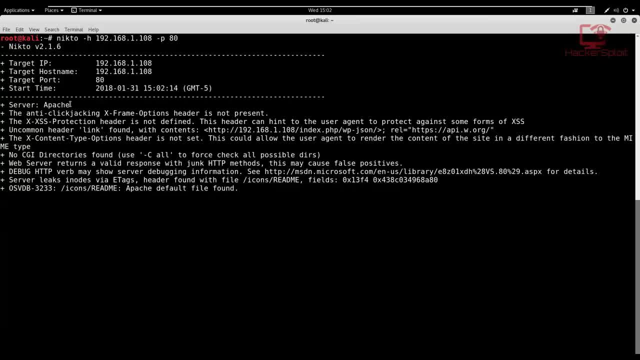 you know file upload, vulnerabilities, all of that good stuff. because a lot of you guys have been asking me about bug bounty, uh hunting, and how do I get started? because you know hacking on the web is it's quite tricky because every site is configured differently. all right, so it's returned the results. 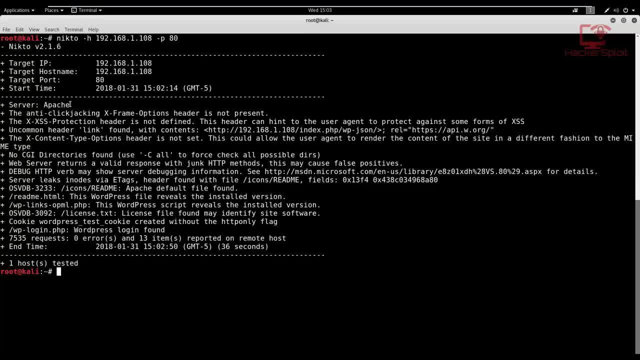 and you can look at all the vulnerabilities that, uh, it was able to find out. um, so the WordPress script reveals the installed version, which is, as you can see, that that looks like a CVE version. uh, cookie WordPress. uh, so, yeah, there's not a lot of uh important stuff that we were able. 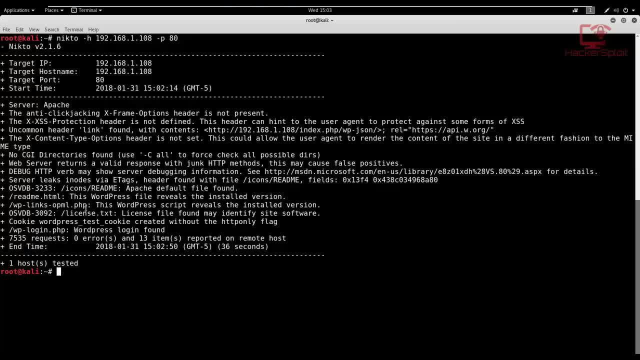 to gather from here again, it would be much more wise to scan a WordPress site. WordPress scan, but for other websites, this is fantastic. um, so that is how to scan for vulnerabilities that exist on a web server- uh, in this case, a WordPress site. now let's look at one. 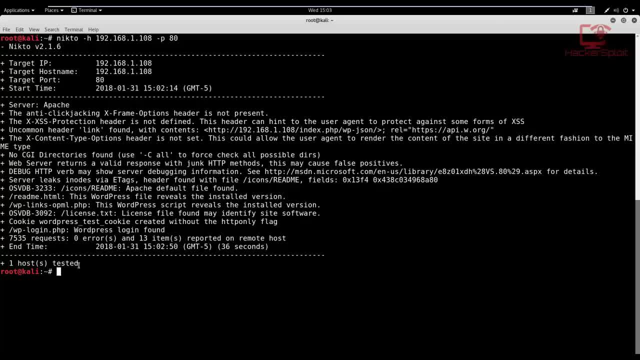 more command, which is the output command, which is very, very important. so we are going to try and output this on the desktop. so I'm just going to change my directory to my desktop. uh, so, like so, and let me just clear the terminal. so we're going to use the same command, um, which is nictoh, which. 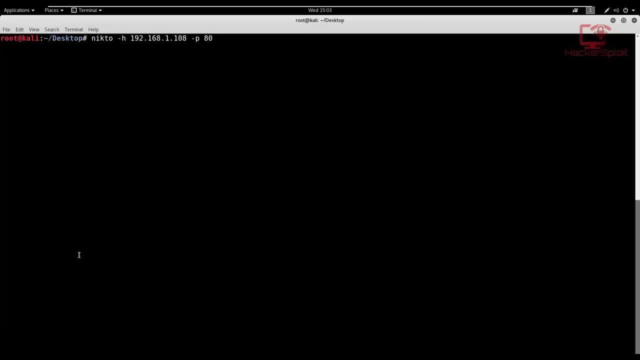 is ghost, 192.168.1.108. uh, we're specifying the port, which is port 80, and now we have to specify the fact that we are using um, the output command. so, oh, and we specify the file name, which we're gonna say, uh is, let's see, let's just call it results. uh, let's just call it nicto results. 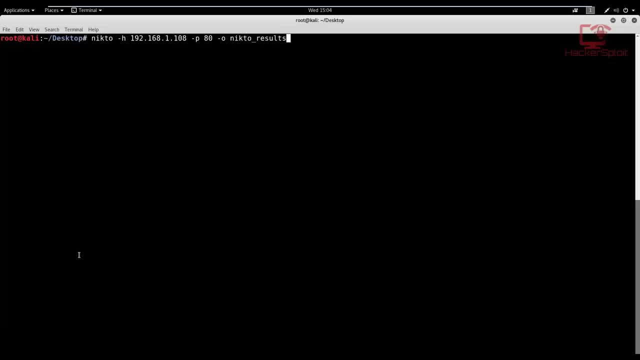 results always good to name your uh, your documentation, appropriately. and now we want to specify the file type, which, in this case, we can just say: we use the command F, capital, F, uh, to specify the file type, the file extension. in this case, I'm just going to select dot txt, just to keep things basic, and I'm going to hit. 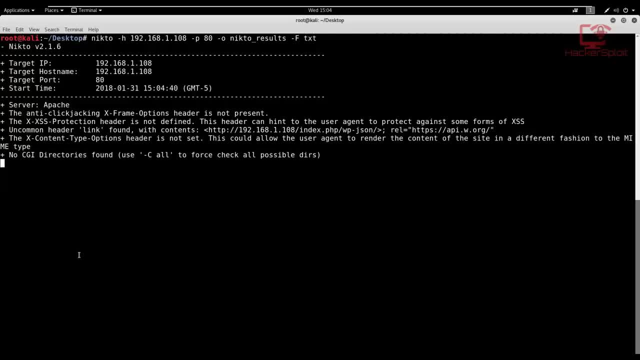 enter, it's going to start the scanning process and once the scanning process is complete, it's going to save- uh, it's actually saving the data right now, uh, in real time, as it's performing the scan. all right, so just give it a few seconds to complete the scan and we'll be able to see. 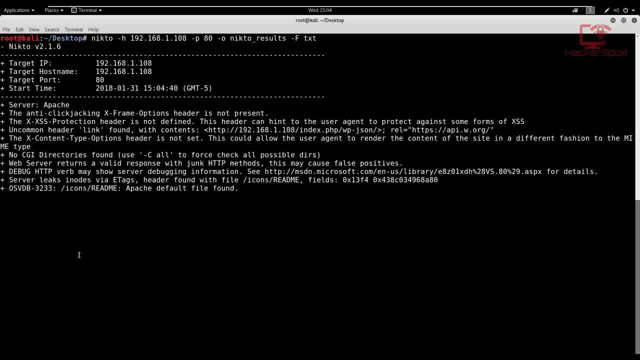 whether or not the information was stored in the file that we specified it to be stored in. all right, we'll be looking at all of these vulnerabilities, uh, as we move along. but the first thing is to understand what we have got and how to gather information about a web server or a website, and this is the basic, you know, just getting started with. 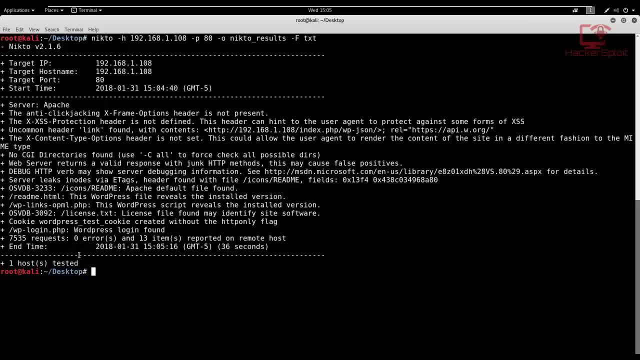 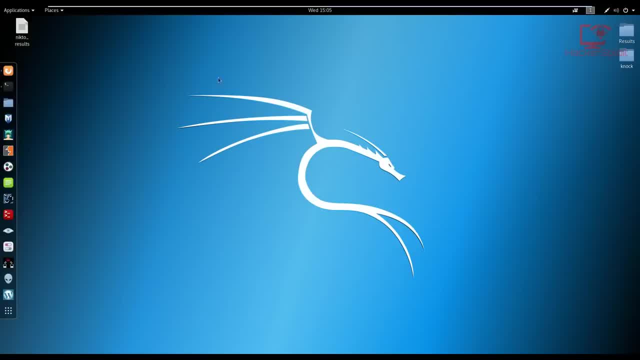 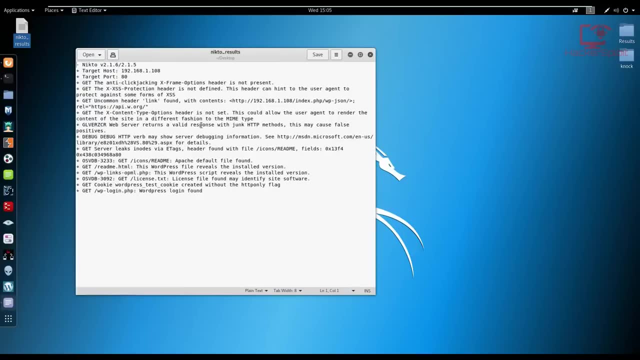 it. it's a very, very good to get accustomed to the tools. all right. so, as you can see, uh completed And if we just check the desktop here, we have the NICTO results. There we are Fantastic. If I just opened up the file and it has stored all the information, very, very important that 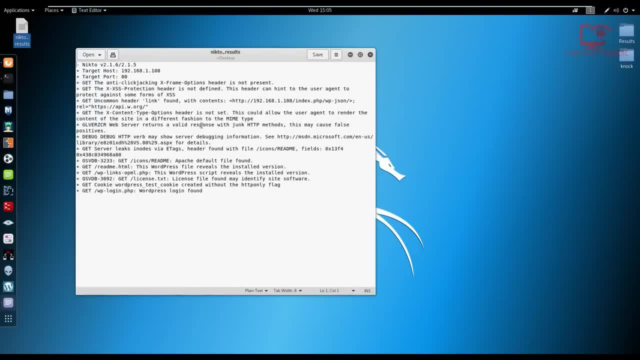 you store this information. it acts as a good way of of showing, or it acts as documentation, And that is very important, especially for a penetration tester. Alright, so that is going to be it for NICTO. We'll be moving along swiftly after this And you know we'll be looking at. 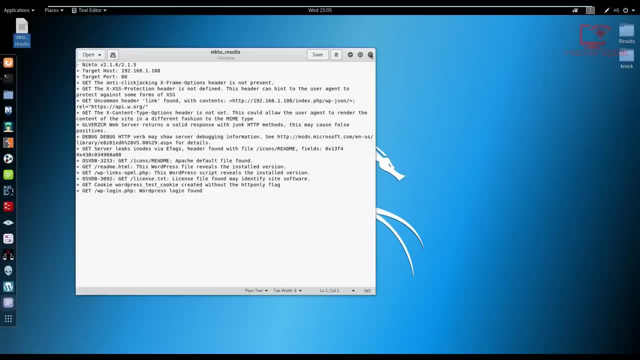 cross site scripting, how to use burp suite- all of the great stuff, Alright. so I want you guys to stay tuned for that. So that's going to be it for this video, guys. I hope you guys found value in this video, If you did. please leave a like down below If you have any questions- any at all. 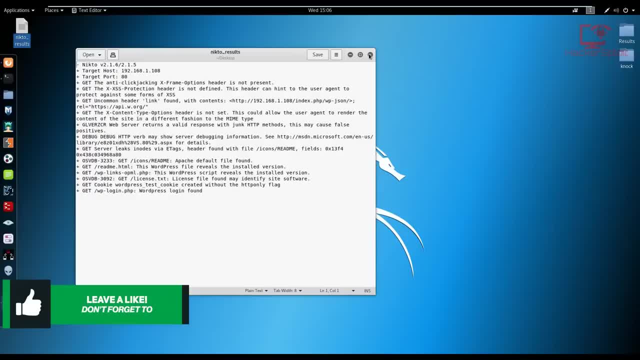 hit me up on my social networks or or, you know more specifically, you can hit me up in the comment section. If you have any personal questions, please hit me up on kick. One more thing, by the way: if I do not reply to your comment or question, it doesn't mean that I do not want to. 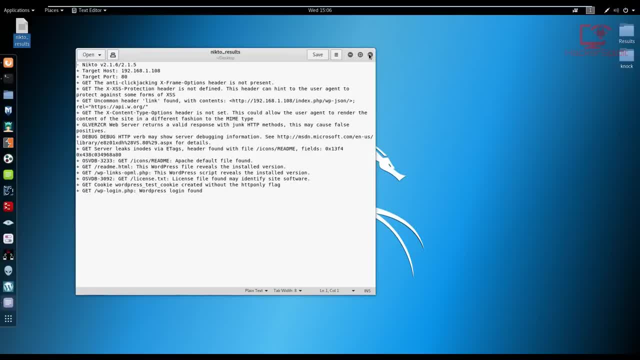 it's because there are a lot of these comments and I have to go through them as much as I can And I try to reply to all of them, because the comments are increasing as the channel is increasing. And you know, if I don't reply to your message, please don't take it the wrong way. I will reply just. 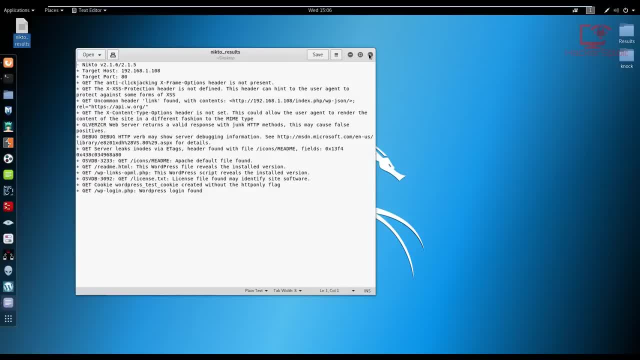 give me a, you know, up to one or two days at the latest. I just want to thank you for all the support, guys. Thank you for supporting me, and I have something really, really important that I want to announce soon For those of you who are watching the video till now. you know, stay tuned. 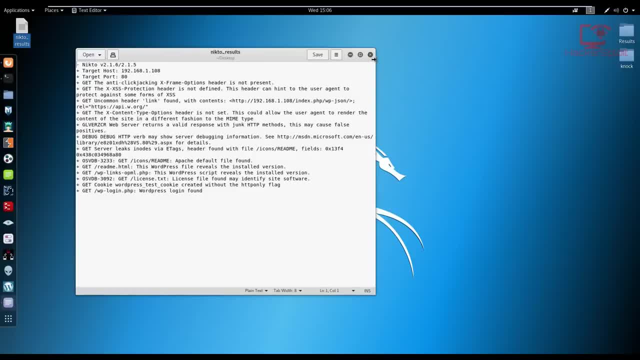 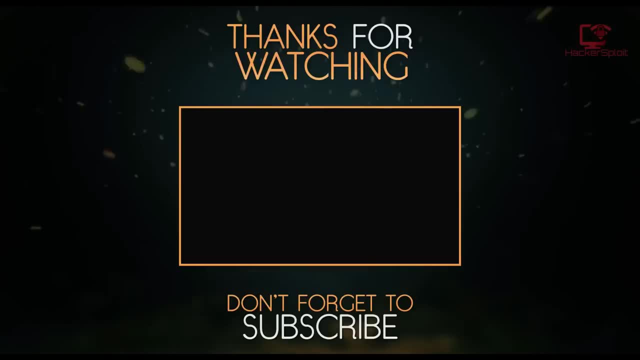 for that. I will see you in another video and I will see you in the next video. will see you and let this video be the last video, so don't forget to subscribe t and yeah, I will be seeing you in the next video, Peace. Hey guys, goes like to back again within a video and into this video We're going to be looking at like My channel. in case you want to support this channel, if not, my channel on Facebook. This is my channel, Yeah. 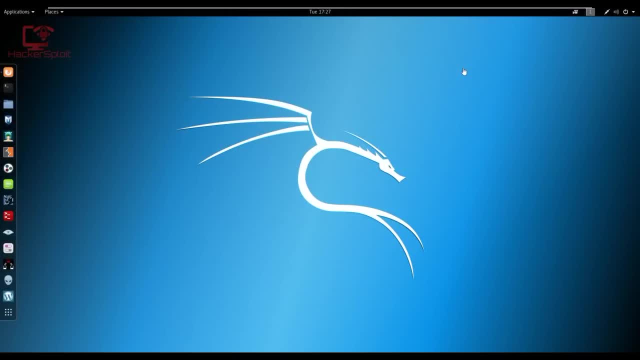 It's the kind of thing where you look at, we'll try to correct more money when we go to per want to explore the world for that opinion And I will see you in another video. See you then, Come on, see you now. 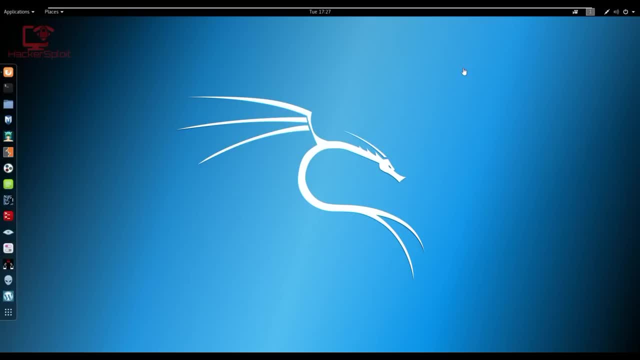 Bye bye at how to exploit WordPress. more specifically, we're going to be finding the username and the password on a vulnerable WordPress server or, in this case, we're actually using a virtual machine that has WordPress running on it. now the reason I'm doing this- and a lot of people ask me this- 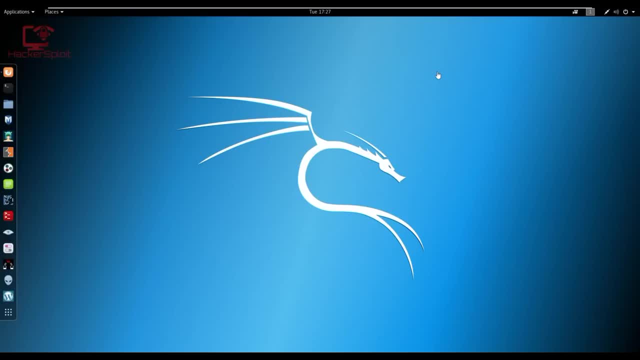 question is: why hasn't your channel got any copyright strikes? and that's because I perform everything in my virtual lab. that means I'm not attacking anyone or causing harm to anyone apart from you know the targets in my lab, so I have downloaded a vulnerable WordPress server that 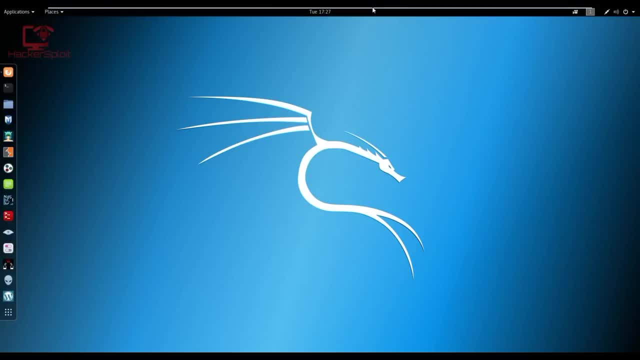 is running on Debian from turnkey Linux. I'm pretty sure you know that site. right now they have a lot of virtual machine, they have a lot of VMs that you can use for testing etc. and you know you can learn and practice a lot of stuff. so I have it right here and I've started, I've configured it up and 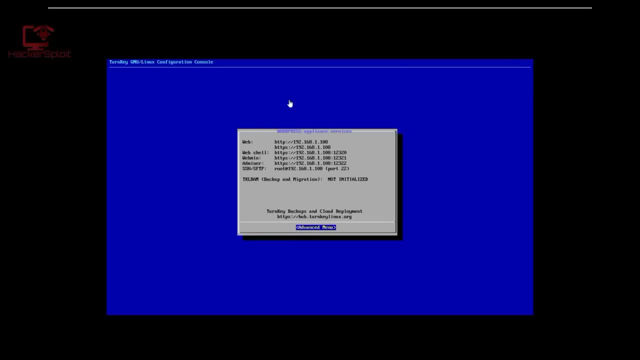 I've used the default, I've used the default credentials, so I actually don't know what the username and password combination is, and we're going to be doing it live. so there's some information here that it's giving you, which is pretty helpful. we know that the, the server, the IP address, the local IP address, is 192.168.1.108. 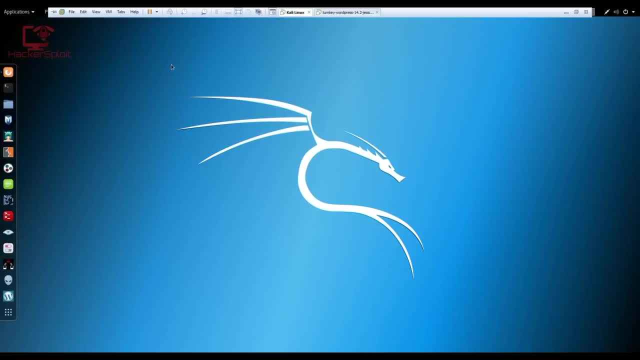 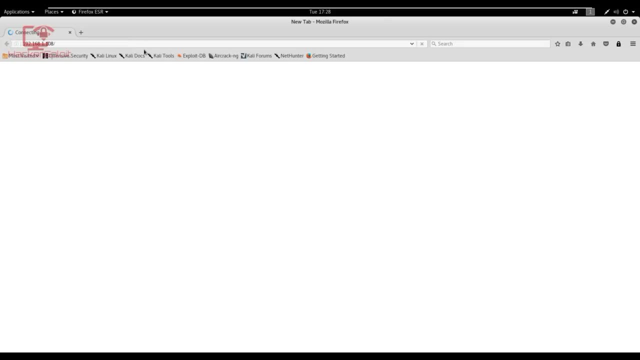 all right, so let's get started. so what I'm going to do first is I'm just going to start off with 192.168.1.108, right, and obviously it's going to be a WordPress site, as you can see, here and now, the most important thing is to 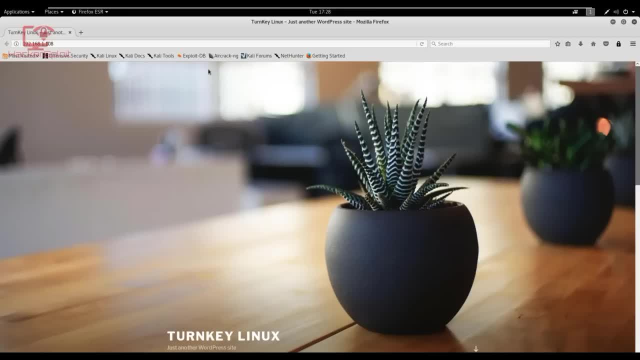 start enumerating the username and hopefully we can crack a password. now I, you know, like to just tell you that I'm using a, a word list, a special, well, a basic word list that I found quite a few years ago. that has been actually quite helpful, so I have that already downloaded and hopefully we 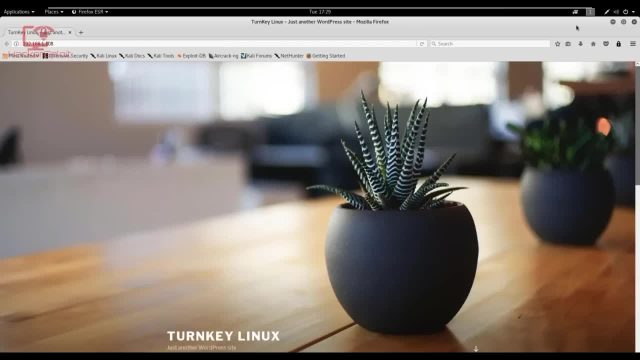 can find the username and password here, so it's using default credentials, so it will be much easier. but I'm just explaining- and this is just a a bit of a practical explanation as to one- how one would go about doing this using WordPress scan. Alright, so we know it's running WordPress And 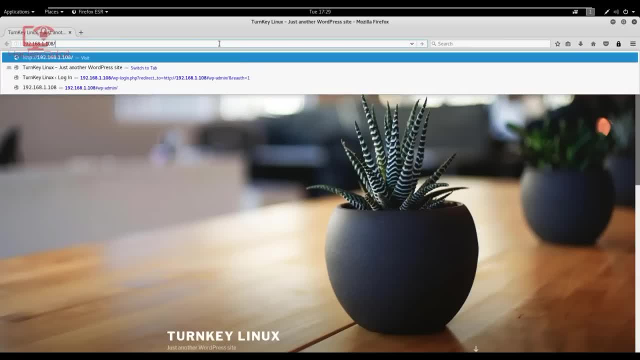 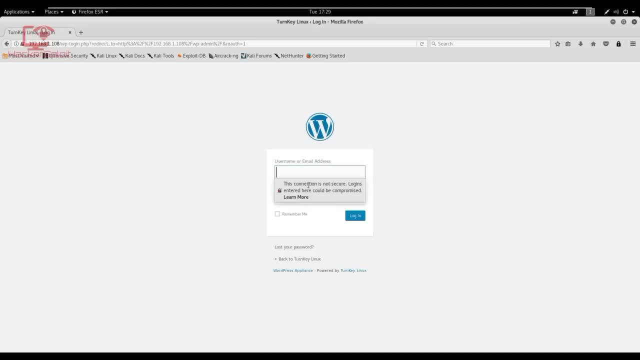 you know if you, if you're familiar with web penetration testing, you know that WordPress sites have the WordPress admin page right that allows you to log in, So we know we can actually log in here. Sorry about that, Alright. so anyway, it's working really really well. So WordPress is. 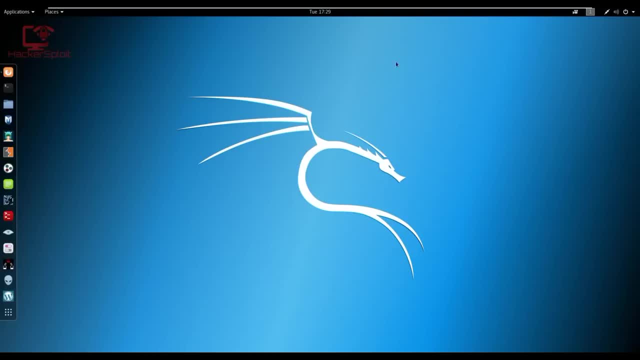 actually running And I do not know the login credentials, So we're going to hopefully try and find them. Now. we do have the server IP And obviously we do know that it's running WordPress right, So the first thing we need to do is we need to open up WordPress scan or WP scan. Alright, 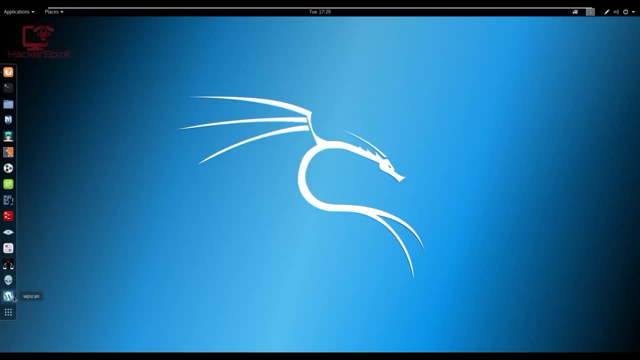 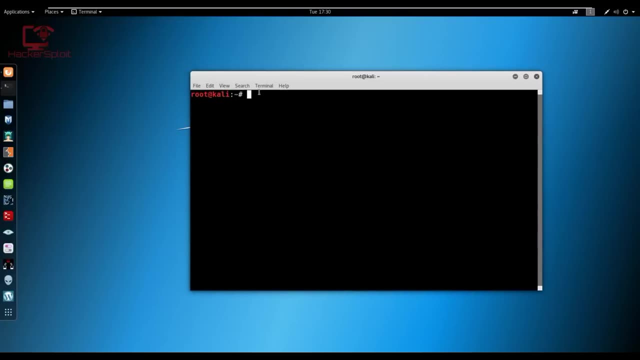 so, as you can see, I have it on my favorites or on my dock here, And to launch it it's really very simple. You can just go to your terminal and you just hit WP or WordPress scan. So W whoops, my bad, Sorry about that guys, Apologies there. 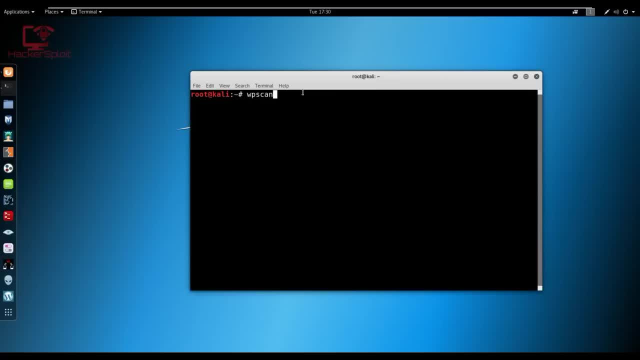 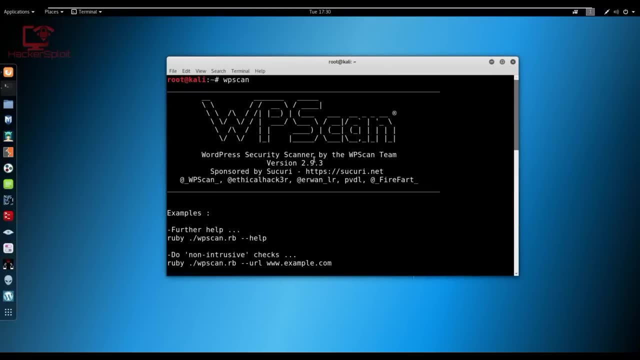 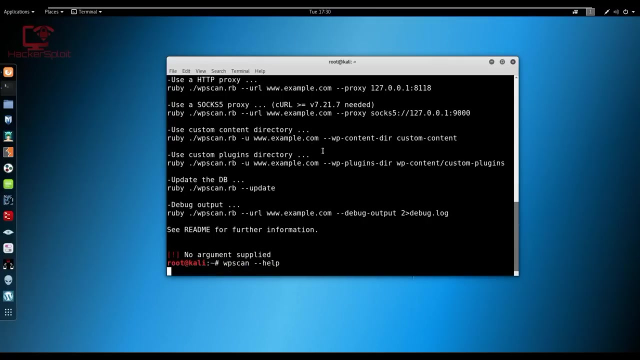 I was smashing on my spacebar, Alright. so W WP scan, Alright. and if I just hit Enter, it's going to give me the help options. There we are. So there's a lot of options And we'll be covering most of them here. We can also use the W scan Help, Alright. so to enumerate the 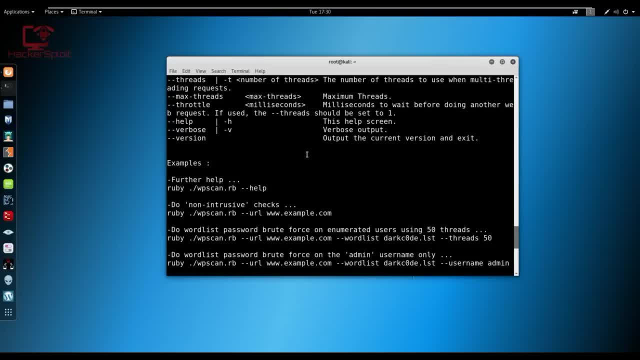 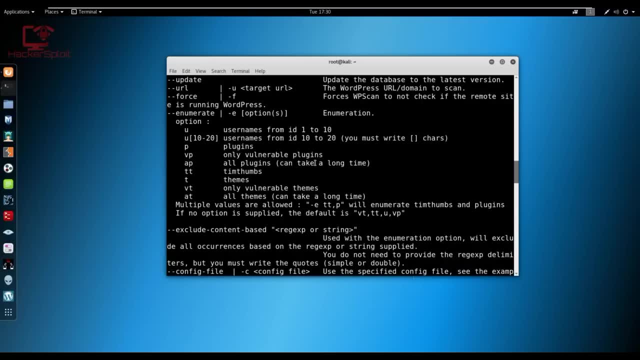 help options. There we are. So we have the help options And we're going to be using some, some basic commands here, But I'll be explaining what they do, Alright, so let's get started now. The first thing we need to do is we need to enumerate the usernames, And this can be done. 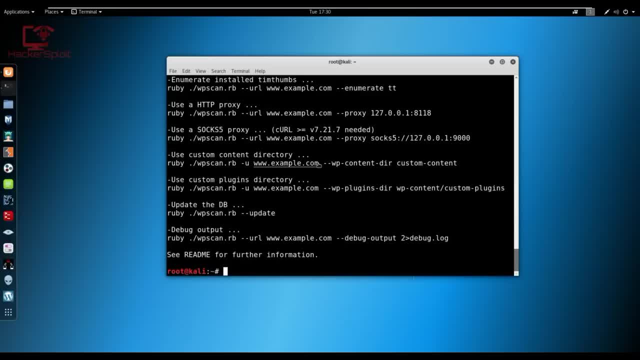 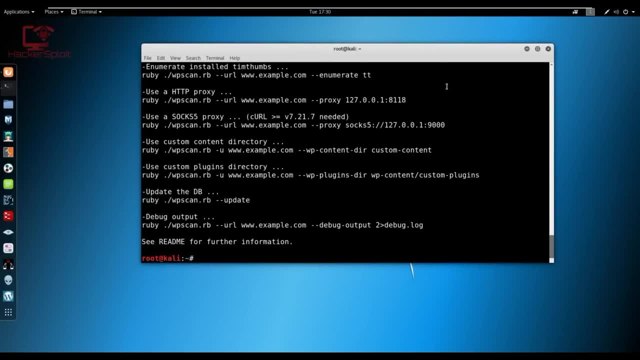 you know, by exploiting the vulnerable plugins Now by default, as I've already said, this WordPress version is vulnerable and it is set up to be vulnerable, And it's just a way of me explaining how this goes, really. Okay, so let me just clear that up And we can get. 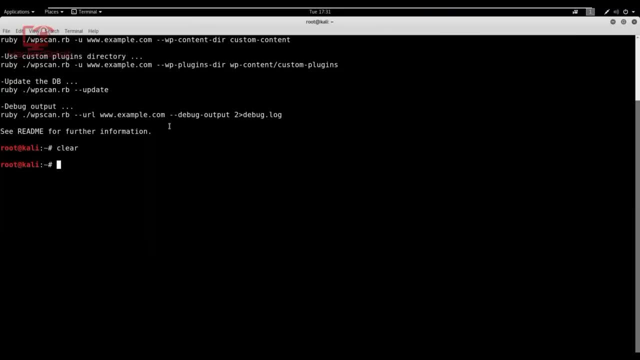 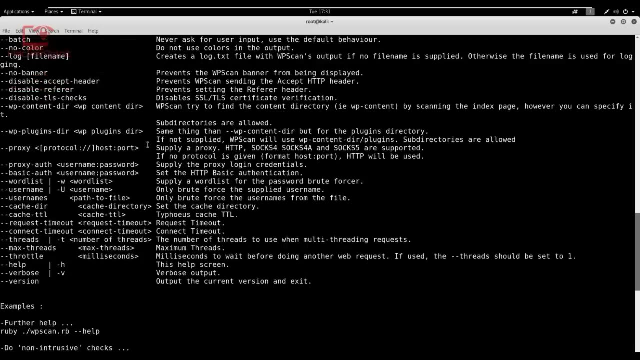 started. Let me maximize the terminal, because we're going to need all this, the real estate that we have, that we actually need. All right, excellent, Let's begin. So now we're going to start with. let me just enumerate the help. Yeah, just to get started. So we're going to actually. 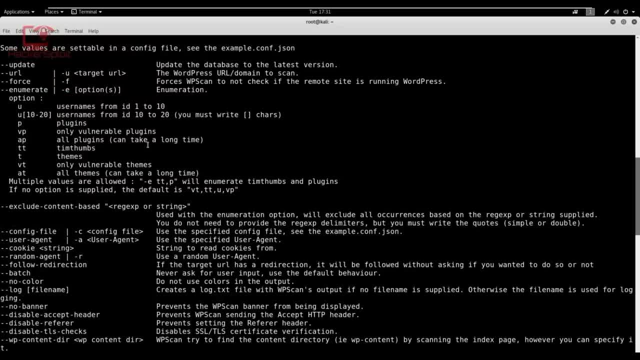 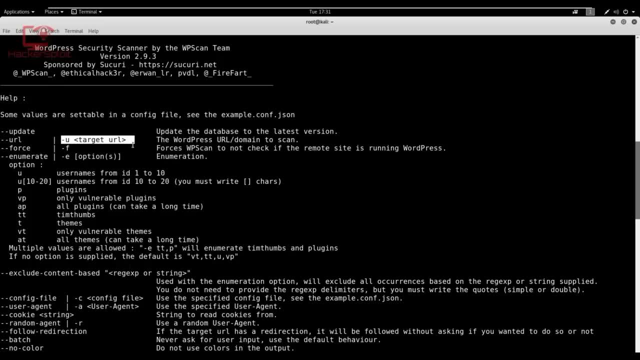 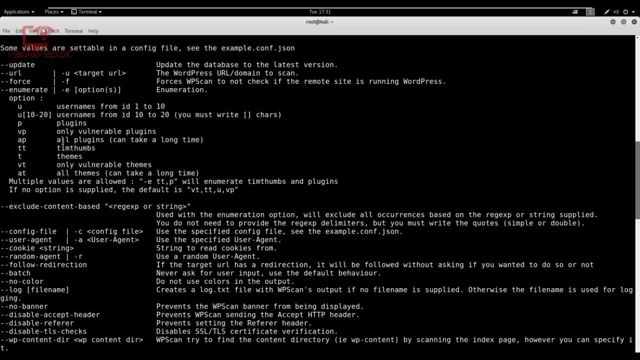 start enumerating the username. So the username. of course, we're looking at the basic syntax here. So again, since we're using the U command because we are targeting a URL, so the syntax will be pretty simple, We'll be using the U command, we'll be using the E command, If I can find it here. 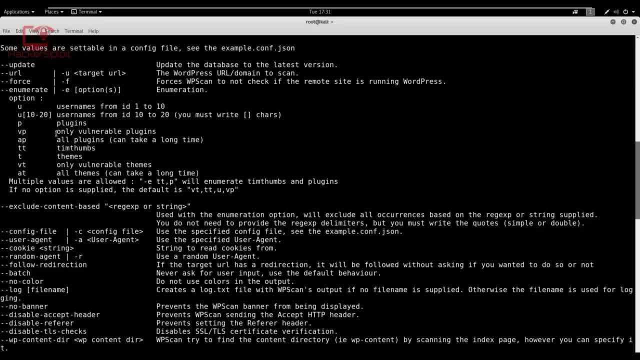 Yeah, there we are there to enumerate options, And then we're going to be targeting usernames. So, again, it's going to get usernames here And finally, we're going to be targeting only the vulnerable plugins. Alright, so that is right here, VP: only the vulnerable. 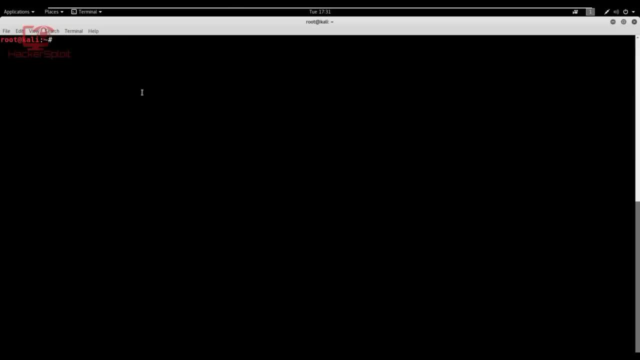 plugins. So let's get started. I'm just going to clear the terminal again And there we are, So WP scan, And after that we use the IP address, So 192.168.1.108.. Excellent, Now we use the E to. 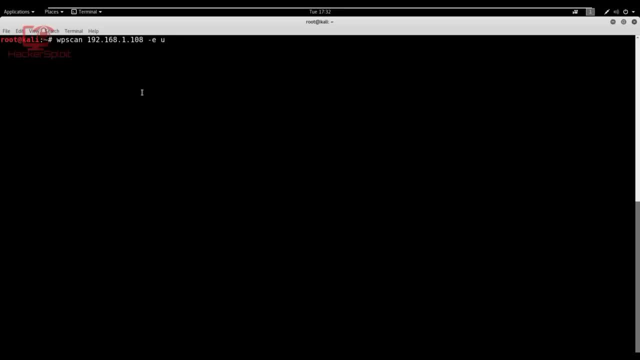 enumerate All right, the E command. Now we use U All right, because if I enumerate username, so U is not actually an argument or a parameter. It's more of an expression of enumerate Right, so EU, so enumerate usernames, and I want you to. 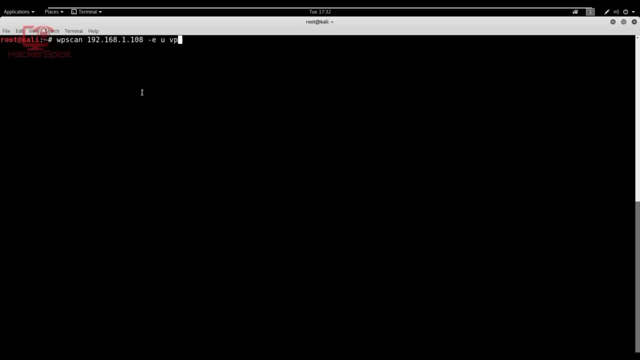 target only vulnerable plugins. There we are, So hopefully this returns the default username. So great, enter. And this should be relatively quickly because again, the username is not. is is going to be the default username, So I'm just going to hit enter. 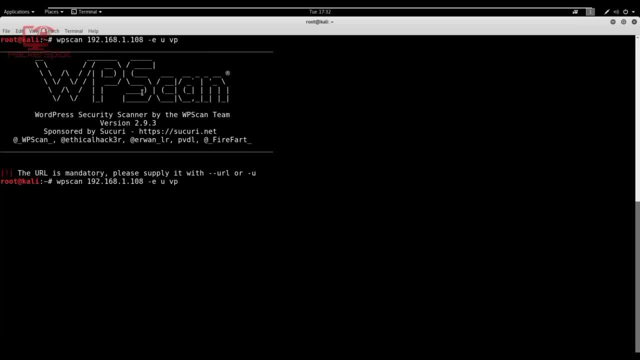 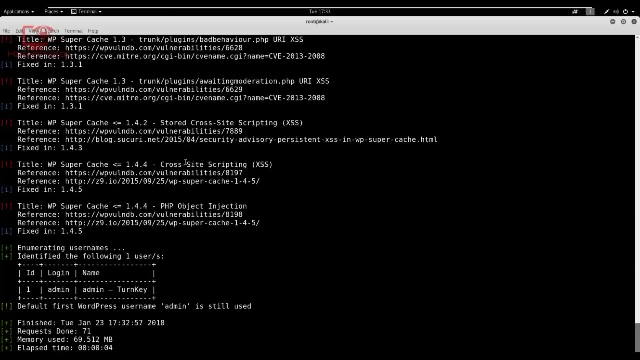 Oops, sorry about that. Oh, my bad Apologies. I forgot to specify the the U command there to target the URL. So once we hit enter, this should give us Alright. so there we are, And it's targeting the Oh immediately. we've got it Alright, awesome, As you can see. 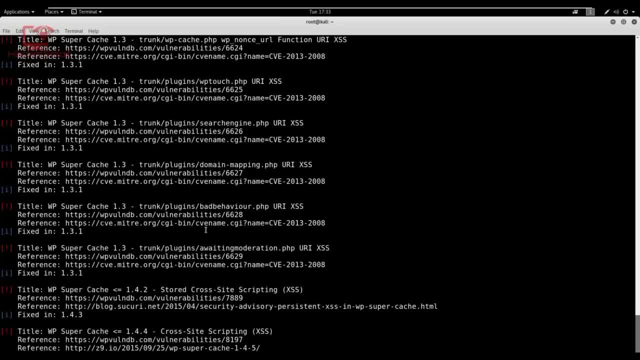 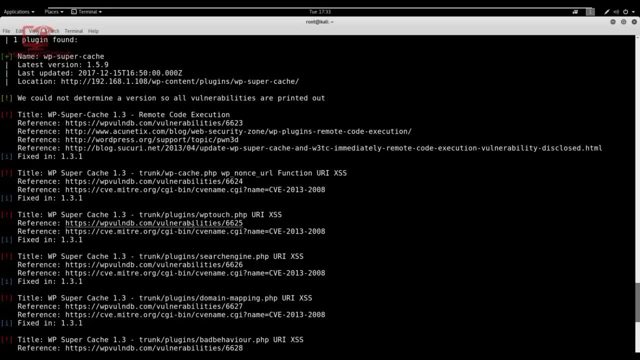 the default WordPress username is admin, So that's the really really easy way of targeting vulnerable plugins to find the username Again. you know, targeting the vulnerable plugins, it's super important And this gives you an awesome, as you can see, WordPress super cache. 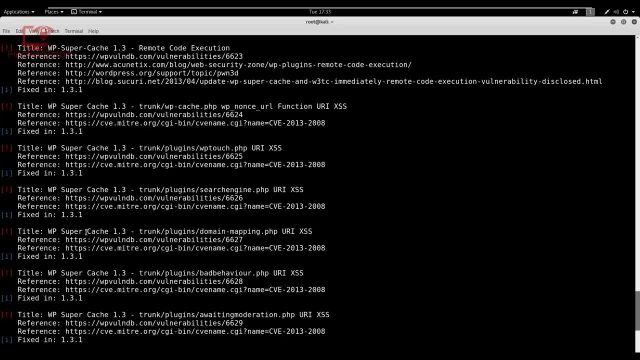 actually have used this plugin before And actually they've fixed these issues now, But this was something really, really big. I actually remember a lot of people exploiting this back in the day. The WordPress super cache essentially just speeds up your website and purges the files. 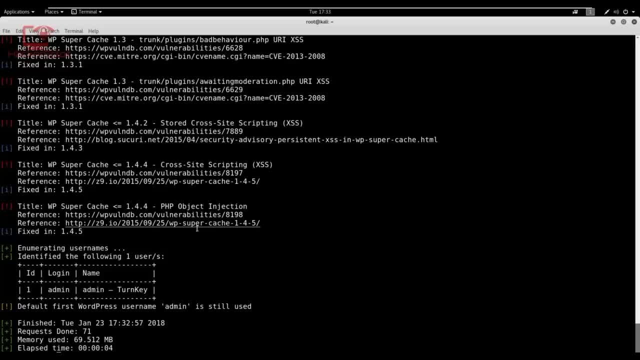 on your website to make it load faster. Anyway, as you can see, it's performed. it's enumerated the username and we have the username as admin- Fantastic. So we need to enumerate the password. we need to actually brute force for the password. 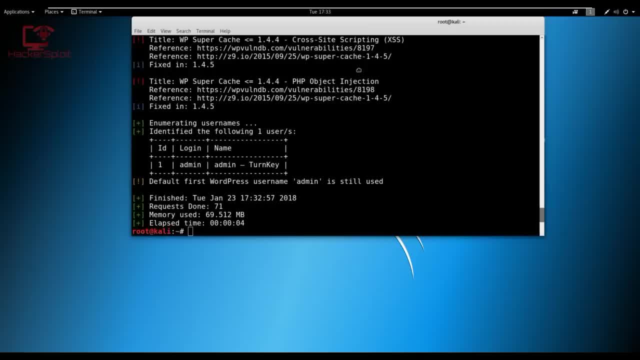 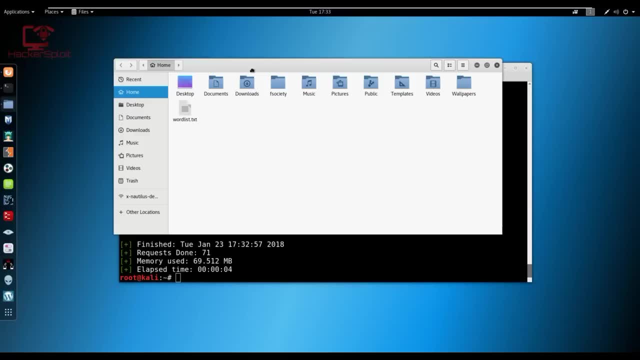 Right. So I already have a word, a word list that I've created or I had for him from a long time ago, And it has all the default username and password combinations for most of the top websites you know in the world, So, for example, Yahoo, Gmail, you know, Twitter, it's all of that stuff. 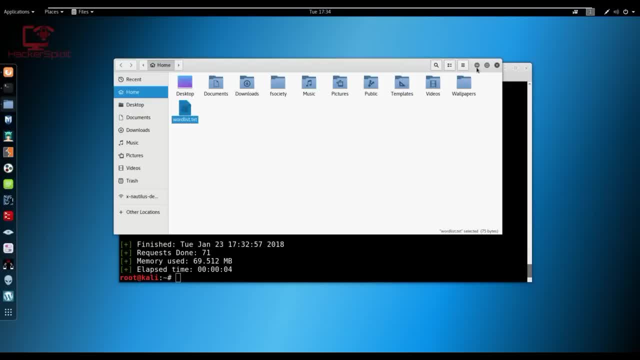 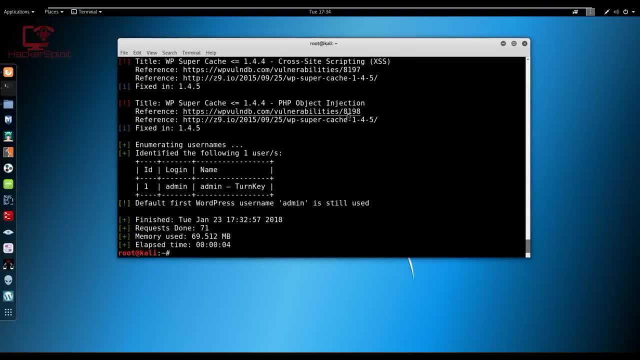 So I have it right here, And I've already modified it and sorted it so that it takes, you know, less amount of time for the WordPress scan to actually get the password. Alright, so I'm going to clear this out. So we've got the username and now we're getting 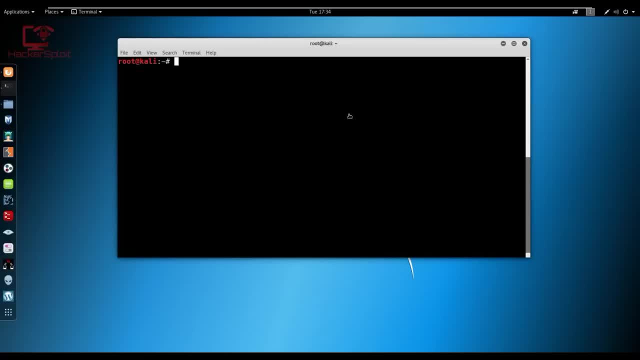 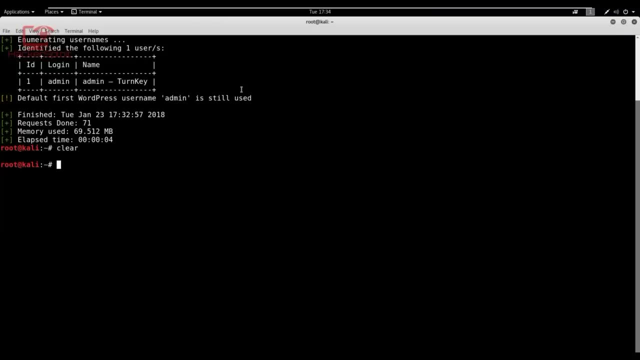 the password, Awesome. So now we essentially need to get the, the password. So WordPress scan. let me just enlarge the terminal here And clear that again: WordPress scan. there we are. WordPress scan you 108.. That's the IP address, or the URL, for that matter. Now we are also enumerating usernames. 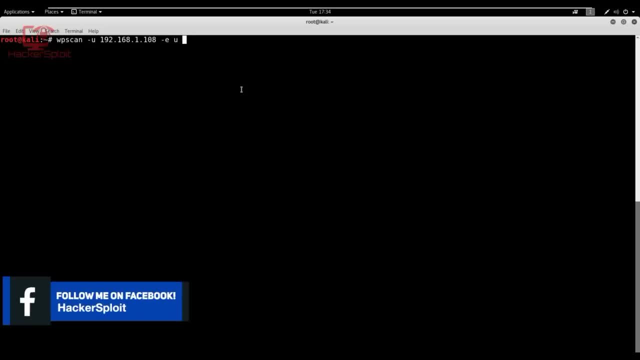 whoops enumerating the username, because it's also very important to enumerate usernames with the password combination. Right now we specify word list, So we are specifying a word list here, All right now. after we've specified the word list, we can then select the directory of the. 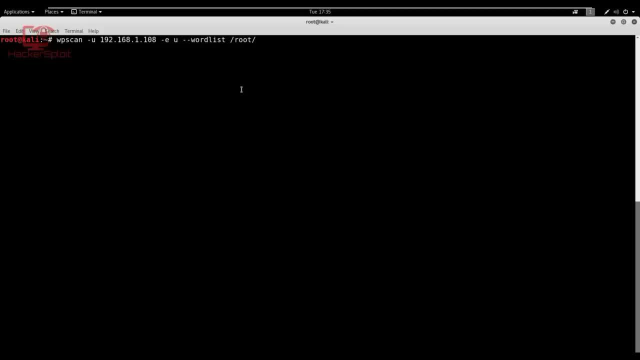 word list. Mine is in on my route And on my. it's actually an in my root directory, So I'm going to just select the word list dot txt file. There we are And let's hit enter And let's see what we get. It should actually do this really really quickly. 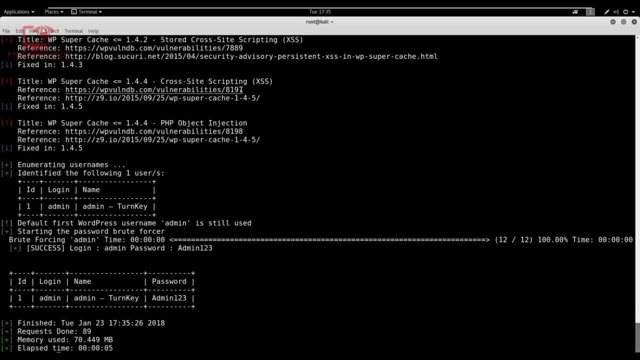 This, this word list is: Oh there, we are Fantastic. I did that really really quickly, And again it's used the brute force and it took like zero seconds. I believe there we are, So log in the admin. username is admin. password is admin 123. 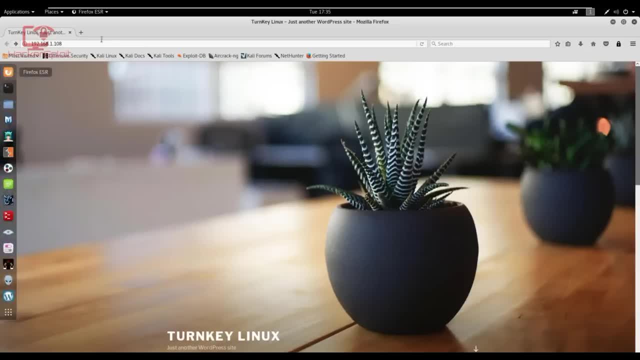 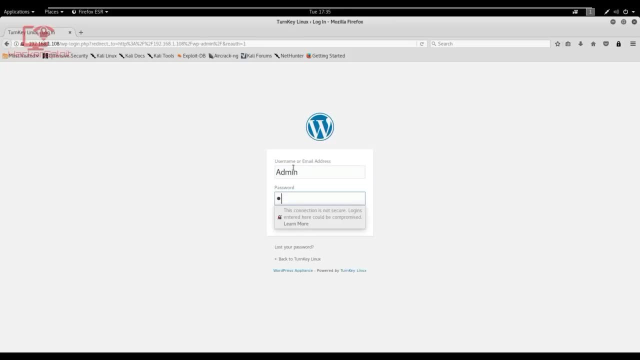 And let's actually try that right now. That was really really quickly. That was really really quick. So WordPress admin And the. the username is admin, password is admin 123, I believe are actually. I believe the username was admin with the lowercase, if I'm correct. 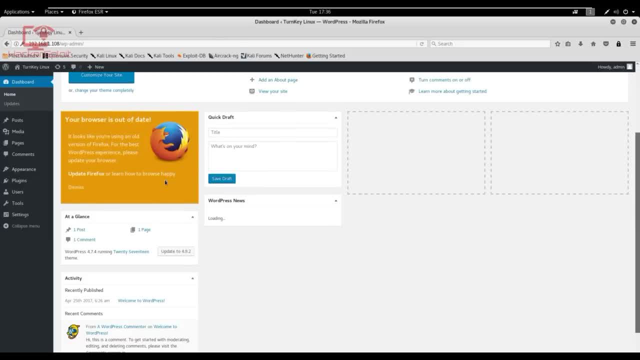 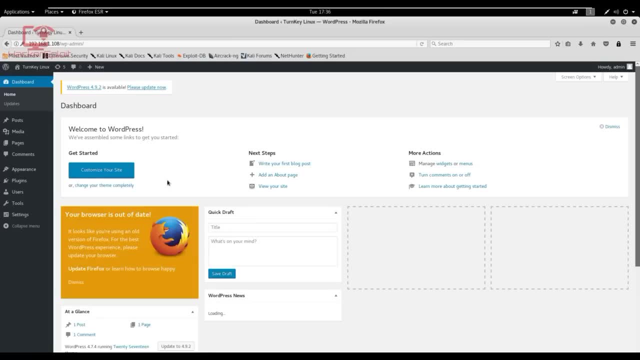 Yeah, I can actually see that it's telling me to there. We are alright And we have successfully. we have successfully explain that word right, know, granted that 60rån 60담, that it's running the. you know quite an old version of WordPress, WordPress 4.7, point four. 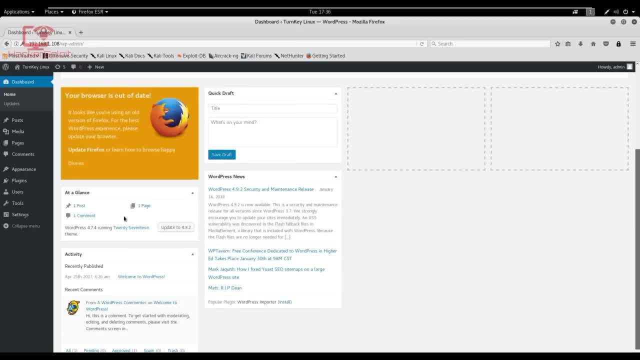 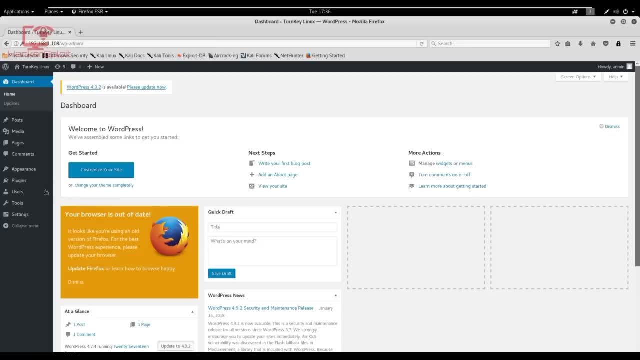 regardless of that, with with the plugins that it does have installed, we were able to exploit it really really easily using WordPress scan, And it's a fantastic tool really. Now one would go about usually what a lot of the black hats do is: they would go to plugins and they would add new. 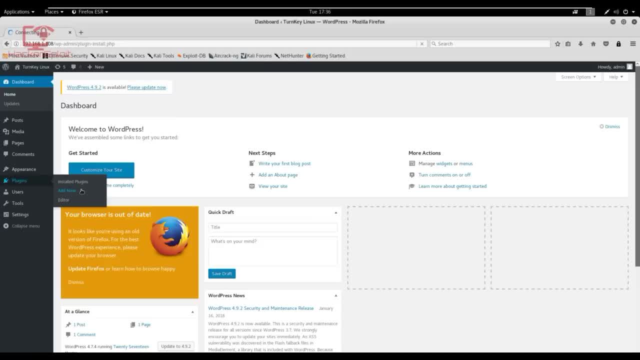 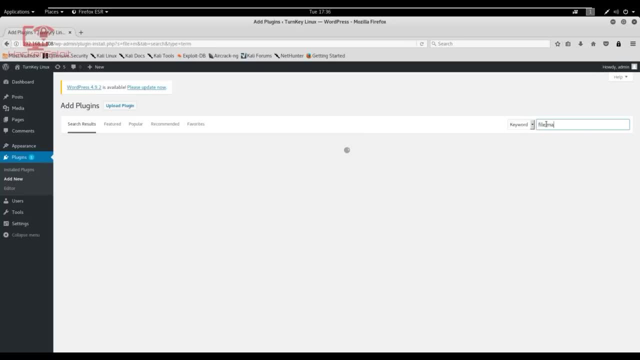 and they'll go to the file manager. Alright, so let me just show you this right now. We'll go to the file manager And they would look: whoops, they would actually install the file manager, go to plugins and install the file manager plugin, And then they would get a reverse shell and 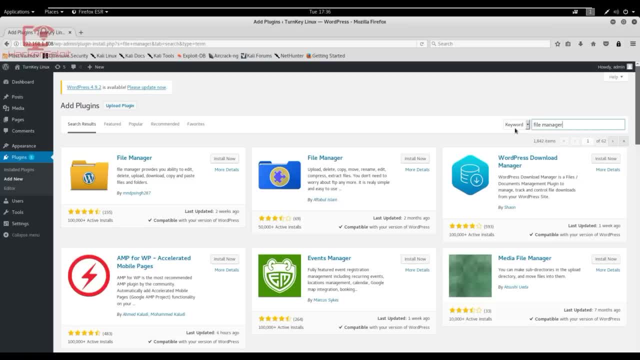 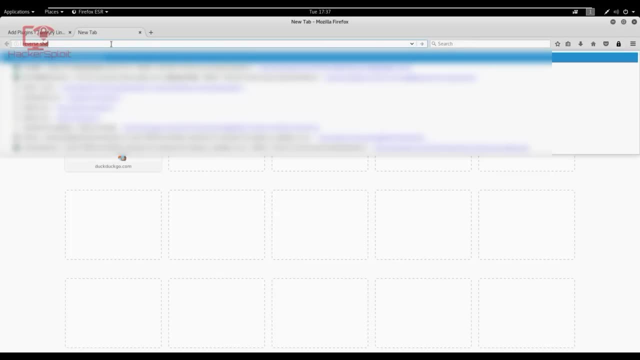 replace it with the 404 page and then actually trigger that page and the essentially have access or a reverse, reverse shell or a matter pretty shell, Alright. so they would install the file manager and if I just, you know, if I just search for reverse shell, oops, reverse. 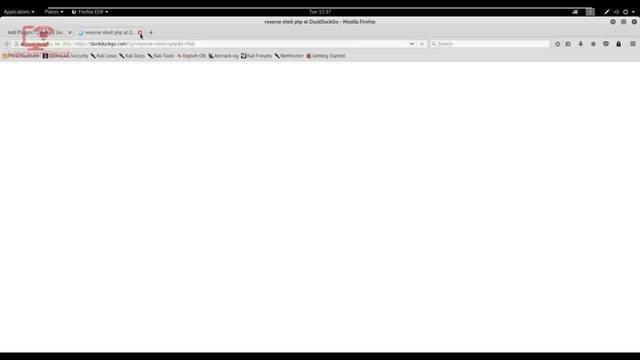 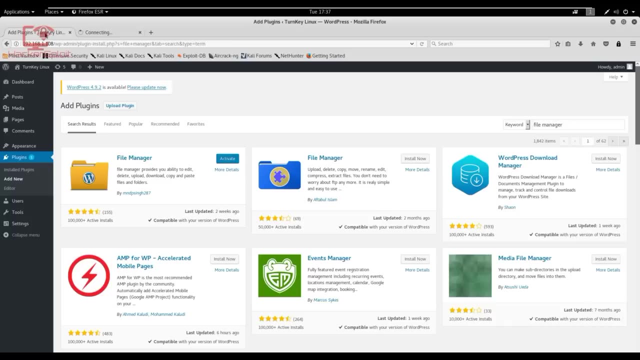 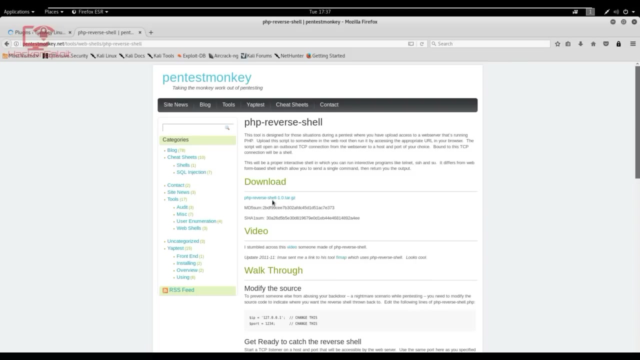 shell PHP. there we are, reverse show PHP, And this should actually return quite an easier. there we are PHP reverse shell. That's the one they use a lot. So I'm just going to activate the file manager here And I'm just going to download it. It's a pretty small file. I'm going to save it's. 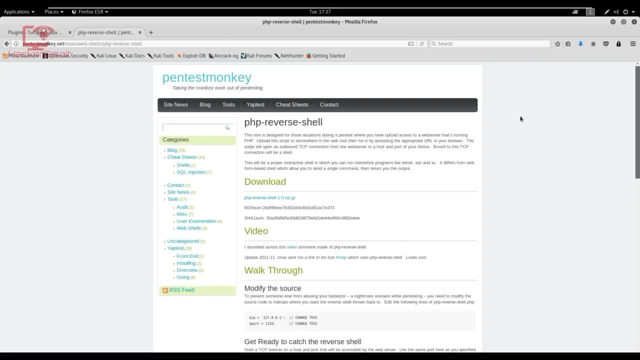 essentially a very, very simple PHP. Of course, it has to be in PHP because you're replacing the actual 404 PHP file. Alright, so there we are. I'm going to open it up And I'm just going to open this up And just open that up. Let me extract this here And we have the PHP reverse. 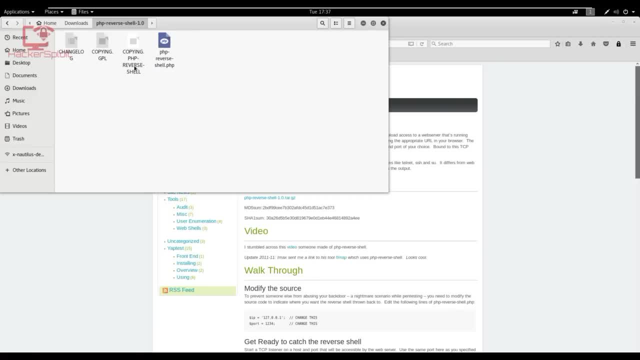 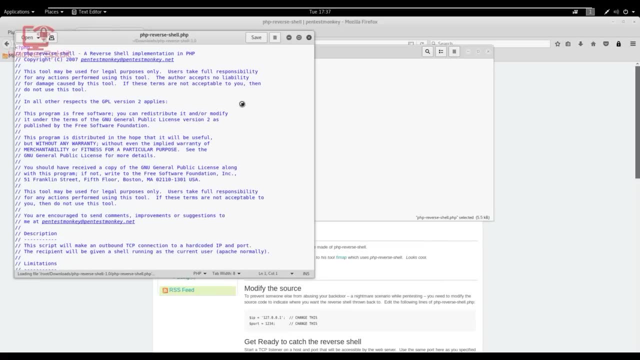 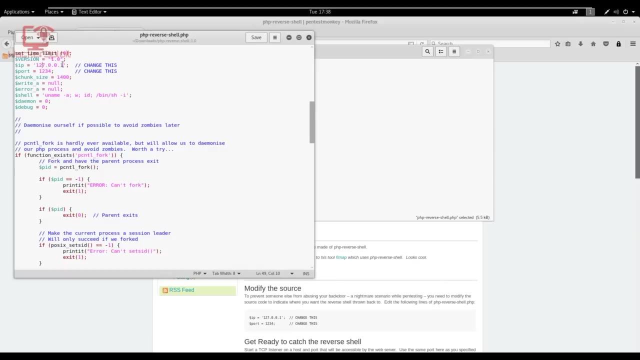 shell there: PHP reverse shell. copying the PHP reverse shell, You can read the read me and you can configure the PHP reverse shell obviously to connect to your IP address. here, As you can see, there's a few there. we are changing this, So the IP address, you essentially change that and the 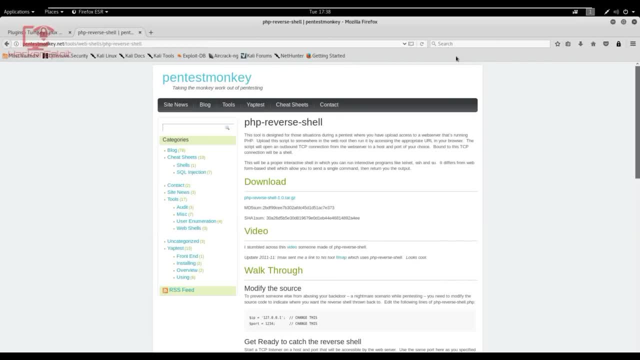 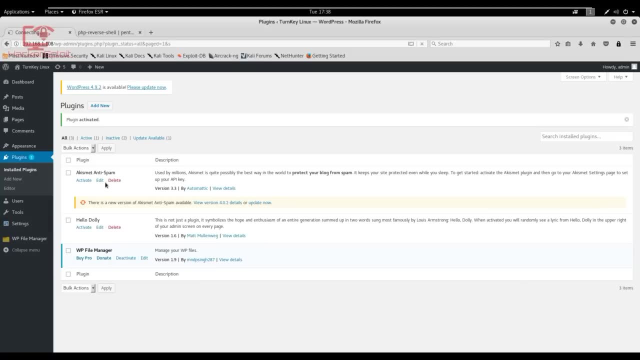 port you want it to connect to. And, yes, you upload it and replace it. You replace it with the editor here, settings, And you go to general. I believe is the general. Yes, you go to general or appearance and customize. There we are. appearance and editor. There we are. 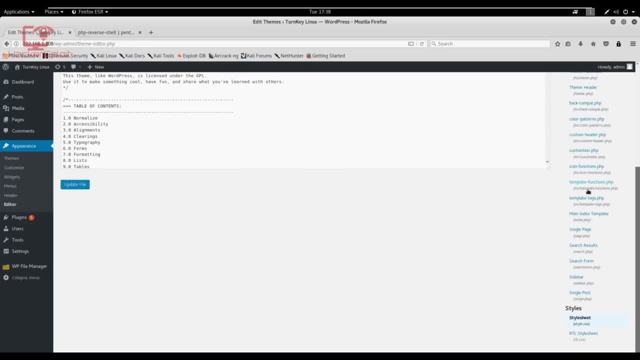 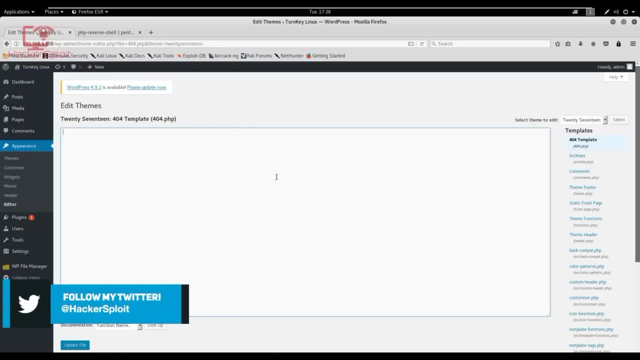 that's what we have to go to And one would go to the 404.. If I can find that, there we are for for template And they would replace the in. they would just get rid of all of this And they would replace this 404 script here and update the file. And what happens is when you go to, for example, 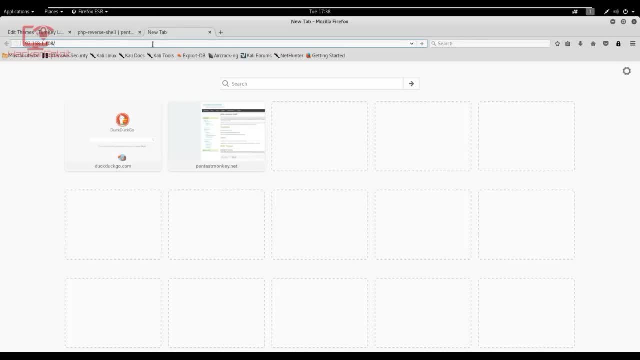 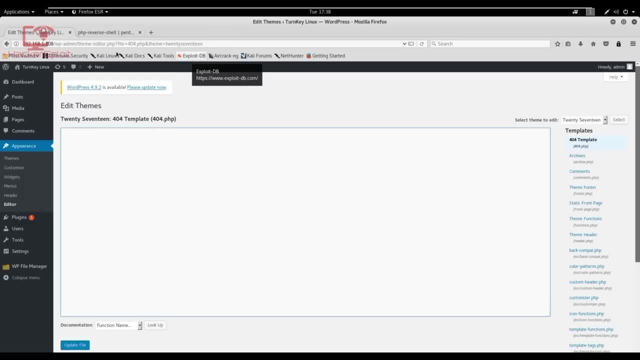 192.1, 68.1, point 108, and you go to the 404 page. there we are. it would essentially load the script And you know they go for a photo of PHP, for that matter. So that would grant you, you know. 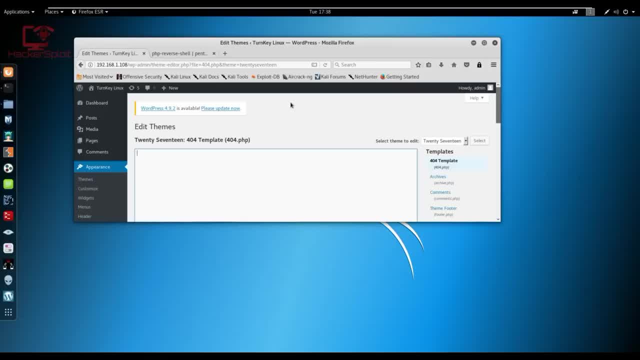 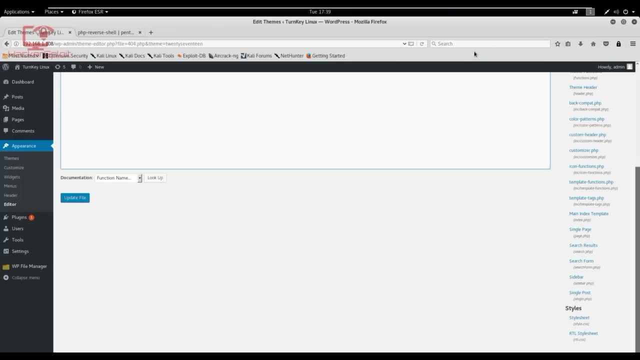 that would actually act as a backdoor into the WordPress system And they go. so that's essentially how to exploit a vulnerable WordPress system. I know this was quite basic But again, it's very important to understand the flow, the flow of content. 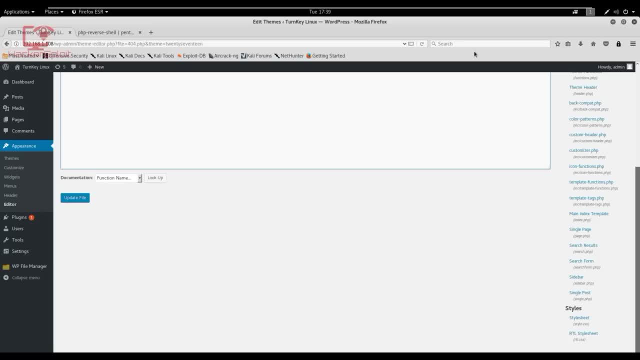 procedures and how things work. So we started off with enumerating usernames, passwords, and then we log in, and then you need to, you need to find a way to maintain access, And then there's clearing up your tracks, But in this case, in most cases, the black hat hackers will you know. just take 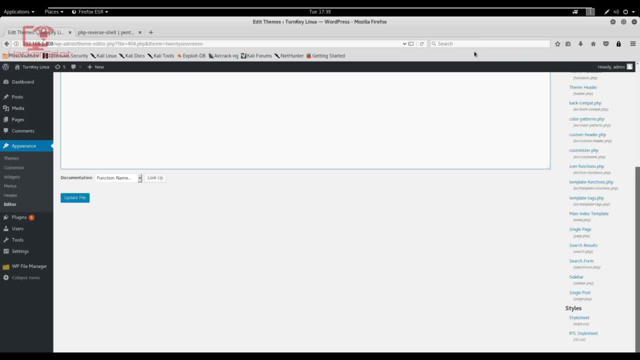 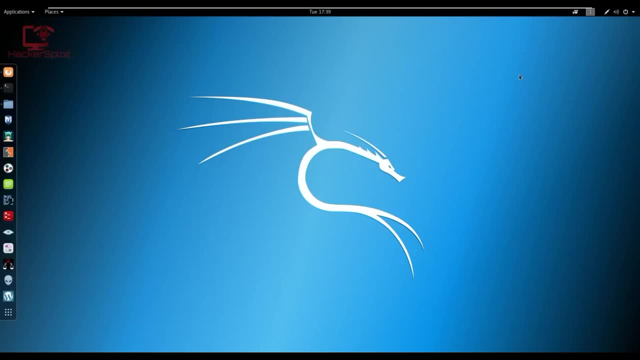 over the entire WordPress site and they claim responsibility immediately. So that's how it's done And hopefully this also gives you great awareness and a few security tips you can take away from this. If you're a WordPress site owner, get make sure all your subdomains are you know. 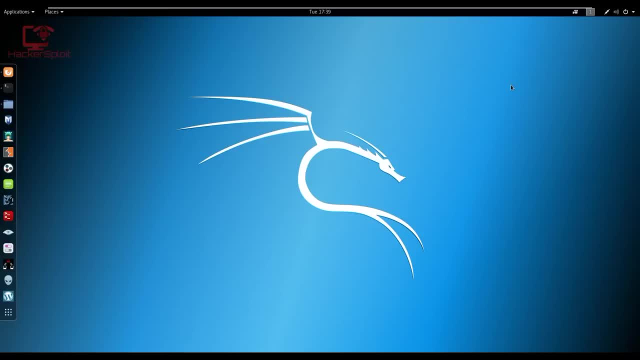 if you, if you have a subdomain and you're performing some testing on it and you know you're running some really some really really vulnerable scripts, please do not list them. just work on them in your own you know modularized environment and do not upload. 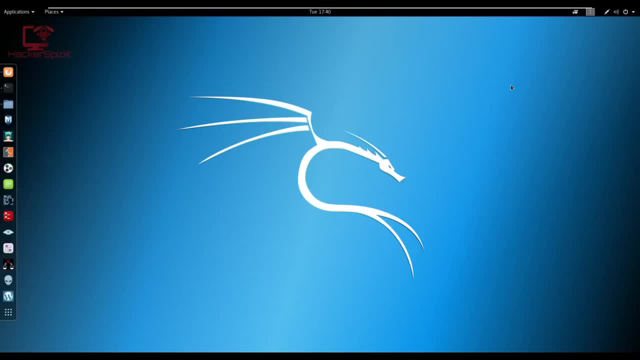 them to your server until they're ready Right. The next thing is to keep your WordPress updated and keep your plugins updated. That's very, very important, And I would really really recommend that you do not install any plugins that do not have good ratings. 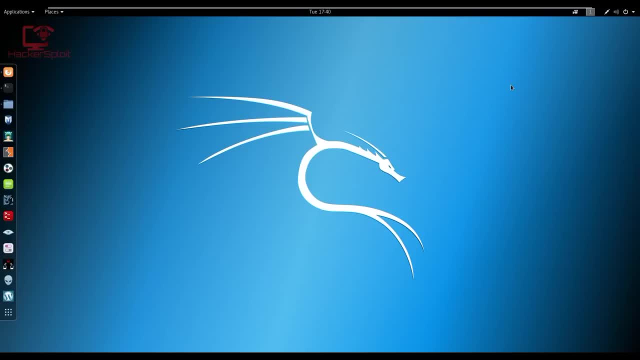 irregardless of whether or not they perform a task you know, really recommend that use the the most popular and the highest rated ones, because they are, they promise, the best security. All right, And the last one is to take regular backups of your site So that you know in case. 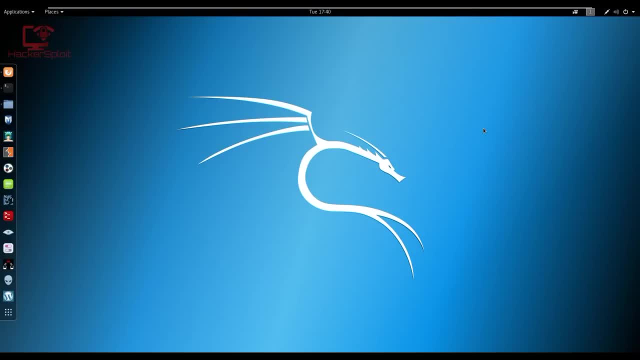 of anything, of any breach, any hack, you can easily- you know, you can easily- get ahold of your site and you can re upload it to another WordPress server and you're pretty much good to go. So that's going to be it for this video, guys. Thank you so much for the support. We are now pushing for 50,000. 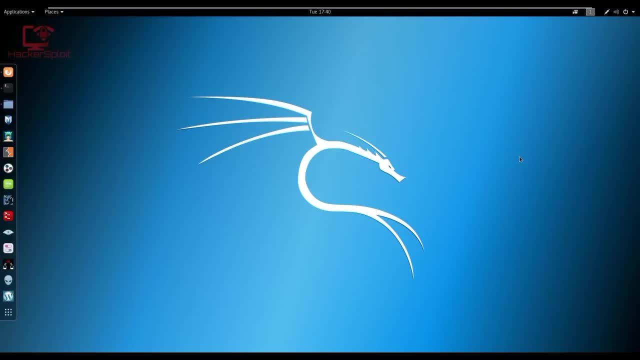 subscribers. I appreciate all the support And you know it's time to get work videos every day. And yeah, if you found value in this video, please leave a like down below. If you have any questions or suggestions, let me know in the comment section Or you can hit me up on my social. 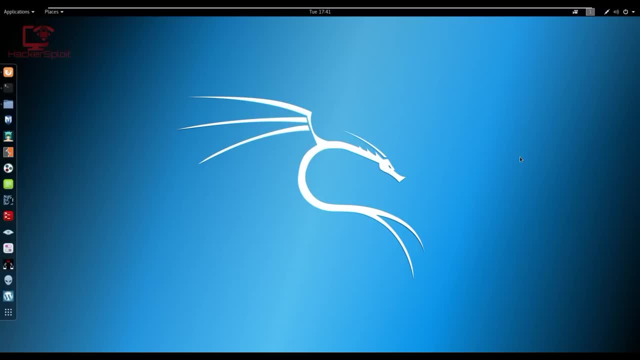 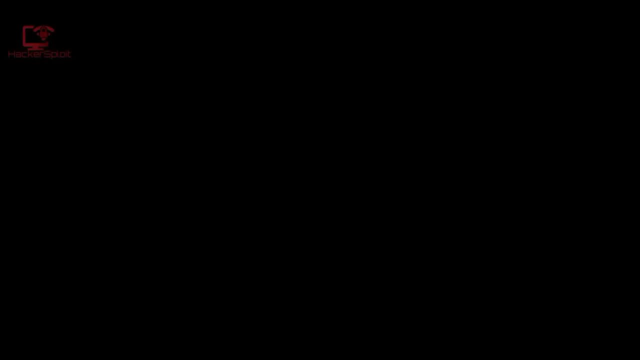 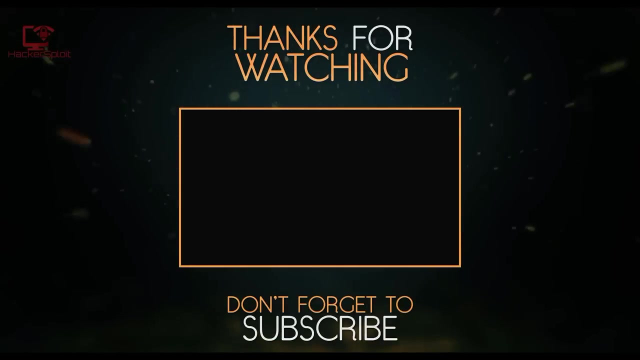 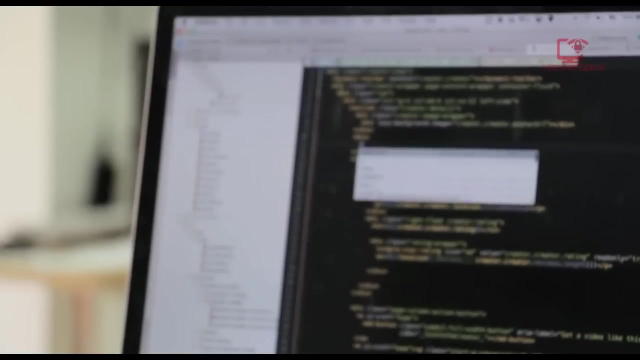 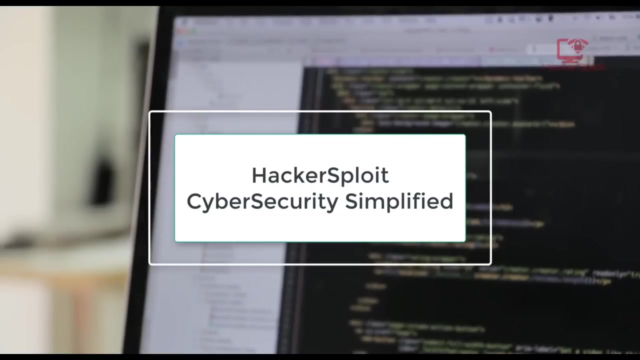 networks or on kick And you can get the latest hacking news and resources on my website, HS. plug it and I'll be seeing you in the next video. Peace, Yeah, Yeah, Yeah, Yeah Yeah, Hey guys Hackers. 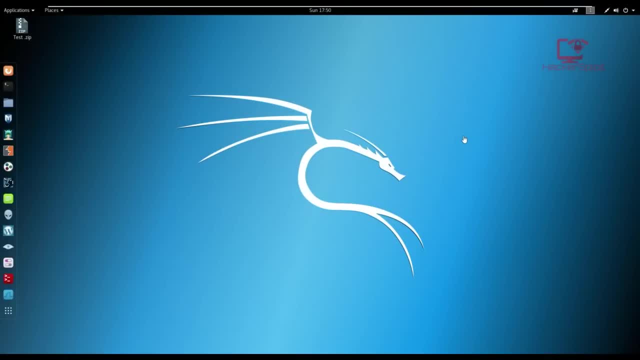 Mommy, Damn, Gotta get in with another video, And in this video we're going to be looking at password cracking, more specifically, password cracking with john the Ripper. Alright, so a lot of you guys have been asking me for this. 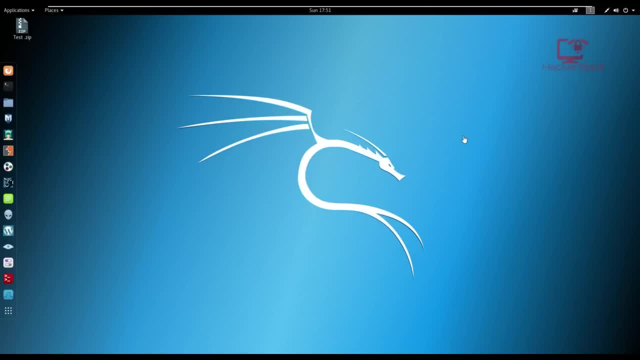 And this is probably a very, very important section that I realized that I haven't covered before- And obviously this section is password cracking, more specifically, password cracking using john the Ripper. Alright, so john the Ripper is a fantastic password cracking utility, that is. 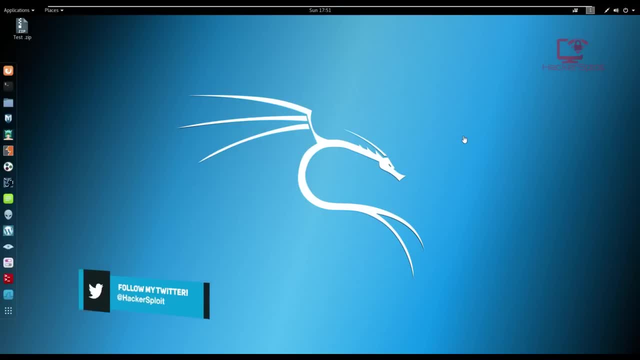 used to crack in our passwords, system passwords, etc. etc. It's also very, very good for password hash cracking. Now, for those of you asking for the more advanced videos on the channel, do not worry at all. I was planning this for a long time And I've really, really listened to. 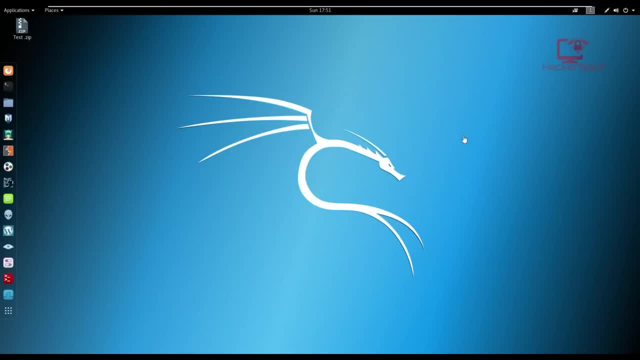 what you guys have had to say. And yes, on the channel and you know, until now I haven't covered a lot of advanced videos And that's because I wanted to fully cover the beginner video so that anyone who watches the channel can go through the beginning tutorials and then get. 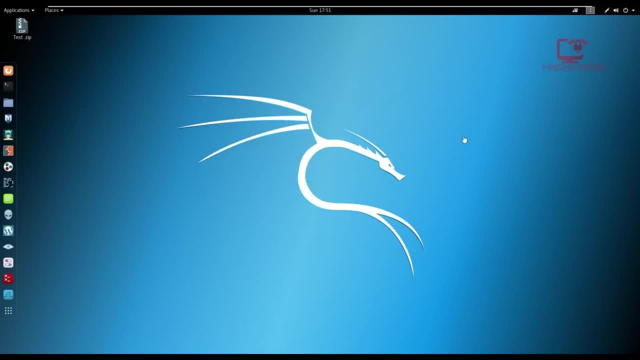 competent enough to move on to the advanced series. Now, for those of you already advanced enough in this field, you want to see advanced videos. don't worry about that. I've been working on the web penetration testing series and some more other advanced series, And I was scheduling. 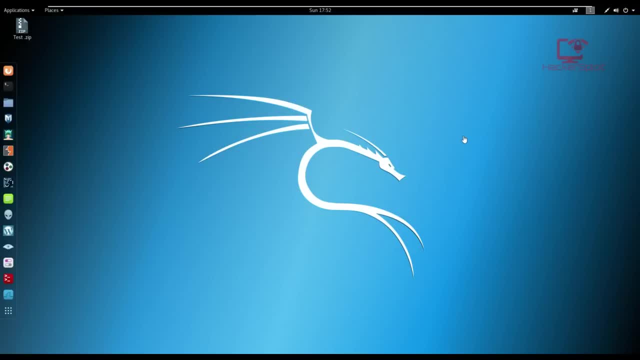 to upload the videos at the beginning of March, But since you want, since you want them early, what I'm going to do is I'm going to start uploading them from this week, from one day onwards. Okay, so I've actually recorded and edit them, edited them And now I'll move on to 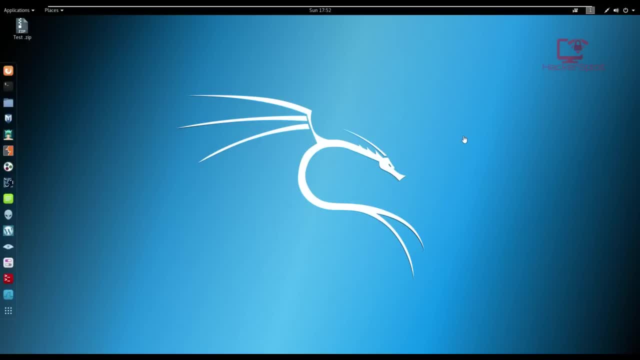 to actually uploading them. So again, thank you so much for waiting. You know, I just wanted to make sure that I covered all the basics first and obviously I can cover both sides of the spectrum where you know beginners can find. 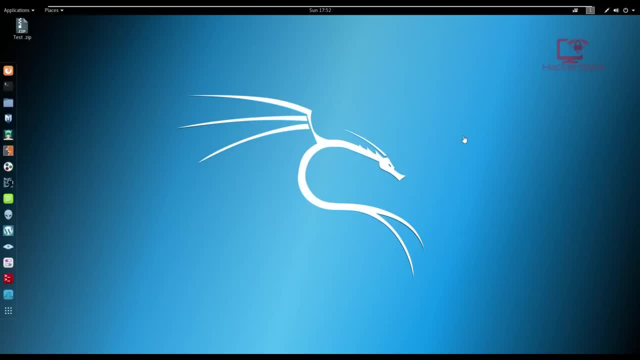 value on the channel And also the advanced users can find value on the channel. I really value both, both both experience levels, if that's what you, what you want to call it. So you know, beginners should not feel intimidated at all And the advanced users should not feel like the channel. 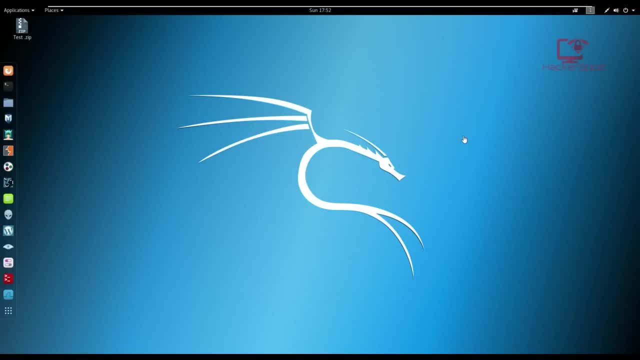 is becoming very, very basic in terms of the types of videos I'm uploading. So you don't have to worry about that. I'll be uploading the advanced videos, So I'm going to try and get a balance. Anyway, as I said, I've not really covered the password cracking section. 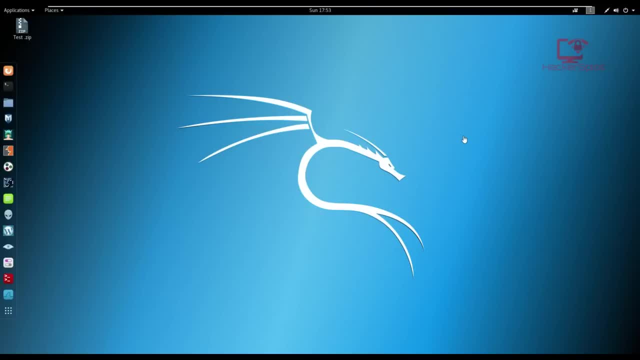 And today we're going to be looking at how to crack the zip and raw passwords with John the Ripper, Alright. so the surprising thing is not many people or people actually find this really complex because you know they don't understand the password, the the password hash cracking. 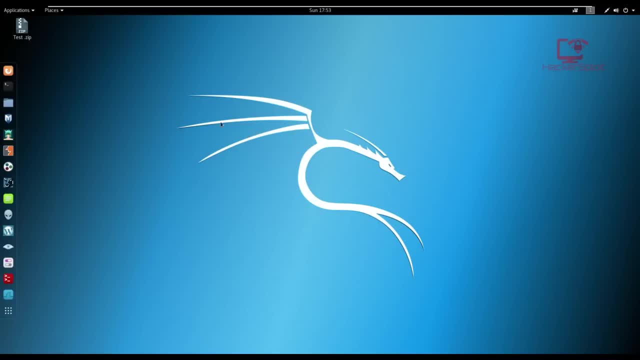 process and how the cracking process works Alright. so, essentially, John the Ripper is a fantastic tool that you know, in its full power, is great for cracking password hashes, And once you crack a password hash, you essentially get the password. Now, in this case, 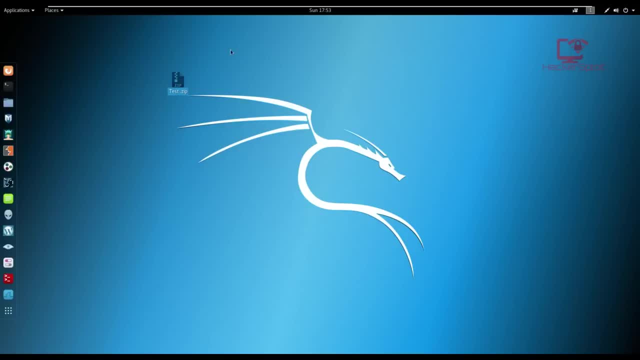 I have an encrypted zip file here that is encrypted behind a password. I created that on my Windows operating system and I just give it a. I don't even remember what password I gave it. I probably gave it a very, very simple password. And that's because, again, depending on the complexity of the 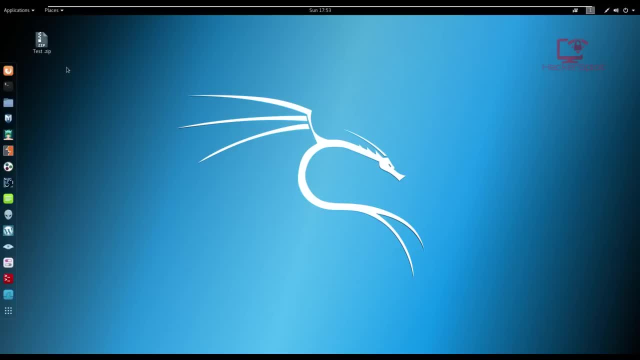 password. you're cracking the, the. the process can take, you know, a short, short time to a longer time. If the password is more complex, it's going to take longer. If it's less complex in terms of the character set that you're choosing to use, 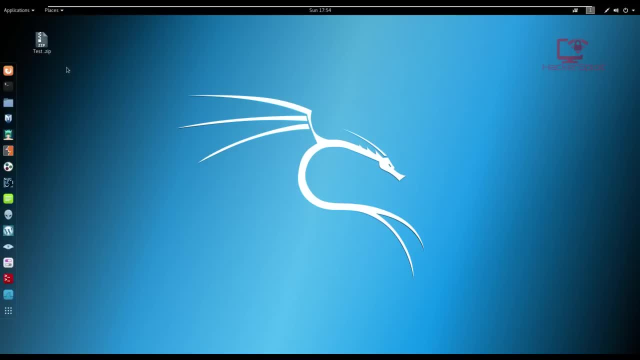 then obviously it's going to take a less amount of time. if the amount of characters is is limited, or you know you have more characters and it's the you have the use of numbers and symbols, then obviously the process is going to be longer. But enough said, let's get started with John the 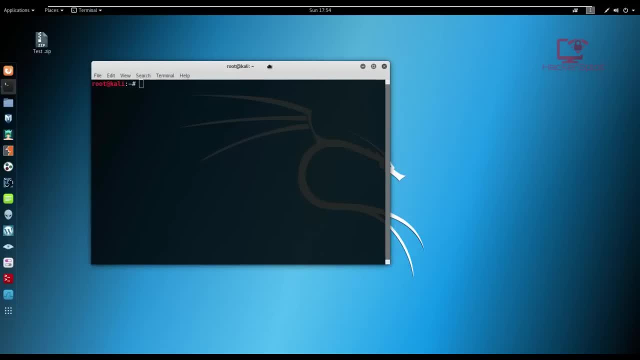 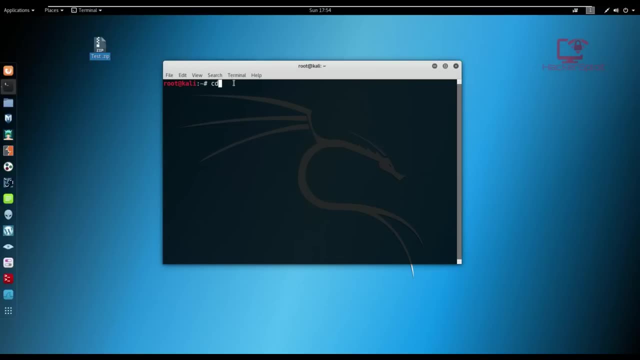 Ripper, Right? So John the Ripper is pre installed on Cadillac, which is awesome, And, as you can see, I have the test file on my desktop, So I'm just going to browse to my desktop here. So change the desktop change directory into my desktop And we'll clear that out. And now we can get started. 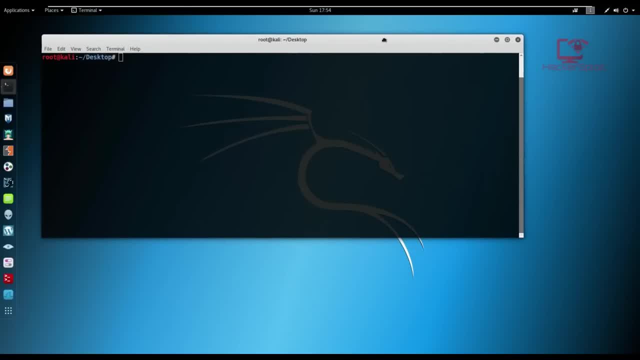 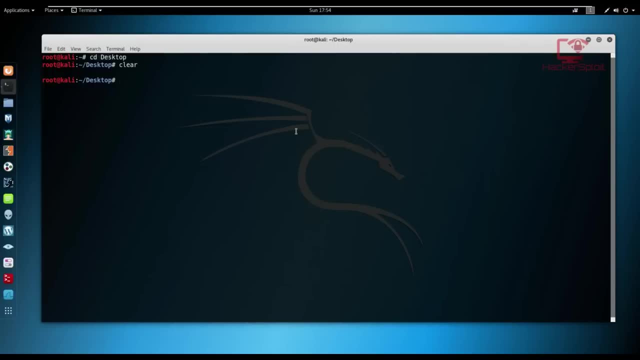 with the process. So the first thing we need to do is we need to get the password hashes, And that can be done by using a tool called zip to john. it is part of the the john the Ripper package, So let me just show you what it's used for. It's used for getting the password hashes. 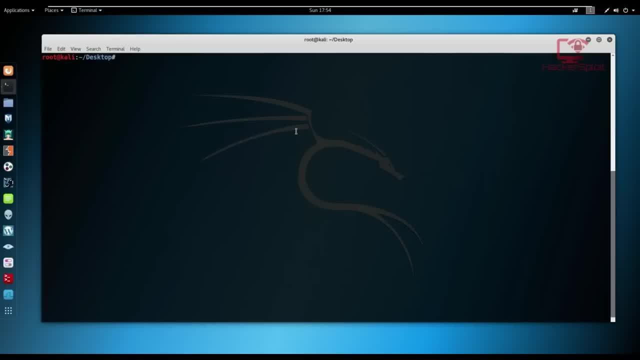 Now, depending on whether or not you're using a zip file or a RAR file, the process is still the same or it has a utility for both of these processes. So if you're using a file or you want to, you want to get the password from a zip file. the first thing we need. 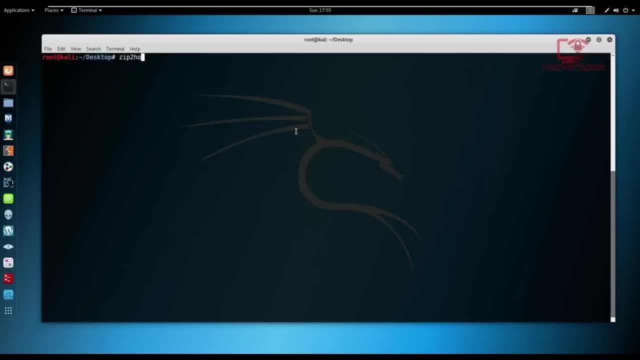 to do is we need to use zip to john? alright, so zip to john. sorry about that, zip to john. And then after that we specify the file And then, if we hit enter, it's going to give us the password hash, or we can output the file into a txt document, which is the preferred way of doing. 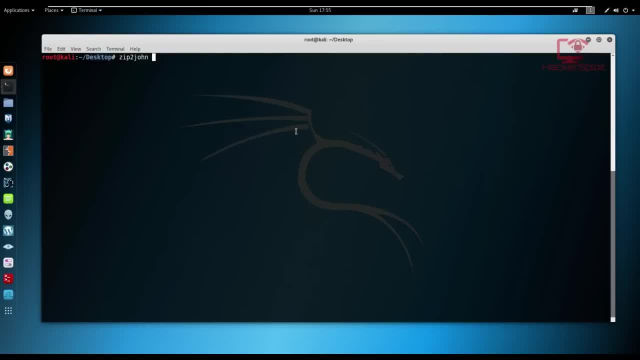 so, Once you go into becoming a penetration tester, it's very, very important that you save all of the results that you're getting and everything that was involved in the process. So, again, this is why I was talking about you know, really, really covering the basics. 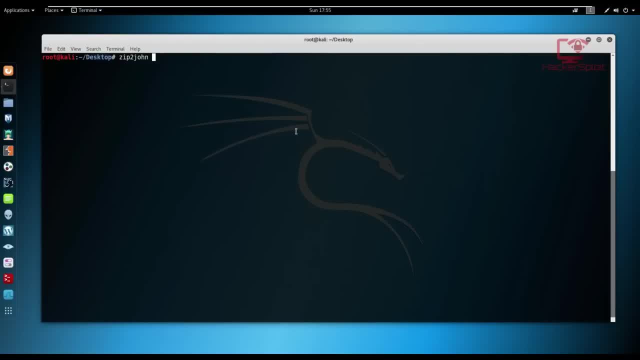 so that people learn you know penetration testing the right way, Alright. so, as I said, if you're using a zip file, you can use zip to john. if you're using a RAR file, you can use RAR to john, Alright. so the process is relatively simple. In this case we're using a zip file, So 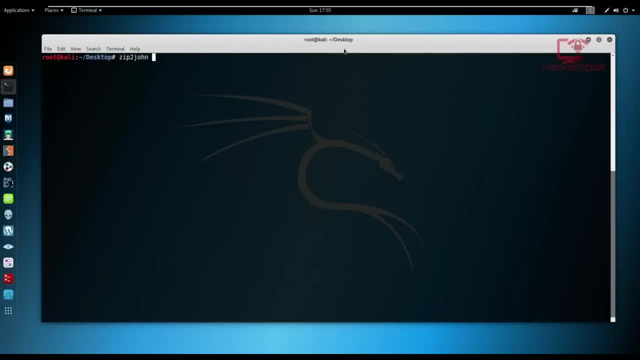 I'm going to use zip to john And then now I'm going to specify the file name, which in this case is called test dot zip. So I'm just going to test dot zip. Whoops, sorry about that. test dot zip. 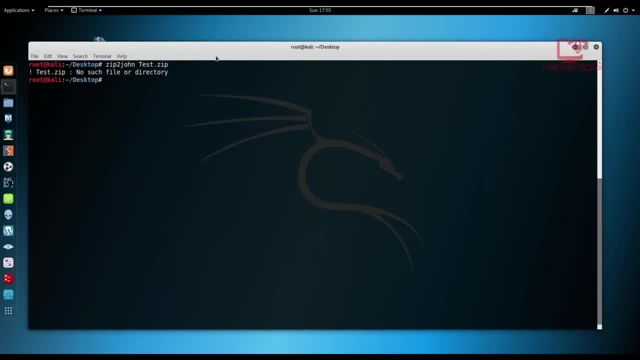 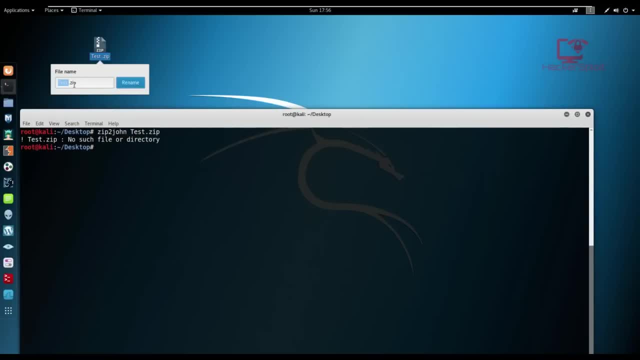 And once I've specified the file, if I hit enter now it's gonna oops. for some reason we've got an error there. Oh, there is a space in there, So let me just see if I can rename this and get. 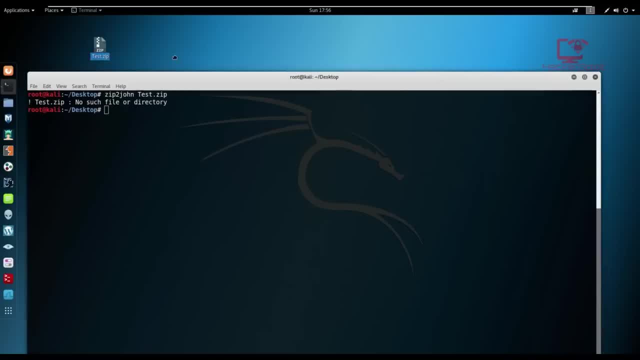 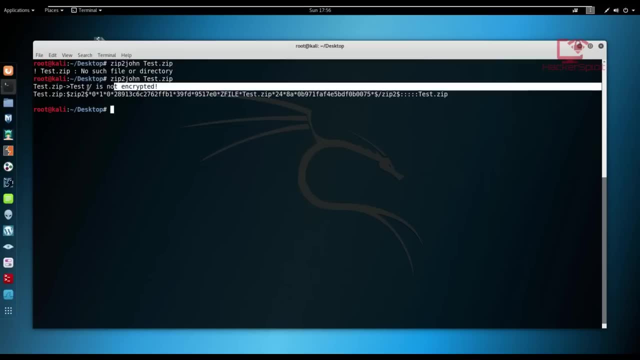 rid of the space between there. There we are, let me just rename it: Fantastic. Okay, so now we can go zip to john test dot zip Now. once I hit enter, it'll give me the password hash, don't worry if it. 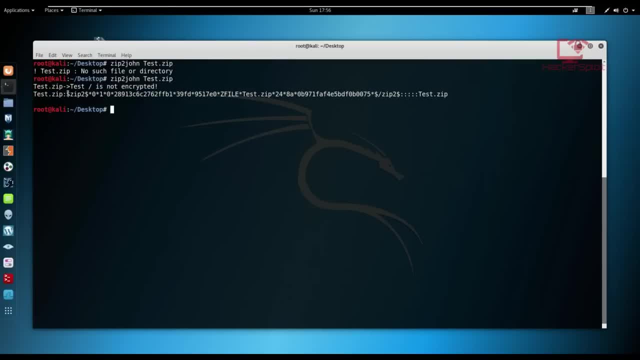 gives you the error that the the file is not encrypted. Regardless, the password hash starts with a dollar sign. that is a hash, So it ends here, or actually here, Alright, so it starts with the dollar sign and ends with the dollar sign. That's how you know what a password dash is. So now we 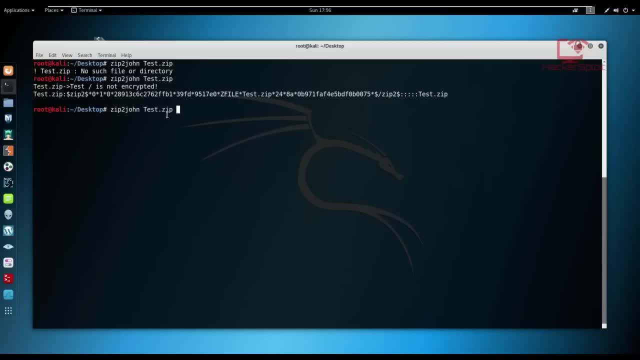 need to crack this. But first I want to export it into a txt document. So to do that, we just use the output denoter, which is the greater than sign, and we give the name of the, the document In this case we're using. we're storing it in a text document, So I'm just going to call it hash, oops. 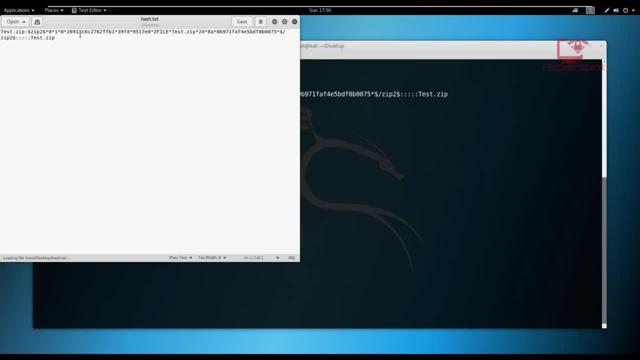 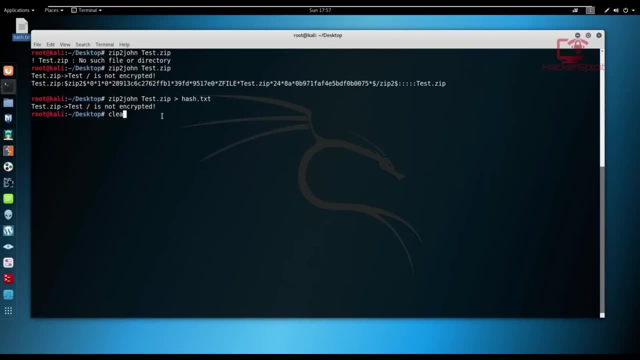 hash dot txt. I'm going to hit enter, Save the hash for us in here. There we are fantastic, And now we can get started with the password hash cracking process. I'm just going to clear the terminal now And we can use john So. 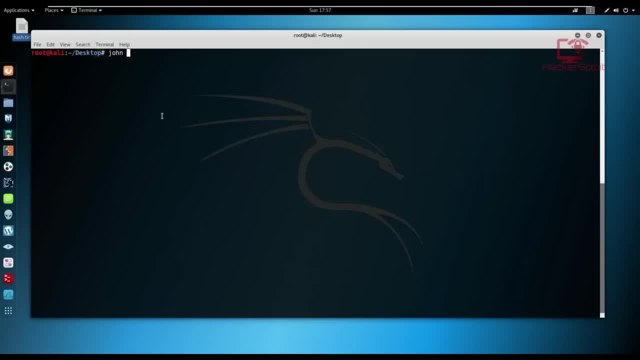 now we have to use john And we now need to select the format of the of the file that we're trying to crack, and then specify the hash or the, the document that contains the hash. So we say john, and then we use the format denoter, So that is the format command And that is denoted by a double. 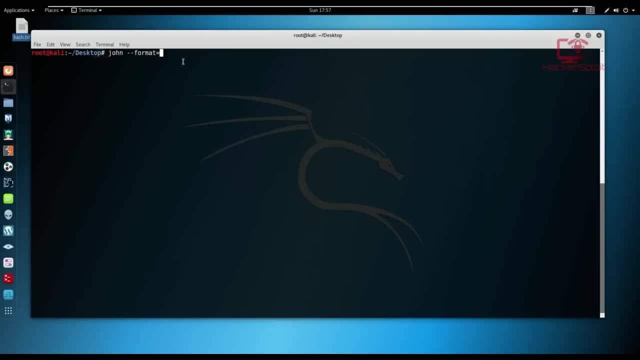 dash and format: Alright. so after that we then say: format is equal to zip. Now again, if your file is a raw file, the process is the same. you just need to change this into a raw, Alright. so in this case, 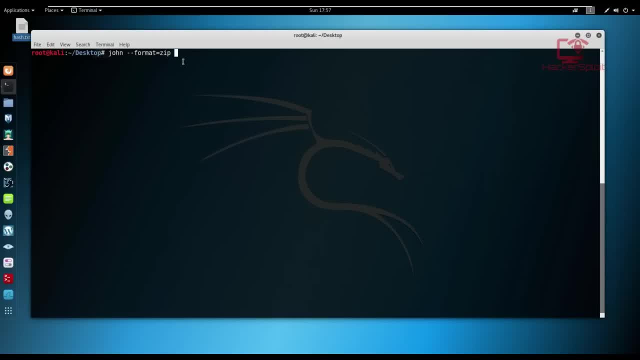 mine is just zip And then now you have to specify the hash. So if you have copied the hash you can just paste it in yet here directly. In this case we have saved it. on documents, I'm just going to specify the document name, So hash dot txt, and I'm going to hit enter And the the password hash. 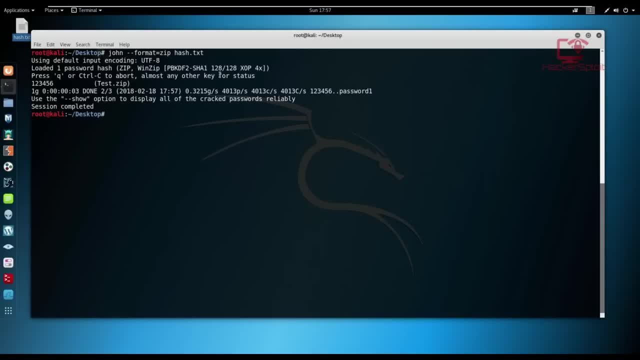 cracking process is there. As you can see, it was a perfect, perfect, perfect, perfect, perfect, perfect, perfect. As you can see, it was performing the cracking process and it got it in a few seconds And, as you can see, the password is really really simple: 123456.. Now, the reason I chose this is: 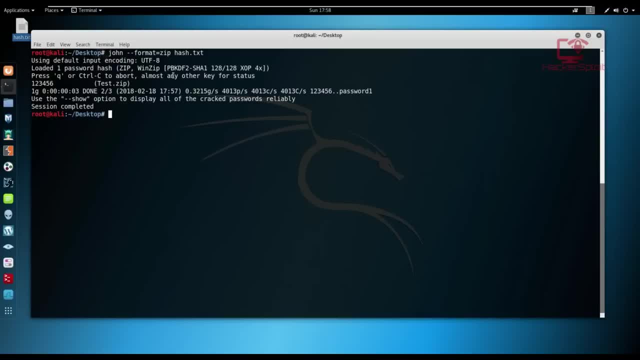 because, again, I did not want something very complex, otherwise it would. it would have taken a longer time, And that is the thing you need to understand about password cracking. Even when you use tools, when you're cracking, you know logins like the SSH login. 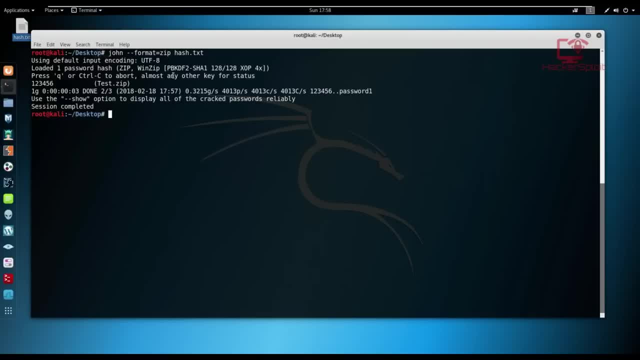 and you're using tools like Hydra. the process is quite quite a while, you know. I remember you're cracking passwords when I was learning or when I was, you know, in my first job. the process- the password cracking, you know- took almost probably about 12 hours. So yeah, 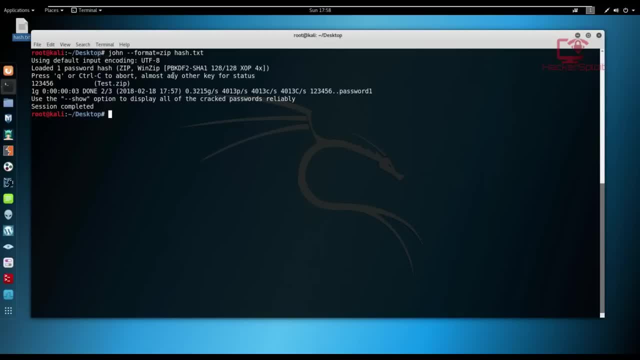 it's going to take a while, And that is the probably the thing about password cracking. whether you're performing a brute force attack or you're you're trying to crack against passwords, logins, you know, or even if you're using a dictionary attack, you know. 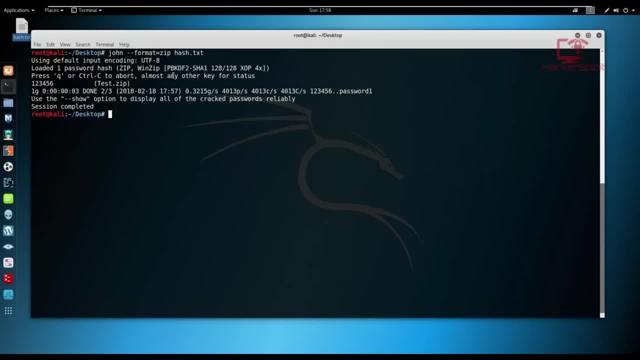 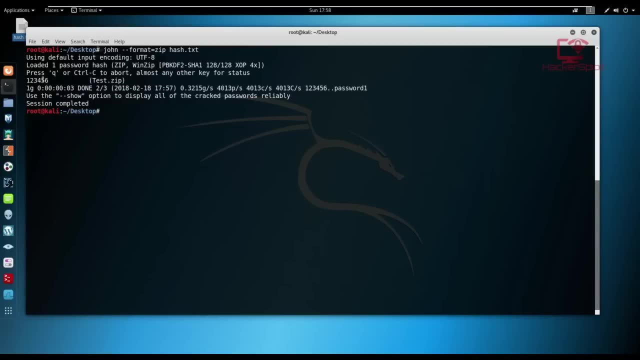 it's. it's pretty much just about time. Alright, so that is how you to crack a zip file or a RAR file. the process is still the same And there's your password. So now we know the password is 123456.. Let us confirm that by actually trying to extract our file here. So I'm going to hit. 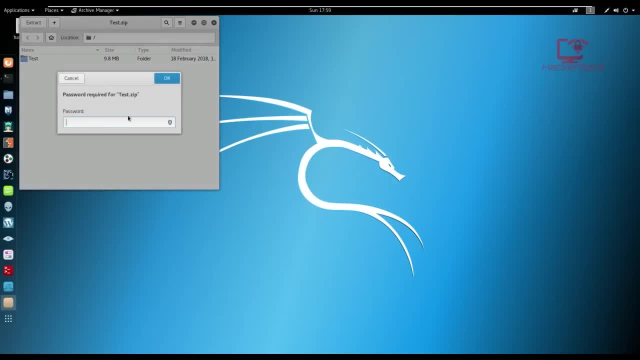 extract here. I'm going to extract to my desktop. there we are extract and I'm just going into the password And I'm going to hit OK And there we are. extraction completed successfully. Fantastic, we can close that up. And in my test file I just had some really basic files. Yeah, 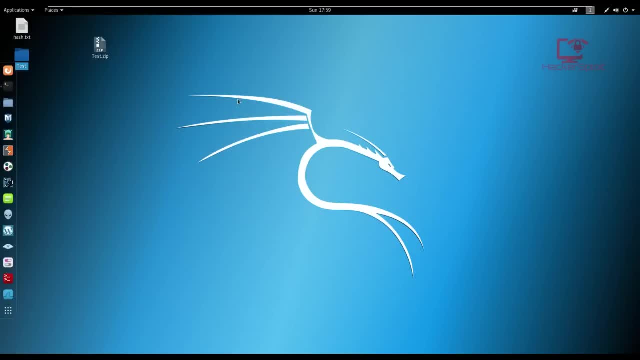 there's a setup there just for synergy, which is awesome, Alright. so one more extra thing. I'm going to give you guys an extra bonus: I'm going to show you how to crack Linux passwords with john. Alright, so with the thing about Linux passwords is Linux passwords are. 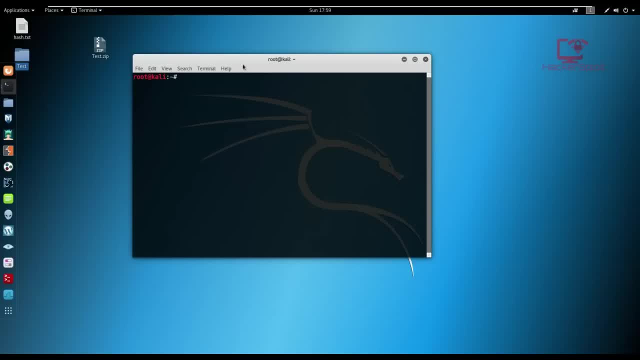 stored in the etc and the shadow folder. Alright, so I'm pretty much most of you are familiar with that. those of you who are advanced users should be familiar with the file structure of the Linux file directories and where the passwords are stored. But the thing about them is the file is encrypted. 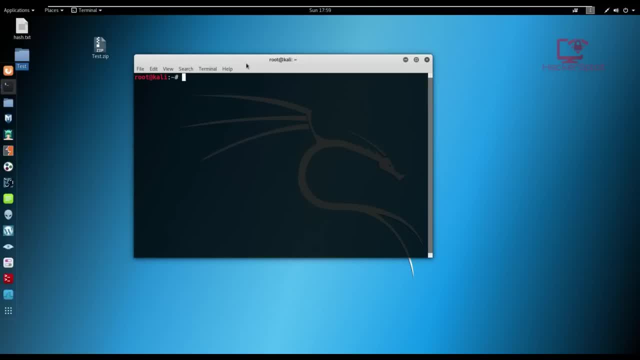 so you need to crack it. So, by default, what I'm going to do is I'm just going to create a user, So user add, and I'm just going to say the user username should be: let's just call it user user two. 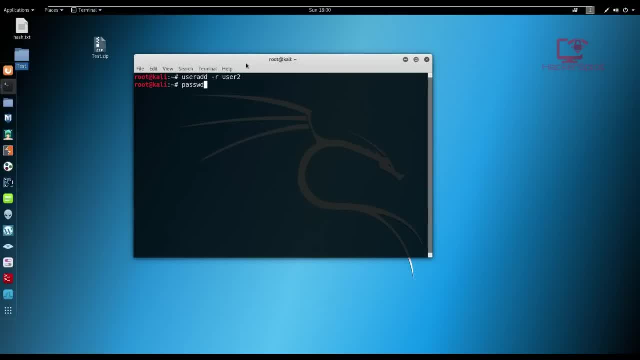 alright, I'm going to hit enter and it's going to add the user and I'm going to change the password of user two. So essentially, what I'm doing right now is I'm just creating a user and a password and I'm going to show you how to crack it. Obviously, the Linux usernames and passwords- 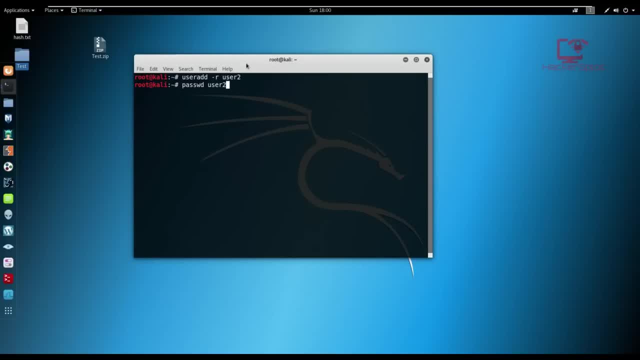 so you can actually crack the passwords that belong to all the accounts on the Linux operating system. So I'm going to give it a password. So it's going to ask me to enter a new Unix password. So again, I'm just going to enter a really, really simple password. 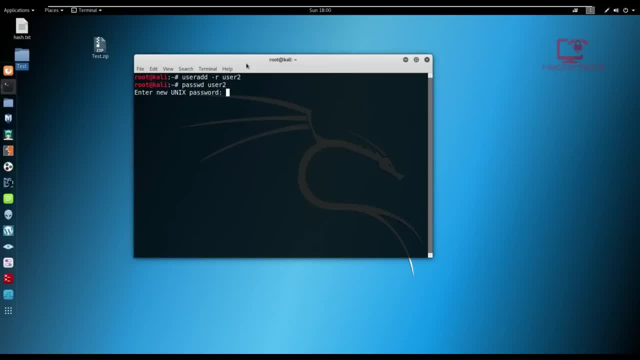 1234567.. Let's make it a bit complex, So 1234567.. And I'm going to hit enter And there we are. password updated successfully. So to crack the, to crack the, the shadows file. the shadows file exists in the, the, etc. And, as you can see, if you specify the shadow file, you can see that the 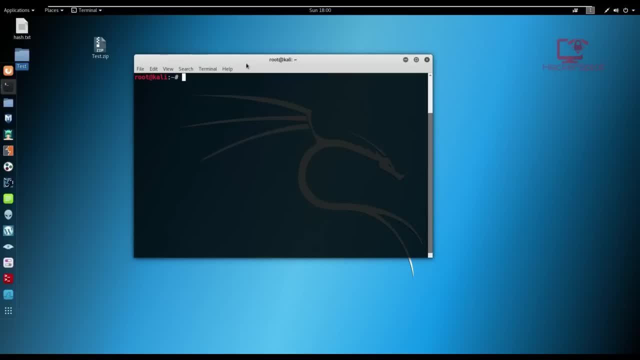 shadow file exists in the, the, etc. And, as you can see, if you specify the shadow file, the shadow file exists in the, the, etc. And, as you can see, if you specify the shadow file like this, the etc. shadows file, you will essentially that that is where all the passwords are stored, So we can use. 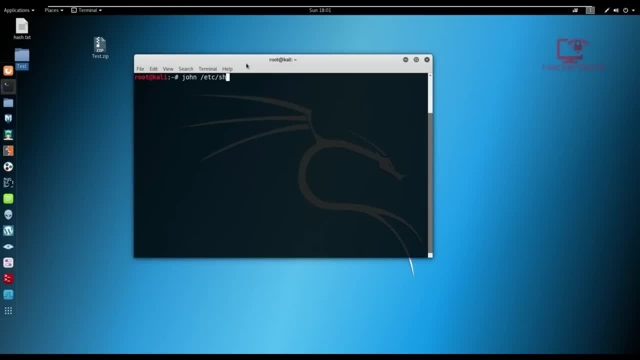 john, And we can say, etc. Shadow. If I just open that up, there we are shadow. there's a shadow file Again, by the way, it is a file, So we just hit shadow And once we enter, it's going to start. 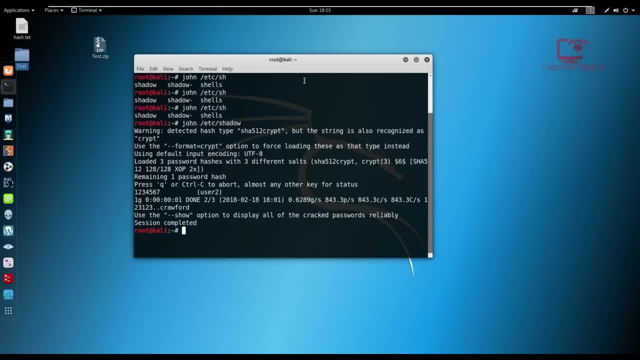 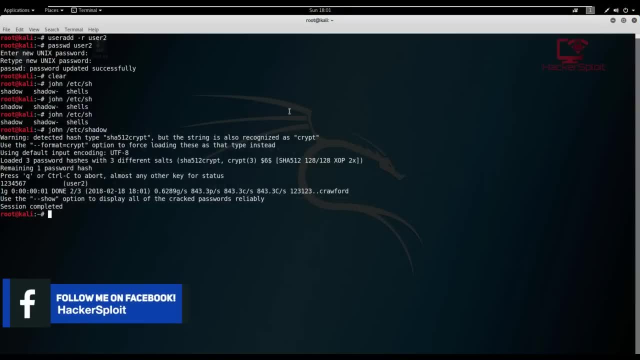 cracking the password hash And it's going to give us the results, As you can see: 1234567.. So that was really, really quick. Now let me explain the results that we've got Here, because it may feel a bit, a bit confusing. So, as you can see, detected that the hash type was 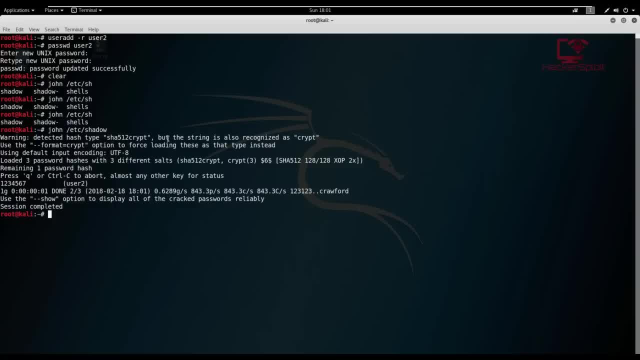 a sharp 512 or 512.. So that is an encryption protocol or an increase encryption algorithm. Sorry about that. very, very powerful And again it was able to crack it really quickly. Now, by default is telling me something here that it loaded three password hashes with three. 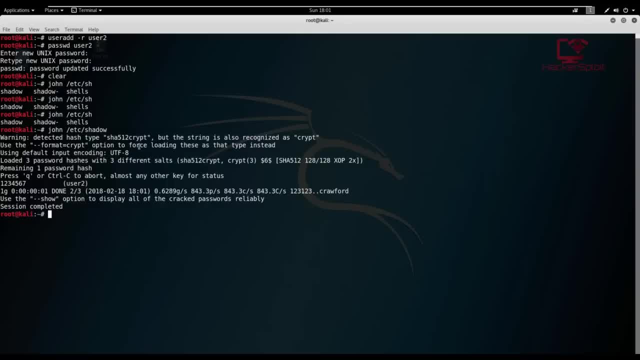 different salts. So what this means is: yes, I have performed this cracking before and it found the password hashes and they were correct. So what it's saying is: I had three accounts that were cracked before and it will. they've already cracked the hashes, So it's not going. 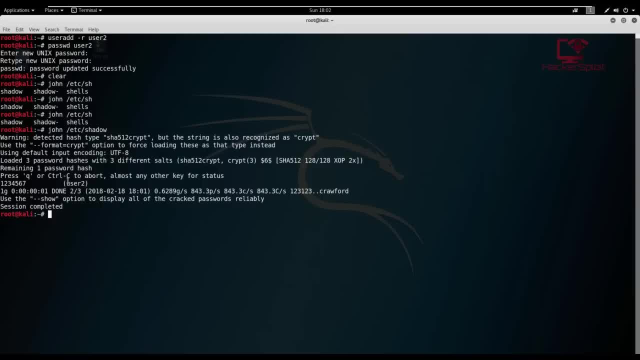 to crack those, the password hashes for those accounts. it only cracks the ones that do not build, that have not been cracked. it in this case, which was user two, And it got the password there, which was awesome. So that is essentially how to crack Linux passwords. really very simple. 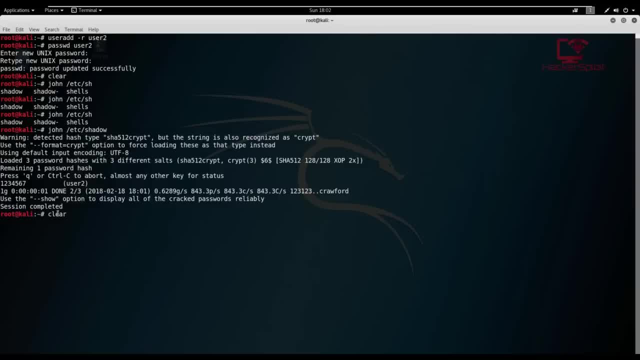 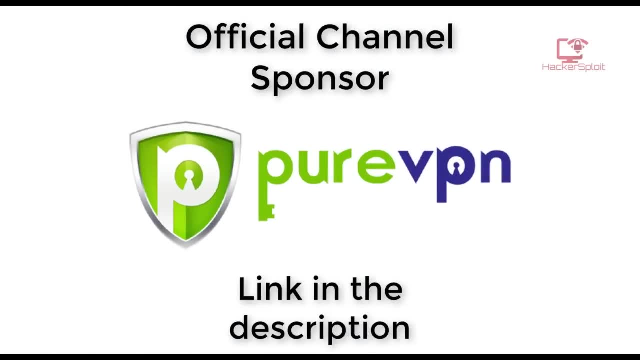 As I said, people just, you know, really over over they, just they just make things a bit too complex for themselves. And the process: if you understand the process, the then performing, the techniques you know to exploit a system or to, in this case, 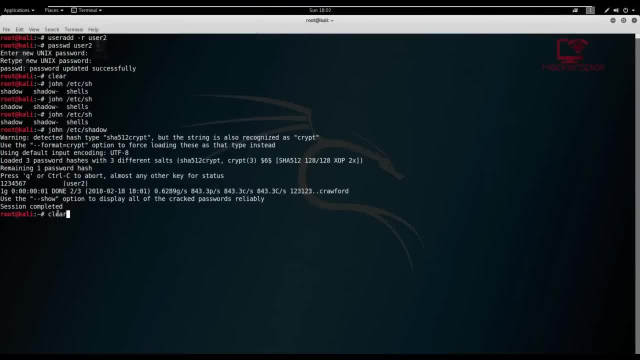 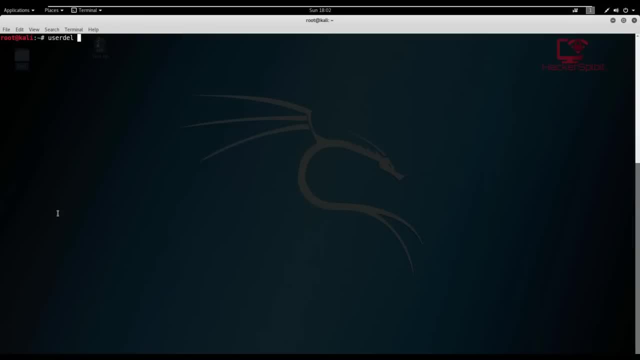 cracker. passwords are really very simple. It's just about time, patience and prudence, Alright, so I'm just going to clear this up, And what we're going to do now is I'm just going to delete the user that I created. user delete. Well, oh, I'll do that later. Anyway, thank you so much for watching. 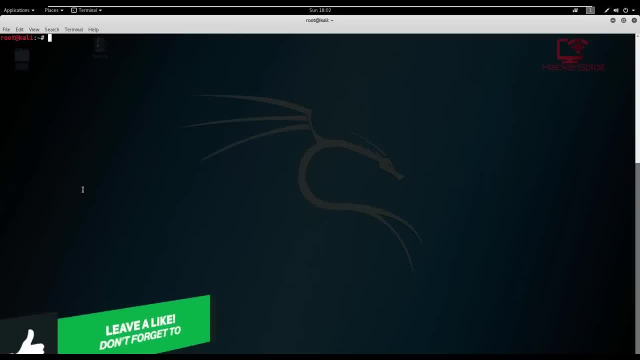 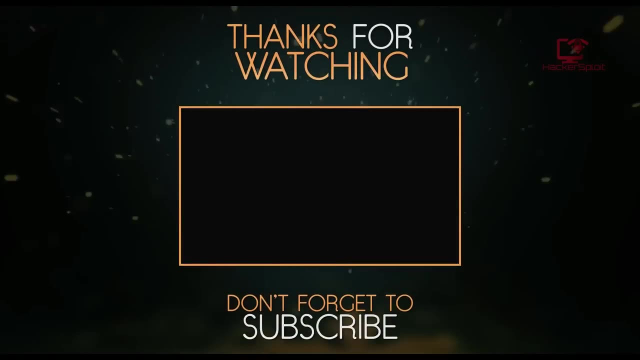 this video. guys, I hope you found value in this video. please leave a like down below. If you have any questions at all- any at all- just leave them in the comment section or on my social networks, Or you can hit me up on kick. Thanks so much for watching, guys, and have a fantastic day, Peace. 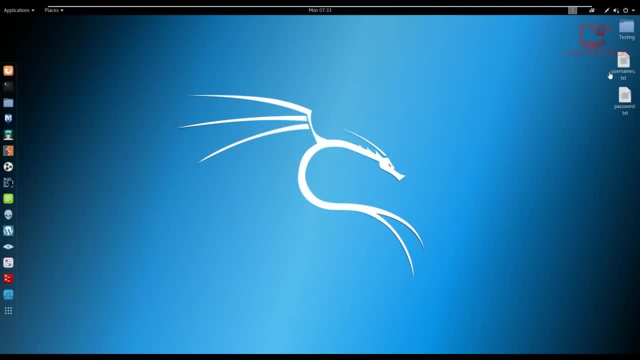 Hey guys, Hackersploit here back again with another video and I apologize, guys, for the lack of uploads. I was just completing the web penetration testing series and I had some work that I needed to get done, So I'll be uploading those promptly, But now I 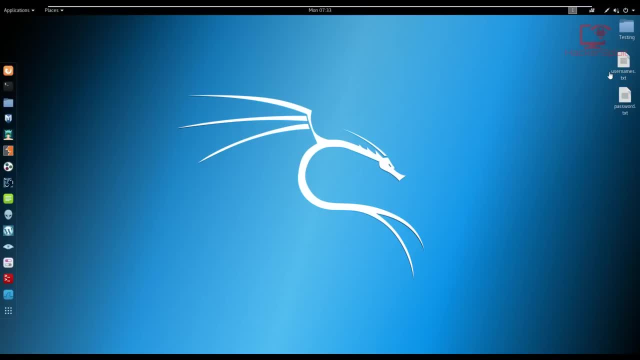 really wanted to show you guys probably one of the most important tools that you should be familiar with And you should be able to use, and that is Hydra. Alright, so for those of you who have never heard of Hydra, Hydra is essentially a very, very good password brute forcing or a password cracker. 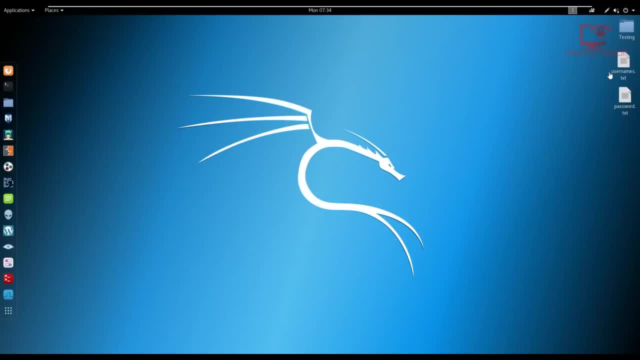 for that matter. So it allows you to crack, you know, online logins, etc, etc. Now, in this case, what we're going to be focusing on is how to attack SSH, or how to actually brute force using a dictionary attack. we are going to brute force. 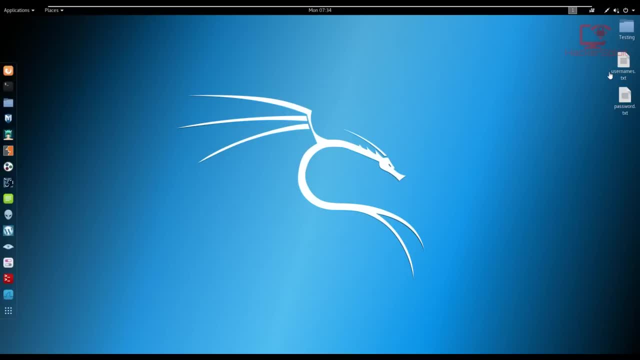 the SSH port. Alright. now you might be asking yourself: well why is this such a viable thing? Well, the truth is, if you're looking at this from a black hat perspective, let's say, you have access, you know you have access to a network and organizations network, And now you want to gain. 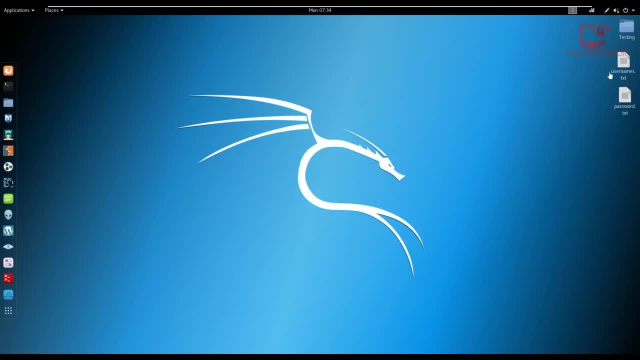 access to a computer. well, SSH might be a very, very good attack vector. that could obviously give you- you know- a large amount of access, or could give you access to a, a senior or- you know- systems administrator or something like that, for example, a router, etc. etc. And obviously 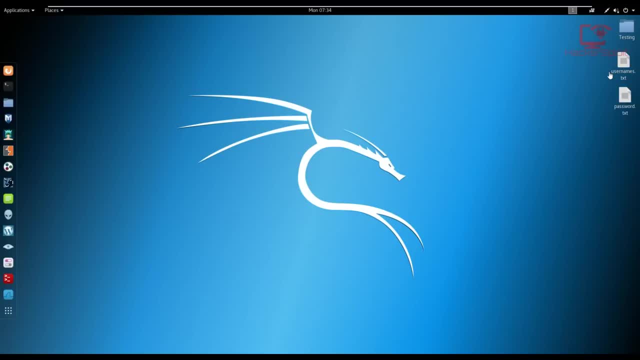 from then. you're now escalating your privileges even further. So again, you can target really really important things. you know, in an organization, for example, you can target the systems administrator. you can target, you know, probably one of the, the one of the most important. 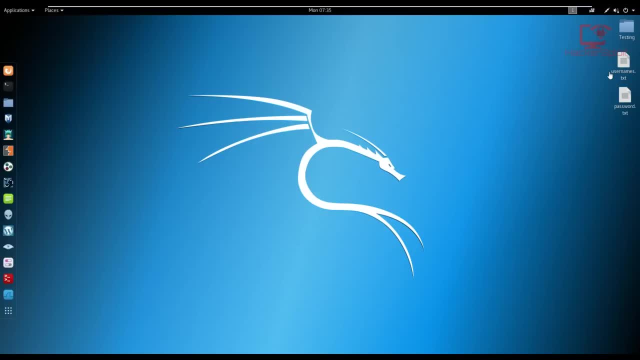 post computers. you know, for example, the, the CTOs, a computer, etc. etc. Right now, in this case again, I'm going to be stepping out of using Metasploitable Now, in this case, I'm just going. 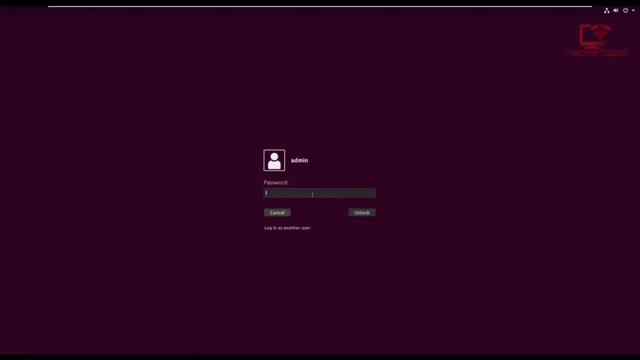 to be using a standard Ubuntu. I'm just going to be using an Ubuntu operating system here that is again connected to my local network, And this will offer us a fantastic understanding of of how to use Hydra to perform an attack. Now, when I said we're going to be using Hydra, 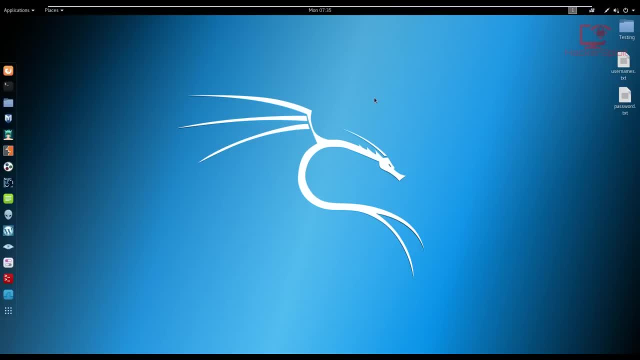 we're obviously going to get started with using x Hydra. Now, if you've not heard about x Hydra, don't worry. it's essentially the graphical user interface for for Hydra, And you might be asking yourself: why exactly are we using x Hydra and not Hydra? Well, I'll show you exactly why. All 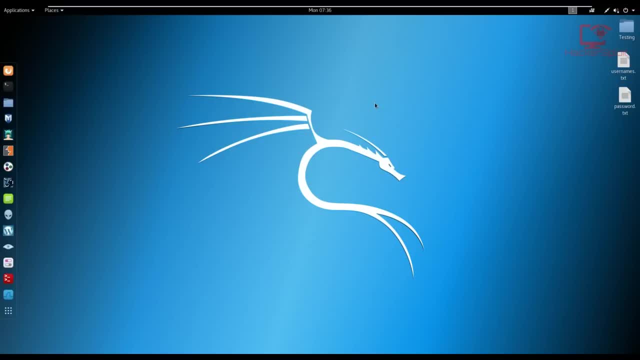 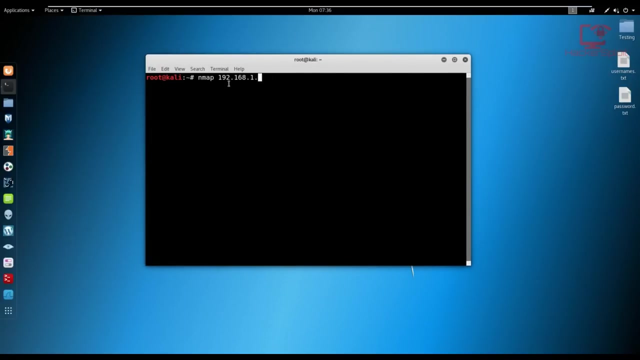 right. So the first thing we need to do, you know, following the, the standard steps, is we need to identify the, the targets, we need to identify what ports are open in the target. So for that we'll just perform a basic Nmap scan. you know, we'll just scan for the, for the simple ports. the IP address for my target is: 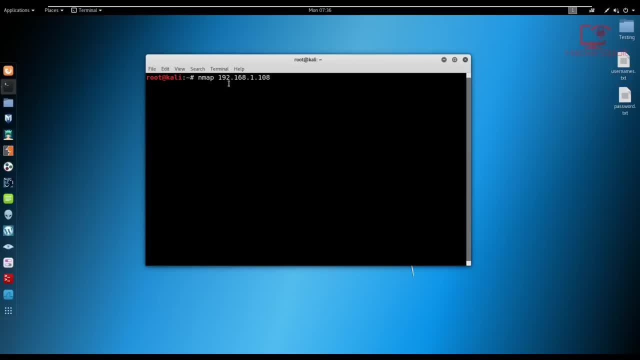 192.168.1.108.. Now, if you don't know your targets IP address, you can just perform a an Nmap scan as well on the entire subnet And you'll get the IP address that way, Or you can use net discover. 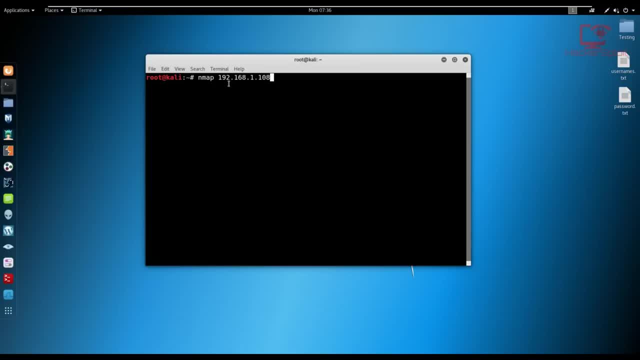 depending on what you, what you like. Alright, so I'm just going to hit enter And, as you can see, the only port open is the SSH port And, by default, I created a new user with, with its own password, the admin user with its. 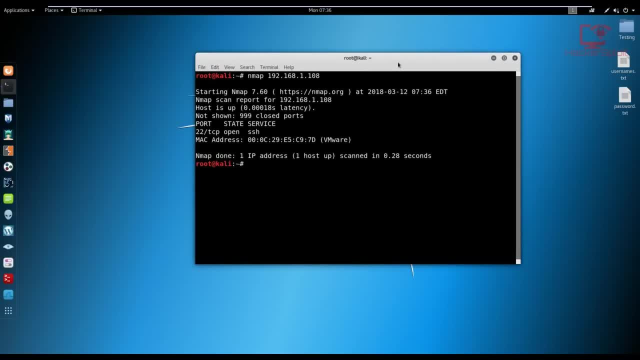 own password. Now by default, of course, you'll not be knowing the username and the password. So we are going to be using word lists are to perform a dictionary attack. If you perform a brute force attack it becomes too long because you know some word lists have about. you know like. 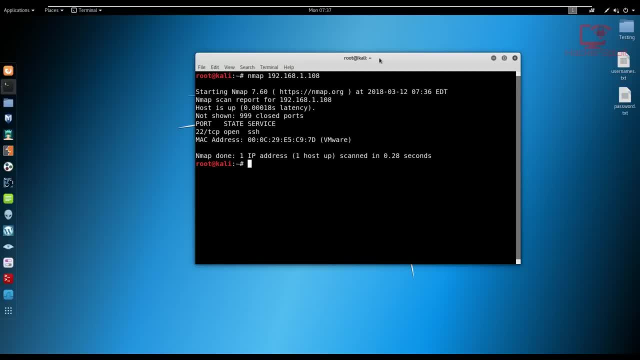 for example, if you use the rocky word list, it could have in the in the minimum of 12 million combinations And that that's going to take like a week. Now you can see why this is getting really, really tedious is because if it's going to take a week and you're on the network, meaning you're. 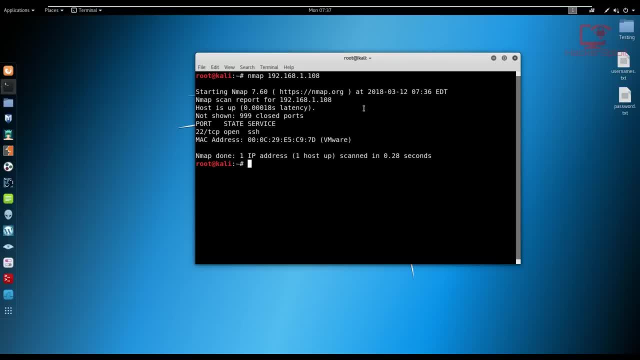 actually inside the organization, probably have not connected through it externally. But you know you, you're on the network, you need to. you need to get something really really fast. Now, again, we're going to be targeting default usernames and passwords, But again it can be different. 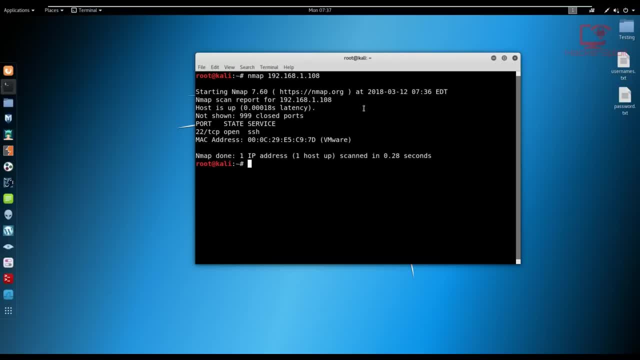 depending on the security protocols set up by the network. So we're going to be targeting default usernames and passwords, But again it can be different depending on the security protocols set up the company or the organization. So you can use the default word list that's come with Kali Linux. 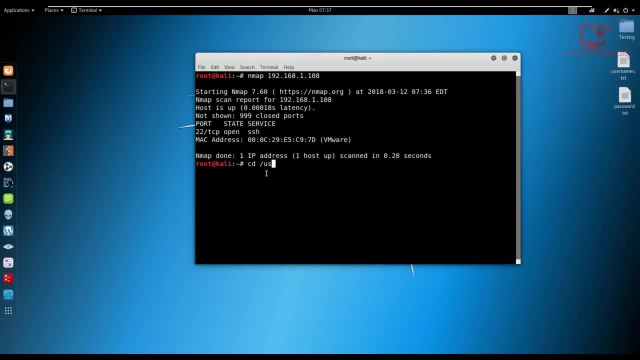 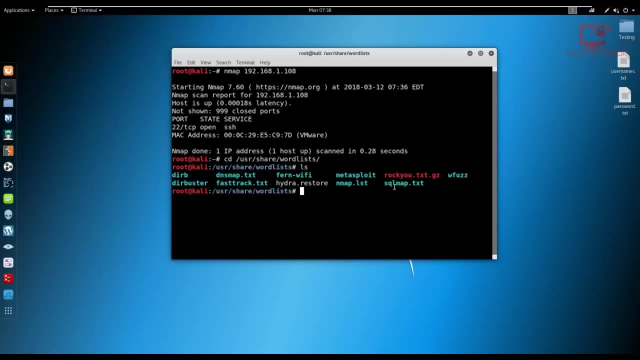 which are extremely powerful. that can be found in CD- sorry, not CD- command share, change directory, user share And I believe they're in word lists. There we are. So if you list the word list in here you can see you have the rock, you you have the phone Wi Fi. 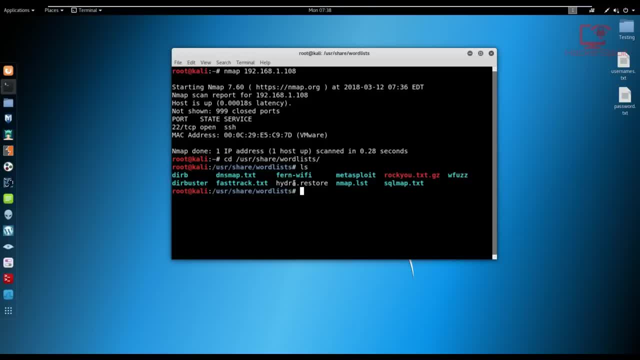 which is again set up by the phone: Wi Fi cracker, the fast crack, the fast track, sorry, dot txt. And these are some that you can just experiment with, And they are fantastic as well, Alright, but in our case, what I've done is I've just created my own word lists. 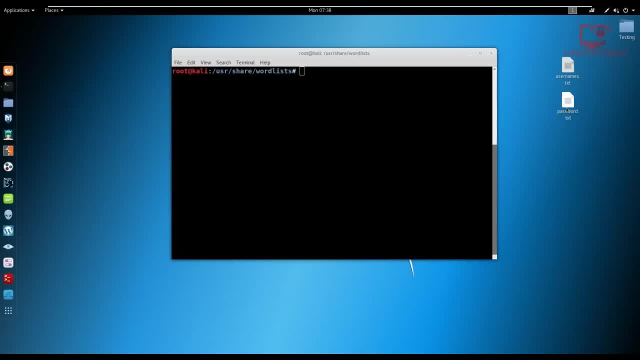 here. they're sorted out in usernames and passwords, Because if you, if you know the username, then you're halfway there. all you need to do is brute force the password. But in this case I'm just going to have created a usernames and passwords Again. it's a simple one. 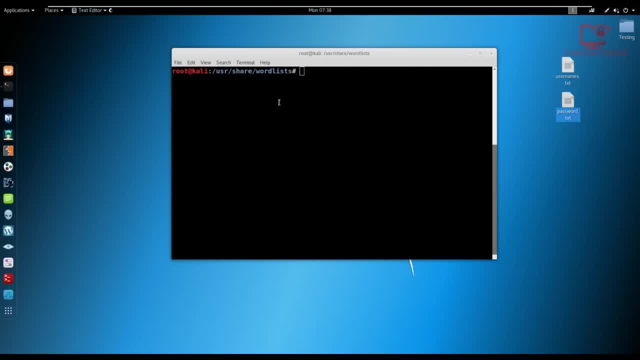 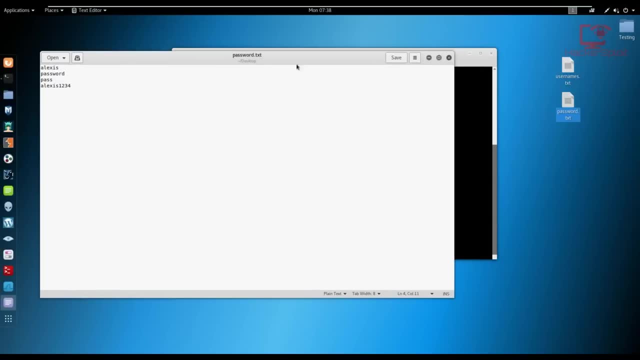 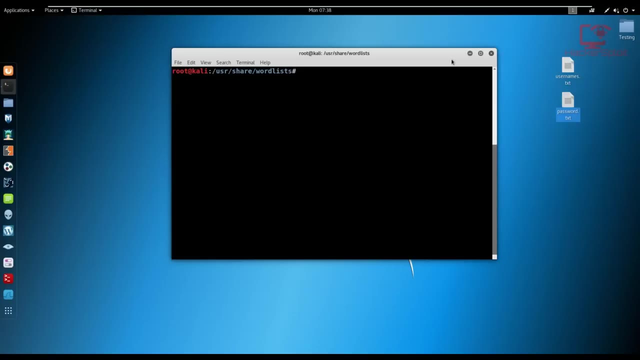 with you know, with you know, possible ones and the passwords, As you can see, for the SSH is Alexis 1234.. I've just kept it as basic as that you know, so that I can save time and I don't have to, you know, go through the cracking process, which can take up to a week. 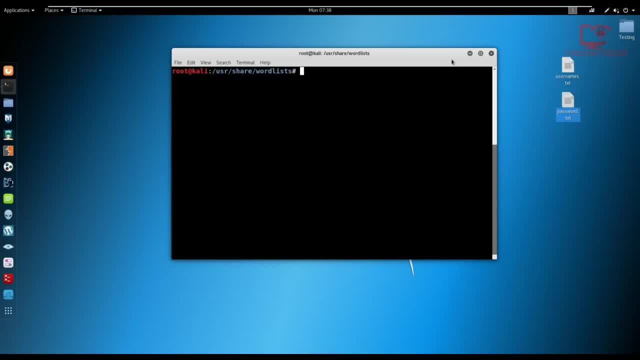 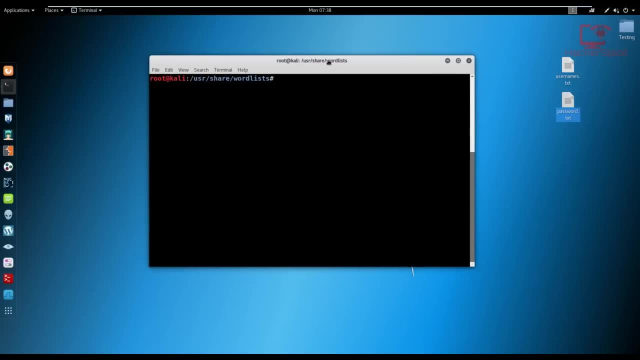 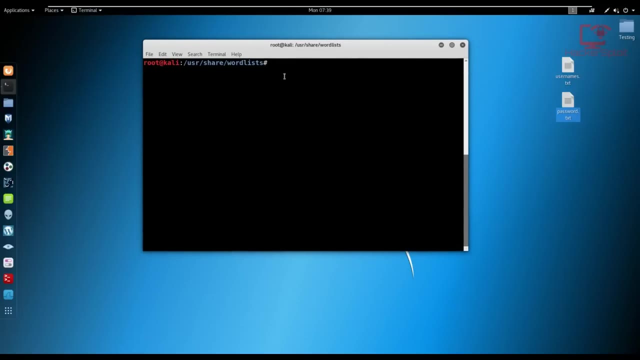 and then, or you know, a few hours, depending on the complexity and where it lies, on the word list or in the word list. Okay, so again, I'm just going to be explaining how everything works here and how it's done. Excellent, let's get started now. So we know that the the port 22,, which is the 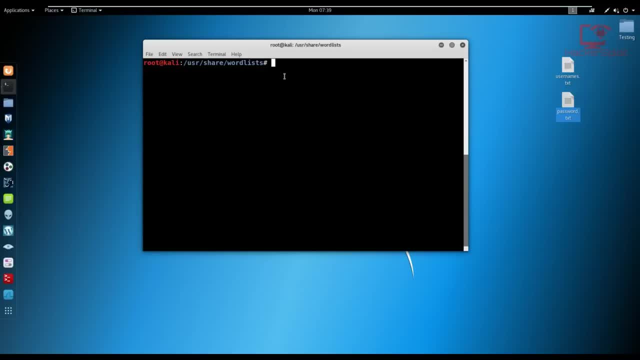 is currently open. you remember, it's very important that it is open. if it's not open, then you know. many people have tried to tell me that they are trying to attack a target, But when you look closely you can see that the that specific port is closed. So that means it won't. 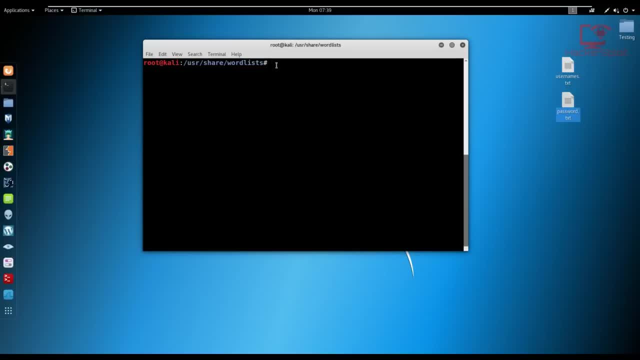 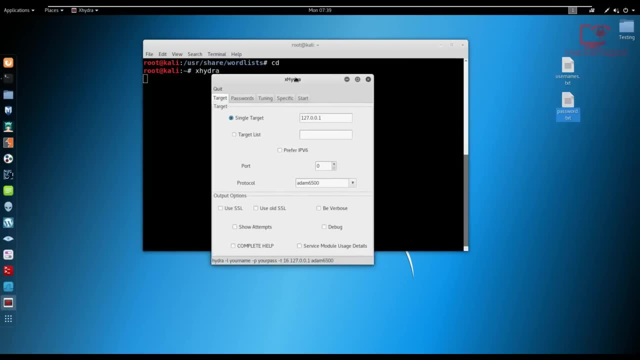 really work. So again, make sure that the port is open. So, once you're ready, what you want to do is we just want to just type in x Hydra, x Hydra, like so, And once you type in x Hydra, it's going. 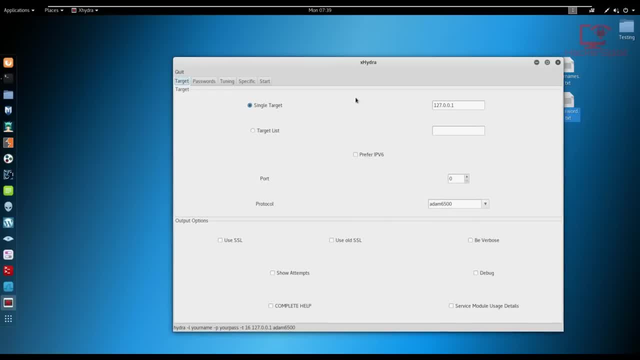 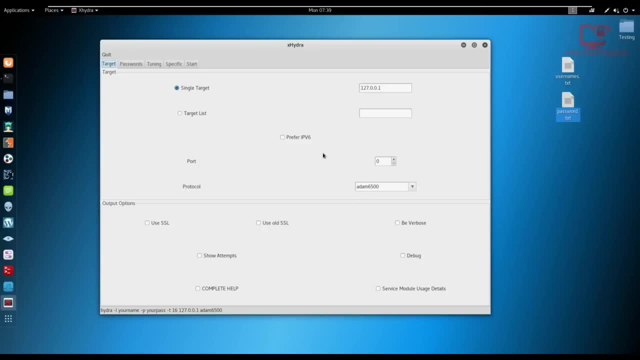 to open up the graphical user interface And let me expand that. Alright. so now we want to select a target. Alright, so it's sorted out in target passwords, tuning specific and start. we'll get to all of that. So our target is essentially a our target. if you're targeting a single target. 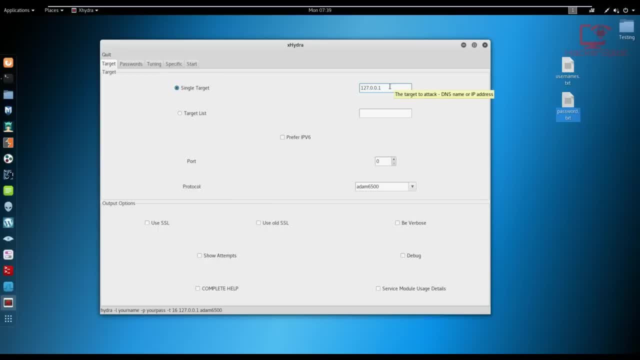 you can enter the IP address here, whether it's a global or I mean a public or local IP address, or you can select your target from a target list. Alright, so we're just going to select a single target and we're going to select the, the IP address, point 1.108.. And again, if you're using 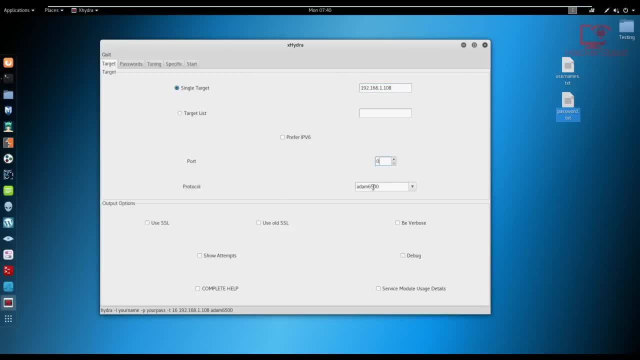 IP v six. you can also specify that. As for the port, we know that the port is open, So we're the default port for SSH is port 22.. It could be incorrectly in, it could be incorrectly configured, So you can also watch out for that. you then have your protocol. In this case, we want to scroll all. 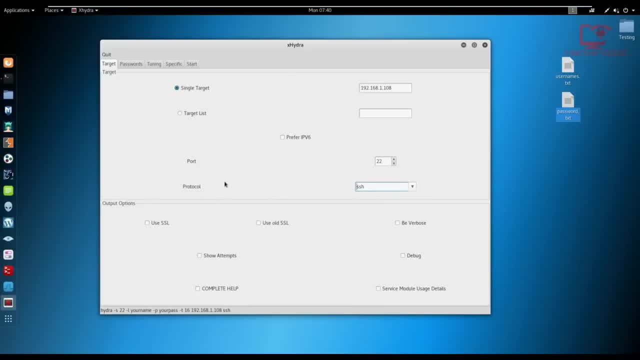 the way down to the SSH. So again, you can look at how to use Hydra for the type of other types of cracking, But for now just allow less focus on the SSH, because one of the most popular ways of being cracked. Now for the output options. this is very, very simple. you have your be verbose. 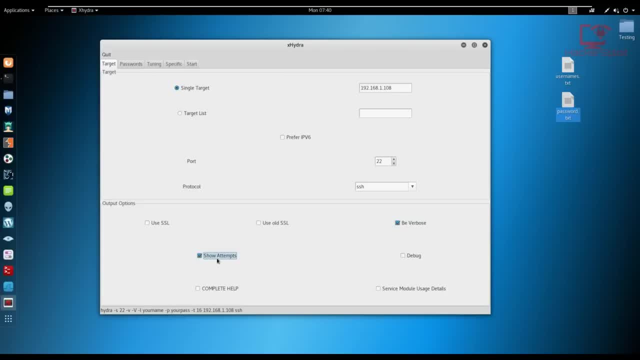 so it's going to give us additional information and show the attempts very, very important. Now, why am I using x Hydra and not Hydra? The reason is: if you want to learn, if you want to learn how to use Hydra or any other. 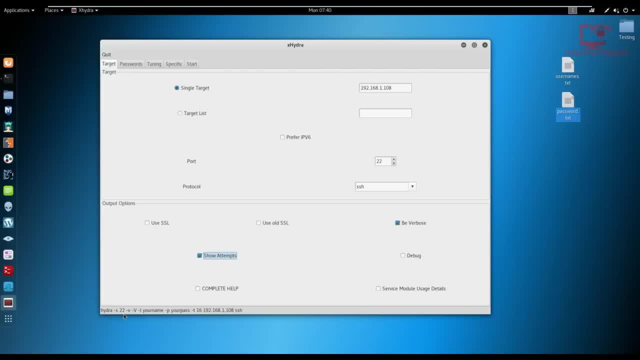 tool I would recommend of especially Hydra In this case. you can see that it gives you the syntax that is being used right under here, And from then on you can then try it on your own with the command line. Alright, so again, it's going to just list down to you here how you would go about. 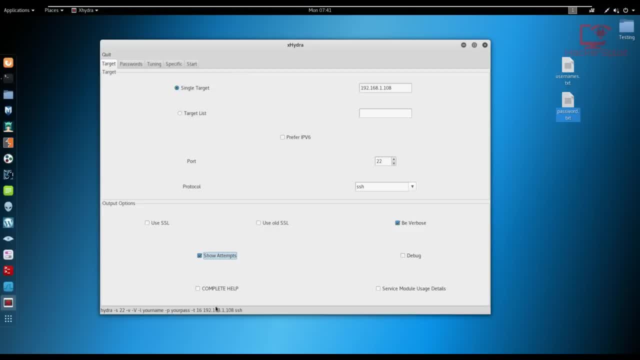 typing this out. How would you? you would go about using Hydra in the command line. Alright, so those are the options we're selecting there. Now let's go to password. So, again, you can select a default username, if you know the username, or you can select the username list, which is what I'm going to do. 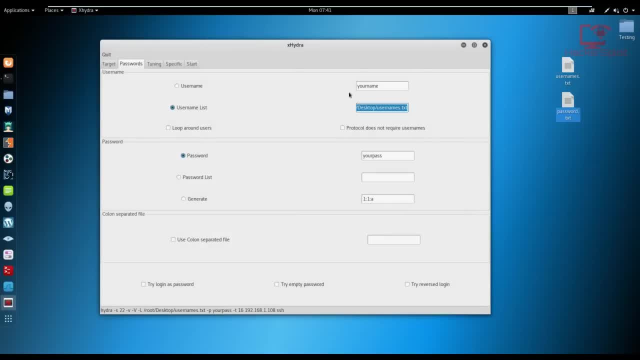 which is stored on my desktop and usernames dot txt, And we open that now again. I've said this word list already contains the username, So it's not going to be a long cracking process. I'm just explaining the theory here behind what's going on. Again, I don't want to go through the entire. 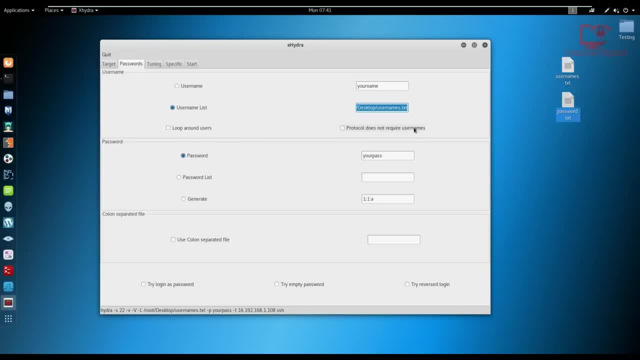 cracking process, because that would be pointless and you're wasting computation power. Alright. so as for your password, again, you can select the password if you know it. Well, if you know the password, then it really doesn't make sense, unless you want to know the username, which is again, very, a very viable option. So 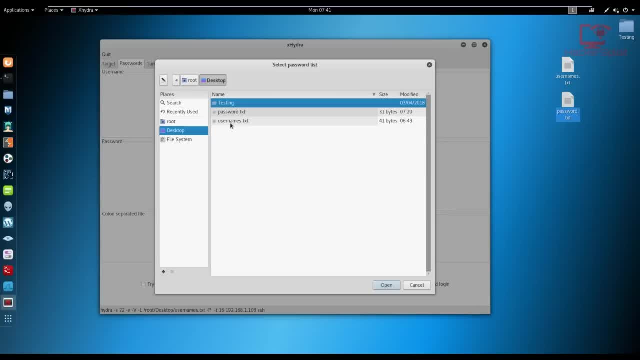 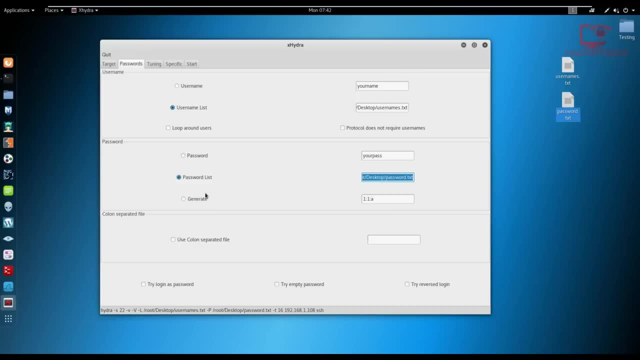 let's select your password list or your password, And you want to go to. I'm going to go to my desktop and I'm going to select password dot txt, And you can also generate your own password. That's an advanced feature. we'll not be looking at that right now. As for the option the other, 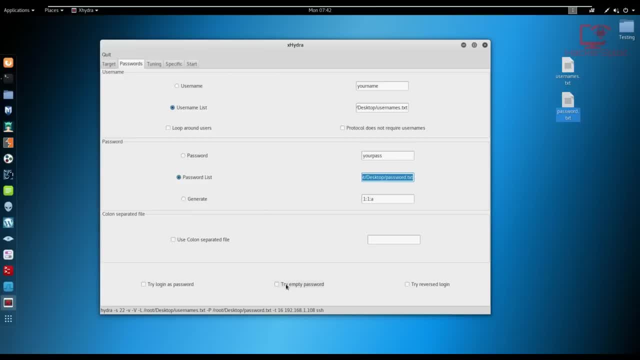 options, you can try logging in as a password. As for the other options, you can try logging in as a password. This essentially means you can try the default. So if it was incorrectly configured and the systems administrator or the network administrator was a really 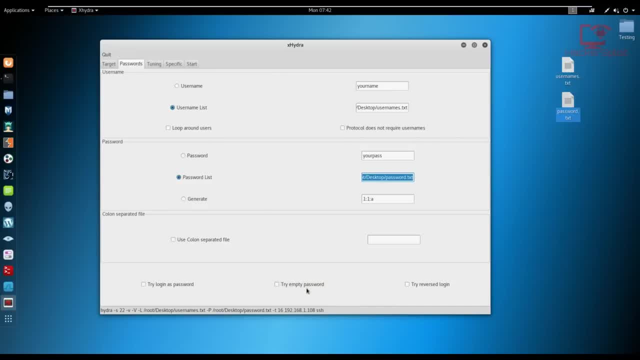 well, he wasn't really keen on security. you can try an empty password, which works most times, believe me. I've tried this And it's actually just shocking, especially for smaller companies that don't really have the budget to do, you know, to do- to hire serious security guys and 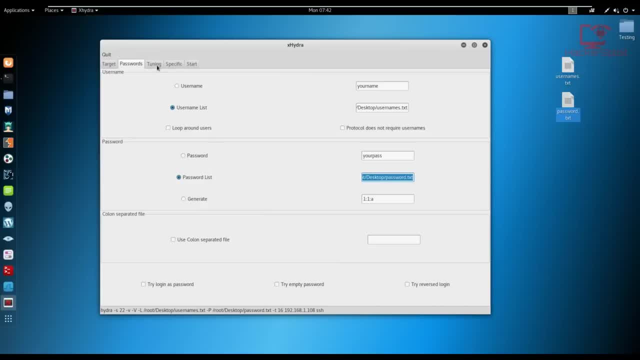 stuff like that. But irregardless of that, what we want to move on now to is the tuning, Now tuning. why is this so important? Well, we talked about number of tasks. what this means is these are going to be the number of login attempts being made. Now, as again I said, if the security 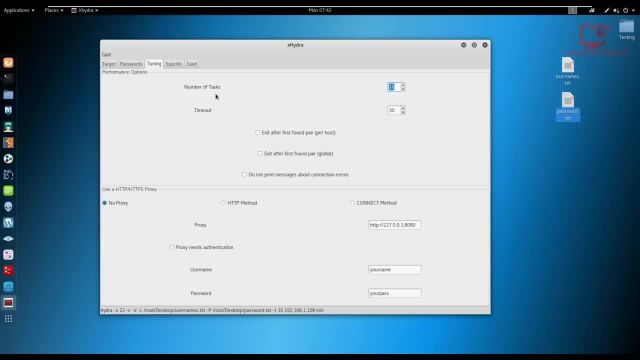 protocols in place are very, very high and you're trying- you know you're trying- to attack a company that has the security at the top, at the top notch level. you want to reduce this to about five because, again, what will happen is if you, you know, most companies usually have the 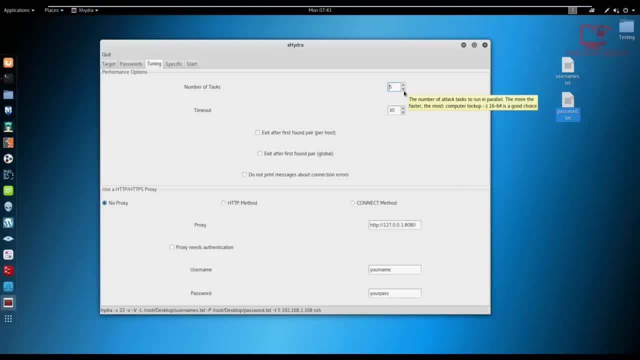 protocols of: if you enter five passwords incorrectly, it logs you out and it'll you know, it locks SSH for about five minutes. So again, I would recommend that you keep it at about five And for your timeout we can just change that to something really, really nominal, which is 10. 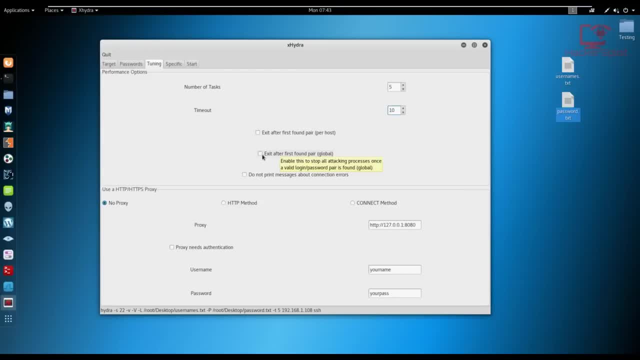 seconds to timeout. So again, you want to make sure you select exit after first of after first font pair global. So again, you don't want to make sure that your key you keep on looping around moving back to the passwords. So sorry, what am I saying? not the passwords? going back here: exit. 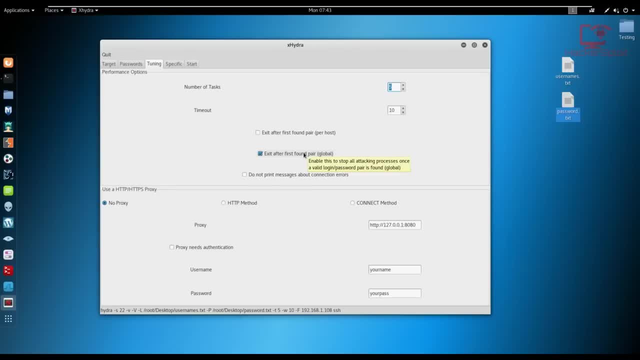 after the first phone pair. So this will essentially mean that it, once it gets the password and the username and the password pair, it stops the, the brute force method. Now, again, you can also use- you can use the HTTP and HTTPS proxies here, which is again something advanced. 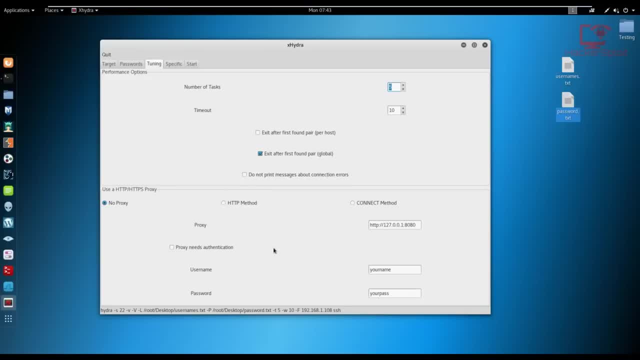 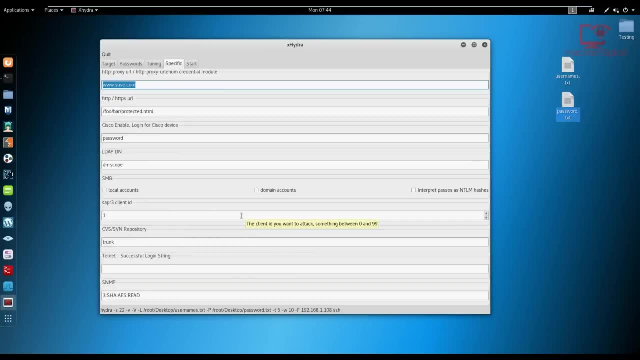 but right now we're not using any proxies, But again, it might be useful if you're using a proxy. going on to the specific settings, we don't have to change anything here. this usually come in handy when you're targeting, you know, telnet or FTP etc. 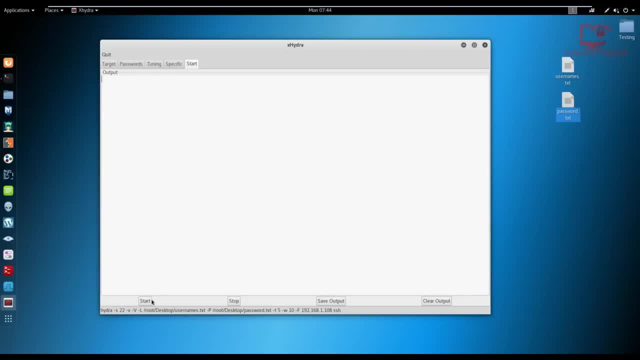 And now, once you're ready, just hit start. And you want to go into this bottom button here and you just want to hit start, All right, and it's going to start and immediately, as you can see, it got the, the login as admin and the password as Alexis 1234.. Now, again, this took a. 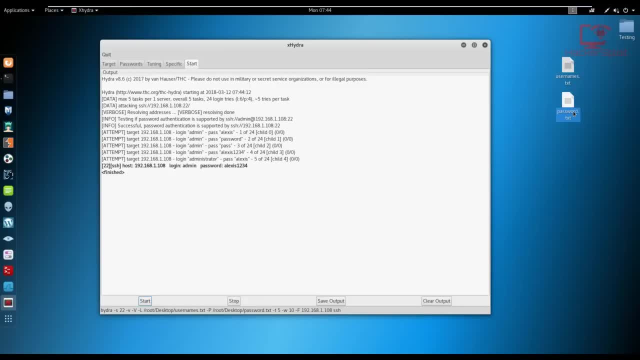 really really short time, probably because the word list is so small. Now, if you talk about a huge word list like the rocky word list, that contains 14 million different combinations, So you can imagine how long that will take. So, again, a good, good sense of information gathering really works here, If you can get the usernames. 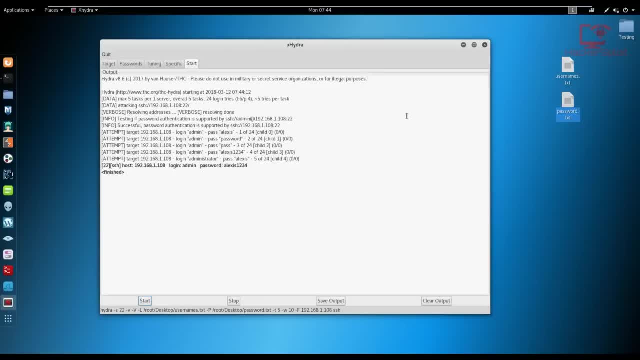 of the computer or off your target. that will be excellent as well. And you can also try the default usernames Because, as I said, most of the smaller companies do not do not actually care about security, if I can say that. Alright, so we've got the username and the password Now. 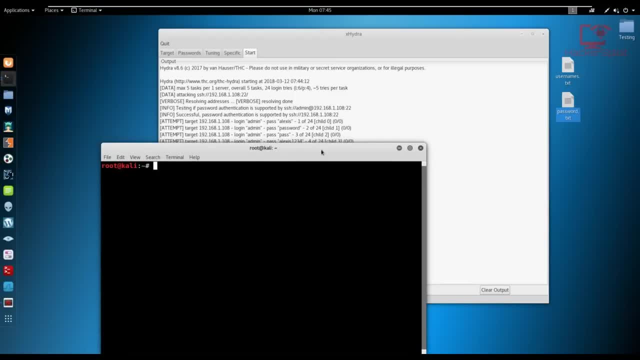 let's try and log in via SSH. So I'm just going to open up a terminal here And I'm going to say SSH, I'm going to select the username, which is admin at 168.1.108.. And once I hit enter, it's gonna ask me for the password, which in this case is Alexis. 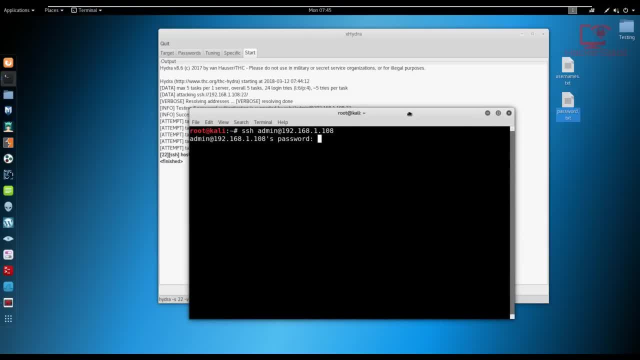 12341234.. Sorry, oops. And once I hit enter, it should log me in. Oh oops, Something's happening here. I'm not out there. We are alright. so you are successfully logged in And that is how to. 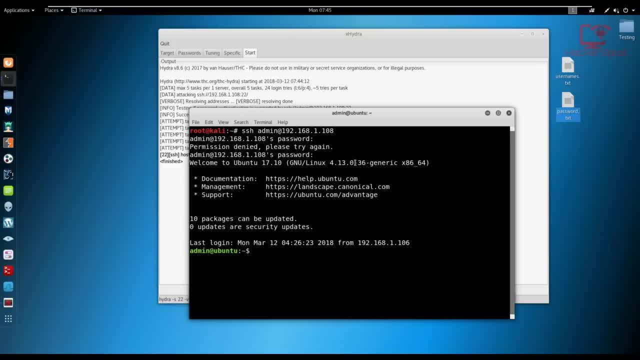 target SSH and how to use Hydra for password cracking. As you can see, it's really an efficient tool when it comes down to what you're going to be using, So we're going to go ahead and hit enter. It does best, which is password cracking. you know more specifically, really extremely. 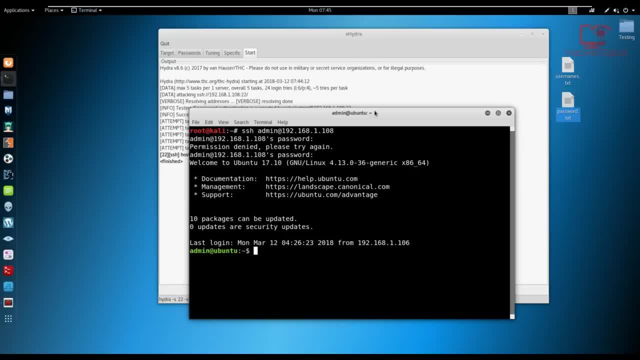 difficult protocols. you know things like FTP, which can be extremely useful if you see the use case. But directly from here you can see that we have got access And you know you can imagine the damage you can do if you get access to a target's computer or you get access to the. 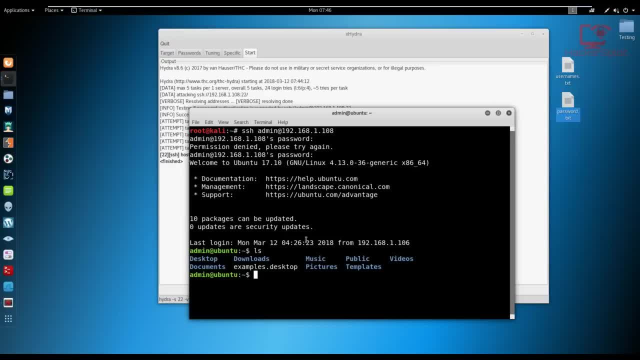 systems administrator computer you can reek, you can really really damage stuff on the network. But again, I'm not encouraging that. this was just a video of me showing you how to use Hydra, you know, to understand the cracking process. And finally, 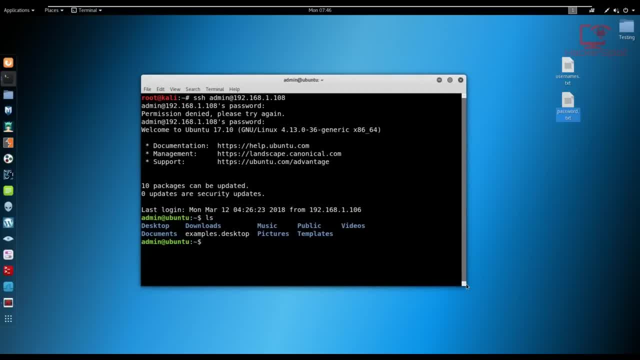 using Hydra is is always something that comes in handy, especially when you'll be performing penetration tests, if you're looking at being a penetration tester, Alright, so that's going to be it for this video. Don't worry, in the next video we'll be moving on back to web. 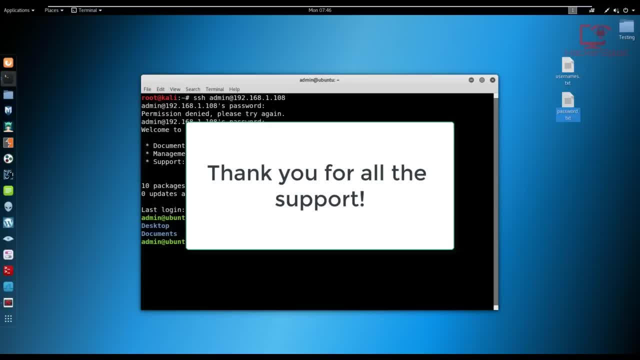 application penetration testing. I've made all of the videos now, So I'll just be uploading them daily. And yeah, thank you so much for the support guys. We're almost at 50,000 subscribers As of uploading this video. I really appreciate the support and have awesome things planned for you. 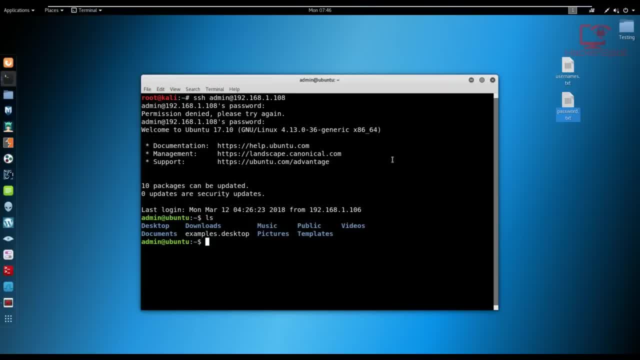 And I'm also planning a giveaway, So stay tuned for that. I love you all. Thank you for the support. It's been unbelievable And you know I couldn't ask for more. Thank you. This is all. this is all thanks to you, So that's going to be it for this video. Again, if you liked the video, found value. 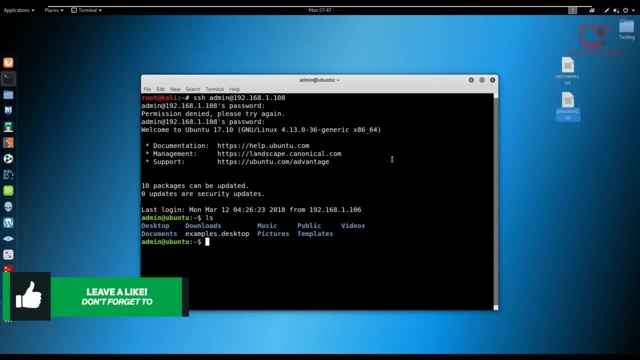 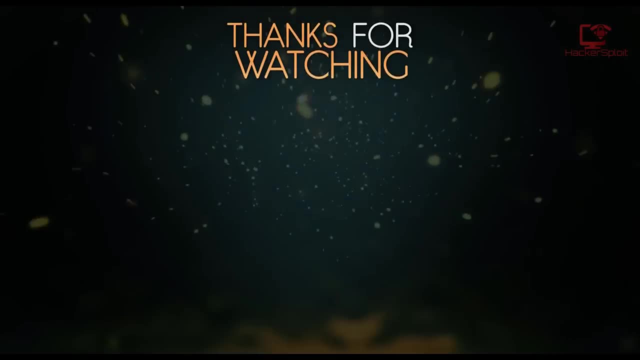 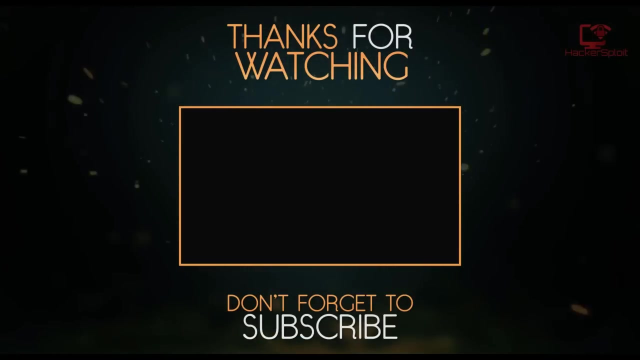 in it. please leave a like down below. If you have any suggestions, questions or comments, leave them in the comment section, on my social networks or on the website. Alright, so that's gonna be it for this video And I'll be seeing you in the next video. Peace. 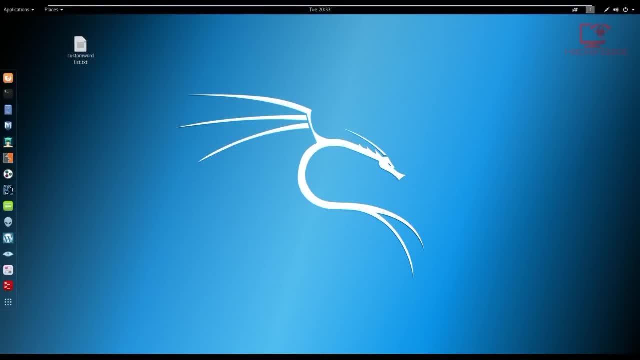 Hello everyone and welcome to this video. In this video, we're going to be looking at password cracking with Medusa. Now you might be asking yourself: what exactly is Medusa? Well, Medusa really simply is a very, very similar tool to Hydra. It is lightweight and powerful. Now that's. 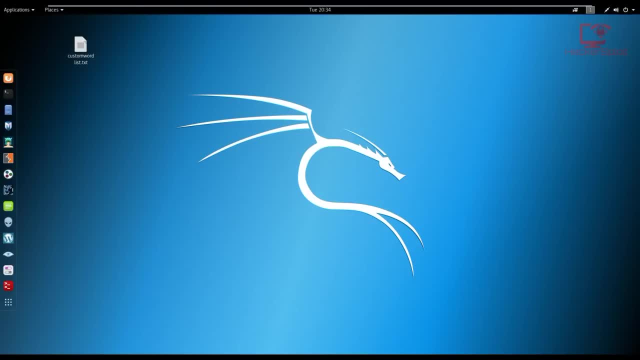 one of the things I like about Medusa is it's it's much more of a cleaner. you know, login cracker or password cracker, Alright. so the thing I like about it is it's multi threaded, which allows you to, you know, scan multiple hosts at one time. Now, the great thing about this is it. 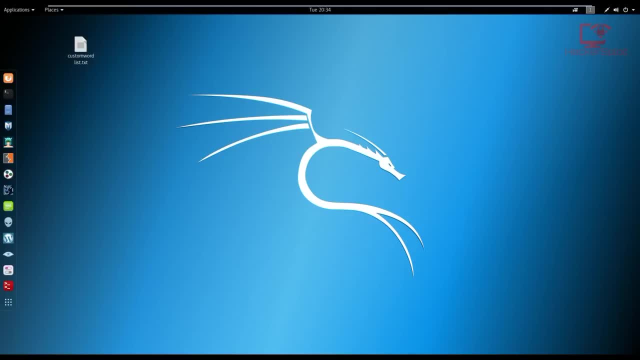 works on many, many services. Now, the great thing about this is it works on many, many services, for example, FTP, HTTP, MySQL, telnet. you have your SMB NT. you know multiple services that are awesome. If you, if you know, you're trying to crack them. Now in this video we're going to be trying. 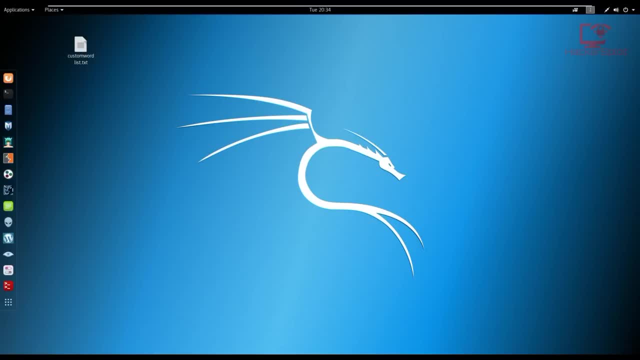 to crack the SSH port. Now, in the previous video, when we were using Hydra, I showed you how it's done the correct way. Now, in order to show you that you know tools like Hydra and Medusa work, in this video I'm going to actually create a word list that contains the login credentials. 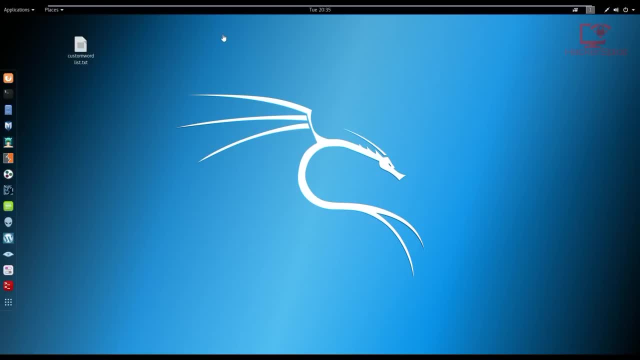 for the SSH port. Now, why am I doing this? The reason I'm doing this is I'm going to show you that, indeed, it can actually crack these passwords. Okay, so Medusa said is a really, really simple tool to use. it may have a lot of commands that you need to specify, But in the long run, I would. 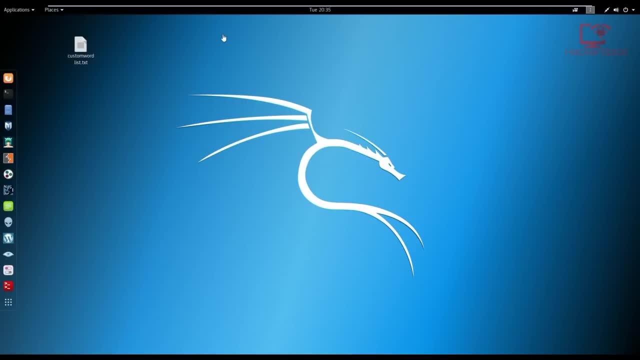 prefer to use Medusa over over Hydra. Now, Hydra is great for cracking. you know, online portals and stuff like that. For example, if you integrate it, you're going to have a lot of commands, that it with burp, suite, etc, etc. But for services like FTP, telnet, MySQL, your SSH, it is a fantastic. 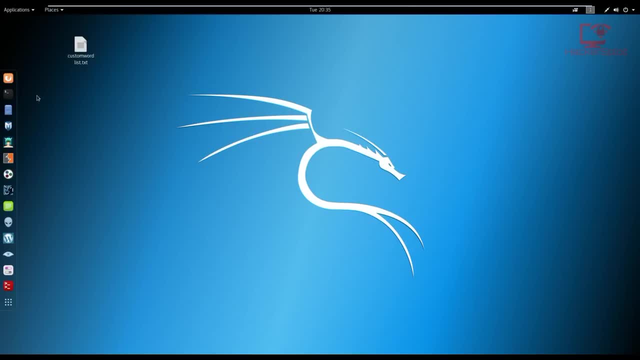 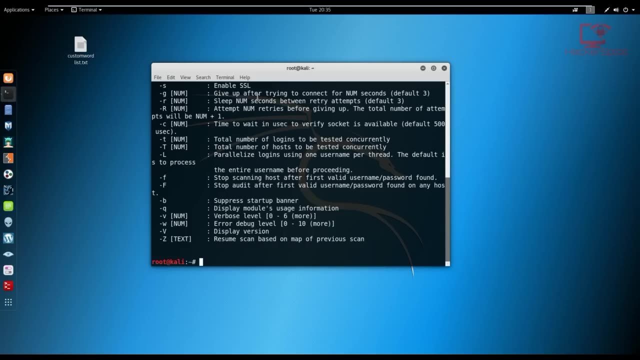 tool as well. Alright, so let's get started with Medusa Now. by default, it is a pre installed on Kali Linux And you can just launch it by typing in Medusa. Alright, so Medusa. and once you type. 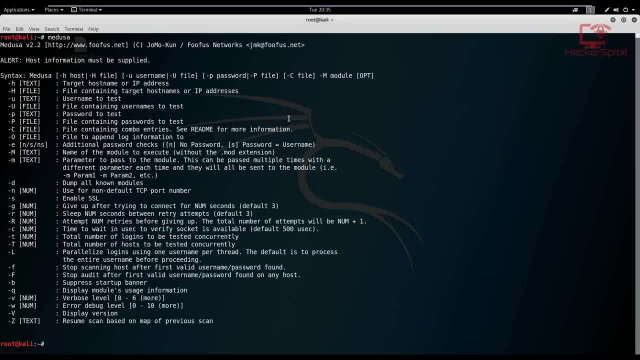 it in. you can see that we have the help menu here that contains all the commands that we're going to be using Now. by default, the commands that we're going to be using is the H. Alright, this allows us to type in the commands that we're going to be using Now. by default, the commands that we're going to be using is the H Alright. this allows us to type in the commands that we're going to be using Now. by default, the commands that we're going to be using. is the H Alright. this allows us to type in the commands that we're going to be using. is the H Alright. this allows us to select our 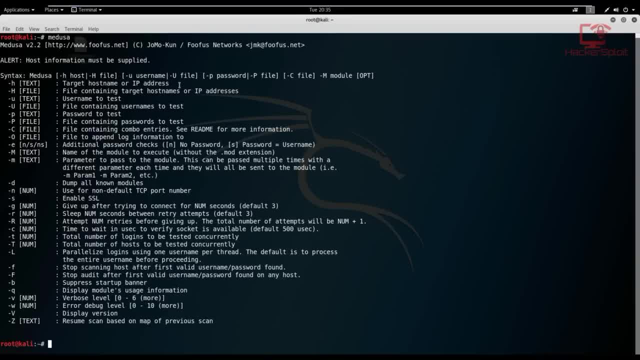 target hostname or IP address. The next command we'll be using is we're going to specify the username, which, as I said, is root or MSF admin. Alright, so once you crack the SSH, the SSH service with Hydra, you will find that the username and the password are both MSF admin. 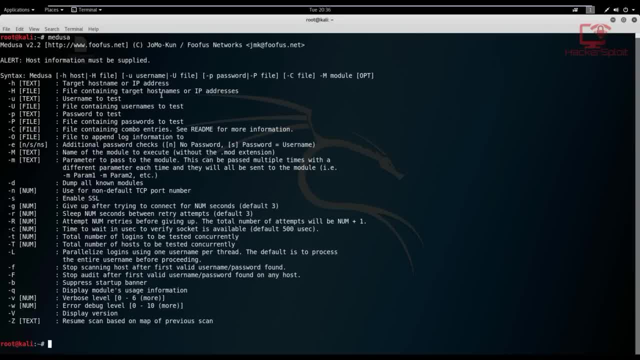 Okay now, sorry, so sorry for telling you that, but it is very, very important for me to show you how Medusa works. Okay, so these are probably the commands you'll be using the most, So we're going to be using the H, which allows us to select our target host name. 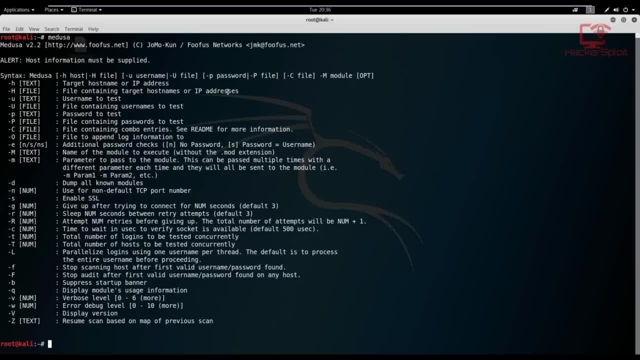 or IP address or you can actually use a file that contains target host name. So if you have just come straight from the information gathering section of the course and you gathered your hosts or you added your hosts in in a in a text document, you can scan multiple hosts, All right. 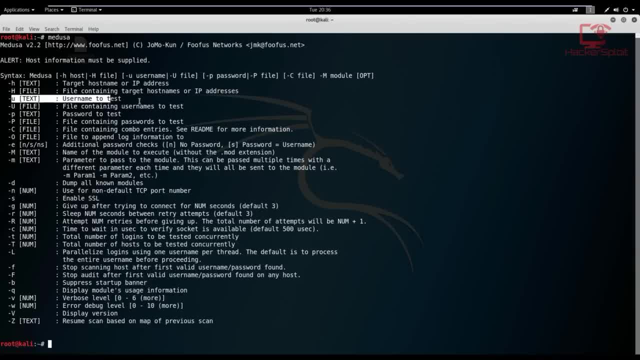 so that that's what I really enjoy here. You then have the username to test against which we'll be using. you have the the file containing usernames- again awesome that we have that option. you have the passwords to test the file containing the passwords. you have your file containing combo. 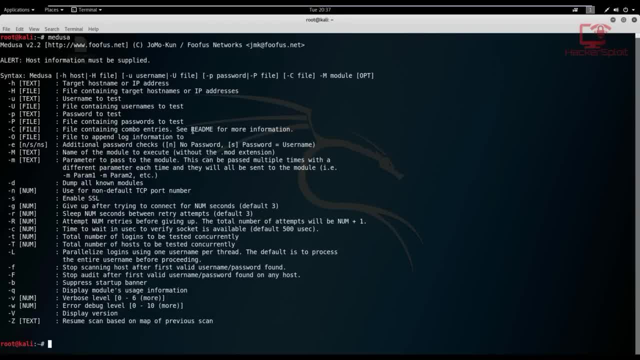 entries, which is also quite powerful to use. The other command that we use, will be using, is the C: the C command, which allows you again combo attacks. you then have your module, which allows you to select the module. Now, the module essentially means the service or the port that you're trying to. 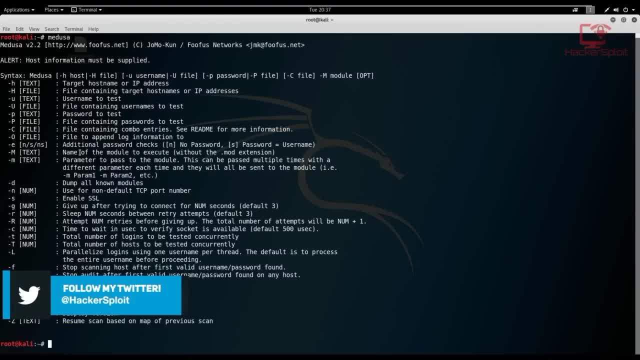 perform the attack on. So that's what that means. All right, so getting now to performing the attack on the, the H port on our metasploitable to virtual machine, Again, we just need to get the local IP address, which is the. 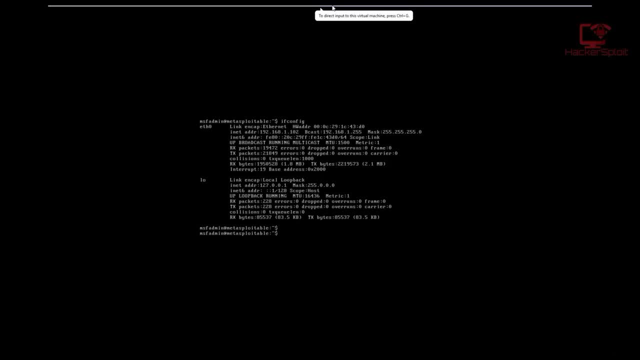 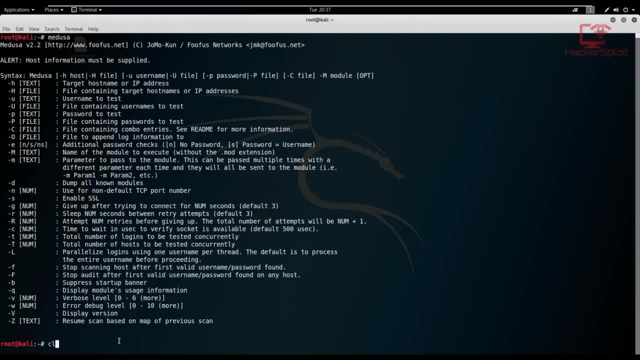 same as the previous video, 192.168.1.102.. All right, so the the the cracking process is slightly different now because you have to specify a few things. So, before we get to the actual cracking process, as I said, instead of using the word list that comes with Kali Linux, I'm going to 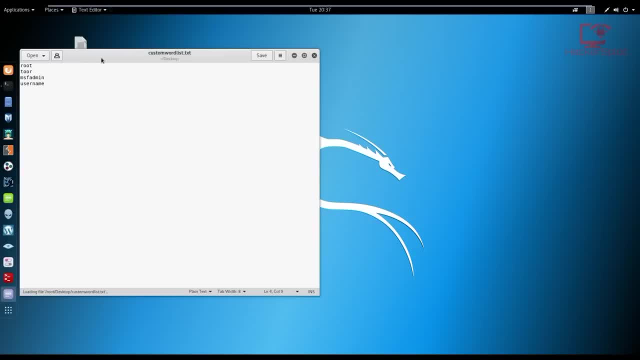 I've created my simple word list here that contains the credentials. All right, so it explicitly contains the credentials. Now, this may not seem like a word list, because it does contain the exact credentials. this will be more of a dictionary attack, But in reality it is going to use the same 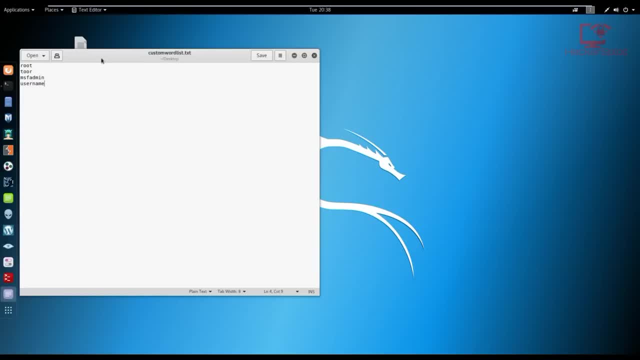 technology behind a, behind using a word list, where it's going to test against every combination. Okay, so by default, the username for the SSH port is MSF admin and the password is also MSF admin. I've just thrown the rest of these just to make it, you know, more authentic. Okay, so that is going. 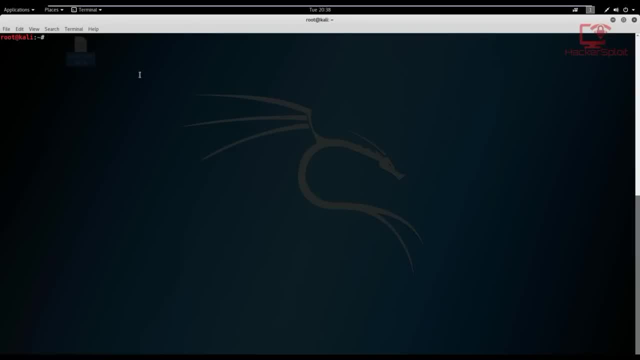 to be stored on my desktop. So let's get started with the attack process. Alright, so to launch it, we use Medusa. Now we select our host, which is H, And that is the local IP address of the metasploitable. 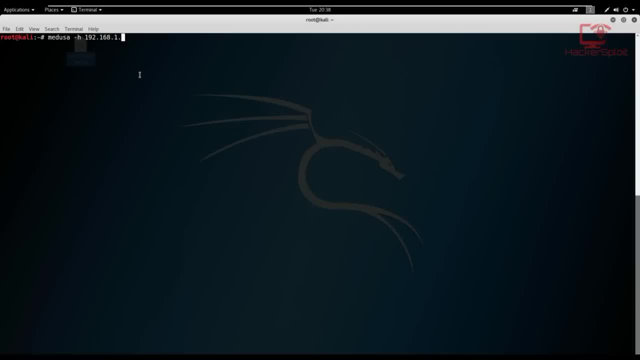 to virtual machine, which is 192.168.1.102.. All right, that is the IP address. as simple as that. Now we need to select the username, which, in this case, the username we're testing for against is MSF. 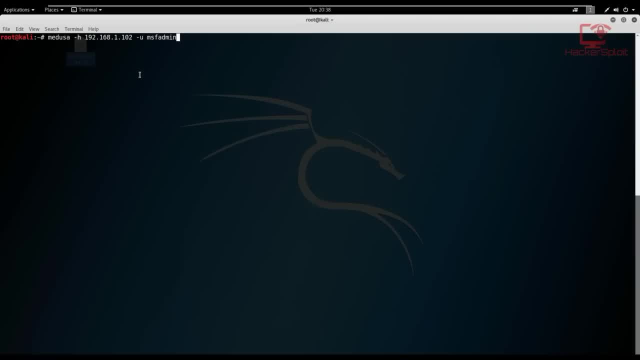 admin, MSF admin, like, so that that is the username that we're going to be using. Now we need to select the password file. All right, and that will be specified by using the capital P command, as we looked at in the Help menu. And now we select the directory, which in this case is on my 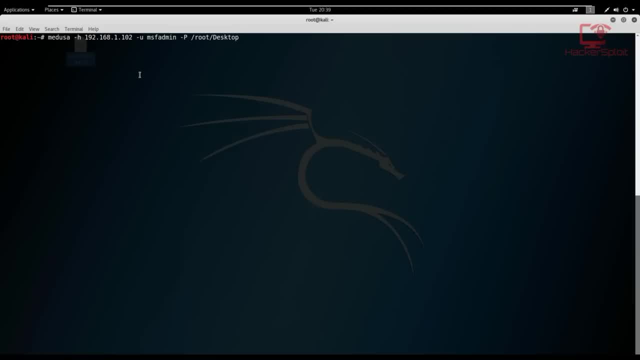 desktop, root desktop. Now, by the way, you can use the the word list that come already with Cal Linux, or you can create your own, if that's what you're looking for Now by default. I already told you, I know the credentials. 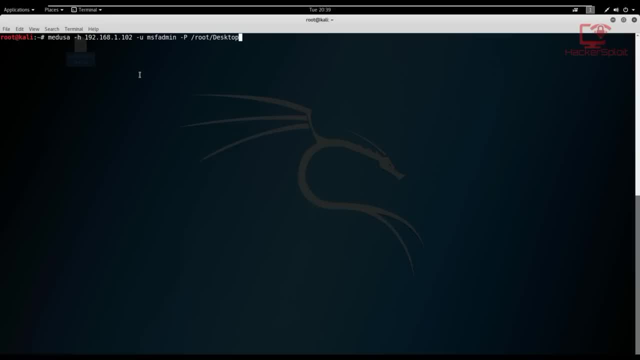 So it's not really a cracking process. But if you are performing this on a real target or on a real server or you're performing penetration testing, I would recommend that you use the word list that come with Cal Linux, for example the rocky word list or the the SQL map. All right, So in this, 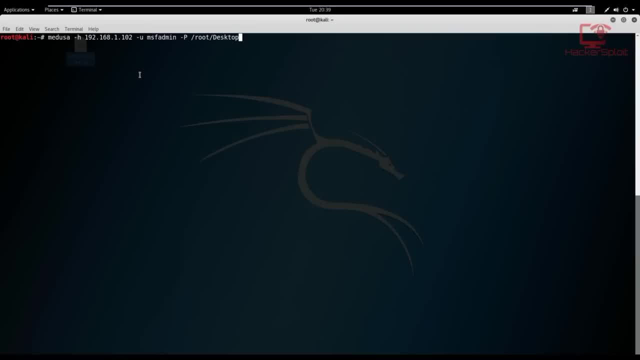 case, we're just going to be using the one I created just to show you that the cracking process does work. All right, but it's going to go through it as a word list, All right. it's not going to use a dictionary attack. So root desktop and we're going to select the 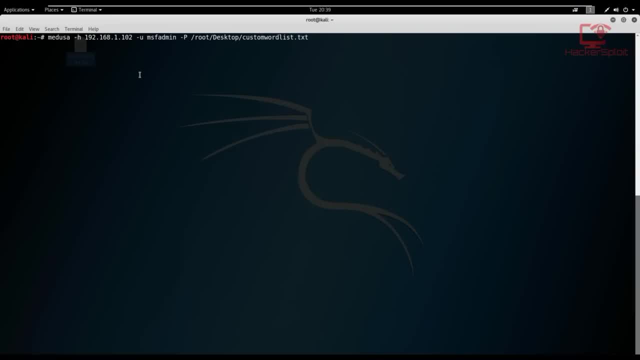 the name of the word list, which is custom. custom word list, dot, txt. All right, And now we need to specify. we need to specify the module, which can be done by using the M, So the module is SSH. And now we specify the end, the end command, which allows us to select the port, which, in this case, is: 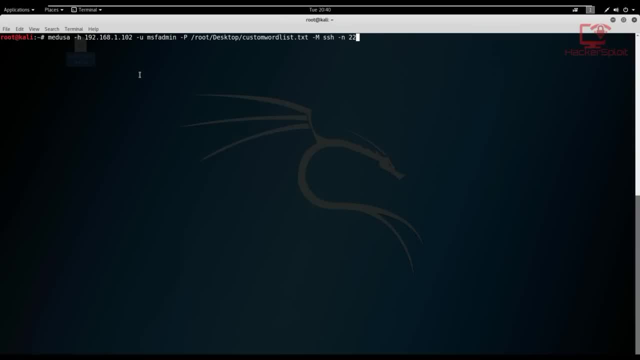 port 22.. That is the default port for all SSH connections. All right, So once we're done, let me just go through the, the command or the entire sequence here. So what you're saying is we're saying Medusa, so startup Medusa, initialize Medusa. we then use the. 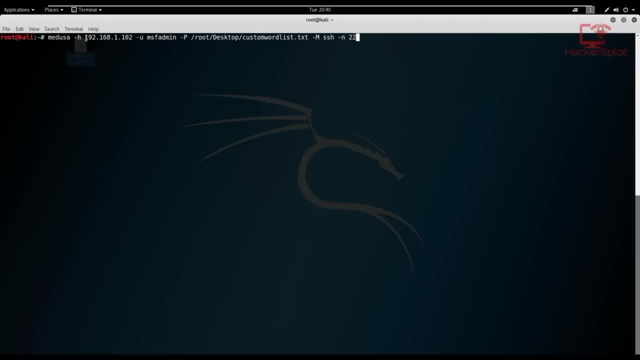 H command to specify our host. Now, if you use a capital H command, you can specify a list of hosts that you have saved in a txt file. you then have your U command, which selects your username, the username you have to try against. you then have your P command that selects the word list or the. 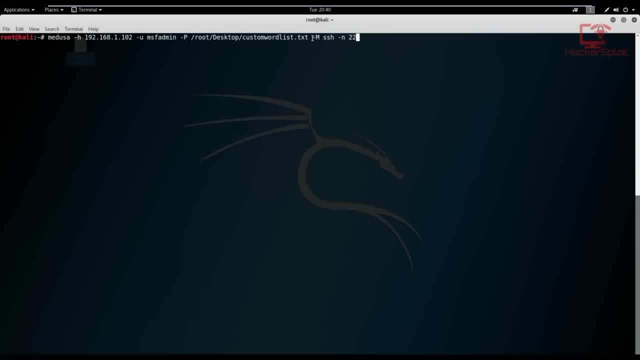 password, or the list that contains the passwords that you want to test for against. Now you can also select a password that you want to test against. You would use the, the, the lowercase p. you then select the module that you're going to be using. 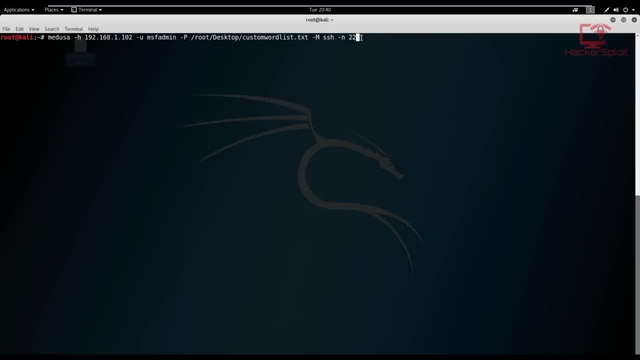 which, in this case, is SSH. you then have the port that you're going to be using, which is port 22,, which is the SSH port. All right, And once we're done, we can just hit Enter and it should start. 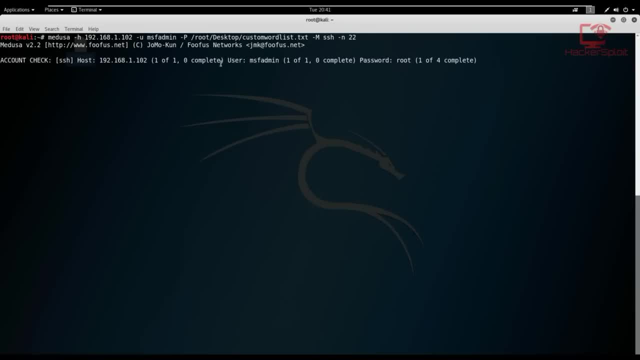 the cracking process. There we are, just give it a few seconds Now, as I said, it's going to go through it as a brute force and it's going to use it as a word list attack And, as you can see, by 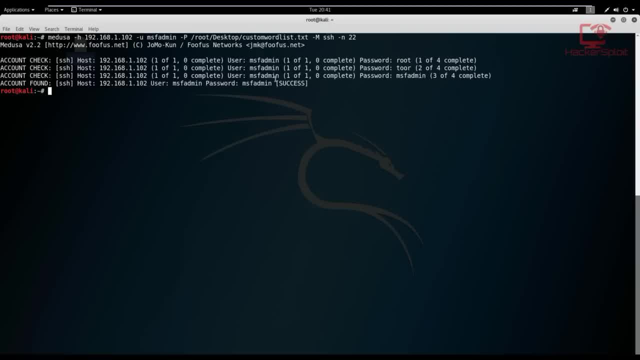 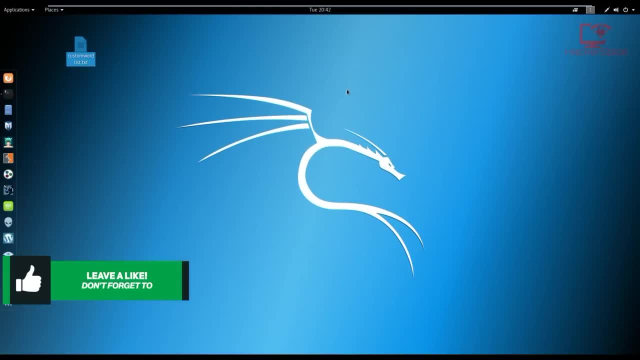 default. it went through all of them, the combinations that it could go through. Now, if you go through and there we are, username is msf admin and the password is msf admin. we use Medusa for password cracking. more specifically, we were cracking the SSH service And, as you can, 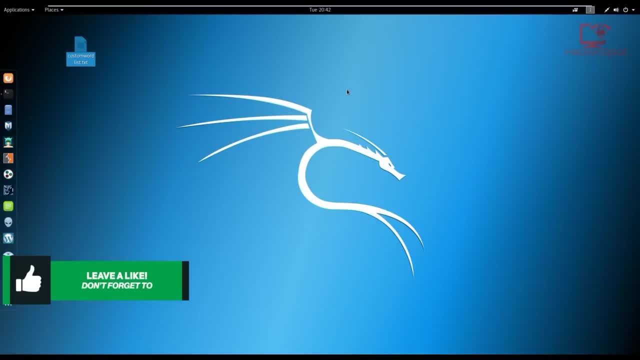 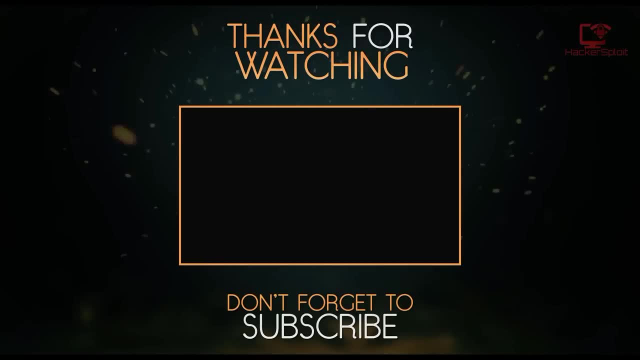 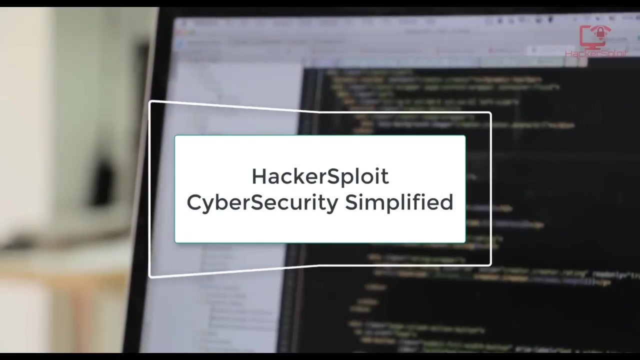 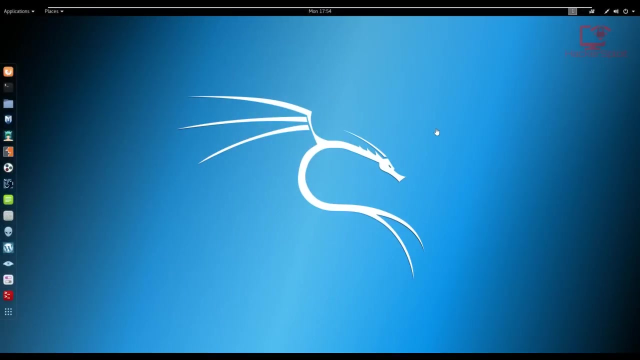 see we got the default username and password, which is fantastic. All right, so let's get started. All right, so let's get started. All right, so let's get started. All right. so hello everyone and welcome to this video. In this video, we're going to be looking at client. 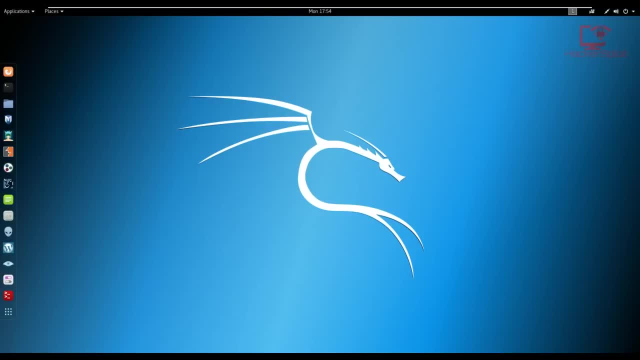 side exploitation. More specifically, we're going to be looking at client side exploitation with the beef framework or the Beth framework, depending on how you want to pronounce it. All right, so you might be asking yourself: well, what exactly is client side exploitation? Well, simply put, 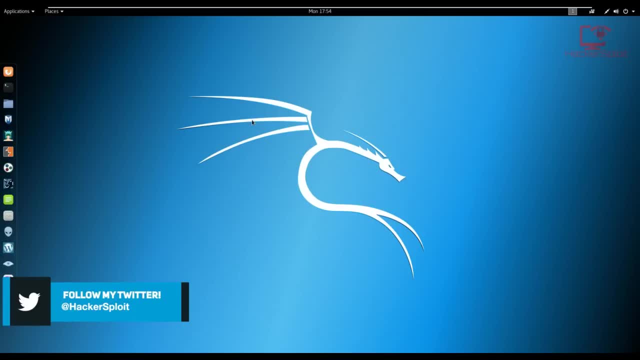 client side exploitation is the process of attacking a client, Specifically attacking the operating system and the programs that are installed on the client's computer. All right, you're doing. what the main objective is is to find the exploits that run on the client's operating system and, more specifically, on the programs installed on that operating. 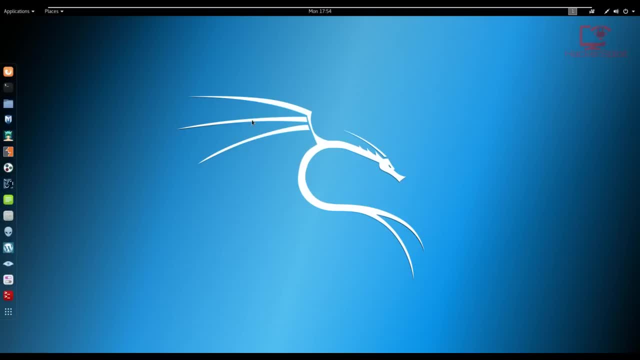 system and to exploit them. Alright. so now you might be asking: well, what exactly are we looking at in this video, when, in this video, we're going to be looking at how to use beef to essentially exploit the browser, All right. so you might be asking yourself now again, what is before beef essentially allows you. 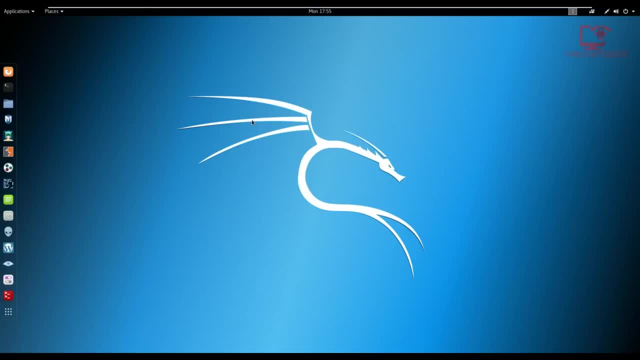 to find and exploit vulnerabilities in browsers. All right, so it is a fantastic exploitation tool that allows you to hook browsers and then to exploit those browsers on the client operating systems and computers. Okay, so it is a fantastic phishing tool. It is a fantastic tool that allows. 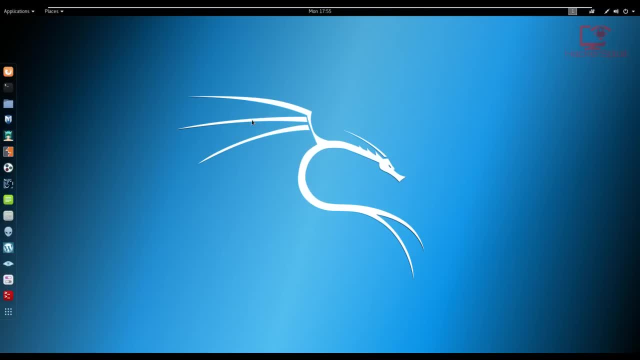 you to perform phishing attacks, That it runs on a web interface, All right. So now we have to look at some very, very important terminology and some prerequisites for the video. Okay, so by default, we're going to be running this now on a client, All right. So what do I mean by this? we're not going to be running this on a 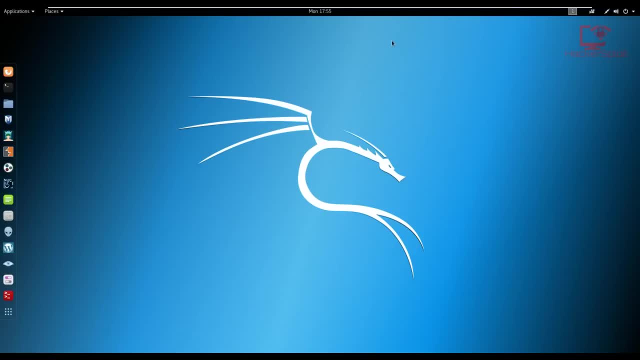 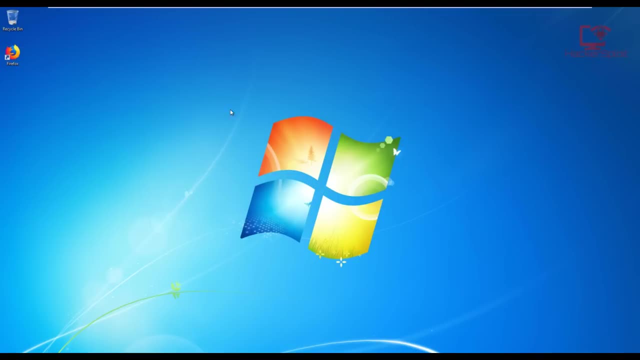 server. So no meta exploitable to this time. we're going to be instead using the window. we're going to be using a Windows operating system. more specifically, we're going to be using Windows seven and we're going to be exploiting or hooking the browser, which is, in this case, Mozilla. 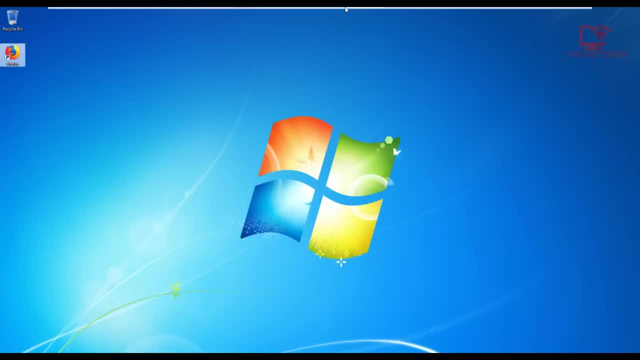 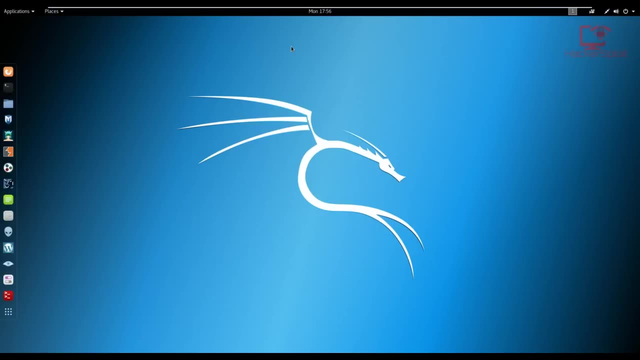 Firefox, We're going to be finding exploits that we can run on the browser. All right. so beef is a fantastic penetration testing framework that allows you to test for vulnerabilities and exploits on browsers. So let's get started Now. by default, as I said, we're going to be using Windows. you can use any. 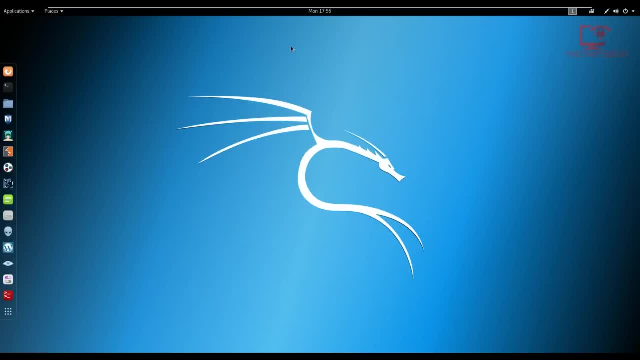 operating system, any Windows operating system or computer that is running on your network. Okay, so this this is going to be performed on our local layer network. So if you want to use beef on on computers or clients that are outside your network or in in, simply put: 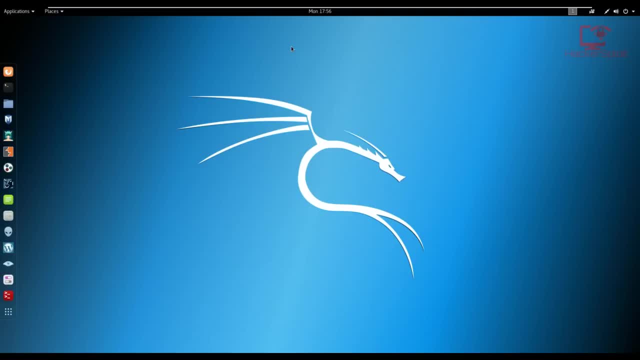 computers that are, you know, across the world via the internet. you then need to set up port forwarding, But that is an advanced topic that we will hopefully probably discuss in another course, But for now we're going to focus on performing this on our local layer network, in a, in our virtual 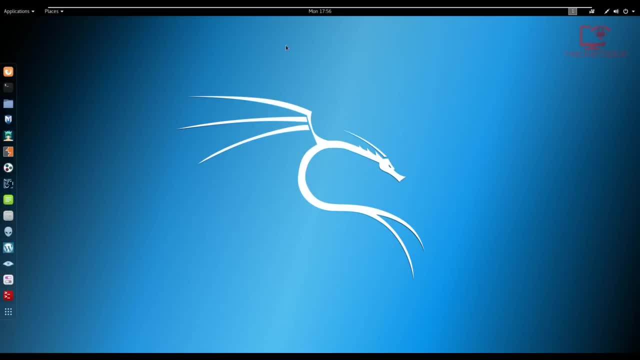 lab. Okay, so by default the beef framework is pre installed on Galin next, which is fantastic. all you need to do is just update your repositories and update your packages and have it installed to the latest framework. So it is usually found on the dock here, So on your left, if you just go to this cow image here, by default you 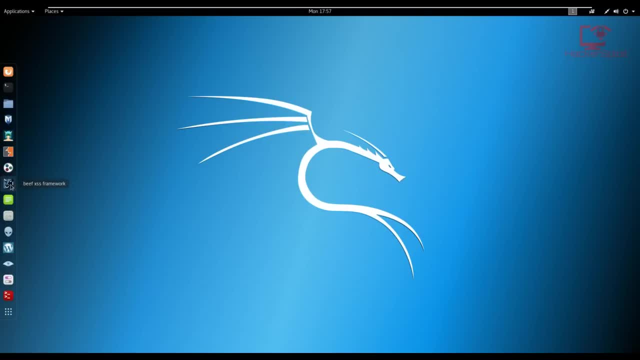 have the beef cross site scripting framework. So that is what XSS denotes. All right, so it can also be found in the applications menu. If you go to the applications and you go to exploitation tools, you will find it under the Armitage. you'll find it there: beef XSS framework. So you can start. 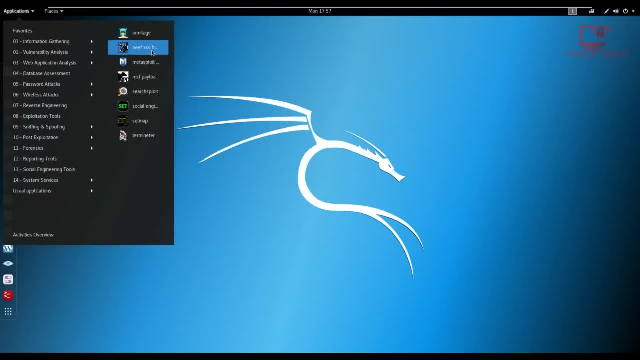 it directly from here and it's going to start the beef services. it's going to start the beef service for you. Or instead, you can go to the, the user directory, and the, the actual beef directory, and start the service from there. I'm going to be showing you two of those, two of those ways of. 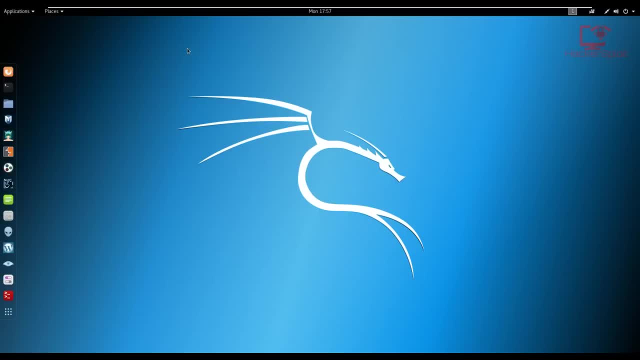 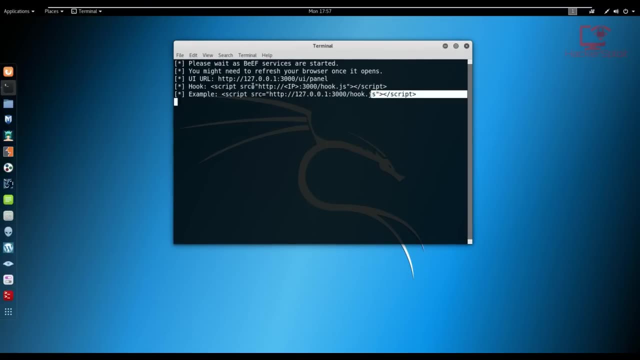 starting it. So if we started from here, if I just click on this or you started from the dock, it's essentially going to start the beef services And it's going to give you information about. it's just going to display some information here. that is very, very critical. So I want you to 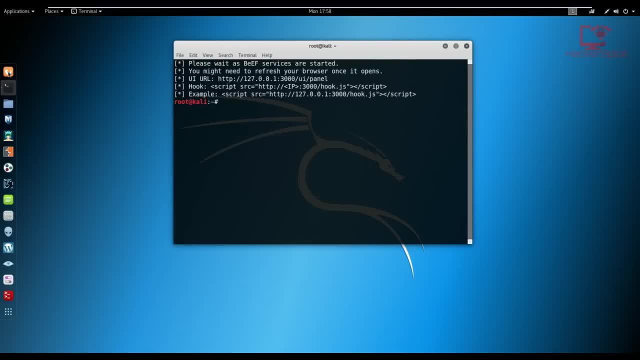 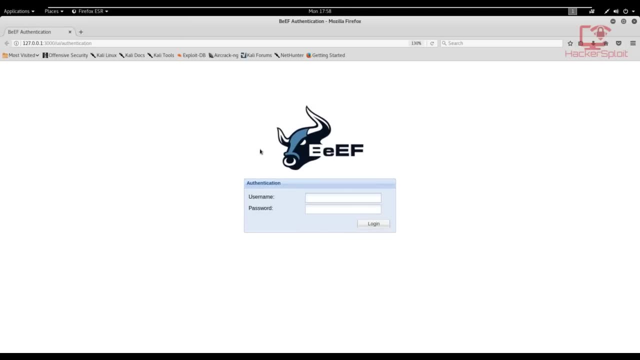 leave this terminal open And once it's done, it's going to open up beef in your browser. So give it a few seconds. There we are and welcome to beef. So now it's going to display to you this authentication screen. 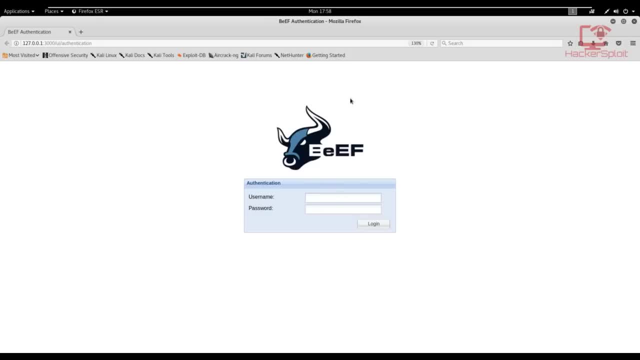 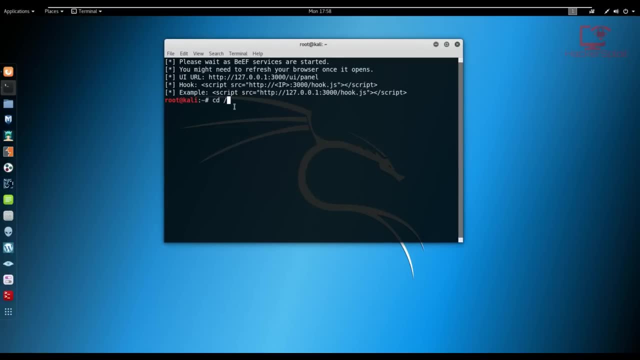 don't worry about the username and password combination. we'll get to that in a second. So that is the first way of launching beef. The second way is going to the, to the directory which can be found at CD user share and the beef cross site scripting folder. So if I click on that and I just 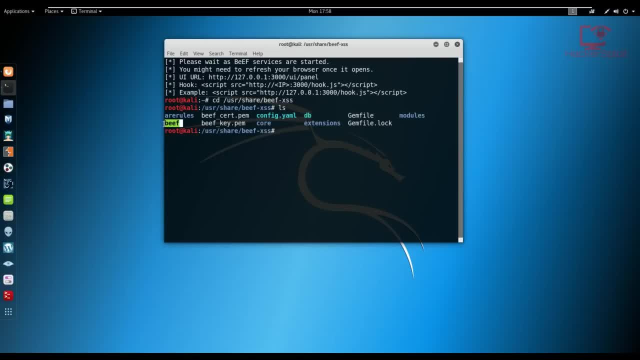 list the files in here you can see we have the beef executable. So if we just launch it by using the shell execution here, so we just type in beef and just hit enter and it's going to start up beef from there. Alright, so we have already started it, So we do not have to do it that way. 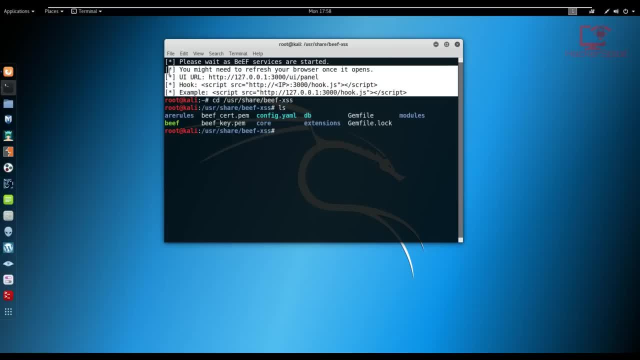 Now it's going to display some information here that is very, very important And we need to look at some of the terminology before we get started. So you might have heard of me saying things like hook Alright. so the most important thing with beef is hooking Alright. so you might be asking: 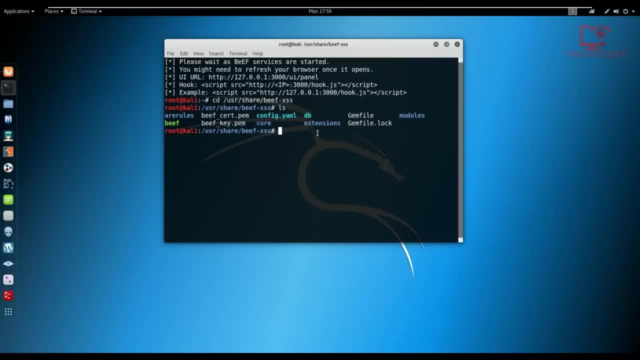 yourself: what exactly is hooking? what is the hooking process? alright, so the hooking process is essentially getting the client to click on a link that contains the JavaScript file, the hook JavaScript file, and then that JavaScript file will be processed by the clients web browser and then it will tie their browser back to the beef. 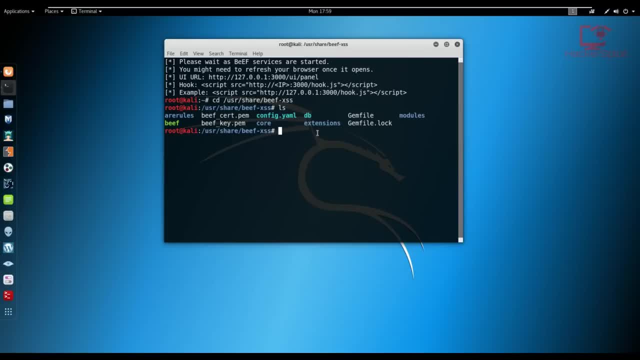 server. alright. so simply put, essentially, what the process of hooking is is getting your client or your target to click on a link that contains the JavaScript hook file. that JavaScript hook file will then be processed and then that browser will be will be hooked or tied back to the beef server. 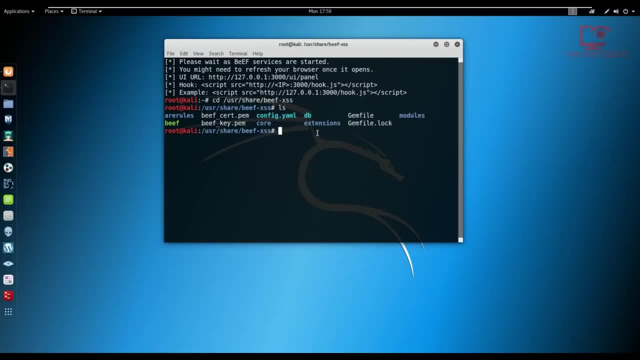 alright, so that is the hooking process. so you might be asking: how do we go about doing this? well, as you can see, the information provided to you firstly is the beef server URL, or the interface URL. as you can see, it can be found by going to HTTP 127, point zero, point zero one: the 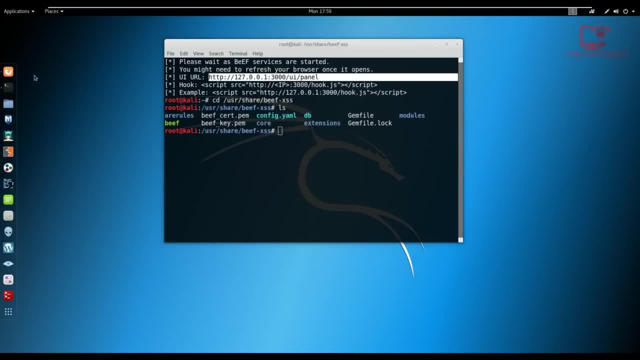 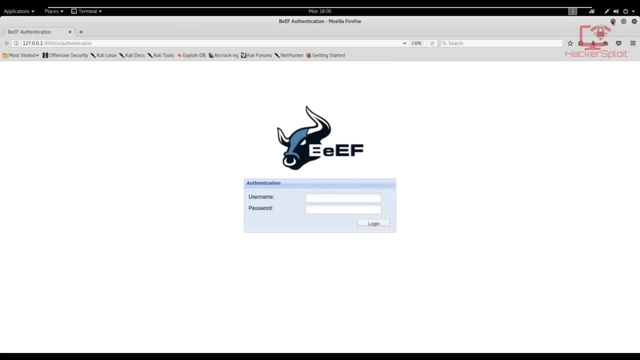 port is 3,000 and UI panel. so if we go back to the browser, you can see that indeed it is running on that. so that's the process of hooking the client to the beef server and then the client will then go back to the server and that is just the beef framework. looking at the hook, the JavaScript file. 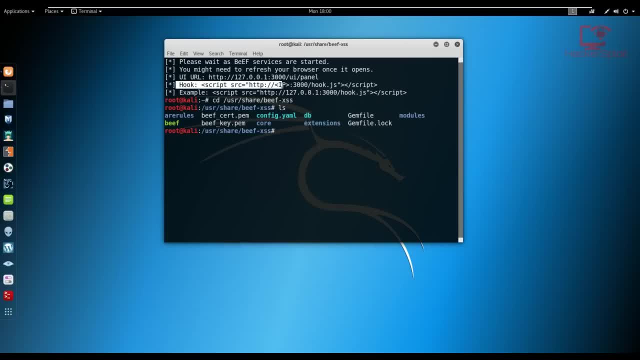 you can see it right here, right? so it's going to give you a hook right here. so the hook- this is very, very important. it is essentially a JavaScript file that you would include in a web page, alright, so now you might be asking: well, how are we going to actually emulate this on our 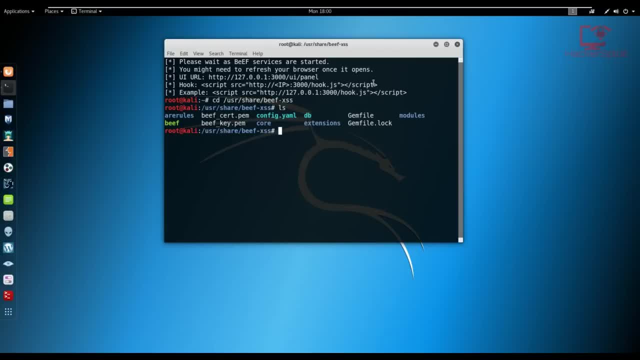 virtual environment. well, what we're going to do is we're going to start a local web server here on our Kelly next machine, and then we are going to incorporate this, the JavaScript, this script, right here into the header section of the web page, and then we will then send the IP address to the. 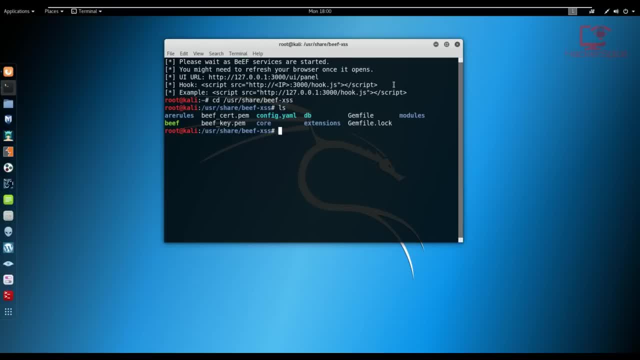 browser that we want to. we want to hook, and it's going to open the web page and, furthermore, the browser will then be hooked. okay, so the first thing we need to do is we're going to be using the Apache web server on cali index, right, so that is very important. the second thing we need, as you. 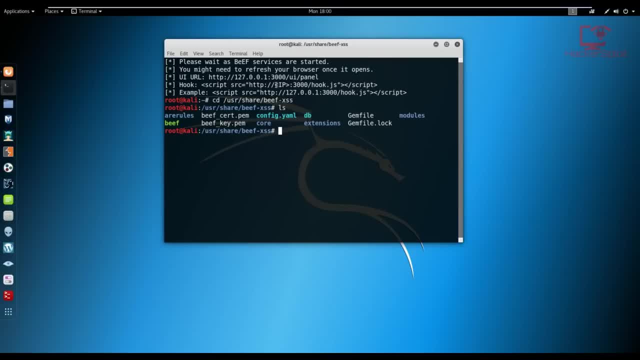 can see. if you look at the script right here, it's going to give you an option to enter your IP address. now, the IP address that it's asking for is the IP address in which the beef framework server is running on. in this case, it's running on the calendar X or virtual machine, so we need to 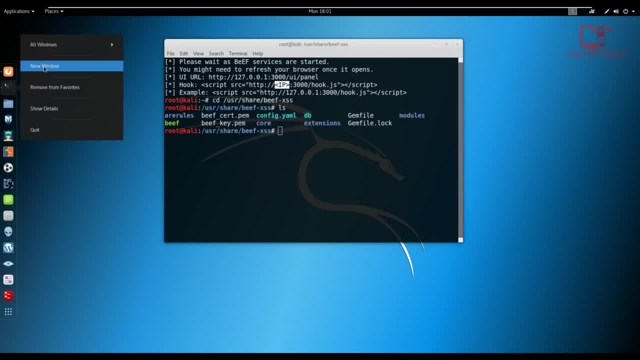 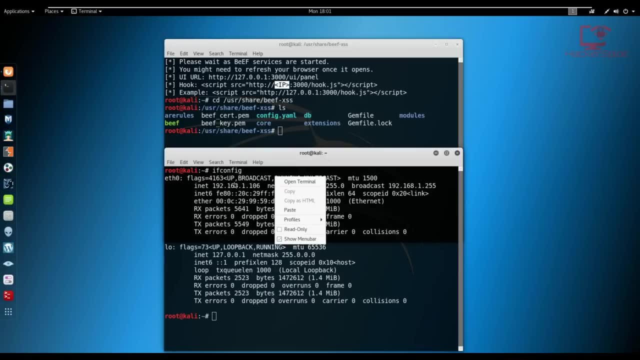 get the calendar X IP address, in this case the local IP address. so we're gonna click on a terminal and we're just gonna hit I have config, all right. and once we get the local IP address right here, which is 192 point one, six, eight point one point one, oh six. that is what we needed, all right. 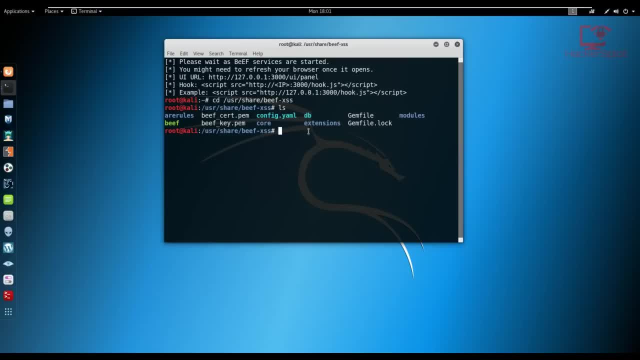 fantastic. so we just need to keep that in mind. and now we, as I said, we need to start the, the local web server, which in this case is Apache. how do we start that service? we go to service Apache to and start right. so very simple to how we started our network services. so I'm just 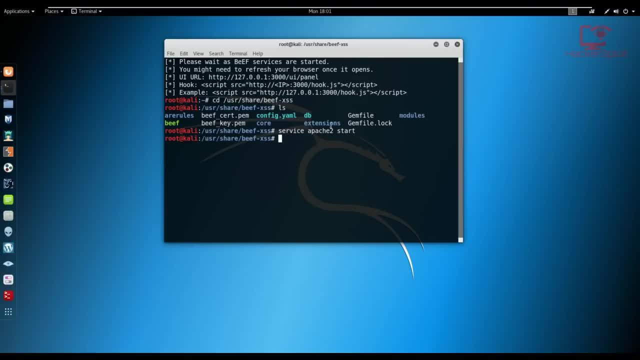 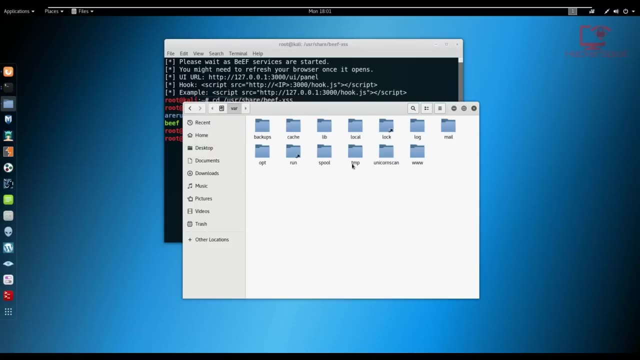 gonna hit enter, fantastic. so now the web server is started. now we need to actually edit the web page file that is hosted on our web server so that can be found by going into your file explorer and going into other locations, going to your computer, going to your var folder, into your www folder. that 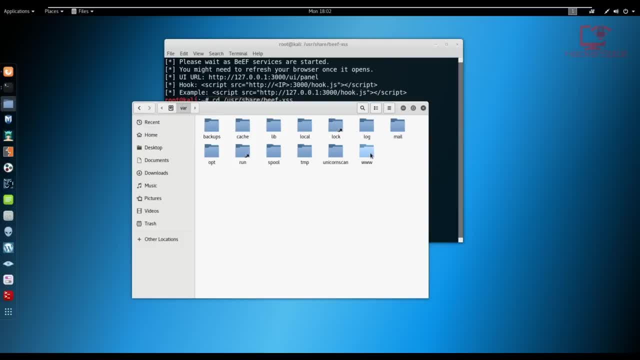 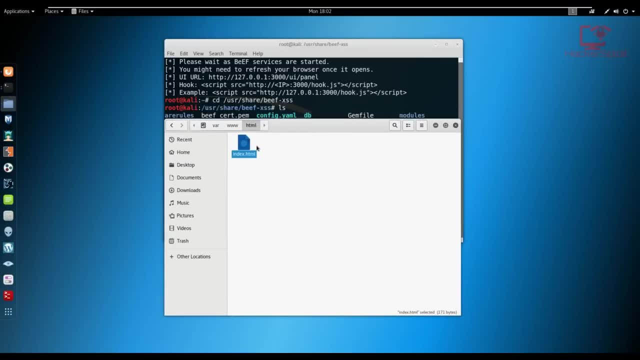 is where your web server files are going to be stored- your local web server files. just click on that and then you'll find an HTML folder. click on that and then you'll find an indexhtml file in here. if yours is empty, just create an indexhtml file and we'll we'll add some code into it, to just 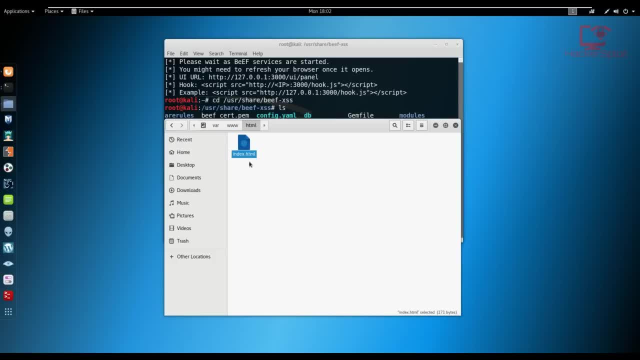 make it a simple web page, okay. so if you do not have any files, just create one. if you have any files, just get rid of them and create a new one. all right, so I've already created one. so what I'm gonna do is we're gonna edit it with our text editor, so I'm just gonna open up, I'm just gonna. 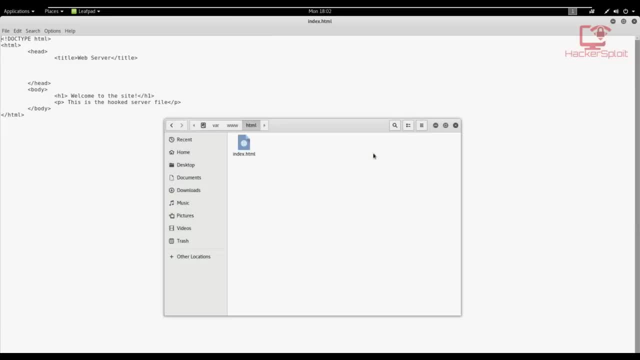 open it up with leaf pad. all right, fantastic. so once I've opened it up with leaf pad, you can see that I've just created a simple HTML template here. if you're familiar with web development, you know this is a very, very simple website, essentially what's. 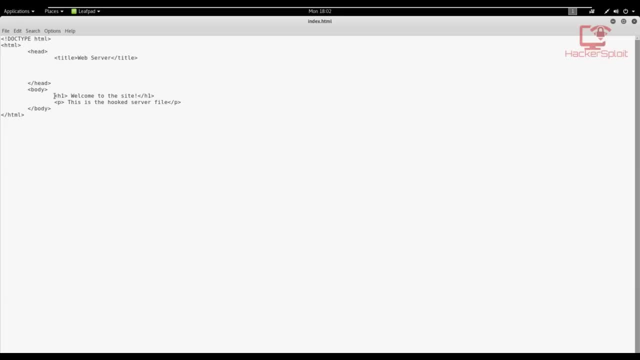 happening here is it's going to essentially display welcome to the site and it's gonna say: this is a hooked server, so we know that this web page has been opened successfully, all right. so, as I said, by default in HTML, any JavaScript code is supposed to be included in the head. 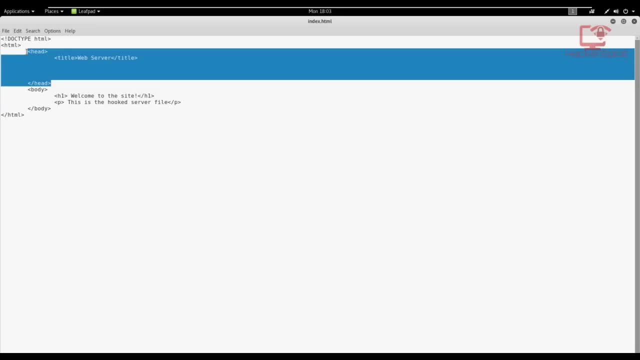 section of the web page. all right, so it's supposed to be included within the opening- closing tag, at the opening and closing head tag. all right? so what we're gonna do is we're just gonna go to the information that I was provided to us here and we're gonna copy this script file. 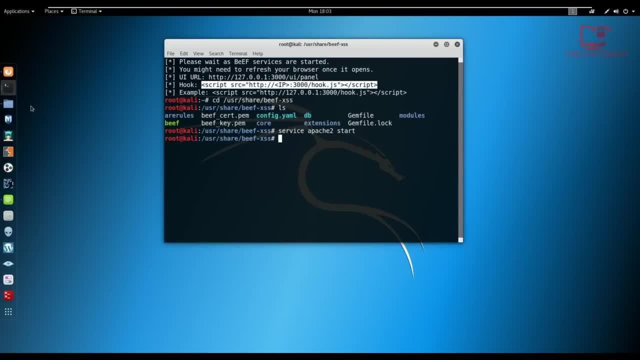 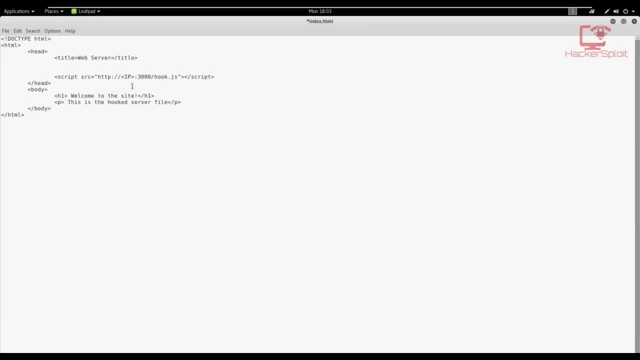 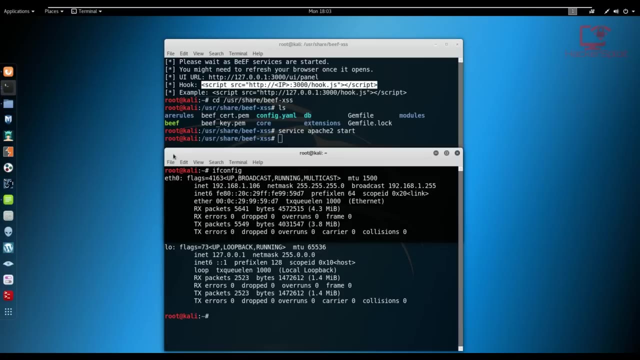 all right, so we're just gonna copy it like so and we're gonna paste it in the head section here. now we need to change the IP address to the IP address or in which the beef framework server is being hosted, which in this case we saw as the Cali Linux IP address here. so there we are: 182.168.1.106. that. 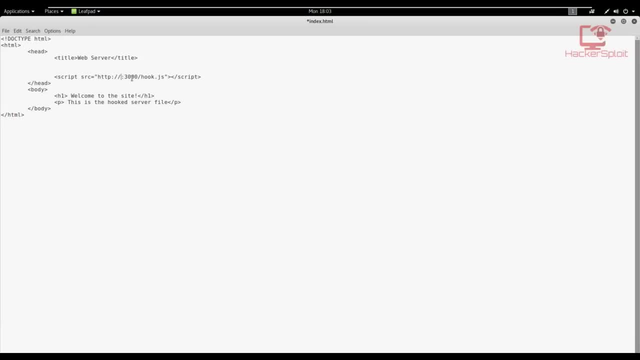 so we're just gonna change it to that. so, 192.168.1.106, and you want to make sure that the port is 3000 and it is using the hook JavaScript file? fantastic, so let's save this. and now, essentially what happens is when anyone will access this IP address here, in which we have 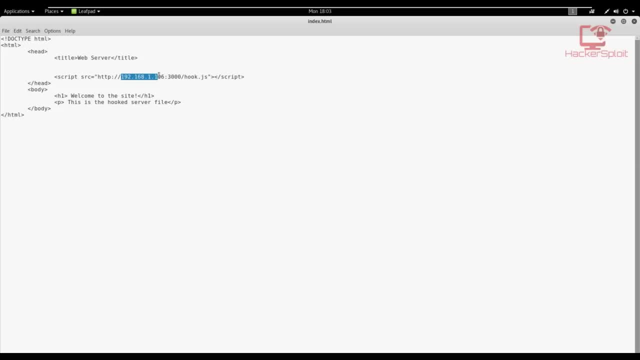 hosted, the local in which we have the local host or the local web server. it is going to execute the hook to JavaScript file and that will tie the browser to the browser, or we'll essentially hook the browser and we'll be able to access and exploit it from. 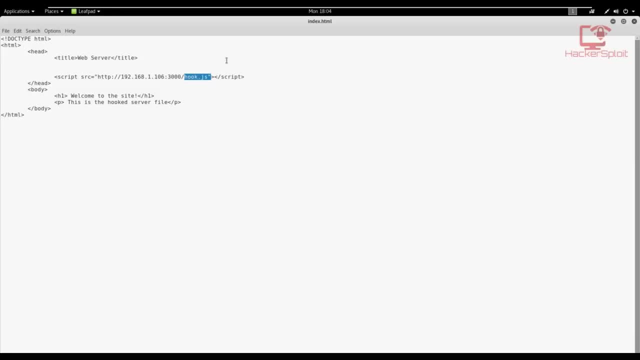 the beef framework web interface. all right, that we already have opened. okay, that was a mouthful. now let's get to actually executing this on our of our browsers. so once you've hit save, so you can just save it, and I've saved it, so we don't need to worry about that. about that now, pardon me. 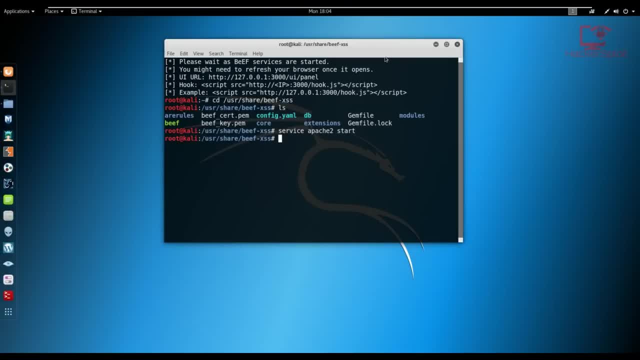 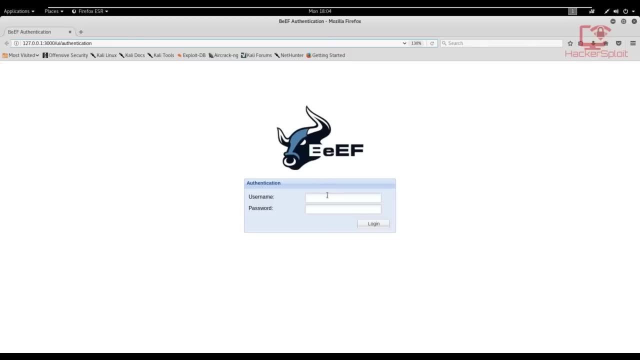 so now what we need to do is we, we just we- can close that and we can leave this open. now we've started the Apache 2 service. now we need to log into the beef framework um user interface. so the default username is beef- all right, and the default password is beef- fantastic, that's quite simple, isn't it? so we're just going. 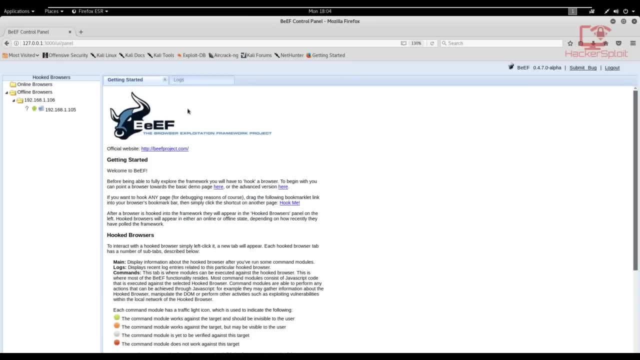 to log in and welcome to beef now, by default, the interface that you will get if this is your first time running it will be pretty much the same, apart from having information here. so, for example, I already have been performing penetration tests with beef before, so I already have an IP address. 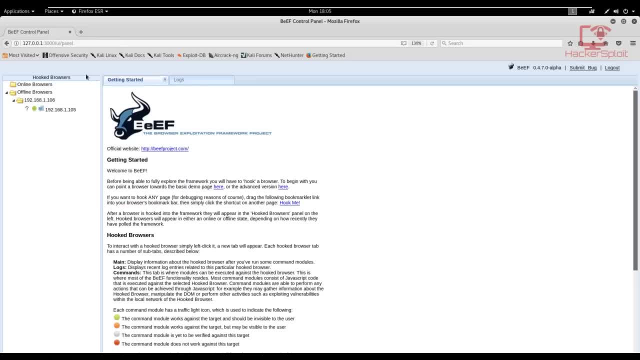 or a browser hooked here. so don't worry about that. essentially, what? uh, if you look at the basic interface here, it's really really simple. uh, on your left tab, you have your hooked browsers and they're sorted in terms of online and offline. in this case, I have an offline hooked browser here and I have no online. 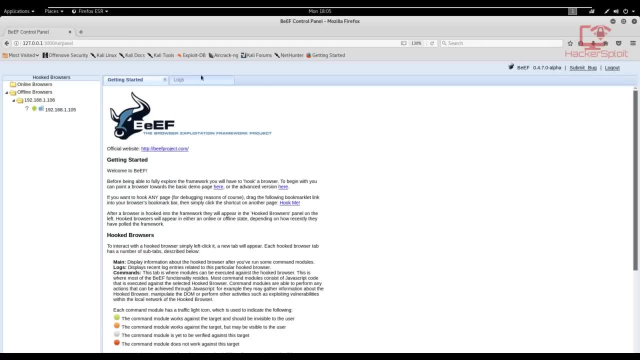 browsers. but we'll be getting to that in a second. you have your getting started guide here and you have your logs here. we'll be looking at that in a second. fantastic, so we've started the beef framework. now we need to actually run the HTML file on our browser, in this case. 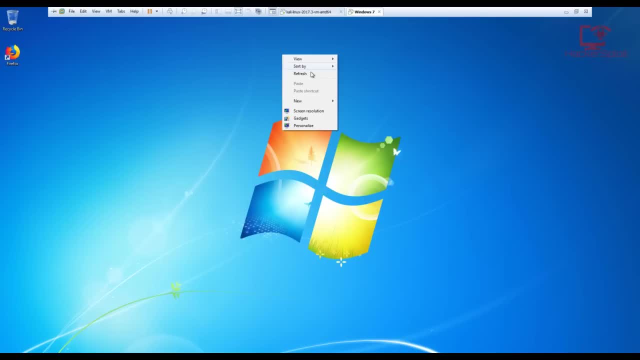 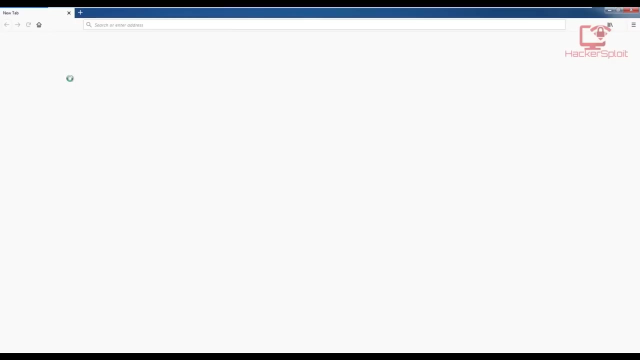 we're going to be running this on our Windows 7 operating system here. so this is a fantastic- uh, you know, a fantastic- opportunity for me to actually demonstrate what a client would do. so, for example, now, if I just opened up my browser, all right, and I sent, I sent, uh, I sent my client or a target that 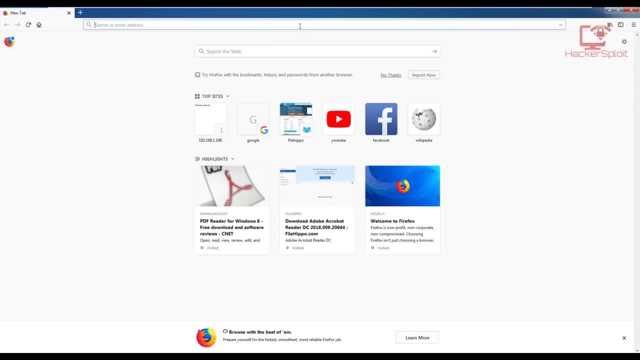 I want to attack. I sent them a link that contains the JavaScript file. so in this case, the link is: uh, it's hosted on our local servers, which is, in this case, 192.168.1.106. so once I- if once I- hit enter, it's going to load up the local server and it's going to display the HTML file that we created. 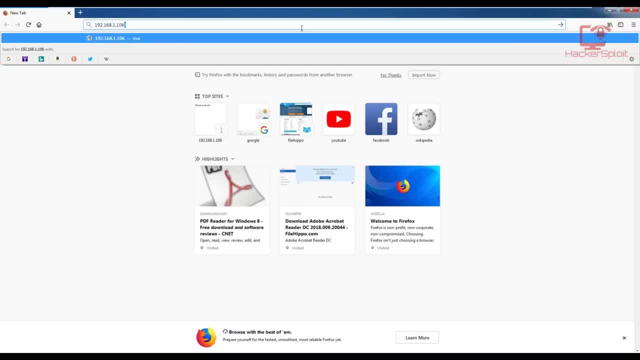 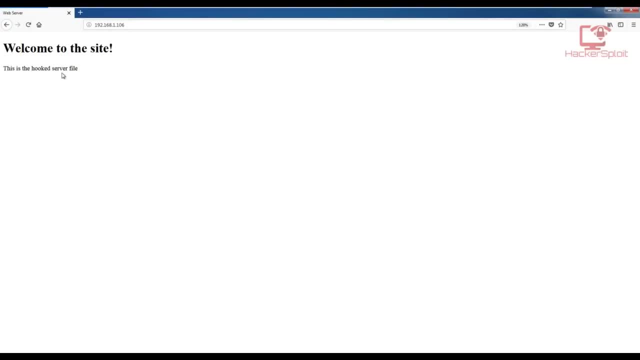 and the file that contains the hookjavascript file. so once I hit enter, as you can see, it's going to display the information that we added to the web file, which is welcome to the site. this is a hooked server file. now you might be asking: well, what is that exactly has happened? has this browser? 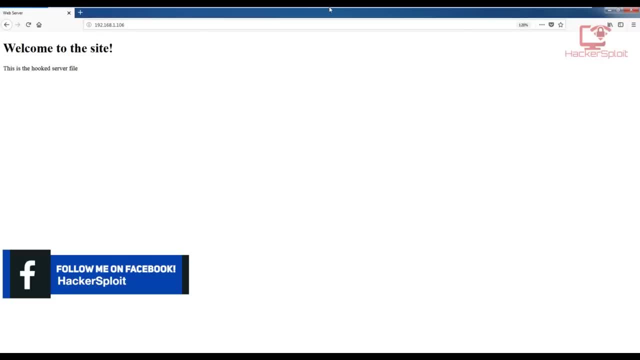 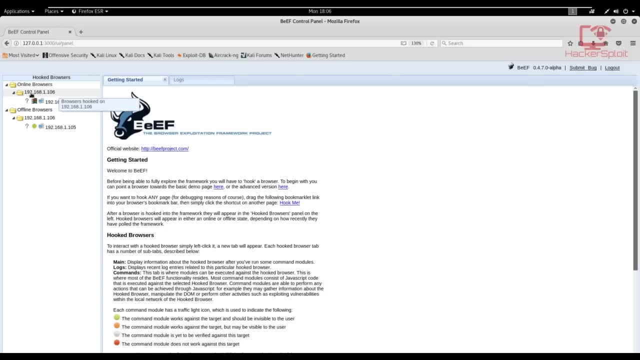 been hooked? the answer is yes, it has been hooked. if we go back to the browser and we go back to the app and go back to kali Linux and we open up our Biff web interface, you can see if we go to online browsers it has been hooked and the IP address is 192.168.1.110. so you might be still skeptical. 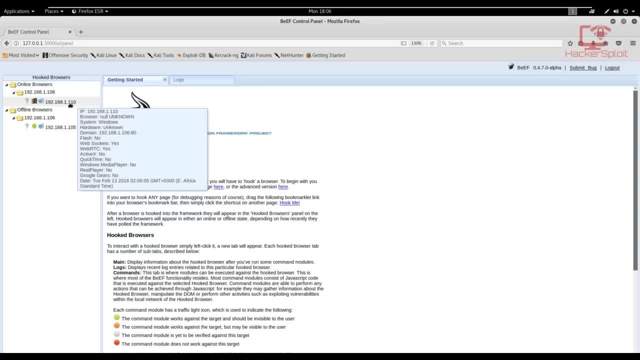 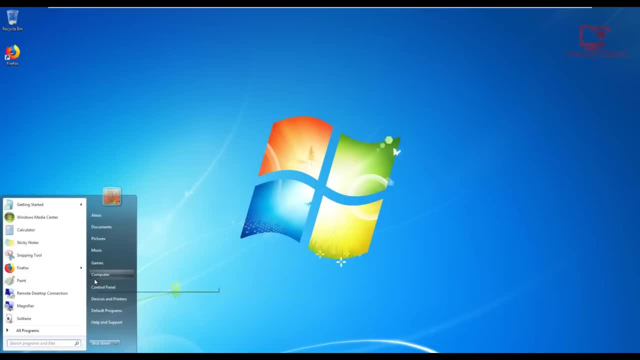 and you might be asking: well, how do I know that's the? that's the correct browser, that has been hooked. so let me just go back and I'm just gonna run an ipconfig command here to just show you that that is the correct IP address. uh, oops, for some reason I I just launched it from there. so 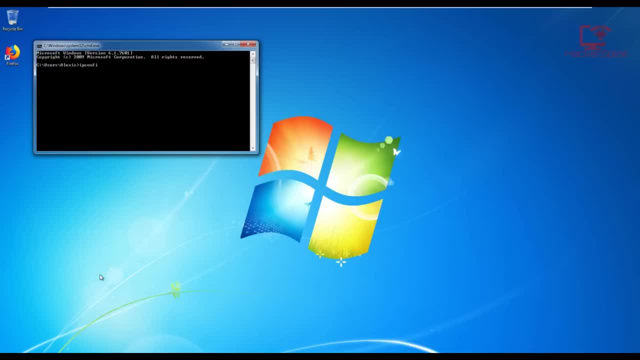 let's go back to the code and we just see that our Gpd file, it's finally accepted and we've got the me. just open the command prompt, IP config, And, as you can see, the IP address is 192.168.1.110.. 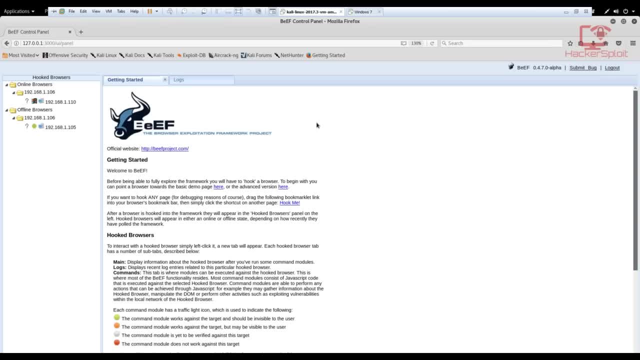 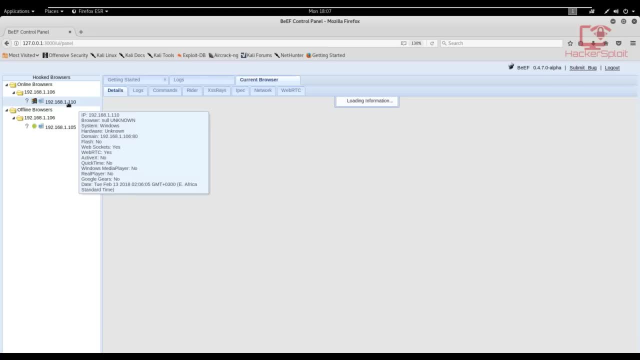 Fantastic, So we have hooked a browser. Now you might be asking: Well, what do we do now? Fantastic, we've actually hooked a browser. how do we get to exploit it? Well, the first thing we need to look at is we click on the hooked browser here. it's going to display some information here. 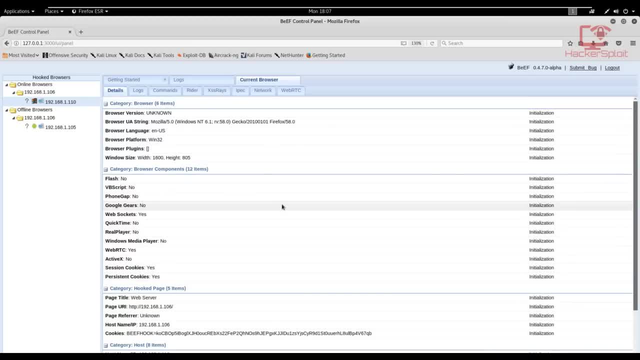 which is very, very important. It's going to display information about the browser, So by default is going to display information about the browser, So you have your browser version, the browser string, which, in this case, was information about the browser. In this case, 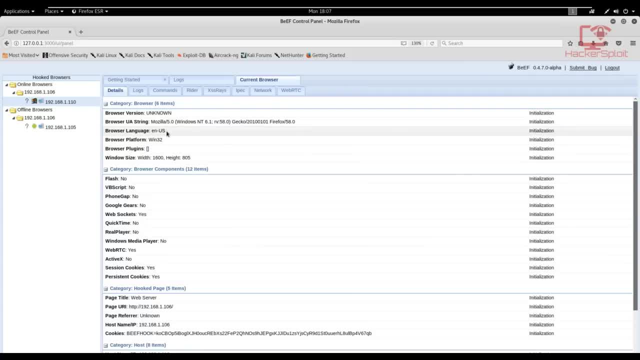 it is running. Mozilla. we have the browser language, the browser platform, which in this case is Windows 32 bit- Excellent. you then have the window size in terms of what is the resolution of the window of the browser. we then have the browser components. So is it running? 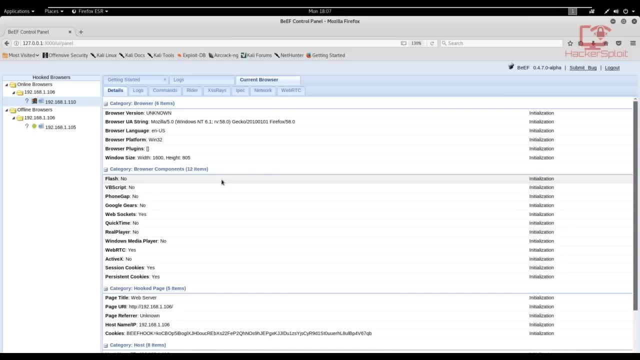 Adobe Flash. So that means we won't be able to exploit any Adobe Flash vulnerability. It is so again, information gathering is also a part here. Okay, so we then have information like session cookies Interesting, So that means we can actually get some session cookies Very. 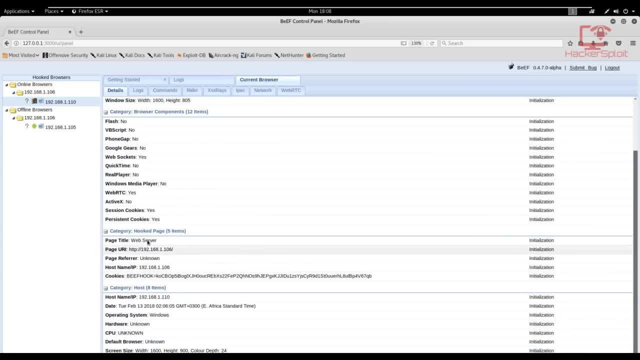 very important thing to keep in mind. you then have information about the hooked web page, which is the web page we created. you then have information about the host, which is the operating system and the hardware, which, in this case, we have not been able to get. 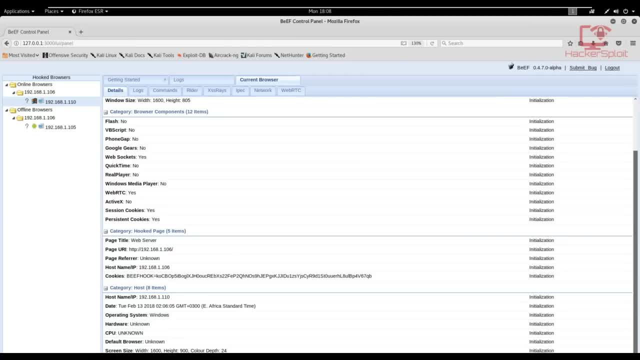 it also displaying useful information like whether or not the device is running on the touch screen. In this case it's not. So now it's time to look at some basic exploitation. Now we have looked at already how to hook the browser. Let's look at a very 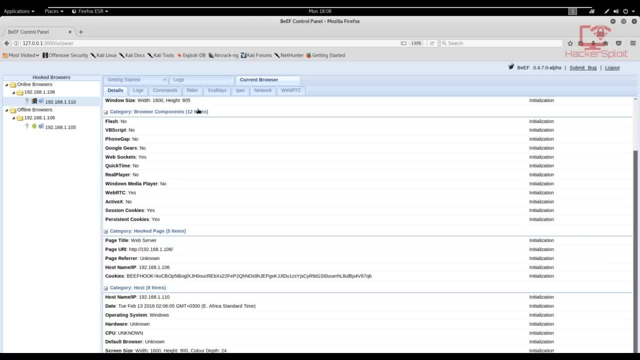 very simple exploit process Now by by default. I just want to say something: not every browser is going to be a fully vulnerable browser, in the sense that all the major browsers that you'll find out there- for example, Mozilla Firefox, Google Chrome- will have export exploits patched or fixed. 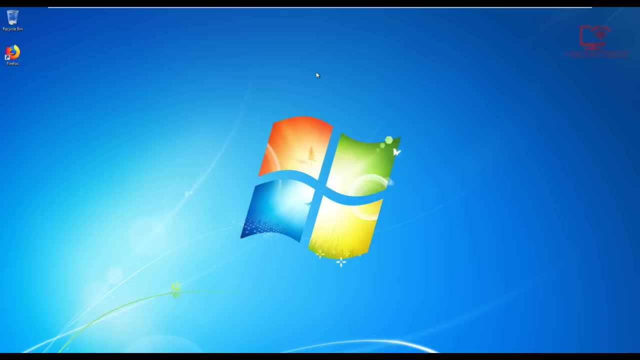 So it's going to be very, very difficult or very tricky to find exploits that are not already patched Alright, so you can only get a certain amount of information. If you're lucky and a browser has not patched a certain vulnerability, you can, you can, essentially. 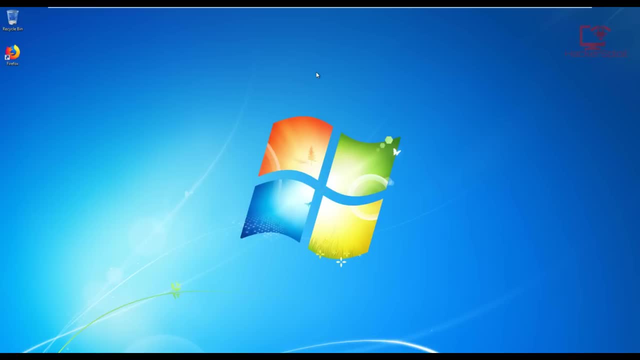 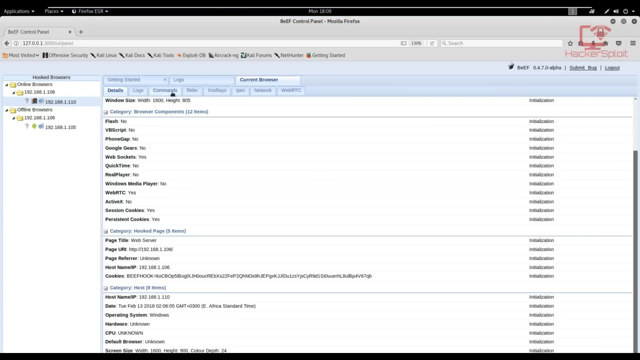 get information from there- Alright, but by default, beef can be very, very powerful if you actually find a vulnerability. that works, Alright. so we're going to go into commands. all the modules can be found in commands- Alright. the rest of the sections are more of an advanced 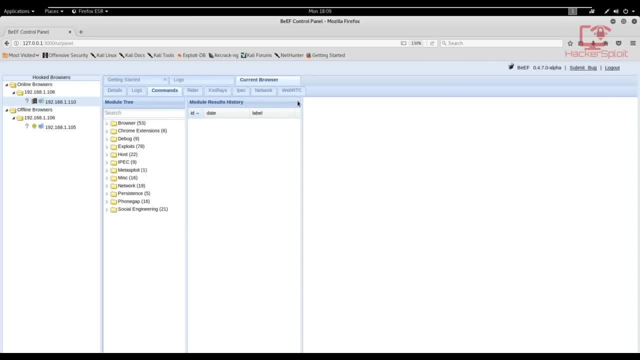 feature. that will probably look at an advanced course, But for now let's look at some basic benefits of Adobe Flash, once we'veBarbarians, Alright. so what we can do is if we look at the modules here they're sorted in terms of browser Chrome extensions, That is, if you're running a. 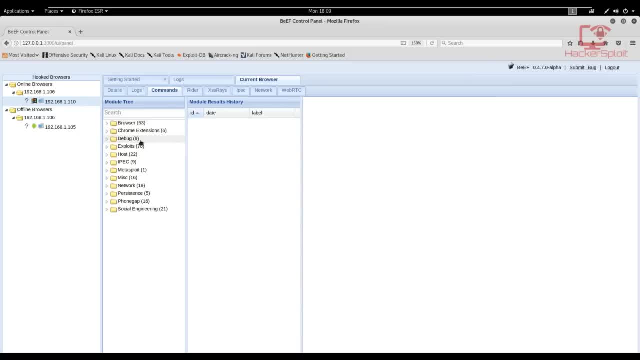 Chrome. if you're hooked a Chrome browser, you then have your debug, your exploits, Metasploit. you can run Metasploit exploits on it, you can perform social engineering, etc. etc. Alright, so now we're looking at information that we can use here. 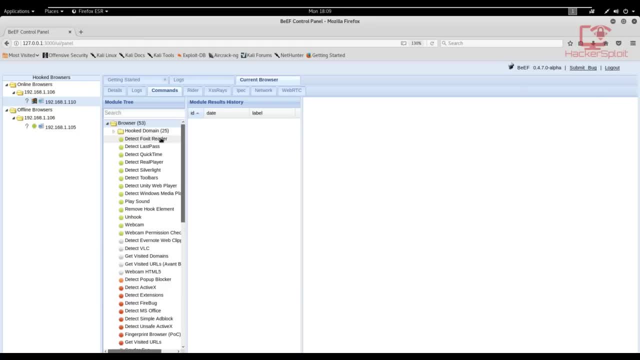 we already knew that we do not have Adobe Flash running, so it would be pointless trying to to actually run Adobe flash exploits. okay. so looking at some of the modules, we can actually run. we can play a sound. we can remove the hook element. we can unhook the browser. we can you can take pictures using the. 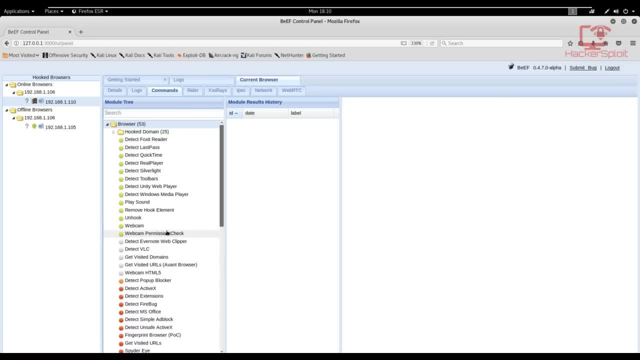 webcam. now, by default, as I said, this might not work, depending on the browser that you're using most of. if the if your client is running an outdated browser, then it might work, but by default it'll not work. alright, you can look at the visited URLs. so if you check for a URL here, 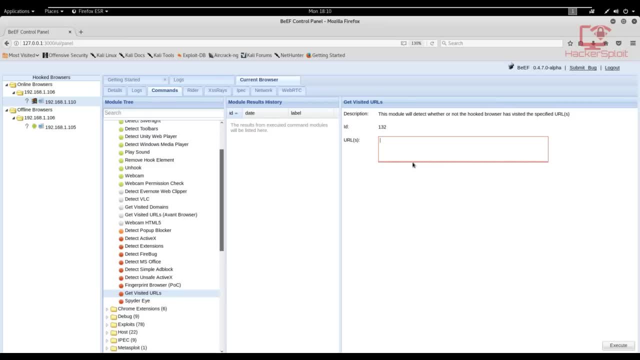 so let's see if I tested something like: let's say we wanted to know if our target has visited a website like wwwbbccom, we would enter that in here and we would hit execute, alright. and once we hit execute, what would happen is a command would be stored in the module results history section. 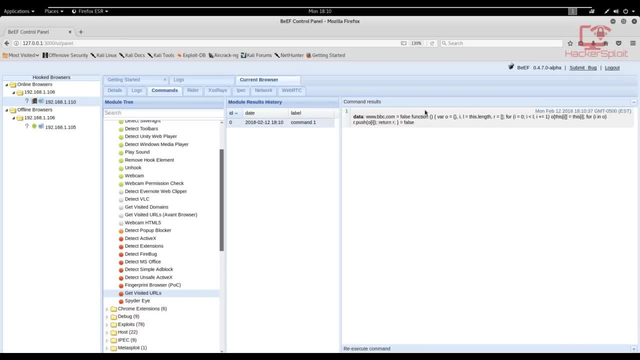 here that will log the commands that you've entered and, as you can see, it's going to give you the command results. so in this case it's going to tell us that: did the client browser? did it access bbccom? it's going to return it as false, which means that no, it did not access that, that URL. so that is an. 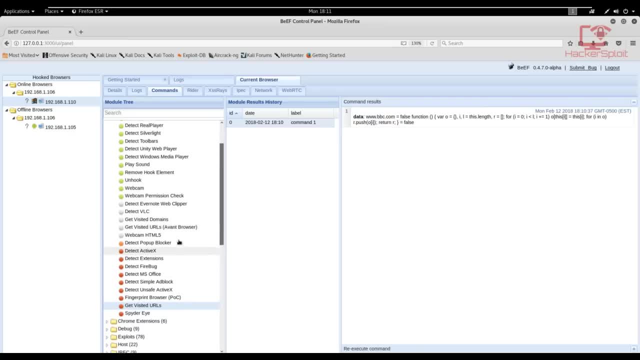 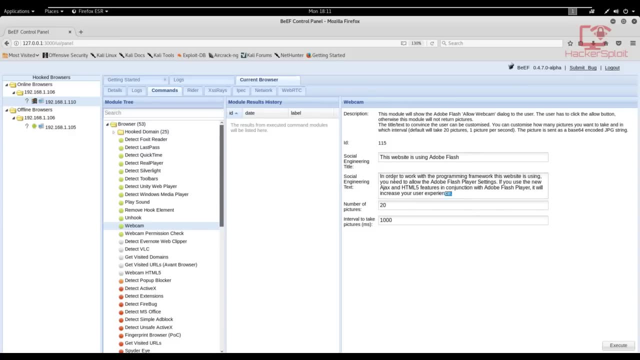 exploit that works and you can test it out for yourself. looking at things like the webcam, this uses Adobe Flash, so you know, essentially, you, you, you can use your social engineering text here if it had Adobe Flash installed. what you would need to do is actually allow them the webcam module to. 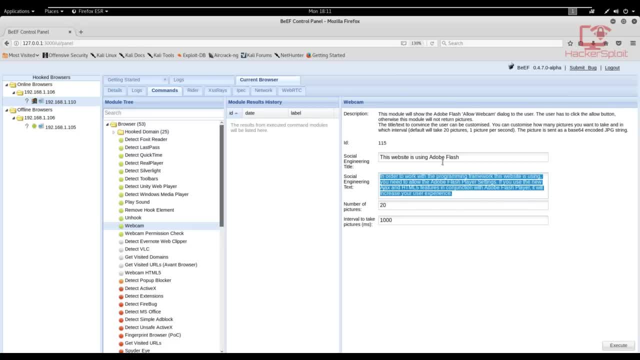 be installed here. so what we can do is we can just change the text here. so let's change the text to something interesting. we can say: hello, you have been hacked, all right, something really, really simple like that, and let's see whether it is actually able to exploit or and. 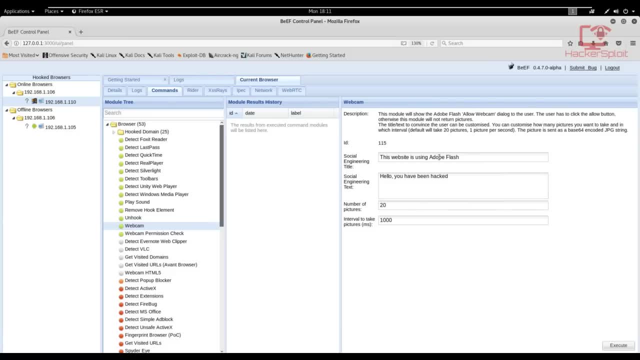 run this social engineering text by default. it is not going to be able to take any pictures with the webcam because, as I said, the browser is not running a Adobe Flash, all right, so we'll change the title to say: you have been being hacked, all right. and if we hit, execute. 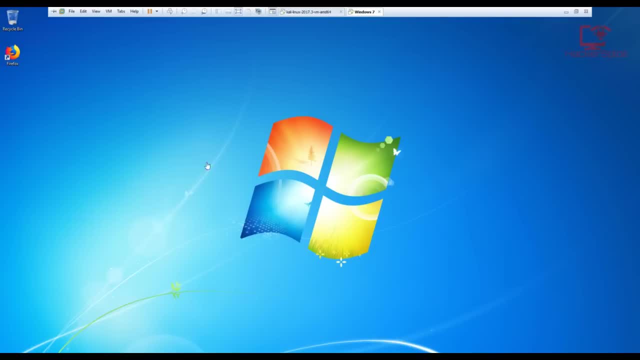 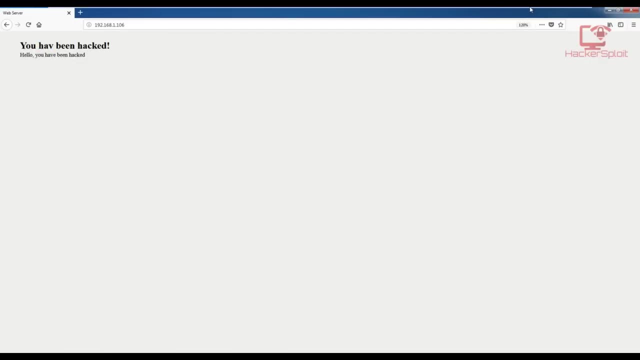 we can go to the Windows 7 operating system and we open up our browser and, as you can see, you have been hacked and for some reason I misspelled have there. let me just change that and make sure that that is correctly spelled and we can execute that again. so you have been hacked. let me execute that. 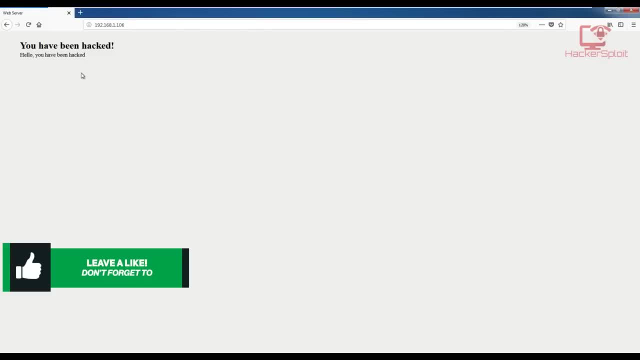 again and voila, as you can see, it displayed a message. now, by default, it's supposed to ask you to install or to enable web the webcam to take pictures, and by default, a user will be smart enough to do that, and that is something very, very dangerous to do. so it's really about social. 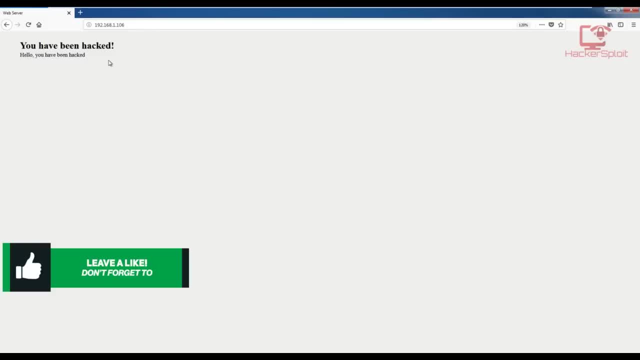 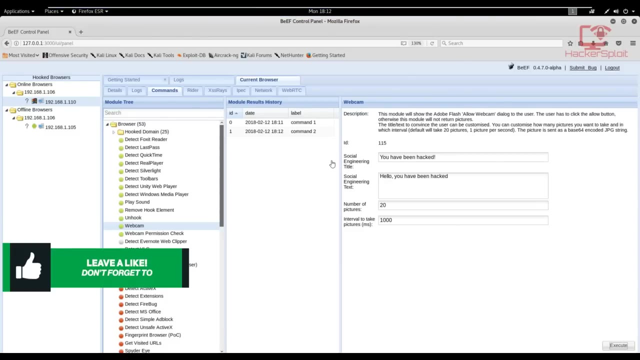 engineering and getting the client or the user or your target to click on things that will eventually exploit or get their browsers exploited. so that was exploitation with the beef framework, more specifically, client-side exploitation, and it's really really interesting to see how you know these exploits can be readily done and be and performed even on a small scale on your local. 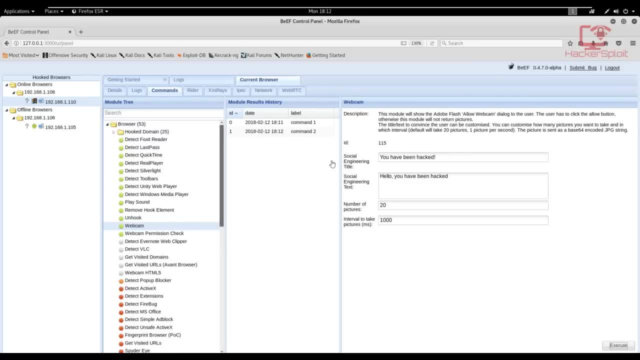 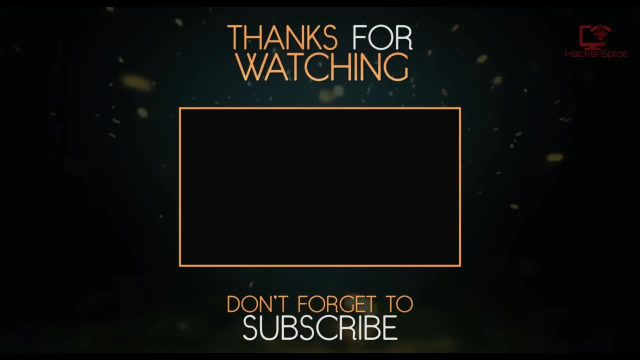 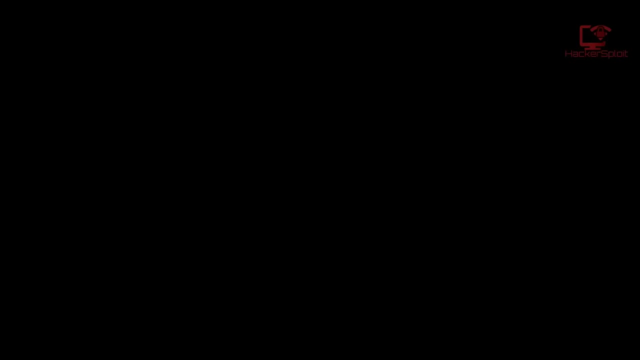 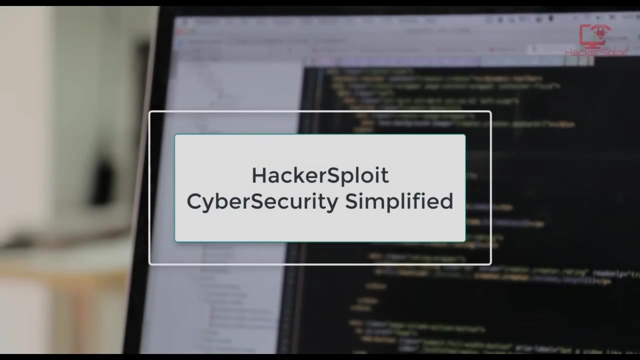 area Network. all right, so that's going to be it for this video. in the next video, we'll be looking at client-side attacks, this time using the social engineering toolkit. so I'll be seeing you in the next video. hello everyone and welcome to this video. in this video, we're going to be exploring Armitage all. 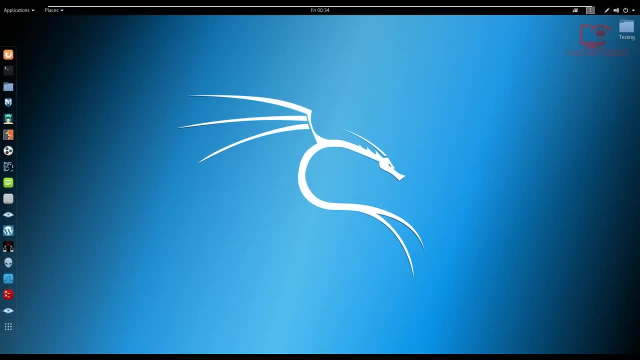 right. so we're actually going to be performing exploits on our vulnerable operating system, which, in this case, is meta splitable too. so I hope you're really, really excited. so you might be asking yourself: what exactly is Armitage? well, Armitage is simply the graphical user interface. 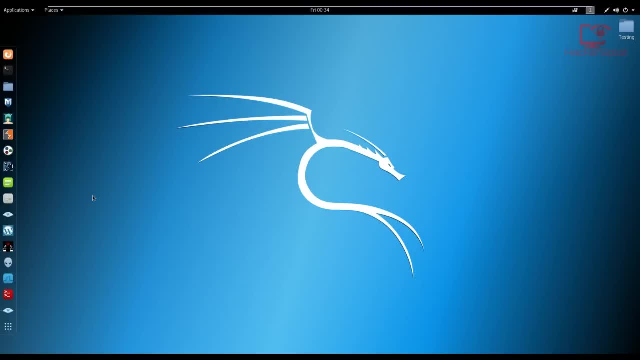 for Metasploit. all right. so the way you have nmap and Zen map, and map being the command line interface, and you have your Zen map, which is the graphical user interface, that is the same way. so you have your Metasploit console and Armitage, so Armitage is the graphical user interface for 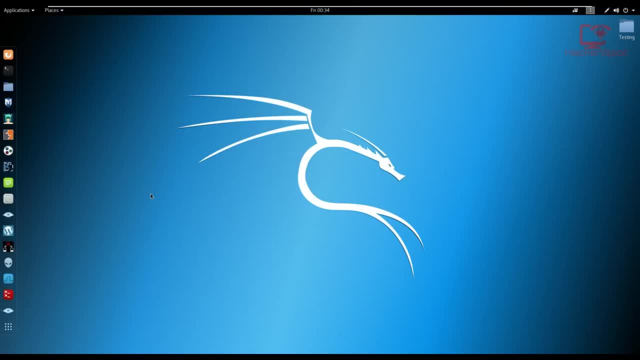 Metasploit. all right. so some of the advantages are: it gives the user much better idea of what's going on. so great ease of access and the user is able to understand the, the scan process and how everything is being exploited. and you just give the, the user, graphical representation of the scan and the. 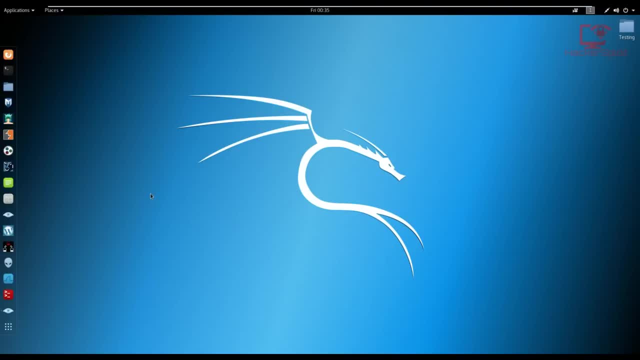 exploitation technique. all right, so let's get started now by default Metasploit- uh sorry, Armitage- is based off the data that you have, which has been. we start by taking all the documentation by the tagging, we start by taking off the local user information and next these are the license. 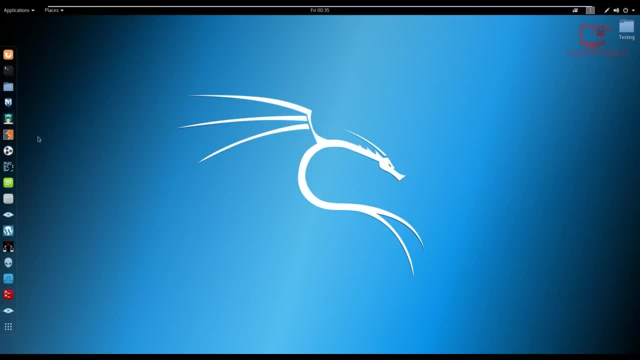 codes chosen, as well as the table fields, we can do all the things we need to do. when you go into the data to see how you can run up some기도 what we're working on here, you have analoge log squid. you gotHub fairly long log file and this allows you to know this is a local master. 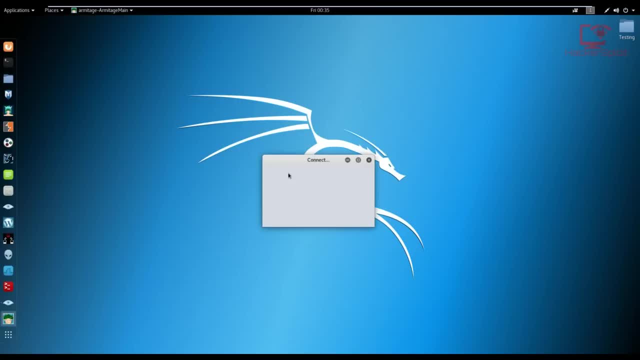 or whatever the host is, and this allows you to identify which host it is and the number of there we are. It's going to prompt you to connect to the localhost and the port. just hit connect, do not change anything here. And once you hit connect, it's going to prompt you to start the Metasploit. 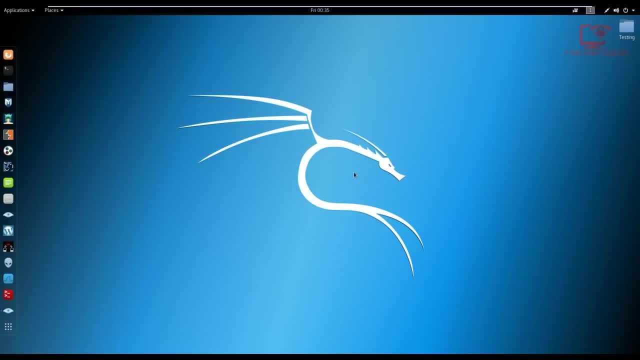 RPC server. So just hit Yes, we want to do that, And now it's going to start connecting to the remote host and just give it a few seconds and we should be good with Armitage, Alright. so the great thing about Armitage, as I said, is that the exploitation is is then the exploitation process. 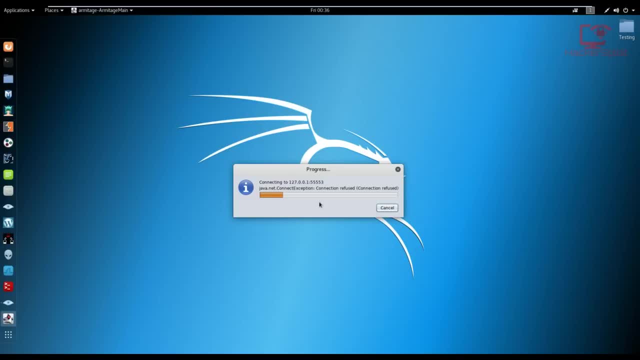 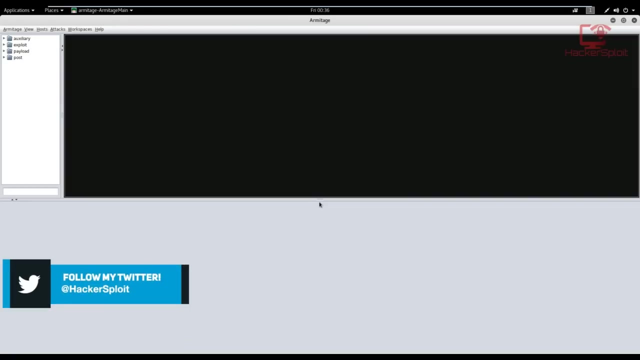 is automated as well, as you know the, the setting of hosts, the setting of targets. but you know vulnerability analysis. you know it also offers, you know, functionality like that And we'll be looking at this when we'll be exploiting our, our Metasploitable 2 virtual machine. Alright, 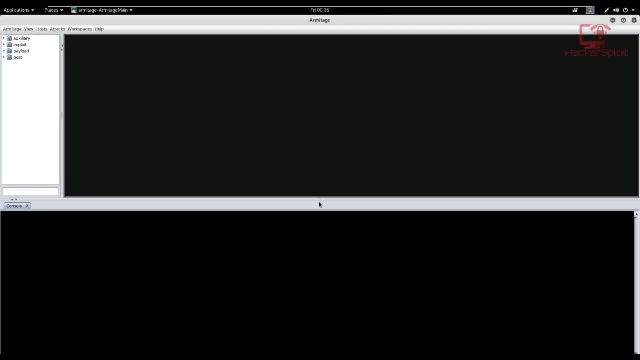 so, as you can see, Armitage is loaded up and you might be a bit confused with the interface, because you heard me tell you that it was a graphical user interface And now you're seeing a Metasploit console. Yeah well, don't worry about that. the Metasploit console there is is there to aid you in what's. 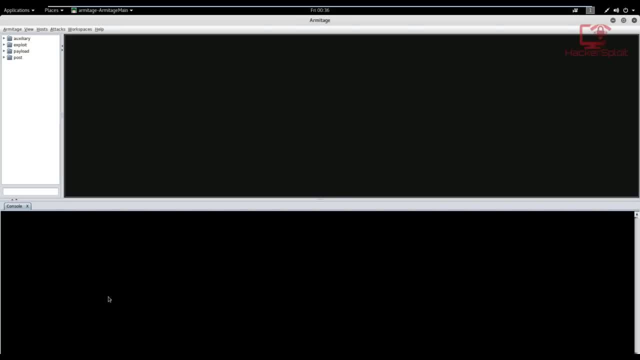 what exactly is going on? Alright, so the first thing I'm going to start with is I'm going to start with this little toolbar up here. this little toolbar is very, very simply put So in Armitage you can, you can set, change settings like add a new connection. you can check the. 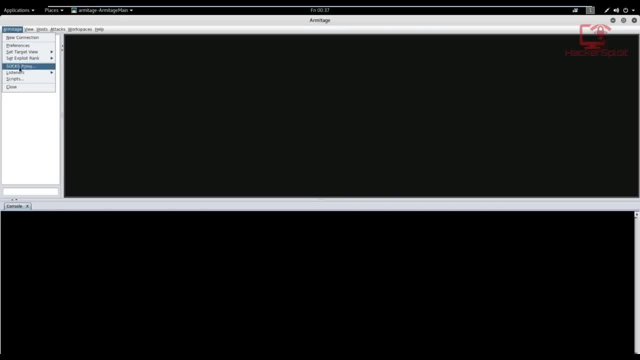 preferences. you can set the target view sets. you can set the target view set, the exploit rank. you can use a SOX proxy, like we did in the proxy chains video. we can look at the listeners so you can connect to or wait for. you can set the lhost, the listening host. 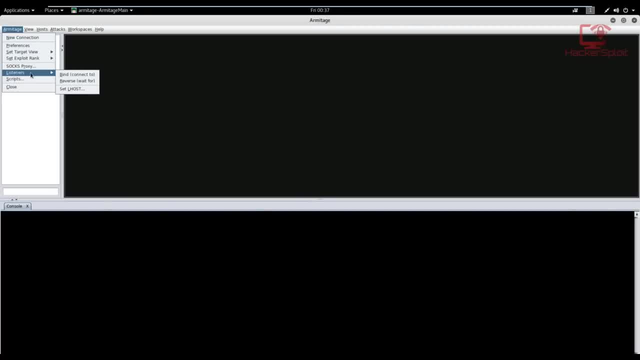 if you want another listening host, for example, if you're running Kali Linux on another computer and you want that computer to also listen to you, you also have your scripts and you can close Armitage In terms of the view. this is just to edit the view When we look. 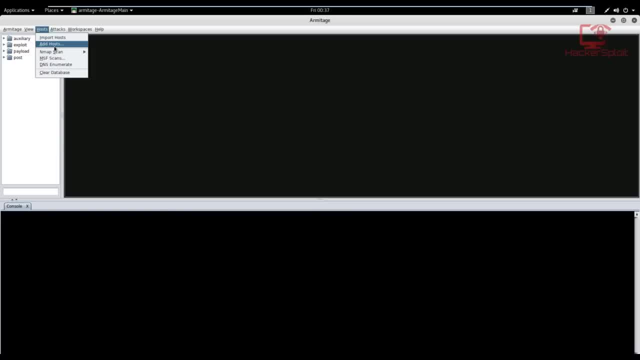 at hosts. you can add your host. So, for example, we'll add our Metasploitable 2 virtual machine here, But we'll do that in a few seconds. We have nmap scans, which is awesome. you can automate nmap scans directly from Armitage. you then have your Metasploit scans, which 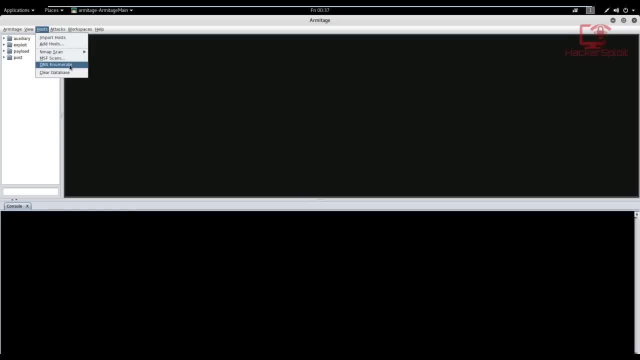 is awesome. We then have your DNS enumeration, which we looked at in the information gathering section. I hope you remember. so everything can come together really, really beautifully And that's why I really enjoy using Armitage, And you I'm sure you'll see why, right you? 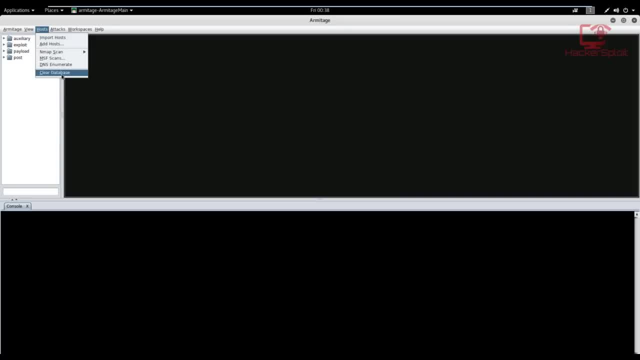 can then clear your database, which is essentially just clearing, you know, any of the leftover scans that you had performed or exploits that you had performed. you then have your attacks, where you can find attacks On your target or your host, and you have Hail Mary, which is something we'll look at. 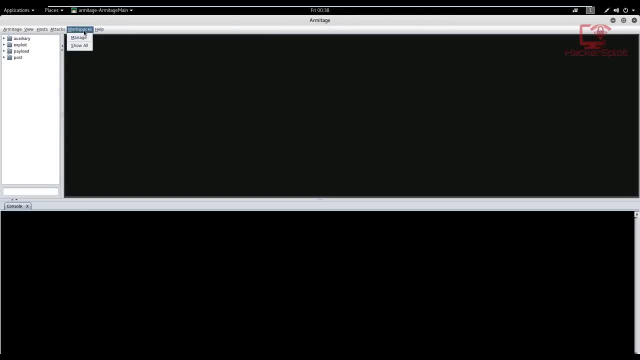 in a few minutes. Okay, looking at the workspaces, you can manage and show all your, all the workspaces you currently have In terms of help. you have your homepage, your tutorial scripts and your bot section. All right, fantastic. Now let's get into the interface. So the interface. 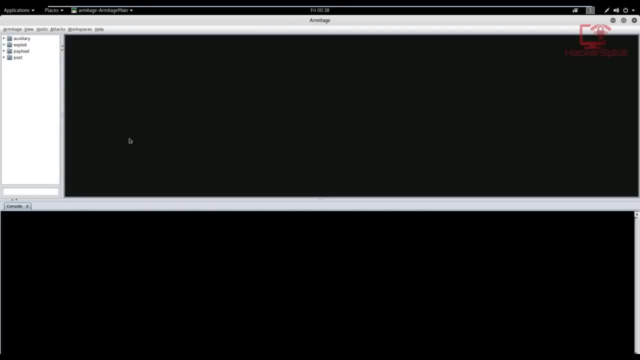 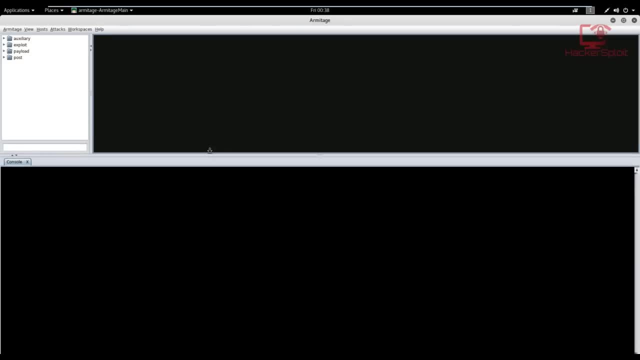 is sorted into three sections. All right, you have your, your first section, your second section and your third section. All right, so you can enlarge them and resize them, And resize them depending on how you want them to be displayed. So I usually like having 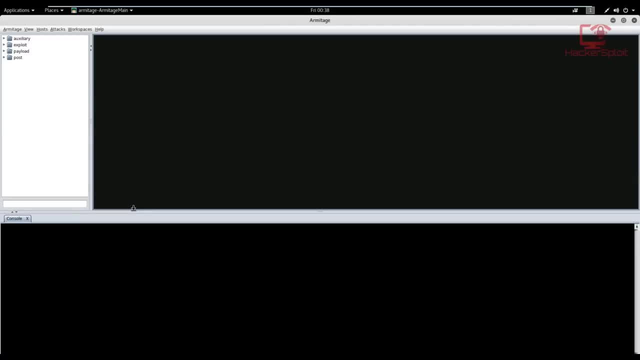 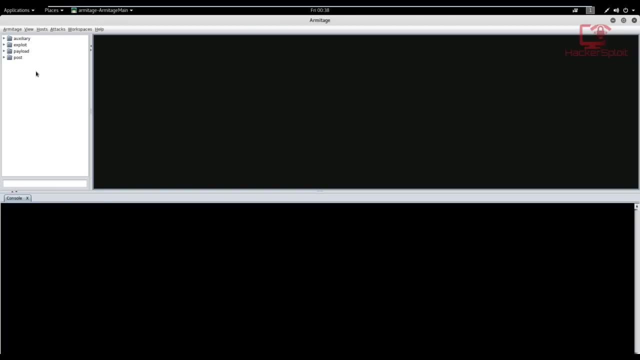 mine like this because I like having to see what the console displays. But as much as I like that, we'll be looking at the first section here. In the first section, essentially what is being displayed here is your pre configured modules. All right, so you can also search. 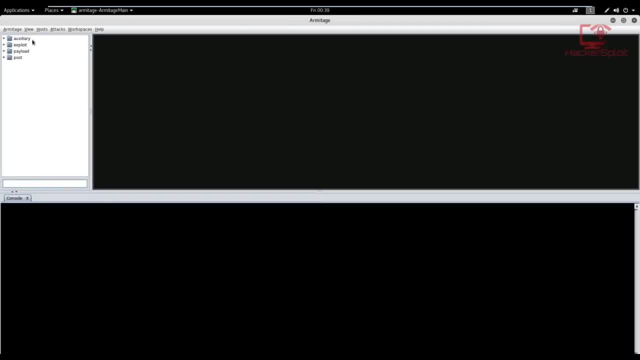 for modules here, you know, in this little search bar. So this is where you have all the modules sorted in terms of auxiliary exploits, payloads and the post which will look at in a few seconds. When it comes to the second, the second interface here, the 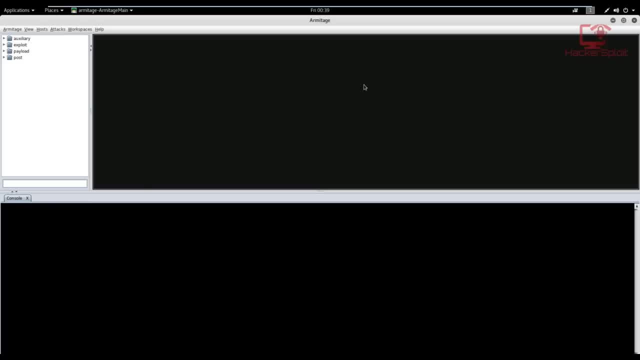 second interface is used to display your active targets that we were able to exploit against Alright. so this is where all your active targets will be displayed in forms of computers. We'll look at that again when we'll get started with Metasploitable 2.. As for the console, 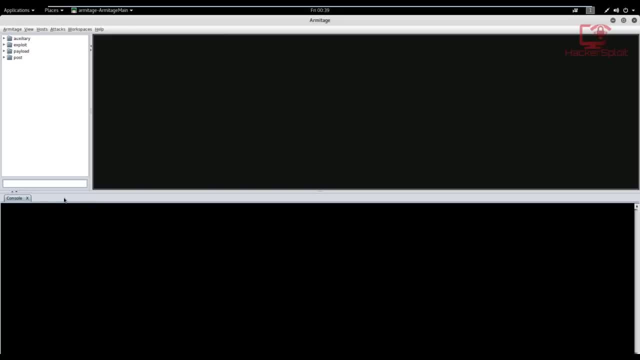 this is your Metasploit console, and it will be well. your activity will be sorted in forms of tabs. Here again, you'll be looking at exactly how that happens, And essentially it allows you to to run your Meta Predator or your console sessions simultaneously- something 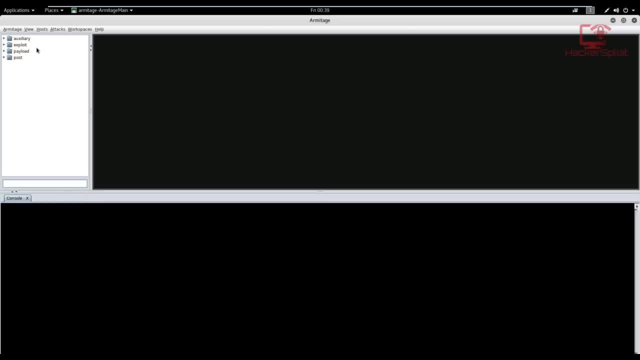 really, really awesome And I'm sure you'll appreciate it. Okay, let's get started with your module section. So, as I said, your modules essentially contain your- all your modules in this section, and they're sorted in terms of auxiliary exploits, payloads and post. 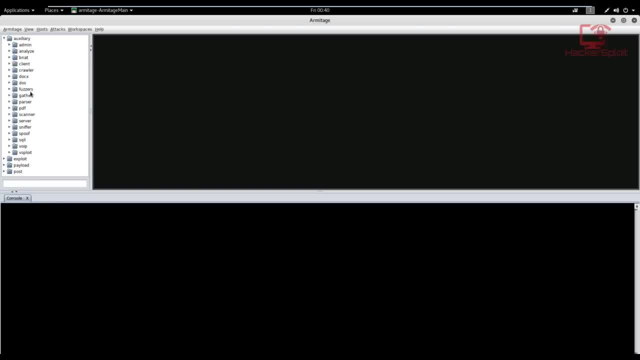 and you can go through them. So, for example, we have auxiliary. you can look at the auxiliary scanners. you have your scanners, fuzzers, you know your sniffers, spoofers, etc. And etc, etc. You have your exploits, where your exploits are sorted in terms of their, their, 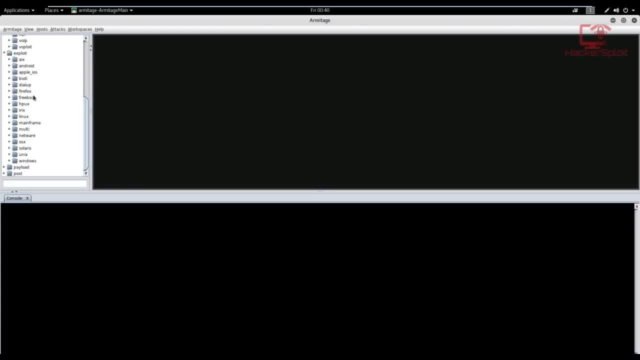 platform that they're running, on an operating system that they're running on. For example, you have Android, Apple, iOS, Firefox, FreeBSD, Linux, Unix, Mac OS X and Windows. you then have your play payloads that are also sorted in terms of their platforms and the operating. 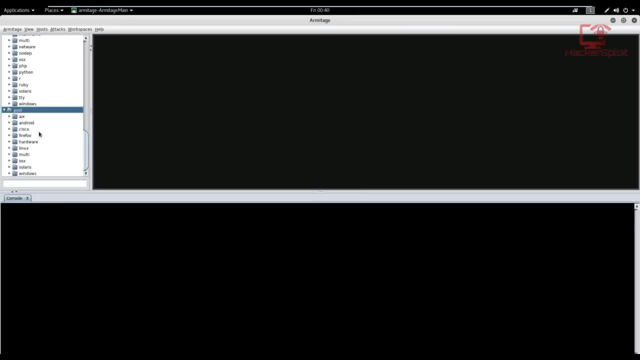 systems that they're currently, that they are to be exploited on. All right, you then have your post, which is also similarly sorted in terms of their, their, their platforms and the operating systems that they are designed to be exploited on. So let me just close every. 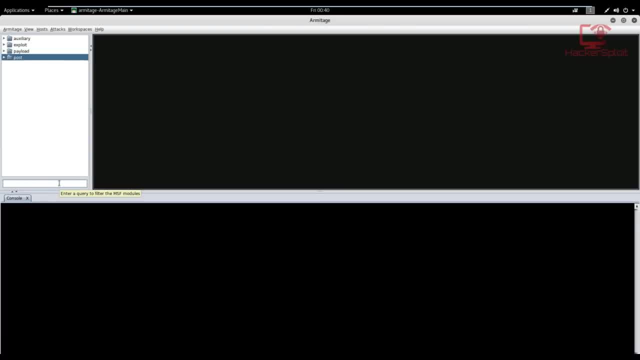 one of this And, as I said, you can also use the search, the search bar here to search for the Metasploit modules. All right, now let's get started with some actual exploitation, And we're going to start off with Metasploitable too. All right, so what we're going to do. 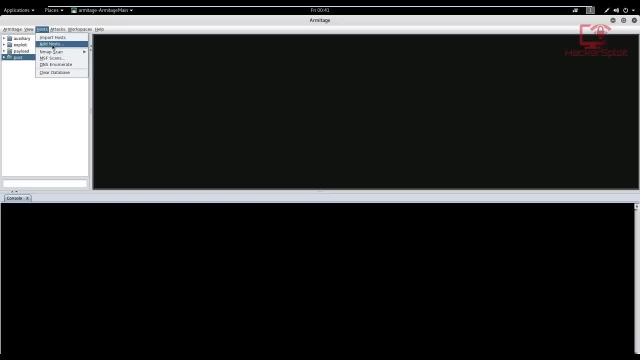 is we're going to go into hosts All right now in hosts you can import hosts or you can add hosts. we're not going to add a host yet, And the reason is I'm going to use an NmapScan to also perform some information gathering while adding the host. So what I'm? 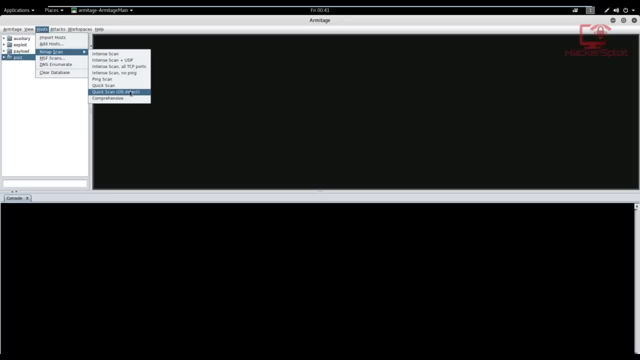 going to do is I'm just going to go into NmapScan And I want to perform a quick scan at that will detect the operating system that is running on our target, or our host, for that matter. So I'm going to click on that And now it's going to prompt you to enter your host IP. 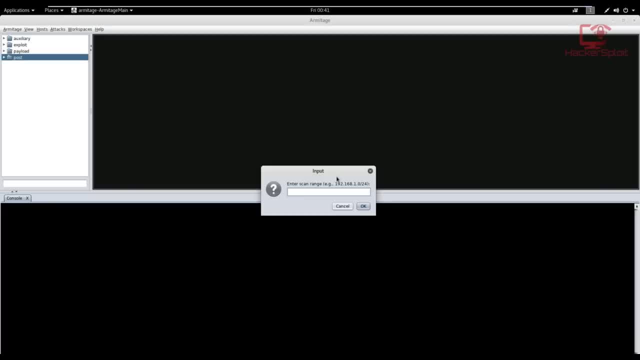 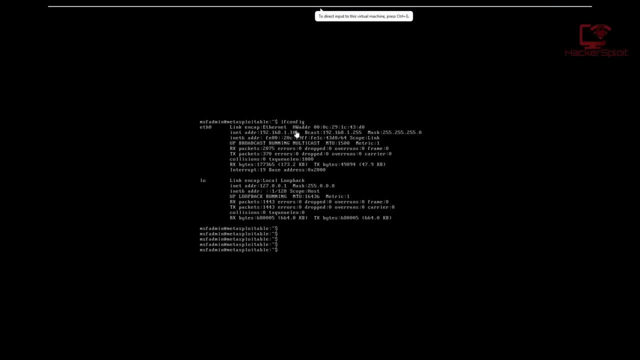 address, or your target IP address, or the range, if you want to scan your entire network. In this case, what I'm going to do is I'm just going to get the IP address for Metasploitable too, And I'm going to enter my IP address here, which is 32.168.1.106.. So we're just going. 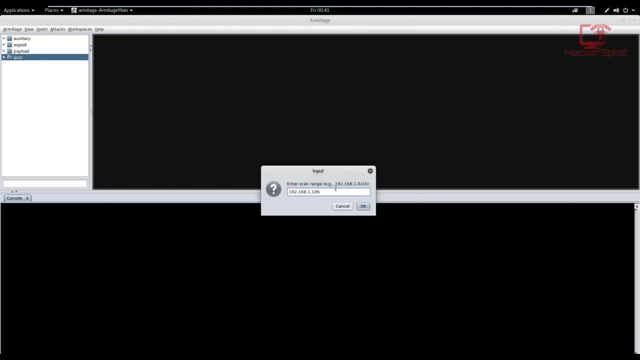 to enter that right now. Excellent. So once we hit enter, it's going to perform the NmapScan And it's going to detect what operating system is running Now. as I said here, the activities are going to be sorted out in terms of tabs. So your console is still open and your NmapScan is still. 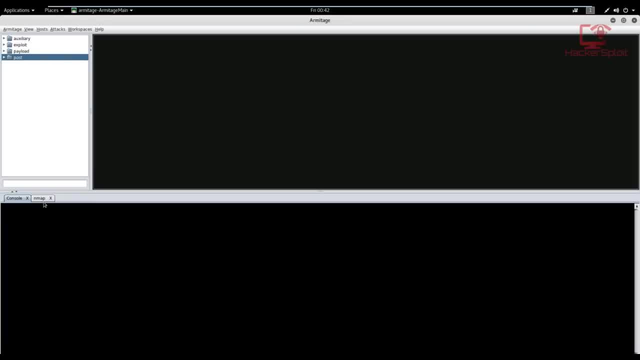 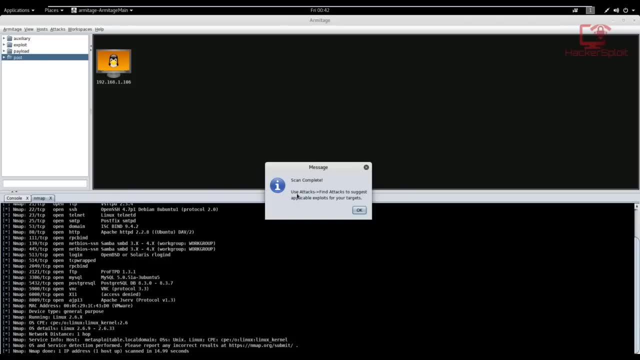 ongoing here, or it's just started, And you can run them both simultaneously, which is fantastic, right? So the scan is done, And it should give you a prompt here saying the scan is complete. Voila. So it's going to give you an option here saying: use attacks, find attacks to suggest applicable exploits. 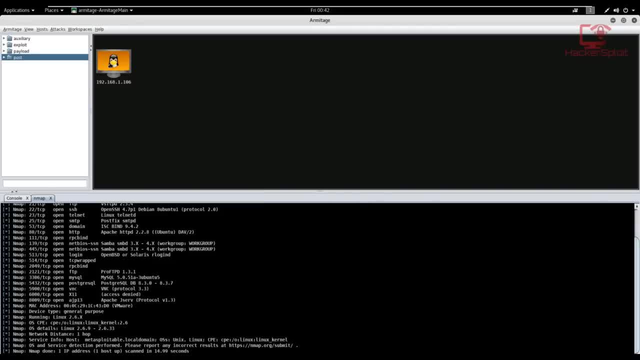 for your targets Interesting. So I'm going to hit OK. And what do we have here? Well, we have a little cute little penguin here to represent Linux. So we know it is running Linux 2.6. And the kernel is not specified more than that. Alright, so you know you. 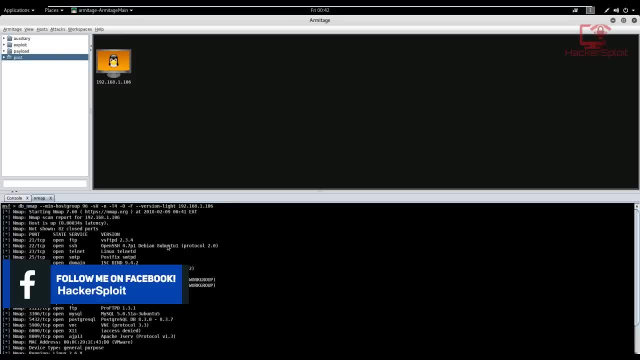 can see the services and the ports, that are, the ports and the services running on these ports, with the NmapScan. So we were able to get information about our target And now we understand what operating system is running on it And we can see the services running. 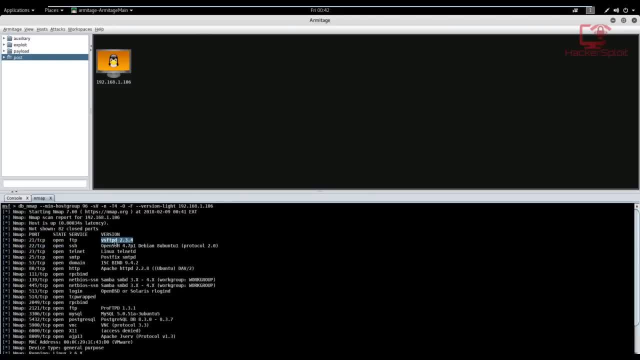 on the ports. In the previous video we looked at exploiting the FTP protocol or the FTP port with the FTP, the F, the VS, FTP D backdoor. And how did we do that? Alright, the first thing we did is we know that it exists as an exploit, So we're going to go into our 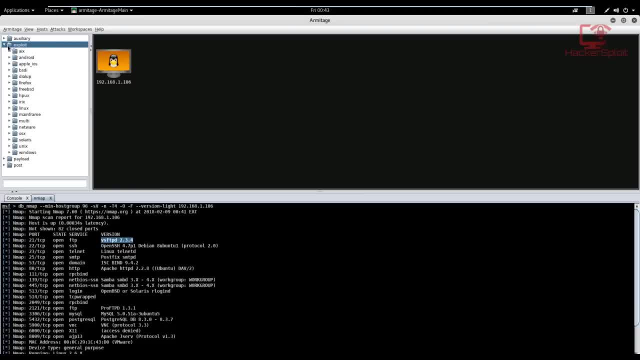 modules and I'm going to show you exactly how to find it. So we're going to go into exploits And we are going to go into Unix because it is a Unix. It is a Unix exploit, And once I click into Unix, we're going to then select the protocol which, in this case, 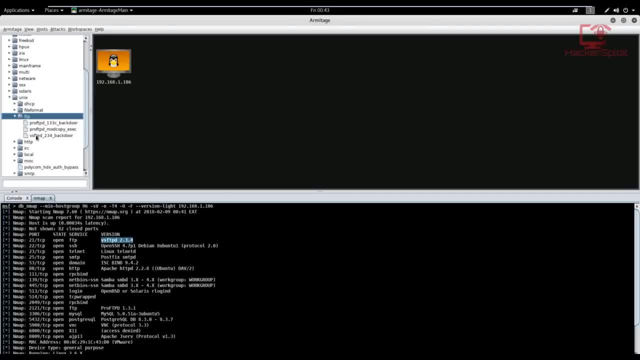 is the FTP protocol right here And we're going to expand that And voila, you have your SVS FTP D 2.3.4 backdoor. So, if you want to, if you want to execute this, what we do is we just double click it. Alright, and once we double click, it is going to give. 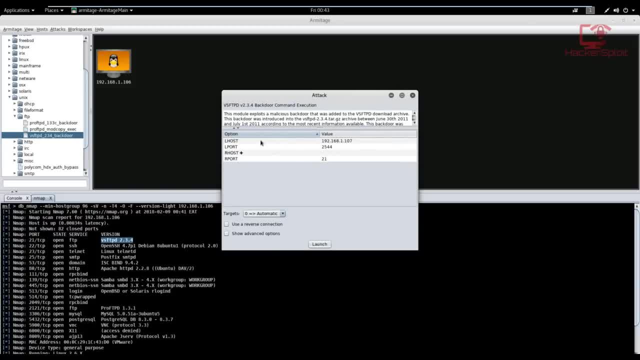 you the options that we used in the previous or we used in the Metasploit console, And once we double click it is going to give you the options like setting your R host and the R port. So, by default, the L host, which is your listening host, which is your IP address. 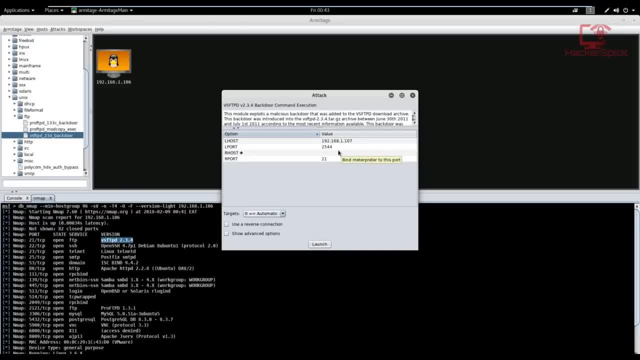 is default, is set by default, So 192.168.1.107.. And the default listening port is also set by default. all you have to do is just enter your R host, which in this case is 192.168.1.106.. 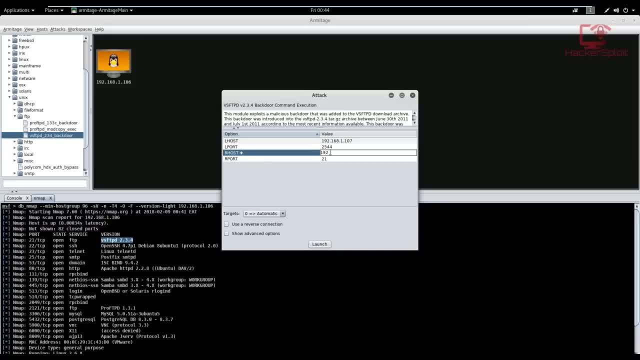 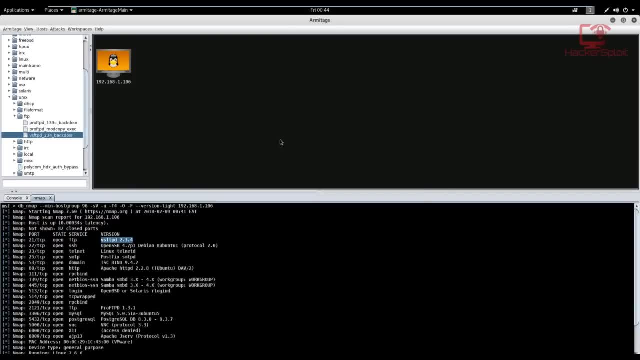 And we will exploit the backdoor using the FTP service. So 192.168.1.107.. So 192.168.1.107.. And once you're ready, you can just hit launch. All right, and it's going to launch the exploit. 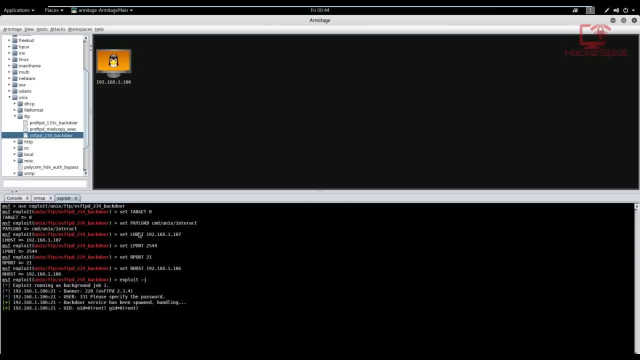 So just give it a few seconds And it's going to open up a new tab over here, the exploit tab. just give it a few seconds, here And there we are. phone shell command shall open and voila, we have backdoor access. Now you might have noticed something, also very, very. 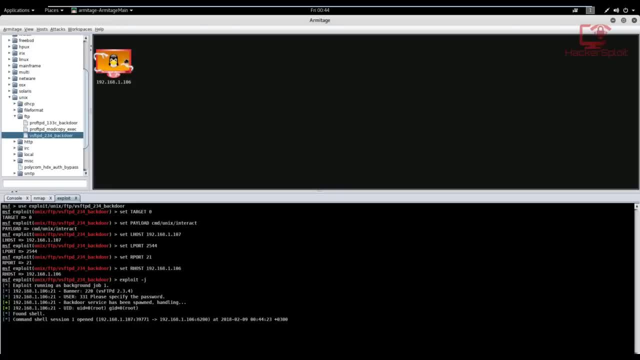 interesting. The Linux computer here is now surrounded by lightning or electricity And it is turned red. Now this means that we have successfully exploited this system in one way or another, Right? So this is fantastic. Everything is automated really, really well. 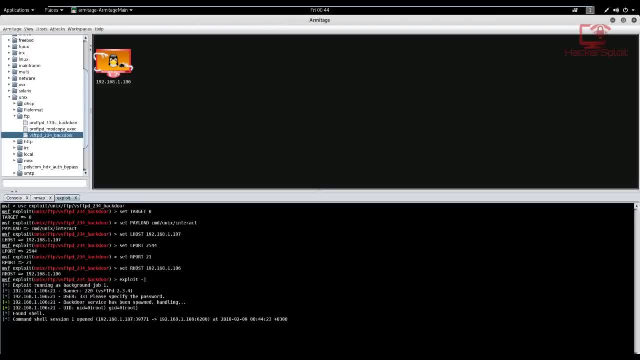 But now you might be asking: I want to exploit more things with meta exploitable. What can I do now? All right, tell me what I can do. So what we're going to do is we're going to close up this menu here, And what the awesome thing is, I said, is the automation. But before 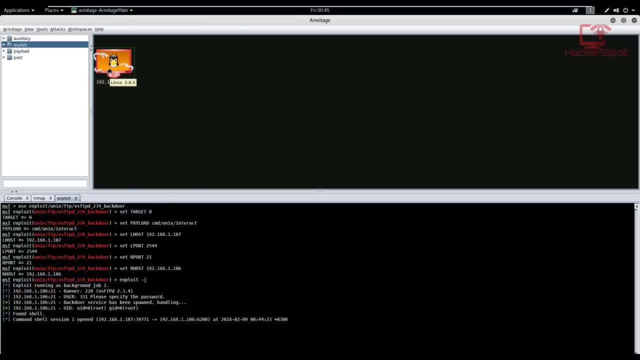 that I'm just gonna. well, if I look at the shell that's running, if I right click- sorry about that- if I right click on the target, we can see that it gives us options to log into the default network services. Now that is something just you. 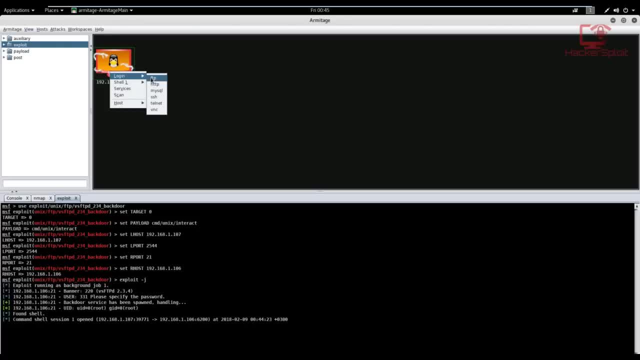 know very, very common. Once you've cracked them, if, if the cracking process is possible, you can then log into things like the FTP protocol, the HTTP, MySQL, SSH. you get the idea Now, the shell that we created, which is what we, the exploit that we used, allows, 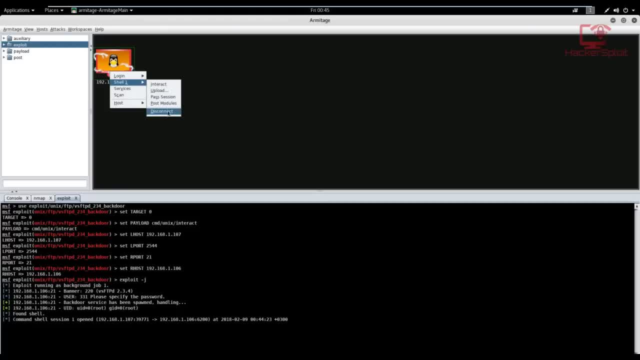 us to interact with it. we can then upload, we can pass the session, we can post modules and we can disconnect. So let's say we wanted to interact with it. So if we wanted to interact with it, it's going to open up a shell for us And again we can list the files on the server, the Metasploitable. 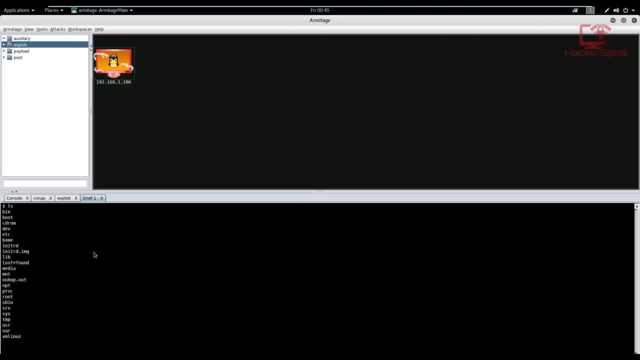 to, you know, virtual machine, which is considered to be a server because it does run some web applications, And voila, you have access to the root folder. So let's see, if we change directory to the home directory And we list the files in there, we have the MSF admin. 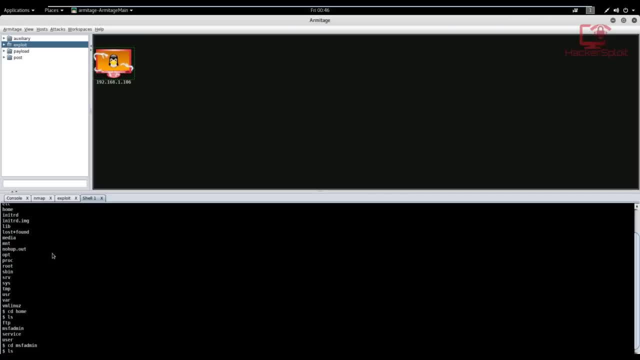 So let's also change directory into that MSF admin And we can list the files in there. we have the vulnerable, so CD vulnerable, whoops, CD vulnerable, CD vulnerable, And if you list there, we have the, we have the, the web services. 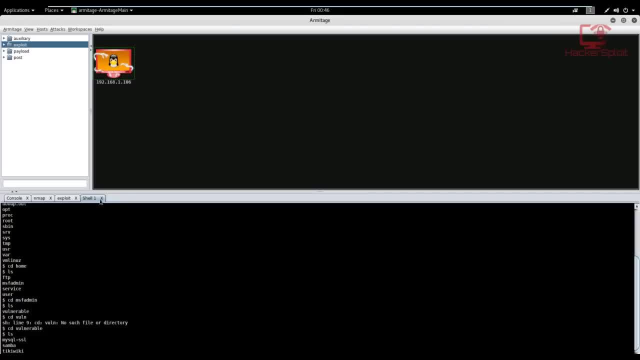 that are running. So you have MySQL, the Samba Tiki Wiki, etc. etc. So I'm just going to close the shell because we're done with that exploit. Let's look at how to exploit or how to find exploits automatically now. So I'm going to close that show And I'm just going 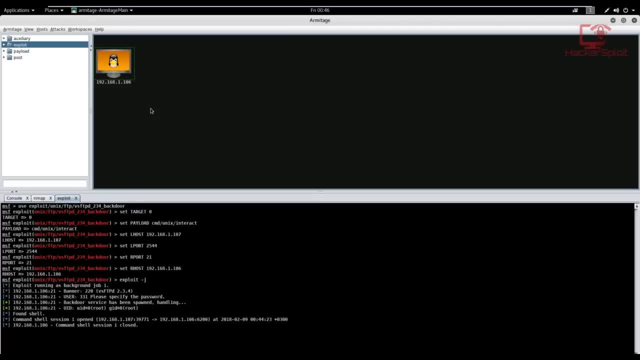 to right click, I'm going to select the L one and I'm going to disconnect because we're done with that exploit, Right? So once it's disconnected, it's going to remove the little icon that denoted the fact that the operating system or the computer was was exploited. Now you 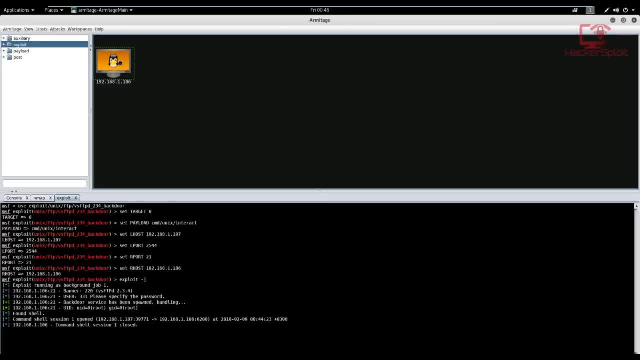 might be asking: Well, how do we, you know, how do we exploit it automatically? Or how do we find exploits automatically? Well, we go into attacks and we find attacks. Alright, so now it's going to find attacks that you can run on the operating system or all the 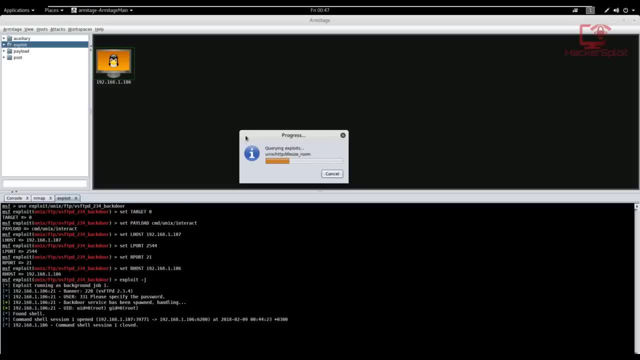 services that you can run on the computer, In this case our target host, which is the Metasploitable2 virtual machine. So, as you can see, it's going to, it's going to query the exploits and just give it a few seconds to go through all of them And once it's done, 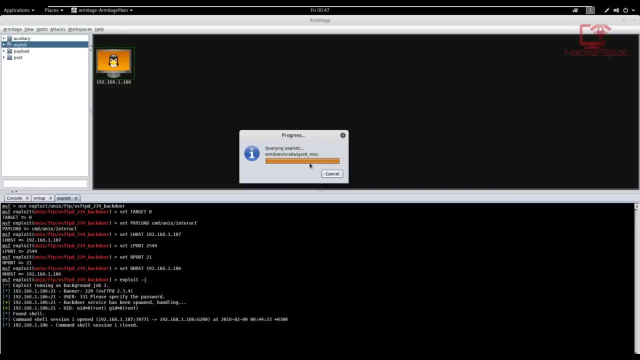 it's going to give you all a list of the compatible exploits that you can use, or exploits that can actually exploit a vulnerability on your, on your, on the operating system or the target that you've chosen. So if we right click now and we go into attack, you can see that is. 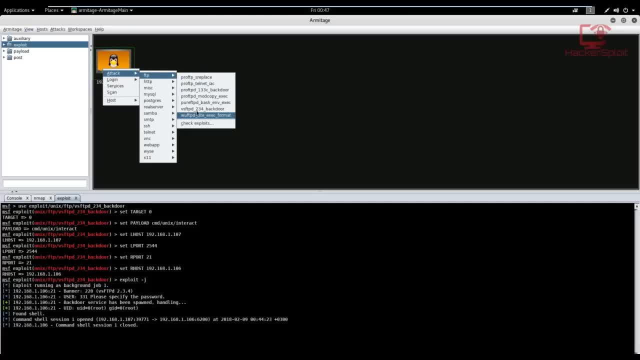 listed. So we can see that we have all the devices that we can crack. So if we go to FTP, we have the VSF tpd backdoor. here we have the pure FTP bash execution. here you can also check for exploits. again, you have your telnet, you have your HTTP vulnerabilities. So these 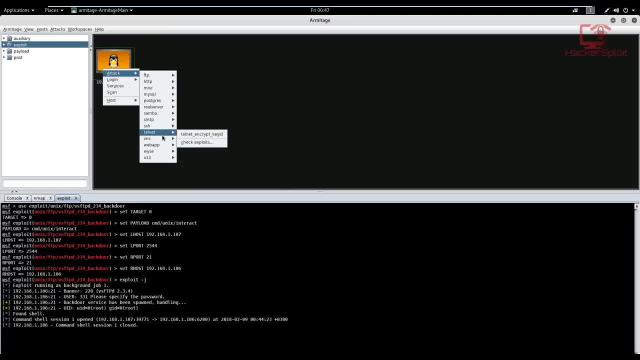 are all vulnerability or exploits that you can run on this virtual machine. So if we go to, for example, something like the web app, we can, or let's, let's get something more practical. sorry about that. If we go into the MySQL, so we are only have one exploit for the MySQL database. So if 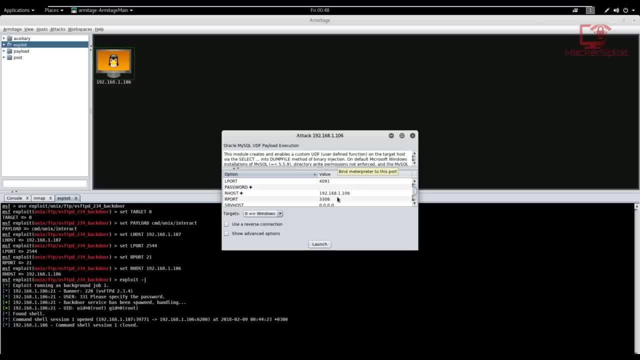 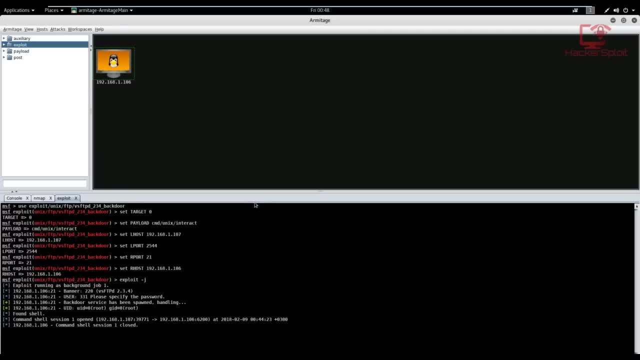 we click on this payload, if we load it and let's see if everything is set correctly. the R host, the arrows. there we are. that that's okay. So we're just going to launch, or let's see if we can get any information Right. so it's going to start the exploit in a new. 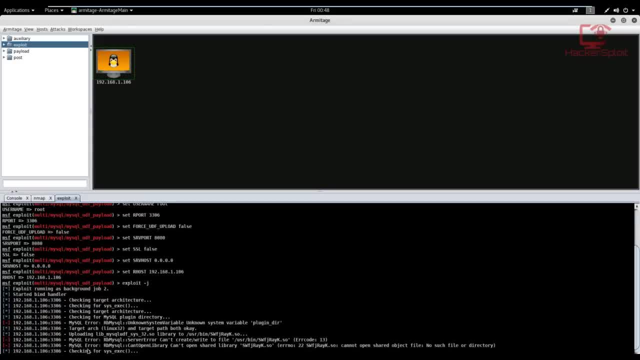 tab. I'm just going to close the old tab, So it's going to start the exploit process. Just give it a few seconds. here And there we are. It's going through a process. for some, the mysql function system execution is not available. so yeah, this exploit did. 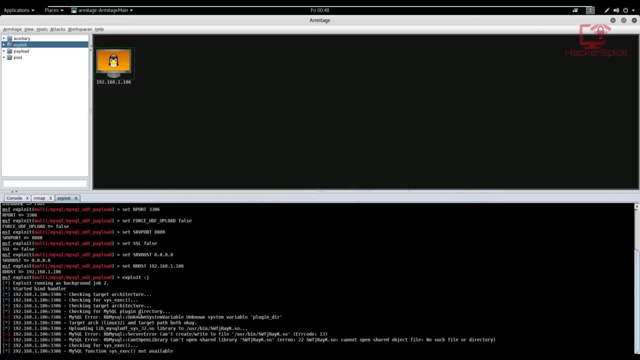 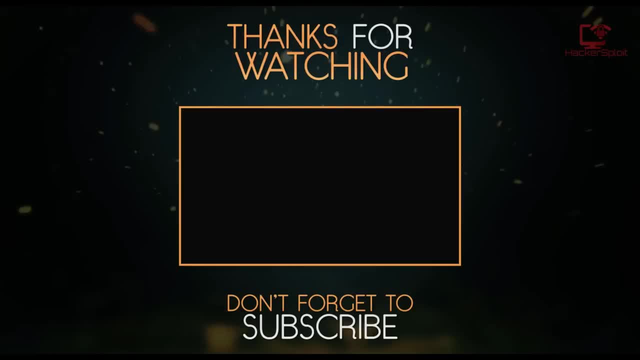 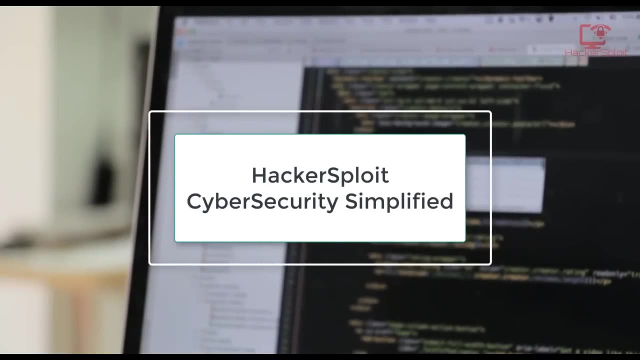 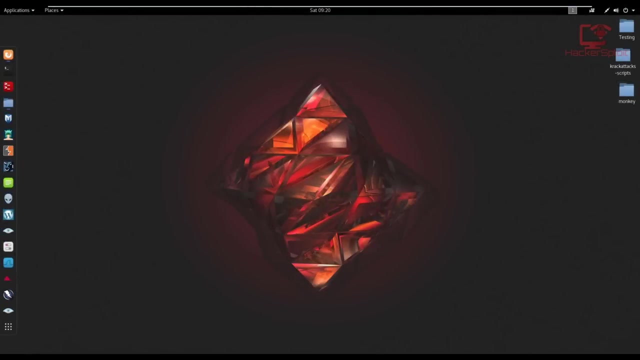 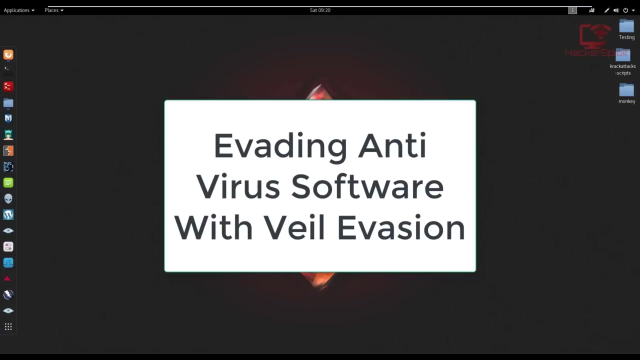 not work. now, this is what I was talking about. now it is going to work. hey guys, hack, exploit. here back again with another video, and in this video we're going to be looking at how to evade or bypass antivirus software's using veil evasion. now again, this is was a 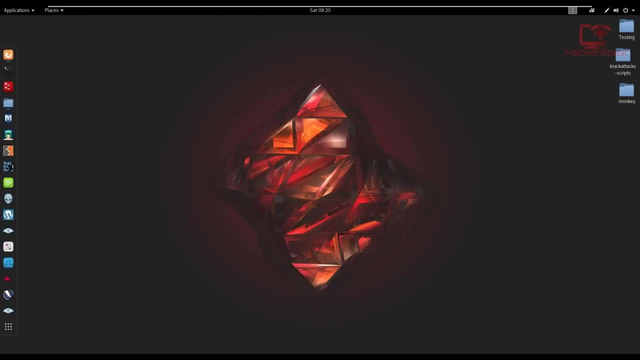 highly requested video and a lot of you guys had asked me to do it, you know, even stretching as far as last year, and finally it's come to to my attention right now because it is the current video on the list. that being said, let's get started. so why is this so important for a 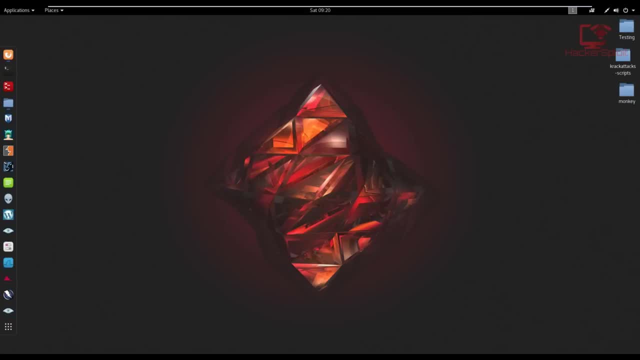 penetration tester. well, essentially what happens is you: you create an exploit or a payload and when you, it's time to send it to the target by whatever means- were they using social engineering? or you're able to send it. to send the payload to the target using an email or whatever means, you use the antivirus. 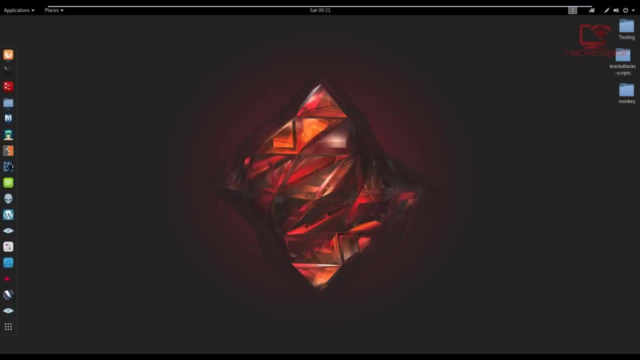 software ends up detecting the payload and your attack fails. so, again, it is very important to understand how antivirus software's work and how to evade them now, that being said, there isn't a way of going about it that will give you a hundred percent evasion. you might reach 98 or 99 percent if you're 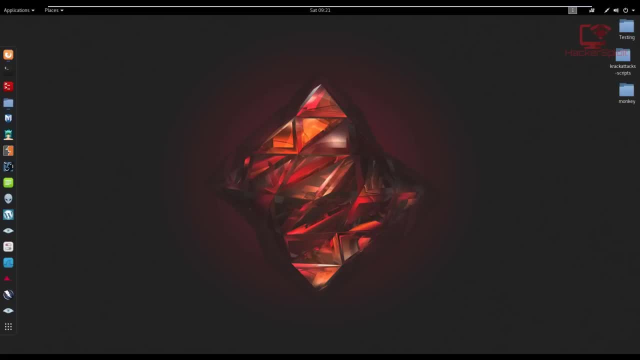 lucky, and we'll be talking about this because I am going to make a series on this, because it is quite a complicated topic and there are many ways of going about it. so what we're going to be looking at is how to to evade some of the most popular antivirus software's, most specifically, the windows. 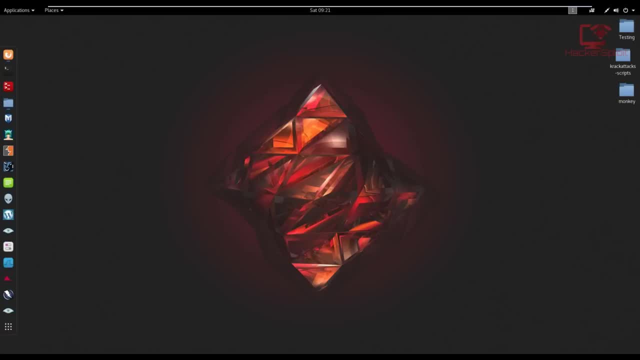 defender antivirus software, because that is the one that people usually have installed. now, I know antivirus software is like Avira, you know Kaspersky, etc. etc. but we're going to be focusing on on antivirus software's that are signature based, all right. so, essentially, what signature based? 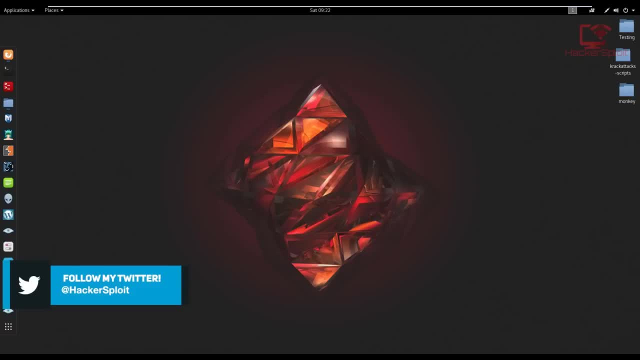 antivirus software's do is they look for strings, and obviously they have it. they have a database of these strings that they can pull from and therefore identify any of these strings in a program or an executable file, which in most case- in most cases- is how the payload is set up. 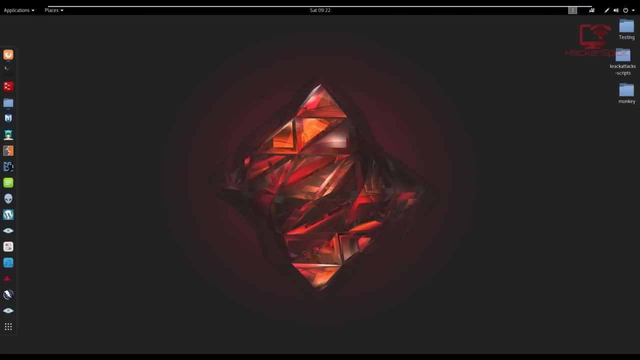 in. it could be in a Java file or a jar file, but in most cases when you're sending a payload, it's in an EXE file. now, this method can also work for a remote access tool, but we're not going to be focusing on that right now. and I said, as I've mentioned previously, you can use different. 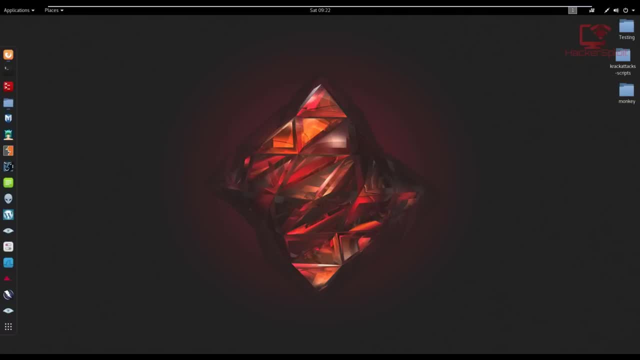 methods, which will be looking at after this, to further your, your evasion, your evasion protocol or your evasion, your evasion percentage. now, when I talk about this, I'm talking about file splitting and headings hexadecimal editing, because you can go into these executable files, split them up and then edit. 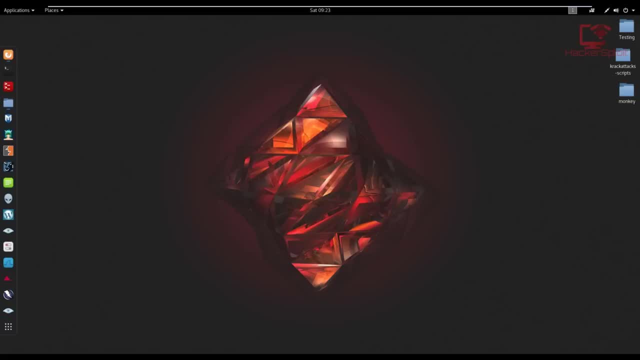 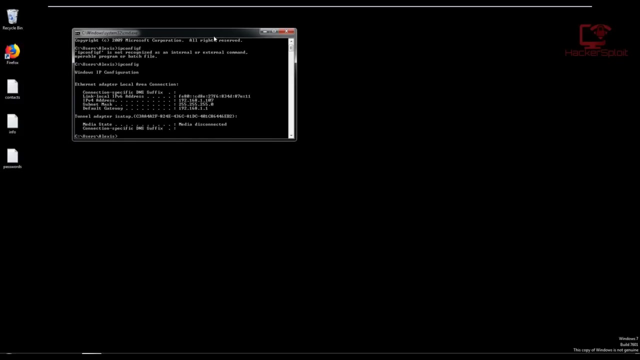 the, split them up and then edit the. edit them with a hexadecimal editor and get rid of those strings, therefore decreasing the chance of the antivirus software detecting the payload or the executable file that is obviously trying to harm that computer. that being said, I can, I am running. 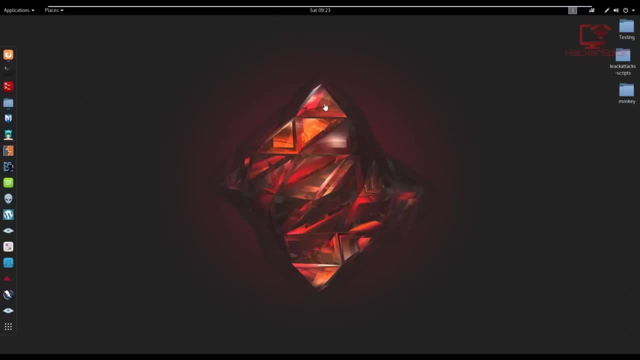 a Windows 7 virtual machine here. this is going to be our target virtual machine. obviously, my host operating system is Kali Linux. now to get veil evasion installed- it doesn't come pre-installed with Kali Linux. you need to just use the aptitude package manager, which can be done by. 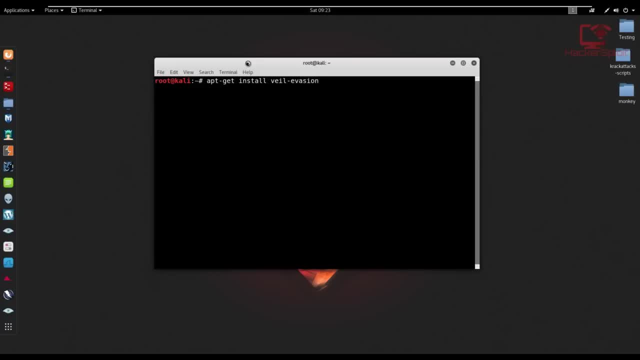 apt get install veil evasion or veil. I'm not quite sure whether it's veil or veil evasion, but any of those will will start downloading it for you. it isn't a big file at all. once it's done, you, essentially after it's done you really you, you want to start configuring it. 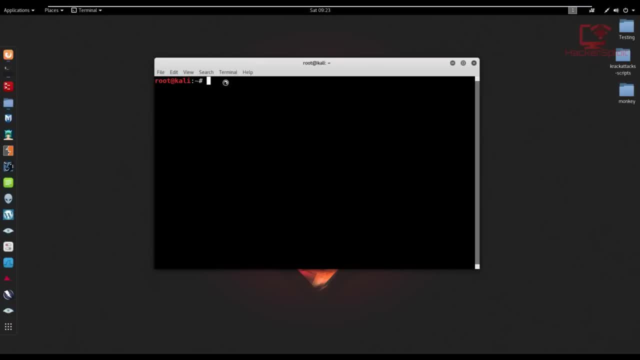 so you would go into the directory which is the user share, user share library and then the veil evasion folder. if you want me to make a separate video now to install it, I will do so because it is quite a lengthy install, because you also have to install dependencies like Python- Python to win. 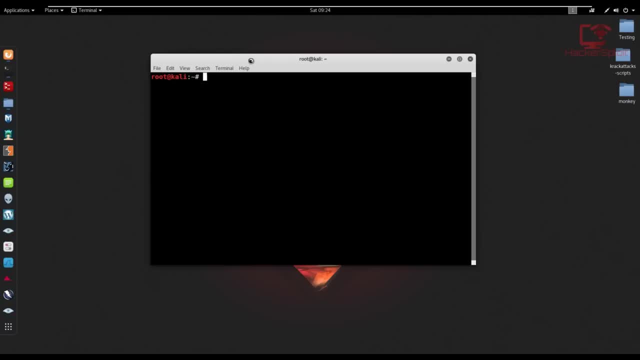 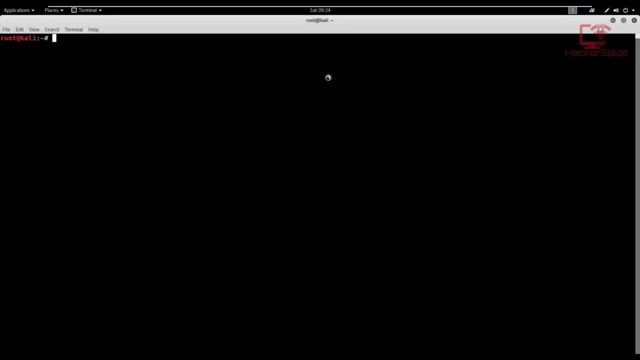 to Windows and Ruby. all right, these are all important prerequisites and and files that you will need to convert the Python or the Ruby payloads into an executable file. all right, so to get a veil evasion started. it's really very simple, by the way, after you've installed veil. 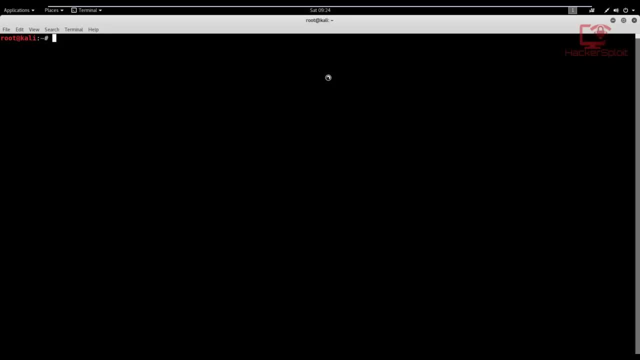 evasion. what you need to do is you need to restart your computer, because if you started directly after installing it, it does come with a few errors and you might get a little bit worried. but don't worry, just restart your computer and start veil evasion again. so you start it with veil as you. 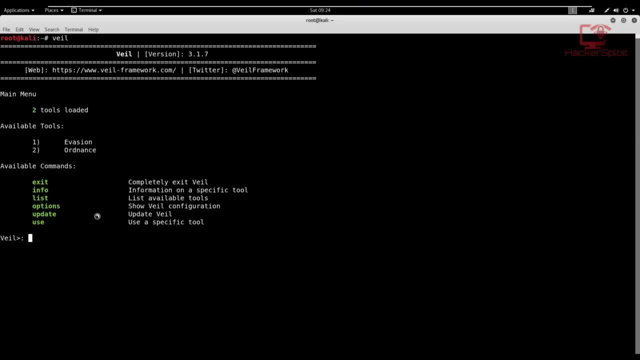 can see, and now it's going to tell you that you have two tools loaded. you have veil evasion and ordinance. we want to use veil evasion, so the the syntax is quite simple, so you have to go to the manual. it is use and we're going to select option one because we want to use veil evasion, so there. 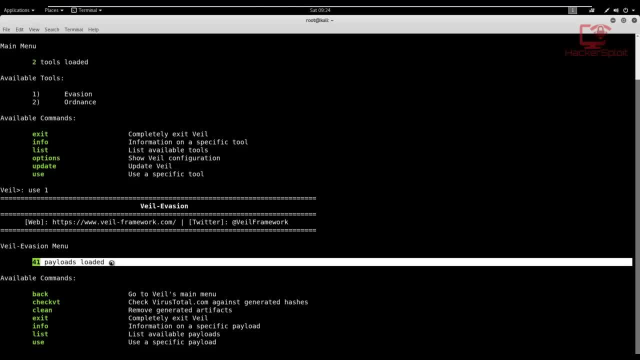 we are. we're going to say use one. and now it's going to give us the veil evasion menu and it's going to say we have 41 payloads loaded. so we want to list the payloads or the available payloads. so I'm going to say list, sorry list. and it's going to display all the payloads we have. now this is. 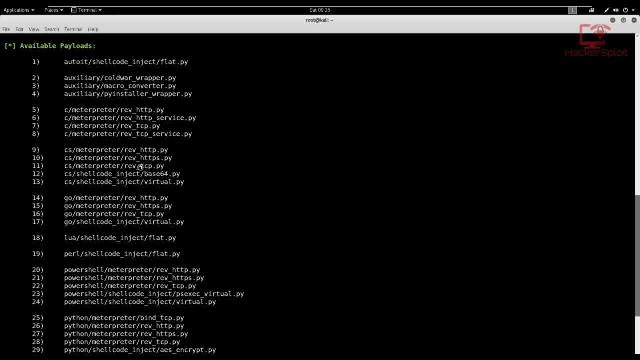 very interesting because these are all the payloads that you can use and will be converted. now. if you remember, in one of my earlier videos, when we were talking about Python programming and creating hacking tools, we discussed a little bit on low level, low lying level languages such as C++, Ruby, and python isn't one of them, for example. you can see that we have a 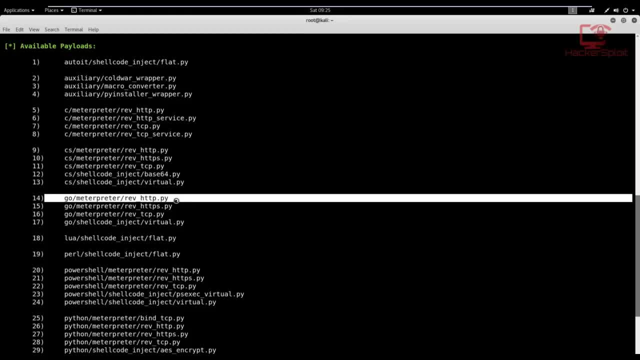 go. this is golang, Google's programming language, which is also very low line, which means it's very close to a machine language. now these programming languages are very hard to detect or very tricky for antivirus softwares to detect, because they are very low line level languages. now, 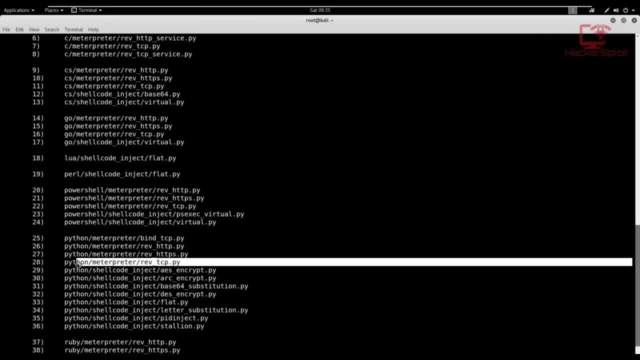 by default. a Python. a Python payload like this reverse TCP meterpreter, which is what we're going to be using right now and I'll show you, will evade Windows Defender, but it will not evade antivirus softwares like Avira, Kaspersky, because it's a Python is is a very, very high level language. 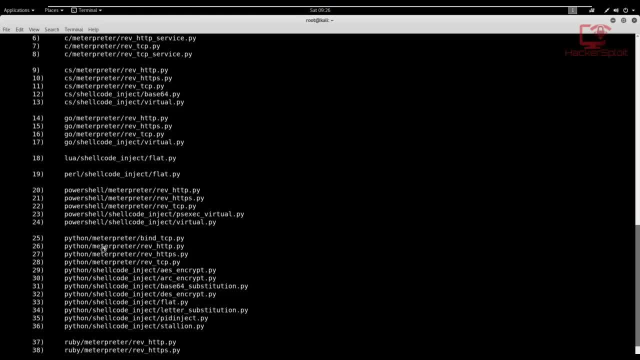 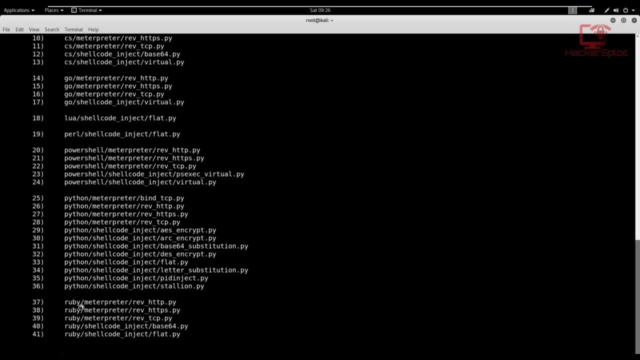 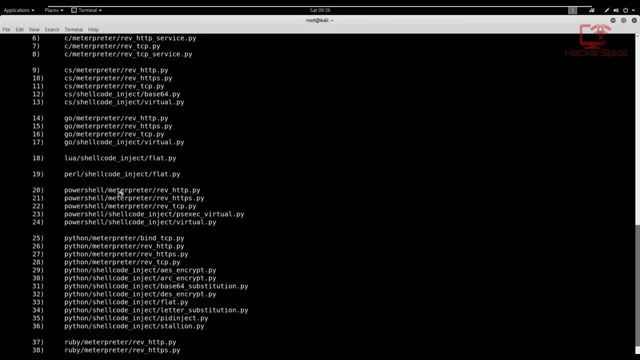 which means it's interacting with the software more, which means, again, it's very easy to to be triggered or to to be detected by the antivirus software. now we'll also talk about some of the other options we can use here, like the injection, the injection, the shellcode injection, which we'll 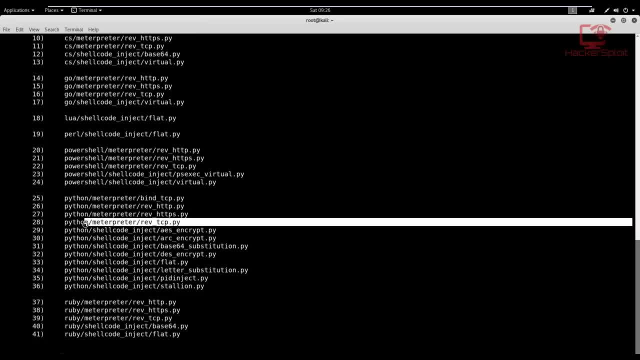 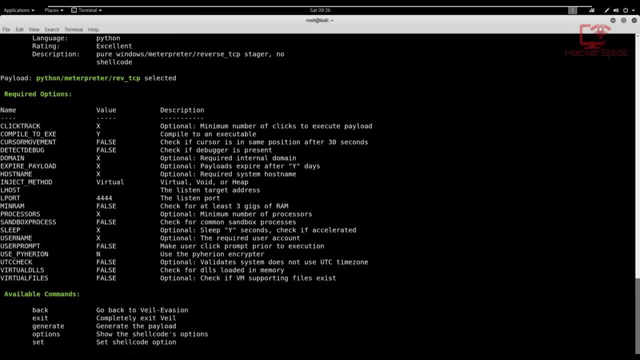 talk about in a few seconds, but for now let's start off with a reverse, a meterpreter session, reverse TCP, which is Python. yes, we're gonna select use 28, use option 28, all right, and now it's gonna ask you to enter your listening, your L host, and you want to remember your L port, or you can change. 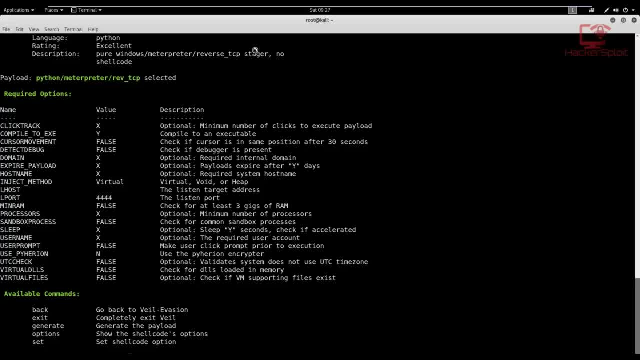 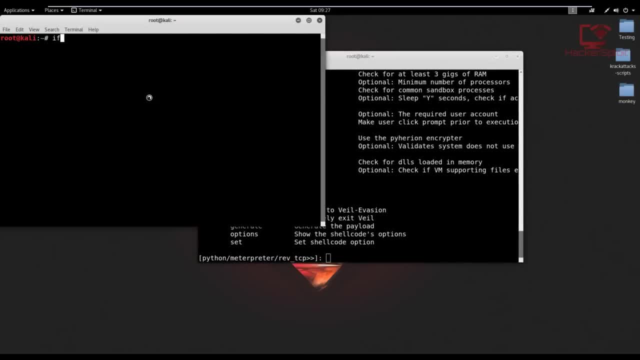 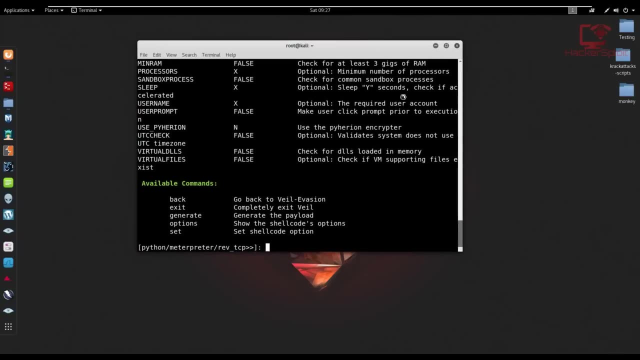 it to whatever you want, that's if you're using port forwarding. you want to go select our L host. so this is essentially your host operating system IP address, the. so you can just perform a quick I F config like: so I have config, and get it. mine is 192.168.1.105- excellent, so we're going to set our. 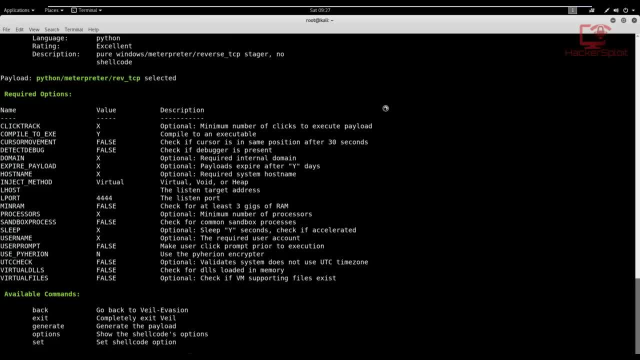 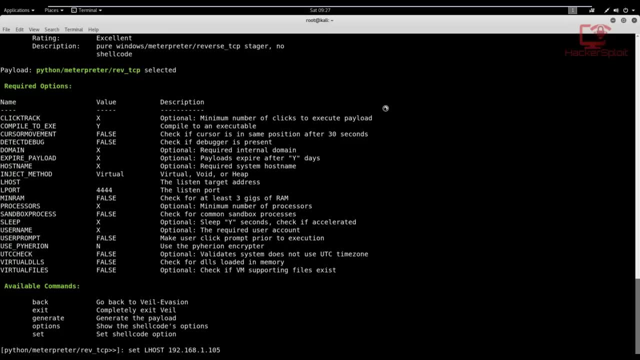 LOS. so the syntax is quite similar to that Metasploit. So L host and 192.168.1.105.. And I'm going to hit enter. All right, now we've set the L host. all we can do now is we can hit generate. All right, when we hit, generate is going to. 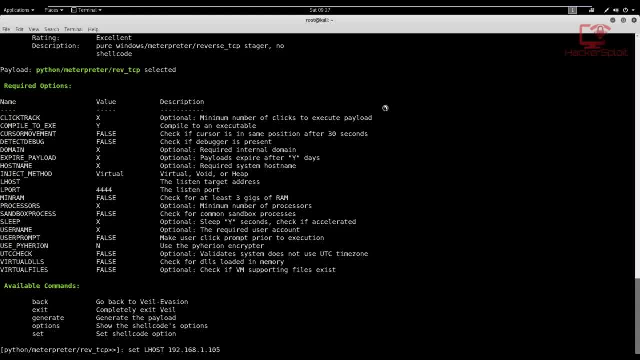 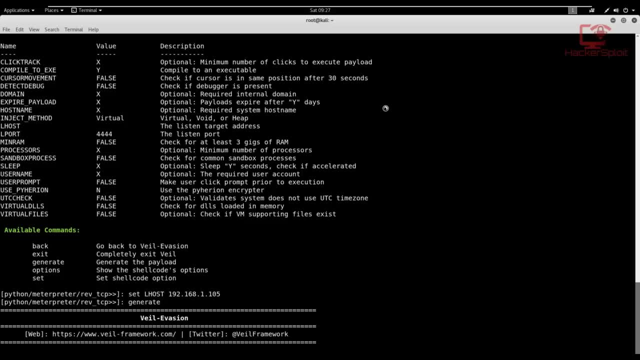 generate the payload for us. So I'm just going to generate. Now make sure you have all the dependencies installed in forms of Python, the Python to exe, or Python to win, as it's called, and I'm going to enter. it's going to ask you to select a base name for your output file, So this: 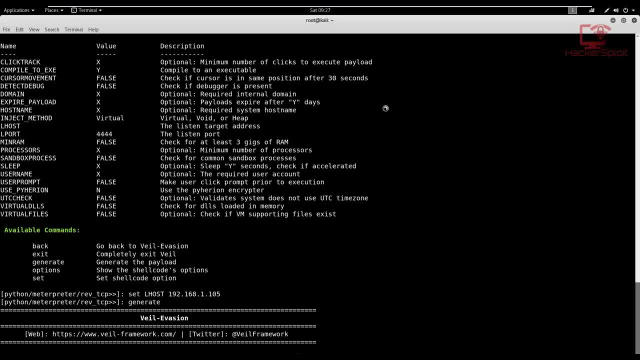 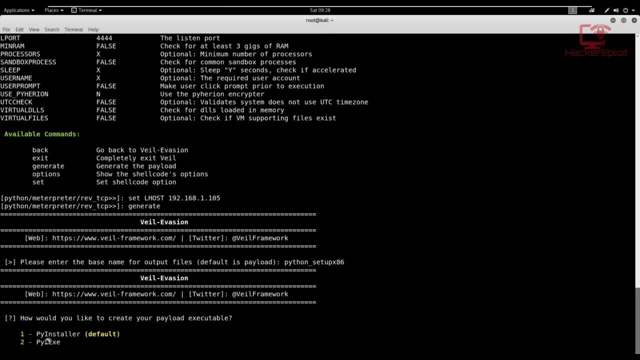 comes in place when you're talking about social engineering. So we can say, for example, something like Python, Python setup, Python setup. we can say x86, you know, just to make it believable, x86. And we're just going to hit enter And now we want to use PI installer. you can also use. 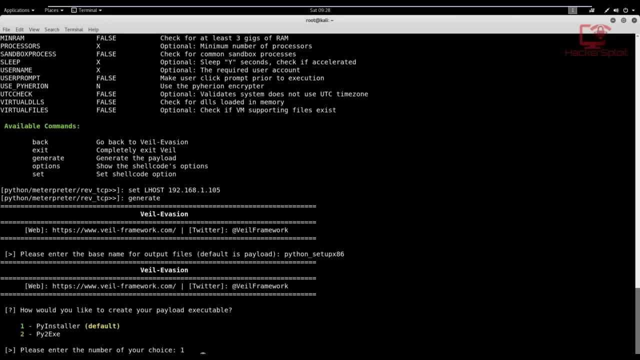 Python to exe if you want to, but I prefer PI installer. it's much more convenient. I'm going to hit one, All right, and now it's going to prompt you, or it's going to start generating it. So we're going to hit enter. And now we're going to hit enter, And now it's going to prompt. 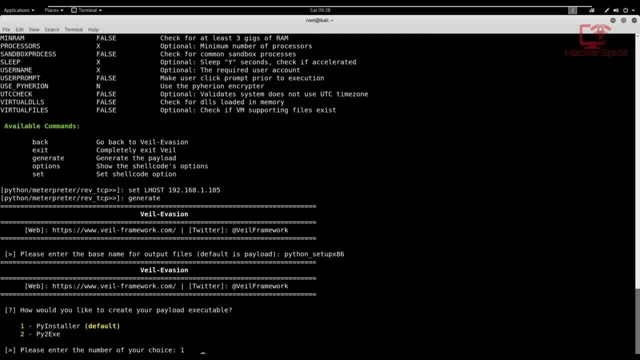 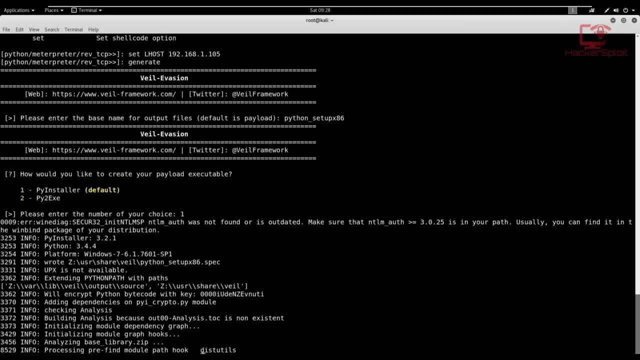 you, or it's going to start generating the exe file. So give it a few seconds here And once you've selected your choice, again, if you have installed all the dependencies, it should start it up. And there we are: it's going to start the the process of converting the Python pay payload. 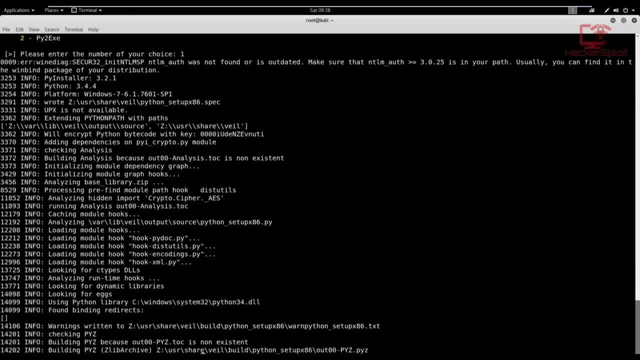 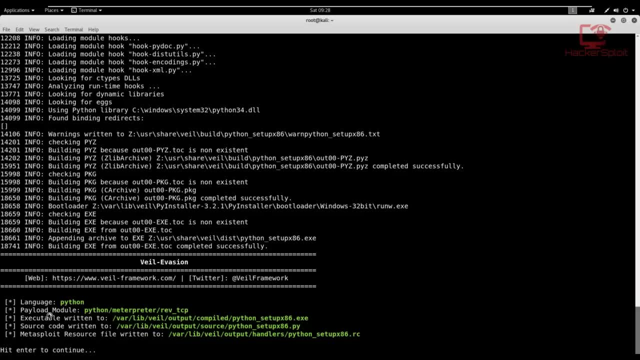 into a, into an executable file, Alright, so give it a few seconds to generate it And once it's done, it's going to display the. it's going to start, it's going to display the output folder. So, as you can see, here, it's given us the payload module, which is Python. 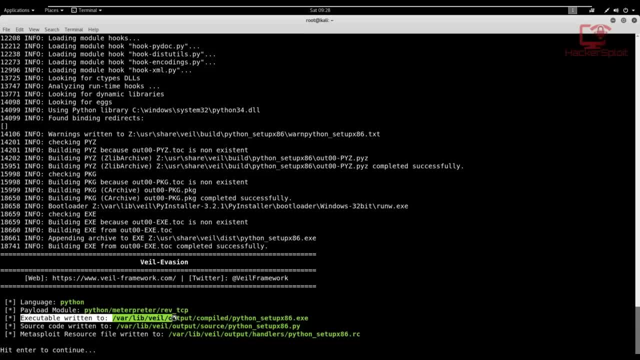 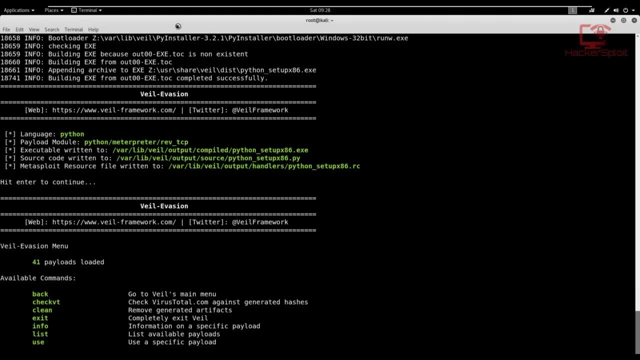 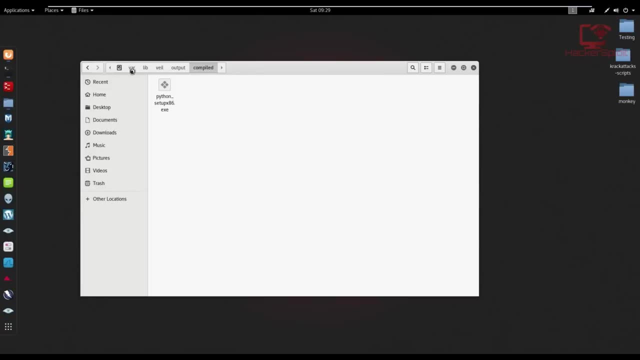 interpreter, reverse TCP, and the executable is written to var, the, the var library veil folder, and output compiled Python setup dot exe. So we're going to hit enter to continue. All right now. what we need to do now is we need to actually browse to the directory. Now I have I have the 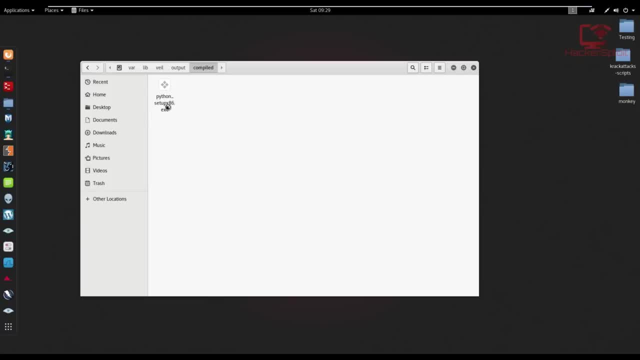 directory open, So it's var library, veil output compiled, and here it is, the Python setup at 32 bitexe. And now we need to copy it over to my Windows operating system here, And to do that I'm just going to plug in my flash drive. just give me a few seconds, guys, So I'm just going. 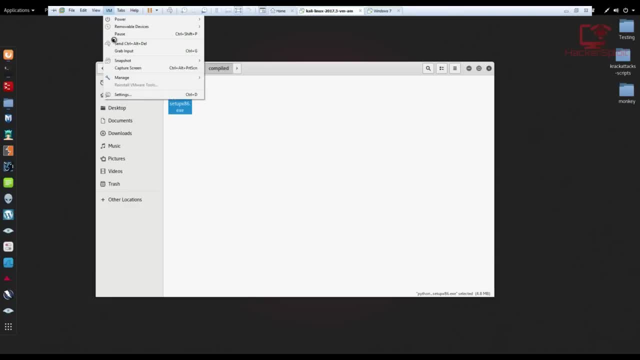 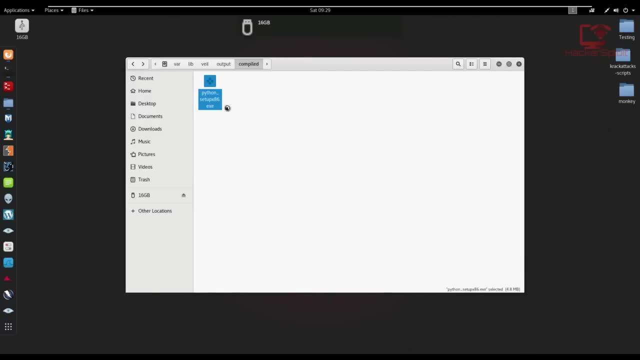 to plug it in here. There we are, And now what I need to do now is I need to go into my virtual machine and go into my removable devices and silicon. there we are disconnected. So, whoops, let me just go back a directory, let me copy this and I'm going to put it on my flash drive. So 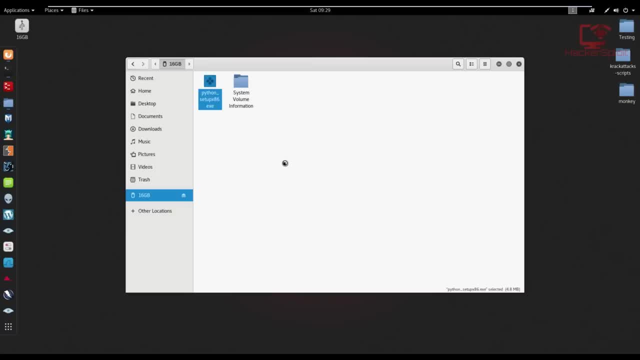 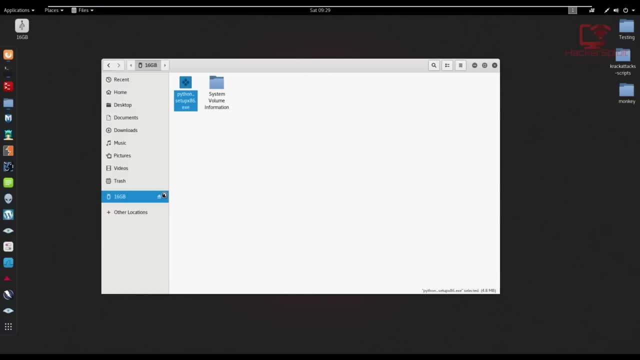 there we are. I'm just going to paste it in there. So this would be also another stack vector, where you give someone a flash drive and you tell them there's a Python setup there And in most cases it might work. But again, this is not a video focused on social. 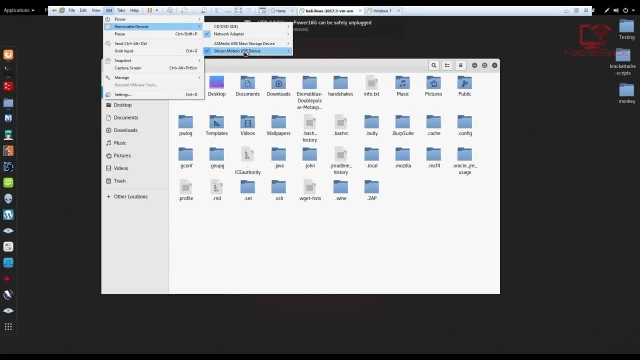 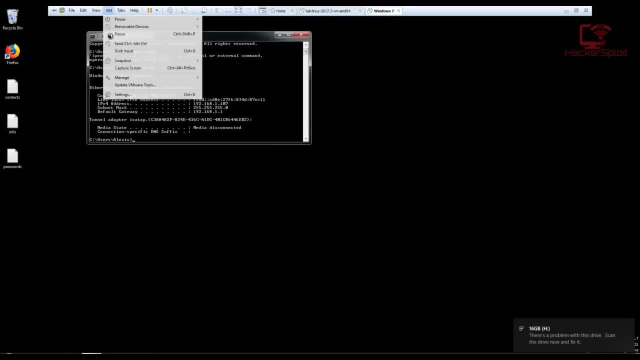 engineering. So I'm just going to eject it And we're going to go into VM And we just want to make sure it is ejected, So we're just going to hit disconnect And now we need to go into Windows And we need to go back into VM- removable devices- and we want to go to silicon and connect And 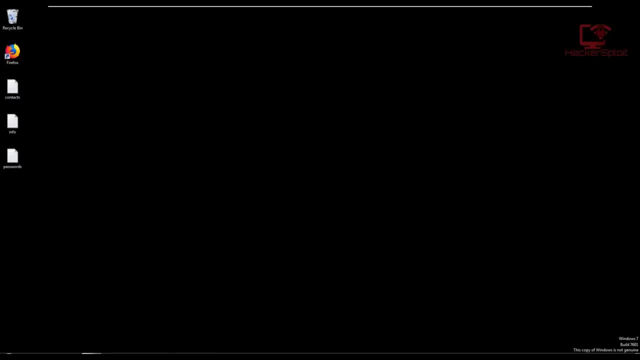 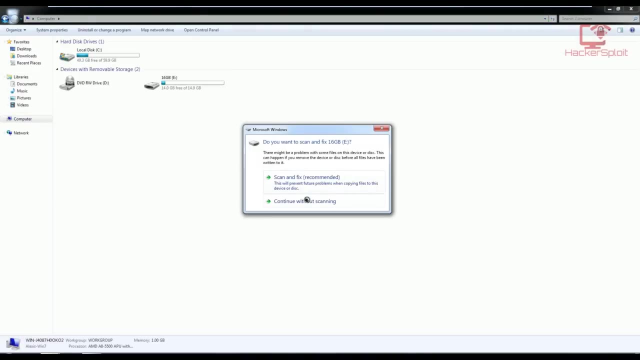 there we are. we're gonna hit OK. And for some reason my mouse always lags when I change my removal devices. There we are. So it should have connected the USB flash drive. Let me just check that. apologies for my virtual machine being so slow. So there we are, No. 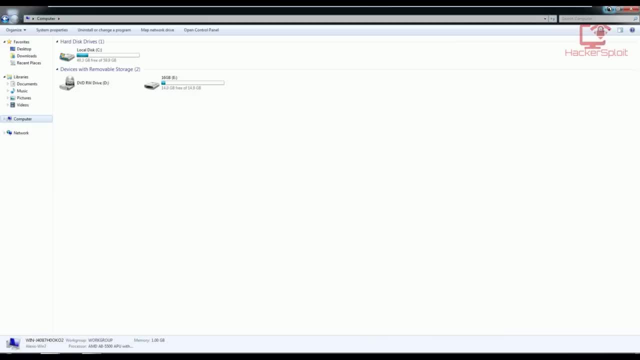 I do not want to continue scanning it. I'm going to open the folder and files And what I want to do now is: whoops, For some reason I minimize that and my virtual machine is really lagging out. man, That's. that's a pity. Sorry about this, guys. if it is lagging out, my sincere apology. So there we. 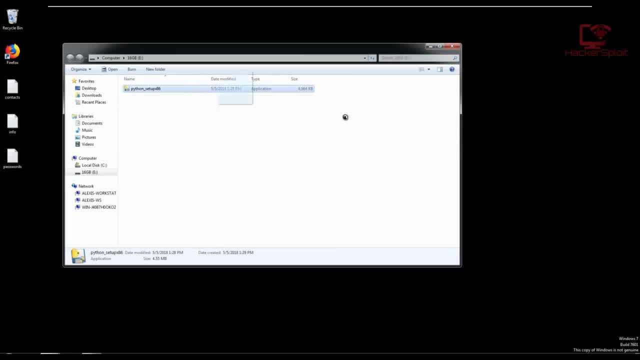 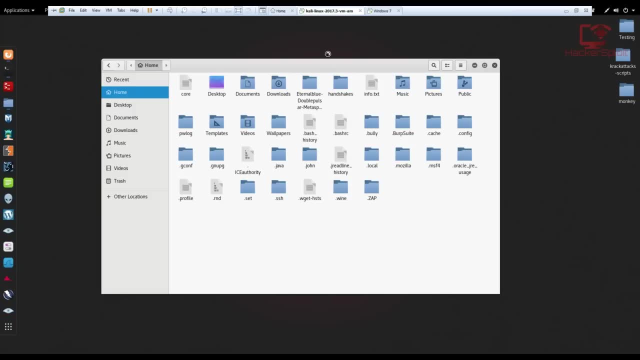 are. that's the file that we've been looking for. It is the pipe On setup and, as you can see, it does look legit. So if we copy it into our desktop, you can see that Windows Defender is not going to detect anything. And now we want to set. we want to set. 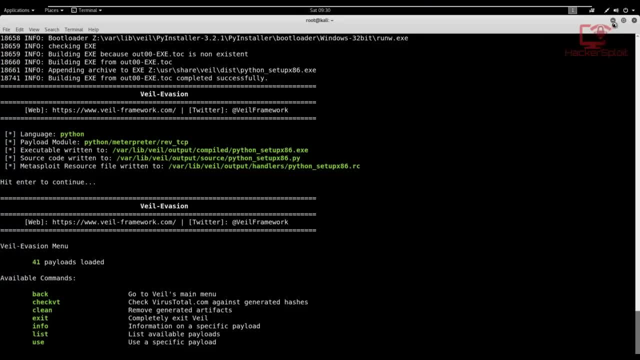 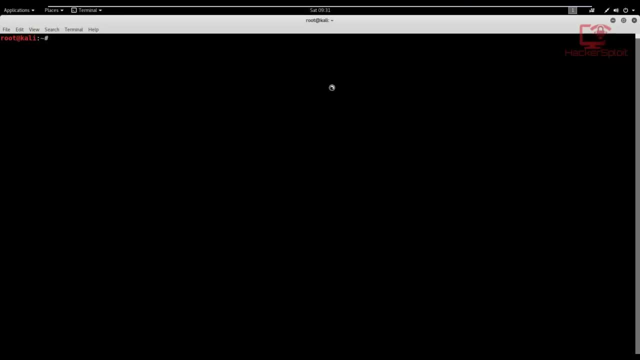 a reverse handler here. So we're going to use Metasploit Now. so we're just gonna open up another terminal here Because we want to perform the listening. So new window, because that is a reverse TCP meterpreter session. So I'm going to MSF console And there we are, we're gonna hit MSF. 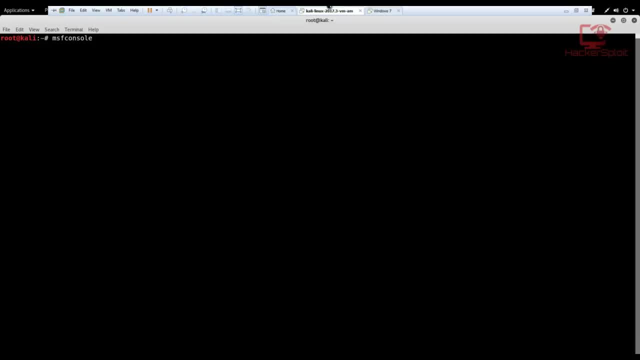 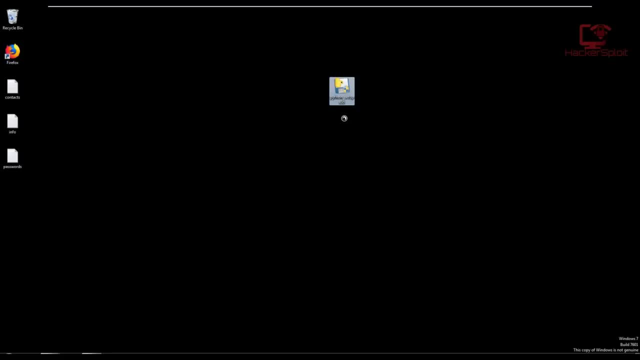 and, by the way, after you have generated the payload with veil evasion, you can perform an online scan for antiviruses, And what I found with the Python version is half of the antiviruses will not detect it. Now, again, this is focused more on the Windows Defender side of things And this 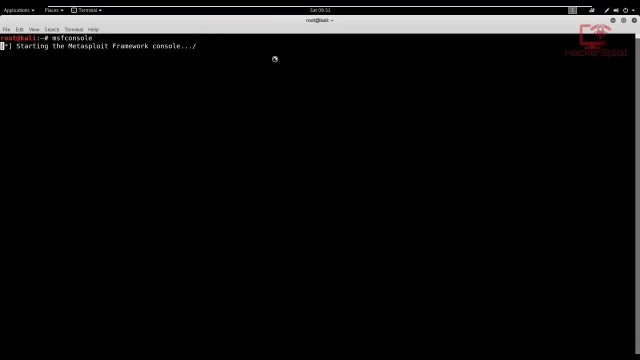 will probably evade, will evade Windows Defender. I would say 98% of the time. when I say 98%, I'm giving the other 2% into the fact that Windows may patch this. However, you can always use low line level languages like Ruby, Golang or C++, But it's really, really complicated to. 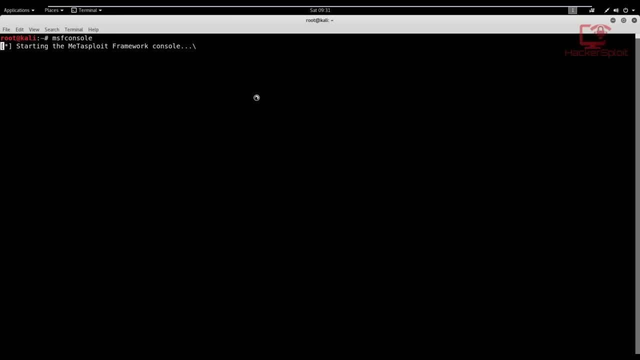 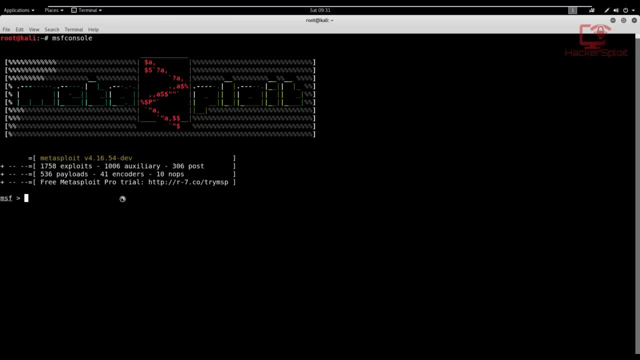 generate a payload with C++, And I'll explain that in a later video, as I still have to continue my my Python programming tutorials And I'm also going to start the C++ key logger tutorials. All right, awesome. So now we want to use the exploit exploit- sorry, exploit multi handler. 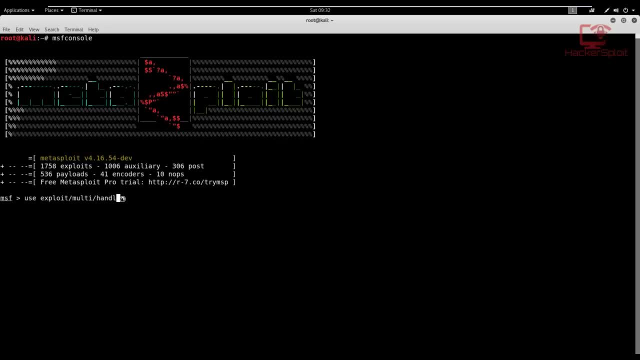 Oops, exploit, multi handler. So now we want to use the exploit, exploit, sorry exploit, multi handler. Oops, exploit, multi handler. So now we want to use the exploit exploit, sorry, exploit multi handler. And now we want to say: use, use Python, Python meter greater, reverse Python. 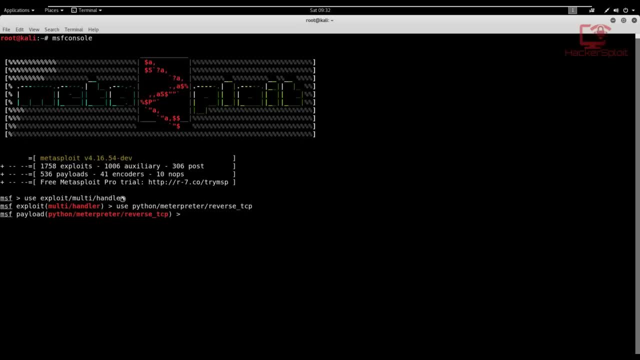 meterpreter reverse TCP. is it an exploit? Yeah, there we are. That's the one Python meterpreter reverse TCP. And now, if we show the, we want to select, select payload. whoops, actually, we what we do. we want to select the payload. So sorry, we just need to exit. I'm not actually. 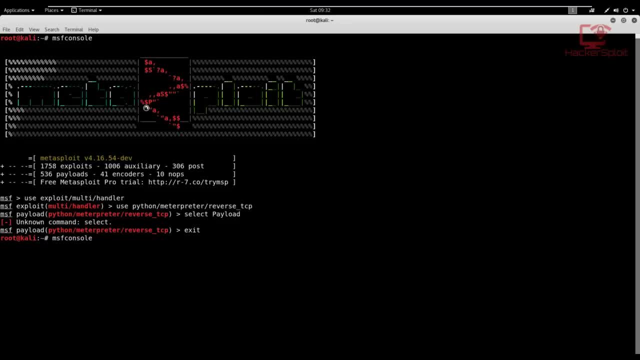 using this exploit, So MSF console. sorry about that, guys got a little bit confused there, Got a little bit carried away. So, as I was saying, this would probably evade Windows seven, Windows eight, 8.1. And also 10, the earlier versions. I'm not sure where they will evade Windows 10.. 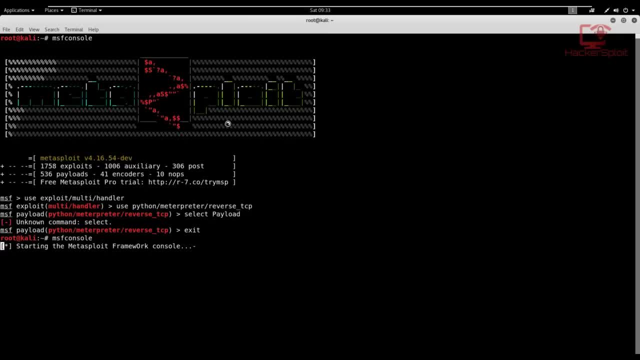 But we will probably look at that in the future. But many of you guys have been asking for this- how to use the elevation- And if you want the installation video, just let me know in the comment section and I'll be. I'll make it, because the truth is it is quite complicated to. 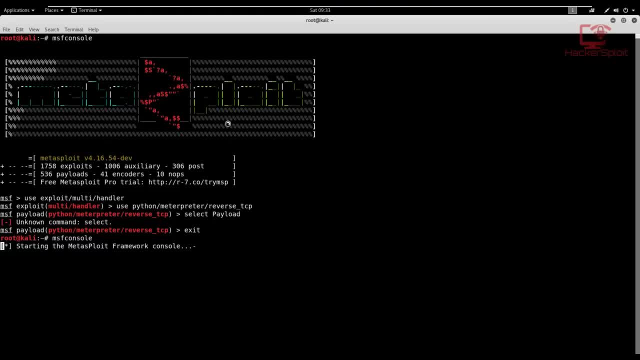 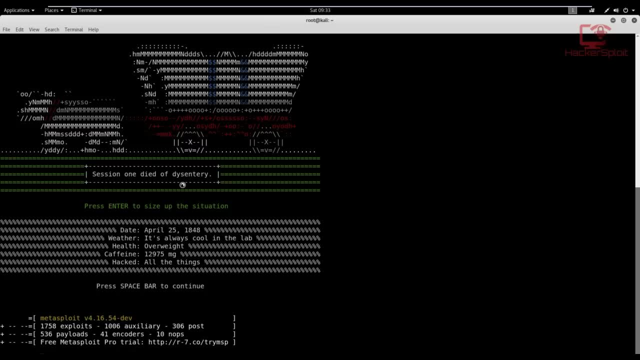 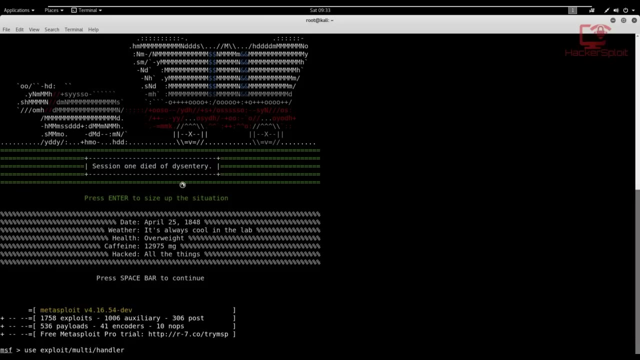 get it set up. But if you have managed to do it, then you're pretty much good to go. Alright, so let's start the Metasploit framework here. For some reason, my virtual machines are really, really lagging right now. So again, use exploit, oops, exploit multi. The multi handler Select. 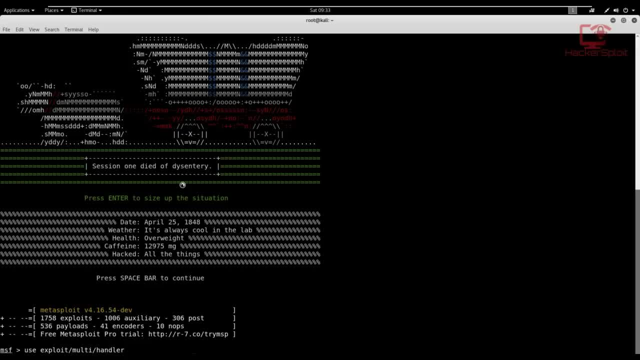 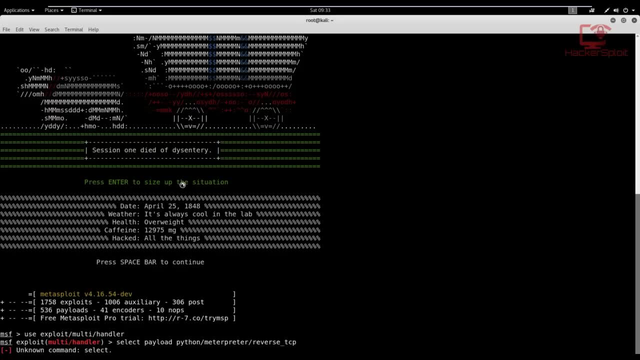 payload, Select payload. And we're going to say here the Python Meta printer, reverse TCP. and I'm going to enter: oops, use payload. Sorry about that, I'm really getting confused today. Use payload. There we are, And 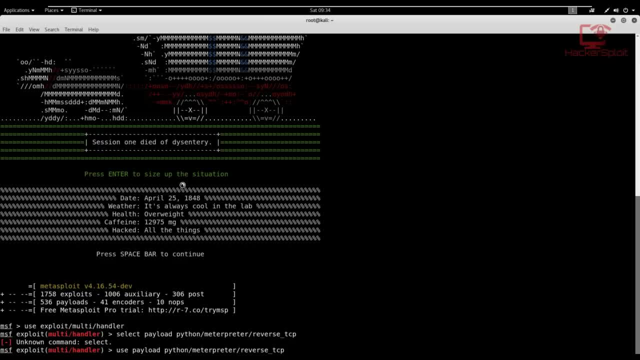 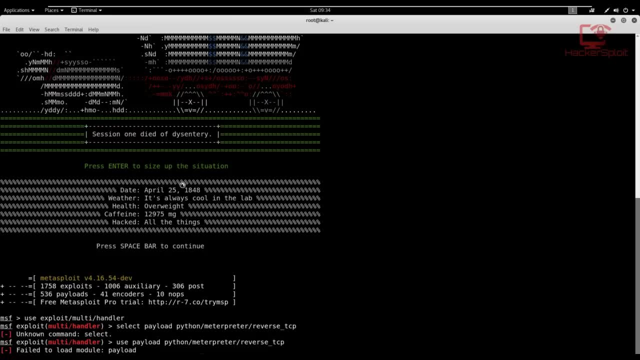 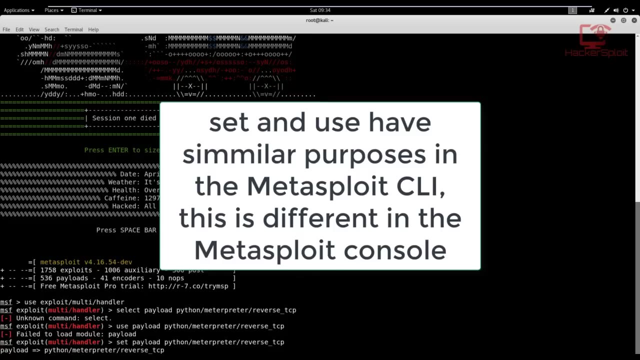 once it uses the payload. once we've selected the payload, we then need to just set the L host, which is our current IP address. the host IP address fail to load module. Oops, sorry, use payload. Hold on about this. set payload. Sorry about that, guys, My apologies. 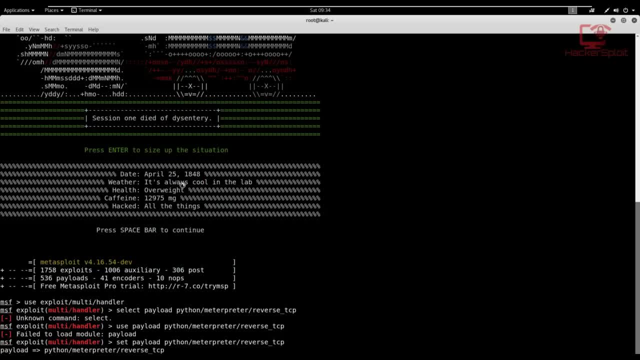 I've got a little bit confused with vaily vision and this because the commands are slightly different. now busy been using the command line, but that's not no excuse. So set the payload. Now we need to set. set the L host. Oops, L host, and the host is wanting to point 168, point 1.4, 105.. So 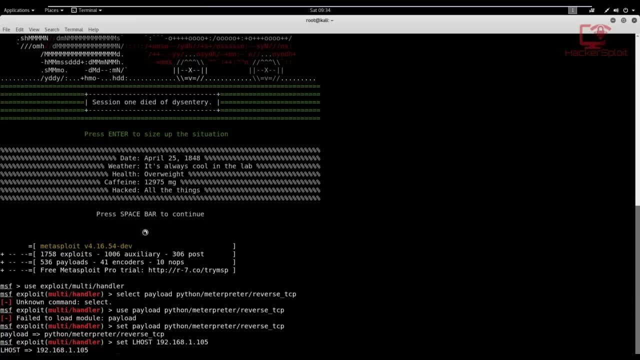 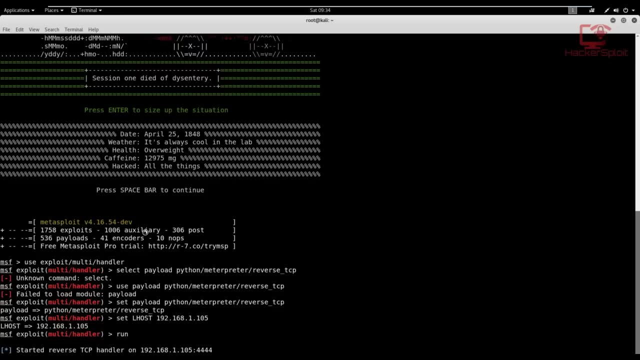 this is your host operating system or Kali Linux, or IP address. So I'm going to hit enter And we've set the lhost, And now we're just going to hit, we're just going to run, All right, and it started the reverse TCP handler. And now what we need to: 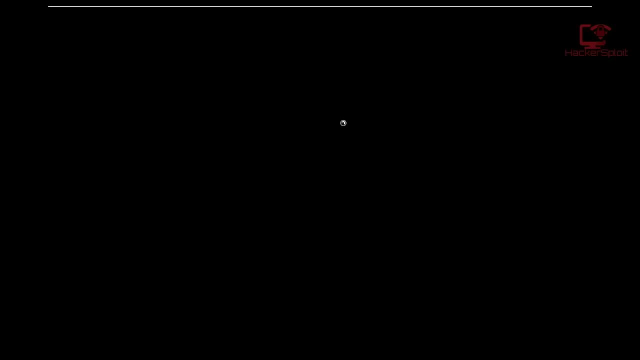 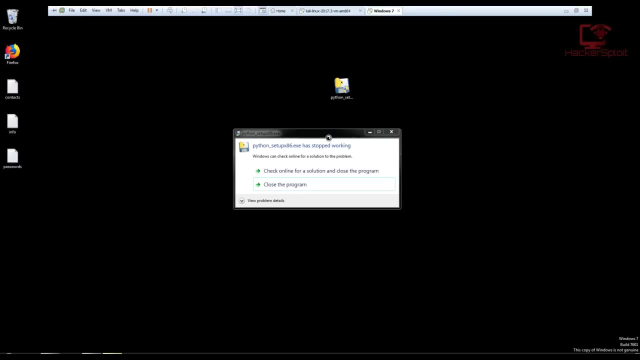 do is we need to run this application. So I'm just going to run it And probably tell us that it stopped working For some reason. my windows has crashed here for some reason, or there we are. The launch, give it administrator privileges And there you are. meterpreter session open and 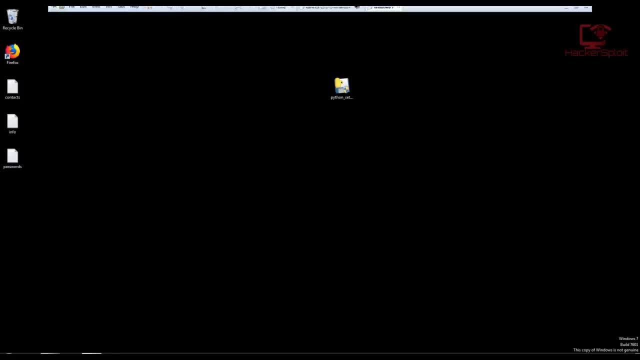 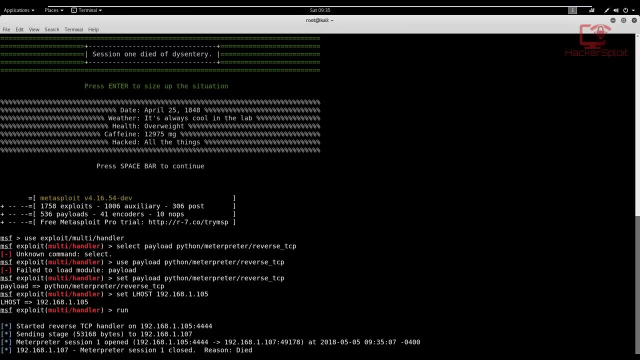 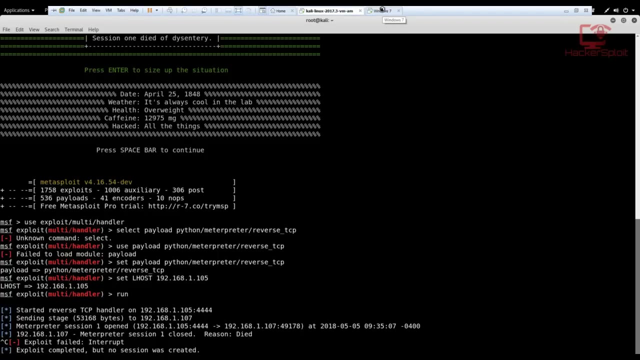 Windows was not able to detect anything, or and the program was able to evade Windows Defender. So you can see, definitely works And you can go ahead and and use the meterpreter session if you want to. Now, when we're talking about the other ways of using veil evasion, and I'm probably just going, 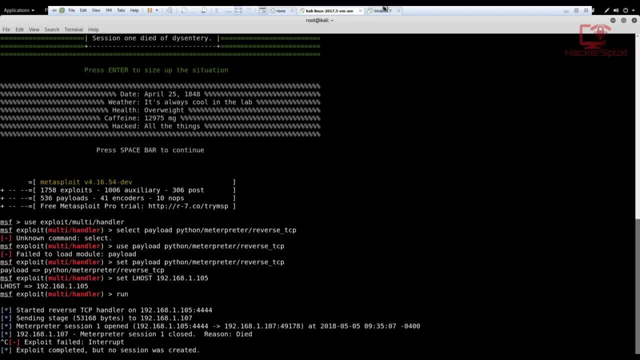 to end the video here because I want to cover file splitting and hexadecimal editing in the next video, Which will come shortly after this one. But if you want to use veil evasion, what I would recommend is to go through the other options that it does provide you with. And you might be asking what. 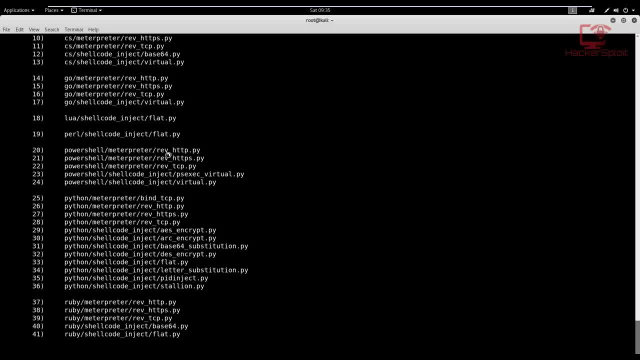 what am I talking about? Well, I'm talking about the, the payloads that you can use. So if I go back to list here, you can see that I have the Ruby meterpreters here, which sorry about that. if you can hear a dog barking in the background, I apologize for that. What I would recommend is: 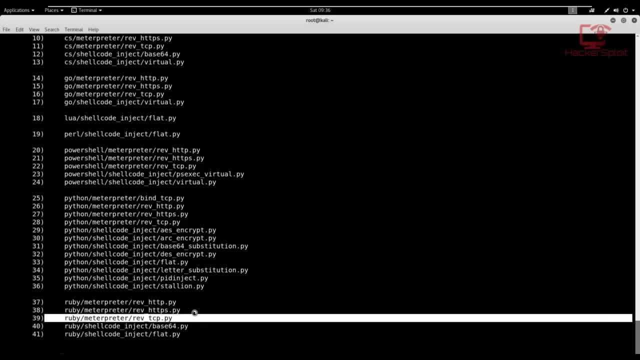 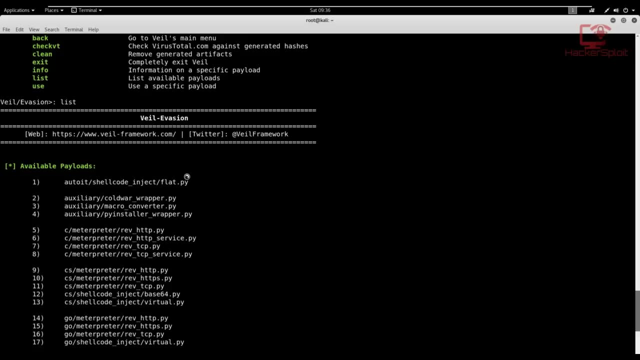 to use the option 39, which will generate it in Ruby. And then, finally, you can, you can then use, you can then use Metasploit again to perform the reverse meterpreter, to give you the to to handle their, the reverse connection. All right, that being said, you can perform different scans on: 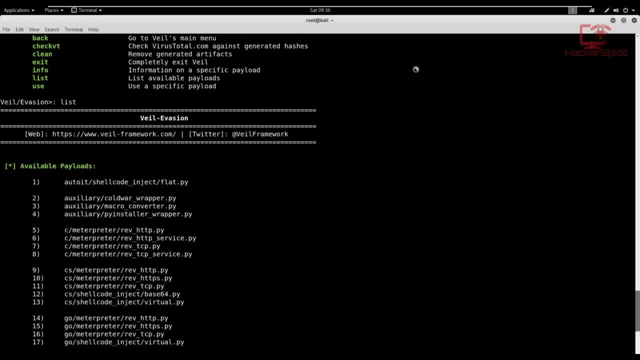 these on the payloads or the executable files that you generate. But you can see that with veil evasion it is all dependent on payloads. Now, in the next set of videos in this series, we're talking about virus, antivirus evasion. I'm going to be talking about file splitting. 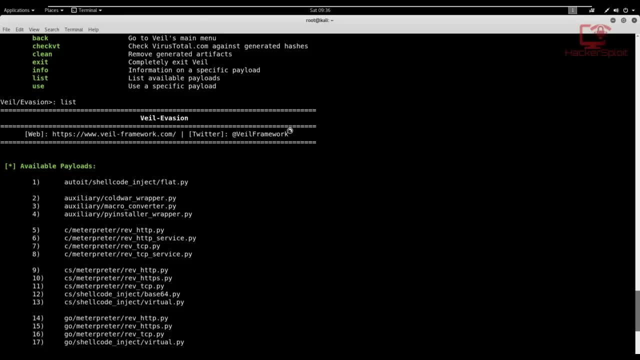 Which really works. you know, to your surprise, you don't need to change anything about the file. you split the files and then you edit the strings with the hexadecimal editor. But it is quite complicated And I'll show you how to perform the calculations, because there is 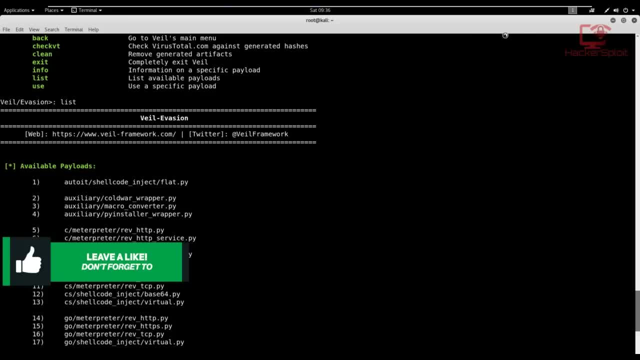 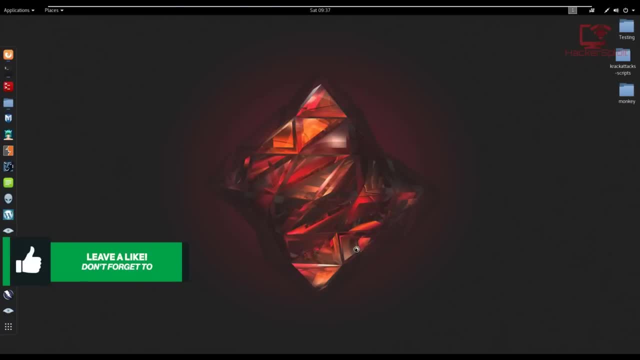 there is, and are, a lot of arithmetic calculations, involve scientific arithmetic calculations. That being said, that's gonna be it for this video, guys. The s7 video is scheduled to be out tonight, latest tomorrow morning, but it should be out on the website, So just stay tuned for that. 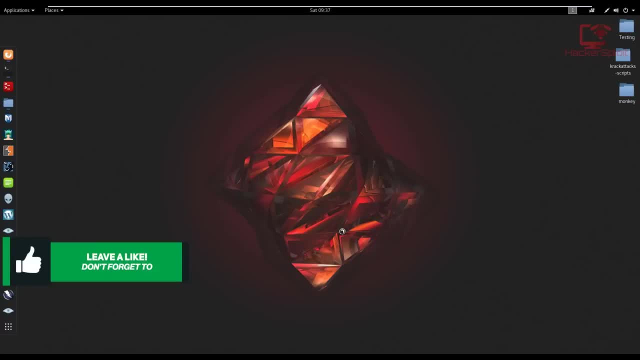 I will be posting updates on Twitter as to when it will be uploaded. That being said, guys, if you found value in this video, please leave a like down below. If you have any questions or suggestions, let me know in the comment section or on my social networks, and I'll be seeing you. 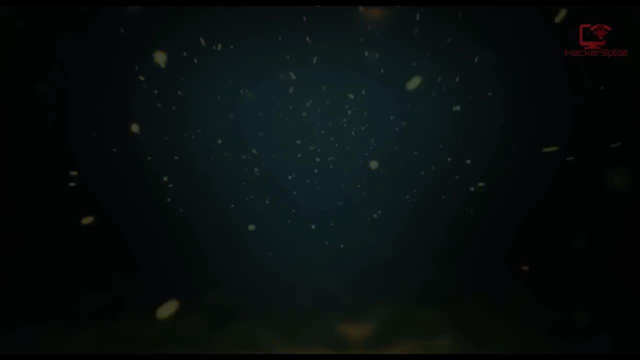 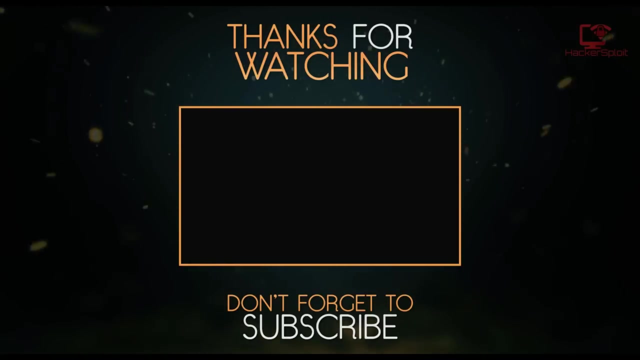 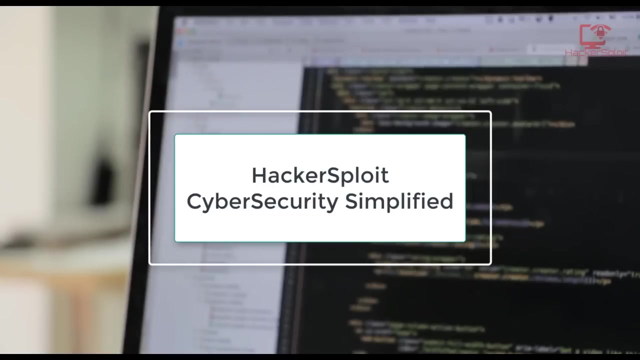 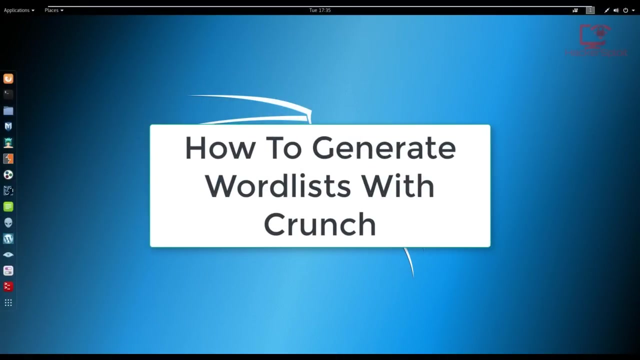 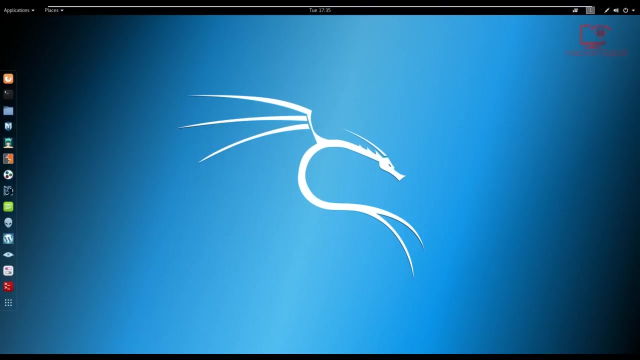 in the next video. Peace guys. Hello everyone and welcome to this video. In this video, we're going to be looking at how to generate word list with crunch. Alright, so crunch is a fantastic word list generator that generates word lists based on the criteria that you pass to it, So it's a fantastic password. 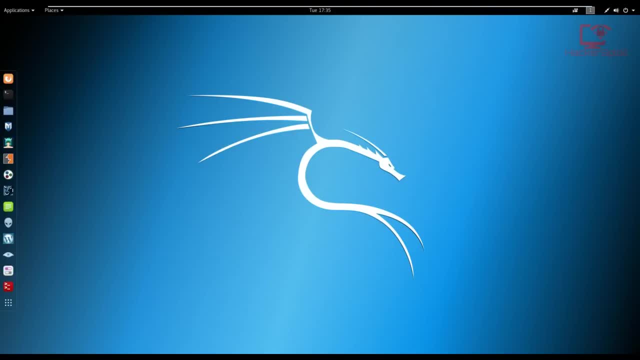 utility that is pre installed on Linux and it's excellent for generating word lists. Okay, so in the in the previous section we looked at how to use word lists for brute force- essentially for brute force attacks- but we did not look at how to create. 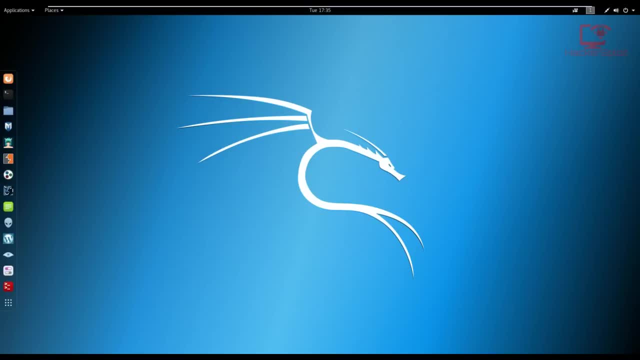 one and how they're used. In this case, I'm going to be showing you, creating you how to create your own word list with crunch. Alright? so, as I said, crunch comes pre installed and pre configured on Kali Linux, which is awesome Right now, before we get started. 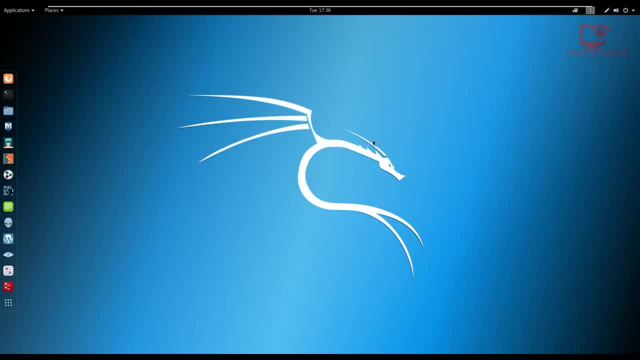 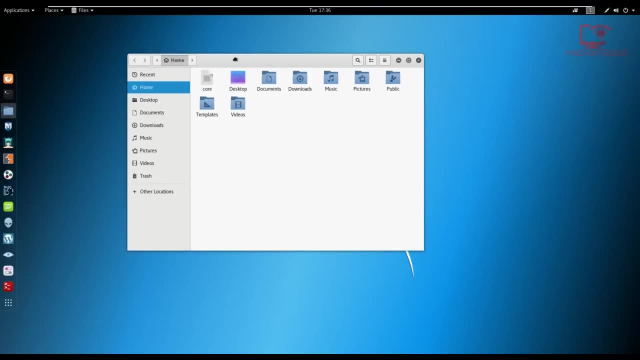 I just want to show you guys something that you know that is really important for you to understand, And that is that if you go into your file directory- and the point here is that Kali Linux already comes with with some pre configured or already comes with some word lists that you can use by default- Now these word lists can be. 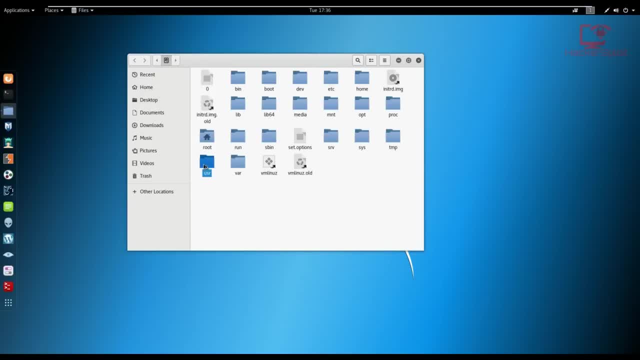 found in other locations. Google your computer and you go to user and you go into your share and you just want to scroll all the way down, or you can use your search menu here and just type in word lists, Alright, so once you get that, just open it up And, as you can see, you have. 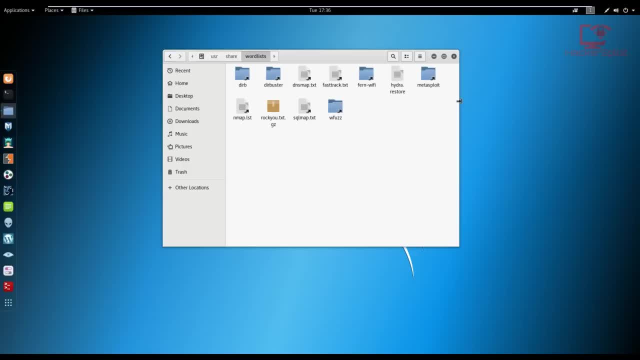 your word list right in here- that are that come pre installed or that come with Kali Linux. And the great thing about these ones- they're not just pre configured, they're pre configured So you can- is they're very, very powerful and they're based on different types of attacks. So, for example, 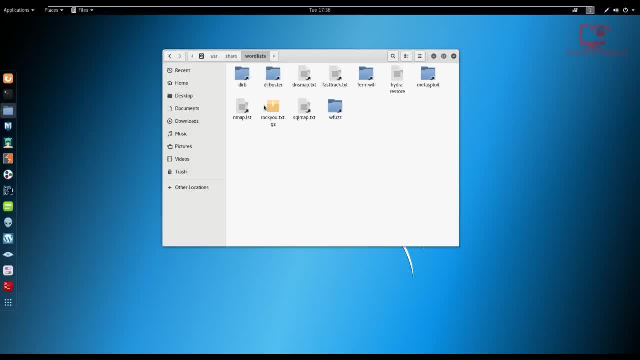 you have your SQL map or word list, you have your N map word list, you have one of the most popular word lists in the world, which is the rocky word list, and you know so on and so forth. So these will come really in handy when specifying a word list And especially, especially, if you do not want 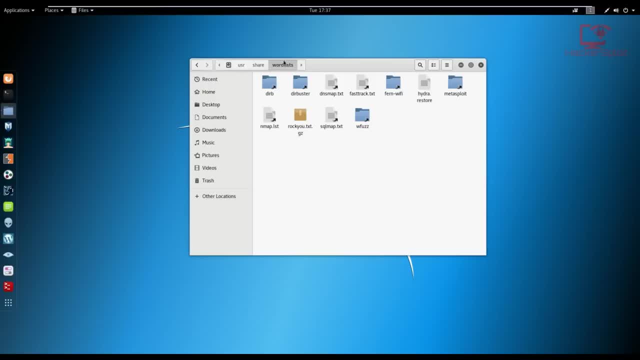 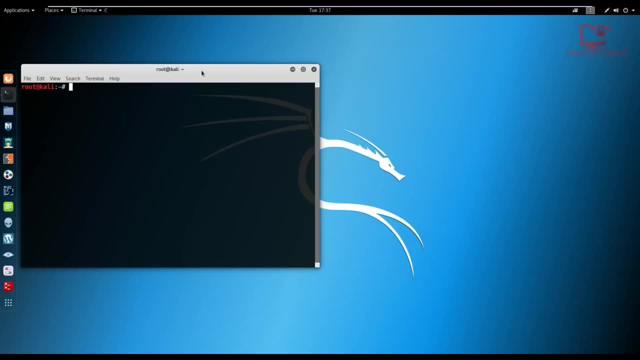 to generate your own. this is a great starting point. Alright, so you just select the working directory, which is user share and word lists. Alright, so let's get back to crunch And let's look at how we can create our own word list. Alright, so the first thing you need to do is you: 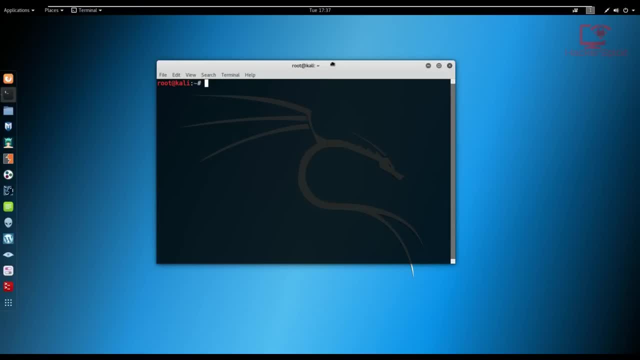 need to make sure that you're working the directory in which you want to store your word lists in. Alright, so what I'm going to do is I'm just going to change my directory to my desktop, Alright, so I'm going to change my directory to my desktop And now in here I'm going to create: 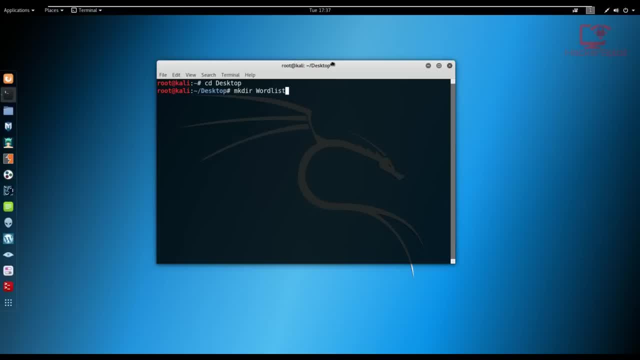 a folder And I'm just going to call- I'm just going to call it word lists, right? so make directory word lists and I'm going to change my directory into that folder because that's where I want to store my word lists. So I'm going to hit Enter. 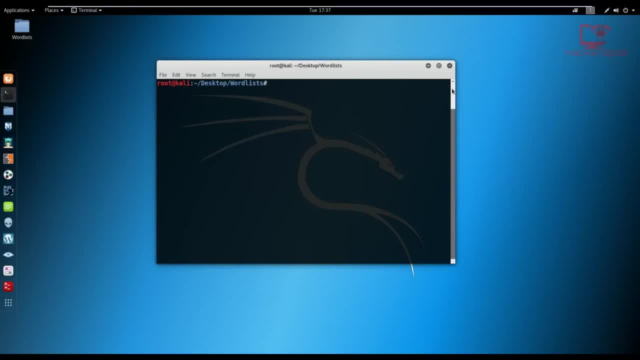 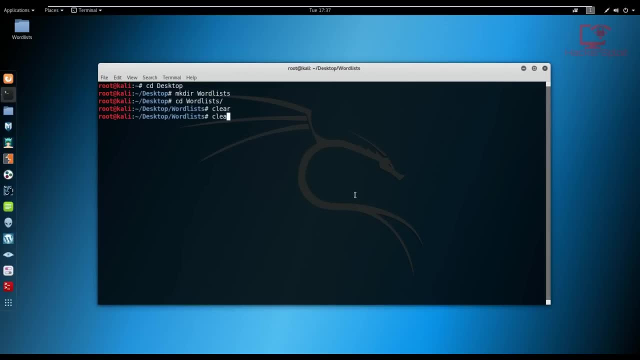 we can clear and now we can get started with crunch. Alright, so crunch is very, very simple to understand And it's very, very easy to start generating your own word lists, depending on the parameters that you want to pass. Okay, so let's look at how to use it. So, 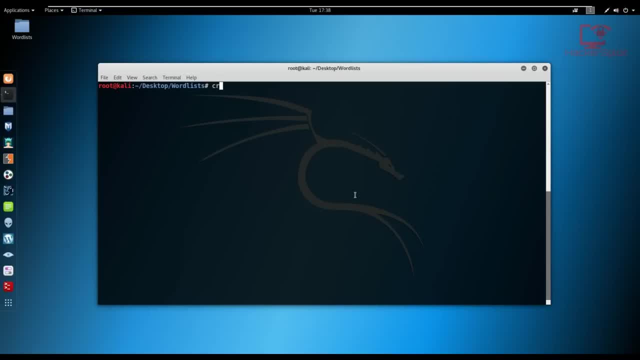 the syntax is very simple. you obviously start off with the, the crunch, Alright, the crunch command, and you can also look at the Help menu if you ever feel lost, Alright. so, as you can see, the usage is pretty much given here. So you have crunch, the minimum, minimum and maximum value, and 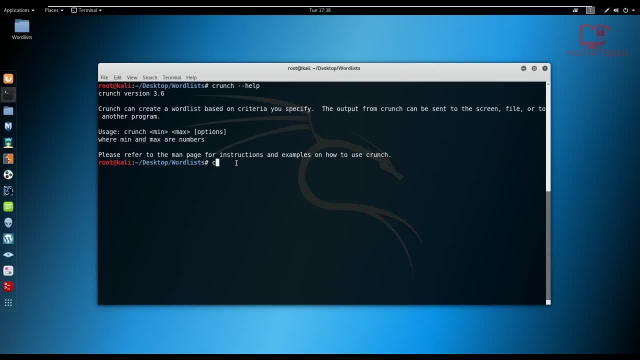 then you select your options. Alright, so I'll explain to you what this means. So if we just clear this and we get started, so let's say, for example, we want to generate a word list that contains words with three or more letters, but the letters should not be less than three and not be 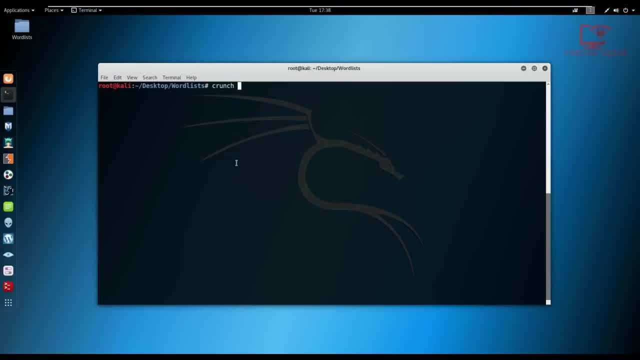 more than something like five. Alright, so what would we do? you would say minimum. the minimum amount of letters to generate or work with, in terms of the words to create, is three. we then select the maximum amount. So the maximum should be three, And then we select the maximum amount. 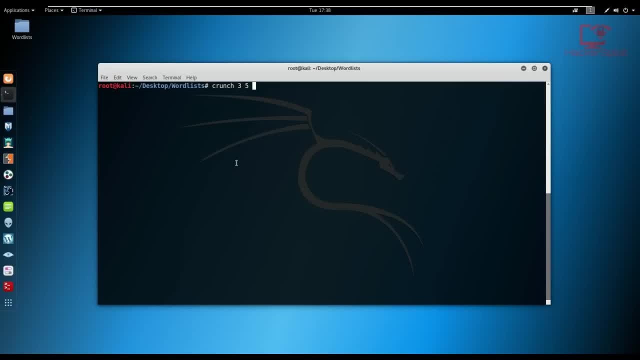 should be, let's see five. okay, so the minimum and maximum is specified. Now. now we need to select the character set that you want to specify. So a character set is pretty much self explanatory: it is the characters that you want to specify to be used in this word list, Okay, so, for example, 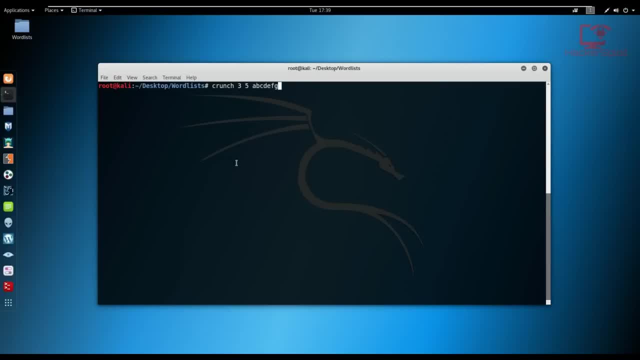 we can say A, B, C, D, E, F, G and only specify ABC, till the A to G essentially, And then we can also specify numbers, So we can say one, two, three, four, five, six, seven. 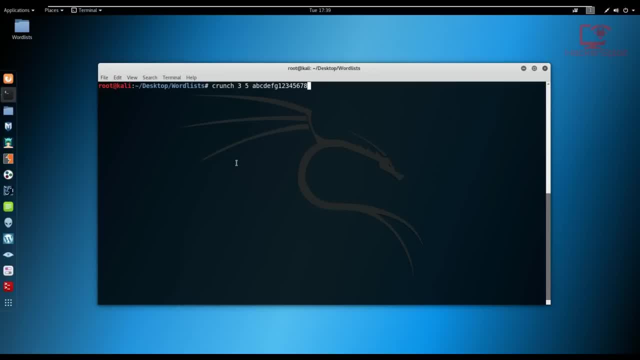 eight. alright, so it will only use this character set to generate a word list. Now, by default, this is not really. it's really not something that you would be looking at, But it comes really in specialized situations when you want to generate word lists for more specific types of cracking or 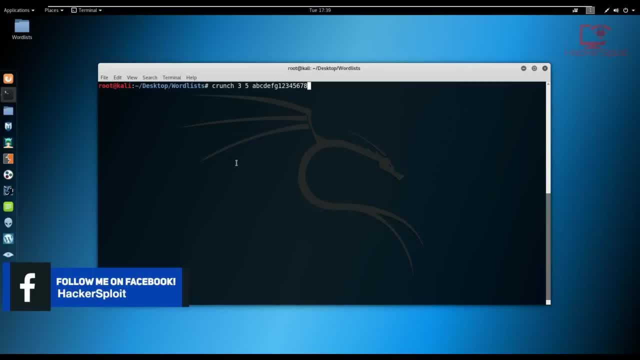 approaches. Alright, so we're just going to, we're going to create this one And I'll show you the correct way of creating one, or the way that I use to generate word lists. Okay, so this is what this the syntax is so far. So we have specified crunch, we have specified the minimum. 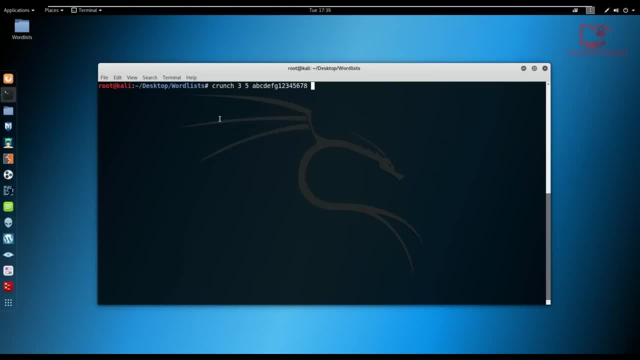 amount of letters, and we have specified the maximum amount of letters. So we know that all the words in the word list will be will be more than three letters, but less than five letters- Excellent. We've then selected our character set, which is the characters that the word list will be. 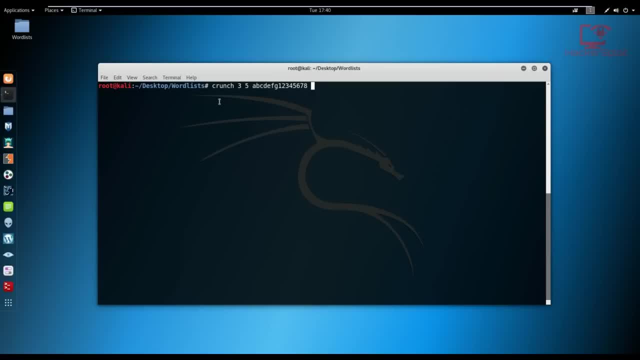 based off. So it's currently going to use ABCDEFG and 12345678.. Alright, now you might be asking: well, how do we output this into a word list? Well, what we do is we use the O command. 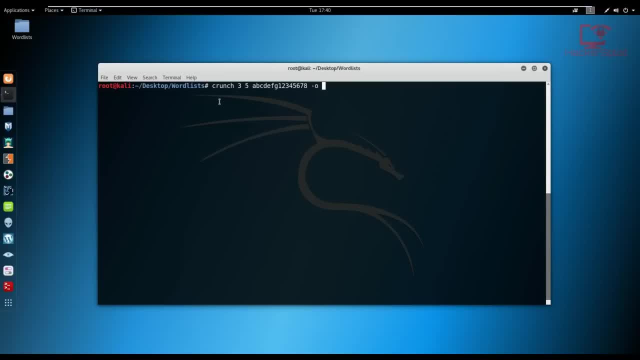 which specifies an output, And then we just type in the name of the word list that we want to give. So I'm just going to call this word list One dot txt. All right, the extension is very important. You can use a dot lst extension. All right. 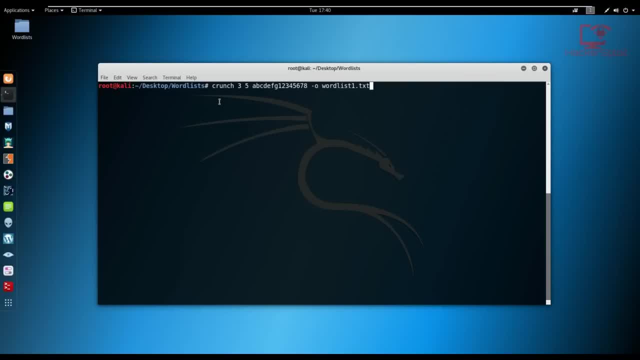 which is also good, Or you can use a dot txt extension, which is also going to work perfectly. Alright. so I'm just going to hit enter And, as you can see, the crunch will now generate the following amount of data, And it'll give you the size or the amount of data in terms of the word. 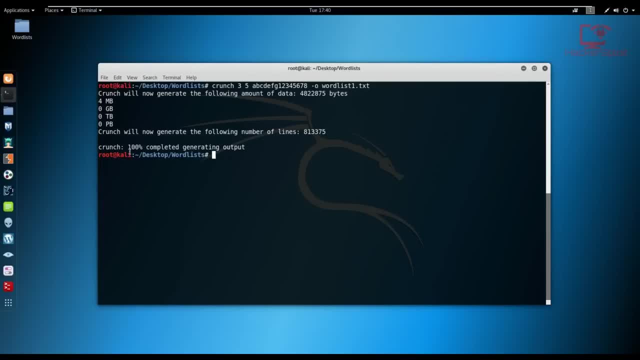 list that is going to generate And, as you can see, I took only about four megabytes. That's because, with relative, this word list is relatively small because of the character set that we've provided. Remember, if you do not specify a character set, which is what we'll- 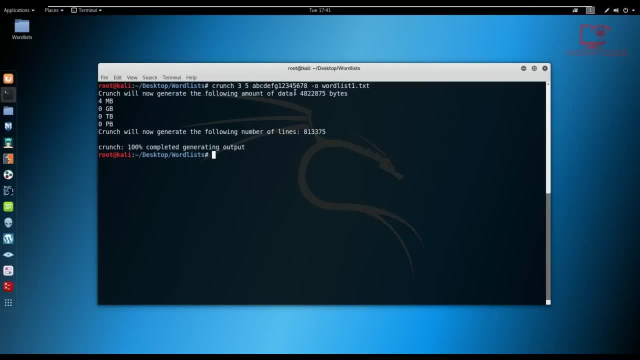 be looking at. it's going to generate a word list that contains all characters. Okay, so you can expect the size to be quite large. As you can see the unit specified here you have gigabyte, terabyte and petabyte, So you know, things can get really, really big And it's very. 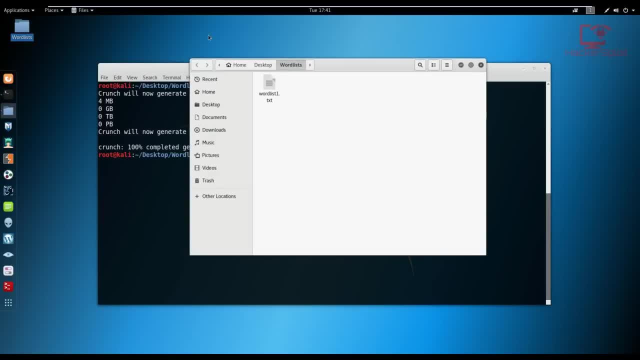 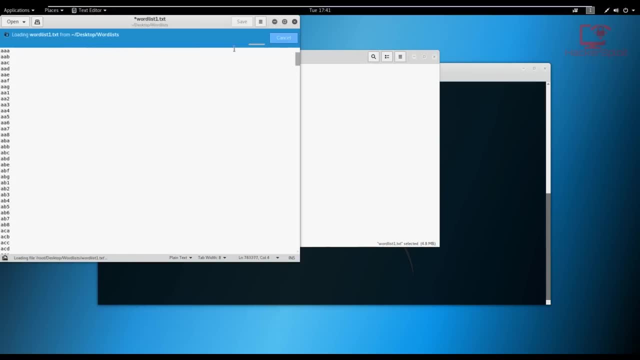 very important to understand that. Okay, so let us look at the word list file Now. if I just going my word list folder and I look at the word list, one dot txt, if I just open that up, you can see it's going to take a while to open up And there you are. So you have characters, you with the. 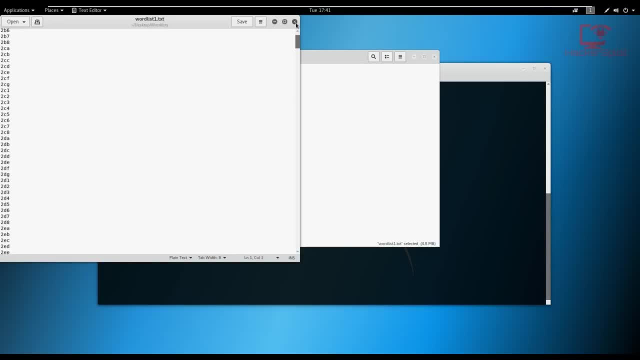 character set, that we we have letters with the character set and the words that have been generated. So you can see some three letter words. we scroll all the way down, you have your four letter words, five and so on and so forth, And it continues all the way down using all the character. 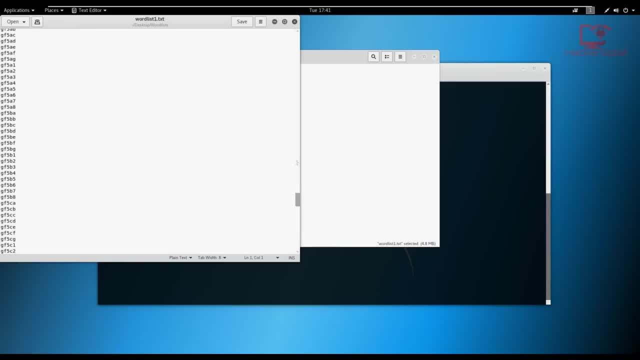 sets and the combinations that are possible. Now you can see that this word list is extremely large, you know, likely, so it is a very, very powerful word list in its own way. Okay, so that is how to generate a word list in, you know, in proper, proper theory. So now let's look at how to create a word. 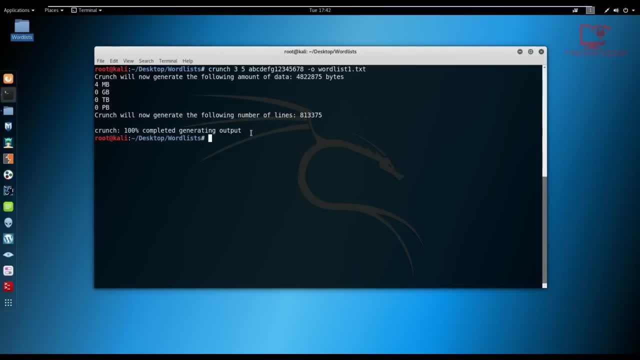 list. that is actually quite powerful. So what I'm going to do is I'm going to say crunch again, let me just clear the terminal. So I'm going to hit crunch, Okay, crunch. Now I'll specify a minimum, And I would specify the same amount of the same range. So let's specify the minimum of. 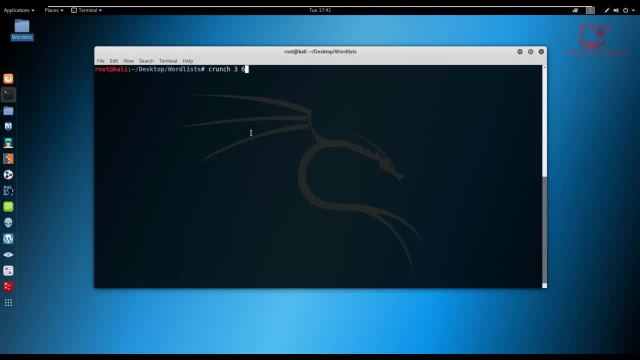 three and a maximum of six. This is usually about a good range to work with, especially when you're trying to crack. you know services like SSH. you know your telnet port, etc. etc. Now I will not specify any character set. that because 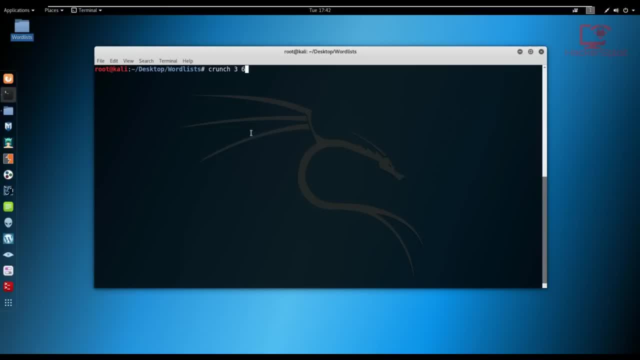 that's because I wanted to use the entire character set, And you know, therefore it is. it becomes even more powerful because the amount of combinations have increased And therefore there's a higher chance of you actually getting the password that you're looking for. So now all. 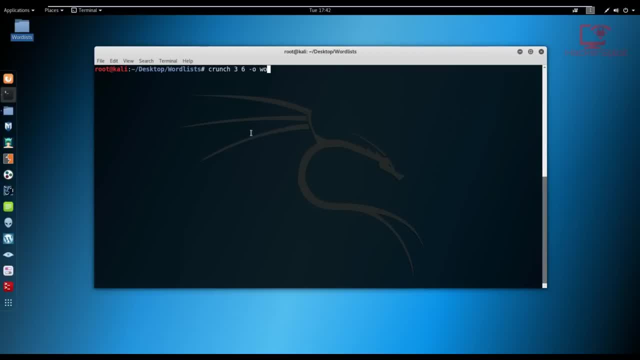 I have to do is I just have to output the word list. Alright, so I'm just gonna call it word list two, two dot txt, And once I hit enter, it's going to output this word list. So I'm going to hit enter And, as you can see, this one is slightly larger, significantly larger. it's two. 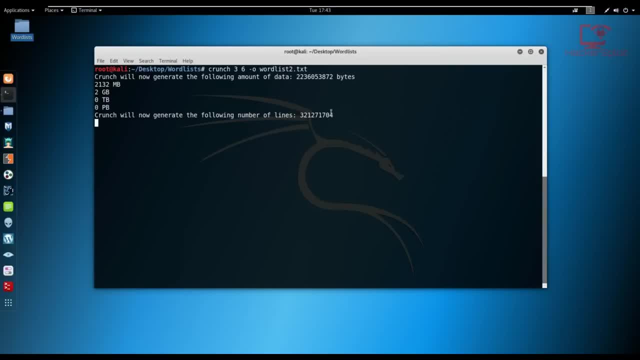 gigabytes. Alright, so now it's going to generate the following number of lines: as you can see, it's going to tell you And, of course, because of the size of it, it's going to take quite a while. So, as you can see, crunch 8% completed generating output. So this is a really, really, really huge. 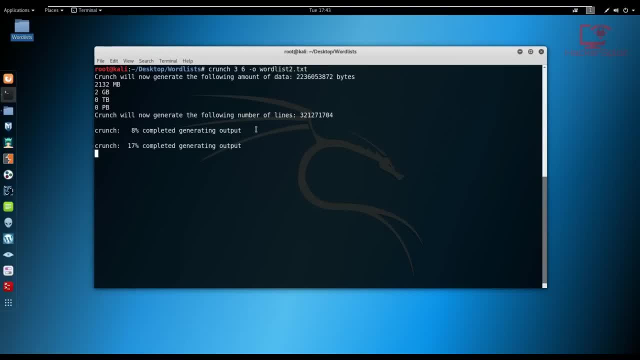 word list. Now, something else I'm going to do is I'm going to go ahead and hit enter And, as you can see, what I want to explain is you can generate word lists using crunch. Alright, so it's, it's a. 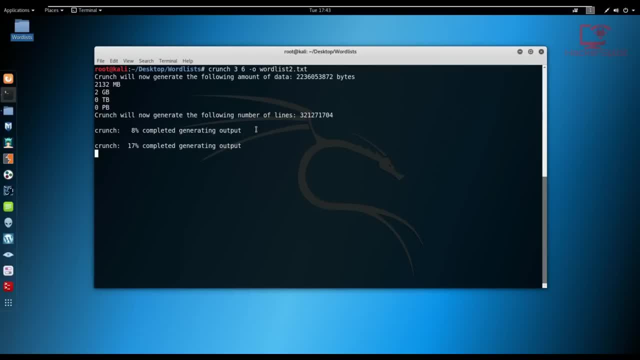 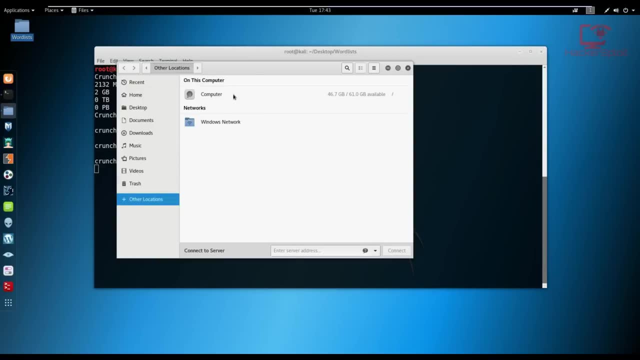 fantastic password utility to generate word lists- Now most of the the powerful word lists that you will find online and, more specifically, word lists like the ones that Kali Linux already comes with, which you can find in the user and you can find it in share And, if I just search for it here, 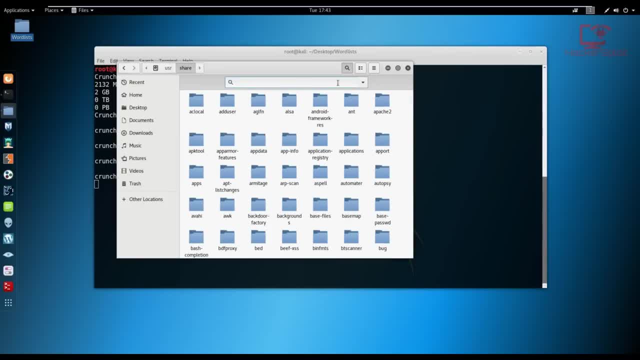 I want to explain a few things while crunch is generating that large word list file- Alright, so, Alright. so let me just open that up Now. the thing with these words- more specifically the rock you word list- is it contains leaked or stolen credentials. 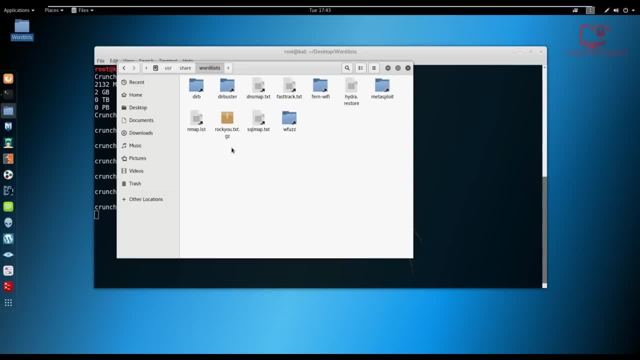 actual, you know passwords. it actually contains passwords that were leaked or stolen from website and then what were released to the public. So this is why these word lists are considered much more powerful: because they actually contain real password combinations that are likely to get. 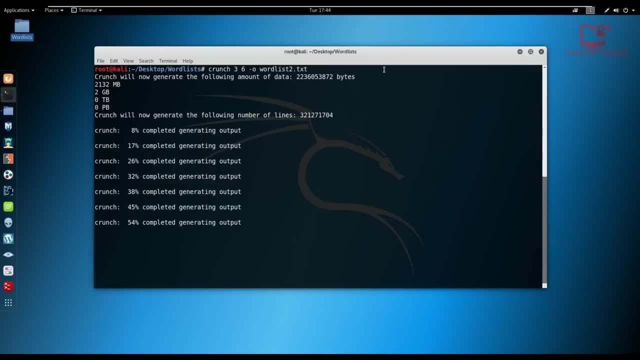 you into a system Now by default. using something like crunch is is like shooting in the dark. That's because you might, you might be able to get into a system where you can actually get into a system where you can actually be able to crack. you know a login or or you know 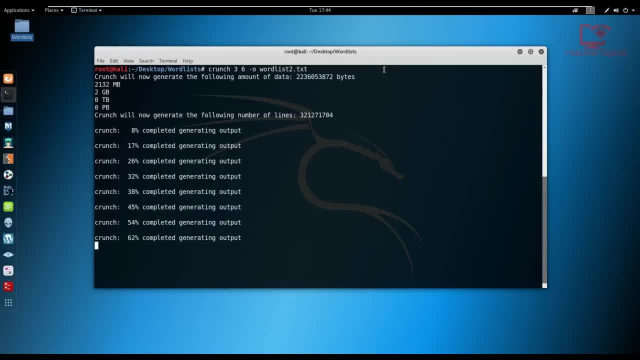 for some reason, if the word list was not good enough or did not contain the correct the correct character set, you might end up with a failed, failed exploit or a brute force attack. Okay, so we looked at performing a brute force attack in the previous section, when we were using 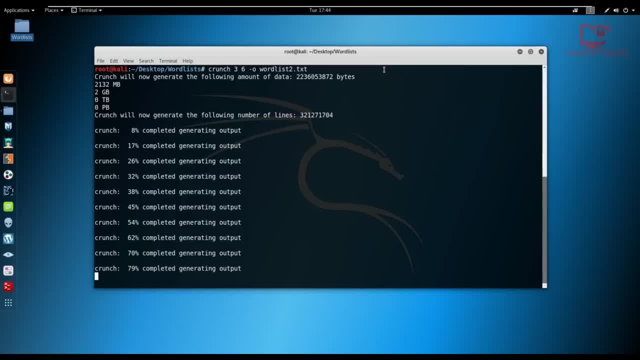 when we were using Metasploit And obviously in the WordPress section, where we are trying to brute force the the login of the WordPress site, you saw that when using a word list it does work. if you have a fantastic character set, Now by default this word list. 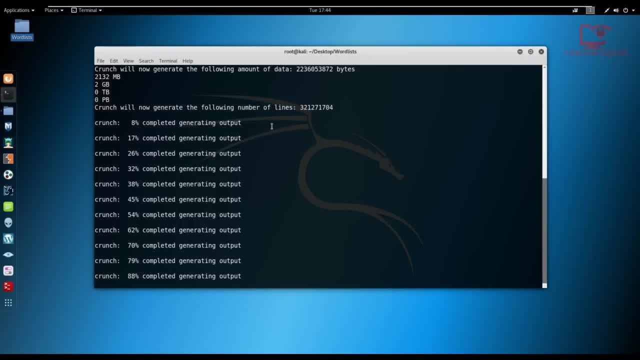 that we're generating with crunch, as you can see, is quite large, more specifically two gigabytes, but it is quite powerful in the sense that you are likely to crack services like the SSH or telnet. you know really, really basic types of services. Alright, so the word list is generated, And now 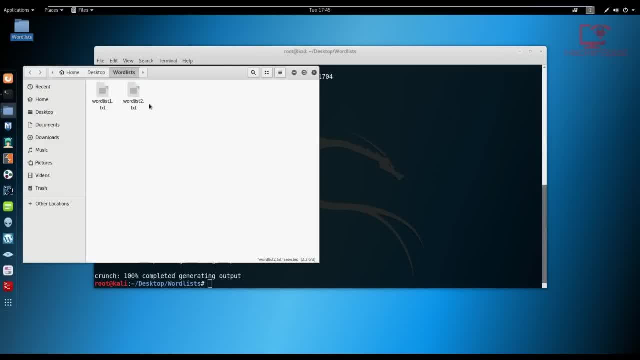 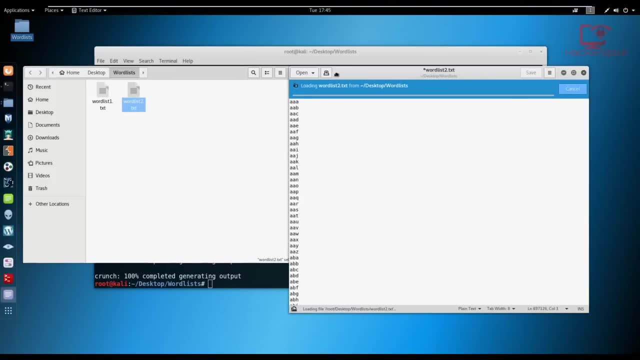 we can just open up our folder and the word list to dot txt. Now, this obviously, depending on its size, will take quite a while to open up with my text editor, And there you are. So now, as you can see, it is still calculating the amount of lines that it contains, which just proves to you how 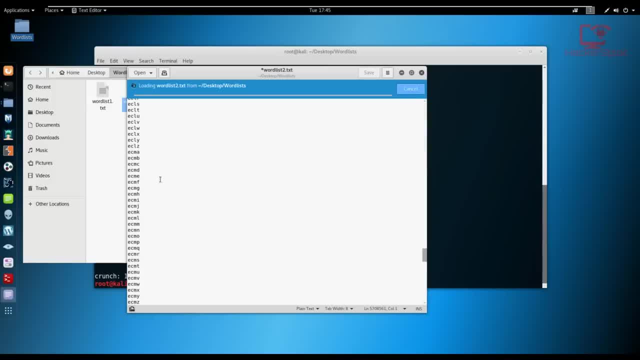 large. this word list is Okay. so even if we scroll all the way down, you can see the number of combinations that you can find here. And we've not even hit the ones that have the ones that have numbers or contain characters. So that was how to generate a word list with crunch. it is a 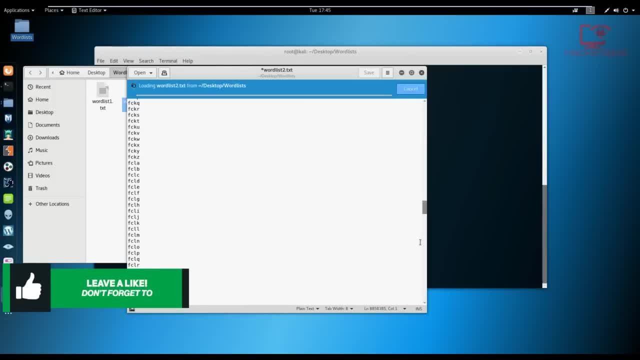 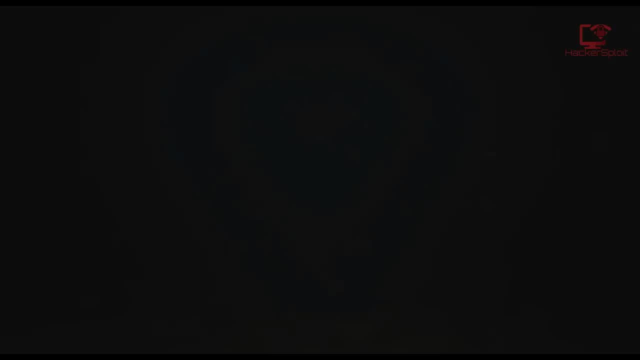 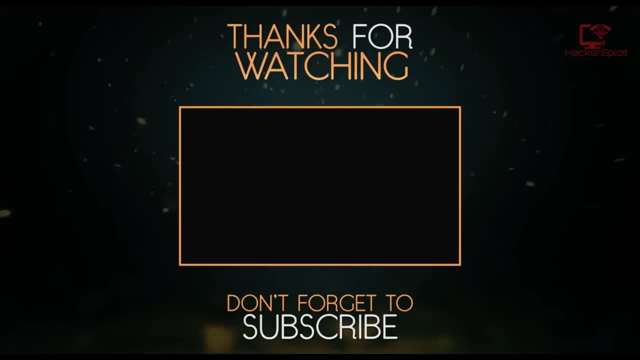 fantastic password utility, And it's always good to know how to generate your own word lists with your specific character sets or user preferences. Alright, so that's going to be it for this video. in the next video, Hey guys, Hackersploit, here back again with. 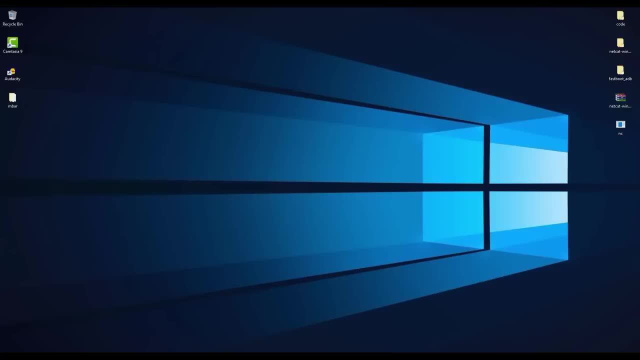 another video, And in this video we're going to be looking at net cat and how to use it to perform a variety of certain functions or tasks, really. So for those of you don't know what net cat is, net cat is essentially almost like or the Swiss army. 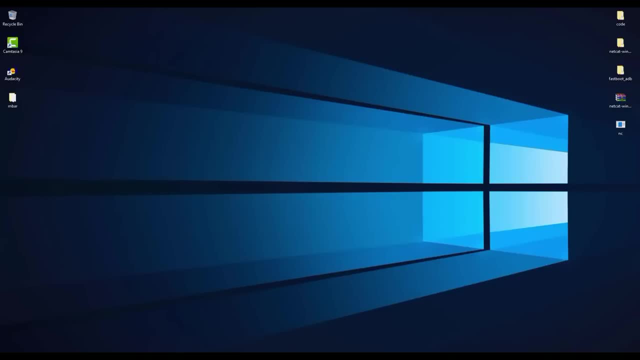 knife of networking tools and and allows us to perform a lot of things like reverse shells, you know, port listening, and that really comes into play when you talk in the ethical hacking field. But irregardless, you know, regardless of of the features that it does allow you to use. 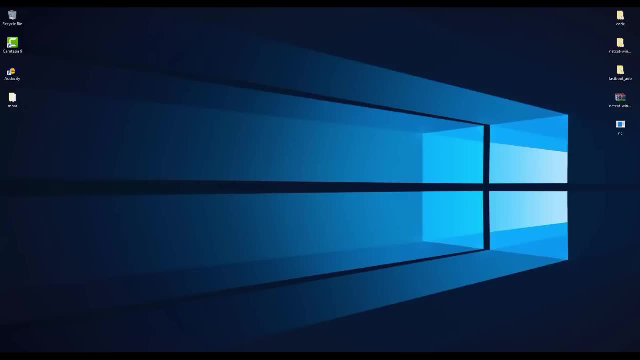 it's a fantastic networking tool that can allow you to communicate between you know two or more computers and allows you to perform a plethora of functions. Now, what I'm going to be doing to illustrate this is: I'm going to be running, you know, Windows and Linux, and I'm going to be 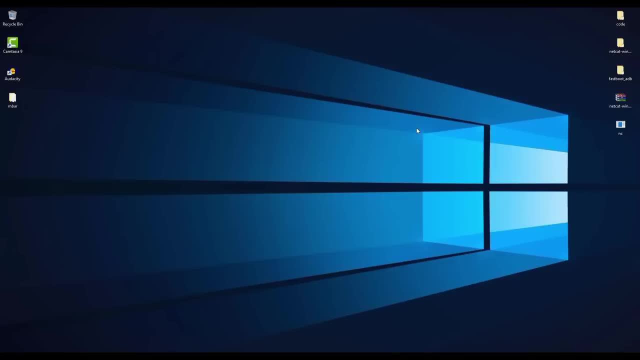 transferring information or communicating between those two operating systems. So I already have net cat downloaded on Windows, As you can see here. the link will be in the description for this download, So make sure you extract it and the net cat executable is on your desktop. Alright Now. 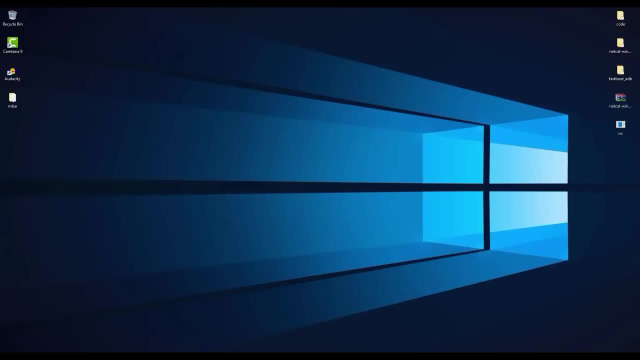 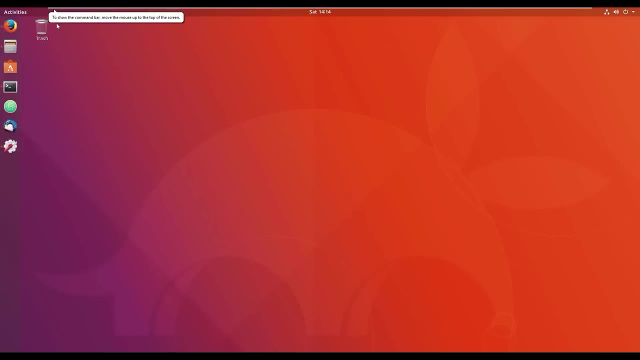 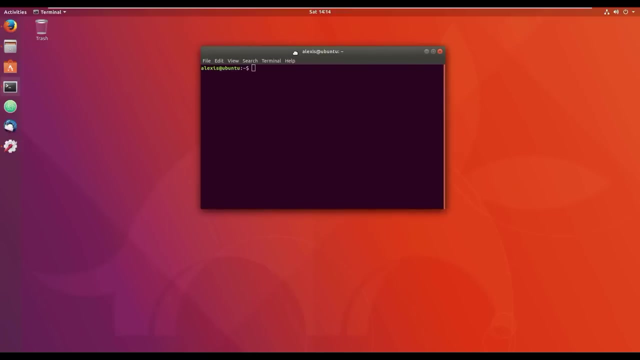 once that's done, again, if you're using Linux- which probably you are, because this is where it really is quite awesome, Let me just unpin that. So, essentially, on Linux, net cat comes pre installed. but if it doesn't come pre installed, you can just. 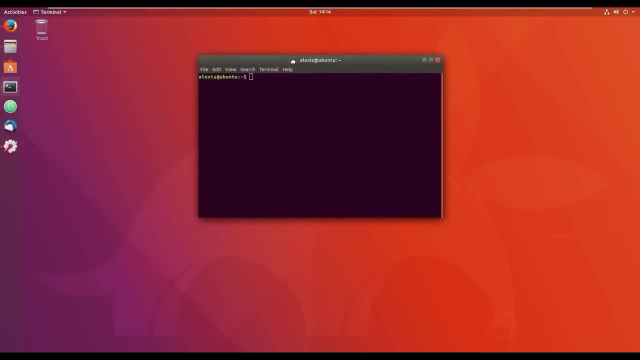 install it using the app You know. you can just download it and it'll be installed for you. I'm running this on Ubuntu, So essentially, it's really really very simple. on how to run it Now, before we actually get started with 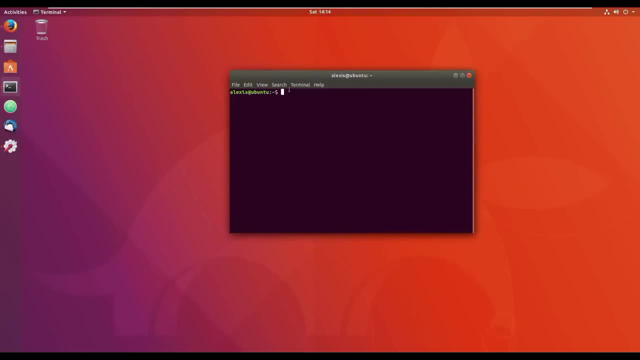 communicating between the two. we will be using net cat to obviously communicate between these two, So we are going to do it locally, not I'm not going to be using the IP addresses- the actual IP addresses- to communicate, but that is an option And from there you can get an idea of the power of this tool. It's quite. 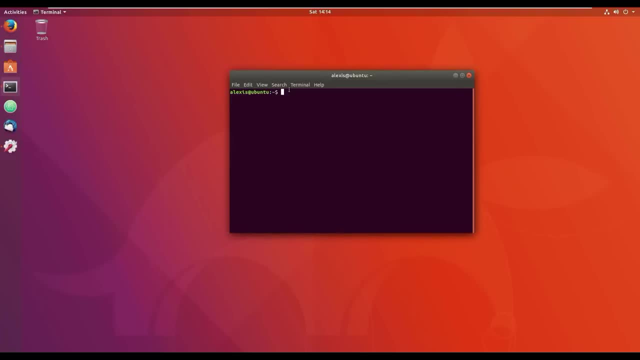 different from secure shell because, again, initiating, you know, reverse shell with net cat is much easier. And again, SSH is really not that awesome, or it really is, isn't, I would say, designed to be used on Windows. Now, of course, we 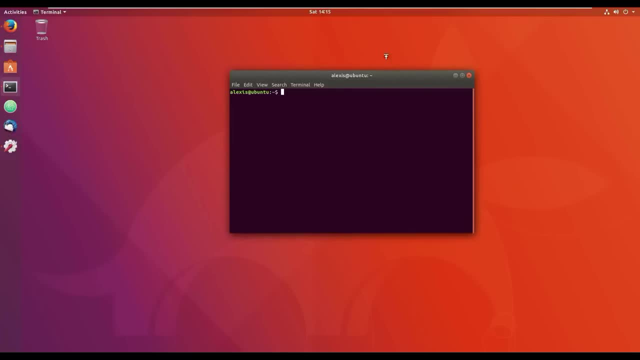 were going to be trying to communicate, but before we get started with communicating between the two, to start up net cat, we can use the NC. All right now. NC is the on. Linux is a bit of an older version. The new one is end cat. All right now. if I hit end cat is against, it's gonna tell me it's not. 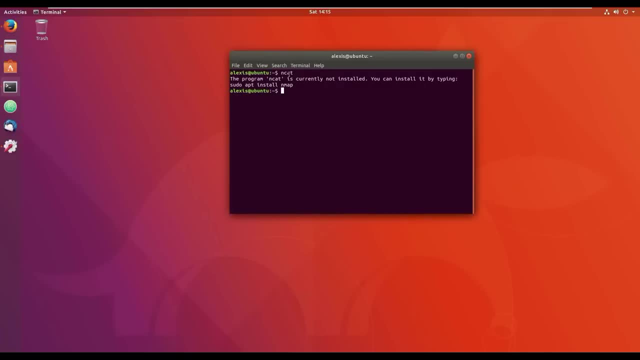 installed, So it's going to give us a bit of an error there, But don't worry about that. Now, if I hit an NC which is net cat and I use the help it's going to give us the. let me just do that. 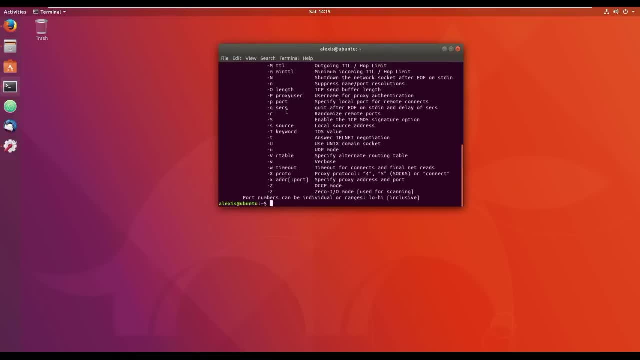 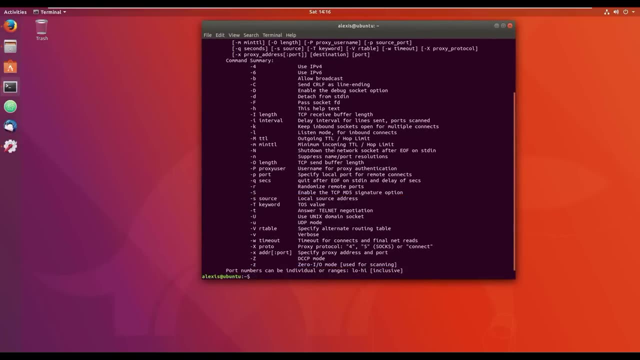 Again, I think it's believe it's help. Alright, there we are. So it's going to give us the information about how to use net cat, And this is very, very useful information. One of the most important commands we're going to be using is the verbose option, right here. 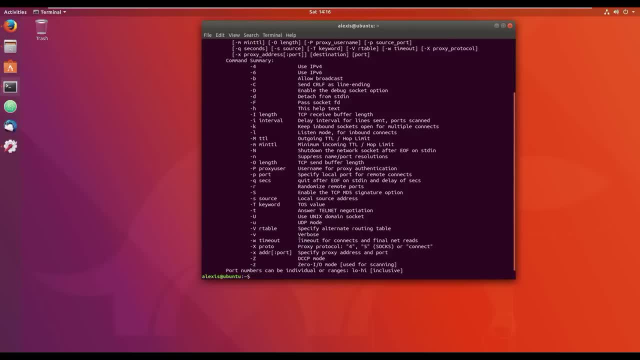 There are a lot of these commands that we're going to be using the verbose option right here. the allows us to verbose output. again, I know what the V stands for. again we can be listening. we'll be using the L port quite a lot to listen for inbound connections, and the we're going to be also using 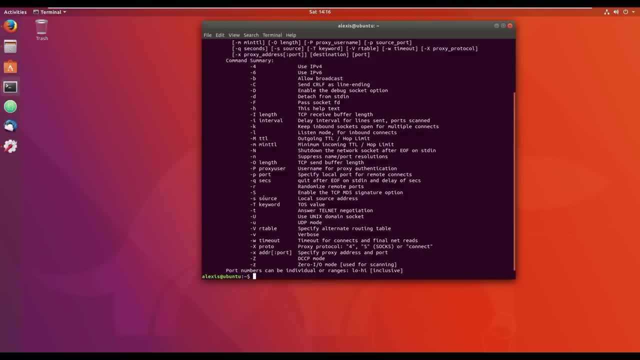 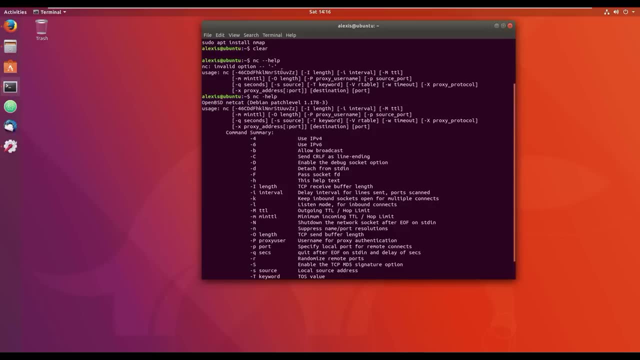 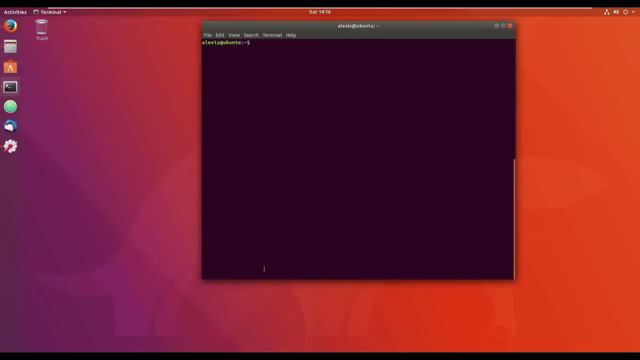 the P for the specifying a specific port right here. so essentially you can just use the help command right here and that'll give you a good information about netcat and how to use it. but I'll be explaining this as we go. so the first thing we want to do now is- or I want to do, is I: 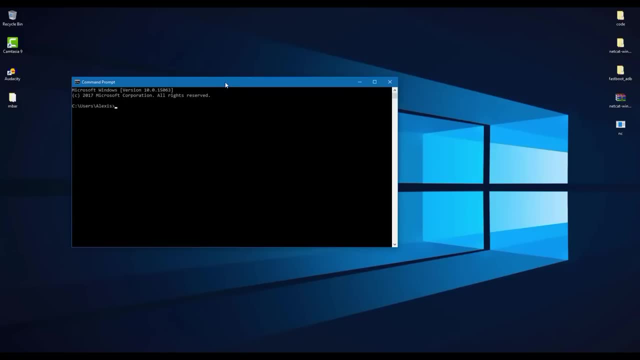 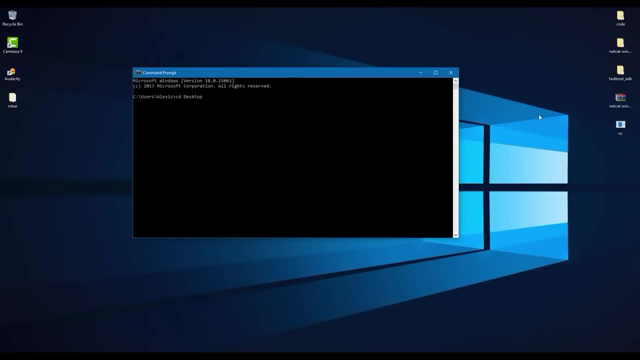 want to just open my command prompt, because this is how you have to initiate netcat, and I'm just gonna browse to where I have the netcat executable stored, which is on my desktop. alright, so once I'm on my desktop, all I have to do is just NC and I'm going to be using the options or the commands now. 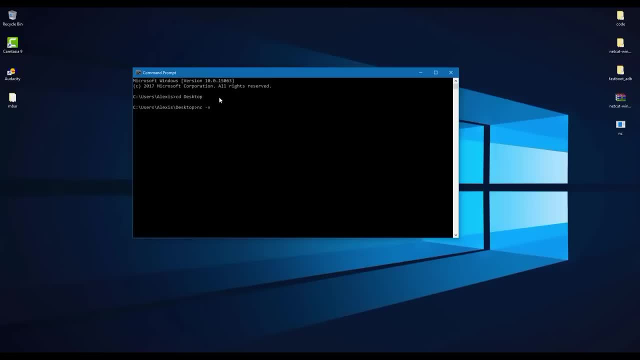 so I'm gonna say V for verbose L to listen, and you the port. of course, those are these just the options that I'm going to be using and I'm just going to listen on a random port, like you know, like something like 1200, I know that's, that's. 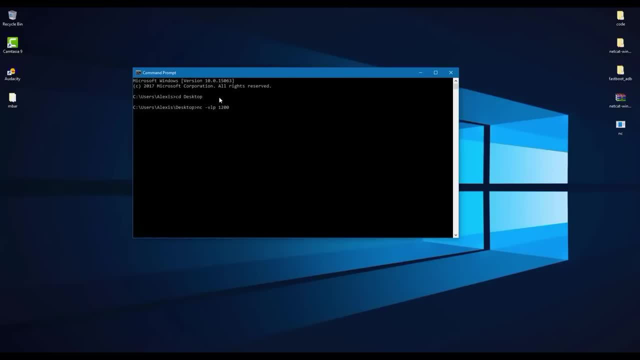 just weird using a random port, but we can just go ahead and use it. or we can use the 1337 ports, but essentially, if I do this, it's going to listen on port 1200. now, what I can do now is I can get the. 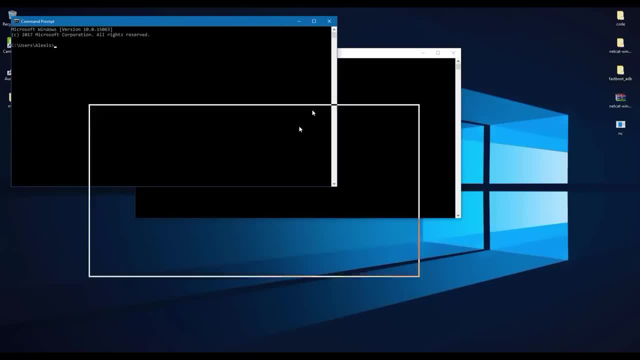 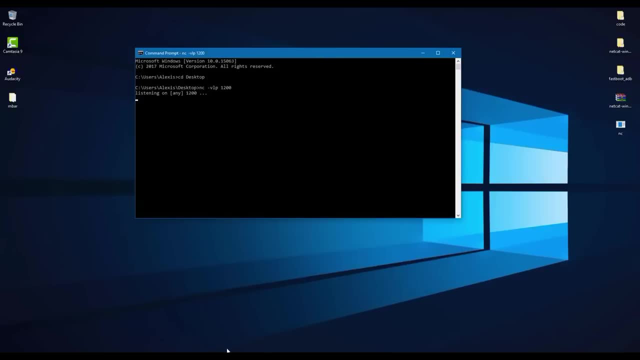 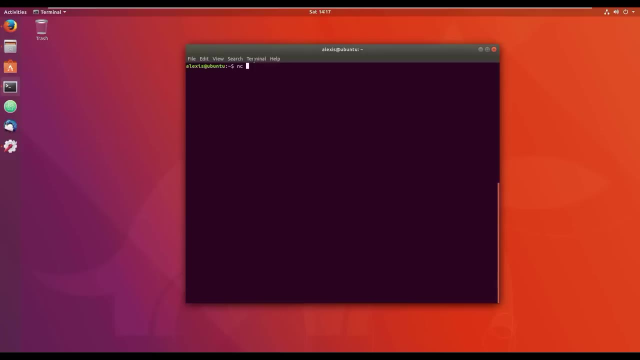 this Windows machine, uh, the local IP address. so that can be done by going to ipconfig and looking up your adapter. now, I already have the IP, I already know what it is, so we can go back into Linux and, uh, essentially what I can do now is just hit NC, um and see, and then, obviously now, since we're 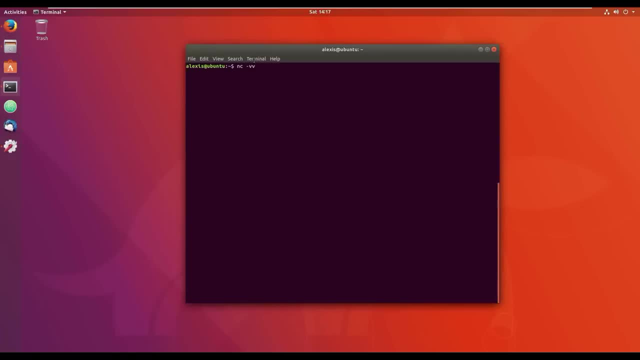 connecting with you can just verbose the output, all right, so it basically displaying the connection and whatever we're doing and the IP, which is 192.168.0.111, and the port is 1200. all right, that's how we specify it. so if I hit enter, it's going to say connection to 182.168.0.111 on port. 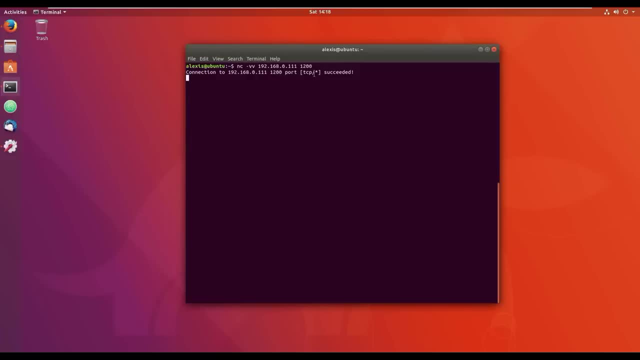 1200 is uh succeeded, so it's using TCP. it can also use UDP. but uh, let's look at what's going on here now. the first thing you can realize is because we have not initiated a reverse shell. we can actually just communicate directly to these machines, and let me show you. so let's say: 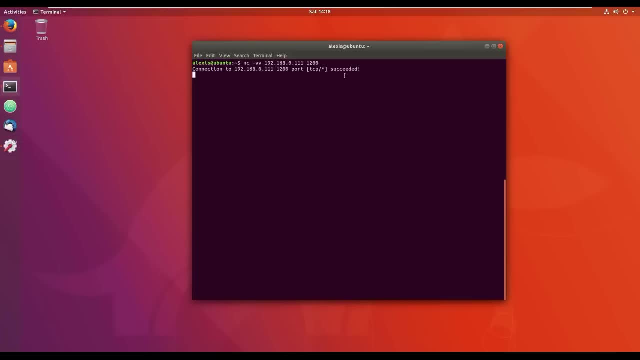 if I type something here, like I can type a message saying: hello, this is a test, um, this is a test message, all right, something like that. and if I hit enter and you, it's not going to display anything here because, uh, we have, we have essentially connected to the Windows machine, but if we go back, 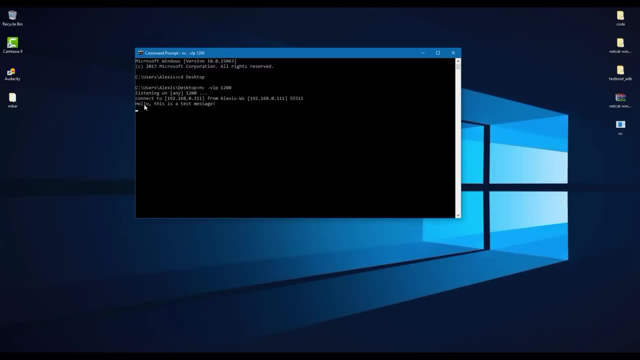 to the Windows machine, you can see it's going to say: hello, this is a test message, so that's pretty, pretty awesome. and you can see the message and you can essentially just communicate back and forth. so you can say: this is the, this is a message, or I can just say hello, it's me all right. and if we go back into the Linux, 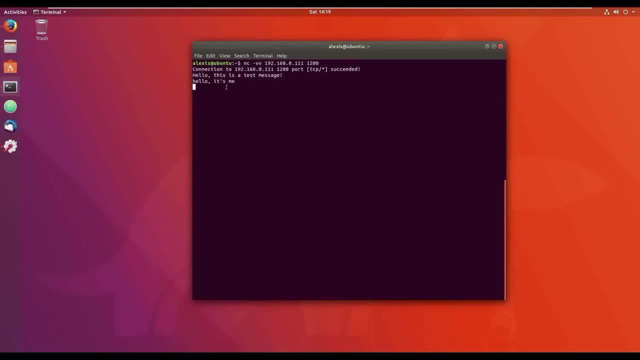 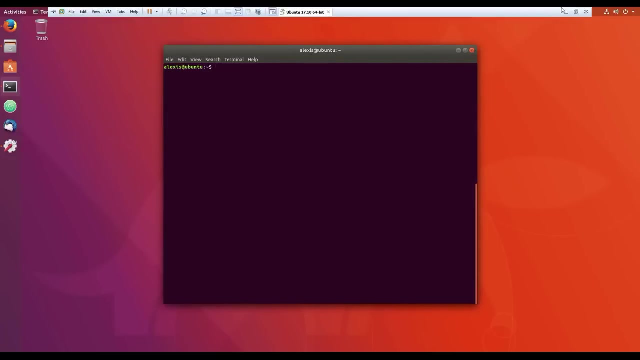 machine. you can see it's going to say: hello, it's me. uh, now, the most important thing now, obviously, is to initiate a reverse shell. so let's actually go ahead and do that. so I'm just going to clear this out. uh, disconnect, so I'm going to stop and, uh, the first we're going to be trying to, essentially, 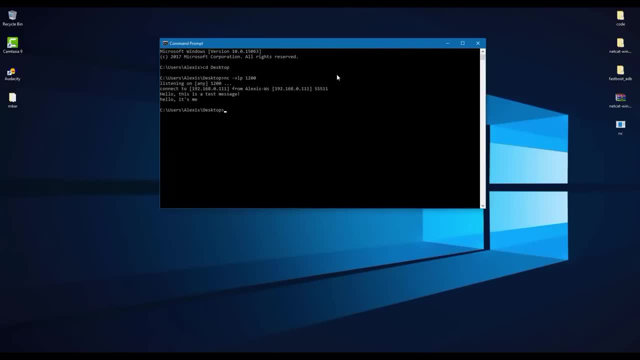 get a reverse shell to the Windows machine. so what we can do now is we can on the Windows machine is we can just say NC. so again, vlplisten to this port or on this port. sorry, and we specify our port here and now. before we, I just want to say you can also use the help command right here. all right, so as simple as. 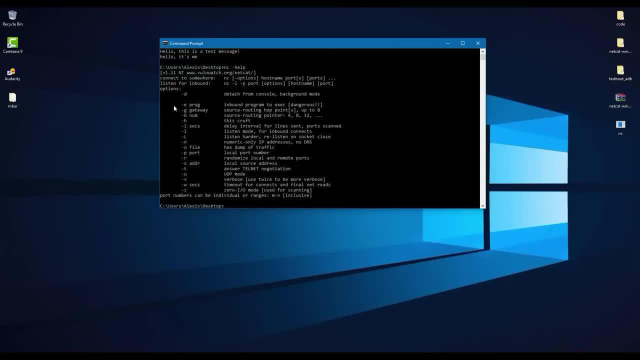 that. and one more thing we're going to be using is we're going to be using the e command, which allows us to invoke a program. all right, so it allow, as you, as you can see, the the what it's written here, the documentation here is it saying: in inbound program to execute. so this will allow. 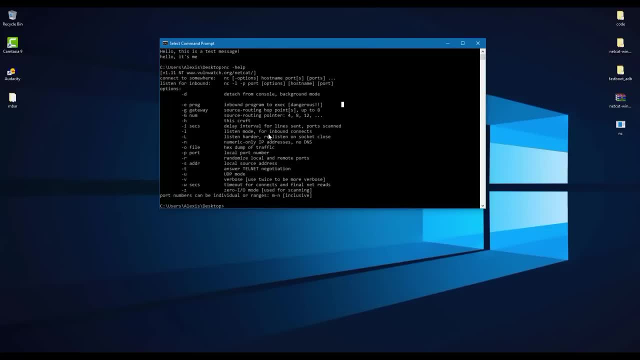 us to, in both cases, either, you know, execute a program on both sides. so in this case we're going to be trying to invoke a reverse shell. in this case, we're going to be trying to invoke CMD. when we reverse it, or when we switch it to Linux, we're going to be trying to invoke the. 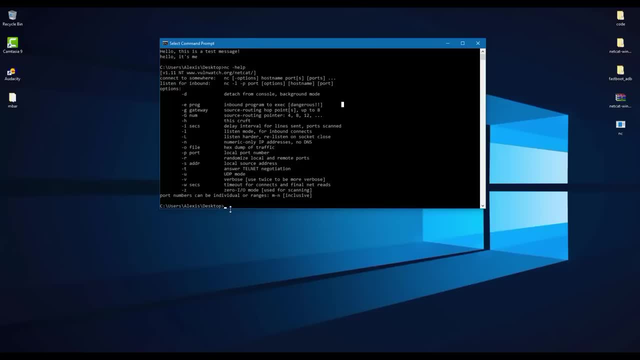 shell, but for now we're just going to be invoking CMD. so NC, VLP, something as simple as that, and our port. you can specify any open port again. that choice is yours and we're going to be using the e option to invoke a program, in this case CMD. 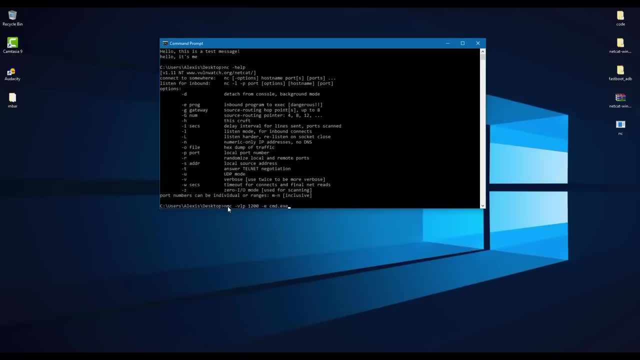 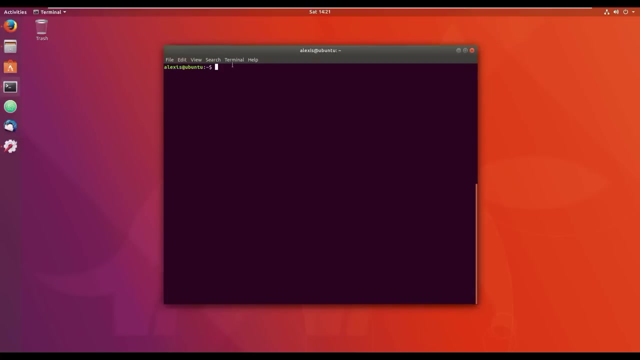 dot exe so you can actually see how robust this is. so once we hit enter: oops, I made a mistake there. sorry about that. I always seem to make really annoying mistakes. all right, there we are. so it's listening on that port now. if we go back to Linux, back here and now, essentially we 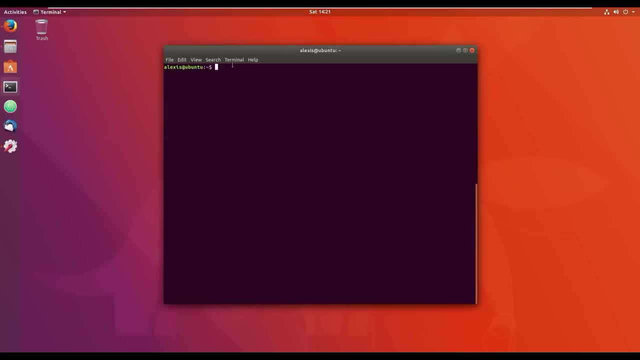 are with. the Windows machine is listening for a connection, and now all we have to do is connect and we'll be able to use the command prompt, because we have initiated a reverse shell. so what we're going to be doing is we're going to be using the command prompt and we're going to 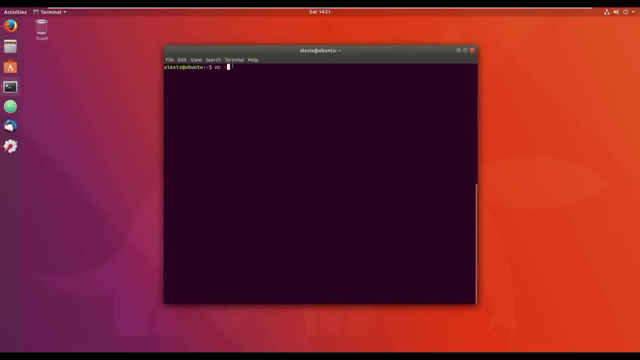 see what it says here that the CMD � words of잖아 so we're going to be using this command prompt São Paulo for that first time and we're going to be using it so we'm going to use this command prompt format there so as soon as Microsoft going to be eliminating guard and let's say I need Canadians 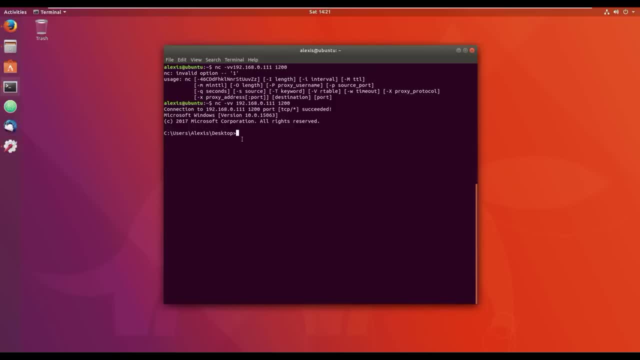 for me, you can really really understand the power of this. and again, we can just run a plethora of stuff we can find. we can see the directories on my desktop, as you can see. we have a bunch of folders there. you can, again, you can create a folder. so test, let's create a test folder, test, and if we 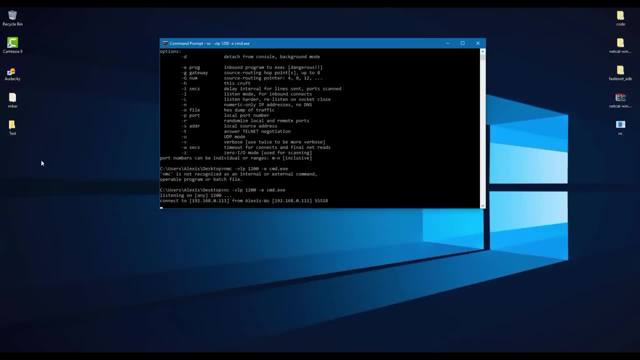 go back there. as you can see, we it did create a test folder, so really this is awesome and it's much, much faster than using secure shell. but again, as i said, secure shell is more, is much more of a popular tool when communicating between linux and you know, your linux servers, etc. etc. 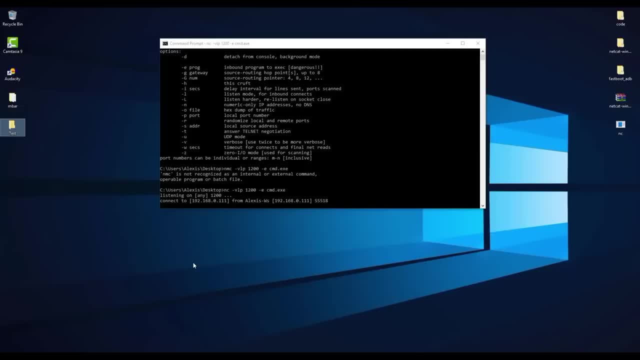 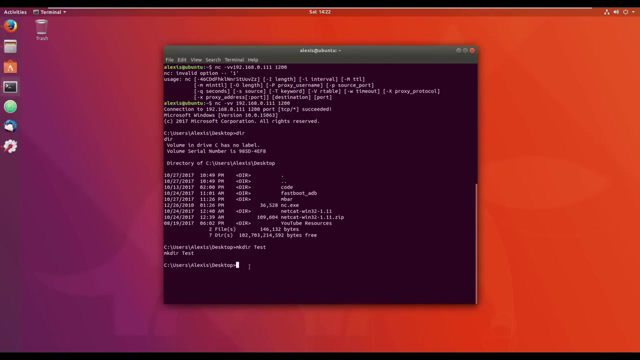 you know, for example, the clients that you have on windows to connect to ssh or or using ssh, are like programs like putty. but that's besides the point now again, where you we've basically invoked a reverse shell on the windows machine so we can run a lot of stuff. uh, but now let's. 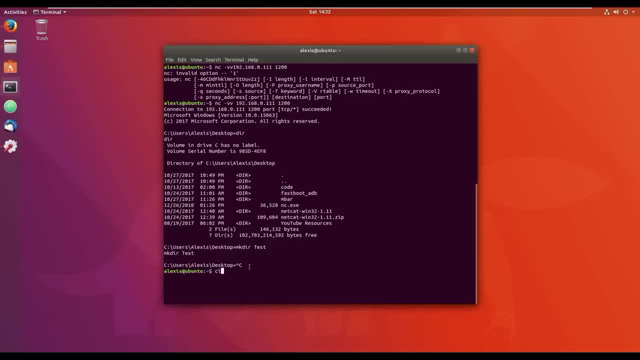 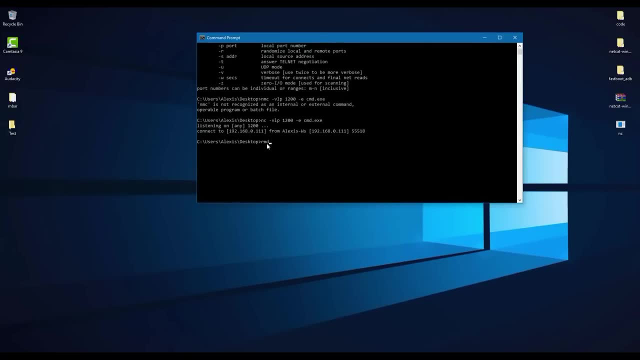 go back to our desktop and we can run a lot of stuff. but now let's run a lot of stuff, but now let's try and do it in the opposite way. so i'm gonna clear this and again: uh, on the windows machine it should have told us that, uh, let me just get rid of this, um, like so, and got rid of that folder. 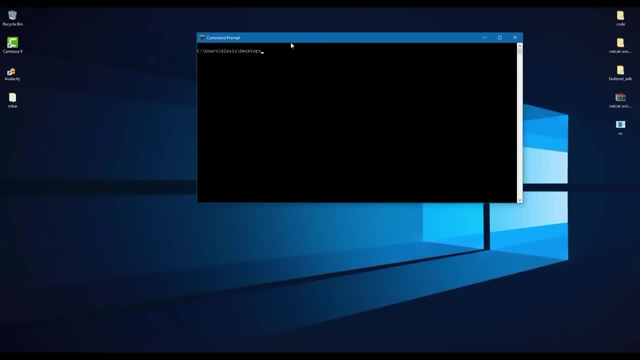 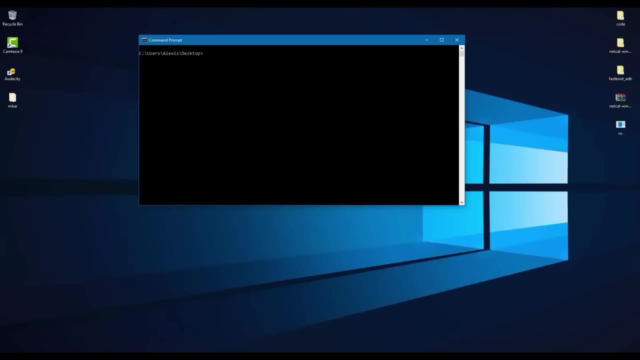 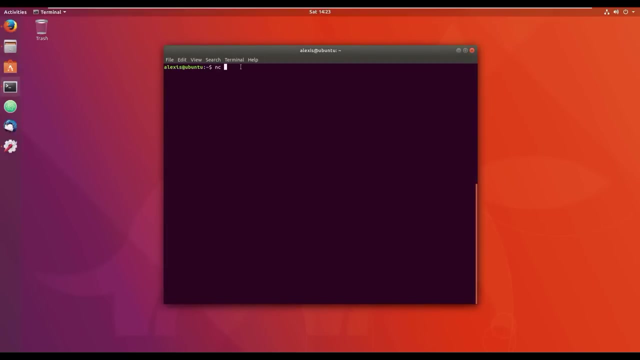 let me clear this out now. we essentially have to invoke a reverse shell on linux. so, on linux, essentially, we're just reversing the process. so what we're going to do is we're going to say nc, and through nc, we're going to say e, all right. now we're invoking, all right. so what we do is: 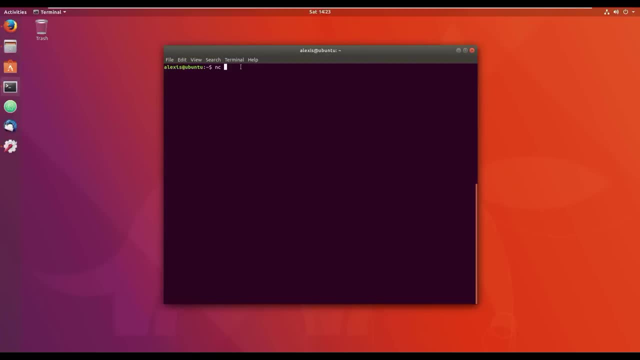 we say nc and e and we're going to say bin, all right, so bin, ssh, i believe, uh, or actually am i using the correct syntax here? nc, uh. let me try the first way which i remember quite uh, i remember quite honestly, which is vlp, because we are listening now on a port, obviously. 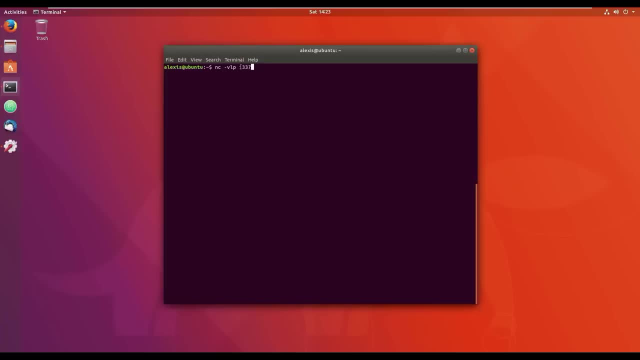 uh 1337 if we just reverse the process or we can use the 1200 port and we use the e to invoke uh. now we're using the shell, so bin uh, sh, right, right, enter uh, invalid option e. hmm, that's weird. n cats. what if i use the newer version of n cat? would that help? now that would essentially mean i: 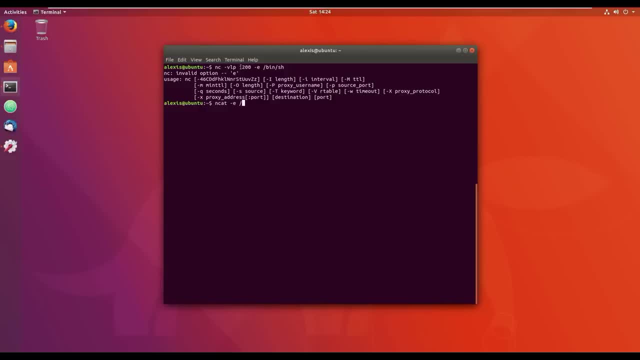 change the syntax slightly and i use the bin sh and i specify the port again. so 1200 and ncat is not installed. uh, oh yeah, i have to actually install the nmap. so this is another thing i wanted to ensure to show you guys. uh is essentially um, let me just 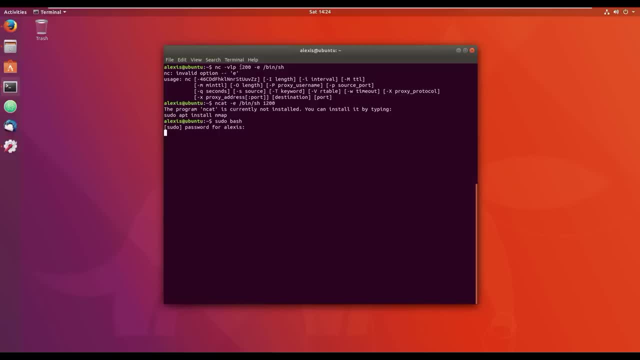 get that password entered, uh, with uh linux, initiating a reverse shell or allowing windows to connect to linux? uh, in this you know, in really a sim, in a simplified form of understanding. what that means is that we'll have to use the latest version of netcat on linux because, again, that 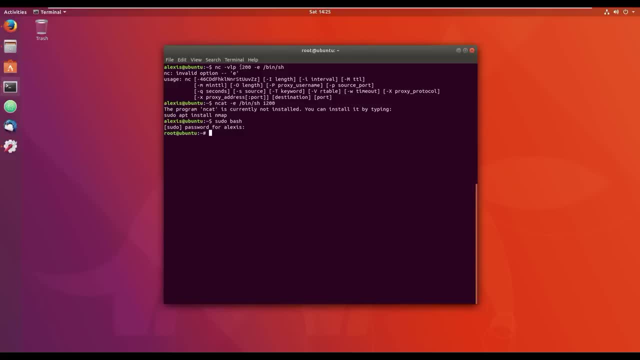 gives us a whole new set of features like uh, you know, using ssh, etc. etc. so what i have to do is just install uh nmap, because i haven't installed that yet on this virtual machine and that could take a while, depending on the download and download process, but i'm going to do that now. 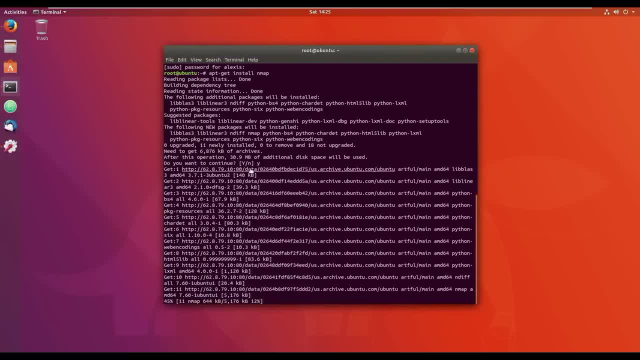 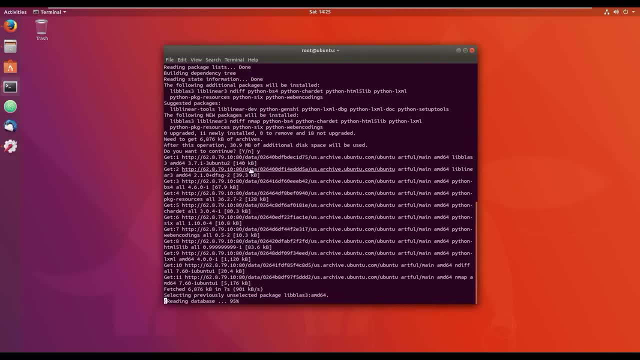 so let's uh actually uh, open up the dotnet app and let's begin. uh, yes, i, uh, i can just add a nasaf anders, my AFK, a nasaf Fei, teams communication coconuts. you could add facebook nut abez if you'd like, but why in the world don't you think that would be better? uh, 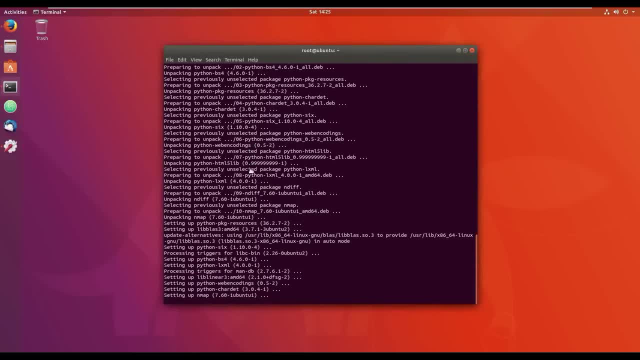 this is pre-installed and again, like i was telling you, one of the advantages of using in thebrow from: uh for my make я не дау. Beginning on the internet, right anger is� ا ا آه. It is nothing to do with the Internet connection, because 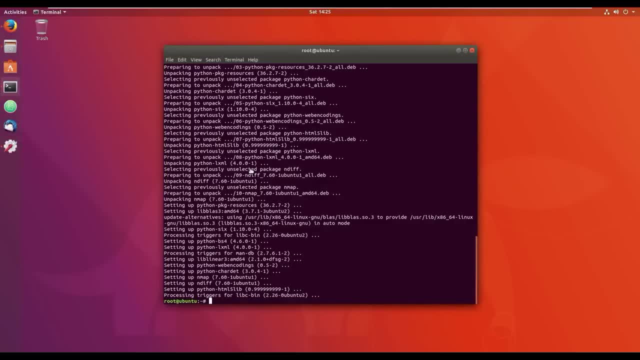 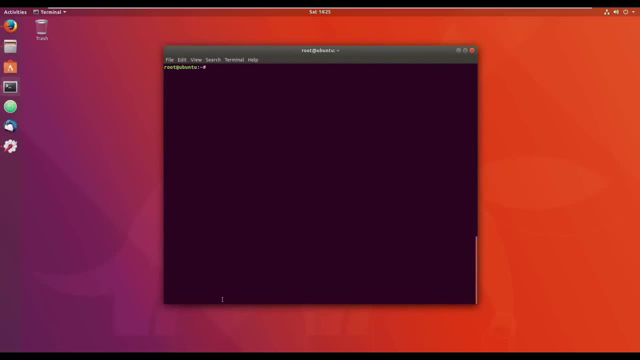 uh, it** is not going to last forever, both sides. now. what I mean by this is: let me just clear this up and let me just show you that it does work now. so what I can do is just say: and kept E, because we're invoking the shell and sh. 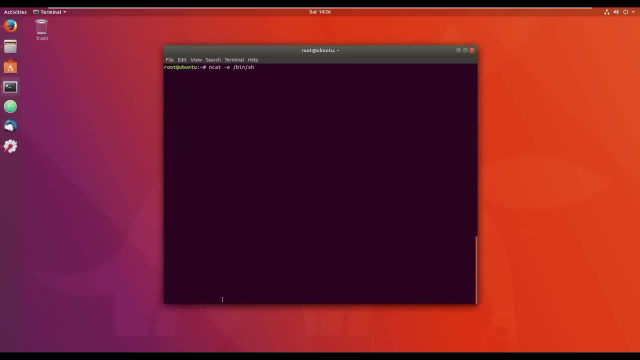 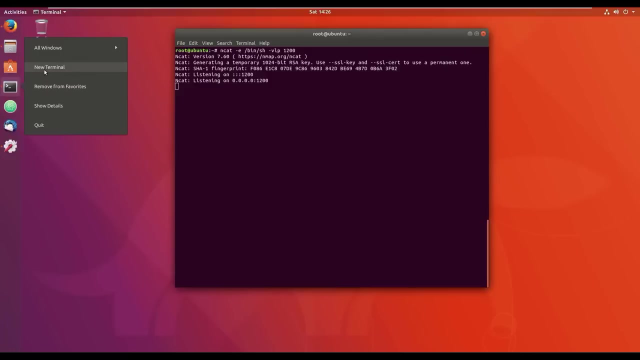 like: so VLP and 1 1200, right there we are. so, as you can see, it's gonna say listening, and now what we can do is: whoops, I forgot. I forgot to get the IP address here, so let me just get that right now. 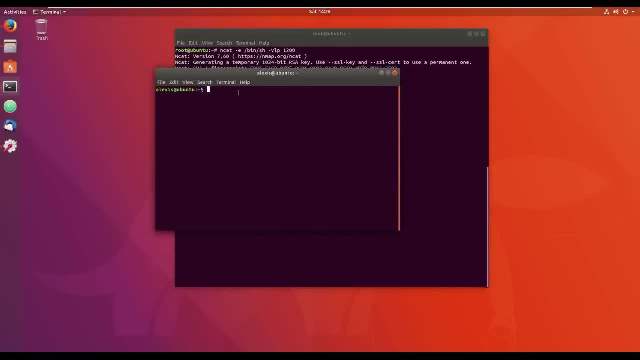 the local IP address. so I have config like. so we're using my Ethernet, which is the virtual machine, and if I just get it right now, there we are. we're using the do 168, 2.1, 28. all right, let me just try and connect back to the server and let's see what we can do here. so let me just 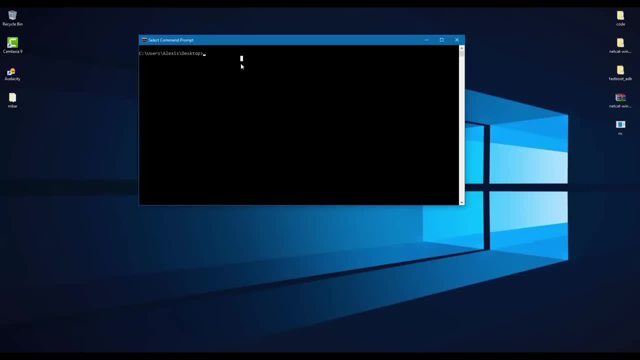 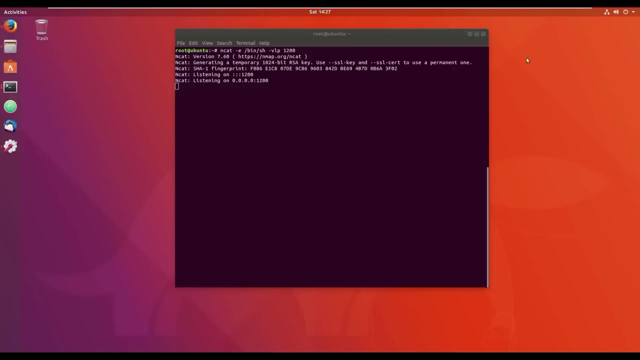 go back now and now through net cat on Windows we essentially just think verbose and 168 point 2.1, 28 I believe, was the IP address and the port is 1200 and hopefully it allows us to connect and let's see if we got we established connection. there we are. we did get a connection and let me 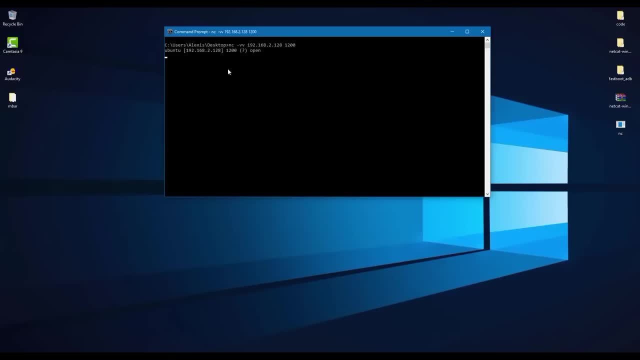 just see whether we can do it there we are going to. we have got connection, so let's try and run something like: who am I and, as you can see, who you root? so you name some simple, some simple bash commands and again we can list all the files on the desktops or CD desktop. again, we can now navigate and we have 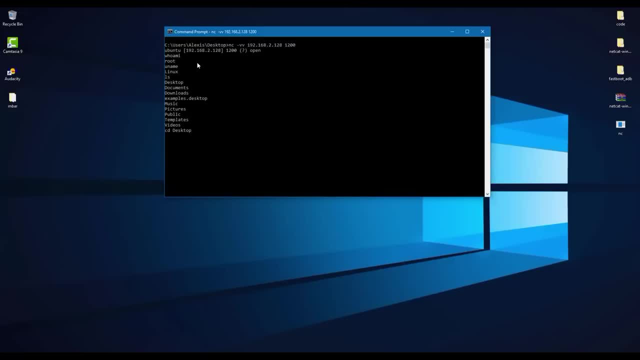 this. we have correctly initiated a reverse shell: LS- nothing on the desktop. so LS whoops and I see L, nothing else. so, yeah, that's pretty much it guys. there's a lot to cover with net cat and I'll be making other videos regarding this, but I just wanted to give you guys an overview. 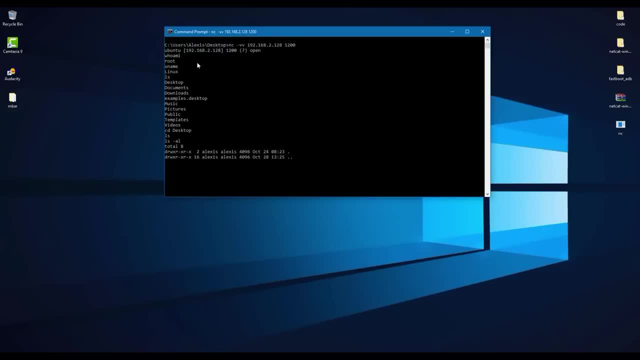 of how to use net cat because, again, it is really really useful and you will find yourself using it quite a lot when trying to initiate connections with multiple computers, whether on the same network or, you know, using the real IP addresses and connecting to them remotely. again, my 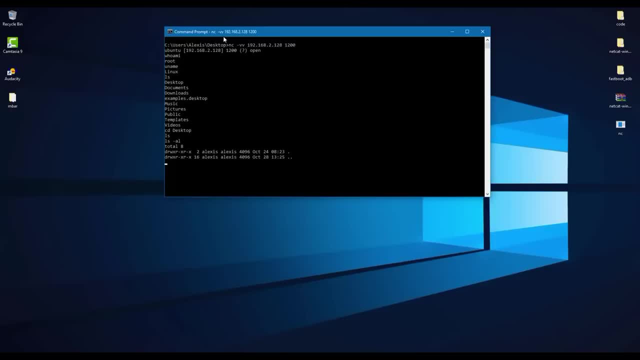 people will complain or say that SSH is much better, and that's true it is, but SSH is really a much more of an exclusive tool, while net cat is more robust in terms of the functions it can perform and the reverse shell connections that you can perform, and is much more suited I would 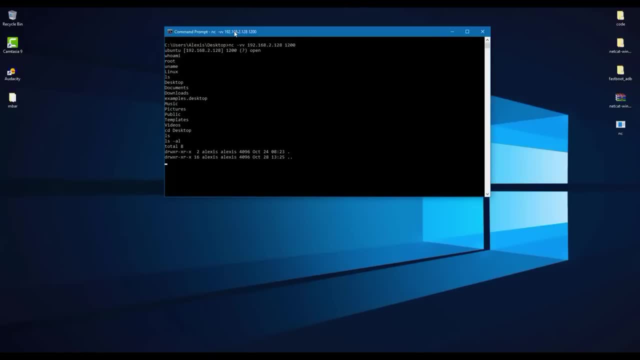 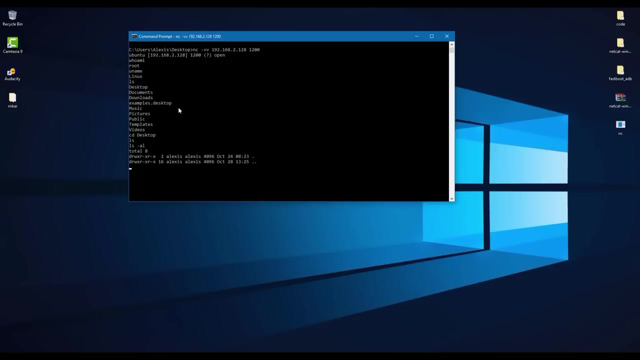 say, for an ethical hacker. I would really, really encourage you to learn how to use net cat because, again, it allows you to listen on ports. and again, if, if I was monitoring traffic, if I just initiated a connection between and I was listening on a specific port, like, let's say, on the TCP ports, I 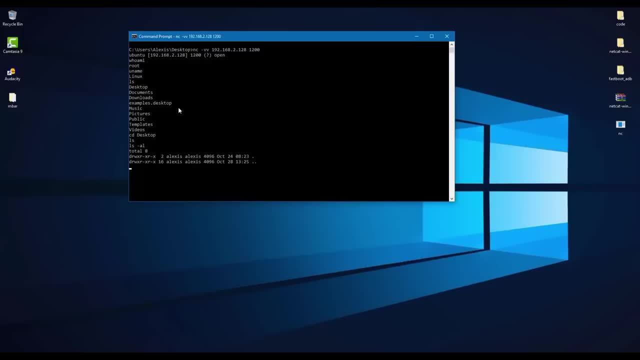 could actually open up wireshark and monitor the packets that are being, that are incoming and outgoing uh, either TCP or whatever the type of port we're listening through. again, as I said, it's a very, very advanced tool that can perform a lot more functions that have just then, uh, that I've 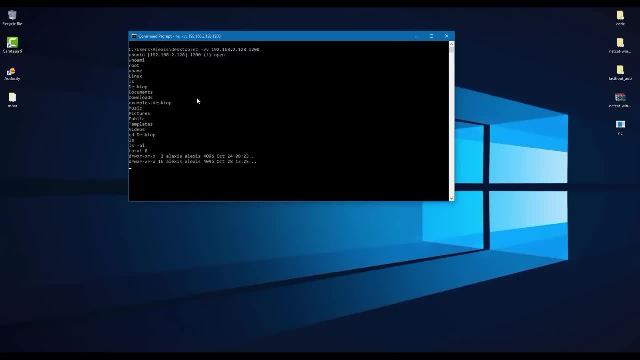 showed more than I've shown you today, but we'll be getting to them as we move along. now we'll be moving from uh Python or into the C++ uh series. we'll be actually creating an advanced key logger, which will be really, really awesome. so I hope you guys excited and we'll be moving a bit into more of an advanced section of 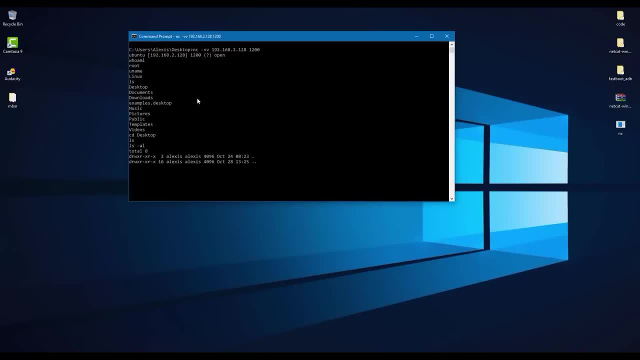 hacking now. anyway, guys, that's basically it for this video. if you like this video, found value in it. please leave a like down below. if you have any questions or suggestions, leave them in the comment section down below, or if you have any personal questions, you can hit me up on my social networks. 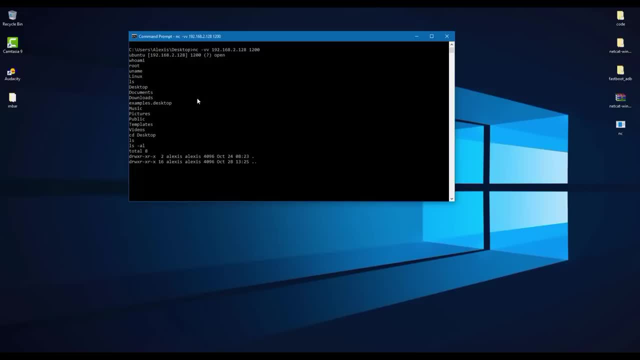 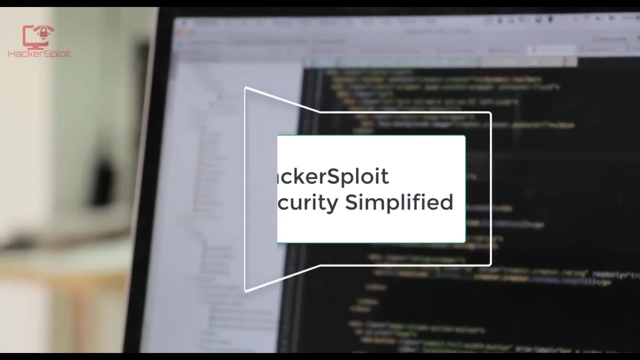 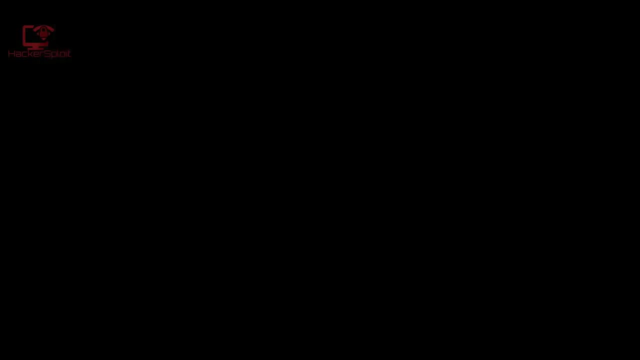 or you can hit me up on kick. uh, you can check out my website for the latest hacking news and resources. and yeah, thank you so much for watching, guys. I hope you had a fantastic day and still have a fantastic day. peace, peace. hey guys, hackersplike here back again with another video and, yes, you can finally see my 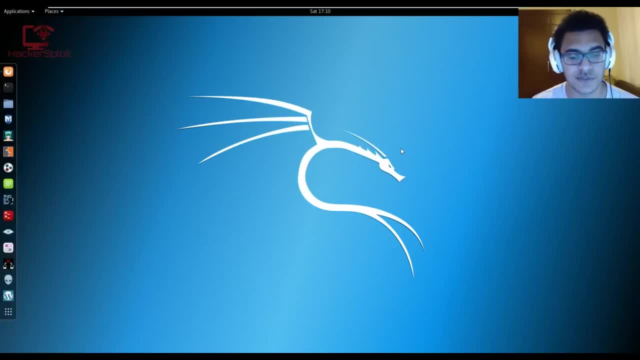 face now. uh, this is something I've been thinking about for a long time, um a long, long time, and it's finally here. so do let me know what you think, uh, whether you enjoy the videos like this with, um, obviously, with my facecam, uh, or you would like a full screen, um, you. 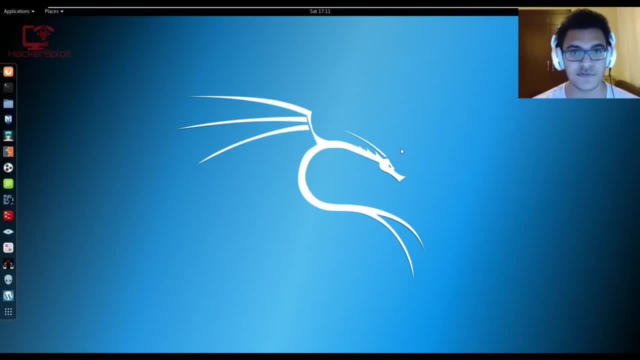 know, tutorial video. uh, just the way I usually do. then, all right, so let's get to today's video. so today's video is going to be about ARP poisoning or ARP spoofing, and essentially, uh, how to allow uh or redirect packets or, uh, you know, traffic to flow through our device. essentially, uh, you know. 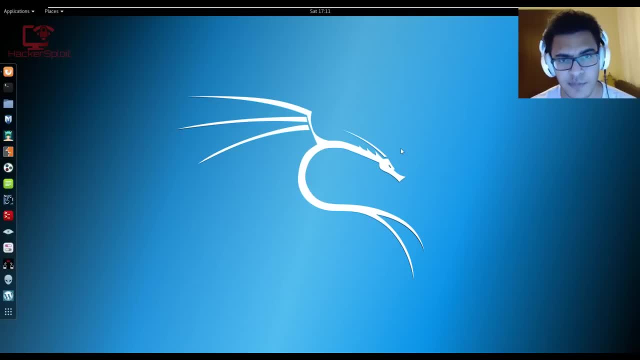 a man in the middle attack. but in this video we'll be focusing more on how ARP works and how ARP poisoning works all right. so you might be asking yourself: what is ARP? is this the first time you're hearing about it? if it is, ARP is essentially a network protocol and I believe it is in the OSI 2. 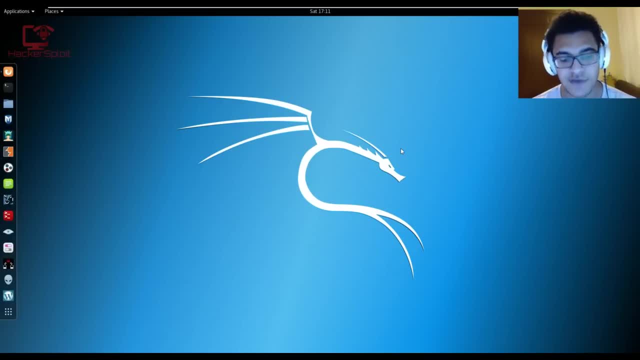 layer. so, essentially it, what it stands for, is an address resolution protocol, and its purpose is to resolve MAC addresses to IP addresses. all right, so, uh, when it comes down to ARP spoofing, what happens is: uh, what we are going to be doing is, and the concept behind the ARP spoofing is that you're going to send an ARP response to a client, all. 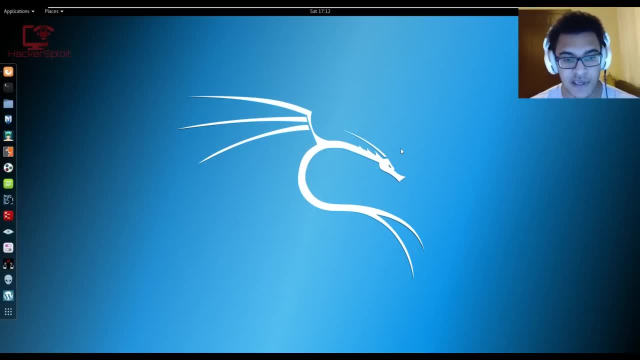 right. so a client on the network, you're, you being the attacker, all right, saying I am the router, all right, and then telling the client, uh, that the device with the router IP address has my MAC router, and there's the router and you have the client that you want to target, obviously through. 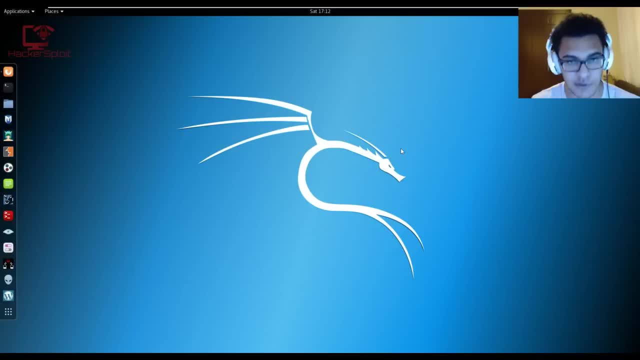 the IP address and obviously this is done locally, obviously because it's on a network, right? so you, you are essentially telling the client, you're connecting to the client with the router's IP address, right? so you're connecting to the client with the router's IP address, which is the default. 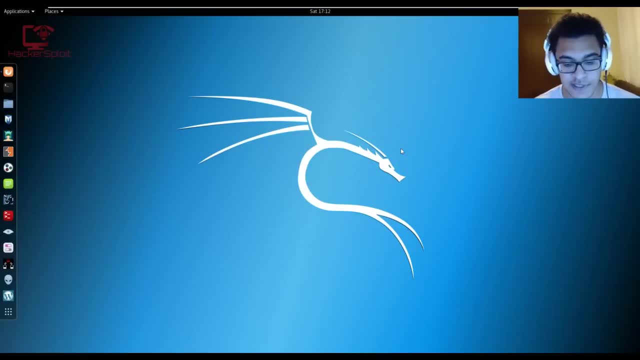 Gateway address and you're telling um. you're essentially telling the client that I am the router and you should pass your traffic through me, right? so you're standing in between the client and the router and obviously you've tricked the client uh by telling uh, by obviously using the router's IP address, but your but the MAC address. 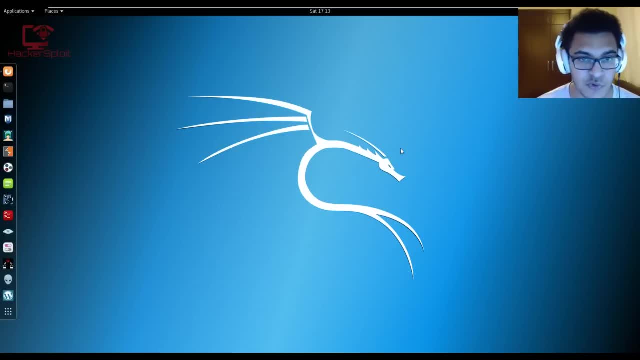 will be your MAC address and you're exploiting the ARP protocol because the ARP protocol, any ARP response, will be trusted. so that's a very, very easy way of exploiting this technology or this protocol. so the tool we're going to be using is ARP spoof, or ARP spoof as it's commonly known as. 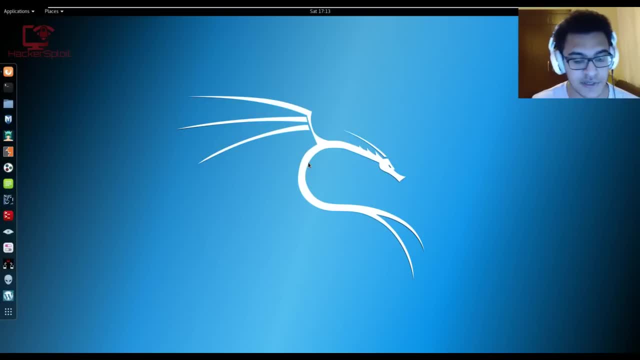 and it's a very, very powerful tool that will allow us to, um, to actually redirect traffic from clients to our device and you know, uh, from that point onwards, you can perform man-in-the-middle attacks and, you know, sniff the traffic, uh. so let's get started. so, uh, I'm on caledon next right now and 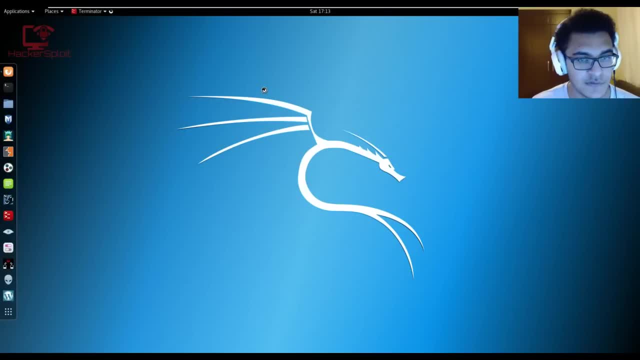 I'm just going to open up my Terminator because I find that this is a fantastic tool that is great for this purpose, and you'll see why. so what I'm going to do is- or actually, I would actually prefer, because I can enlarge the text here and we can have a good idea of what's going on in terms of: 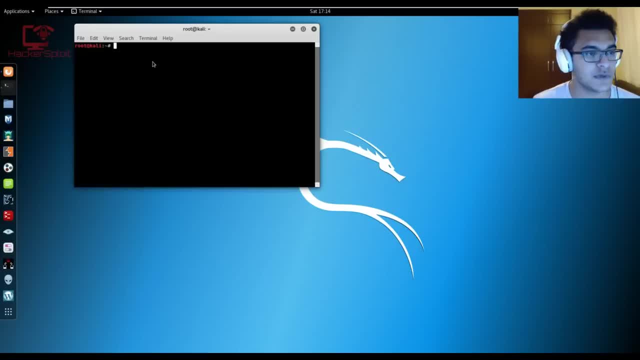 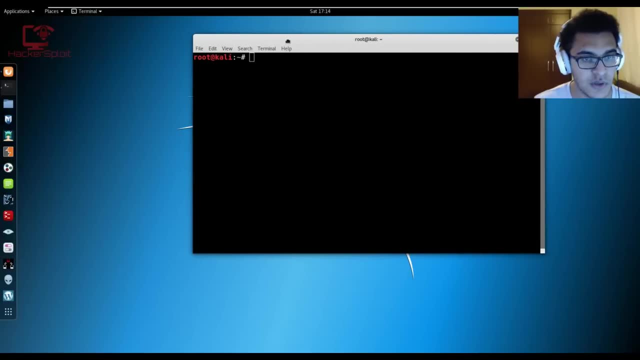 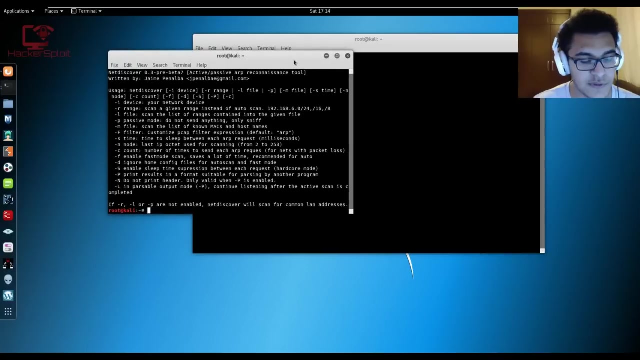 what's being printed out on the terminal, right? uh, so there we are- finally open up the terminal. that took a while for some reason, so I'm just going to zoom in now. what we need to do first is we need to use net discover. I'm going to be using net discover and you can use net discover to discover. 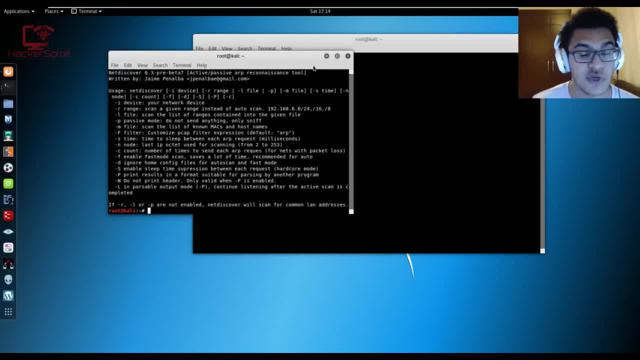 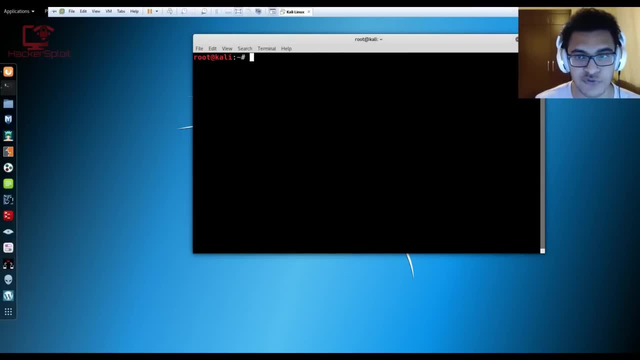 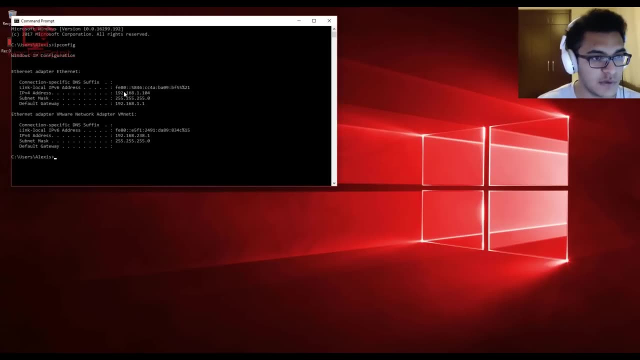 uh, the devices on your network or computers on the network that you want to perform the man-in-the-middle. so what does this mean? so, for example, I'm going to try and target my host operating system, which is right here, so I'm just going to check my IP config. there we are, and my local IP address is: 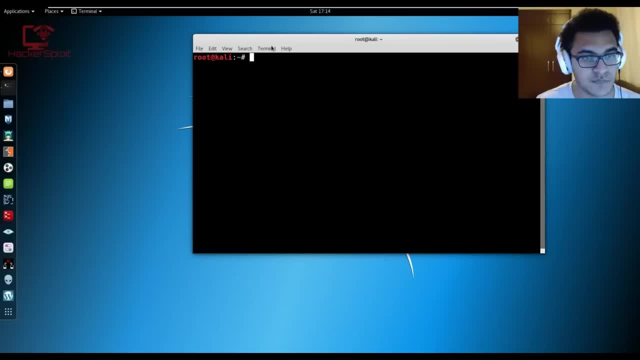 192.168.1.104. all right, so I'm back in caledon x and I've got the uh, the windows on my host operating system address and that's what I want to perform: the erp spoof on or erp poisoning on. so 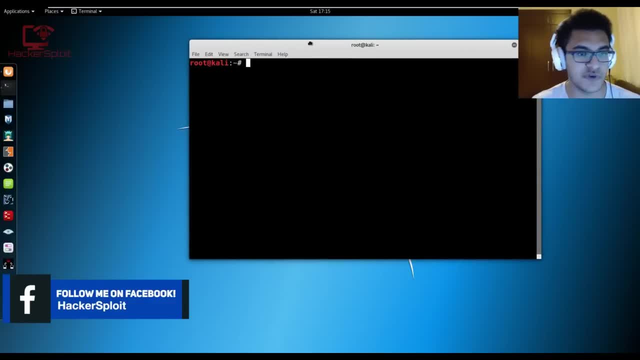 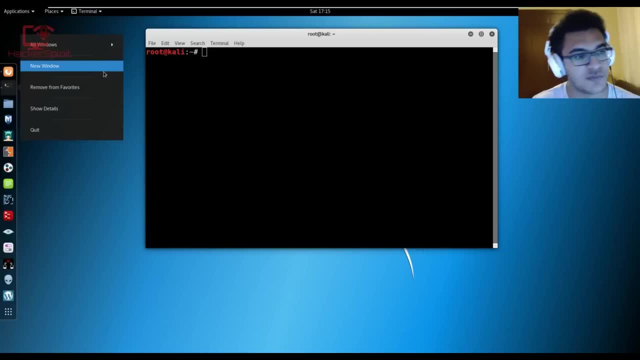 uh. since I already know what the IP address is, let me get started. so, to use the rp spoofing. it's uh, really, really easy. what I'm gonna do is I'm just going to open up two terminals because we're going to need to initialize erp. spoof uh twice. 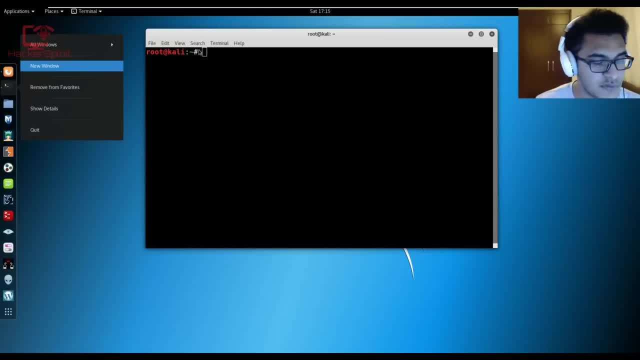 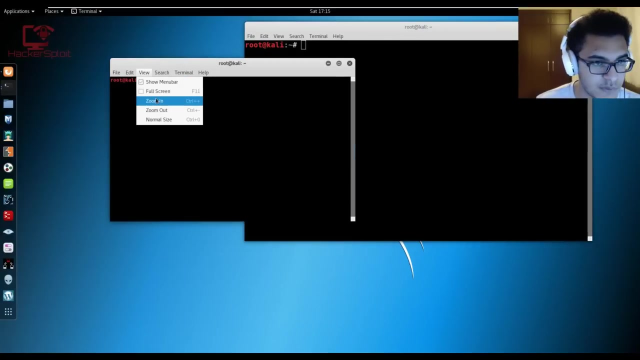 okay. so, uh, let me just open this up. for some reason that's taking really, really long to open. uh, I apologize for this freeze up. I should have actually opened this prior to this, uh, but anyway, uh, just give it a few seconds. oops, there we are. we have some kind of graphical glitch there all. 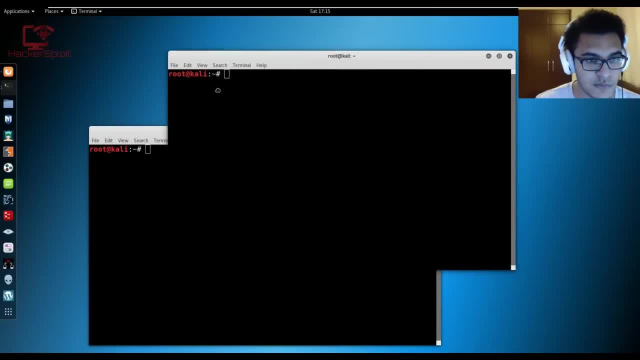 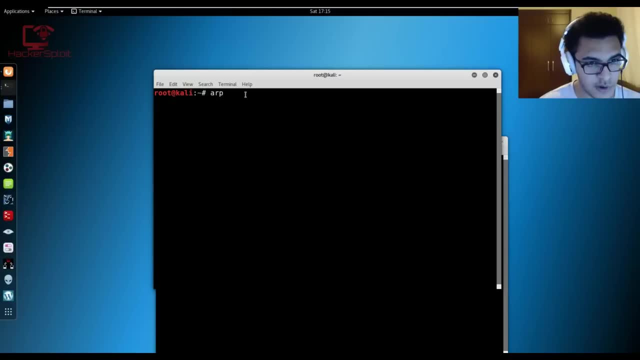 right now. let me just zoom in, okay, so we can get started now. uh, so what I'm going to do is, uh, to get started. it's really very simple. so we use the erp spoof command, or erp spoof, right now. the commands are very, very 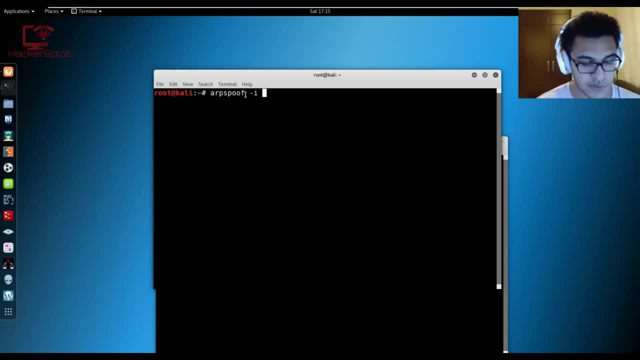 simple. we use I for interface, all right, so the I, uh. now, this is depending on you. if you're using a Wi-Fi card, you can choose your uh, your Wi-Fi device uh name, which is uh. if you're using a wireless adapter, it'll be lan0 or wlan0 and uh. since I'm using ethernet, I'm going to be using 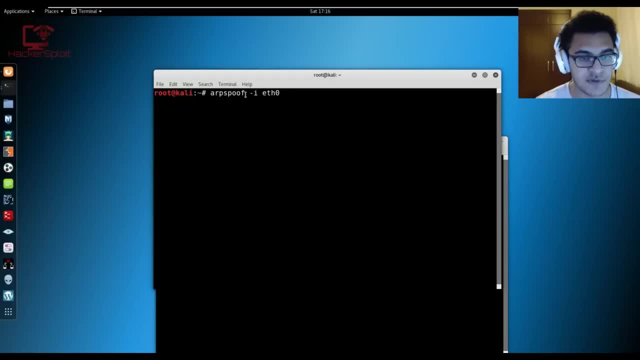 ethernet zero. so those are the default uh hardware names given or device names given to the different uh network adapters that you could be using. all right, the next thing is to use the t command, because this allows us to select the comma uh, the target. now it's very, very important that, since 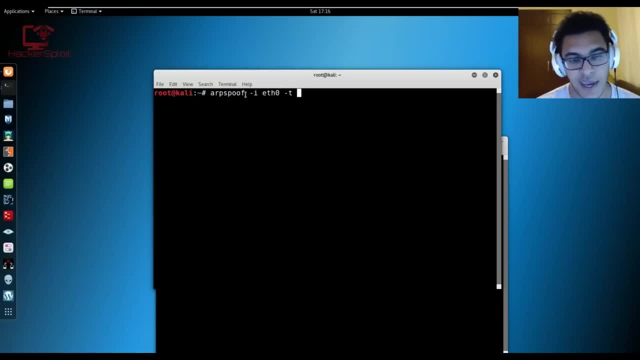 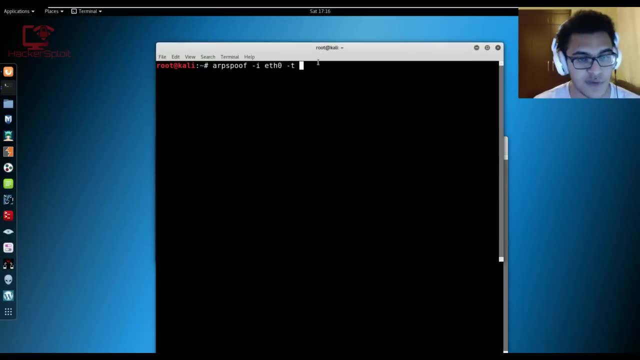 we're going to be running two instances of this because we are tricking both the router and the client that, uh, I am the router and I am the client, so, uh, you'll get the gist once we're moving along. all right, so in this instance we're going to specify the target IP first, so that is going. 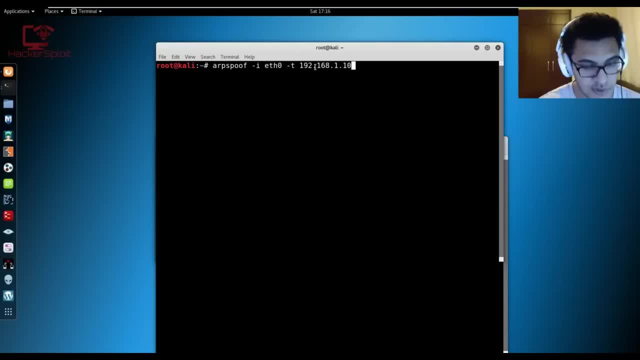 to be 192.168.1.106, okay, and then after that I'm going to target the default Gateway, which is my router's IP address, all right. so essentially what we're doing here is we're essentially targeting the um, the, your, the, your target, or the client in which you're trying to perform the spoof. 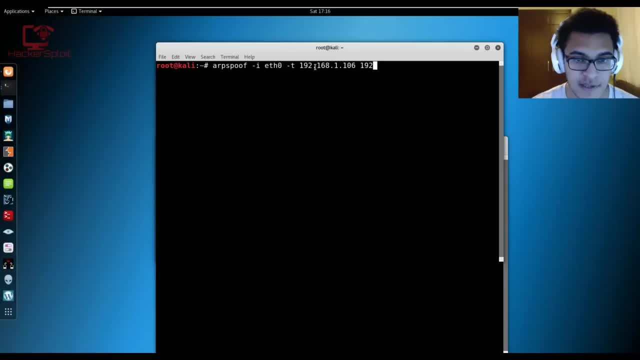 attack on erp spoof, attack on, and we're telling uh that client that we are the router because we're our Gateways IP address, right, so 168.1.1, all right, fantastic. uh, once we've hit, uh once this is good. uh, so essentially, let's look at the syntax again: erp spoof, uh, the your, your wireless adapter, or 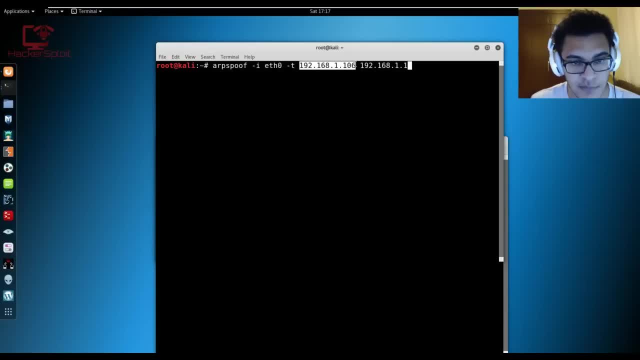 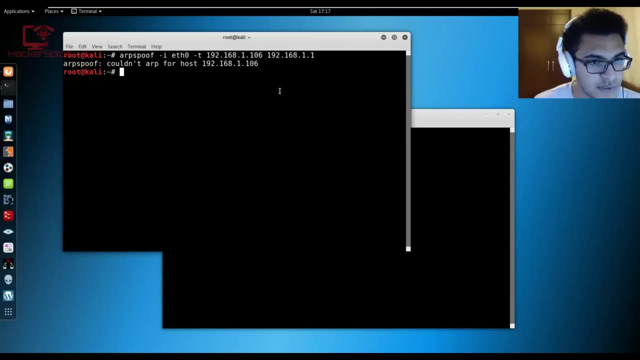 interface name and the target. but in this case we're using the target IP first and then the default Gateway IP after that, and I'm going to hit enter. oops, I'm going to hit enter and it's going to start. airpiece proof on that. and now for the next terminal. whoops, for some reason we couldn't. uh, oh yeah, I actually made. 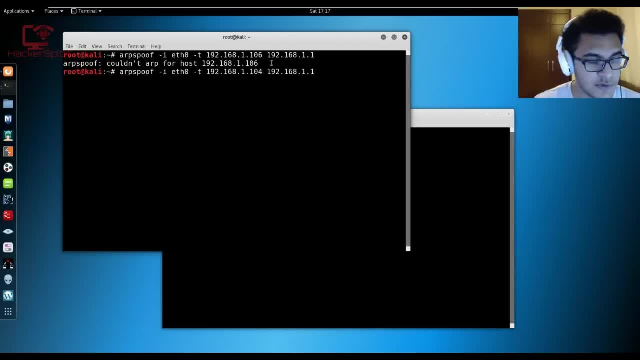 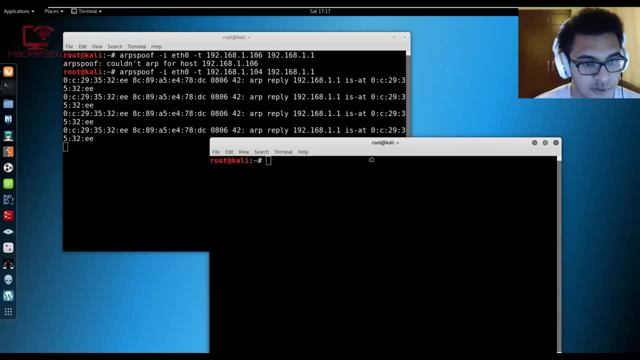 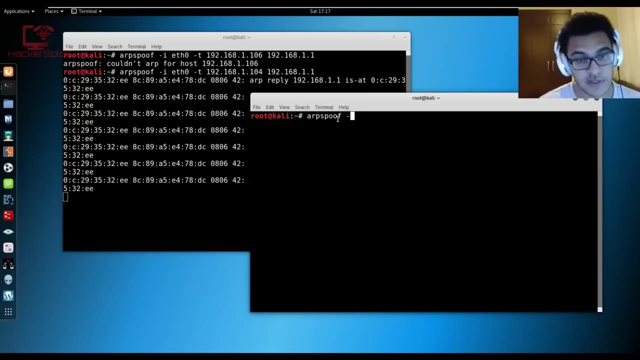 a mistake. the target IP is 104.. let me just try that again. there, we are fantastic. it's working now. so again, depending on what your target IP address is, you can specify that accordingly. now on the next one: erp spoof again. uh, erp spoof, uh. the interface, uh. LAN zero, uh, oops, Ethernet zero for me. 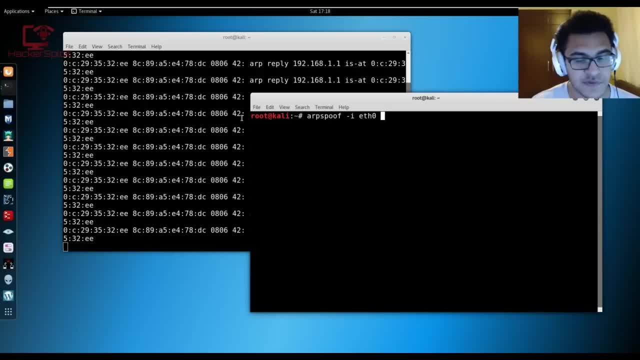 is doing. that really doesn't matter because again it's just sending the requests to the client saying that I'm the router. so we haven't completed the erp spoof uh attack just yet. so now we specify the target, but in this case now we're telling the router that I am that client. I am 192.168.1.104. 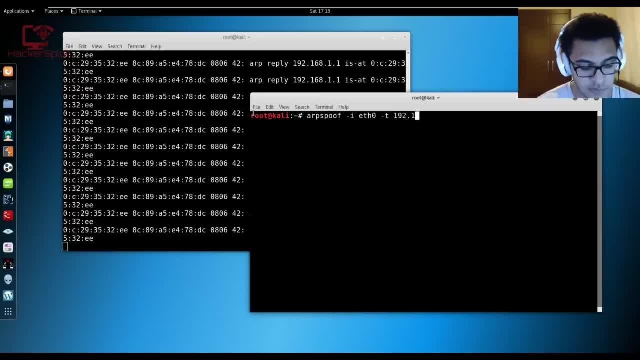 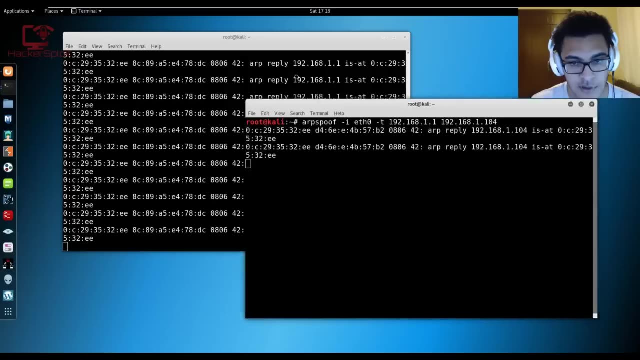 all right. so we use the, the default Gateway, or the router's IP 168.1.1, then we specify the targets IP, so 192.168.1.104.. and once that's done, we just hit enter and it's gonna complete the erp. uh, the airpiece spoofing. 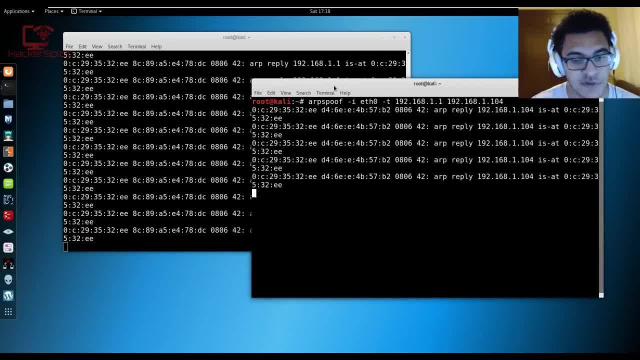 and now essentially all the traffic is going to be passing through us and now you can start using tools like wireshark to analyze or to sniff the traffic. or you can use dsniff, which is part of erp spoof, or actually erp spoof is part of the dsniff package. so if I open up a new terminal, 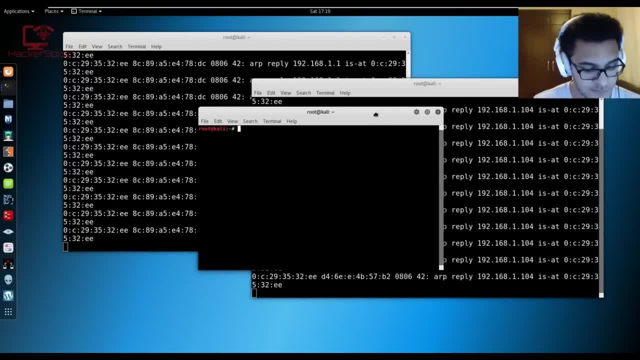 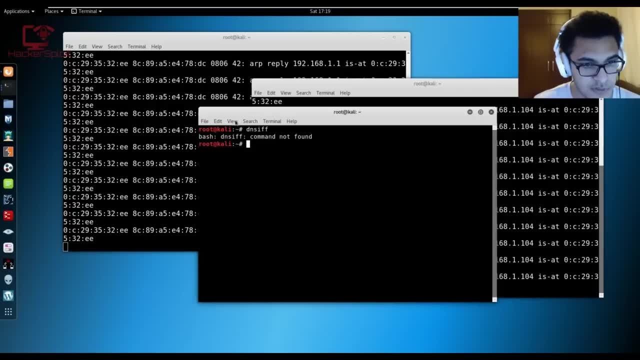 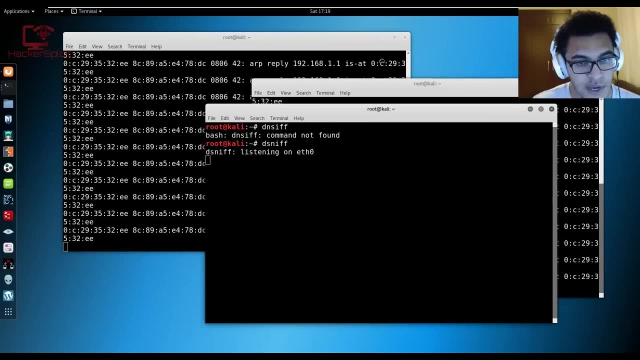 here. let me just see if it I can open that up. so dsniff, uh. if I just hit dsniff, whoops, uh. let me just uh increase the the font size here. so dsniff, right. so if I open up dsniff, it's going to start listening on ethernet zero and it's going to. 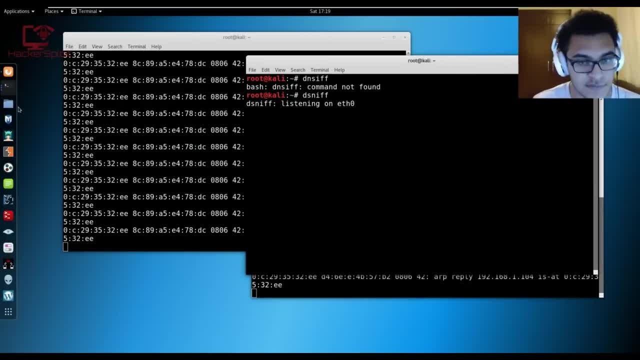 save the files, or the sniffed files that it's got from that- uh, from the client that you're performing the rp spoof on, and it'll save it in the home folder where you can find the log file for dsniff, and essentially what you can do now is open up a- you know, a traffic analyzing tool like 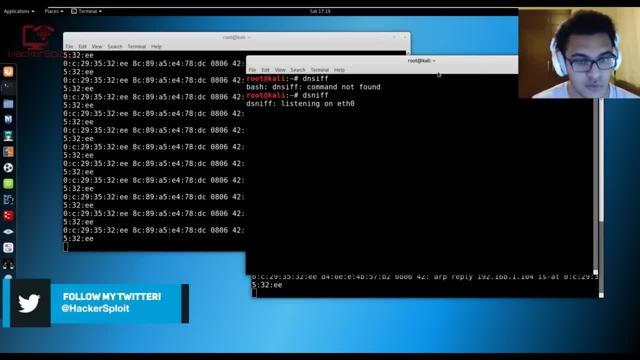 network or or whatever tool you choose to use, and you can go through the packets that are being sniffed, because all the traffic from that device is passing through the attacker machine, which is what I'm using now. so that's going to be it for this video, guys, I hope you enjoyed this video. if 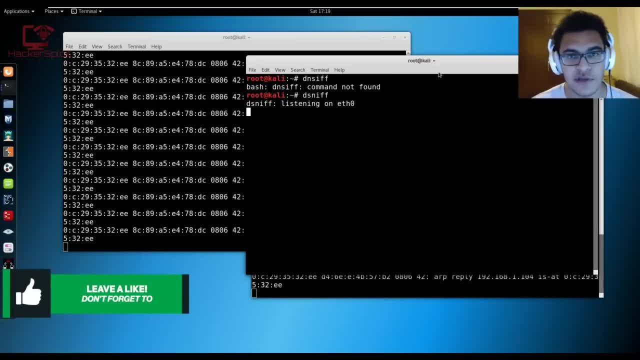 you did. please leave a like down below. thank you so much for the support. I really, really appreciate it. and yeah, one more thing: on the website I'm accepting articles or tutorials, that you guys. uh, if you want to post a tutorial or a guide, just write it up to me. 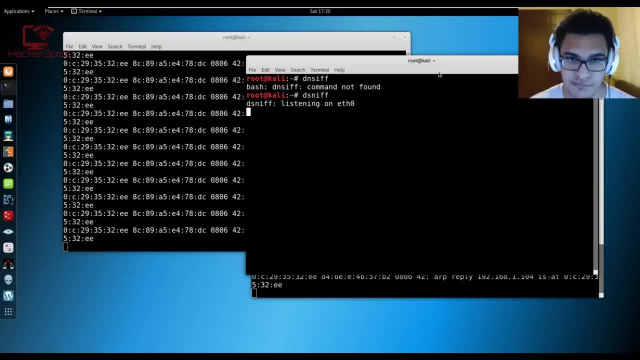 review it and if it's good enough or it's- uh, you know it's- it's giving value to people- I'll publish it on the website under your name. so, yeah, I'm hoping to make it a lot more interactive and I'm going to be posting a lot of more tutorials on their guides- things to help you guys get started. 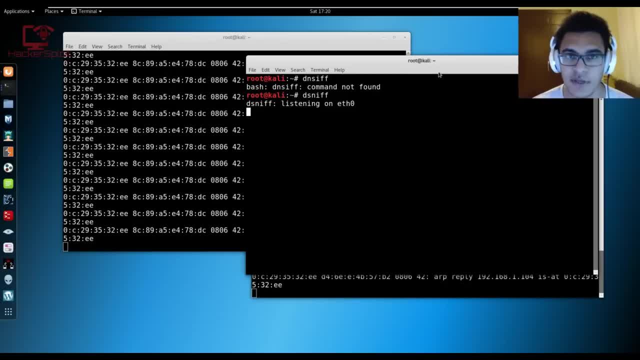 and you know things to keep you guys going in terms of learning about hacking and you know anything else. so if you have any questions or suggestions, leave them in the comment section or you can hit me up on my social networks. and yeah, I'll be seeing you in the next video. peace. 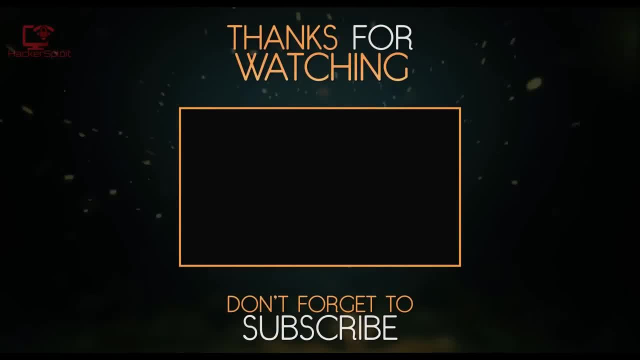 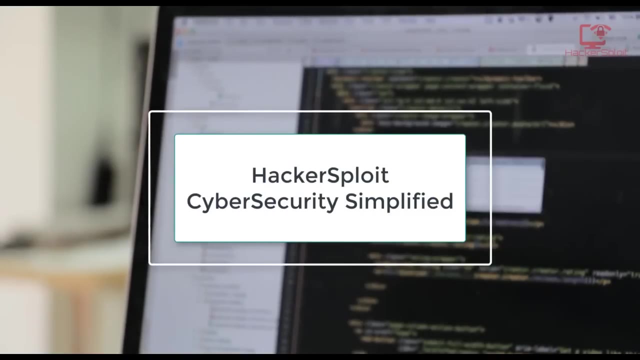 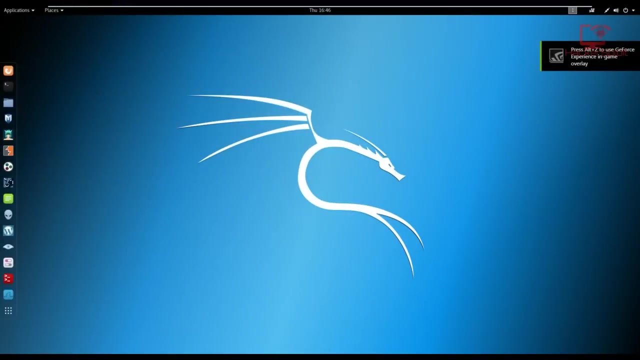 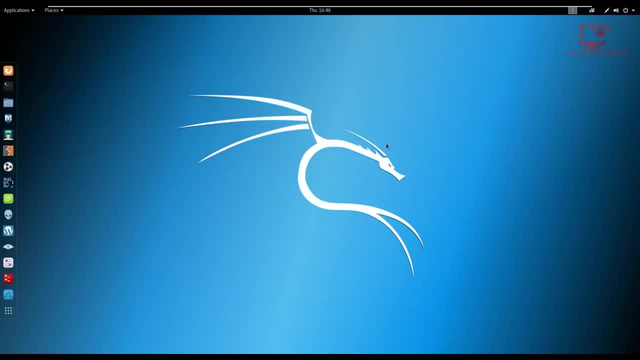 going to be doing a video on hacking, and you know I'm not going to be doing a video on hacking. and you know I'm not going to be doing a video on hacking and you know I'm not going to be doing attack. app is attack. app is a fantastic security tool that allows you to perform man in the middle. 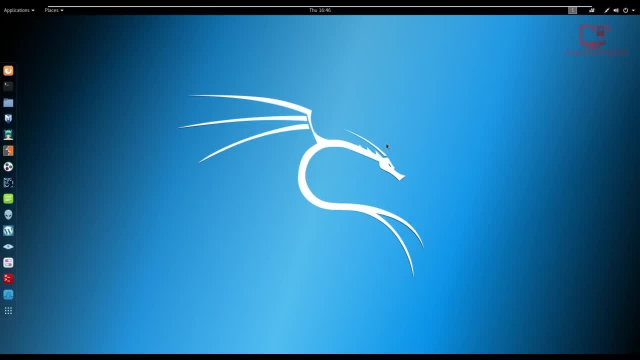 attacks on LAN or on your, on your local network. Alright, so it comes pre installed and pre configured in Kali Linux, which is, you know, fantastic. So you don't have to download or set anything up. All the only thing you need to do is you, if you haven't logged into Kali Linux for a 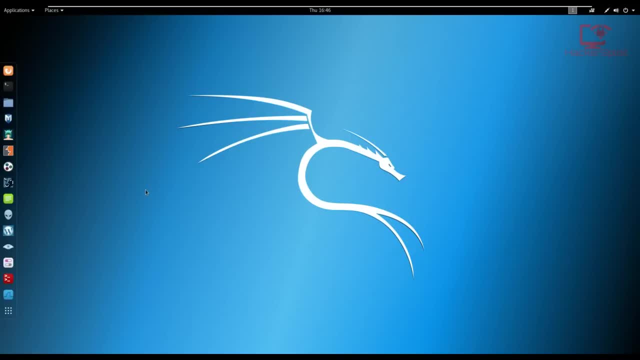 while just update your packages and make sure you're on and make sure you're running the latest version Alright. so in the previous video and we were looking at ARP spoofing with ARP spoof, some of you actually noticed in the comments that I did not forward the packets in the sense. 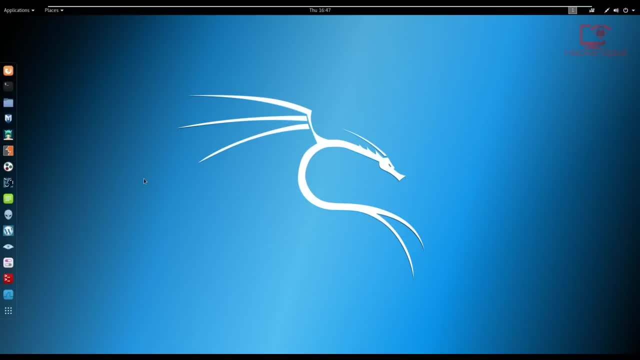 that I did not allow the flow of packets through my computer, being the man in the middle allowing it to flow to and back, you know, through to the router and back to the client, or our target, for this matter. Okay, so hopefully I can explain how to do that right now. I actually did it before the 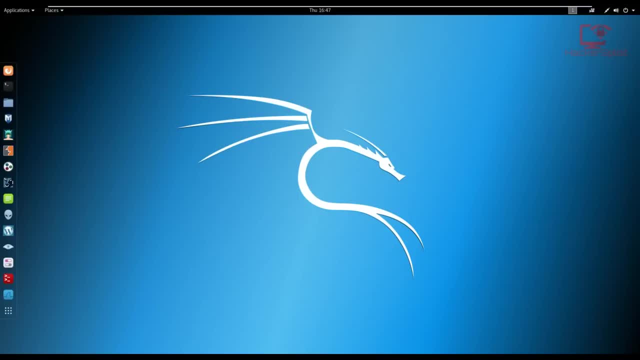 video, assuming that many people know how to do it, And a lot of people were saying that their connection isn't working, And I actually remembered that- yes, that that is an essential step, So I'm going to show you how to do it now. Alright, so just open. 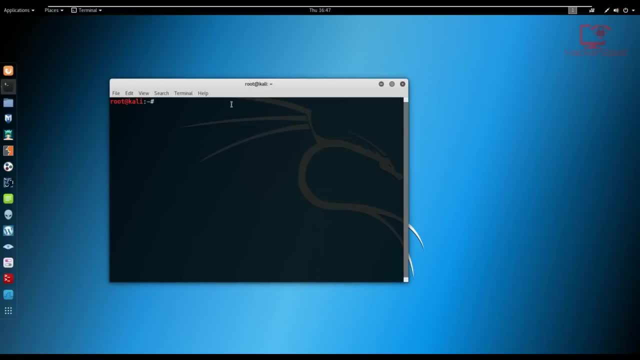 up your terminal and, obviously, make sure you're in route. it always helps. And now we're going to use the system control command. So system control, And we now want to select the option W to write. So W to write and the net dot- what was it? net dot, IP v4.. Yes, we want to forward IP v4 packets dot, IP. 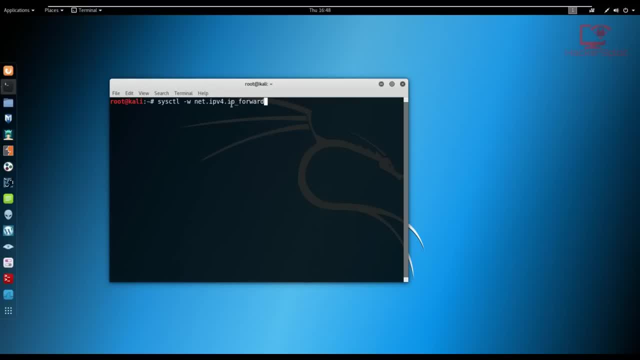 forward, sorry, IP forward. IP forward equals to one, so the value should be equal to one. Alright, so that is the command that will allow the flow of packets through your computer, as you're acting between the router and the client, So just. 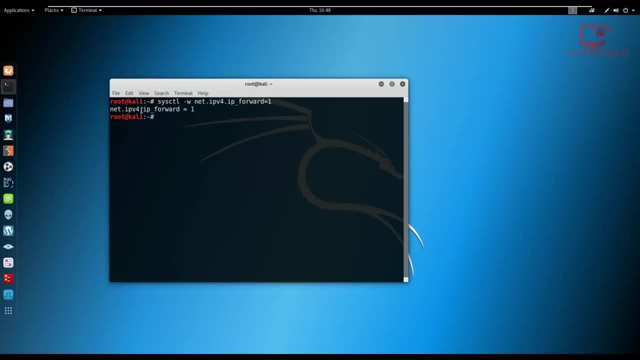 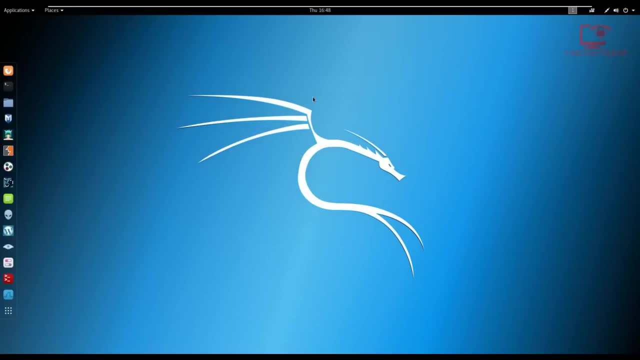 hit enter And it should give you the result saying: yes, the the IP v4 IP will will. the value should be one. Alright, so once you've done, we are done with that, we can get started with a tech app. 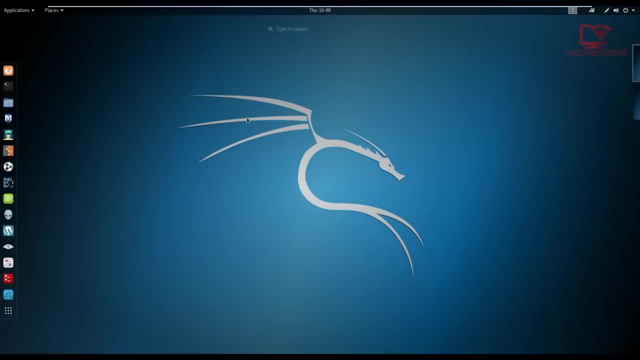 Alright, so a tech app, as I said, is pre installed with Kali Linux, So you can just search for it And you can just go into your search menu and just go into a tech app And you make sure you select at a. 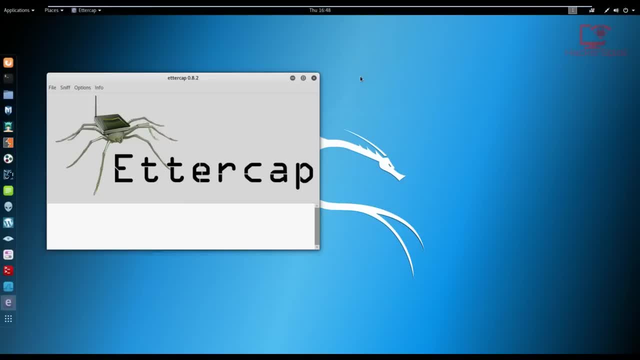 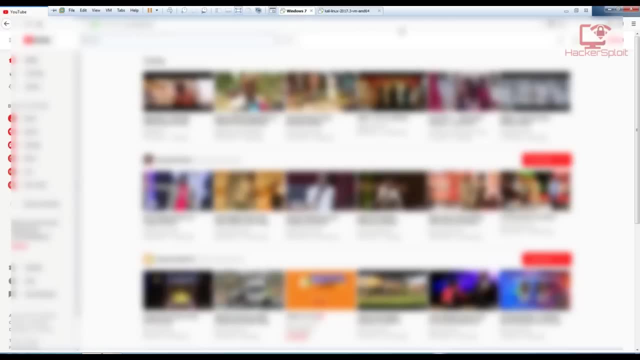 cap graphical, because that's what I'm going to be elaborating in this video, So just click on it Now. before we get started with actually, you know, performing any man in the middle attacks, you need to have a target. So in this case, I have a target here. Alright, so I have a target there, And this is a Windows. 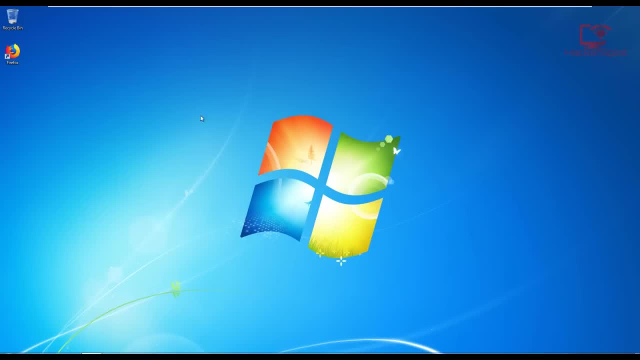 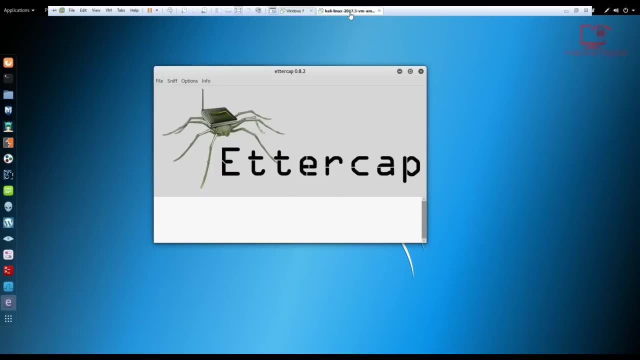 seven operating system. that is going to act as our target. So we're going to try and intercept the packets being sent between them: The Windows seven operating system and my and my router. Alright, so once you've opened up at a cap, what? 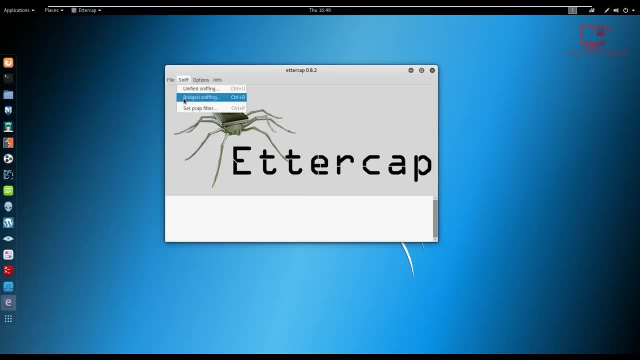 you need to do. the first thing you need to do is you need to select your sniffing option. So usually, if you're connected physically to the ethernet- so what I mean when I say you physically is you're actually connected to an ethernet adapter or to a switch or to a hub- then I would recommend that use bridge. 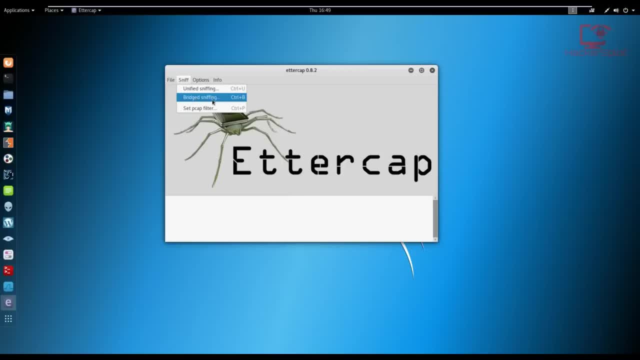 sniffing. So what this means is, if you're in a situation like you're in an organization where you have, you know, your computer is connected to a switch that is also connected to other computers in the organization, I would recommend that use the bridged sniffing. Otherwise, in my case I'm just going to use unified sniffing. 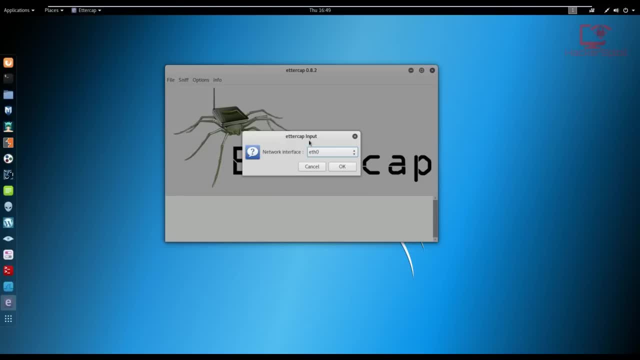 because I only want. I'm only using one adapter. there's no bridged connection. Okay, so now it's going to ask you to select your network interface. I'm going to select Ethernet zero, because I'm using Ethernet right now, And by default you can also select your wireless adapter, if that's what. 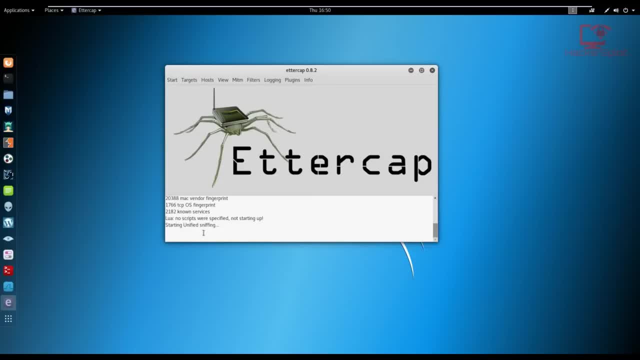 you choose to use. So just hit OK And now, as you can see, it's going to tell you that the unified sniffing process is started, And what you have to do now is you need to add a target. So you want to go into targets and you want to go into current targets. Now, as I said, this is very 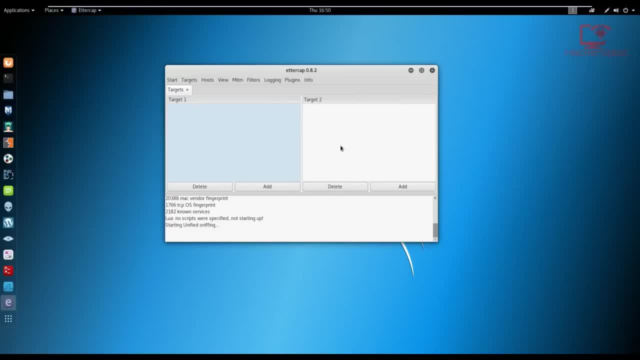 very similar to ARP spoof, where you would simply add your, your router IP address and your target IP address, similar to what you would do with with our spoof. So what you would do with us poof is you would. firstly, the first step would be to select your, to select the target as the router. 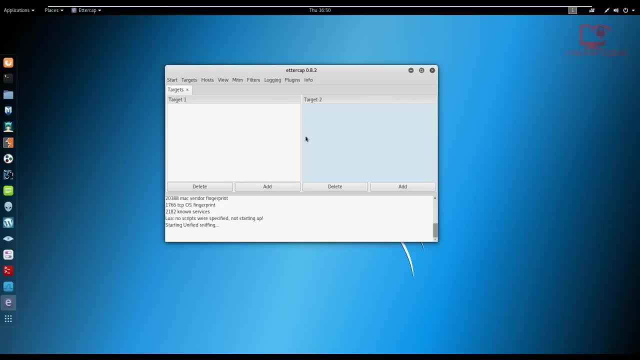 IP address and then you would add your target IP address, And then you would add your target IP address And then you use the your target IP address as the secondary on. So in this case all you need to do is just add your, your, your target one IP address as your router. So 192 point. 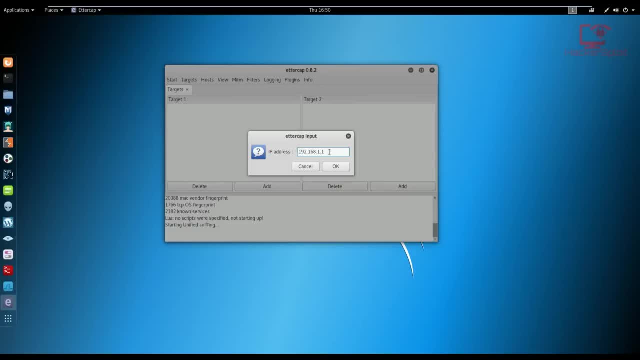 168, point 1.1.. That is my router IP address. it is your default gateway address, if that's what you're wondering. So you can just type in if config and you can find your default gateway and just get that and put it in here. Now you need to get your target IP address, which you can. 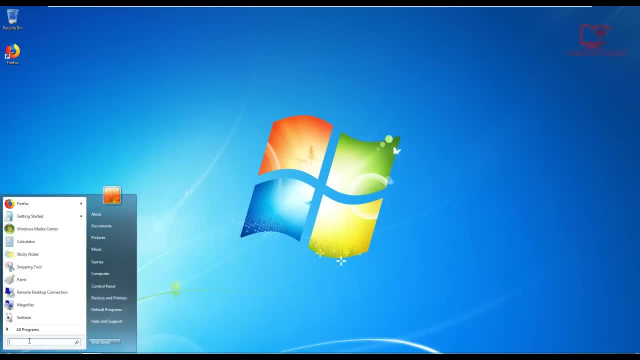 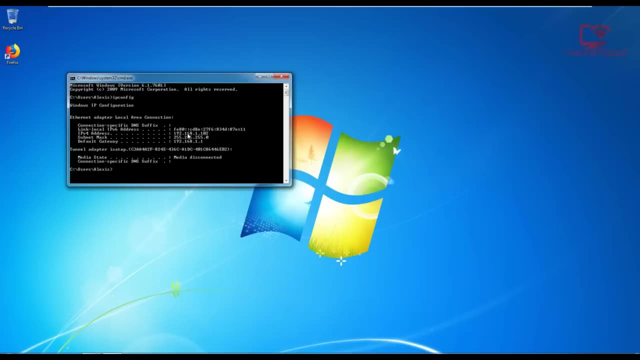 which I'm going to do, and I can do using my command prompt here, using the IP config command. So IP config. it's been a long time since I've used Windows seven, but boy, it feels good. So there you are: 192 point 168, point 1.1 or two, And we're just going to go. 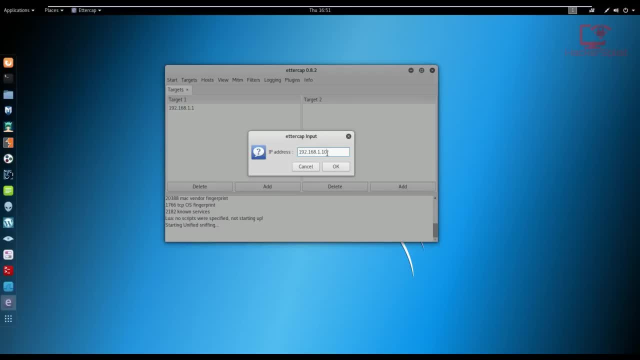 into our target and hit Add, And we're going to say 192 point 168, point 1.1 or two, And we hit OK, Alright, so we've added our target in our IP address and our router IP address. Okay, 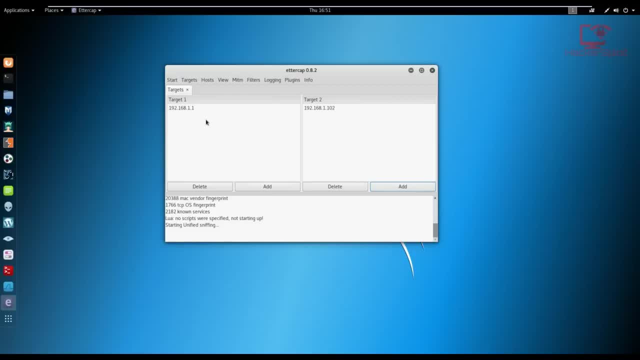 so now we need to actually perform the, the ARP poisoning attack that will give us money in the middle axis. So to do that is really very simple: just going to man in the middle and click on ARP poisoning, And now it's going to ask you for optional parameters. Make sure you check sniff remote. 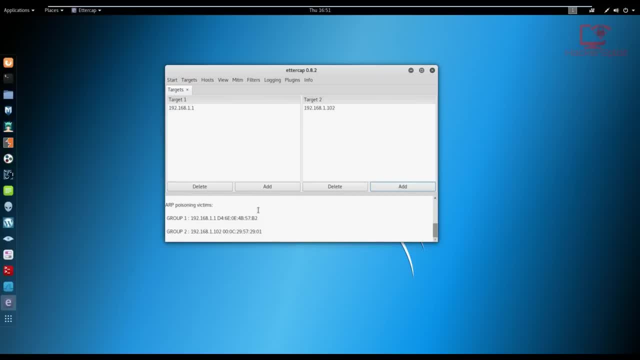 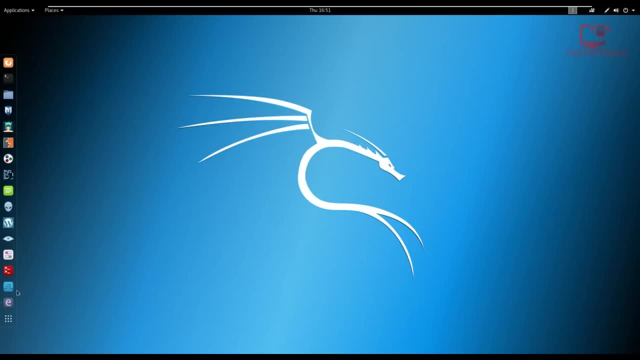 connections and just hit OK. So once you've done that, the ARP poisoning has begun and it's currently running. So now you can use a traffic or network sniffing tool like wireshark or TCP dump, which is what we're going to be using. So if I just open up TCP dump, I really enjoy using TCP. 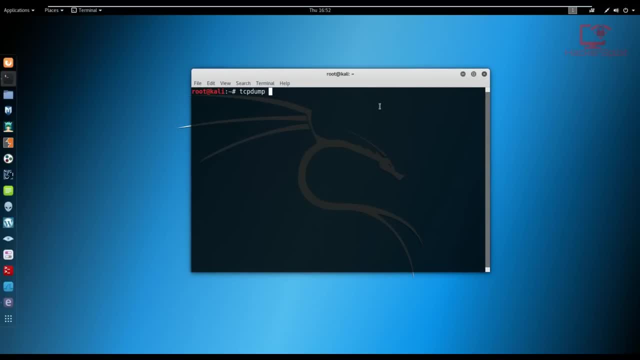 dump sometimes. So TCP dump, TCP dump, and we can say the interfaces Ethernet zero, And we specify the, the port port at the target, or actually the host is 192, point 168, point 1.1 or two being our target, and we, whoops, for some reason we're. 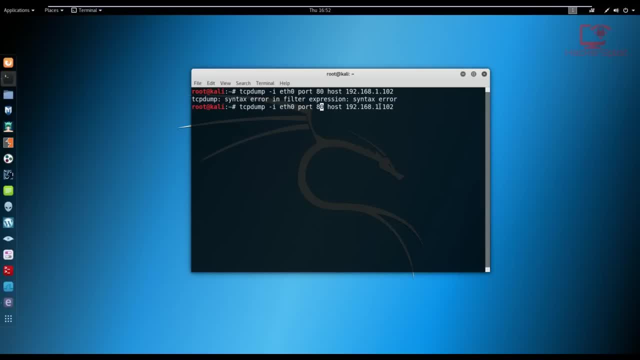 getting an error port at- or sorry about that- In N and at and we hit the port. sorry after the port commander. it's actually been a while since I've used TCP dump And for some reason I keep on getting this syntax error here. So we've 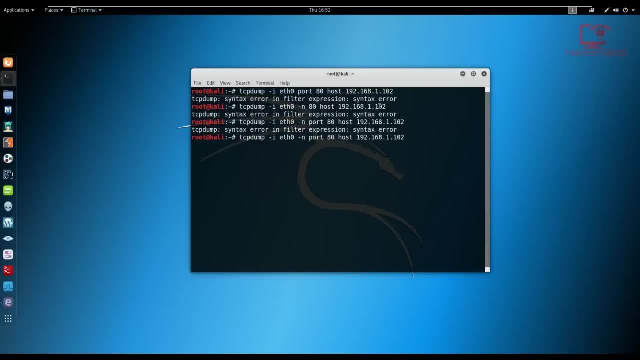 selected our host, So n, port 80,, host and host. So I forgot to add the end. And there we are, Alright. so yeah, the syntax for TCP dump is quite confusing, in the sense that you have to specify the, you have to specify the interface that you're using, you then have to specify the port, which in 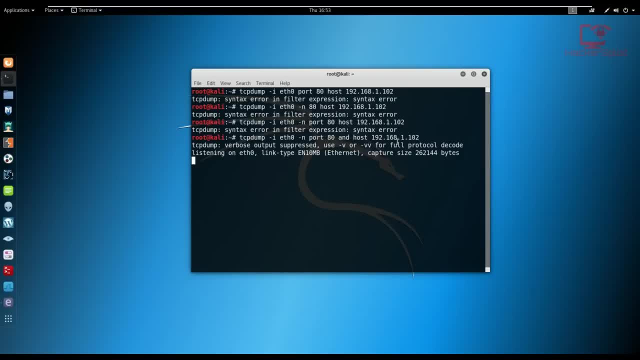 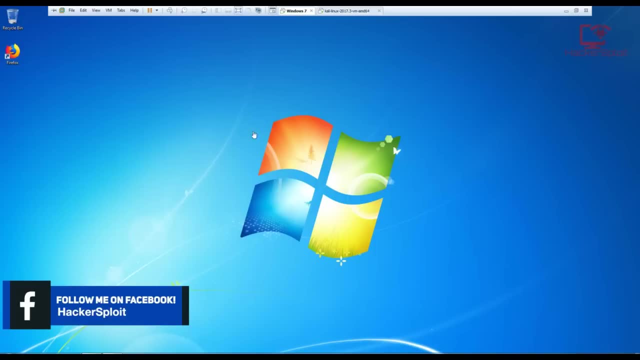 this case we're using the TCP port and our host, which is 192.168.1.1 or two. that is the target IP that we want to sniff the traffic from. So now, if I go into my Windows operating system here, 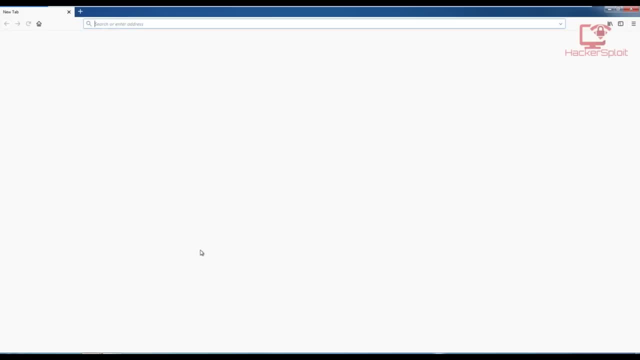 and I just let me just open a new window here like so, And I just try and open a site like redditcom. Alright, so redditcom And I just go back to Kali Linux And, as you can see, there we 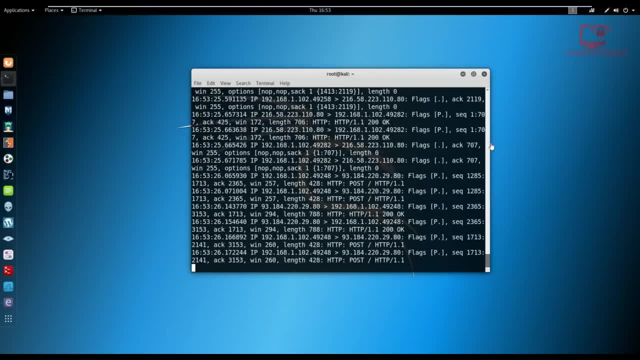 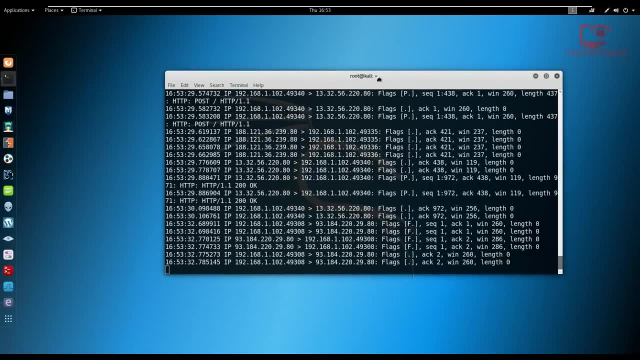 are. the traffic is being captured, just as though, just the way it is being captured, So we can see that as well. And so let me just open up a different one. So you can see that there we are here, And in this case we're looking at our connection, And now we're going to be able to. 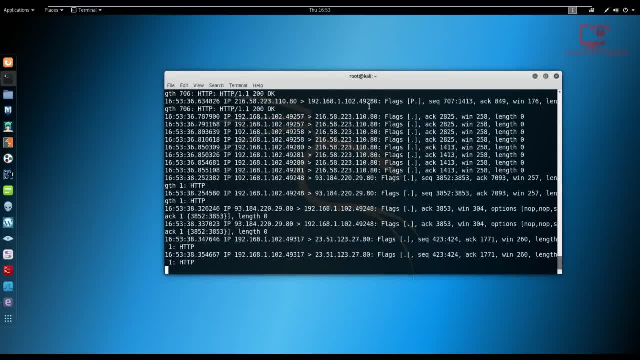 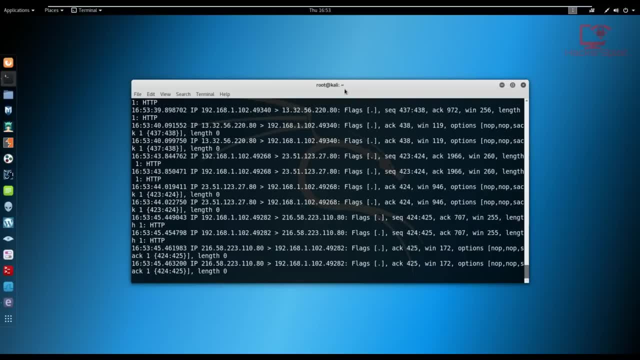 use a RPS poisons method in here, So that's the RPS poisons method. So now here comes the the RPS poisons method, And the RPS poisons method is actually the way we wanted it. Now, additionally, you can use- why? shock, if that is what is comfortable for you. but there you go. 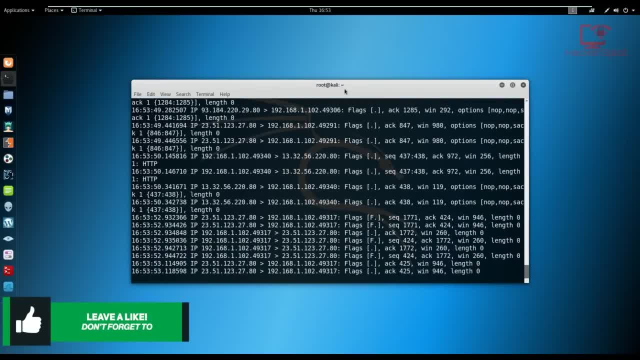 That is how to perform a man in the middle attack with a tech app. It's really very simple. The process is exactly the same as to what you would find with RP spoof, And that's because they're both using the RP poisoning method. 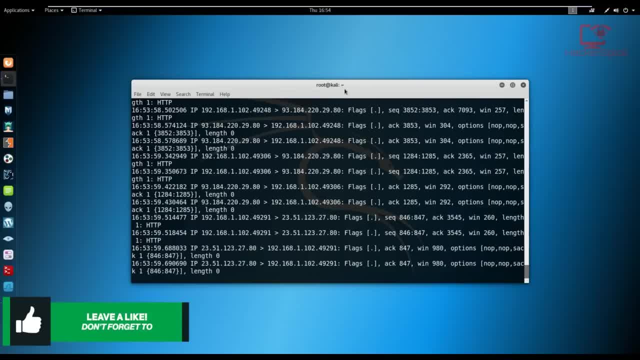 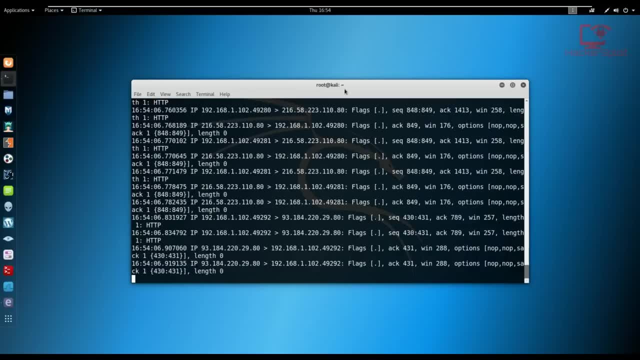 and I'm really, really pushing forward to it. Thank you so much for everything you guys. If you found value in this video, please leave a like down below. If you have any questions- any at all- hit me up in the comment section on my social networks or on kick, All right. 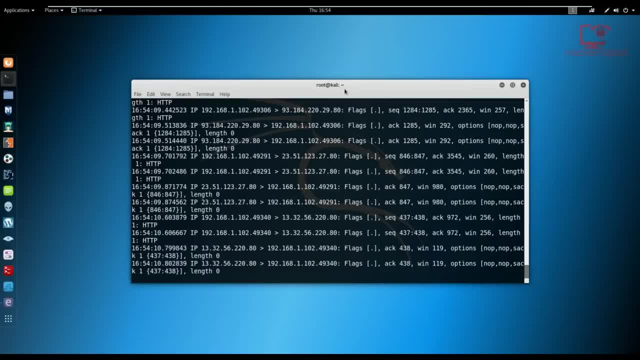 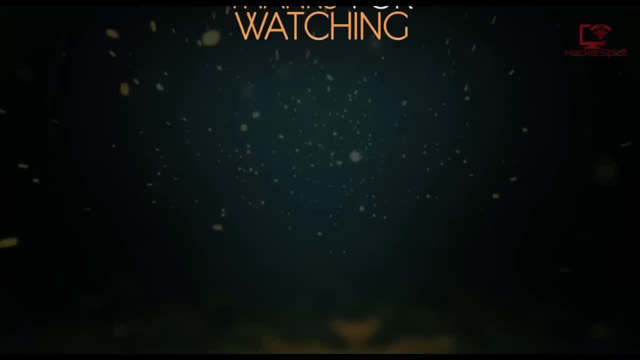 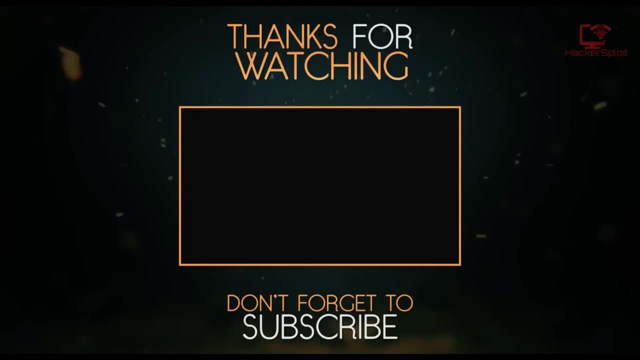 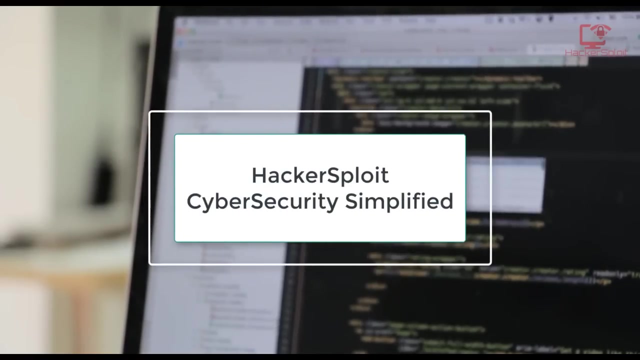 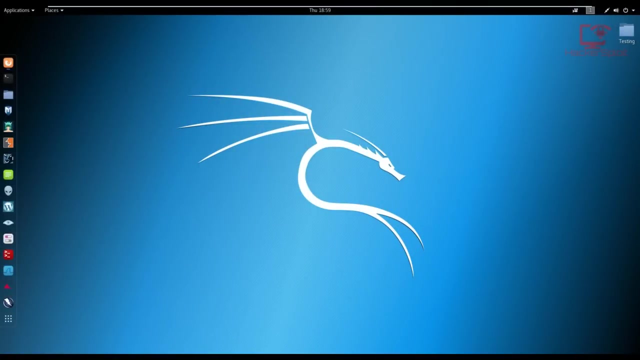 and you can check out my website for the latest hacking news, tutorials and guides. So thank you so much for watching, guys, and I'll be seeing you in the next video. Peace, Hey guys, Hack Exploit here back again with another video, And in this video, 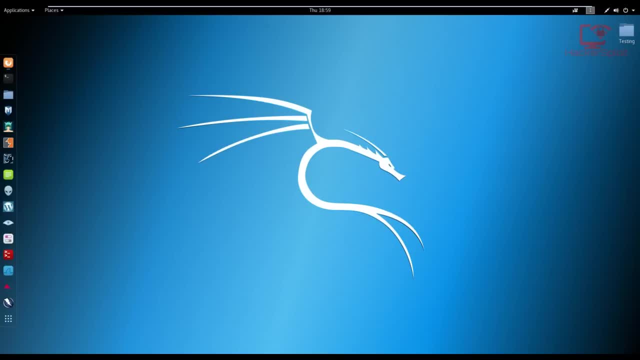 I'm going to be showing you how to exploit WPA or WPA2.. All right, Now again, this is something that I realized was not on the channel. I did really have not focused on cracking wireless networks, And I was thinking of starting off with WEP, but I didn't realize that. WEP wasn't true, So I'm going to be showing you how to exploit WPA or WPA2.. And I'm going to be Start off with WEP. but I didn't realize that WEP wasn't true, So I'm going to be starting off with. 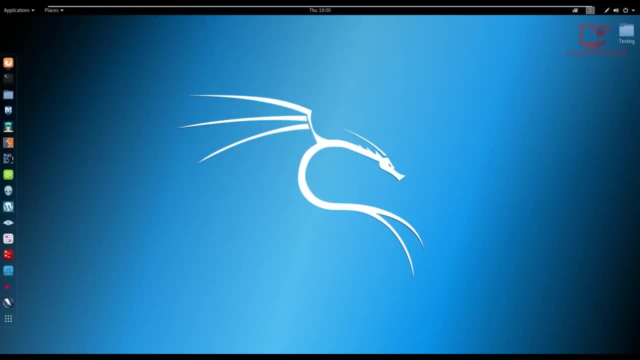 WP is become almost obsolete after you know the arrival of WPA, and you'll rarely ever see a network that uses WP as their means of security. In this video, I'm going to be showing you how to use aircrack NG to capture packets- obviously to capture packets and then to capture the WPA. 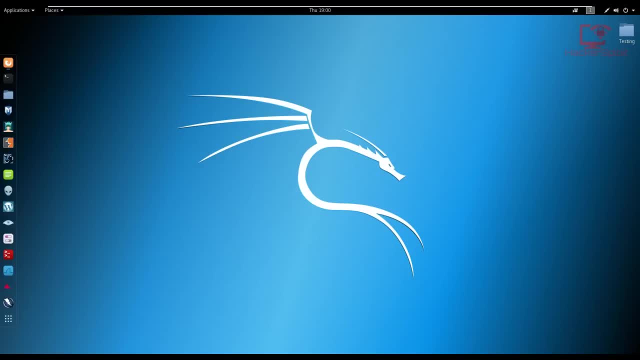 handshake, which then get, which can then be used with a word list to perform a brute force attack or a word list or a dictionary attack, And, obviously, to get the, the password. Now, again, I'm also going to be using airgeddon, which again is a fantastic tool, or as I like to call. 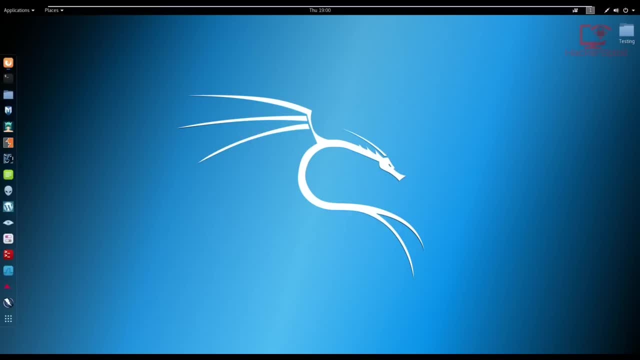 it a framework that makes penetration testing, or wireless penetration testing, a whole lot easier. So we're going to be looking at actually performing the pixie dust attack with airgeddon, using bully. alright, But first I'm going to show you how to use aircrack, how to capture packets, how to store. 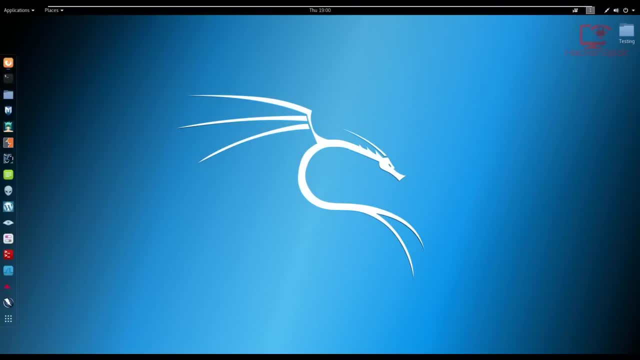 them in a capture file or a dot cap file, not really a dot pcap file, But then I'm gonna also going to be moving on to Speaker 3. Speaker 3: you: how to you know select monitor mode, not to select your adapter and change it to monitor? 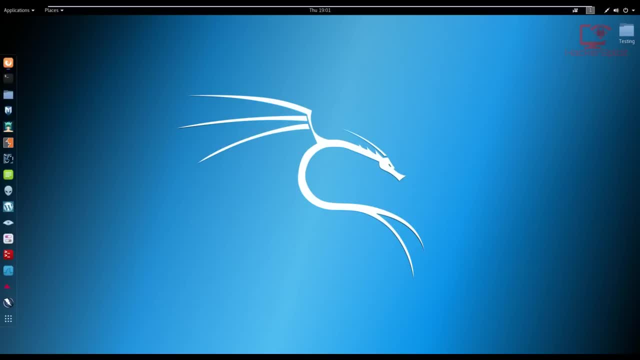 mode. and, finally, I'm going to show you how to how to use air crack ng to crack the password. that being said, let's get started. so for those of you don't know, let me just explain really quickly. WPA is essentially? it stands for Wi-Fi protected access and it is a security protocol that was 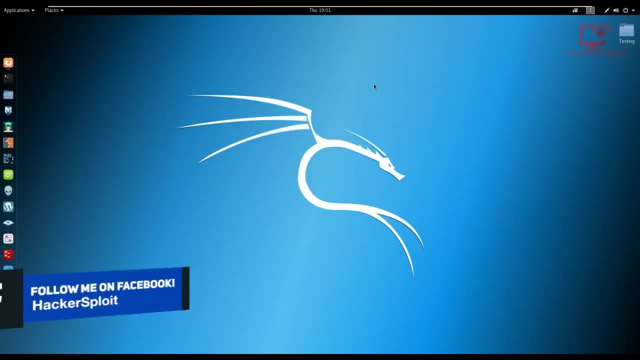 introduced in response to the weaknesses that a WP had. all right, so it's really improving upon WP's authentication and encryption features, and that's what I was talking about. WP e was was able to be cracked within minutes. it was unbelievable, you know, and that's why they had to introduce a. 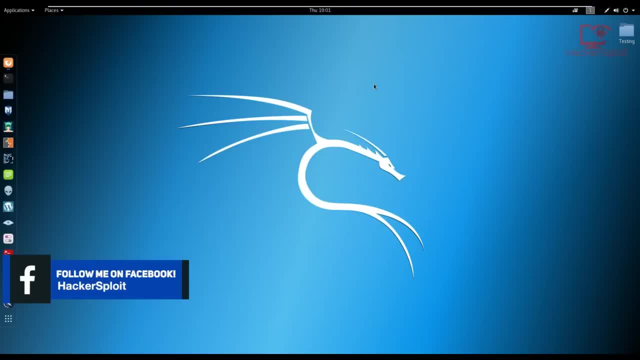 you know another protocol that made networks more secure. the WPA is is quite secure, but it's not the most secure, and he is is quite secure, but it's not at the most secure, and that's whether you know what I'm talking about. so let's get started with the introduction of WPA 3, which is also 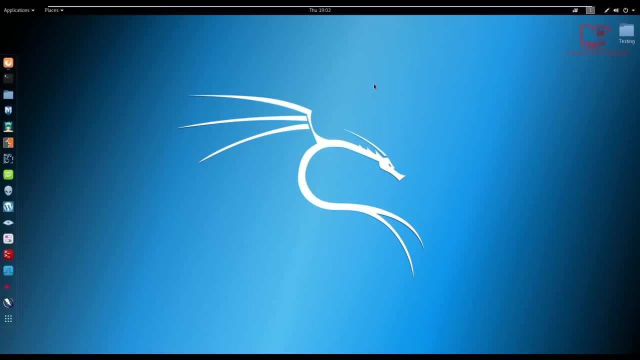 something I'm going to be really, really focusing on in the future, once the new routers are released, which are said to be later this year. so I can't. I can't believe that it's finally out and I'm really excited to get started with it. that being said, hopefully this video acts as a final resolve. 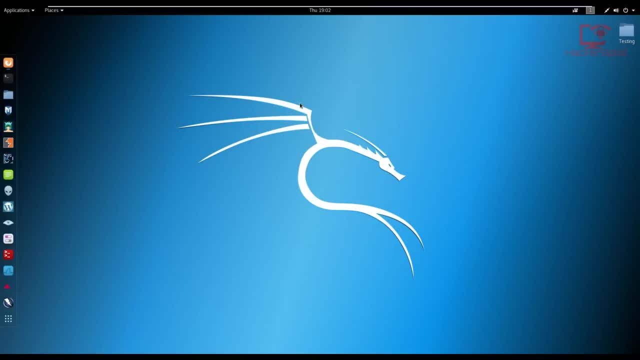 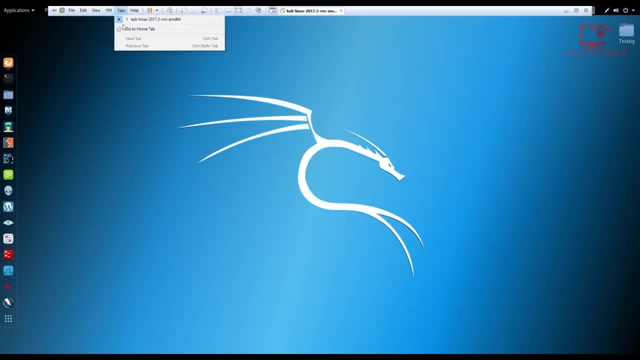 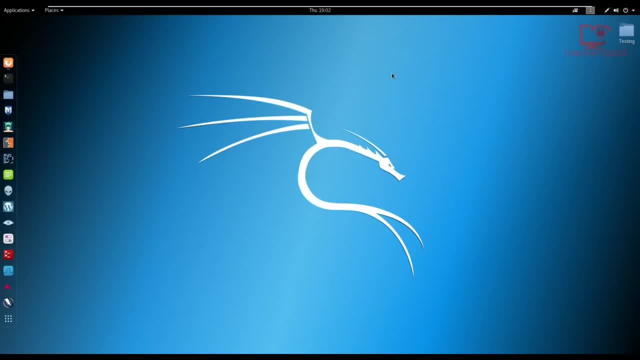 removable devices. you can see that I have my a theorist USB device connected and I just want to take a few minutes to talk about wireless adapters, because this is something that people get really, really mistaken with. you need a good wireless adapter for Wi-Fi penetration testing, it's no. 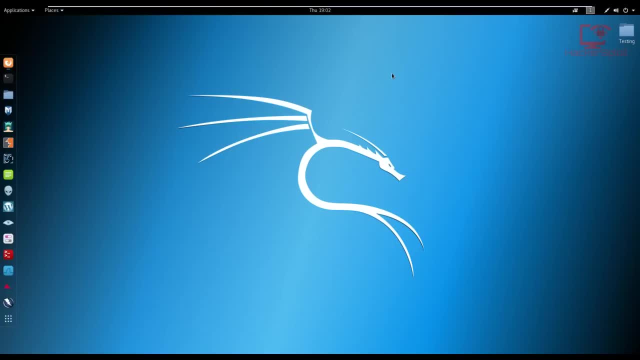 secret, and it's the truth. I don't know whether you've tried performing a packet injection with your wire, your laptop Wi-Fi card, but it just doesn't work. so I'm going to go ahead and go ahead, work, and the success rate is minimal. you can't expect to crack a wireless network with you know. 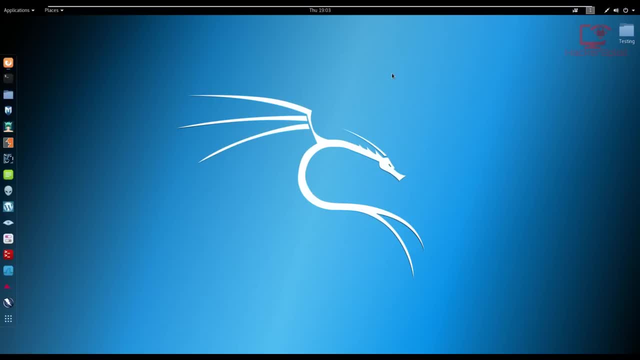 a small little, uh, you know, a small little tp link or well, i'm not saying i'm actually using the tp link, but using the, the onboard wi-fi adapters that come in laptops. uh, you know, it's just not possible. now, coming back to the correct adapters to be using, uh, i looked at the tp link and the. 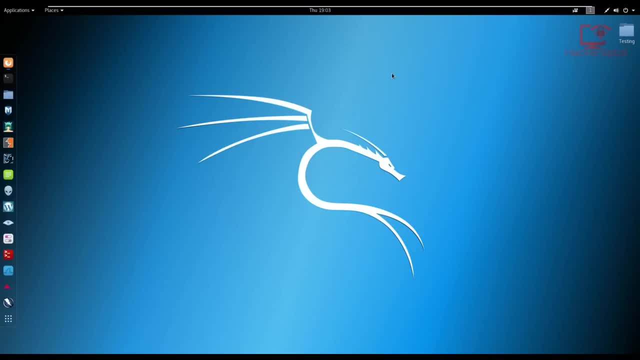 alpha cards and in my opinion, the tp link is the best one out right now. the tp link a tlwn722n version one, because version one is the only one that contains the atheros chipset, uh, which again is awesome for packet injection. you can also try the alpha ones, but the alpha ones were also. 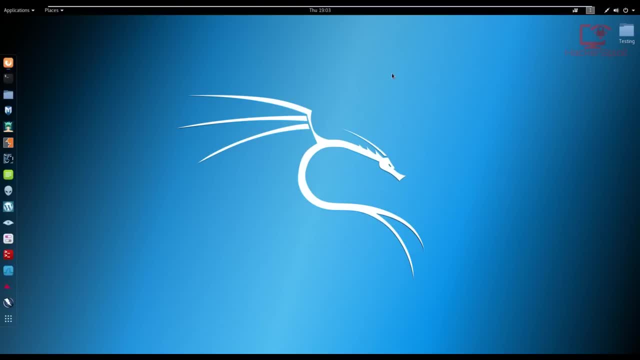 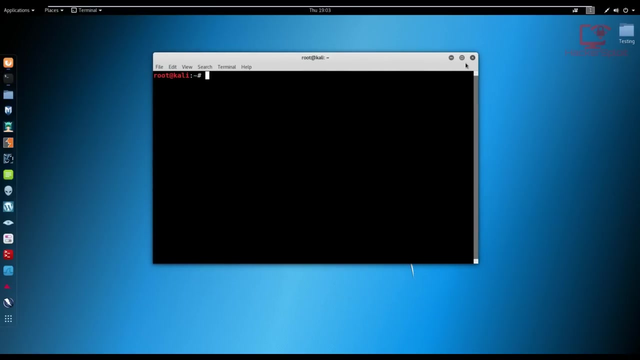 i i would say, in my mind, mediocre. not that they're bad, but they'll get the job done. uh, the tp link one is extremely fast. i was, you know, i've been using it for a while now and uh it it really does, uh work wonders. that being said, let's get started. all right. so the first thing i'm going: 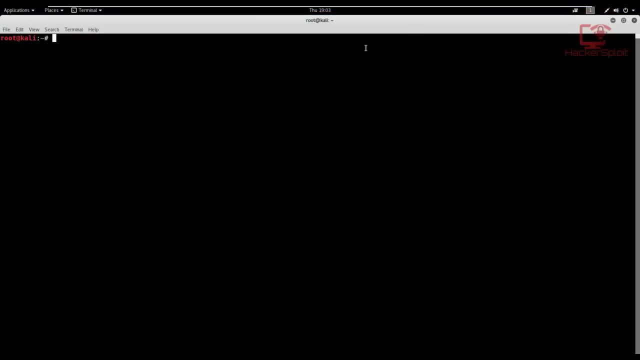 to show you how to do is how to, um is how to to actually enable monitor mode on your wireless adapter. all right, so make sure it's connected and i'm going to type in iw config to show us our wireless interfaces. and my- uh, my wi-fi adapter is already in monitor mode, so what i'm going to do 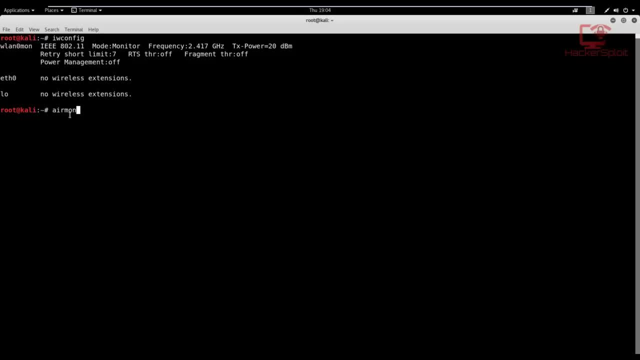 is. i'm just going to. i'm going to disable monitor mode, and you can also do this by typing m on ng. so stop, lan, zero mon, that is the name of the interface in monitor mode, and i'm going to hit enter. all right, and it's going to disable monitor mode. so now let me show you how to enable it. so if i type 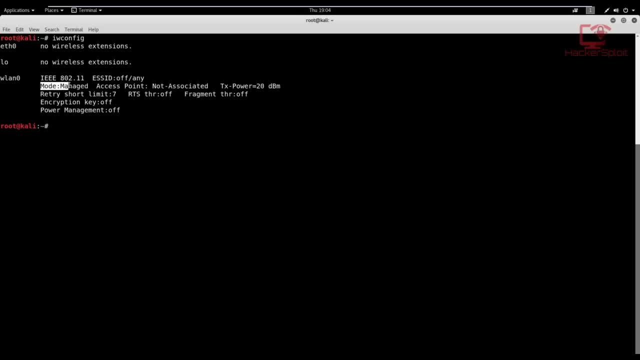 in iw config again. you can now see that it's not in monitor mode, and you can see that right over here. it's saying that the mode is managed. now for those of you who are wondering, what exactly does monitor mode mean, you know why? do we need to even change it to monitor mode? well, monitor mode. 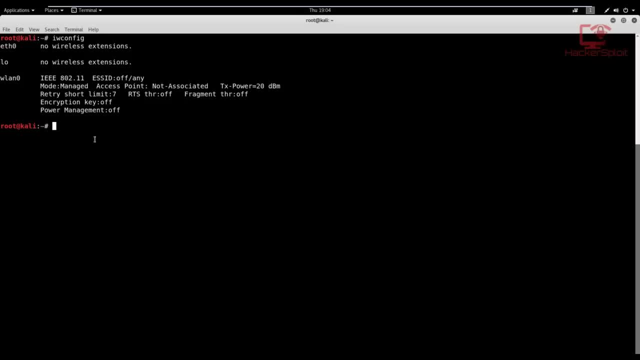 essentially means that your monitor mode is not in monitor mode and you can see that it's not in monitor mode. so what we do is we load in monitor mode from rx and i'm going to leave it here and we come back around, I'm going to click learned to monitor mode and I'll see how this works. 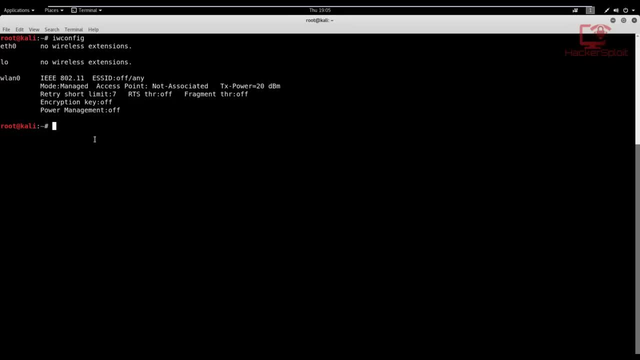 because I no longer need to buy some stuff from the modelling server. this is where we're now gonna click learn, but it says below monitor mode. so you can see the tutorial for monitoring settings. and we're just gonna click here and it's gonna open. it's gonna say monitor mode. 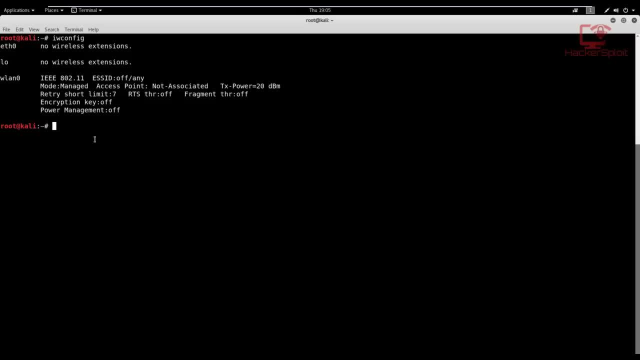 so please remember to download that. so this message changes every time you activate your monitor mode. just let me know if you enjoyed this video. please comment and share if you need some support from want me making good videos, as always, until we see you in the next video. bye, bye. 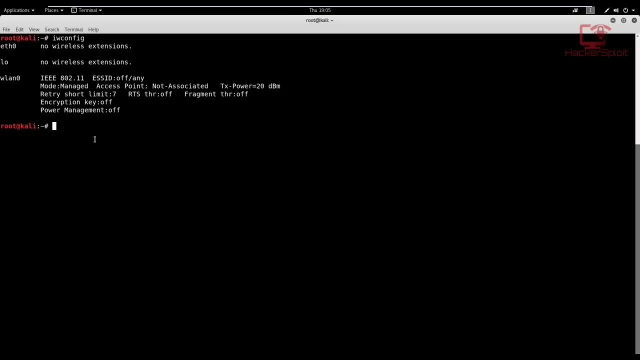 that you enable monitor mode, because most of the attacks will require monitor mode. in fact, monitor mode is essential. so to do this, we use the airmon ng. it is part of the aircrack suite. so airmon ng and we hit start, all right, remember, you can also stop it if you want. and now you select the. 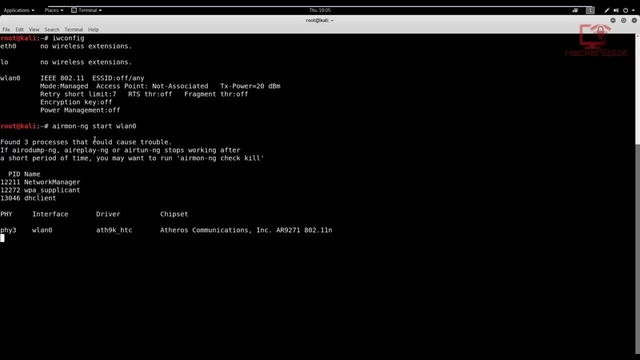 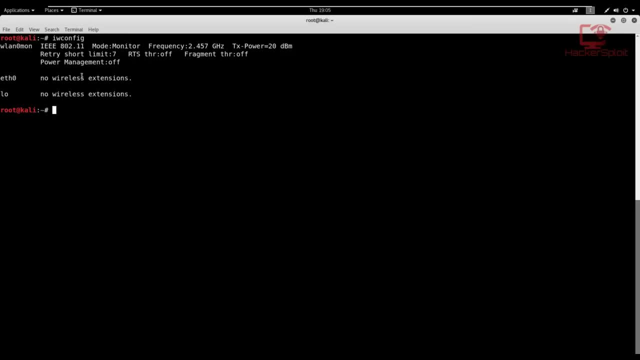 interface name, which is currently lan0, wlan0, and i'm going to hit enter, all right, and it's going to change it for us. so now, if i clear and type in iwconfig, we can see that the monitor mode is currently on and you can look at that in mode, which is currently showing us monitor and the 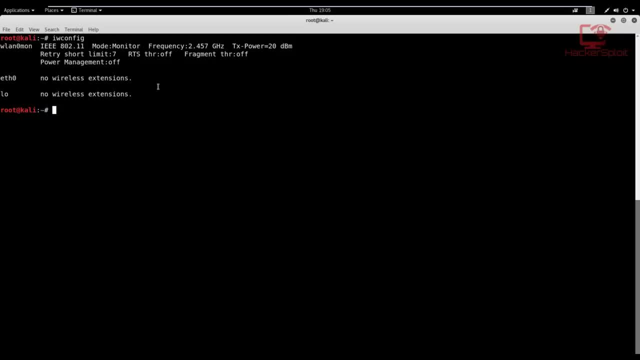 frequency is 2.4 gigahertz. now again, penetration testing on 5 gigahertz is slightly, slightly different and that will require special hardware. but also get into that on the channel. i really won't focus on cracking wireless networks as well, because it is quite fun, um. so let me just clear. 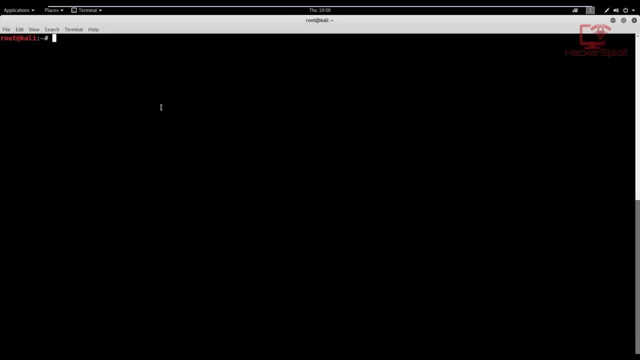 this up now. before we move on, i just want to point something out. most of the other videos on youtube are really just. they have no meaning whatsoever, because they're essentially promising you that you can crack wi-fi with any wi-fi adapter, and that's not the truth. i can guarantee that to you. 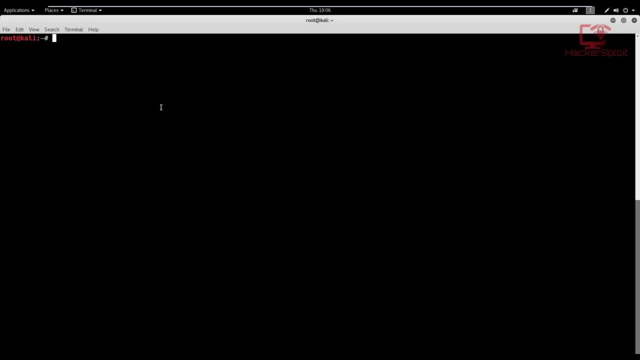 that being said, i just want to. i just wanted to say that now we have enabled monitor mode, now we need to start capturing data, uh. well, we need to start uh capturing data and packets from the access points around us. so we need to start seeing what access points are around us. 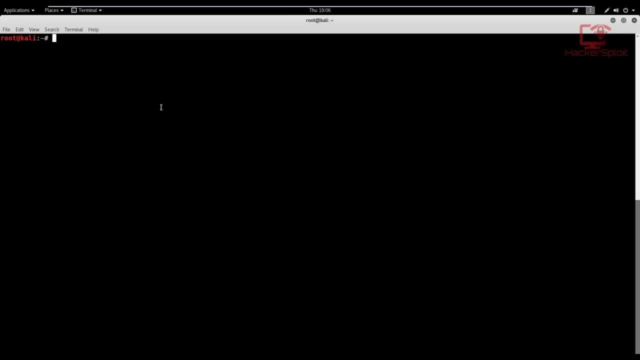 and then we'll select the access point that we want to crack or we want to get the wpa handshake from. okay, and we can do this using the aero dump. aero dump ng. so aero dump ng. and now we select the interface name, which is in monitor mode, which is wlan, zero mon. all right, and 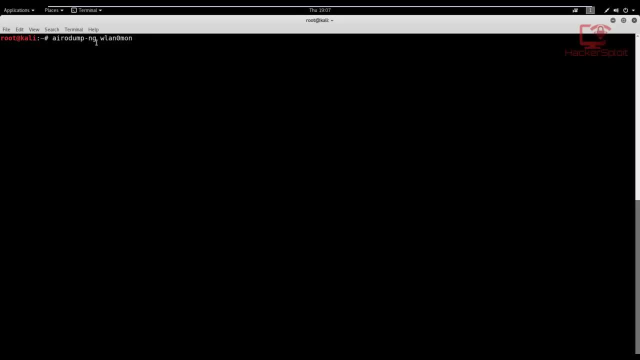 i'm going to hit enter now. uh, this is going to display the wi-fi networks that are around the wireless adapter or around you, and i'm going to be blurring the ones that aren't mine, or if i capture mine immediately, then i'm going to stick to that. so i'm going to hit enter and i'm just going to. 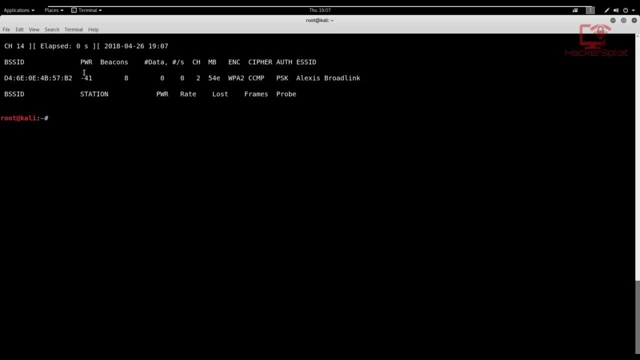 hit ctrl c, uh like so, and you can let it run and it's going to start capturing the wi-fi networks that are around you by default. this is the network that i'm going to be performing the test on. as you can see, it is my router, it's um, it's called alexis broadlink, and let's start off with what each of 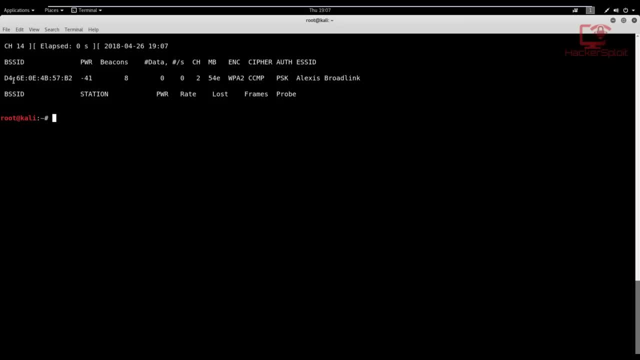 these sections mean. all right, i'm going to just cover the most important bits. so let's start off with the bss id. this is the mac address of the router. very, very important this, in fact, should be. you should actually be copying this immediately. the next thing is the power, which is essentially 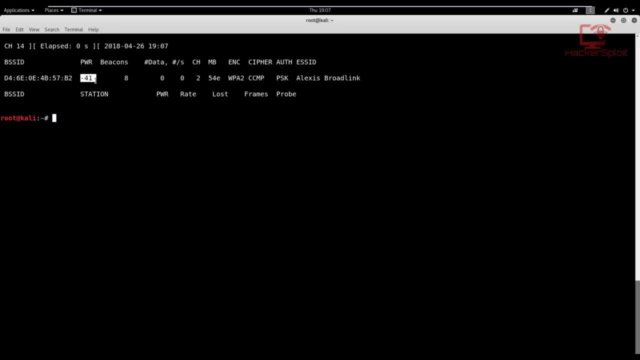 the uh, the strength of the signal strength uh that you currently have, which is not bad. we have uh 41. you then have the beacons. this is the, the beacons being sent, quite self-explanatory. you then have the channel of the wi-fi network, again something very important. this is the channel on which the wireless 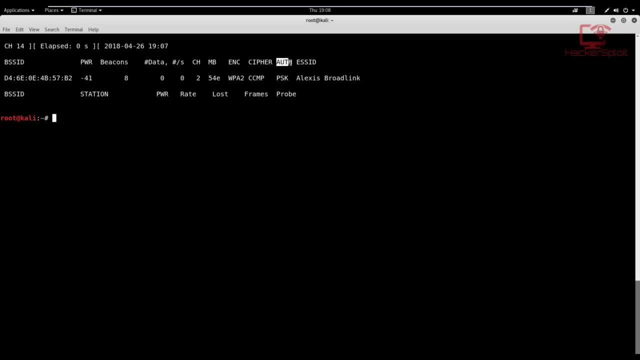 network is running on. you then have the encryption type, which is wpa2. you then have the authentication, which means uh. you know the uh. the security of the network is determined by a pre-shared key, also known as a wi-fi password, and you have the ess id, which is the name of the network. all right, 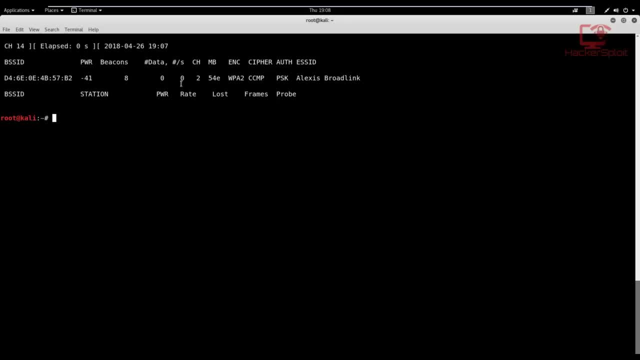 awesome. so, alexis, you have told us how to find the uh wireless networks around. you remember i can i. i stopped the scan as soon as i got the one that i wanted, because i do not want to uh to start scanning devices. uh, you know other wi-fi networks and i really don't want to go through the trouble. 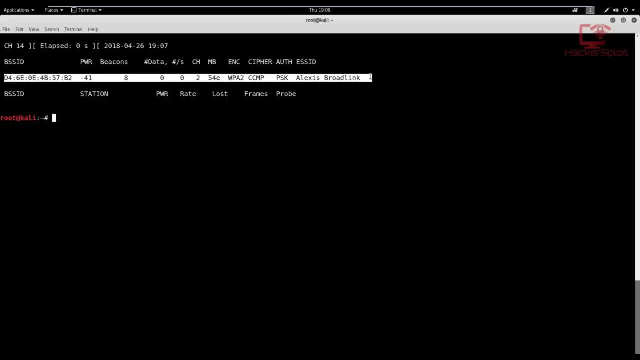 out all right. so once you've you've captured, uh, or you've actually spotted the network that you want to perform the test on, just hit ctrl plus c and it's going to stop. now make sure you have this data in play in plain sight, because we're going to need it. so, uh, what we're going to do now. now, 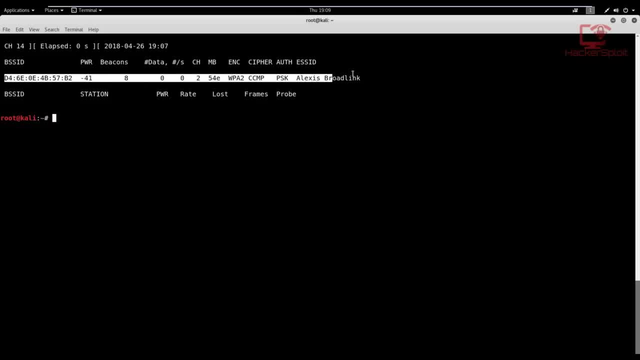 we need to start capturing packets that are being sent to and from on this network, all right. so now we need to focus on this network, so we need to select it. so, essentially, what we're doing now is we're saying: only focus on this mac address or this access point, do not focus on the other ones. so it's going to start scanning the 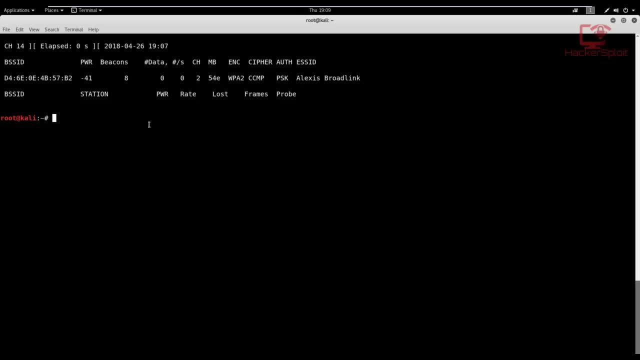 network and it's going to display all the um. it's going to start displaying all the clients connected to that network and i'll show you that in a few seconds. so we can do that by typing arrow dump, uh, arrow dump ng. all right, so arrow dump ng. and now it's going to say, uh, we need to. essentially, 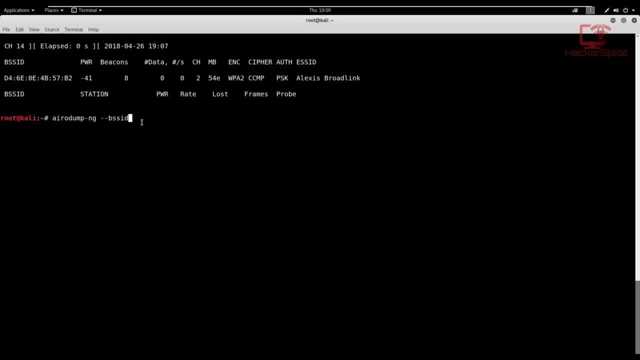 specify the bss id, so you can say bss id, which is done by bss id, and you want to copy the bss id of the access point and we're going to paste that in there. and now we need to select the channel, which you can do like: 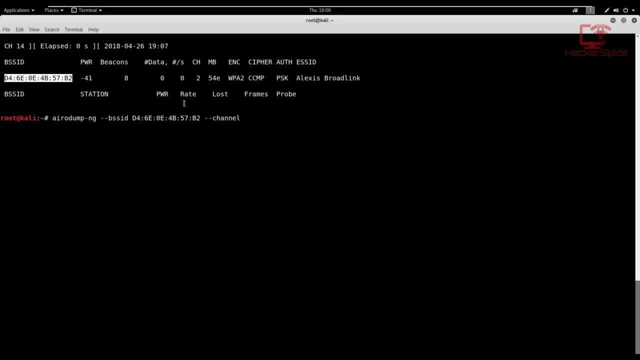 so, or you can just abbreviate with ac, but i like having it as channel. by the way, you can use channel and bss id, where it doesn't matter what comes first, it will still work just the same. all right, so the channel is channel two. so i'm gonna specify: the channel is two. uh, now, what else do you need to? 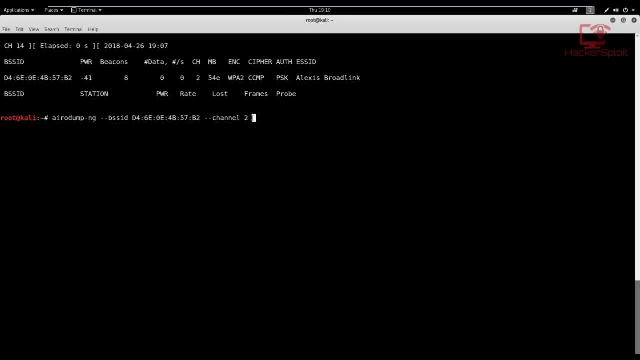 specify. well, now you need to specify um, the wireless access, the wireless uh, the interface name, which is lancer mon. all right, and i'm gonna hit enter and now, as you can see, it's gonna start capturing data. uh, that is on that network, that is being sent on that network. and if i just open up my phone, 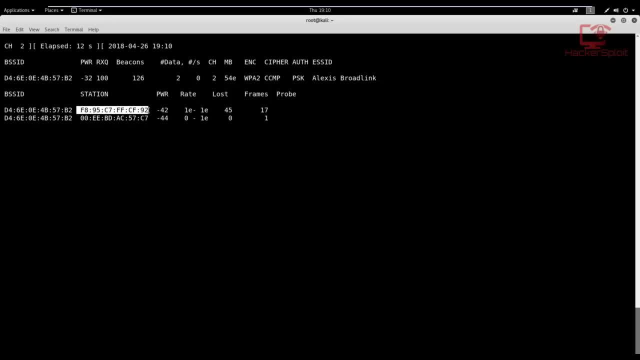 right now my nexus device. you'll start seeing the mac address. there we are. this is my mac address of my nexus. so let me just open up a website here really quickly. so let me just open up a website here and you start seeing the data is already being captured. 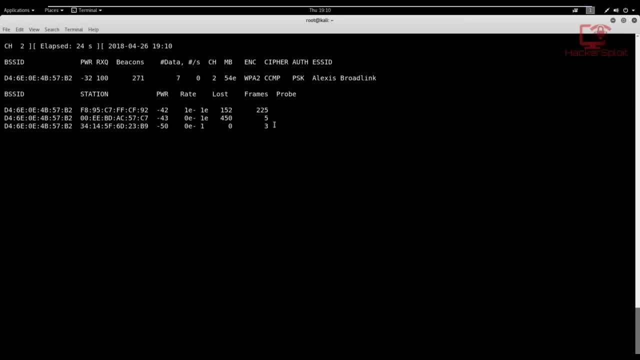 you can see the frames has started increasing. there we are, and the frames will show you the data being sent or the amount of uh whether or not that device is active. this is very important because to capture the wpa handshake we need a device that is active on the network. 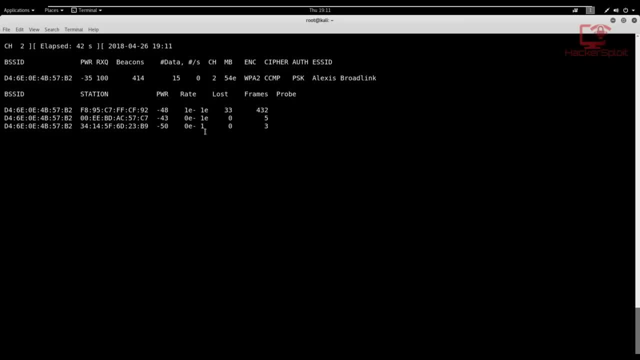 otherwise it will take too long. all right, awesome. so now we are capturing the data, but something is missing. you know this data is important, but it's of no use if you're not saving it. so how do we go about saving? you know, this is where many people make the mistake. 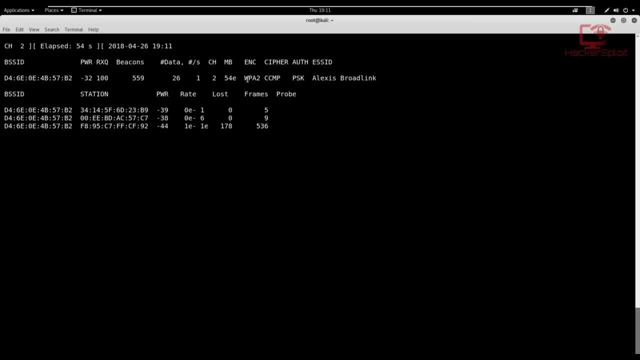 you cannot crack or get the wpa handshake if you're not saving the data you need to save it, the data you need to save it. Well, wherever you choose to save it, I'm going to save it on my desktop And I'm going to show you how to do that right now. So we will need Ctrl C to stop. 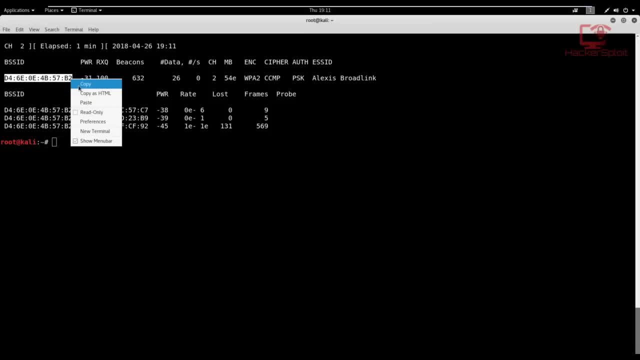 that And we need to clear this out. But before that, make sure you copy your BSS ID and the channel, because we're going to need it again, Except this time we're just going to save it, to output the results to a file. All right, let's clear this up And I'm going to change my working. 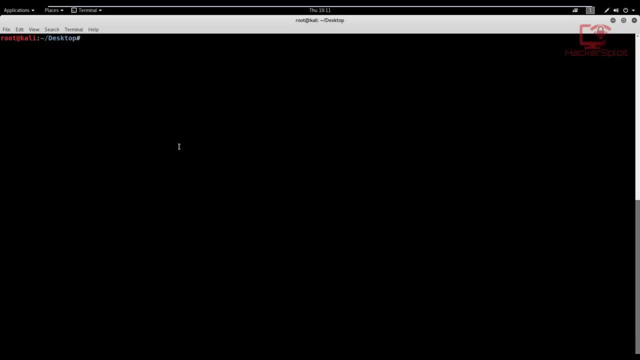 directory into my desktop, And there we are. So now let me just clear that up And we can get started now. All right, we are going to be saving the, the, the data, that is being that we're logging into a file, a capture file or a dot cap file, which they can then be used, which can then be. 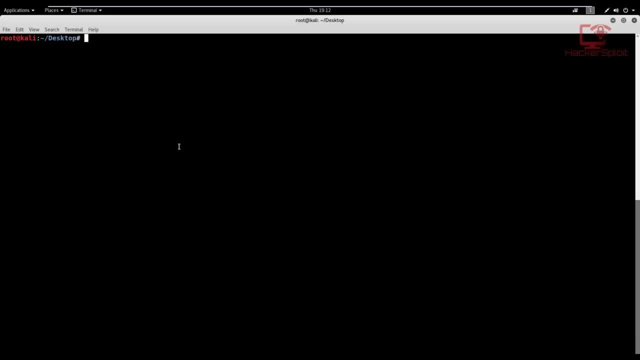 analyzed by tools like Wireshark, But we are really focused on using aircrack to capture the WPA handshake and then crack it. Okay so, I know the video is getting a bit long, but I just want to cover everything here. Excellent, So now we're going to use arrow, dump- ng same commands All. 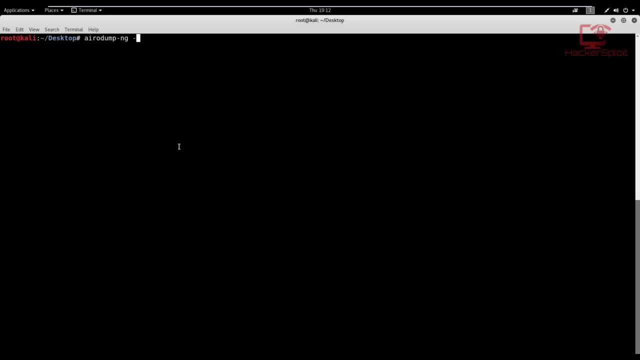 right whoops, arrow, dump ng. And we're going to specify the BSS ID. BSS ID. So I'm going to paste the BSS ID. that's the route, access point, the access point MAC address, And we're going to select the channel, which was: 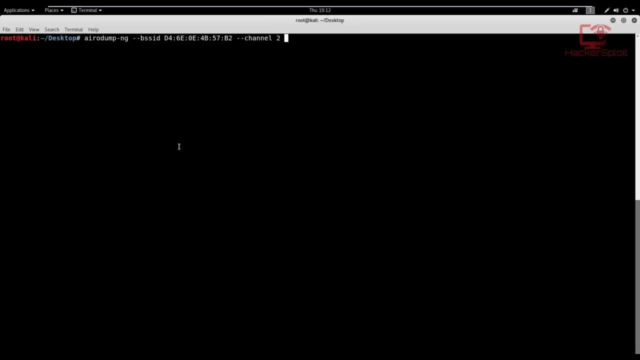 channel, the channel numbers two. All right, And now we need to select the show act. All right. you might be wondering what the hell does that mean? But this is just going to show us the acknowledgement packets. If you've learned about networking, you know that we have your. 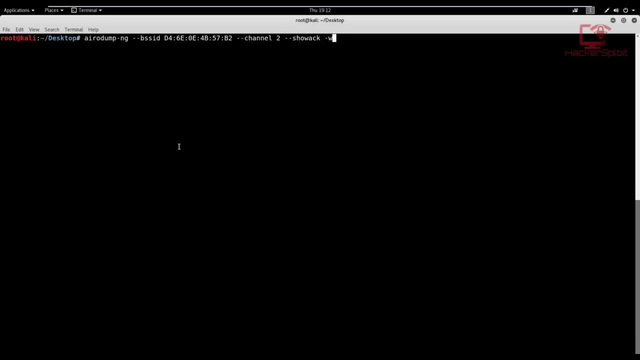 your acknowledgement packets. So this is going to show us the acknowledgement packets And then we want to write. we want to write the output or the whatever data is being captured to a file name. So we select a file name. let's just call it WPA, WPA results, Or actually let's just call it. 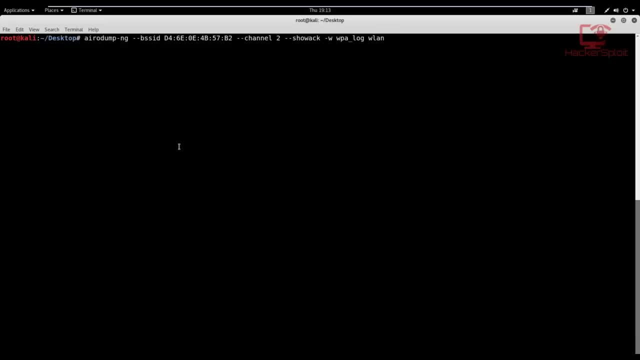 log, because we're logging the data And then we need to select our interface name. All right, so W LAN zero, mon in monitor mode, All right, so let me explain. So we're saying arrow dump, ng. I want you to focus on this access point, which is we have provided the BSS ID. 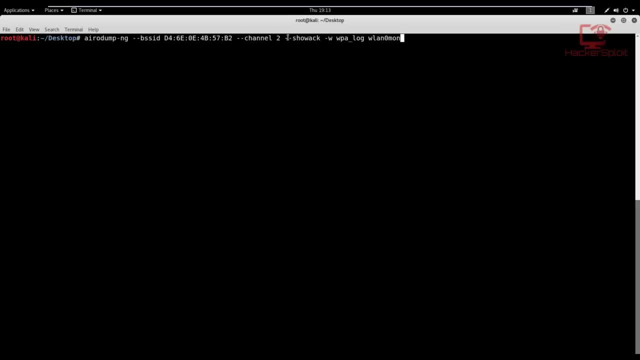 And the channel which is which is the which is on channel two. we now want to show the acknowledgement packets And we want to log all the data into, into this file called WPA log, And it's going to automatically save it into different file formats. The four file format that we're interested in is: 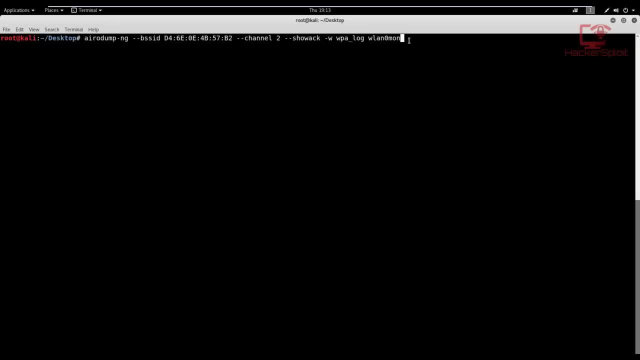 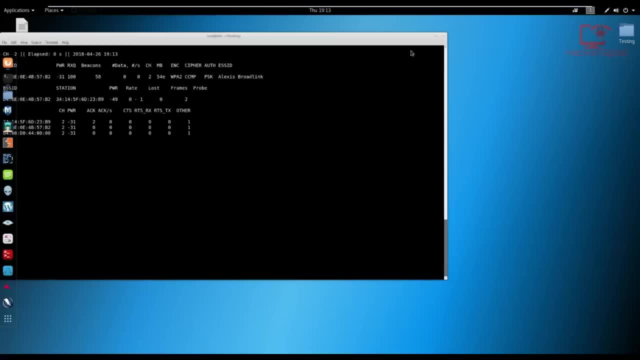 the- the dot capture format. All right, and we've selected the interface that we want to use. So I'm going to hit Enter and it's going to start capturing. it's going to start capturing all the data and it's going to be saving it into a capture file. 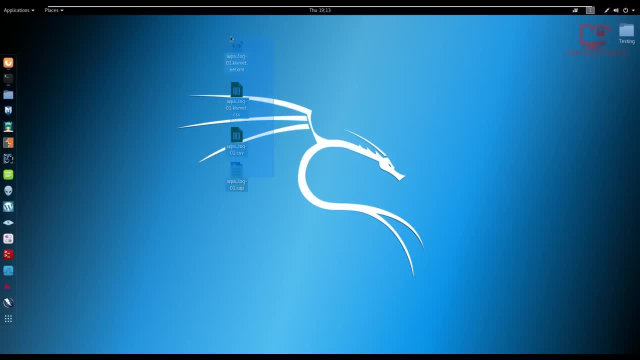 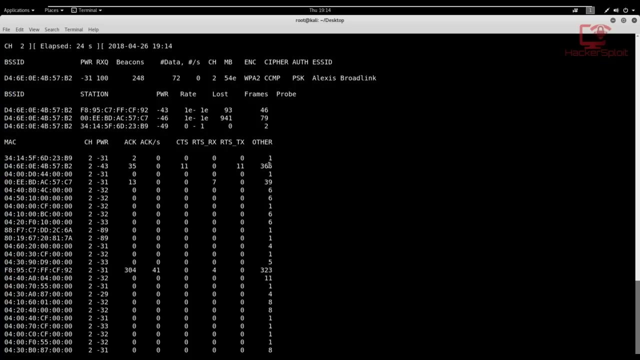 On our desktop, as you can see right here. So if we look at the file, you can see it, saved it in four formats. we have a net XML, CSV format and a cap dot capture extension, which essentially means it's a captured network or traffic. So now, as you can see, it's currently running and it's still capturing. 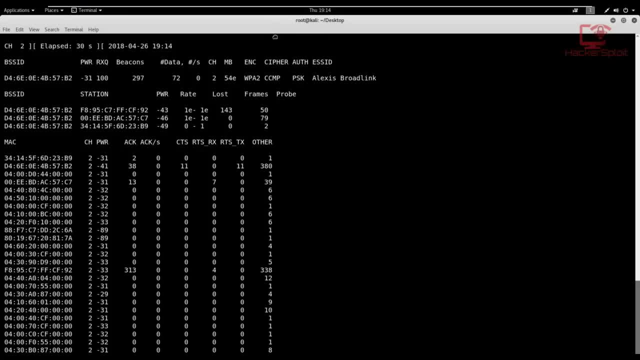 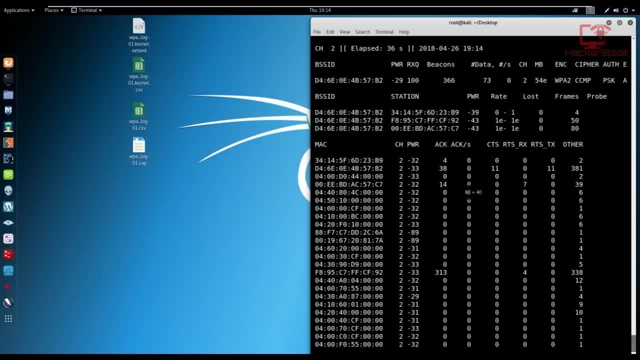 data. So you might be asking: should we actually stop it? No, I want you to keep this running, And what we're going to do is I'm going to open up another terminal. I'm going to leave this running here. Actually, we're going to leave that running. 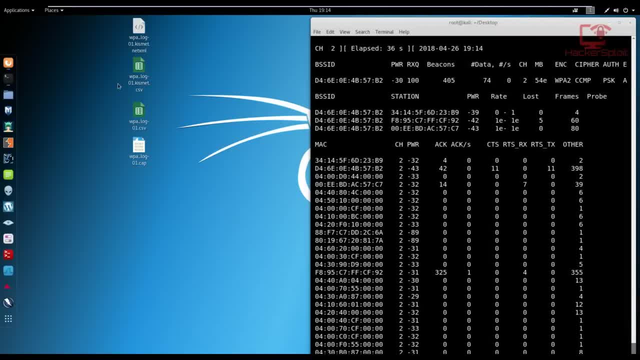 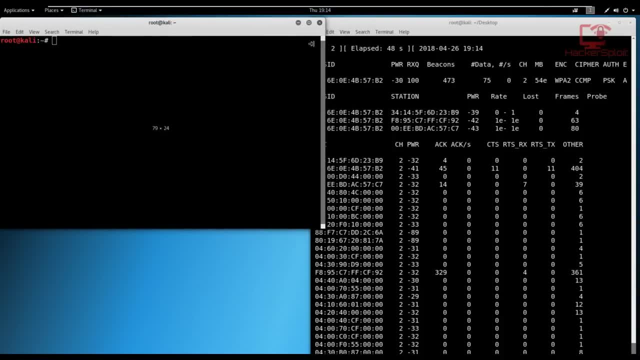 You leave it running because we need it to be constantly capturing data and saving it to this file. Okay, so now we need to open up a new terminal And now we need to perform a D authentication attack. you might be a little bit confused and you might be wondering: what is a D authentication attack? 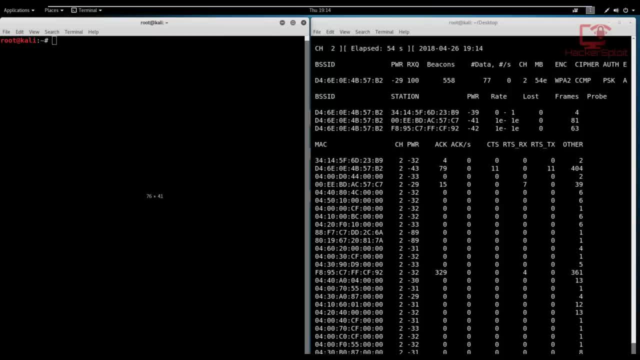 Well, this essentially is an attack where we send a D authentication packets, pretending to be a client on the network, to the access point in in the hopes that we can get a handshake from the access point. Remember, we're not actually connected to the network. 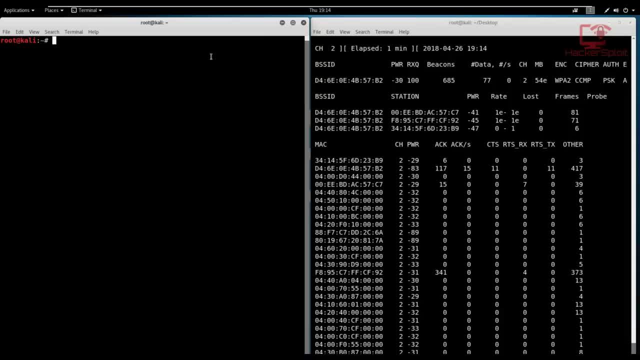 So getting a handshake, very important, And the way we can do this is by performing a D authentication attack to one of the clients connected to the network. So, again, make sure you select a client that is active on the network. So right now the most active client is this one on the top, but I want to use my Nexus. 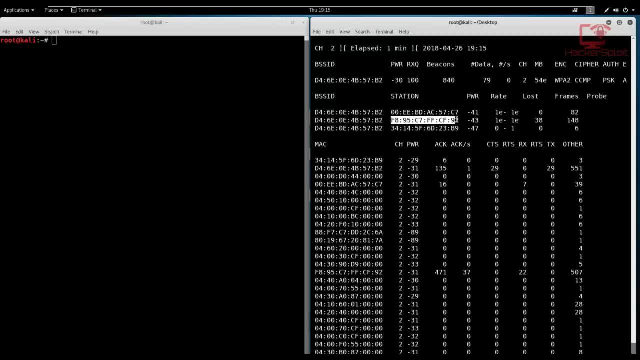 device because that's the most accessible to me. Alright, so this is the MAC address of my, of my Nexus device. So what you want to do is you want to make sure you copy that MAC address. Alright, so just copy it. And now you want to go into the other terminal. 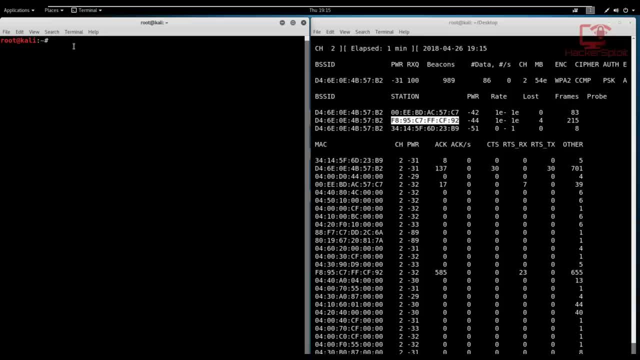 Instance- make sure you don't stop this one- And you need to start entering the following commands: Alright, so we're going to use airplay ng, airplay. Alright, so, airplay ng, although it also belongs to the aircrack suite, airplay ng. And now we need to select zero, which means we're we're using a D. 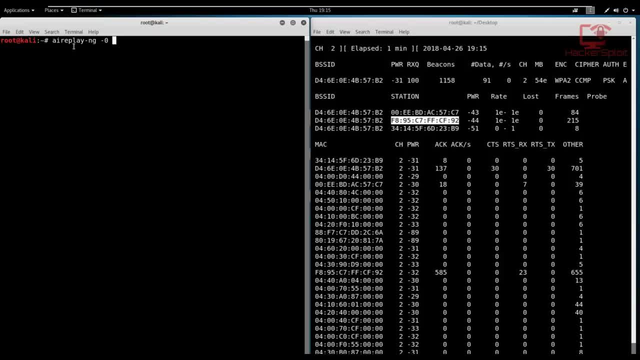 authentication attack. Now we need to specify the amount of the D authentication packets we want to send. Now, if your wireless network, or the wireless network that you're trying to get the WPA handshake, is quite far away from you, you need to increase the amount of the authentication packets you want to send so that there is minimal. 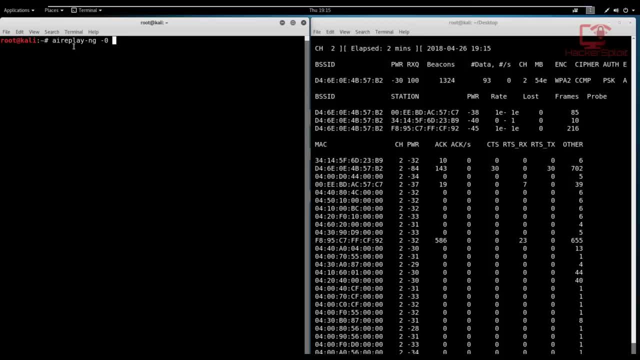 packet loss. And if there is packet loss, you're you're constantly sending so that there's a higher chance of you getting the WPA handshake. So usually I would specify, if it's quite near you, about 20 at the authentication packets. And then now you need to select the access point. The access point MAC. 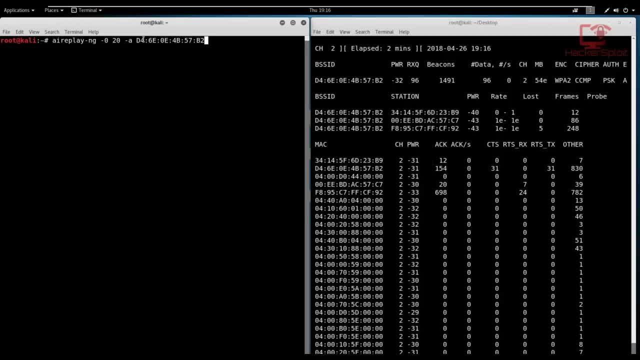 address which you just specify, which is right here. So we just hit Ctrl C and we can paste that in there. And now you set you need to specify the client MAC address, So the you just can just select a random client on the network, one that is sending. 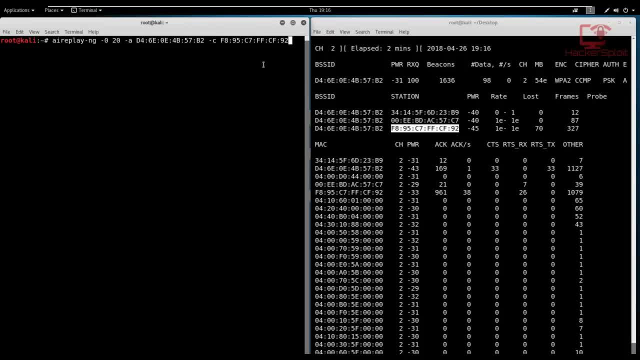 more data preferably. So let's copy that And we paste that in there. And now we need to essentially specify our interface that we want to use, which is lan zero mon in interface, in monitor mode, and hit Enter. All right now, when I hit Enter, it's going to start sending the D authentication, the D authentication packets to: 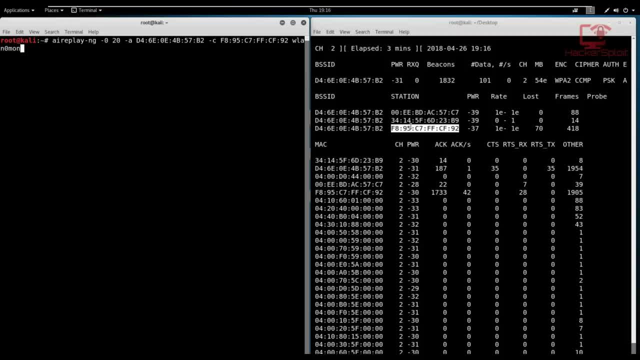 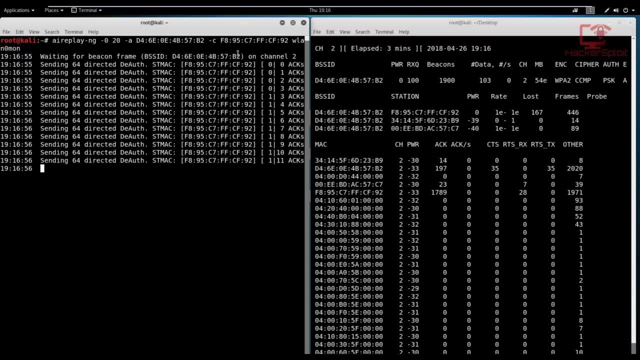 the router, which is essentially going to disconnect the client that you've just selected, the MAC- and it's going to disconnect it from the network temporarily until all the D authentication packets have been sent. So I'm going to hit Enter And, as you can see, it's going to start sending the. 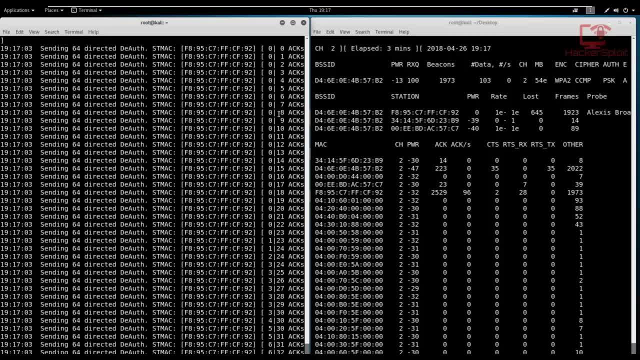 D authentication packets And once it's done, what? what should happen here is, as you can see, it started sending them and, for some reason, will actually. it should have actually sent them by now And for some reason, we're getting an. 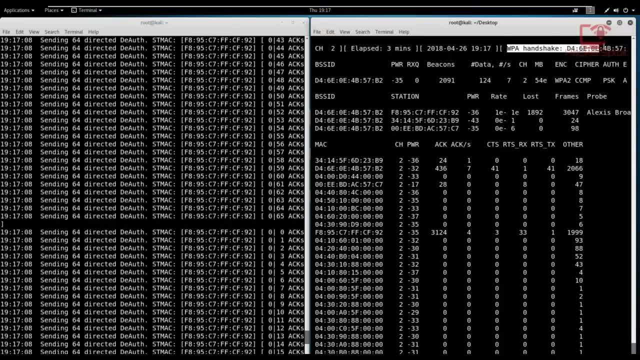 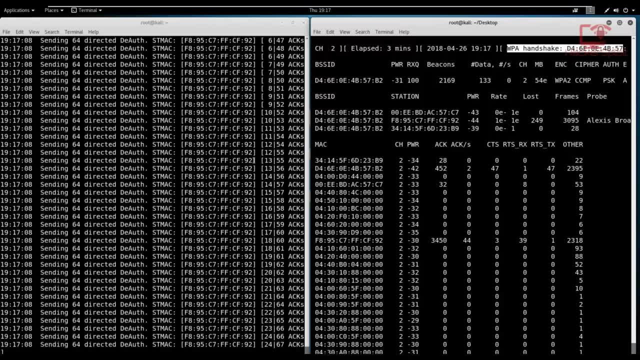 error here. There we are. it's still running, it's still sending And, as you can see, we have captured the WPA handshake right here. And once we have this, you can start using A crack NG to crack it. So I'll show you how to do. 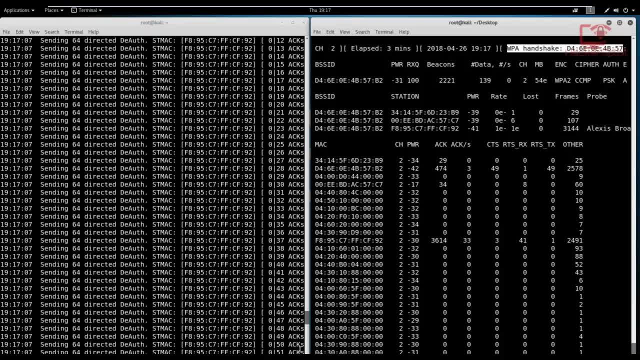 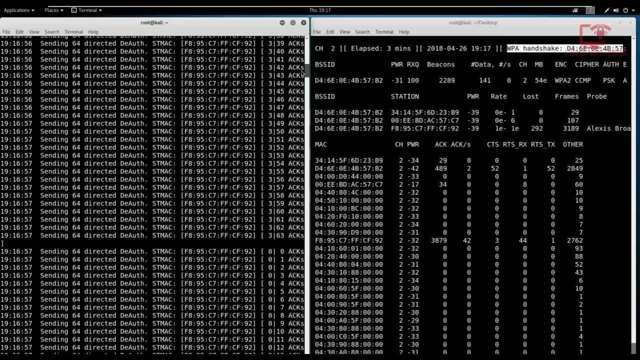 that right now, What you can do is, once the D authentication packets have been sent, right here. for some reason we were experiencing packet loss, So it said quite a few more because they was packet loss. And there we are. you can see that it. 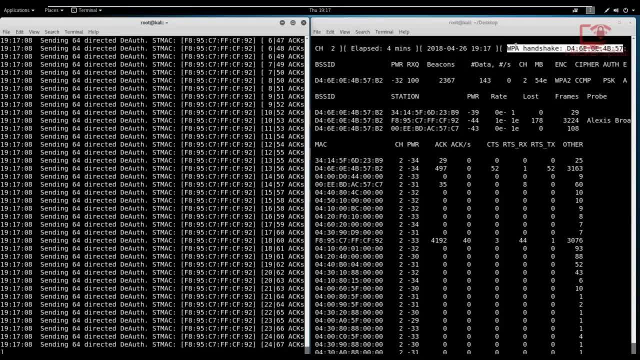 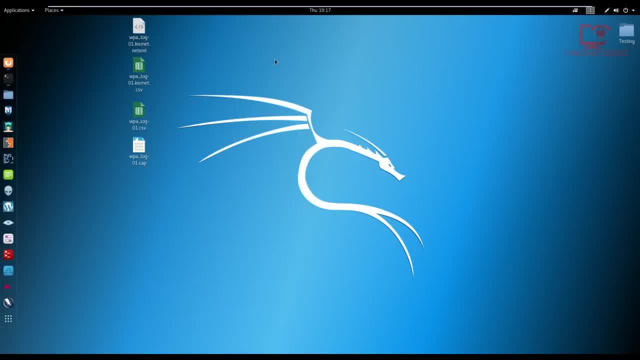 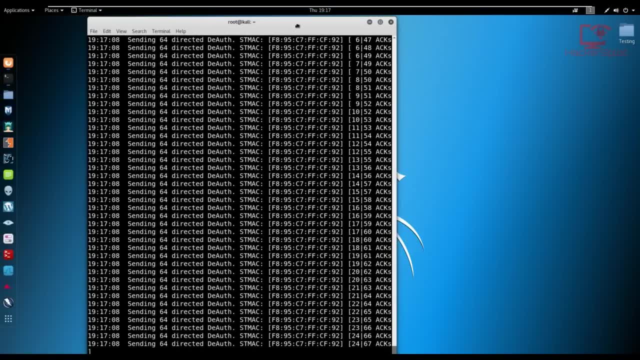 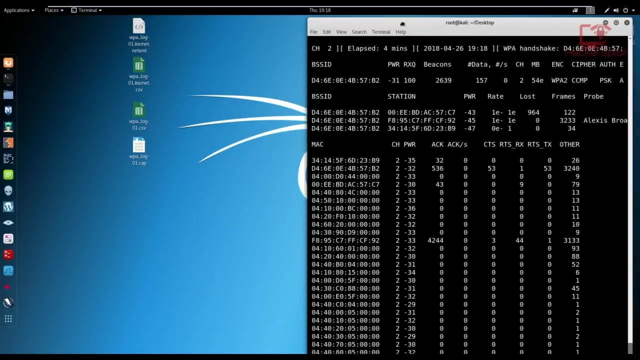 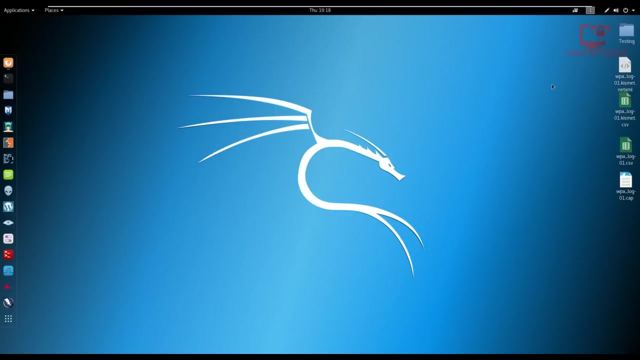 has sent the belt packet And once that is done, it will give you the ability to capture the WPA handshake while this is still running. So it's captured, the WPA handshake- WPA handshake- in the dot capture file here. Okay, now, this may seem a bit confusing, But once we have the WPA handshake, we can now use aircrack to crack it. All right, but I'm going to show you a better way of doing it. You can use aircrack ng and you can. you'll be limited to using a brute force attack or a dictionary attack. Now I'll show you how to do this with an awesome framework in my mind, and I'll show you what it's called. That framework is called the airgeddon framework, All right, so I will have the link in the description, You can. 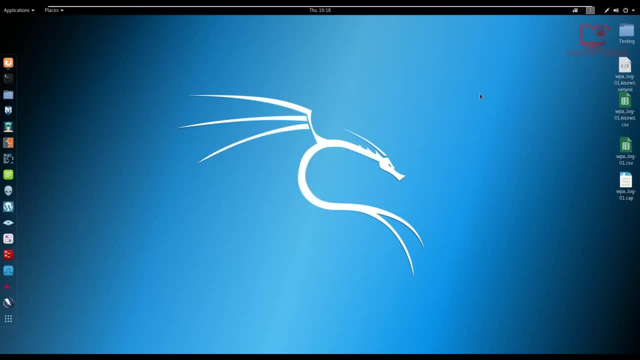 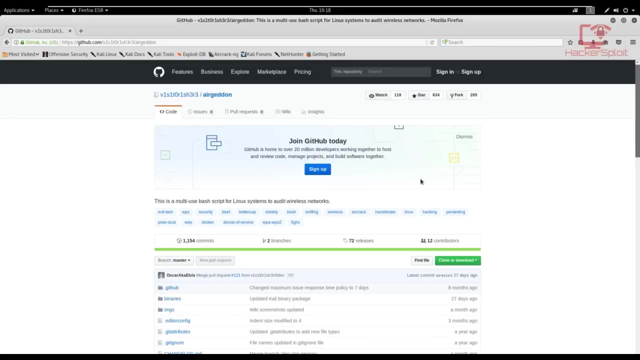 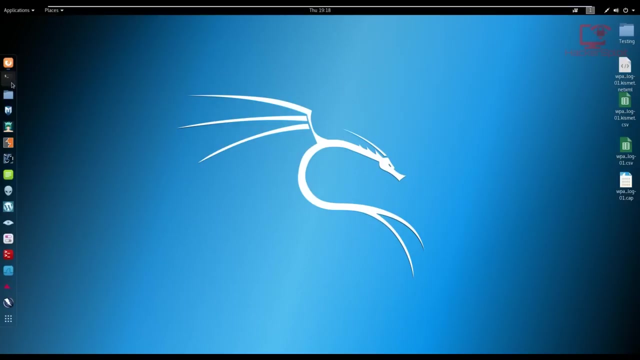 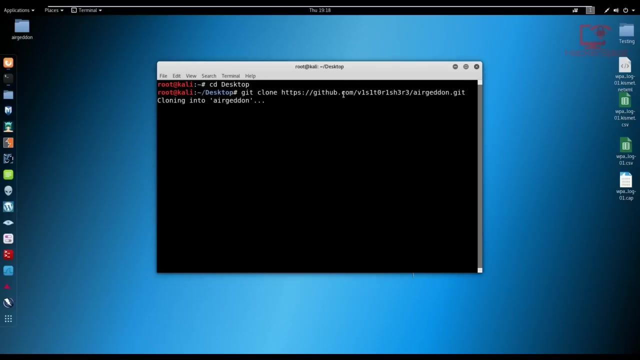 find it on GitHub, And the reason I like this is because it keeps everything centralized, and I'll be showing you the great amount of attacks that you can perform. All right, so open the link in the description. It is the GitHub repository. So just clone the repository. I'm just going to copy the URL right over here. If it doesn't copy, just copied manually. And again, I'm going to save this to my desktop. So cd, desktop, git clone. I'm going to paste it in there, the URL, and let it clone. It's quite a large file, I would say So. 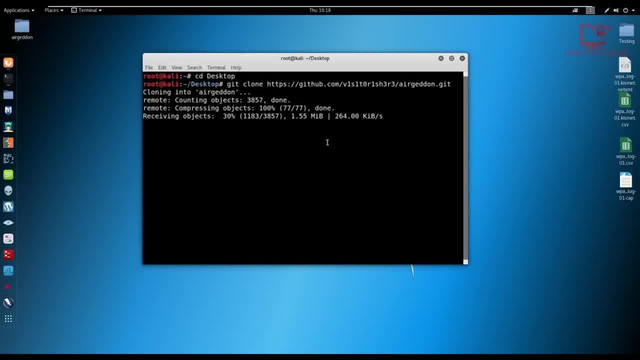 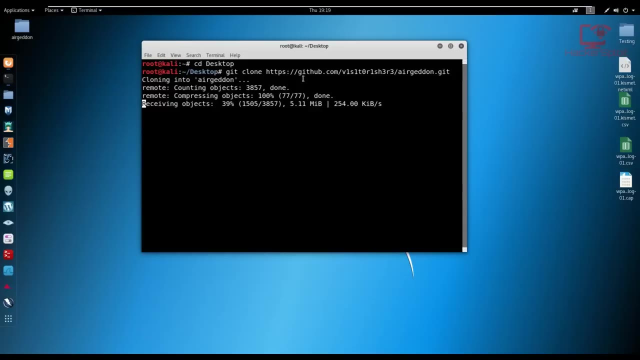 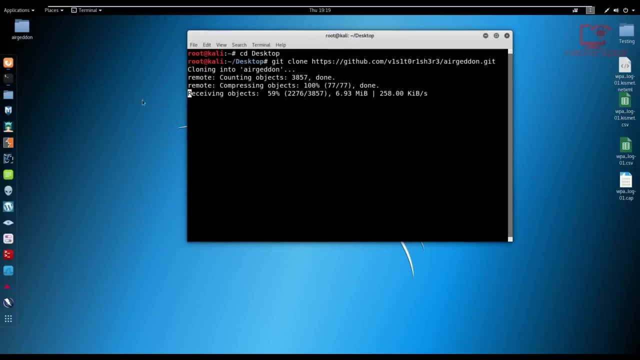 give it a few seconds to copy again. please pardon my internet connection. I know it isn't the most favorable connection right now, But it shouldn't take too much time to get all the files. So let that complete downloading. And I know the video is getting a bit long, But, as I said, I want to cover everything in this video. Okay, So let that complete downloading. and hopefully we aren't. it isn't affecting anything here. I'm waiting, I'm waiting. In the meanwhile, I can show you that you can use aircrack ng to 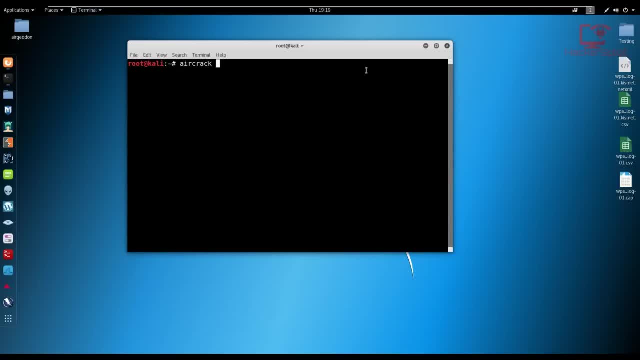 actually crack the, the file here. So what I'll do is I'll show you aircrack ng If you want to start cracking the, the wpa, and check aircrack ng. you don't need to specify the, the Capture file which we used over here. So 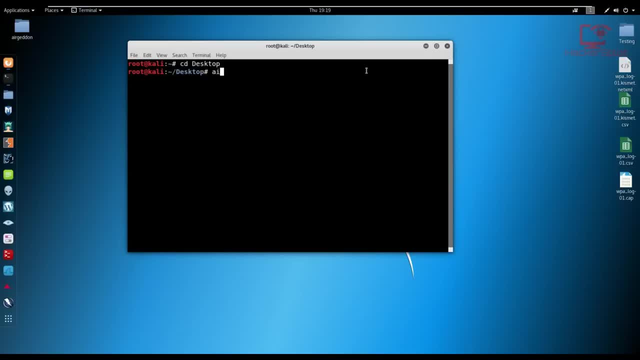 in order to do that well, I would have to actually say cd desktop And there we are. So I say aircrack and g crack, ng And I select the file which is wpa log, one dot Capture And then select oops, dot capture. I select the word list file which I'll use, the rock you word list which. 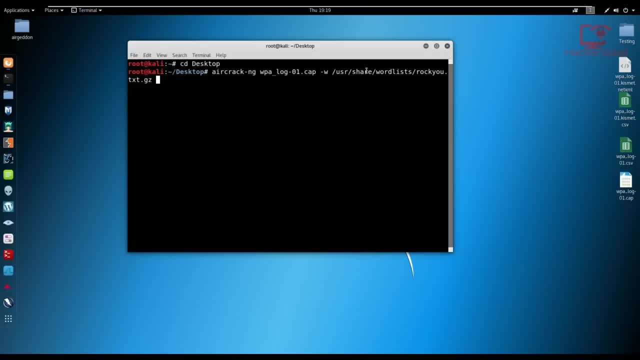 is in user share word lists and the rock you dot, txt, dot gz and probably it will not work, as I said. as you can see here, it only went through. it essentially performed a dictionary attack. now, this is what I was talking about: the chances of you cracking it after you've captured the. 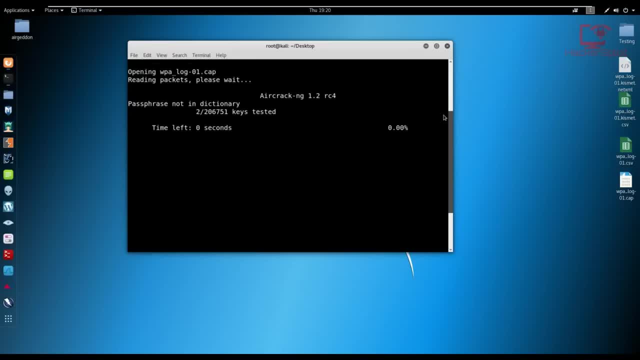 handshake because, again, not enough data has been captured. you'll probably have to leave this run in for about a week. that's what people don't want to understand. there is no five-minute hack. well, there is, and I'll be showing you that in a few seconds. that's why I'm actually downloading. 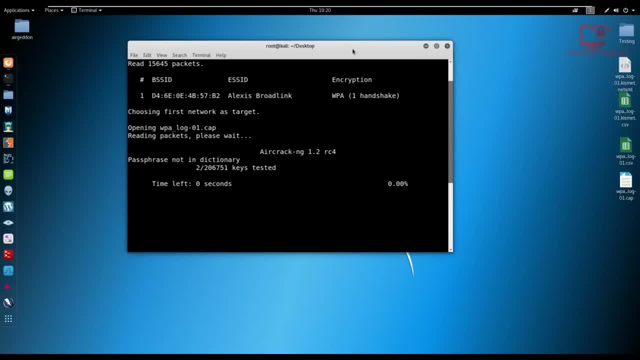 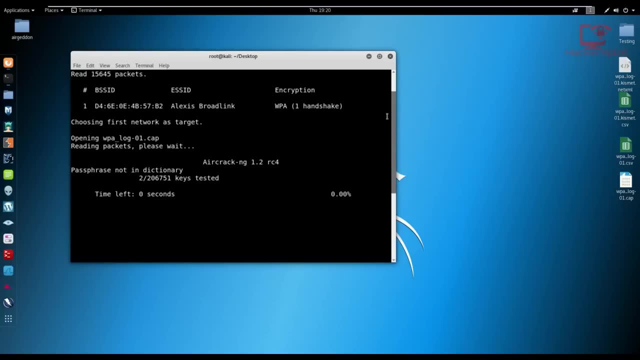 airgeddon will. I'll explain why this. you have only captured one handshake and if we kept the data running- which means if I would have kept the other terminal that was capturing the data- and we kept on sending the deauthentication attacks and we captured maybe, maybe ten handshakes, then we 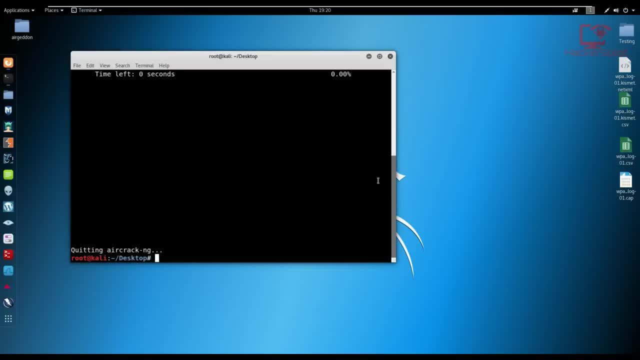 could have actually performed the brute force or the dictionary attack, but this is a very old way of doing it and the chances of you cracking the password are, to be honest, quite low. I would say you have about a 10% chance of getting the, the access point key. okay, so we're just gonna close this up and hopefully, 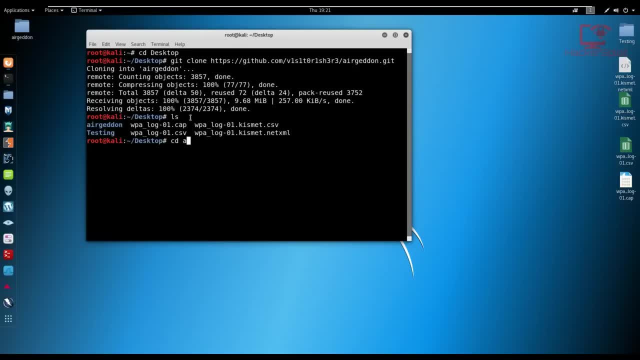 airgeddon has been downloaded- awesome, so I list the files. yeah, we want to go into airgeddon. airgeddon- let me list the files in there. there we are. we have the airgeddon executable, which is currently set to be not executable, so we have to change permissions. so chmod. 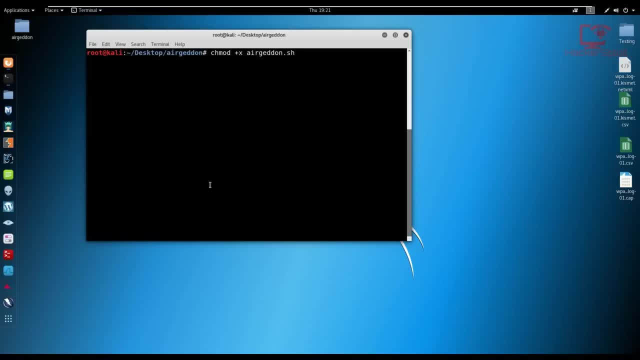 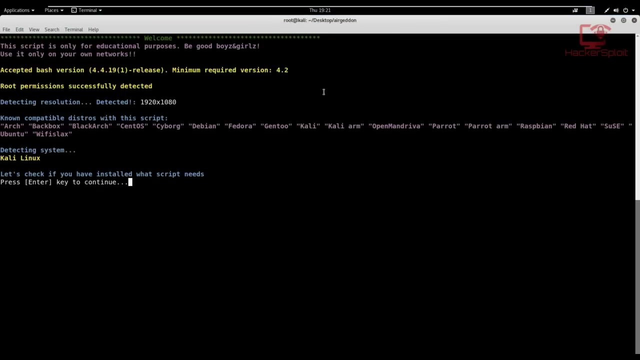 plus X and airgeddon dot shell. I'm gonna list the files there and we're gonna launch it. so, airgeddon, and we're gonna launch it there and it's gonna open up airgeddon. now, this is a fantastic tool and I'm gonna show you right now how you can actually go about doing stuff. so I'm gonna hit. 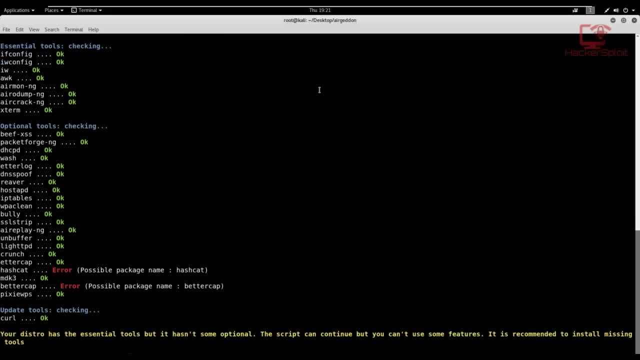 enter to continue and it's gonna start. it's checking for the essential tools. now don't worry if you're missing a few tools like hash cat or a better cap. well, hash cat is very important, I think. in the event, you want to use GPU cracking, which most of you have actually recommended, and 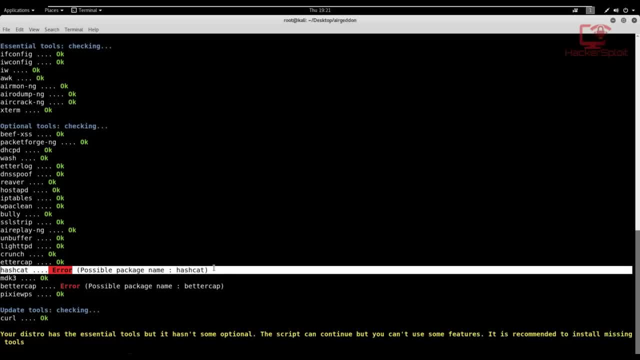 I'll be actually going through that. you know, using rainbow tables, I'm actually finding a quadro GPU, which is the best one, as they are more in tune with with performing more enterprise type GPU calculations. so I'll be getting to that in another video, but for now just make sure that you have the 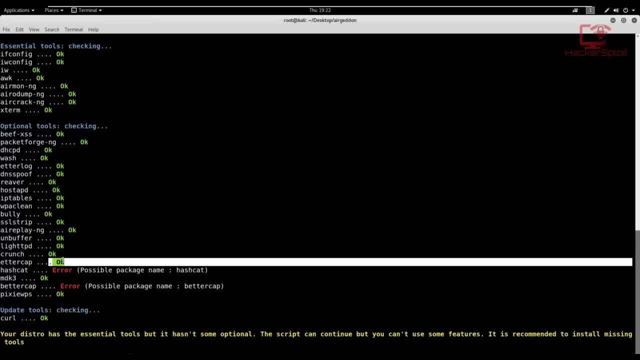 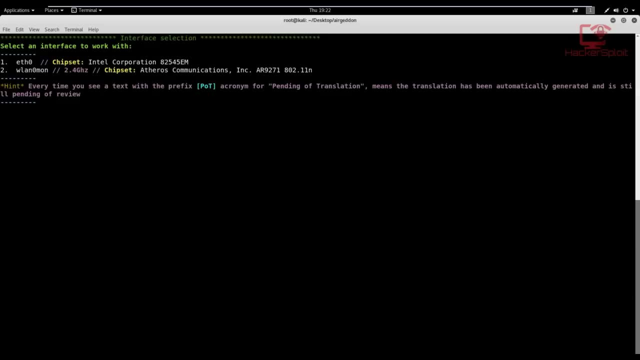 most important things like Reva and bully, all that good stuff installed, you have crunch at the cap. it's it's important if you're performing an evil to an attack. that being said, let's not waste any time. let me just hit enter and it's gonna check for a new version and if it doesn't find one, just 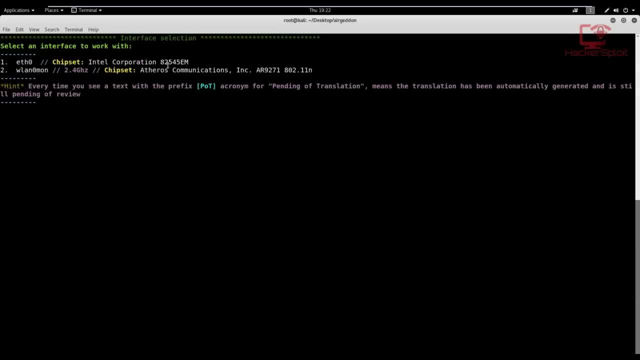 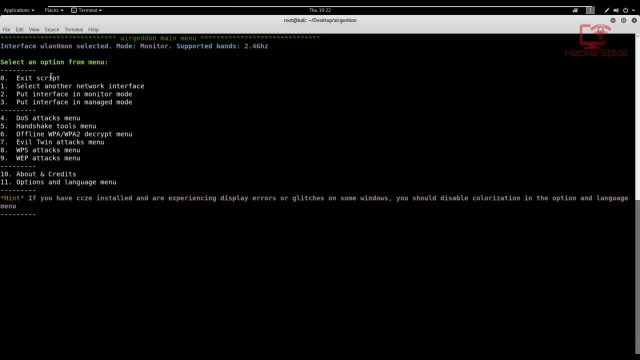 hit enter to continue. and now it's gonna ask you to select an interface to work with. I'm using Ethernet and my lan0mon, which is already in monitor mode, so I'm just gonna select the second one. and now the awesome thing is here, you can see. it's going to give you a menu and it's gonna say: 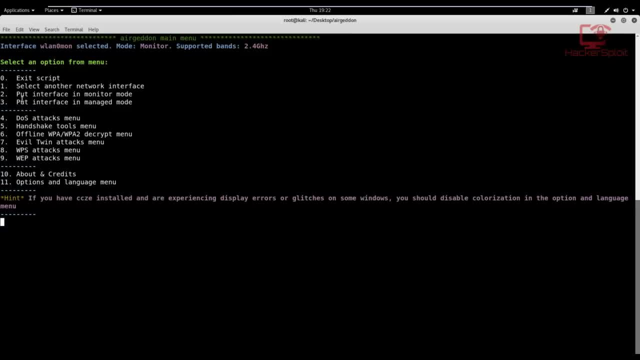 is 2.4 gigahertz, and the great thing is, you can select another interface. you can also put the interface in monitor mode and you can put it back into manage mode. this is the thing I love about. it just makes everything a whole lot easier. now you can see the attack types that we have. here are: 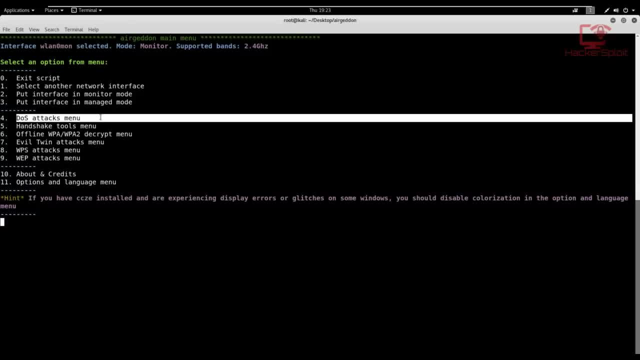 very, very enticing. you have your DOS attacks menu, which essentially perform a denial of service to a specific access point. this is great, for you know trolling. you can also perform denial of service attacks to devices on the network even if you're not connected to the network. and you're not connected. 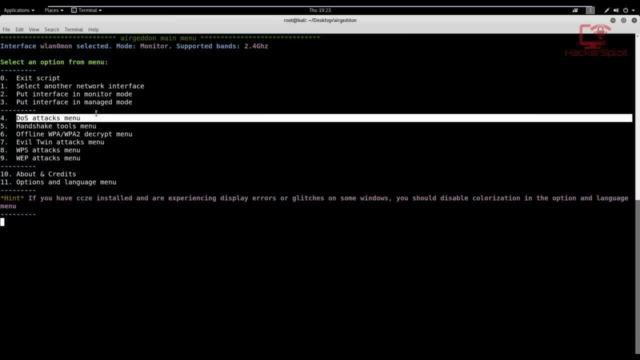 to them so you can see how much damage this can cause. and one of the great things- as I don't know whether I actually shared that video with you guys, but there was a use- using one DEF CON video, or when I was watching one of the DEF CON videos, is a guy was actually able to just perform a denial of. 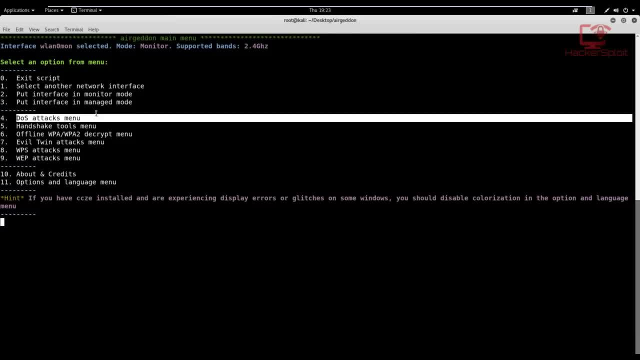 service to a drone that he was not even connected to. so his neighbor actually used to really bug him with the drone you know flying around spying on people using you know through their windows, and that drone actually had its own WPA network connection between the drone and the controller and obviously, because he's not connected, 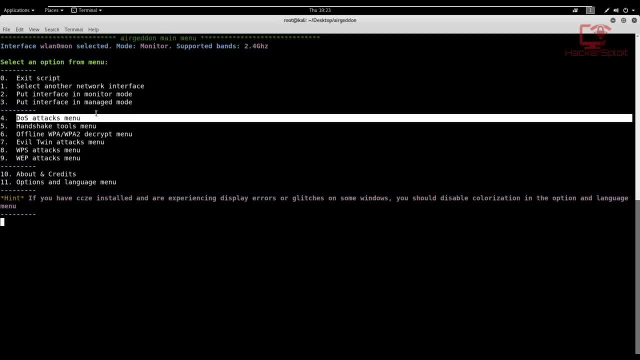 to it. he was able to quickly scan it and then specify that network and then the client being the, the remote controller, was able to perform a denial of service to the controller, which means that the drone was no longer in his control, and you can guess the amount of damage that that can. 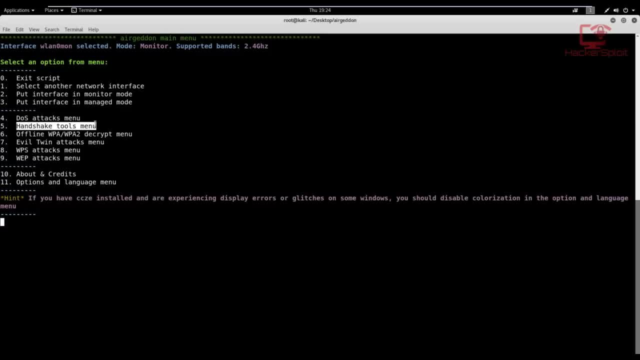 cause. that being said, let's stop wasting time. if you want to perform your own handshake, if you want to capture your own handshake, this can also be done with airgeddon. so let's actually do that right now. so let's hit five, and now it's going to say: well, the most important thing you're going to do, 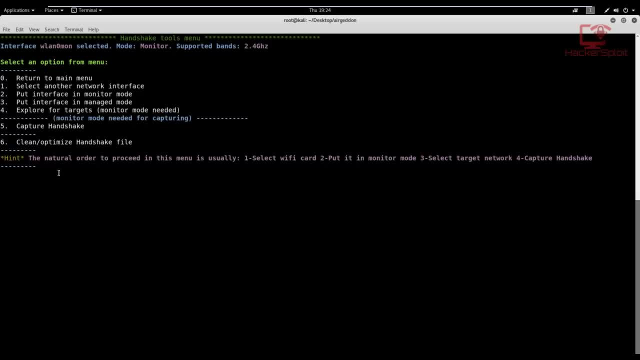 right now is you need to explore targets, which means you need to specify the network that you want to capture the handshake on. in this case, we're just going to hit four to start exploring for targets and it's going to say: WPA filter enabled in scan. yeah, just hit control C to stop. 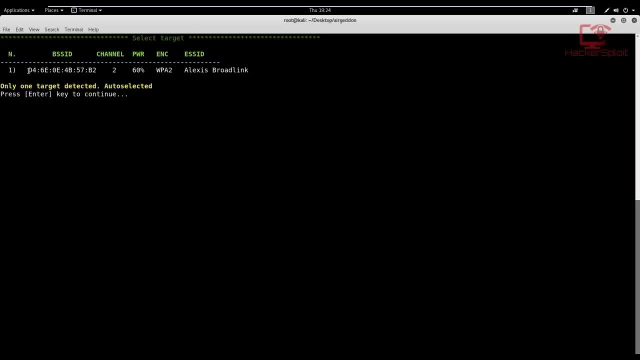 so I'm going to hit enter and it's going to start capturing the the network, and I'm going to hit enter and it's captured the network that we want to target, and this displays the information much better. you have your BSS ID, the channel power encryption and the ESS ID, which is the most. 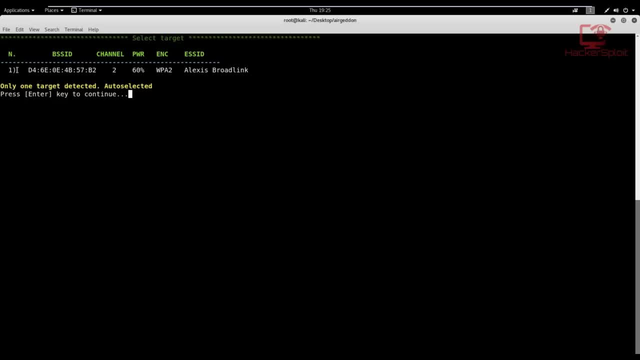 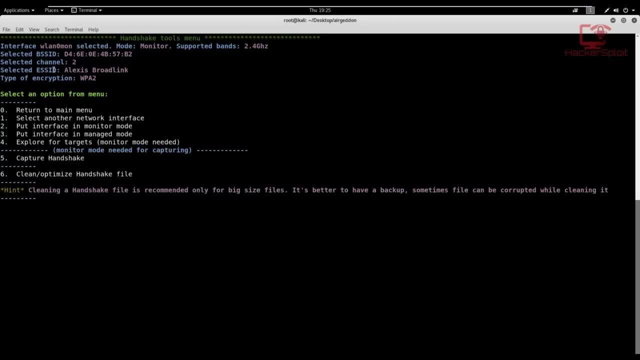 important information. all right, so it's going to say only one target detected, remember. if you have any other, it's going to give you the number so you can select it from there and I'm going to hit continue. so it's selected Alexis Broadlink, and it's going to give you more information about it. 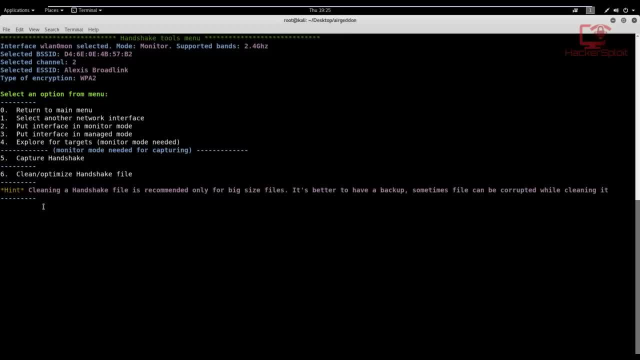 up there. now we need to capture the handshake, which is here. so we can say five to capture the handshake. so let's hit five and I'm going to hit enter to continue. all right, and now it's going to ask us what type of deauthentication attack you want to perform. I usually like the deauthentication of the attack. 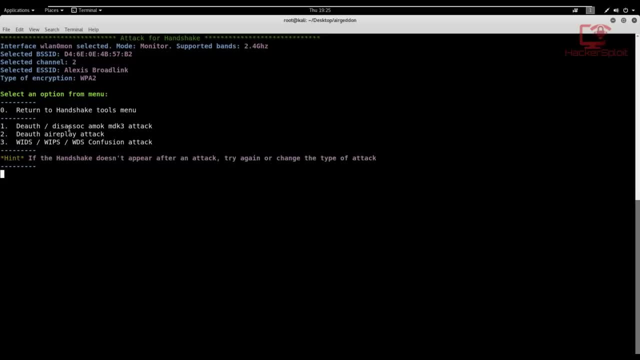 that is done with airplay, or you can use the DS. the DS, the disassociation attack that is performed by mdk3, which is not that effective, to be honest, especially against newer routers. so, deauthentication, airplay attack. so I'm going to select the second option and I'm going to hit enter and I'm going 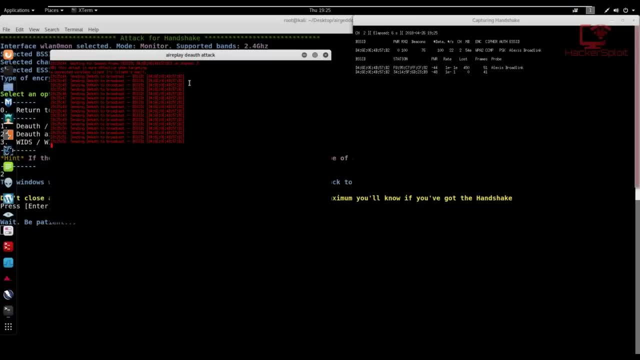 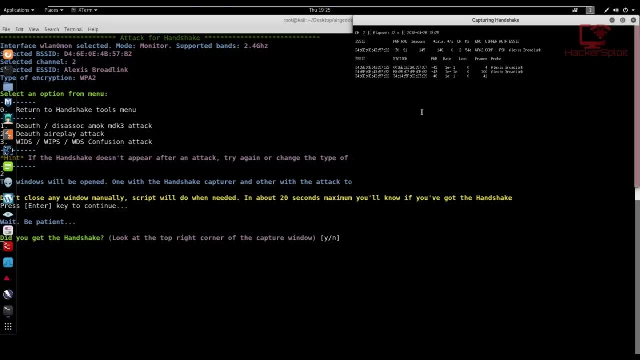 to go back. as you can see here, there we are and you have to wait now until the deauthentication package has been sent and you were able to capture a WPA handshake. all right, so apparently we were not able to capture a a handshake, and yeah, we did. there we are, we were able to capture a handshake. 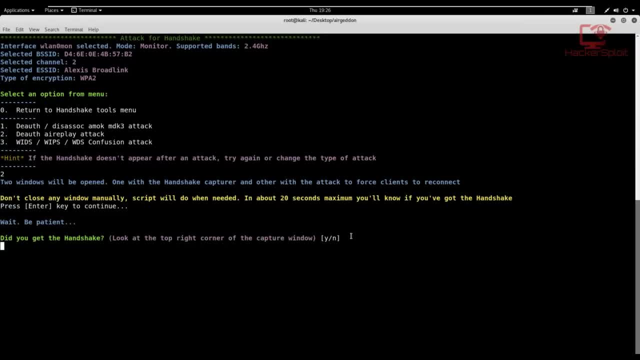 so now it's going to ask you: did you get the handshake? it's going to say: look at the top right corner of the capture window: yes, we were able to capture a handshake, so I'm going to hit yes, congratulations. type the path to store the file or press enter. 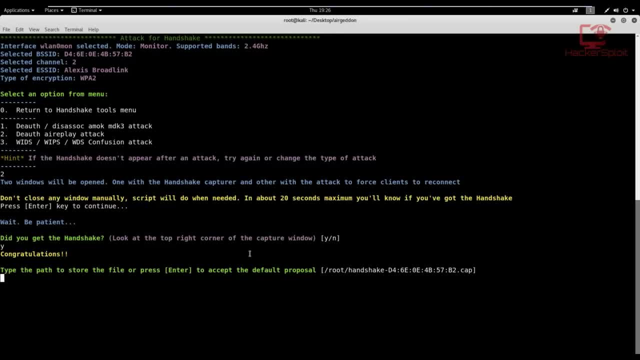 to accept the default proposal. so it's going to save it in root handshake and it's going to give it its own name. so I'm going to hit enter. all right, so the path is valid and you have right permissions. script can continue. so you want to hit enter to continue and now you can go on and 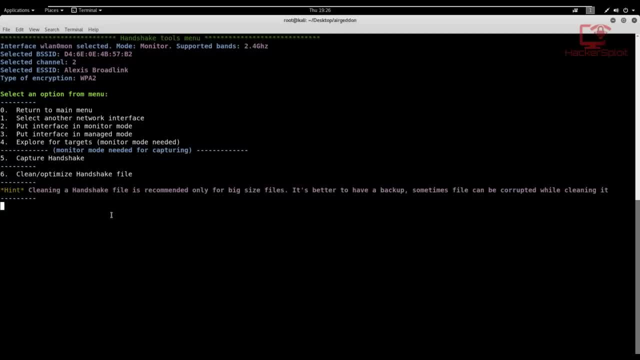 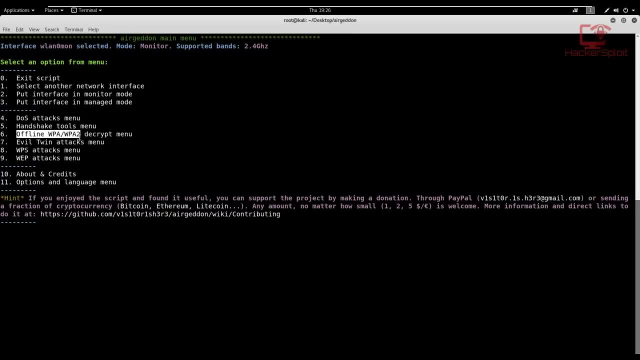 clean or optimize the handshake file, which we don't need to do right now because, again, we have not captured a lot of data. so now we can finally go back to the main menu and we can see, we can look at the offline WPA, WPA to decrypt file. and we can go back to the main menu and we can see. 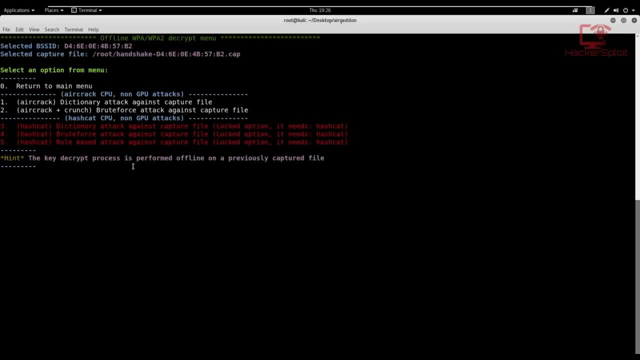 we can go back to the main menu, which is where we can perform the cracking. so I'm going to hit six. and now you can see if you have a hashcat installed. you can use a hashcat to well. it's going to use your central processing unit or your processor, and if you have a bad processor, then it's. 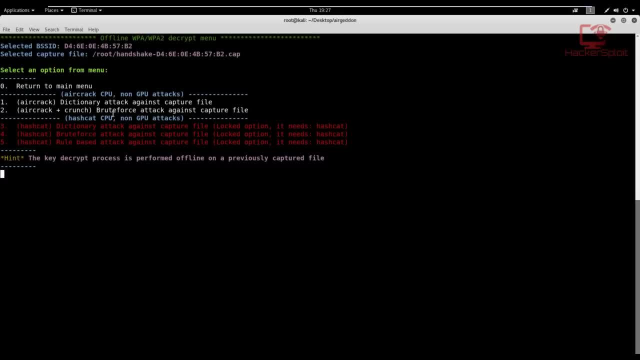 going to take a while, but I'll be showing you how to do it with a hashcat. if you want that tutorial, just comment down below and I'll be sure to do it. you then have your non GPU attacks again. air crack ng is the best option here now. what I would recommend is that you go for 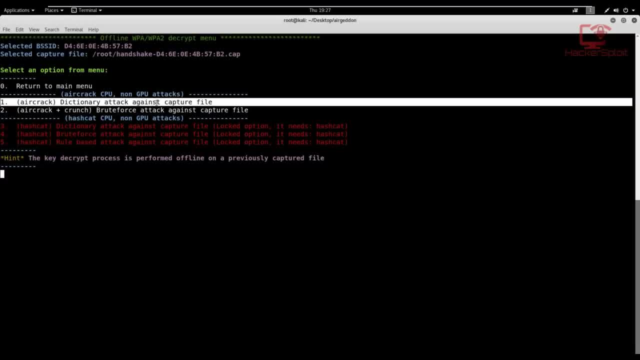 the air crack plus crunch. this will perform a brute-force attack. dictionary attacks will only test the, the current combinations that exist within the within the wordlist or the password list. alright, so I would recommend that you go for option two, which is air crack plus crunch and this: 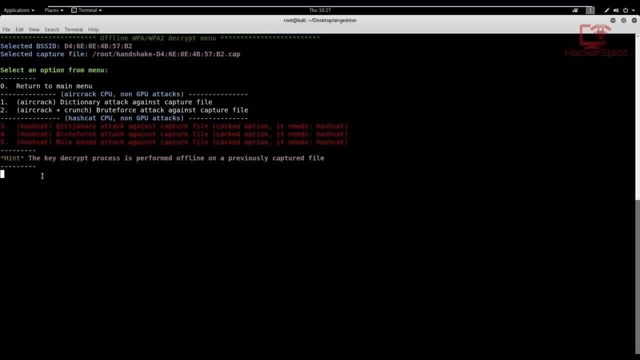 has about a 60% of cracking the key. in my opinion, now again, you might need to leave it on for a few days and some of you might be thinking: what the hell man? that's way too long. and the truth is, if be one 醫. 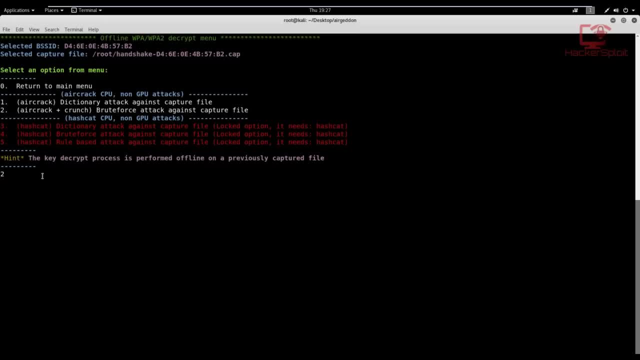 h, k, k, x k network. that's how you do it using the WPA handshake, right? so I'm gonna do. and do you want to use this already selected capture file? so it's gonna ask you if you want to use the capture file that was captured during the session. I'm gonna hit yes and you already have selected the BSS. 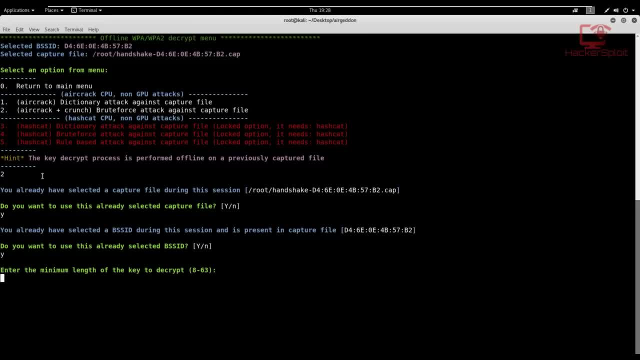 ID you want to, and it is present in the capture file. do you want to use this business ID? of course we do. what is the minimum length of the key to decrypt? all right, so now it's going to ask you to specify, just in your own opinion, what you would expect. the minimum, the minimum length of 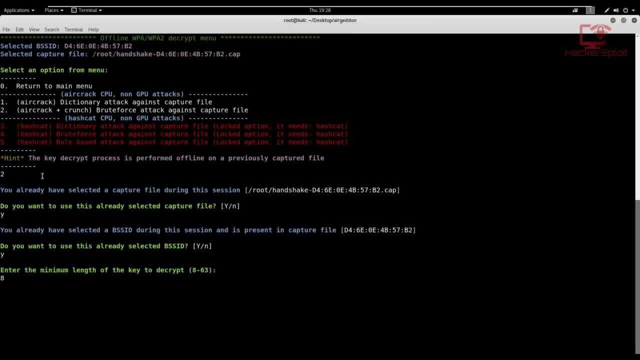 the key is. in my opinion, I would say the minimum is 8, because not many Wi-Fi keys, Wi-Fi routers, are going to let you set a key that is, or a password that is below 8 characters. all right, so I'm gonna hit 8 and the maximum I would say- and no one has a Wi-Fi password that is over 20. 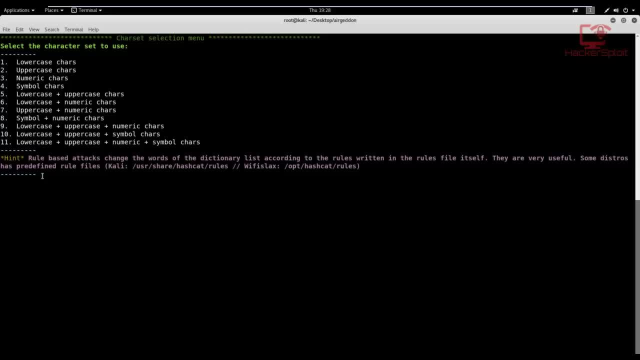 or actually 15. so I would, I would go about 15 and I'm gonna hit enter now. the most important thing, because it's using crunch to generate your own type of word list, dependent on what you would specify. now, most people would usually go for lowercase and numeric. 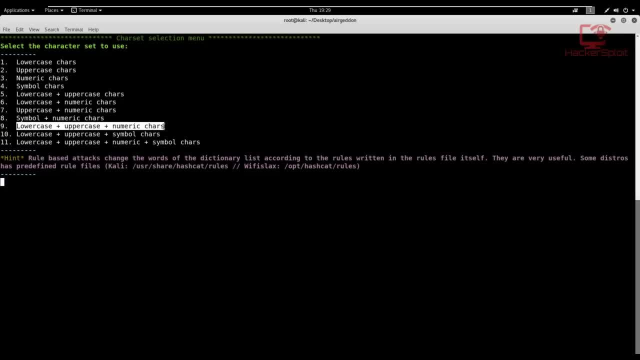 characters or a combination of lowercase plus uppercase and numeric character characters. in my opinion, I've set the password to be quite easy, which, in you know, involves lowercase plus numerical characters. so I'm gonna select option 6. you can go and select whatever you want. it's. 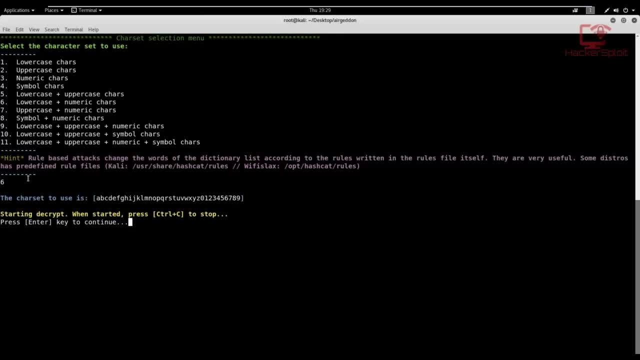 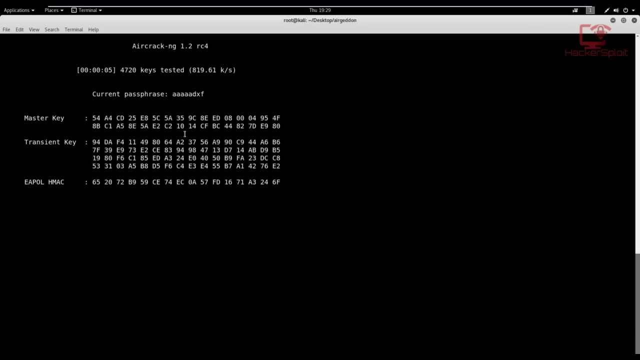 gonna just generate it automatically with crunch. so I'm gonna hit 6 and it's gonna start the decryption, the decryption process and, as you can see, the character set that is going to be using ABCD, the alphabet, and your numerical characters. I'm gonna hit enter. it's gonna start generating the word list with crunch and crunch. 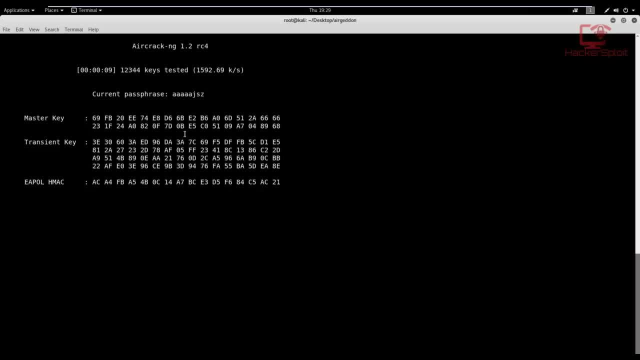 will now generate and the cracking process has begun. so again, there you are. it will use air crack ng to do it for you automatically with your own word list. this is the awesome. the best part about it is the word list can be specified to account for the 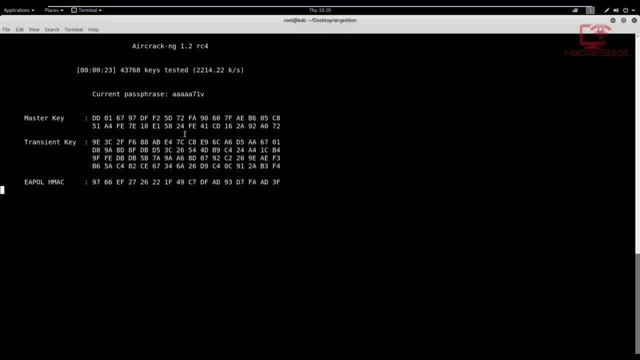 type of characters you would expect in a in a modern Wi-Fi password. so, again, you can see that this is gonna take- yeah, it's gonna take a while, so I would recommend that you leave this on for about two days. in my opinion, it takes about three to four days for a Wi-Fi password that has eight. 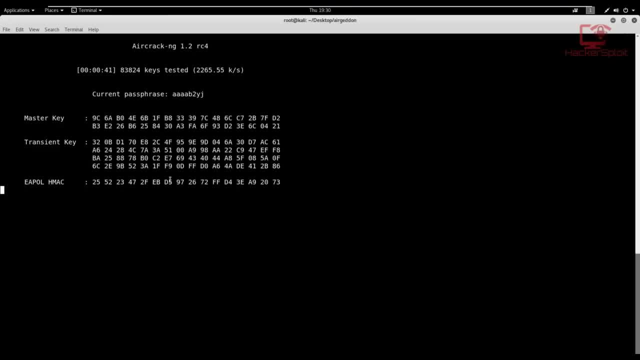 to about 15 characters, again, not that complex. if they are symbols, then it gets even more complex. so you can let this run and once you're done, it'll give you the key. if you're lucky, as I said, the key is 60% if you have specified the right character set. if you're specified a wrong, 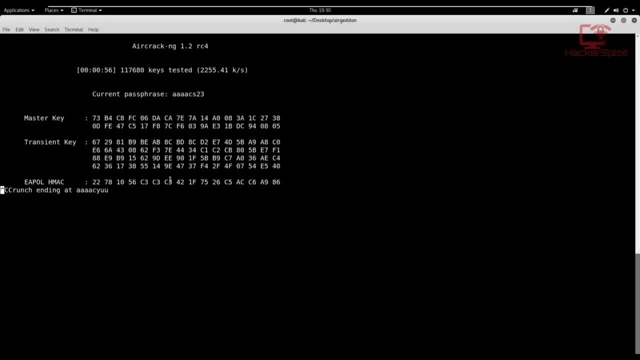 character set, then it'll all go down the drain. so I'm just going to control C and let it just end. don't worry if it gives you this weird thing and it's going to ask you: interruption detected. you really want to exit? I'm going to. yes, and do you want to preserve monitor mode? yes, I want to. 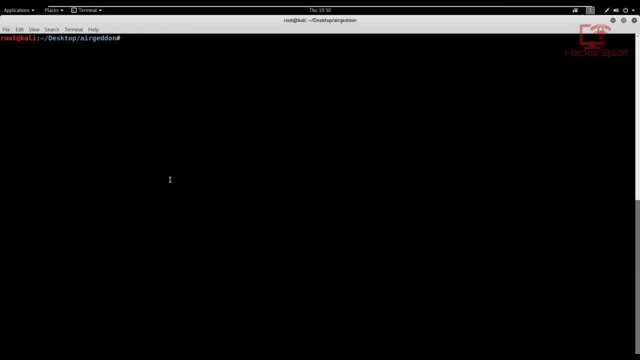 preserve it. I don't want to turn it off. all right, so now let's look at the WPS. all right, the WPS attacks and I'll explain why. most people who buy routers have the WPS feature enabled and they do not disable it. what does WPS? what does it mean? WPS essentially stands for Wi-Fi protected. 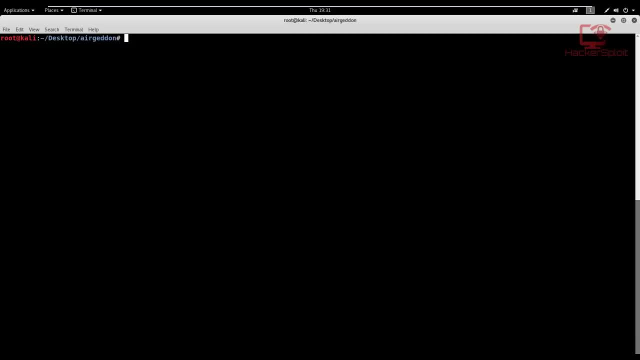 setup, all right. now you might be asking: how does this work? you might have heard of it, what WPS has. a WPS pin, all right, the WPS pin. well, essentially, WPS only works for uh, for wireless networks that use a password, and what this means is uh, WPS essentially allows you. 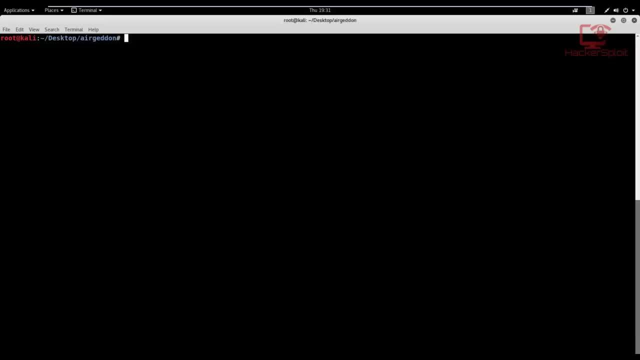 uh to connect using the WPS button on your router and essentially uh deals with uh, a key or a pin. all right, so cracking the WPS pin is essentially it's an eight-digit pin, that uh, even if your router does not have a the, the access point does not have the WPS a button. 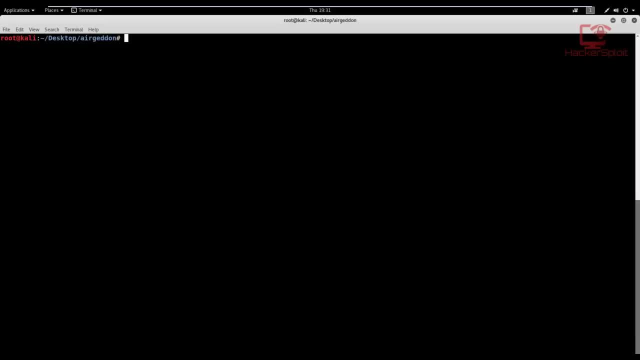 you can still crack it and that will crack the password for you using an authentication attack. all right, so usually people leave it on. now, the great thing about a WPS pin is, once you crack it, once you get that pin, the network is yours for life. It's yours for life, That's because you can never, ever. 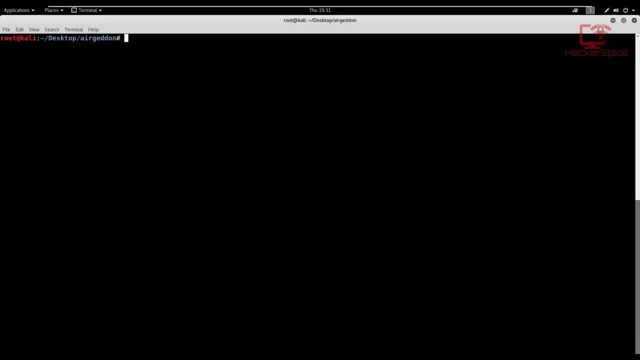 change the, the, the WS pin in older routers. in modern ones, they've actually allowed you to do it, But most people won't even know that it was cracked using the WS pin, the WPS pin, All right, so I'm going to show you how to do that with airgeddon. So let's, let's launch airgeddon again. 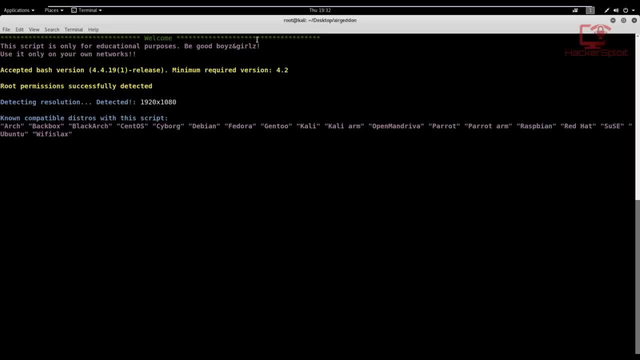 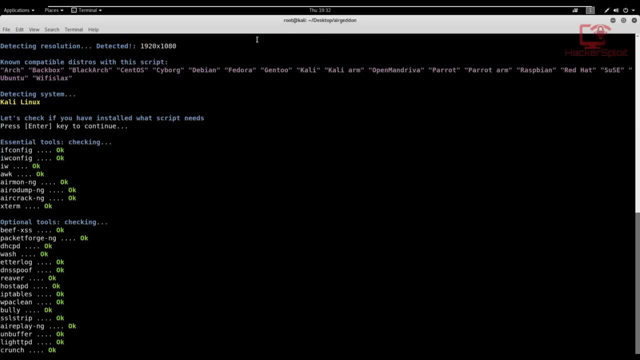 All right, and I'm going to hit enter And let it start airgeddon again, And know the video is getting quite long, but I just wanted to cover everything here When it enter. All right, let me just scan for the tools. I'm going to continue. I'm going to check for a new version. I know this. 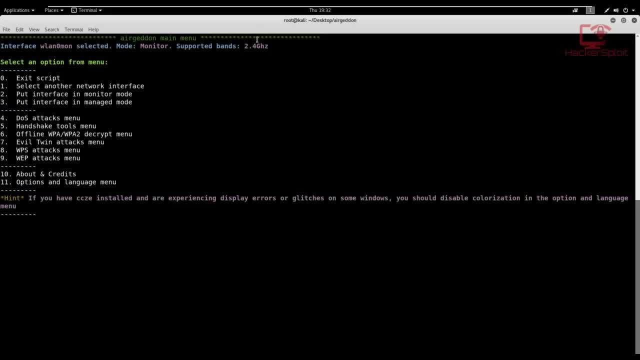 is the latest version. I'm going to hit continue again And I'm going to select my interface, which is already in monitor mode, And I'll go straight for the WPS attacks menu. Remember, you can also go for WP if you're using that type of encryption, If you're lucky to find a network. 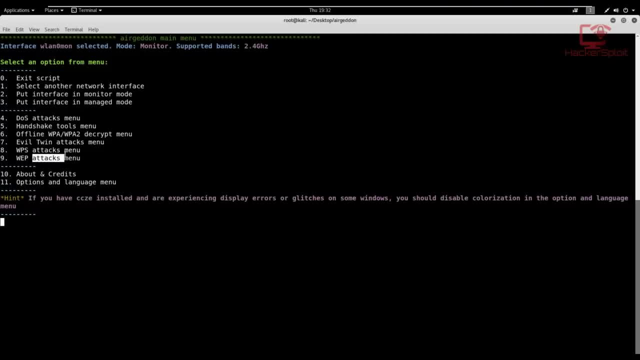 that has WP, crack it immediately. That's a once in a lifetime experience. If you have a network that has WP, crack it immediately. That's a once in a lifetime experience. If you have a network that has WP, crack it immediately. That's a once in a lifetime experience. If you 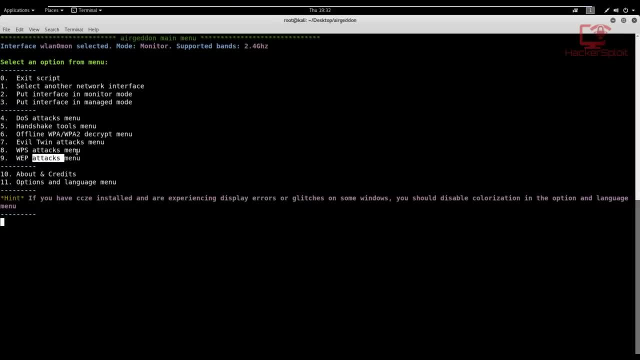 actually even find one. I remember once finding one at a restaurant, but I didn't have my laptop with me, So I had to pass on that. All right, That being said, you can go for your WPS attacks menu, which is eight, And we're going to be using bully. The reason I'm using bully is because river is not. 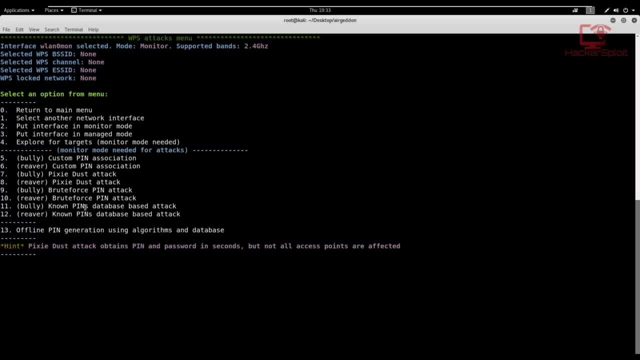 that is not that powerful And even if you're performing the same type of attack, which is a pixie dust attack, you can also use bully for to perform what I would call a brute force pin attack. that, if you have a good word list that has. 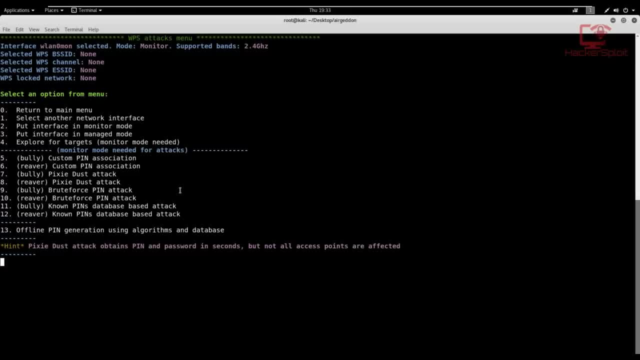 some of the most common, some of the most common pins, the WS pins, then that that can also work as well, But in my mind, this works the best, Alright, so we're going to go for option seven, which is bully. we're going to be performing a pixie dust attack Now. before that, we have to actually 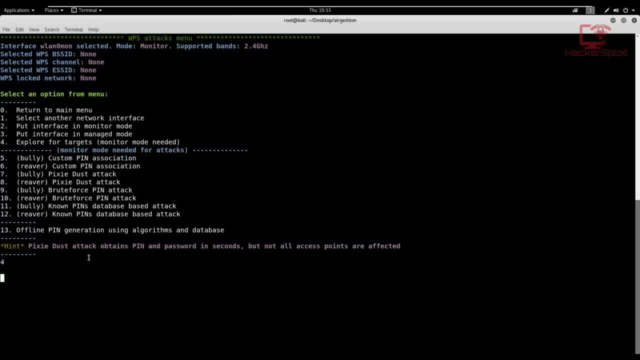 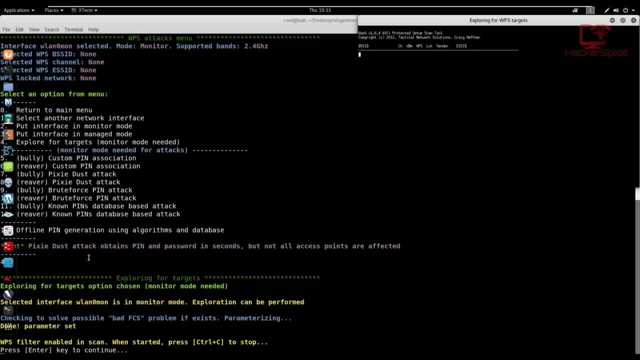 select our, our network. Again, remember, we have to always select our network. So I'm going to hit option four and it's going to start capturing And immediately once I capture it, we should be good. So there we are: it started capturing And once it captures. 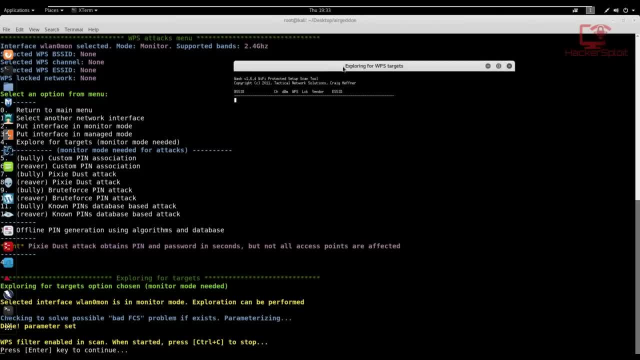 my Wi Fi network. for some reason it's not capturing any network here: WPS networks. Let me just see if my Wi Fi, if my access point is currently open here, is currently online. Let me get back to you once I've checked whether it's online. Alright, so just give me a few seconds. 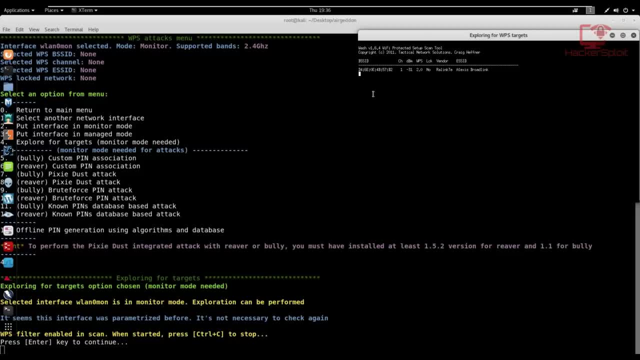 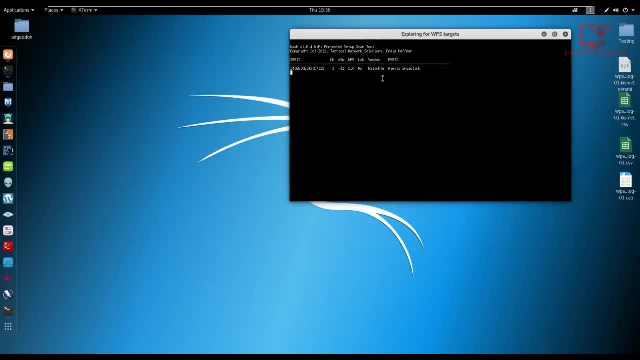 here. Alright, sorry about that, guys. for some reason it was just taking a while to load up And I was just waiting for it here. Anyway, sorry, let me. let me just open up the emulator here. you can see that it has captured that network. 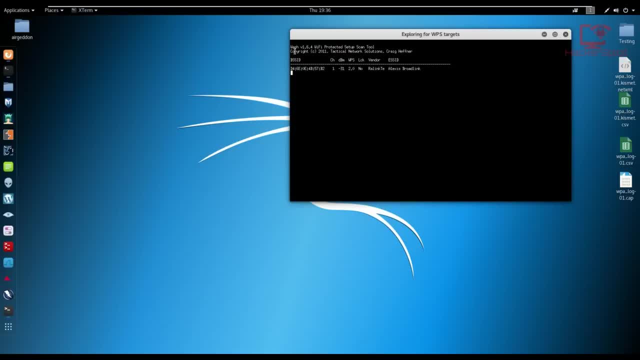 Let me just explain the results here. I'll probably have to zoom this in because the text is really really small. Okay, so it's using wash to to scan for networks, And this is the network that we're going to be performing the exploit on, or we're going to be cracking the WS, the WPS pin. you can. 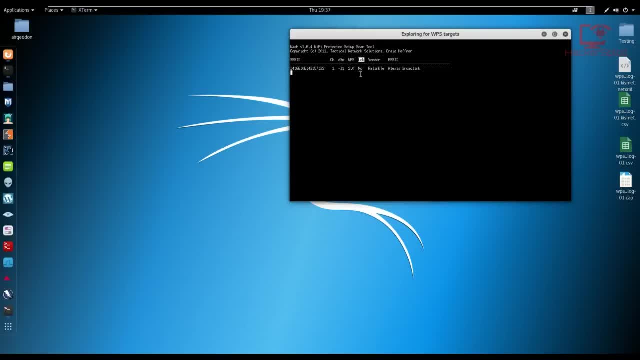 see that it is using WPS version two, And if a WPS is locked, it's going to also show you here, And if it's locked, then you can't use this attack. Alright, so make sure that it's not locked And 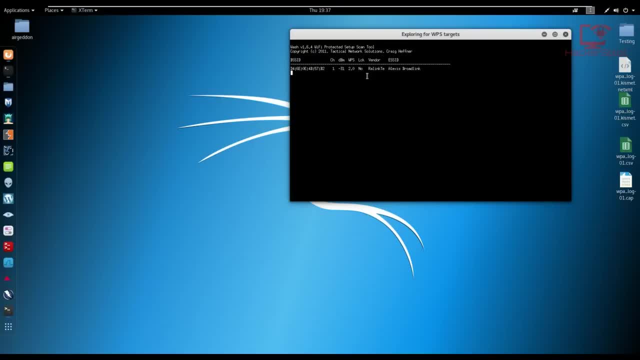 you'll be surprised, I can actually guarantee you. I want you to try this out. Let's see When you're at home. I just want you to scan the networks around you. Let's say there are 10 networks, probably your neighbors. I can guarantee you five of them can be exploited with with the. 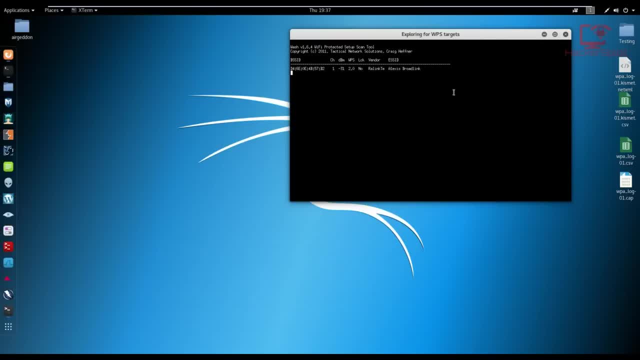 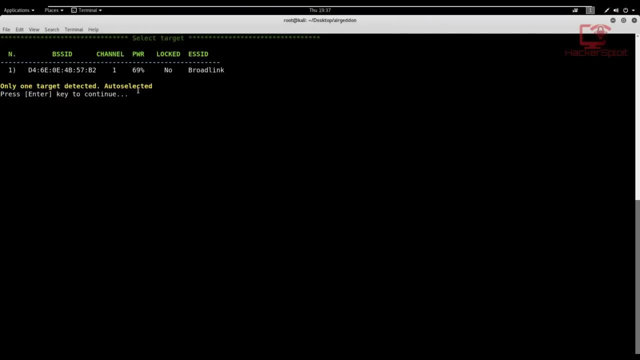 pixie dust attack. Okay, That being said, let me just open up, Let me just hit Ctrl C, because once we're done capturing, we just hit Ctrl C and we go back into airgeddon And, as you can see, only one. 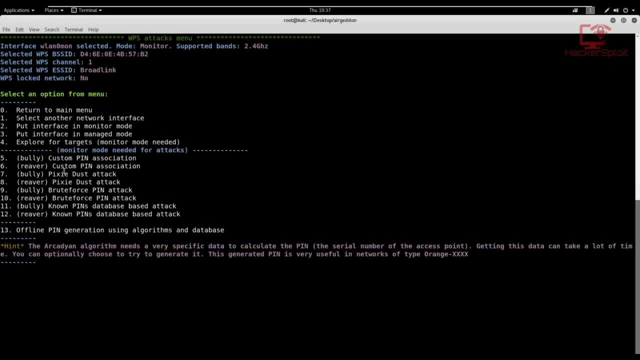 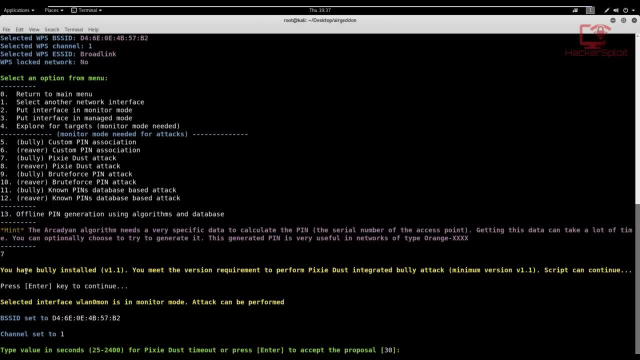 target was detected. it is going to be auto selected. I'm going to continue. And now we can see that the network is working. So I'm going to hit a seven form the bully pixie dust to that you're going to hit enter. you have bully version 1.1 installed. press enter to continue. The BSS ID. 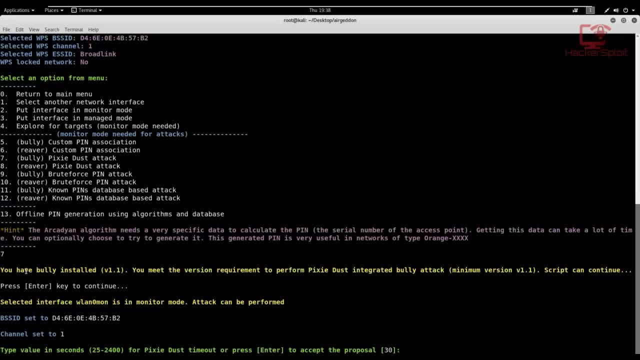 set. the channel is set. Now you need to select the the value in seconds For the pixie dust timeout. if the connection cannot be made by default, it will tell you to use 30 seconds. I also recommend 30 seconds. However, if you're further away from the access point, I would, because of packet loss. 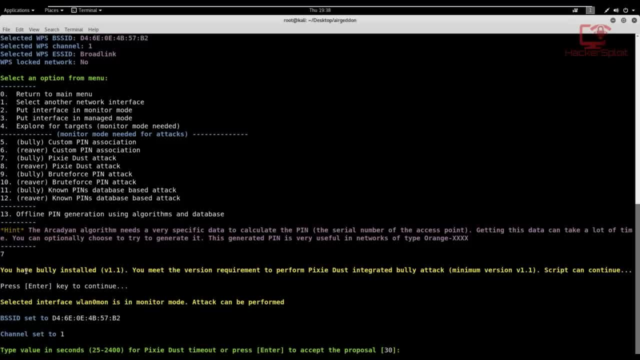 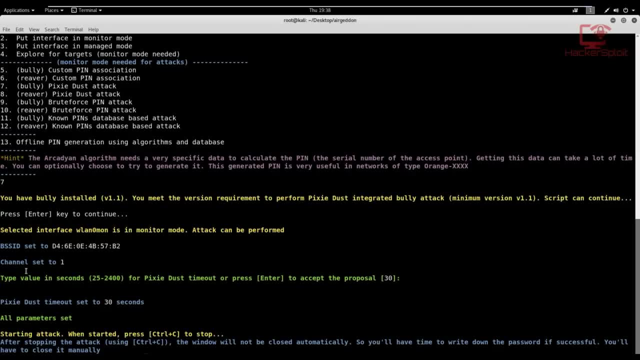 I would recommend changing it to something about 100 or 200.. That's, if you're really really far and you have, you know, really poor signal strength, I'm going to hit enter And all the parameters are set and it's going to say: it's going to say: 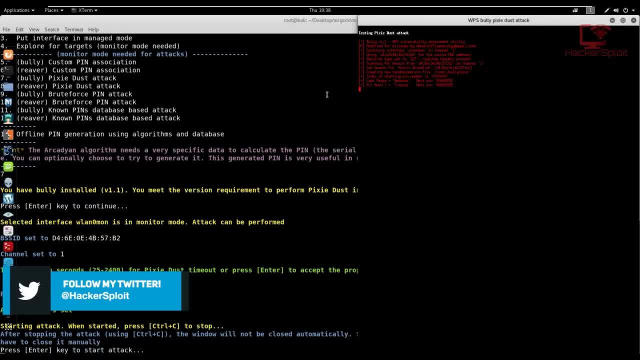 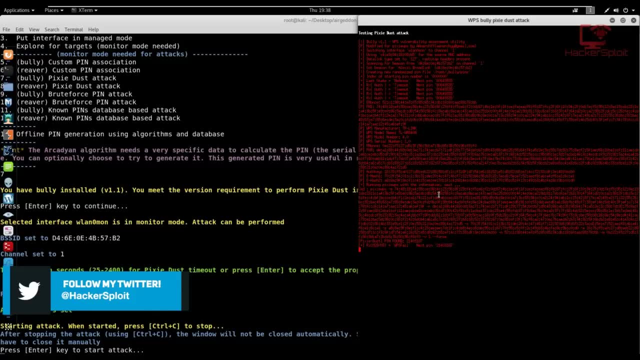 starting attack. when started, press Ctrl plus C to stop. So I'm going to hit enter to start it. And there we are. it's going to start the pixie dust attack. And there we are. For some reason, it is looks like it has got the, it's got, it's captured a handshake here And it's performing. 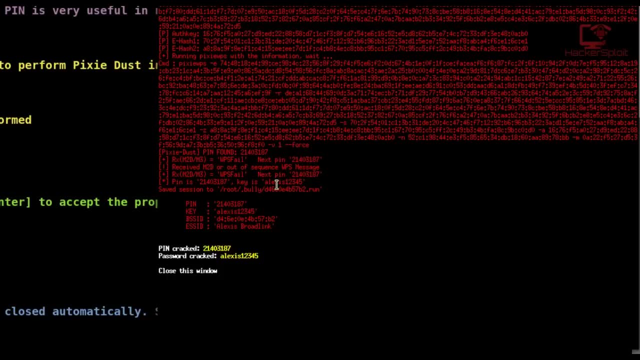 the pixie dust attack with bully. So let it just perform. And there you are: the pin has been cracked And the password has been cracked. How about that? I think this is the first video on YouTube that actually has actually shown that, that it is possible using different vectors. 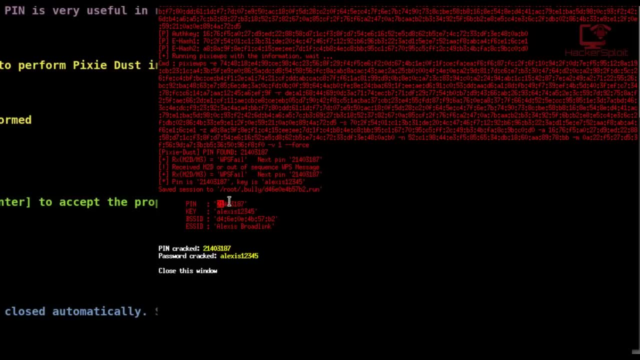 for example, like the WPS with bully. Alright, so you can see it captured, the WS pin. it captured the key, the Wi Fi key which, as you can see, is Alexis 12345.. Now, that's what most people do Now. 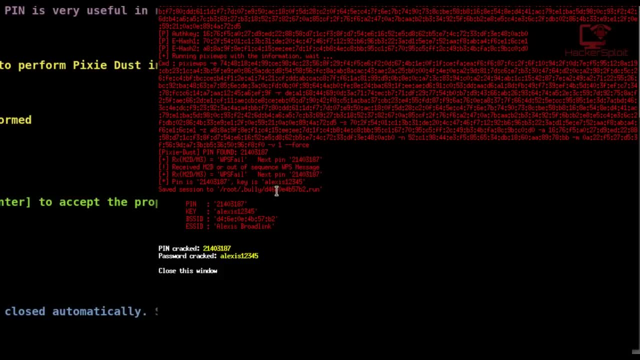 again, most of you are sitting there saying, Well, that's a simple password. Remember, it did not crack the password. it was able to authenticate with the network with the pin and then get the Wi Fi key. it got the BSS ID and BSS ID And there we are: pin cracked password. 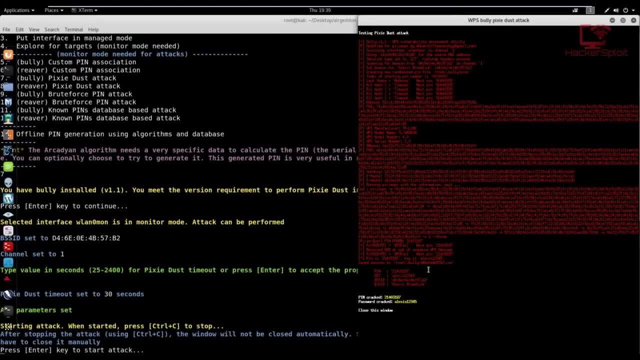 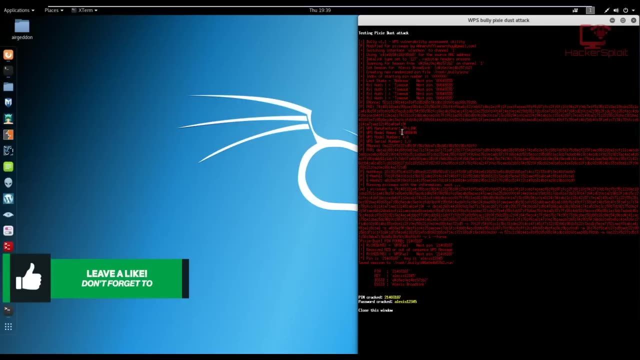 cracked And there you go. you know. that's how to actually perform or exploit WPA using the handshake capture method and how to use WPS- pixie dust attack using bully. you can also perform river, but river will most likely, most likely- give you errors. Alright, so once I'm done, 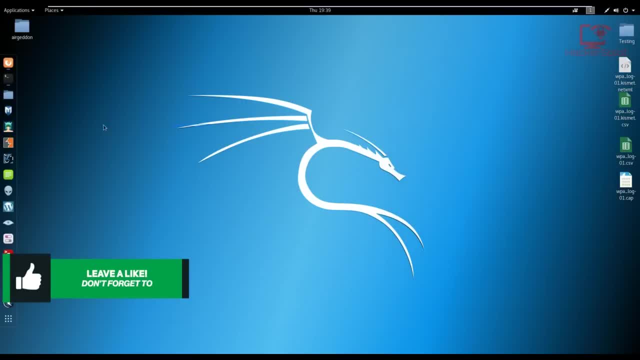 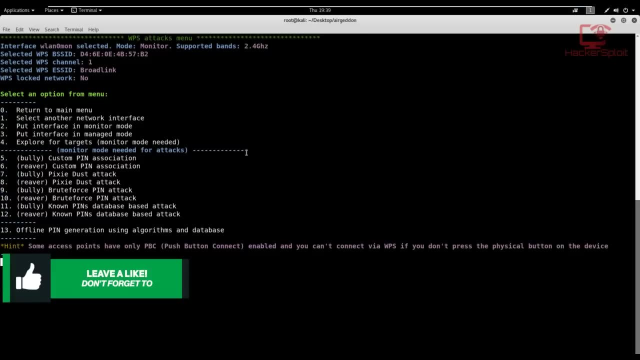 let me just actually close this up. Control plus C, we can close the window and we should be back into into a garden, And once that's done, you're essentially done. So that's going to be it for this video, guys. I know I took this video a bit too long, But I just wanted to show you every. 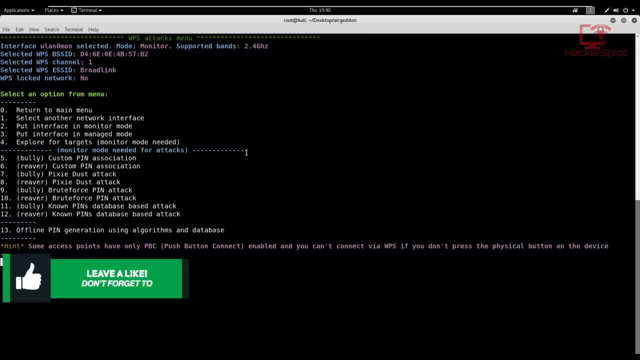 aspect of it And I'll also be moving into using hashcat and GPU cracking, which is very, very effective, especially when trying to cap, when trying to crack the handshake, which you can save and then crack it If you're not near the Wi Fi network. That being said, I hope you found value in this video, If you. 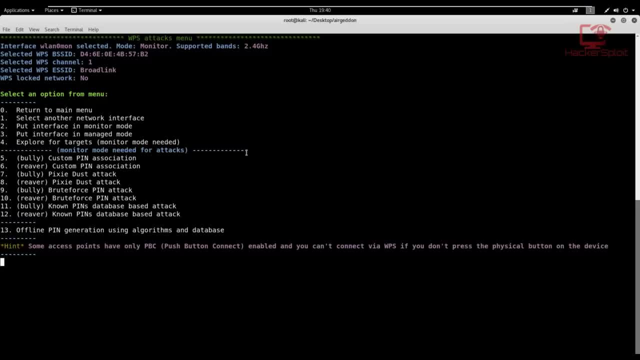 did. please leave a like down below. If you have any questions or suggestions, let me know in the comment section, Or you can hit me up on my social networks. You can also check out my website for the latest hacking news, resources, tools, all that good stuff, hsplaycom, and I'll be seeing you in. 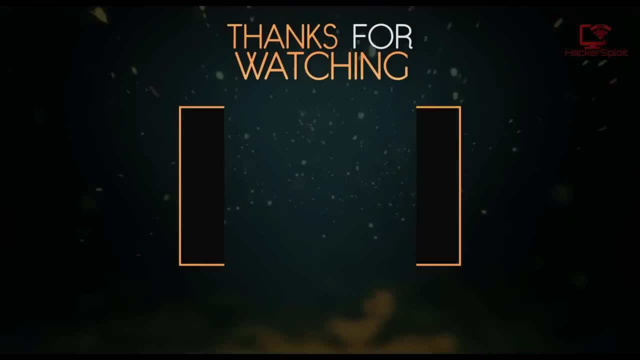 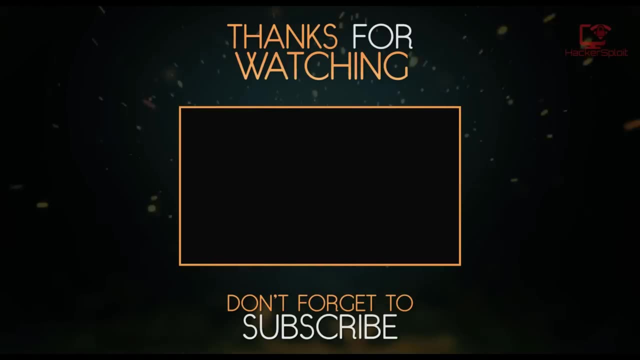 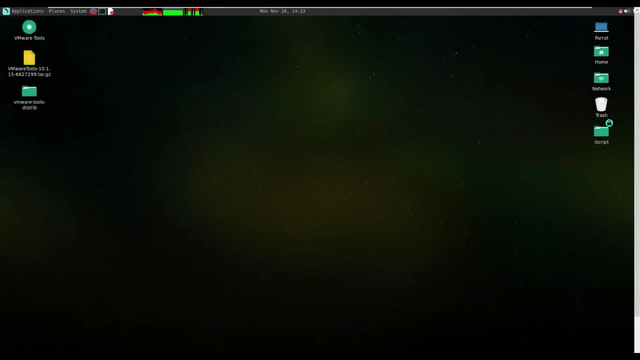 the next video. Peace out is very, very powerful if used in the right way. Now again, this is going to you know. it brings me to the question of of whether you're going to use this for ethical or malicious purposes, And 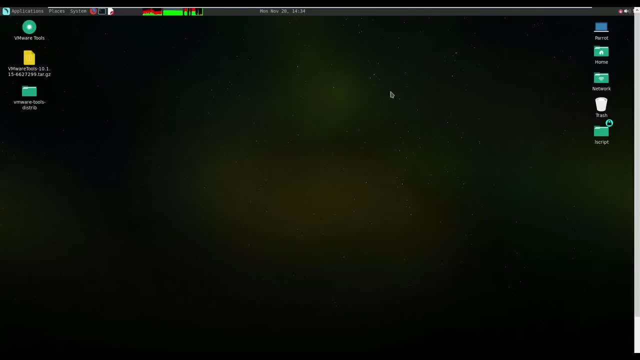 again, I'm not going to be held responsible for any- you know- malpractice that you do with this tool. my job is to show you how to install it, how to get it working and how to use it. how you use it is up to you. And again, I'm going to say this: that I'm not going to be held responsible. Just do. 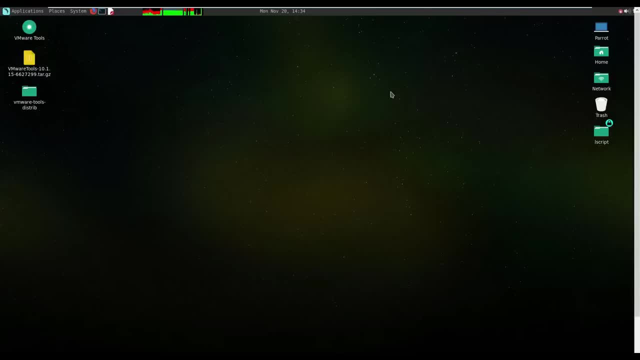 it in a, you know, in your own environment. just use it for testing. Again, you can perform these attacks if you have permission from the owner of the website, you have written permission or you're performing a penetration test, things like that. So you know, having me having given you 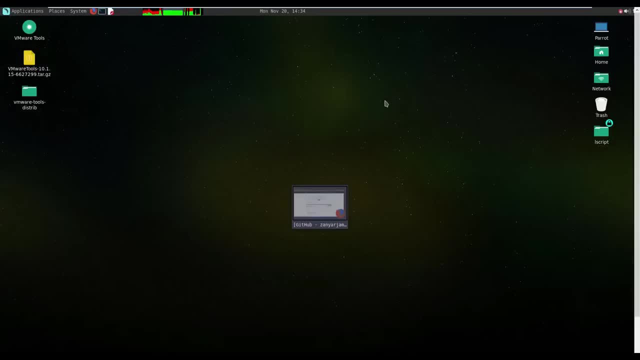 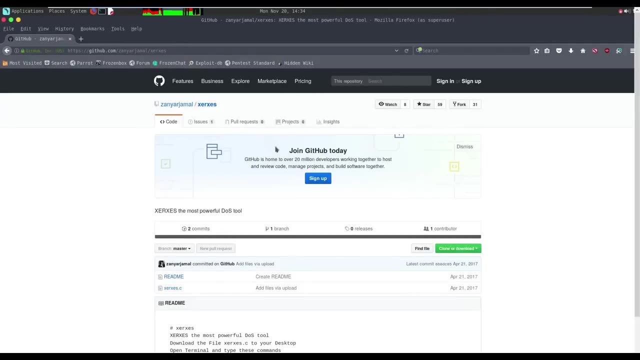 that disclaimer. let's get started. So I have the GitHub repository open up already. the link will be in the description section, don't worry about that. So what you want to do is just go and you can just clone the repository. So I'm just going to copy. 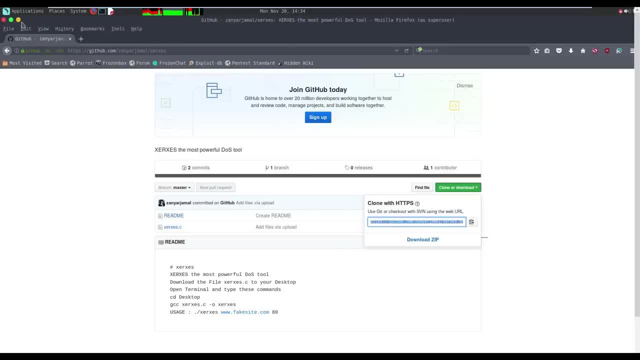 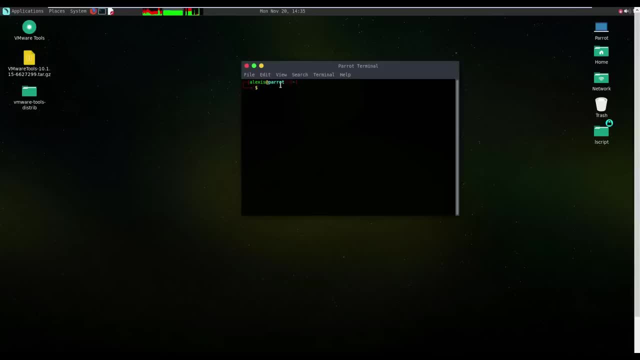 that, or you can download the zipped folder. the process is essentially the same, just that with GitHub, it allows you to clone it wherever you want and extract it for you. So I'm going to zoom in right here, And so we can actually get a good picture. What I'm going to do is I'm just going to 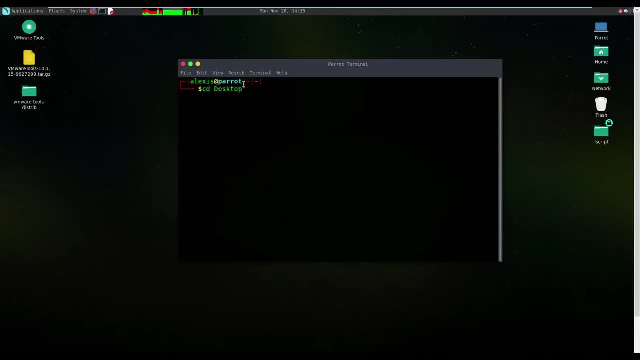 go to my desktop, because that is where the recommended location is for this script. So CD desktop. right, I'm just gonna move from my desktop And in my desktop I just want to clone the repository. So git clone. I'm going to paste the link in there And I'm just going to hit enter So it's going to start cloning. 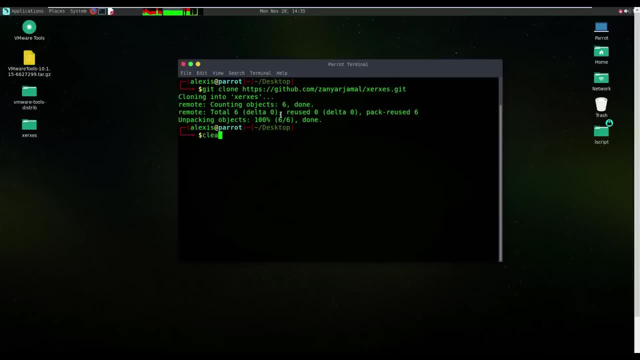 it. And there we are, it's done. shouldn't take too much time. The file is relatively small in size, So I'm going to change my directory into the Xerxes folder, And this is where a lot of people get issues. Why do they get issues is because they try and execute the xerxesc file And that is. 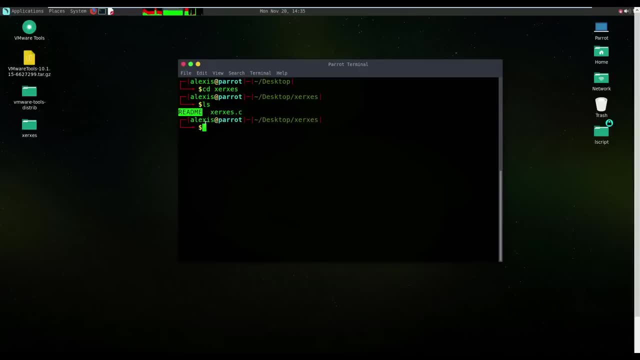 completely wrong Because, as I said, there's a readme file. Please take time to read the directory documentation. it really, really does make a difference, So let's try and read it together. Alright, so I'm just going to print it out. Oops, read me, not the Xerxes file. I almost made that. 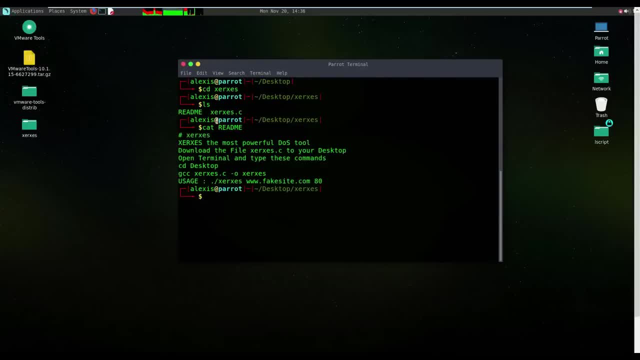 same mistake, So read me Alright. so it says Xerxes is the most powerful DOS tool. Download the file xerxesc to your desktop. Obviously it's programmed in the programming language of C. open the terminal and type these commands: CD desktop. Again, we're using the GNU. 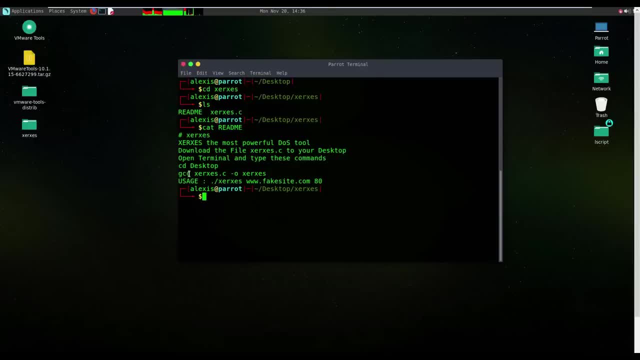 compiler. So essentially, this command right here is going to compile the C file into an executable. Alright, so then we can. as you can see, it tells you here the usage is Xerxes, with the website or the target IP and the port right Report at obviously is referring to the port. 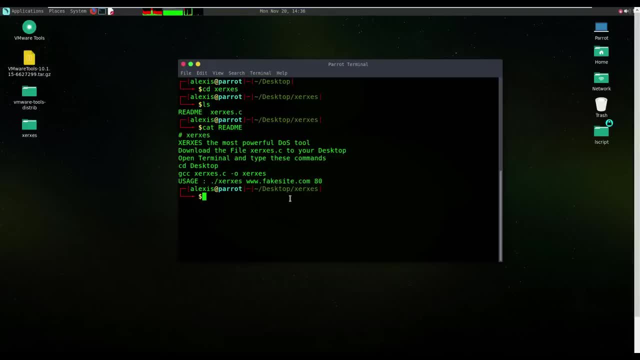 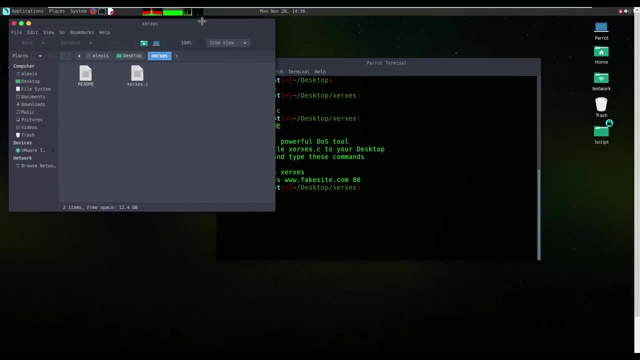 the TCP port where all communication is going through. So again, that is pretty self explanatory. So again, if we open up the Xerxes folder and we check out the Xerxesc with something like the pluma editor or you can use 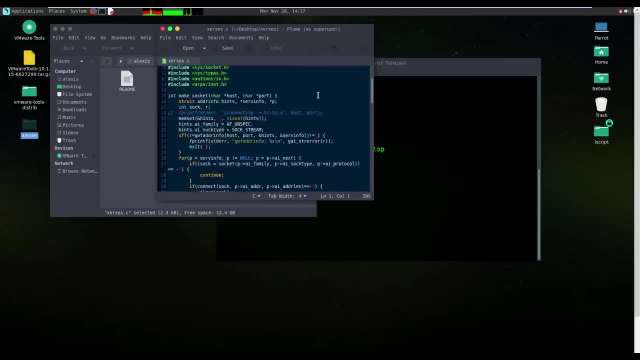 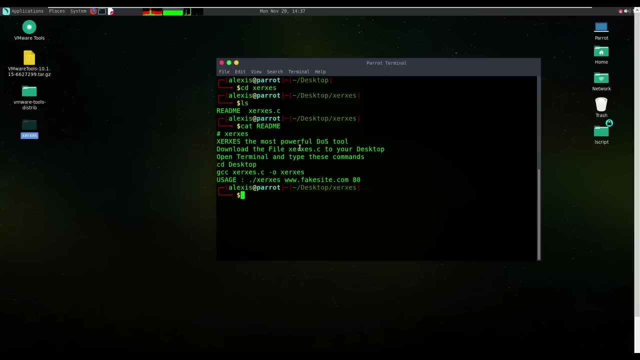 genie. As you can see, it's using the C programming language and we have to compile it, So let's do that right now. Alright. so it's telling us to use the command GCC- Alright, so let's do that right now. So G GNU compiler: whoops. GNU compiler. compiler: Xerxesc. 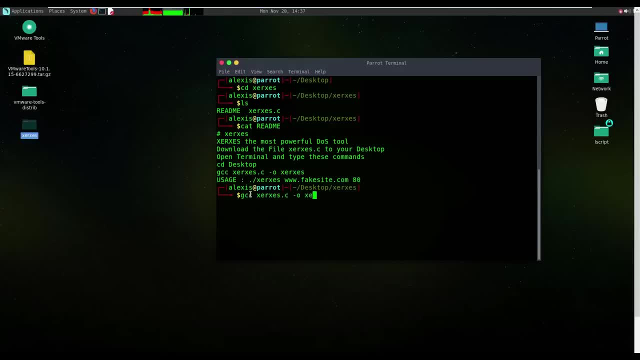 with the output into Xerxes. Alright, so we're just making an executable. So if we hit enter, it's going to create our executable for us. There we are. if I list it, it's just going to be called Xerxes. 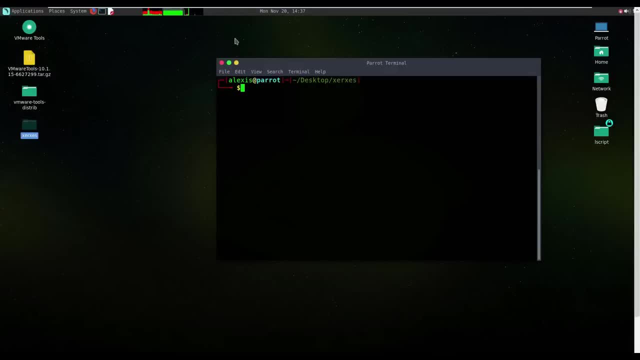 Alright, so let me clear this up Now. you might be asking yourself: what target are we going to try and attack? Well, again, as I've said, I really encourage you when you're trying to learn these things is to run it in a in your own environment, where you control everything, And one of the best 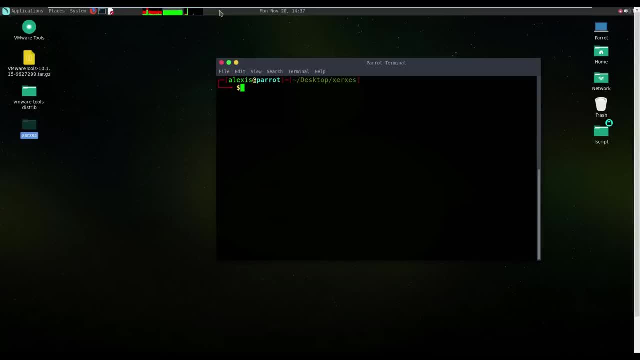 ways is to use. you know, you can try it on your, on your computer. So let's say, let's say let's say on virtual machines, on your Windows device or on an IP that you want to test. Now, in my case, 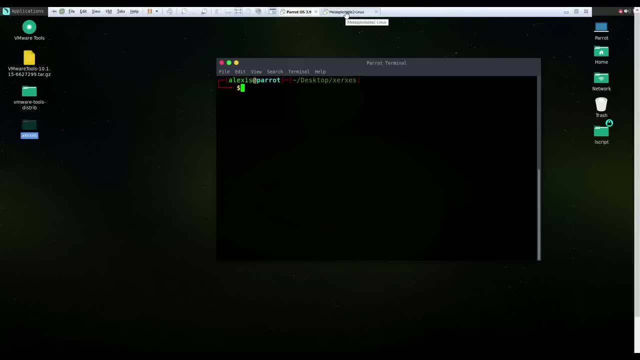 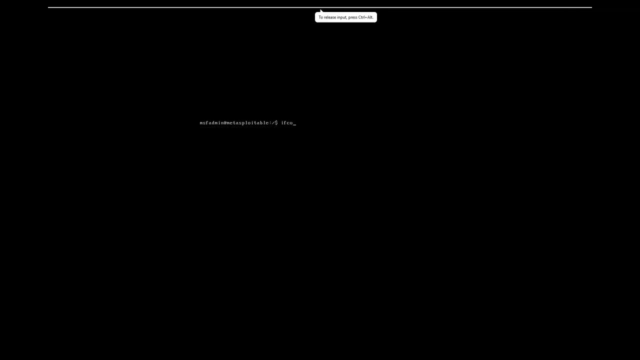 I'm going to be using a virtual machine for Metasploitable 2. Right, So what I'm going to do? I have it running in a virtual machine And, whoops, let me just get my IFConfig back up, As you can. 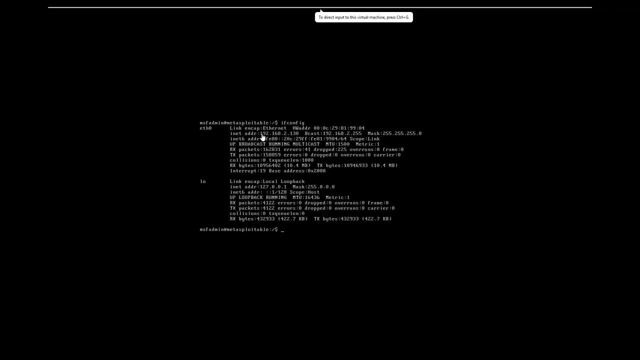 see, I have the IP address here for the Metasploitable 2 virtual machine. We have the 192.168.2.130.. All right, the IP address for the Metasploitable machine. now we do know that Metasploitable has a web server. 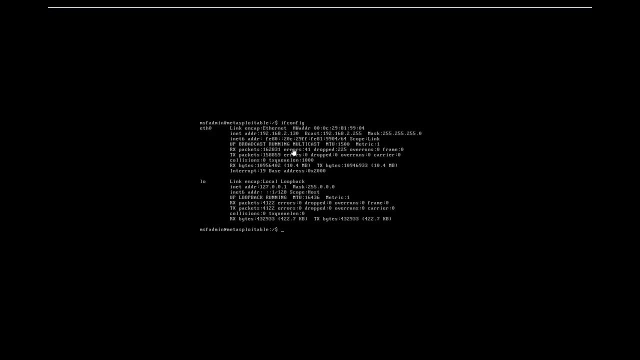 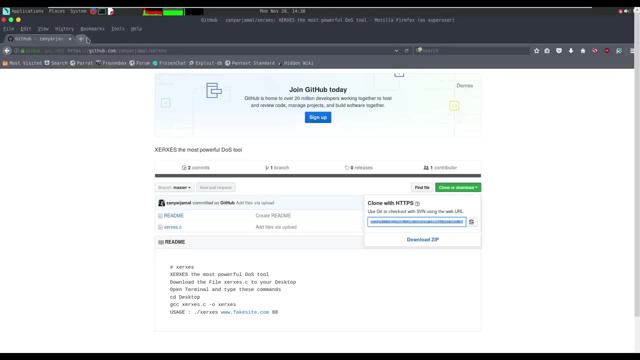 it's running some files on it, so let's try and access that. right now. let me just bring a para to us back again here, and if I move to my web browser, let's try and access it. all right, so one eight, two point one. sixty eight point two point one, three zero. that where it is. so if I 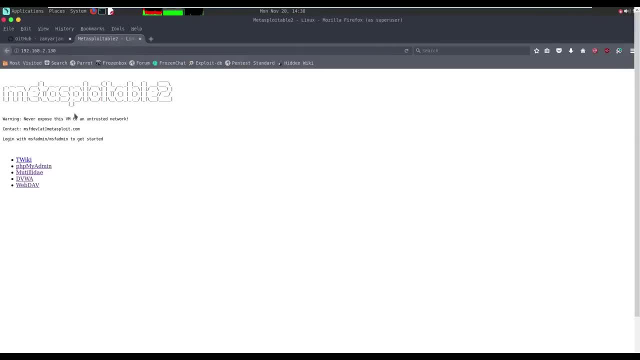 open it. as you can see, we have the web server running a few vulnerable frameworks, like we have the PHP my admin, which is not really vulnerable. it's there for testing. we have the motility, damn vulnerable web application, which we will be looking at, by the way, most of you guys have. 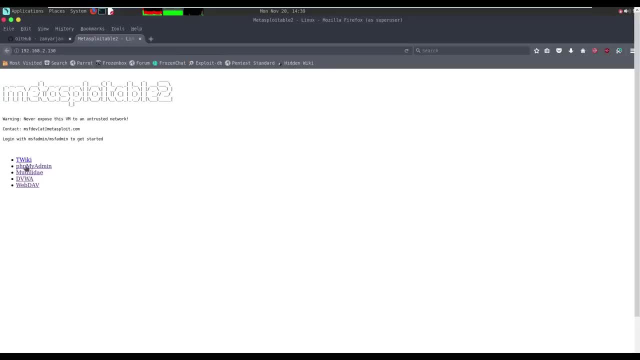 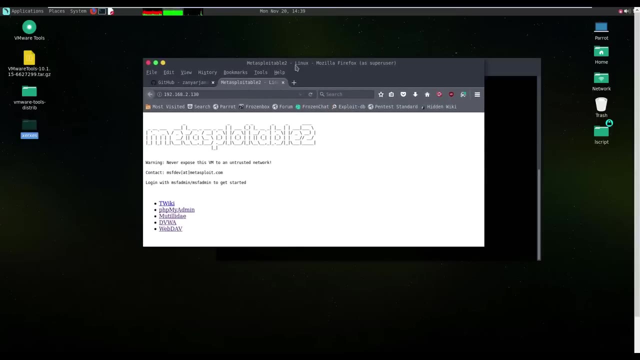 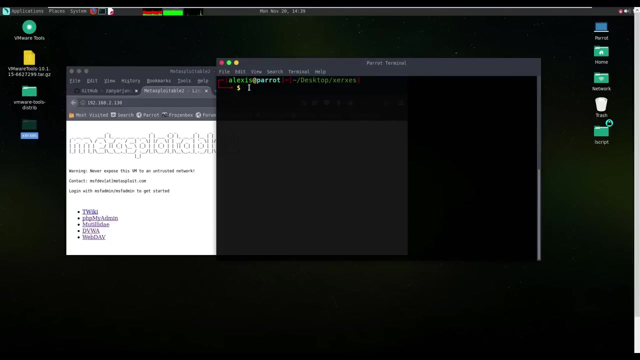 been requesting- literally begging for mysql- mysql tutorial, so we'll actually. or SQL injection attacks tutorial, so we'll be looking into that in other videos. but the bottom line is we do have the webs of running, so let's try and actually attack this and see what happens. all right, so let's execute it. so Xerxes, Xerxes and then it. 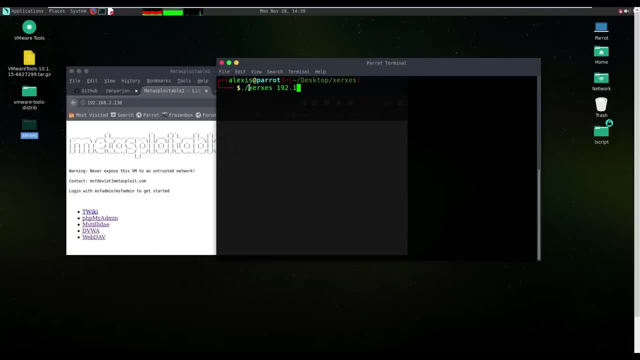 said that we specify the IP or the target. so one ninety two point one, sixty eight point two point one, three, zero, with the port ATP use for TCP connections, and once I hit enter, it's gonna start sending the volleys, which are simply attack vectors. let's see if we can get access to the web. 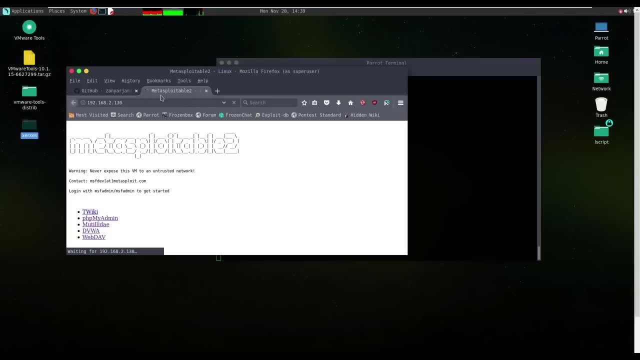 server. and what do we have here? well, it looks like we can get access and, as you can see, as simple as that you are able to perform, in this case, a denial-of-service attack. it could be to any target on your local network, or if you're trying to attack a target, you know. 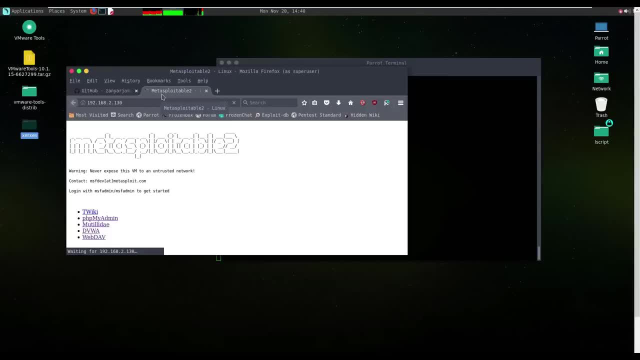 anywhere around the world with, whether it be a website or an IP address. you can see that it does work with great you know, with great efficiency, and it's just amazing to see that such an simple tool, you know, very, very easy to install and and to configure, can be performed in the web server. 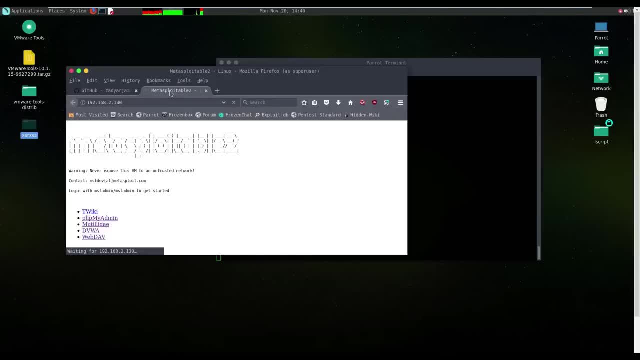 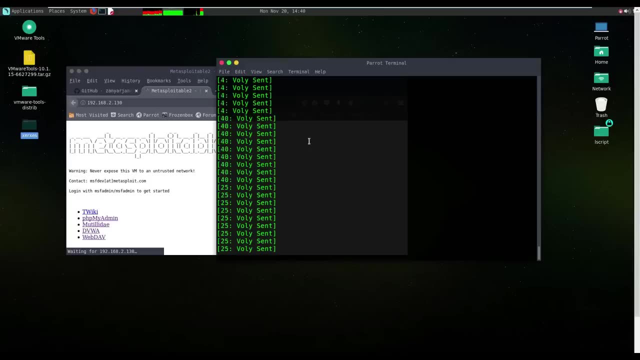 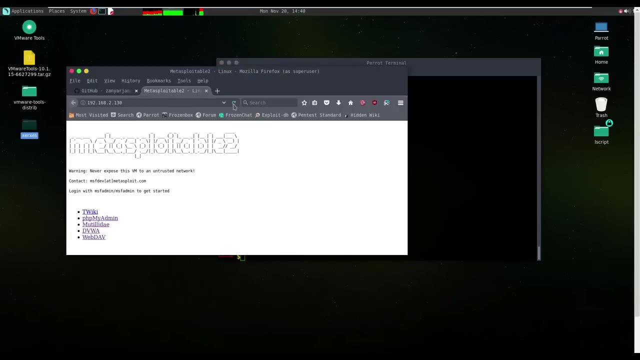 perform this attack. you know this effectively. So, as you can see, it's just going to keep on sending requests in terms of volleys And yeah, until you stop it, which is when you can get access to your web server. So let's try and stop it And I'm going to try and reload it and 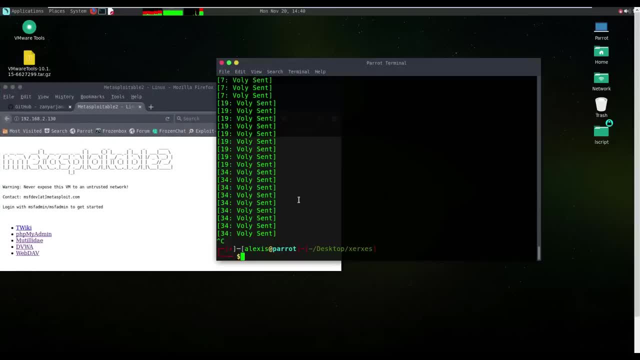 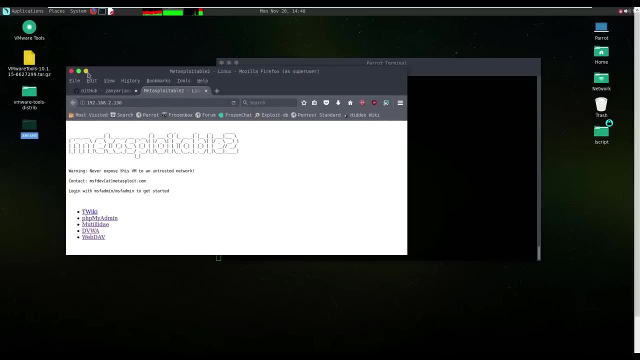 immediately you get access. Now I know if I run this again it's probably not going to work, because the requests have already been said. let's try and see if it. Yeah, it's not going to work Now. that's usually an issue. So what you have to do is run the script again. But again you can try. 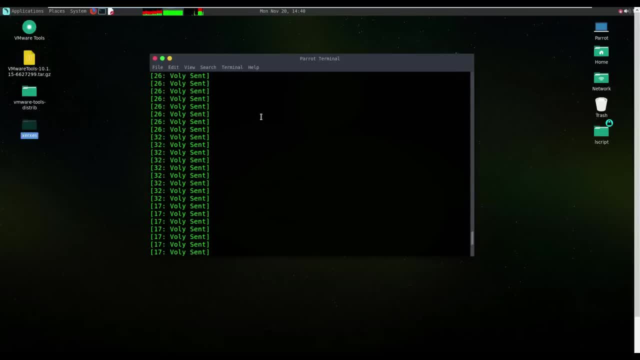 and target even a website. Again, I would recommend that you don't do it to a website into you that you don't have permission to. And that's pretty much it. That's how to use Xerxes. You can use any target that you want. Again, I'm not going to be held responsible if you try and attack a. 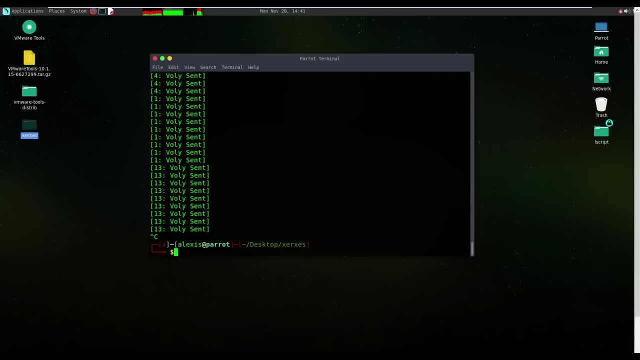 website. you know that you're not allowed to And you know the funny thing is many, many websites nowadays still don't have DDoS or then denial of service protection, which is just amazing to see because you know with with a tool like this and a botnet, you can really do some serious damage. I mean most of the big 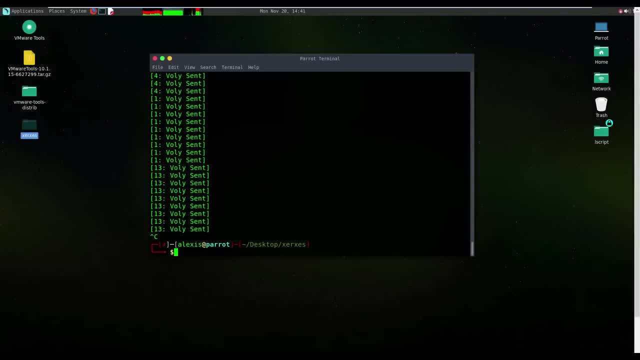 websites nowadays can handle a lot of traffic and performing one, you know an attack from one computer or one one client is not going to be enough. But for many of the smaller websites, you know individual blogs or or you know you know hospital websites or stuff like that. 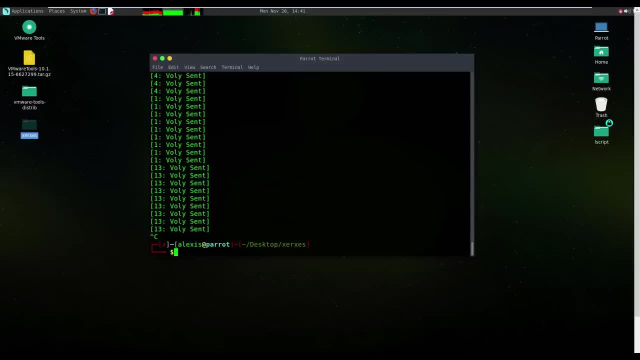 that are really not very important. you can actually bring it down, which is incredible. But again, this is all about learning. we're learning a lot of these new things and how they work, And, yeah, that's going to be it for this video. guys, If you have any questions, please leave them in. 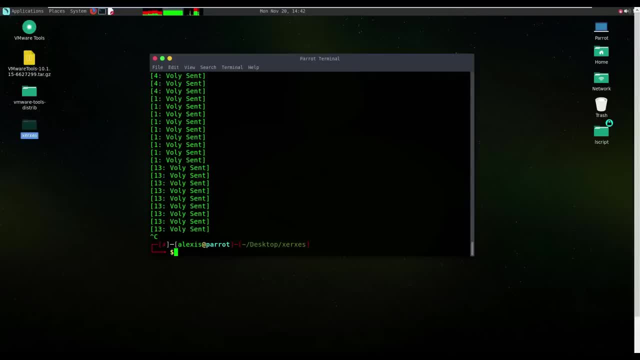 the comment section down below, Or if you have any personal questions, hit me up on my social networks or hit me up on kick. If you found value in this video, please leave a like down below. You know, if you want the latest hacking news and resources, check out my website. By the way, 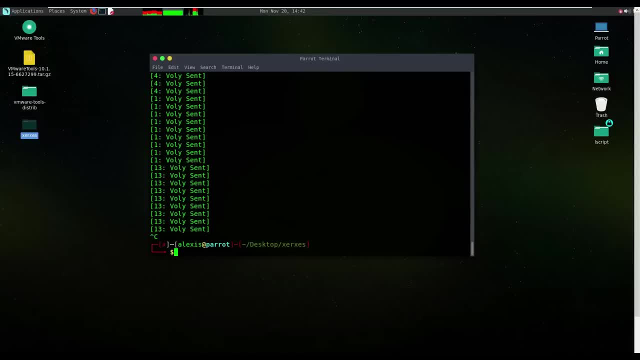 guys, I'm going to be having a q&a section or a q&a video every weekend, probably on Fridays and Saturdays, where you guys should be posting your questions. on my website, hackersploit or hhsploitcom, There is an ask question section where you can post your question and I'll be 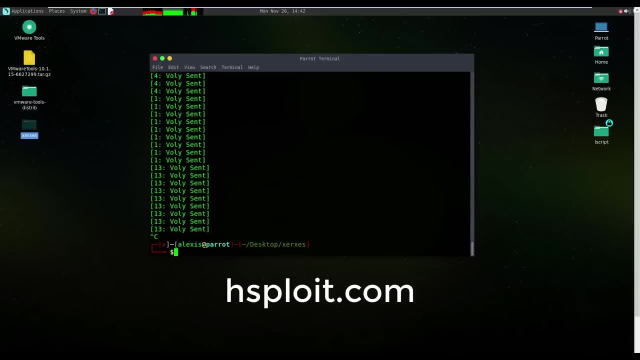 answering all your questions in the q&a video. So make sure you post your question there every week And the best questions will be chosen to be answered. Awesome, So thank you guys so much for watching. I hope you guys found value in this video and I'll be seeing. 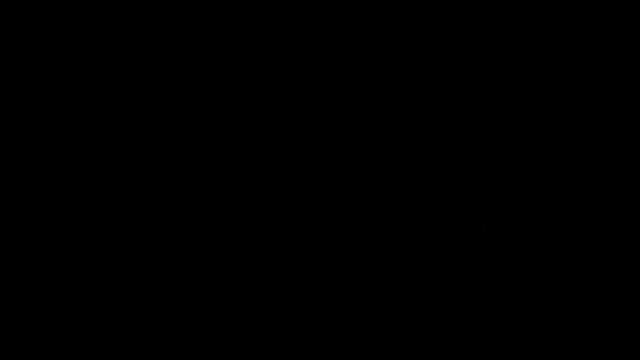 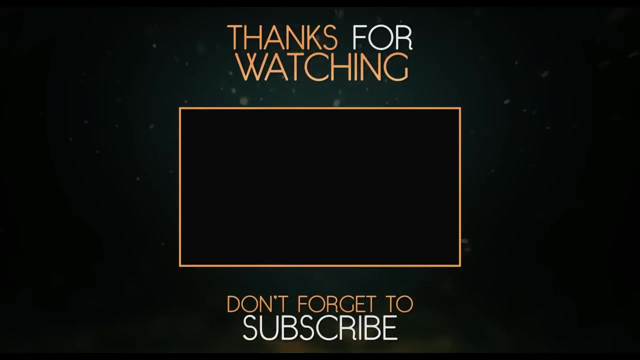 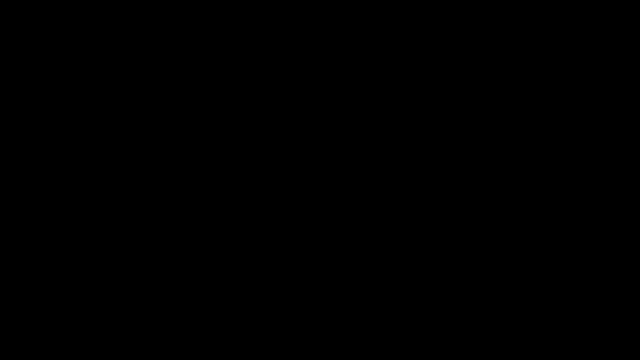 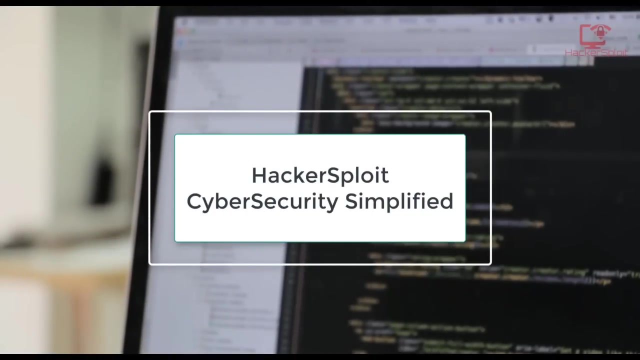 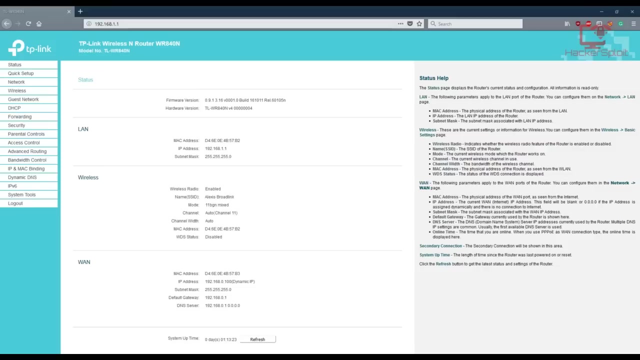 you in the next video, Peace. Hey guys, hackersploit here back again with another video, And in this video I'm going to be showing you some of the security features that your router has in regards to DOS protection or DDoS protection. Alright, so, as you remember, in my Xerxes videos and in my other DDoS videos, 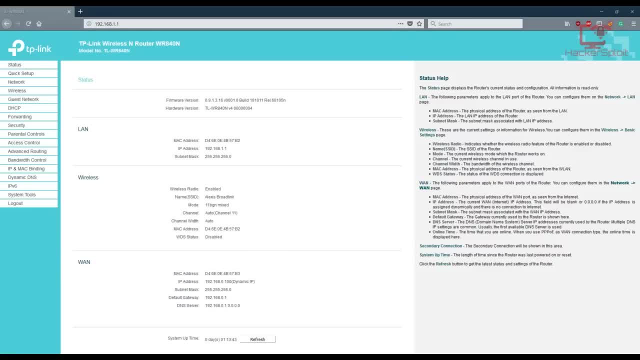 I talked about the fact that you can- you can actually block the ICMP pings, etc. etc. And most of you thought that I was lying or there isn't something like that. So this is a video in response to that And for those of you who are asking me how to do it, this video is also for 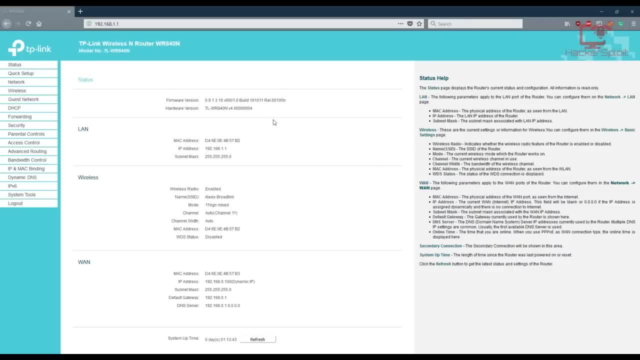 you. So, as you can see, I'm I've actually logged into my router here, the router control panel, And there's- no, there's not going to be anything serious here Because, again, it is a subnet based system. So, in terms of IP addresses, I don't want people coming and telling me that, you know, I saw. 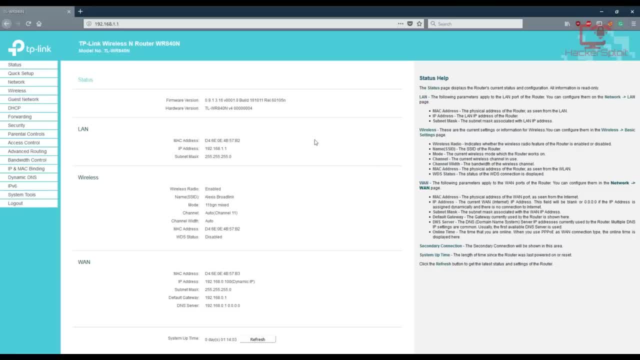 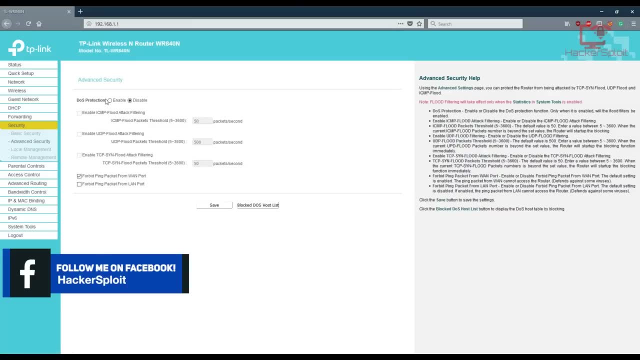 your IP address and I'm going to DDoS you. you know that just doesn't work anymore. So if I just go to the security and I go to advanced security, I have something called DOS protection. Now for those of you who are actually calling me out, and 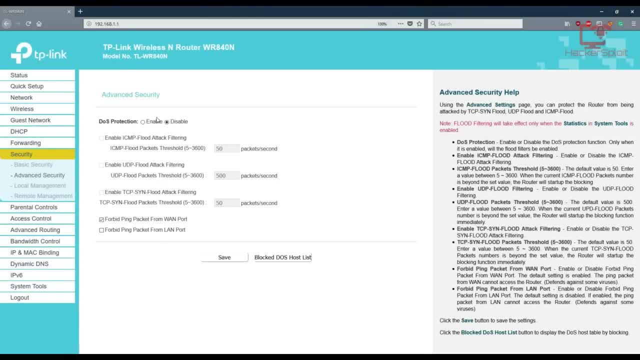 telling me there isn't something like this. what do you have to say about this? Alright, so if you just read on the right here, where you have your help or your documentation, you can see that it allows you to enable or disable the DOS protection function When it's. 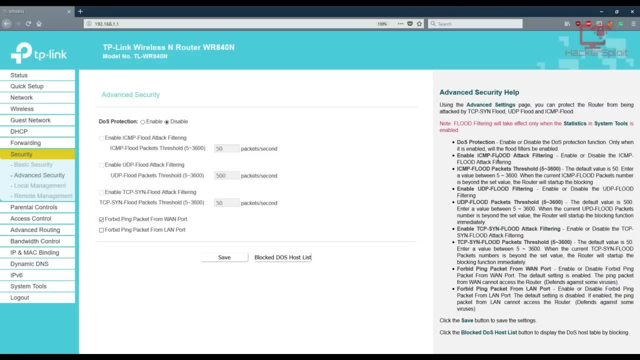 enabled it, the flood filters will be enabled. So again, you have your ICMP flood attack filtering. So what this means is, once you enable this, performing a DDoS or DDoS. DDoS attack will not take down your internet connection, in the sense that it will block the ICMP floods. And when 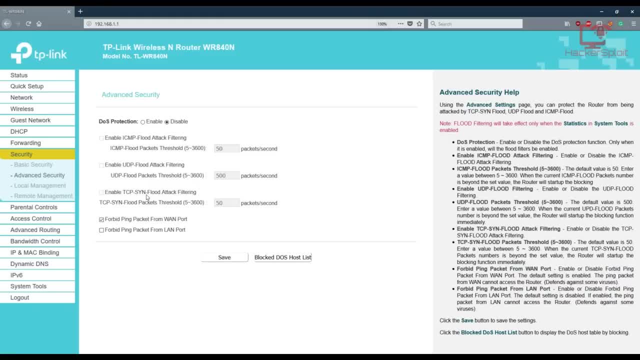 you're talking about, for example, stuff like the TCP synchronized headers for for the packets. you can enable that. So, depending on the type of DOS or DDoS attack you're trying to perform, you know if you have a good access point or a modern route, I would say it should have this. 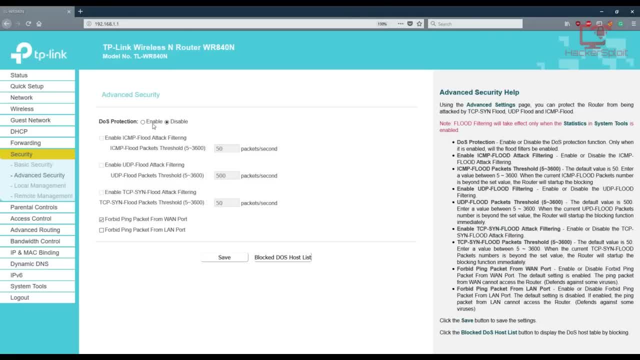 Now I'm not sure, if your router doesn't have this security protocol or security feature, You might- you might be looking at, you know- selecting a new one, if this is what you're really up to or what you intend to do. So by default, you can enable the, the DOS protection, and then 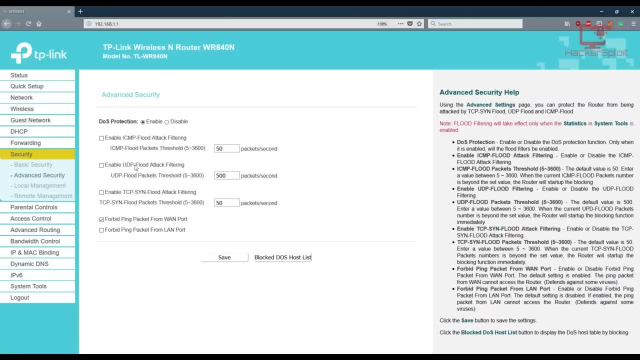 you can find the enable, the type of packets you'll be sending, So you have your user data: gram protocol, UDP, ICMP, TCP, the synchronized flood attacks, which is very, very powerful as well. you can increase the threshold depending on what you have set. so that you know. 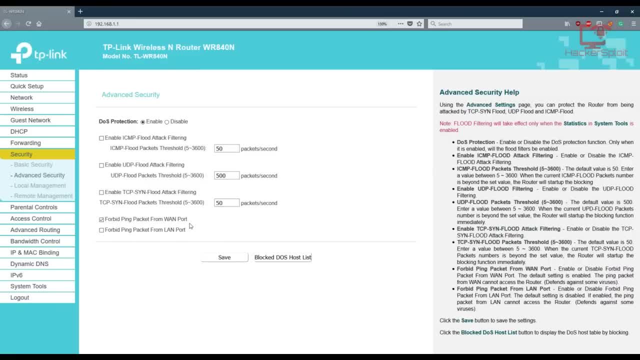 there's no packet loss. And then you can also forbid the link packets from the WAN port and the LAN port. So again, you can forbid it from affecting other computers on your network. All right, but I'm not. I don't perform those attacks or DDoS attacks, for 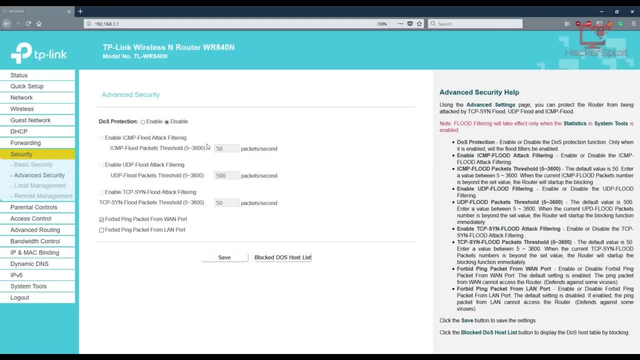 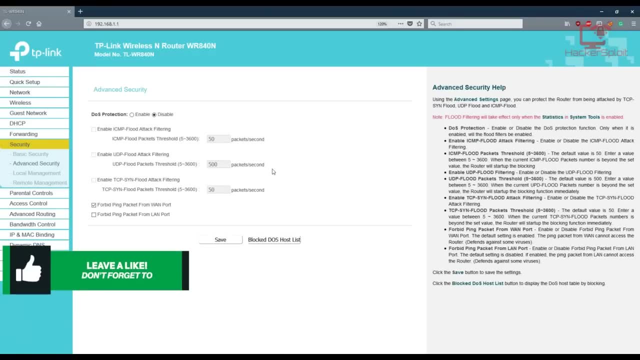 that matter. So, again, I don't need to enable it, But this is the way to do it And for those of you are calling me out, I hope you can see that, Israel, if you're telling me that Xerxes doesn't. 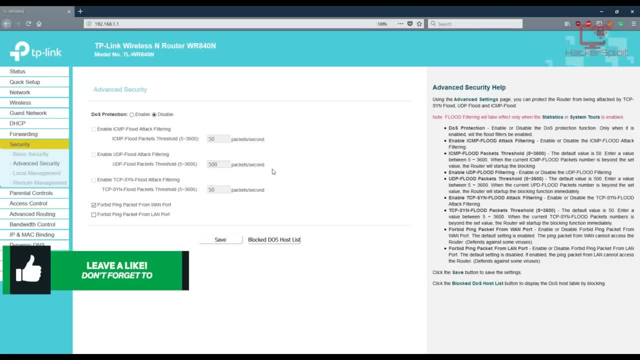 work? it does work. you just need to know what you're doing with your router and you need to understand the flow of packets. So again, this is a short video and I just wanted to clear things up. Don't worry, you know, uploads will be regular now And the the web penetration. 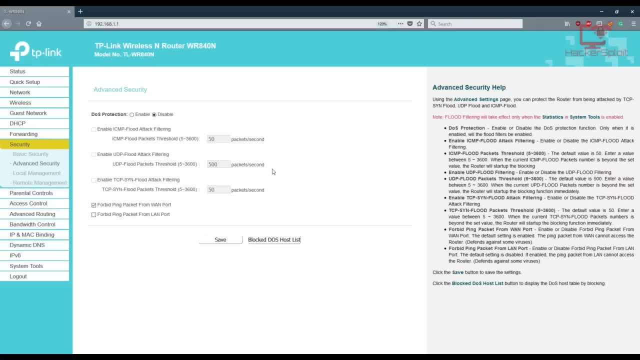 testing video should come straight after this. Anyways, I said that's a small little video just to help you guys who are a bit confused. And, yeah, if you found value in this video, please give a like down below. If you have any comments, suggestions or questions, let me know in the 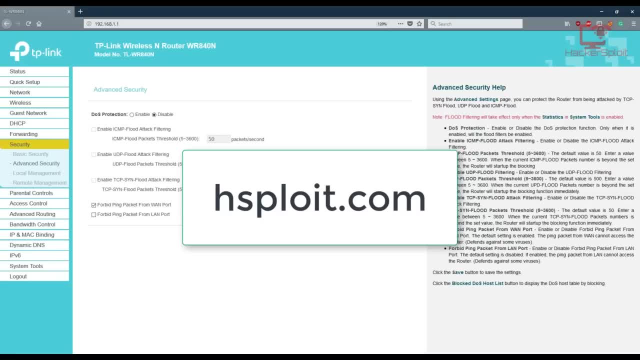 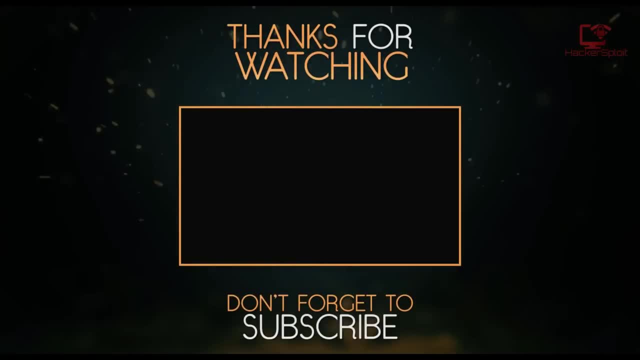 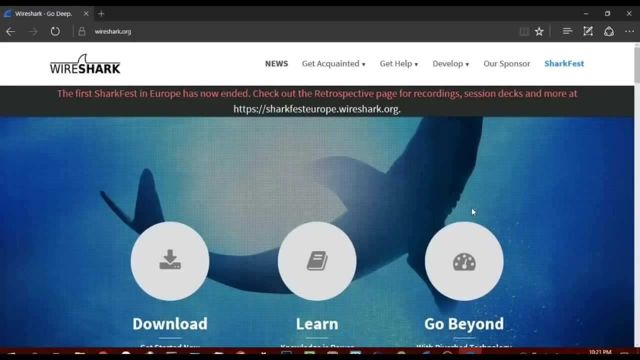 comment section on my social networks, or you can hit me up on my website And I'll be seeing you in the next video. Peace, Hey guys. Hackersploit here back again with another video and welcome to Wireshark for beginners. So in. 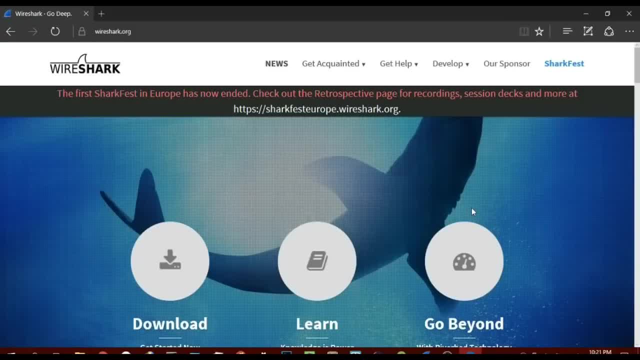 these set of tutorials, I'm going to be teaching you how to use Wireshark And I'm going to be moving you from a beginner level to an advanced level or an intermediate level. So you might be asking: what is Wireshark for beginners? Well, I'm going to be teaching you how to use Wireshark for 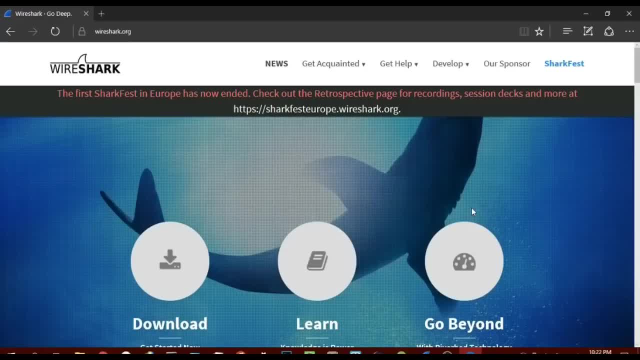 beginners. Well, Wireshark is a traffic analyzer. Now you might be asking: why do I need to learn Wireshark? Well, if you're a network administrator or system administrator and you're interested in basically monitoring what's going on on the network, this would be handy for you. Or if 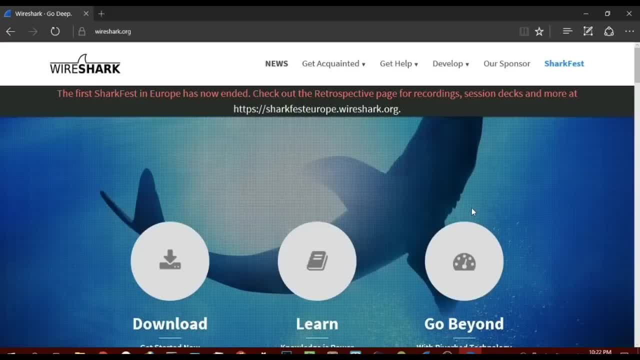 you're just a curious parent at home wants to make sure that your children aren't browsing the web, you know, in more illicit methods. I mean visiting inappropriate websites and stuff like that. So basically it's just a tool for monitoring what's going on on your Wi-Fi network. That's. 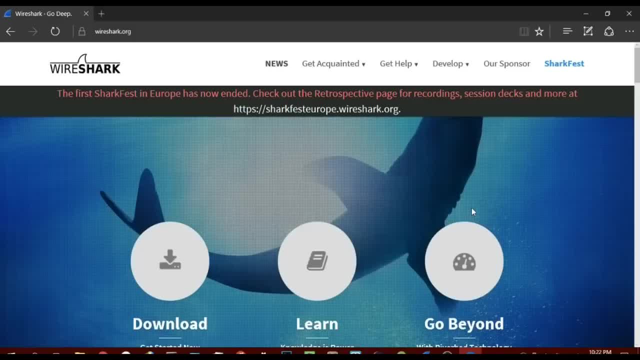 basically it for the layman, So I guess anyone can really learn how to use this tool. It's nothing really hard, So yeah, let's get to it. So I'm over here on their website. It's wiresharkorg. 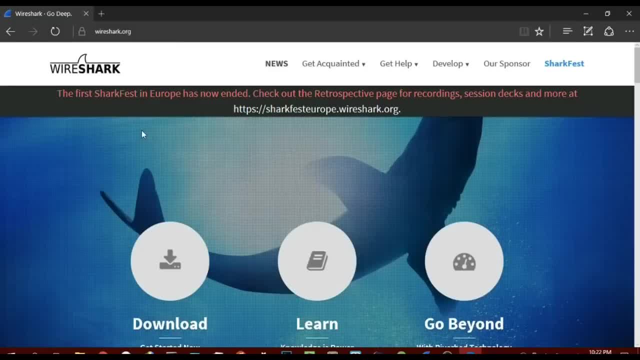 There we are. That's the website. I will link it in the description section If you don't want to type it out. I don't know how long that will take, But yeah, once you load it up, you just want to. 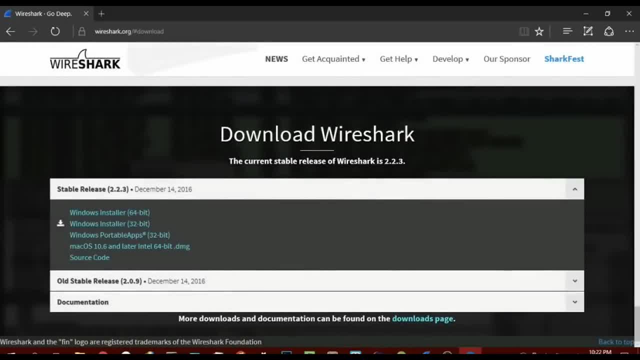 hit download- And it's free, By the way. so the current stable release is wireshark 2.2.3.. So we have the latest stable release. You have your different platforms. you have a Windows, Mac OS. you have source code for. 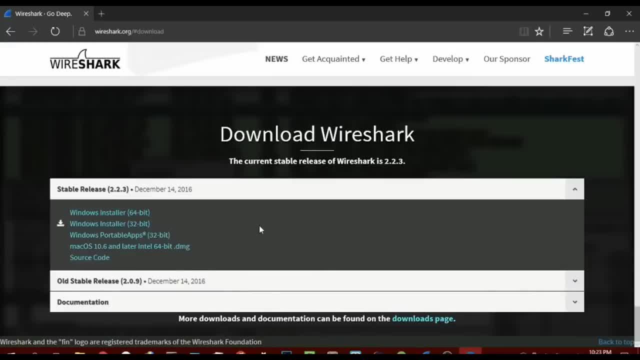 Linux. I do believe that you have to install it through the terminal on Linux. Let me know if you want a tutorial on that. So again, you have your different architectures in terms of platforms. So you have a 64 bit Windows and 32 bit Windows. 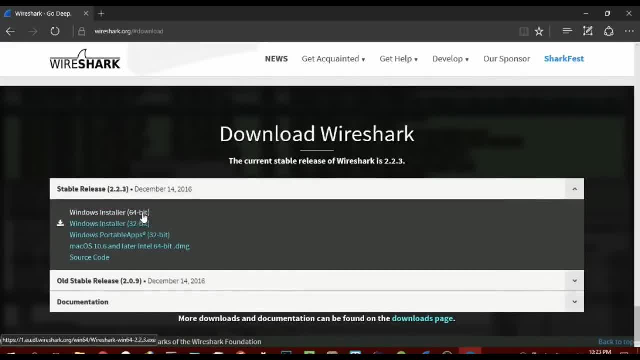 So you can download the 64 bit, because that's the version of Windows I'm running and the processor of basically the processor that I'm running, But I already have it downloaded and installed. Please do note that during the installation, I want to make you have to just 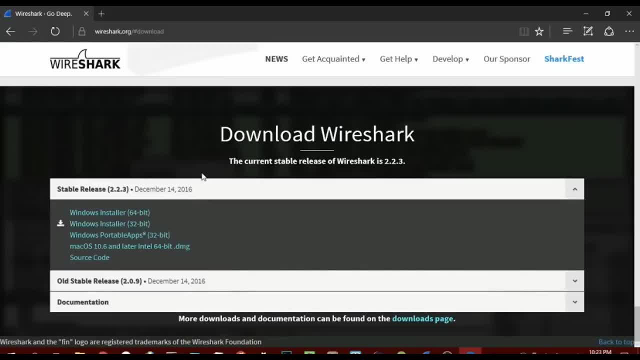 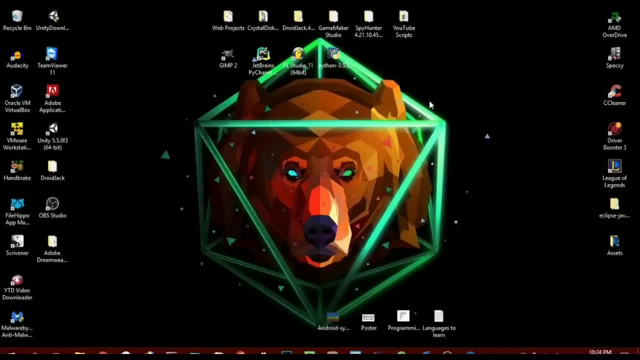 install Windows Win PCAP, That's what it's called. It'll give you that prompt during the installation to install Win PCAP. Now, make sure you do install Win PCAP Because, as again it's the components, that goes hand in hand with wireshark. So once you have it downloaded and 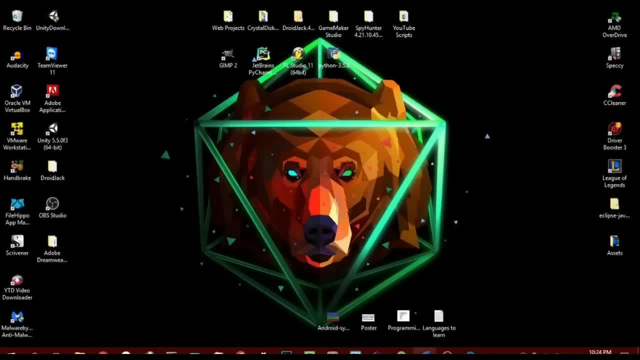 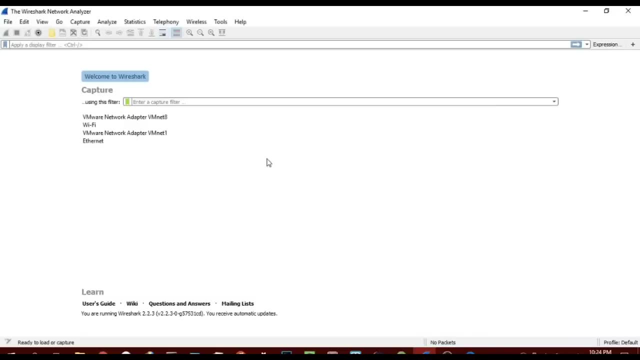 installed. it's very simple process. I have it right here. Very nice icon. It's a shark fin, a blue shark fin. boot it up And you're greeted by what appears to be a loading menu And this very, very, very complicated looking program. But don't worry, it's nothing really complicated. 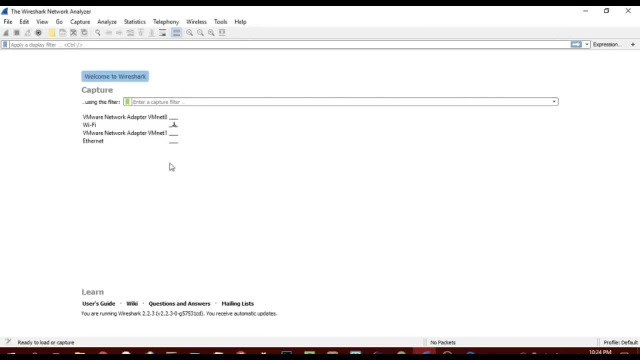 So basically what I'm going to do, I'm just going to give you a basic overview here of what to do. to get started, We're going to look at the advanced stuff in the next video. I'm going to cover that then. So welcome to wireshark. Well, thank you very much. 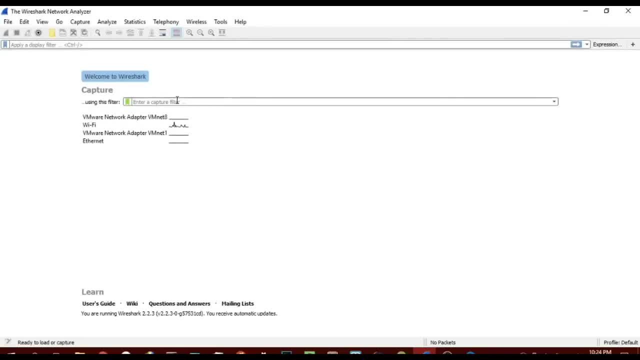 So what it tells me to capture, don't worry about this using enter a capture filter. So basically here, what it's asking you is: what network interface card are you using and want to use to monitor your traffic? So right now you can see there's some activity on my Wi Fi card. That's. 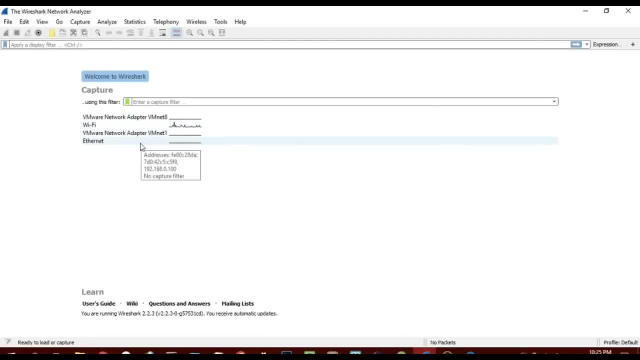 pretty interesting. I'm going to use my Wi Fi card, Although if you're using it Ethernet, just go ahead. Don't worry about these VMware network adapters. I have virtual machines running on my computer. That's why they have these virtual network at that adapters, And I really do know that they might. 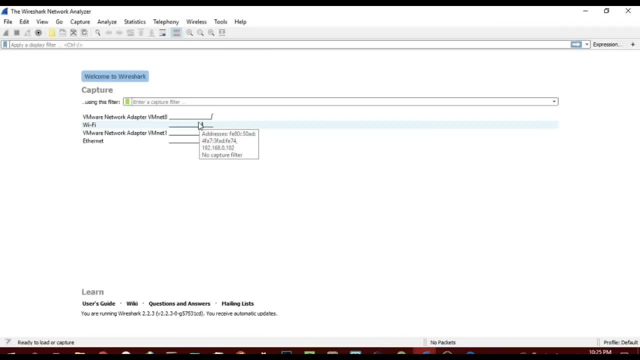 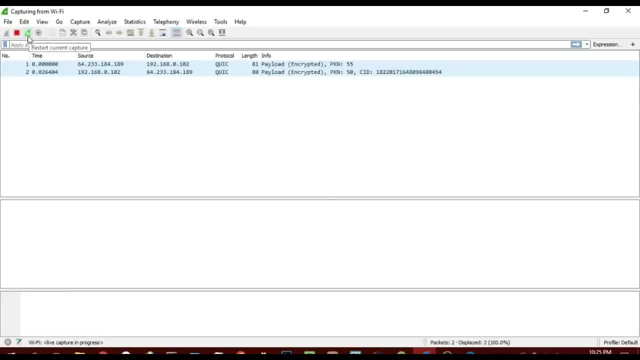 not be working, unless you're actually running the virtual machine, But nonetheless, that's for another video. What I'm going to do is I'm just going to hit Wi Fi. There we are, And it's. you want to hit this green button? Oh, it's already started, So 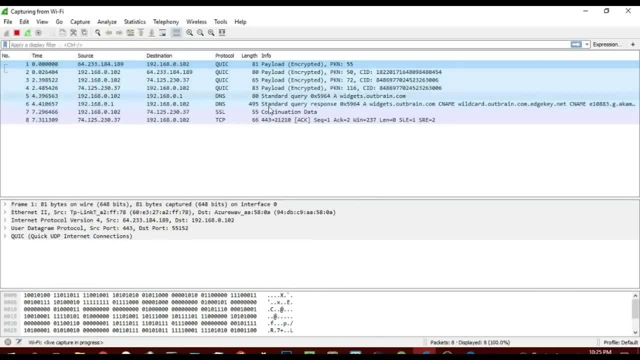 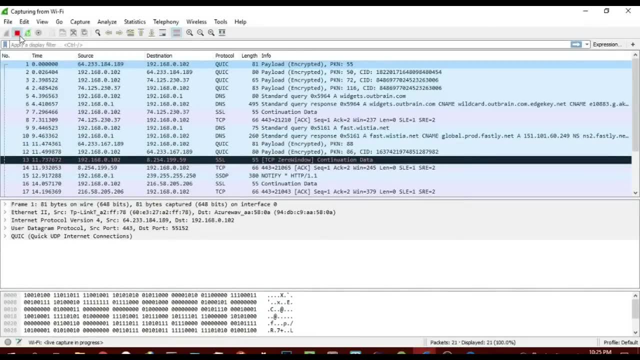 unfortunately, I did not have to press the startup button, it already started for me. So that's the thing. If you want to you, if you want to start capture, just hit the green button. if you want to stop it, hit red Alright, and then, once he stopped, it's going to stop capturing the. 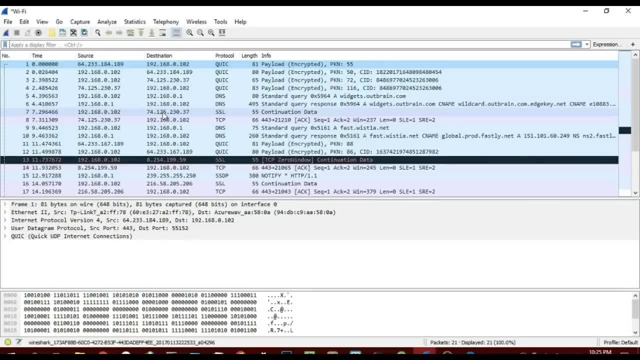 packets. So that's basically how to get started using wireshark. I'm going to cover all the other, basically the tools and basically the all the other nooks and crannies, in the next video. But uh, yeah. so those are all tips on using wireshark in this video while i'm riding to do. 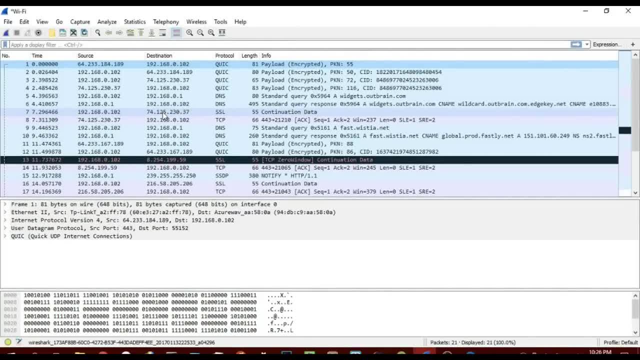 video. but yeah, I hope you guys are interested in this series of videos. I know it's gonna help you a lot, or maybe a lot, I don't know- but if it, if it does, and you really want to show your support, please leave a like down below. again one: 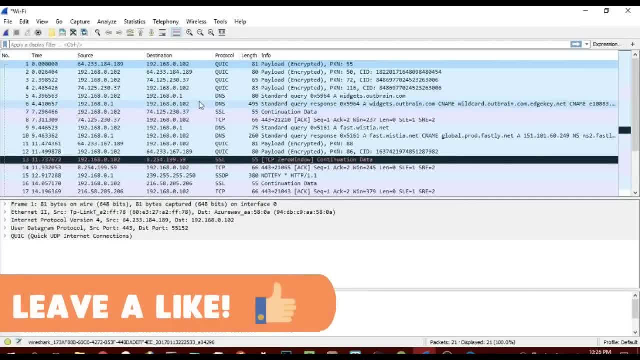 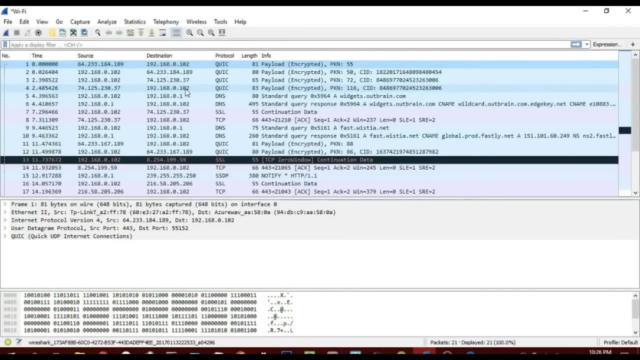 thing I would really request, guys, is that you follow me on my social networks. I need to get some followers on my social networks so they can- it's at least- build a community around what I'm doing, which is basically ethical hacking and cybersecurity. so, yeah, I mean, if you feel like, drop a like on my Facebook. 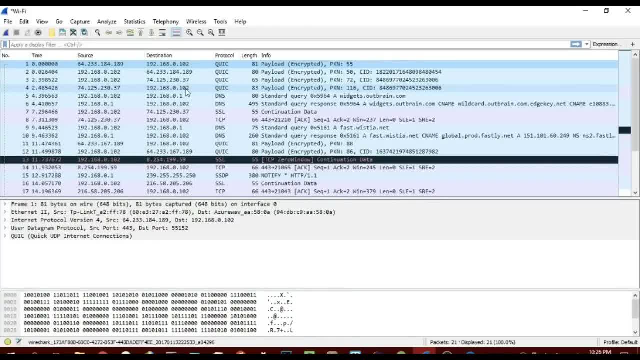 Twitter or follow me on Instagram. no worries, there you'll get all the latest updates on videos are working on and all the other stuff. the other thing is, guys, thank you so much for subscribing to the channel. it's grown a lot since the start of the year. I've grown from 500 subscribers in doing to 700 subscribers. 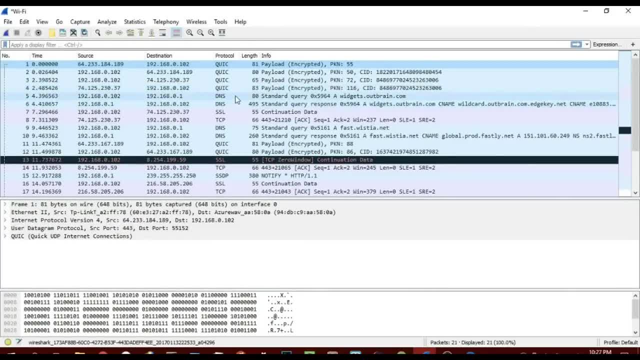 in like one or two weeks and that's that. that's really great, guys, and I'm gonna set a goal for this year, guys. you heard it here first in this video that this year only 10,000 subscribers or even more. so I've committed to the YouTube. 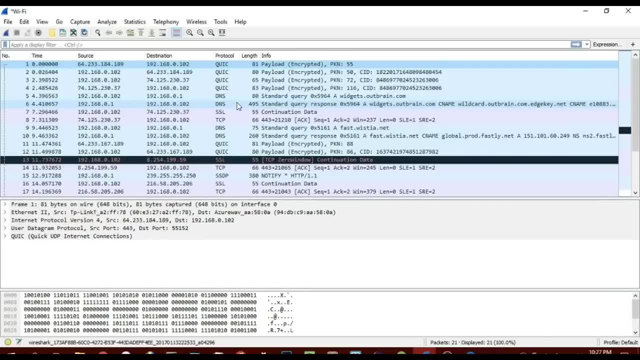 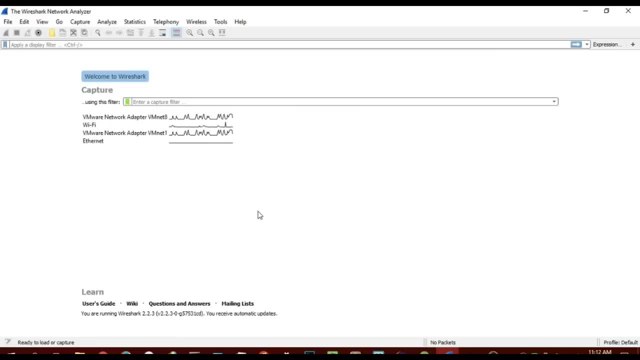 channel. I'm gonna be doing it regularly now. I know that's what you guys want you like: consistency. but enough of the chatter, I'm done. thank you for watching this video. have a great day and yeah, peace guys. hey guys, Hackersploit here back again with enough video now. this is the. 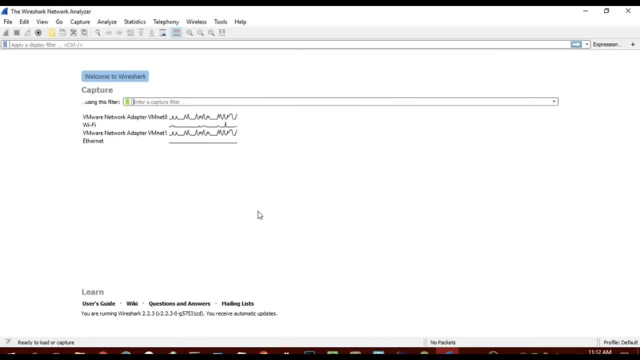 second tutorial of wireshark. so in the last lesson I actually told you how to start capturing packets in wireshark and what these actually mean, so let's start off from there. so again, I told you that these are the network interface cards that are actually going to be capturing the, basically the packets or the data. 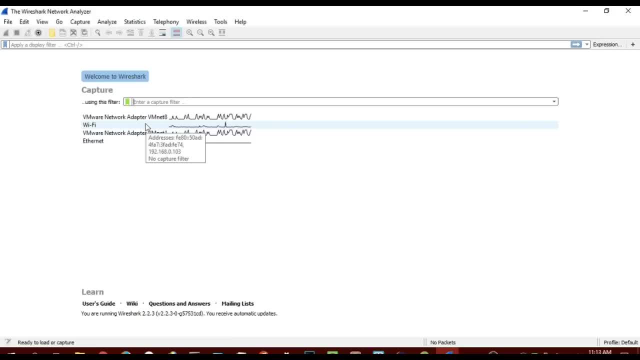 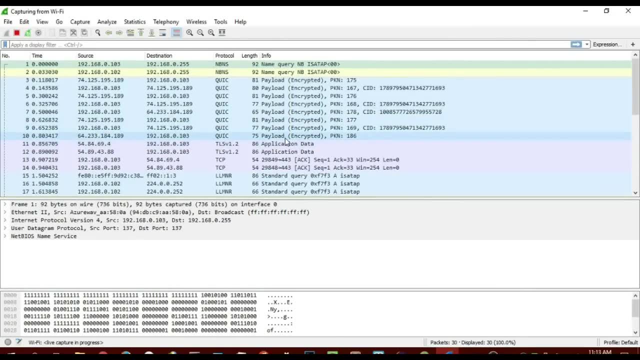 that being transmitted on the networks. so for now, I'm going to use Wi-Fi, because that's what I want to actually capture my packets with. so just click on that and then it starts capturing. so what I'm going to tell you now is how to basically analyze these packets in. 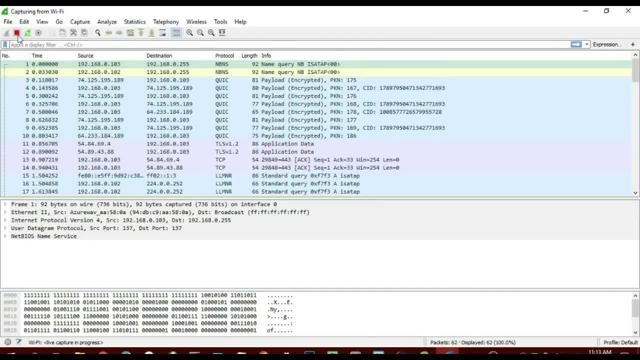 terms of what they are and what they carry. so, as you, as I told you, this is to stop capturing packets and this is to restart or start it. so I'm going to stop it and let's look at what we have. so you basically have three sections over here. 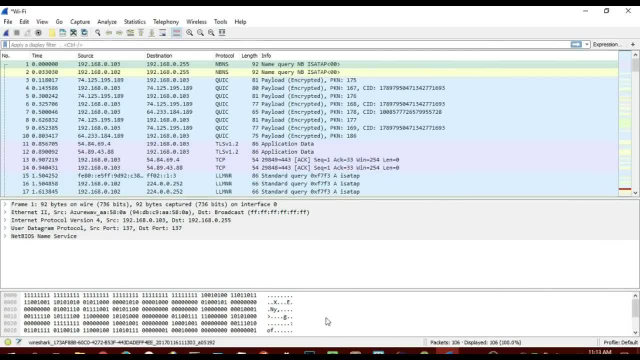 in wireshark. you have this section, you have this one here and you have this last section here. now, this section is basically the packets that are being scanned and have been actually scanned. as you can see, there's something that it's encrypted. now this second portion of the screen here is giving more. 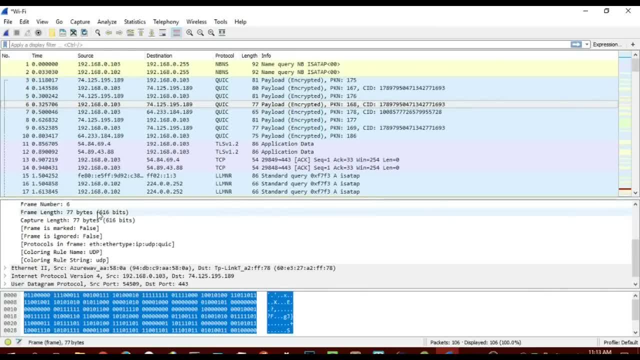 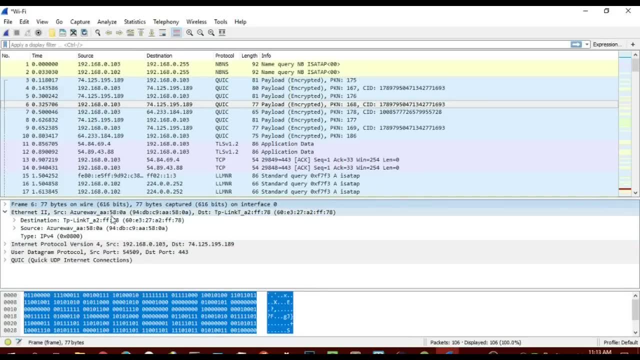 information about the packet. so, as you can see, it gives more information about what the packet is and how it's being transmitted, and the and the, basically the manufacturer of the, of the device that's transmitting it. so, as you can see, TP-Link- that's my router. it's telling me the source. 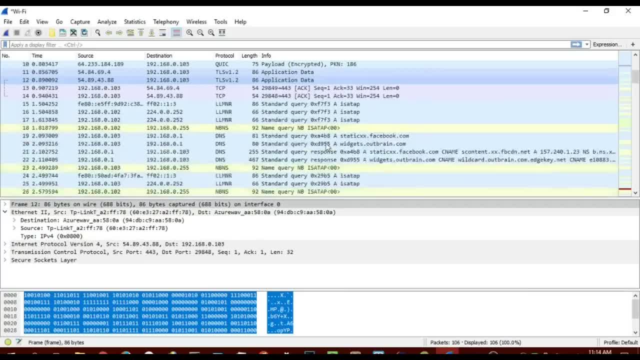 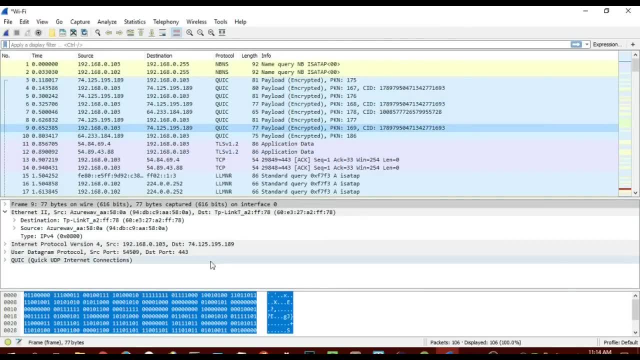 with not really much you can work on, of course, because this is not really a useful packet that has captured. but so, basically, this screen here gives you the packets that being scanned, this one gives you more information about the packets and this screen here is probably the least used in wireshark. this is 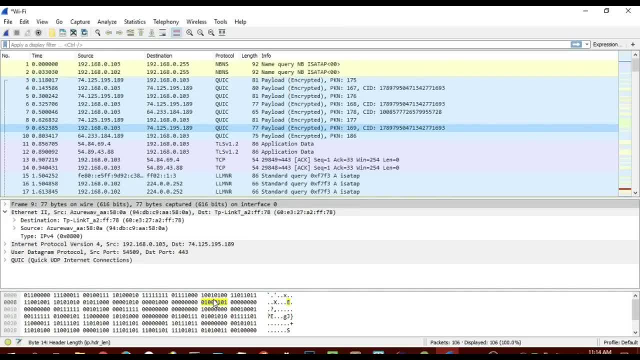 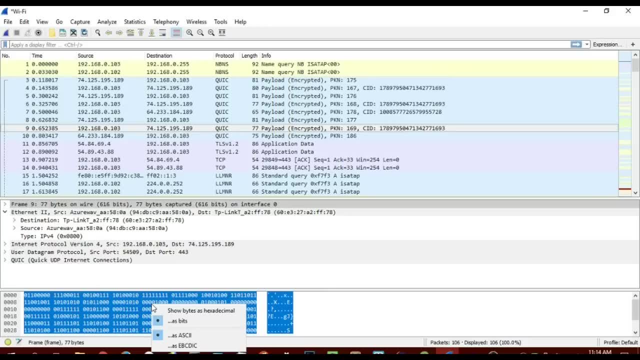 basically the raw transmission between your computer and the router, and what this means is this is how your router and computer are basically communicating with each other. so, as you can see, it's in bits and bytes, and you can say it as bits and you can show it as bytes. so this is basically it. now, the other thing i wanted to show: 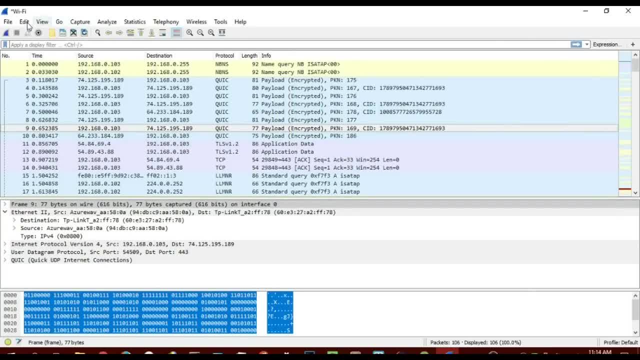 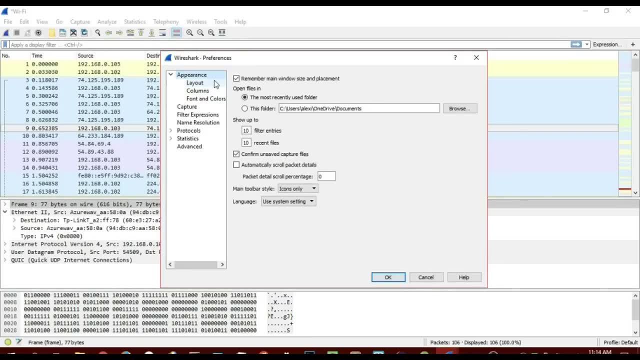 you is how you can basically edit this um interface to your specifications. so you're going to edit and you're going to preferences. now, these preferences are focused more on wireshark as a as for the wireshark layouts. so we have layouts here and, as you can see, you have the different types of. 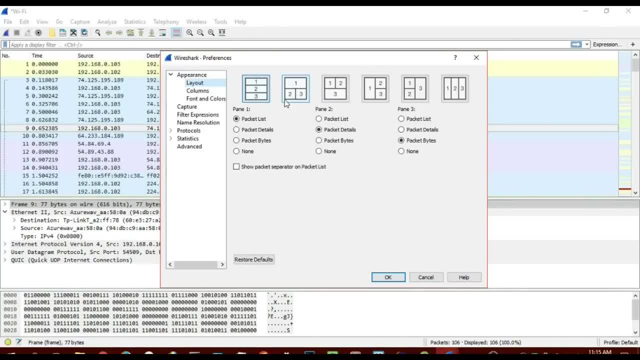 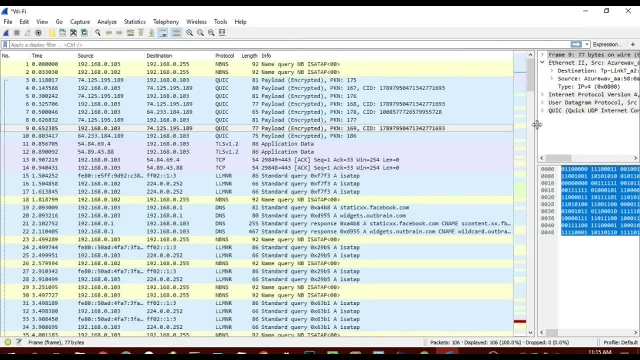 layouts. you can have one, two, three, which is what we have now: one, two, one, two, three, uh. one, two, three, uh. but the one i like to have is this one, because it just basically puts it in a very nice way. we can read the packets in a long and a long type of way and you can basically minimize that one to the. 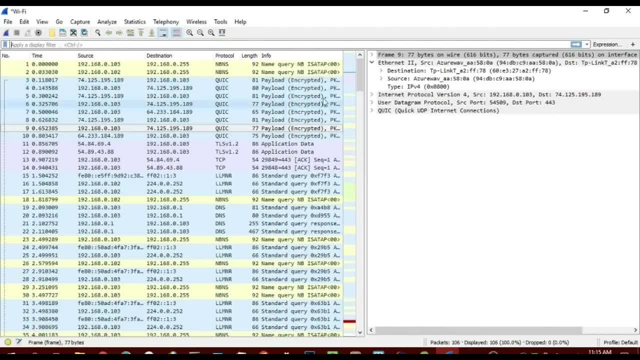 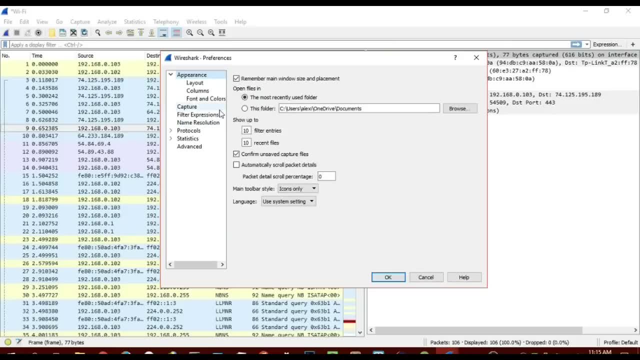 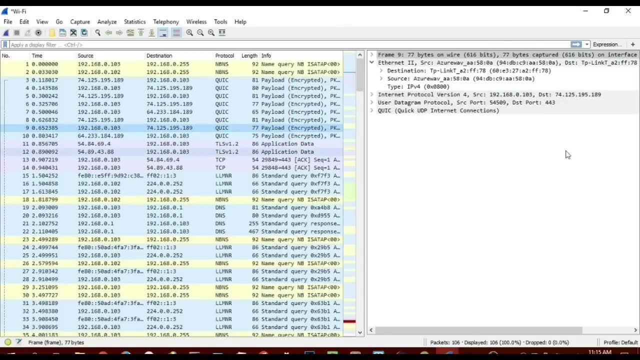 bottom. and yeah, there you are. it's basically split equally and you have more screen real estate for whatever you're doing. so, again, if you go into preferences, it's just the basic layout of all of how you want wireshark to look and how you want it to work for you. so that's basically the layouts and what each of 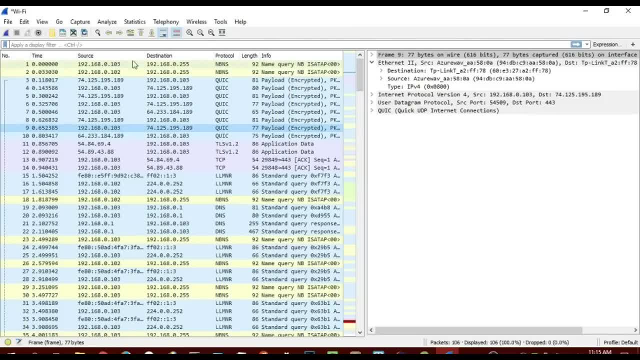 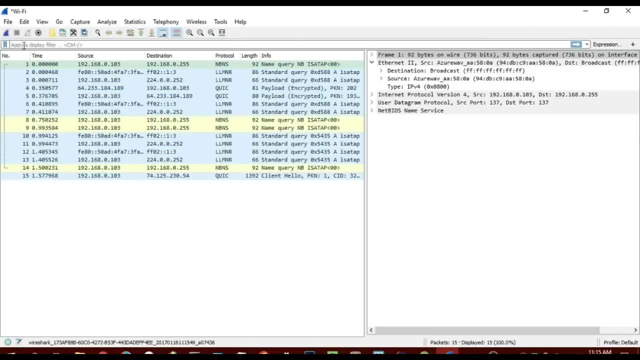 these panels do. now i'm going to talk about the toolbar actions here. so, as you can see, we have a few, quite a few things you can use on this toolbar. so, as we know that this is to start capturing packets, so let's start capturing new packets and you can stop capturing packets, and then you can. 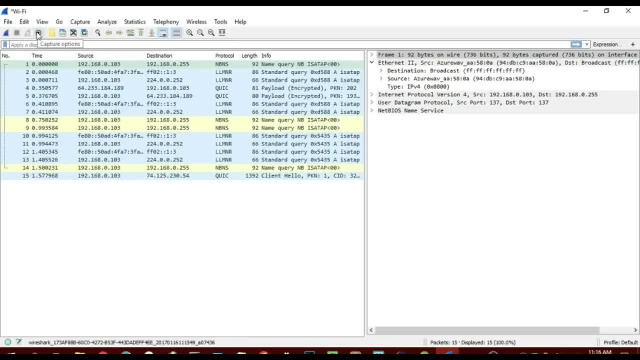 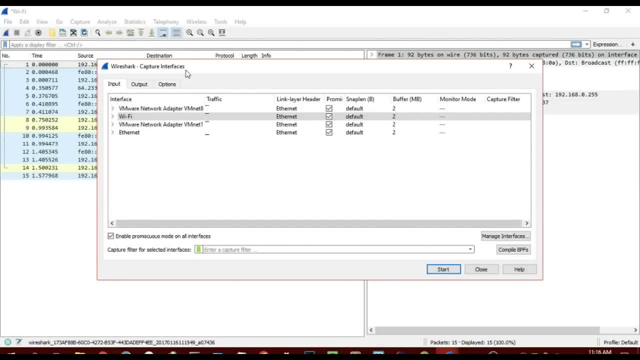 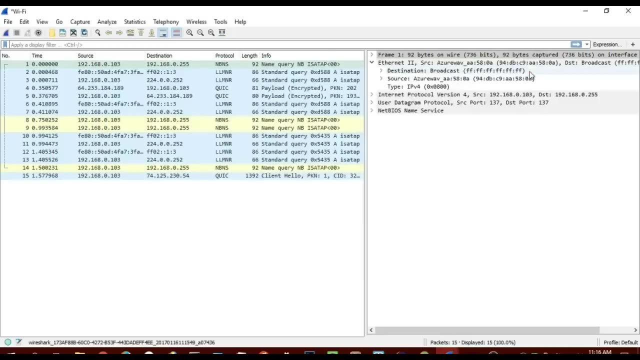 restart the current capture and you have your capture options. now, the capture options is something i'll visit in the next video, because it's a quite uh of an advanced tutorial, the next one where i'll be showing you how to actually specify what packets you want to scan, so we'll leave that for now. you then have open a capture file. 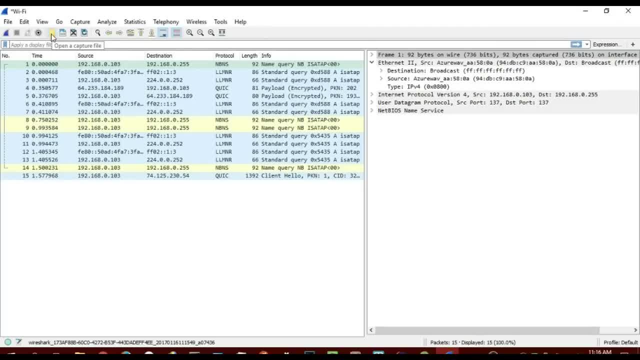 this is, if you have already a saved capture file, which you can do, by the way, you can actually save whatever you've captured. uh, the next one is to basically: uh, open, uh, you can save the capture file that, the one you already have. close this capture file, reload the capture file, find the packet. so 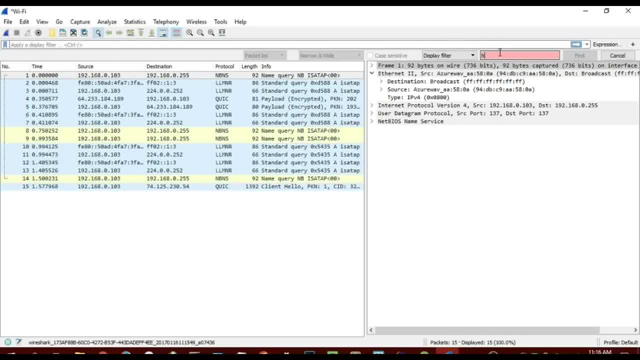 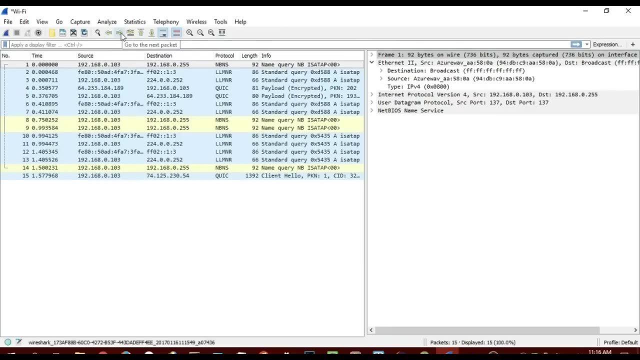 for example, if you want to find a packet that you just can, i'm just going to use a basic protocol, http. um, let's find, and we didn't get any because it did not scan for any http. but we'll get to that, you know, in the next video, um. so here you have, the previous packet. 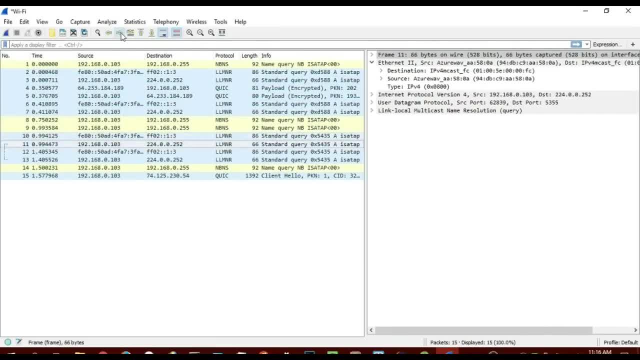 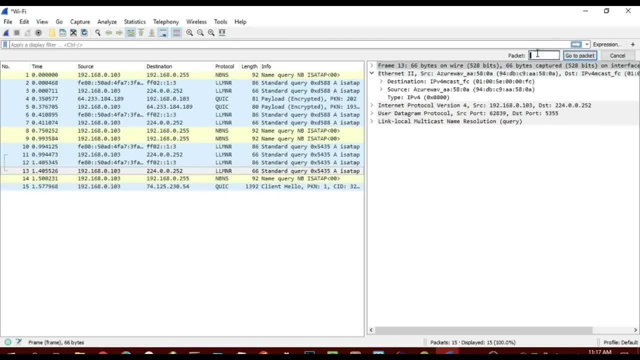 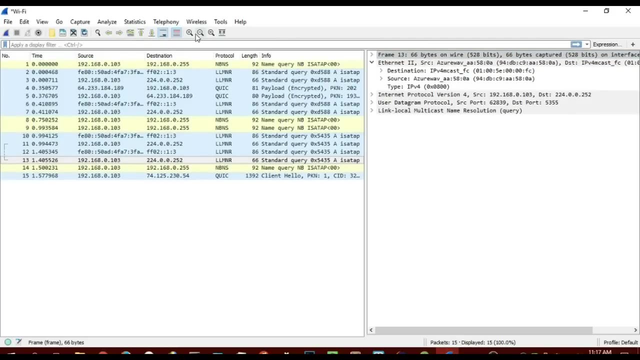 here you have the next packet and, as you can see, it scrolls through the packets, uh, in in the packet list that you've just scanned. then you have uh, go to specify packet and again you can scan via the number, by the number or the id here. so we can say: go to packet and it's going to scan. 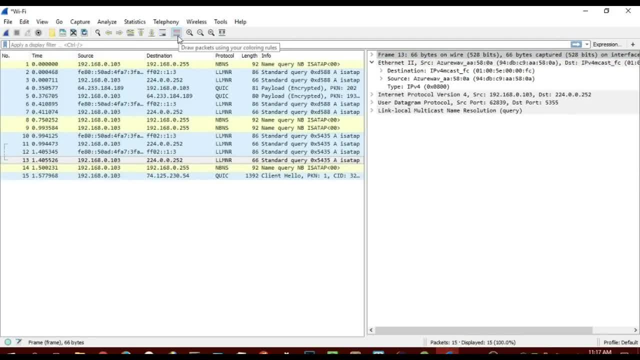 like that: yeah, the next one we have here. uh, sorry, it's here. go to the first packet and go directly to the list. and uh, here we have. go to the bottom packet, which will take directly downwards. the next uh tool we have automatically scroll to the last packet during the live capture. 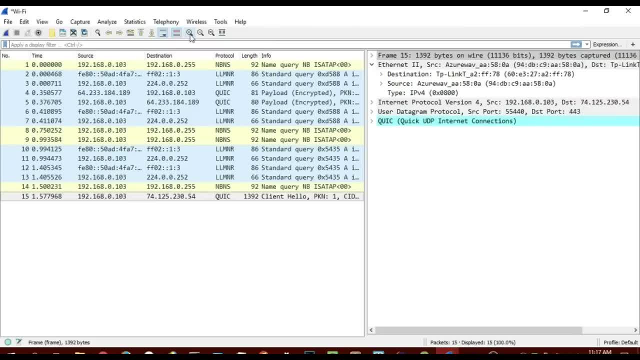 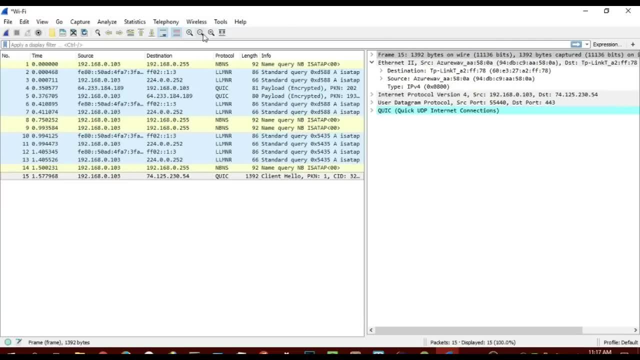 that obviously we know is this one right here. you then can zoom in the interface if you have, if you have problems reading. so that's very, very useful and you can zoom in and out. so basically that's what it is and this will basically apply the defaults to the default. 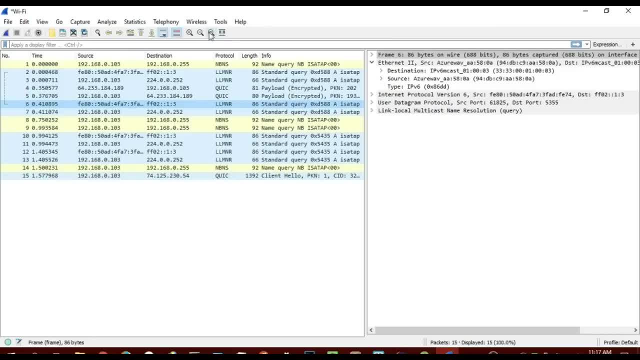 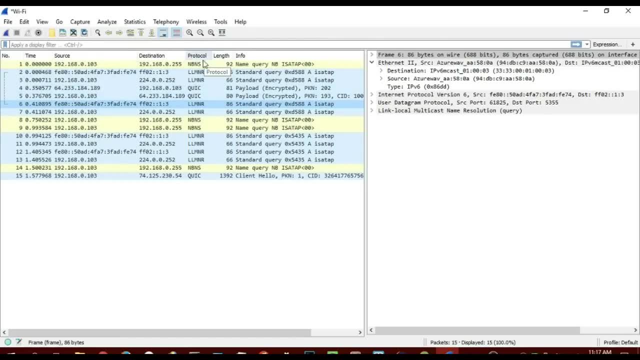 size and it will just restore whatever you've zoomed or zoomed in or out. the next thing is resize the packet column list. this is pretty self-explanatory. you can just resize, uh, these little, these columns here to your, to your liking, all right. so that's basically the. the toolbar actions don't. 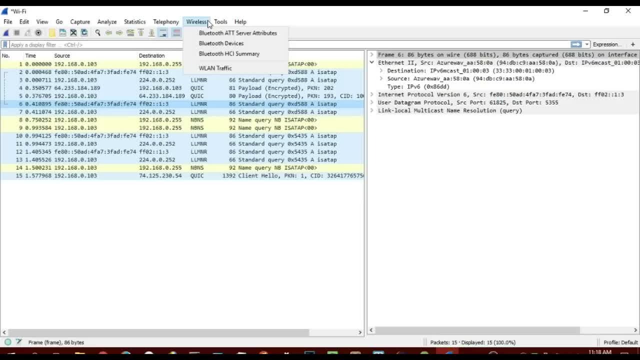 worry about these, um, these little tools up here. these are just uh for another tutorial. i'll be covering them, but you don't really need to need them right now. so that's basically for the second tutorial. uh, the next tutorial will i'll be showing you how to actually scan uh for packets, um, and how. 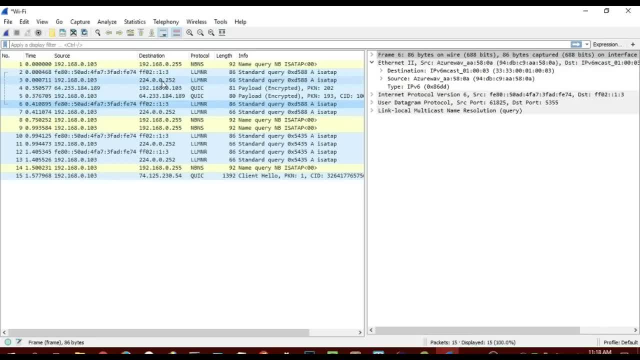 to uh specify what packets you can get so you can actually make some sense of what you're scanning and how to get valuable information from them. so yeah, um, thanks for watching. guys, if this video helped you, please leave a like. follow me on my social networks. they will be in the description. 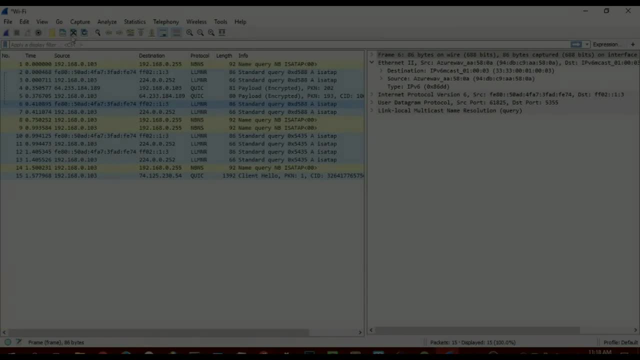 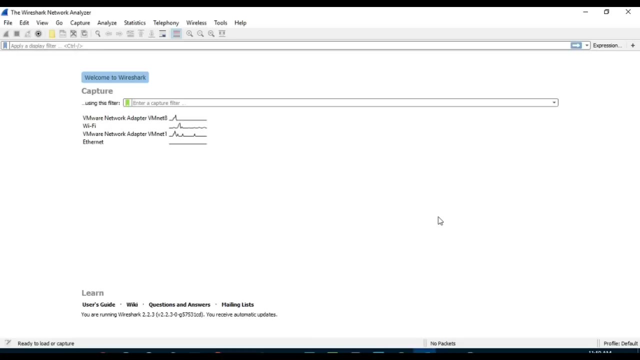 on the screen right now. uh, anyway, guys, thanks for watching and peace. hey guys, hackersploit. here back again with another video and welcome to your third wireshark tutorial for beginners. so in the last video we talked about the environment and how to basically change the layout of the environment in wireshark to meet your specifications. 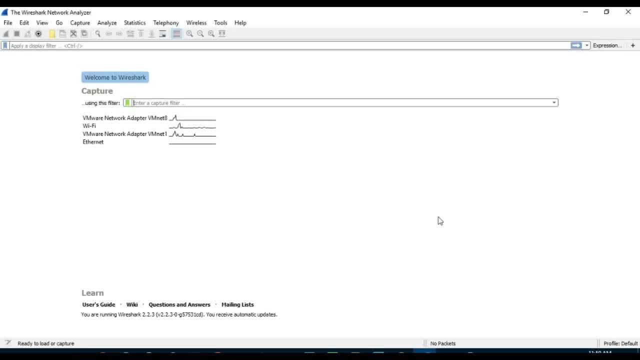 or whatever you feel, uh, more suitable for you. we also looked at some toolbar actions and what the the icons on the toolbar do. now, in this video, i'm going to be talking to you about the capture options and the interfaces in depth. so, again, this is what i'm going to be talking about. 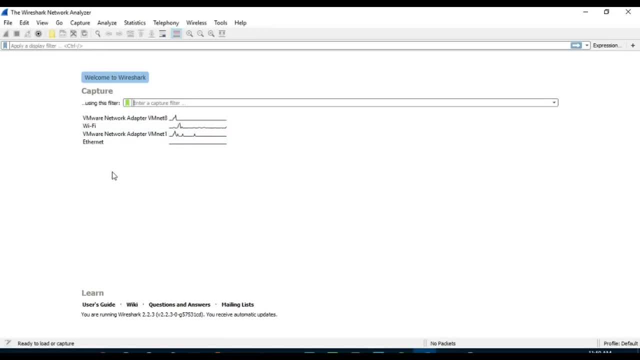 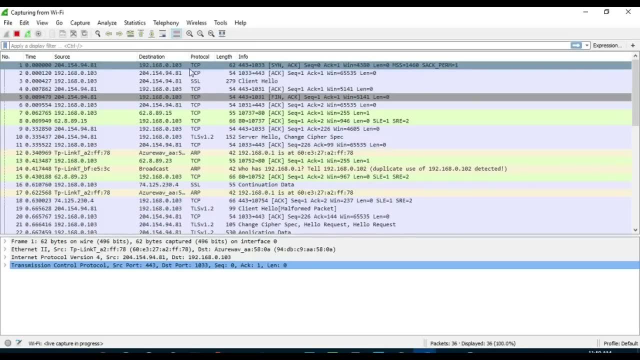 the whole capture options and interfaces just for the sake of this. uh, for the starting of this video, we're just going to select wi-fi. all right, we go, or whatever nick or network interface card you're using. so i'm just going to stop, uh, scanning for packets. 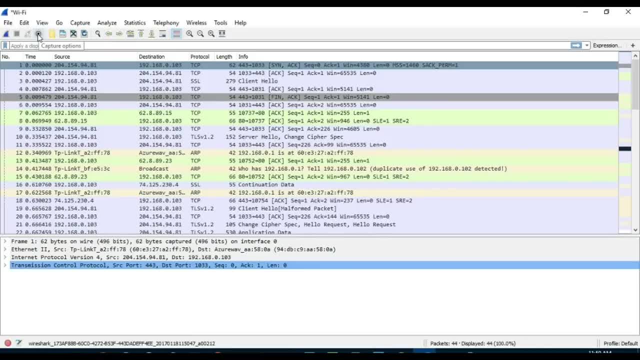 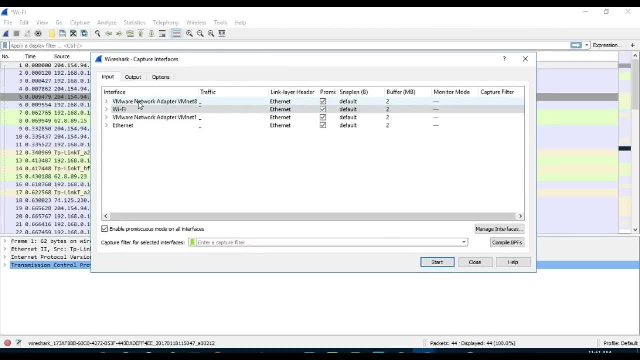 and i want to just show you something here. you want to hit this little capture options icon here and once you hit that, it's going to open this menu. now, as you see, there are about four network interface cards that i have here now. two of them: the vmware network adapter. 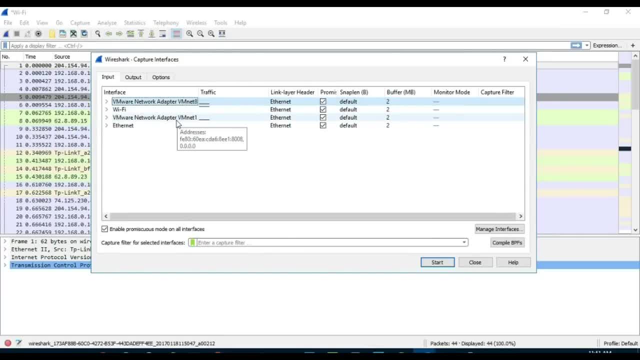 and this one right here. one and eight are not real in the sense that they are not actually hardware, they're just software. virtual network interface cards. these are for my virtual machines. i have two: my wi-fi and my ethernet. i'm currently using my wi-fi card, so that's. you want to select? 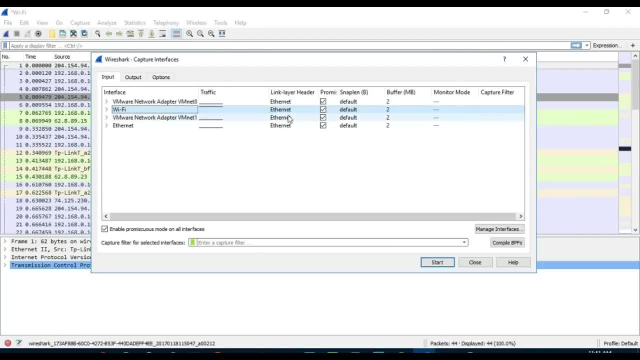 the one that you're currently using. now it's going to give you information, more information about it. now, when it comes to this tab here, the promiscuous mode. what this means is that, whether or not you want to allow your wi-fi card to read packets or read data from other devices. now let me explain. 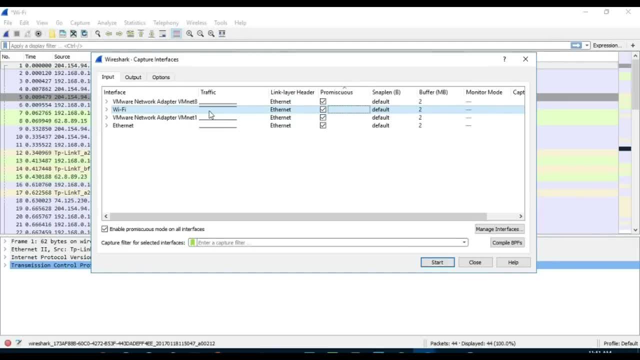 why this is a actually a setting. you have two options: when promiscuous mode is enabled or disabled. when it's disabled, wireshark is only going to scan data or packets that are meant for your computer and it's not going to scan for packets from other devices, from their devices to the router. 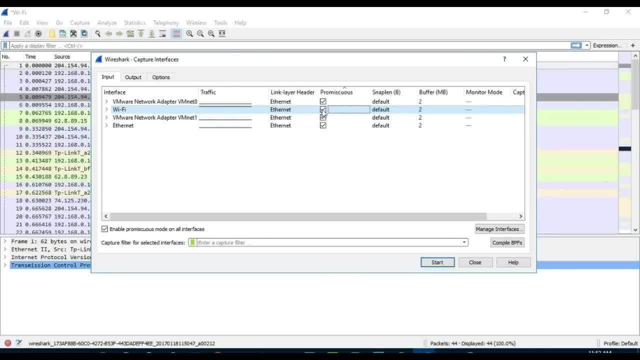 so that's basically what promiscuous mode is. promiscuous mode basically pays more attention to data that's going to and from other devices, so it actually allows you to read packets and data from other devices. now again, this is highly legal without permission. i don't recommend you going and 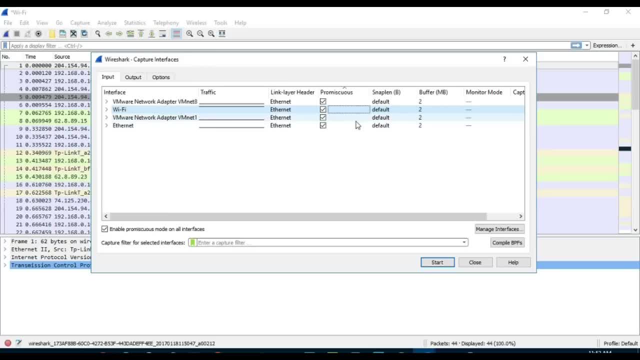 using this, this method, like in a public place, it's highly legal and if you're actually caught you will be apprehended and it's a crime. so again, you have to have permission from your network administrator, or you basically have to have permission to scan the packets on the data. so 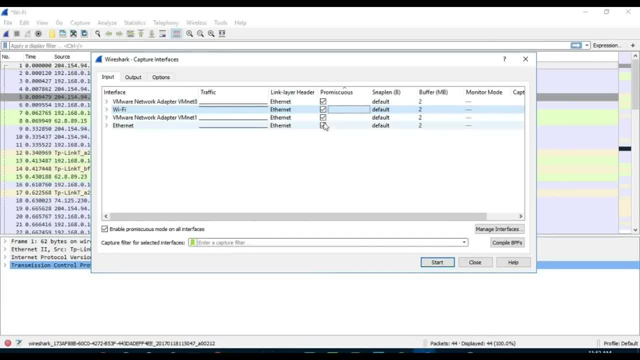 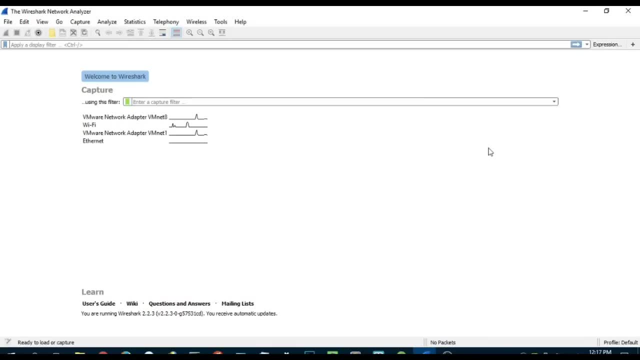 yeah, that's pretty much about, uh, what promiscuous mode is. so let's get started. hey guys, hack exploit. here back again with another video, and welcome to your fourth wireshark tutorial for beginners. now, in this tutorial, i'm going to be showing you, uh, the two different types of filters. 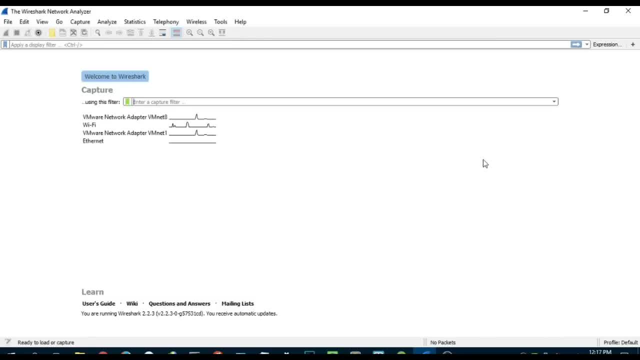 so, basically, a filter is a tool that will allow you to basically fine-tune your search for packets and data that you've scanned or are scanning. so, uh, let me just use my wi-fi card here and let it scan for some data, and i'll explain as we go. 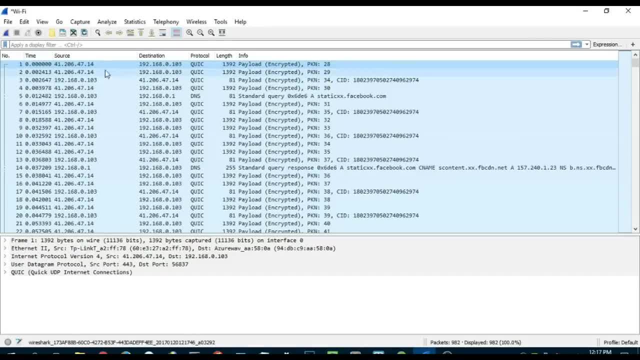 so i'm just going to stop it there now. basically, a filter will allow me to fine-tune, to pick specifically what i want from these packets. so, for example, we have- as i mentioned earlier, we have two types of filters. we have a display filter, which is right here, and we have 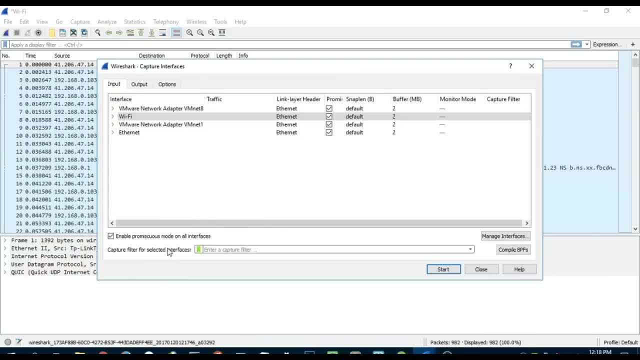 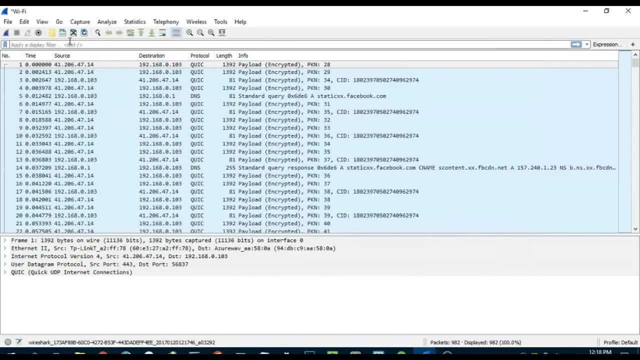 a capture filter. now, a capture filter lies here. this is the capture folder that is specific to the network interface card that you are using. but let's start first with the display filter. so i'll stop scanning and then i'll show you how to use the display filter. so let's start with the display filter. 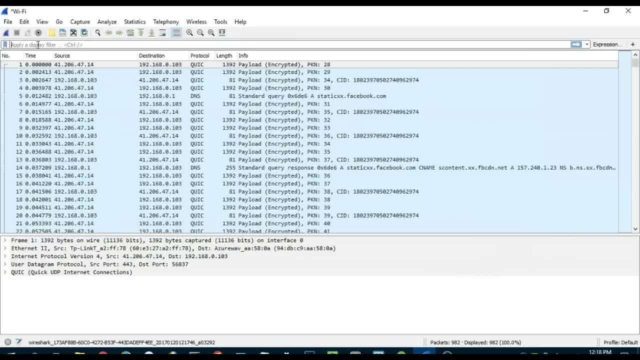 let's say we want to find a specific packet out of all that we've just scanned, a display feature. a filter is basically a filter that it will give you the packets that you want to see or you're looking for, not the packets that you want to scan for. so let's try http and it's going. 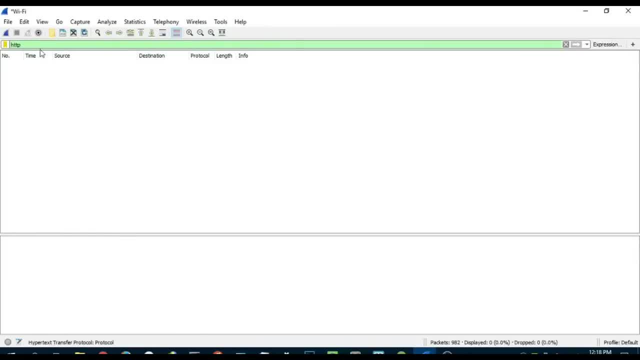 to give us all the http packets. so, as you can see, we really don't have any http packets inside. let's try something else. so i'm going to use dns and, as you can see, here we have some dns. they're going to connect into Facebook and, yeah, that's pretty much how to use. 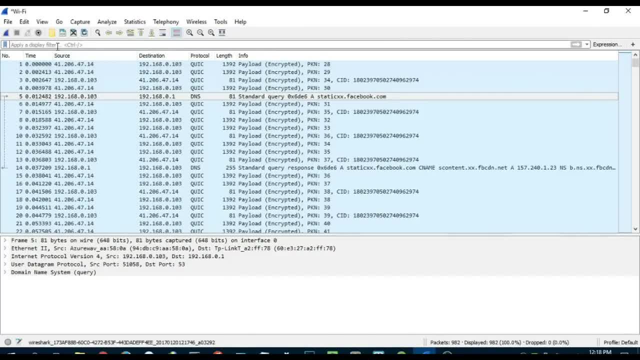 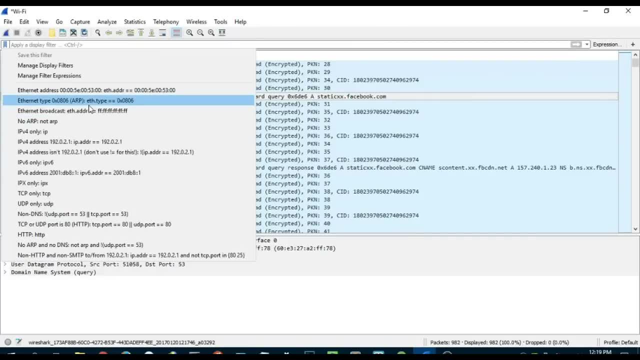 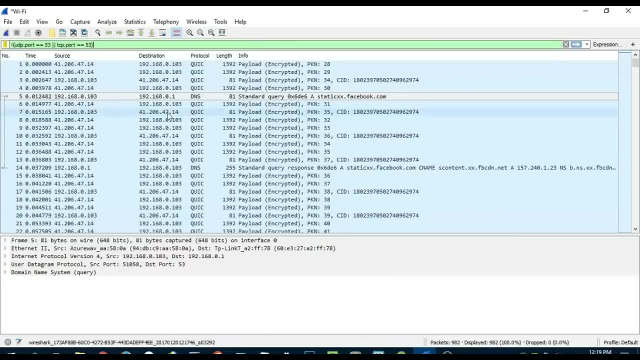 the display filter to your advantage. now, as I mentioned, there are a lot of filters that you can use, and some of them are here. as you can see, these are the most popular filters. we have Ethernet address and IPv4- IPv6. you have TCP, UDP and non DNS, so it will scan for non DNS packets of data, and here they. 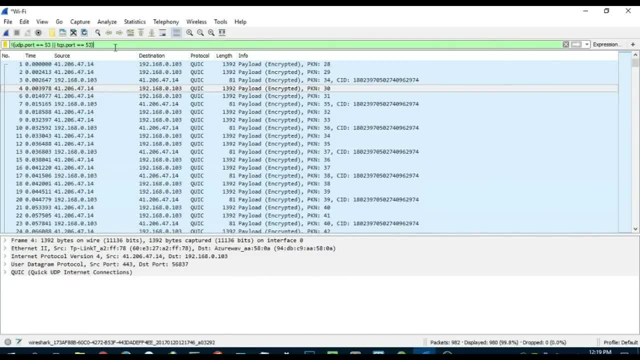 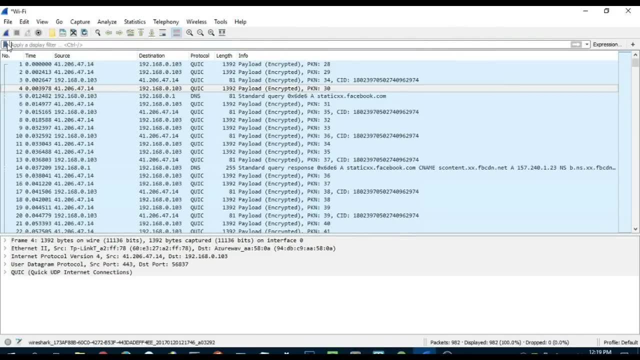 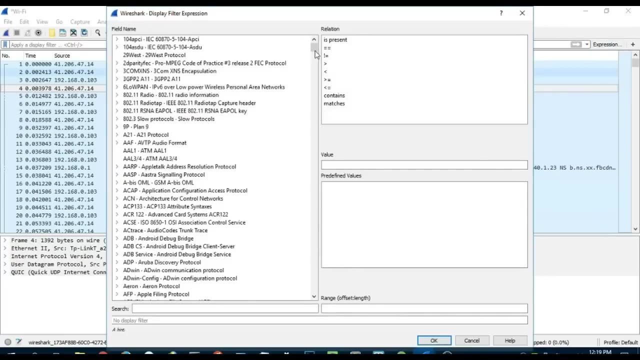 are and you can just apply it. and if you're once you're done looking for once you're done, basically using your display filter, you can just hit the X button there or the stop button and you'll be good, right here now. the next thing I want to show you is expression. now, expression gives you all the different 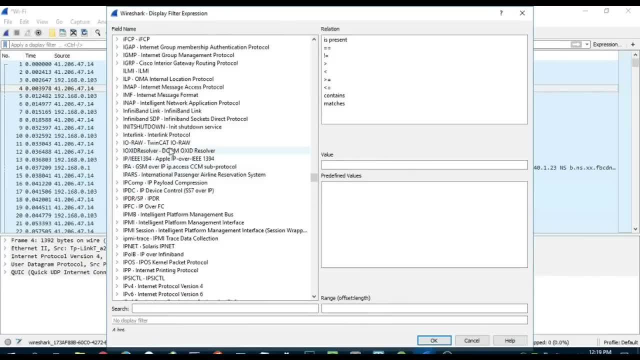 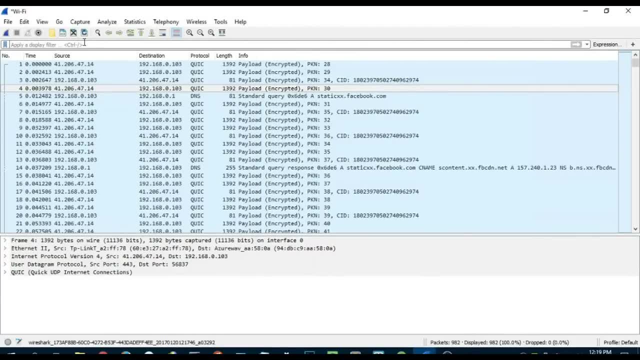 types of filters that you can apply with: with basically with with capture, more advanced capture options, some that may not exist over here, and the most commonly used. so I'm going to give you an example. let's say we're looking for HTTP packets, but only HTTP get packets. no, not post us. so let's try that HTTP. this is the 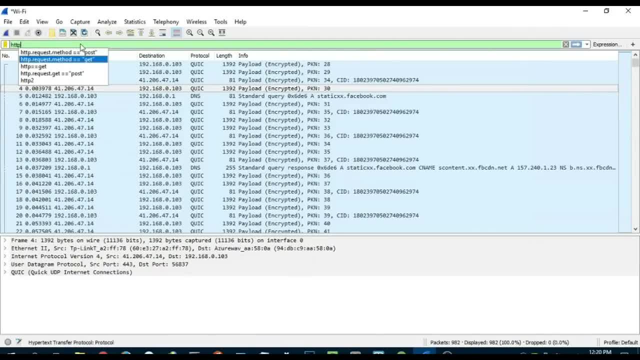 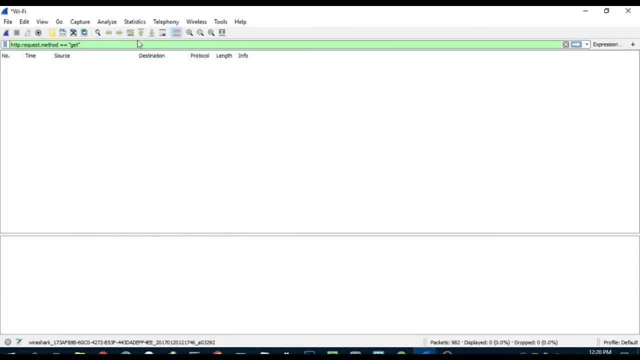 basically the filter that I'm going to use and I already made some here. so we have HTTP, HTTP request, dot method, dot get. so I'm going to type that in and again, we don't have any HTTP yet. so let's try post, post and let's close that. 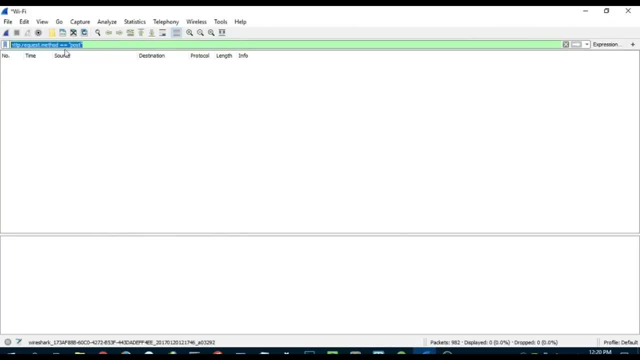 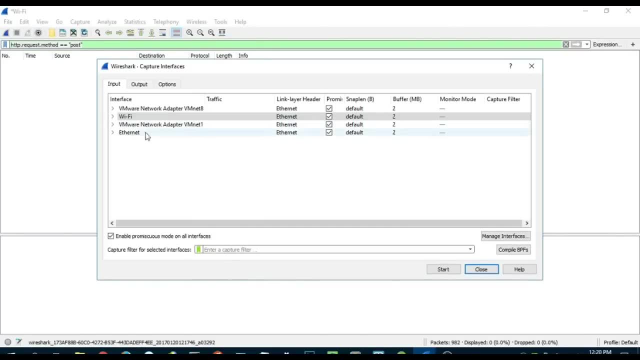 and still nothing. that's basically how you can find your packets. you want to, what you want to see from the packets you already scanned. now, when we go on to the capture filter, a capture filter is the packets that you want to scan. like, let's say, you want to scan only for HTTP, you only, it will only. 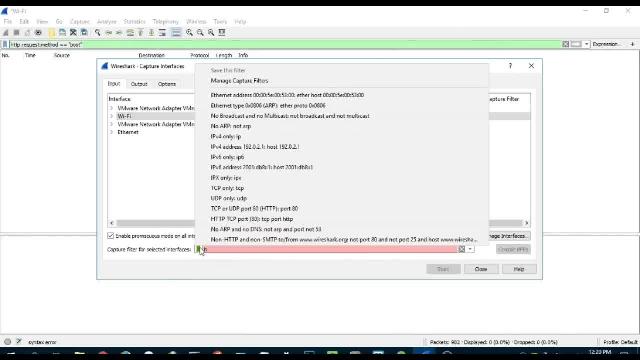 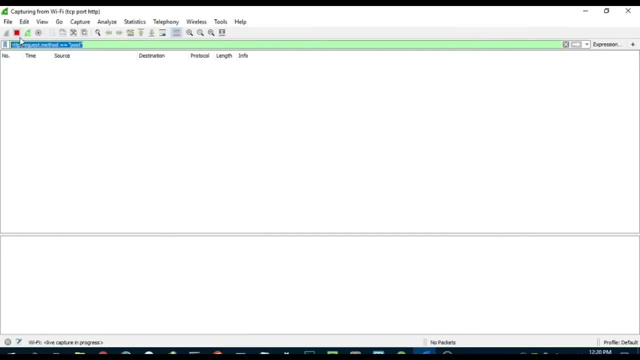 scan for HTTP. so, as you can see here, if I go into the most common one, so let's see HTTP, TCP, port, HTTP, and we'll start capturing from there and then we can stop it and so on and so forth. so that's basically the types of filters that you can use in wireshark and 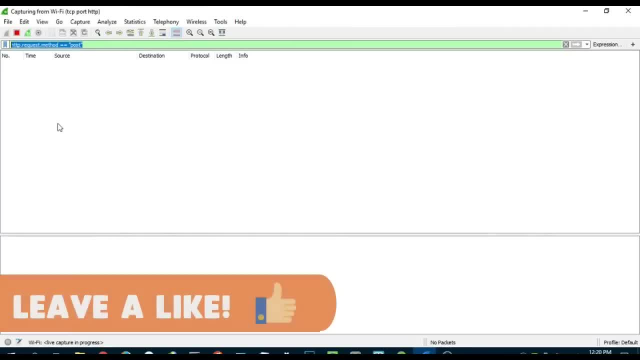 now you can use them to fine-tune your results on packets or what you want to see from the packets you've just captured. so, yeah, guys, that's pretty much it. pretty much it. thanks for watching this video. if you enjoyed it, leave a like and yeah, peace. 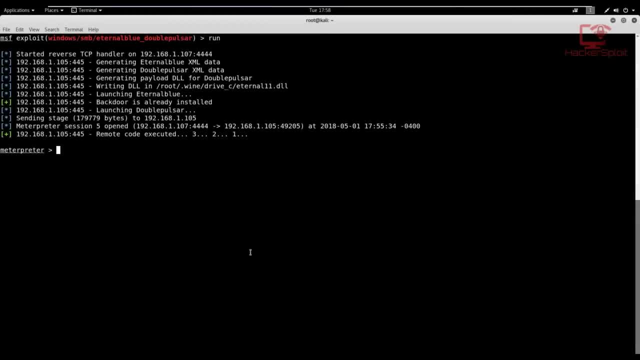 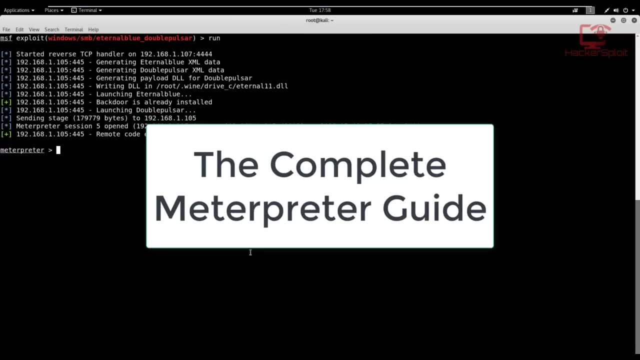 hey guys, Hackers, out back again with another video, and in this video I'm going to be showing you how to fully utilize meterpreter, or a meterpreter session, for post exploitation, privilege escalation and finally clearing up your tracks, right? so I've mentioned previously in the 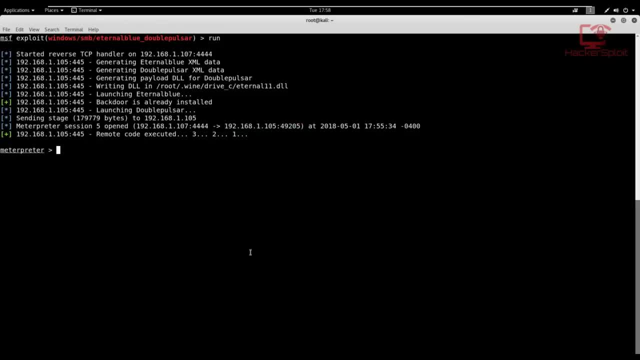 community section of the channel, the reason why the s7 video is not yet out and the reason for the lack of uploads over the last pop-up over the past two days, and that is because I'm I was actually feeling a bit sick and I'm feeling much better now, but if my voice 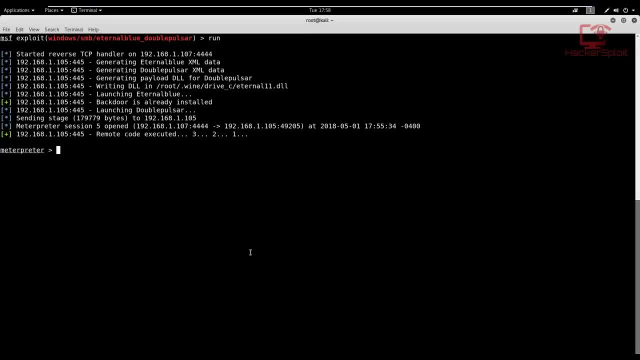 is a bit low during the video. I apologize and yeah, that's what I wanted to pass on. that being said, let's get started now. I'm going to assume that you already have a meterpreter session. most, you know, it depends on what exploit you perform, but for me, I'm just gonna be using the most. 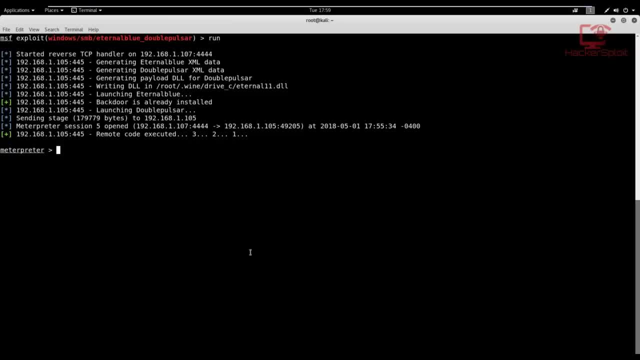 recent one, which is the double pulse exploit. and for those of you asking why I made the video so late, I didn't make, I didn't even plan on making the video. someone suggested to me to make the video. as I said, I follow them. I usually put all the videos in only a video that I've made before, but we'll see how that goes. make the video. as I said, I follow them. I usually put all the videos in one few minutes, and those videos are usually in the group, and that's why all the videos have been uploaded. so the third one is an extended version, and instead of a video like this, one is simply making one, and that's why this is something I'm making. 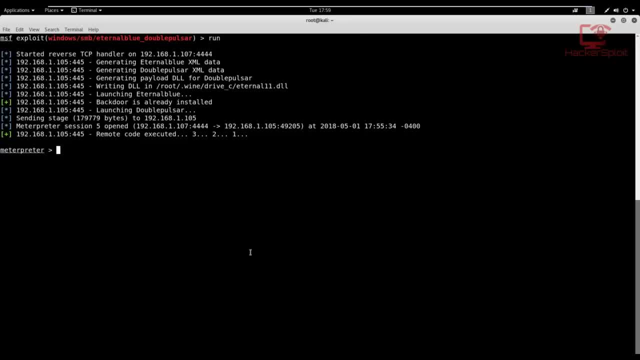 follow them. I usually put all the videos in an Excel spreadsheet and I follow them as and when they were posted. So if you have posted a video suggestion, it will come, or I will usually put in an Excel sheet and it will come independent or in relation to, to to when you posted it in. 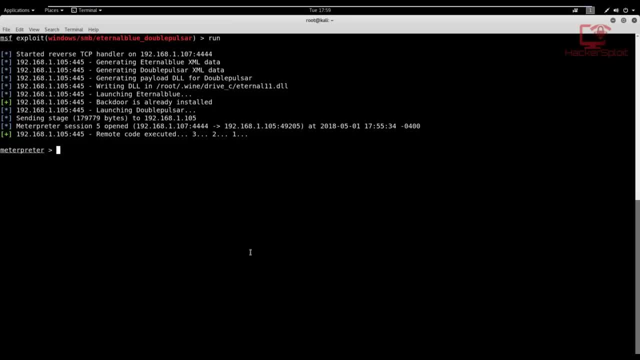 terms of date. Alright, so I'm currently going through all of them And I'm making videos, as you can see, of all of the topics you guys requested. That being said, let's actually get started. So in the previous video, I really didn't do justice when we exploit, exploiting the eternal. 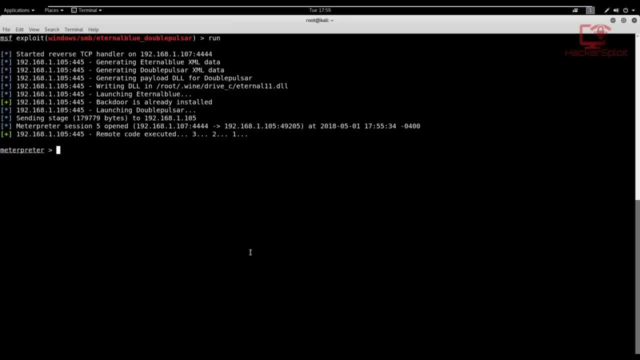 blue double pulser. I really didn't do any justice as to what you should do after you've gained access to the system. That's because that video focused more on the exploitation side. That being said, I have the Windows seven virtual machine currently running And, as you can see, we have 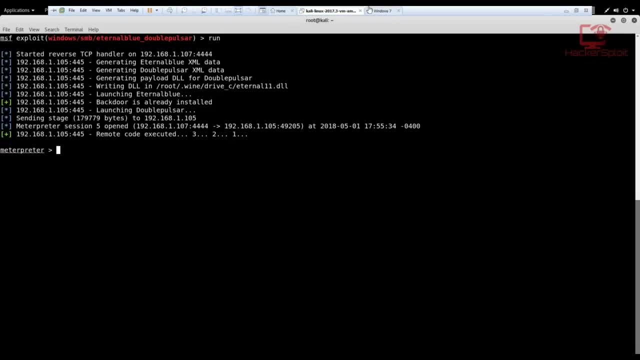 a matter of practice session. So we're not going to be focusing on how to get out, to exit the system. So we're not going to be focusing on how to exit the system. So we're not going to be focusing on how to get out, to exit the system. So we're not going to be focusing on how to exit. 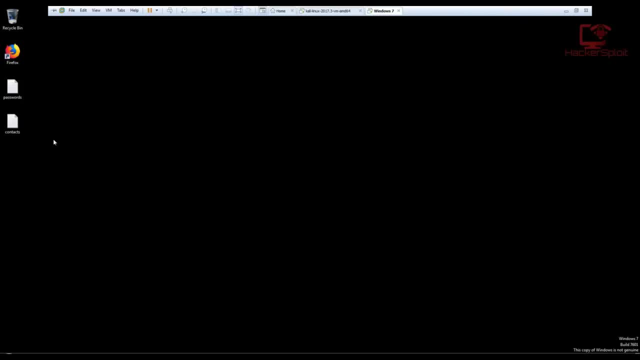 exploit it, because we've already looked at that. But, as you can see, I have a few files that I've just created on the desktop here that I'll use to illustrate how one can download files from from the target operating system onto your operating system, how to clear your tracks, how to perform. 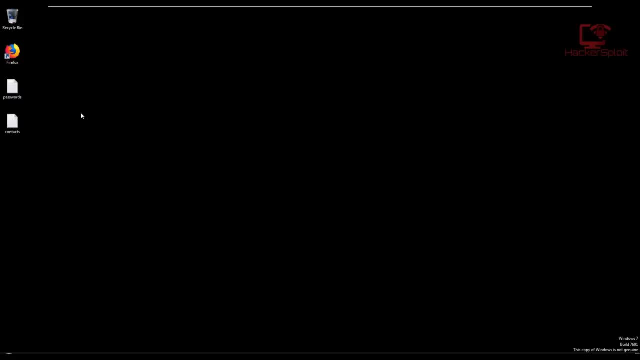 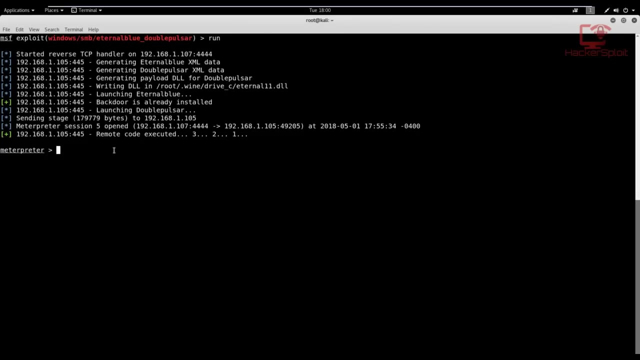 privilege escalation, how to launch different exe programs, how to edit files- all that good stuff, right? So let's start off first with with the basics. as you would know, you have the meterpreter session. Let's start off with the help command. Alright, 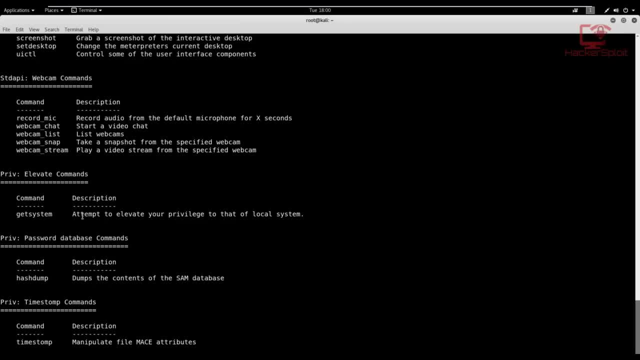 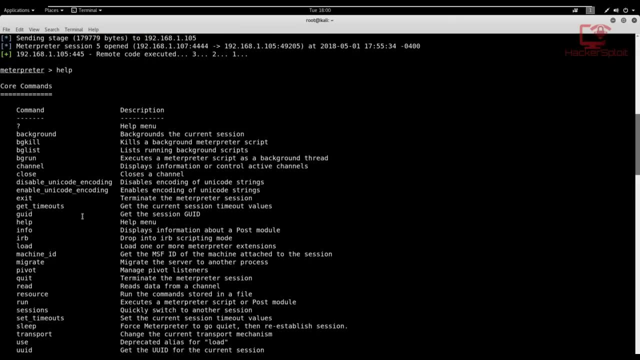 so the help command is extremely useful, as I've said many, many times before. Alright, and you can already see that, it's going to give you a list of all the commands that you can use, And they are sorted out in terms of core commands. you then have your file system commands. 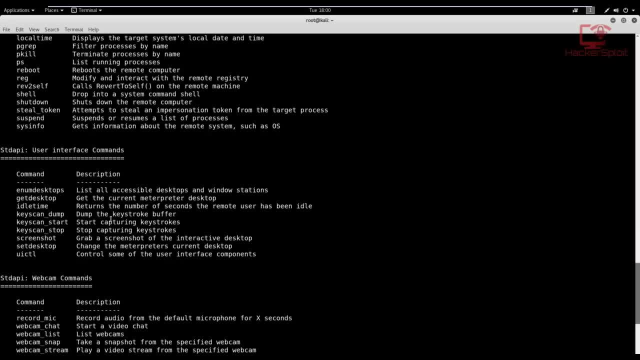 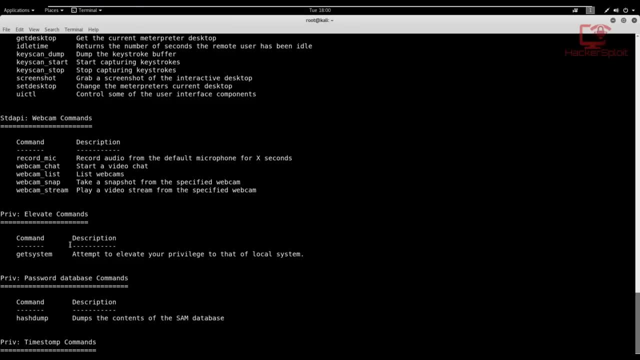 networking commands, system commands, user interface commands- very important- webcam commands, also really important. you then have elevate commands which will, as you can see, get system and that will elevate your privileges to that of the local system, meaning you'll get administrator access- I was about to say root access, but in with Windows. 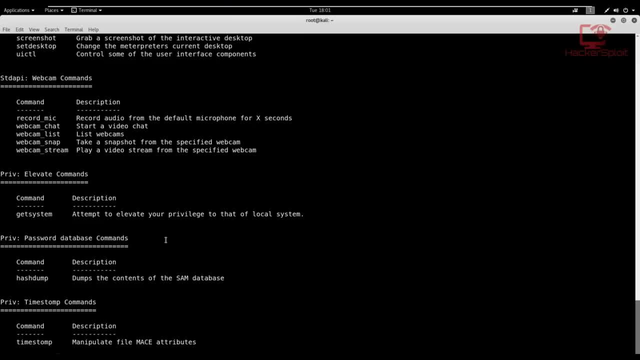 it's slightly different. Alright, you can then get the password database commands- very important. you can perform a hash dump that will dump the, the contents of the SAM database, which you can then use to decrypt and get the password for the user or the or any use on the computer. All right, 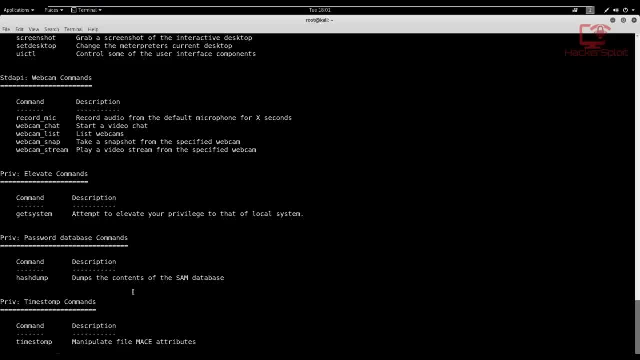 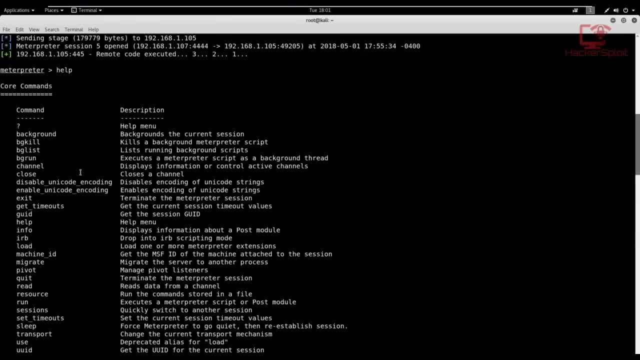 So you can see- and we start off with the core commands- you have your background processes of the current session. you can kill a background exemples script. these essentially core commands that deal with how the metaboliser session is handled. So you can see, you have the channel close, you can exit, get timeouts, you can get. 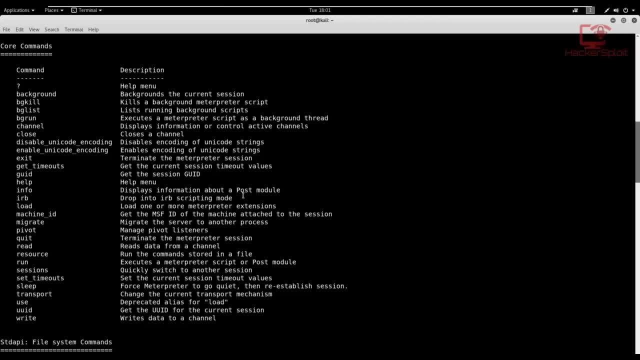 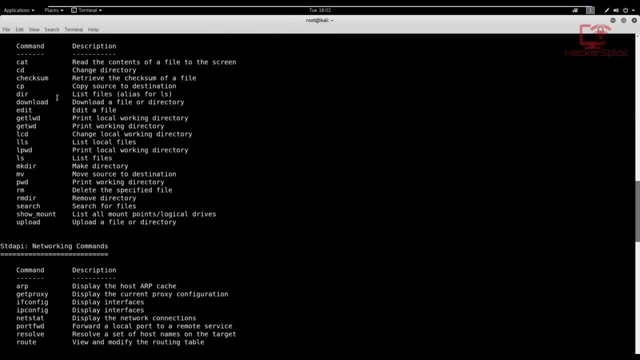 in four And if you look at in four displays information about the post module. So this is more focused with the interpreter session. When it comes down to the target operating system, you can can see here you have the cat command which will read the contents of a file. So similar to what. 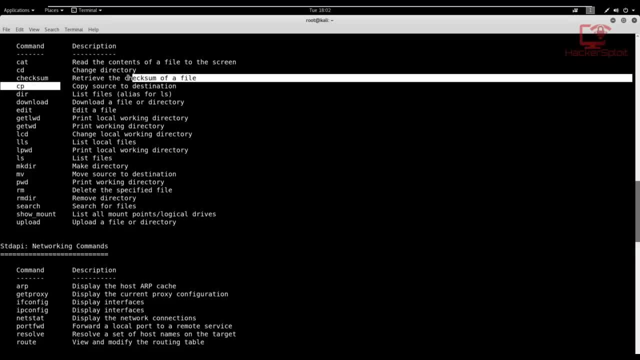 you have on Linux. you have your change directory retrieve. retrieve the checksum, copy all that good stuff. you then have upload, download and I'll show you how to use that. in a few seconds you have the move, the to delete. you can print the working directory. create a directory. 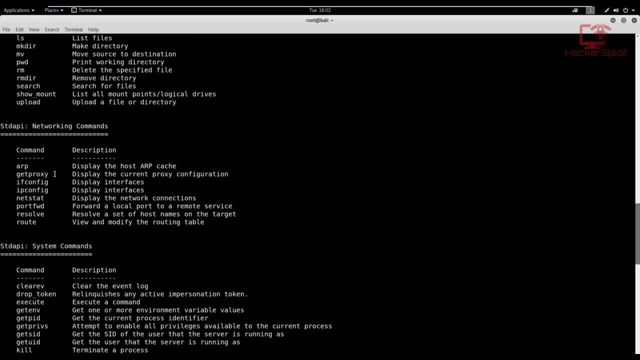 all that good stuff. They'll come in handy in a few seconds. All right. you then have networking commands where you can perform the ifconfig and ipconfig that. if you have a shell, I'll show you how to launch a shell. here you can display the host ARP cache. Let me just move on a bit quickly. 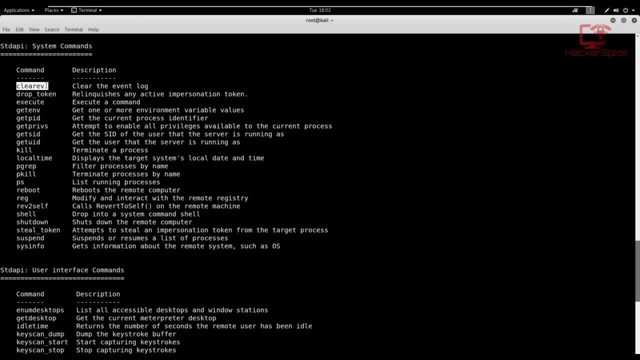 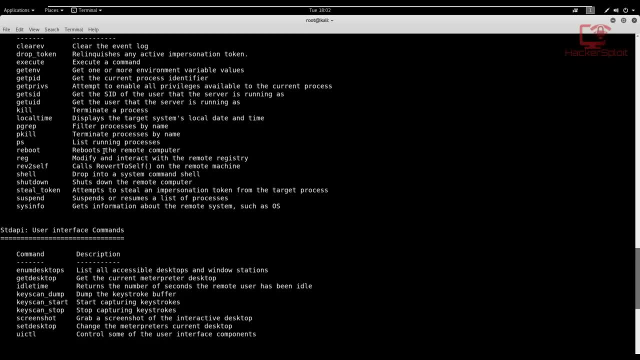 We have, then, the clear, the clear, the clear event log. this is very important for wiping your track screen. I'll show you that in a few seconds. All right, so let's get started Now. I've gone through this and you can go through it yourself. All the commands are listed out here. 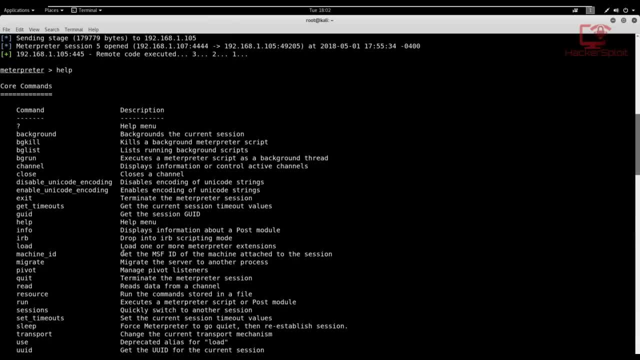 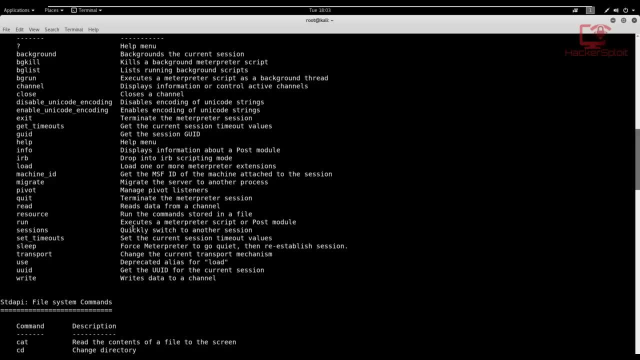 And it's quite simple. Now, one of the most important ones that you might be asking is, again, we are talking about privilege escalation. All right, and I think it will be better if I just show you how that works. I think that that would help a whole lot more, All right, 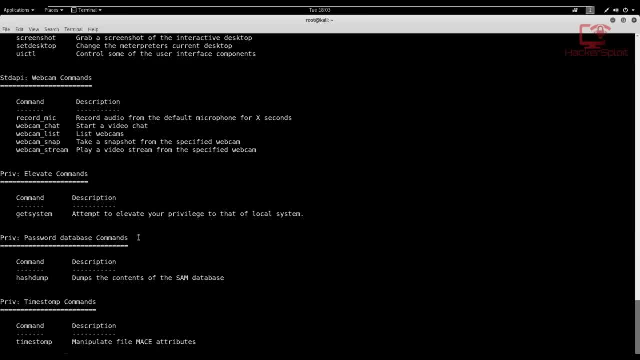 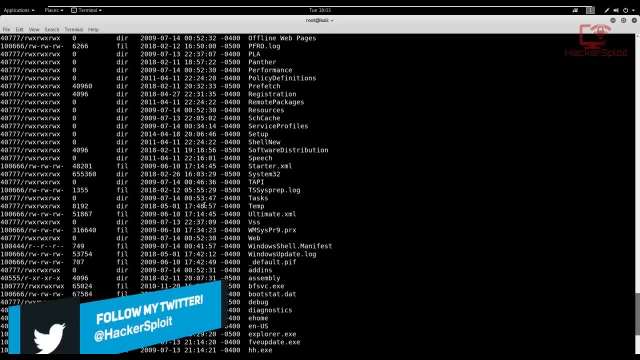 so let's get started Now with the first one and the most important one: changing directory. as you can see, I spoke a bit about that one right now And you can also list the current working directory And, as you can see, mine is in the system 32 folder. So if I just go back, 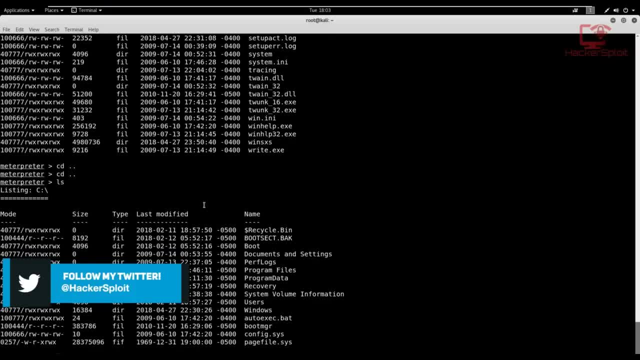 and back again. you can see, now I'm in the- I mean essentially the C drive- And, if I change my view, my working directory to users and to Alexis, or let me actually list and show you the users that I currently have there, as you can see. 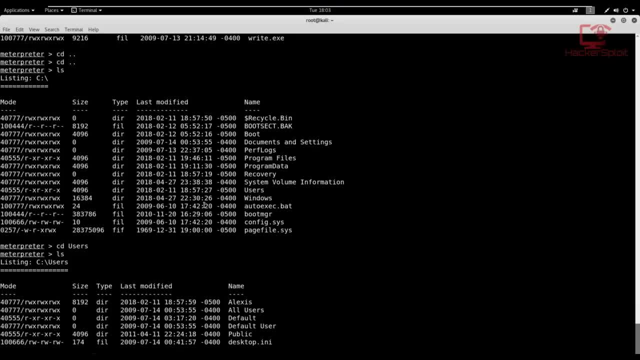 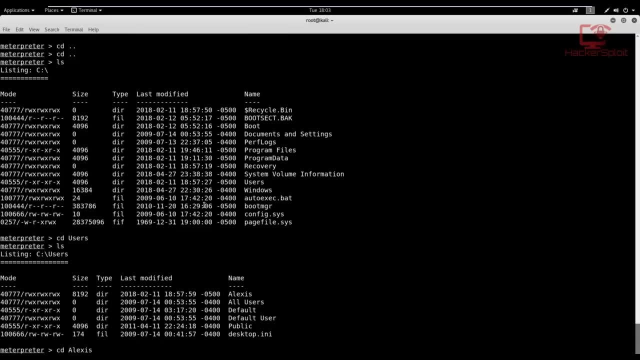 Alexis. so I'm just giving you an example of what you are- a hacker or the person who's exploit to the system might be doing. So you've gained access And now you're trying to see if you can download the entire. you're trying to see if you can download files that that target might be might. 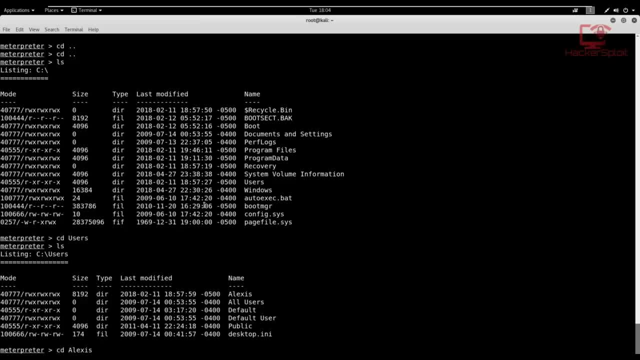 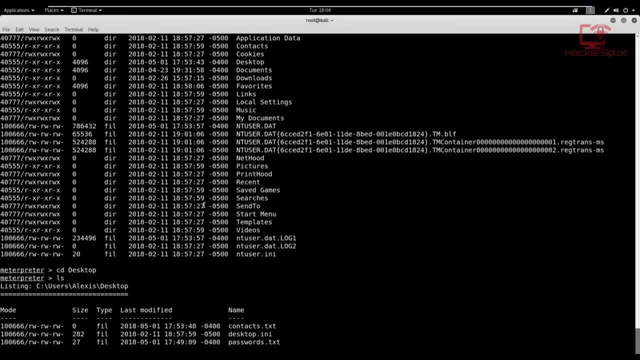 have or files that are potentially important, Alright. so if I list files here, let me go into my desktop, Alright, and if I list the files now, you can see we have. I've just created these two txt documents, or txt files. you have the contacts and passwords. So again, someone asked me: how would 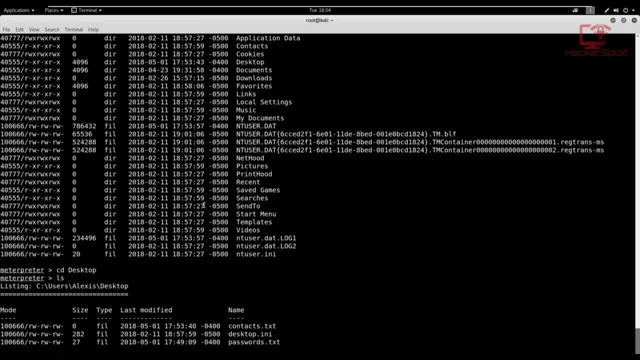 you go about downloading, because in the previous video it kind of failed on me And that's because I actually I went back a directory And you know I was talking about privilege escalation, But really if you're in the working directory, 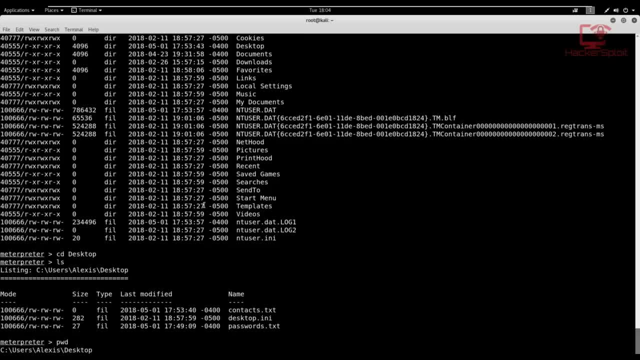 I'm going to go to the print working directory. if I perform the print working directory, you can see we are in C users, Alexis desktop. So that means I can essentially just download the files without specifying the location. Alright, so you might be asking: well, where will it save it on your local? 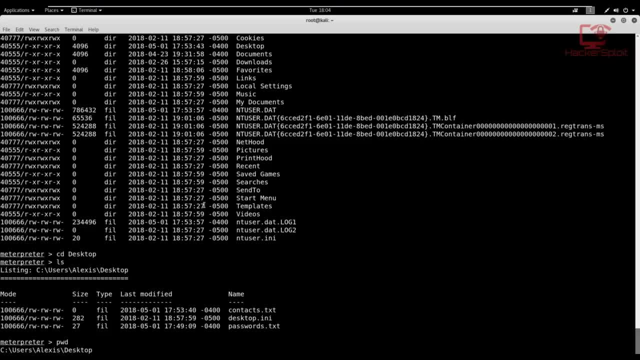 operating system. it will save it where you launched Metasploit and where you launched the meter present, the meter pretest session. So if you launch it in your desktop, it's going to save the files on your desktop. if you launched it in your home or root directory, which is what I've done, 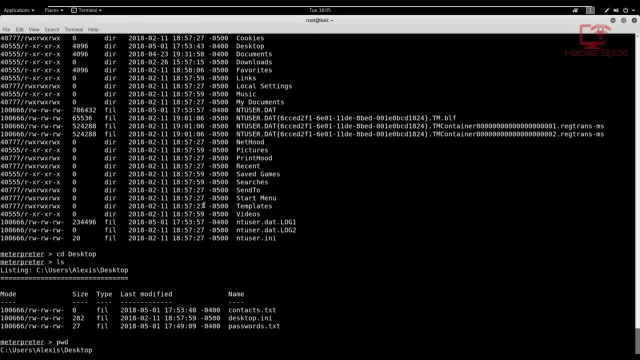 and what most of you will do. I'm going to save it there And I'll show you that in a few seconds. Alright, so let's say I wanted to download, I type in download and I just type in: let's see passwords. passwords: dot txt and hit. 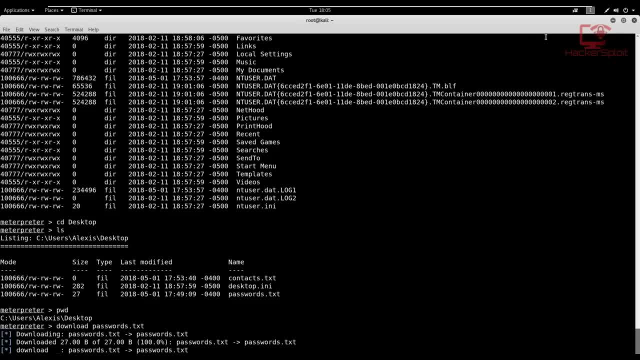 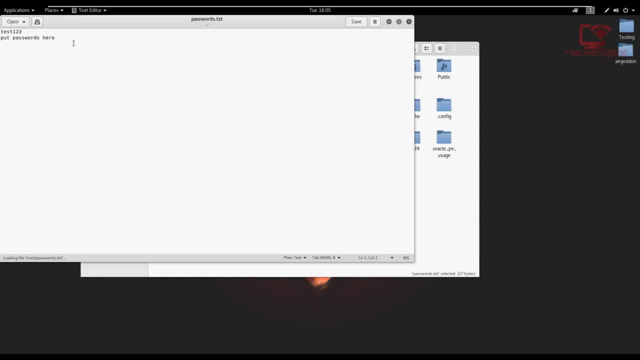 enter And, as you can see, passwords dot txt is done Alright. so you might be asking: can you show us proof that this actually exists? If I go into my home directory here you can see I have the password dot txt. And there we are, just put a few just random information there. test 123 put. 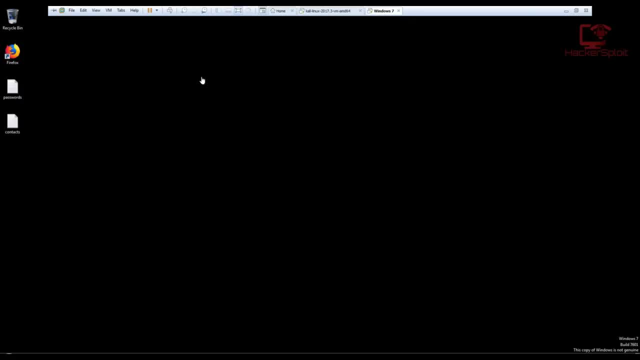 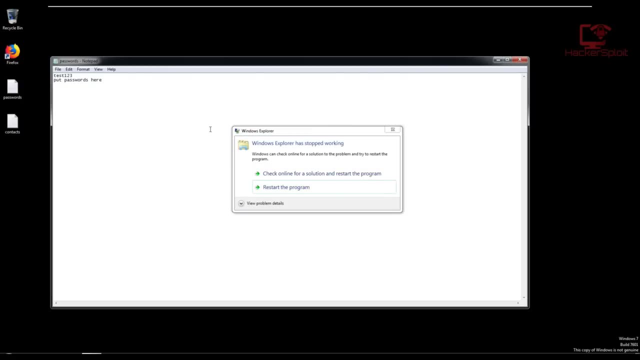 passwords here And you might be asking as well: how do I know that's the real file? I'll show you up There. we are test put passwords here And usually what happens is with this, with this exploit you can see, we got the Windows Explorer stopped working. this is to do with the double 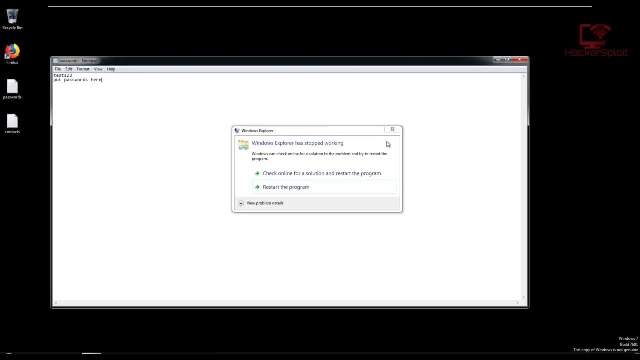 pulse exploit. if you try and inject the, if you try and inject the exploit in into the Windows Explorer, which is what I recommend, then usually on the client computer or the target operating system, they will be faced with this issue. But it doesn't matter whether they restart it. you will. 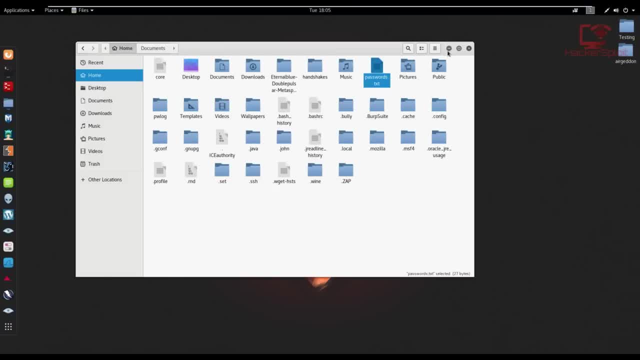 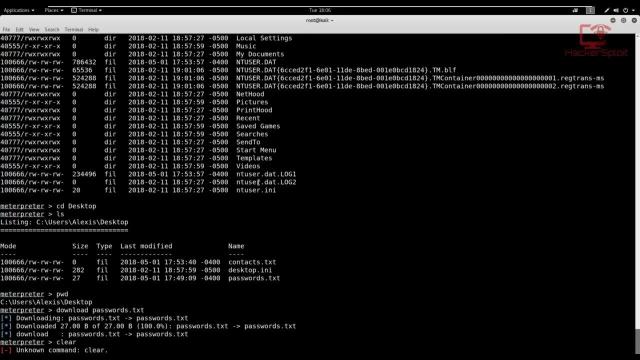 still have access using the meter pretest, Alright, so let's get back in Here and let's go back into my terminal And that's how to download a file, Alright, so whoops, sorry, Now let's look at at the other command. So we've talked about downloading files. we'll be 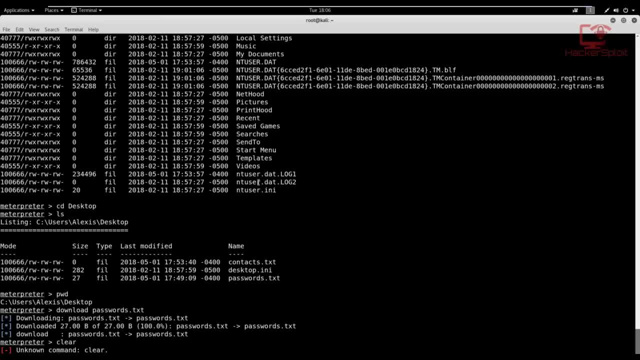 looking at clearing tracks at the very end of the video. Alright, that being said, let's look at some of the most important ones. We've talked about changing directory. you can also use the cat command, which I'm pretty sure you're familiar with. So cat, let's see cat passwords, dot txt. 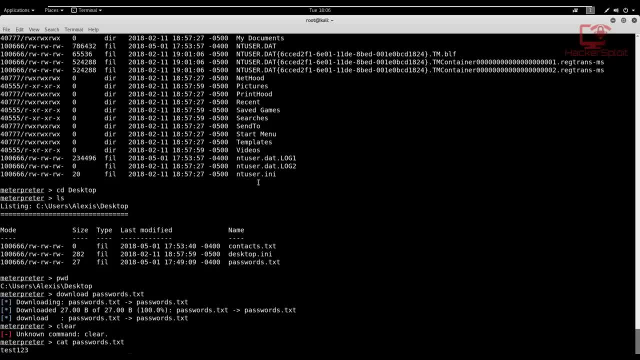 And I just hit enter and it's gone. You can see, it's just gonna display the information that is in that, in that file. Okay, you can then perform one of the also very important command, and that is to actually view what user you're currently. 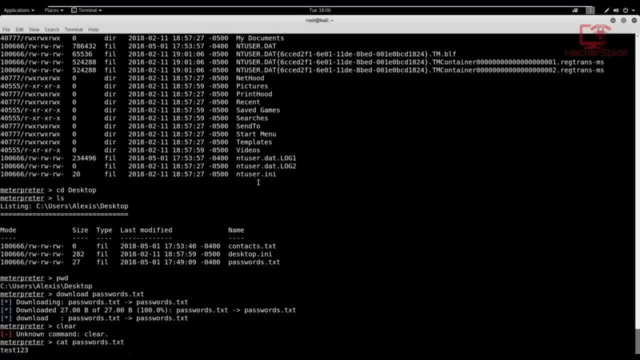 using. And you might be asking: Well, how is that important? Well, it's really very, very cool actually. So this is, I would say, a hybrid Windows slash, user slash, Linux command, And that is: get user ID books, get user ID. 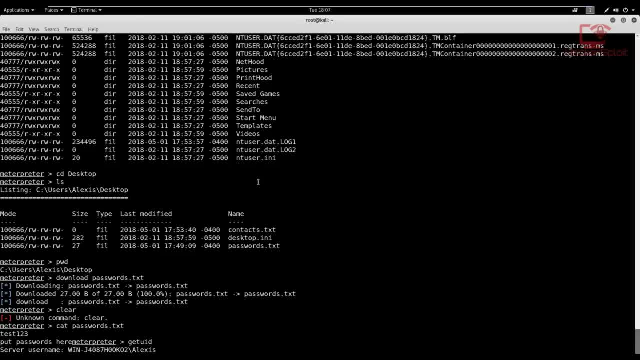 And I type that in. as you can see, you have the computer name and the username. the computer name is very important, As you can see. server username: that's what this computer is going to be called on your local network, if it's on the local network. If not, this can give you a good idea that you've 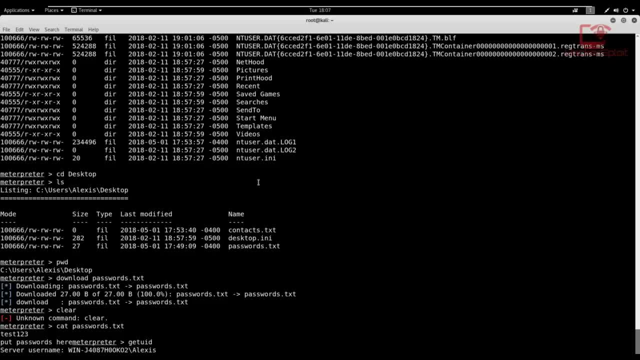 hacked into an organization and you want to know what exact computer I've hacked into. there you are. you have the name there, the system, server name, server username, the network ID. I'm pretty sure you know what that is if you've been using Windows for a long time. 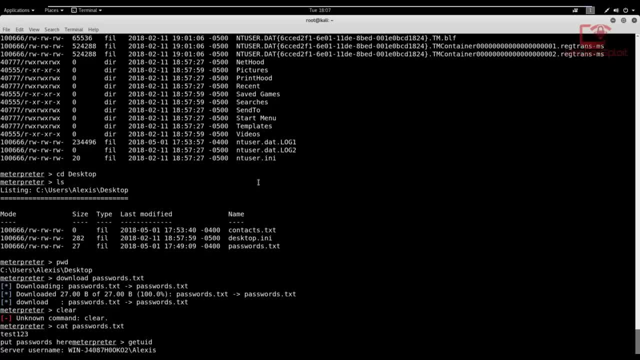 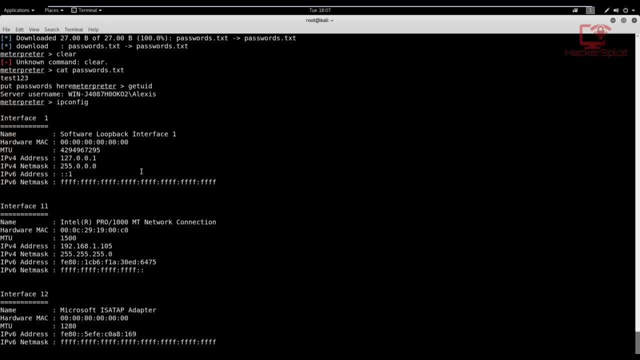 All right now looking at the other con, the other commands. if you wanted to know the local IP of of that computer, again, this would come in handy if you're in an organization type of situation. Alright, so if I type in, I have IP config. as you can see, here is going to start displaying the 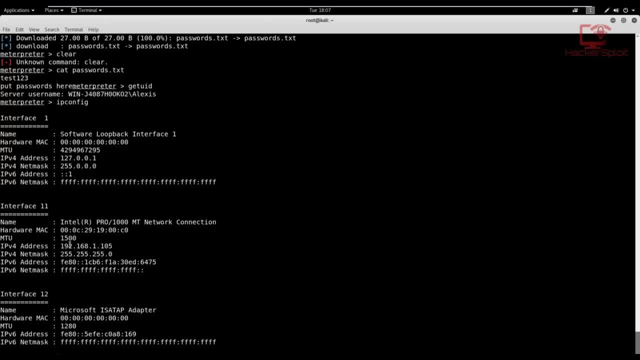 current connection, which is writing interface 11.. And you can go ahead and look at the IP address that it that has been assigned to it and the hardware, Mac, which in this case is the VMware. Mac VMware provides to us. Alright, so that's how to get network information. You can also use other. 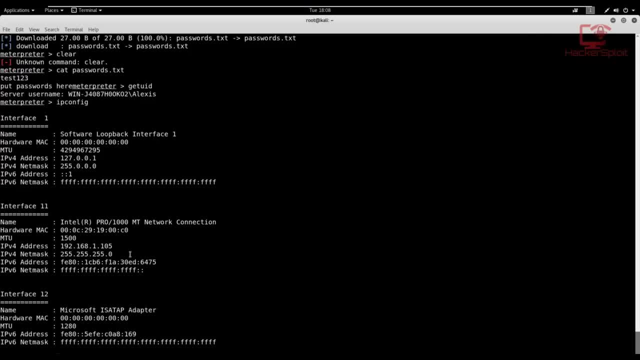 commands. Let's see what else we haven't talked about. the upload command: Yes, what if you wanted to upload a file, If you wanted to upload a file onto a current, into your current working directory that you currently have? So, for example, we can say: let's see, we are currently in the root. 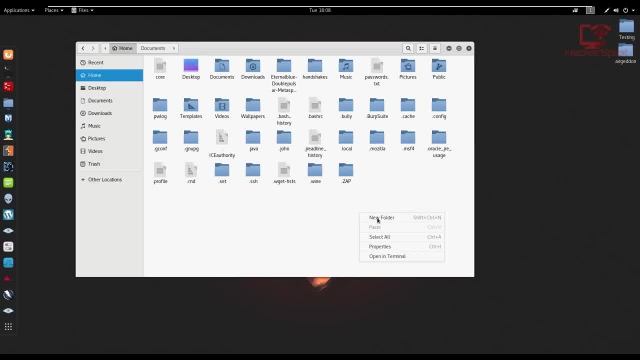 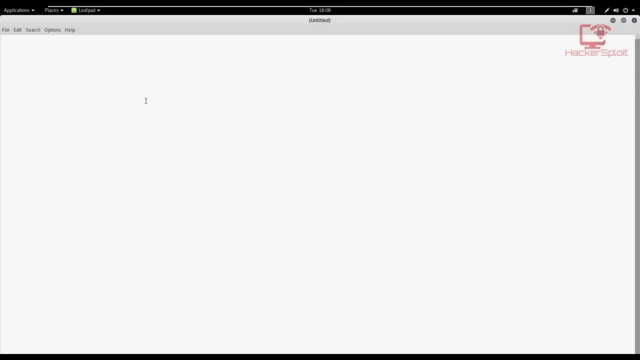 directory. So what if I was to just create also a simple text document? Let's see What I'm going to do is I'm just going to create a simple text document here on liftpad and just say information, and we'll just call this flag, flag one, Upload Alright, just to make sure. 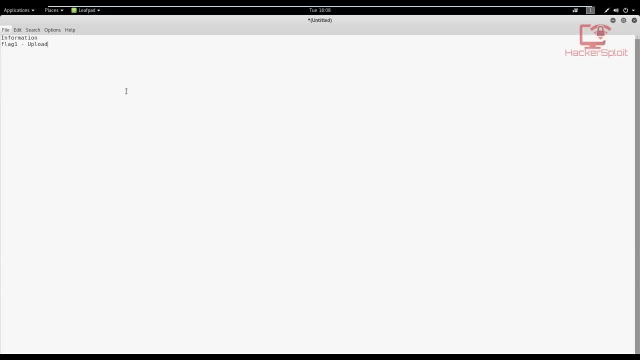 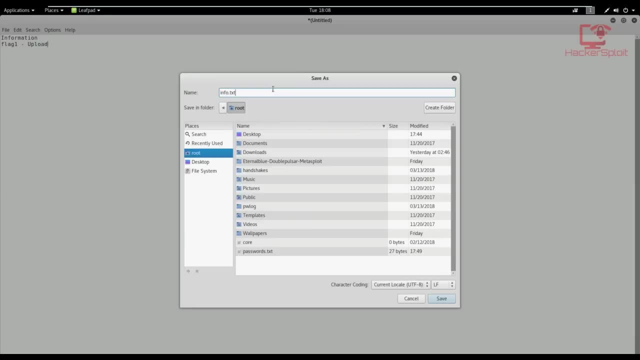 that we have got the correct file And I'll I'll save this as let's see route and I'll just call this info dot txt. So we want to upload this file And this can also come in handy if you're trying to upload a virus. 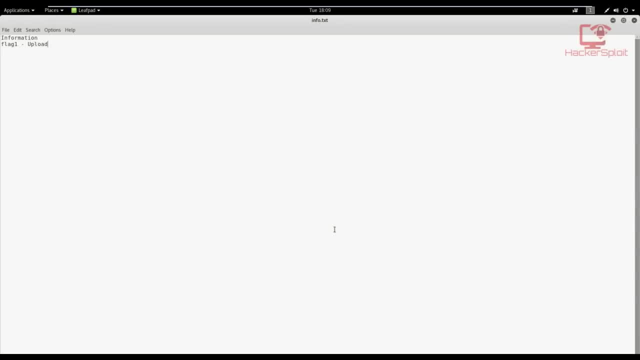 Or a Trojan, So, for example, you could be trying to upload an exploit- or a remote access tool, So you have backdoor access then, or a reverse PHP shell, But that really doesn't come in handy here. What I would recommend is a remote access tool. Alright, so what up? So we've actually created. 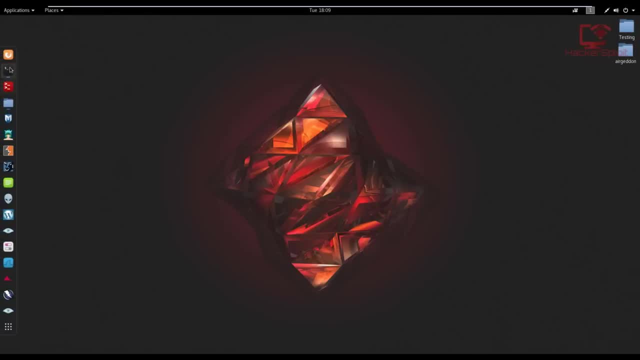 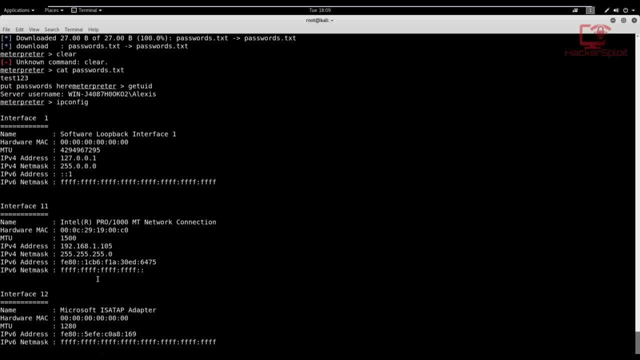 that file And, as you can see, it's info dot txt. So how do we go about uploading that file? Well, what we would do is we would say upload, upload, and we would specify the file info dot txt. And in its I was actually got confused. That's what I was getting confused in the previous video, is you? 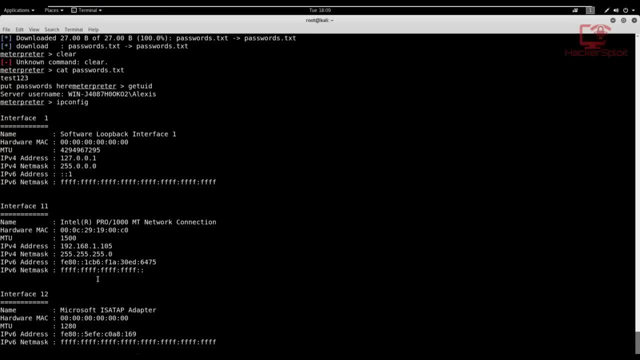 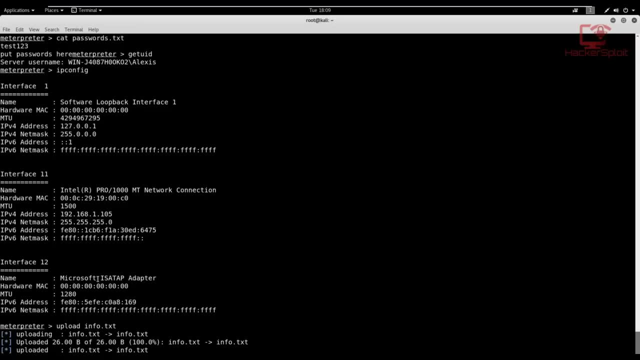 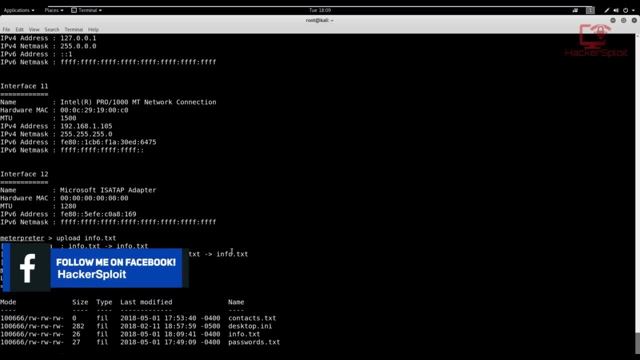 need to specify. So, for example, we could say, well, actually, let's see if it. if we can just upload it directly Now, that means it's uploaded it to our current working directory. So let's see if it exists. If I list the files in there, Yes, you can see. we have the info dot txt If you wanted. 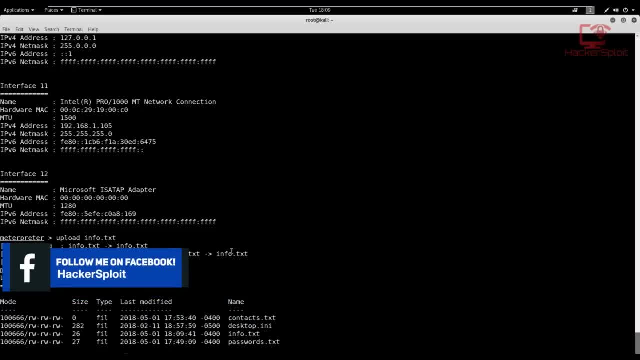 to specify the location. what you would do is you would use the C command and then you know you'd specify So, for example, Windows. you then specify like the system 32.. This is where I would go about hiding a remote access tool, Even if you've used value vision and you've evaded the antivirus software. 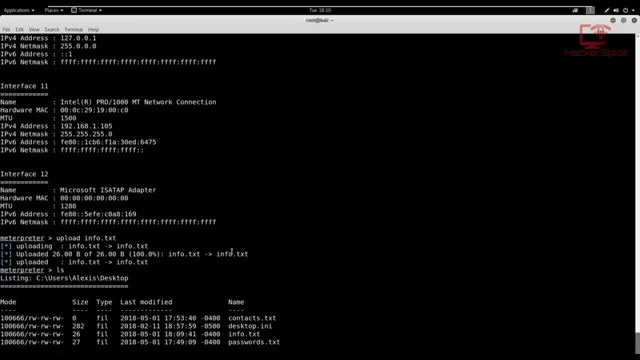 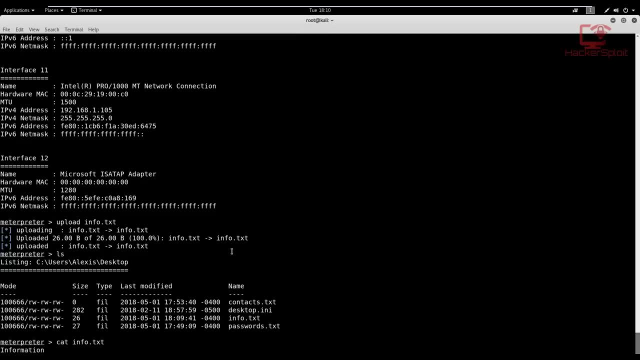 you get the idea Right. So that's how to upload files, really very simple. And if I just you know the info dot txt here, if I just catch that information, you can see we have flag one there. we are really really simple. Now in terms of the webcam commands. Now I cannot demonstrate. this because I'm not really a webcam. So I'm not really a webcam. So I'm not really a webcam. So I cannot demonstrate this because I'm not really a webcam. So I cannot demonstrate this because I'm not really a webcam. So I'm not really a webcam. So I cannot demonstrate this because I'm not really a webcam. So 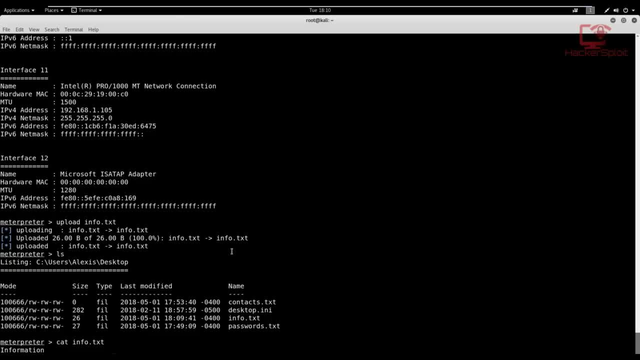 I'm not really a webcam, So I'm not really a webcam, So I'm not really a webcam fan. And the reason I even got a webcam was for YouTube. but I don't have it connected right now, So what you can do is the. 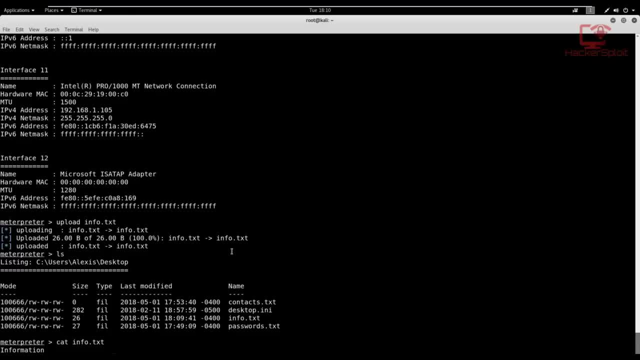 most important command to test first of all whether the computer actually has a webcam connected, is performed. the webcam, webcam command, webcam list- I think it's list. Yes, that will display the Yeah, there we are And that will show you whether the computer has any webcams installed. This is very 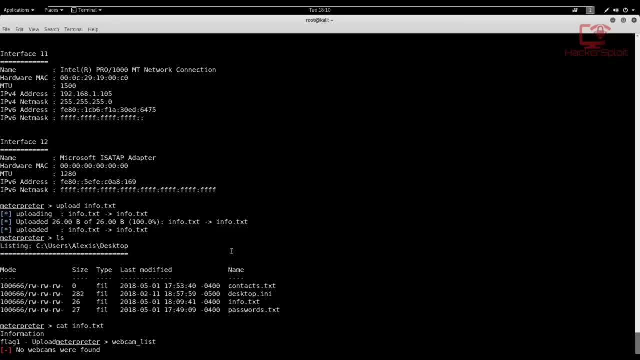 very important, especially if you have a laptop. if your target is a laptop, All right. you then have the webcam. you might be asking: how do you capture? How do you capture any images? Well, this comes in two, in two types of setting, into two types of configurations. the webcam snap command. 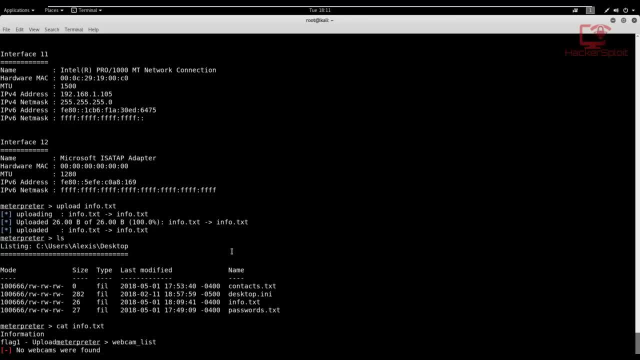 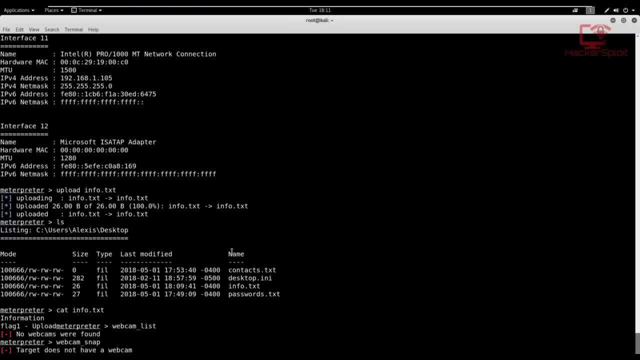 right. So this webcam snap: if I just type a webcam snap, it's going to tell me target does not have webcam. But if you want to view the help or the commands, you can also issue with this command or the parameters you can specify, Usually the webcam help. 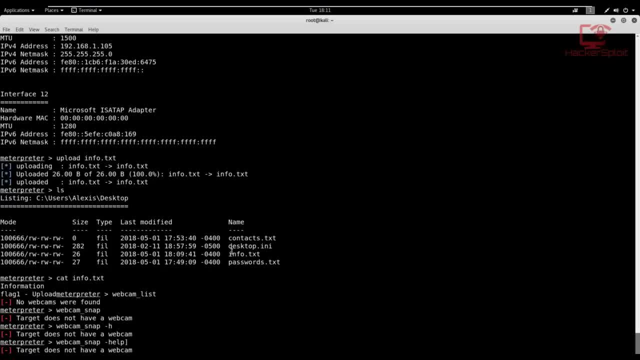 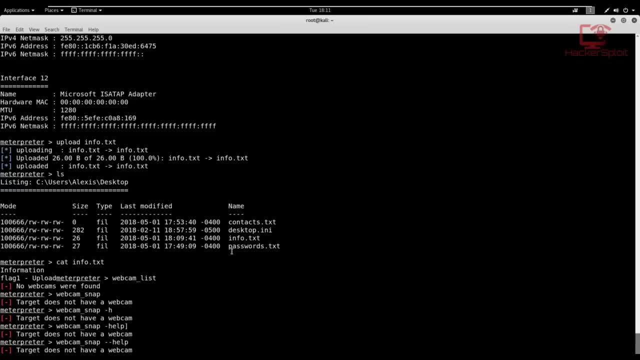 whoops, sorry my bad webcam snap help And yeah, okay, So if it does have a webcam, it will display the help menu which will show you. it will allow you to specify the resolution or the the quality of the image that you want to take, you want to snap Now. the other awesome thing is that 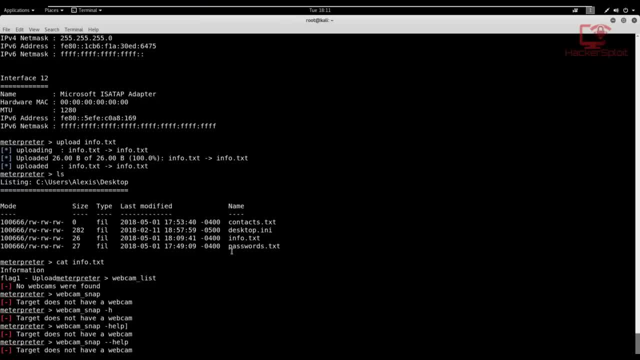 you can get the- let me just finish off with- with things like audio and video first, And then we can look at privilege escalation. I'm not, I actually don't remember. It's actually quite embarrassing. I don't remember how to how to use the microphone, But I'm guessing. 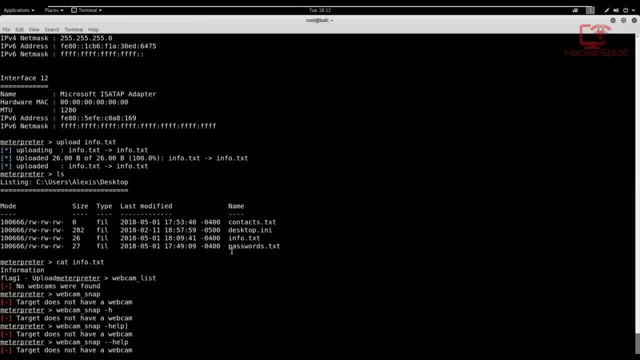 that that will not come in handy right now, Because if you're using a laptop, the microphone commands are really not that important. That being said, I'll actually look into it. I haven't touched on a microphone in a long time. Let's look at privilege escalation, All right, And this is 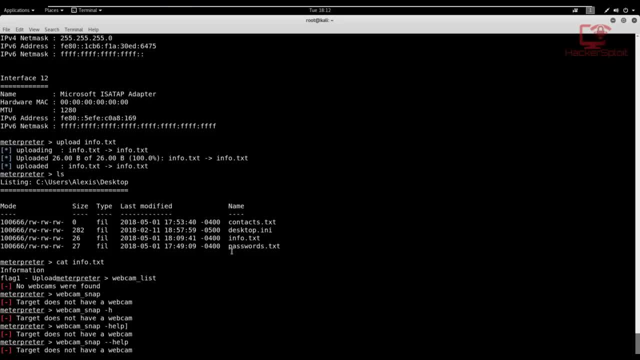 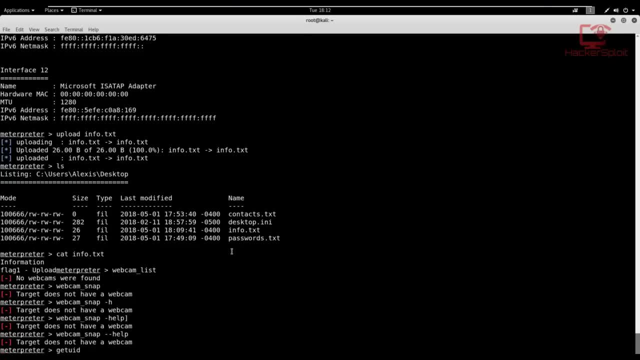 something that's also very, very important. Now, when I talk about privilege escalation, I'm just talking about giving yourself a better access. So, as you can see, get user ID. if I type that in, you can see I'm logged in as Alexis. Now, if I want privilege escalation, I want to be the 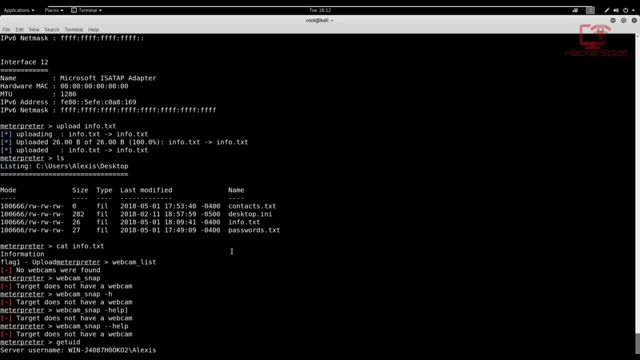 administrator. I won't administrate, administrate administrator access, sorry about that. that and that allows me to essentially just do whatever I want. That comes in two types of situations. So the first thing I could do, or I can do, is I can use the execute command and I 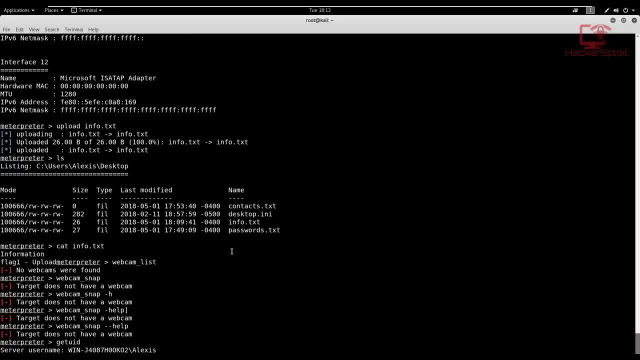 can execute the command prompt, All right, which will give me that, And of course I'm searching for the SCM alias is working, and then I'm equity flooding. And now I have- I have a route that I couldn't use- the Hallelujah requestercll command. 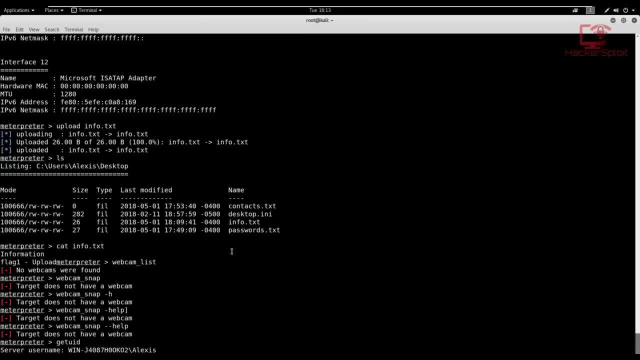 But I can figure out the route of that route and I also have asey yay, Screen red. So, yeah, that's all the documentation I'm about to teach you And that's really how you do it. Everyone knows that REST, but you can search what host is not existing. 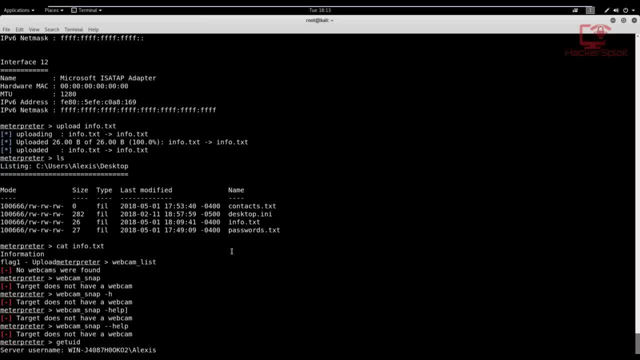 what's not from your server. All right, first of all can you" So when weremos on the first option- actually curse those assets. you can months on end, right, this is apart from goals. we're stains. So, first of all, we're so very so. 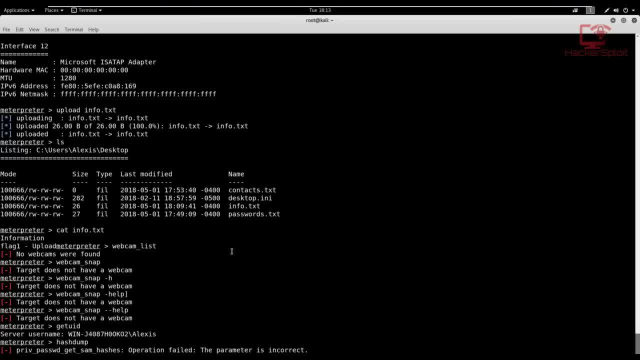 in hash dump And operation Well, password get. Yes, my bad, Sorry. What the hell am I doing? Usually have to specify the location, similar to what you have on Linux. So it's a run post, windows gather- Yes, it's in gather and obviously hash dump. Hopefully that gives us the hashes. 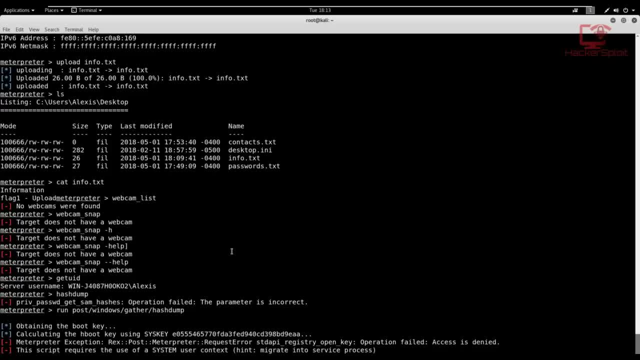 the password hashes. There we are obtaining boot key and meterpreter obtain access. Alright, so we have to escalate privileges, obviously, So we can just actually launch the shell here And now we have shell access here, as you can see, and then you can go ahead and perform the hash. 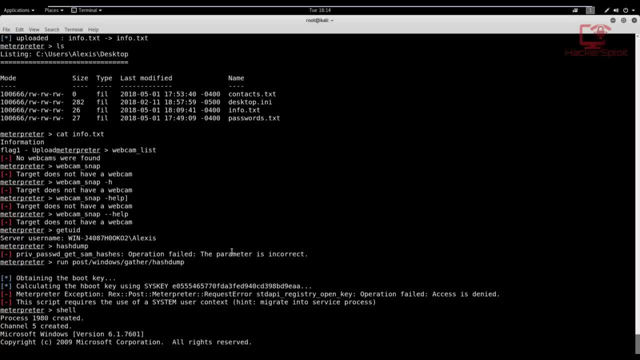 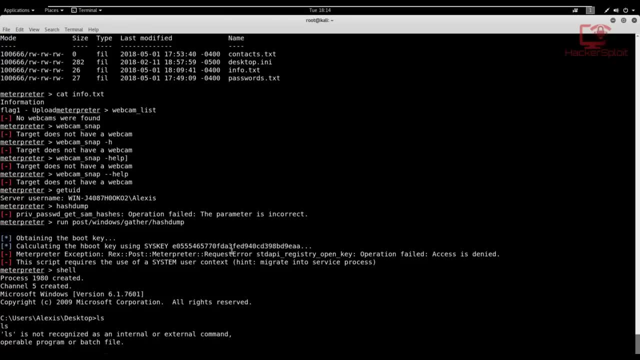 dump. But you need, you need a meterpreter instance And, as you can see, if you launch the shell, then you then have a command command prompt. So now I, as you can see, I need to press dir. This is, these are Windows commands, now native. 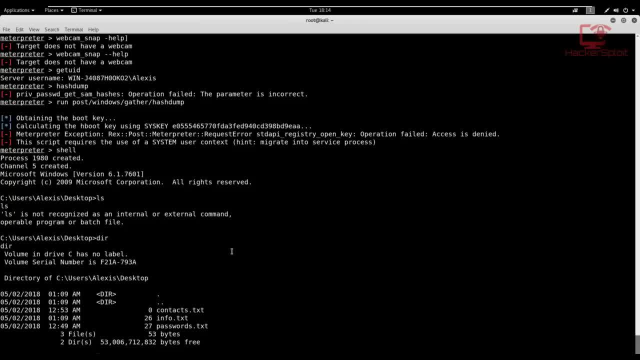 Windows commands. And there you are. that's how to gain access, not the computer, And then from then onwards, if you wanted to use the Windows commands, you can go ahead and use that. So I think I've pretty much covered all the important ones We've talked about upload, download listing. 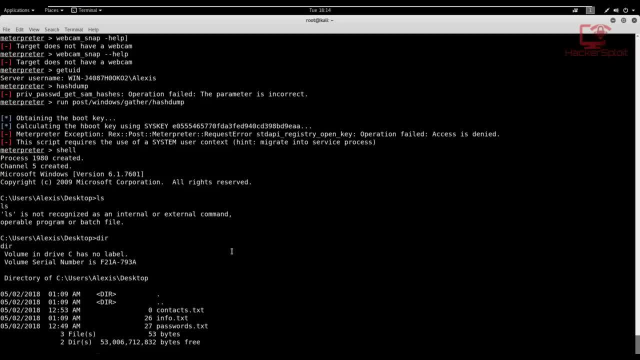 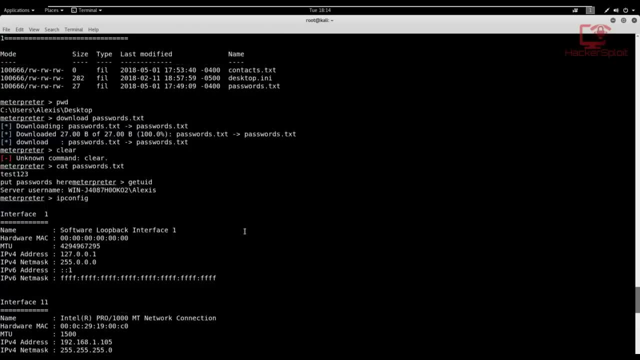 all the files using the shell, searching webcam commands. What else have we talked about? Let's see, we've talked about the shell. just now We talked about IP config, changing directory, uploading files and then specifying the directory. And yeah, that's pretty much all the important. 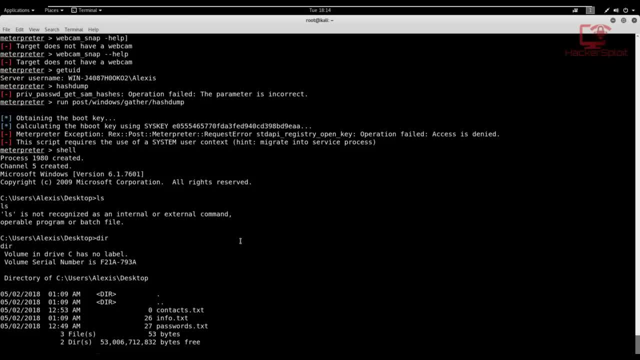 commands that you can use with meterpreter to obviously, oh, we forgot one, we forgot one. So I just want to talk about something really important here, All right Now. if, for example, we wanted to clear our tracks, we will go about this by using the clear, the clear track utility. 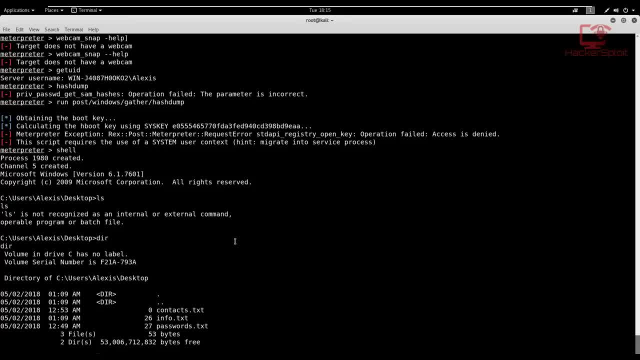 that comes with Windows And you might be asking: well, what the hell is this? If you've never heard about Google, I'll explain it to you in a few seconds. So if I just type in here in the Windows library, and I type in, as you can see, it's not going to give us access. That's because we don't. 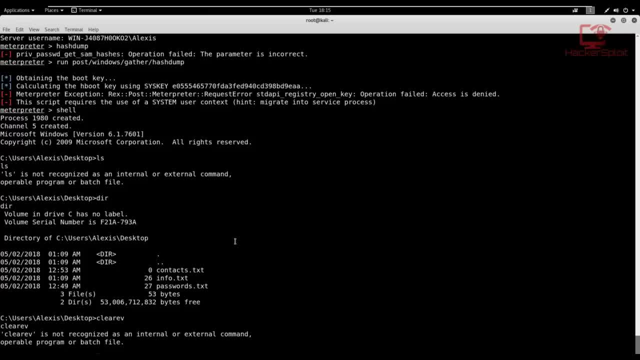 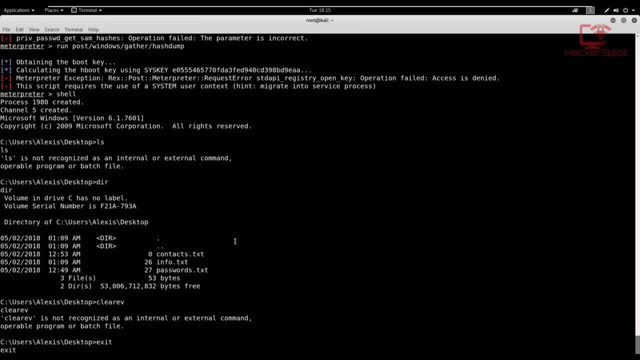 we are currently not using the meterpreter, And you might be a bit confused there. Well, essentially, what we would have to do now is we would have to exit the exploit, And now we are in the meterpreter. we've gone back a step. Okay, so now we would use the clear, clear EV. All right, 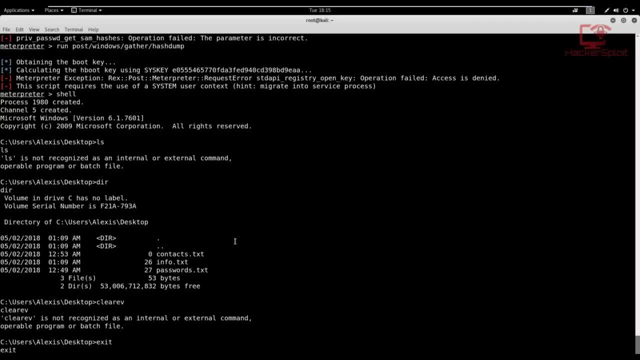 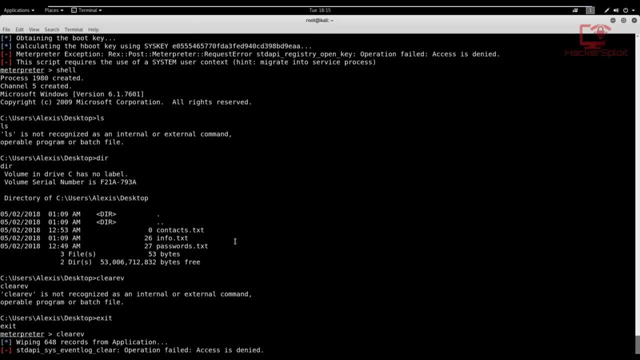 And essentially now, this will allow you to clear your logs, And if I just hit enter, it's going to show you here wiping, wiping, 648 records. So that's what we're going to do here, And then we're going to create records from application, And now you'd have to obtain a root access here or administrate. 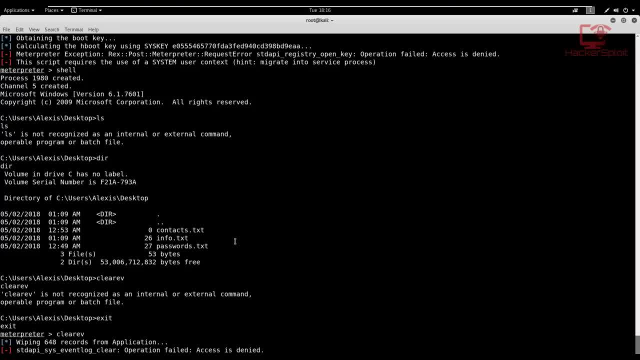 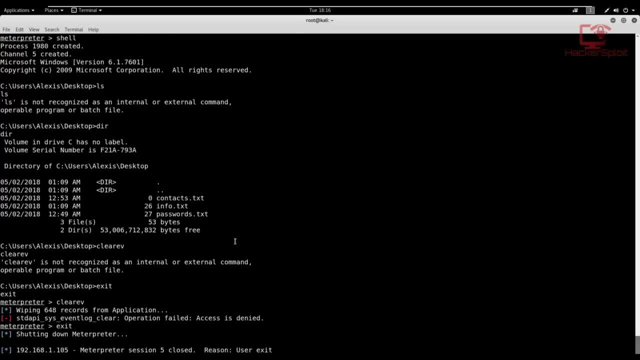 access And then you can. you can then go ahead and clear the other logs, which are the the system event logs, And once you've done that, then you can just hit exit And you're done with the exploit. you've cleared, you've cleared your tracks, you've uploaded a rat, whatever you wanted to. 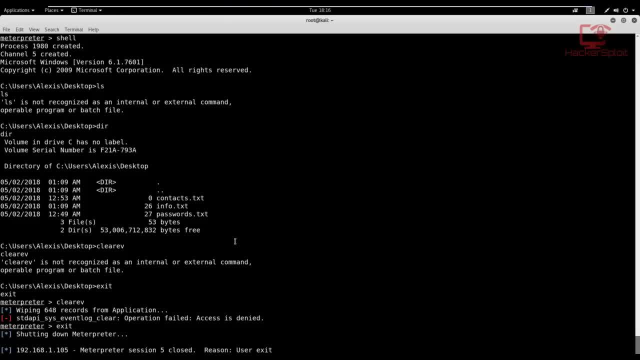 you've downloaded files, all that you've wanted to do, and you've cleared your tracks at the end and you've pretty much should. you should have performed whatever you wanted to do- post exploitation privilege escalation- uploaded the files, downloaded whatever you want. 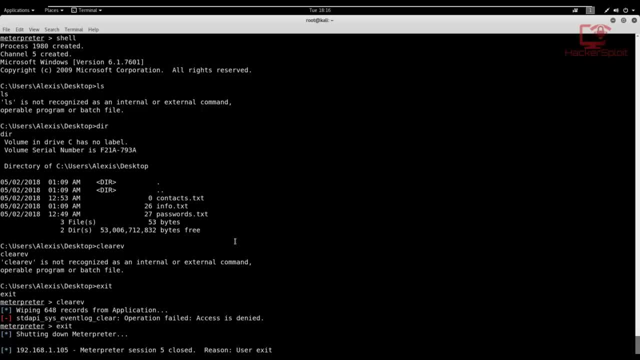 and then you've cleared your tracks and you're done, And that's the trademark of a successful hacking or exploitation. And I think I've covered a lot about exploitation And now I want to cover more about maintaining access. you know stuff like that And we'll be looking that at that. 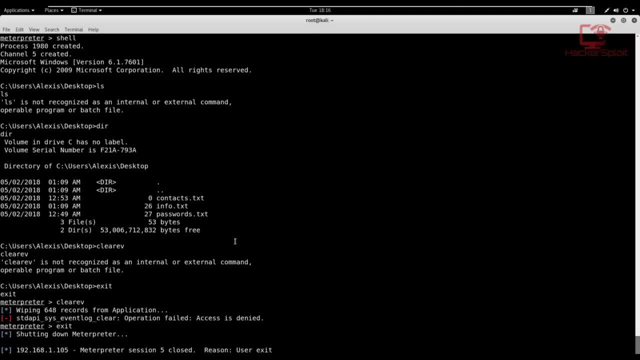 when we talk about- you know things like these- the CTF challenges, and we'll be talking about hack the box. I'm actually creating a series on that. will be going through all of them, actually went through a lot of them, And I've 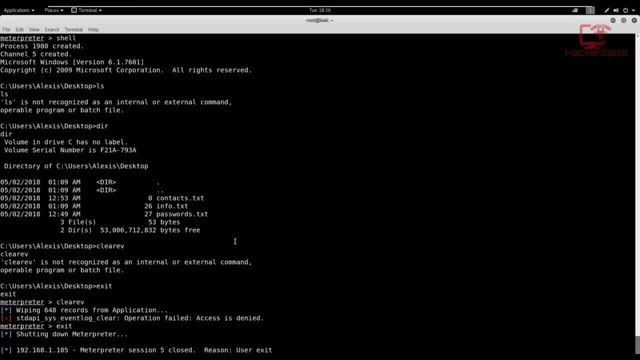 remembered. it's actually quite easy to be honest. the starter ones I'm not going to show off here. That being said, the web application penetration testing series is also going to be continuing. As I said, I'm feeling much better now, So uploads will be regular on a daily basis. 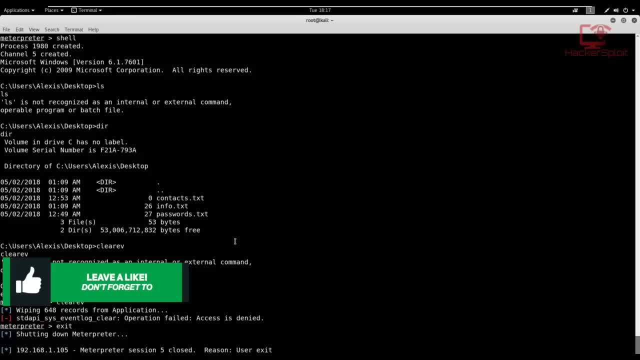 And I'll be focusing on your video ideas, the series that we currently have running and the SS seven video, which is which is due, and it's going to be coming as soon as I get my legal, the legal requirements and satisfy them, And I'm pretty sure not a lot of you actually knew that. 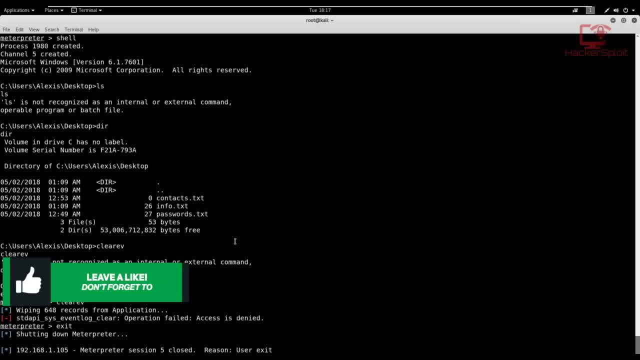 And I didn't know that That actually needed permission to demonstrate such an attack on a mass, on a mass on a system that is used, you know for, for mass service. I'll explain that later. But, that being said, hope you enjoyed this video. if on value in the, if you did, please leave a like down below If you. 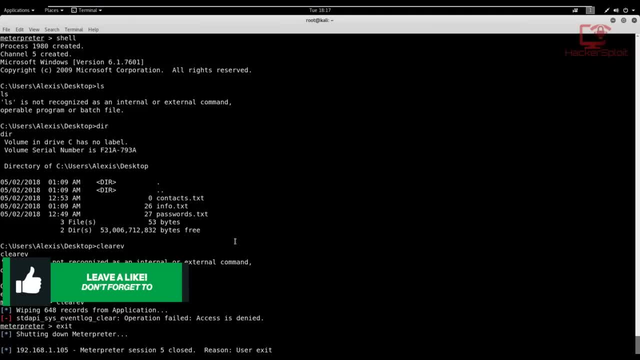 have any questions or suggestions, let me know in the comment section or on my social networks, or you can hit me up on my website and I'll be I'll be sure or happy to answer your question. That being said, guys, have a good day. 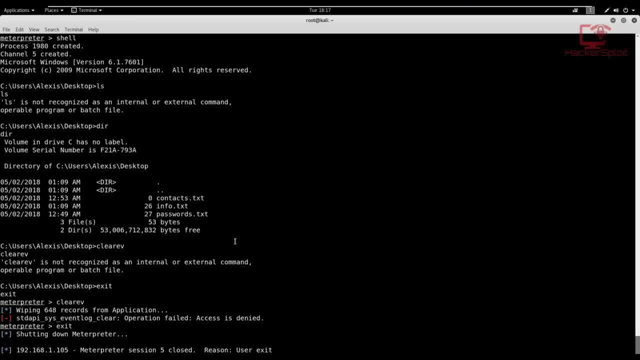 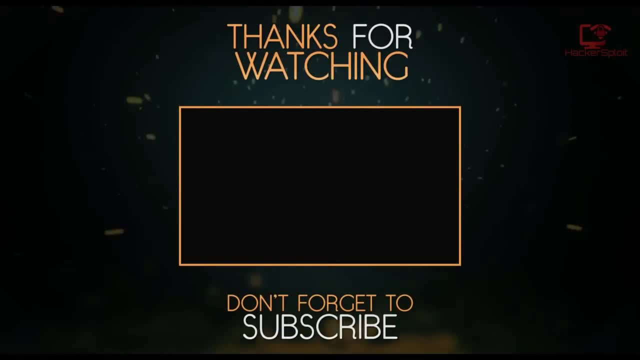 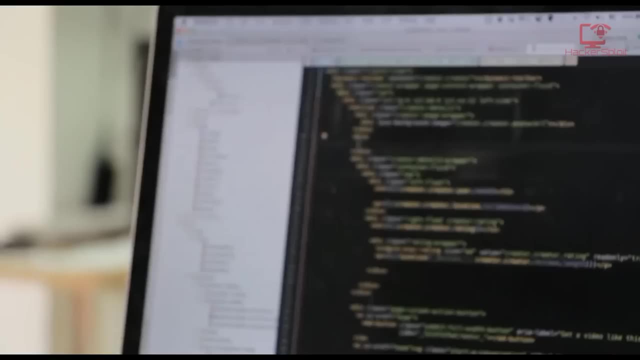 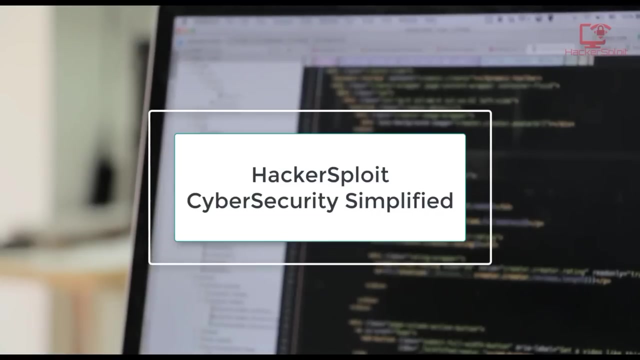 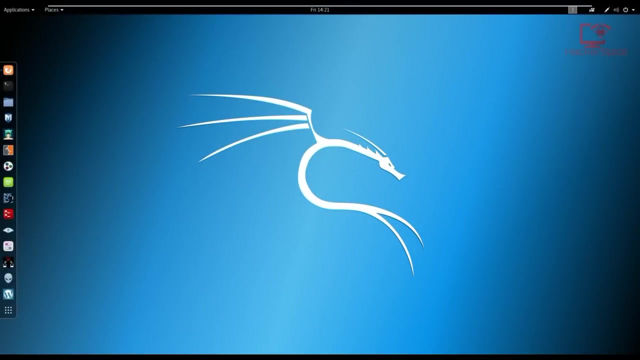 Have a fantastic day and I'll be seeing you in the next video, Peace. We're going to be looking at how to generate a backdoor, or a PHP backdoor, with Weavley. All right, so you might have heard of Weavley or you might not have heard of Weavley, And essentially what? 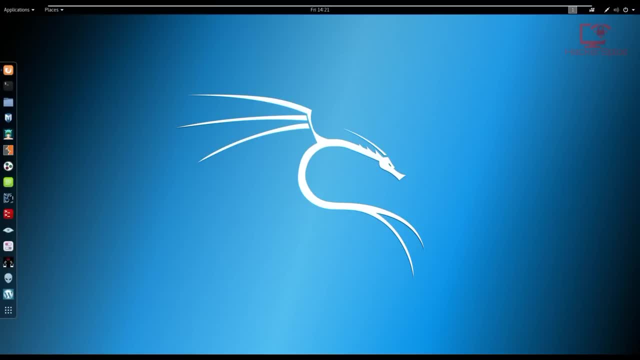 Weavley is. it is a PHP shell that will give you a connection like SSH, so that you know you can execute system commands, And it essentially gives you backdoor access to the server that or you know, the, the target that you have hacked. All right, so it comes pre installed with Kali Linux and. 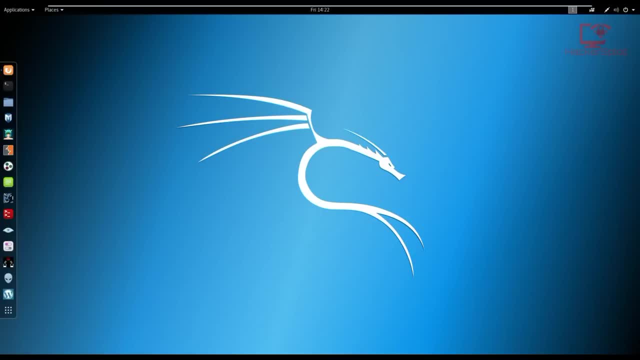 para toast, So you're pretty much good to go. You can find it in GitHub. it's very, very easily. just search for it on GitHub. it's Weavley w, double e, v, l, v l y okay. So it offers a lot of a lot of post exploitation. you know advantages. 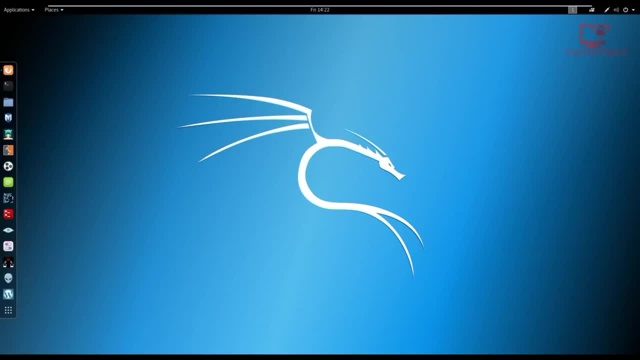 in the sense that you can, you can spawn reverse shells, you can execute commands And you know that is pretty much all you're going to need. once you, once you've exploited a server, you know you want to leave, you want to maintain access in that server whenever you like, And Weavley is fantastic, It's. 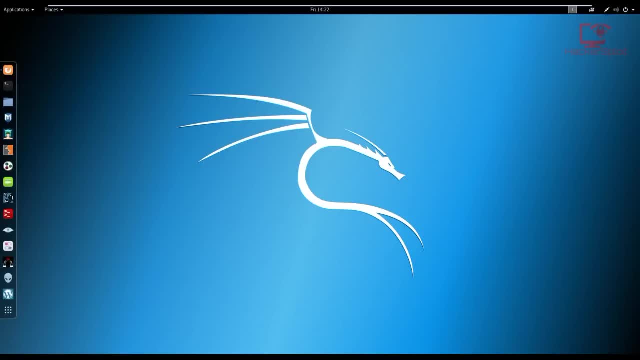 actually really, really powerful. Now I know I actually mentioned on the community section that I'll be making a video on Nikto and and you know, things like the Medusa or or the other web vulnerability scanners, But actually I'm going to be working on an entire new series for that. 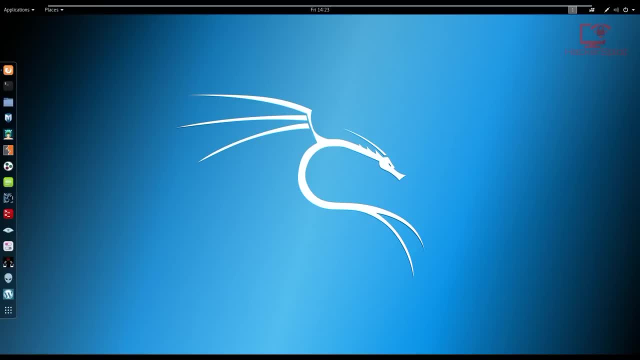 because it is a large topic And I don't think that I can cover it. you know, I can give it its full, its maximum potential, few set of videos, So I'll be working on a large project for that. So, as we did, 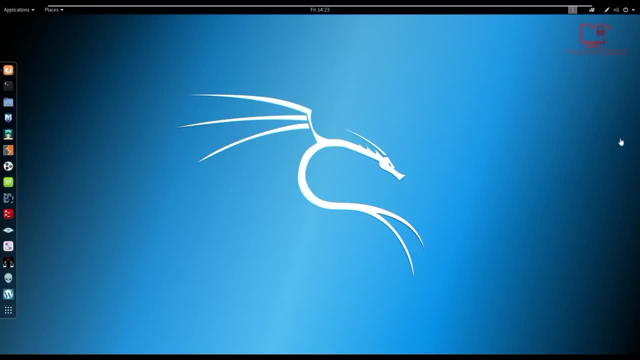 in the previous video, when we were hacking WordPress, we managed to brute force the WordPress installation. we got the username and password. so we have got, we have. we have successfully exploited the system. Now we need to maintain access. So it's getting a little more interesting. 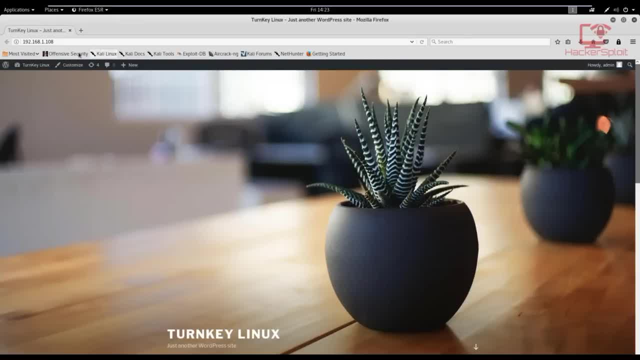 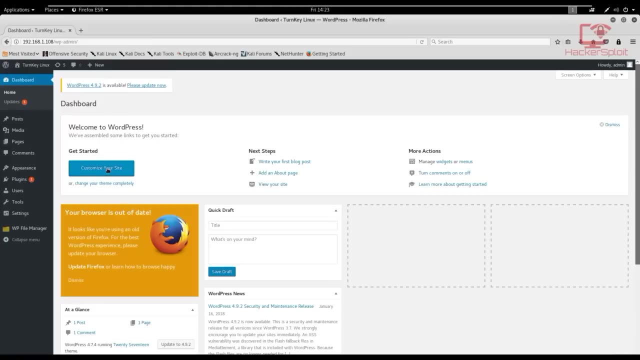 So I already have the WordPress server running and I already know the password, So I'm just gonna go to the. there It's already loaded up, So I'm just going to log in now. Oh, it's actually logged in already, So I can just go to WordPress adminphp, like so, And there we are. All right, So we're already logged in. And now, as I said, you know, we can upload a PHP file that if we redirect to- and we obviously know the name of the PHP file- if we upload it to the local directory, it means that the web page will process your request and it will return that. 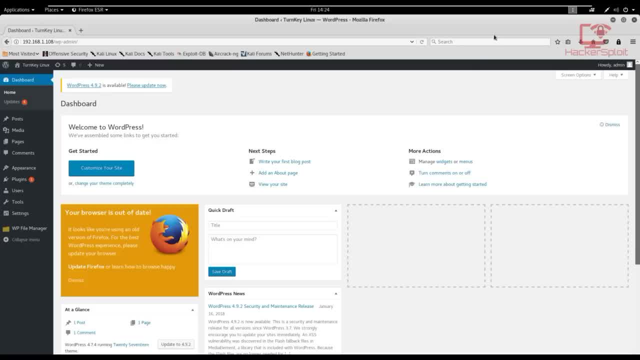 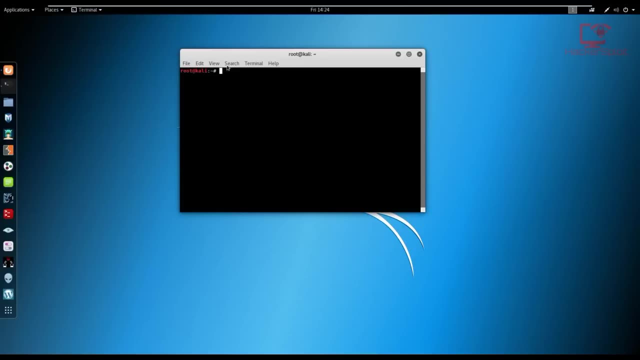 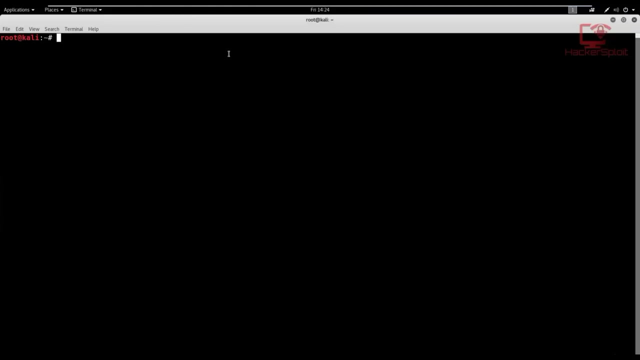 And then you can, you can connect to the, to the, to the shell that you've uploaded, which, in this case, will be generating with Weebly. All right, So you know, generating a PHP shell with Weebly is really really easy, And we're going to be looking at that right now. So just open up your terminal, Right, And I'm just going to zoom in so we can see what's going on. All right, Awesome, Let's get started. So the syntax is really really simple. 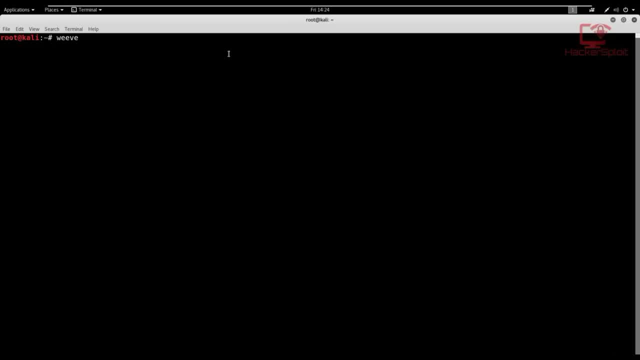 So Weebly, Whoops, So it's Weebly, So it's pretty much as simple as that: W-E-E-V-E-L-Y. Okay, so, Weebly, And then we want to use generate, Right, So we're telling Weebly to generate, So it already knows that we're telling you to generate a PHP shell, So it's going to now that the next piece of information you need to enter is the password for the shell. All right, This is very important so that only you have connection and only you are able to generate a PHP shell. 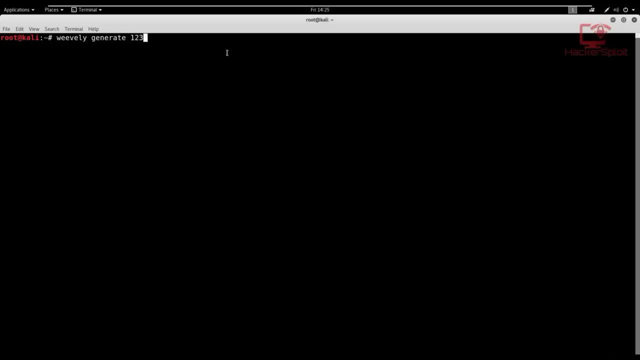 So let's continue writing on this one, All right. So Weebly is connecting to a 그리고 and it is then going to generate the password for the shell. So we're going to need to use this backdoor, Right? so I'm just going to use a simple password like 12345.. You know something really, really simple, because I don't want to use anything complex. Now I'm going to store the PHP file on my desktop, All right. So you, I'm just going to specify the location, I want to store it into a root desktop And I'm going to give it a name. So I'm just going to give it a name. Now, this is where social engineering comes into play. Now, obviously, most of you know we're talking generally speaking, and I know I'm doing this on my lab, But in fact, I'm going to write a general code here. I'm not going to write a name, So I'm going to put a command here. I'm going to write a command code. 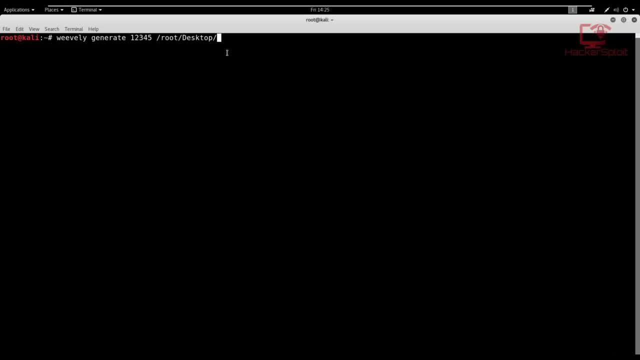 in reality. now, web servers are probably going to be monitored by the, you know, by security teams, and they're going to be snooping around for you know, weird, weird files with weird naming. So if you name it backdoor, you know you're just looking for trouble And that can you know. 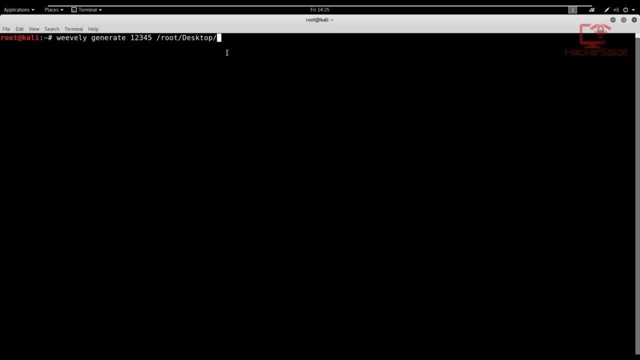 that that can expose you really really badly. And you know I'm talking, I know I'm talking from a black hats perspective, but I'm just giving you an idea of how you know how these things are thought through. So what I would do is I would name it something like: let's see something. 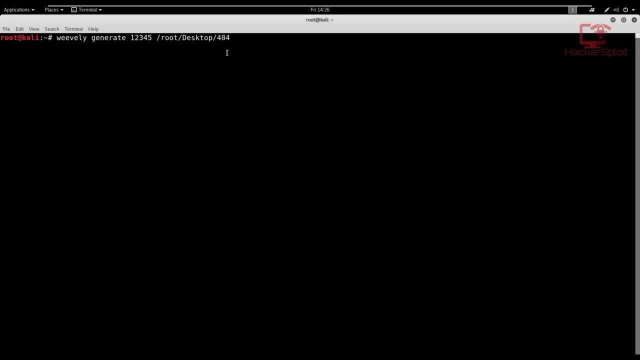 interesting, like, as you saw in the previous video, a four, four redirect. all right, so four, four dot PHP. right, that is the extension that we're going to use. So now, if, when I hit enter, it's going to generate it. There we are: generated backdoor with password 12345 in root. 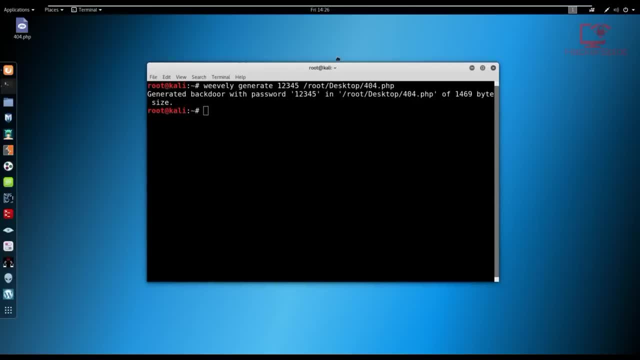 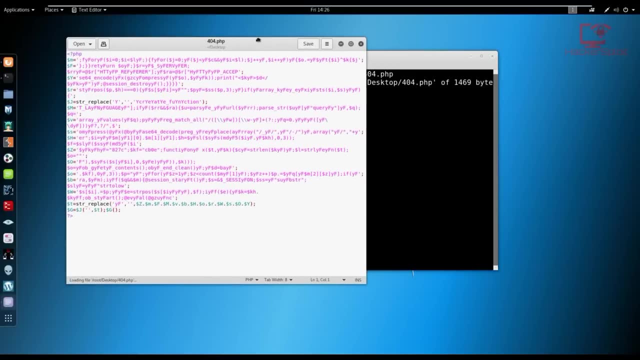 desktop and it's 1469 bytes in terms of its size. And here it is. So it's a PHP file. if you open it up, everything's encoded. So it's you know. if anyone found it, it would be a matter of of you know, reverse engineering it. Alright, so we need to upload. 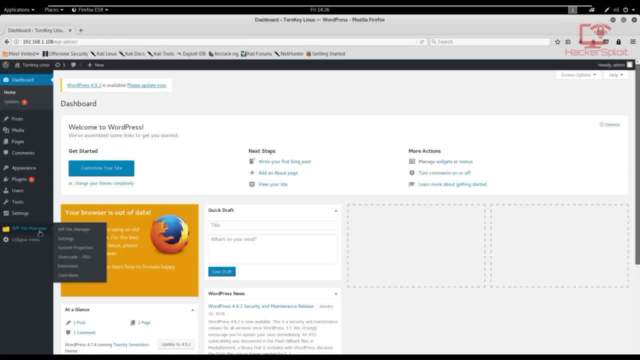 this to the server And luckily for us we have the file manager installed on WordPress And you know it's really really simple to do this And obviously if you crack the FTP protocol you can also upload it like that. So one would go to the WordPress file manager and you need to. 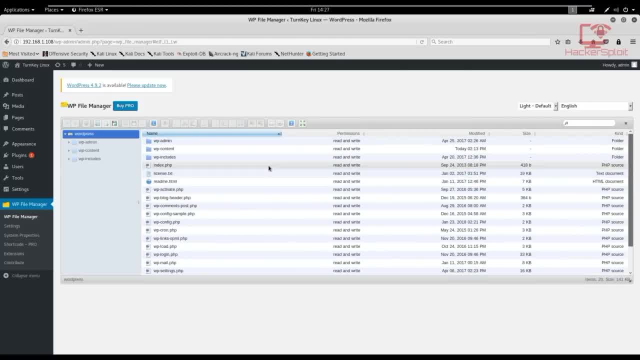 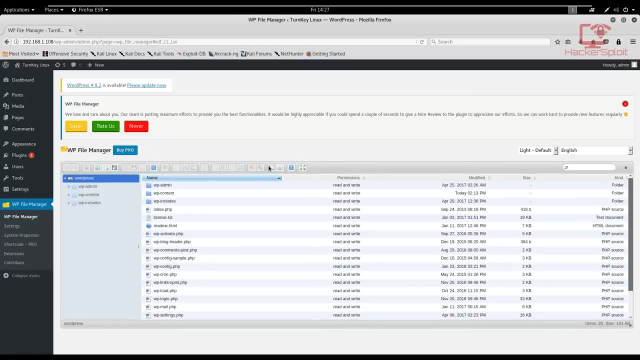 upload it to the root directory. Otherwise, you have to upload it to the root directory And you have to, you know, go through subdomains, which is also a great idea. if you upload it, you know, in with the image specification and use image upload vulnerabilities, you know. 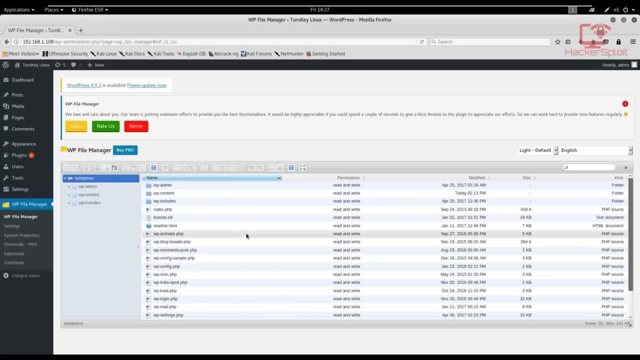 that's basic web penetration testing. But for this we're just going to keep it simple. you know, I'm just going to right click and I'm going to- whoops, it's not allowing me to upload the upload files And I'm going to select the file which is on my desktop. there are four, four dot. 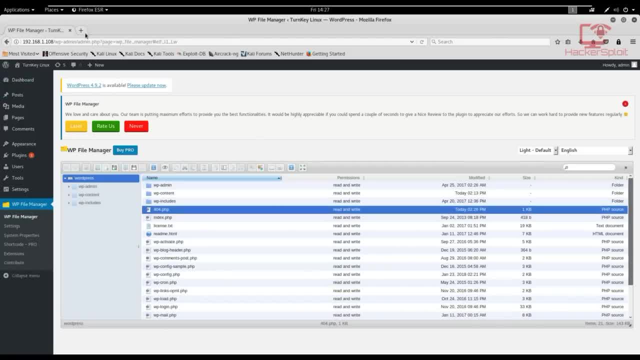 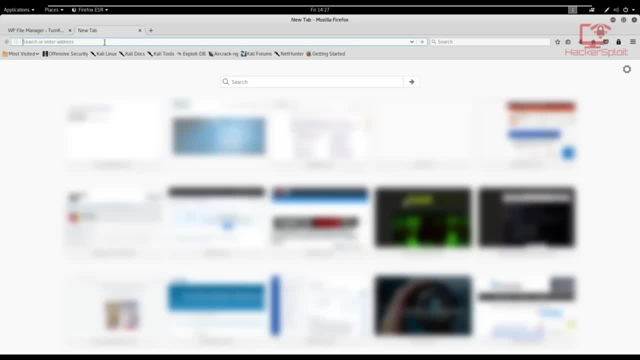 PHP and it's already uploaded. And now you know, usually if I hit an unknown web page, it would reply with something that is completely vague, right? So what I'll do now is I will, just I will enter the address. So 192.1168.1.108 and 404 dot. 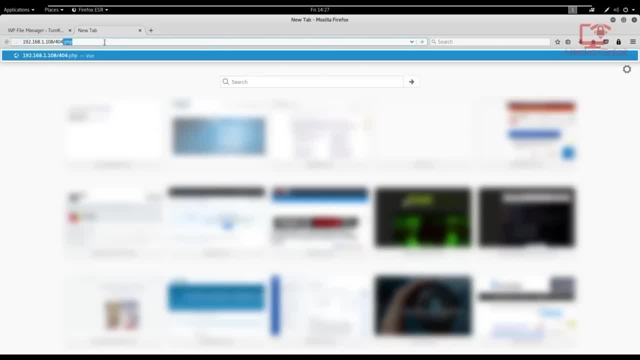 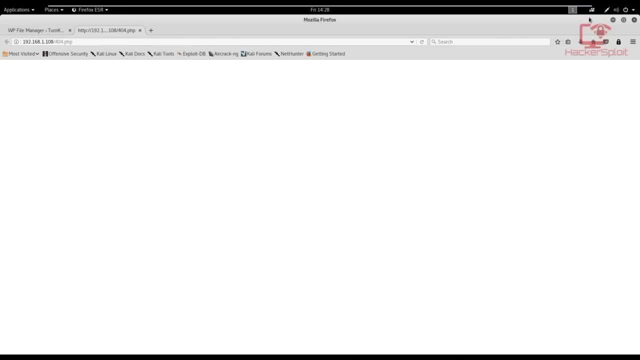 PHP because it's uploaded locally to the you know local directory. So I'm just going to hit Enter And there you are. Now. this is a good sign. if it doesn't give you any result, it means that the script is already active. Now you might be wondering: well, what do we do now? How do we do this? 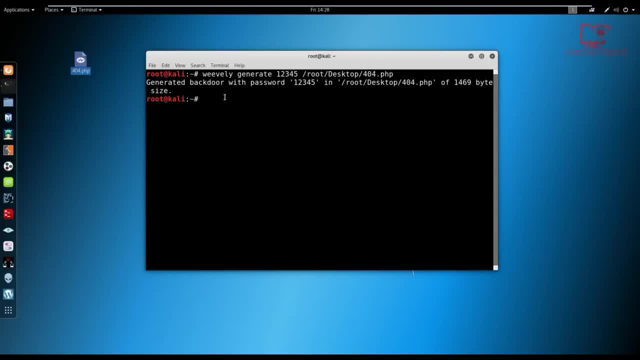 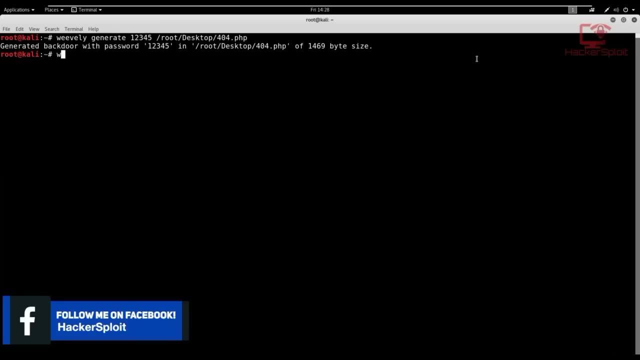 Well, we connect to it the using Weevely- Alright, so let's get started with that right now. Alright, so what are you going to do is really really very simple. We're just going to use Weevely- Weevely as the command, obviously, And now we need to connect to it, So we're going to 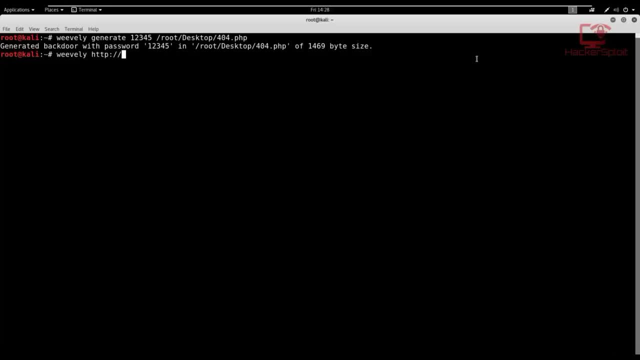 specify the web page, So HTTP. we have to use the protocol, So 192, point 168, point 1.108.. And we're connecting to that script or that shell, So 404, whoops dot PHP. and then we specify the. 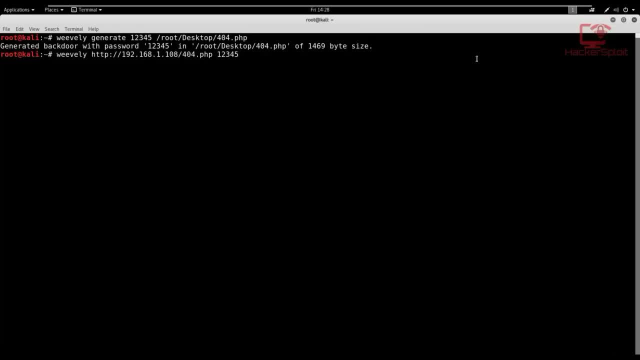 password, which in this case was 12345.. And it should exploit it immediately or give us back door access. So I'm just gonna hit enter And there we are, And now we can execute commands. Awesome man, This is so cool. So if I hit LS, you can see we can access all the files that exist on. 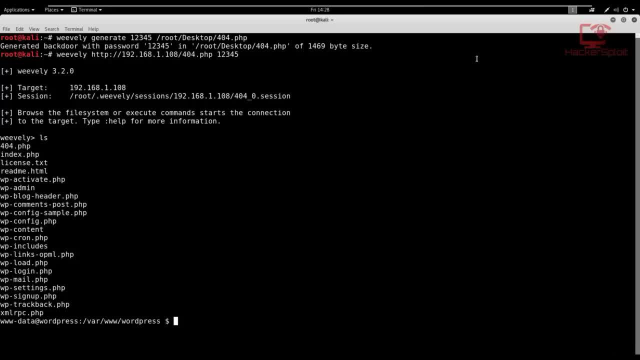 the website And this is extremely dangerous. You know this is just giving you access to anything on the web server And you know you have complete access of everything And, as you can see, if it's running on a server- which it is- you can then, you know, navigate backwards and you're essentially 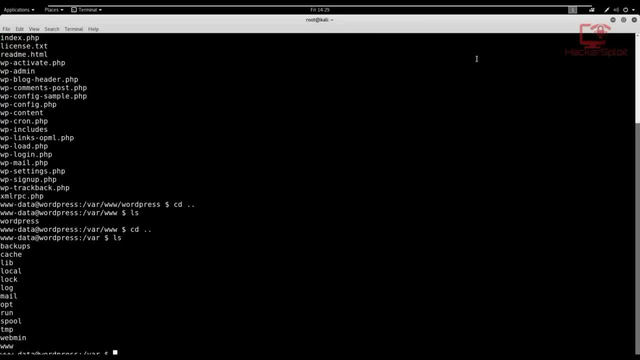 in the, in the root directory of the entire Linux server, which you can, you know, exploit further and cause a lot of damage. Now that again I'm passing out as a disclaimer. I do not encourage you doing this to any site because this, you know, this, can cause a lot of damage And yeah, that's. 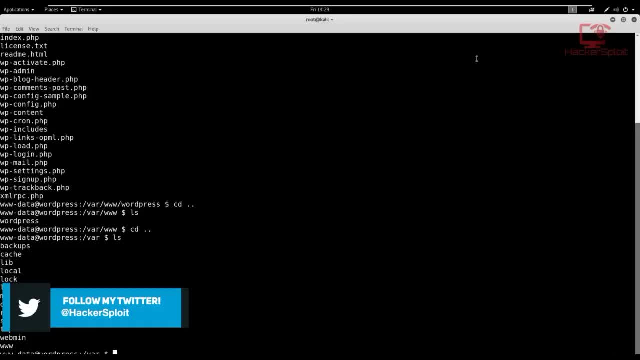 essentially it, How to generate a backdoor. I know it's pretty, pretty simple, but again, really really powerful. But the real trick is, as we know, is exploiting a system. that is the real trick, you know once. 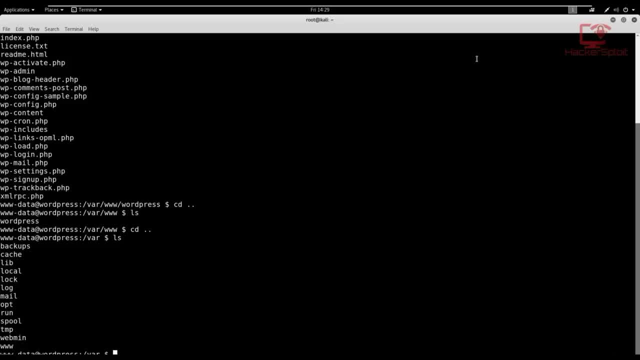 you're in, you can do a lot of damage and you can maintain access and the systems administrators wouldn't even know a thing. You know usually well. I actually had first hand experience with this where I was a system and administrator, and you know the image it was actually hidden in. 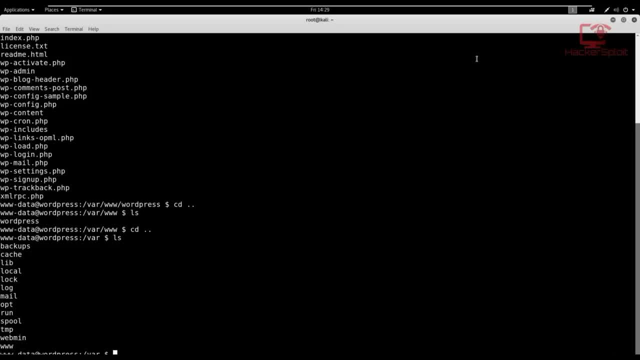 the images folder we're using. you know the image upload vulnerabilities that essentially allowed a user to will exploited the upload system where the user was able to- you know, with burp suite- were able to modify the upload. They were essentially 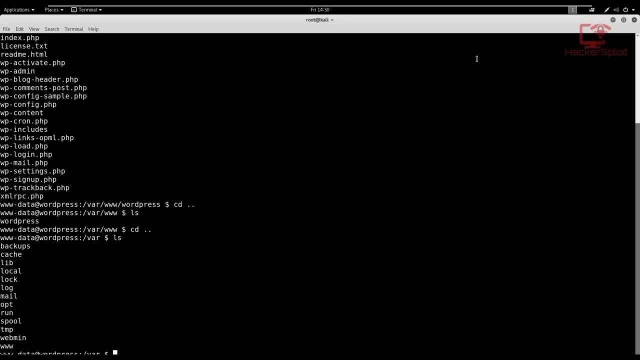 able to, to change the extension of the image to a PHP file after they had uploaded it. And then, you know, to burp suite, they had forwarded it and the packets, and it got sent and the images uploaded And you know, there you go, exploited, as simple as that. So again, 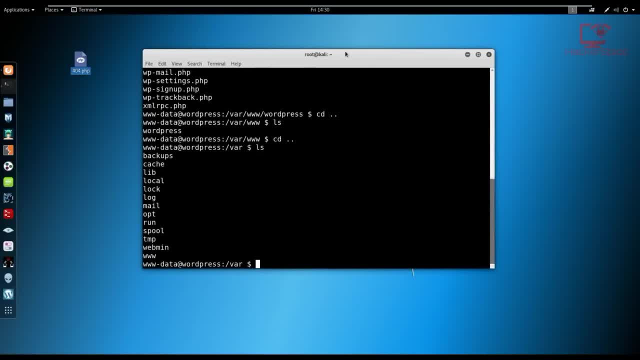 website security is also supposed to be top notch And, yeah, hopefully you guys found value in this video. If you did, please leave a like down below. If you have any questions or suggestions, let me know in the comment section down below, Or you can hit me up on my social networks If you have any. 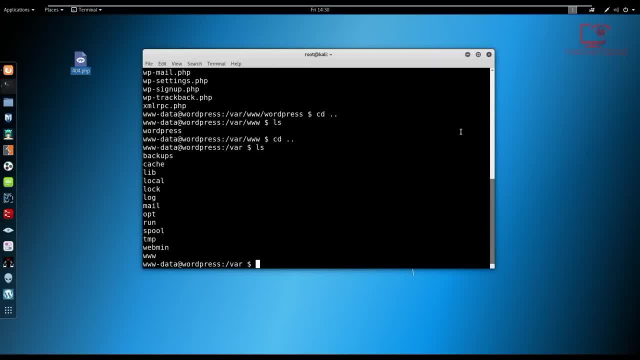 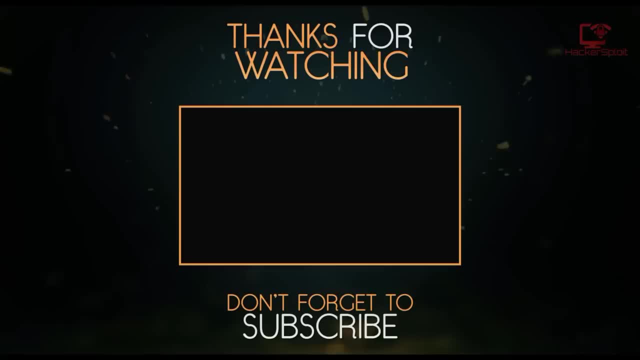 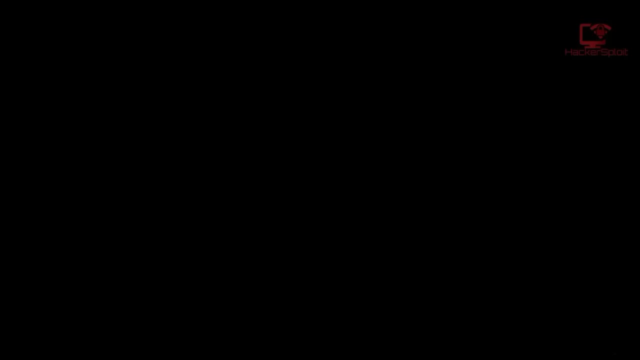 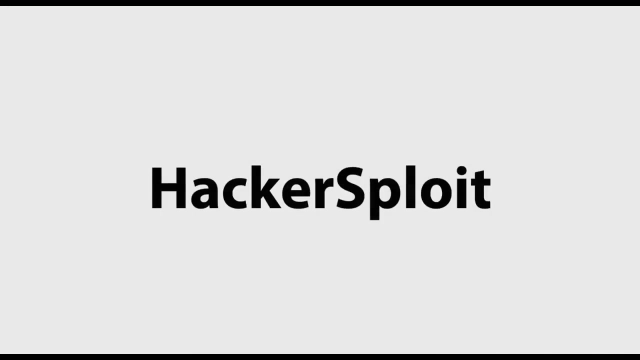 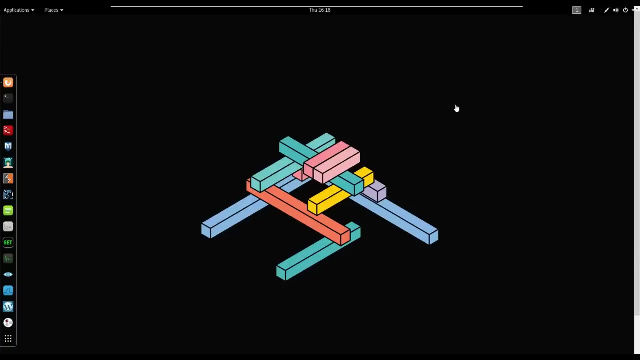 personal questions. hit me up on kick. And yeah, thank you so much for watching, guys. I'll be seeing you in the next video, Peace, Hey guys, hackersploit. here back again with another video, And in this video I'm going to be showing you how to install and use. 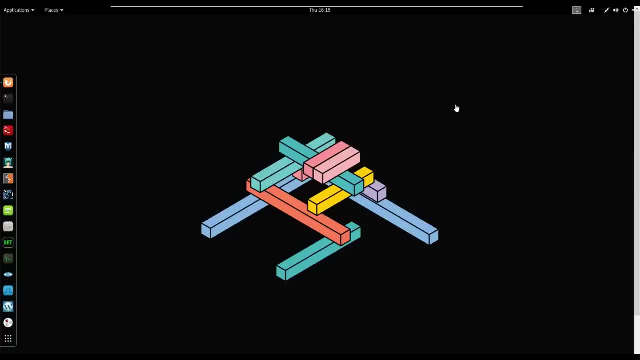 B logger on Kali Linux to create a key logger that can be used on Windows. So, again, we're going to be using B logger, which is a very powerful tool, But it does have some issues which we'll look into in the next video. So, until then, thanks for watching And I'll see you in the next video. Bye, bye. 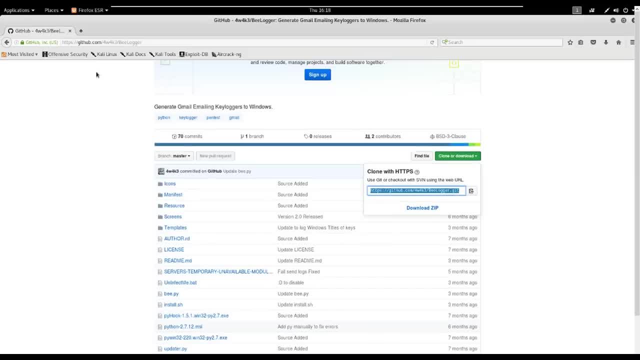 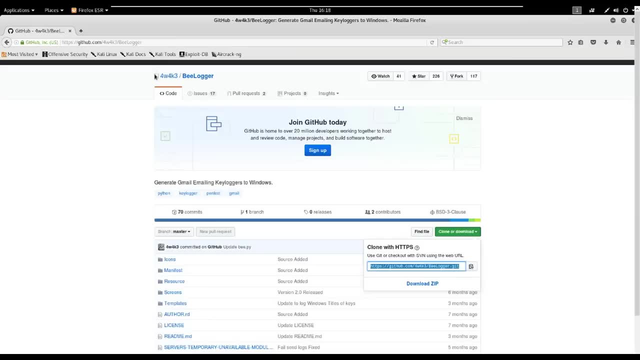 next step. So let's get started. So what I'm going to do now is I'm going to be using the GitHub repository for installation. Additionally, you could use the lazy script to install B logger, which is much easier. But if you guys are going with 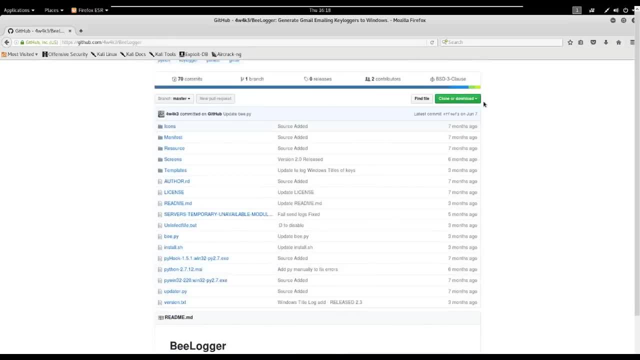 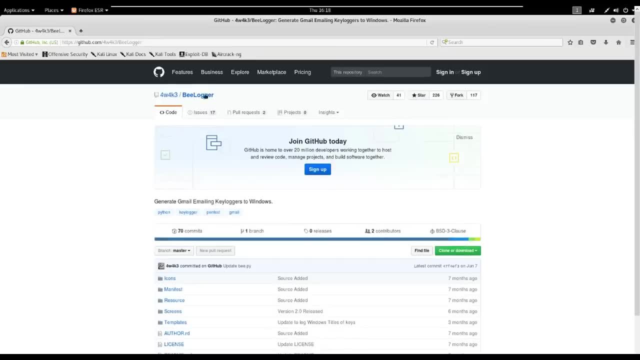 this method. it works perfectly as well. So what you want to do is go to the GitHub repository. I will leave the link in the description section so you can check it out for yourself. So all credits go to the hawker, which is: four w, four k, three has one who 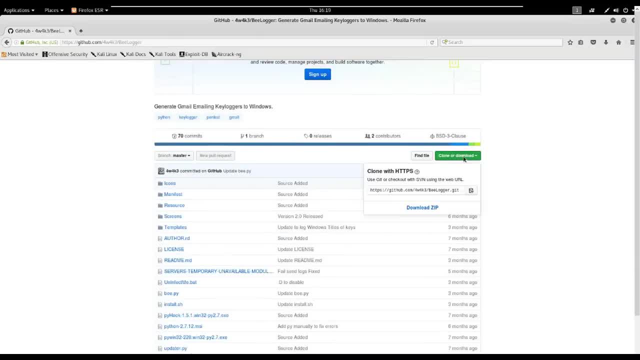 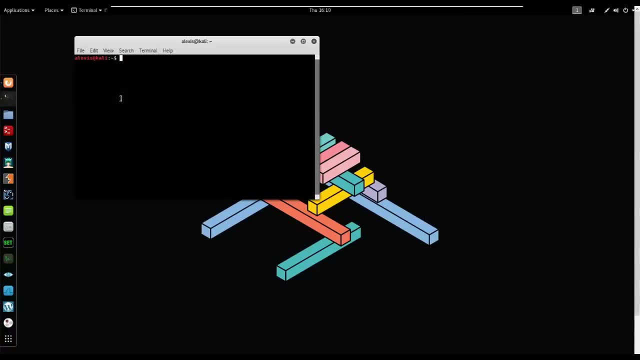 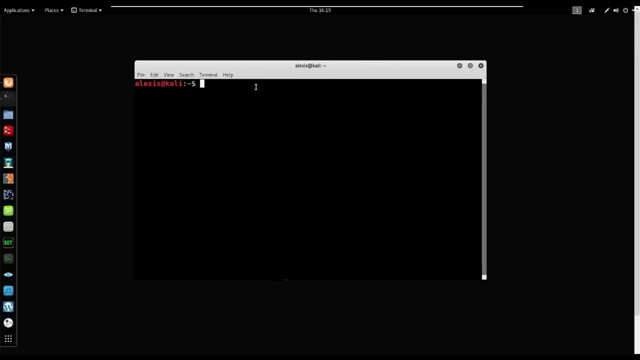 created B logger, So all credits go to him. So what we're going to do is we're just going to clone this GitHub repository, So I'm just going to copy the link and we can get started with the terminal. Alright, so first things first. let me just enlarge the terminal so we can see what's going on. Alrighty, so, 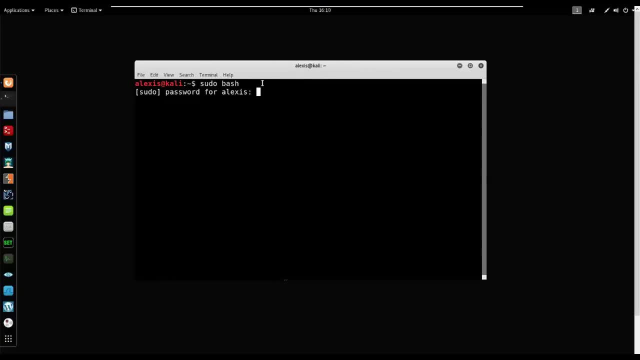 the first thing I'm going to enter root sudo bash and let me enter my password in. there we are. So now I want to browse to my desktop, because that's where I want to install B logger. download and install the files for B logger. 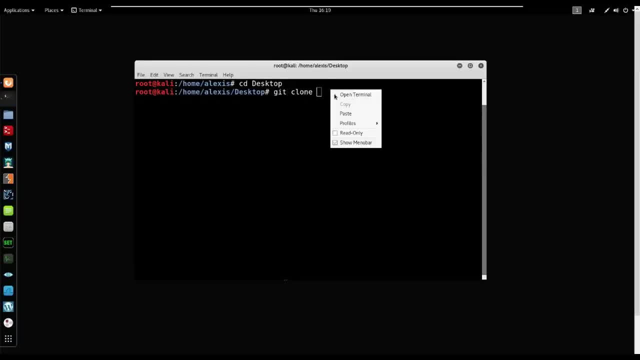 So we're going to clone the repository, git clone, And I'm going to paste in the GitHub link that we copied And I'm going to hit enter And, as you can see, it's going to create our B logger folder And hopefully this shouldn't take too much time. I'm using a VPN for my 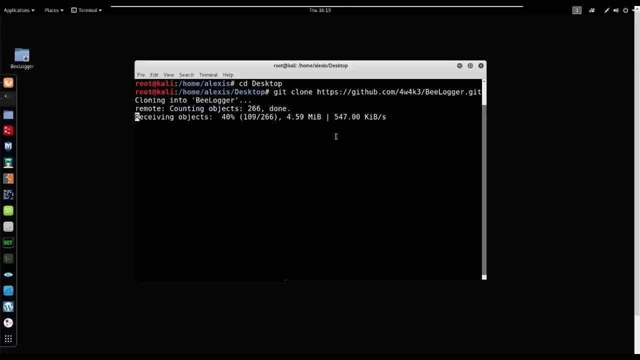 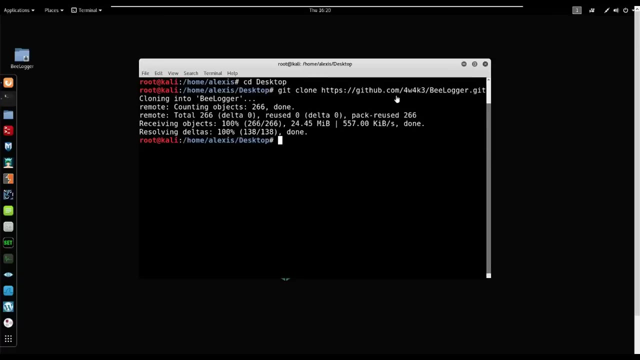 connection, which is why it'll probably take a few seconds to download. So, again, yours might be different if you're using your active ISP connection, but I'm using a VPN that's limited to 500 kilobits per second, So I'll meet you when it's done. Alrighty, so once it's done downloading, we can actually continue. So we're going to browse into 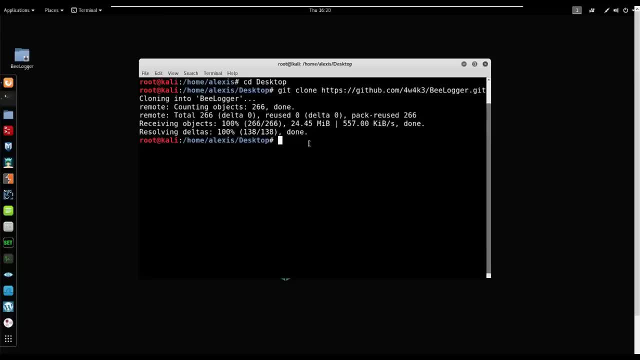 the, the B logger. We're going to browse into the B logger folder, So we're going to change the directory. Oops, let me just clear that out. So cd B, B logger, like so, And now we can look into the B logger folder and we have the installed on. 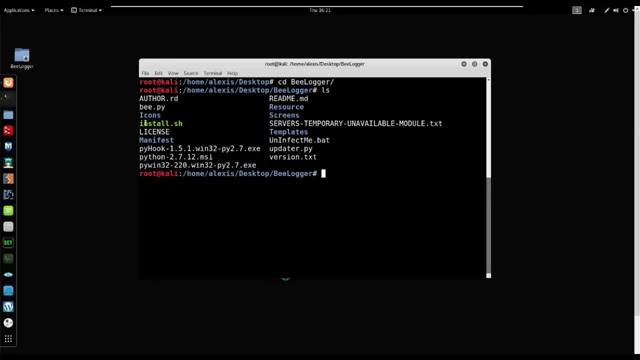 each file, which is a bash script. So, as you can see, we do have the permissions to run it. So it shouldn't be a problem at all to start the installation process. So I'm going to just use the installation. So install dot sh, okay, and it's going to begin the. 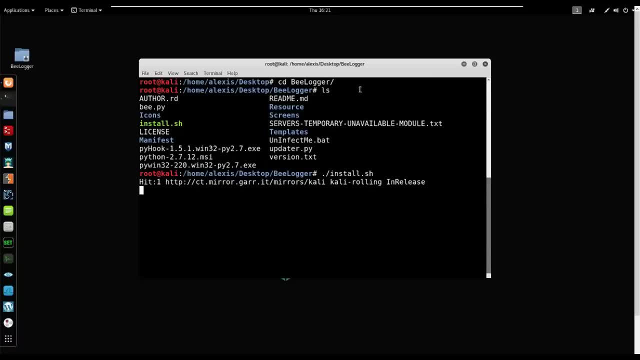 installation process for the B logger script. So just give it a few seconds to start up, because it does need to set up additional dependencies, like wine and Python or PyCharm, for example. So just let it start reading the package lists and we can get started with the installation process. So, as I said, just give it a few seconds. it shouldn't take too. 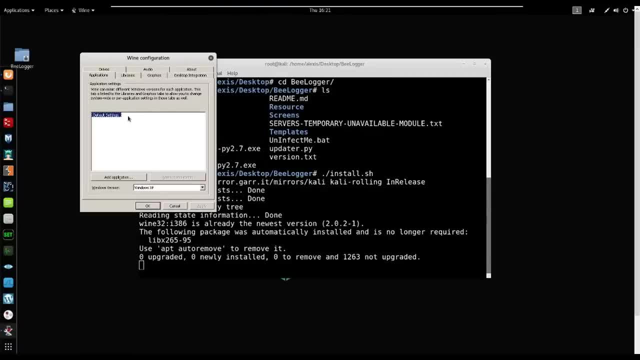 much time And, as you can see, it's going to ask us for our wine configuration. So I'm just going to hit default settings and maybe change it to Windows seven and hit apply, And then I'm going to hit OK, All right, And after that it's going to ask us to set up Python. 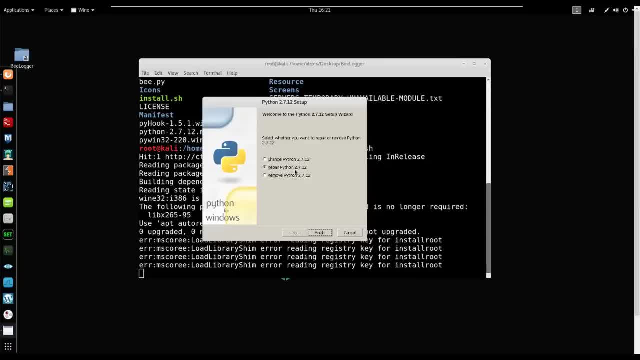 2.7.. So, as you can see, I already have it installed. So I'm just going to hit finish And it's going to just repair Python. But in your case it'll prompt you to install Python additionally all over again, or in install it. 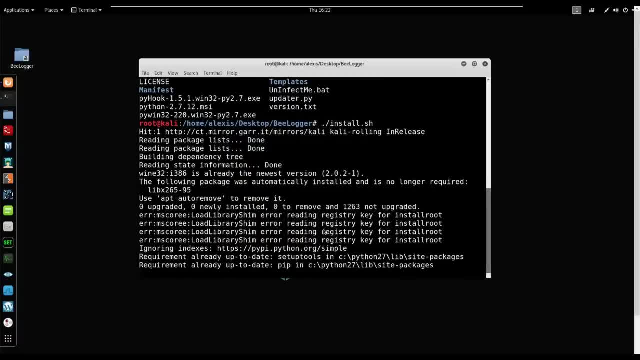 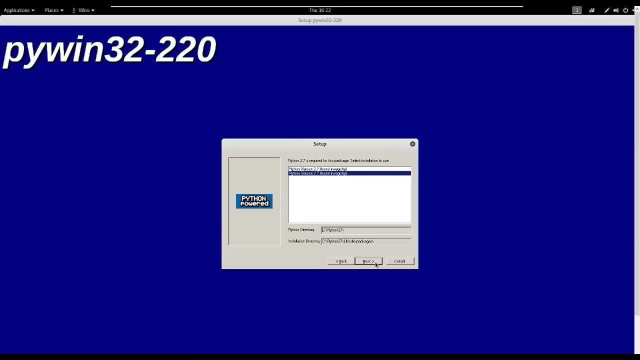 fresh, So make sure you do that. And I've already installed Python. then the next thing is going to ask me to install is pi win, So the two bit version. So I'm just going to hit next and next And it's going to install that for me. Pretty simple, So just let that complete. 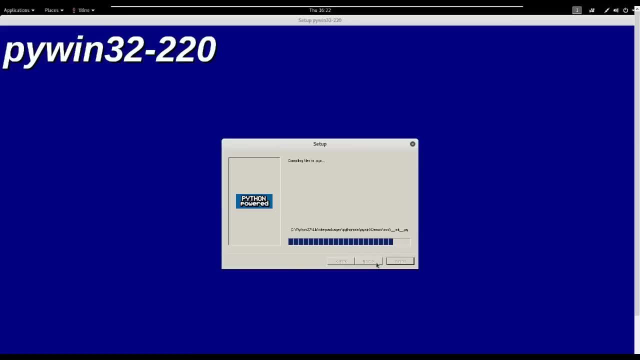 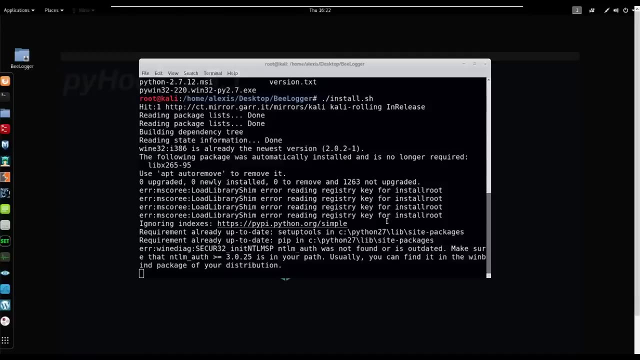 And it shouldn't take too much time. now, There we are, Alright, so just going to finish that installation. And now it's going to ask me to install pi hook. right, pi hook is very important in this. So, as I said, I already have mine installed, So it's. I'm just going to breeze over these, these. 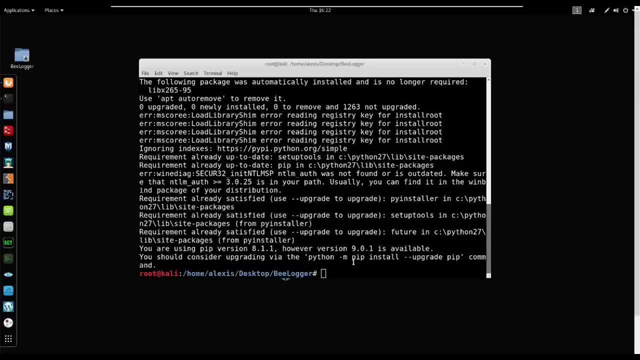 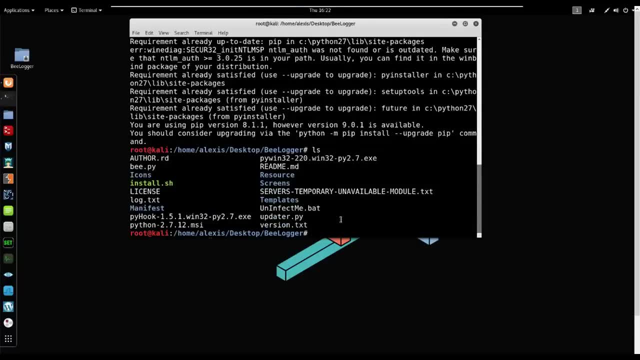 installation processes. And there we are, So we've installed, be logging up. And you might be asking yourself: well, how do I access blogger? if we view the? if we basically look inside the folder, we have the B dot P Y, so Python and B dot P Y. and if we start 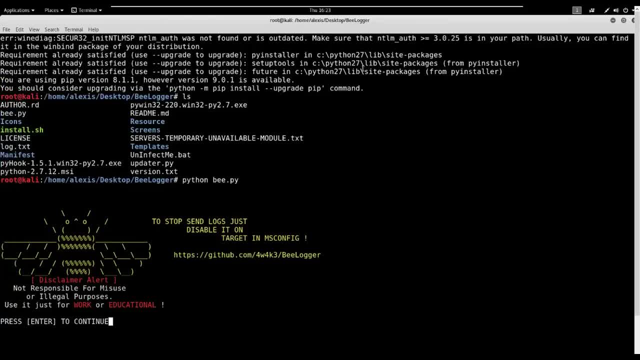 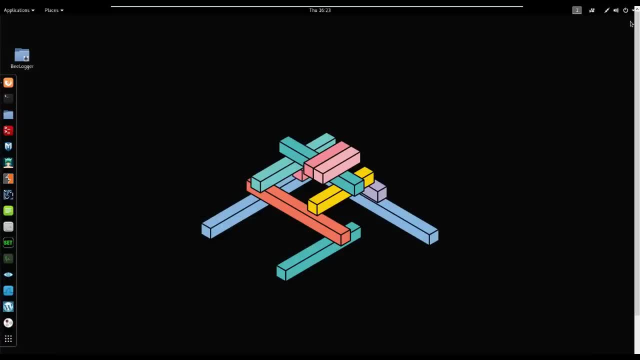 that up. as you can see, we have the B logger opened and running. so, in addition, what I'm gonna do is I'm just gonna. what I'm gonna do is I'm just gonna exit and I'm gonna stop in a new terminal altogether, because that has brought a. 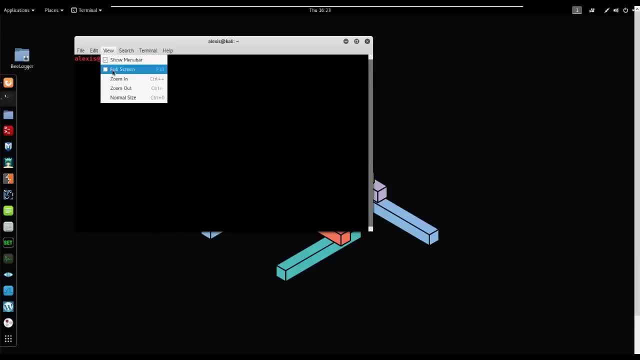 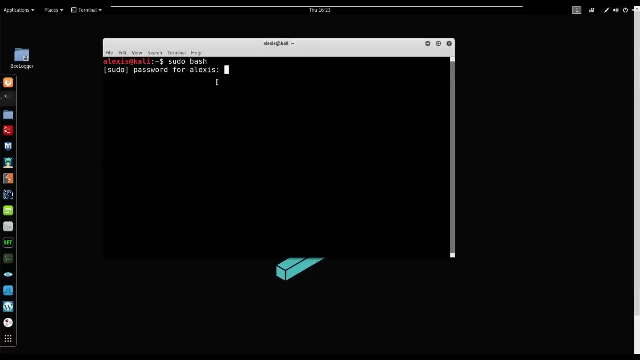 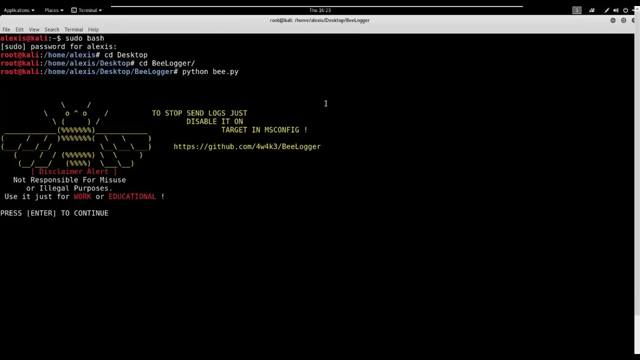 few issues before after I've installed the PI hook. so what I'm gonna do is I'm gonna enter root again- excuse me, like so- and see the desktop and obviously see the B logger and Python B dot PI. like so, and there we are. so we're currently in the B. 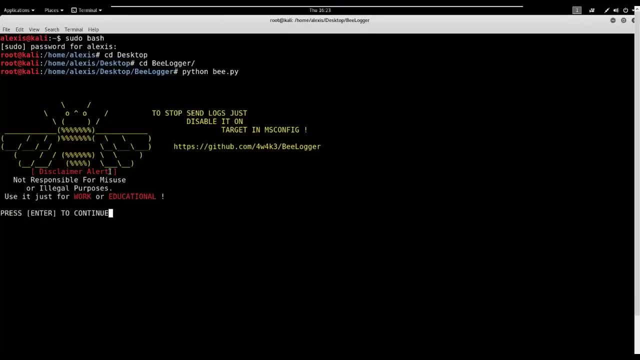 logger script right now and it's gonna ask you, as I said, it's gonna ask you now to hit enter and, before we get started, as you can see, use this for work or educational purposes. so I have to you, as I said, it's gonna ask you now to hit enter and, before we get started, as you can see, use this for work or educational purposes. so I have to. 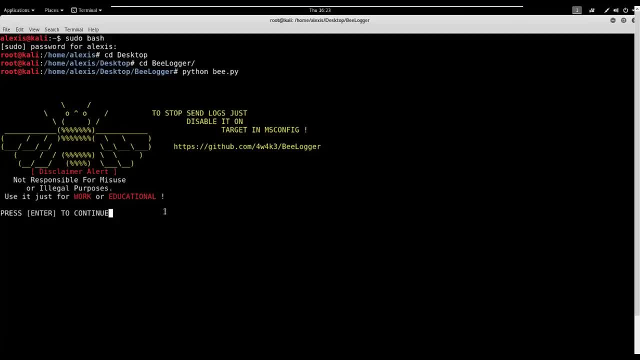 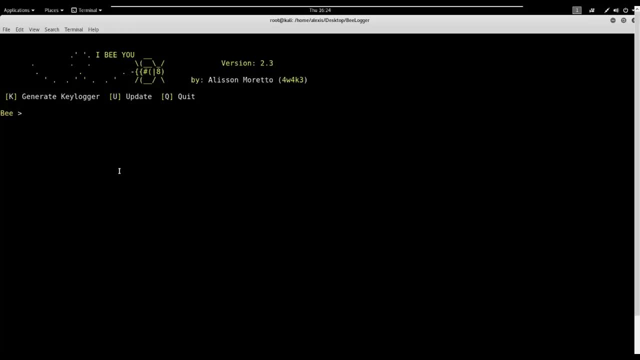 throw out a disclaimer that please use this at your own discretion and you know I'm not gonna be held responsible for anything you do with this tool. so just hit enter to continue. and now the options are pretty simple. it's gonna ask you, it's gonna give you three options, K being the option to generate the key. 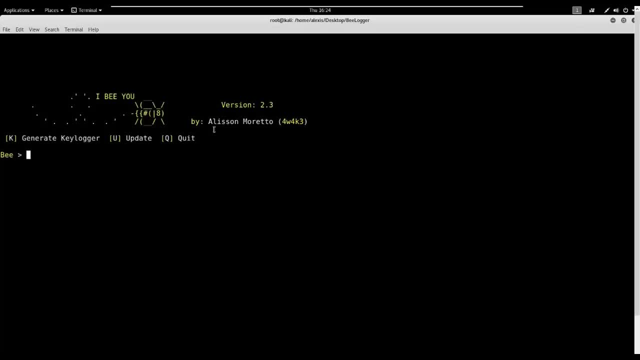 logger, you being to update the B logger, which is quite awesome that he added that all credits go to Alison Moreto and Q to quit. so we're gonna generate the B logger, which is the key logger, which is the key logger, which is the key logger, is done by using the key K key, so once you hit that, it's gonna ask you to. 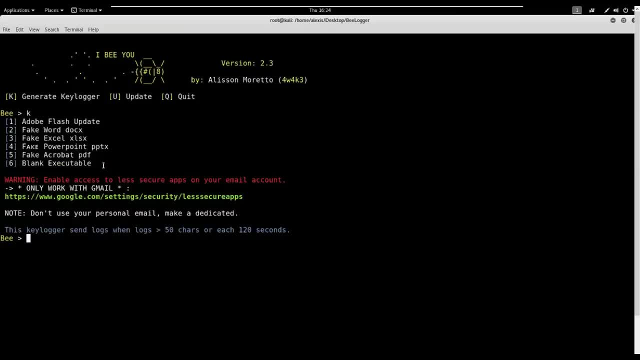 select what type of key logger you want to mask exactly. so you can choose an Adobe Flash update which is pride group quite good and will help with social engineering to some extent. you then have your fake word document, which is really not convincing, especially for users who are pretty familiar with computing and 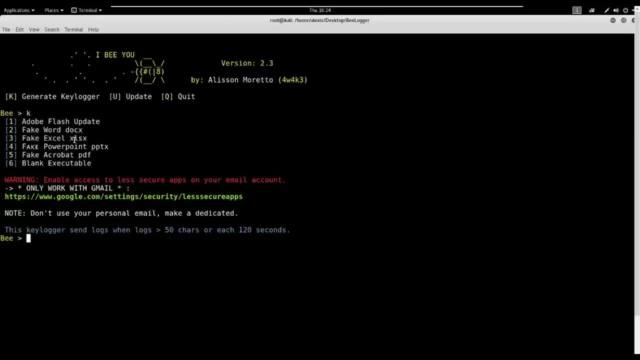 we then have the fake excel sheet, which again is not very convincing because it is going to be an exe file. we then have the fake PowerPoint, which is quite convincing because it is a PowerPoint and less people come in contact with PowerPoint, with PowerPoint files as common compared to excel and word documents. we then have the fake 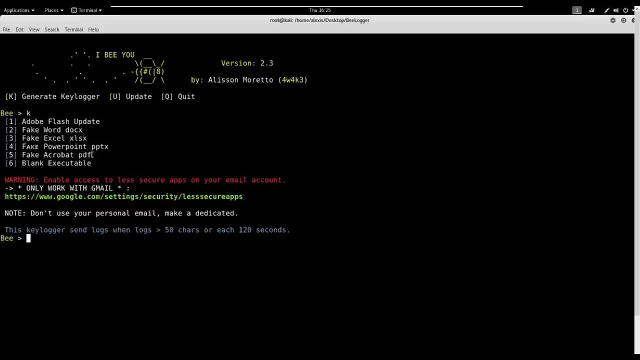 acrobat PDF, which is also quite convincing. we then have the blanket executable. and now, before we get started with creating the B logger, the thing about a B logger is that it's very easy to create a B logger. when I say create a key logger, what I mean is not to actually create a key logger by yourself or to script it. 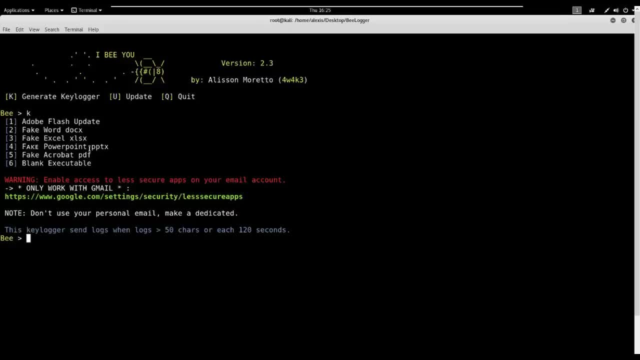 but to create a B logger that you're using to gain in information or you know you're trying to use for either malicious intent or or for testing. it really comes down to how you're going to install it on your targets computer, how you're going to run it on your targets computer, and that's where social 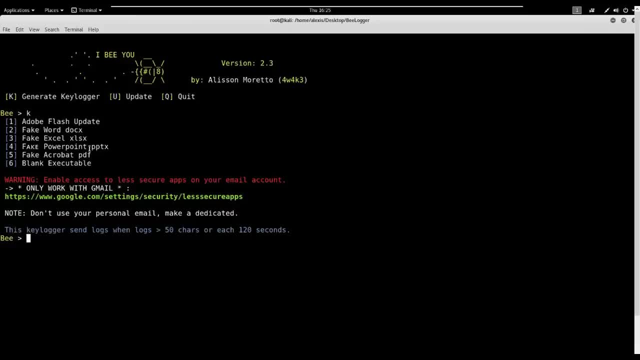 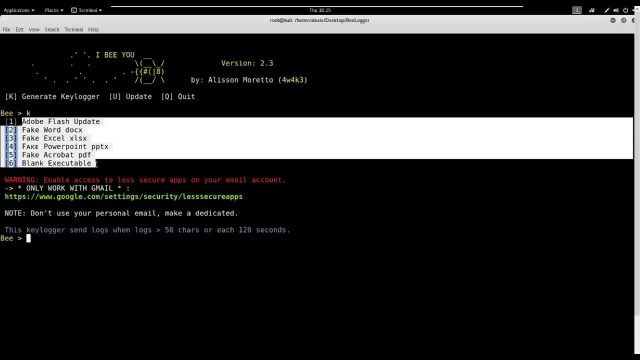 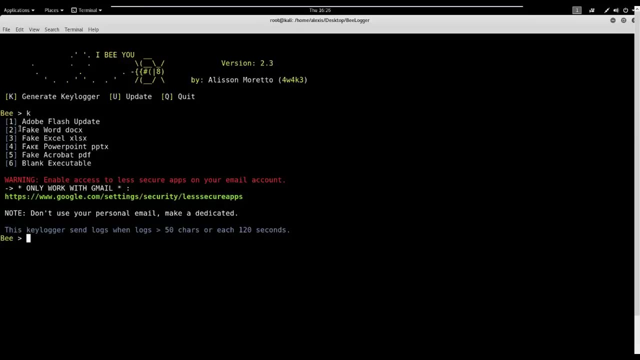 engineering comes into place and we look- we'll be looking at techniques or not- on how to be using this, and what I'm coming to really here is: all of these will be detected by if you try and send any of these, these key loggers, in forms of, for example, an Adobe Flash, update, Gmail and 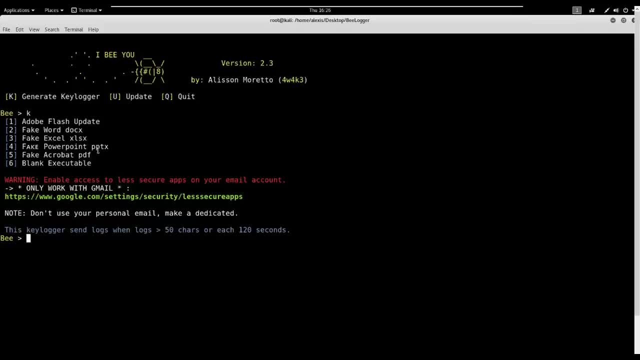 all of the other top email providers will detect this as a virus and will probably throw the mail in spam or will alert the user or the target that this does indeed contain a virus. so you really have to be smart and if it comes to you down to using a rootkit to mask the key logger or to avoid 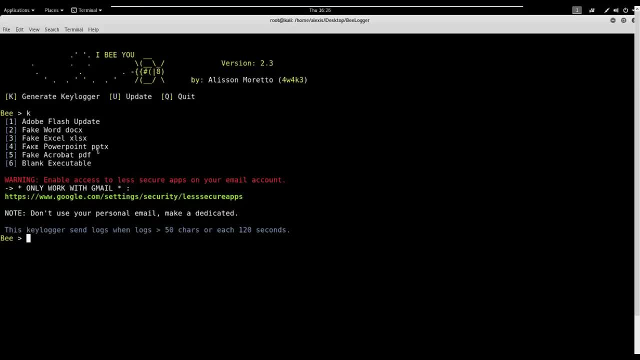 antivirus detection- you know that that's where all the whole social engineering process comes into. but, as I said, we'll be looking at that in future videos- and how to mask all of these exploits or just basically how to mask your program or key logger to avoid detection by anti viruses and, of course, by users, because 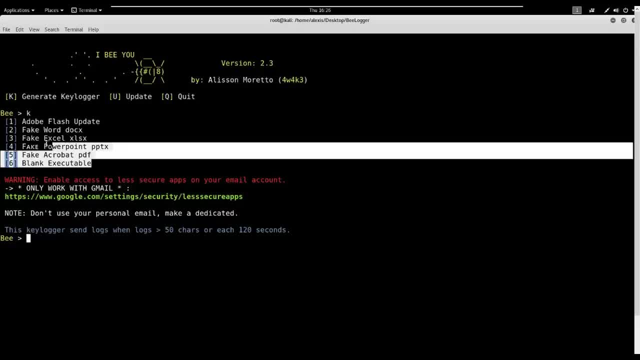 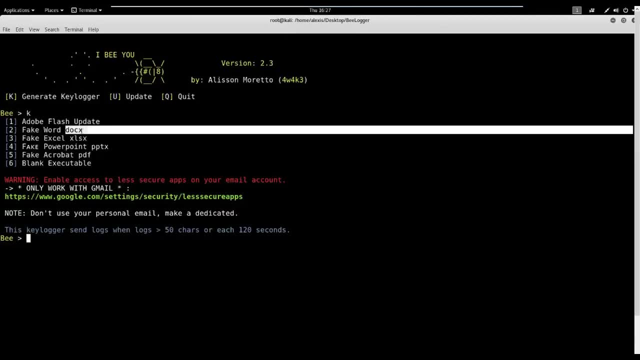 I said, it's going to be less likely that you can people with things like this: for example, a fake word document that contains the the doc X extension file, but also contains the exe extension. so it's really important to understand that. so let's get started with actually creating. 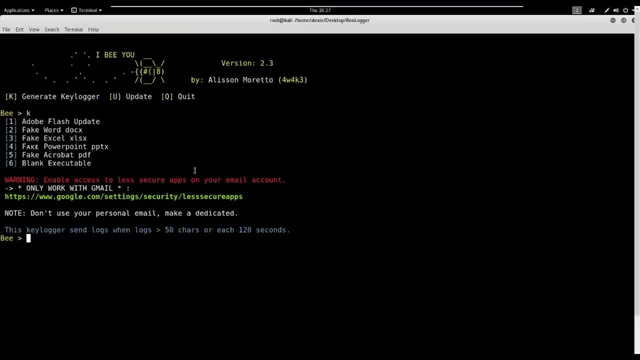 this keylogger, so it's going to tell you: warning: enable access to less secure apps on your gmail account. now what this means is you have to. actually, it's going to ask you to use a Gmail, as you can see. it's going to tell you only works with. 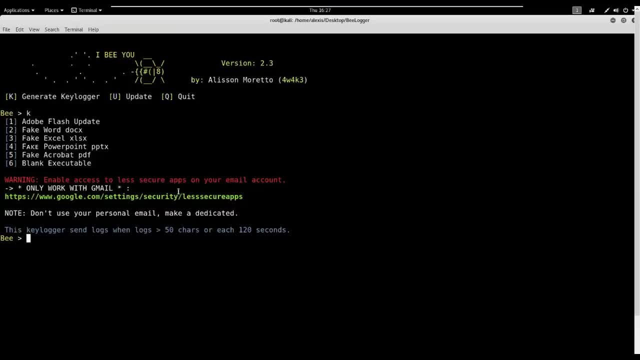 Gmail. now, why you need to enter your or create a gmail email for this is because you're going to need an email in which the keylogger program will be sending back the results to. so I would recommend creating a separate gmail account just for getting your results back. but as you can see, don't it's going to tell you. 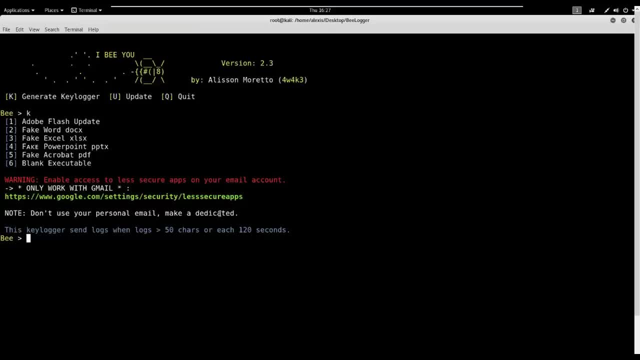 here. don't use your personal email. make a dedicated, separate gmail account, specific, specific for the, for the gathering of results. so what you're going to do is you're going to create a separate gmail account. once you've created it, you just want to click on this link. you can just open the. 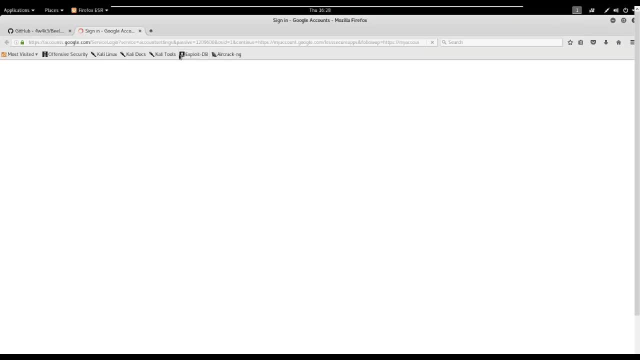 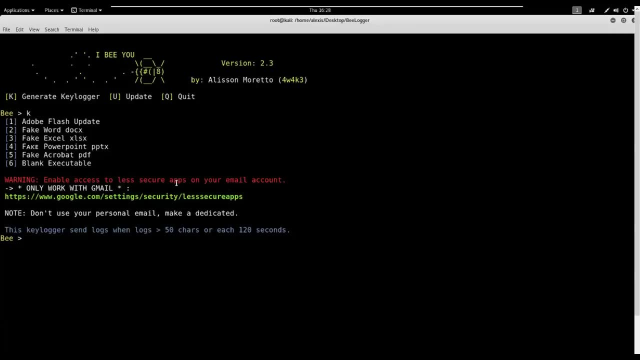 link in a new tab and hopefully does that here, and it's going to ask you if you're signed into that gmail account. it's gonna ask you to disable. it's going to ask you to disable less secure apps on your email account. what this is going? 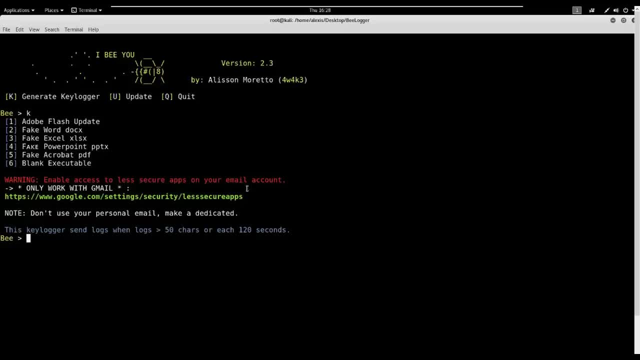 to do is it's going to allow your email to be under the control of the keylogger, so the keylogger will be able to log in and send requests and send the results from what it has gathered from the from your targets computer or your gmail app. 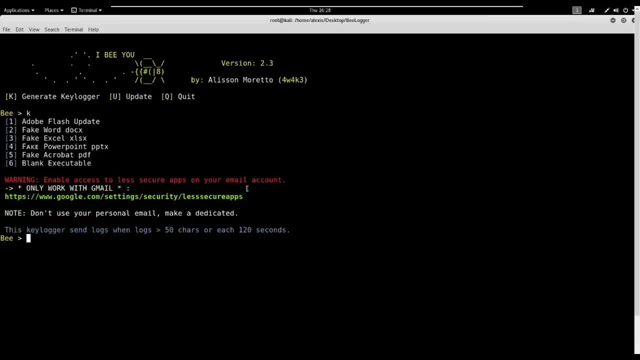 system and it'll save them on that email. all right, so, as you can see, this keylogger will send logs- 50 characters or each in 100, in intervals of 120 seconds. so again, very, very powerful and you're getting extensive information. of course, this will become ineffective if the user is not connected to the. 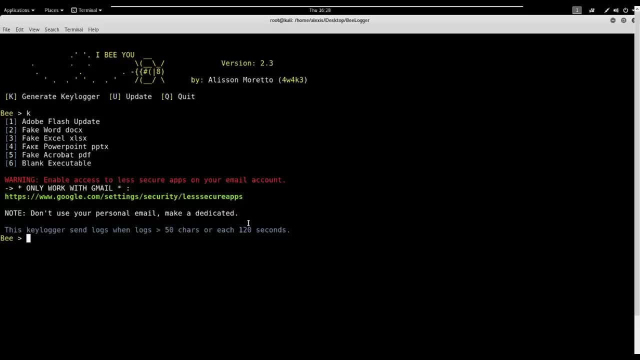 internet. but again, you know this is how these things work and there's always pros and cons to each of the side. so what I'm I'm gonna do, I I've not created an email for this, because I'll be explaining how to mask this key logger in the next videos, where I'll be showing you how to. 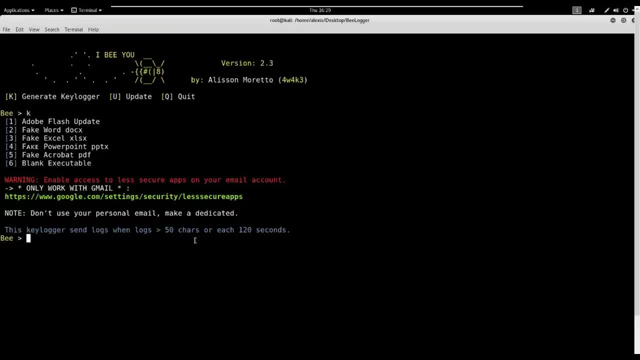 use social engineering to avoid detection, antivirus detection and obviously to mask it so that users cannot detect or, you know, it does not look obvious that this indeed is a virus or malware. so I'm just gonna enter a. I'm just gonna enter a simple. we're just gonna be using a just a fake email. 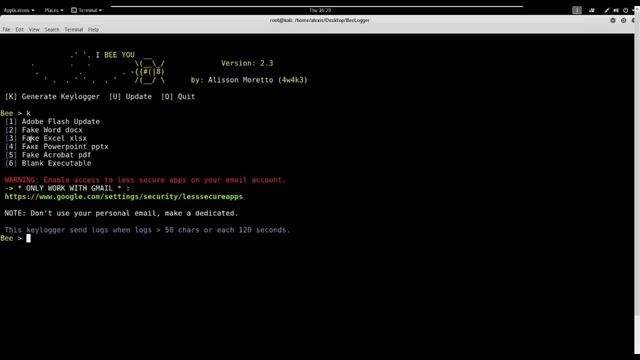 address. so what I would recommend, if you're going to be using this, is to use the Adobe Flash update. the reason I'm saying this is because people, when they see Adobe Flash, they already know that this is an executable program and from that, if it's an exe file, they won't be as hesitant to running it as if you. 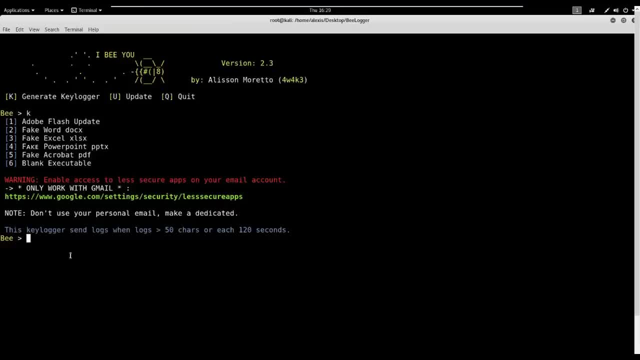 would have found a document with the exe extension. so again, I'm going to use the- and this is obviously for social engineering purposes. so Adobe Flash update and it's gonna ask you type your Gmail to receive the logs. so I'm just gonna hit test at gmailcom. as I said in the next video- the follow-up videos- I'll 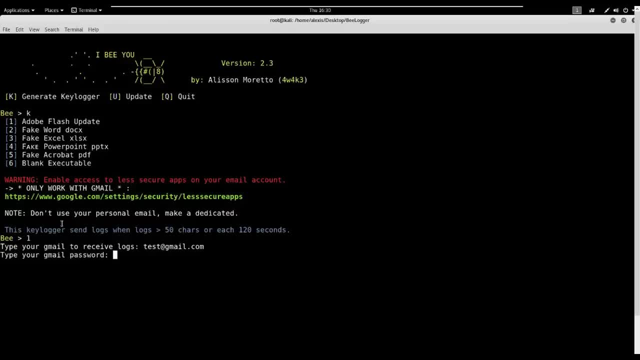 be making and I'll be showing you how to essentially hide or to mask these key loggers and other malware from detection. so we're just going to enter random password, so test also, of course, these. this email does not exist and this password, again, is not real. 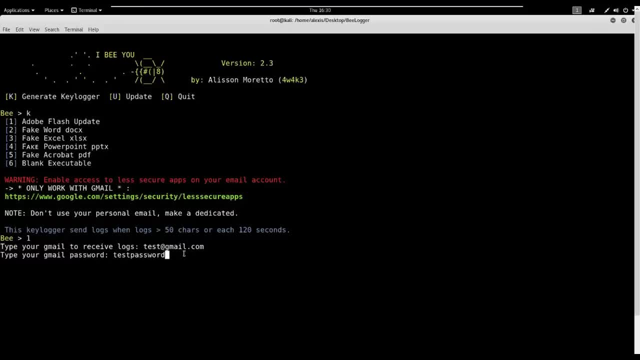 I'm just using it to show you that indeed, it does create the key logger. so once you've entered the password, just hit enter and it's going to ask you if this information is correct, and I'm going to hit yes and it's going to start the. 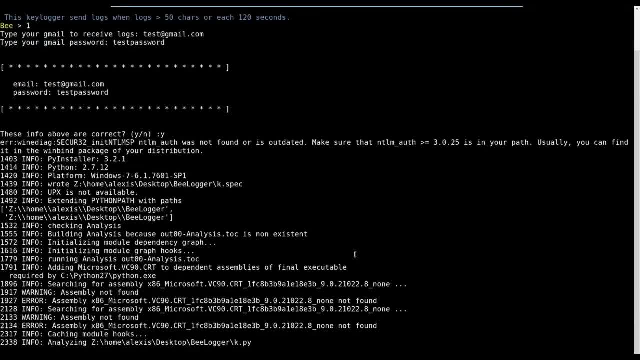 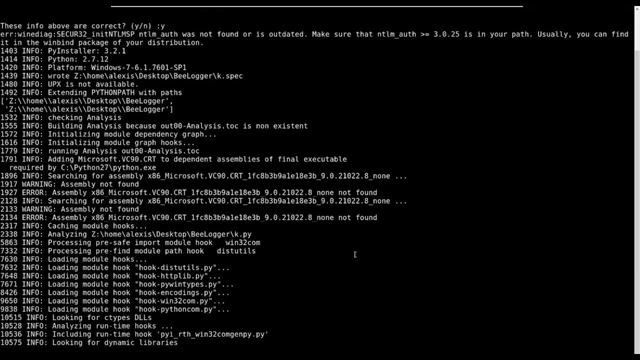 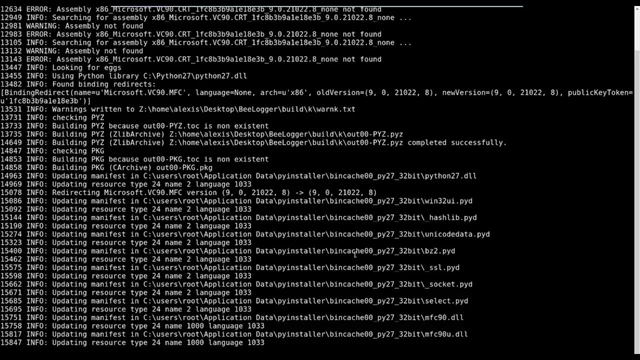 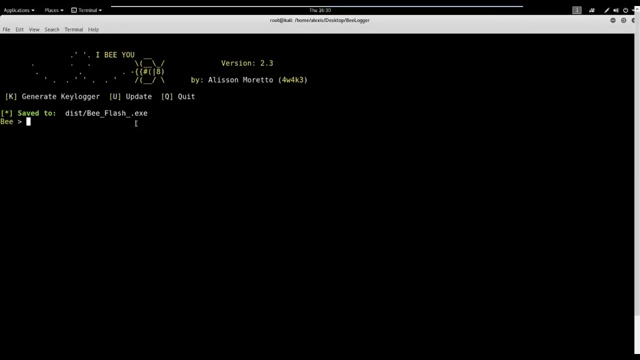 creation process. as you can see, it's creating the key logger and just give it a few seconds. hopefully it shouldn't take too much time again. the it will take different times depending on what type of executable you choose, whether you choose the flash update or the word documents or excel documents, etc. etc. so 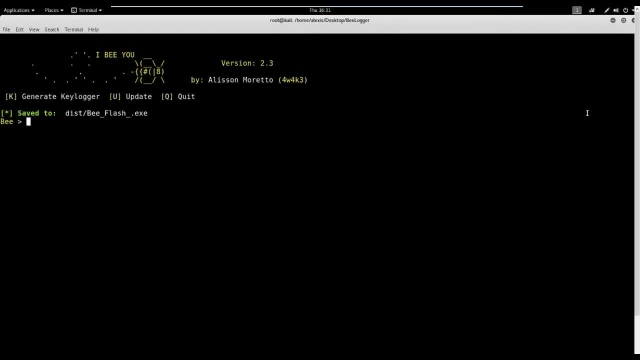 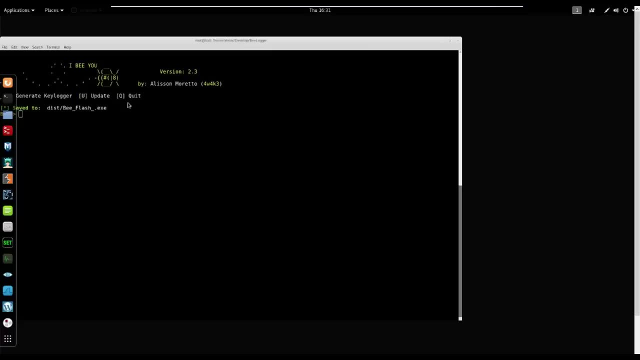 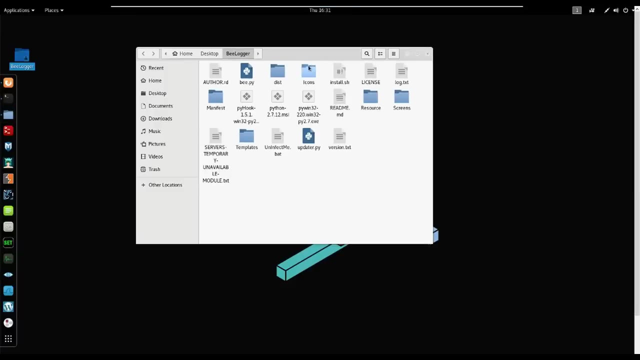 that's actually done now and hopefully I don't know where exactly it or there we are saved to dist slash be flash dot exe. so obviously, again, as I mentioned previously, it's going to save it in the be logger folder that we created in the dist folder. 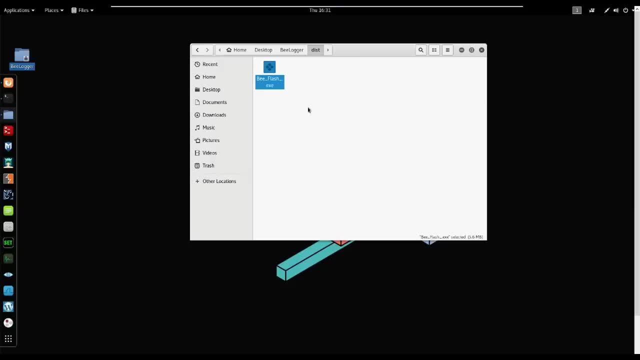 now what I was talking about here again when, when comes down to social engineering, this is the key logger file, very, very powerful. but again, the trick is, the trick has always been making sure that this runs on your targets computer without detection and without he, he or her, him or her basically finding out. 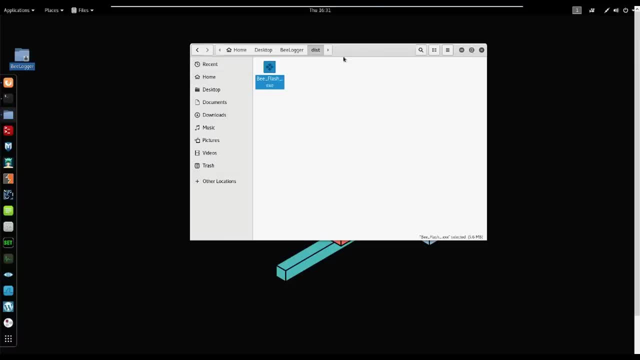 that it's running now with be logger. as far as I know, once you run this, it will basically install it, and the only way to disable it as a service is through the msconfig utility in windows. so again, it does have the ability to be disabled, or? 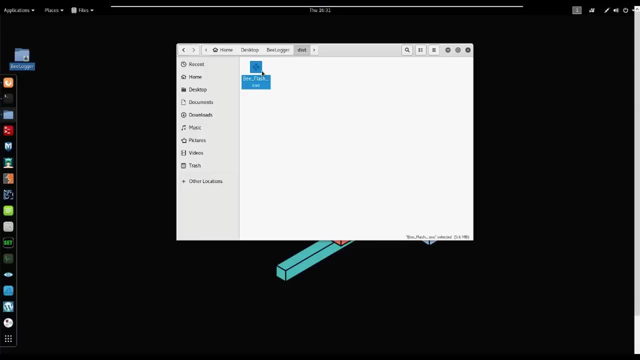 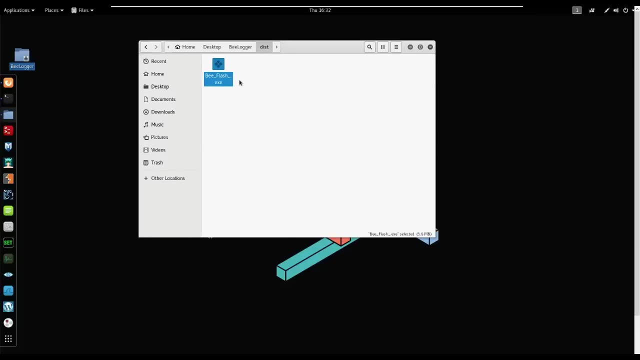 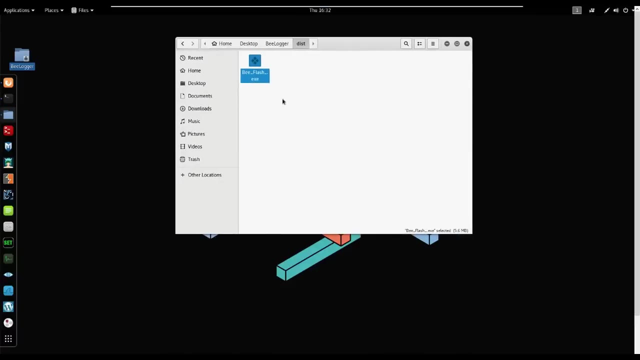 to be stopped. so that was just a little tidbit haunted to throw in there for you. so again, a bit of you could do, a bit of you know social engineering and renaming this to look like an Adobe Flash update. and I would say six times out of ten you. 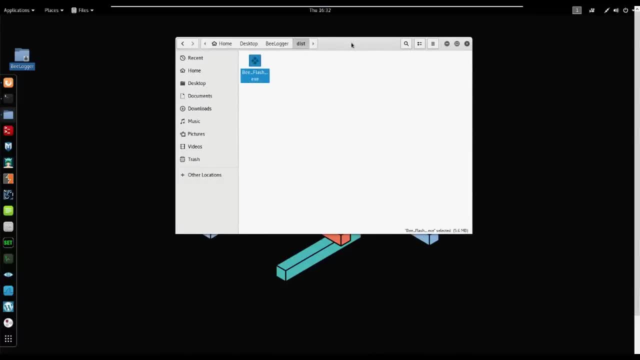 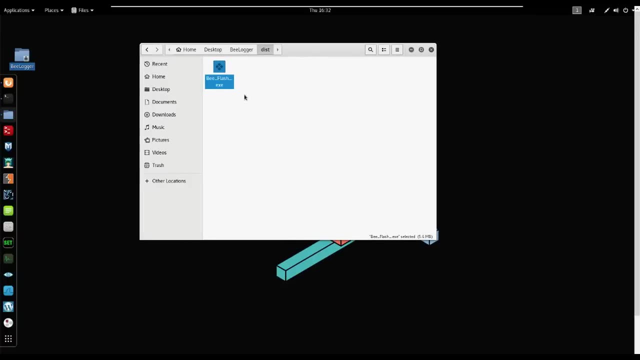 can get your target to run this without them knowing that this is in is indeed malware. now I'm not going to be running and testing this because, as I said, if you try this on a modern Windows installation with Windows Defender enabled or running or any other antivirus software, it's going to detect. 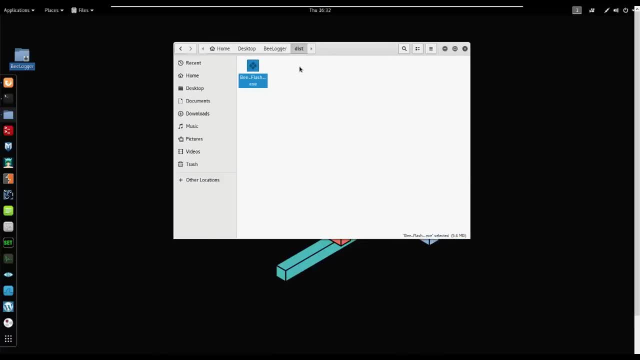 that this is a virus, and even if you try and upload this to Gmail, it will automatically detect that this is a virus. so, again, we'll have to do a bit of social engineering. in addition to that, I'm going to be creating a special little small course exclusive to the msconfig utility, and I'm going to be 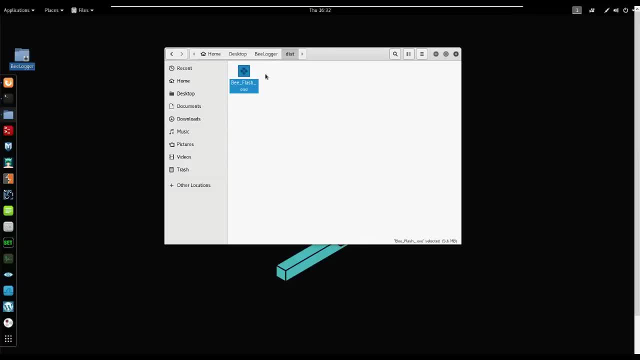 showing you how to create your very own key logger with C++. now, the reason for that- there are obviously some specific advantages of using C++- is that it is a very low lying, or it's a very low, it's a very low level language in the sense. 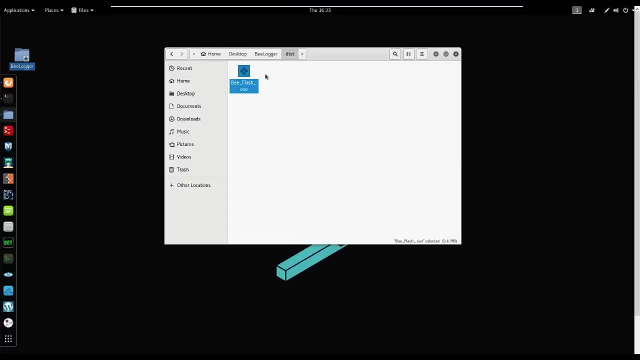 that it, if I was to create a key logger, Windows, nine times out of ten would not detect that this has anything to do with malware or is malicious content of any type. in addition to that, it has a very low level of language. so if you want to, 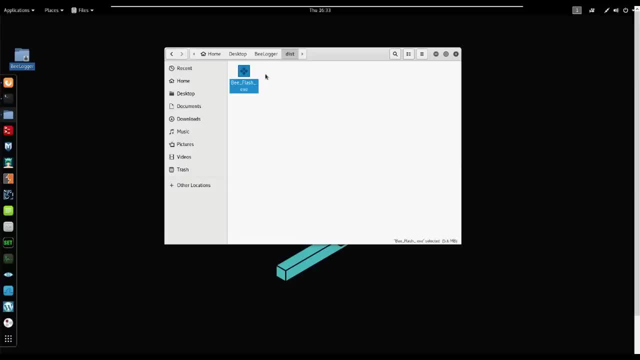 create your own key logger with C++. it's going to be very easy to do that, and antivirus software would not have been able to detect it. so that's basically it for this video. guys, as I said, I'm going to be making follow-up videos to this. 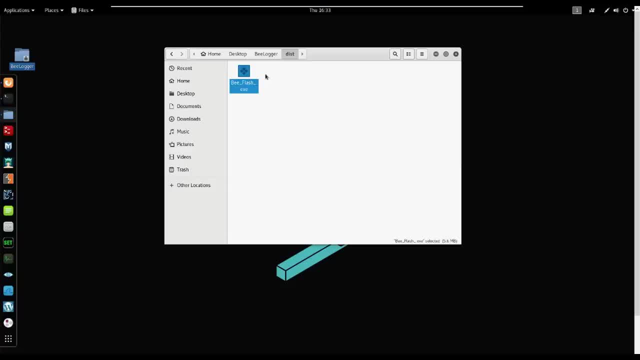 whole be logger section that I've created, or, in in the larger context, the key logger section on this channel. so stay tuned for that. I hope you found value in this video. if you guys enjoyed this video, please leave a like down below. if you have any questions, suggestions, you know you just want to. 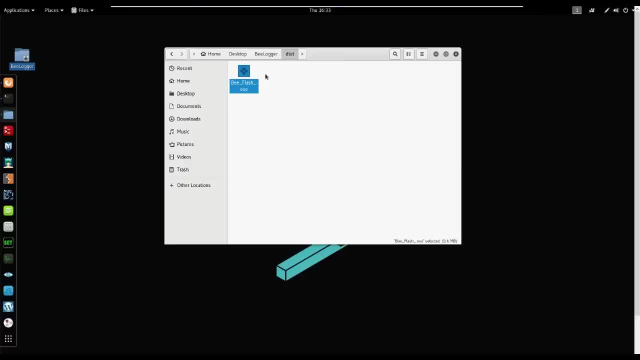 have a chat comment section down below. in addition, you can check out an in-depth guide of this video on my website. you can also check out the discord server that I've created for the channel, where we'll be having discussions and where you can send me your video suggestions and where we can basically just interact. thank you. 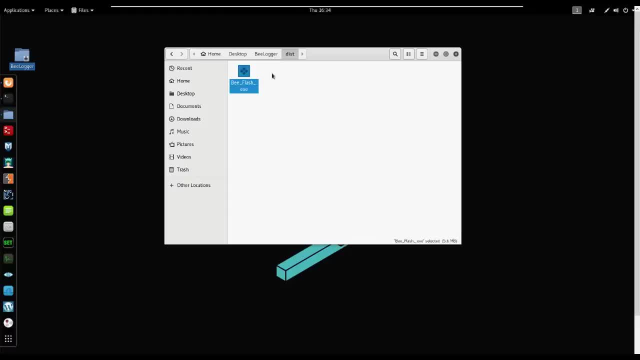 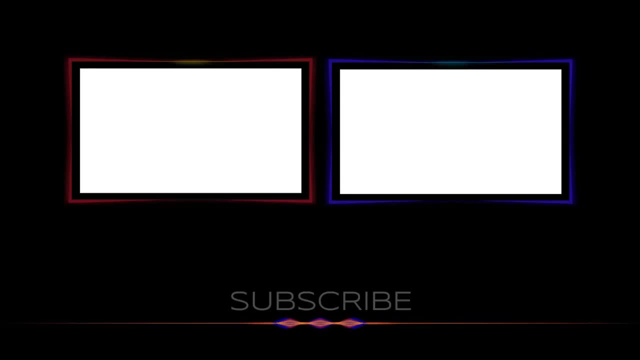 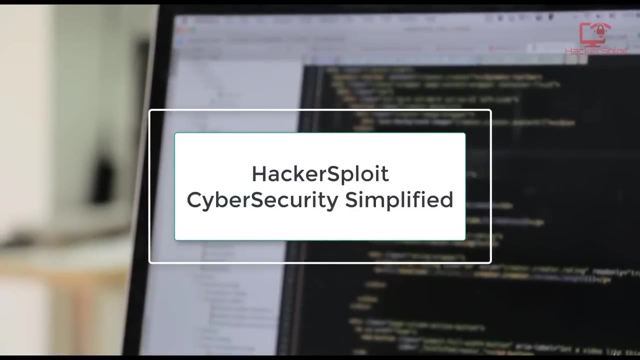 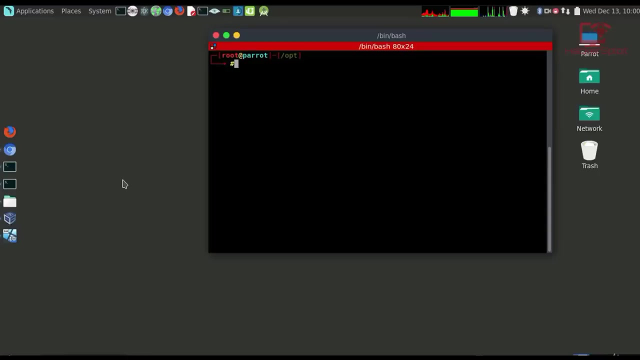 so much for the support and I will be seeing you in the next video. peace, hey guys, hack exploit. here back again with another video and in this video so looking at Saint. so you might be asking yourself: well, what is Saint? well, Saint is, simply put, is a spyware generator for Windows, and it is coded or developed in 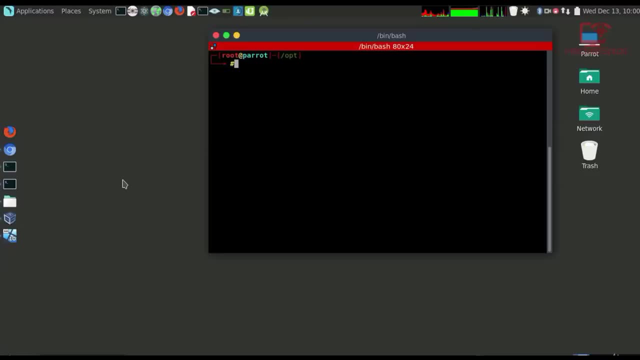 Java. all right. so essentially, what did the functionality that it give is? it gives you the, the key logger functionality and the key logger function, so you'll be able to get keystrokes sent back to your host email again. I'll show you how to do that right now. you can take screenshots of the: the target. 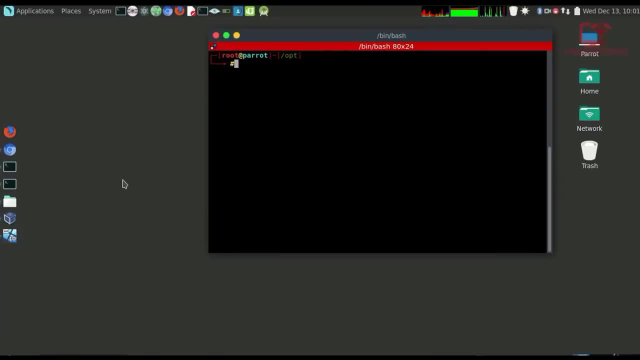 computer. you can capture, you know, images with a webcam. you can also. you also have persistence, all right, so let's get started with me showing you how to get it installed or to configure it, and then we can create the malware- or the spyware for that matter, and how to move it to your operating system of choice, your test. 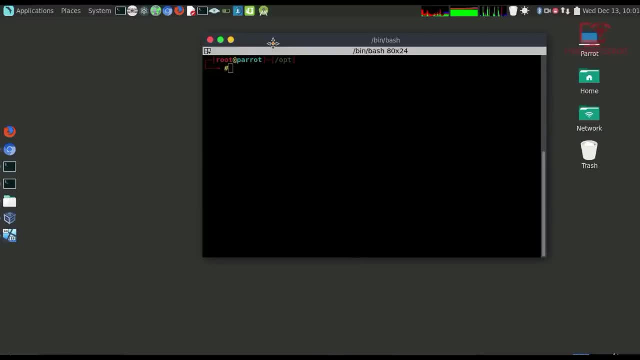 operating system. again, I do want to throw out a bit of caution, because this can cause damage and I do not want you to perform anything or to use this in any way that may infringe any any laws, so please make sure to stay on the right side, all right? so I already have the link open up here. it is a github. 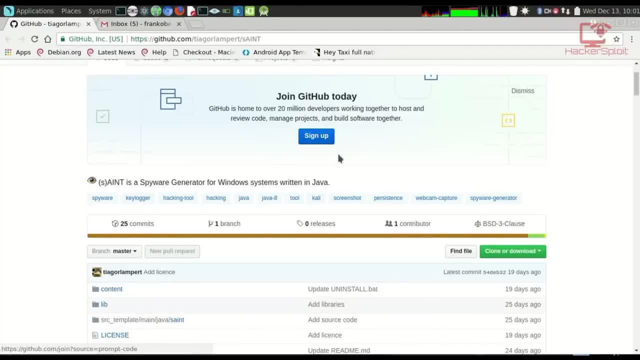 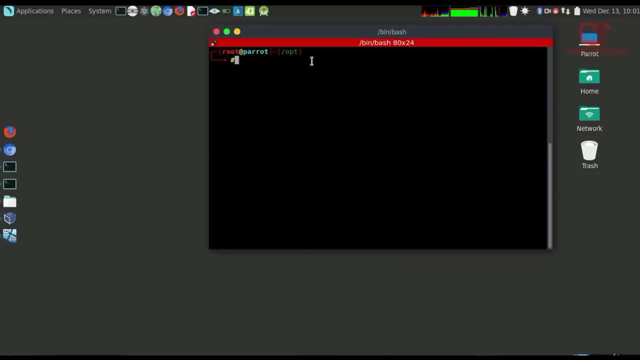 repository, so the link will be in the description, as always. and, yeah, you can just clone it, and we need to install a few things before we can move on to the next video. all right, so I already have it cloned here, but you can do that for yourself. I. 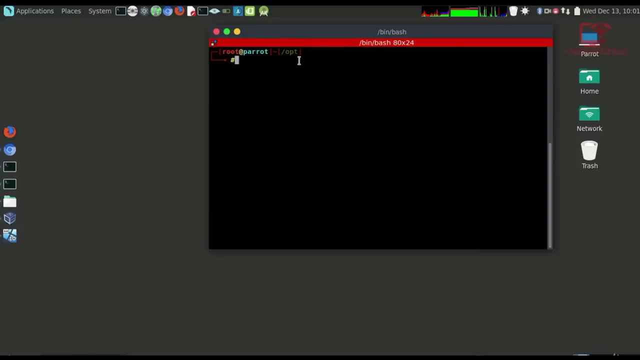 usually keep all my scripts that I'm not really keen on, or you know, scripts that I don't really trust, in my optional folder. again, it's a good way of separating your experimental folders from your, you know, the folders that you can really hold as part of your system. so, as you can see if I list it down here, 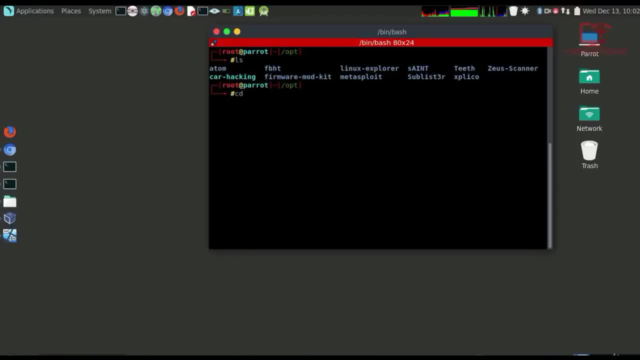 I already have it here, right here, Saint, so I'm gonna move into the directory. you will have the same with. you will have the same directory, alright, so, Saint, and if I list gets inside, there's a few files you have inside. now. the first thing you need to do is you need to look at the, the 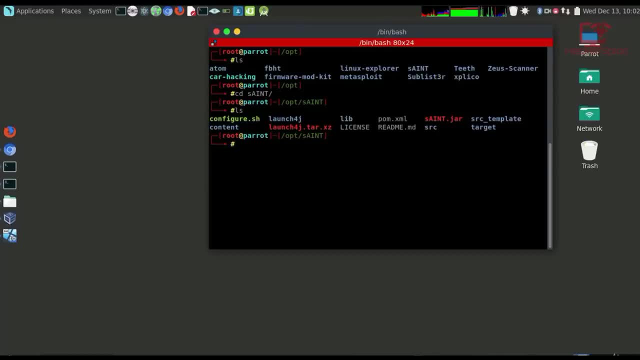 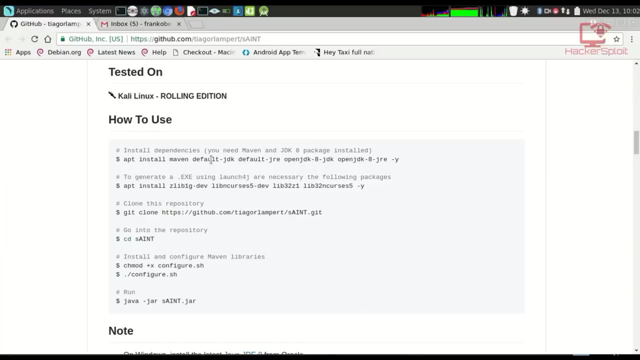 dependencies that you need to install, and one of them is the oops. let me just get that open right now. one of them is the maven libraries for the Java JDK, so it's very important that you install these maven dependencies. as you can see right here, we need the maven and JDK package installed, so maven is 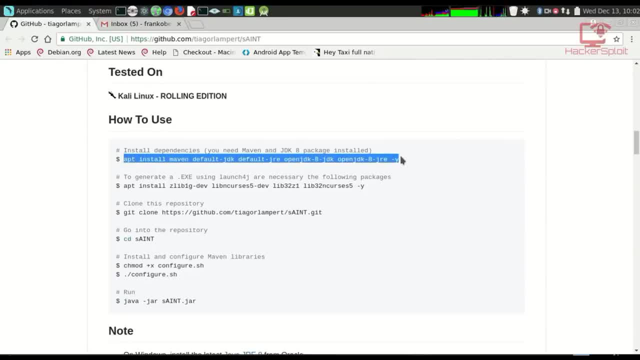 essentially library for java. so make sure, get that installed. i already have it installed. the next thing you need are the libraries that will allow you to generate an executable file, or a jar file, which is a launchable java file. all right, and once you're done, again it'll tell you to clone the repository and then you can move. 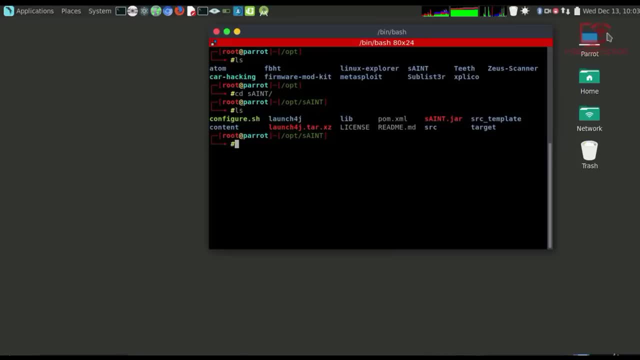 into the folder and then you change the permissions for the configuresh. all right, so we can do that right now. so chmod, whoops, chmod. uh, there we are, plus x, and uh, the configuresh. right there we are. and once that's done, you can then hit configuresh. so we can do that right now. so configure, whoops. 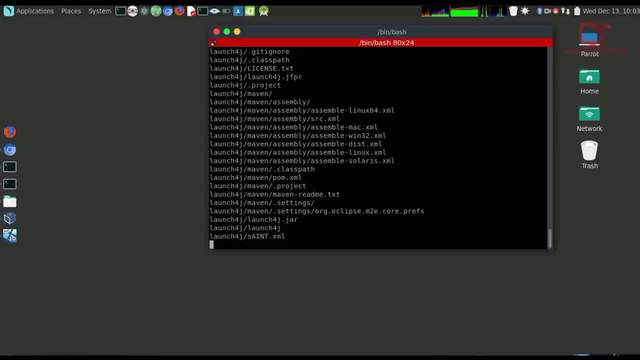 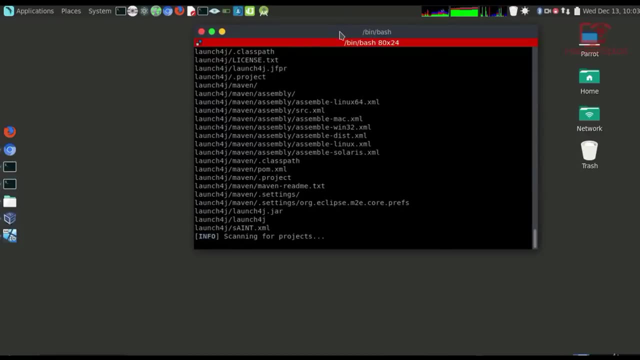 dot sh and i can run you through what. what's going to happen now? all right, so just give it a few seconds to start up. if you've installed all the dependencies, uh, you should be good and it should start up right now. okay, so give it a few seconds and what i have already. so there we are. it's going to start configuring. 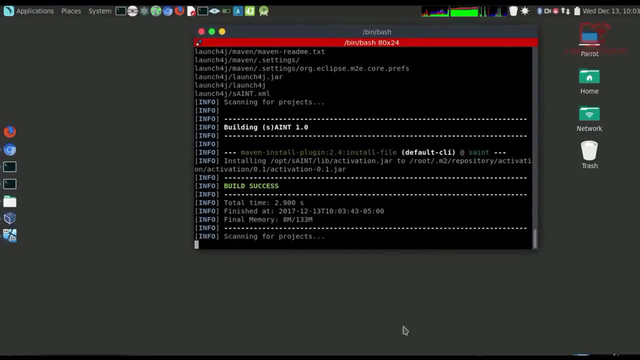 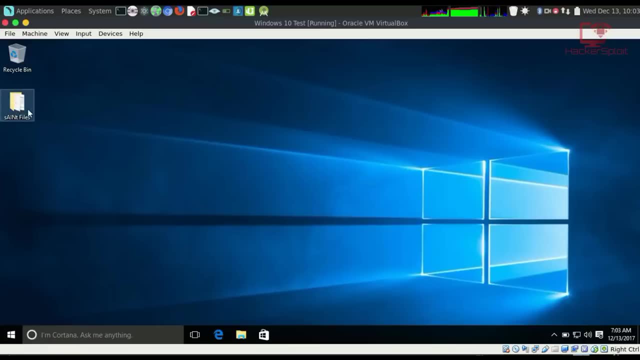 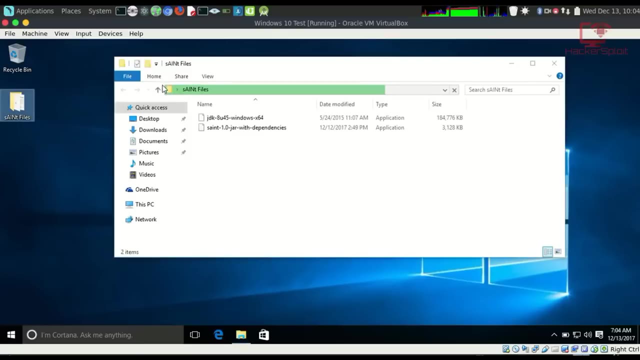 and building all that is required right now. uh, i already have my virtual machine here, my windows virtual machine, and i already generated the spyware and i've you know, i've put it on my virtual machine but i haven't ran it yet. all right, so if i let me just open the folder that contains this: 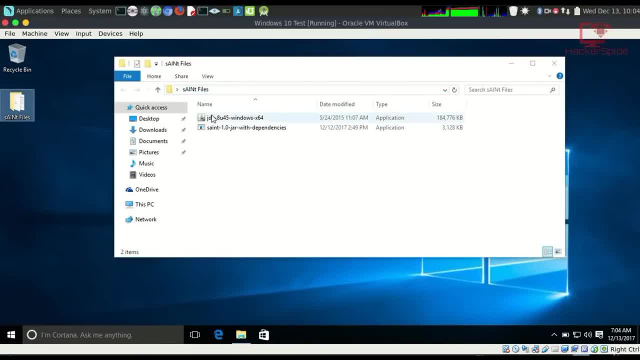 so one more important thing is to make sure that your, your target operating system, has a a version of java jdk or the Java runtime environment version 8 installed. that is very, very important and, again, it should be the appropriate version according to the process and operating system architecture: 32-bit or 64-bit. so once that's installed, let's. 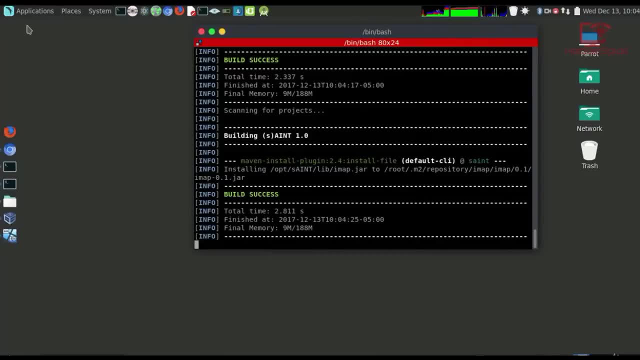 just go back to the generation here. alright. so, as you can see, it's still building the files that we require here, and just give it a few seconds again. shouldn't take too much time before we can actually get it running and we can generate our spyware. alright, so what it's doing right now is it's building. 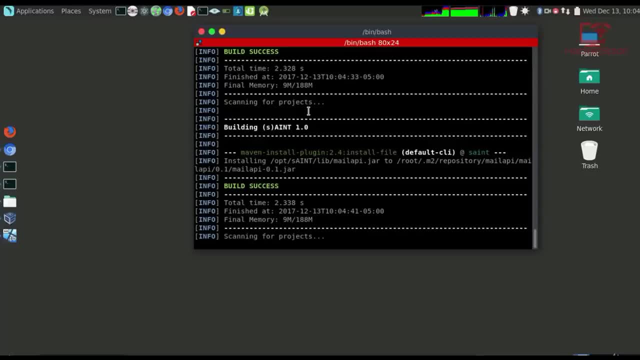 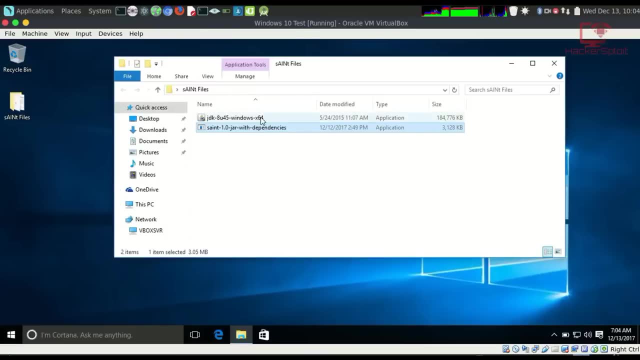 all the files required and, again, it shouldn't take too much time. it's really really fast. so, yeah, give it a few seconds and, as I was saying, make sure you have JavaJDK on your target operating system. and it's going to generate two types of files. alright, so this spyware will generate two types of files. it will 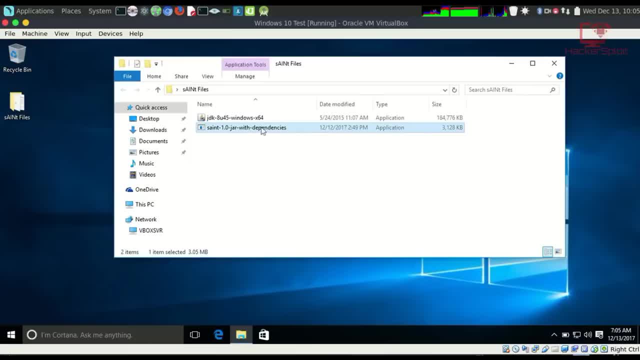 generate a executable version and the Java, the jar application- which is, again, it's up to you on what you want to do with it. you feel is more appropriate to install because, again, when it comes down to client-side attacks, it's more about social engineering. alright, so let me. 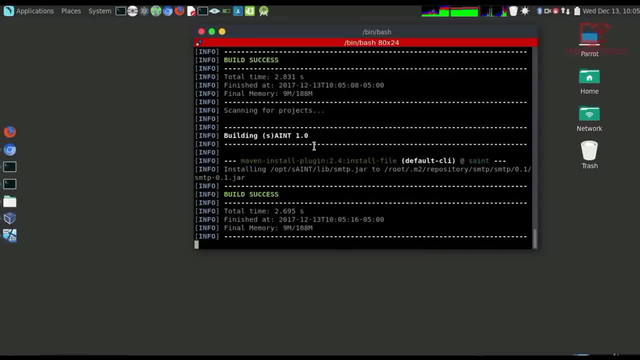 just close up my virtual machine right here and let's let's look at the process that we have here and whether or not we can speed it up again. it shouldn't take too much time, just these a few. it just has to compile a few stuff here and 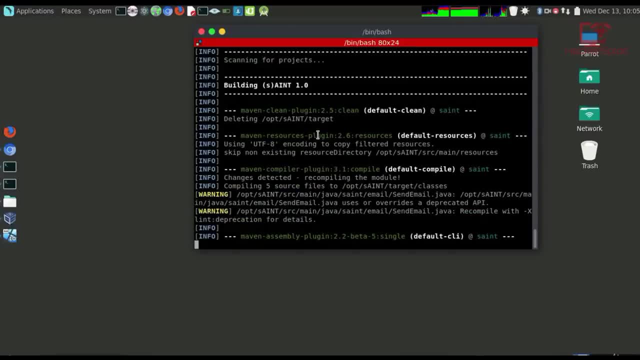 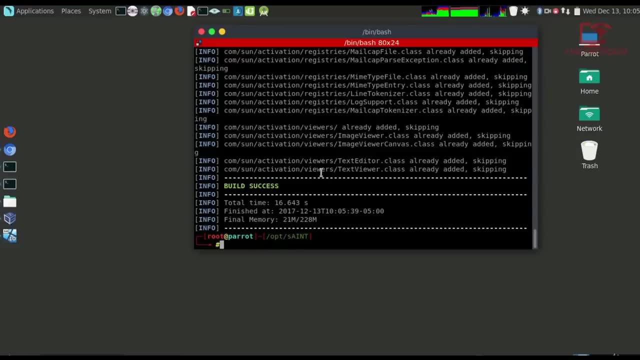 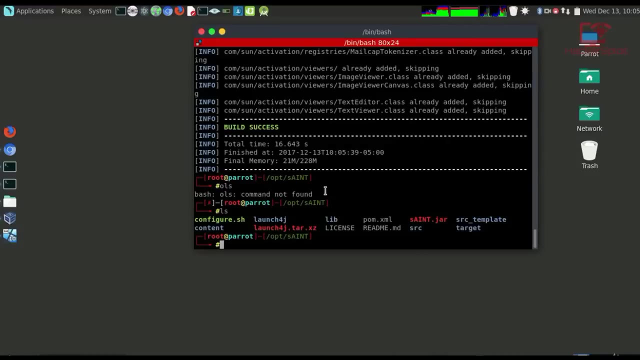 build the required libraries and the plugins. alright. so again, just let it complete and it should bring up the interface, which is a command line interface. there we are, alright. so let's list the files again, and directly here you can look inside the folder and once you've configured it, we can get started. right, so you might be asking yourself: 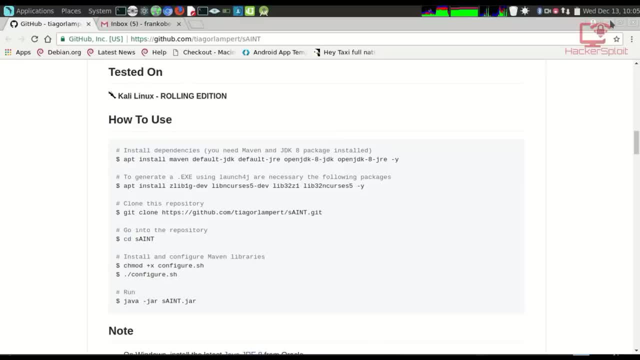 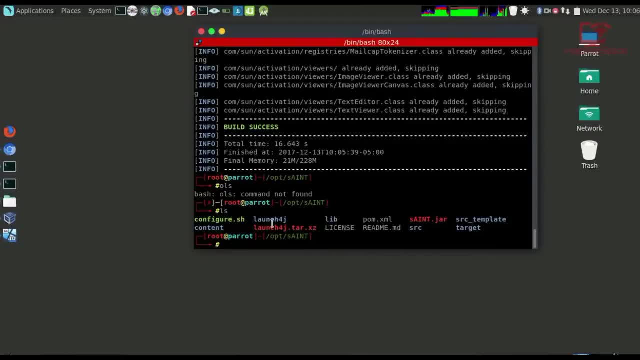 how do you get started? well, we are. as I said, you need to have Java installed, and that is on the operating system in which you're creating the spyware. so Java. we are essentially launching this right here, right. so again, if you want any help, you can check the repository and I'll give you. 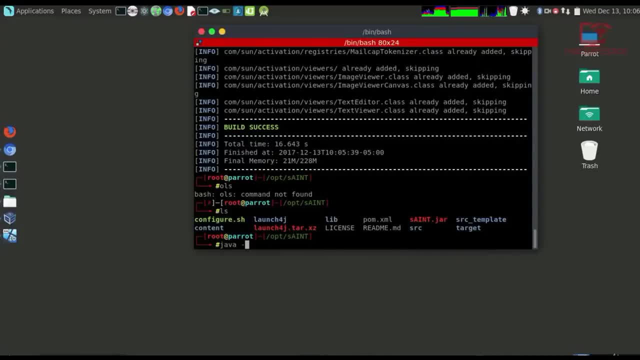 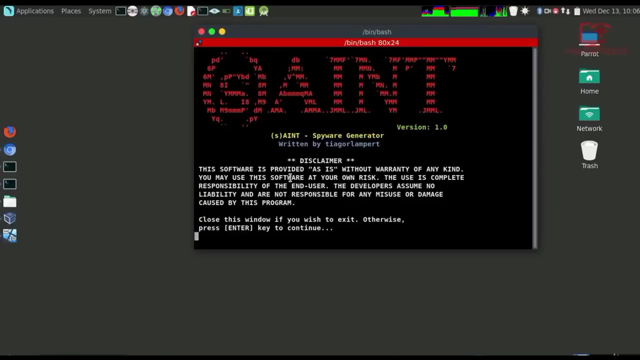 instructions. so Java jar, right. so let's Java jar. Saint oops, oh my bad, right. so Saint the jar. and we launch that. and, as you can see, it's going to say: this software is provided as is, without warranty of any kind. you may use this software at your own risk. the use is complete. the use of this is complete, you. 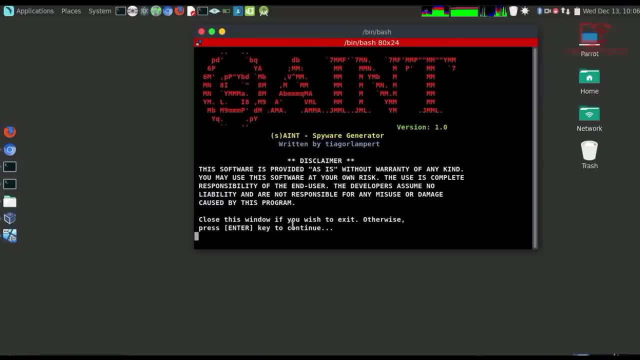 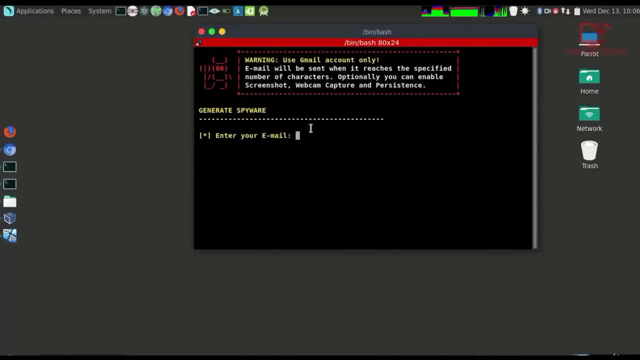 hold complete responsibility. so, again, I'm just passing off the disclaimer. all right, so once you're ready to go, just hit enter and it's gonna ask you for your Gmail. all right now, this is a very important thing. you need to create an, a gmail account where it'll send the results now. 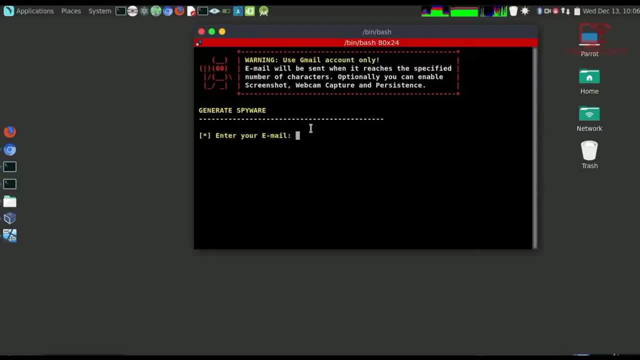 I do not recommend that you use your personal email g gmail address. if you do that, well, I think, if you just leave the video right now, if you really are thinking of doing that, so I already created my email, I've already generated the spyware, so I'm just gonna run you through how you would do it all right, so? 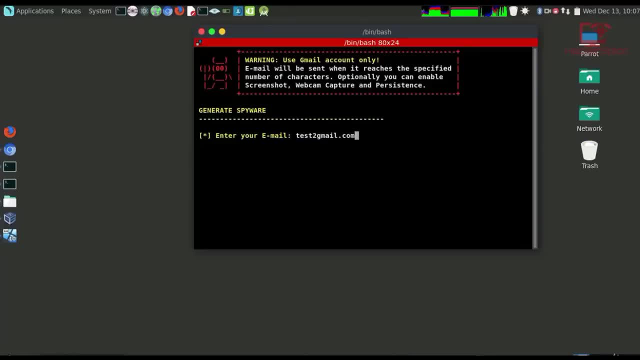 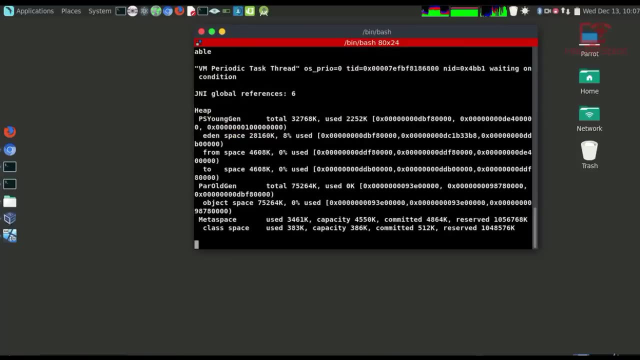 you would enter your email. so let's say: test gmailcom again, implementouverfulgmailcom chat. but let's just check and see, let's think about that and here is what you're saying from this Twitter. then you can just click: this is not my, my real email that I used. so test at gmailcom, enter your password. it could be you. 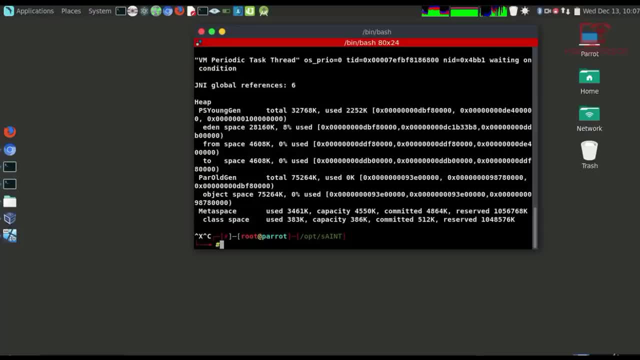 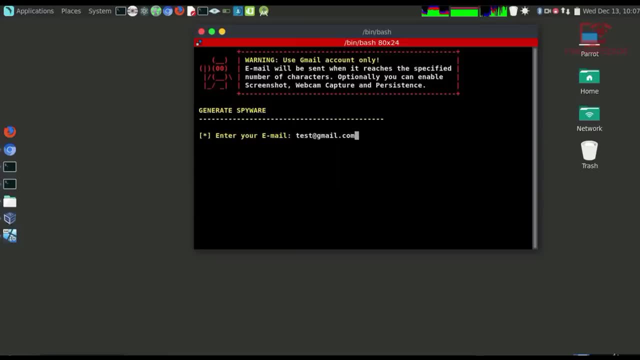 know. so oops, oops, all right. my, my bad. I think I actually just caused a bit of an overflow there, so let me run that again. so test at gmailcom, all right, and I can say: you know something really simple in integer password. and then here the options come. do you want to enable the screenshot? 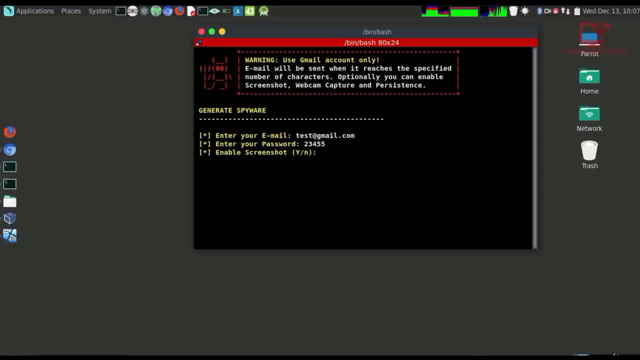 functionality, which means it will take a screenshot every few seconds and it's it'll send it to the email. yes, that is very, very handy. do you want to enable webcam? now? again, this is: it'll not work on virtual machines, which I just wanted to get out of the way, but on a real host machine. 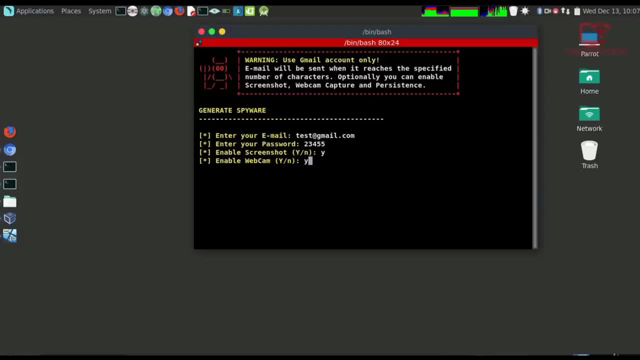 if the the target does have a webcam? yes, it could be helpful. yes, do you want to enable persistence? yes, we do. do you want to keep the data on the computer? again, something very, very important here. the thing with this spyware generator is it's going to keep the, the files that it's generating. 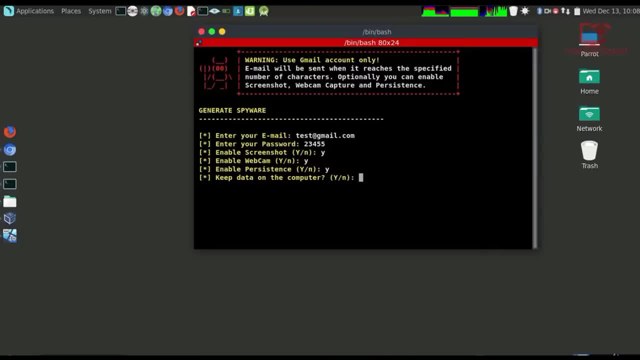 or it's or the key logged your data. it's going to all store it on the computer if you want it to so. usually it will store it in the app data folder where you can find all the files. again, it depends on your target. if your target is a text tech savvy user and knows what's going on in his or her system, it might be a good. 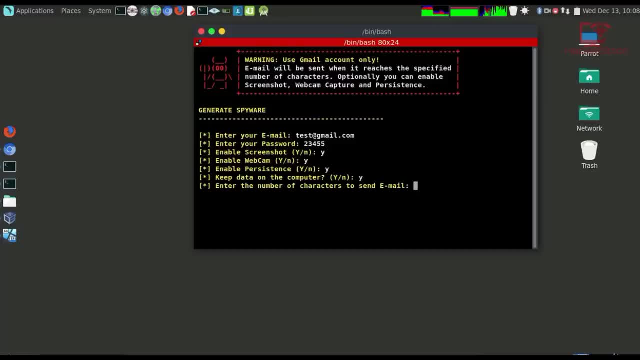 idea to say no, or you can just hit yes and once that you hate yes, it's gonna ask you enter the number of characters to send the email to all. right now. what this means is the amount of keylogger to to grab before it sends an email. so you could enter something like if you wanted to. 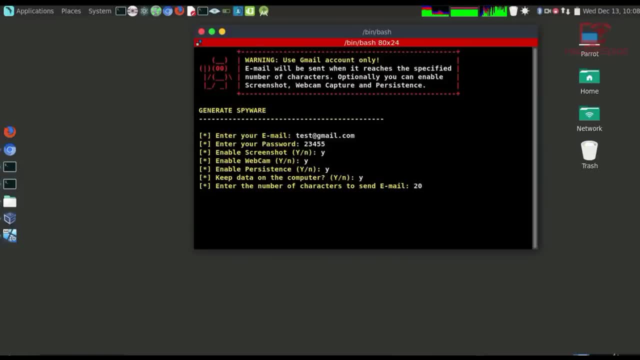 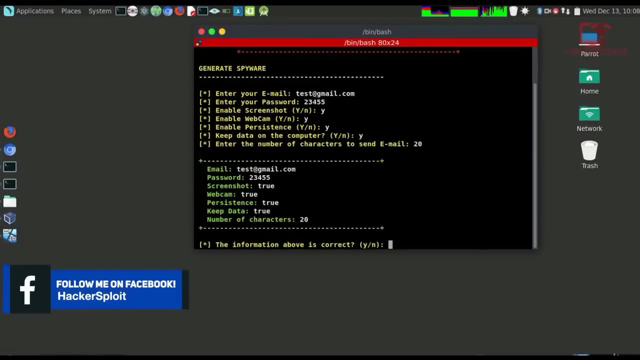 grab a lot. you can say something like 20. that's an appropriate amount because you can grab 20 key logs or keystrokes, and then you'll send all the files to the email. all right, so once you're done, just hit enter. and I don't want to create one because I already have, so I'm not gonna hit. 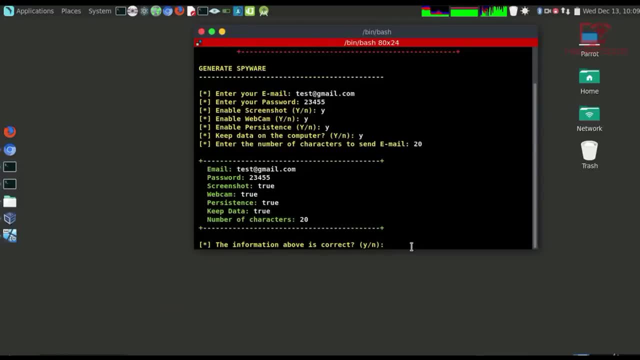 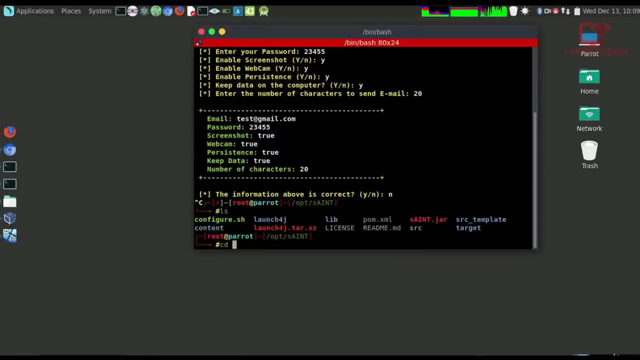 enter. so, yeah, once you, once you're done, you just have to check if the information is correct. if it um, what will do? it will store it for you. let me list the files again. it will store it, uh, in your Target, all right. so in your Target folder, right? so if we list the files right here, as you can see, 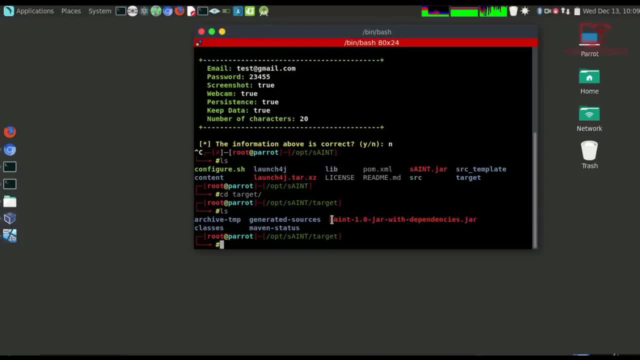 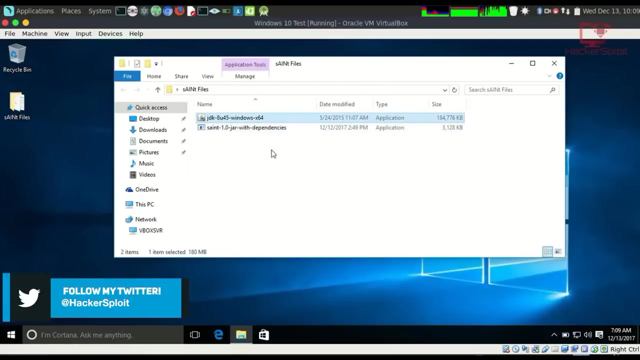 I already copied the file from there, the exe. it's going to generate a Saint, a 1.0 jar with dependencies, uh, dot jar or a dot executable, all right. so I already copied that to the virtual machine. and again, make sure your virtual machine or your target operating system is running Java or 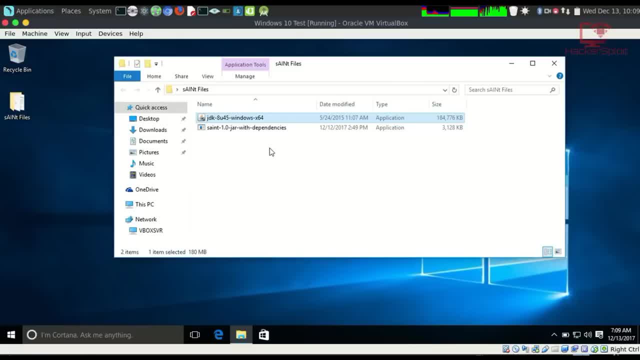 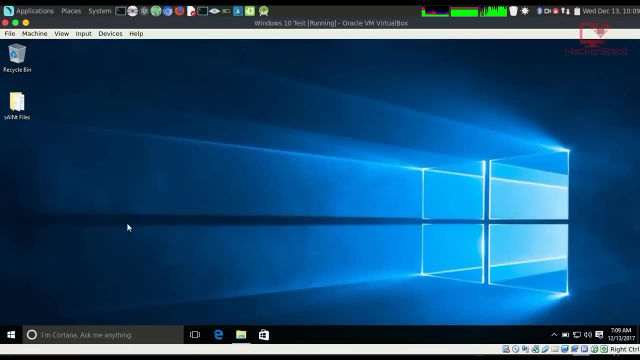 has a any version of Java 8 available, whether it's the development kit or the runtime environment, all right. so, once you're done, just hit this right here, just open up the executable. it'll not give you any graphical user interface, it'll just start up and, as I was saying, you, you, you actually have. 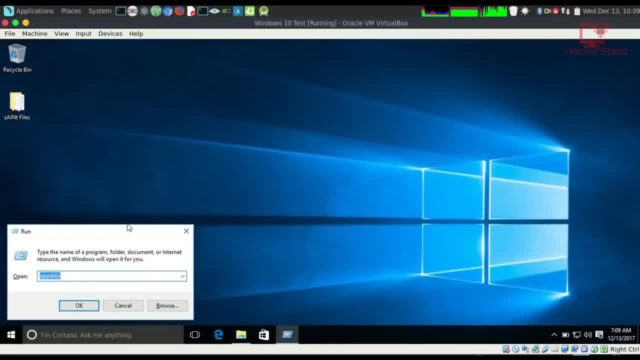 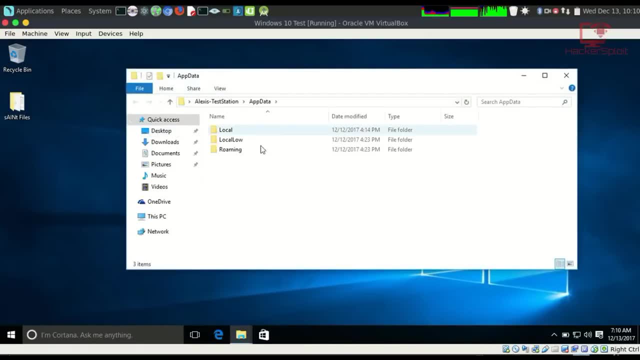 the ability to check the files, as you can see here. so it is. it is in the app data folder that that is where the files are going to be stored. if you chose that option, so let's open that right now. and you want to go to local or? 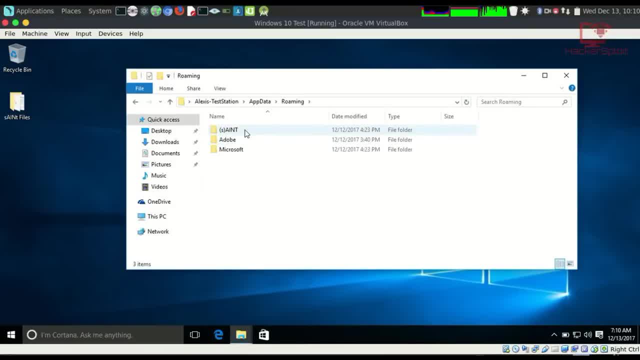 roaming. that is where it stores it most of the time. there we are. so, as you can see, it generated the folder Saint and what we can do now is, uh, let's just open up, let's type some stuff in here. so I apologize if my virtual machine is a bit slow, uh, so what we can do is we can just try and open. 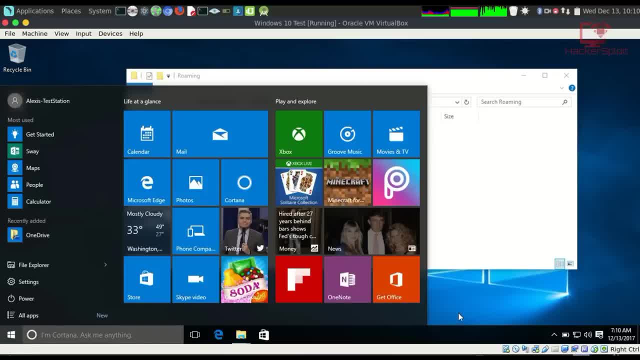 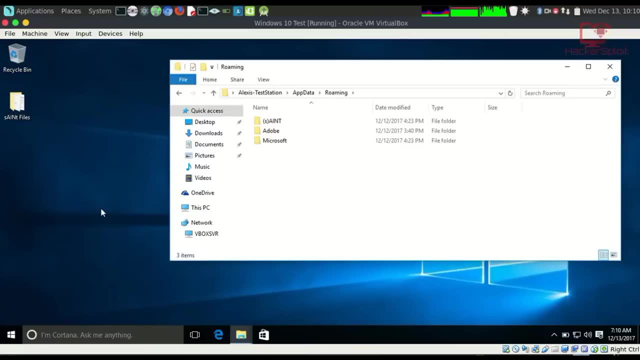 up a notepad here, if that lets us open it. I don't want this to freeze anytime soon, because I'm actually running this in quite a low resource virtualized environment, so what we can do is um, or we can just type in some random searches here. so we ran app data. uh, let's see, we've ran a. 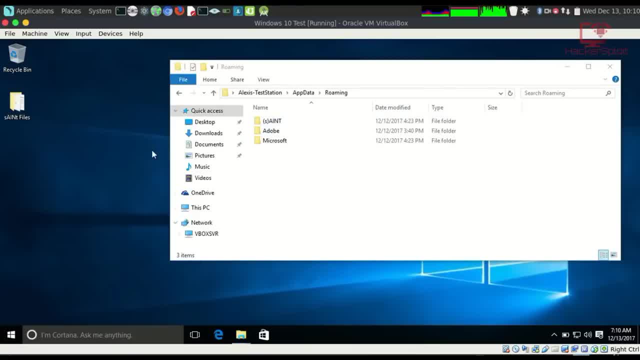 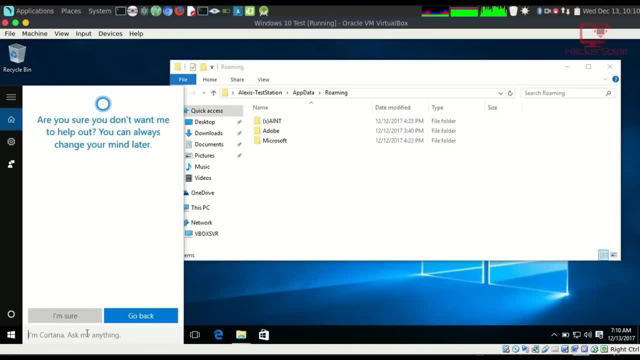 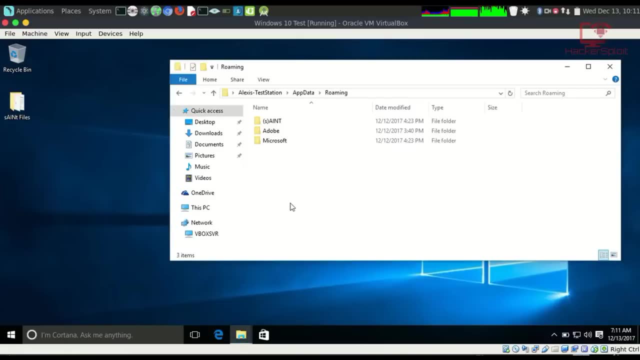 few commands there, uh, so I'll open this in a second, but first I just want to um, so I'm not interested in that. let's just type some weird stuff like email. you know what a normal person would be typing in or would be typing in some documents, and yeah, you can just enter as many keys as you want. and now, 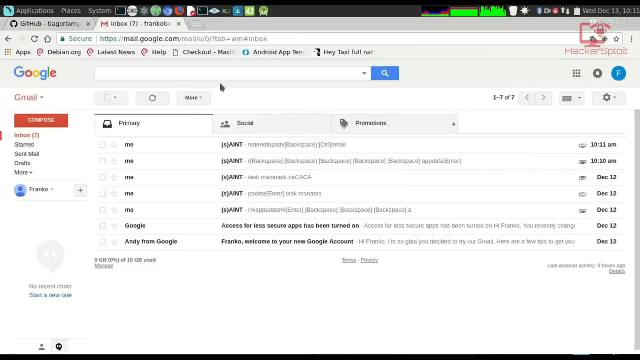 uh, the email that I used and, as you can see, yes, it has sent us stuff here, uh, so let's look what it sent now. these ones are from yesterday, when I was testing this, and these two are the latest ones. all right, and I'll show you that it does send all the files, so let's look at the latest one, all right? so 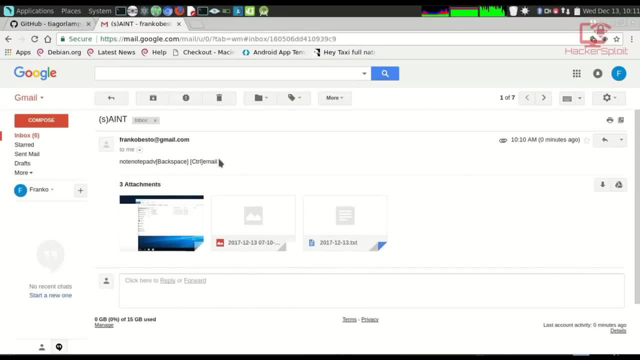 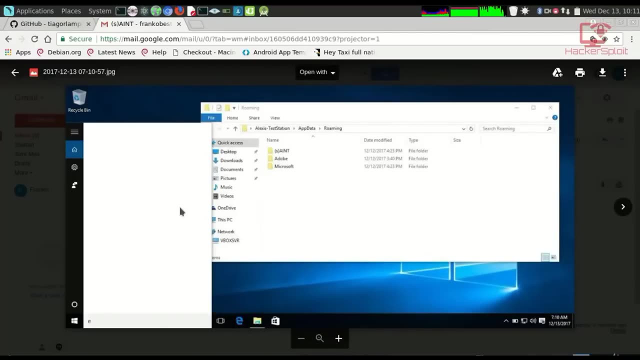 the latest one. it does send it with the the logged keystrokes. as you can see, we entered email, we hit control email, backspace notepad, and it didn't launch the notepad. how sad about that. so let's see, as you can see, it took a perfect screenshot. amazing, you know. really, really powerful. uh, let's. 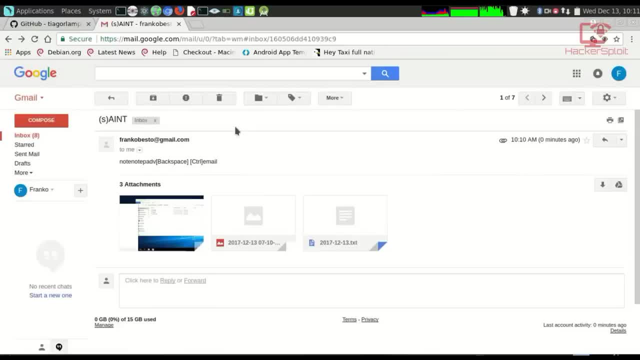 look at the next. uh, the next one is the webcam. but again, it could not take a picture of the webcam because I've disabled webcam functionality on my virtual machine and on my main operating system right now. and then it gives you the text document which is your key logged or your keystroked. 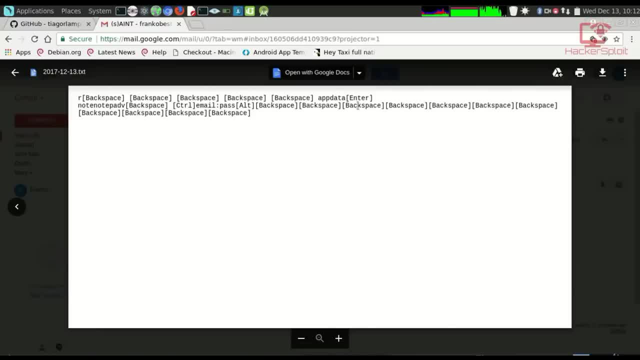 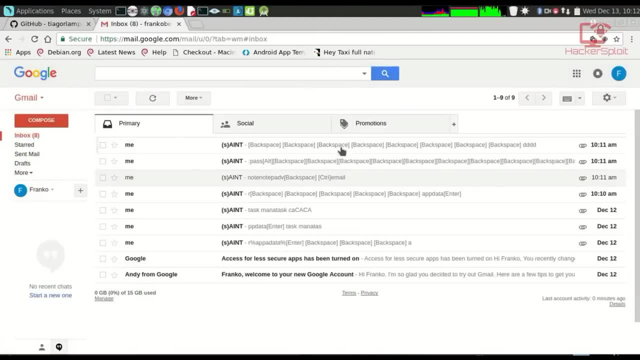 characters. so if you open that, as you can see, backspace, backspace, backspace, pardon me, notepad control email. so all that I typed is going to be sent to you. so let's go ahead and go ahead and send, all right, and, as you can see, it's gonna keep on sending it, uh, as the as time goes by. so it's. 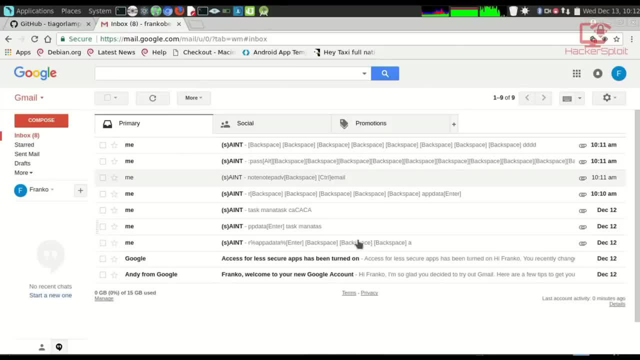 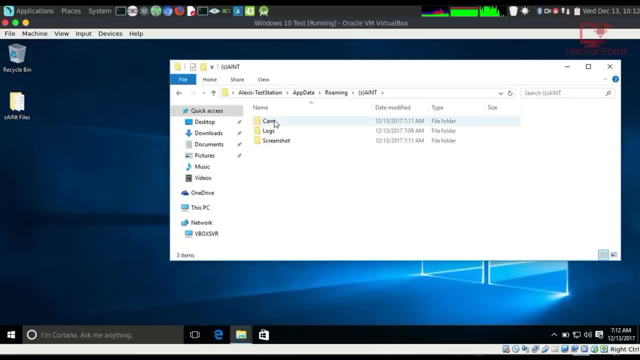 just gonna keep on flooding in. so awesome. you know it's almost like real time. uh, you know it's like a real time. uh, remote access tool or a rat, all right. so if we look on the updater folder you can see that, uh, yeah, it does store it in the cam, but again, nothing is gonna open here because I've disabled. 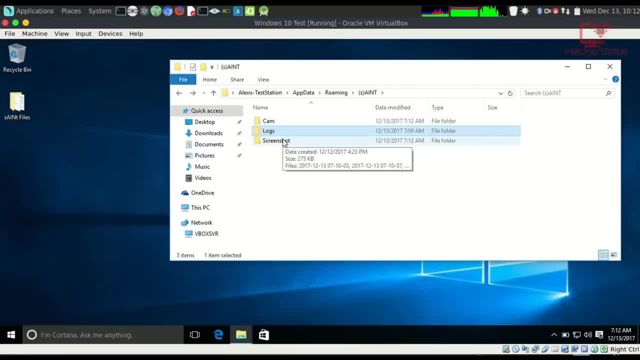 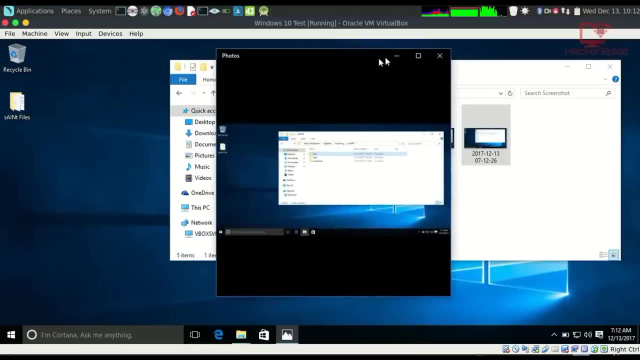 my webcam. you then have your logs, which is your key logger, or your key log strokes. you then have your screenshots, which are going to be saved in files, as you can see right here. right, so you have that, which was the latest one, and if you just open that up right now, uh, hopefully Windows, you know, doesn't let me down opening an image can. 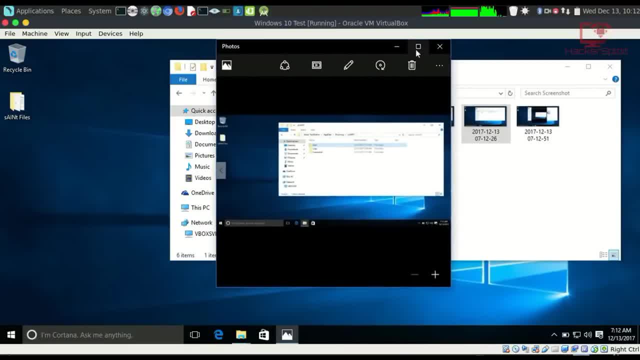 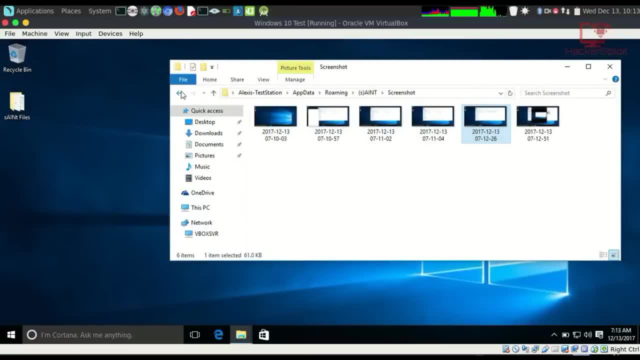 be that difficult, right? so, yeah, there we are. as you can see, you can see all the screenshots taken. and now this is. this is very important because, as I was saying, uh, if you want to keep your files on the on the host computer, uh, again, it's really up to you and you can experiment with what you like. 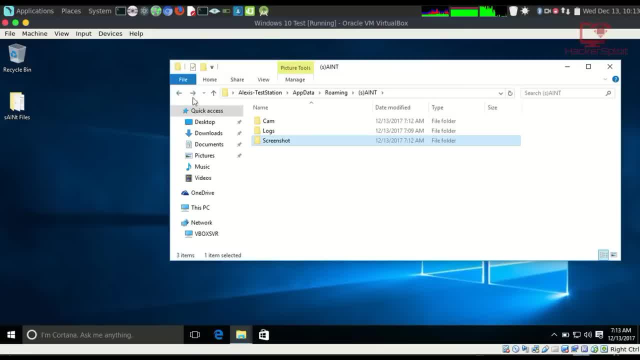 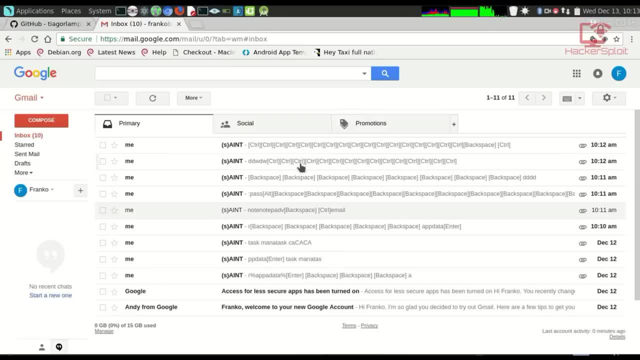 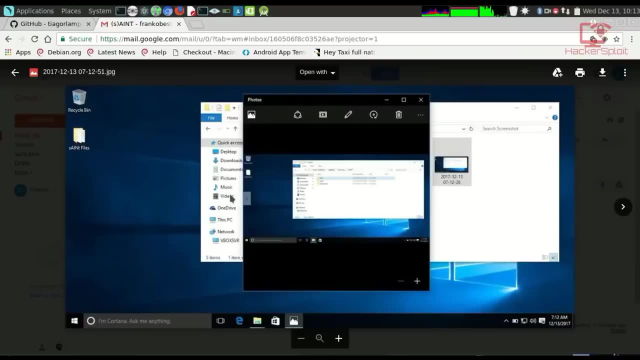 but the the real trick is using social engineering. so, yeah, that's how to use Saint and how to use it correctly. so, again, if we take a look, as you can see, it's sending all the key log keystrokes that are entered and everything is just generating and sending to me real time. as you can see, there's an image of what we just opened. 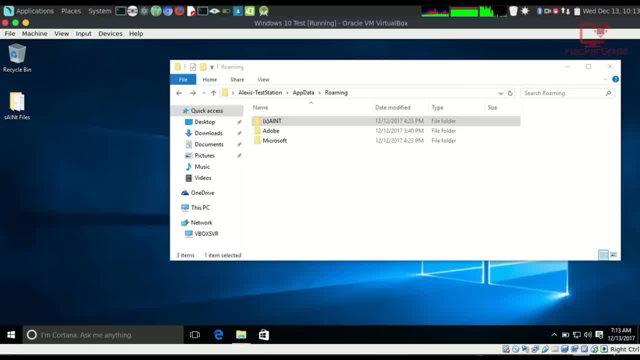 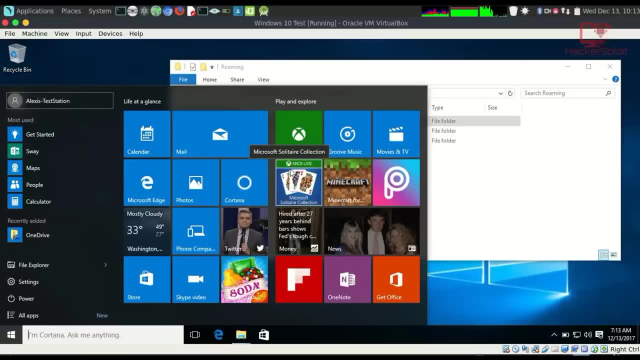 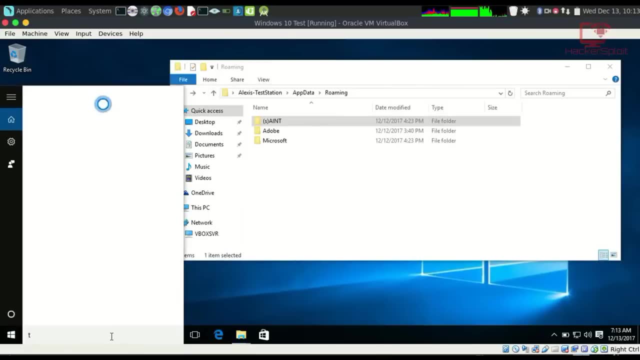 fantastic, right. so in the do know that it's working. now, if you're running this on your virtual machine, like I am, and you're wondering how the hell do we stop this, well, it's really very simple, and this is again maybe one of the disadvantages of this piece of spyware, is it? uh, you, you can actually disable it really easy, easily, or you? 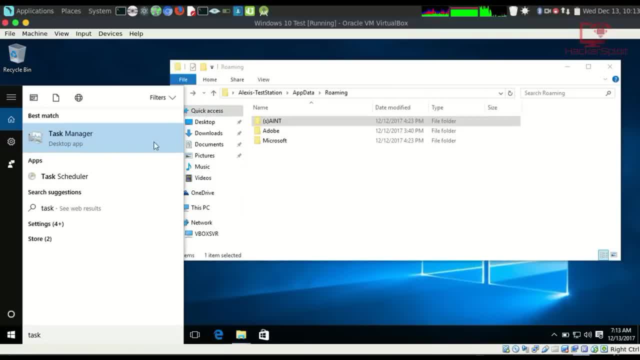 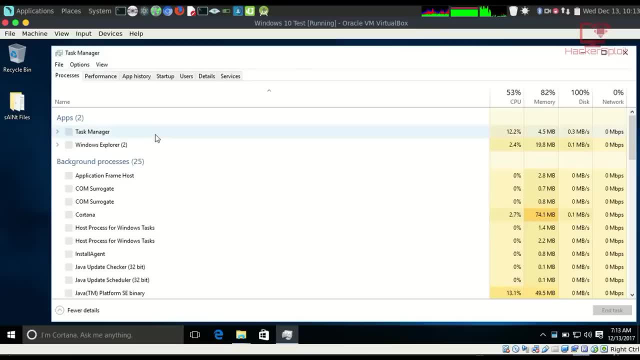 can actually find it really easily if you just open up your task manager. if you're in Windows- the default task manager that it comes with, that Windows does come with, all right. so what I'm going to do is I've just opened it up and you will see that the Java platform SE library will be open and 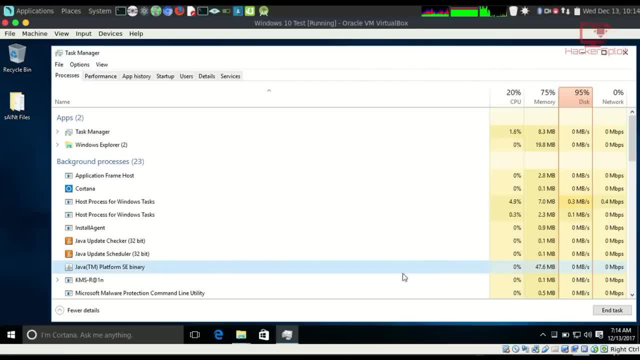 that's essentially what the the applet is running on, and if you disable this, it will immediately stop it right? so it's taking a fair bit of time to do that, so I'm going to go ahead and do that from memory. as you can see, it's taking about 46 megabytes. again, it's not the best optimized piece. 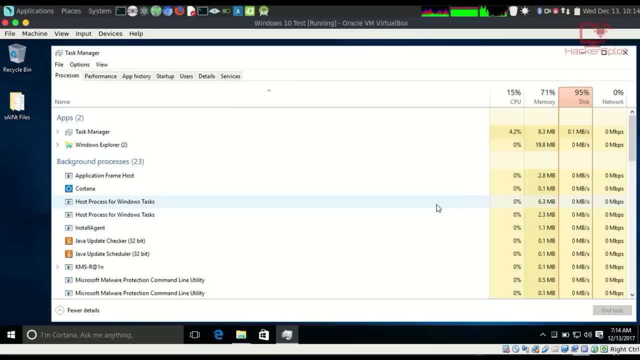 of spyware I've seen, but it's. it's really good for beginners, you know, to understand how this really works. so yeah, guys, that's it for this video. I hope you found value in this video. if you did, please leave a like down below. if you have any questions or suggestions, let me know in the comment section. 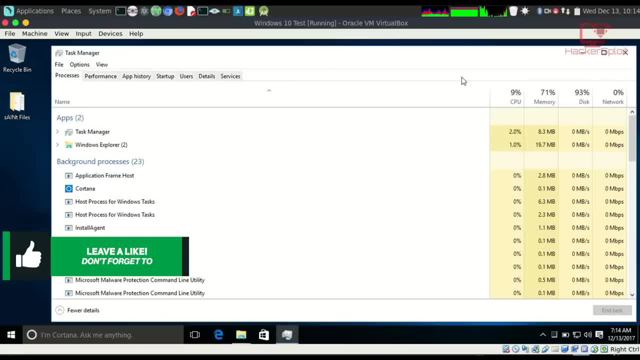 or you can hit me up on my social networks. you can also hit me up on kick and you know. if you're on the latest hacking news and resources, check out my website hsploitcom. link will be in the description and I'll be seeing you in the next video. peace. 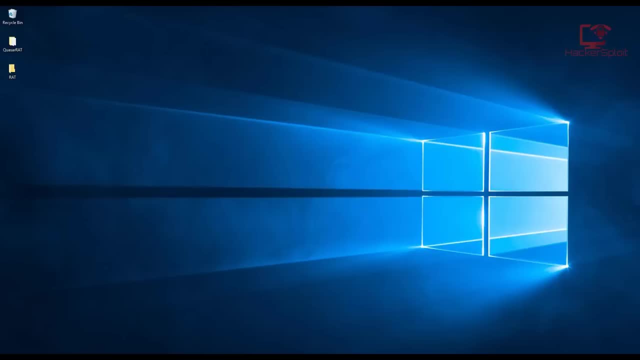 hey guys, hack exploit here back again with another video, and in this video we're going to be looking at case a rat. all right, so let's get started now. before we get started, I just want to make a quick exploit app and I have completed it now and I'm looking to get it published by 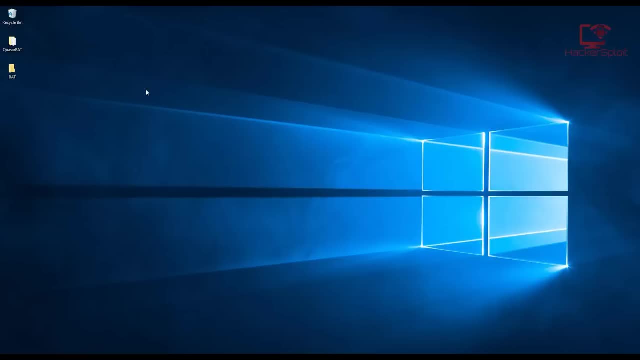 tomorrow. I had a few delays with the app and getting everything up and running, but no need to worry now. the app will be released on Monday and will be on the Play Store- the Google Play Store- by Tuesday, the latest. alright, so I'm looking to get that verified on the Google Play Store and. 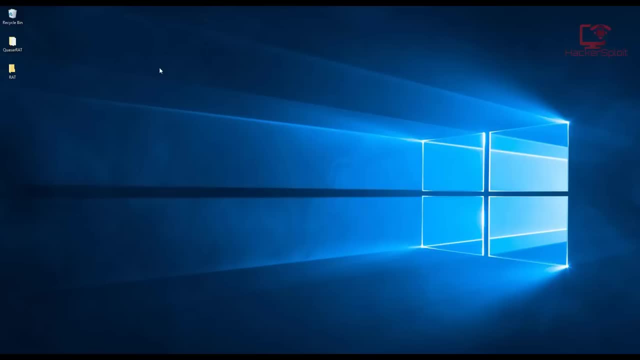 I'm going to go ahead and start the video. so, as I said, this video is about how to set up and how to use case a rat. all right, so you might be asking yourself: well, what is a rat? you could be asking yourself. so, for those of you who don't know what a rat is, a rat is essentially a remote access tool. 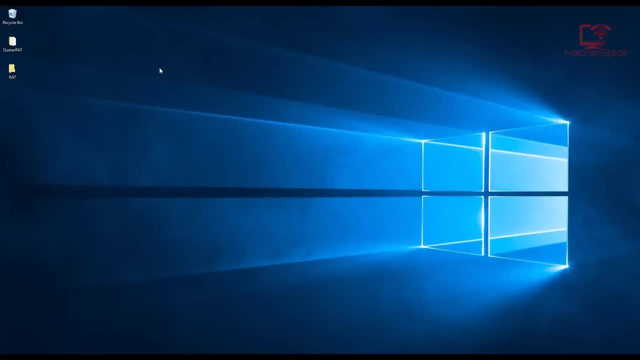 and does essentially what the name- uh, the, the name you know- describes it to do. it gives you remote access to a operating system or a computer, or even a mobile device, but in this case case a rat is a works or is made for Windows, all right, so this will give you the functionality to use it on. 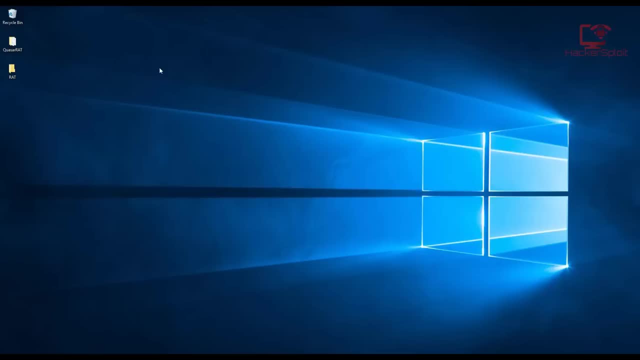 Windows. all right, so it's coded in C sharp, so that will just give it a whole lot of stability when running on Windows as an operating system. all right, so it does have a user interface and it's fantastic. right now, looking at some of the features that we have, some of the best features have to be: 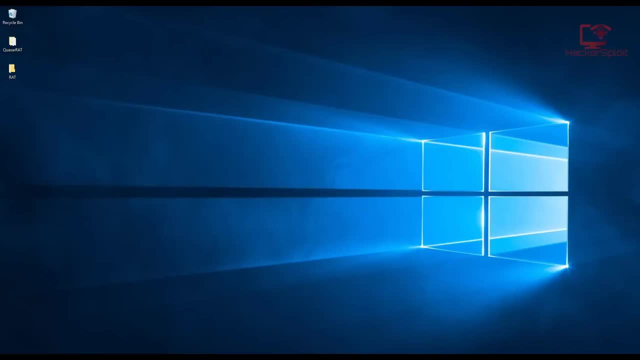 the the fact that it gives you the noipcom support, which means you can use a dynamic DNS and you, if perform your port forwarding, which is essential if you're trying to run this over. you know the internet using your public IP address. all right, so you can. uh, the other awesome features are that you 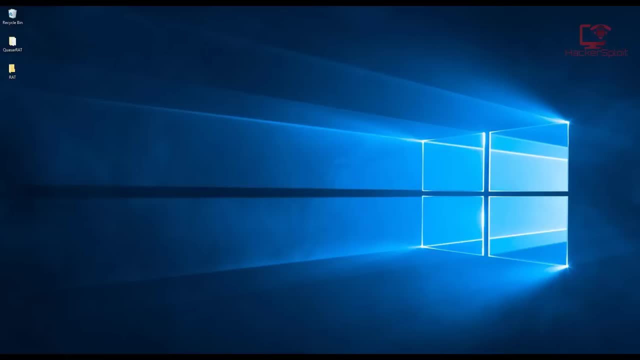 can view the task manager on the client or the targets computer. you can view the file manager. you can use the startup manager. you can perform a remote desktop connection. all right, you can perform remote webcam commands, meaning you can take pictures, record video. uh, you have the remote. 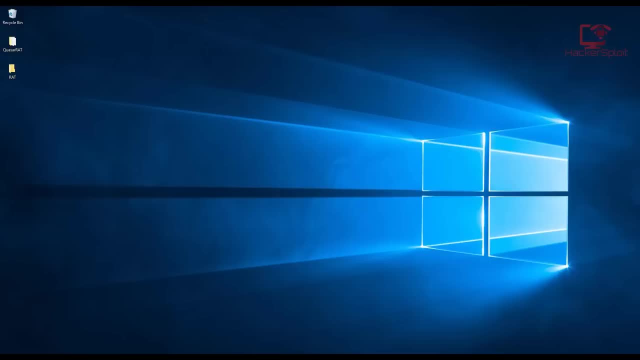 shell. you can upload and execute. you can download and execute. you have a key locker. you can perform computer commands like shutting down, a restarting and to and standby. you can use reverse proxies- all right, which means you can use reverse socks- five proxies. so if you're using proxy chains, you know you're good there and you have your registry editor now. 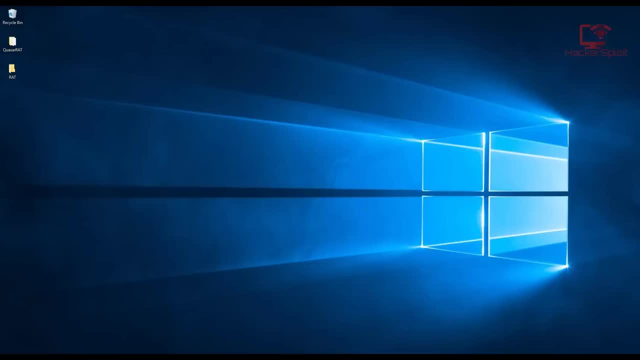 that is a lot of power. so I have to throw out caution. please, please, please, do not use this in any legal way. I have to throw their disclaimer and you know, whatever you do with it, I'm not going to be responsible because again, this is going to be. it just gives you a lot of control over you know. 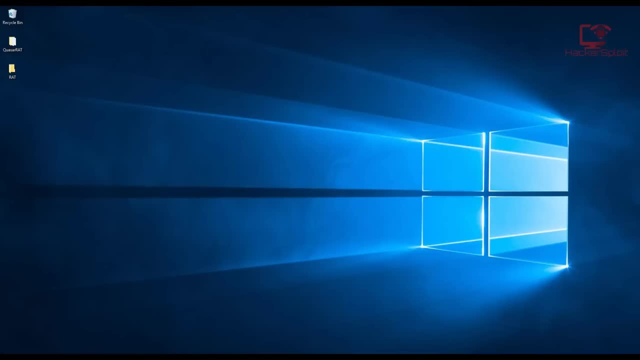 whoever's computer you try and attack. if that's what you're going to do, so again, I'm not going to be irresponsible for this. I'm just going to show you how everything works and how to get it up and running all right. so the simple requirements are: is that you need net framework installed on the 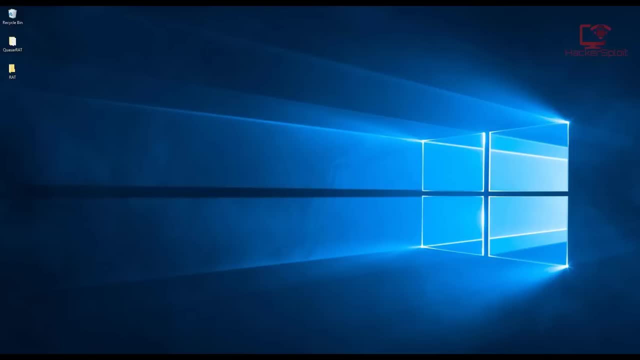 client and on, uh, on on your host operating system. right, so it does work on both 64-bit and 32-bit. you have, uh, the operating system supported our Windows XP all the way to Windows 10.. fantastic, right, so let's get started now. I have already have the GitHub repository opened up right here, so it's. 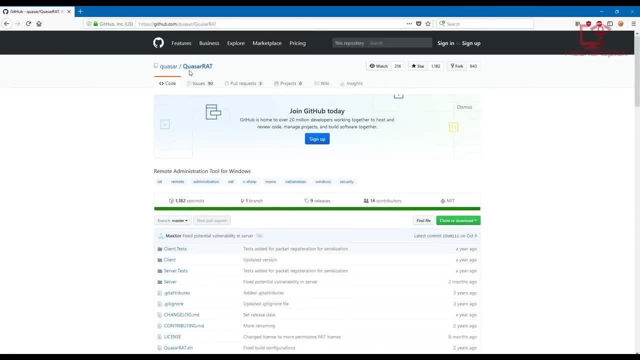 case a rat, I'm not sure if I'm pronouncing that correctly. so, again, all credits go to the uh, to the rightful author, and although you guys have been asking me, uh, why I'm doing these of these, these type of videos, and the reason why I'm doing them is the, the special tools that I'm showcasing give 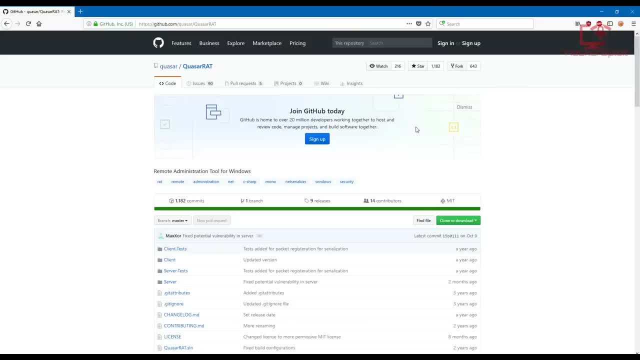 you. so, uh, essentially what I'm trying to show you here is I'm going to show you the tool and hopefully that will get your curiosity running and you'll be looking into making one of your own. so that's all I'm trying to do, right? so, and plus, this is a fantastic tool if you're using it the right. 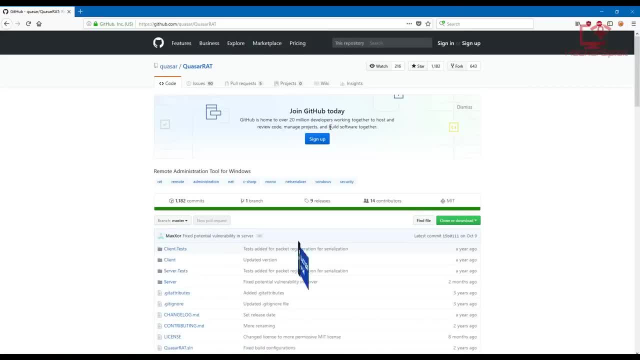 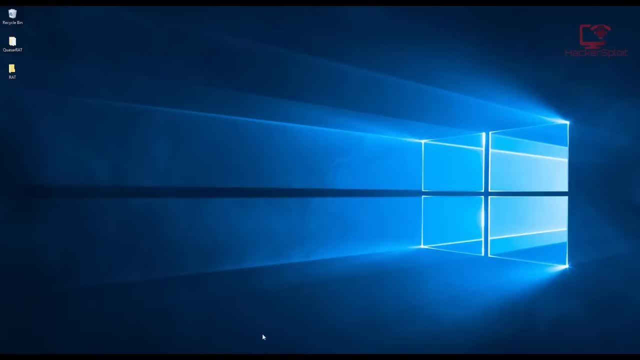 way right. so, again, it's really very simple. you can just clone the repository- and I'm going to be working on Windows, because that's what it recommends- and you need net framework. so, uh, what I'm going to do. I already have the rat installed, uh, downloaded, and 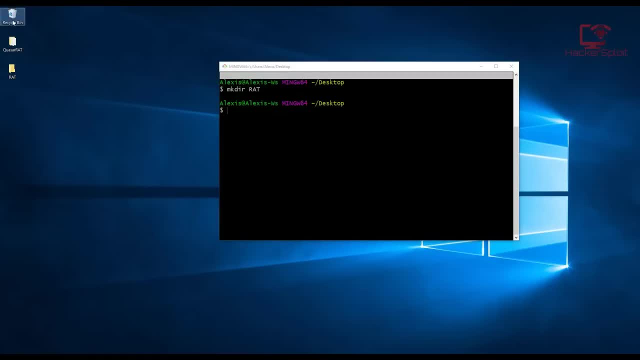 I have it set up and I'm going to be using that for demonstration, right? so what I'm going to do is I've created a rat folder on my desktop, so I'm going to save everything in the rat folder. so I'm using um, I'm using GitHub on Windows, which is, uh, it allows me to perform the clone commands, and 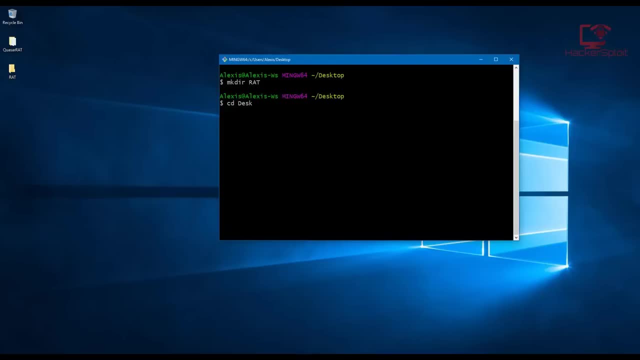 just allows me to download all the files much more easier. all right, because I use this a lot for my code management, right? so what I'm going to do is I'm going to- whoops, let me just go back here. I'm going to browse into my rat folder. you can save it on your desktop if you want to, which is: 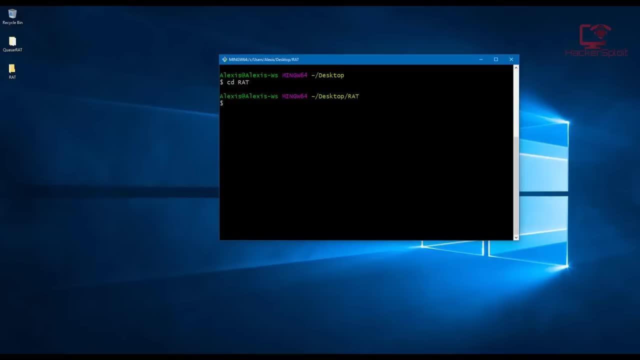 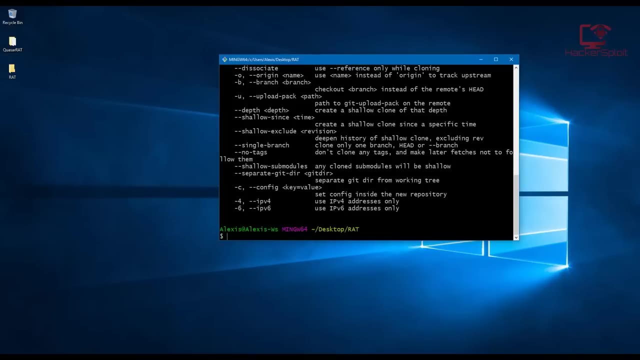 what I've done, but I'm just going to be showing you how to do it. so I'm going to say: git, clone, all right. so I'm saving everything in this file, just for the purpose of showing you how to download the files. whoops, uh, did I copy the? did I clone the repository? there we are, we've copied it. uh, let me. 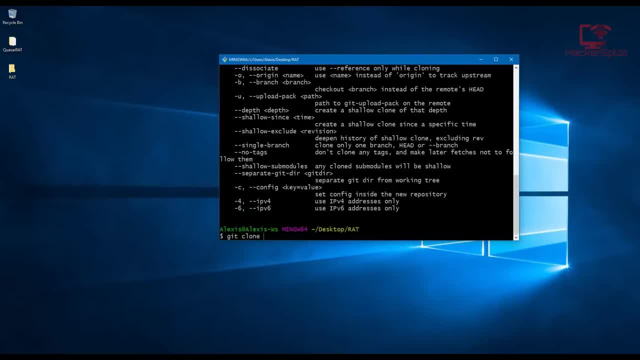 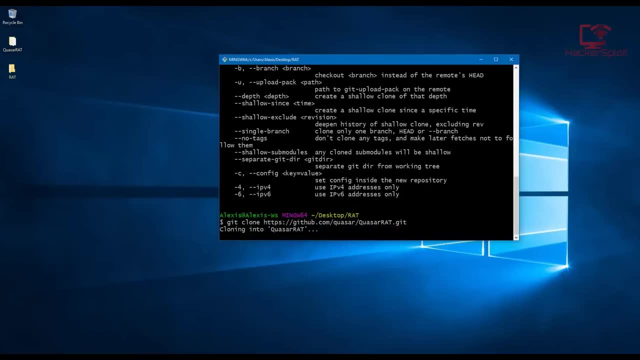 just do that again and I'll paste that in here, right? so paste that in there and I'm going to hit enter and it's going to start cloning. it's going to download the files. uh, the files are quite large. uh, a few megabytes. I'm not quite sure of the speed, so 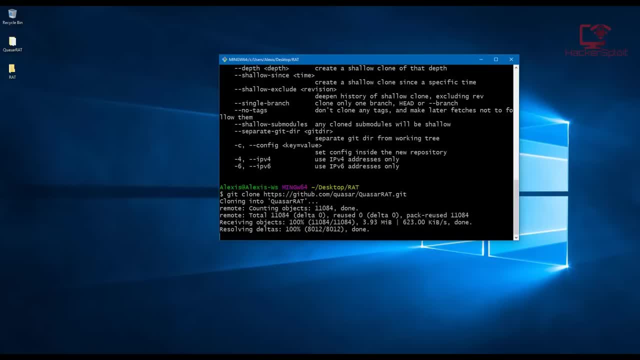 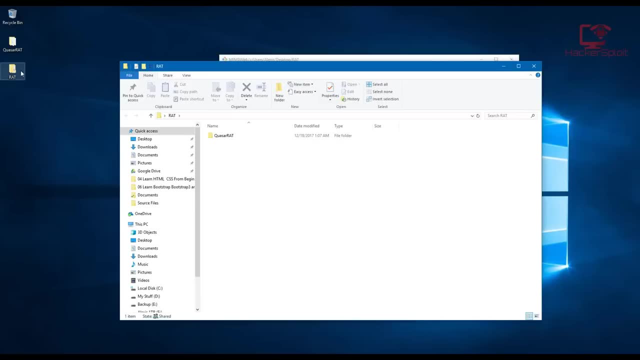 please do pardon my internet speed. it shouldn't take too much time if you have a very, very good connection. so let's open up the folder that we saved all the files, into which is the rat and, as you can see, case a rat. all right. now, when you open this, you might be a little confused. all right, so 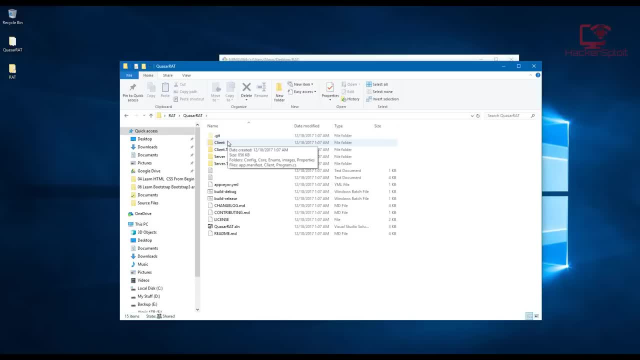 don't be confused. it's really really very simple. you have two options of building the. you have two options for this matter. you can, uh, use the Visual Studio solution file right here, which allows you to open the project in Visual Studio and to compile it or to build it, all right. so if you're looking, 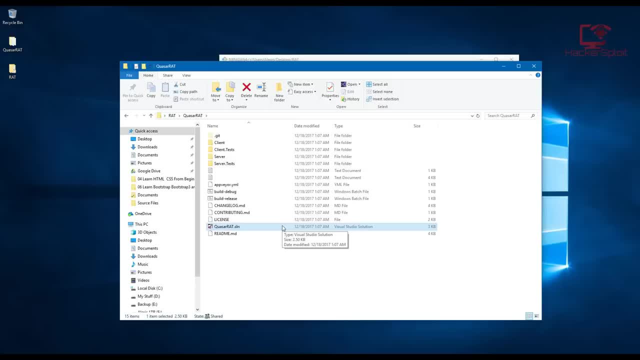 at. if you want to look at how that code works, you can again look at that and you can, you know, perform some reverse engineering as to how it works, and you can learn a lot really by by doing that. but uh, we're not going to do that because I want to. I want to really show you how it's done. 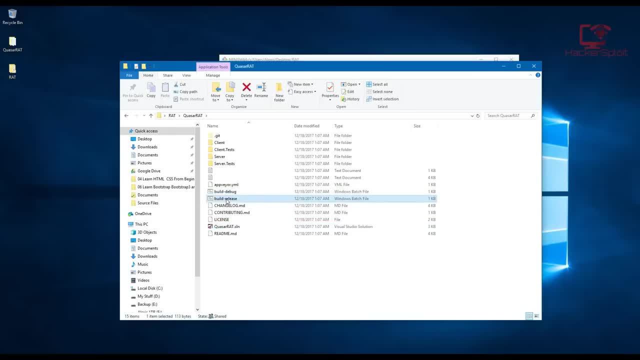 debug any of your release. so obviously we want to run the release because, again, that is the release version. the debug version won't allow us to use everything, so you just want to open that up and it's going to start building the release version. give it a few seconds. it shouldn't take too much. 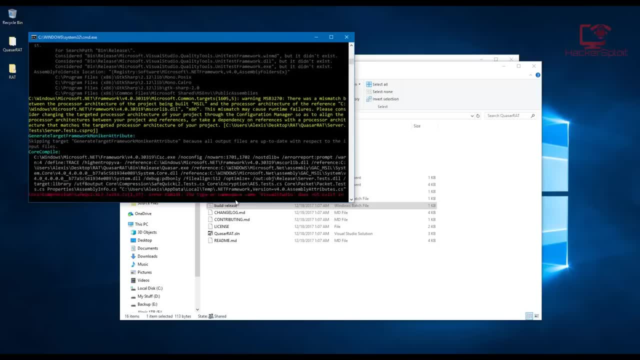 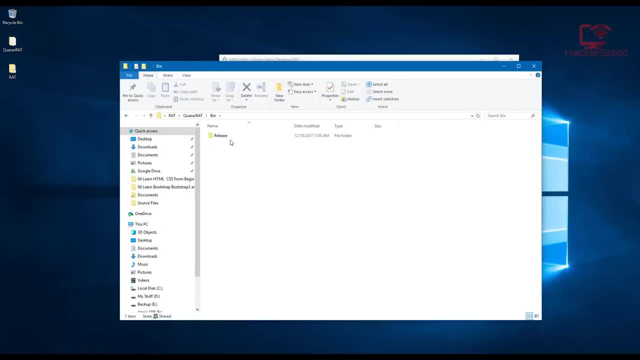 time. it shouldn't take any time at all, don't worry. it gives you a few errors, don't worry about that, and it's going to build everything into the bin folder, all right. so enter the bin folder and enter the release folder, and there we are. that's your executable rat folder, your rat file, all right? so 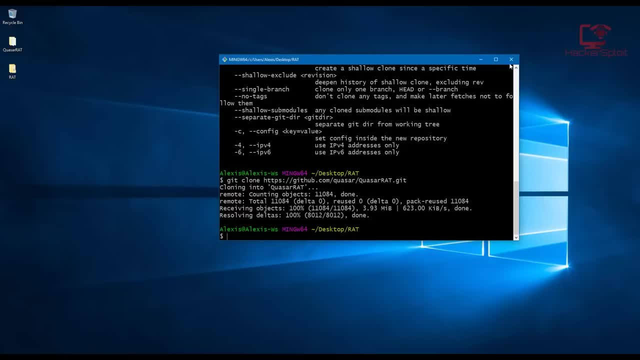 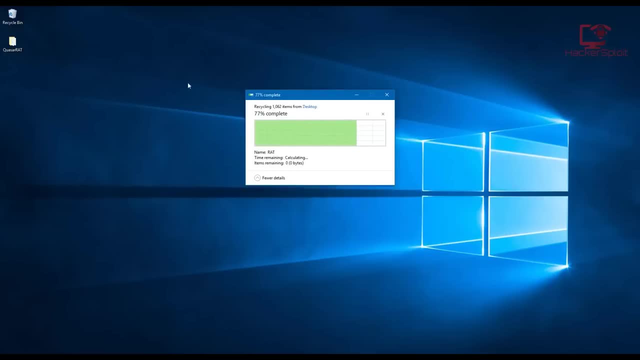 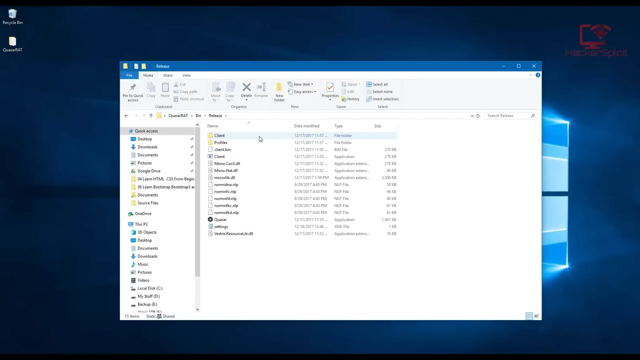 I'm going to close that up and, since I already have it downloaded, what I'm going to do now is I'm going to delete that because, as I said, I've already downloaded all of that, and I'm going to open up my folder, which I already created, and I'm going to go into my release. right, and I already created the the. 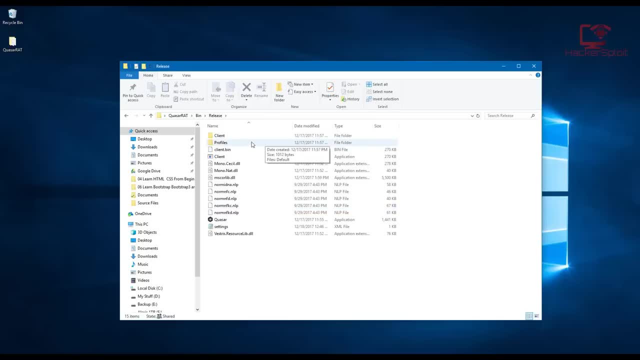 remote access tool, and I've already logged it onto my other Windows computer on my network and I'll show you that it does work. but I'm going to blur out some of the information for my privacy as well, so I'm just letting you guys know that. 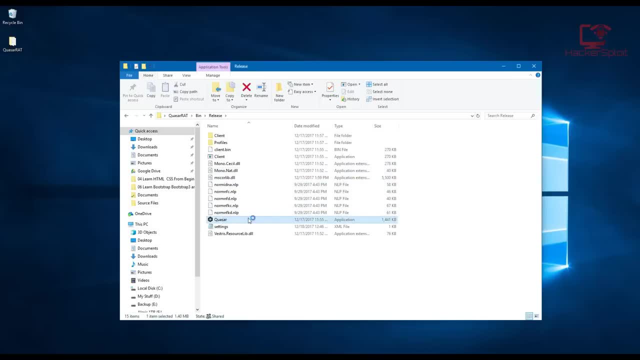 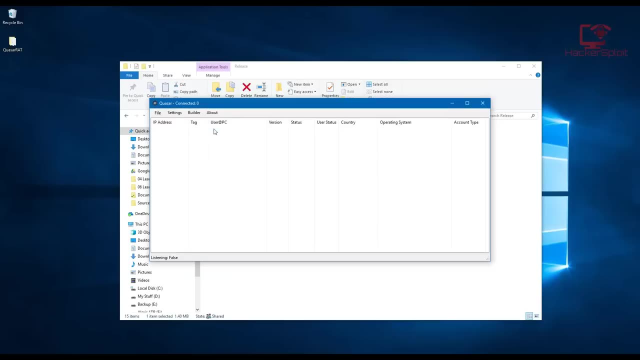 so once you open up Kesa, to just open up like that, and as you can see, right now we have nothing because I'm not connected that computer to the network yet and that's because I want to just showcase how to run this. all right. so the first thing is to let's look at the file and that's. 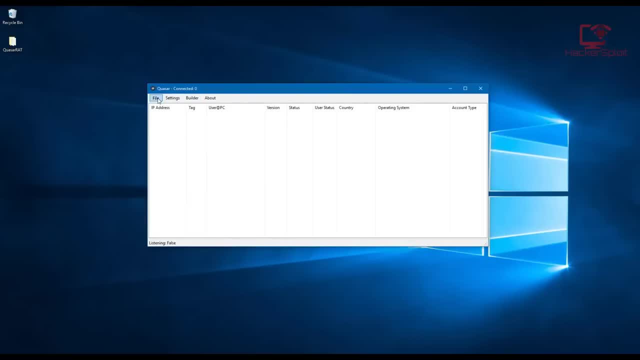 pretty simple. it allows you to close it. so that way it's really really simple, right, and in here you have your all. you have your computers or your clients that are going to be connected. so, as you can see, they are sorted into IP addresses. you have your tag, your user, PC, which is the name, the version. 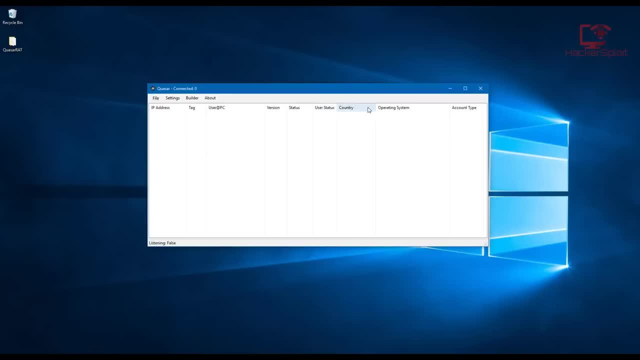 status, user status, the country they're in, the operating system they're running and the account type: all right. account type being administrator or UAC: all right. in the settings we have something very, very interesting. you can set the port you want to listen to. I recommend just using the default port that they give you. it's really not, uh, you know the best thing to. 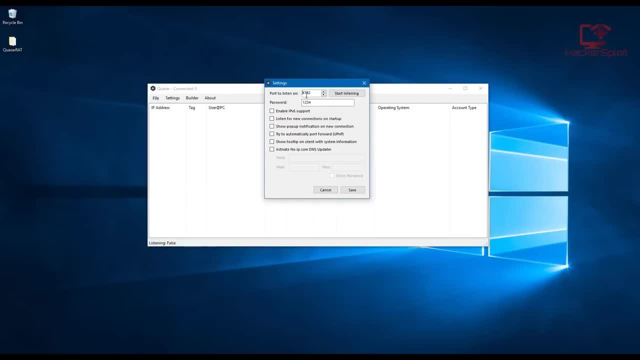 uh, to change the ports. and then you know, make a mistake when building the file and you know you're listening on a different port, right, so leave this on the defaults again. you can whatever you feel like. if you're confident in doing that, you have your ipv6 support, you can. 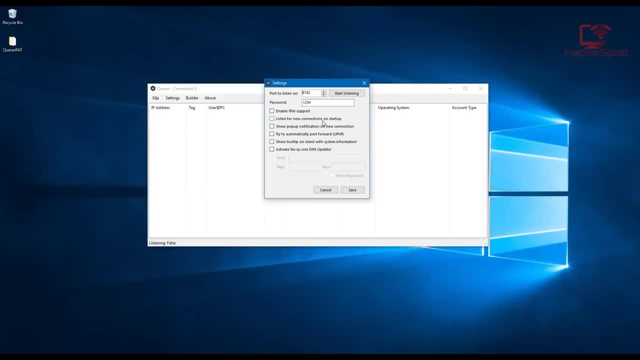 listen for new connections on startup. so that's, if you want to run this as soon as you start up your computer, you can try and port forward. also very, very important: you can also activate the no ip dns updater. i told you about that, which is really really important, or one of the best. 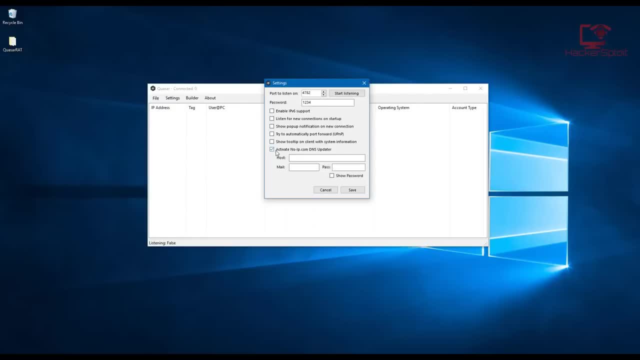 services when running a remote access tool over the internet. what i mean is, if you're connecting using your public ip, you're trying to create the reverse connection right, because that's how a remote access tool works. you're not using the target's ip, you're using your ip, so it's very. 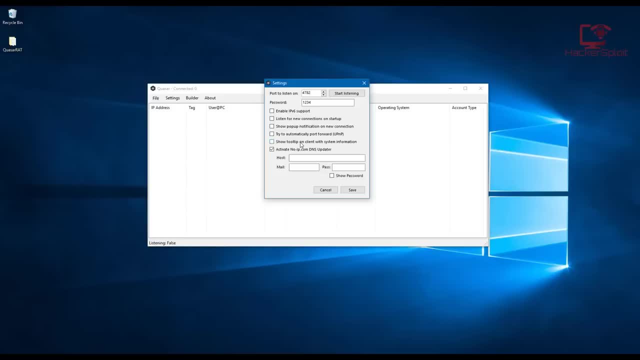 very good or important to shield your ip in case the person finds out and is able to reverse engineer that and find out what ip or what is the going, the outgoing connection right, whether or not it's coming through a port that is not listened to. uh, you know, i hope you get the idea. so we're not going. 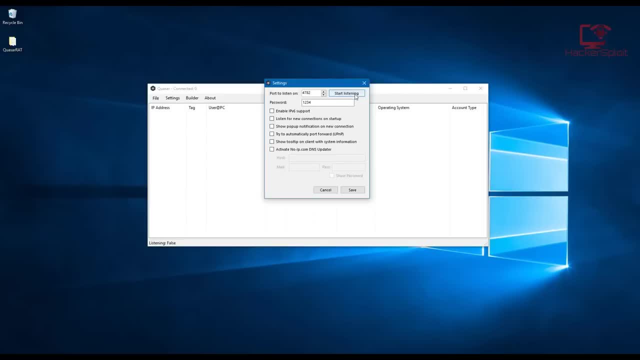 to do that because i'm going to be demonstrating this on my network. again, this is my lab, i run this lab and that means that everything is going to be running on my network. so i'm going to be running on my computer. i'm not hacking someone else's computer. so for those of you asking why, 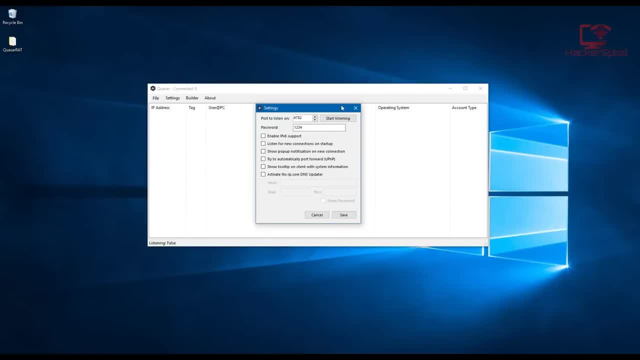 my youtube channel is isn't getting copyright strikes. it's because everything is running in my lab and i'm doing it in an ethical way, right? so i'm going to close that up and we're going to go to the builder section now. now, this is very, very important right here, right? so, as you can see, 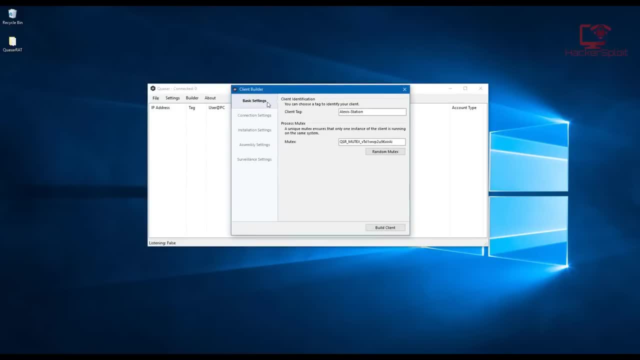 we have the basic settings first. now in here you can select your client tag, and that's the, the name of the client that you want to specify. so let's say, if you had a computer, uh, this is just the name that you want to give to the computer you're going to be listening to, right? you then have your process, mutex, and this is 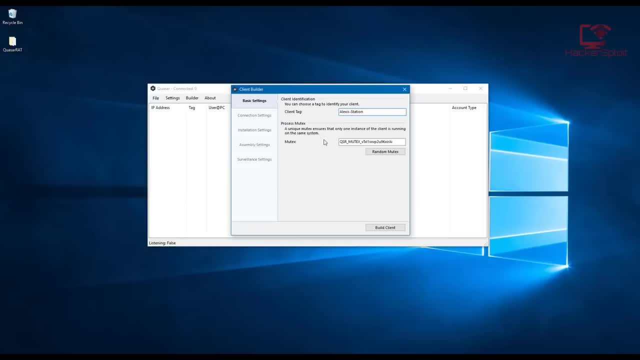 something i wouldn't recommend, uh, you to touch if you don't know what it really means. this is a. this is really when it comes down into understanding the process management in a computer and how windows handles it. so if you're, if you have understood how that works, you'll understand. 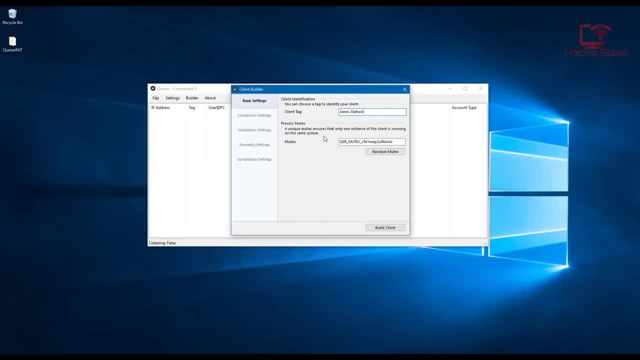 what a mutex is. so, as it says, a unique mutex ensures that only one instance of a client is running on the same system. this just means that you can only run the. the rat is running on one instance on that system instead of it running multiple times and giving you multiple instances, right, uh? so let's look at the connection. 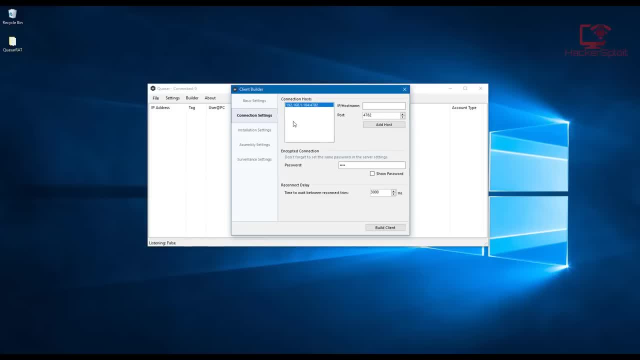 settings now. now again, as you can see, i'm running this on my local network and i've already set this computer, my host computer. i've set the local ip address and it's listening on that port. to do that, just enter it here. it's important you need to, otherwise you're not going to get any connection. 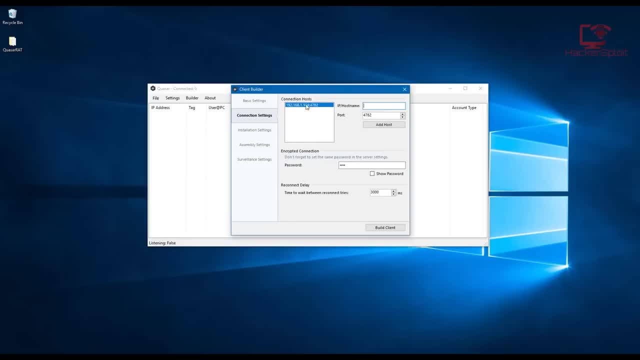 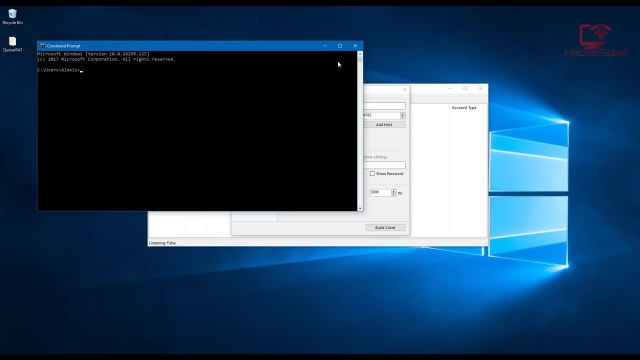 when you create the file. so if you're a local computer you're going to have to set the local network. uh, you want to select, uh, this ip networks. uh, you know ip address, this computer's ip address, local ip address. again, if you're trying to do it the public ip way, i'm sure you know how to do that. 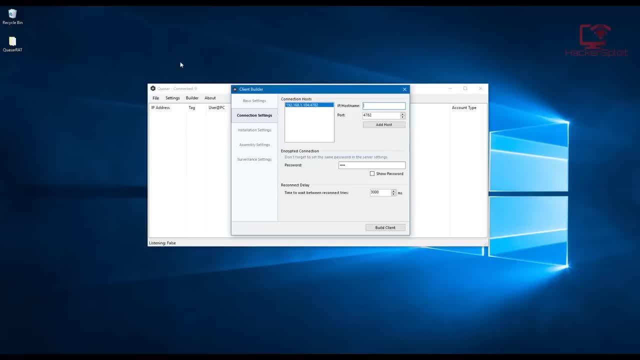 as well. but again, if you're going to do that, i highly recommend that you use a dynamic dns. okay, so once you've added you, may you have to make sure that this port is the same as the one you're going to be listening on. very, very important, and this is for your encrypted connection. 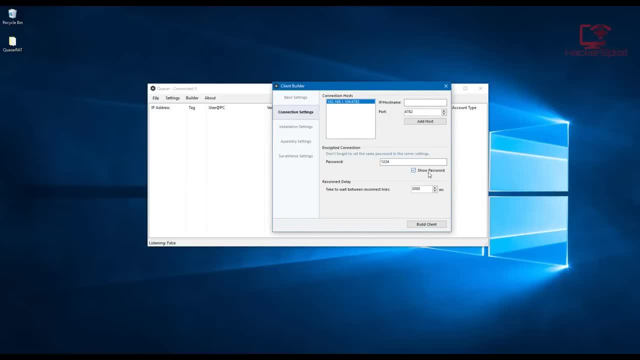 so let's leave that as default. the password is one, two, three, four. you can change that if you're interested in doing that. the installation settings: very, very important now. now, this is where social engineering comes into place, a little bit right. so your installation settings, you know, depending on your target, whether or not they are tech savvy or they understand how. 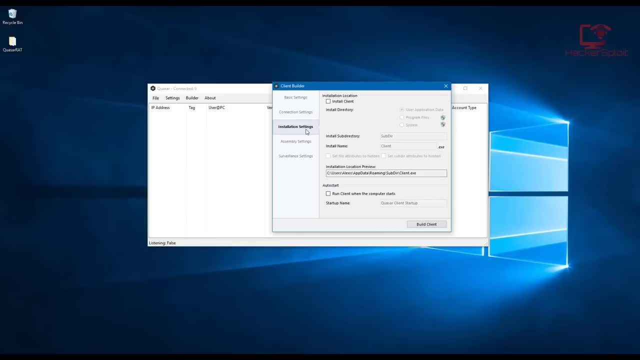 processes work in windows and whether or not they- uh, you know whether or not they understand what's going on in these systems and, like normal users who don't really understand, you know what. what the task manager is about: where you install. it is very, very important because, again, if a user is snooping around, 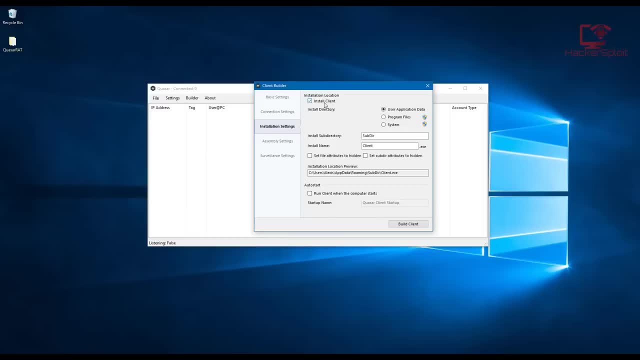 their- you know their- system files and they find this weird name- you know that's currently running. and, for example, if they perform a netstat command and they see that there's outgoing traffic to a, you know you're using a very weird port, as you just as I just showed you right there they're. 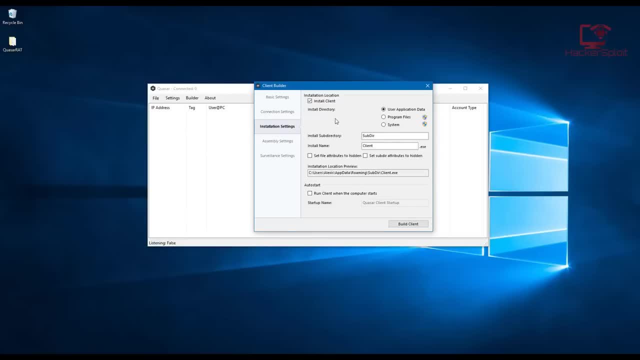 gonna get suspicious. so you can choose to install the client, which is. I would recommend that, but you have to be really, really smart about how you name the file and, uh, in what sub directory and directory you install it in. for me, the best place to install it in is the system folder, because 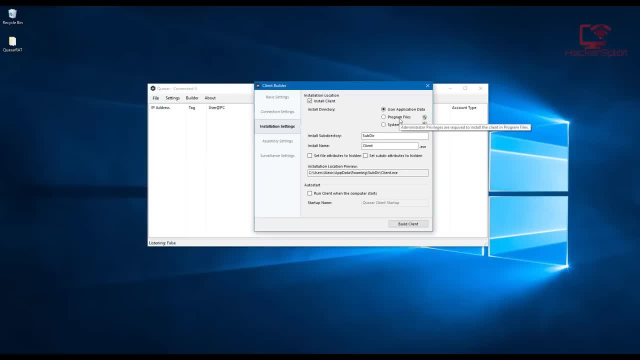 obviously I'm. I'm gonna just uh tell you what I think, and this is because not many people will suspect that they're going to be malicious files in their system folder. usually most people that I've seen you know quite tech savvy people usually like to go through the program files or they go. 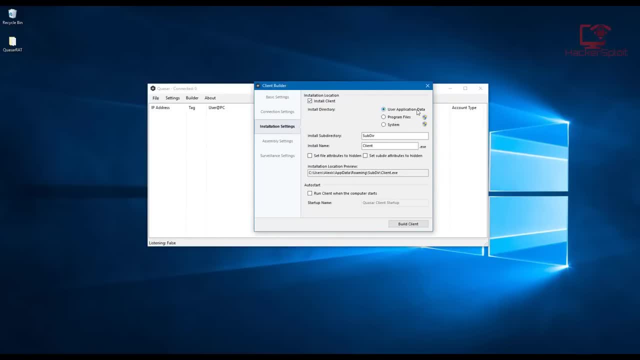 right now, app data is good. not a lot of people check there, but you know, if you're caught, uh, it can be really really bad, right? so, uh, you can choose to do that. I'm not going to do that. uh, you can also choose to run the client when the computer starts, which is awesome. now, again. 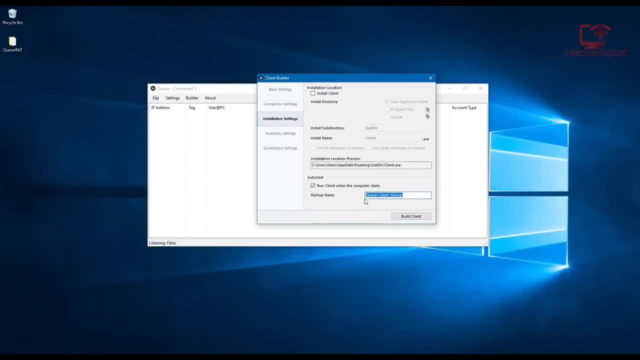 this is where it all comes down to: uh, social engineering. if you leave this like this right and someone checks their task manager and goes to the startup option and they find something with a name like case, a client startup, uh, they're gonna get a bit nervous. so you know, stay away. 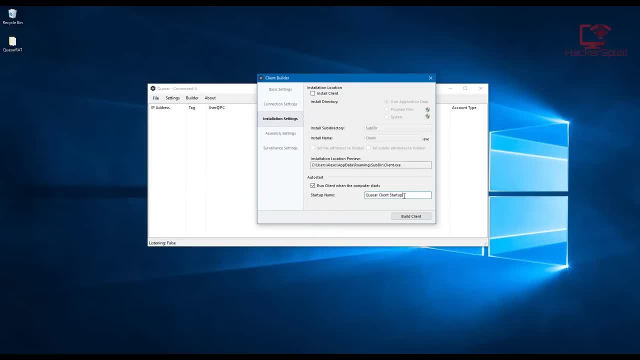 from naming things that obvious. you know you could name it something like Java updater or something like that, so Java updater, and you can then build it all. right now, going to the assembly settings, here is where you can just change the file information again, if you're trying to make. 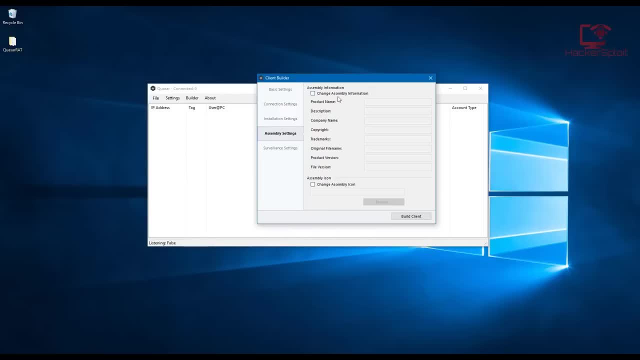 it look a bit more believable. you can change the assembly icon. so, really, this rat is giving you a lot of freedom in whatever you're doing. you have, then, your surveillance settings, which you can enable, your keylogger- fantastic right- and you can again enable the kilo, the. 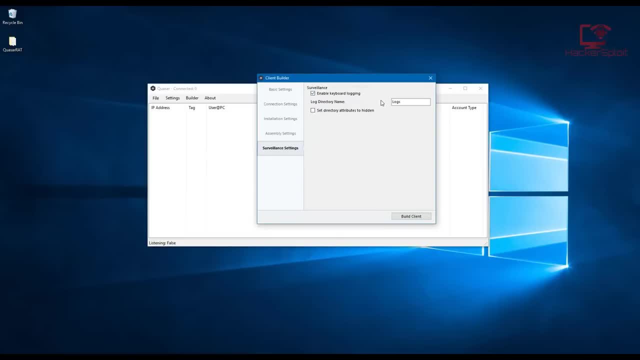 keyboard logging. you can then log the directory name and you can set the attributes to hidden so that it's not found by any snoopers or users that are quite smart with and understand what's going on, right? so, uh, what I'm going to do now is I'm going to hop onto the network. uh, no, I don't want. 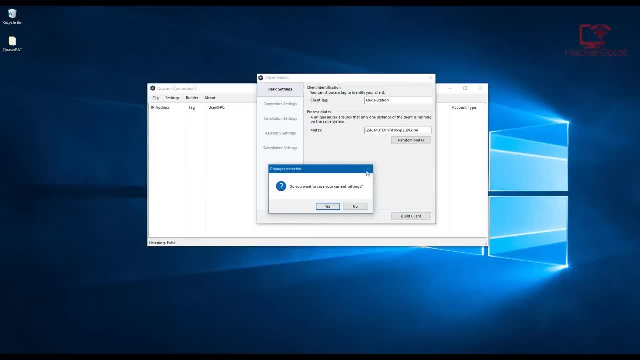 to save my settings. oh yeah, sorry, I forgot to tell you guys, uh, something, uh, once you're done with your settings, just hit build client and it's going to build it. uh, and it's going to save it. um, whoops, pin, and it's going to save it in a folder that you specify. I've specified client and this. 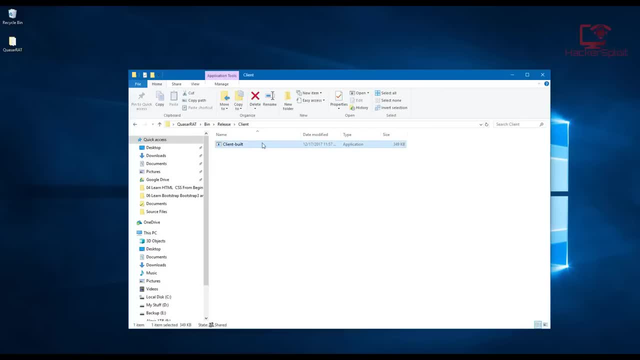 is the program right here that you're going to copy over or somehow move it to your targets operating system. however you do that, you know that's up to you. um, so what I've done is I already have it running on one of these Windows computers on my network which I use for testing malware and 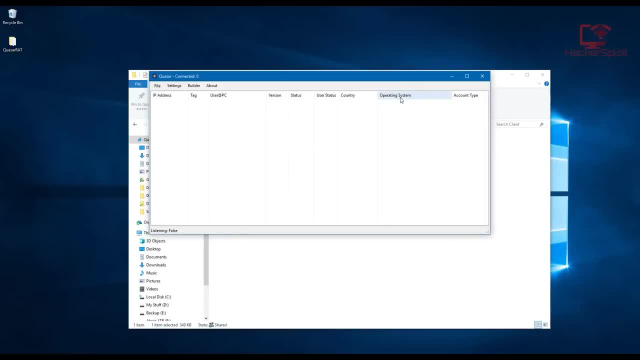 uh, I use it for a lot of- uh, really, you know, weird malware stuff that you know I have to virtualize because there's a lot of stuff that can go wrong, and what I've done. so I'm going to connect to the network and what you're. 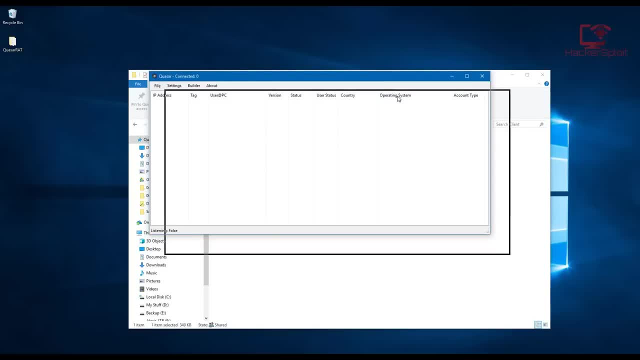 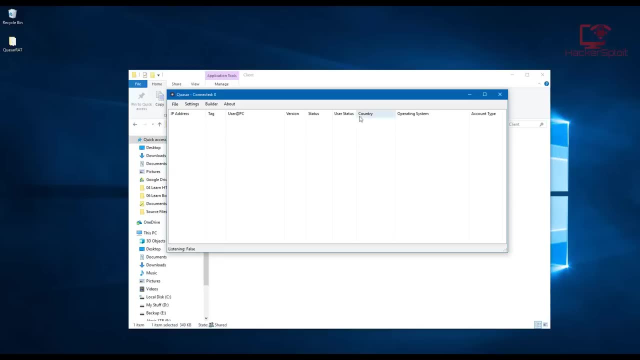 going to notice now is it's going to come up. my computer is going to come up and I'm just going to, I'm going to blur out what is important here so that you guys, uh, do not you, you guys, you know I have to, you have to respect my privacy. I hope you understand that. so what I'm going to do is I'm 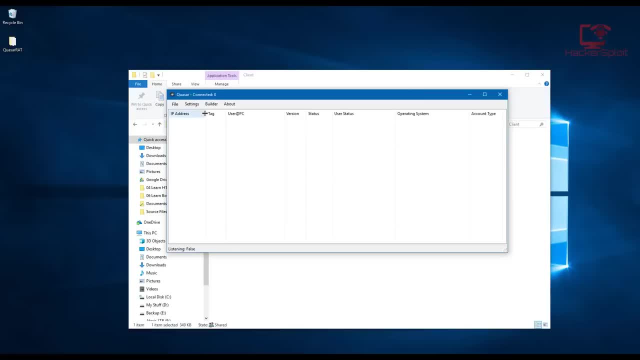 going to block out the stuff right here. so I'm going to block out the IP address, right and um, and the operating system will leave that the way it is. uh, but I'm going to connect to the network right now, so I'm going to change the country and the IP address. so you know, just to preserve my privacy, I 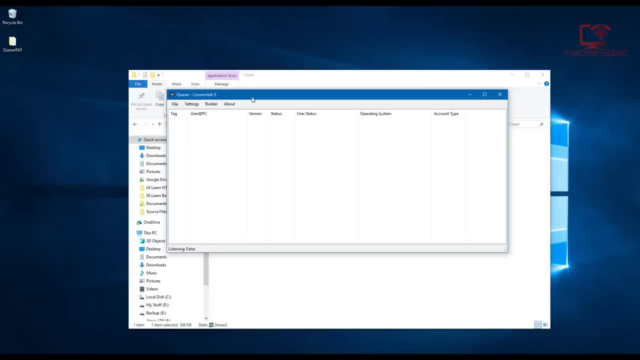 hope you guys understand that. so, um, I'm gonna run this on the computer now. I'm doing that right now. it's right in front of me. all right, that's running. uh, the next thing, by the way, this is not detectable there. so, uh, when you're ready, just go to settings and you want to hit, start listening, all right, so 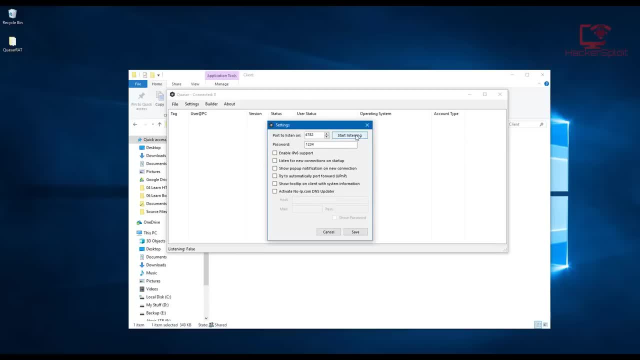 that's going to list on that, on that port for a connection, for an incoming connection, reverse connection. so I'm going to start listening and I'm going to save that and we're gonna have to wait now for it to detect me on the network. I'm gonna there, we are all right. so, as you can see, uh, we. 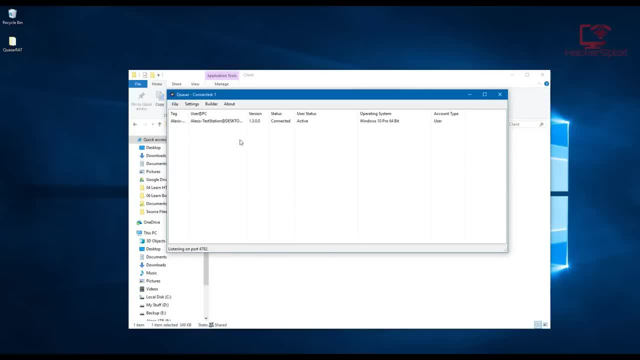 have found the computer, which is fantastic, and, as you can see, I'm running it's. the tag is a Lexus. I call it that because that's where I run all my weird stuff- the test station. so it's going to give you a username and your PC name, right, you then have your version, the operating system version. 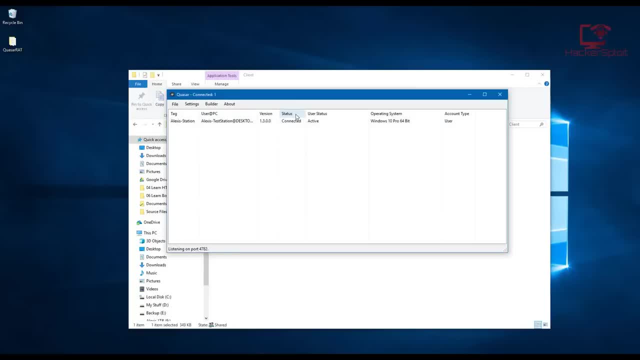 you have the status. you have your user status, and I said it'll give you the IP address, but I'm not going to show mine for privacy. uh, you then have your operating system, which is Windows 10 Pro, and the user account type, which is, uh, the user. all. right now, you're most interested in what we can. 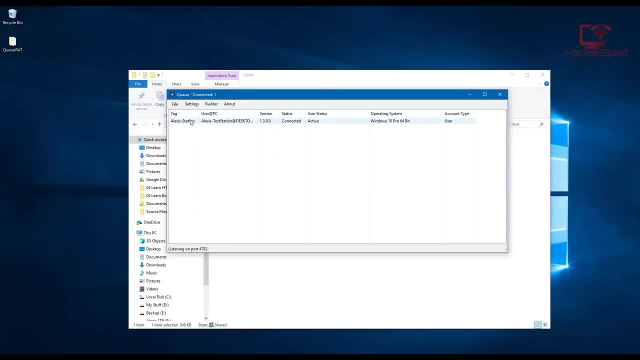 do now, all right, so let's let's check out what we can do exactly. so the first thing I'm going to try and do is: uh, I'm going to show you these awesome tools. we're going to start from the beginning. all right, the first thing you can do is perform a connection. 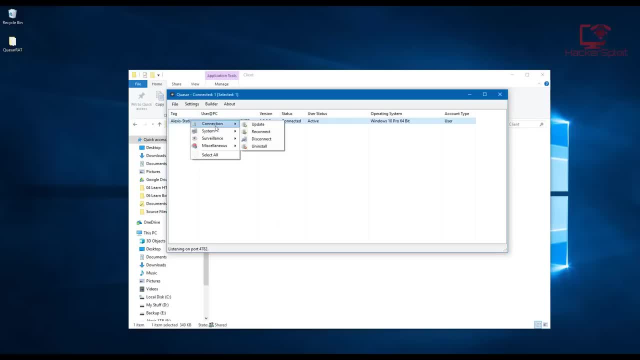 uh, you connection management really, where you can connect, update or disconnect. you can also uninstall the client, which is awesome. it gives you that ability remotely. you then have your system, which gives you system information. it gives you the ability to access your file manager, your startup manager, task manager, your remote shell TCP connections- reverse. 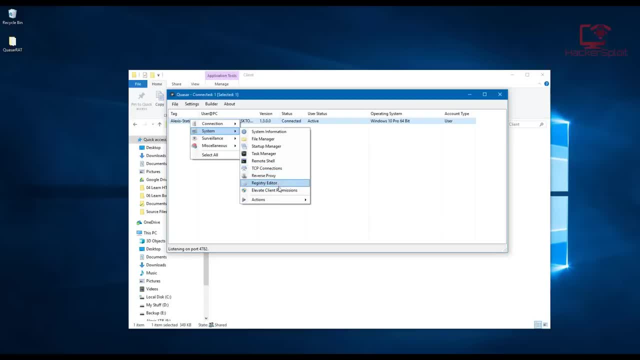 proxy Registry editor and you can elevate the client permissions. this is just incredible. I mean you know, the amount of power you have with it is incredible. and not to mention, you can shut down, restart or standby. I mean I remember back in the day we used to run these different uh PHP rats and 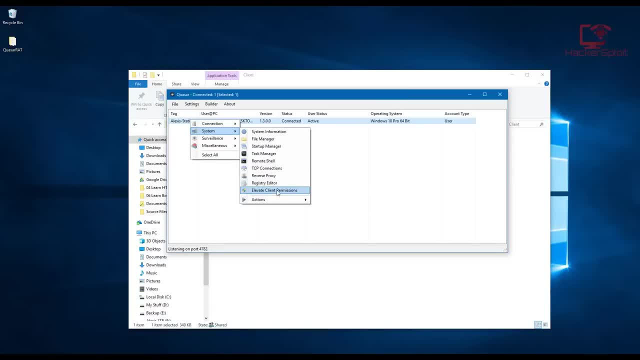 they would. we would write scripts to turn off the computer, like when I mean turn off, I mean like, just without warning, not correctly shut down, and yeah, we corrupted a lot of uh computers. yeah, we did a of weird stuff. um, but going back to what we can do here, we have surveillance which allows you to. 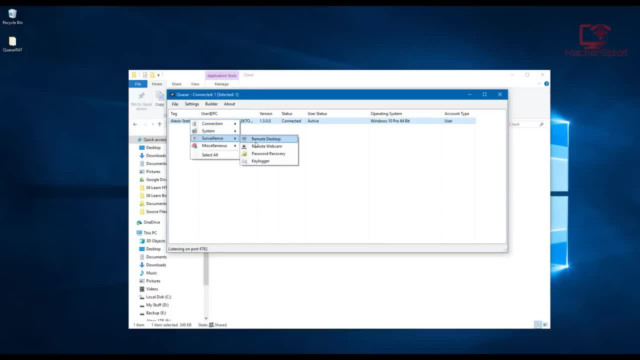 check out your remote desktop, remote webcam, password recovery and your keylogger. all right and miscellaneous, allows you to remote execute a local file, which means you can execute an executable from this, from the host computer, and you can visit a website or you can show a message box to mess with people, all right. so again, some of these things are quite nice to have. 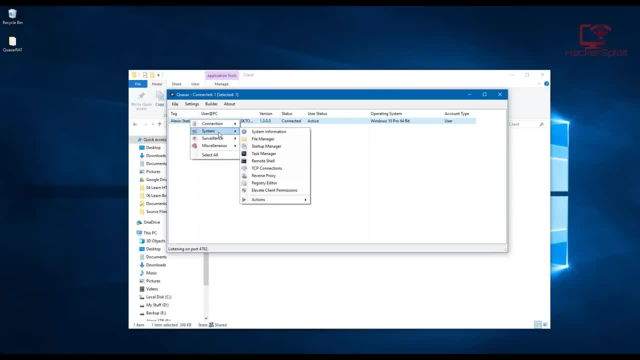 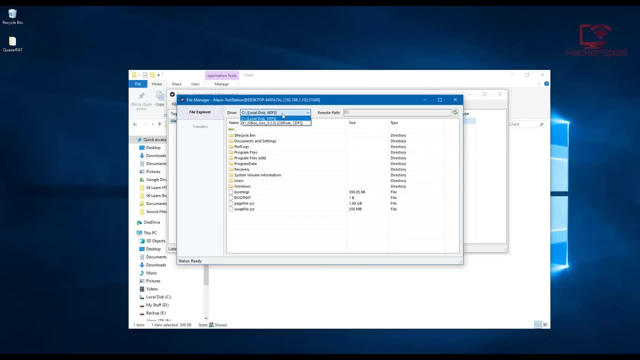 um, now let's look at the system again. you can look at the file manager and there we are, awesome, fantastic. you can look at the different discs installed. so let's say, we go to users and we can go to my user and we look at my desktop and, as you can see, we still have the saint file. 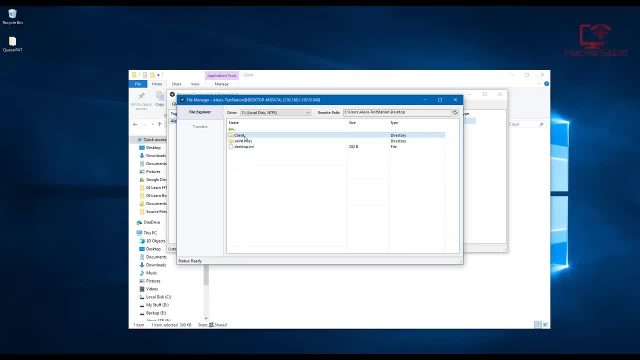 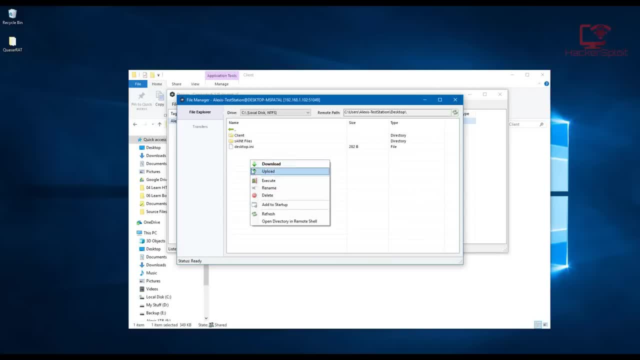 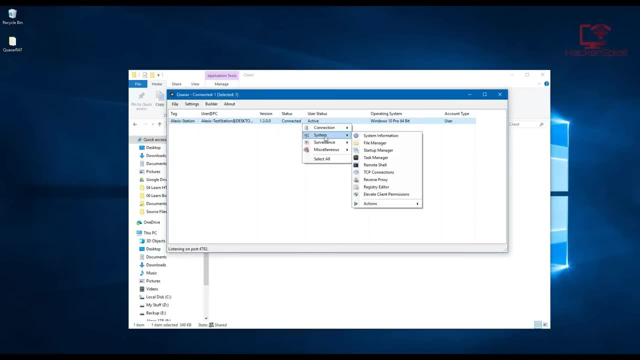 name the files, you can literally do everything to the files that you want, which is incredible. all right, so that's the file manager, pretty self-explanatory. the next is the startup manager, which allows you to you know to run what services start up, and i've not installed much on this. i. 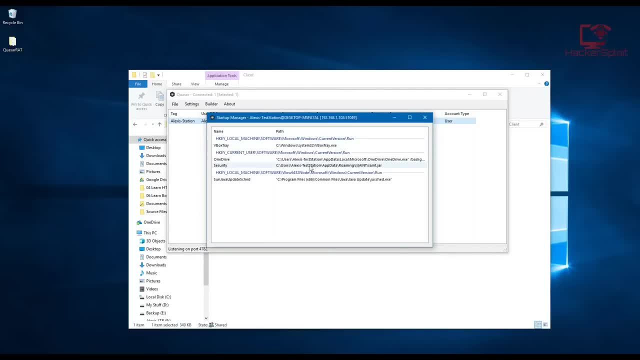 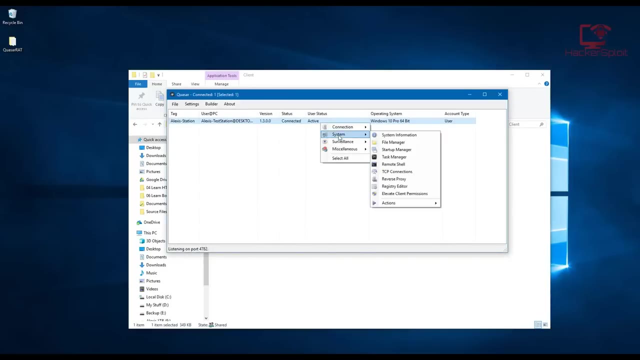 have my one drive. uh, i have the security, which is uh, um, which is the saint um which we looked at in the previous video. we then have the java update tool, right now, looking back at the system, we then have the task manager, which will look at the current tasks running, which is it's quite nice. 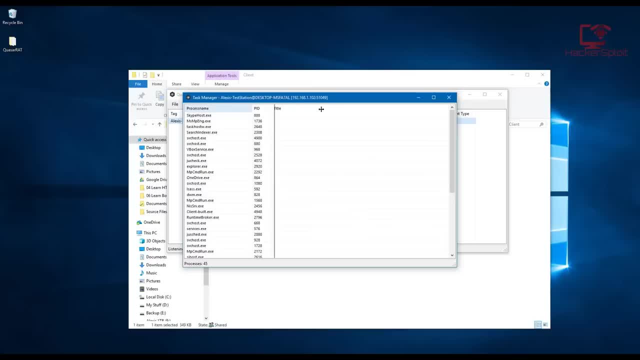 to have this and to understand what's running. so we have skype running. that's just windows for you. you know, windows has weird services running in the background. all right now let's look at something else. we have the remote shell, so you can- you can write your remote uh shells right here. so 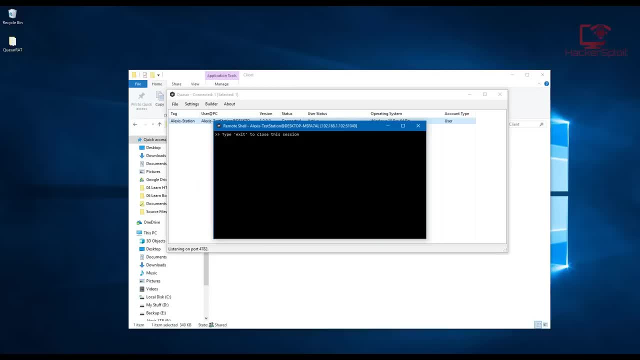 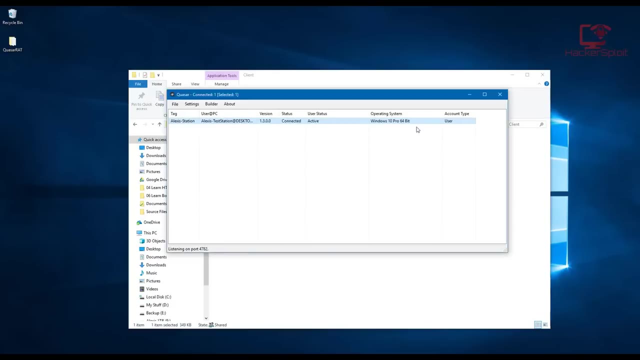 we can perform an ipconfig. whoops, uh, we have nothing. oh, there we are. we actually ran the command. so, yeah, it's using the windows. uh, reverse shell and you can. you can see the ip, the local ip address, there, and yeah, that's working perfectly so we can run remote shell commands. really, really. 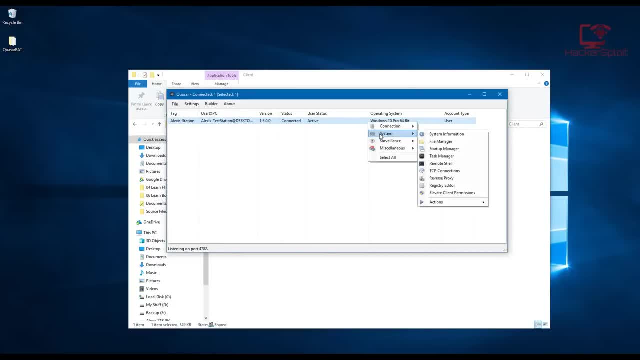 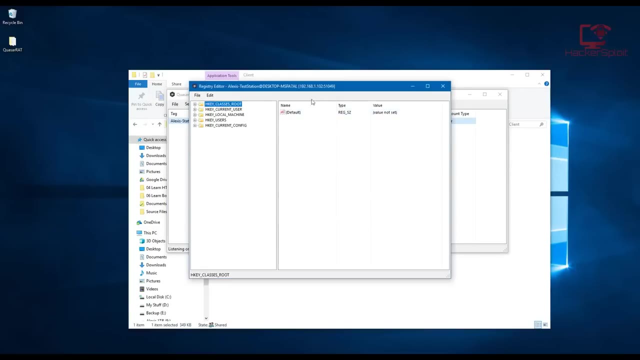 well, uh system. we then have your tcp connections, which i'm not going to show you for obvious reasons. reverse proxy registry editor- something very, very interesting. all right, so you have to elevate the privileges to run the registry editor. so there we are, fantastic and we can. you know the damage you can do is. 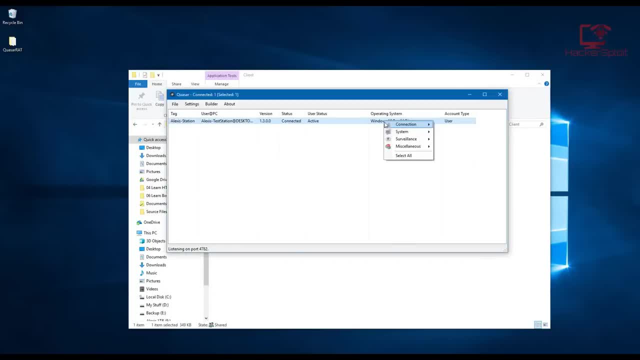 unbelievable, right so system now, what else do you have to look at? we can actually run the. we are not going to shut down or restart the computer right now, because that would be somewhat stupid. all right now, let's look at something that i really, really love and that. 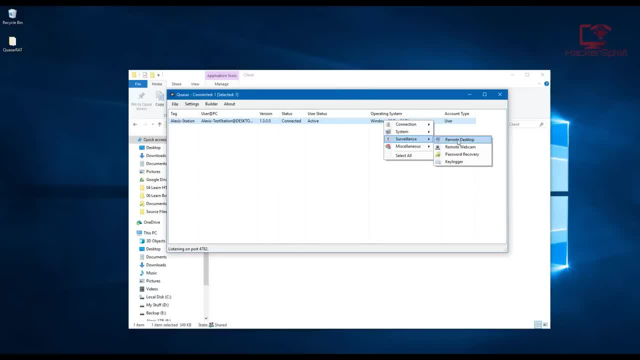 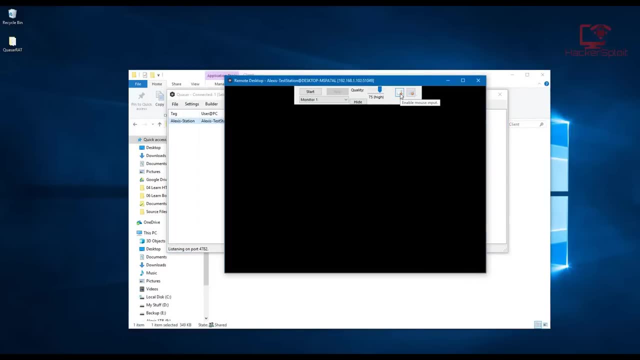 is remote desktop, all right. so what i'm gonna do is i'm gonna start up the remote desktop right now to give you a lot of options here. you can enable mouse input. you can enable keyboard input. you can change the quality- right, you can change, uh, you know, if the computer has multiple monitors, you 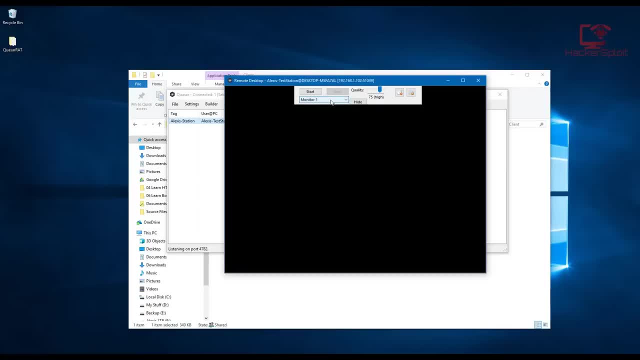 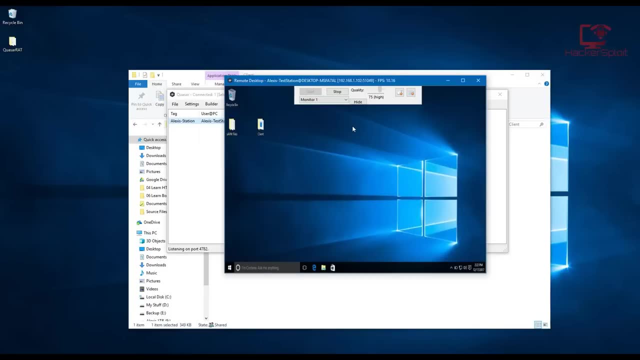 can monitor both the monitors and you can finally hit start to get started. there we are fantastic. so this is what i'm currently running on that computer, the test computer. so i'm going to open up the start menu right now. uh, so let me just do that. hopefully that doesn't lag out, because 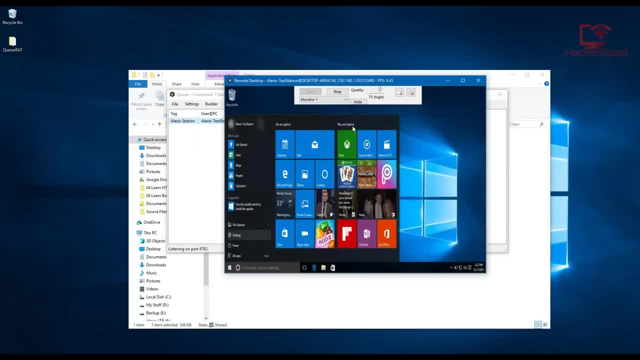 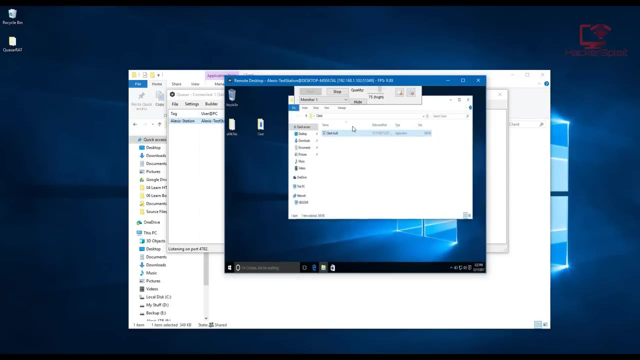 i am running a virtual machine and there we are. fantastic, right, that is working splendidly. uh, let's try and open my files here. this was the client file that i just ran. uh, as you can see, client build and that is essentially going to be, uh, the file that we ran, that which is the 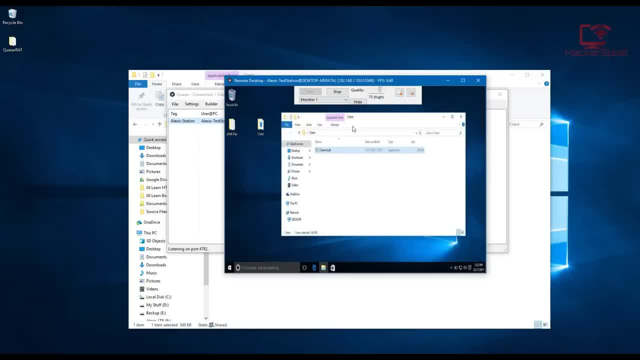 rat all right, so fantastic. that's working out really, really great, uh, and yeah, that's basically it. now, if i enable uh the mouse input, it'll allow me to control the computer from here. so if i open that up, uh, there we are. it did open up to open microsoft edge, uh, which i don't recommend you do under any. 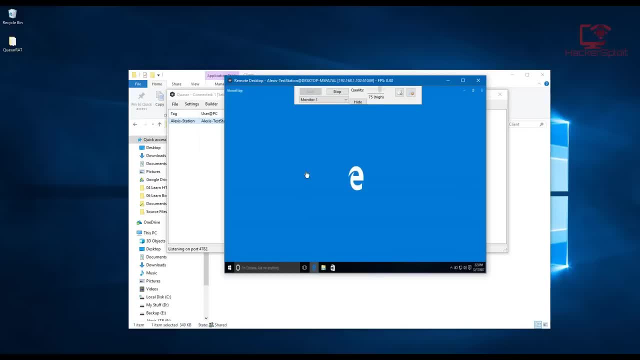 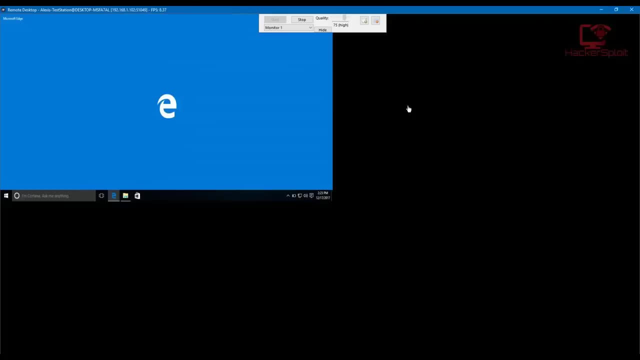 you know normal circumstances. uh, for obvious reasons, right. so that's working up. let me just expand that so we have a better resolution of what's going on. you can enlarge that and have quite a good idea of what's going on on your targets computer. but i'm going to close up edge. 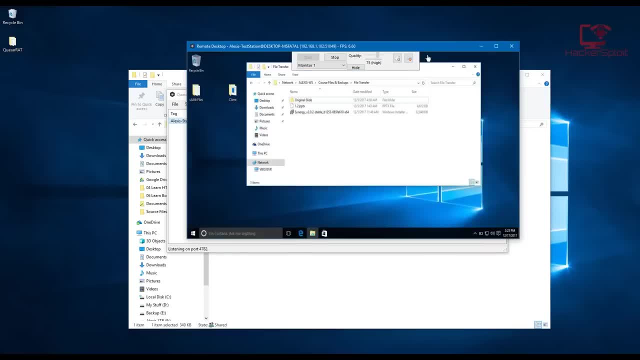 because i'm running this virtual machine on some really really low resources right now. so that's how to use your remote desktop- really really exciting stuff, all right. so i'm going to stop that and i'm going to close it up. and now i'm going to. 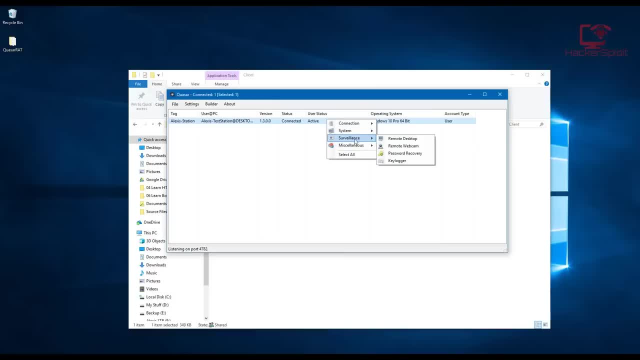 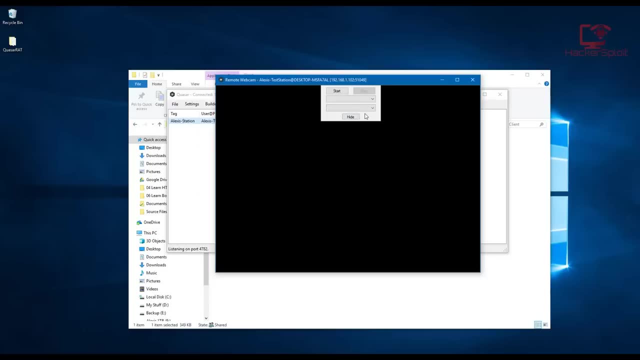 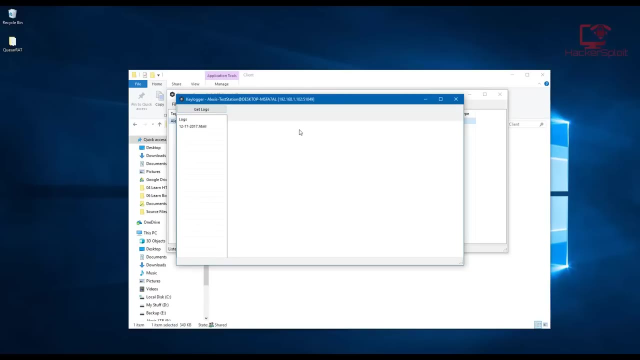 try and use the webcam. hopefully it allows me to start it. so yeah, that's because i've disabled the driver, for obvious reasons as well, so i'm not going to be able to show you that. looking at surveillance, you have your key logger, so let's get logs. so there we are. we did open the html file. 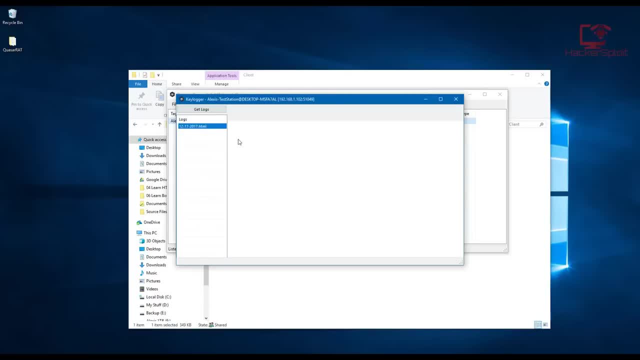 which was opened by microsoft edge. so i'm going to try and log some new files in here. all right, so, uh, what i'm going to do is i'm just going to type something like cmd. uh, again, pardon my poor performance on my computer. let's see if we can get anything new. the logs are stored in the html file. 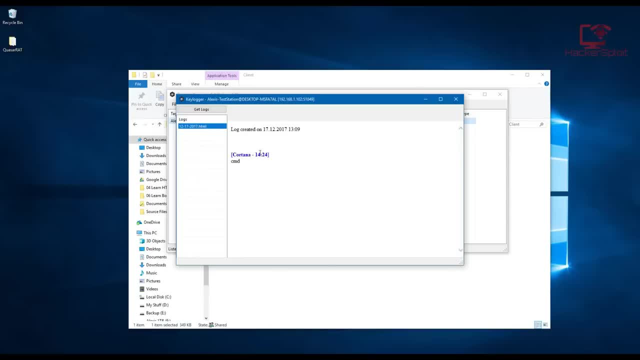 there we are and there we are. so we got the commands cmd. uh, let's try and run another one. so let's see: um, let's say you're trying to log into your username. so let's say you entered your email like: so, so, hackersploit. 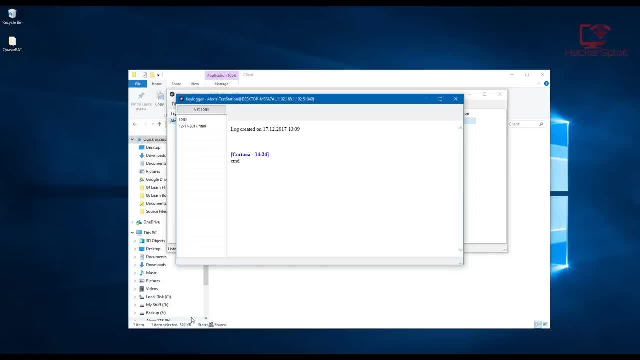 at gmailcom. there we are, and if we get the log just to see if everything worked, it takes a while to update back, back back. all right, updated. yeah, there we are. it does work. so it does give you keystroke commands as well and some of these special keys that you could be. 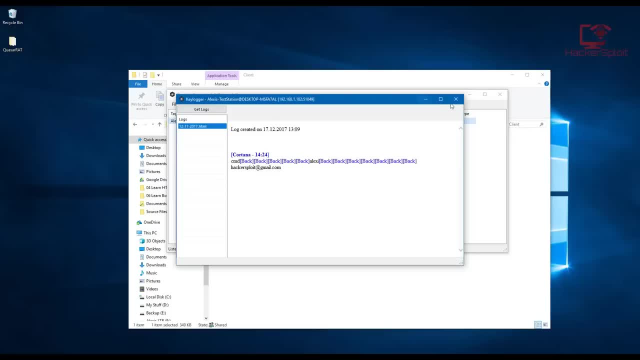 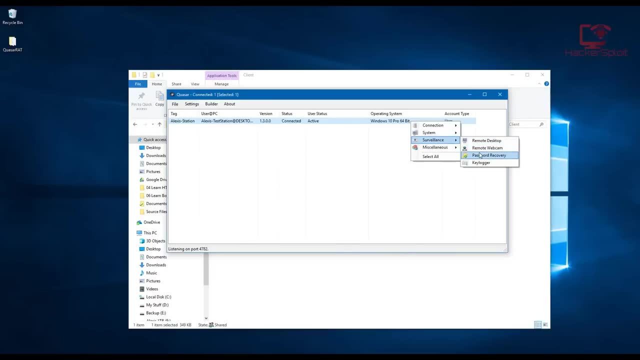 running awesome. so, yeah, we're getting to uh the last, uh, you know things that we can do and yeah, you have the keyloggers: password recovery. that is just for recovering passwords. uh, you know, through uh password files and stuff, totally as you can see, it's gonna uh, it's gonna automatically get. 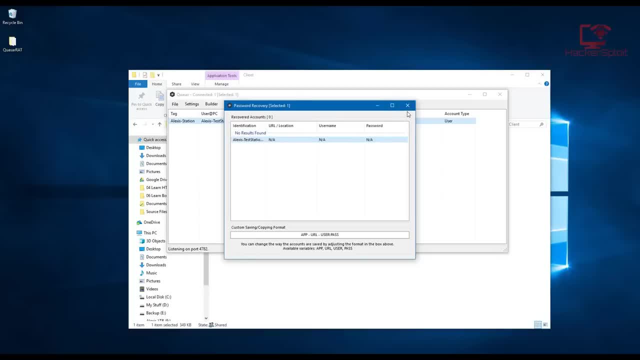 and i've not, uh, entered any passwords on my keychain on this, on windows 10, because it does provide you with one, regardless of the browser that you're using. all right. you then you have remote execute, uh and visit website, so you can enter website that you want to visit. so let's say, 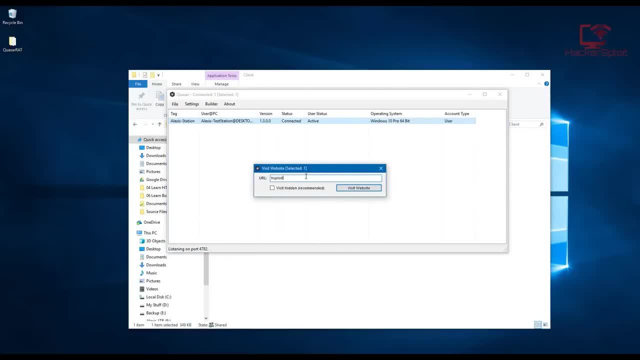 hsplitcom. that'll be pretty cool if it does show. if it does show up, so visit website, um. so let's see if that opens up. um, it's obviously going to open up up on Microsoft Edge, right? so again, just I'm just gonna give it a few seconds. 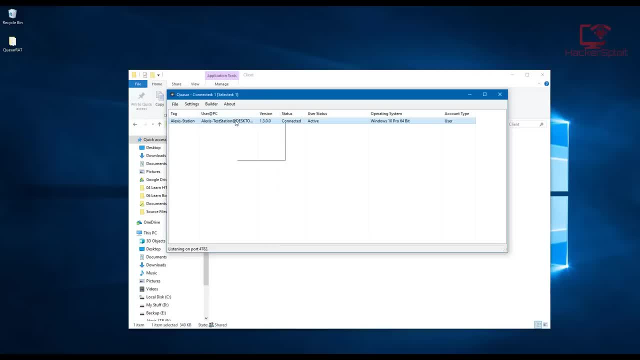 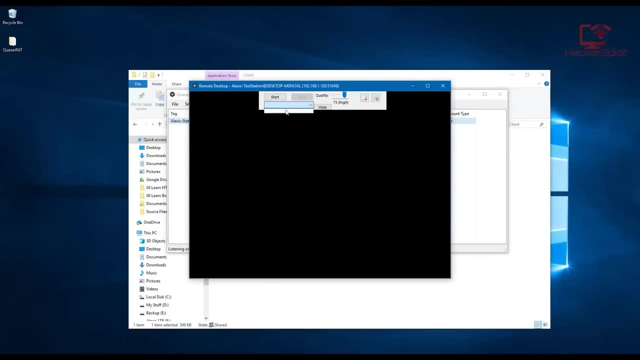 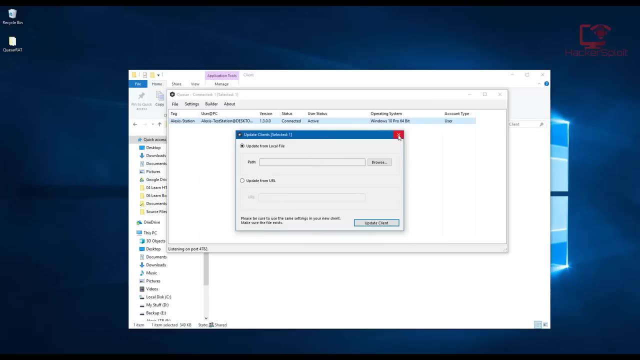 here. what I'm gonna do is I'm gonna open up the remote desktop so you can actually see what's going on. whoops, for some reason we're not getting that connection right now. but let me, let me just connection, let me update it. whoops, so it's still connected there. we are so miscellaneous what I'm going to. 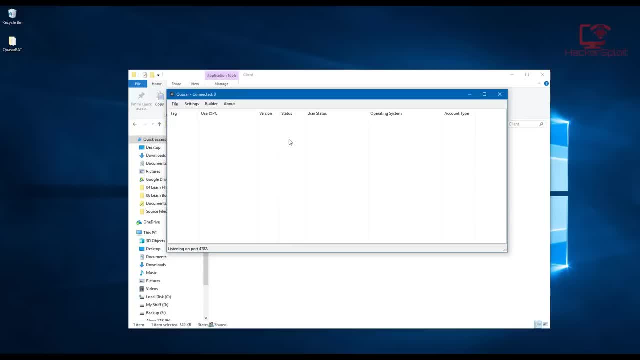 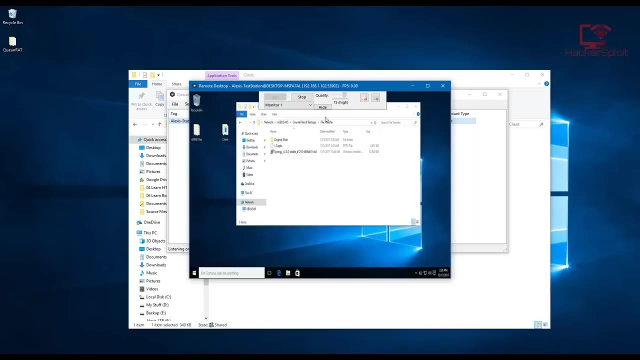 remote desktop. hopefully it opens up. right now it's probably trying to open up the web page. let's see if we can access the file manager. oh yeah, we still can. so there must be an issue there with the remote desktop connection. oh there we are, it's working now. and that the URL did not open. but that's probably because 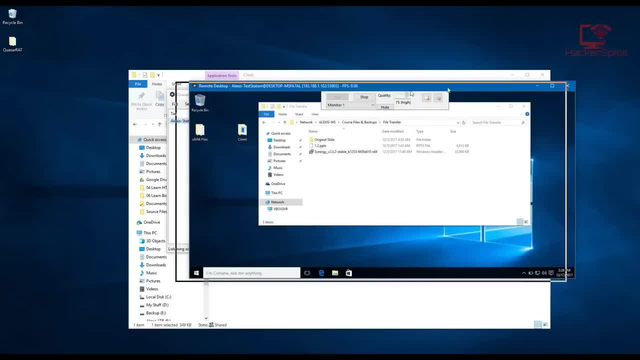 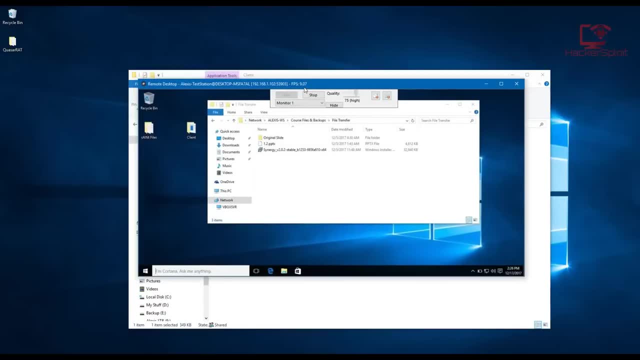 of the overflow and, as you can see, one also. something also very, very cool is the ability to check your FPS right here and, depending on your connection- you know from your, since it's remote, it's a remote we're doing, it's a reverse connection. the speed or the quality it is determined by the client that you've installed this on. 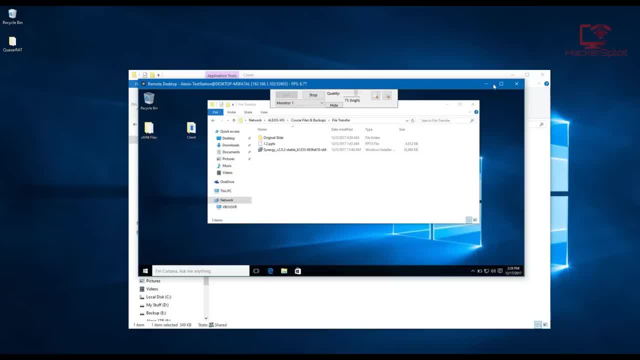 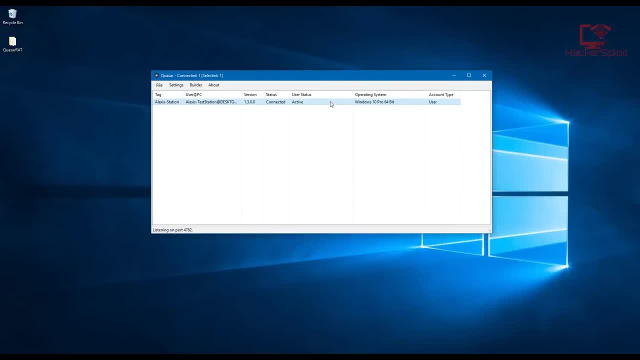 but that's it really. you can see the power that comes to you when you use you and use case a rat. so you know, thumbs up to the author. and yeah, this is a fantastic tool. you can, you know, go ahead and check it out and understand how it. 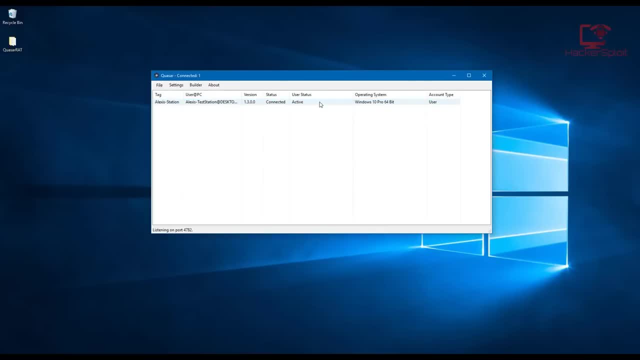 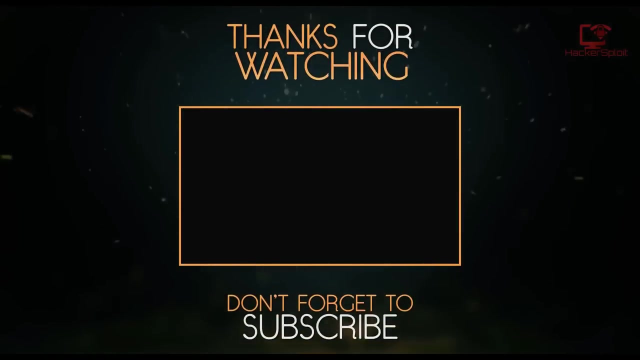 works and yeah, so that's going to be it for this video, guys. thank you so much for watching. I hope you enjoyed this video and I'll see you in the next one. peace, Bye.